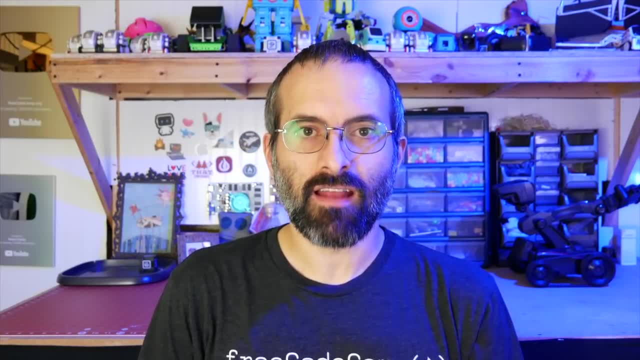 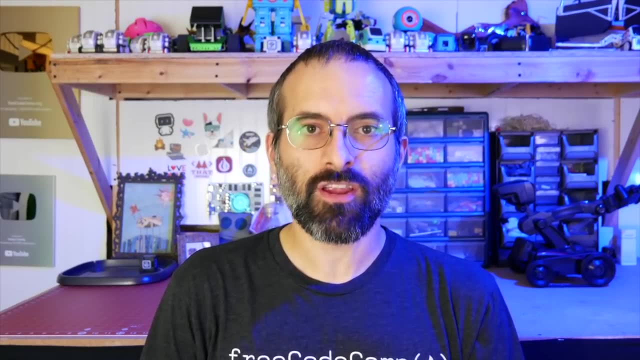 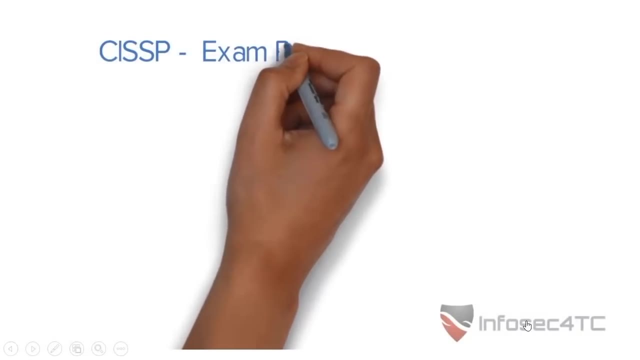 The CISSP is a popular cybersecurity certification. This preparation course has already helped tons of people pass the exam, and now we are releasing it for free on the FreeCodeCamporg channel. Hello and welcome to the CISSP exam preparation course. My name is Mohammad Atif. 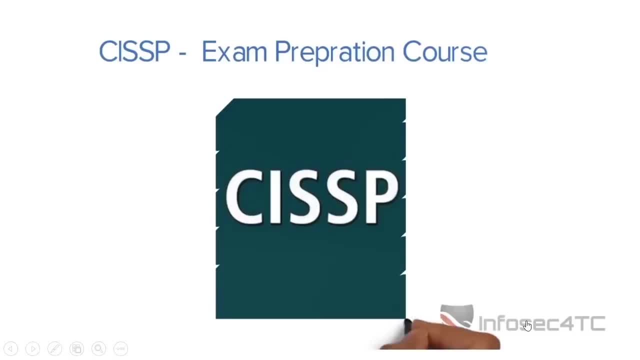 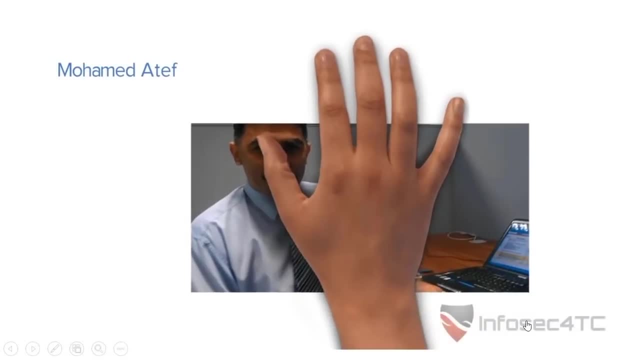 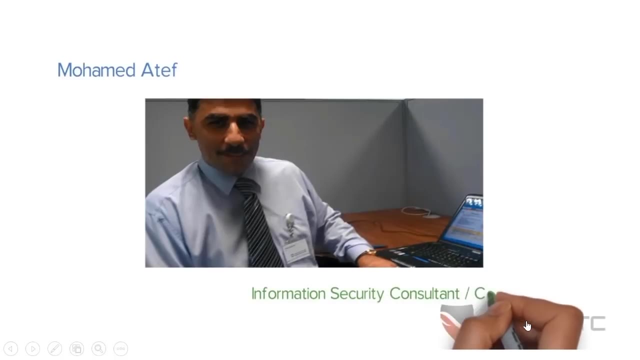 I am an information security consultant and a certified instructor with more than 20 years of experience implementing and managing information security management system project, with a strong background in implementing different information security compliance framework and regulation. I worked with different type of organization- government, multinational organizations- and I worked with different type of organization. 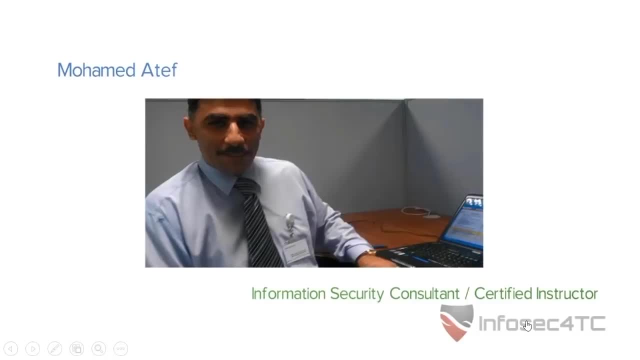 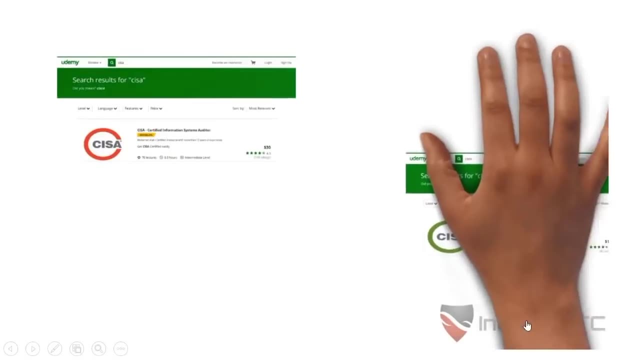 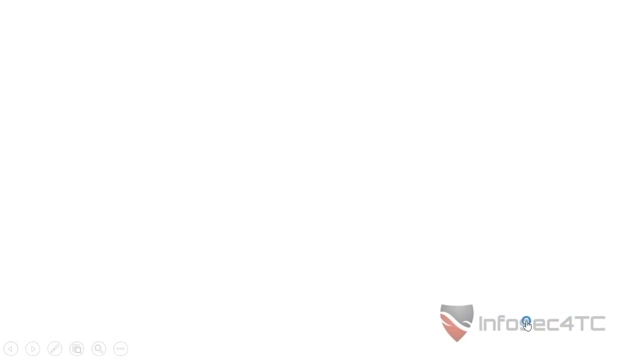 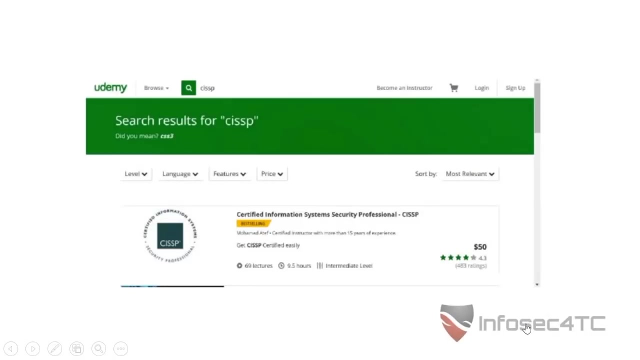 such as IBM, private sectors and law enforcement, And I have 16 courses published online. Nine of them are bestseller courses and all my courses are in information security and ethical hacking. My previous CISSP training was a bestseller courses for two years. 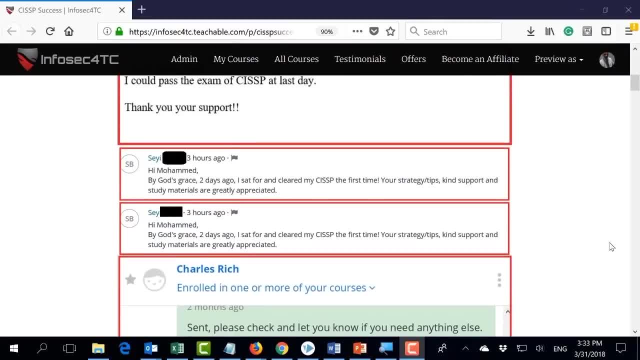 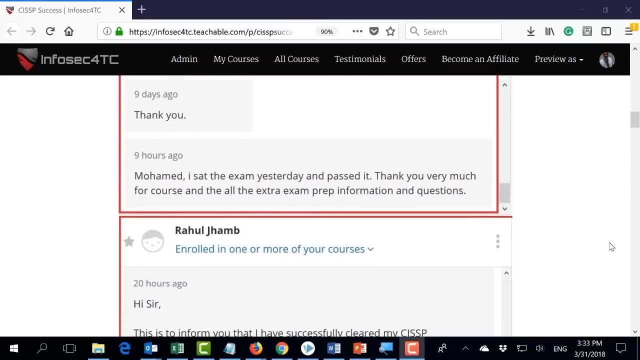 and I'm proud to say that I have been able to do it for a long time. I would like to say that I helped hundreds of students to clear their CISSP exam from the first attempt and get certified and joining the information security career, which has 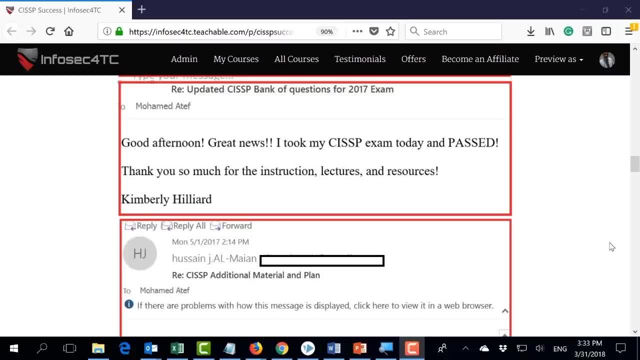 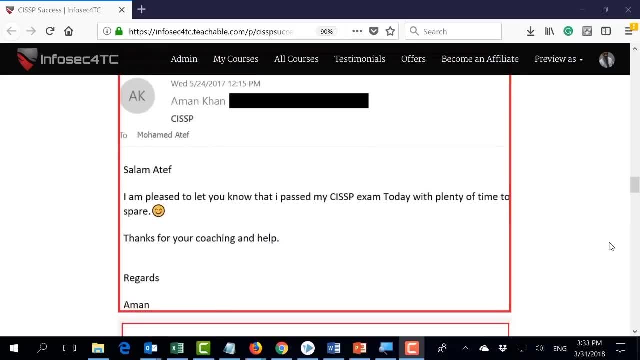 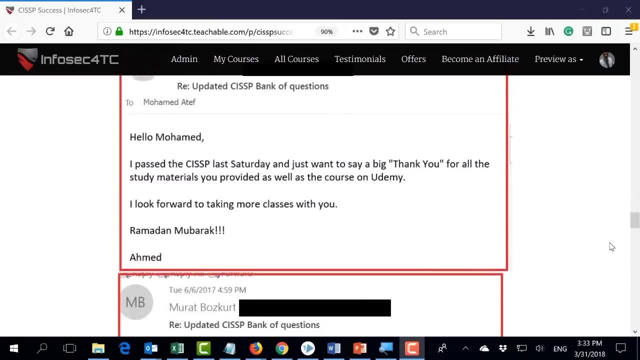 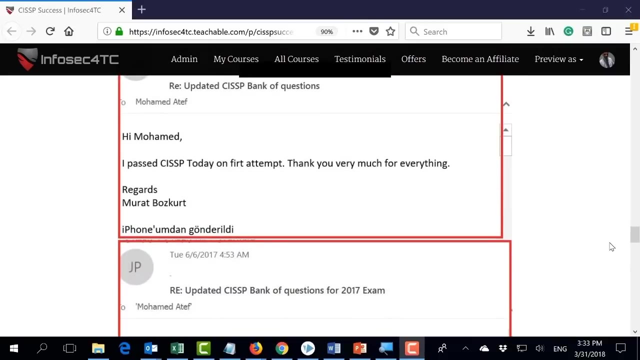 a very high demand in the market today. So the course is not just about the skills and knowledge that you will learn, but also it will guarantee that, if you follow my plan and use my resources, you will be able to achieve your goals. You will be able to pass the CISSP exam easily, which is a must if you plan to get an information security job or position. 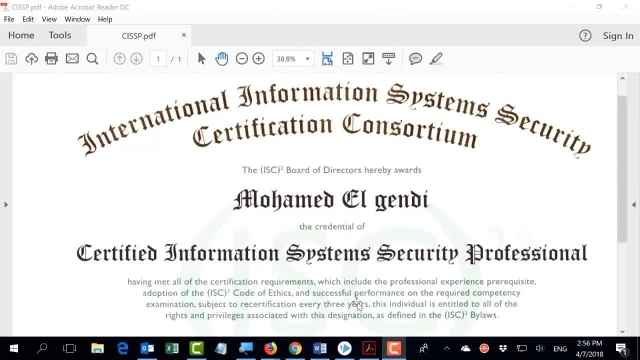 Before starting our training, allow me to give you a brief about the value of the CISSP certificate. What is exactly the CISSP certificate? If you know about that, you can skip this lecture and move to the next lecture. But if you are new to the information security, 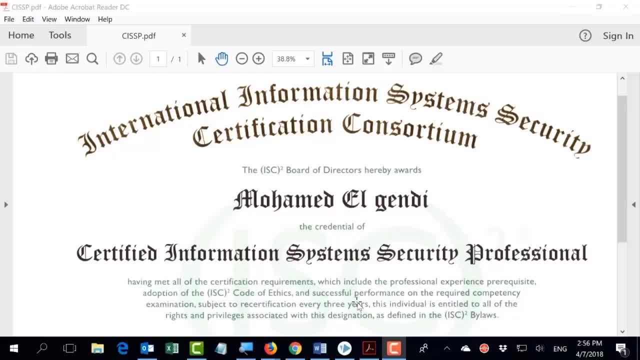 And you need to know more about the information security field and what kind of certificate you need to hold to be able to find a decent job in this field. Maybe you need to listen to this lecture and the upcoming lecture if you plan to work in information security or you are moving from your current. 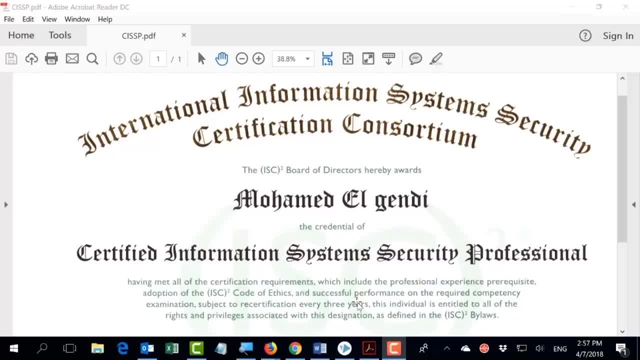 career To information security career. you need to hold a professional certificate. Holding a professional certificate in this field it's like holding a license. Think about it: If you know how to drive a car but you don't hold a license, you don't have a license, a driving license- no one will allow you to drive its car. 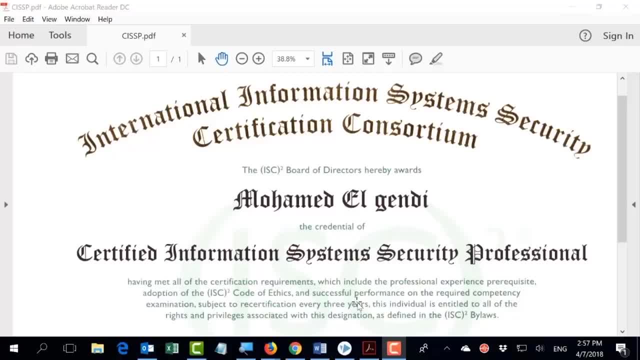 While if you have a driver license, it means that you know how to drive a vehicle, No one will allow you to drive a car. While if you have a driver license, it means that you know how to drive a vehicle, No one will allow you to drive a vehicle. 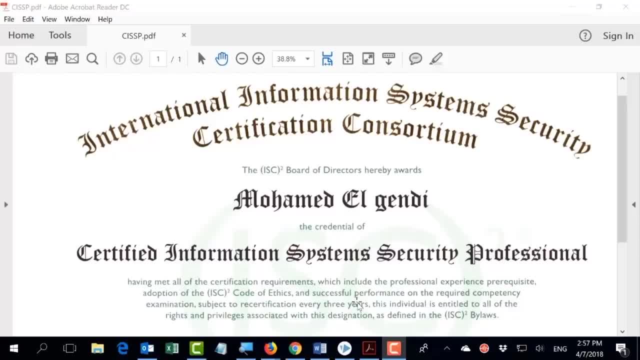 And how to manage a car. Same concept apply for information security. If you plan to work in this field, you need to hold a license. So holding an information security certificate is like having a license, And usually when we are doing interview for candidate for information security position, if they hold a certificate like CISSP, it reflect that they have a good knowledge. 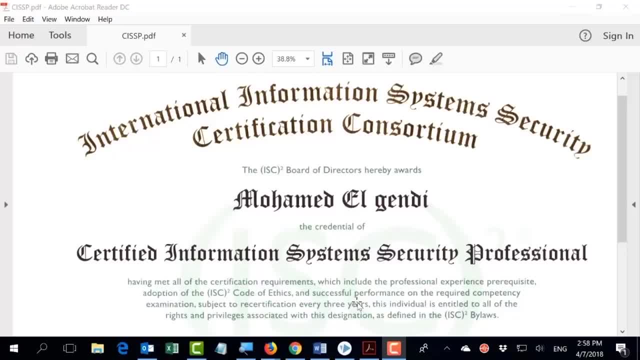 In information security and sometimes we can skip some questions because just by having this certificate, it indicates that those people know about information security implementation. So it's a very, very valuable asset to have if you plan to work in information security. Now, it's not the only certificate in information security. 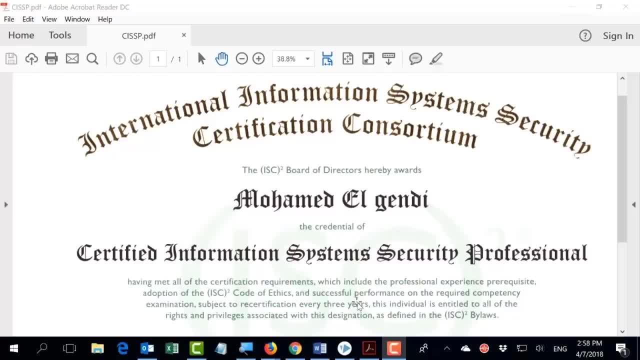 We have a lot of certificate. We have the CISSP, We have the system. We have also certified information security manager. We have the CISSP, we have certified information system auditor. we have a lot of certificate, but what is the value of the certificate? should I start with it or should I start? 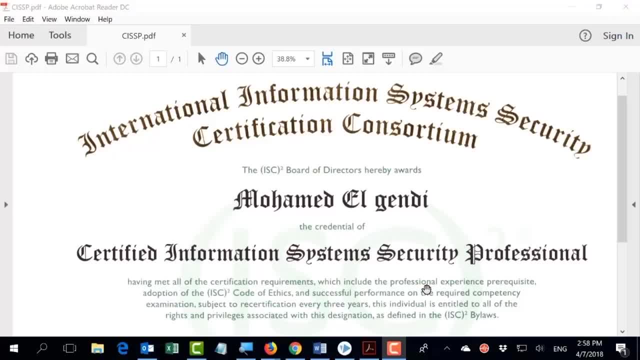 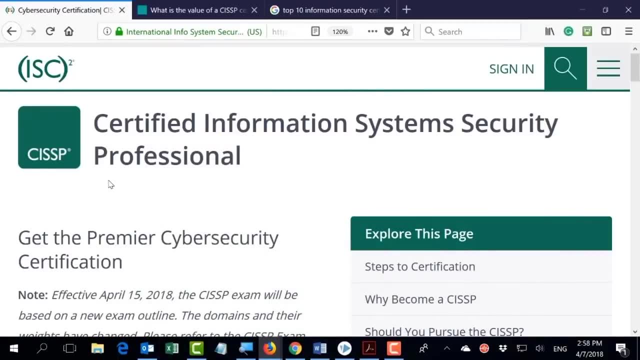 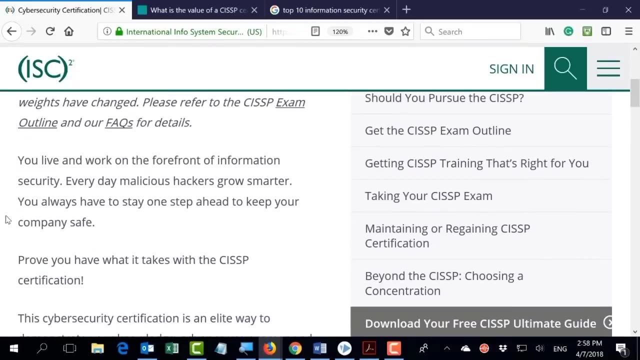 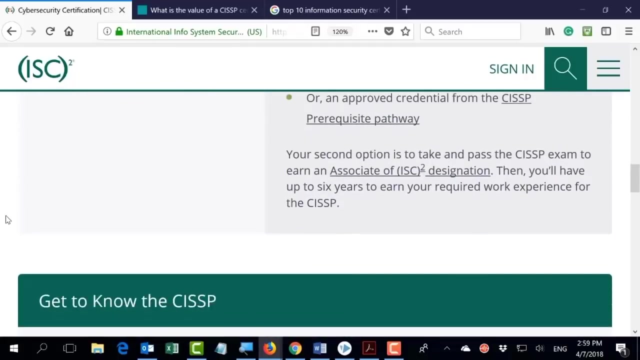 with another certificate. CISSP or certified information system security professional is certificate issued by IC square and you can go to their website, know about the certificate and the value of the certificate and how to hold certificate was, what is the prerequisite for the certificate and so on. but if you 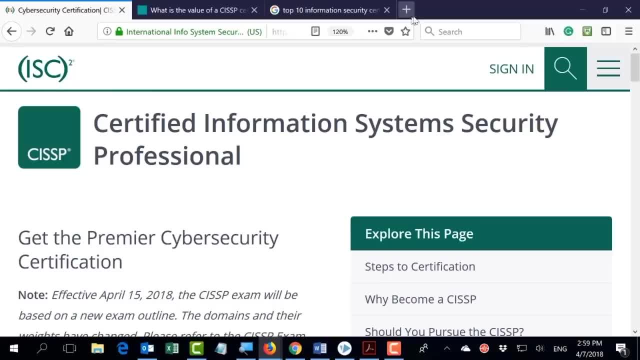 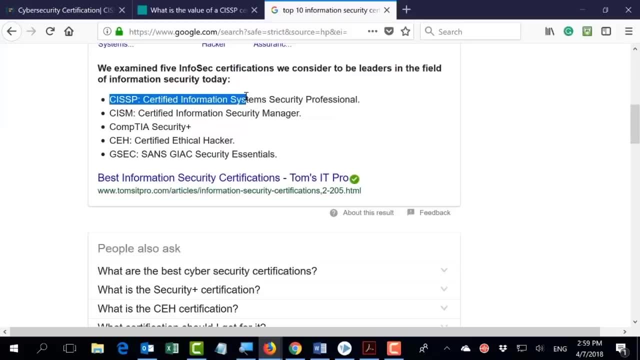 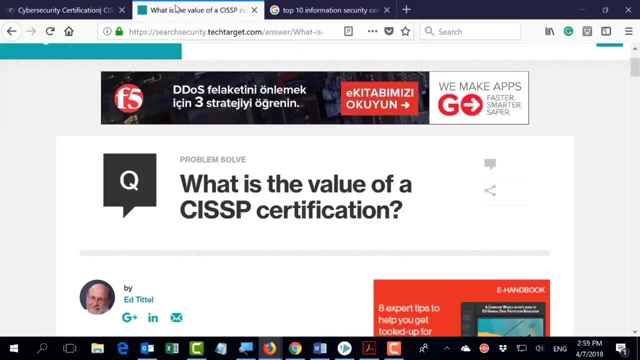 do a little research yourself about the top 10 information security certificate, you can find that CISP is the first one. we have other certificate but still CISP is the most valuable certificate. and if you do more research about the value of the CISSP certificate, you can find out that the 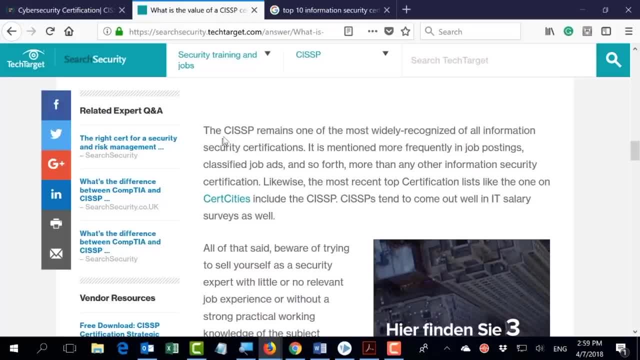 most recognized certificate in this field is the CISSP, remain one of the most widely recognized of all information security certification and it's mentioned more frequently in job posting and classified job ads. so you can do your homework, you can do some research to know which certificate. you should start with and you will end up that CISSP is the most valuable one now. it's not a hard certificate, all it's not a technical certificate. you need to be aware of that. CISSP. it's more into the information security management area. 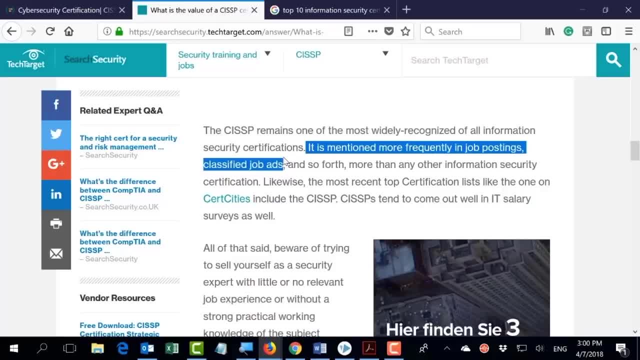 so even if you have, like, a weak technical background, you don't have to worry. you may spend more effort and more time and I'll be supporting you the full way until you get certified. but you should not consider this as a technical certificate, because CISSP is not a technical certificate, it's more into the. 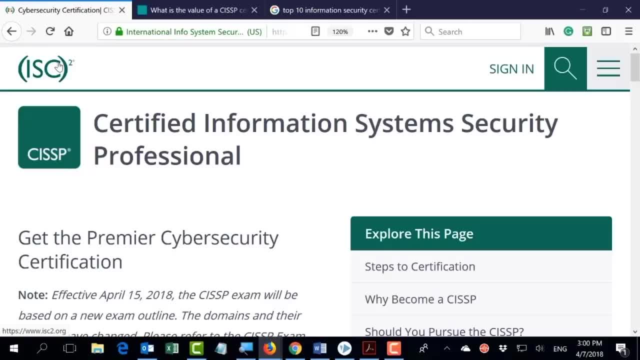 information security management certificate. so this is quite important to understand that even if you are just starting, it will take you a little bit more time and it will take a little bit more effort, but you don't have to worry about it, because to be able to get the certificate, it's not about the amount. 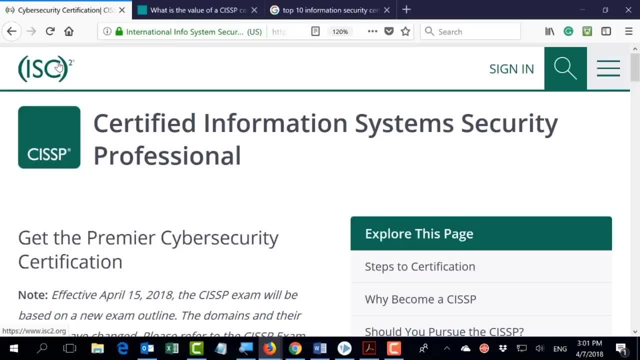 of knowledge. you know it's about thinking as management or thinking as information security specialist. this is not thinking as a technical people, and actually I know a lot of people that came from a technical background. some of them were network administrator or security administrator. they came from a 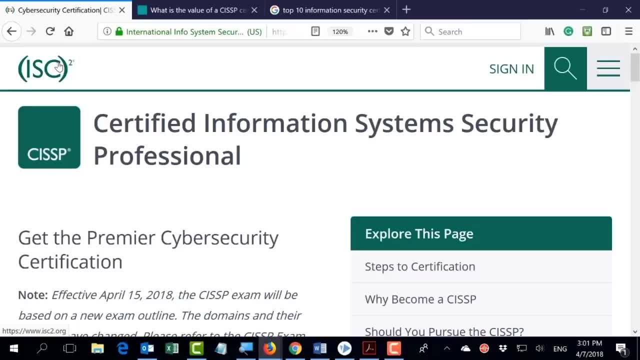 pure technical background and they failed the exam because they are not qualified to be a CISSP. because they are not qualified to be a CISSP because they depend only on their technical knowledge, which is not the main issue here. okay, and in the upcoming lectures, I'm going to give you some idea. 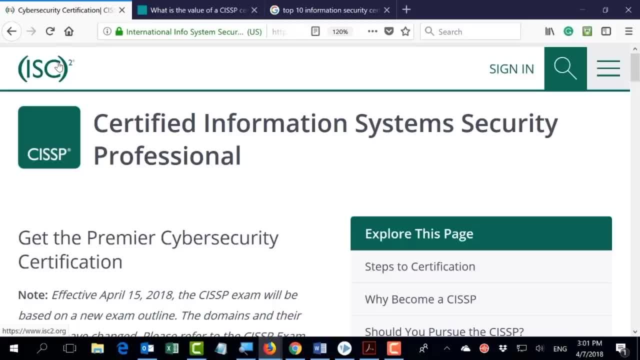 about what I'm talking, about, how to think as an information security manager or information security officer, and so on, but the objective of this specific lecture is to show you the value of this certificate and, as you can see, it's very, very valuable and very, very recognized. 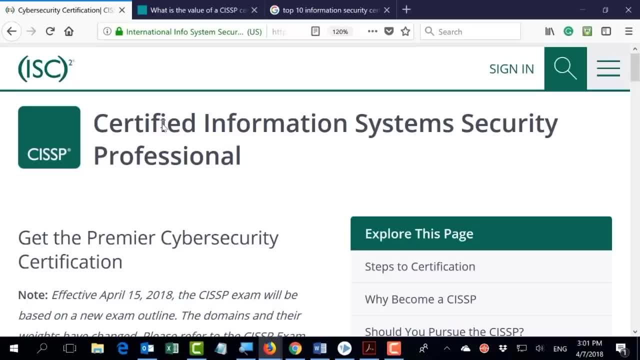 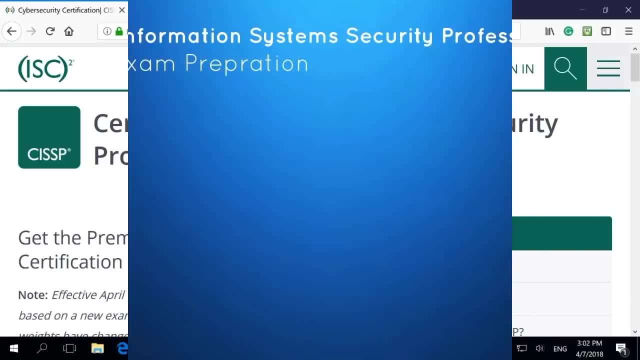 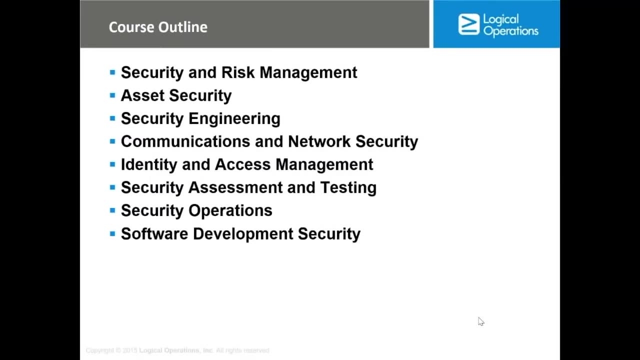 so it works. it's a very good investment in your effort and your time until you get the certificate. CISSP curriculum consists of eight different domains and to be able to pass the exam and get certified and find a decent job, you need to not just understand. 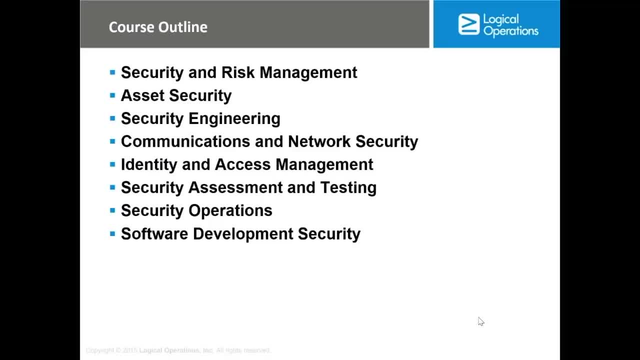 the terminology and concepts related to those eight domains, but also you need to know how we should implement them in a real environment or a real organization. that's why I will not depend on your background, but I will start from scratch and I will explain all the terminology and definitions. but 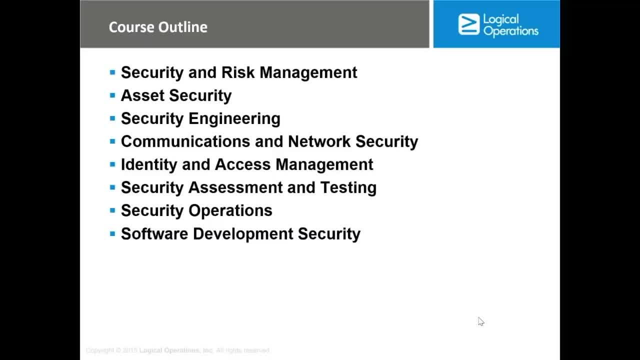 But also I'm going to show you how we are implementing them in a real life environment. How, if you get hired in a specific job, how can you do a risk assessment, The type of risk management or, I'm sorry, the type of risk assessment that we are following. 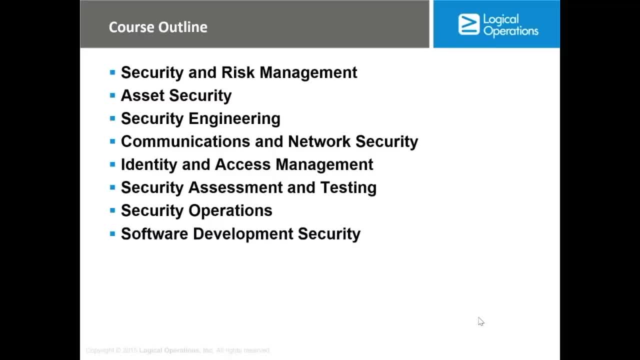 What is asset management? What is the asset security? What is the different domain in any information security management system, And how realistically are we doing it? So what I'm trying to say is that the objective of this training it's not just to read the slide or to explain a definition or a terminology. 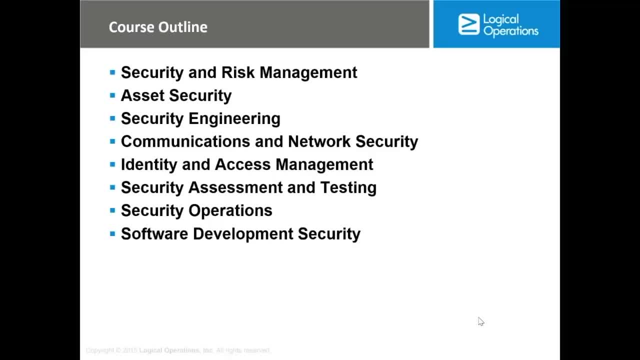 It's not like that. It's to give you the real experience, in a sense, that if you get hired tomorrow after getting certified, You will be able to start working in this environment and start doing your task in an effective way. So I will be sharing with you a lot of plans, documents, templates showing you how we are doing it in real organization, and so on. 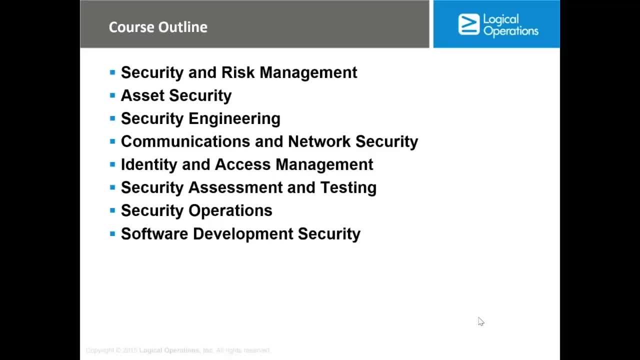 So the eight different domains in the CISSP curriculum would be first, the security and risk management And the first part of this domain. it's like an introductory part where we are talking about what do we mean by security, What is the different element of information security and so on. 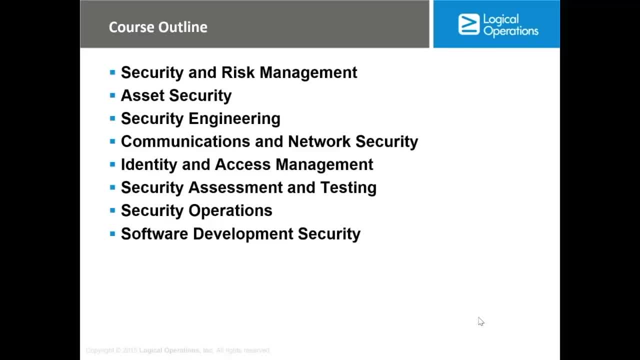 And then we're going to move to a very, very important topic, which is the risk management. Usually risk. it's one of the initial tasks that we are doing in security implementation. You need to identify what risk you are facing to be able to consider what security control you need to implement. 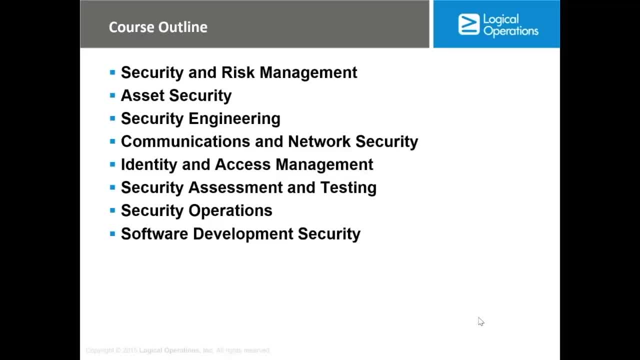 Then we're going to talk about the asset security Again. the first two domain is the first Step: to implement an information security management system. Think about it: If you are implementing security in your home, you need to buy some alarm system, or you need to buy some or hire some security guards or something like that. 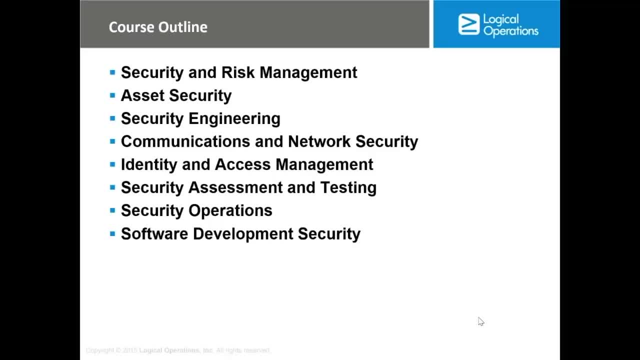 How much you're going to decide how much you will be spending on that, on security, It depends about the asset values that you have- What do you have in your house, Right? And it depends about what risk you are facing. Those are usually two main steps you are doing to be able to decide about what kind of security you will be implementing, because if you don't have that much assets at your house, you should not spend ten or twenty thousand dollars to secure your house. 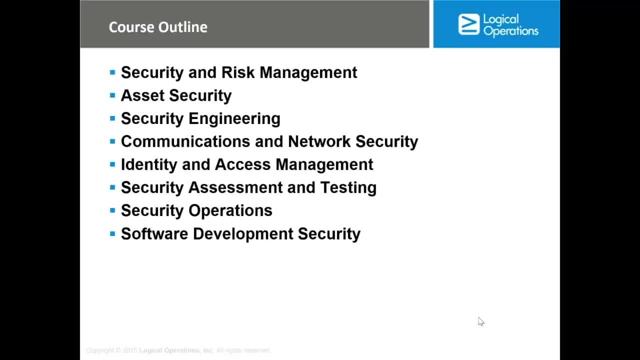 It doesn't make any sense if you live in a place where it's a very secure area. So the risk it's not that high And maybe you don't need to spend that much. So same concept apply on business, but in a bigger scale. 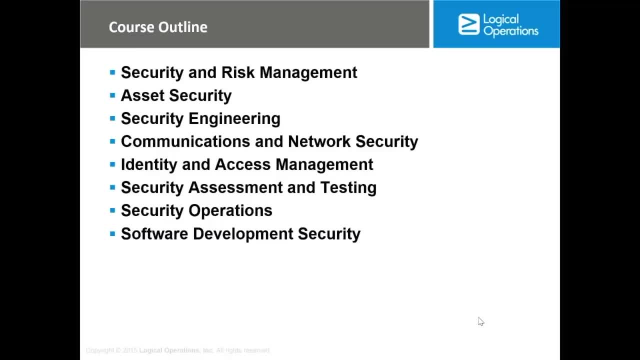 So the first two domain: if you understand them very well, You will know how to start implementing information security from scratch, how usually you are starting this field. Then we're going to talk about security engineering. The fourth domain will be about communication and network security. 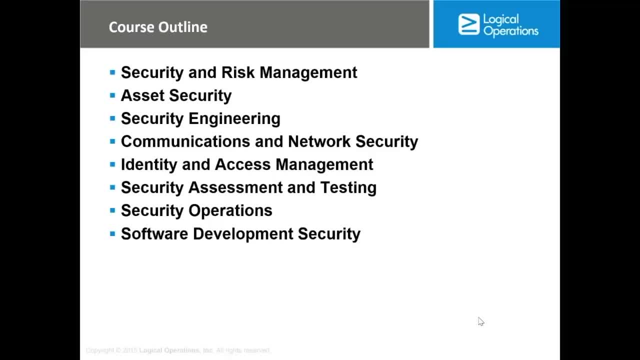 This domain was the previous, in the previous Version of CISSP, and still the same. And then we're going to talk about identity and access management, Then security assessment and testing and security operation And finally, software development security. So those are the eight different domains that we will be covering in our training. 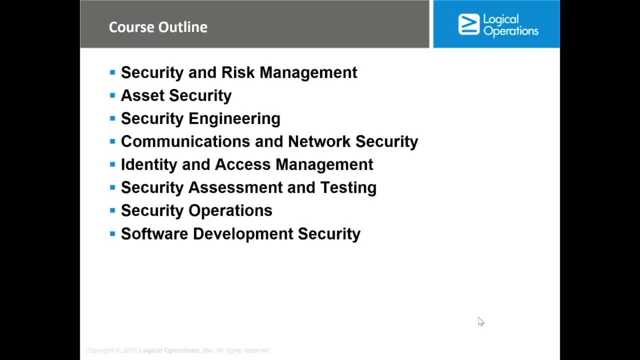 And, as I told you, it's not about the terminology, It's not about because, actually, Inside the exam, they are not testing the amount of knowledge or amount of information You know. they are testing how you can utilize them for implementing information security management. 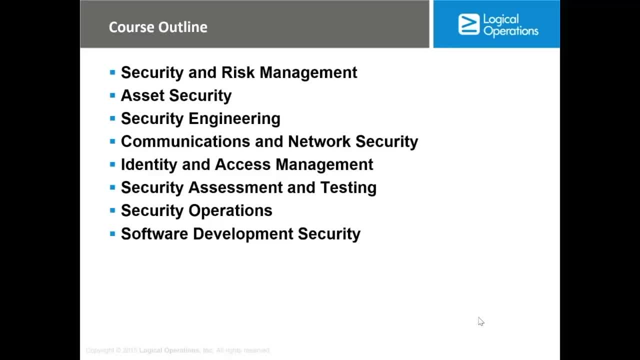 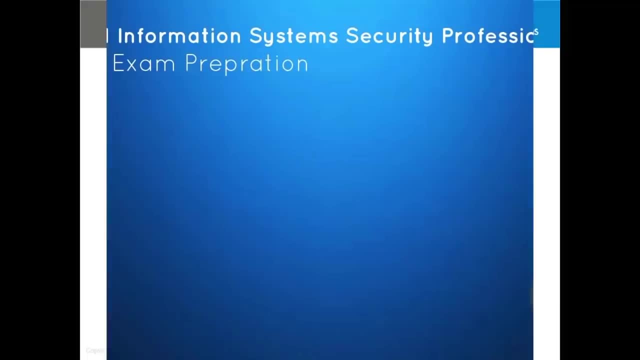 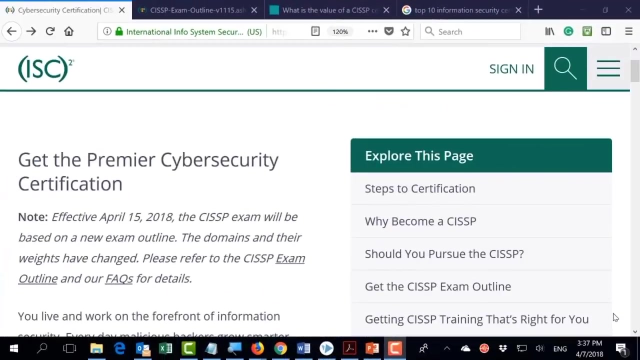 So it's quite important to relate or map whatever we are explaining to real life scenarios. This is the best way that will allow you, in a very short period of time, to understand the concept and How's the exam- Two things you need to know about the CISSP certificate. 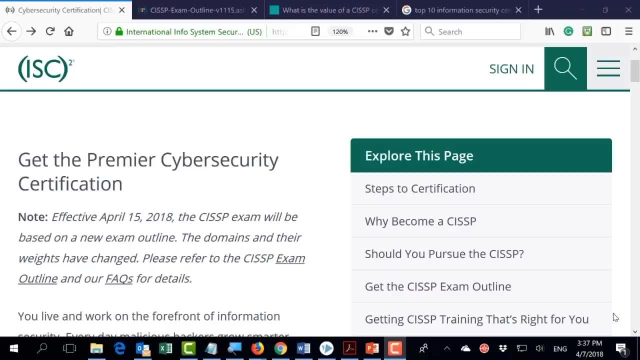 First, this certificate is technology neutral. I mean it's not explaining a specific technology, It's talking about general terminology related to security. After all, this is not a technical certificate, as I mentioned before. Second point says the CISSP: 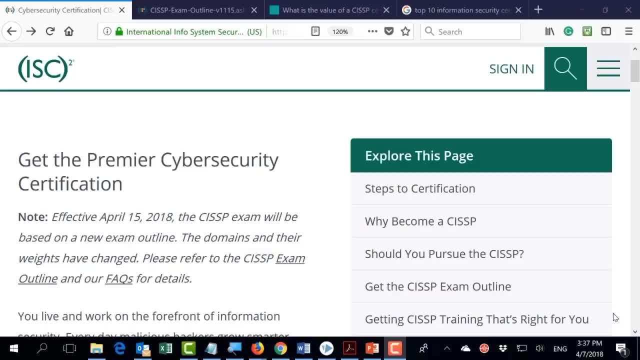 Keep changing. Sometimes they change the curriculum And sometimes they change the exam, And they do that every couple of years, So it's frequently keep changing. The one that is covered by this course is the latest one. This course is fulfilling the latest CISSP requirement. 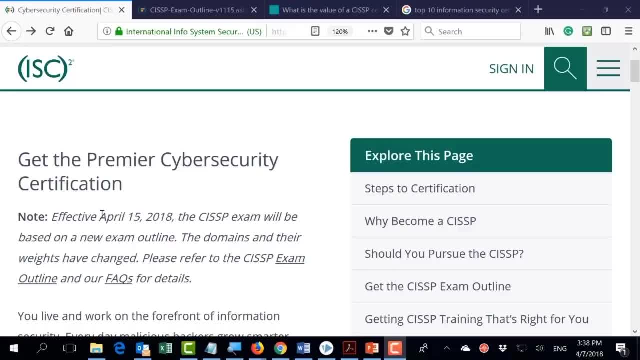 According to IC Square, the CISSP exam will change in The 15th of April 2018.. So this course is for the new CISSP exam that is effective after April 15, 2018.. It's the same curriculum. 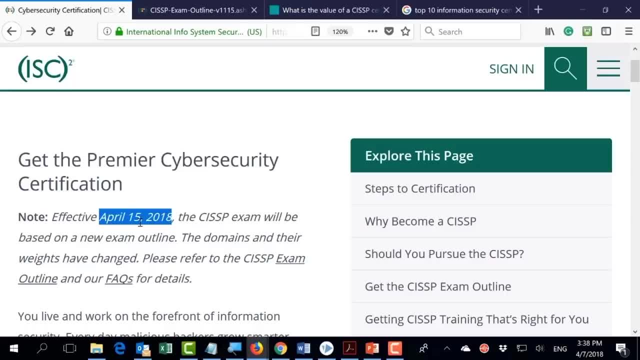 It's still eight domains, but the ways that they will be or the ways that they are changing the exam It's completely different than the previous one. in the new exam They have specific topics from the course that need to be Be covered very well to be able to pass the exam and get certified. 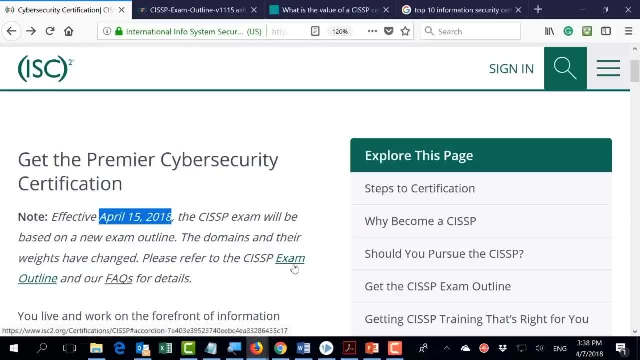 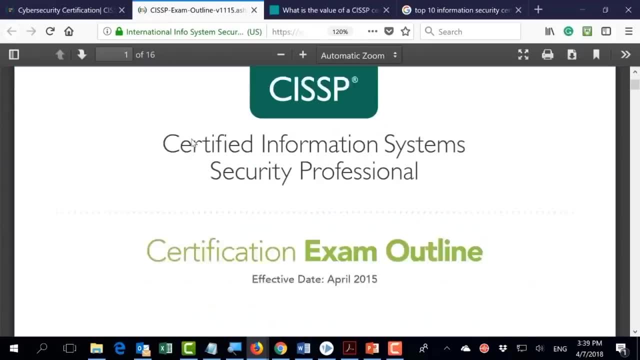 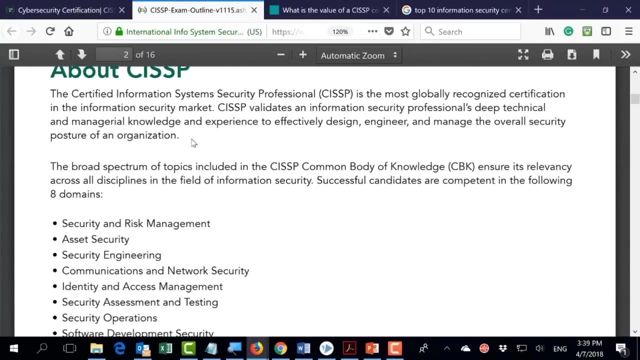 And in IC Square you will find a link. If you click on this link, it will show you all the details about the new exam. So this is the document from IC Square website. I will attach this document to the lecture, but you still can go yourself to IC Square website and download it. 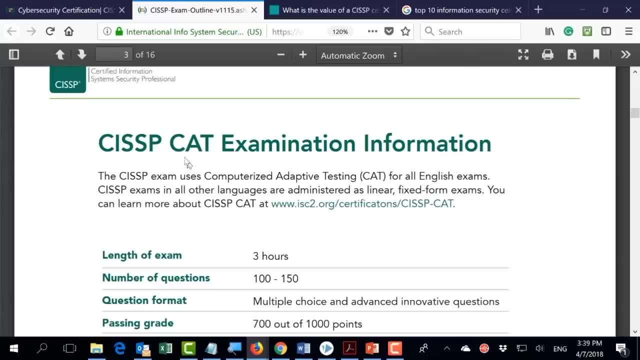 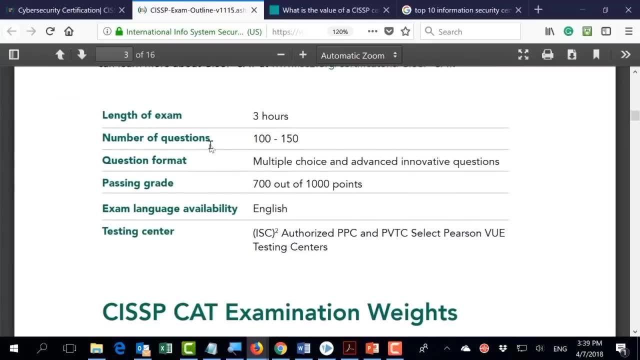 And here you're going to find the new exam information right now: CISSP. It's more interactive exam. It's called the CAT exam. It used to be six hour, Right now it's three hour and it has from 100 to 150 questions and multiply choice. 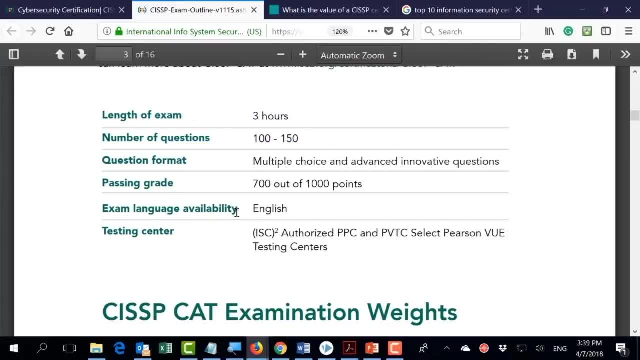 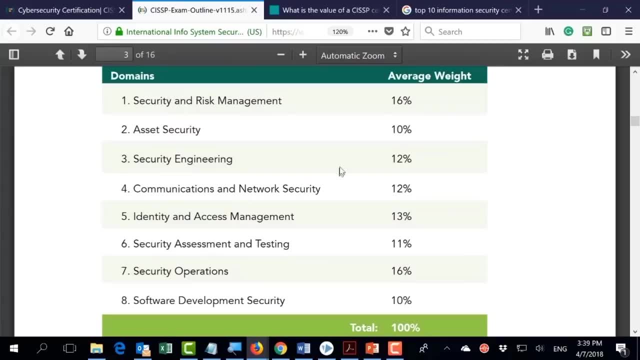 Passing rate is 70 percent, still like previous, and the exam language is English and where you can take the exam Now. those are the eight domains that we will be covering inside the course. The amount of questions related to each domain is here. 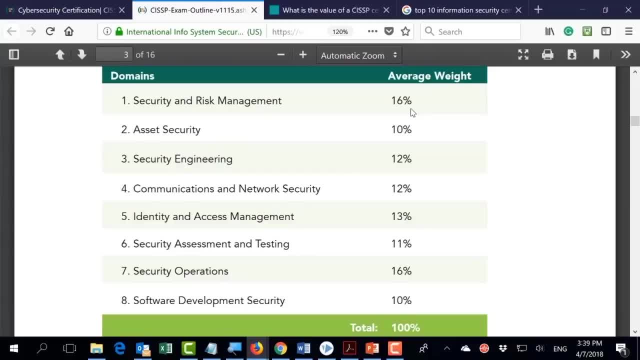 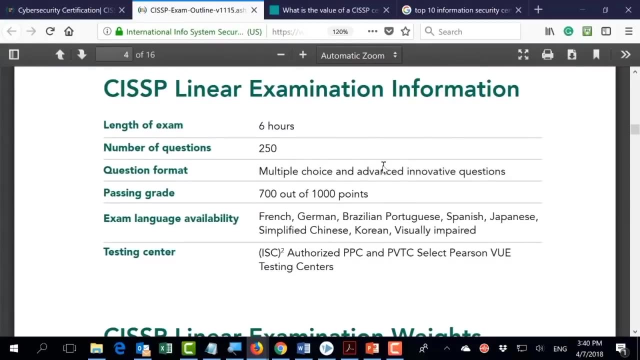 So risk management: Sixteen percent of the exam, which is a high percentage. asset management: 10,, 12.. But still you need to give attention to all domain. You don't want to lose any question. And this was the old exam. information used to be six hour, 250 questions, but it's not there anymore. 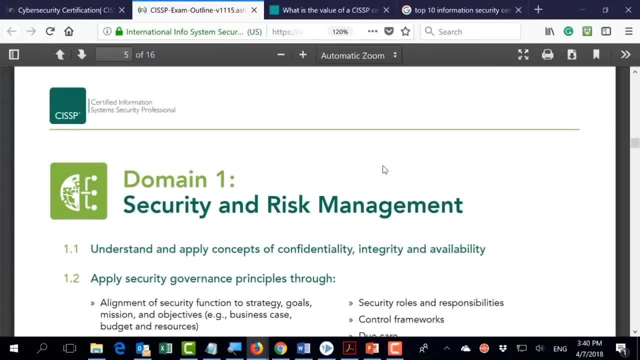 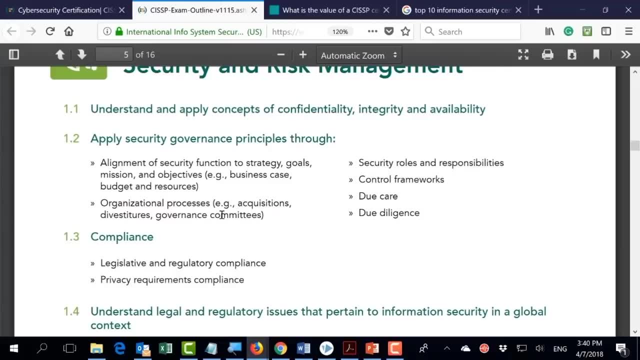 And it used to be ten domain, But right now it's eight domain and in each domain you will find what actually are the important Topic that you need to be aware about for this domain. So you need to understand the security governance and principle. 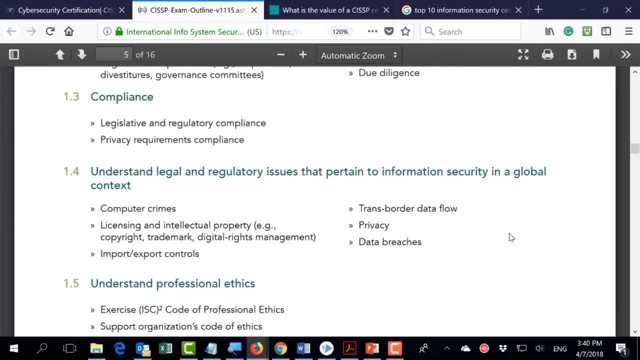 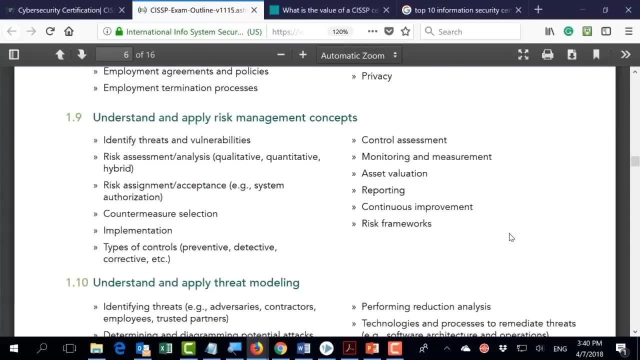 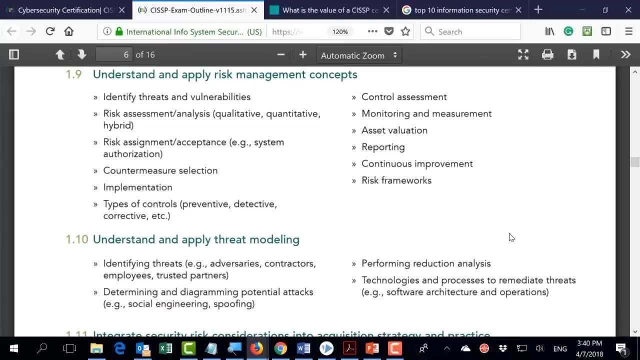 You need to understand the compliance, You need to understand the legal and regulation and so on. So it's like highlighting the important point of each domain, which will allow you to map those point to what you are learning in this training or in any other thing. 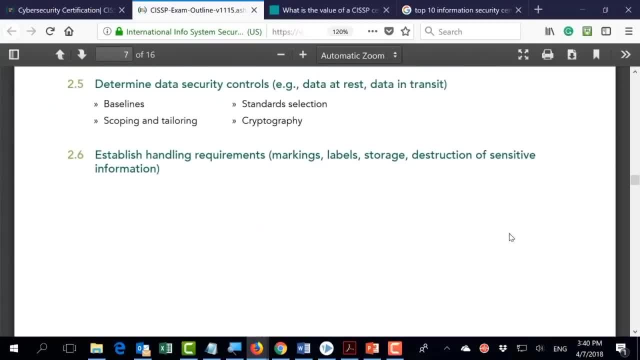 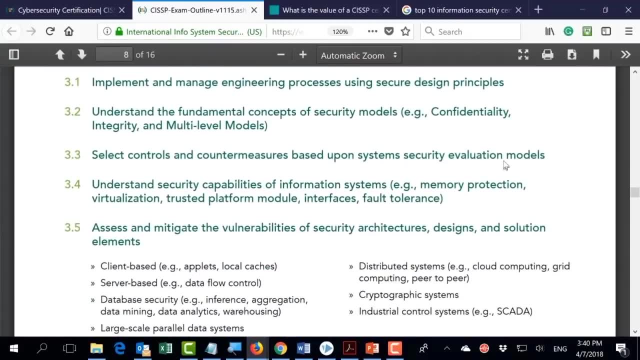 So it's quite important that You print this document and you keep it beside you And after finishing each domain, you need to understand or need to highlight the points that has been covered and you are comfortable with those points, And you need also to highlight the points that was not that clear. 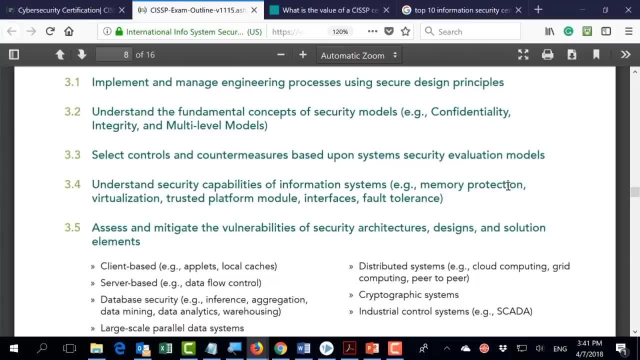 And You're going to have a channel to contact me directly in case you are missing any point or you need some additional resources or you have any doubts or A question about any specific point. but after all, this would be your reference before sitting inside the exam. 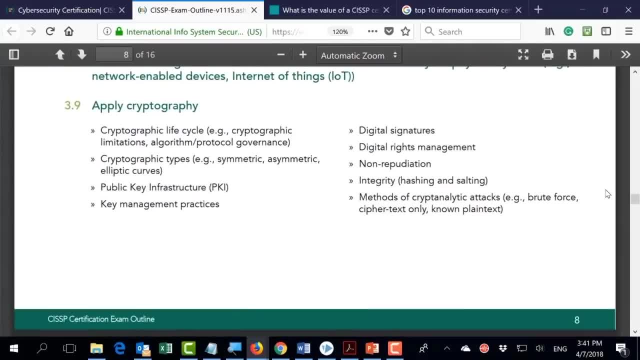 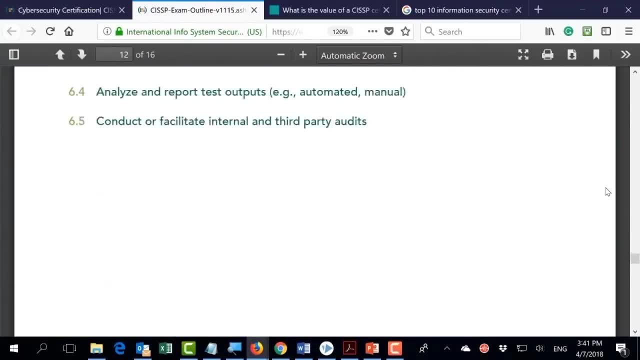 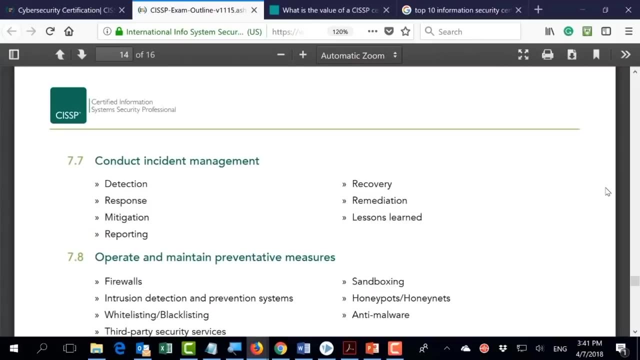 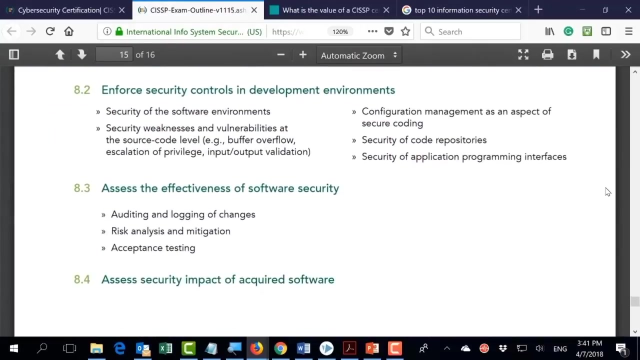 You should have a check sign beside each one of those points. So this is a very, very important topic, or a very important issue to consider. What are the requirements for the new exam that Is launched After April Two thousand and eighteen fourteen of April two thousand and eighteen? 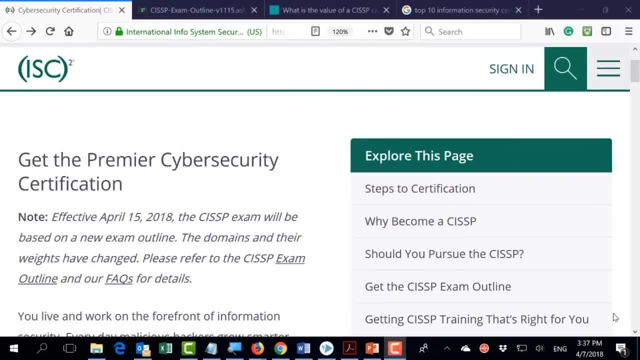 Two things you need to know about the CISSP certificate. first, this certificate is technology neutral. I mean, it's not explaining a specific technology, It's talking about general terminology related to security. After all, this is not a technical certificate. 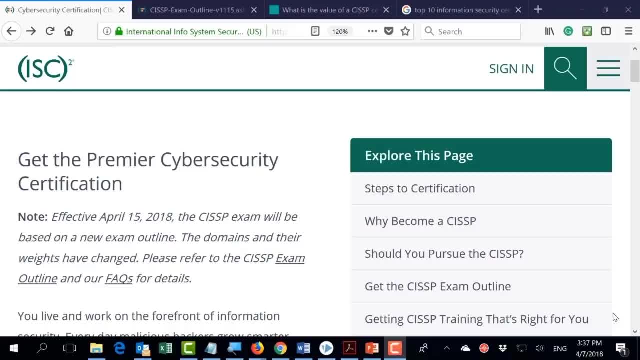 As I mentioned before. second point says the CISSP Keep changing. sometimes they change the curriculum And sometimes they change the exam, And they do that every couple of years, so it's frequently keep changing. the one that is covered by this course is the latest one. 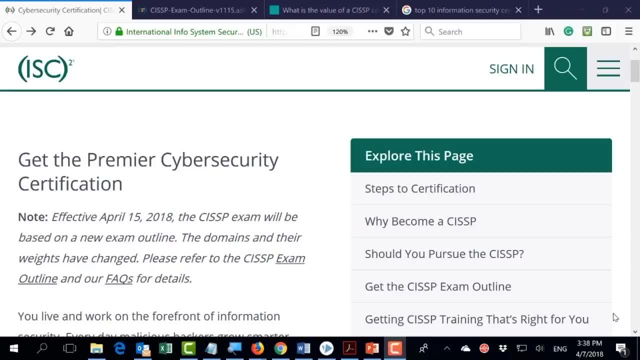 This course is fulfilling the latest CISSP requirement. According to IC Square, the CISSP exam will change in 15 of April two thousand and eighty, So this course is for the new CISSP exam that is effective after April 15,. two thousand and eighty is the same curriculum. 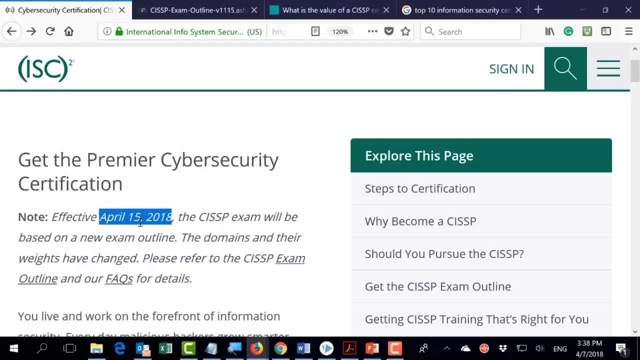 It's still eight domains, but the ways that they will be or the ways that they are changing the exam It's completely Different than the previous one. in the new exam they have specific topics from the course that need to be covered very well to be able to pass the exam and get certified. 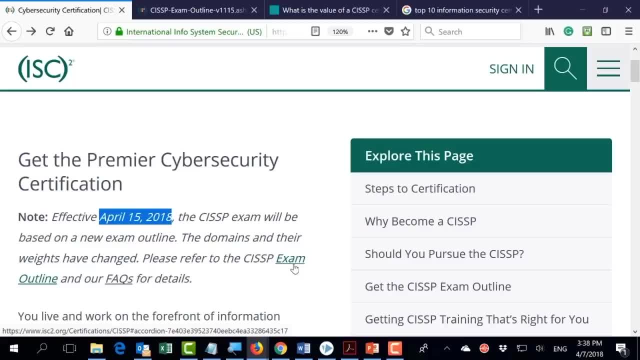 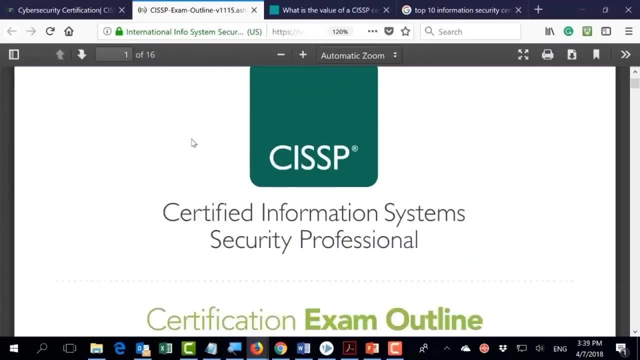 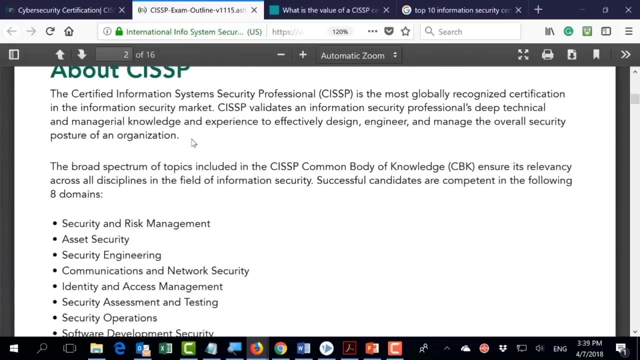 And in IC Square you will find a link. If you click on this link it will show you All the details about the new exam. So this is the document from IC Square website. I will attach this document to the lecture, but you still can go yourself to IC. 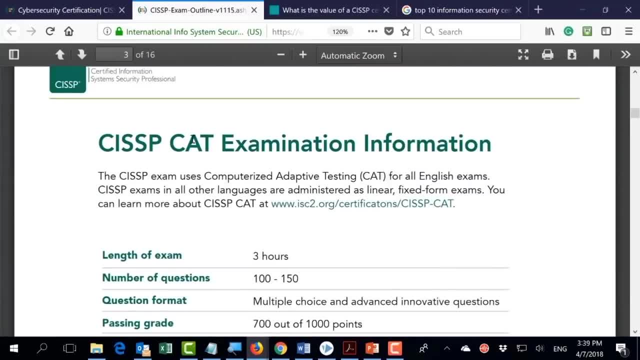 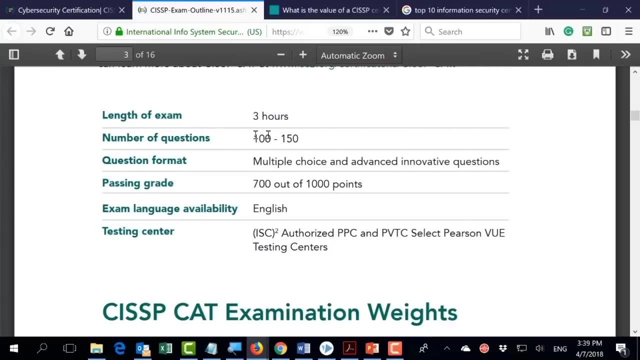 Square website and download it. And here you're going to find the new exam information right now CISSP. it's more interactive exams, called the CAT exam. It used to be six hour, Right now it's three hour and it has from one hundred to one hundred and fifty question and multiply choice. 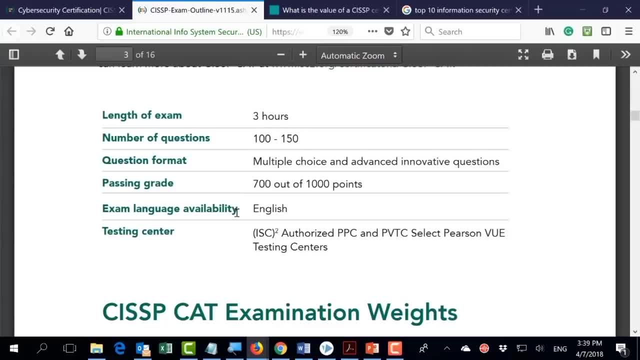 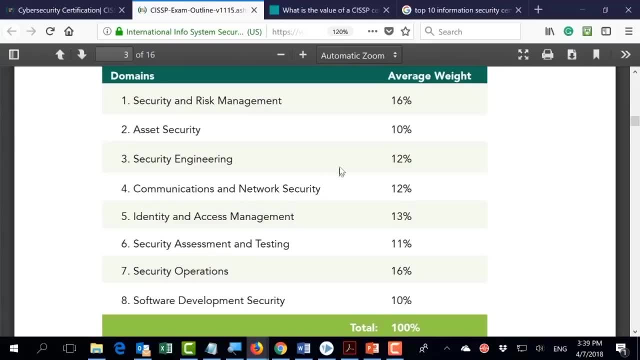 Passing rate is 70 percent, still like previous, and the exam language is English and where you can take the exam Now. those are The eight domains that we will be covering inside the course. the amount of questions related to each domain is here. 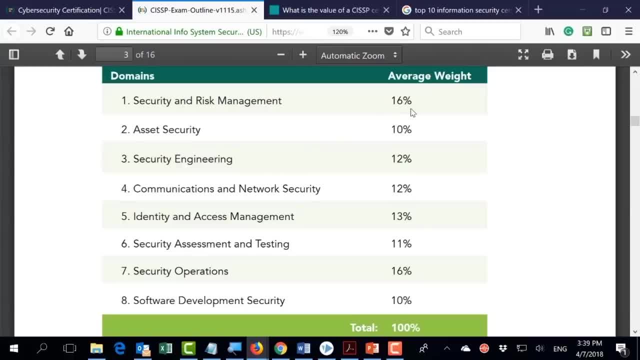 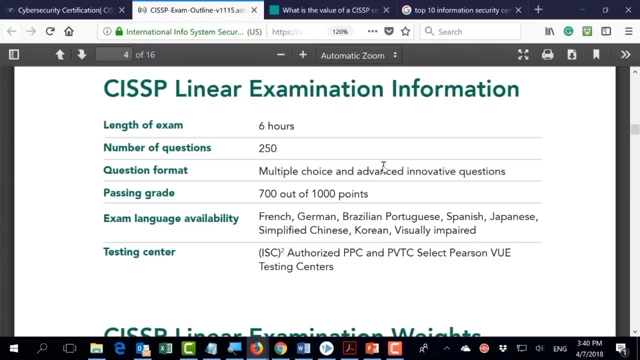 So, risk management: 16 percent of the exam, which is a high percentage. asset management: ten twelve, But still you need to give attention to all domain. You don't want to lose any question, And this was the old exam. information used to be six hour one hundred and fifty questions, but it's not there anymore and it used to be. 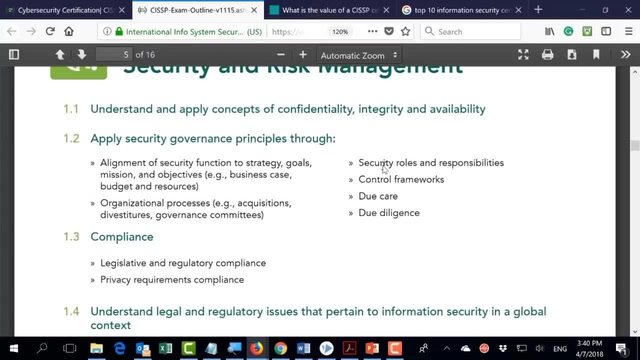 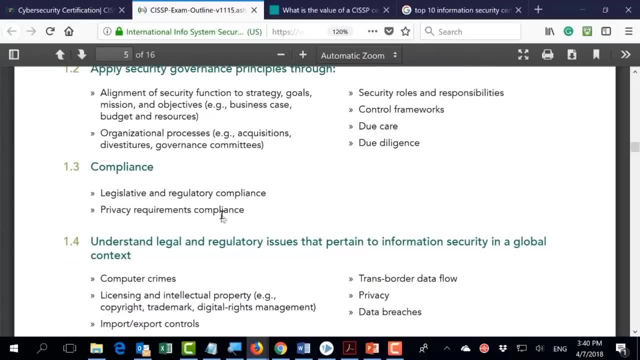 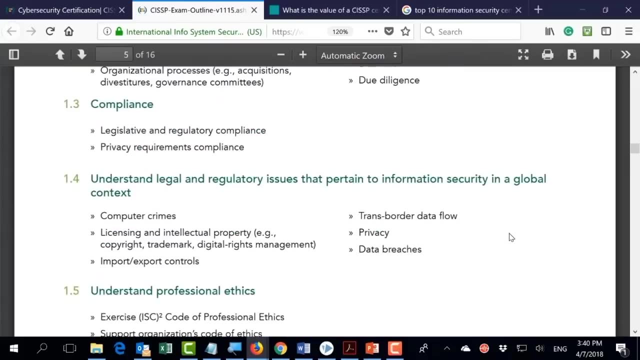 ten domain, But right now it's eight domain and in each domain you will find what actually are the important topic that you need to be aware about for this domain. So you need to understand the security governance and principle. You need to understand the compliance. 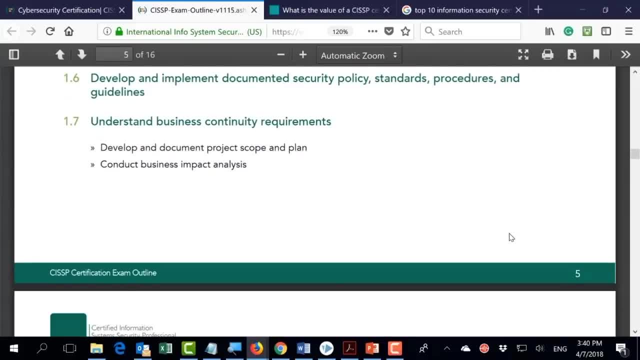 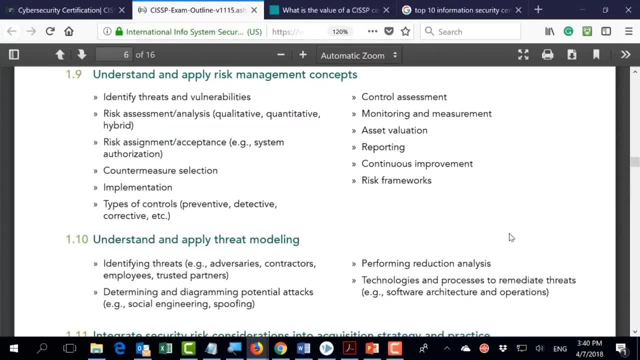 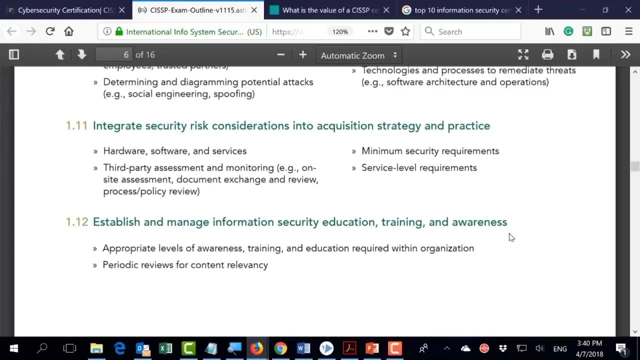 You need to understand the legal and regulation and so on. So it's like highlighting the important point of each domain, which will allow you to map Those point to what you are learning in this training or in any other training. So it's quite important that you print this document and you keep it beside you. 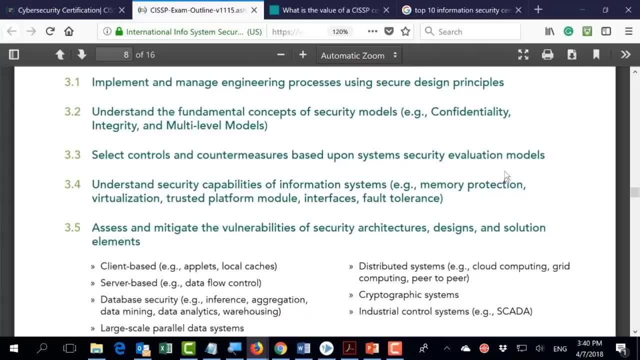 And after finishing each domain, you need to understand or need to highlight the points that has been covered and you are comfortable with those points, And you need also to highlight the points that was not that clear And You're going to have a channel to. 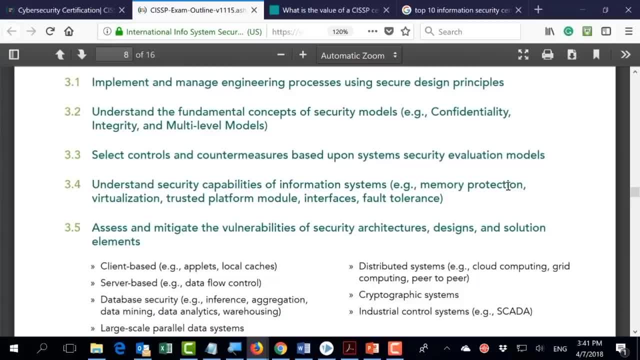 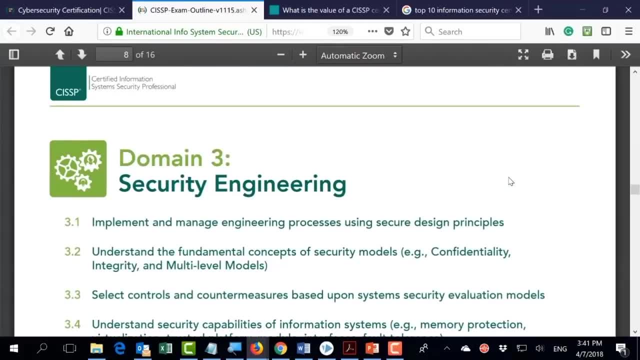 Contact me directly in case you are missing any point or you need some additional resources or you have any doubts or question about any specific point. But after all, this would be your reference. before sitting inside the exam, You should have a check sign beside each one of those points. 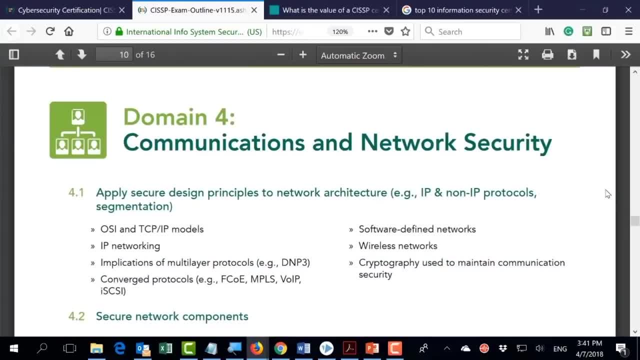 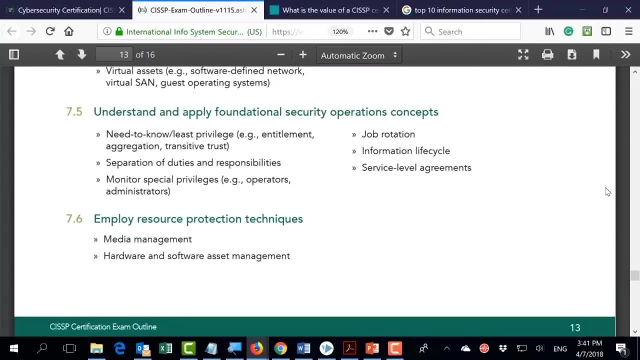 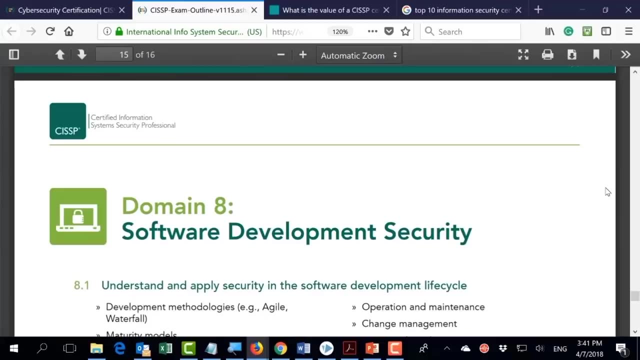 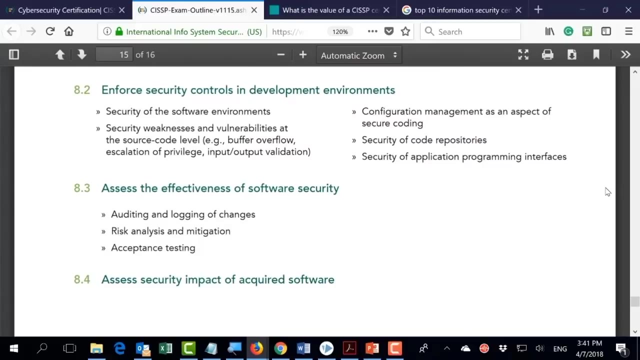 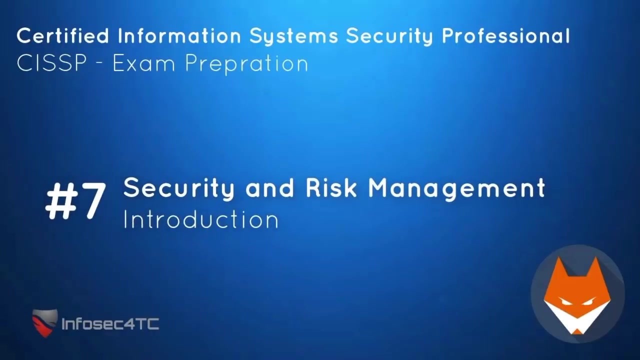 So this is a very, very important topic, or a very important issue to consider. What are the Requirements for the new exam that is launched after April two thousand and nineteen fourteen of April two thousand and eighteen? The first domain of this course will be about security risk management. 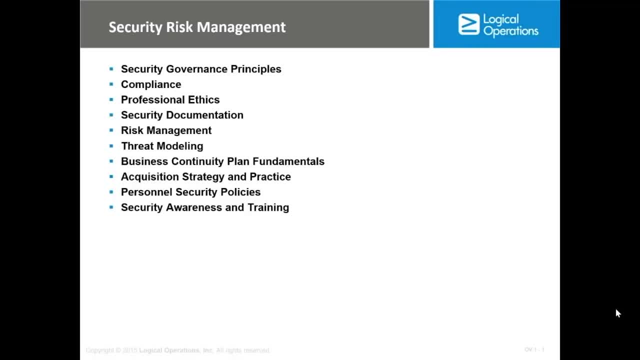 And this is a very important domain And it includes A lot of point topics that we will be covering, And even inside the exam you will find good amount of questions related to risk management, because actually, The first approach to any security implementation should be from the risk management perspective. 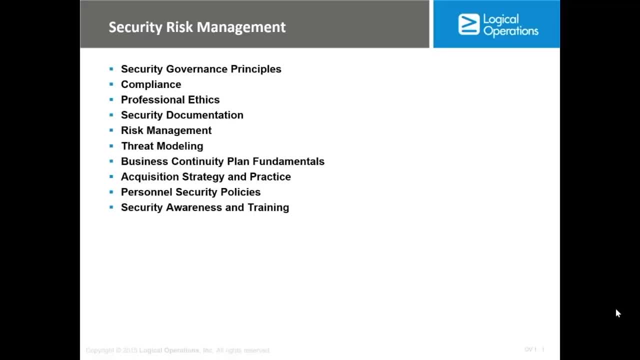 So you need to understand What do we mean by risk management? What is risk in the first place? Can we calculate risk? Do we have risk management strategy? So you don't have to worry, because you're going to start from scratch and we're going to explain the risk management process step by step, with a lot of real life scenario and a lot of templates that will help you, if you are doing a risk assessment yourself, to be able to understand how it's done. 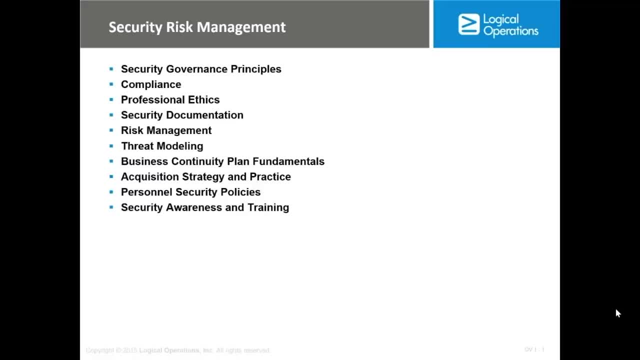 But the domain is not only covering risk management, But we're going to cover a lot of other points like, for instance, we're going to start with some definitions, which is quite important to this training, So you need to understand what is risk, what is threat, vulnerability, governance, compliance. 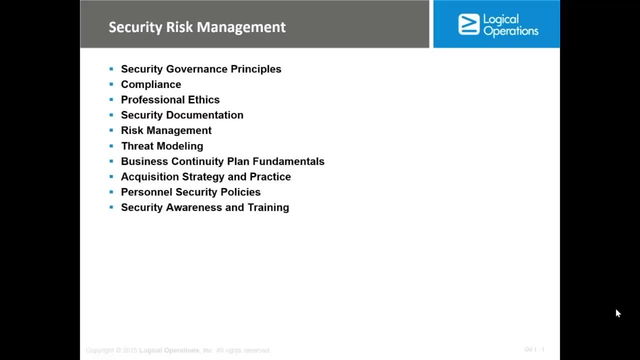 Those are very important terminology for anyone who is working in information security. So we're going to start with some definitions: What is CIA? and other relevant definitions. Then we're going to talk about security documentations. Realistically, you will be involved with a lot of documentation in your work policy, procedures, guidelines. 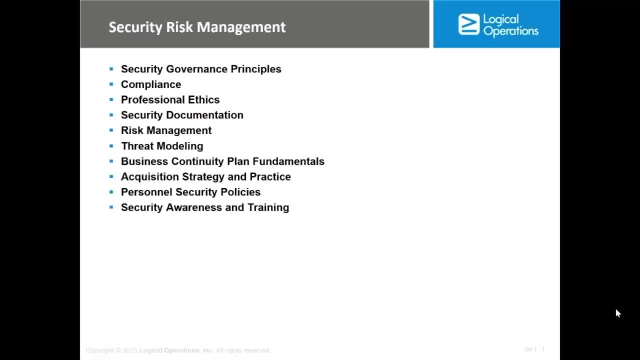 You need to understand how it's done. from where can you get templates? What is the difference between the policy and procedures and baseline and guidelines and so on? So it's important to know the main documentations that we are using. And then we're going to talk about risk management. 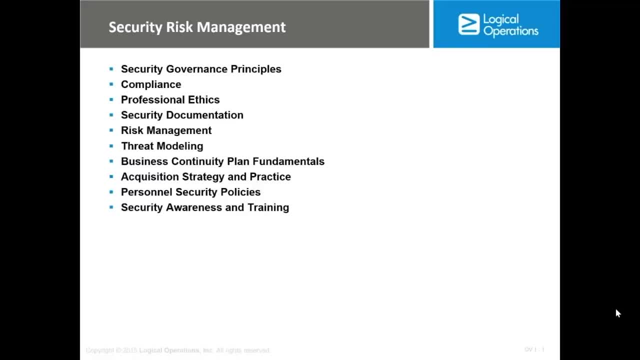 This is a very, very, very important topic. You need to understand risk from scratch, because it's a main core of any security implementation. Then we're going to talk about threat modeling. Also, we'll be talking or covering the business continuity planning. 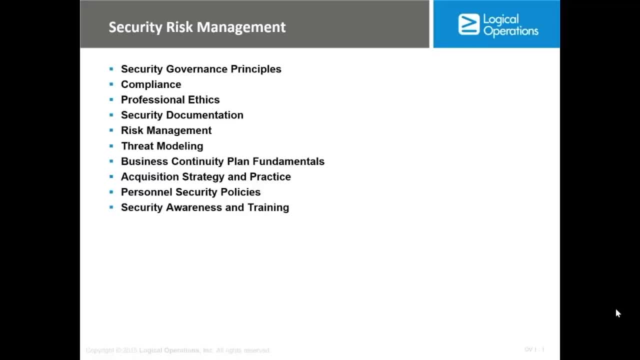 And I'm going to show you how it's done and what is the difference between business continuity and disaster recovery. We will be talking about risk management. We will be covering accusations, strategy and practice, personal security policies and security awareness and trainings. 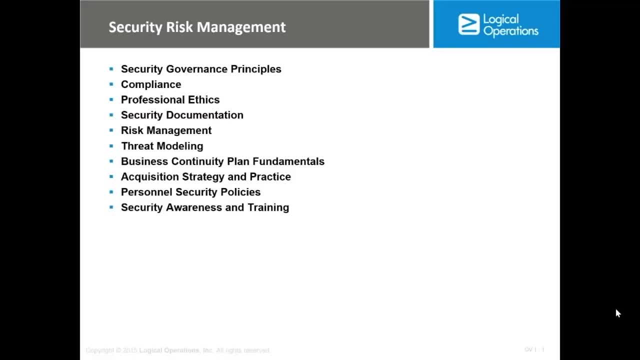 So those are some of the points that we're going to cover in this domain, But It's not about the definitions, because it will not help you if you just understand the concept. It's not really what we are looking for. I want you to relate whatever we are explaining with real life implementation. 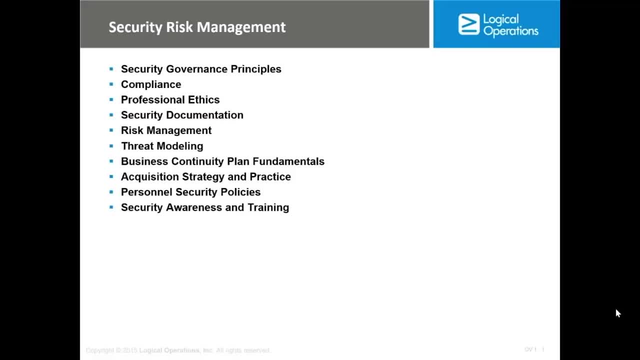 So, for instance, if we are talking about risk management, you need to understand what is risk management. What is risk assessment? is a different type of risk assessment, How it's done, What is the risk management strategy? Can we calculate risk? 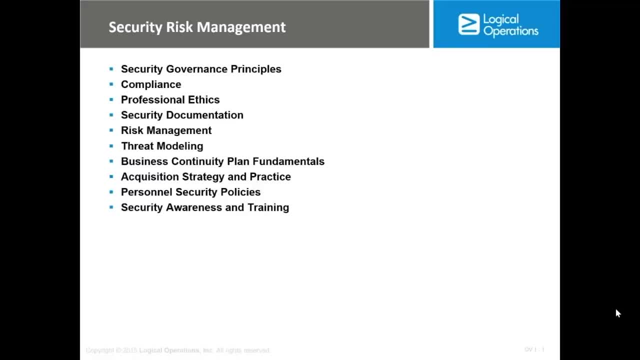 So you need to start from scratch and you need to know how it's done with real implementation or real documentation. That's why, on the student portal, you will find a lot of templates. So if we are talking about risk assessment, For instance, and you need to know how it's done. 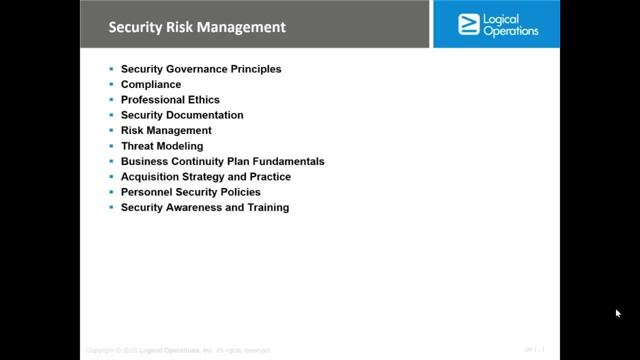 I will show it to you. but also I'm going to keep some templates on the student portal that will help you. If you are doing that realistically or if you get hired somewhere, you will be knowing or having some documents that will guide you how to do it. 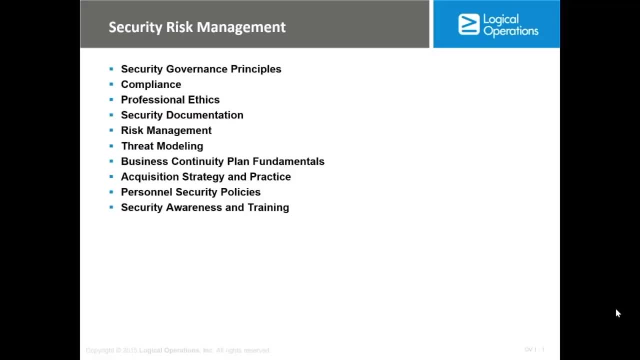 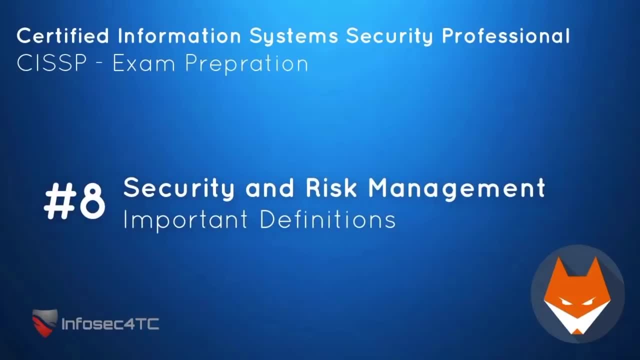 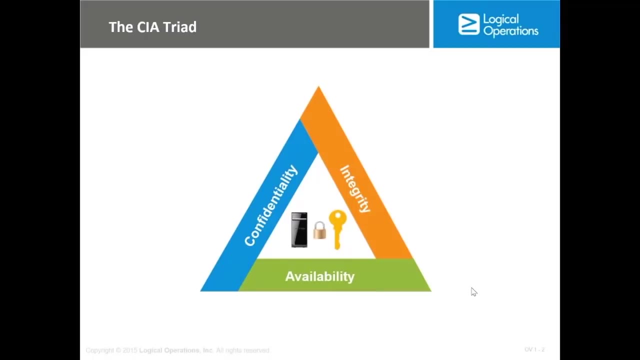 So it's important to relate whatever we are talking about with real life implementation. In this lecture, We're going to explain some important information security terminology. Those terminology Will be used during this training and you will use them realistically in any job or any position. 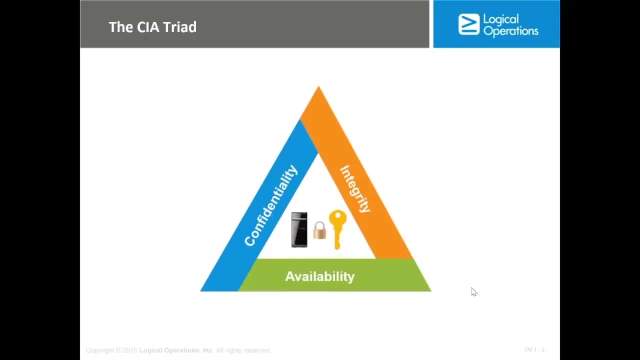 So we're going to start with a very basic definition, which is the CIA terminology. Right CIA, which stands for the confidentiality, integrity and availability, Is the definition of the security. Let me explain it in a different way. How can you define? 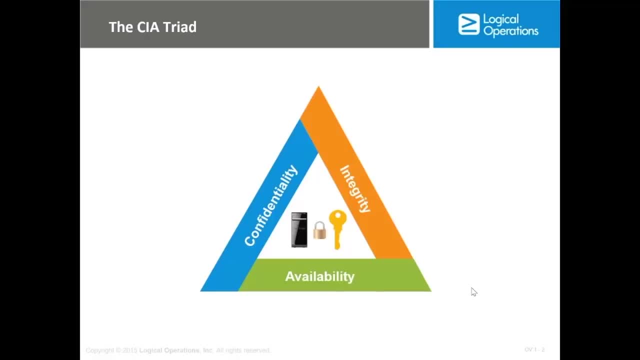 Security. How can you say that Your company is secure? or let's take it on a smaller scale: If you have a laptop Or a smartphone, How can you see that this smartphone is secure? If you just assign a password on it, you will consider that secure. 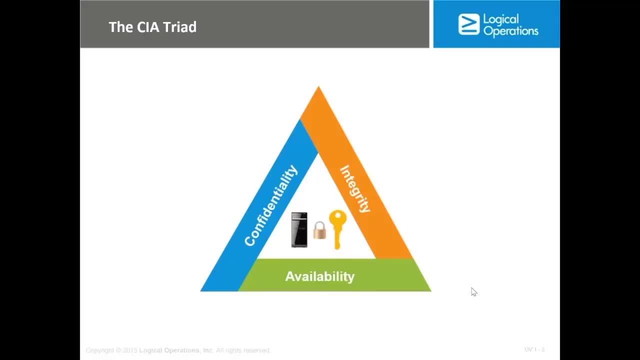 Okay, maybe you have a smartphone and you did assign a password on it so you can prevent unauthorized people or unauthorized access. But what if you lost the phone? That's mean you lost the information. So I cannot say say, saying that just by assigning a password we will consider that security. 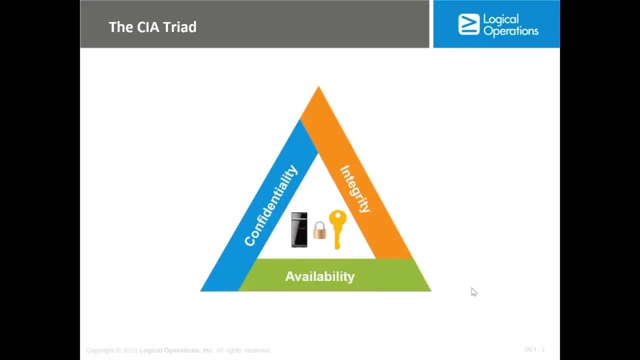 So security is to provide three different elements. First, confidentiality, Which is making sure that no authorized user can access the information, And a good example will be a password- Assigning a password on my computer or on my smartphone or on any system. Why I'm doing that? 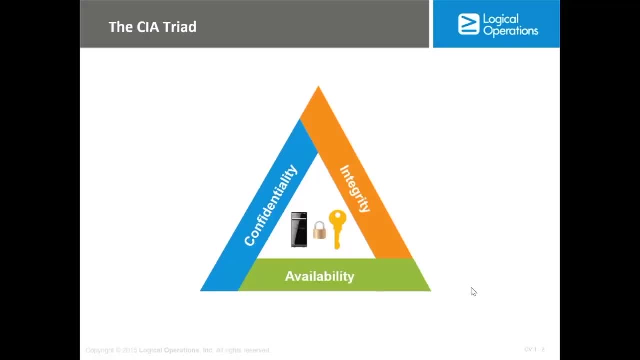 Because I need to make sure that only people who got the password will be able to access the information, Which reflects that only people who are authorized can access the information. But if someone is not authorized to access the information, I will not give him a password. 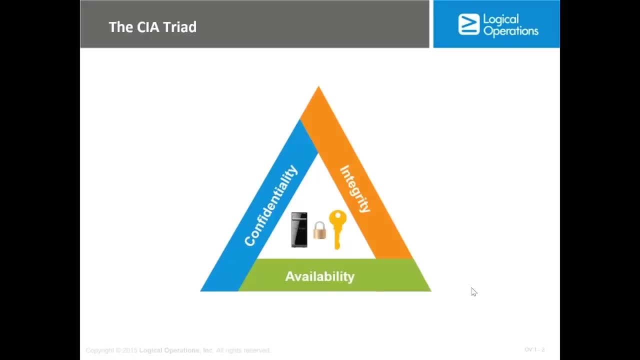 This is a small definition of confidentiality. Okay, Integrity, Which means data should not be manipulated Or should not be changed. So what? I have a lot of critical information. They have not been hacked or stolen, but they have been modified, So I need to prevent that. 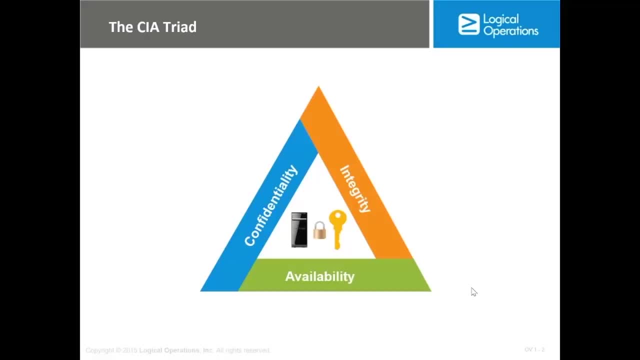 I need to put some control. that information should not be been modified unless it's authorized. So I cannot have a bank account that has $1000. And tomorrow I check it's $50.. Someone logged in and changed the information. He didn't steal the information. 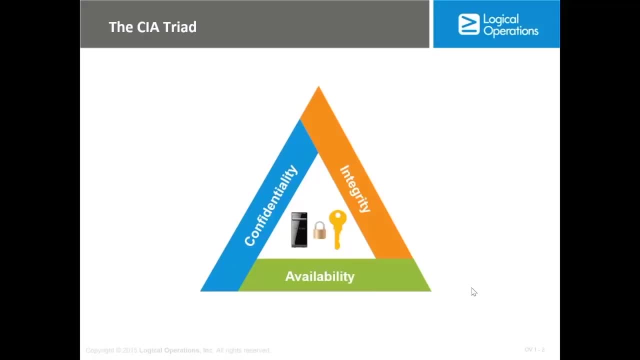 He changed it. So providing integrity is one of the security element. Third is availability. So also one of the important element in any security is to Make sure that the information is available all the time And, if you are take, If we are talking about the security, 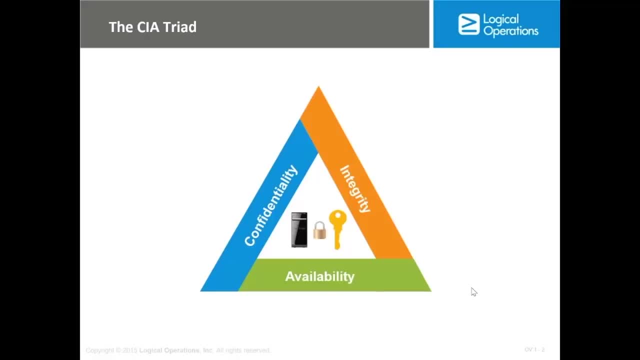 If we are talking about the same example, which is your smartphone, And assume that this smartphone has a lot of important information- Contacts, emails, personal picture, personal videos and so on- And you did secure it with a password, but you lost it. 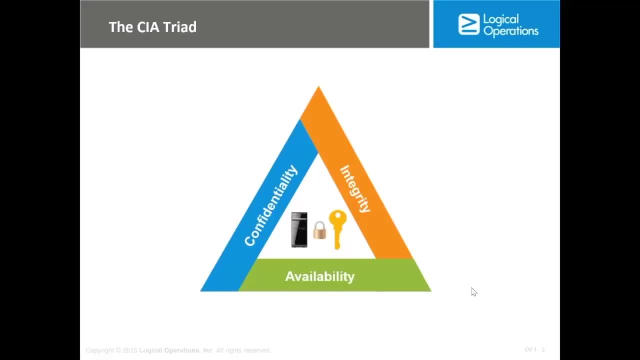 You lost the information. The password didn't help you, But if you are taking backup of the information and you lost your phone And the information- it's backed up so you can restore it on any other device- Then you provided availability for the information. 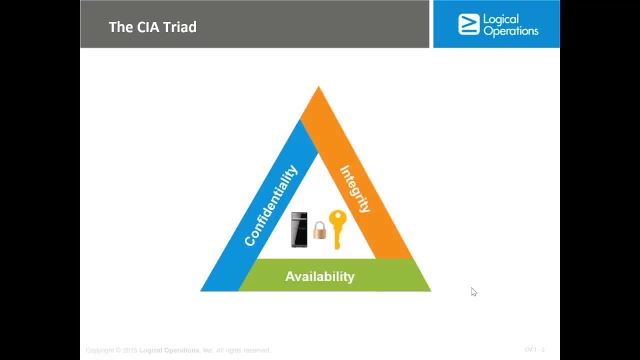 So my point here: whatever we are doing in information security should provide one of those three elements. If you are assigning password, we are talking about access control and assigning password, We are doing that to provide confidentiality. If we are encrypting the information, we are encrypting the information to provide confidentiality and integrity. 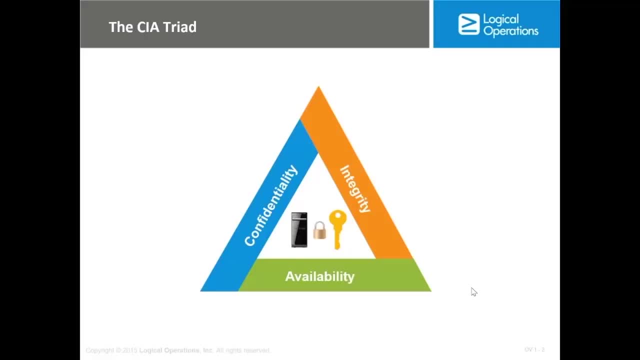 And we're going to see that, while we are talking about cryptography, If you are taking backup, it's for providing availability, And usually we are writing that in most of our security documents that we did this solution to provide the following element: Confidentiality, integrity, availability and so on. 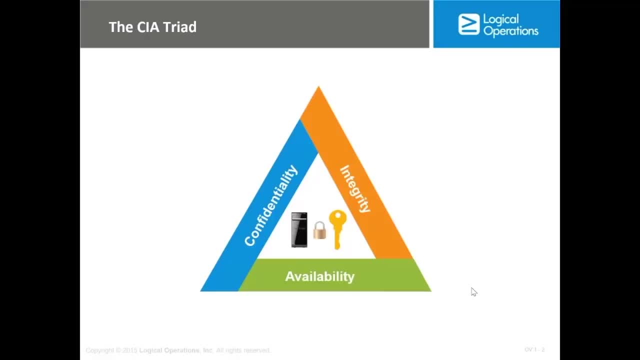 It may seem easy to understand, but sometimes you get some question about that. It's kind of tricky. Sometimes they will ask you, for instance: Backup is for providing what? Is it confidential? Is it integrity? Is it availability? Backup has nothing to, I'm sorry. encryption. 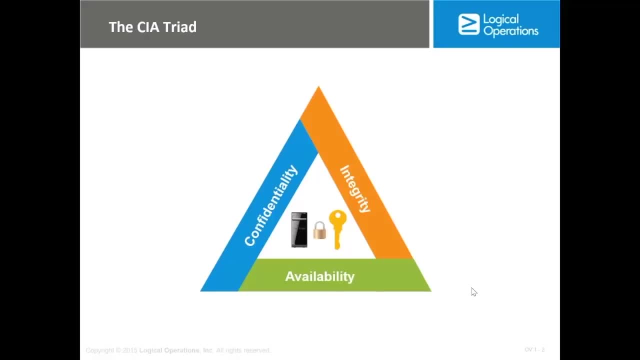 Encryption is for providing what It's for providing confidentiality and integrity, And it has nothing to do with availability, While backup it's availability solution and so on. So whatever we are doing in this training should be- or actually in information security in general should be- to provide one of those three elements. 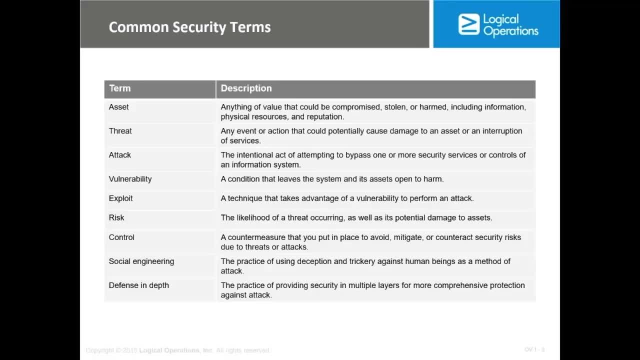 The second important definition set of definitions that I would like to refer to Will be the following: first, assets: What is an asset? Now, to be able to explain the asset, we need to like distinguish between physical asset and information asset. OK, 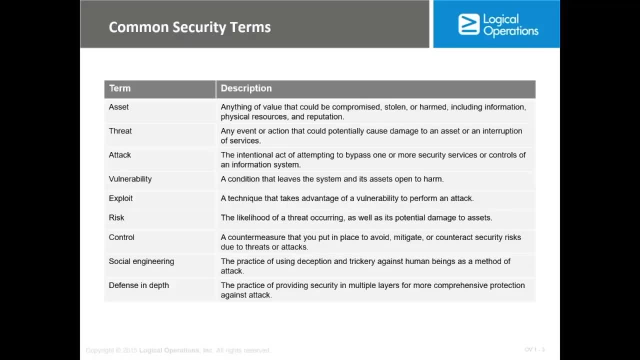 So, for instance, let's take your smartphone one more time. Your smartphone has a lot of information on it, right? This information you know could be very important for you. You may have important contact, important email, important document, picture, and so on and so forth. 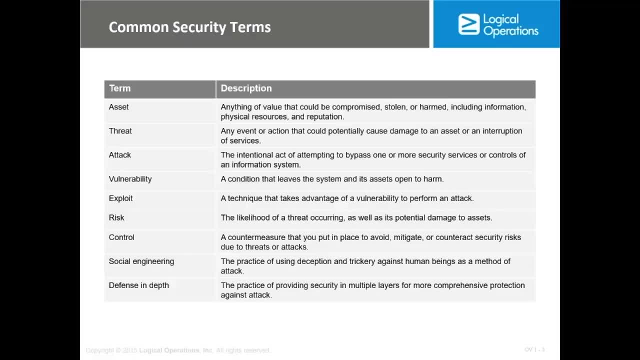 If you lose your phone for some reason, you forget your phone somewhere or you lose it somewhere- What will be your main loss? It will be the phone, It will be the phone price or it will be the information on your phone. Most probably, you will be more upset about the information on your phone because it will take you time, especially if you are not taking backup frequently. 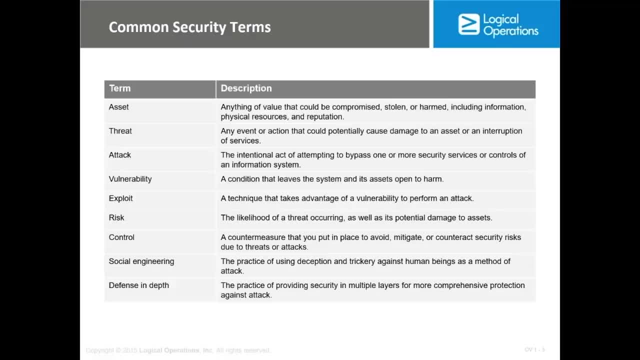 So you need to get all those contact again and you need to get all those emails and all those information one more time Right? So we usually have two different types of assets. We have the physical assets, things like computers, disk shares and so on. 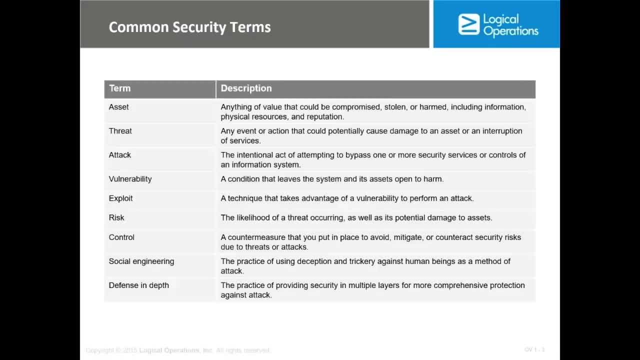 And we have the information asset, which is most cases, are more important to any business or personal than the physical assets. So most of the time, the information that you have on your laptop, it's more important than the laptop itself, Or on your smartphone or on your tablet, and the same concept is, and even more it's, on the business perspective. 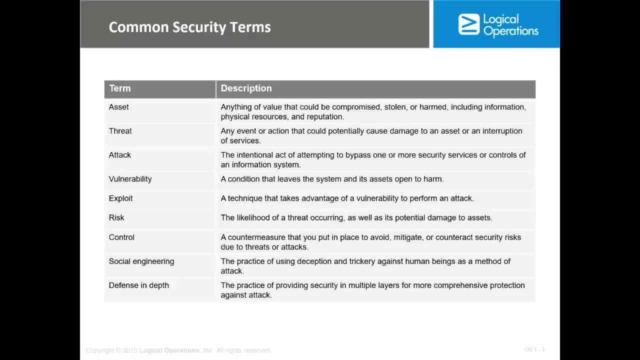 So usually business the information that they have. It's more valuable and more important than the physical assets. Think about the bank In a bank, The information that they have, all the customer information and all the financial information, transaction and everything. 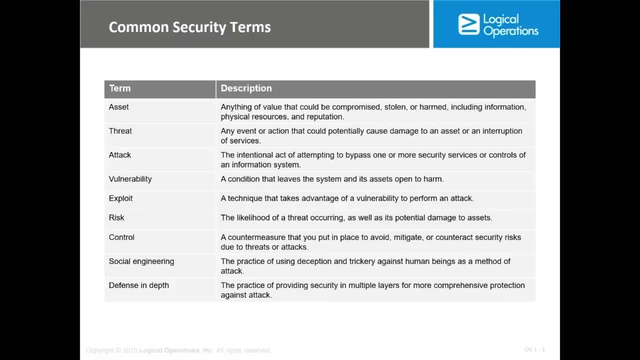 Is this more valuable than the physical asset of this bank, Like shares And table and so on? I mean, for instance, if a bank lost a share, share get broken or a computer get broken or crashed, It's some kind of damage. 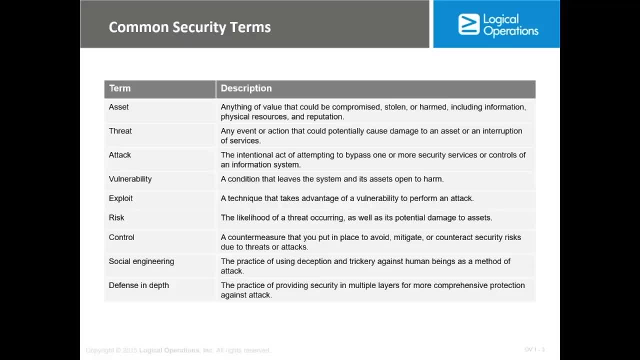 Okay, It will cost them some money, But what if they lost their customer information? What do you think about that? Think about the bank that lost all the customer information and their balance. What will be the loss, The damage, The low cases that will be against them, and so on and so forth. 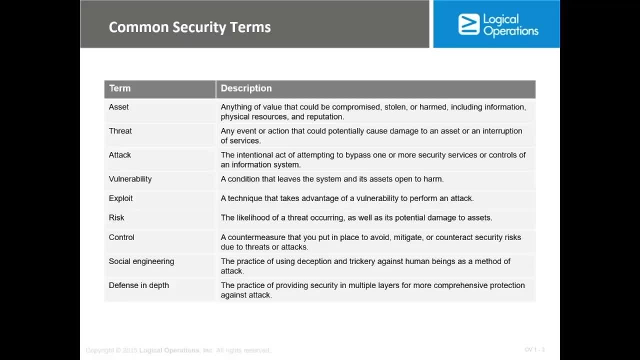 So usually, and because we have a specific domain about that, as an organization you should have A list of all your assets, especially the information assets. A lot of people will have an inventory for their physical assets. They know all the computer, all the shares, all the tables. 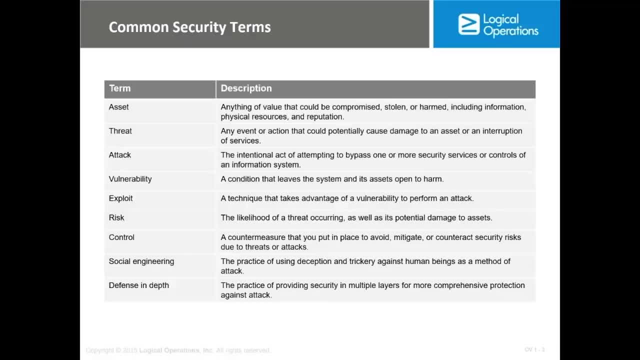 They have an inventory for them, But Many companies don't have the same list. that includes the information asset, which is realistically more important than physical assets. So it's quite important to understand what we are protecting, Because in another like way, I cannot have an assets that worth million and spend a couple of thousand of protecting them, or vice versa. 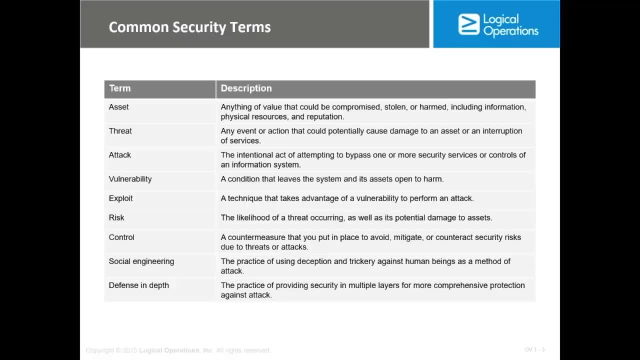 I may have assets that doesn't worth that much And spending one million to protect it. So it's an important concept to understand. But don't worry, we'll cover that in upcoming lectures. So you need to understand that I need to identify what exactly I am protecting. 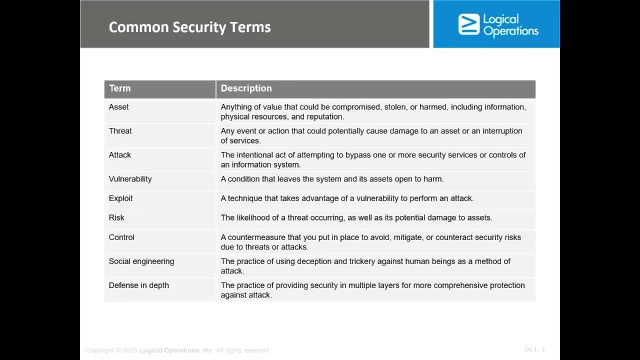 What is my assets? Information assets, which is more most important, and physical assets as well. Now we're going to talk about threat, vulnerability and risk. I will not spend a lot of lectures talking about definitions, Because I will divide the definitions on different relevant lectures. 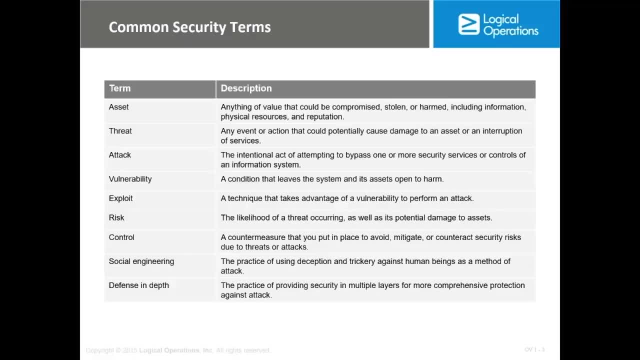 So what is a threat And what is a vulnerability? Okay, Vulnerability is a weakness in your system. Now, before explaining this part as well, you need to understand that we are not talking only about technical security. We are talking about technical security in this course. 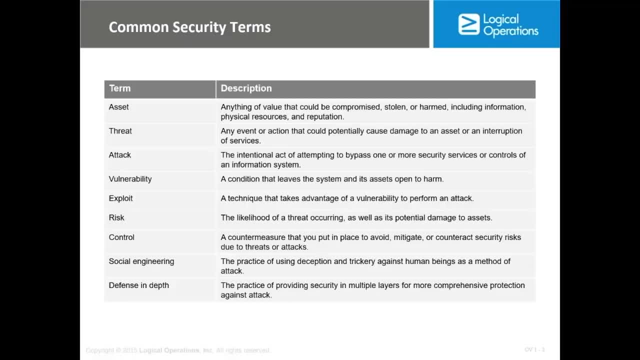 And physical security and administrative security. So when I'm talking about weakness, I don't refer only to weakness into the computer system and the servers and so on. I'm talking about any kind of weakness. So, for instance, you may have a door that doesn't have a lock. 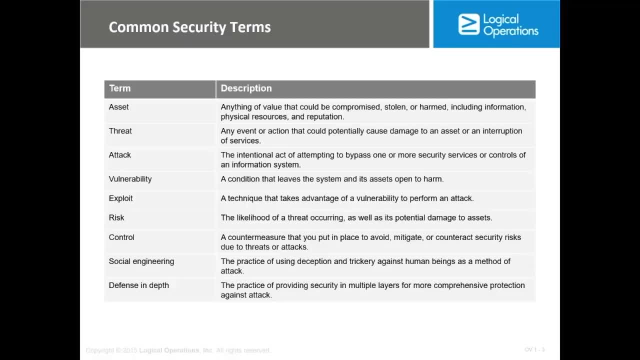 It's a weakness. You maybe don't have enough firefighting equipment. It's a weakness. So you need to understand that security is a very generic concept And when we are talking about information security, we are talking about securing them technically and physically, and administrative security as well. 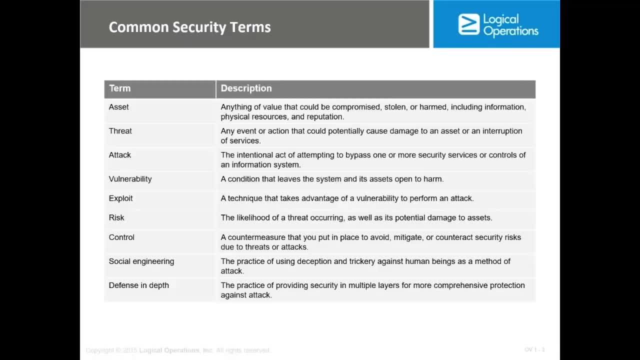 And we're going to give a lot of examples while going through this course. But again, vulnerability is a weakness in the system, While threats it's an event that potentially may come and may do some damage. Let me give you a small example. 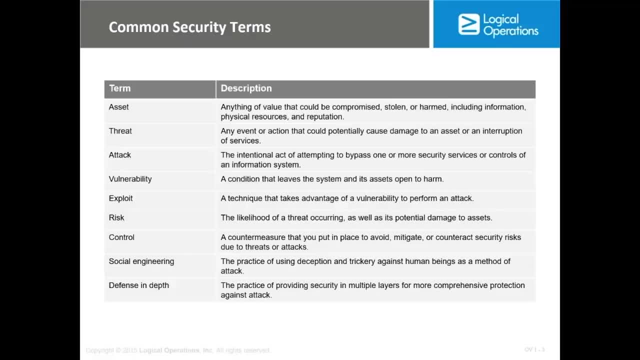 Let me start with a technical example. If your computer doesn't have an antivirus, this is a vulnerability. It's a weakness. What could go wrong because of that? You may get infected with a virus. This is a threat. If you don't have a firefighting equipment in your building, this is a vulnerability. 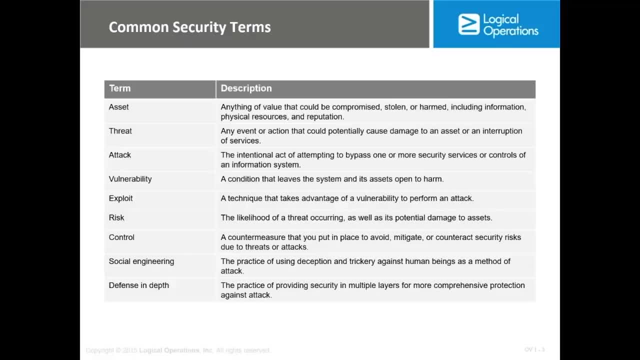 What could go wrong because of that Fire may happen. This is a threat. So this is the difference between a vulnerability and a threat. Not all vulnerabilities will have a threat, So, for instance, I maybe don't have an alarm system in my company. 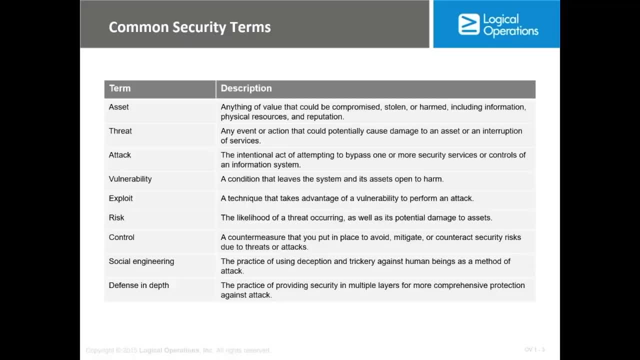 It's a vulnerability, But I have an alarm system in the whole building, So I don't have a threat because I already have an alarm in a different place, But in my company I don't have. So what I'm trying to say is that not all vulnerability will have a threat. 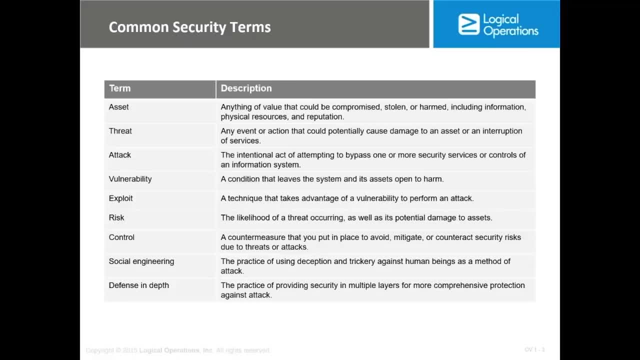 I may have an open port on my computer. It's a vulnerability, But I don't have any program or any service that can be hacked because of this port, So I don't have a threat. So usually when we are identifying all vulnerability, we need also to identify the threats related to them. 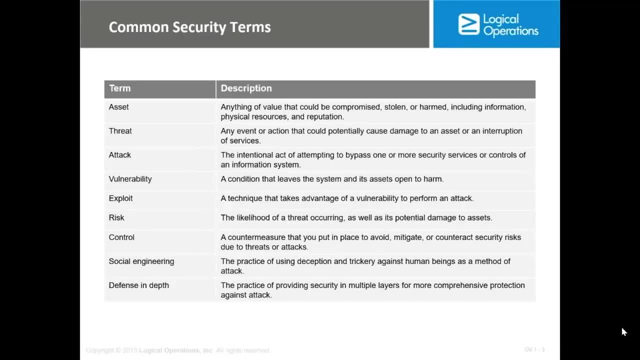 I will not spend too much time explaining definitions because I decided to divide them on different levels- Relevant lectures- But I will go through the important part. So I explain the assets, the threats, the vulnerability. I need to talk about risk, which is the main concept in this domain and a main concept in security in general. 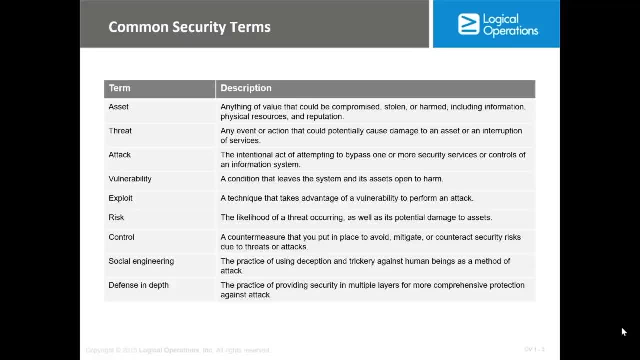 What is risk? A lot of people think about risk that it's a technical terminology, which is not: It's a business terminology. So what do we mean by risk? Because you need to distinguish between threat and risk. What is risk? I'll give you a small example, because in this domain, you're going to learn how to calculate risk. 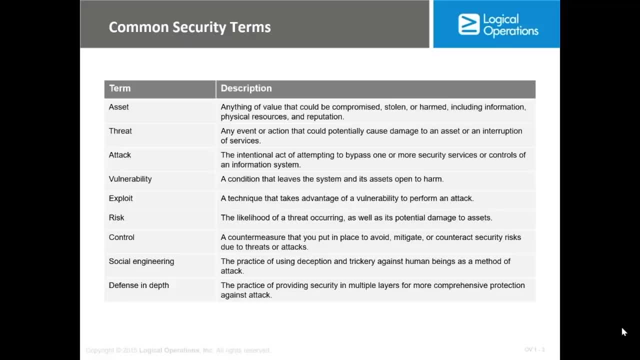 It's important, So I will assume that we have. we don't have enough firefighting equipment in our company. What do you consider that? Is it a threat or a vulnerability? It's a vulnerability that I don't have enough firefighting equipment, sprinkles and so on. 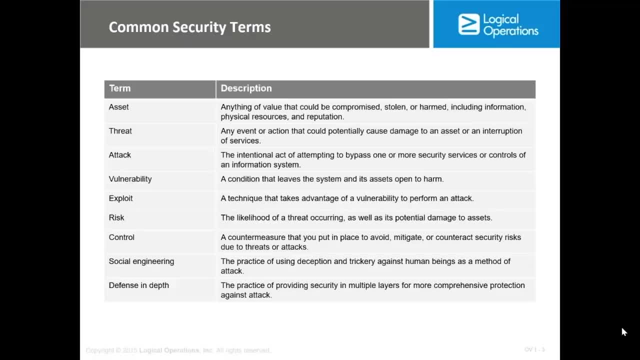 Now, What if a fire happened? What do you consider the fire? It's a threat. So what if a fire happened And, according to that, There was some damage in the company that was one hundred thousand? What do you consider that this is the risk? 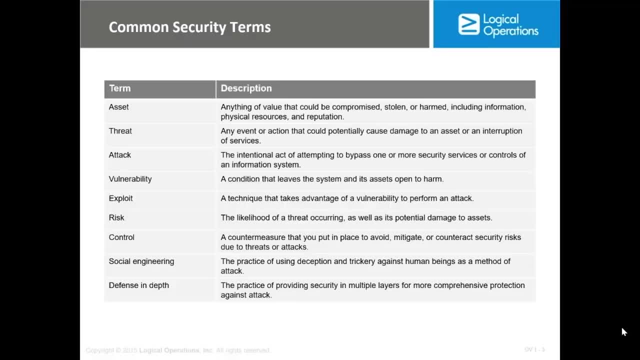 So the risk is the likelihood of a threat occurring, But most important is the damage That will happen because of the threat, And we're going to learn, And we're going to learn how to calculate that, because actually this is your approach to management. 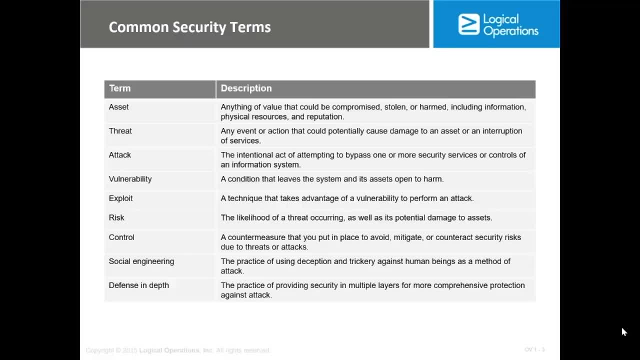 If you need to implement information security management system in any company, you need to explain the management, If anything went wrong, how much they will be losing and accordingly, how much do you need to as a countermeasure. So I can say for my management: OK, if a fire happened, we're going to lose one hundred thousand. 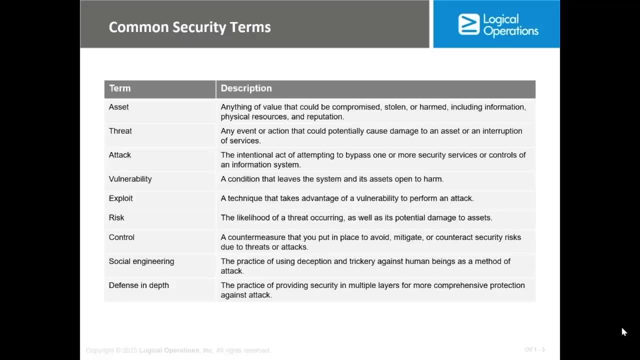 So I need ten thousand to buy some firefighting equipment. It makes sense, Right. But if you go there and you tell them you know we need two hundred thousand to secure against fire, No one will will, will, obey, No one will understand that you need to have figures. 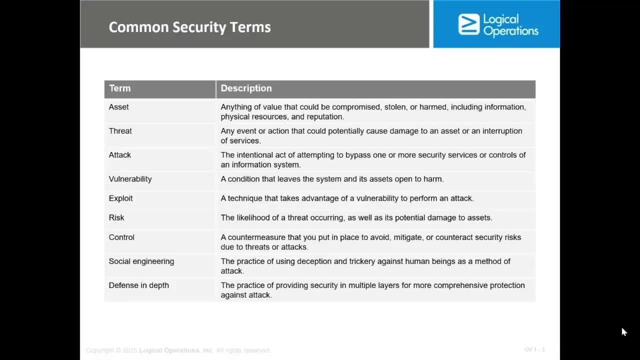 So the risk is the amount of loss That the company will lose in case of any threat occur. We also have a terminology: control, which is the countermeasure If I install an antivirus to mitigate risk. again, we're going to explain all those definitions in the risk management part. 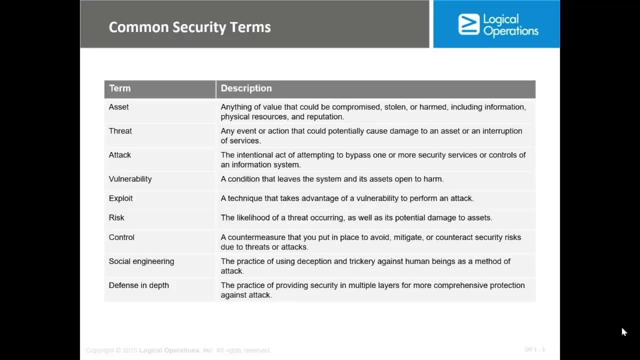 What do we consider that control? I'm putting an antivirus. If I'm assigning a password, it's a control. If we are like getting firefighting equipment, it's a control. So it's a countermeasure that we are using to mitigate the risk or try to reduce the risk. 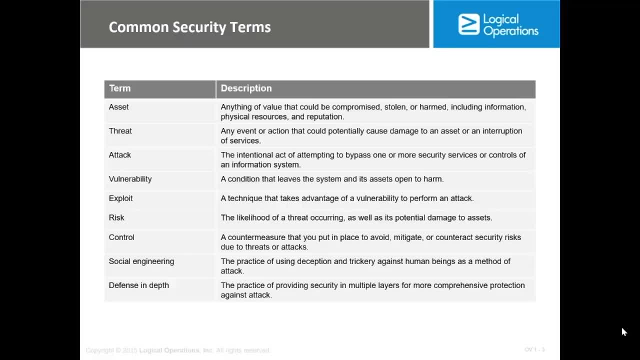 OK, Social engineering is Weakness into human play people, And we're going to explain this part by the end of this domain. So social engineering is a type of attacks that target people, try to compromise a system from, So it's a type of attack. 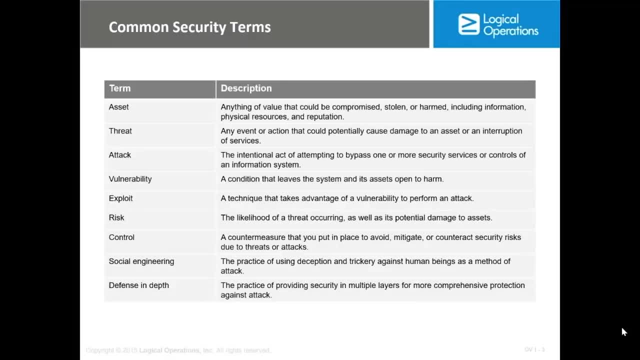 Sometimes you know someone is calling an employee in a company and ask them for, like some information, their credential. It's an attack that Target people. It's not targeting technology or physical security and so on. And finally, defense in depth. 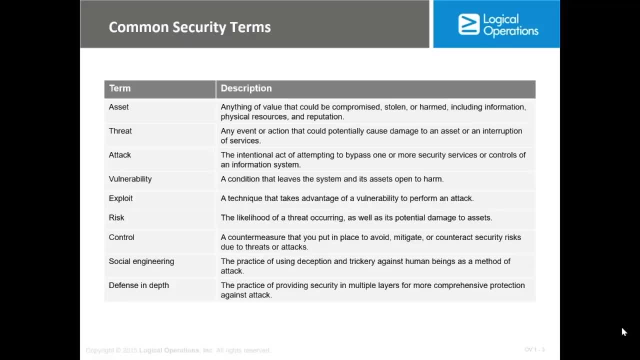 Which reflects that you should have different layer in security. I should not depend on only one layer. So only having a password on my smartphone and consider that security, or having a password on the company laptop, And this is is the best security I can implement. 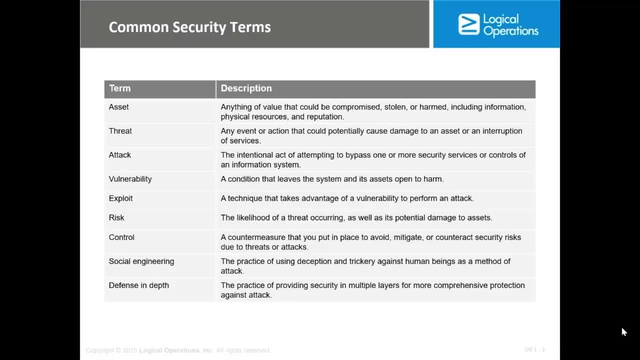 But if I'm have, I have a password on my computer and it's inside a room that has a lock or an access control outside, And I'm also taking backup in case anything crash. So you should have different layers, So if one fail you can use the other one. 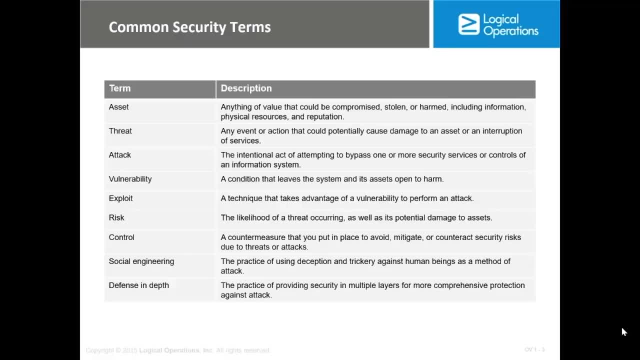 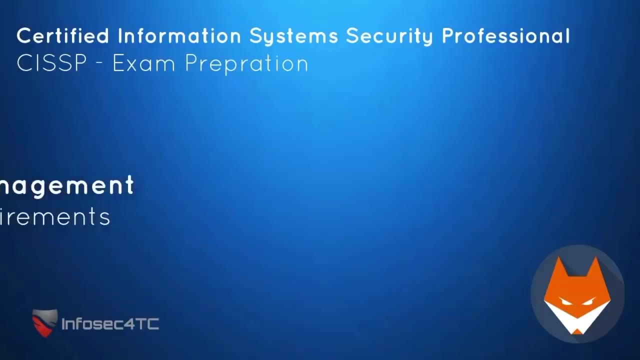 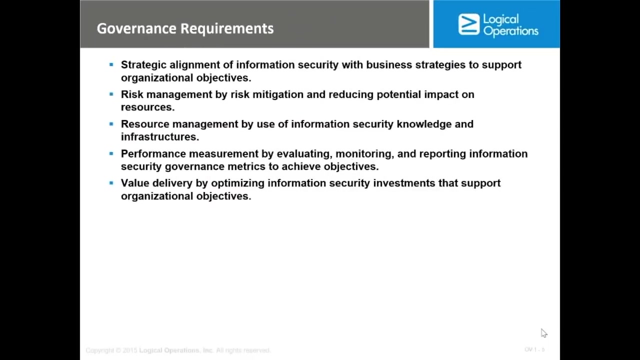 So those are some of the definitions that I need you to be aware of while we are starting our training And to understand The different terminologies that we are going to use. Okay, We still in the introductory part, And let me ask you this question. 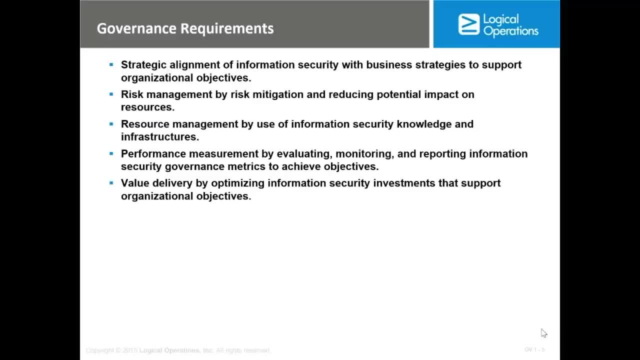 Why are we implementing information security in any organization, Why we are buying equipment and hiring resources and spending money to secure the information in any organization. Yes, I agree that it's because the information is the real asset of any business, But what I'm trying to say, is it an option? 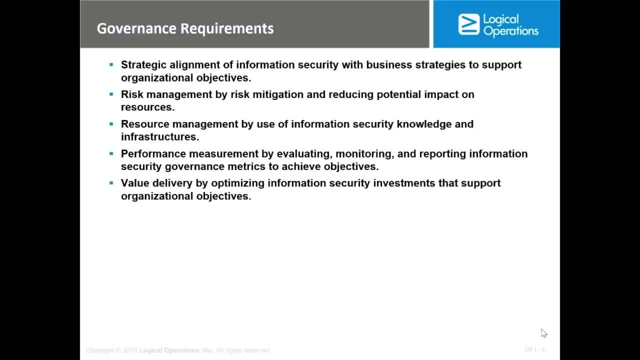 Can any organization today decide not to implement information security and deal with whatever threat? It's not Information security in any business today. It's more as a mandatory, It's not an option And there is a lot of regulation and compliance and governance that enforce the implementation of information security in any business. 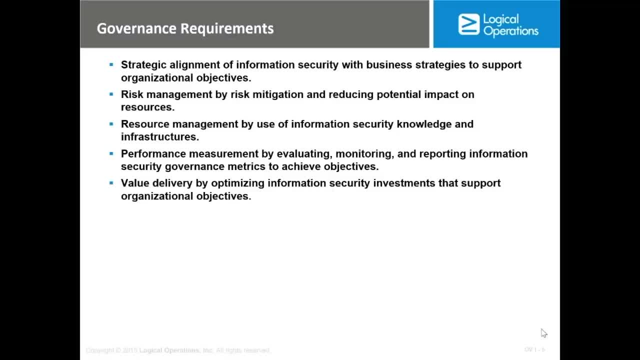 So, for instance, if you are holding credit card information from your customer, you need to follow the PCI DSS which you're going to talk about It's. it's a standard that you need to follow If you are working in. 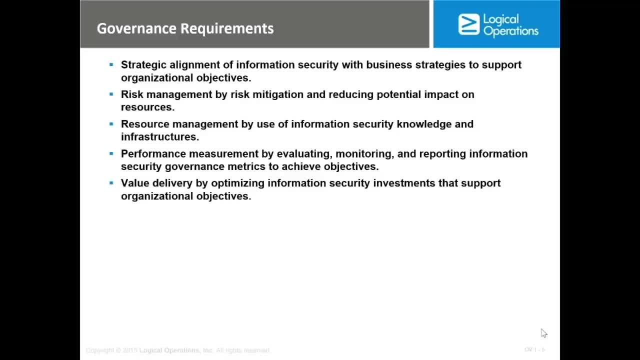 Health industry Or health business, Hospital or a clinic or something like that. You are following HEPA law And so on and so forth. So what I'm trying to say is that the first approach to the implementation of information security it's to understand. 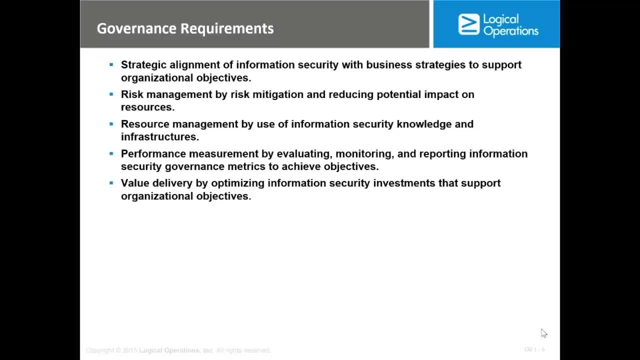 Which standard or which compliance or regulation You are following as a business. And if you get an interview in like a hospital, for instance as an information security officer or whatever the title is, you need to know about the HEPA law. What is needed to be implemented to follow the 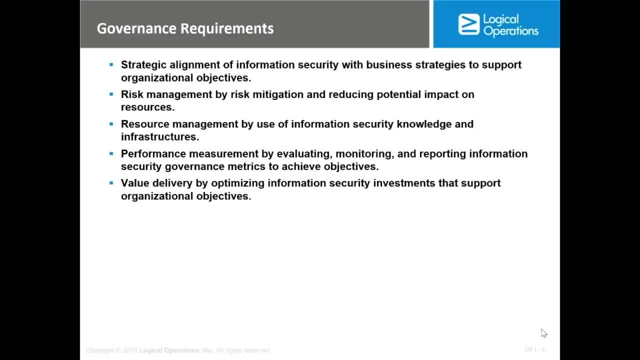 Because it's not an option And if you do not comply with the regulation, there is some legal consequences for that. If you get hired or you have an interview in a bank as an information security specialist, You need to know what rules- I'm sorry- what law and regulation and compliance they are following. 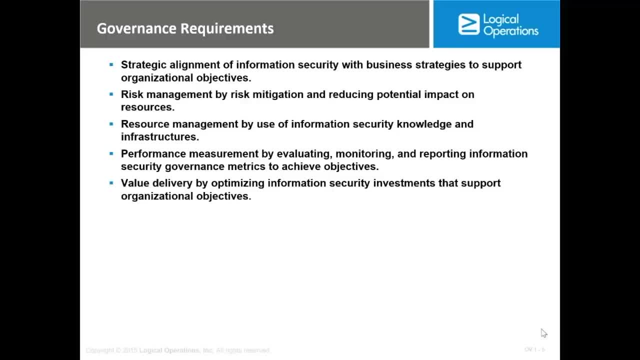 So implementation of information security? it's not an option And this is why there is a lot of like needs for professional information security right now: To implement and to comply with the law. Otherwise there will be a lot of consequences- Legal consequences- for them. 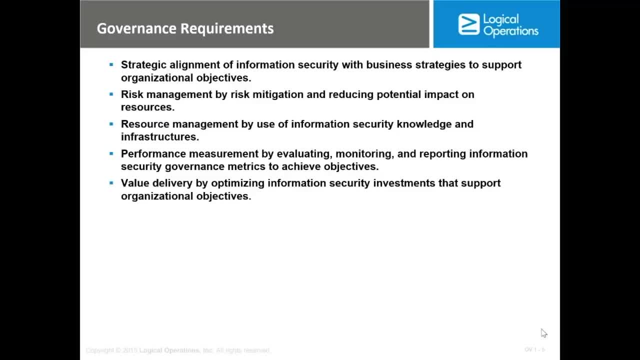 So implementing information security, it's not an option and it should align with the business. It should not be holding the business down And this is also quite important- Some people think about securities- that you go somewhere and you just block everything. You do not allow USB on your computer. 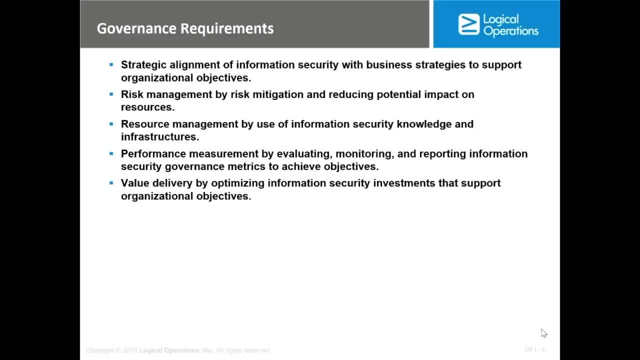 You do not allow people to connect to the Internet, You do not allow people to download anything, You do not allow people to go to the Internet, You do not allow people to go to like different places inside the company, And you know they think this is security, but it's not. 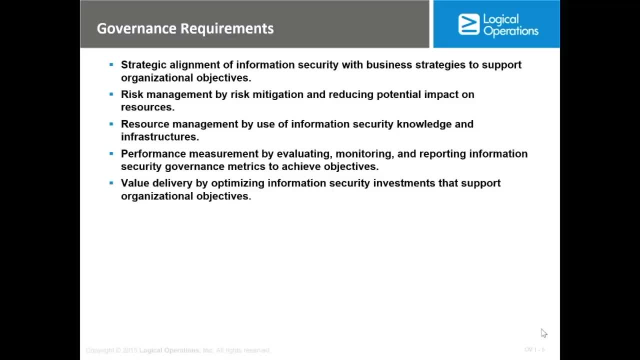 You need to balance between the efficiency of the business and between the security. Besides, as we just spoke, that information security is should be aligning with the business strategy and objective and law and regulation as well. So, for instance, If you are working in a hospital and you fail to implement the requirement for a specific framework, it may end up with a big fine on this organization. 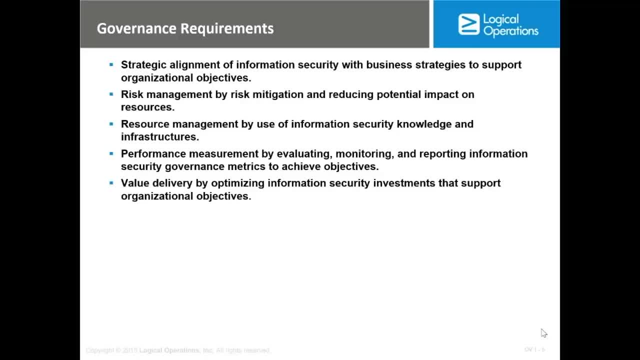 And maybe some jail times for the CEO or for the senior management. So you need to align with that. You need to implement the information security to secure the customer information And, most important, secure all kinds of information, not just the customer information. 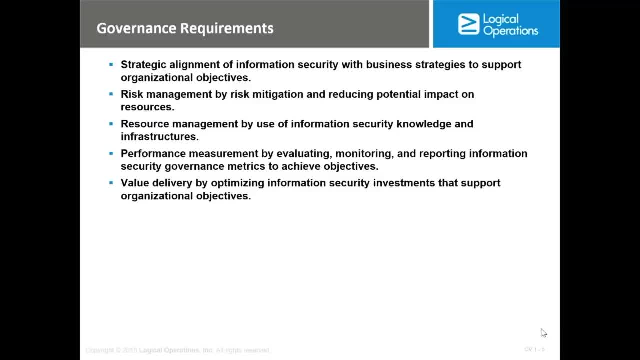 But all the business, information and, most important, to comply with the law as well. So keep that in your mind: That business should align- I'm sorry, Security, information security- should align with the business strategy and it should follow the law and regulation and standard. risk need to be mitigated, which we're going to cover very well in this domain. 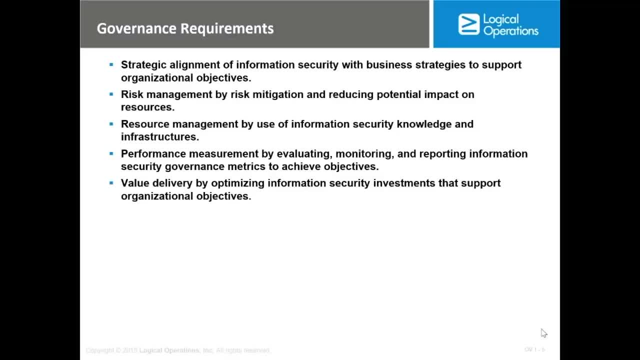 Resource management. You need to measure the performance by evaluating, By evaluating and monitoring and reporting information security governance. So it's not just implementing but you need to know how effective is it, And this will involve things like incident management and log management. 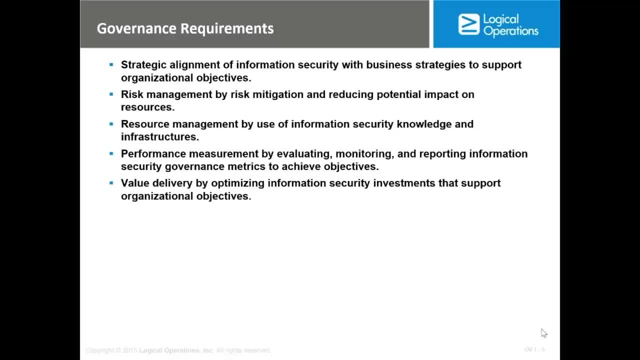 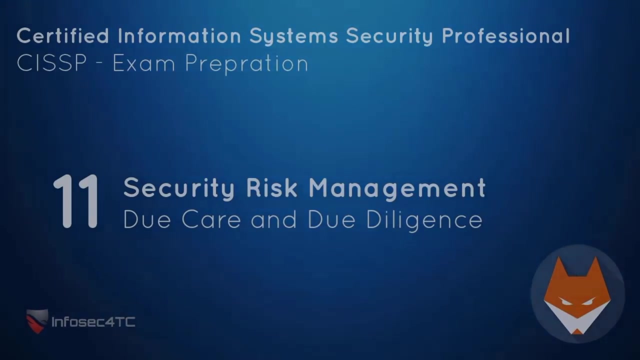 And we will cover those topics, But as an overview about the importance of information security implementation and how important is it to follow the compliance regulation And even certificate like ISO 27000.. In the previous lecture we spoke about the importance of information security implementation. 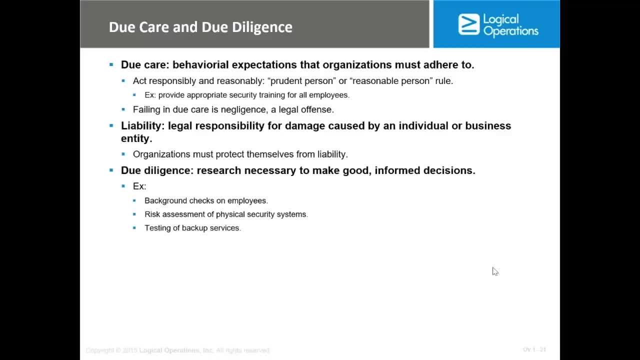 And we clarified that this is a requirement, sometimes legal requirement or compliance requirement or standard requirement, But after all, it's requirement. Now I would like to Focus about two different terminology. is that you should expect a question about them inside the exam, because it's quite important. 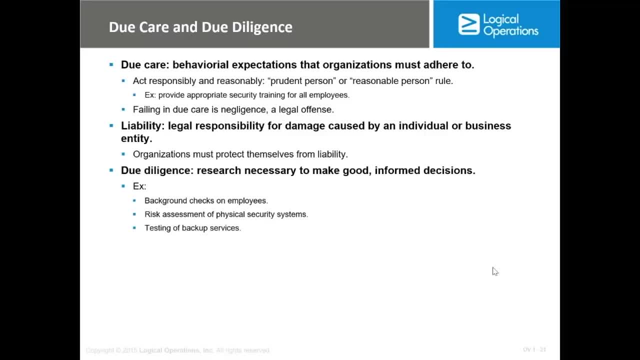 Do diligence and do care. What do we mean by that? Instead of reading the definition, let me give you a small example and let me know what you think about it. Assumes that you get hired in a bank as an information security officer, in a sense that you will be the one who are responsible for securing 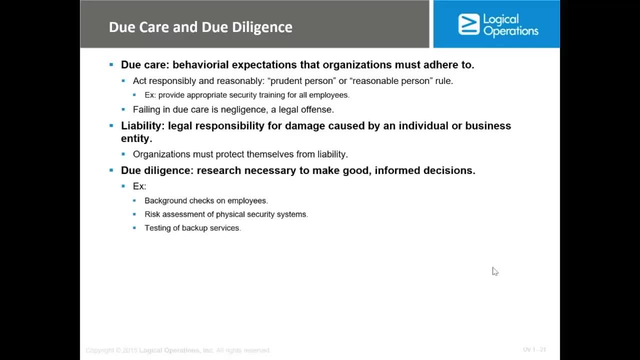 The information of this bank- customer information, transaction information and so on- And assume that this bank has been compromised, has been hacked and some financial information, like credit card customer credit card information, has been stolen. Now, Whose responsibility is that? 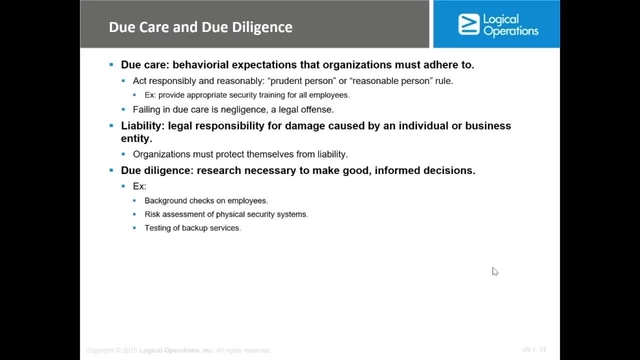 Is it your responsibility? Definitely it's yours, because you were hired to secure this information Right. So it's your responsibility, And it's not just like a regular responsibility is a legal responsibility. So what will happen in this case, if the bank get hacked and some information gets stolen or lost? 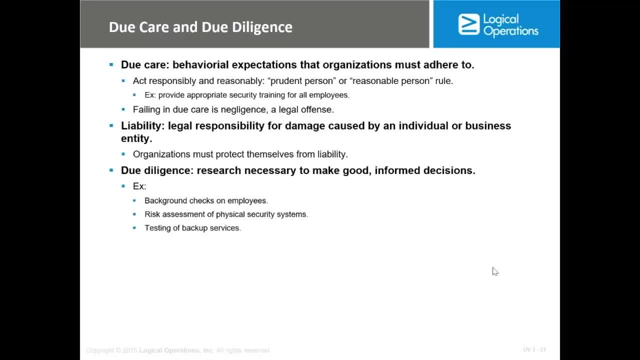 Most probably, you will be taken to the court. Now, when you go to the court, They will ask you two different questions. The first question will be: Are you aware of those vulnerability and those weakness in yourself? You were aware that there is a lot of weakness inside your system, technical and physical, and so on. 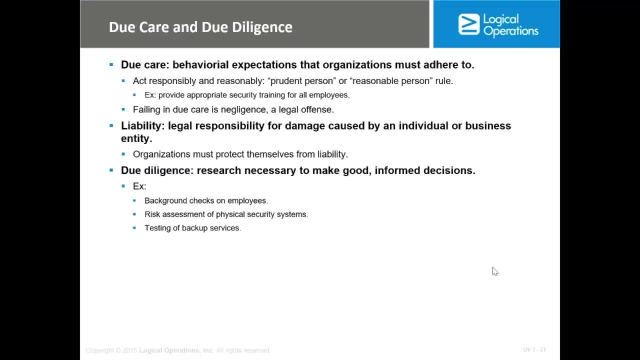 OK. so if your answer was yes, I was aware because I used to do a risk assessment. I used to do vulnerability assessment, penetration testing, So I used to check the weakness in our system and I was aware that there was weakness that may lead to compromisation. 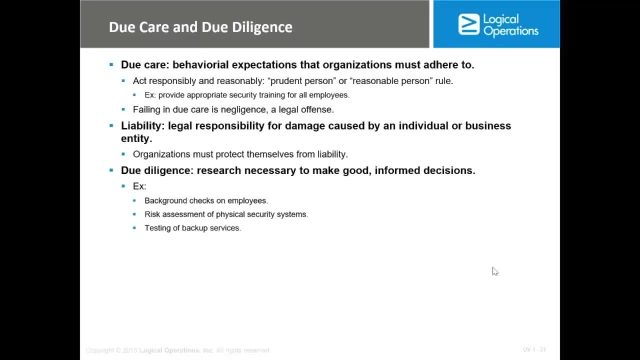 This is called due diligence- That you did your research, You were aware about your setting, your infrastructure, your equipment, your software, And what is their weakness. The second question from the court would be: What did you do to secure those weakness? 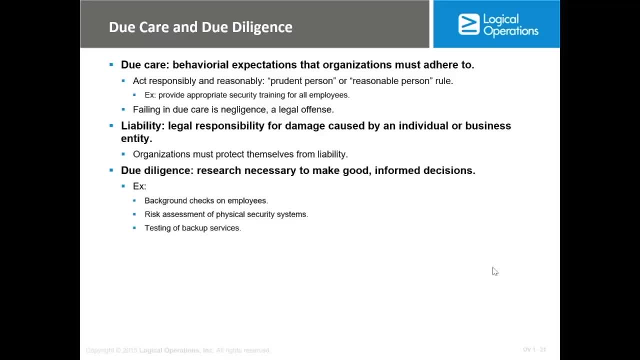 Did you follow the standard, Did you request, like some additional resources, Did you update the software And so on and so forth. So this is called due care That you were following the standard, the best practice, the compliance to mitigate those risks. 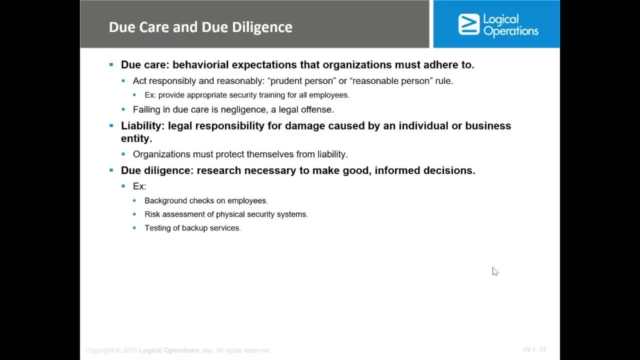 To fix those vulnerability. This is called due care. So what if you answer Yes, I requested some equipment, I requested some resources to the management Because I knew that those vulnerability was risky, But management said we don't have the budget this year. 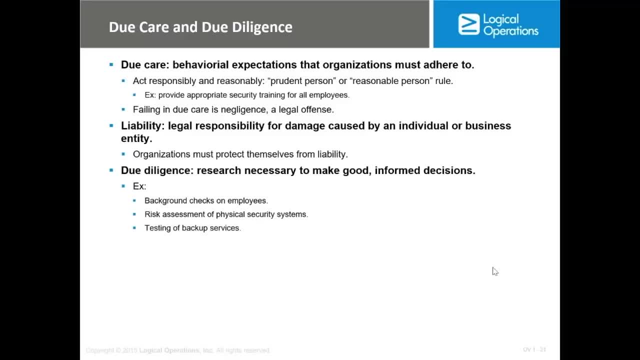 Now whose responsibility it became? right now It became management responsibility. So the point here- the due diligence and due care concept said: When you get hired somewhere, You need first to be aware of the weakness and vulnerabilities that they have, And we can do that usually by checking the 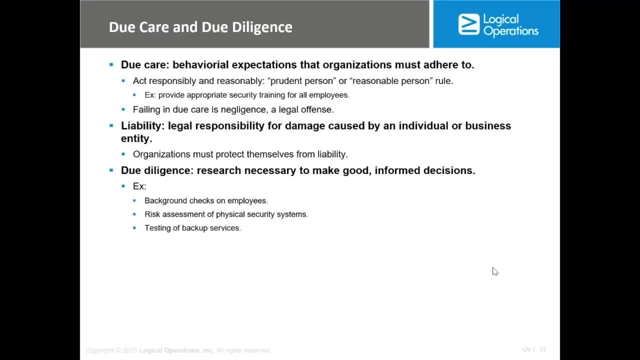 Or doing a vulnerability assessment, Doing a risk assessment, Which you're going to do in this domain- Doing a penetration testing, Following the standards. There is some standards that we're going to talk about in a few lectures That you can follow just to be sure of the awareness. 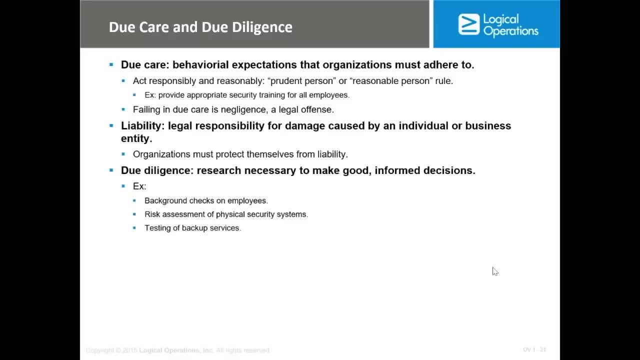 And I'm sorry to be sure of the weakness and vulnerability, But this is not enough. You need also to take action to secure them. This is called the due care, And liability here means who's responsible For securing, For securing the business information. 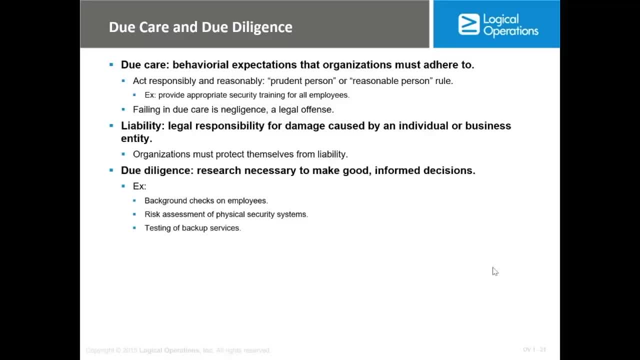 And securing the business assets, Because the role and responsibility should be quite important. If you have a policy and procedures in your organization And all your employees are aware of that And they break this policy, It becomes their legal responsibility. But if you don't have a policy and procedures, 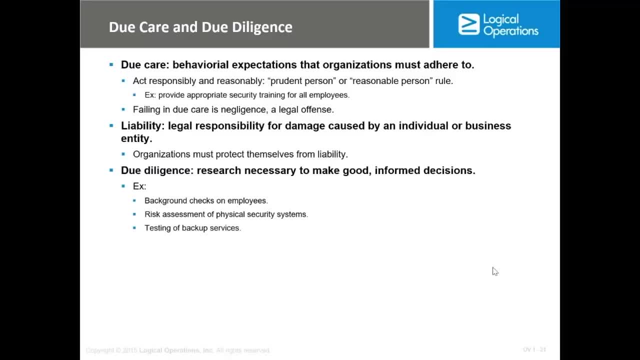 And some employee did something wrong, He do not hold any responsibility. It's your responsibility That you didn't have a policy, That you didn't have a policy and procedures. And even if you have And the employee is not aware of. 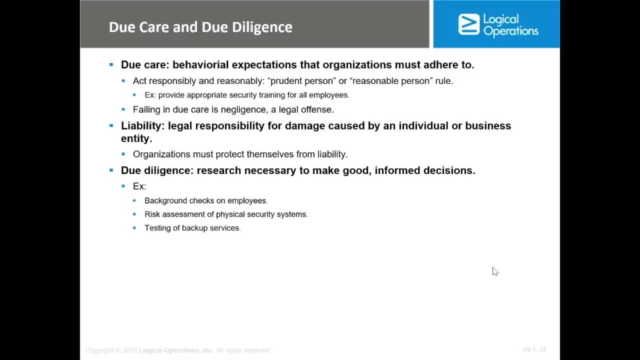 It's useless. That's why we need to do awareness for people, Telling them this is according to the company policy, It's not right Or it's not, It should not be done, And after that They can take responsibility from their action. 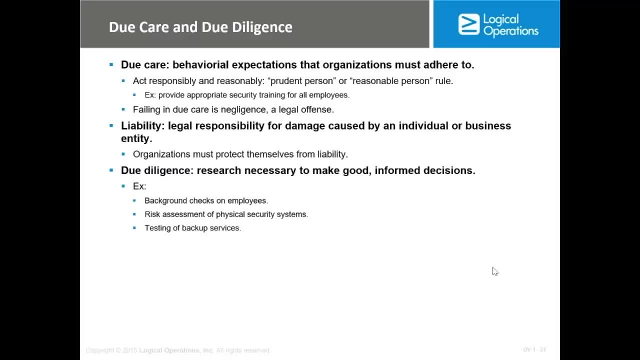 And a small example For the liability part. Assume that you have a password policy And we're going to talk about the policy And the major policy in your company Saying that policy should not be shared. If you have a password, You have a password policy. 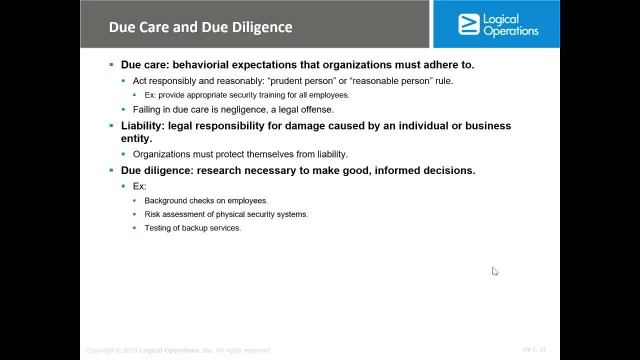 And the password policy is saying That password should not be shared. So each employee knows that If he has a password to his account, He should not share it with his colleague. His colleague, Okay, And maybe this makes sense. But realistically, 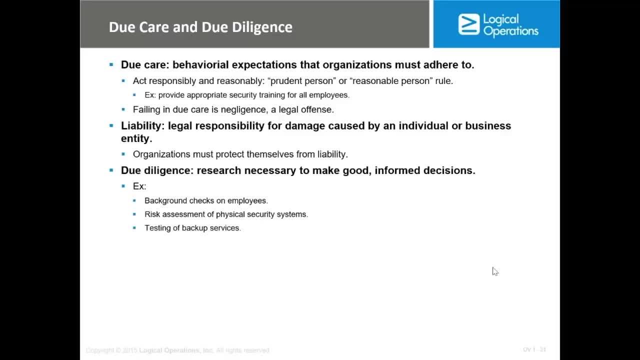 What I saw in many companies, That sometimes someone take a day off So he will give a policy to his colleague So he can follow up with the task, Daily tasks that we need to do. Okay, If there is a policy saying that. 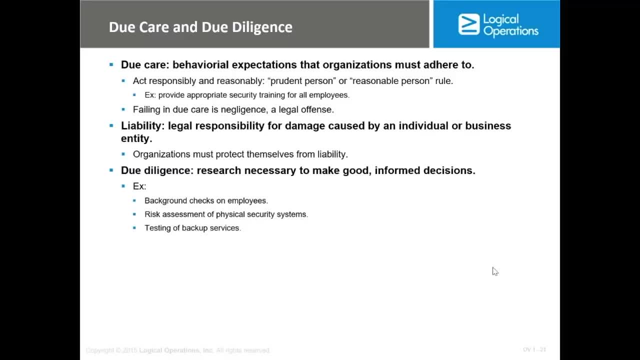 And you find out that one of the employee Gave a password to his colleague And, for some reason, the password get lost, Or someone logged in with this password And did something wrong. Okay, He will take responsibility for that, Because he knew that there is a policy in the company. 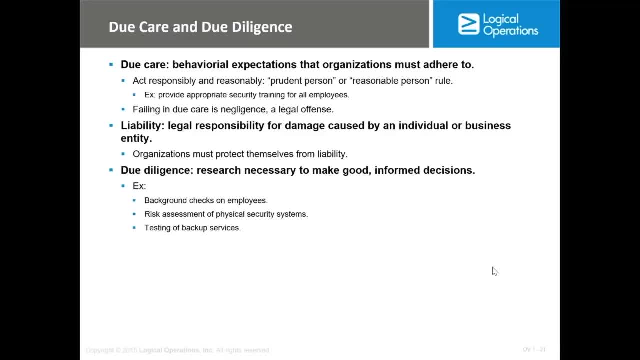 And you as an information security specialist Or officer, You did some awareness about the major policy In your organization, So he will take responsibility for that. But if you don't have such policy And the same scenario happen, What you can do about it? 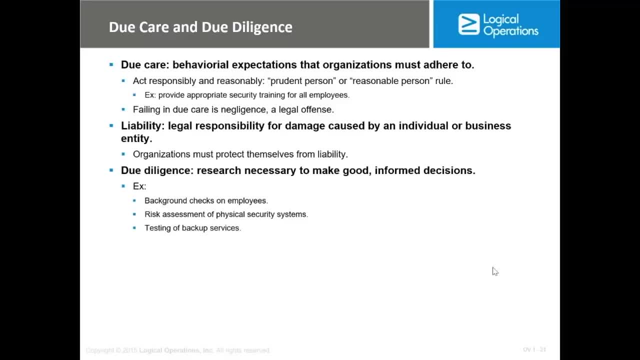 You will take the responsibility for not having a policy. So those terminology And due diligence And due care And liability Is quite important Because, after all, You will be involved in some legal requirement, So you need to be aware of that. 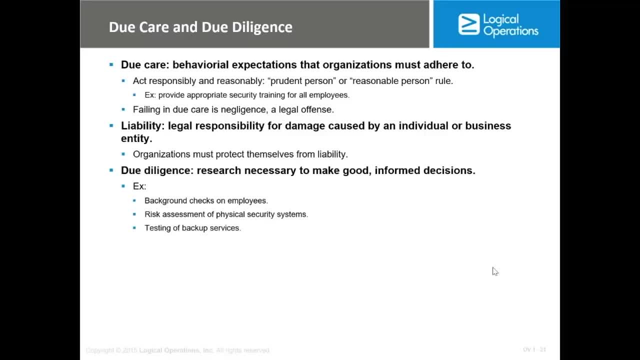 You need to be aware of the legal requirement for any system. Let me end up this lecture with another example. If your company or your bank Most probably has a surveillance cam Where you are capturing video And or recording video And keep them for a while in your organization, 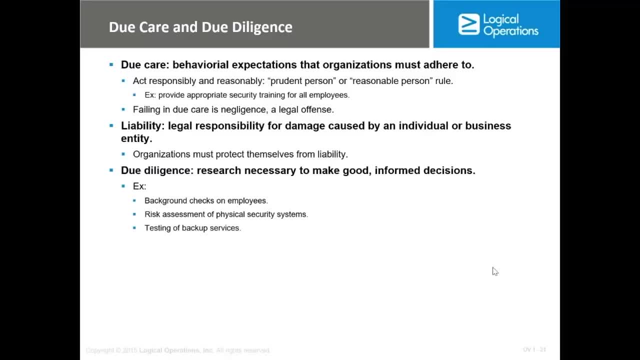 How long it should be kept, Those surveillance cam, Because it's one of your responsibility. How long it should be kept? Should it be kept one month? Should it be kept two months? What do you think? Okay, Whatever number you're going to answer with, 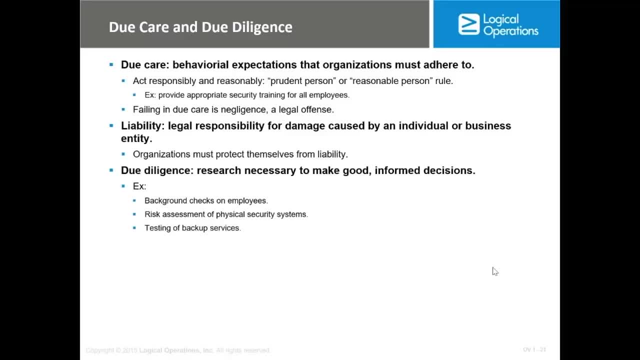 Is wrong Because you need to know, According to the law and regulation to your country, How long it should be kept. So I'm working in some places Where they have to keep all the logs, Or let's say the recordings, Surveillance recording- for 90 days. 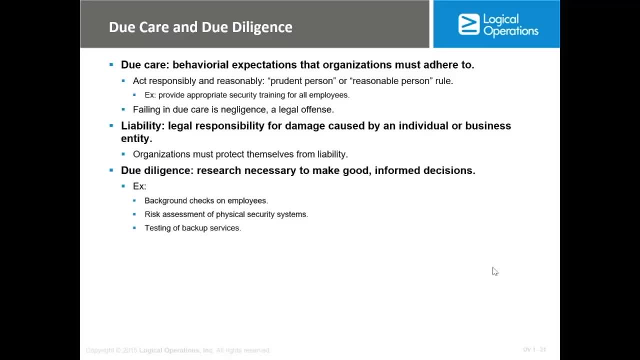 If you, as an information security officer, Are not aware of that And you decided to capture them for only 30 days To save storage on your servers And some incident happened, Like someone breaking or any incident happened, And law enforcement came to you. 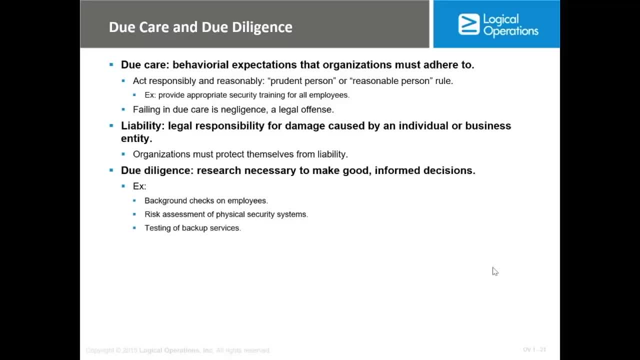 And told you show me the video recording From two months, And you said: I don't have that, I only keep them for one month. This is a big problem for you. Okay, A legal problem, It's not that. So you need to be aware of the legal requirements. 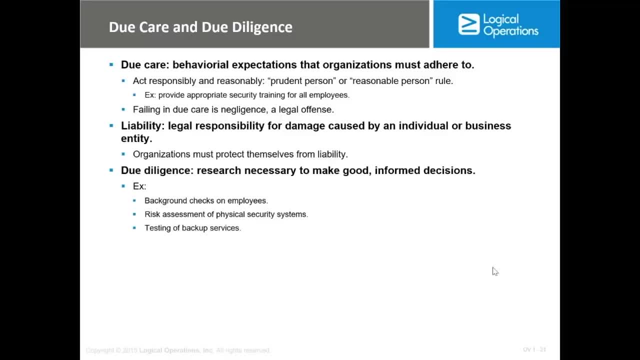 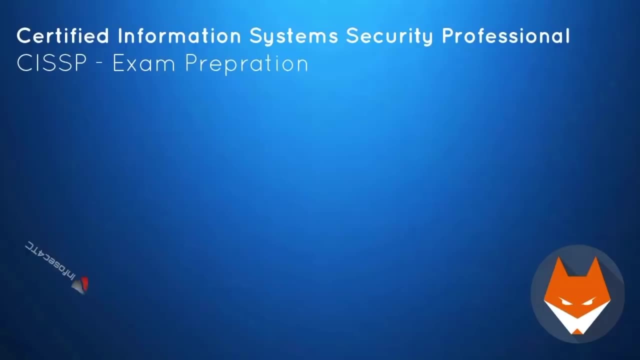 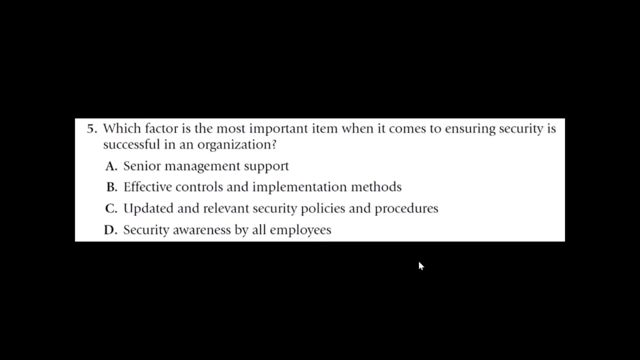 The compliance, The standards, The liability, Because you don't want to get into legal problem In your position. Information security positions are getting paid very well, But they also have a big legal responsibility. You need to be aware of that. I know we didn't cover that much yet. 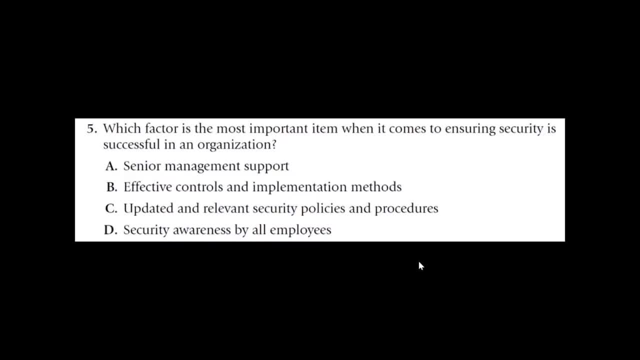 But let's take a question related to the introductory part, Just to give you an idea, Or to relate the topic or the points that we covered so far With real exam questions. So the question is: Which factor is the most important Item? 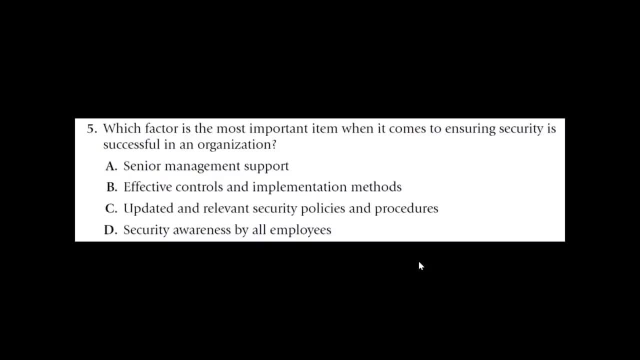 When it comes to ensuring security successful in an organization, Is it senior management support, Is it effective control and implementation methods, And is it updated and relevant security policy and procedures? Is it security awareness by employees? Actually, all of them are important to implement security in any organization. 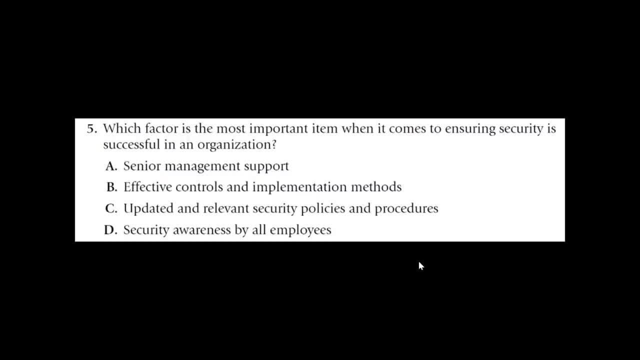 But which one is the most important? Now think about it. If you get hired somewhere to work as an information security professional Officer or specialist or consulting, Whatever the title is- And you need to implement information security And, as we agreed, 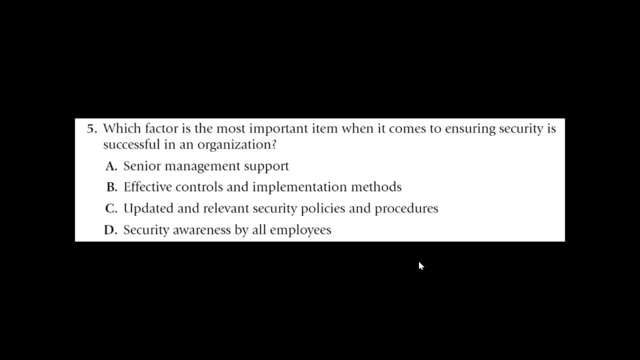 Information security is not just technical security. It's to implement technical security, To implement physical security, To implement administrative security, To implement administrative security, To implement Administrative security and so on and so forth. Right To be able to do that. 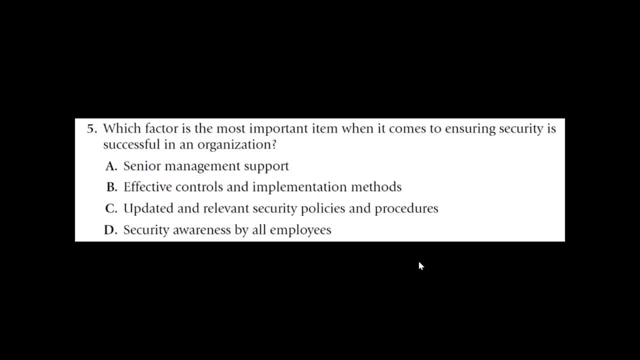 You need to People. You need the employee of this company to support you in a way or another, Giving you the requested information, Explain to you their business function To be able to decide about what controls they need to have, and so on. 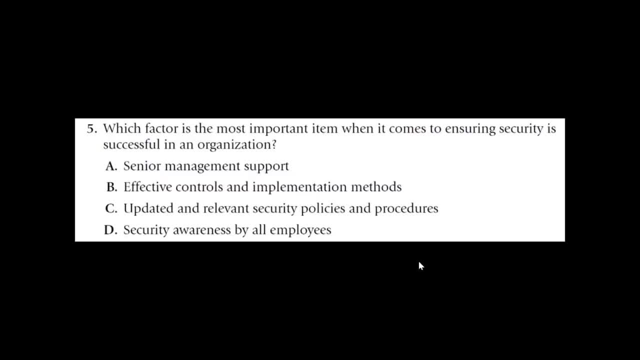 If you do not have management support for that, No one will cooperate with you. But if you have a senior management support at the beginning, In a sense, that management sent an email for all the people in this company- Or, I'm sorry, All the employees in this company, telling them. 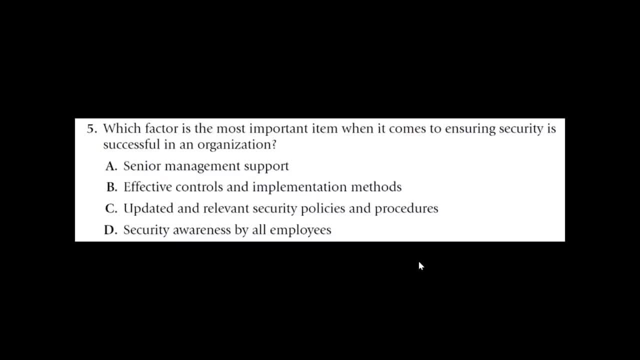 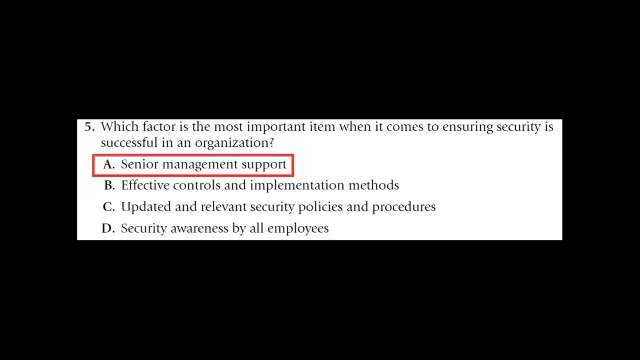 That we are implementing an information security management system And you need to cooperate with this specific person, Otherwise no one will give you support. So the right answer for that Will be senior management. So it should start If you get hired at any organization. 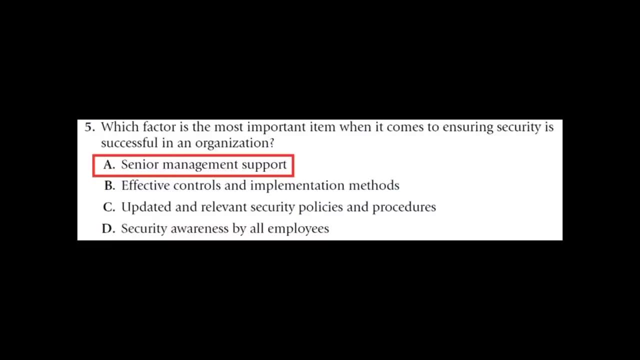 It should start that you need to sit with management and tell them That you need to have management support, Otherwise you will not be able to implement anything. No one will cooperate with you, Not because they want to do it this way, But unless they have. 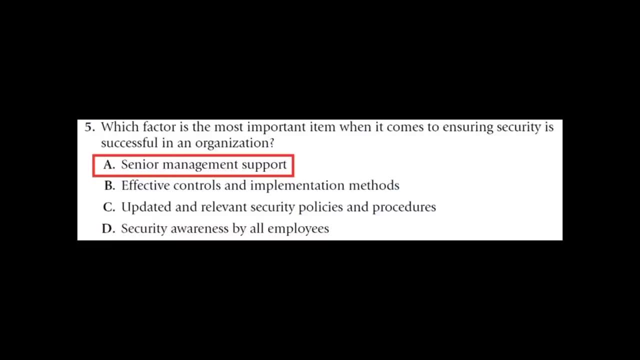 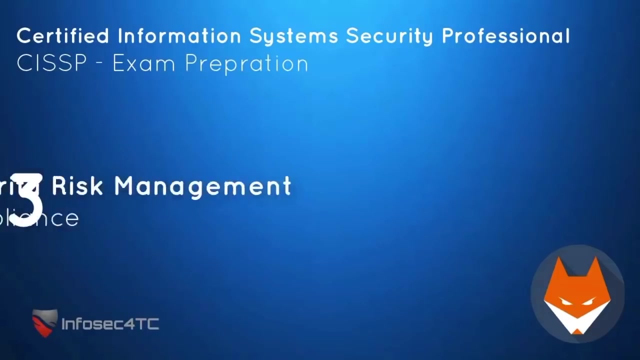 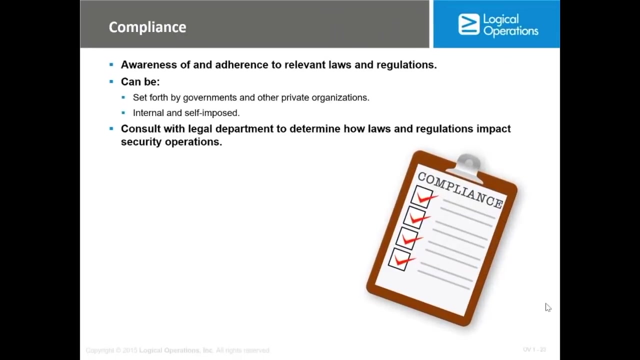 A management requirement Or it's. I'm sorry. Unless it's a management requirement, You know they will not consider that as a high priority. So it's a very important point That security without management support is useless. In previous lectures We spoke about the concept and definitions. 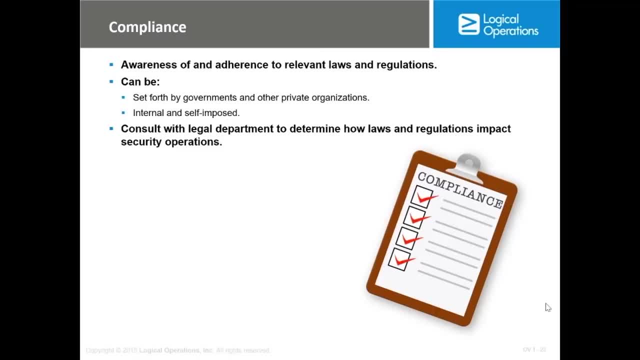 Related to information security. So from where should I start? If you get hired somewhere Or you got this question in any interview- How to start the information security implementation? Should I start requesting hardware and software And requesting a document and requesting? Should I start working right away? 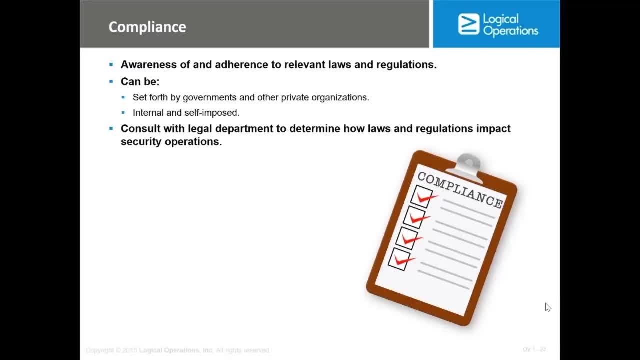 If I get hired in a bank or In any organization, I should start by checking the compliance Because, as we agreed That the implementation of information security, today It's a legal requirement, So I need to know What compliance do I follow? 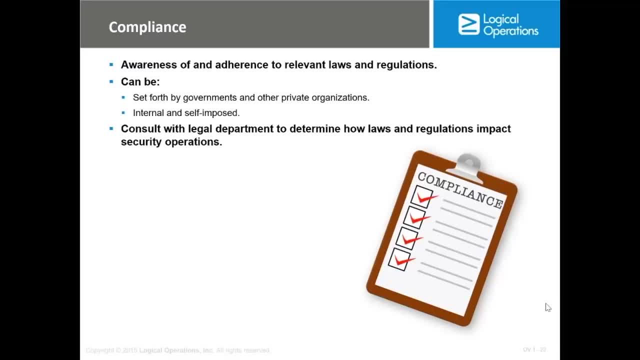 If you are a bank, You are following specific laws and regulations, While if you are a hospital or clinic, You are following Other laws and regulations, While if you are a small grocery store, There is other law and regulation as well. So you need to understand. 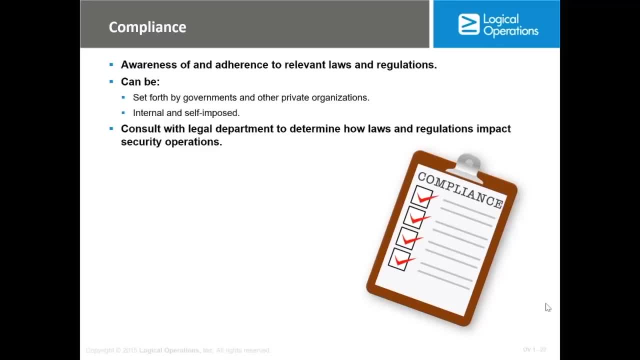 What is the legal requirement When it comes to information security? So it's not by buying the latest and greatest equipment And hire the most sophisticated Expert in the field. It's not like that. You need to understand what is needed According to the law and regulation. 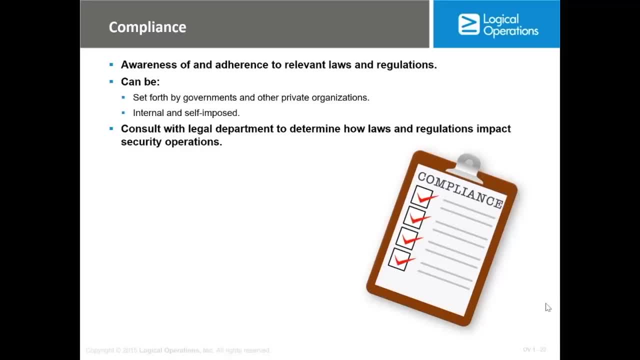 And this is the compliance. So this is from where you should start, And you will find a lot of like similarity Between different compliance, So most of them will request you to do a risk assessment, For instance. You need to identify the risks that you are facing. 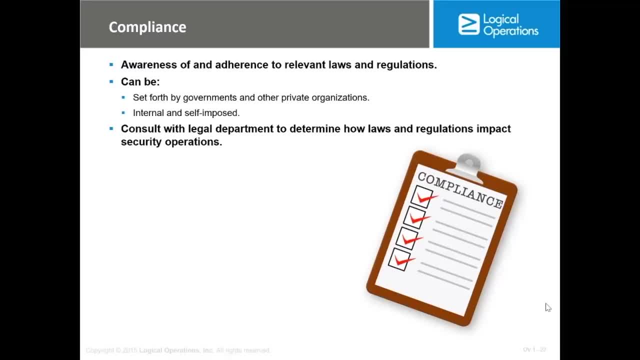 To be able to select Or to be able to get the right counter measure for that. Most of them will request to have, like, A annual penetration testing And vulnerability assessment And so on and so forth. So it's not that hard. 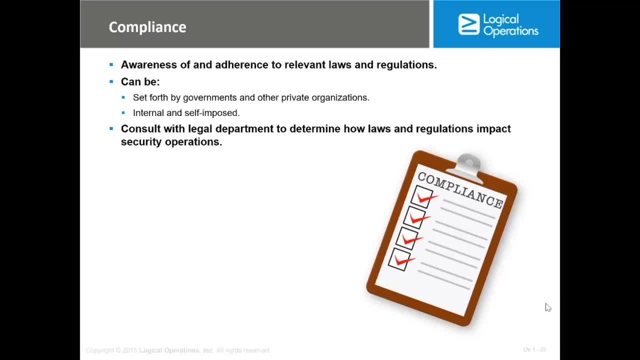 But the thing is, You need to start from there, Because you're going to build your policy and procedures And whatever is coming According to that, And I believe I already gave you an example In a previous lecture, For instance, The surveillance cam. 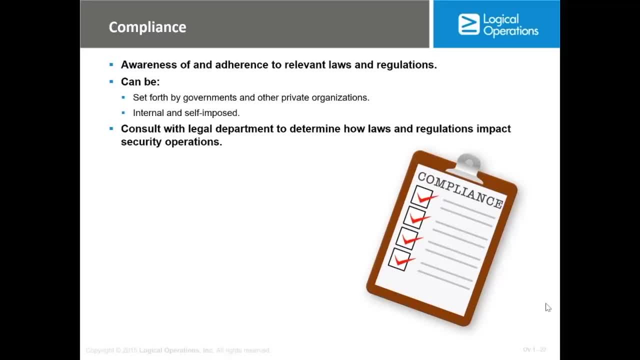 The surveillance video recording. How long should you keep it? Okay, This is critical Because, if you are not aware, This will not Be like an excuse That I didn't know that I should keep it for 30.. For 30 days. 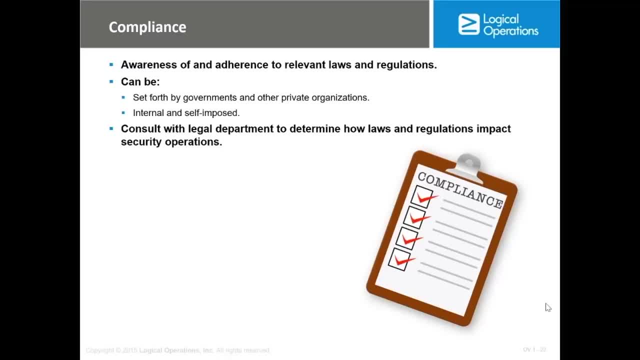 Or for 90 days Or so on. It would be a legal problem. We don't have something called. I didn't knew about that. You need to read the compliance. You need to sit with the legal department And ask them. 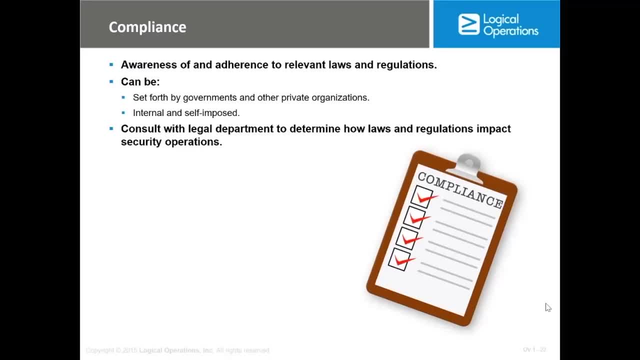 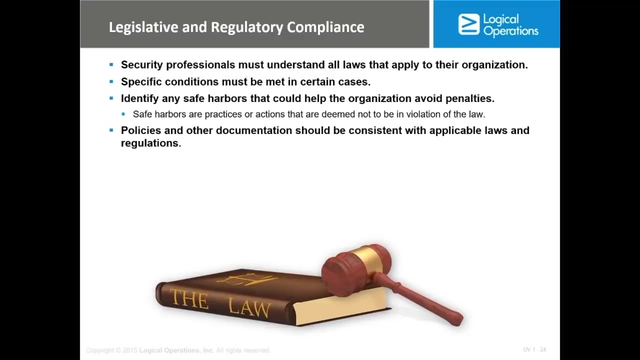 Which compliance and regulation And law we are following. So you should start from this point, Because there is some critical point That you cannot ignore. So compliance is quite important In our business And, as I was saying, You should start by sitting with the legal department. 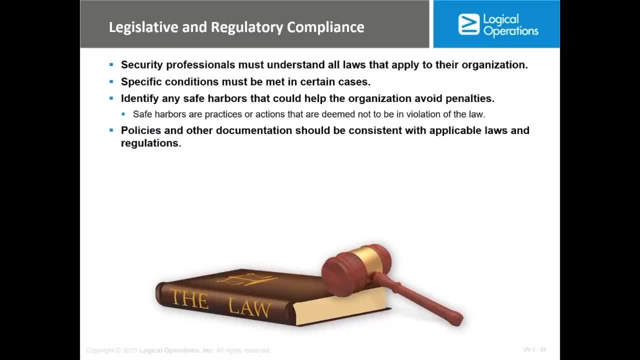 And ask them: What is the regulation and compliance That we are following? And you need to understand those law very well And consider them In your information security implementation. Identify The safe Harbors That could help the organization. 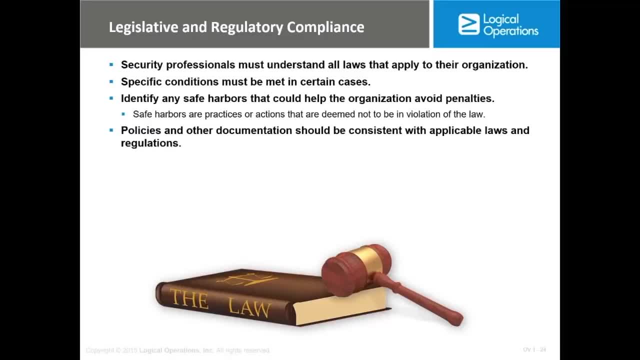 Avoid penalties. You didn't know that you need to keep those Recording Video recording for 90 days. You will hold some legal Consequences And the organization It may end up with fines. It may end up with some jail times. 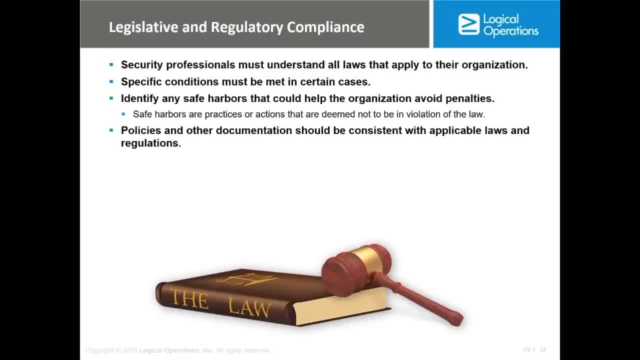 In some law and regulation. So it's not easy, It's critical. So, for instance, If you are following HEPA law, Which is a regulation, And it's a compliance for holding The patient information In any health business, So you are working in a hospital. 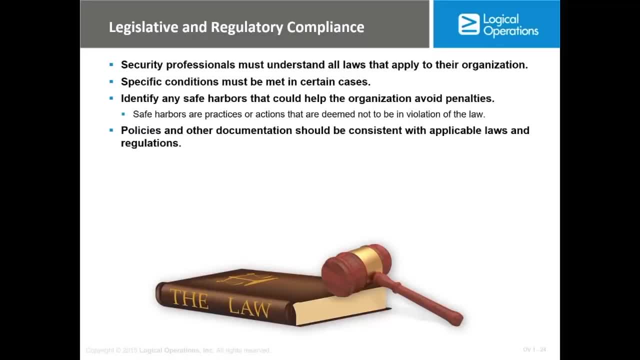 And you didn't implement the right control To secure the patient information And for some reason, It get leaked or compromised Or even lost. I think it's a very big fine On the hospital. I think it's 200 million. 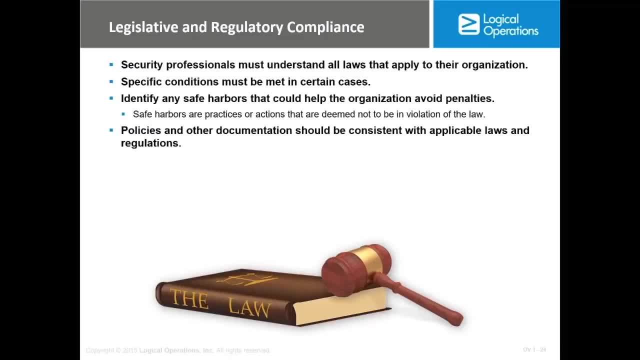 Or something like that. So it's not an easy Punishment, It's a hard one. So it's very important To start from this point And I suggest As A An assignment That you can do, Because I don't want you. 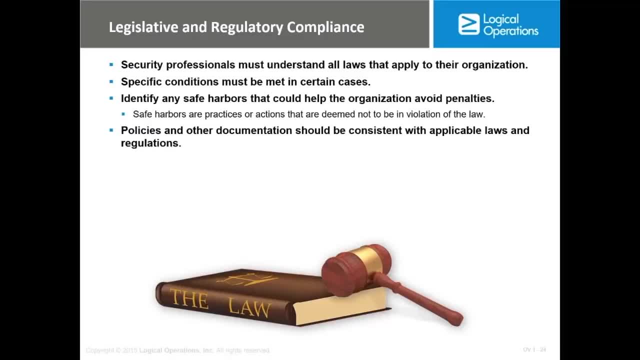 Just to depend on those videos And the resources And the books That I will provide you. But I need you to do Some research Yourself Because I don't want you Just to depend on those videos And the resources. 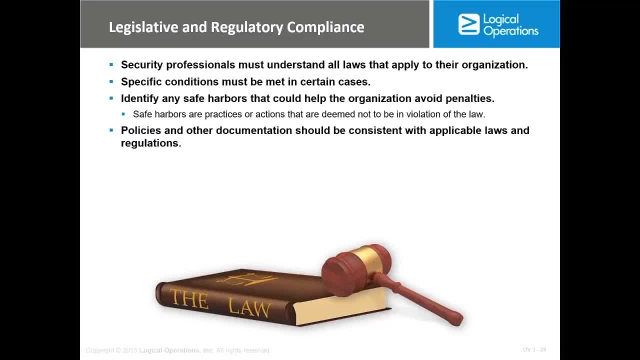 And the books That I will provide you. But this is not an easy exam And I need you to do Some research Yourself. So I want you To check, for instance, Some information About HEPA law Or some information. 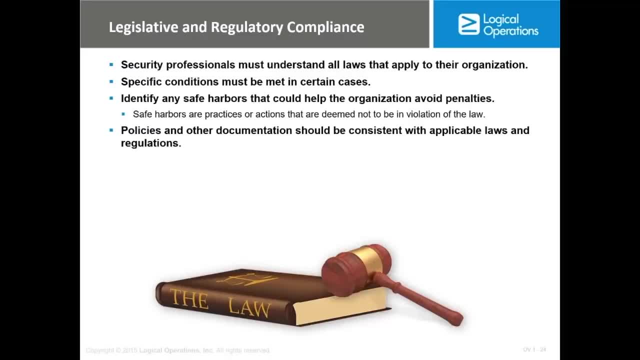 About some standard Regarding, For instance, Holding a credit card Information. If you are Taking credit card Information, You are Accepting payment By credit card And you are securing I saving them. Do you have some Standards? 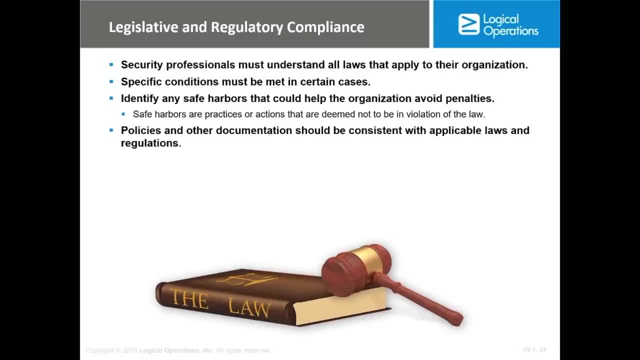 That you can follow. Do you have Some that you can follow? expect that this is like an interview- questions and let me know, is there any standard related to credit, to holding credit card information? I will keep that as an assignment and feel free to drop me an. 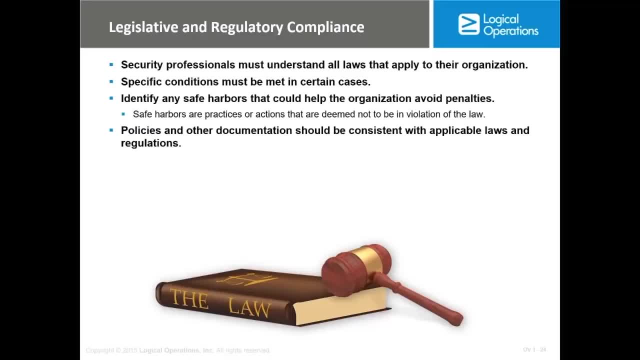 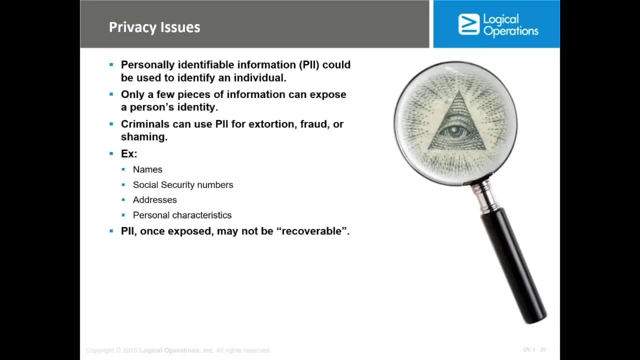 email with your answer and I will let you know what I think about it. another point that I would like to raise here- and this has become very, very common right now- which is a privacy issue: okay, the personal information that you are keeping in your organization, do you have any like right using them? and I believe 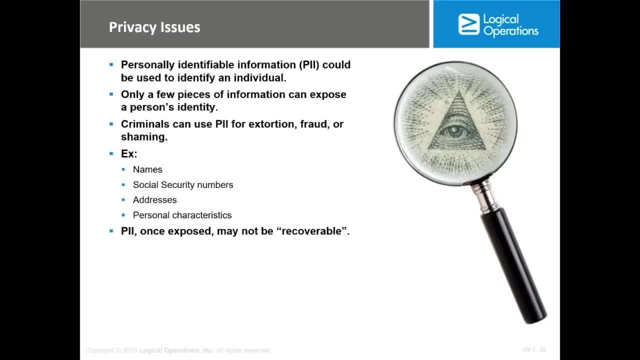 you know, those day you are following this Facebook case and this sessions that happen in Congress regarding the leakage of some personal information. this is an exact privacy issues that we are talking about and people who are working in security in Facebook if they find out that they didn't kept those personal information safe and they didn't because they say. 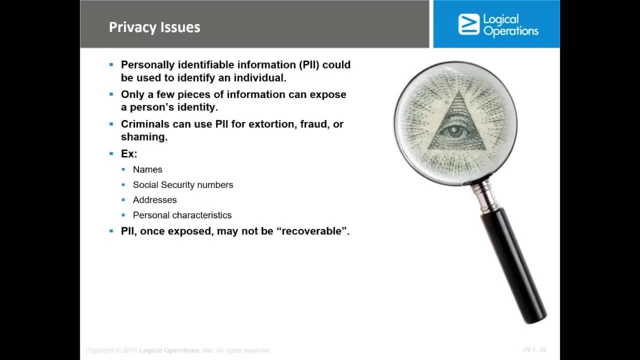 the point here is that they were selling those information to other vendors. so did they take permission from the owner of those information that they will give it to vendors or other business and so on? so here we have a very important terminology is called personally identifiable information, or PII. you will 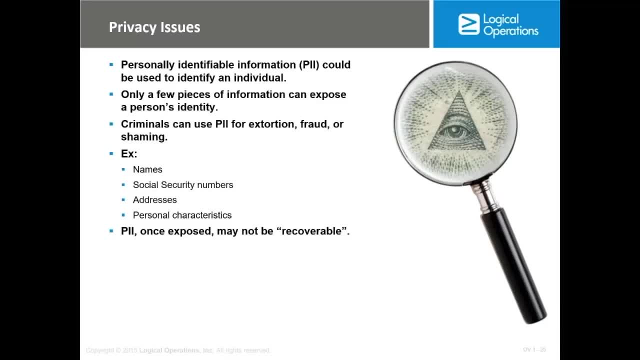 find this terminology in different places. okay, which is: what are you doing with the personal information? who are getting access to this information? do you have the right to exchange your personal information with someone else who is not those information, or sell this information to other marketing entity, or something like that? 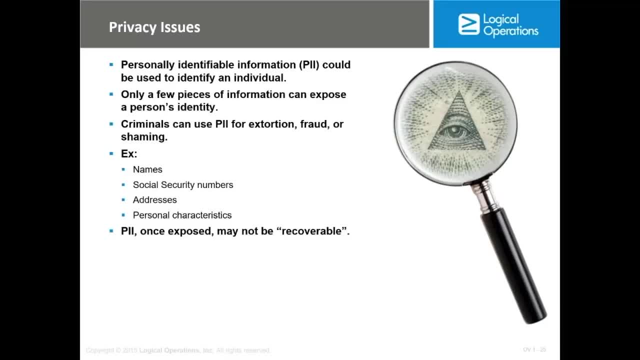 this is quite important. so holding personal information is a big responsibility and you need to make sure that you are following whatever law and regulation regarding personal information. personal information could be something like your name, social security number, your address, your phone number, your email- all those is considered personal information. 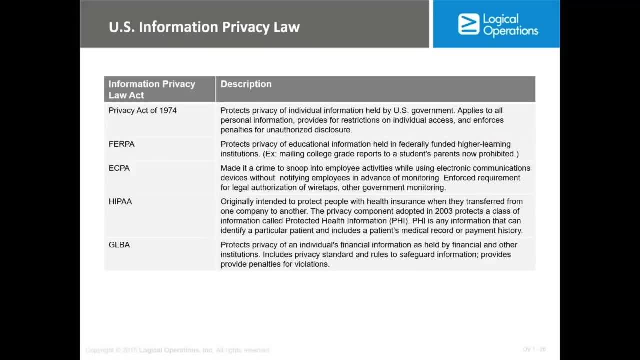 finally, i would like just to refer to some us information privacy law. i want you to have a look about them. you know some information are related to privacy. we are not actually. it's not a legal course, you just need to have an idea about it. most probably you may get one question inside. 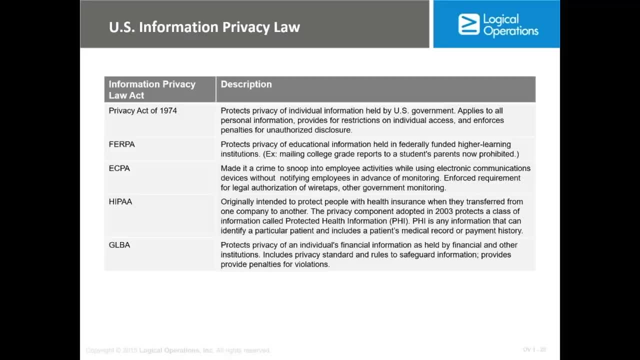 this exam about that or or not, because, as you may know, those laws are only applicable in us and we have a lot of international students. so in the exam itself you don't find that much of question related to a specific us law, because most of the information law are related in europe and us. but still, getting a brief about 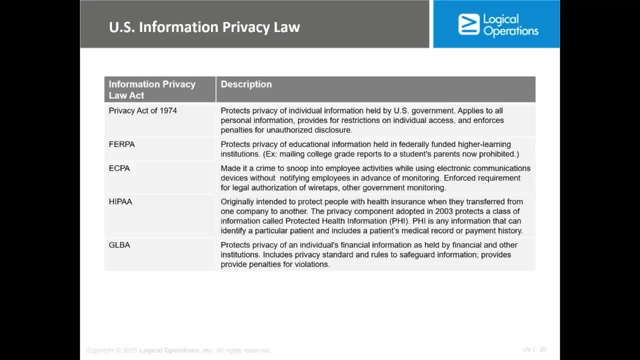 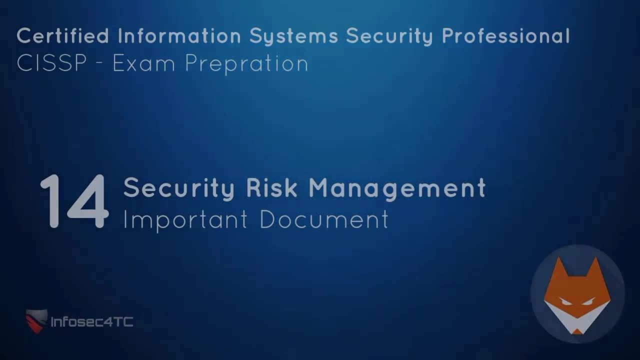 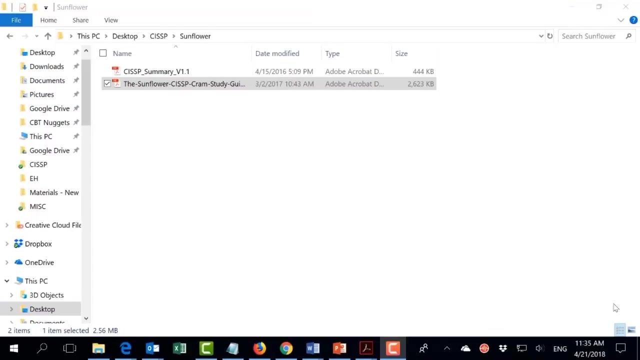 the law with the name of it will not hurt you. at least you will know that there is a law related to health, industrial, or there is a law related to privacy, and so on and so forth. so, before resuming in our domain, i would like to refer to a very important document that you need. 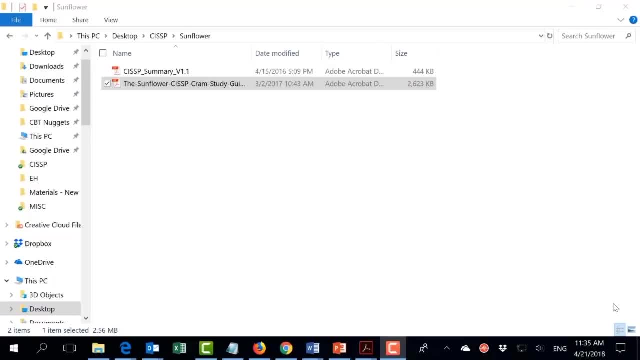 to have while preparing for your exam, which is the sunflower document. when you enrolled in this course at the beginning, you received a lot of material and resources- books and pdfs and presentation and so on- which goes through the different topic and terminology and explaining everything related to the curriculum. but there is a document that you need to have. 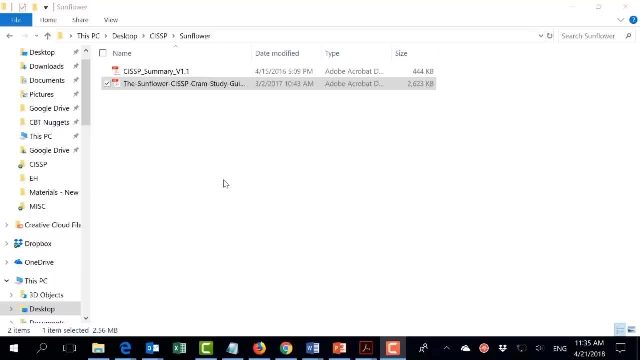 which summarize everything inside the cissp, which is the cissp sunflower document, the sunflower document. it's a document that summarize all the definition inside this course and even point to some of the important point and like tricks inside the exam. so i would like to refer you to the summarization document when you finish the course and actually 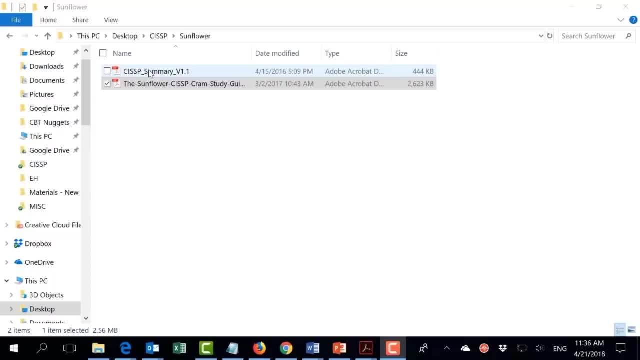 while you are studying the course. whenever you finish one domain or another, you need to go through the related terminology in the cissp document, and there is two different version: the first version with 1.1 under the name of the cissp summary, and the second version with the. 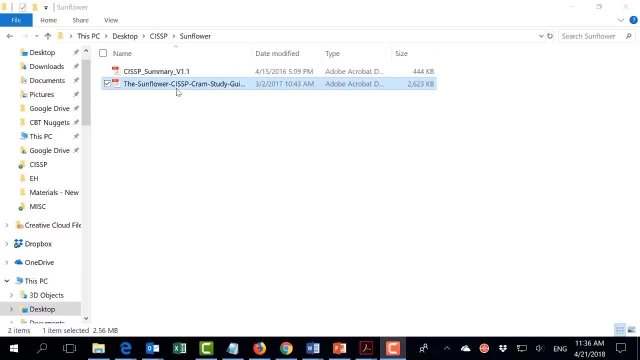 version two under the name of the sunflower cissp. so let me show you how the document look like and then let me give you my recommendation about which one you need to study. so the document consists of 25 page and it's divided by domain. 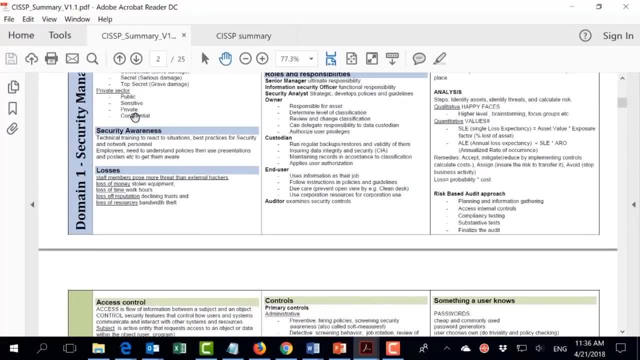 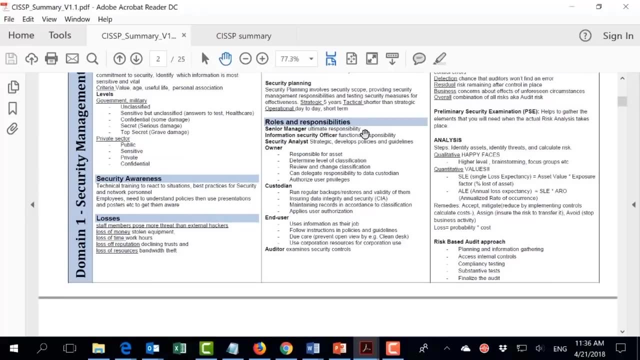 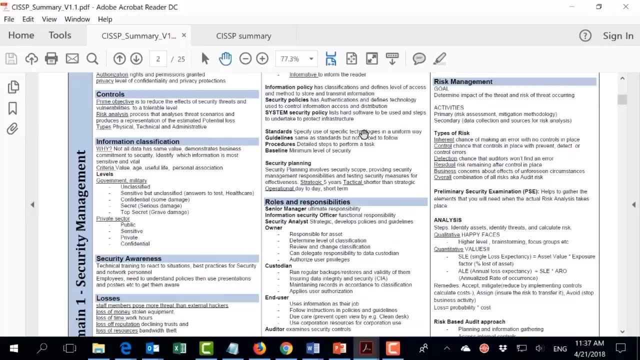 as you can see, we have domain one in different color, where all the concept and definition about domain one is explained here, and even sometimes you will find that they are pointing to some important terminology by putting them underline or in capital letter or something like that. so you know domain two, domain three: 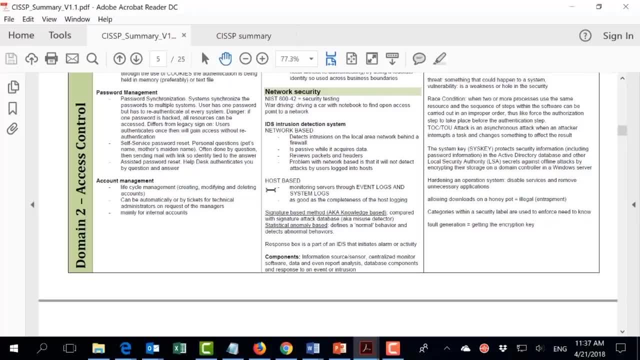 so sometimes, as you can see here, they are writing a definition about the hosted based ids and they are putting that it's getting the event from the log system, for instance, and they put that in capital letter, which reflects the importance of this piece of information. and actually i saw a question where they are asking you from where they are getting the. 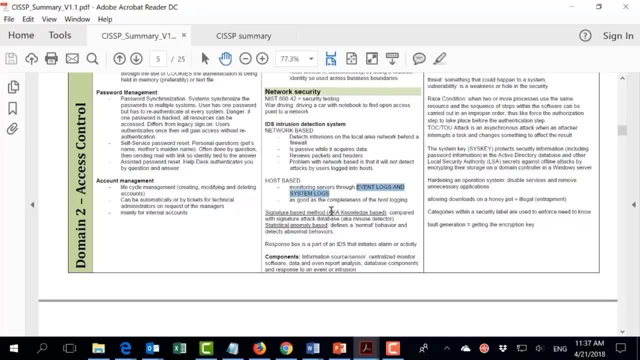 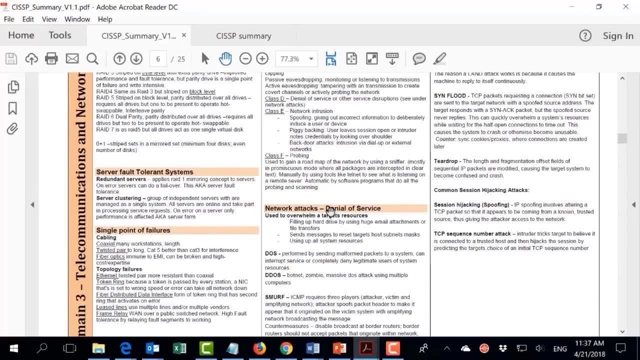 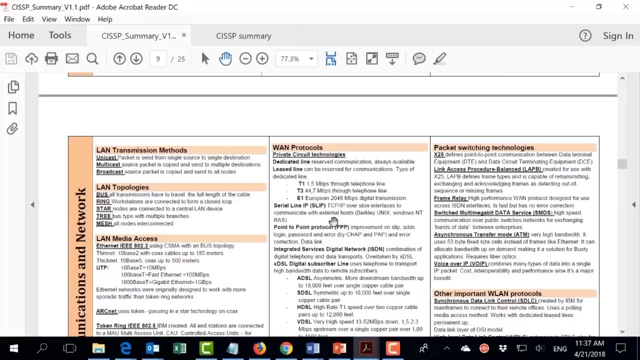 ideas from where he's getting the event. So you will find this kind of pointing to the important point and, as you can see, each domain has different color and what. I usually suggest that you should print it on an E3 paper and literally you need to memorize all this. 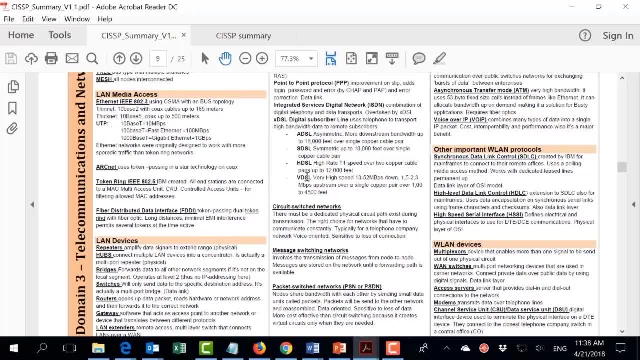 document before setting inside the exam because, as you may notice, CISSP it's filled of definitions, So it's covering too many topics. Okay, but just a brief about each topic and this is the concept related to the CISSP. It's one mile wide and one inch deep. 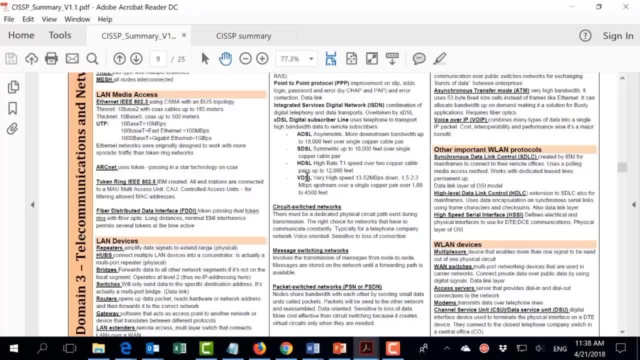 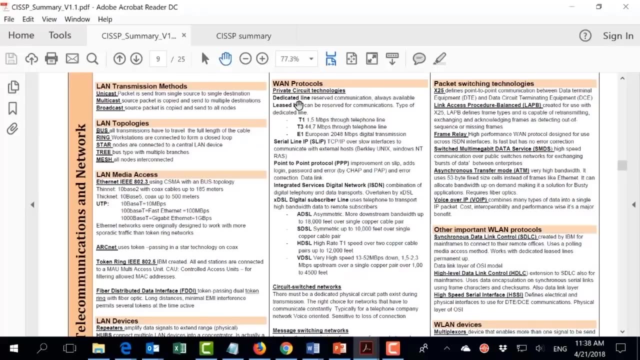 So we are covering a lot of topics but just a small definition about each one of them. So you need to have all those definitions related somewhere or written somewhere, because actually some of the question- unless you know, I mean not all the question- are scenario based, but we have a good amount of question which is actually 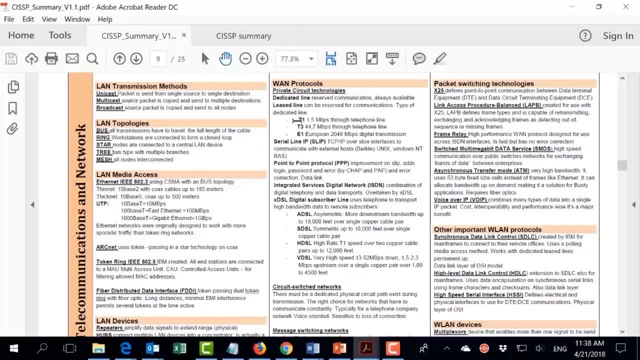 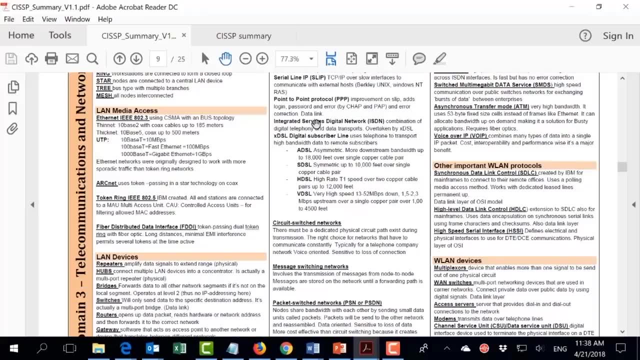 description or a definition about something. So he may ask you about the speed of T1 least light. So you should know that the T1 is 1.5 megahertz. So all the definitions are combined in this document and it's very, very important that whenever you finish any domain, 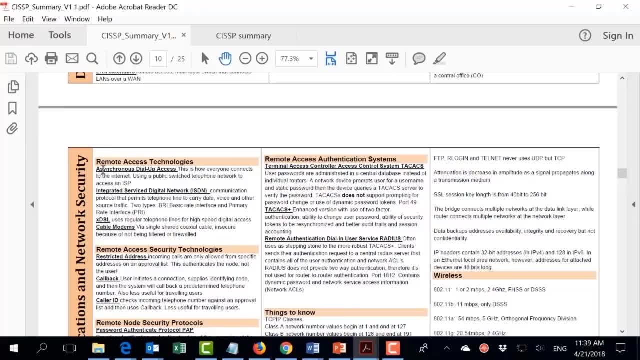 to go to the relevant domain In the sunflower, go through all the terminology and highlighted the point that you are not aware of or it's new to you, and after a while you will find yourself memorizing most of the content of this document. This is a very, very critical document that you need to study. 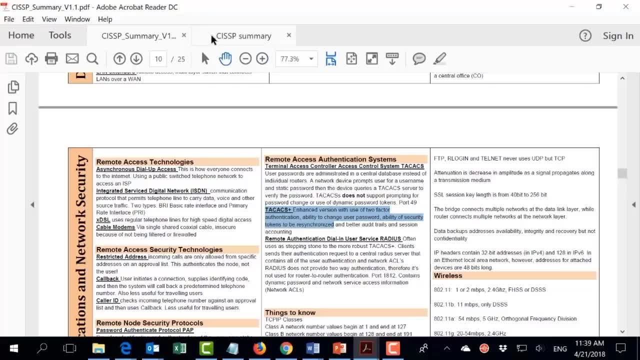 to pass the exam. Now let's get back why we are using two different version. We have 1.1, which I just show you, and we have version 2. 1.1. With the previous CISSP edition, which was 10 domain. 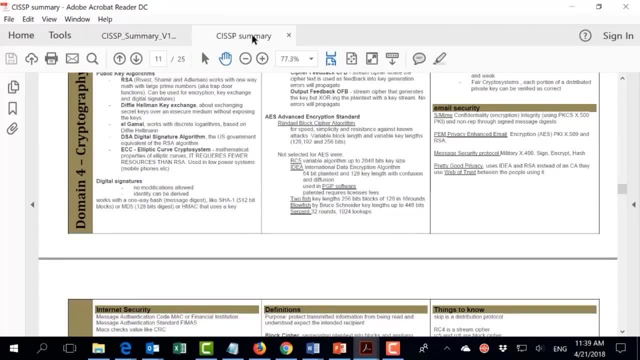 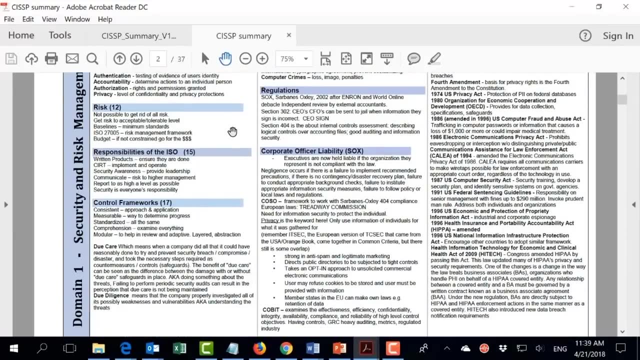 So you will find the structure of the 10 domain, while version 2 is a new version, which is the 8 domain. Now the point in the point is why I should not use only version 2. Since this is a new one. 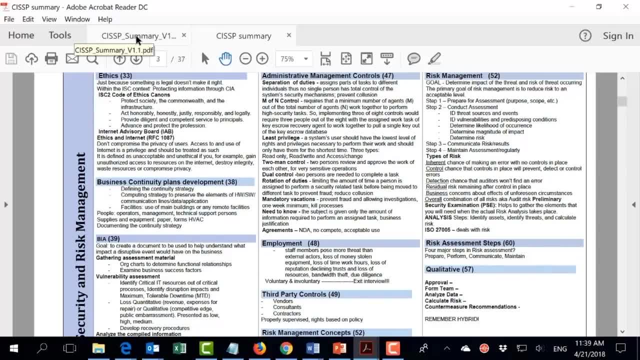 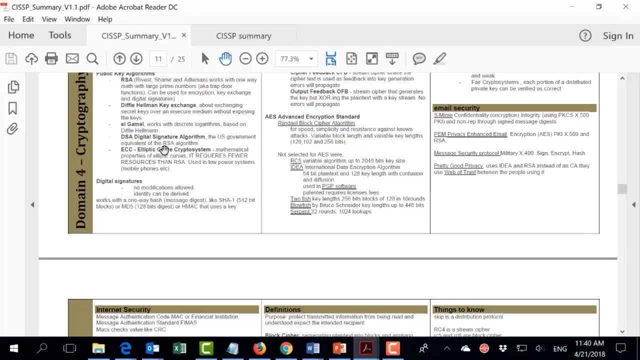 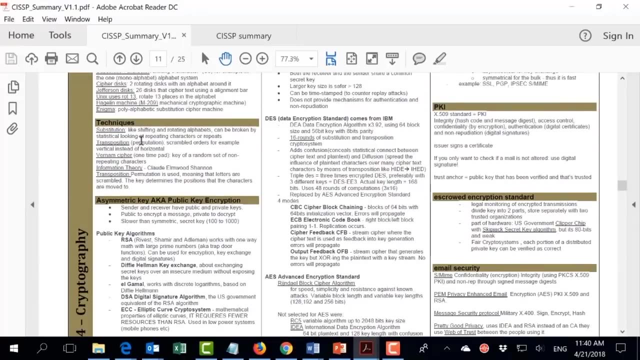 Actually I still find the version 1.5 1.1 more effective. Maybe it will take some, It will Take you some effort to find out the terminology in the old structure of 10 domain, but I can see that this one was really. 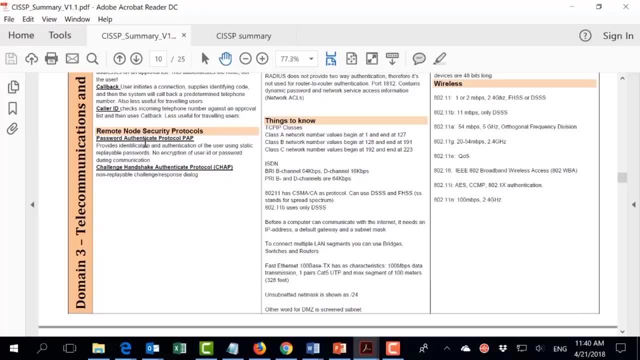 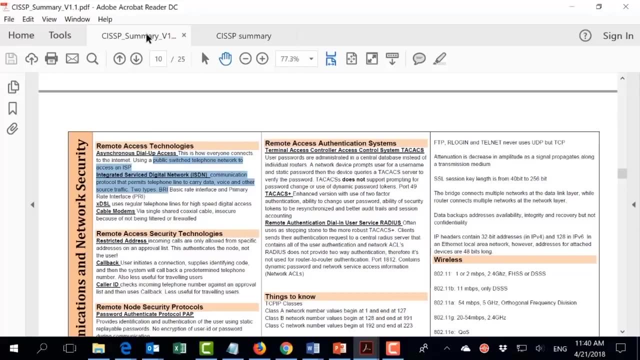 well made in the sense that whatever they are writing, It's very, very applicable to the exam. So I still trust this one than the new one, I don't know why. so I recommend that you study from the version 1.1, even if it's not going through the same structure of the domain. 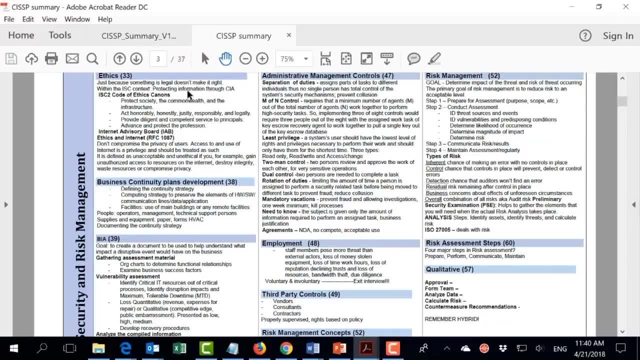 Or if you are comfortable with version 2, is fine. You can study for it. but compare between them. Just take the first domain and see how it's covered in 1.1 and how it's covered in version 2.. If you are more comfortable with version 2, is fine. 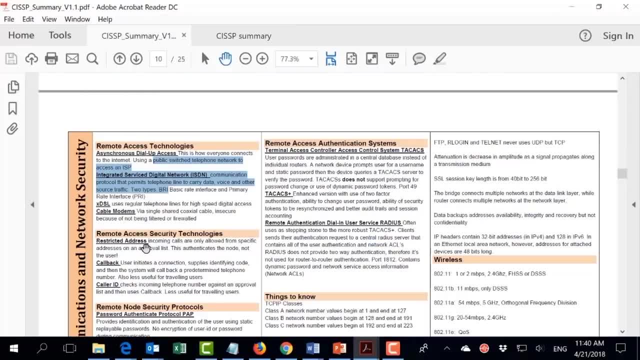 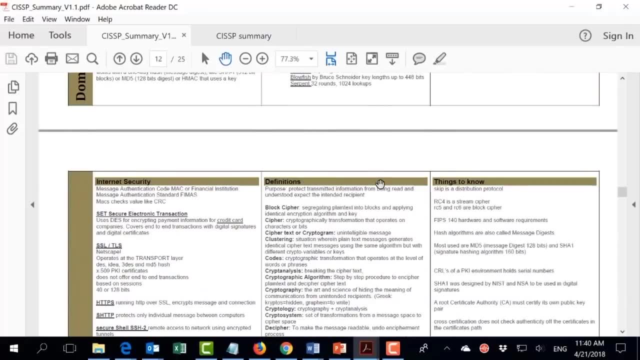 But keep it in your mind just to go through it, especially the important points, ones that is underlined or bold or something like that. Keep that in your mind because I believe it's a very, very effective document. So, At the beginning, please keep that on your desktop. 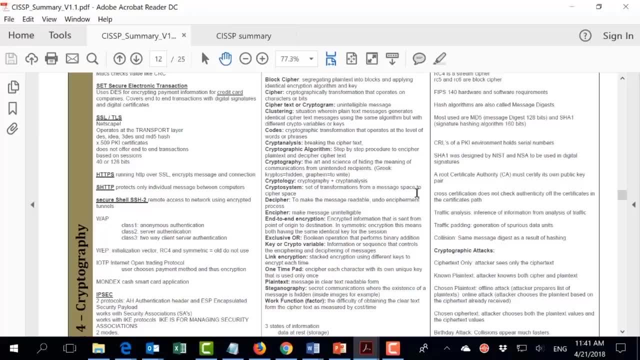 You don't have to wait until you finish the course, then study starting study the sunflower. Now you should work parallel, parallelly. So whenever you finish domain, please go through the equivalent domain in the sunflower and start reading all the point and the. 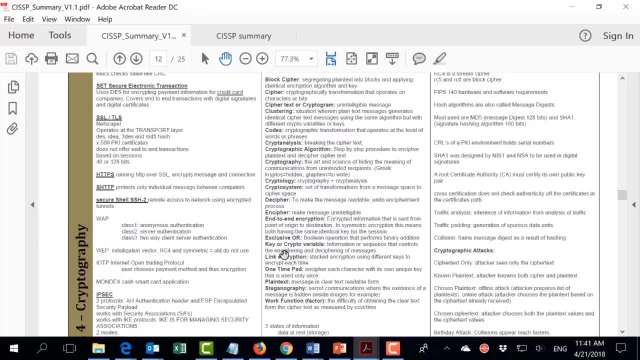 clarification and, as you can see, it's quite summarizing. So it's. it will not Take you that much of effort And take notes, highlights, important points by, but literally before sitting to the exam, Make sure that you went through all the domain from here and you are not. 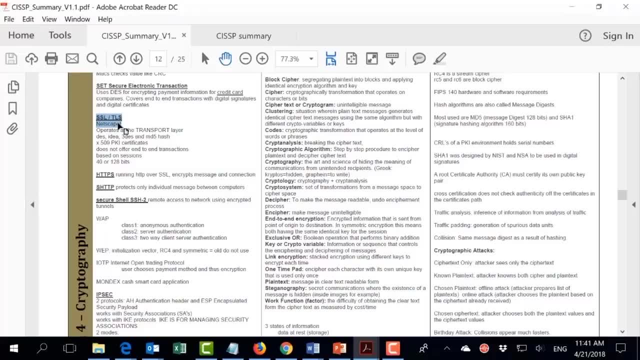 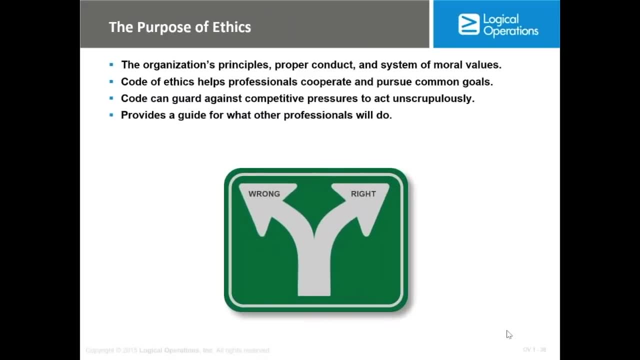 missing any terminology or any definition. In this lecture we're going to talk about ethics and the purpose of encouraging ethics in any organization. Now we all know that ethics cannot be enforced. You cannot enforce someone to have good ethics, but you can encourage good. 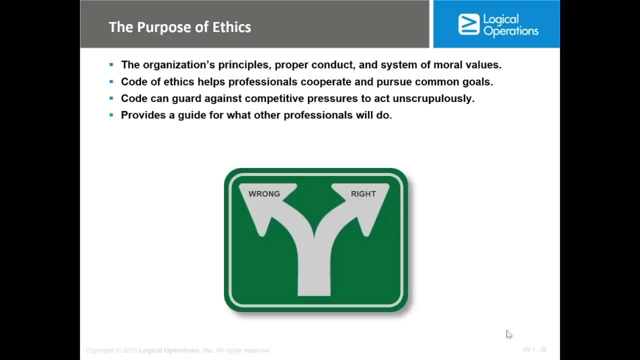 ethics in any organization- and right now a lot of organization- when you get hired, they will give you the code of ethics and you need to read it And sign on it. So it's a kind of theoretical topic, except you may expect a question about that. 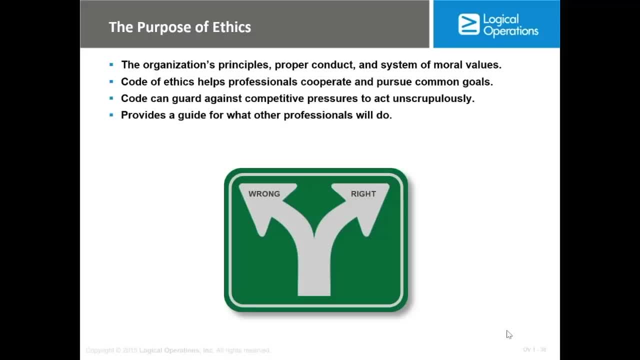 inside the exam, especially related to the well-known code of ethics. So I see squares. They have their own code of ethics. You need to be aware of the internet They have. the code is their own code of ethics, which we're going to talk. 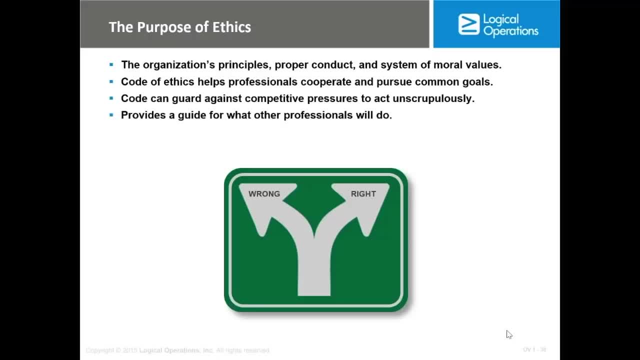 about it. So we'll go briefly about the causal code of ethics, because a lot of those points make a lot of sense, and then I'm going to show you how you can find an exam. How should you expect The question about that inside the exam? 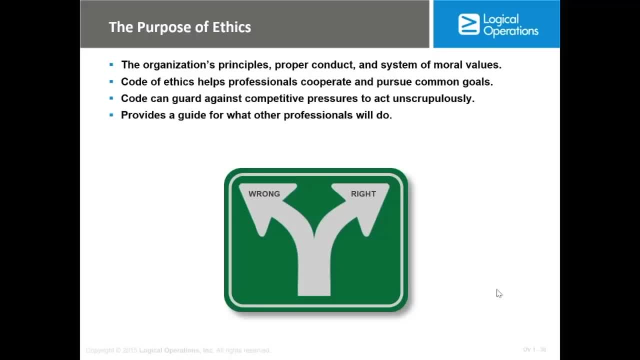 So obviously any organization need to enhance or need to encourage the good, good ethics in their organization and the moral values and so on. And, as I just tell you that right now, some organization, when you get hired, they will give you a code of ethics to read and it make a lot of sense. 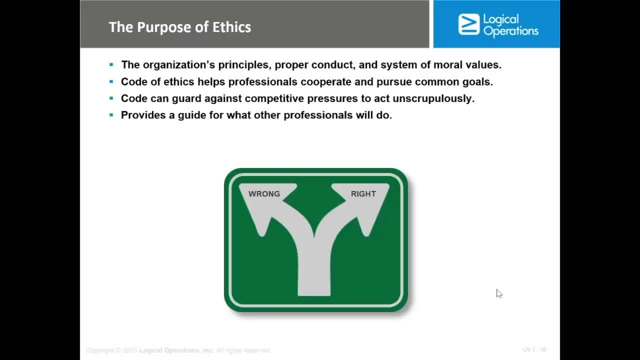 Like you should act responsibly. You should do. You should not do anything illegal. You should be working like this kind of things. I'm going to show you a few of templates related to that, But in general it's not about the policy and procedures only because the thing 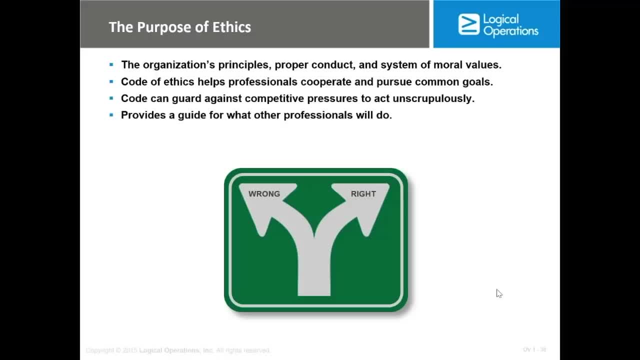 is in the upcoming lecture We're going to talk about. any organization when it come to information security. One of the Main task, or one of them main things, that they should have a folder that have all the policy and procedures and user need to be aware of those policy and procedures. 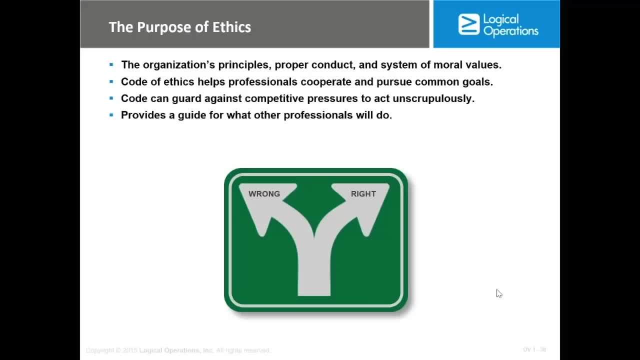 because if they break any policy or procedures, You have the right to take an action against them, legal or regular action. but ethics is different story. You know it cannot be enforced, but you can encourage them. So how exactly it's working? 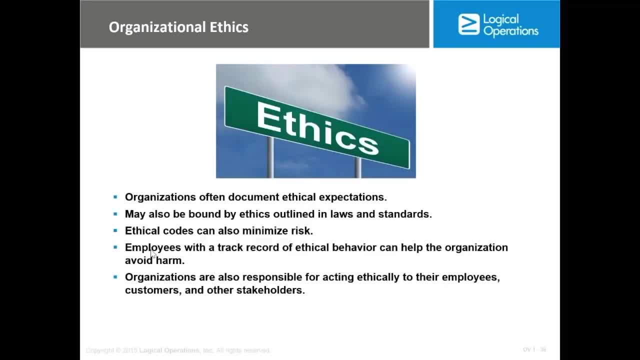 How can you encourage good ethics in your organization? So organization always document The expecting ethical behavior and they share that with their employee. This could be Ethics that is related to legal or low or not, in a sense that Maybe someone can misbehave, but it's not. 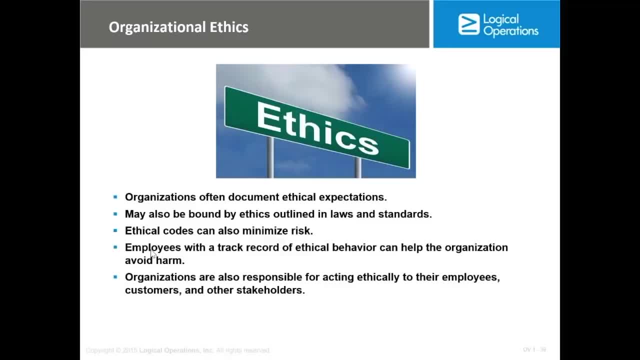 Illegal issue. So is it acceptable? So if someone, for instance, like took some information, he didn't sell them to any competitor or do anything illegal, but he just Erase them in a way or or did something like that, Do you accept that in your organization? 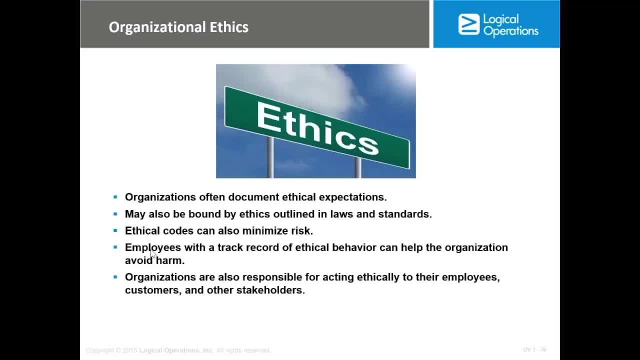 So you cannot take a legal action against him because he didn't do anything wrong, But still it's unethical. So this is what we are trying to say: that you need to encourage the ethical behavior and not just to prevent legal action, but also. 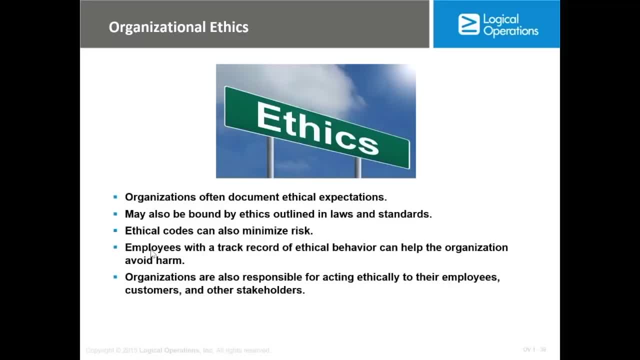 For people to act responsibly. So how it's done? It's usually done by code of ethics and I will encourage you to go online and search for, like some of the well-known code of ethics and read what is inside them. And, as I told you, you know you'll not be surprised, because a lot of those points make a lot of sense. 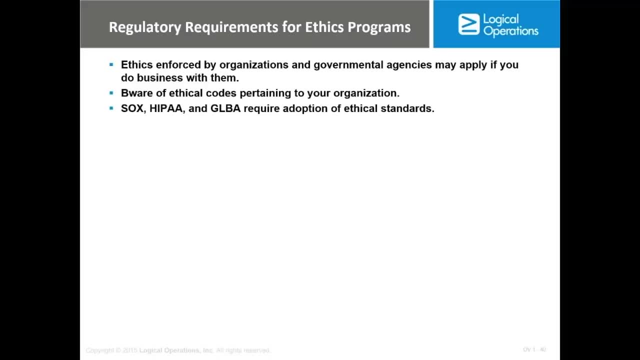 So what we're going to do is that we will share with you Two of the main code of ethics And If you get a question inside the exam about code of ethics, most probably it will come from that. I'm going to show you questions once we finish this part related to code of ethics. 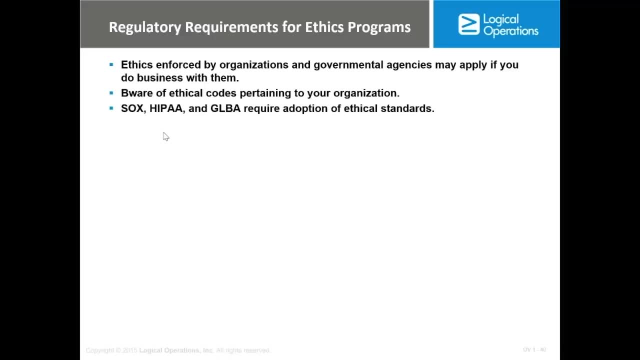 So, as you can see, there is a lot of code of ethics where you know related with HIPAA socks. So if you do a small research online, you will find a lot of that. Let's move to the first one, And actually I saw a couple. 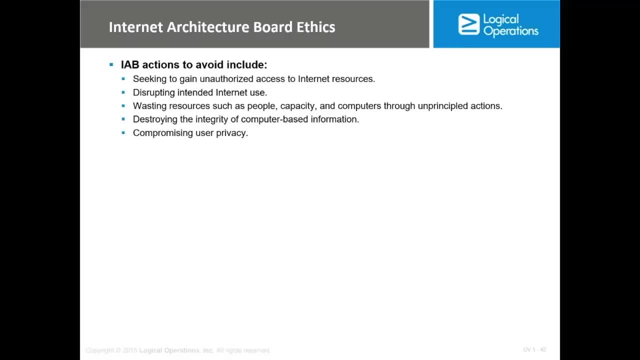 Of question related to this specific one. A lot of people do not know that there is something called the IAB or internet architecture board of ethics Where, in brief, they are saying: if you are using the internet, you need to prevent those kind of action. 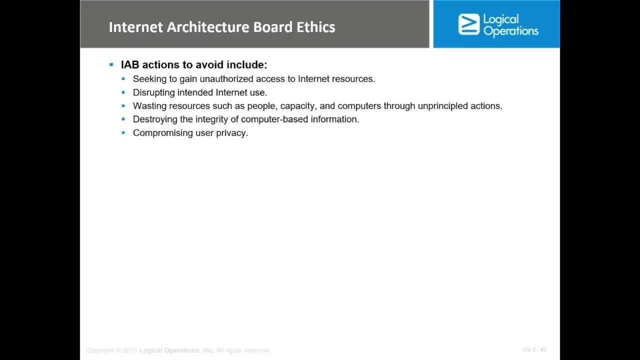 Now, a lot of people are using the internet. They are not aware of that. So, for instance, you should not try to unauthorized access to any of the internet resources. You should not disturb any internet user. You should not wasting resources such as people capacity. 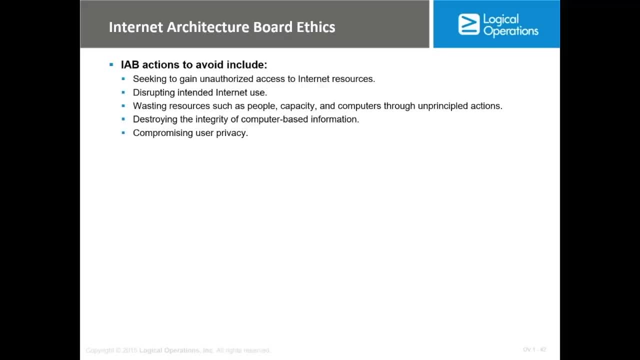 You should not modify the integrity of the computer-based information, So you should not also compromise privacy of people. A lot of point which is quite obvious, right? I remember the question. who came inside the exam was asking: If you spread- I don't recall the exact like sentence. 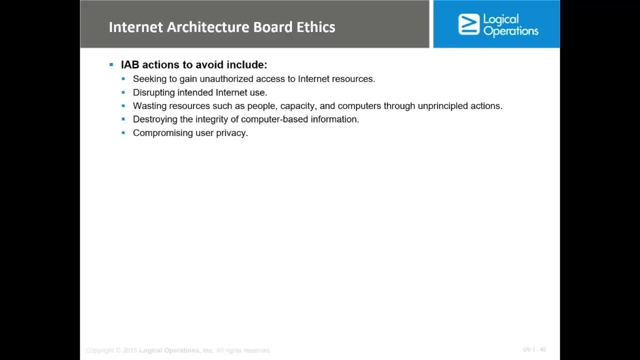 But the idea was: if you spread a virus on the internet, is this against the internet architecture board of ethics? And if you take the question straightforward, spreading a virus on the internet. it seemed wrong But it's not in the internet architecture architecture board of ethics. 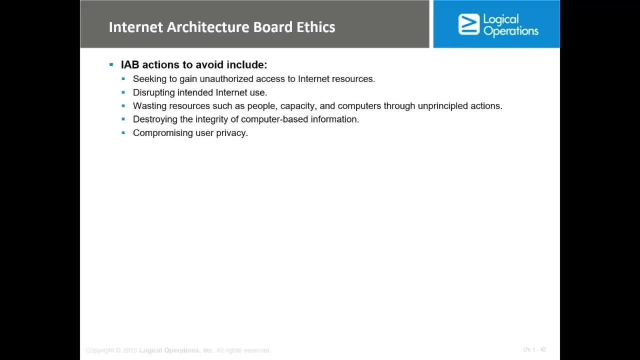 So that's why you do not just count that You will use the common sense To answer the question. No, but sometimes it will be kind of tricky questions, as you can see. So this one, I will strongly like focus on it, and you will see that this is one of the code of ethics in the sunflower document. 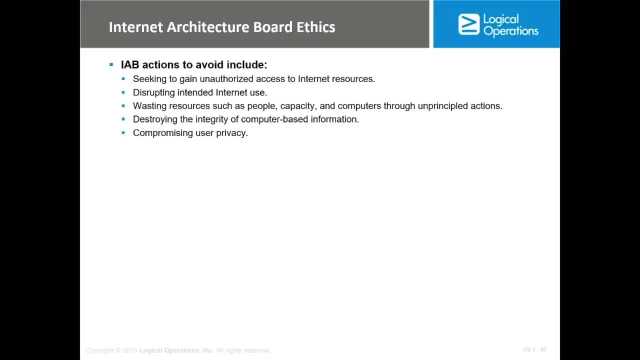 So please write those down, you know, and you don't have to write them down Actually, just read them and memorize them, because if you got a question inside the exam, most probably it will be about them, Because a lot of people do not know that there is an internet architecture board of ethics. 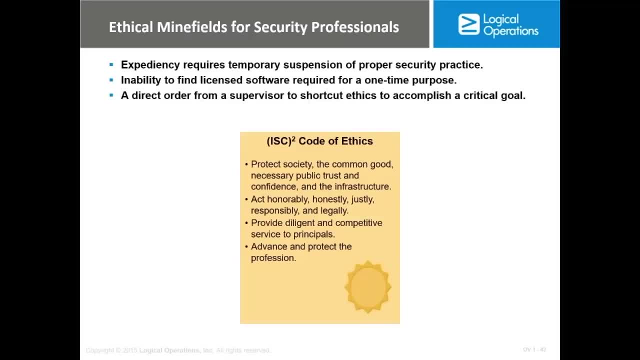 The second one, which is the IC square code of ethics- and still is the same concept- that you should be acting responsibly. You should behave the good conduct. You should not like share any information that affects the business- kind of information. actually do not break any law. 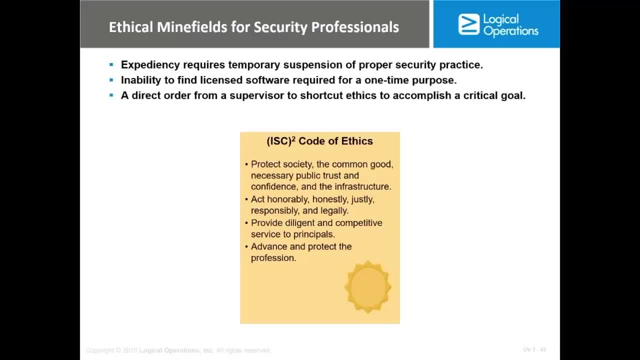 Or legal issue and so on and so forth. Now this code of ethics, you're going to need to sign it and send it to IC square Once you pass the exam to be able to get certificate. So once you pass the exam to get the certificate, you need to download the IC square code of ethics from their website and sign it and send it back to them. 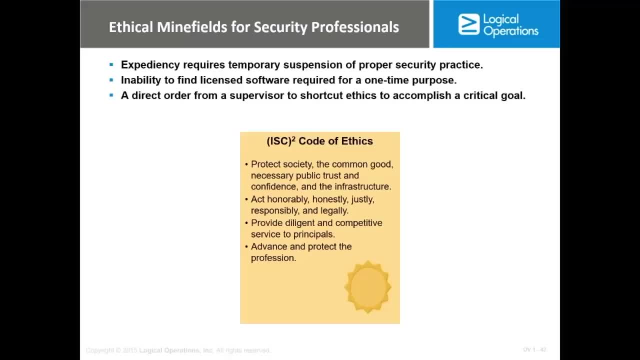 And I have to tell you they are quite serious about that. if you break any law, if someone like report You to IC squares that you didn't follow the good ethics in any way, they will suspend your certificate. I knew few cases where it really happened. 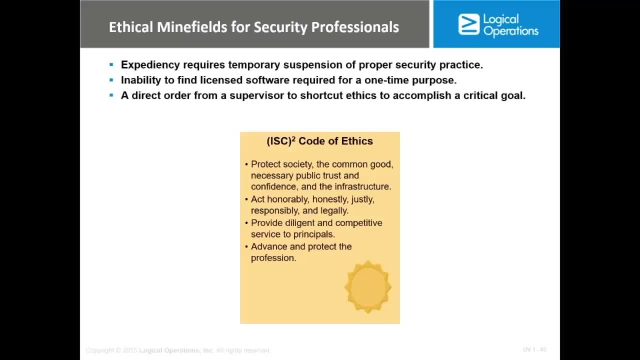 So it's not just a piece of documents that you sign and that's it. No, actually they are taking that quite seriously and you should know that working as an information security officer or any related position, It's a big responsibility. Those are the measures code of ethics that I wanted to share with you, and I wanted to tell you that it's not just a theoretical part. 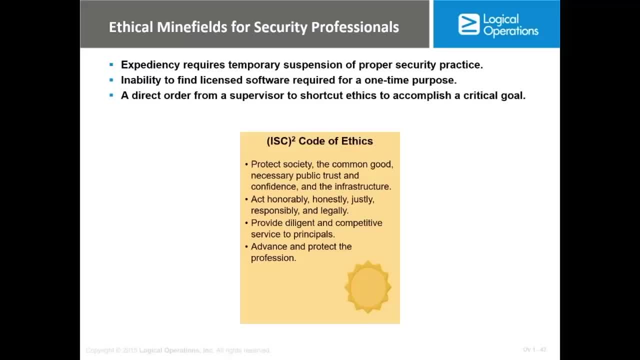 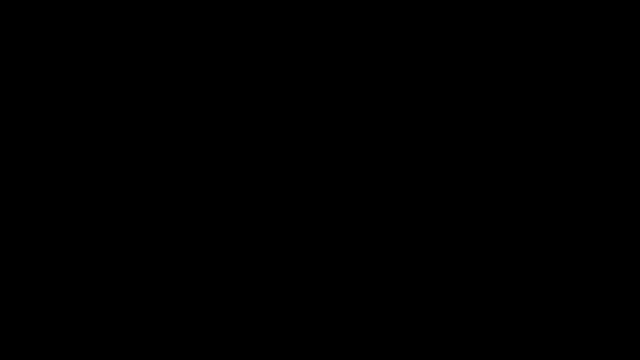 Also, you may face a question about side side the exam. besides, realistically, the last few years I can see that they are raising concern in any organization or business to encourage the good ethics in their business. Let me share with you an exam question Related to code of ethics. 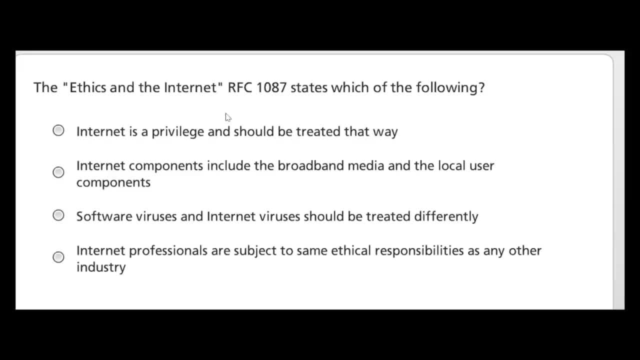 So the question was about the ethic and the internet. RFC 1087 state which of the following now, if you remember, in the previous lecture we spoke about the internet architecture board of Essex. So is it saying the internet is a privilege And should be treated that that way? or internet components include the broadband media and the local user components, or software viruses and internet viruses should be treated differently? 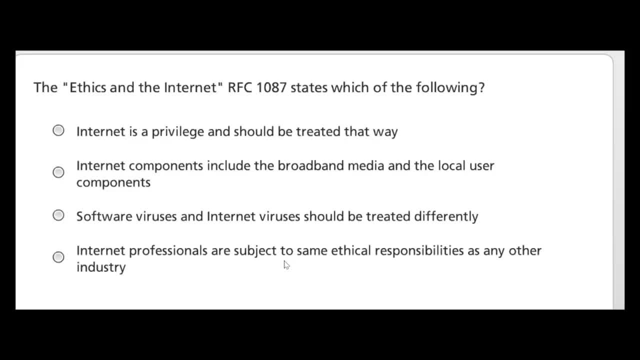 Or internet professional are subject to same ethics responsibility as any of other industry. now I know that a lot of people will not be able to memorize all those kind of codes and all the definitions in this course. Some of them you have to actually, but some of them it's not easy to memorize- all code of ethics and this kind of statement. 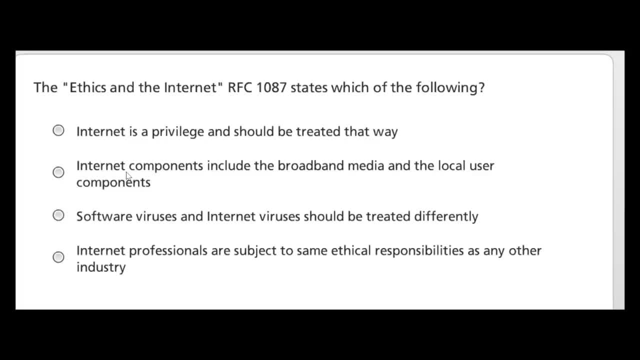 So let's remove the things. that doesn't make any sense Definitely. number two, which is the internet component, includes a broadband media and the local user components. It doesn't seem related to the Code of Essex, right? So number two should not be like, should not, should not be there. 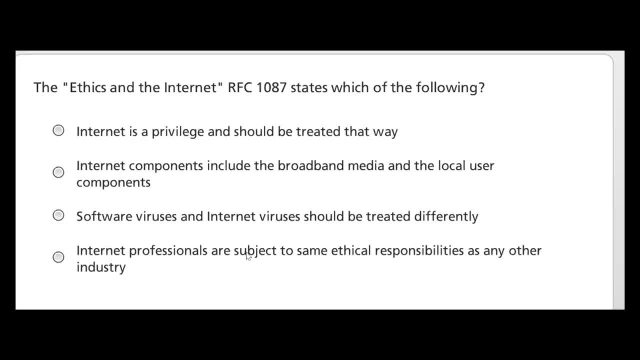 Number four. Also, it's really weird- internet professional are subject to the same ethical responsibility as any other industry. It's really general. So if we exclude two and four, we're going to have one and three remaining. now Many people selected number three. 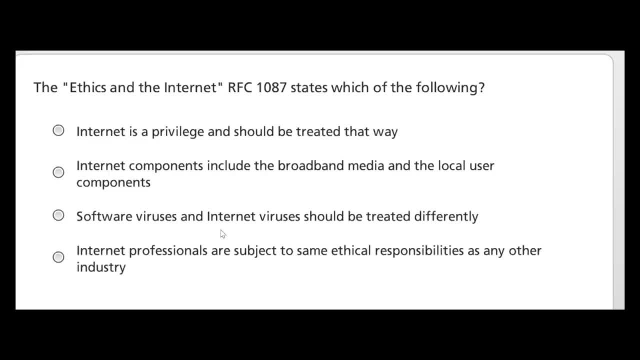 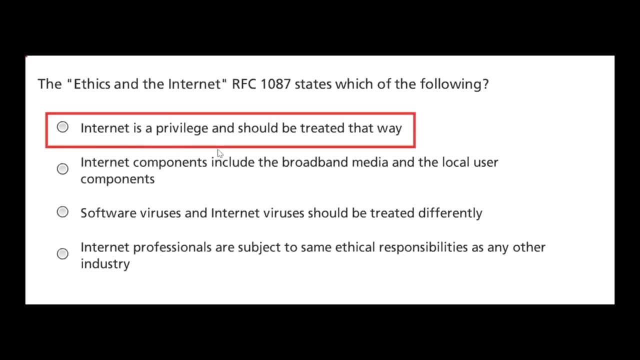 The right way that software virus and internet virus should be treated differently. But actually The right statement If you went back to the previous lecture- is the right statement: with the internet is a privilege as and should be treated this way. This was the first code of state, first statement in the internet architecture board of Essex. 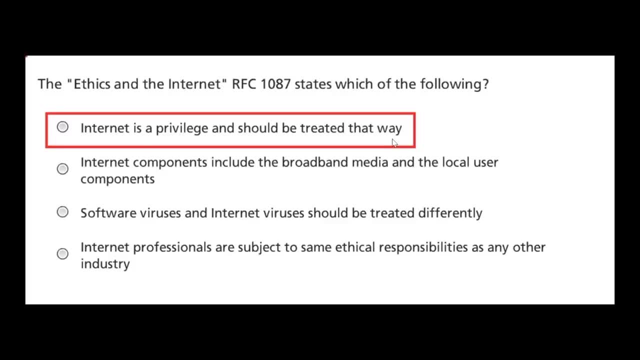 That's why I'm telling you that, when it comes to the code of Essex, you have just to, you need to get an idea about the major one, which is the internet architecture board of Essex, because a lot of people do not aware of it, and the IC square code of Essex. 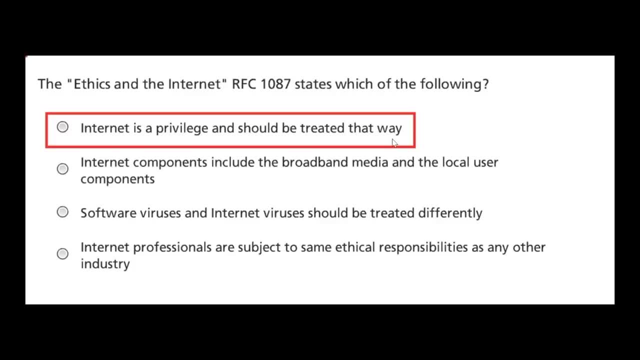 My expectations that they will not ask you about the internet- the IC square code of Essex- because this is something that you're going to need to sign after finishing the exam. But if you're going to ask about anything related to the Essex, It will be the internet. 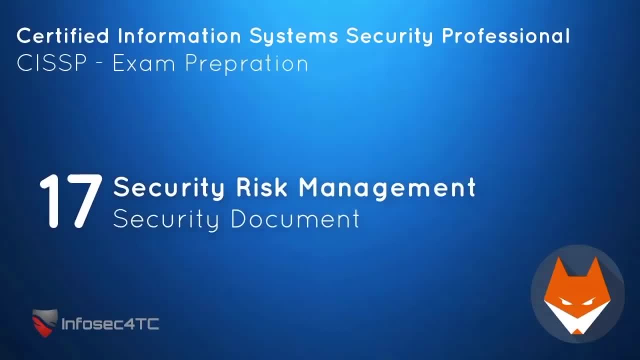 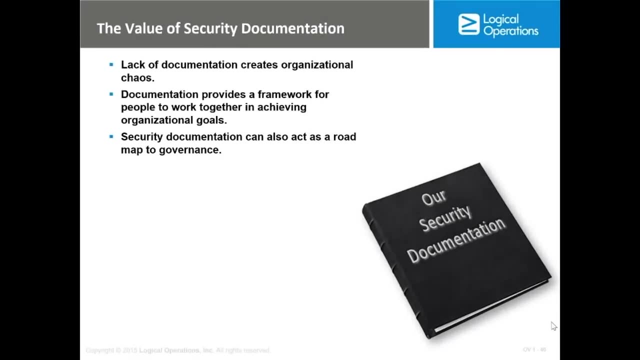 Architectural board of Essex. All previous lectures, with more into the introductory part, talking about what is the element of security, talking about the Essex, talking about the definition of threats and risk and vulnerability and so on. but starting from this lecture we're going to go into the real implementation. 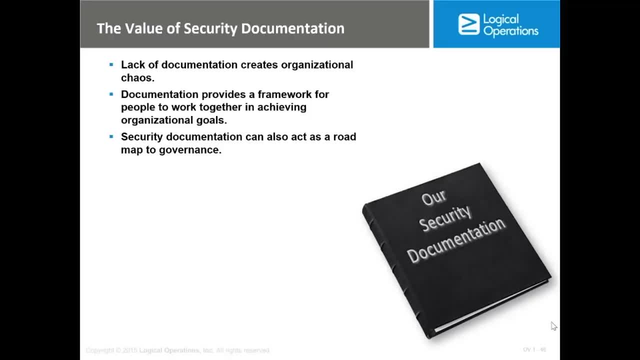 Of information Security in any organization, And he started from here. I would like you to start taking notes Into what we're going to talk about, because the point that we will be covering, starting from now, It's very important for the implementation of information security in any organization. 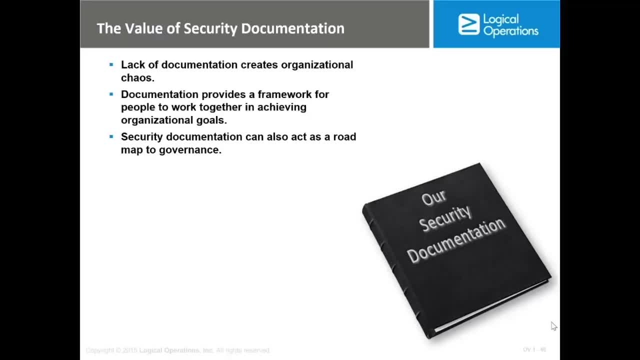 It's very important to pass the exam is very important for you. if you sit for any interview And we're going to start with the security documentation, A big part of your job will be to prepare a lot of security documentation And in security, everything need to be documented. 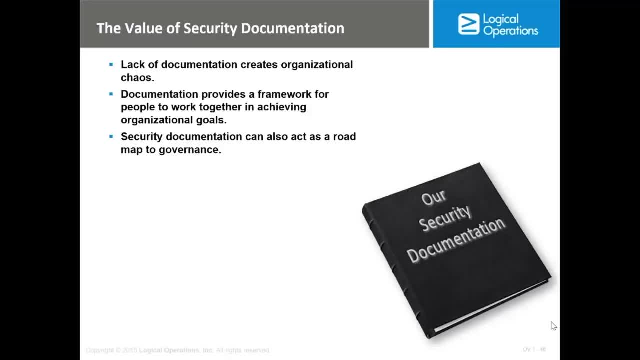 It's not enough to say that I know about it. It need to be documented. So, for instance, if you have a business continuity planning which you're going to cover in a different subject, It's not just to be aware of the plan, but it need to be documented step by step in. 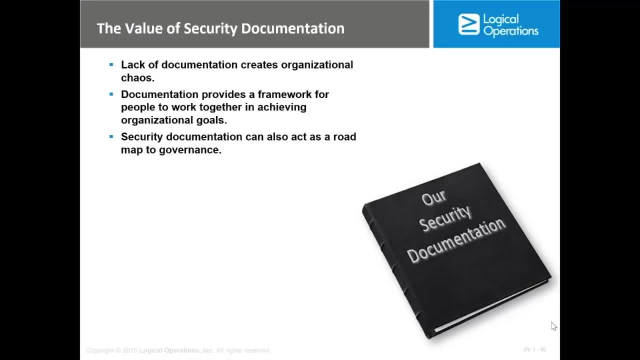 In case of any disaster or any incident, what should be done? If you have a policy related to how are you get rid of information? If you are working in government or military, they have a specific way destroying their information. Is it written? 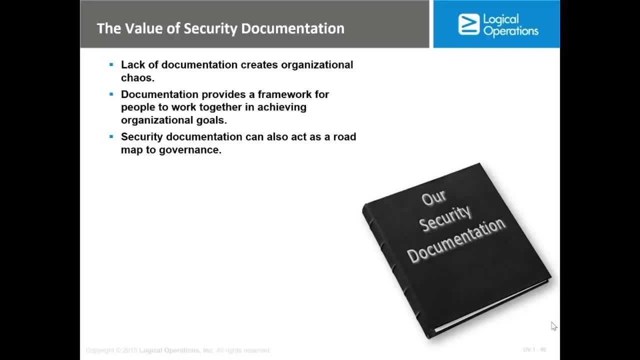 If you have a policy related to for instant creating an email if a new employee join your company, How we should request for an email. Is there any policy showing what is the step for creating an email or what is the requirement for creating an email? 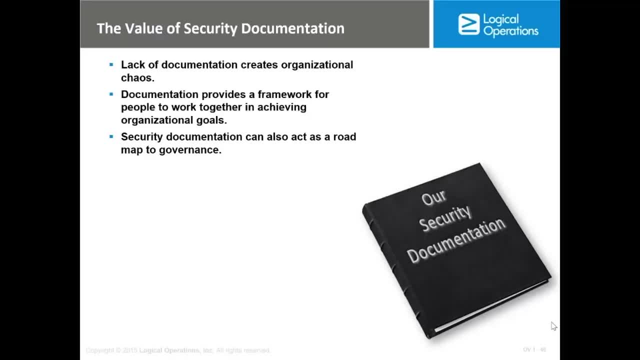 So everything in security need to be documented. This is one point. Second point: People need to be aware of that. So if I join a company as a regular employee, I need to know that this company has their own information Security policy. 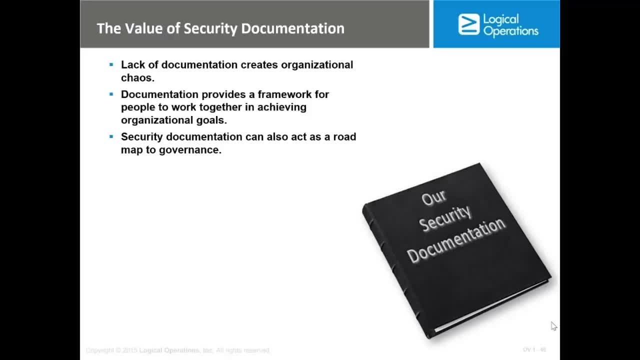 I and I should be aware of that and we're going to cover that in some upcoming lectures. that awareness need to be there to tell your employees that guys, we have information security policy and it's located in this specific directory or this specific website. Because if they are not aware of the policy and they break the security for any reason, intentionally or unintentionally, 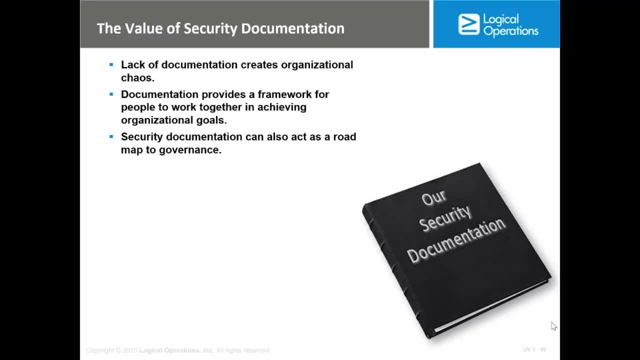 You will not be able to do anything about it. But if you inform that that there is a policy and in case they broke the policy for any reason, Now we can take action against them, considering that most of the major incidents that happens the last 10 years with because of people, due to people, not due to technology. 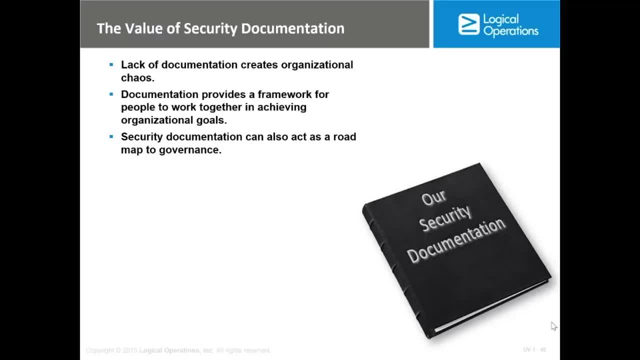 So all of the major compromisation of organization like different company- RSA, Aramco, Saudi Arabia- and different kind of compromisation that happened to company and led to lost of millions of dollars with because of people. So that's why this specific part of the course is quite important. 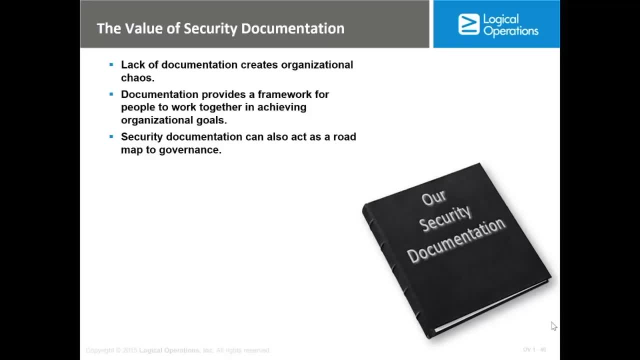 Talking about security documentation and specific documentation that I would like to refer to, but, as a beginning, need to understand that a big portion of your job It's to prepare a lot of security documentation And, if you are following any framework like ISO 27001 or HEPA or PCI DCS- all of them- 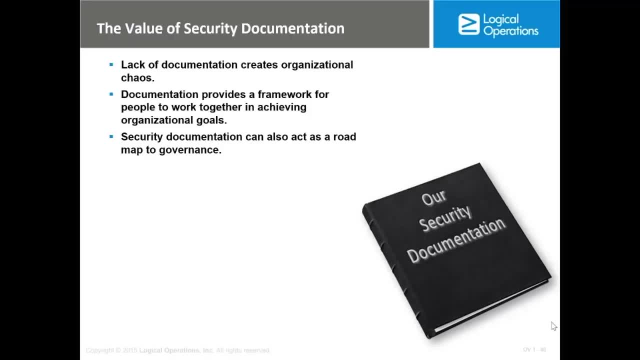 Request the organization to have a security policy and procedures And if you have any audit, if you is any audit coming to your company- one of the main questions that they're going to ask you: Do you have a security policy and procedures? and they're going to check it and then they can ask people. 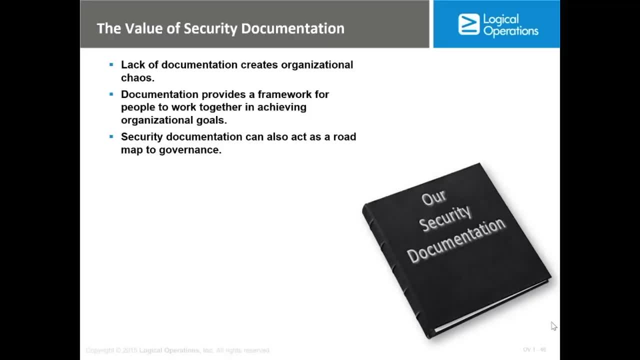 Do you know that your company have a security policy And procedures? So I just want you to give some attention to this lecture and do some research about it. Now we're going to talk about what are the main security documents that should be inside your organization, and your role would be to creating them. 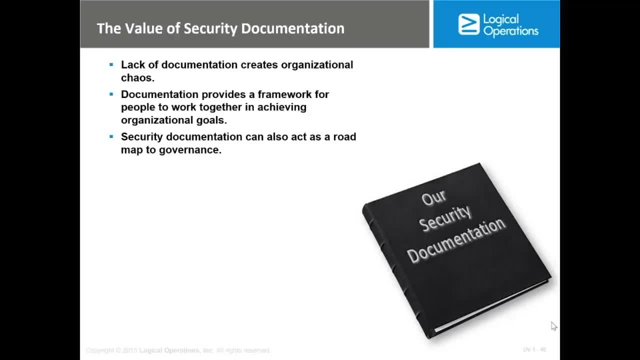 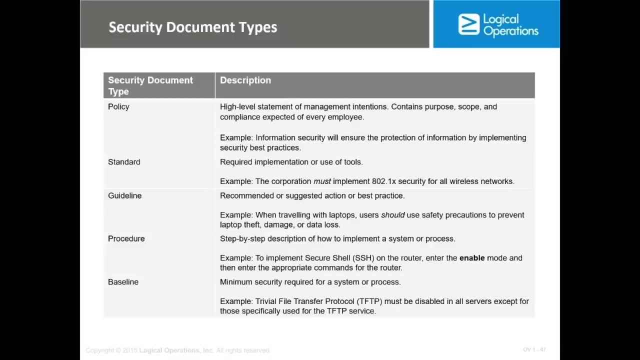 If they are not there from the beginning, but also reviewing them annually and modifying them if any modification is needed. So what are the main security Documents? first, the policy. You should have a policy for every process and everything related to information in your organization. 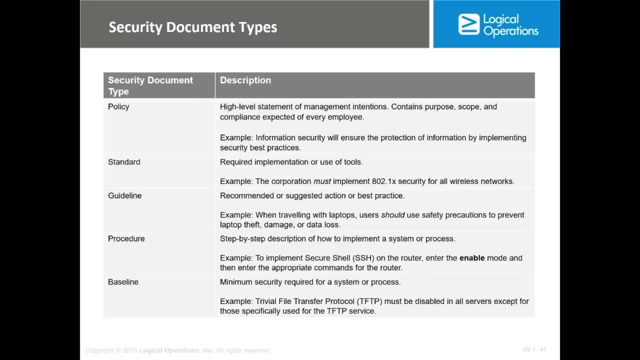 For instance, You have different system in your organization and you are giving people password so they can access the system according to their like job description and their functionality. Do you have a policy? Do you have a policy related to the password, your organization password? 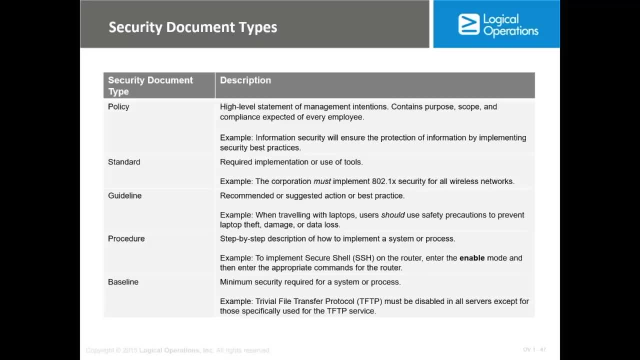 For instance, the policy should say that the password should be Complex, So password should be changed every 90 days or whatever duration. the password should not be shared. The password should not be easy to figure it out And people should be aware of that. 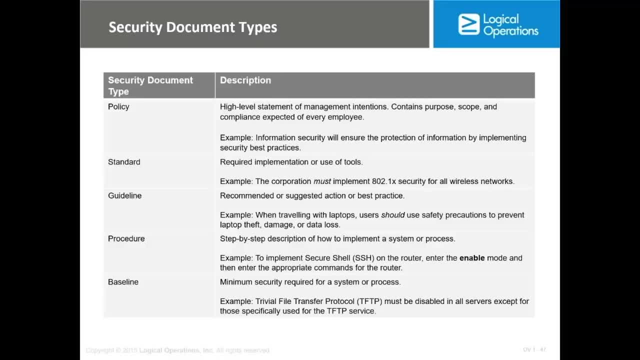 So if any problem happened because someone shares his password over the internet or to someone or something like that, he cannot say: I didn't know that, that there is a password policy. So this is a very small example that you should Have a password policy written. include everything that should be inside the password. 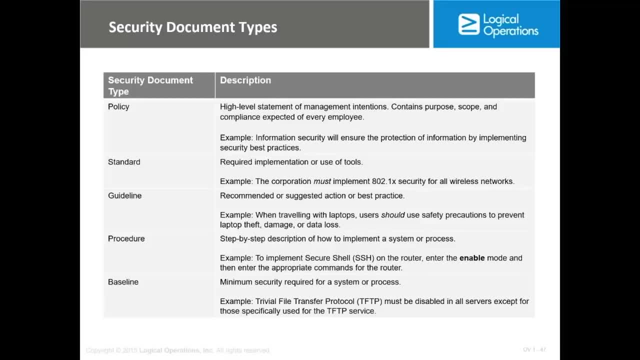 If you are exchanging information, you have different department, your organization or you are dealing with customer and you are giving this customer information, price list, offers and so on and so forth. You have a policy regarding information exchanging. Maybe some of the information are critical. 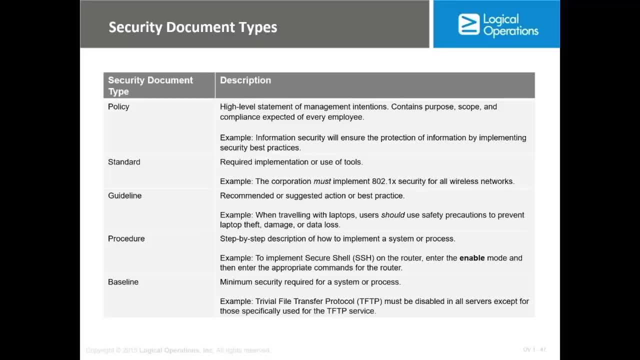 How are you dealing with critical information? If you are an entity like government or military And you are destroying the information from time to time? You have a policy regarding information destruction that, like document, should be for instant Destroyed using a shredder. 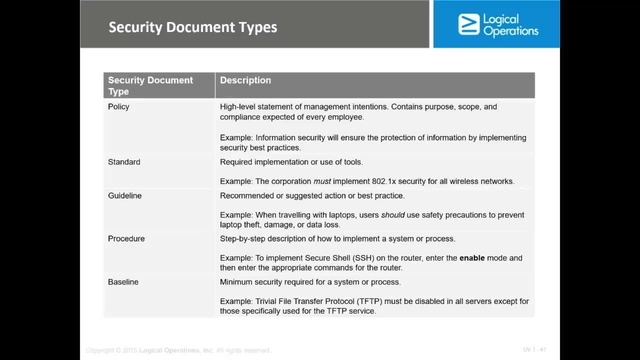 You should not just write or throw them in any recycle or in any place. No, it should be cut by shredder So it cannot be reassembled one more time, Because, as you know, one of the attack it's to check in any company garbage or something- for any critical information. 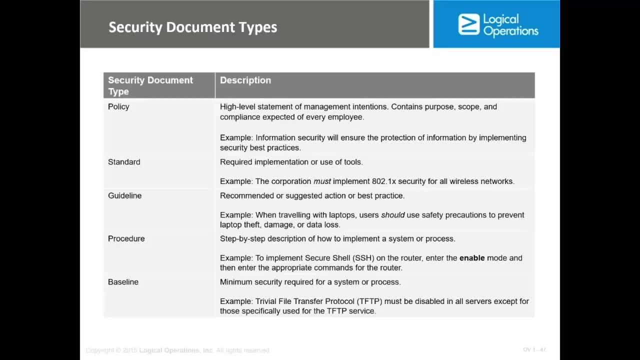 Okay, what if you, as an organization, all your critical and sensitive information are on the computers? So what are you doing if you plan to change the laptop and the computer that you are using? Okay, Are you just going to format The hard drive? 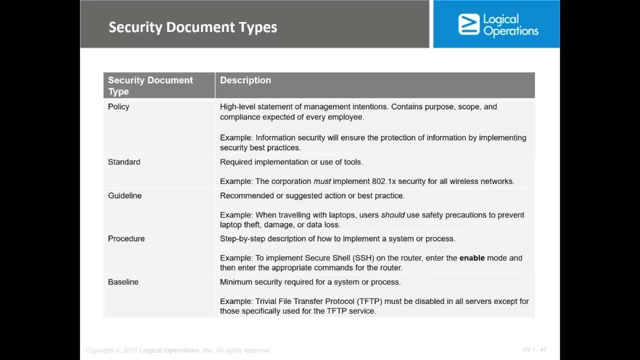 And that's it. You know that even if you format your hard drive six times and rewrite on it, you can retrieve whatever was in this computer. So they should be a policy related to exchanging the computer. Whenever we are changing the computer, We have a policy to make sure that no information that would or was originally on this computer. 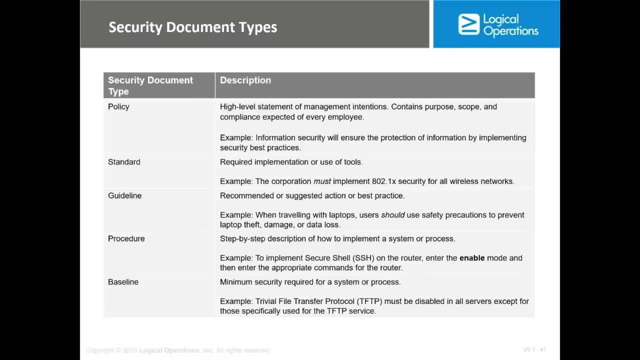 Has been can be recovered. So the policy, It's a very, very important And actually you should have a policy about anything related to information. So we are talking about information exchanging, We are talking about information, This, this drawing, we are talking about password. 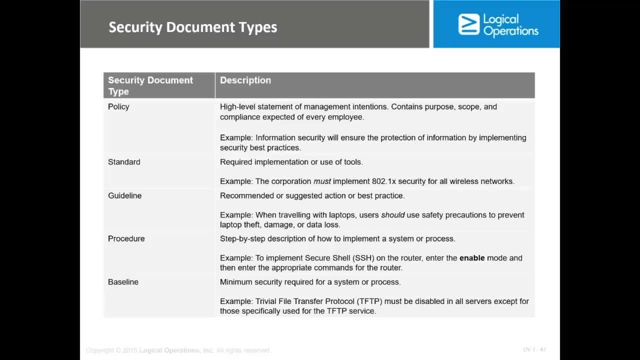 We are talking about, for instant encryption. If you are using encryption to secure the information, to have a policy regarding that, and so on and so forth, I will show you a very good source from where you can get a lot of policy, because it's not an easy document to write, by the way. 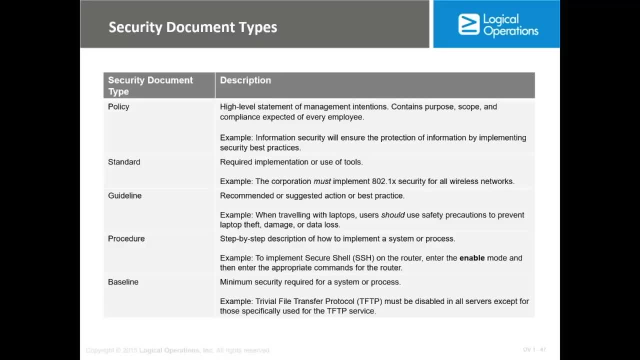 Okay. So it's better to start with something like templates or a good resources from where you can get some policy. Then we're going to explain the difference between the policy and procedures and guidelines and so on. Now, before showing you the source from where you can get policy, 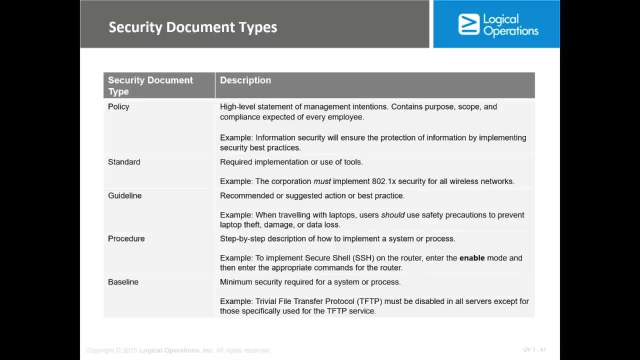 You need to understand that policy, as a definition, is a high-level statement of management And it just contains the purpose and scope and compliance mapping, in a sense that the policy Will not include how to do it. So, for instance, if you have a password, policy should say that policy need to be complete, complex and it need to be changed every 90 days. 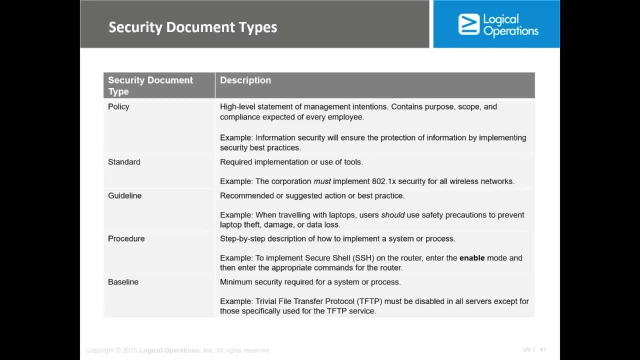 But it will not say how to go into the system or to your computer and change it to a complex password. It will not say how to, step by step, how to assign or how to make to enforce the password to be changed every 90 days. 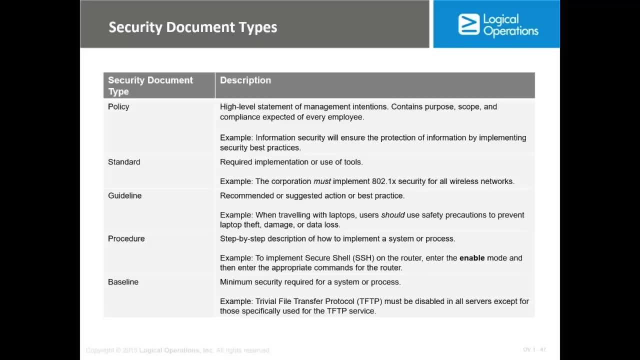 It will not Explain how to do it, but it will just mention The policy, what it's saying and, most important, mapping with the compliance. So it will say we should have a strong password because ISO 27001 in this specific section, This specific control is requesting that, and PCI DCS in this specific section, and the specific control is requesting that. 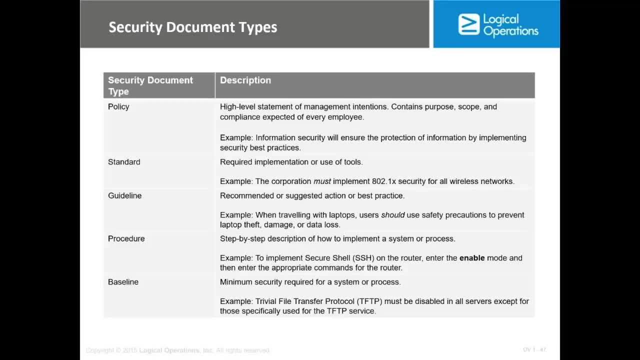 And so on and so forth. So you should map the policy with the requirement. So because if you got any audit, they will check the compliance and saying, okay, show me the control related to that, So you can show them that you have a policy that is saying: 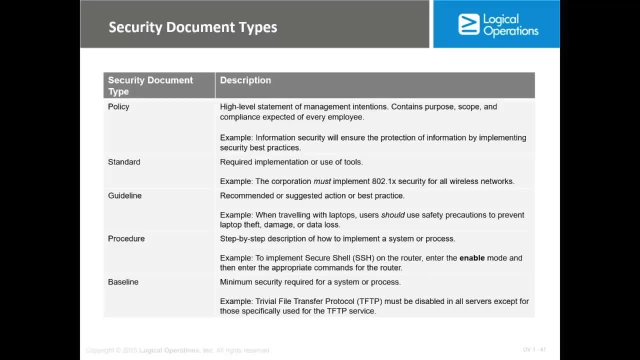 12345. So it should be mapping or mapped with the compliance or framework. before moving and explaining the different Kind of other security document, Let me show you some of the policy or some of the resources or website from where you can get policy as a template and you can use them in your company. 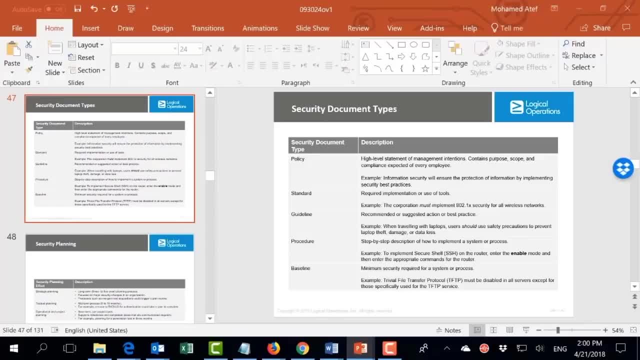 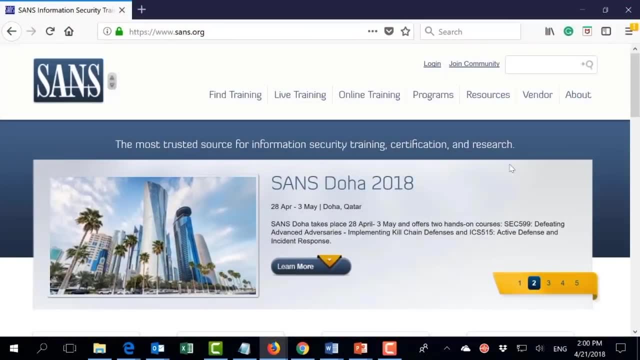 A very good resources, for that will be sans website, since they have their own website, since it's a very huge security organization And if you go to their website and go to resources And you go to this Security policy project, You will find. 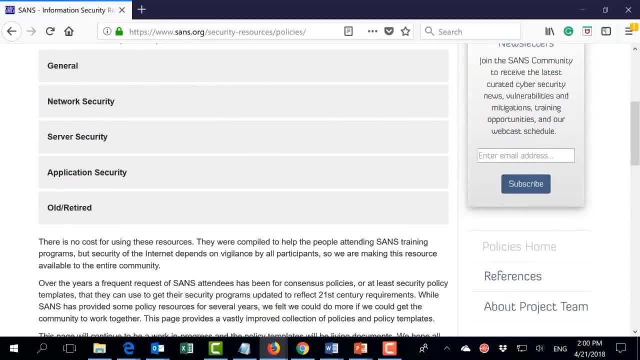 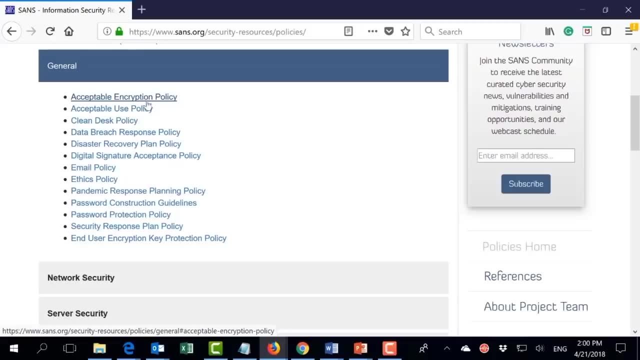 They have a lot of templates that you can use. So, for instance, you have general policy or you can click on it and you can see we have acceptable encryption policy. We have, for instance, clean desk policies, that all the employee should have a clean desktop. 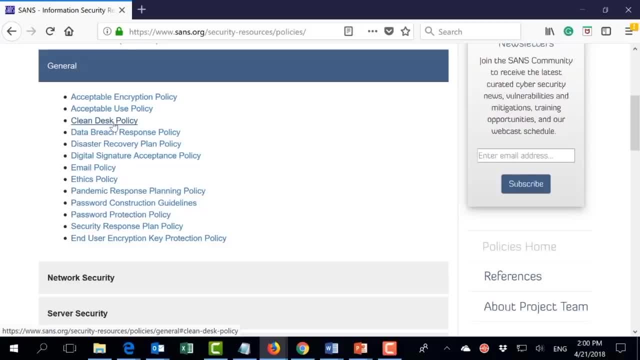 You should not leave sensitive document on your desk. We should not leave sensitive information. Maybe it gets stolen or lost. It's a policy. Okay, not all policy are technical, as you're going to explain in a few minutes. We have for instant data recovery policy. 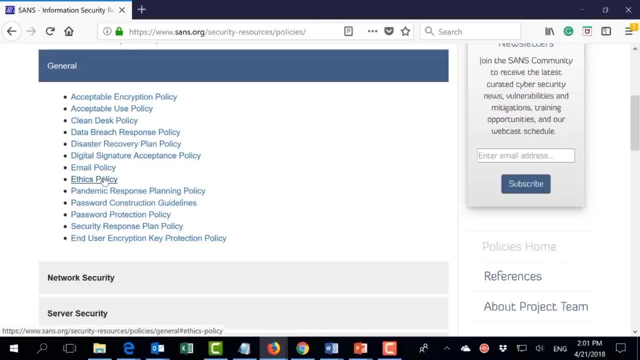 We have digital signature policy. You can download whatever you need to download, according to the business and the process You have. one policy is quite important: The email policy. People are using the company email. They don't know what is the regulation when it comes to using the company email: that you should not use this email or you should only use it for business purpose. 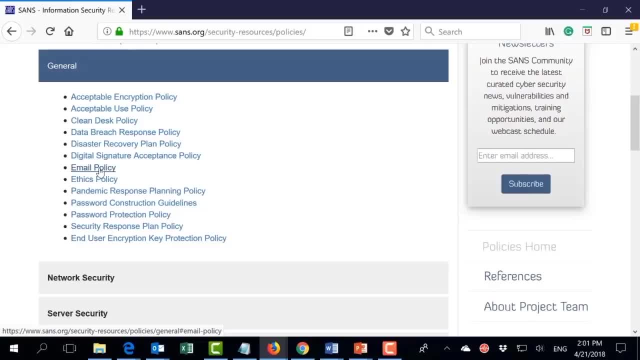 You should not use this email for anything offensive to your employee. You should not use it for threatening people, This kind of thing. And again, it's not enough to have the policy, but people need to be aware that there is a policy, because if they break the policy then you have the right to take a legal action. 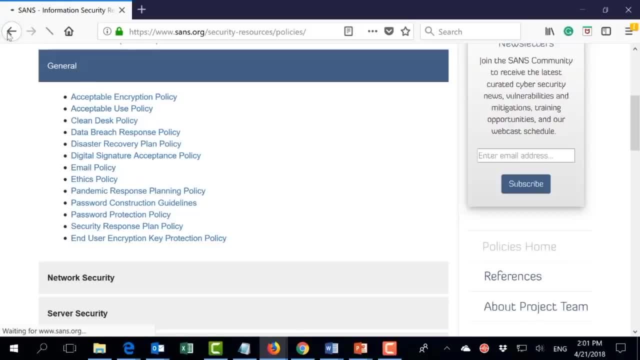 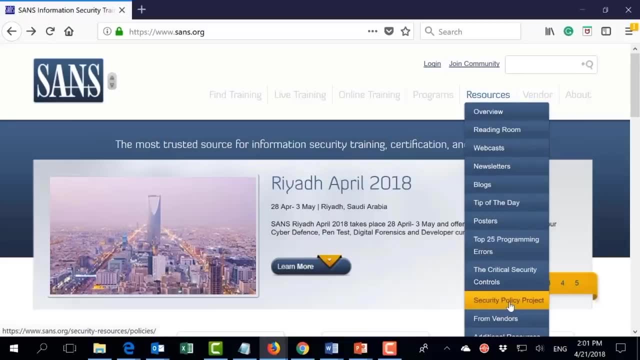 So those are like password policy, the general policy. Okay, going back, You'll find other kinds of policy. For instance, you're going to find the network policy, You're going to find that. So it's a very good source from where you can download templates that you can use: application policy and so on and so forth. 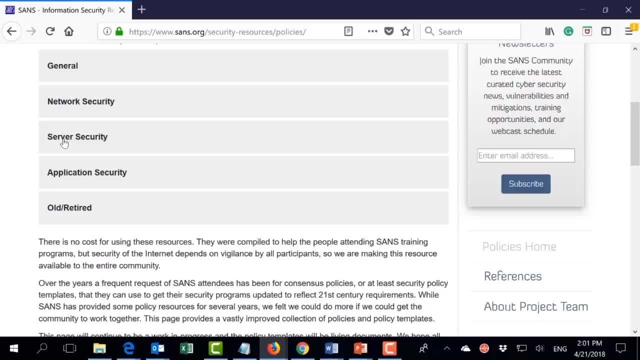 Okay now, before moving to the other kind of document, you need to understand that we have two different kinds of policy. One is a user policy and non-user policy. You can categorize them. So things that is related to the user, like for instant password, somehow for user, need to be aware. 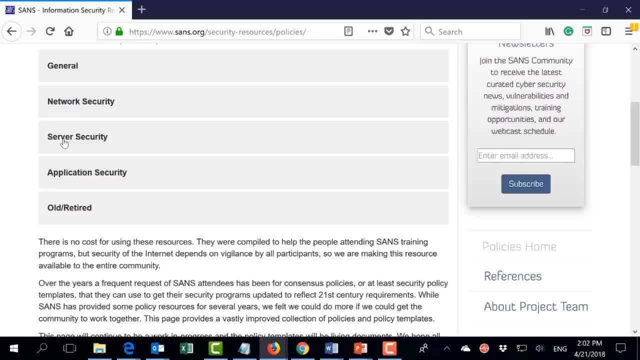 That what need to be followed when it comes to password, especially. think about sharing password. Do not write a password on a piece of paper and or sticky note and put it on your screen. This is user password. email policy. This is user password. 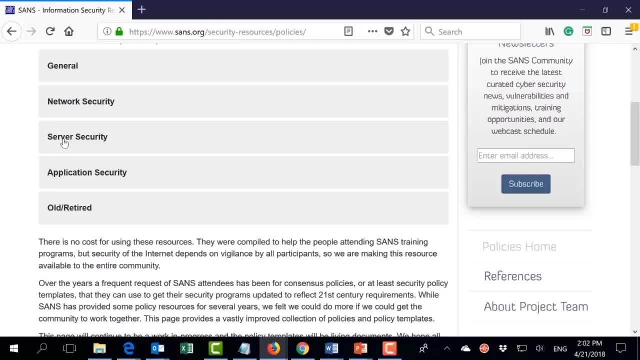 User need to know when it comes to using the company email. Is there any restriction? Okay, but some other policy will be technical policy, like network policy, encryption policy. User has nothing to do with that, Okay. software development policy and so on. 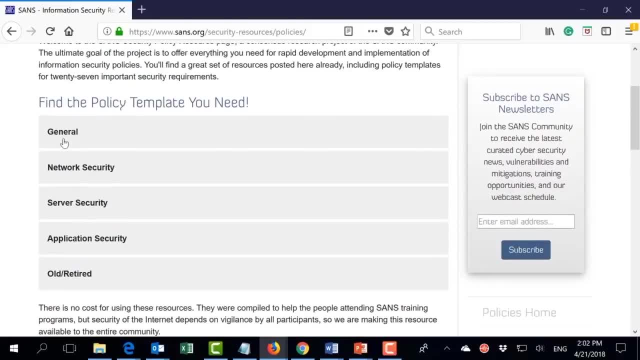 So forth. So to summarize that one of the first step in information security implementation, that the company should have an information security policy related to whatever assets they have. The assets is mainly information. So how they are dealing with information, how they are dealing with exchanging the information, deleting the information using the email, using the 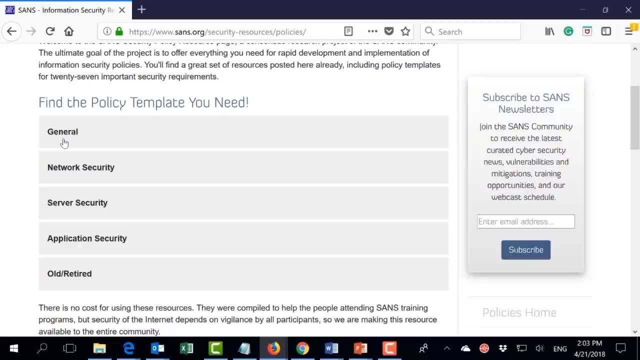 password As a beginning. this is quite important and it's a main requirement for any compliance or framework. How it's working: Usually we are writing those policy and putting them in a share folder And allowing or notifying user. that guys kindly be aware. 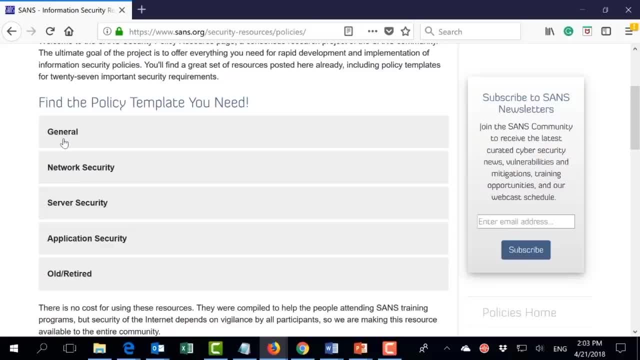 That if you are using any of the company assets- because the email is considered a company Assets, information is considered as a company assets, The list of customer and supplier is considered the information assets, and so on- If you are using any services or you are using any company assets, there is a policy that controls it. 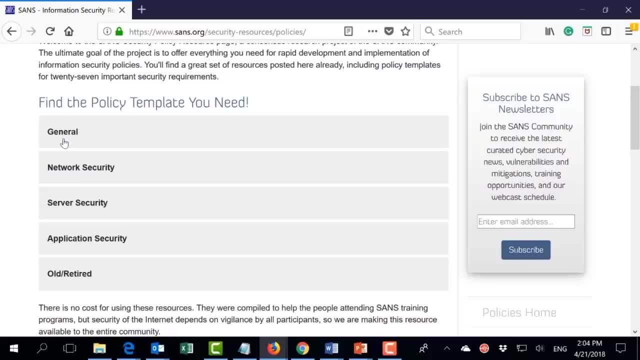 And this policy is located in this specific share folder or on the company portal or website. by doing that And thinking about the legal issue and the liability, Now you are saying to the employees that if you are not aware of the policy, This will not be as an excuse if you did anything wrong because you are not aware of the policy. 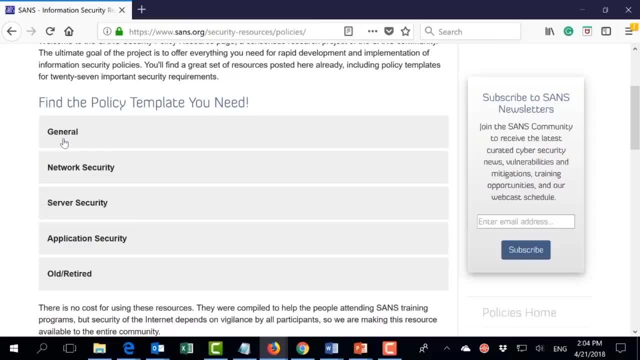 So getting the policy is important, But also, as informing using, say, is this same importance that user need to be aware of the policy. Last point, before moving to the next lecture, is that policy need to be reviewed once per year. So it's not enough to have a policy, but it need to be reviewed once per year and need to write on the document control. 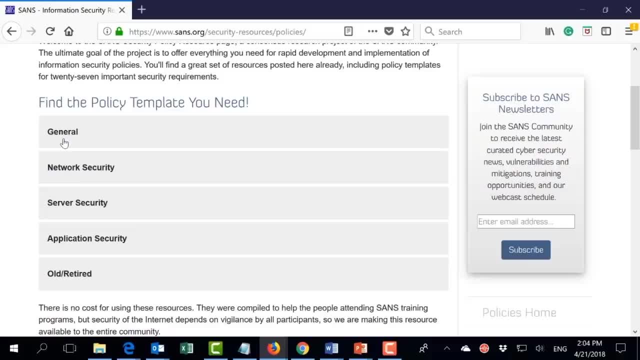 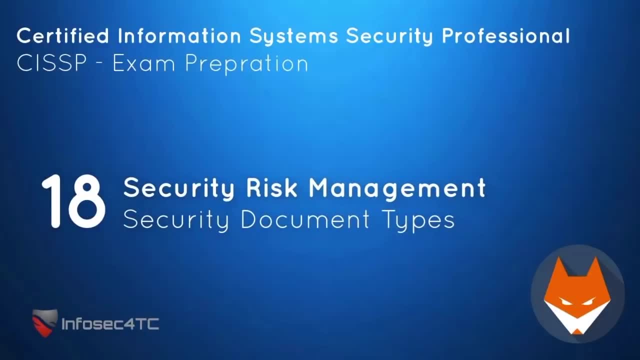 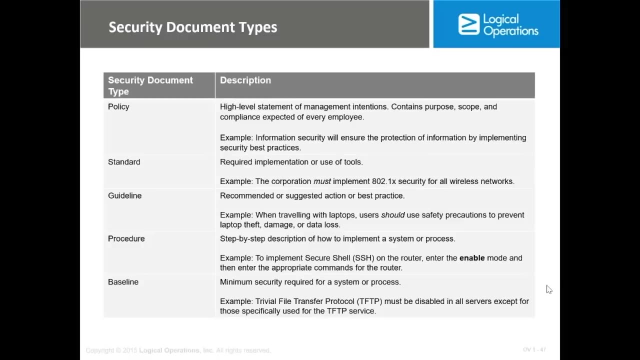 As you can see later on, that it has been reviewed this year by this specific gentleman, and so on. In the previous lecture we spoke about the security document and specially the policy. What is a policy and why it's important to have a policy? 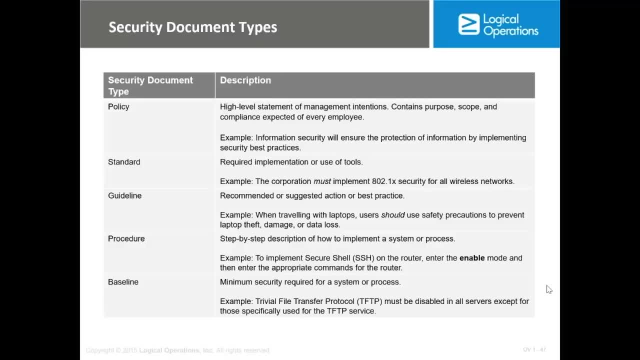 And why it's important for user to know about the company policy, and so on and so forth. In this lecture we're going to talk about the different document, because it's not only the security The policy is that you need to have, but also need to have standard procedures, guidelines and so on. 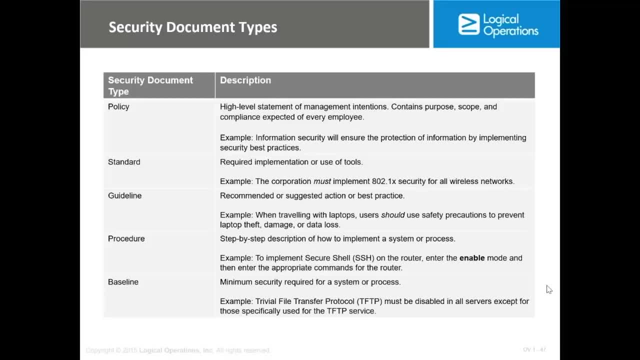 So you need to distinguish between them And most probably you're going to get one or two question about that inside the exam because security document It's quite important in any organization And, as I Just mentioned in the previous lecture, that in any audit the first thing that they're going to ask about will be the show me the policy that you are following in your company. 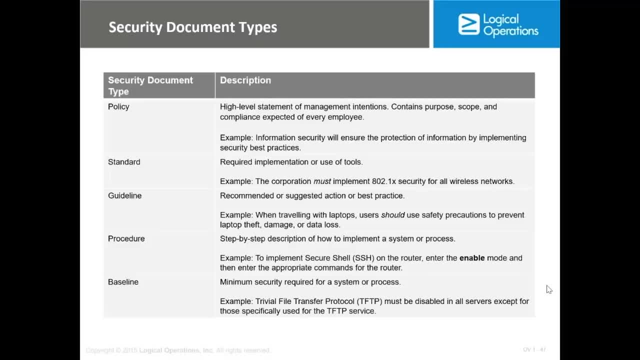 So everything needs to be written. So we already spoke about policy, which is a high-level statement. It doesn't include any steps for doing anything, but it will tell you. for instance, if we are talking about email policy, it should not be used in something that is not related to work. 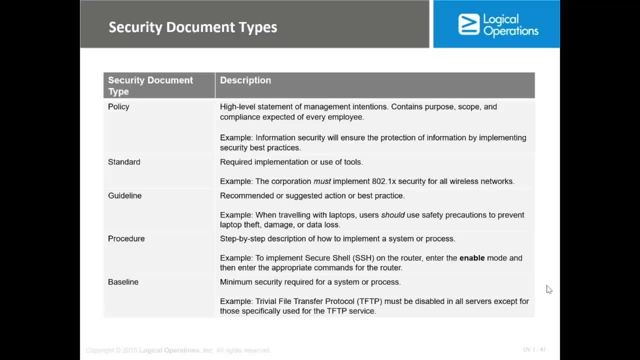 It should be business-oriented. You should not Be using it for any offensive Way. the attachment should be the maximum. attachment should be that much. each user of the company should have like storage capacity of that much, and so on and so forth. Then we have the standard. 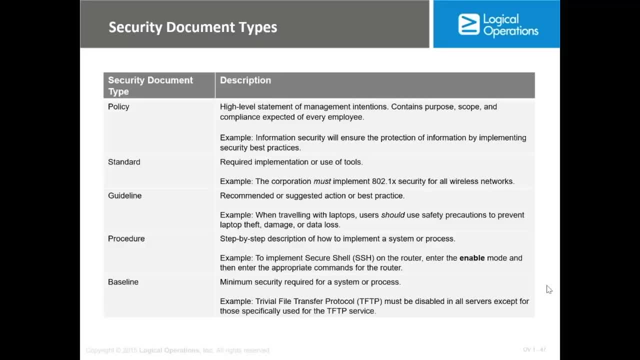 And the standard. it's more than what need to be followed when you are doing the policy. So, for instance, when we are talking about password policy, Standard usually is eight character that include letters and numbers, small and Captain and special. This is a standard. 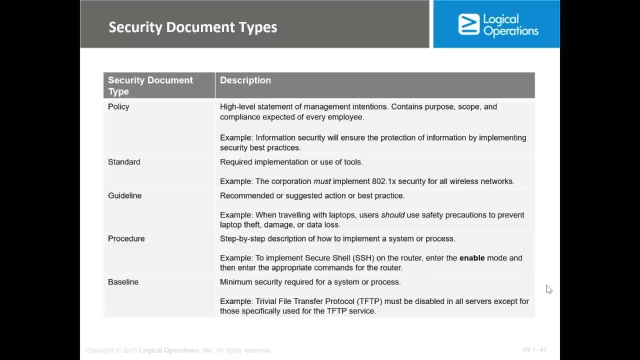 So the standard is something that you should refer to when you are creating the policy. guidelines is more as an optional. I mean you should follow the standard when you're creating the policy because it has to be followed, but guidelines is more Like an option. 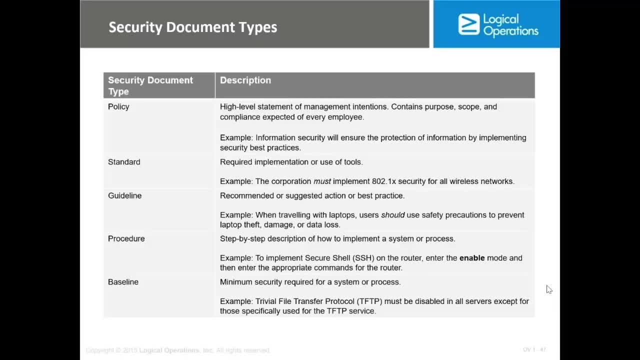 So, for instance, standard could be that the password should not be less than eight character. You should follow that when you are creating a policy, but maybe the guidelines will tell you that 10 will be better or 12 will be better. You can follow the guidelines, except it's not really mandatory. 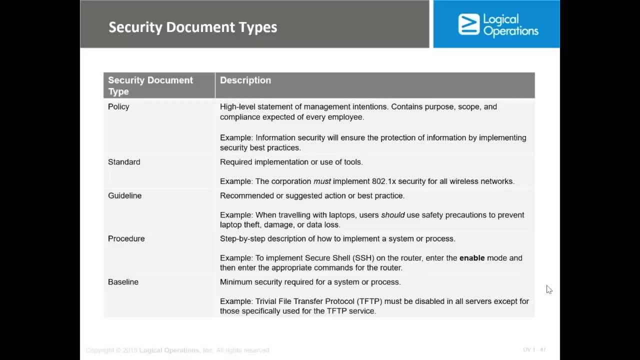 It's option. Procedures is the step-by-step process, in the sense that when someone is joining the company, how are you creating the email? So you have, You have a flow chart that showing that you receive a request from HR and approval from security team that this guy signs the contract. 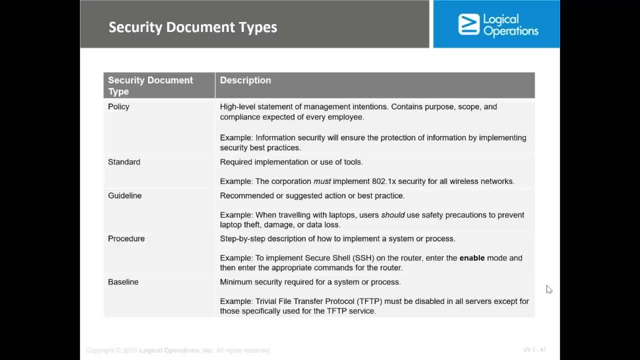 He signed a non-disclosure agreement. He did that. So you create, you forward this request to the technical team, to the, to create a email for it. So it's showing you step-by-step how things is done. So policy is more general work procedures is step-by-step guide. 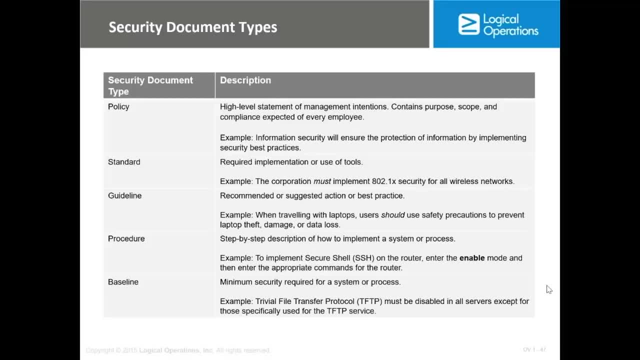 And I will share some of those document attached to this lecture, just as a guidance. Baseline is the minimum acceptable security in a sense that, for instance, if you buy a new computer and you're going to join this new computer or laptop to your company network, 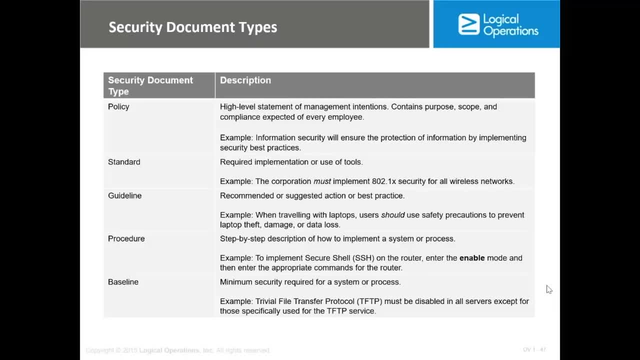 What should you do? first? You should remove access to the USB. You should remove the unused services. You should install the latest patches. You should do this So you have a checklist For any computer. you cannot attach any computer to your company network. 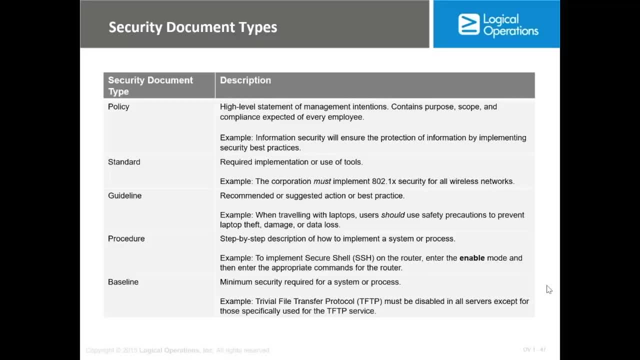 Unless this checklist is fulfilled. This is called baseline, So most probably he will give you a question about a specific document, Like: what document should include the step-by-step implementation procedures, or high-level statement is a policy, So it's very, very important, not just for the exam, but realistically it's very important also to be aware of. 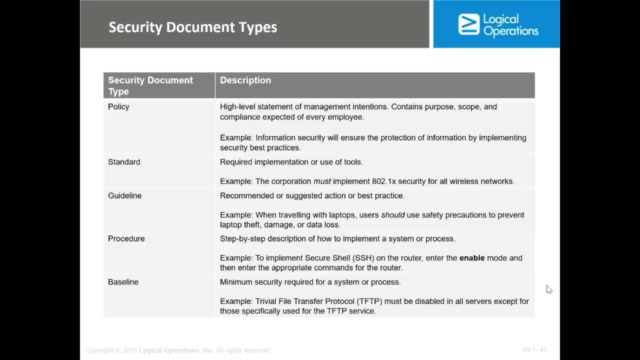 What kind of policy any company should have. I already, like pointed to a very good website from where you can download those template and use them, But also I'm going to attach few of those documents in this lecture that will help you identify how the policy look like, or the standard or guidelines and so on. 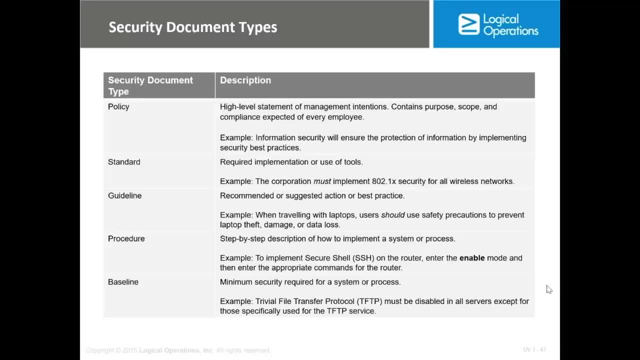 And again, it's not just to have them, especially the policy. I keep repeating that because it's quite important, because I saw in very, very many interview that auditor will come to any of the company employee or user and ask him: Do you know that you have a policy in your company and many people didn't know about it. 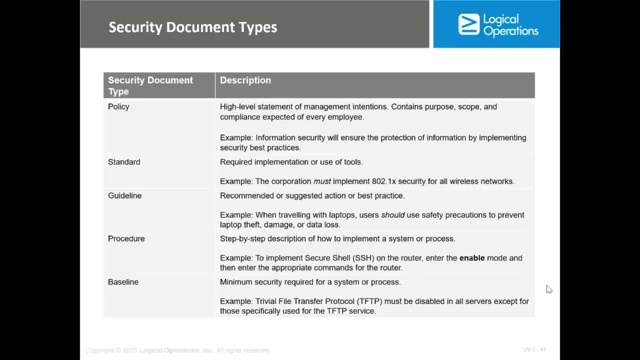 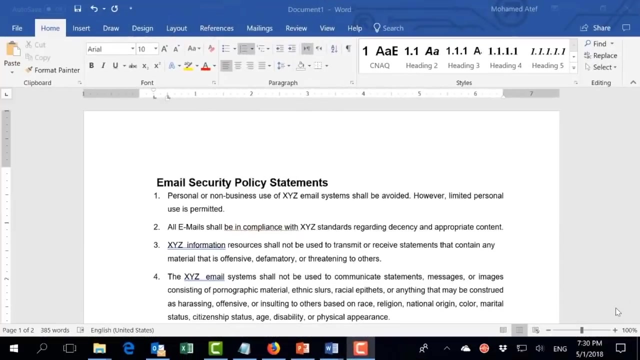 So you, as a security team, you get a part of the blame because of that, because you should inform the user and the employees that we have information security policy related to all our services and assets, And it's located in this Specific location. Let me show you a sample for a policy. 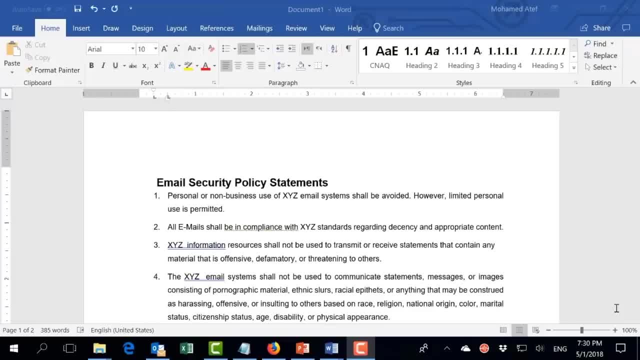 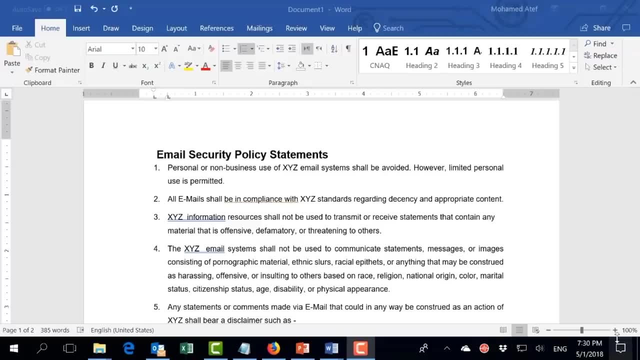 Now, This is an email security policy. As you can see, a lot of common sense statement is there, like: personal should use the email for business. It should not be used for personal use, You should not be using any offensive Email, and so on and so forth. 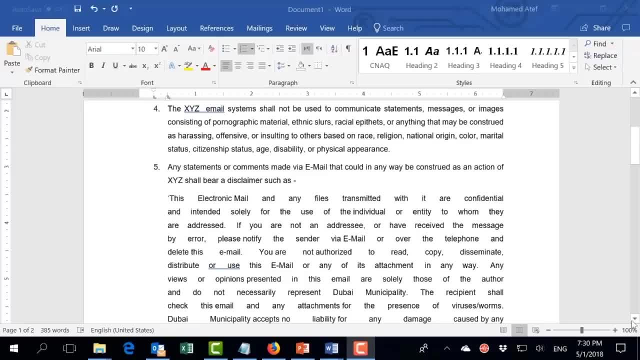 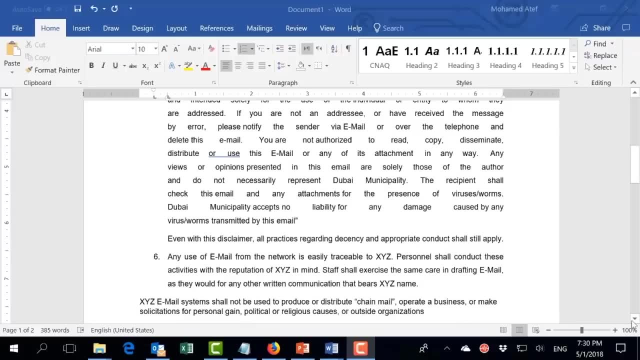 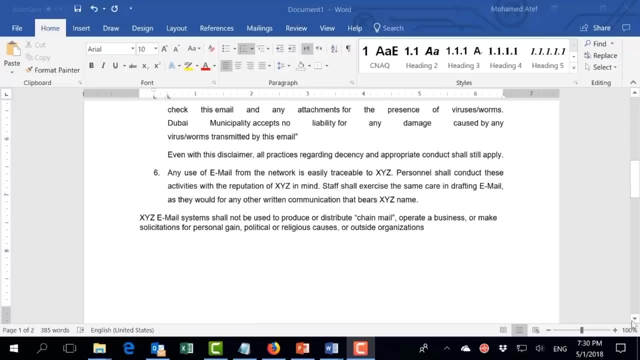 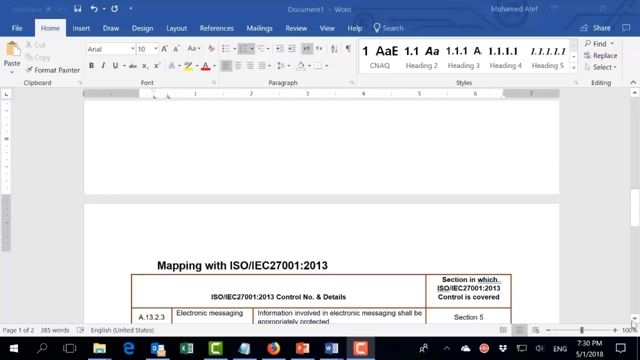 So, as you can see, The email policy, it's common sense, but it's not important about the policy itself. The important part of the policy, It's to map it with a well-known framework or standard that you are following. This is extremely important. 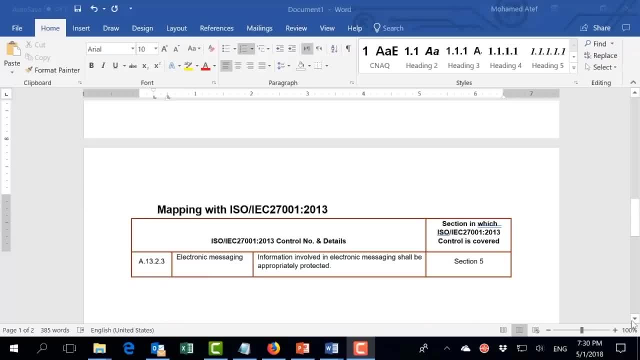 So it's not to have As much policy as you can, but you should have a policy that match or that map Different system or standard or framework that you are following. So here this policy: It's a part of the ISO 27001 and you have to specify which control. 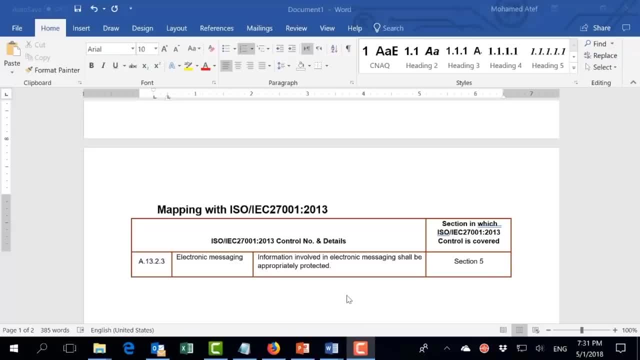 And what is the name of this control? So this one was requested or it was a requirement from ISO 27000.. This is the number of control and what was the control name. It was the electronic message and this is the statement that was required. 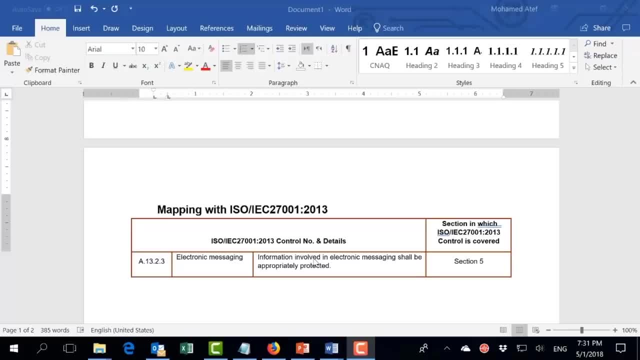 So my point here is that when we are doing a policy and procedures, It's not just to have a policy, download them from the internet and then use them in your company. This is not the right way. The right way is to check which framework you are following, or which standard you are following, or which regulation you are following and doing a policy that fulfills. 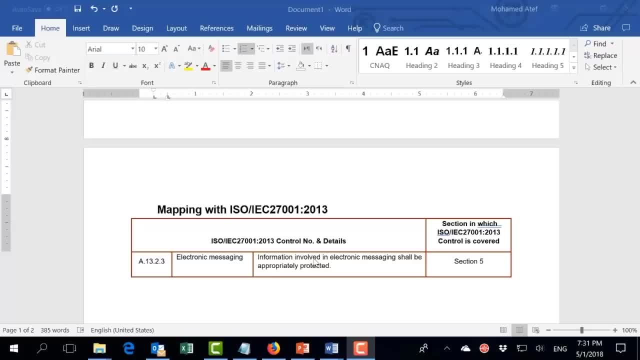 This requirement and, accordingly, if you get an audit regarding this framework, you can show them that, regarding this control, We have a policy. Now what will be remaining is to show them an evidence that user is aware of this policy. So I wanted to show you a part of a policy just to indicate or just to clarify what is what should be mentioned in the policy. 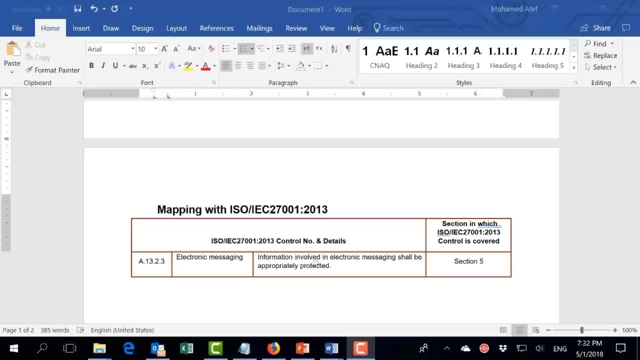 Now there is other part that I will Share on the student port, and I'm going to put a lot of like policy templates beside. I already showed you places from where you can get policy and procedures, But my point is The policy format. 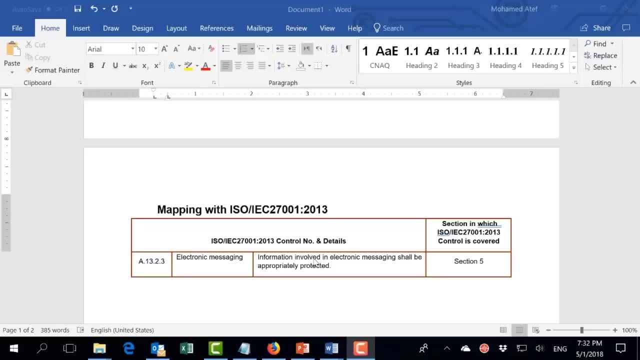 It's well known. You have a document- controls, and you have the scope of the policies and you have the policy itself. Then you have, like the, if you have any exception, and then, which is very, very important, Mapping The policy with the framework, because, as I keep saying and I will keep saying that, that information security 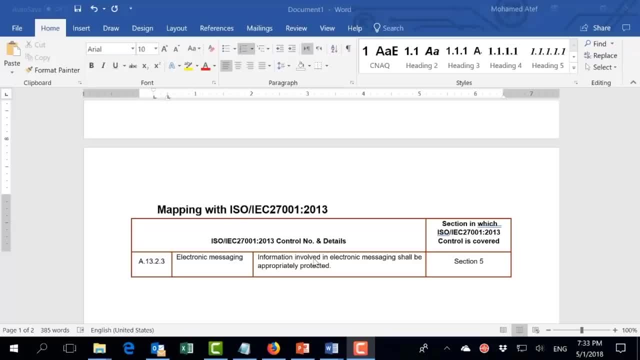 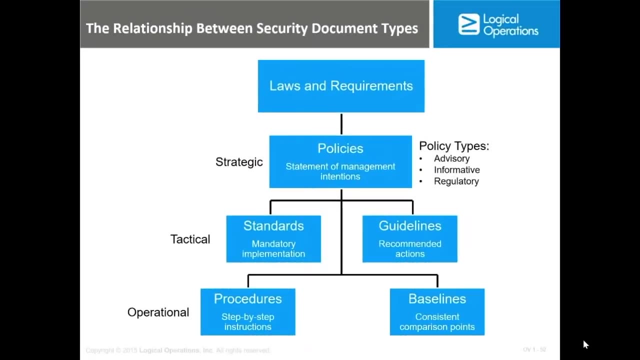 It's not a field- Well, you should try or ask people what should be done. It's just a field where you are following the best practice or standard or regulation. Before moving to the next topic, Let's discuss the relation between the different security document. 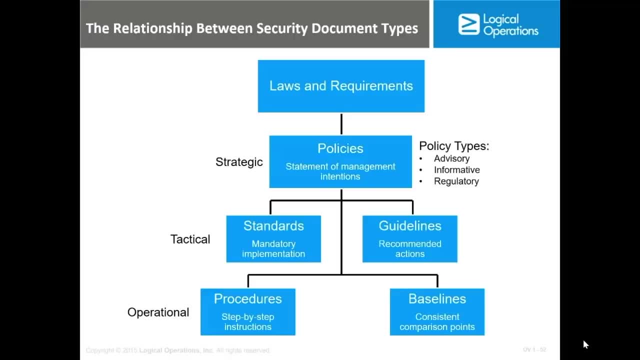 In a sense that from where should I start from creating a security document from any or for any organization. from where should I start? And definitely I should start, as it showing in the following chart, from the law and requirement. So usually you should know what is the law and regulation related to your business, as we mentioned earlier, and according to that, 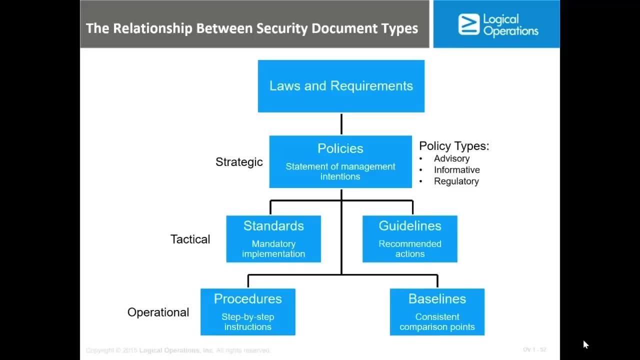 You should create policy which don't forget policy. It just is a statement of management. So, for instance, if you are following PCI DSS or if you are following ISO 27001, where there is a requirement for an or a domain for an access control, 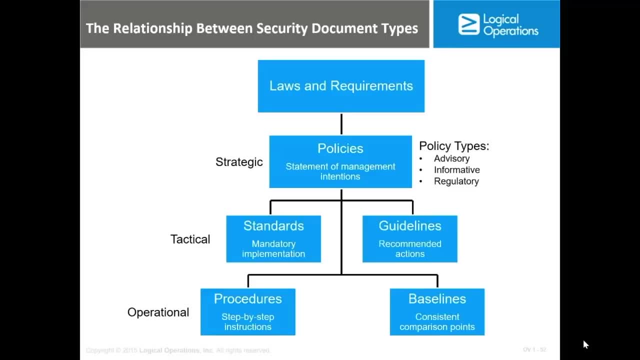 So you should have the policy related to access control and management will say that that we need to have a policy related to access control And from the policies and we can create the standard and guidelines and procedures and baseline and so on. So the point here is that we usually start from the law and regulation. 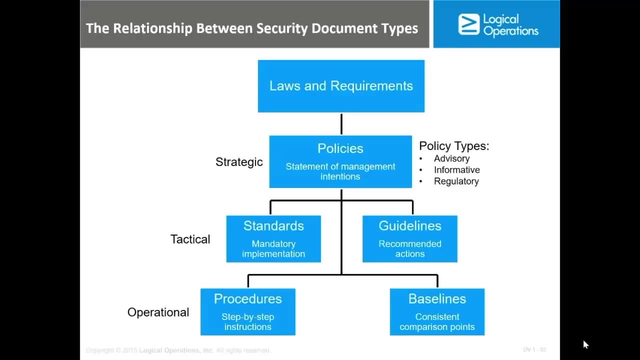 It's not just by creating a huge amount of policy. It should be mapping different kind of stand controls into standard and framework. This is quite important, as I showed you in the previous lecture. Also, we have different kind of Policy. we have a regulatory policy. 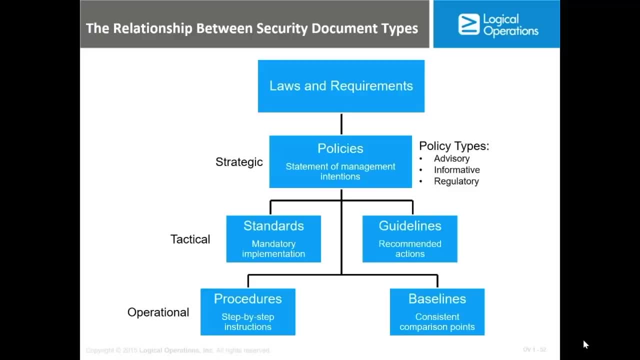 This is that should be done according to the law. We have an informative policy. We have advisory policy, things like for instant social media policy that you should not use or should not publish personal information or work information on social network. It's more into advisory. 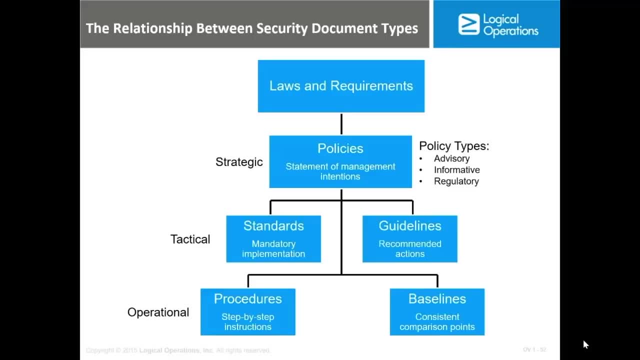 It's not like if you break it- actually if you break it against the law- but some of the policy will be more into the advice part, But some of them will be more into the compliance part- that if you break the policy it's against the law. 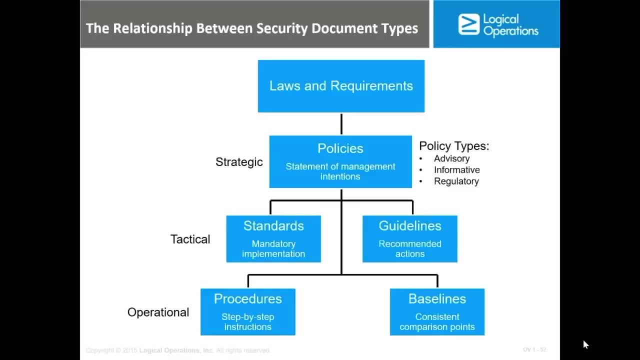 So even in policy we have different type, then, from policy We are creating the standards, the guidelines, the procedures and the baseline which we already explained in the previous lecture. So this is a relation, and what is quite important is from where we should be start. 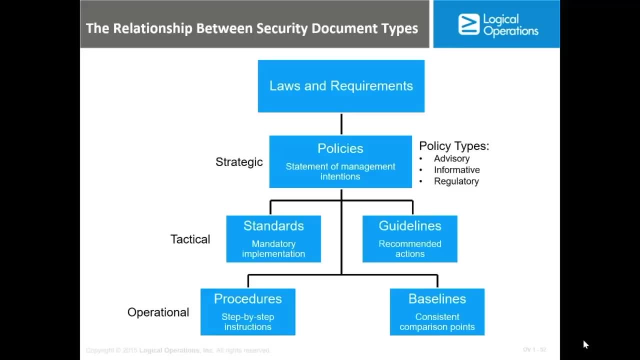 So, if we are following ISO 27001. Which we have different domains, for each domain, We should have a policy that maps The control required in this domain. This is the right approach. If you are following PCI DSS Also, you need to create policy that enforce the control in this standard, and so on and so forth. 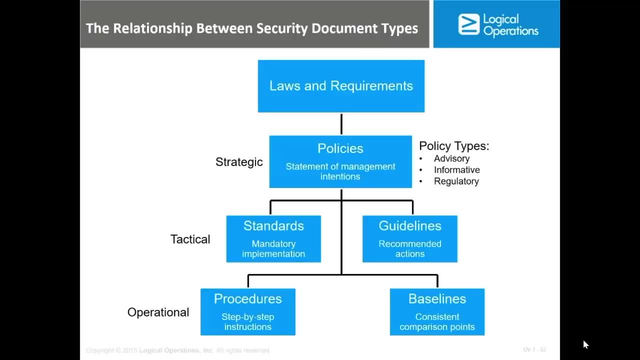 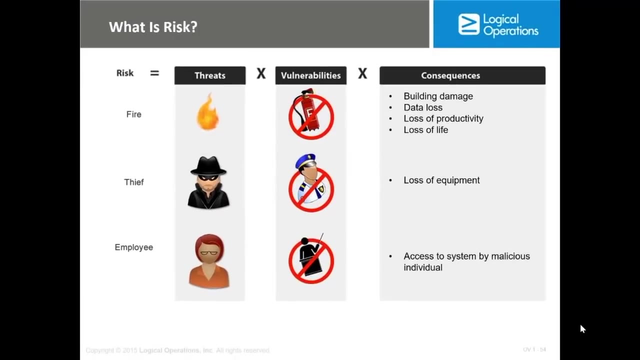 So this is the proper approach for creating a policy and procedures and guidelines- All of the security document needed for any organization. This is a very important topic in our course, which is risk management, and it's not just important for the exam purpose, But actually as a security specialist, you need to understand the risk in a very deep way. 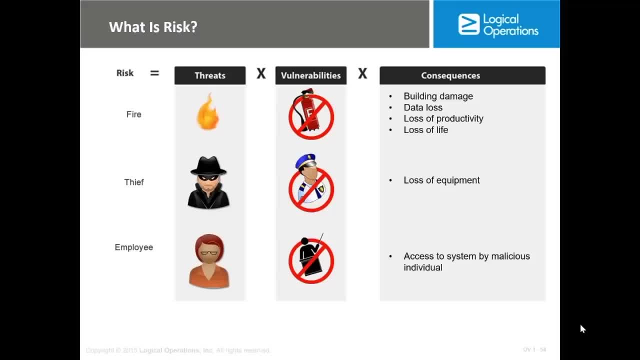 You need to understand what is risk in the first place. Then, what are the risk mythology, risk assessment mythology- How can I do risk assessment? What is the risk management strategy? What is the residual risk? It's very, very important, And not just for the exam, but also, I believe, if you attend any interview, this will be one of the main questions that you're going to get. 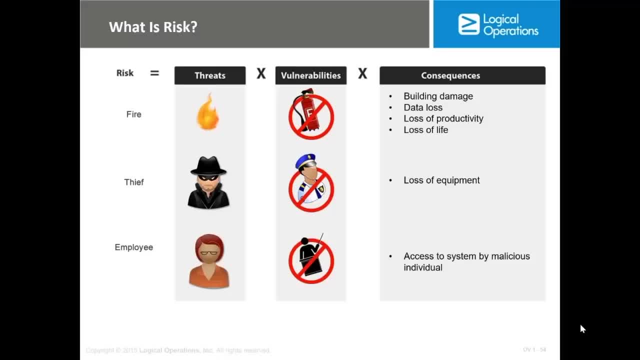 They will ask you about risk in a different way. So it's quite important to understand the risk. That's why I'm planning to give you a lot of lectures related to risk- even deeper Then the course content- just to let you very familiar with risk. and let me explain to you why. 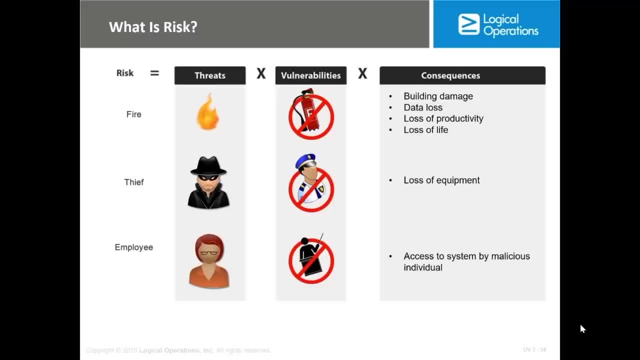 If you get hired somewhere and they ask you to implement security in their organization, from where should you start? I know we already mentioned that you should start by checking the regulation and law and so on, But even so, from where should you start? or let's take it in a simple way: if you need to implement security in your house, if you need to, 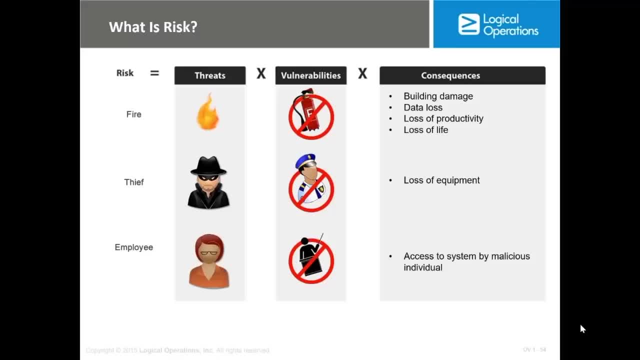 secure your house. From where should you start and what will be the factors that you're going to consider When it comes to spending on security? how much you're going to spend on your house? If you need to like secure your house, what should you get? 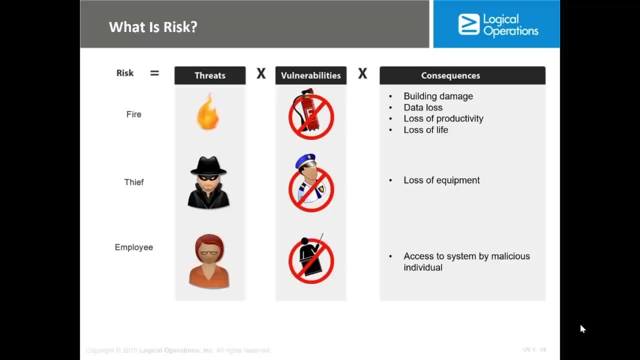 Should you get an alarm system? Should you get like a security guard surveillance cam? How much you willing to spend It depends. It depends on two different factors. First, It depends about what do you have. What are you securing? I mean, it doesn't make sense that you spend $10,000 to secure your house that have some assets that worth $2,000. 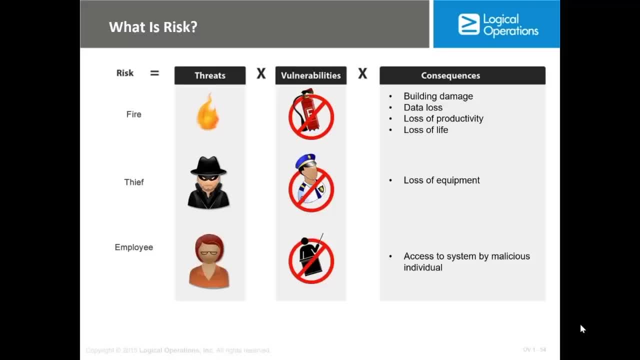 You should not spend 10,000 to secure 2000, right or wrong. The second point is the risk that you are facing. So if you are in risky or bad neighbor, maybe you're going to spend more that if you are in secure area. 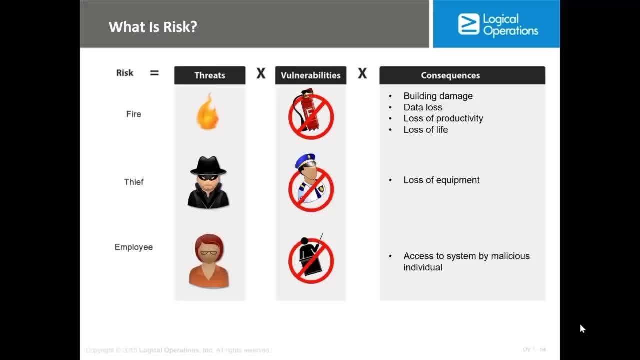 If you are located in a place where there is a lot of earthquake, there is a lot of tornado and the weather's problem, maybe you're going to spend more because actually security is not just against hacker and malicious hacker. You are securing against any kind of threats- fire, tornado, anything that may lead to losing your. 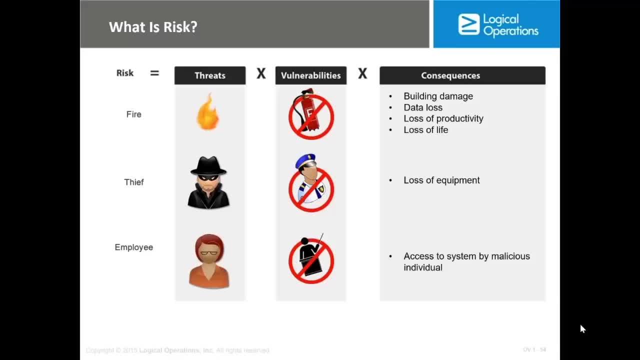 assets. So the first point is the value of the assets and this will be explained in depth in the next domain. Second point would be what risk You are facing. So if someone is living in like secure neighbor, definitely he will not spend money same like someone. 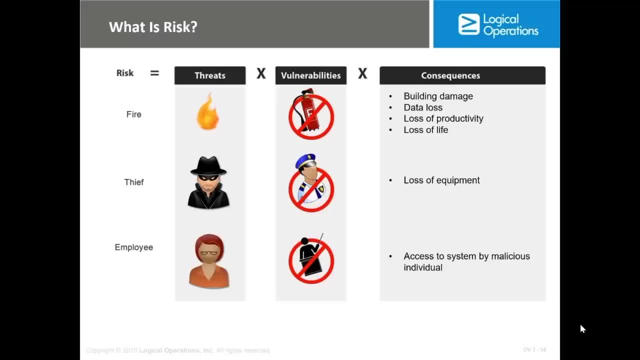 who are living in a bad neighbor. So risk, allow you to first consider how much you're going to spend on security. This is one point and we're going to see that in the next lecture. Secondly, what is the priority? So, if you are a very 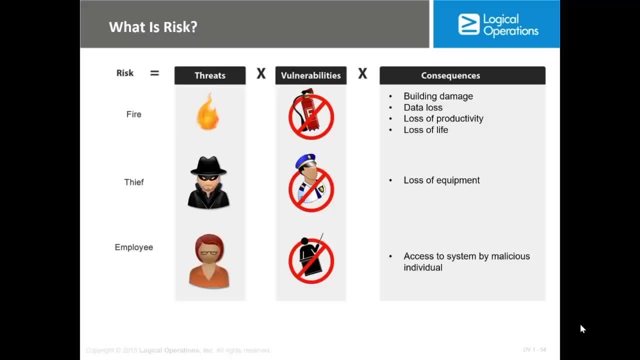 Located in a good place where you don't have any kind of earthquake or tornado or floats or so on, you will not spend money on devices, or you will not spend money or for something to prevent that. because you don't face this kind of problem, Maybe the probability of happening is very low. 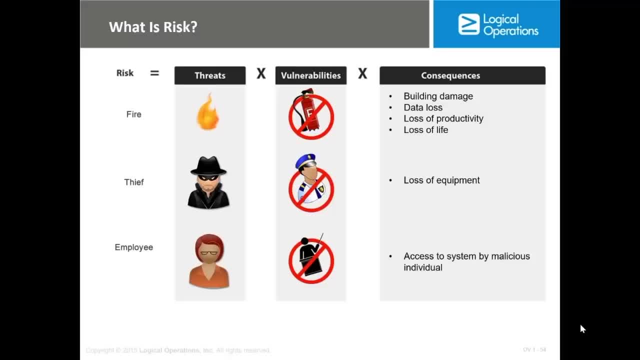 The earthquake is happening one of every 50 years, So I should not buy any things to secure my home or my company against earthquake, for instance. So it's quite important to understand risk. So first let me explain what is risk. We already explained at the beginning the threats and vulnerability. 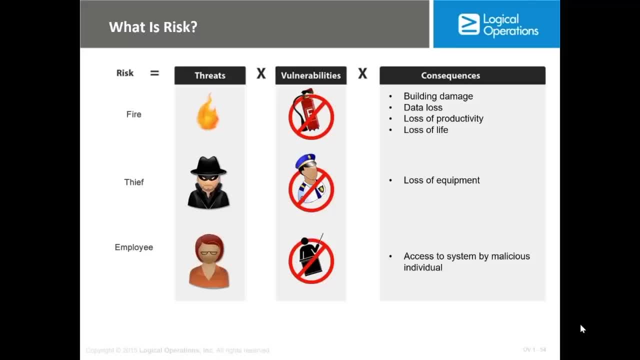 So what is a vulnerability? as I told you before, is a weakness. So if I don't have a firefighting equipment, this is a weakness in my company. What could go wrong? a fire may happen, which is a threat. Okay, because of the vulnerability and the threat, what could be the consequences? 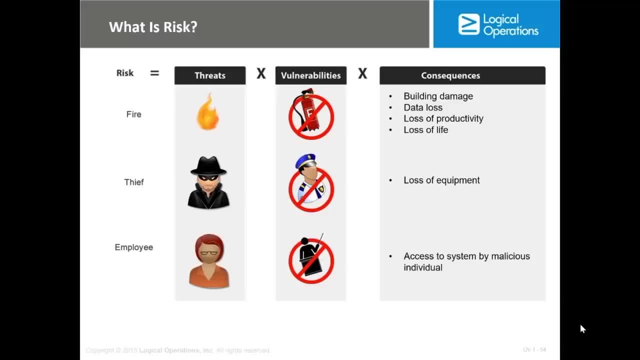 I'm getting damage, I can lose data, I can lose productivity, I can lose life because of that. This is the risk. the consequences of a threat multiply vulnerability. By the way, you can learn how to calculate risk, because it's quite important to calculate risk. 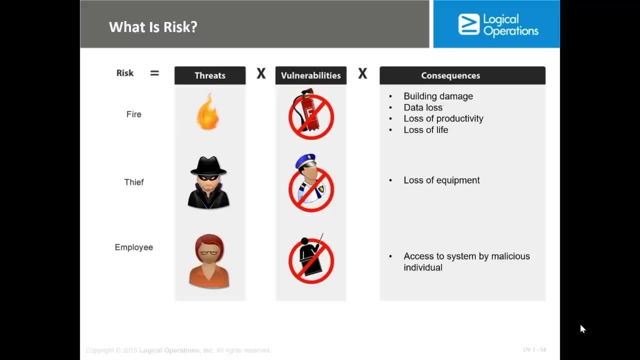 So you can know what is a priority, What is a higher risk than what is lower risk. If you don't have a security guard, what do you consider that? a vulnerability, weakness? What could go wrong? A thief or someone could break in. 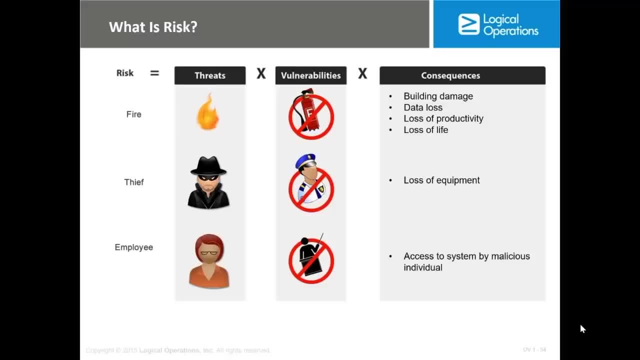 What It will be the consequences of that- lost of equipment or lost of data. This is the risk, and so on and so forth. So this is the definition of the risk. now, in the upcoming lectures, We're going to first explain this in like a deeper way. 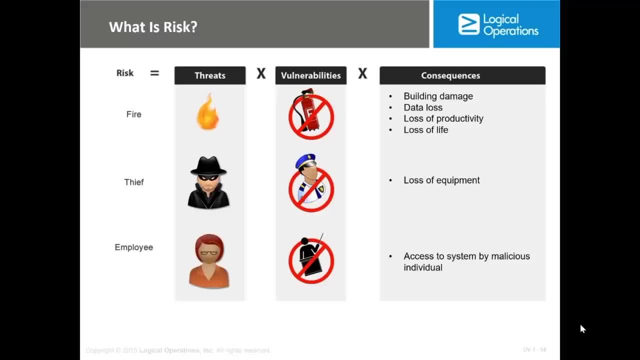 We're going to talk about the framework that we are using to do a risk assessment. Then I will show you a couple of risk assessment tools, because actually doing risk assessment is not easy. Even I see square recommend to use an automated tools because it's not easy to keep thinking. 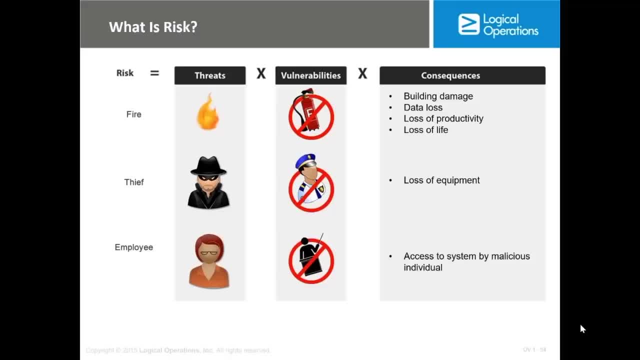 about everything that could go wrong and what would be the consequences of that. you know it needs a lot of experience to do that. So after explaining the risk, I will not just depend on that to explain the risk, but also I'm going to add a couple of video, first showing you a couple of product like: what are the risk? 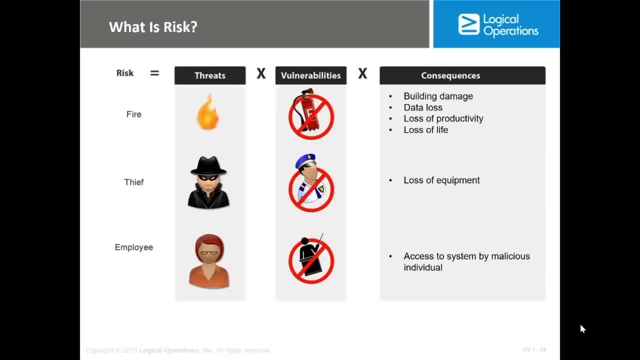 assessment products that you know, because usually we are doing, According to a couple of survey which I will share, on the student port and sit with people and give them survey and according to that you can understand the risk beside. you are using a lot of templates, but there is some products that you can use to do a risk assessment and 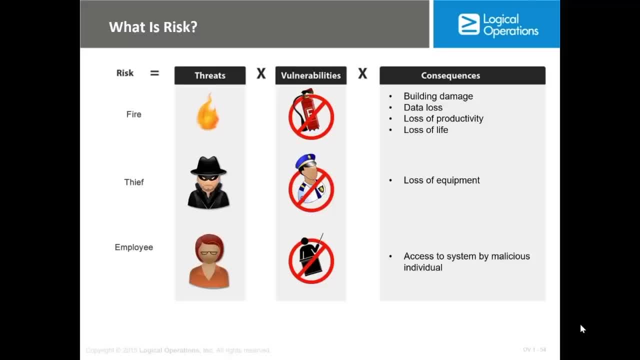 it will give you better result, because if you mitigate risk- which you're going to explain in the next lecture- which mean you are like working on or spending Money to decrease the probability of happening, This will be a good approach. But the point is: 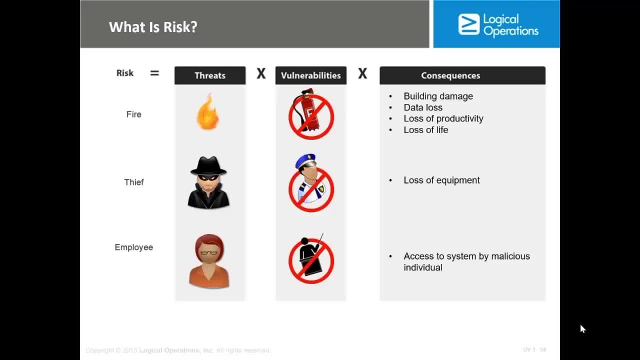 After explaining the concept, I will also utilize or explain the. it's not advertising for anything, because those are not cheap products, but at least you need to know what is in the market. And, by the way, if you need to get the best of this course, do not just depend on the lectures. 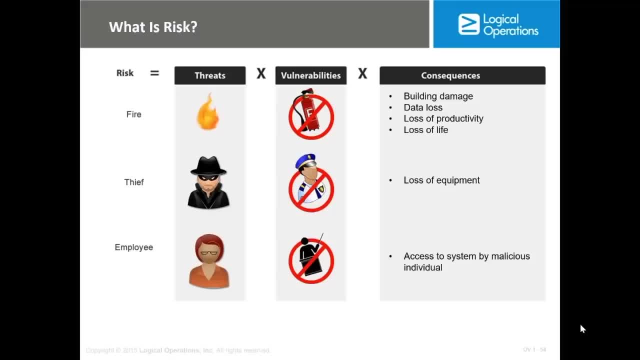 and the knowledge you are getting from the lecture. But, for instance, if we are talking about risk management And we are explaining that you should do some research, What are the best products that do risk assessment? What is the difference between those different products? 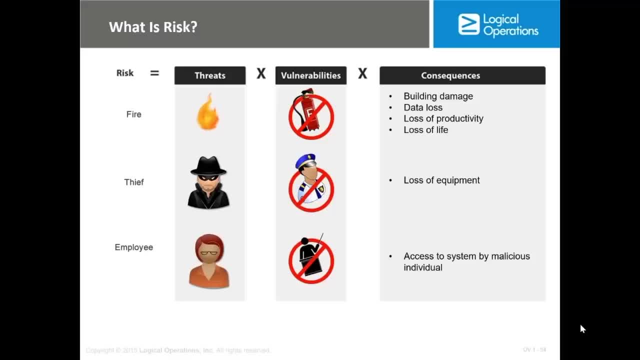 Because if you go to an interview, He may be asked you about definitions, but he will also ask you about what is in the market today. That is doing that: What is the best DLP, What is the best Chris, assessment tools and so on. 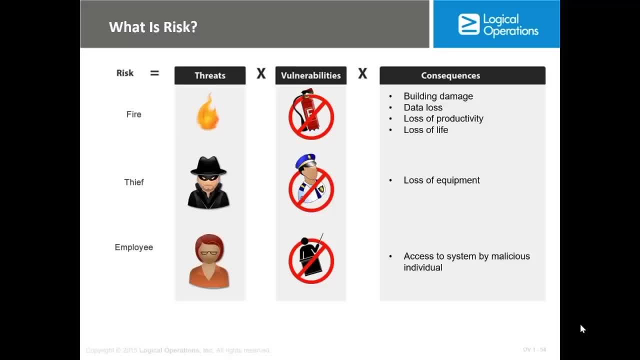 So I strongly suggest that you keep a piece of take notes about the knowledge And, whenever you finish a subject which is quite important like risk management, I also suggest that you go and search for product. that doing that just to be familiar What is in the market? 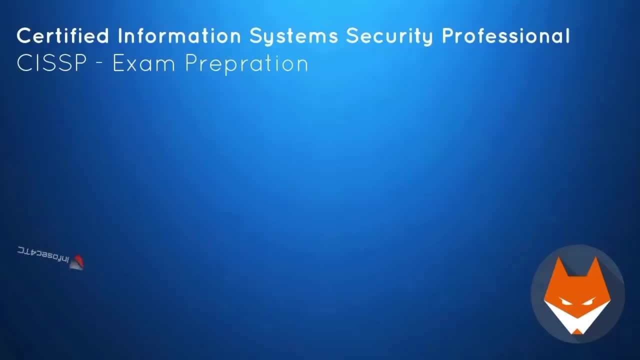 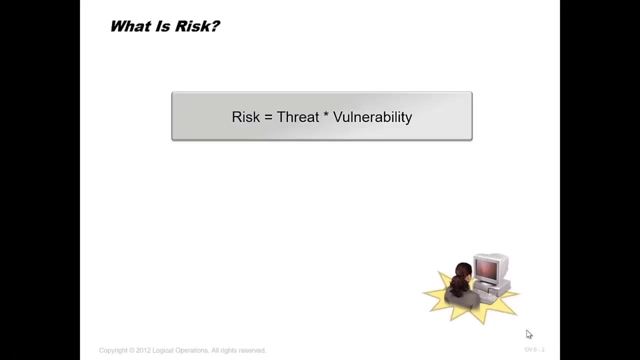 Not just to get the theoretical part. So risk it's not a threat, It's the damage that may happen if a specific Weakness or threat has been exploited. That's why usually we have two formula for risk. It could be risk equals threat into vulnerability or, sometime, risk equal probability into impact. 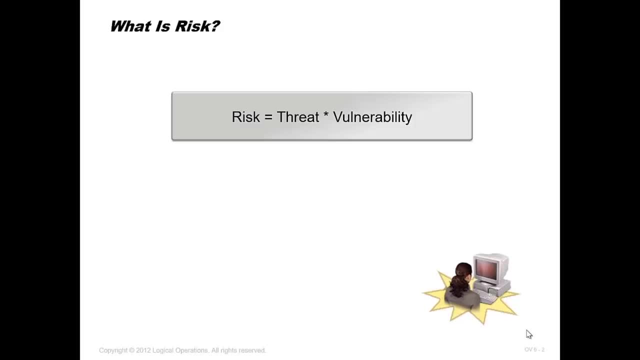 So if we have a specific risk, vulnerability, That or weakness that has a probability of happening 10% and if it happened it will cost us $100,000.. So the risk will be 10% into 100,000, which is 10,000. 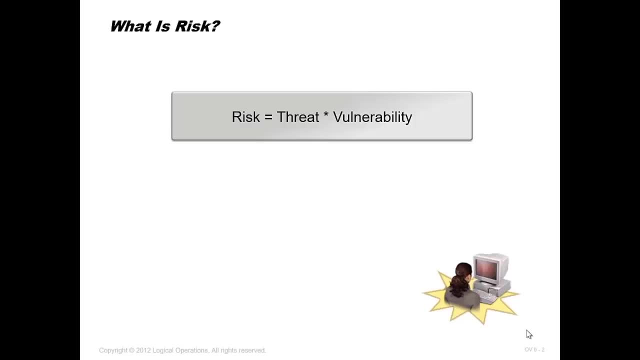 This is how to transfer risk as a number And, by the way, risk management. It's the only module or the only domain inside the scores that has some formula that you need to memorize, and we're going to see that during This domain. 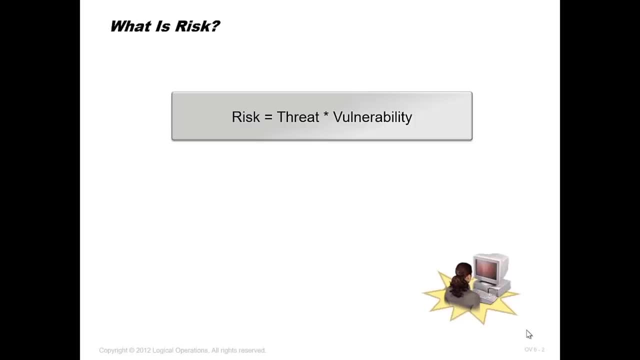 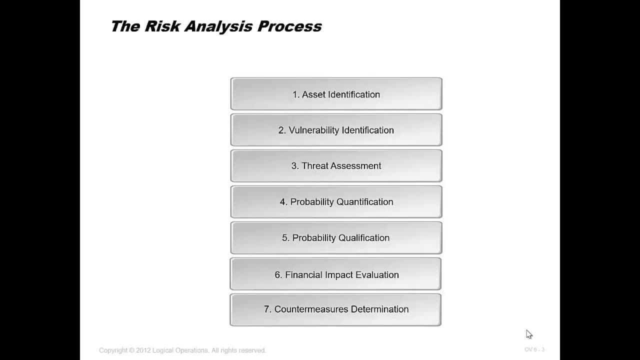 So risk is the amount of lost or amount of damage that happened If a specific vulnerability, if a specific threat has been exploited. Now, as I told you, security approach used to come from the risk itself. So, if you like, get hired to implement a information security management system or any kind of security. 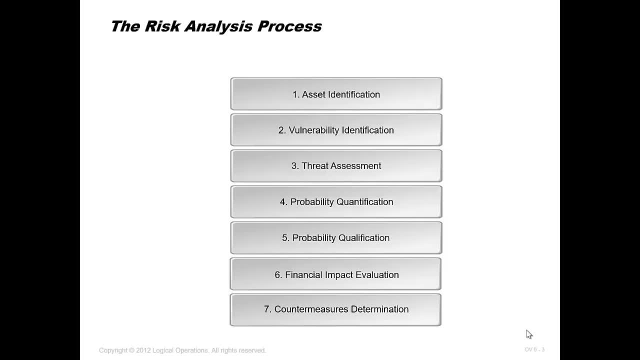 Implementation in any organization. from where should we start? So, as soon as you get hired and a bank or a company ask you we need to implement some security to secure our information, from where should you start? Should you just tell them: Yes, we're going to buy the latest and the greatest equipment and appliance, this and by doing that, this is how will be come secure? 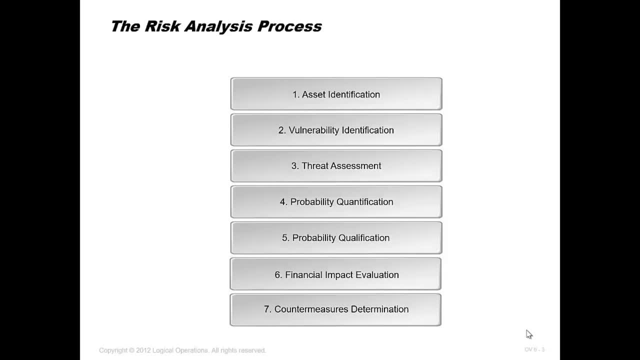 No, it's not going this way. There is a risk analysis process that you need to be aware of, So it should start by assets identification. What do we have as an assets? What exactly do we protect? and assets actually do not mean only shares and computers and tables. 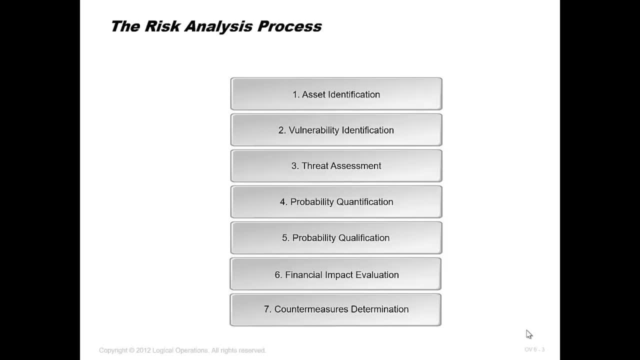 But there is some assets that is more costly than that. Like the company information. This is an assets. Can you tell me a bank, a huge bank, the information that he have, how much it worth If there is a bank and has a lot of customer information and the financial transaction and all the financial information? 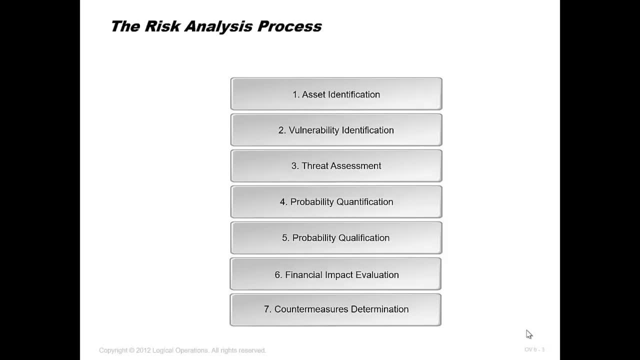 How much do such information worth? What if those information get compromised? What will be this bank lost, right? So you need to start by identifying the assets, and not just the physical asset, but also the non-physical, as company reputation As an assets, what exactly it represent if we have a big, big companies that if you get compromised, no one will trust it anymore. 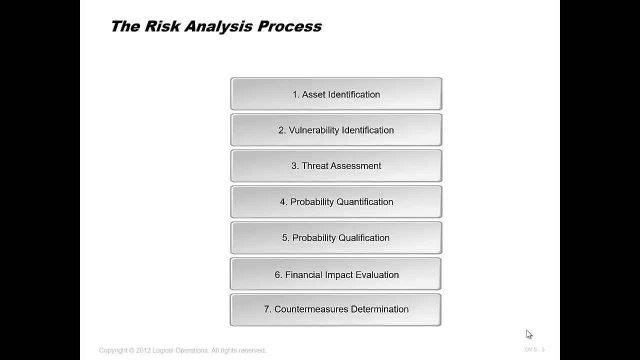 And we saw a lot of stories the last few years about majors company that people lost confidence because they get compromised more than one time. This is an asset that has been lost, So we need to identify the assets first, Then we need to identify the vulnerability or the weakness. 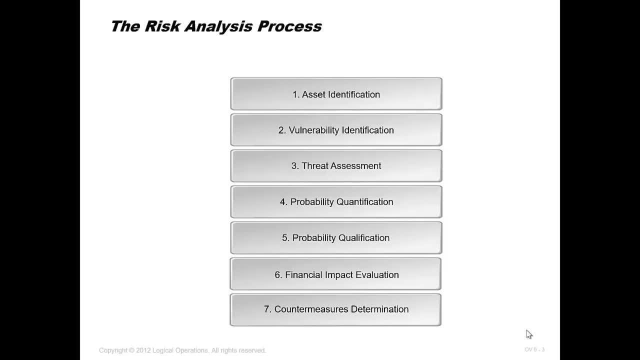 What weakness those people have, what A vulnerability they have. Those vulnerability could be technical vulnerability. So, for instance, they are using some old operating system, some legacy system. Their website is not HTTPS. Those are vulnerability, And then we need to identify the threat. 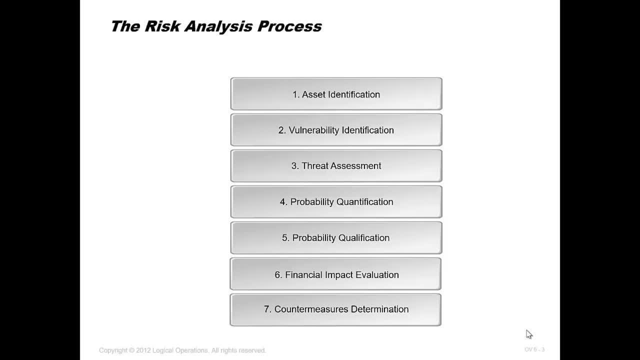 Can those vulnerability be hacked or exploited? I mean, I may have an open port on my computer- This is considered a weakness of vulnerability- But this open port doesn't. I don't have any service, So no one can hack it, So I don't have a threat for that. 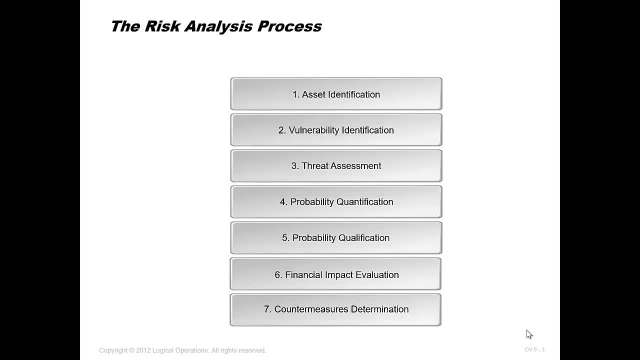 So I should identify the vulnerability and then check which vulnerability has a threat associated with which vulnerability can be exploited. Then, number four, we need to do four and five: probability, quality, probability, qualification and quantification. Now, qualityfication mean based on quality and quantification. 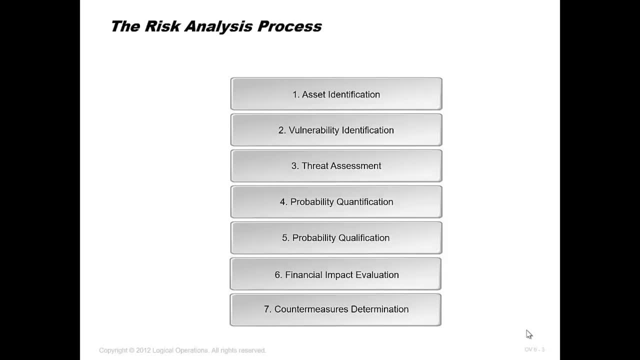 Based on quantity. The point here is: okay, We are identifying the vulnerability and we are identifying the threat. What is the probability of this specific threat to happen? For instance, let's talk about fire as a weakness. So we are working in a company. 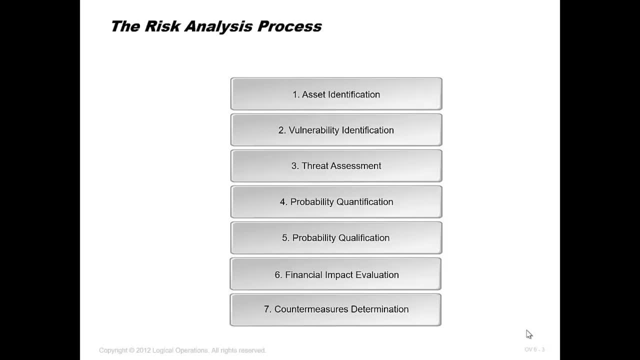 We have a lot of electrical equipment. We have a data center. We have a lot of electrical devices. A problem may happen. A fire may occur right Now. this is a vulnerability: The threat that a fire may occur because of that. 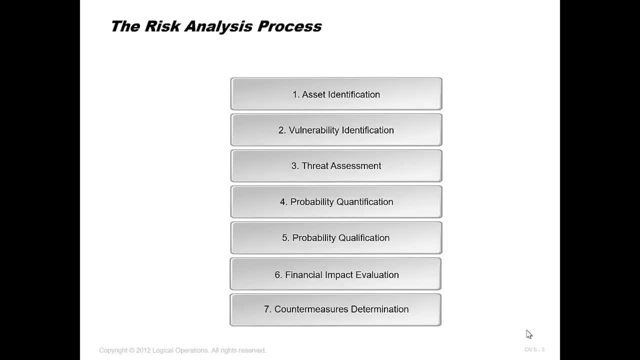 Now, what is the probability of that happening? I may have some previous information. I mean, I notice like every 10 years a fire happened. So this is called the quantification. It's based on quantity because I have figures, I have number. 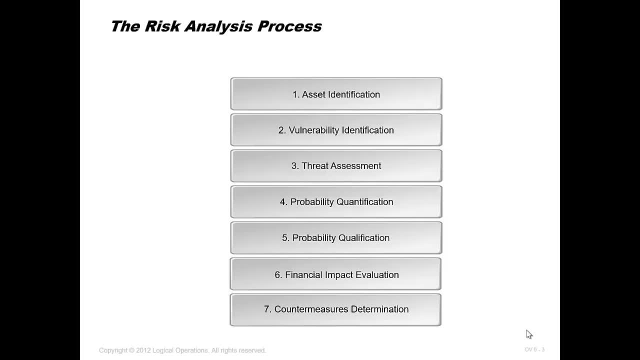 While if we are talking about qualityfication- mean I'm assume based on other people experience bit, So I don't have a solid background about that- Then we have to identify the financial impact and actually going to do all those process by some formula later on in this domain. because after all, if I'm expecting to have a threat to like a fire, 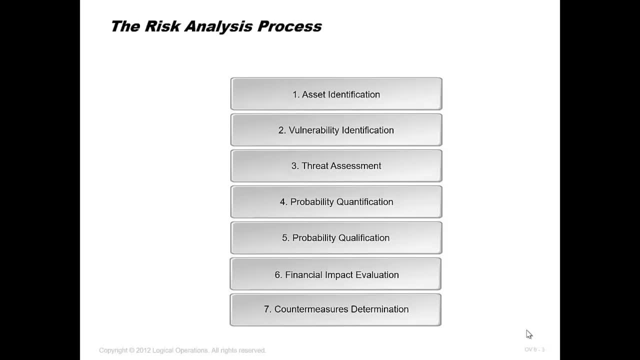 Okay, so if a fire occur, What will be the amount of loss? I need to evaluate the financial impact because according to that I'm going to decide- and this will be done by numbers within few lecture, I'm going to decide- how much I'm going to spend on this specific impact. 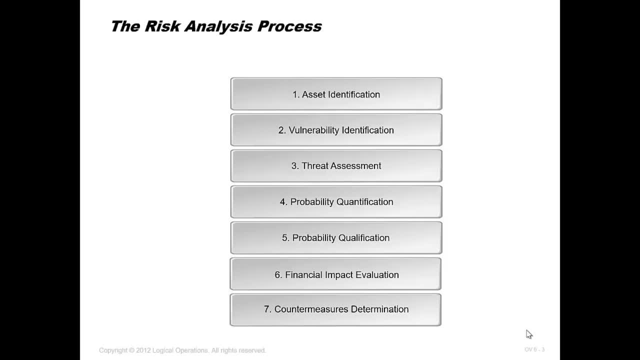 So we are saying for instant That if a fire happen it may cost the company 100,000. So I need to buy equipment that works Less than 100,000. doesn't make any sense that you know if a fire happen and my lost will be 100,000. 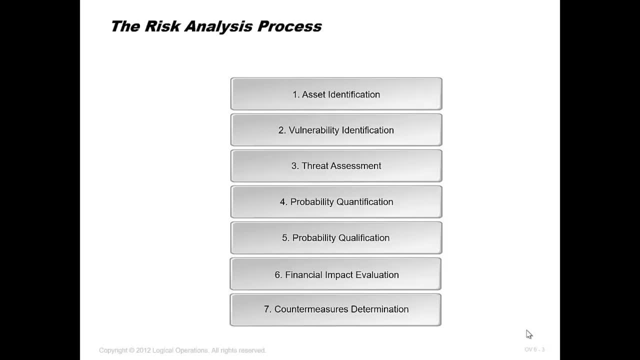 I will buy an equipment with 10,000, with 1 million dollar. So financial impact because you have to do a cost-effective solution and this is how you'll face the questions as exam, They will not ask you how much you're going to spend. 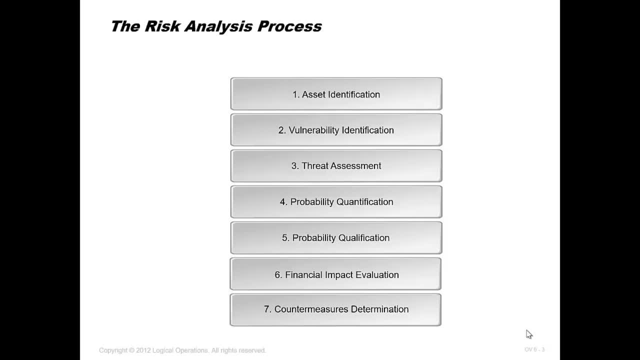 They will give you a scenario and they will tell you they spend that much on this specific threat And is it cost-effective? So you have to calculate and you have to see the asset value and you have to see how much is the loss and then you have to see how much they spend and according to that, 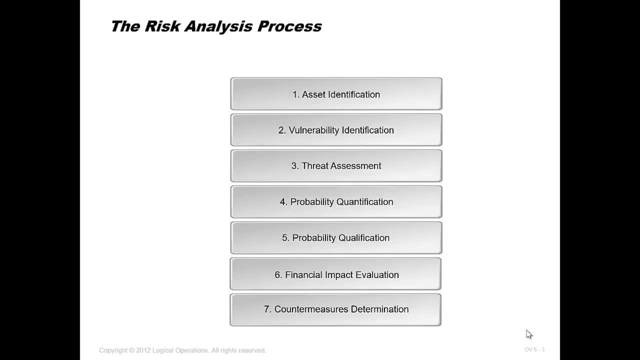 You decide if it's effective or not. And finally, in the risk analysis process, you need to determine the countermeasure based on the financial impact and also the risk itself. I mean it should reduce the risk of happening. This is one of the framework. 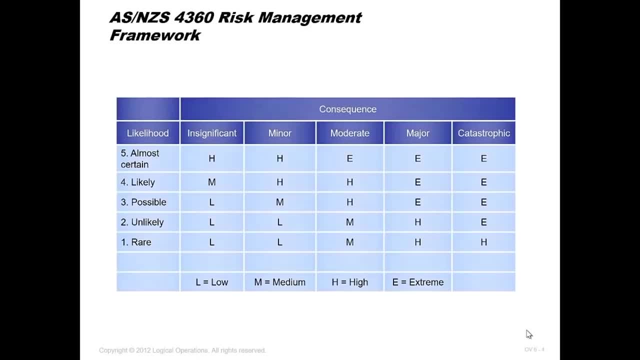 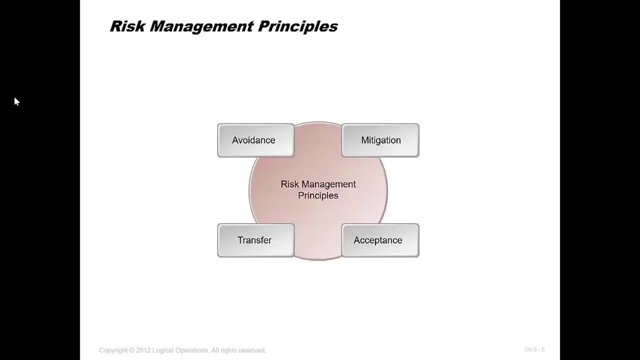 This is related to fire department, something where you know this is how they are doing the qualification, like you know the likelihood, the probability of happen They put value and the impact they put Insignificant, minor. This is qualitative probability. Now, when we do a risk assessment and we start identifying the threat and vulnerability and financial impact, 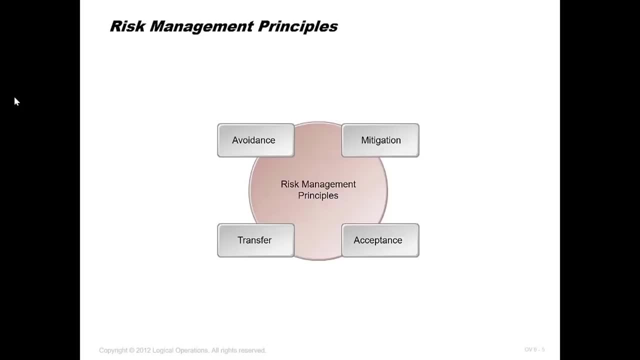 I have four different strategies that I can take. first one, It's to mitigate the risk: mitigation. So mitigation mean I'm going to spend money to reduce The risk. So, for instance, I have a web application that is very important and if it get compromised, this is an e-commerce website. 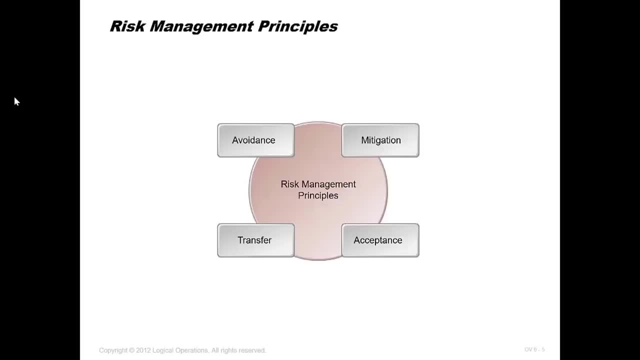 I'm going to lose a lot of money, like Amazon or those sites that they are benefit by, by minutes. So what I'm going to do, I'm going to buy a web application firewall or some appliance to protect my web server. This is called mitigation. 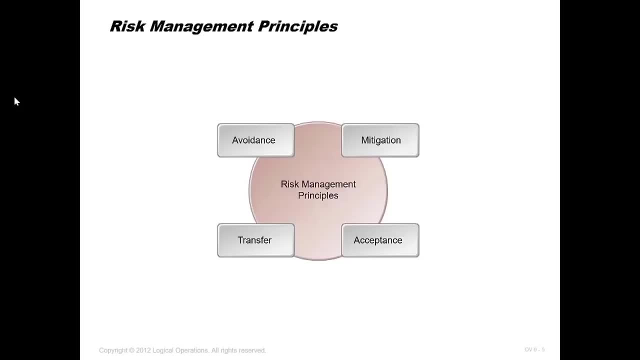 I spend money to reduce the risk. I cannot reach risk zero. I mean risk. Please write it down. risk cannot be eliminated. They will always be a risk, but I try to reduce the amount of risk. So mitigation means spending money to reduce the amount of risk. 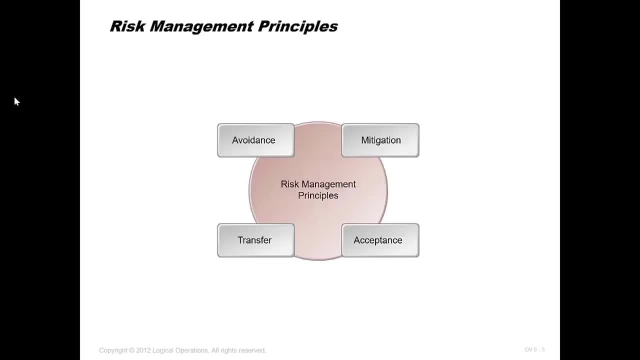 I can accept, mean Okay, I found that to reduce the amount of risk, I have to spend a lot of money and I don't have a budget. So what I'm going to do? I'm going to accept the risk because, after all, risk is an uncertain event. 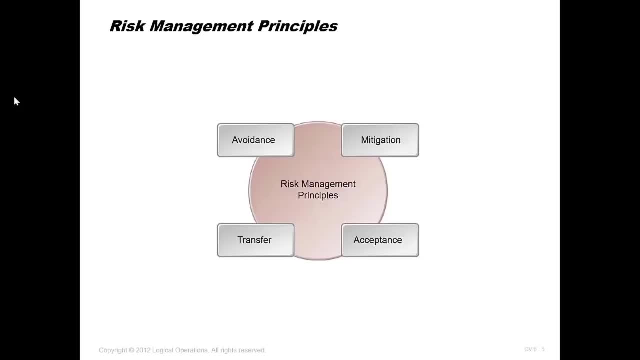 I mean it may happen Or not. So I decided, okay, it will cost me too much, So I'm going to accept the risk. That's mean, if it happened I'll find a workaround, if not good. So accepting the risk mean doing nothing about it. 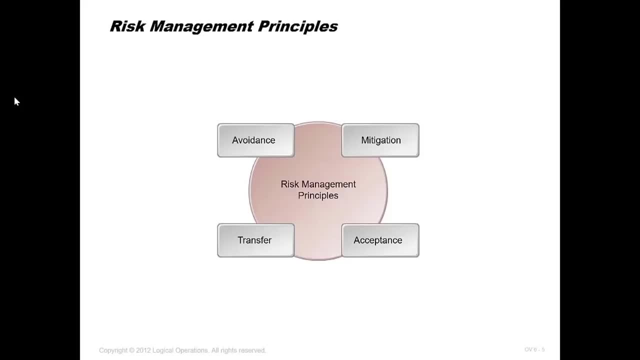 Okay, we have avoidance strategy. Sometimes the risk is too high. So, for instance, we are opening a business in specific areas. It is very, very risky and it has a lot of Like a bad area and people may get hurt, So I decided not to open a branch there. 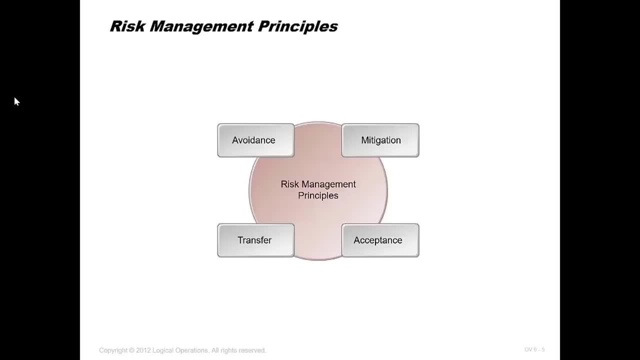 So I will not do even the activity. So it's different than accepting. acceptance mean I'm going to do the activity and if it happens, risk happen, I'll find a workaround, avoid. I will not even do the activity because the risk is too high. 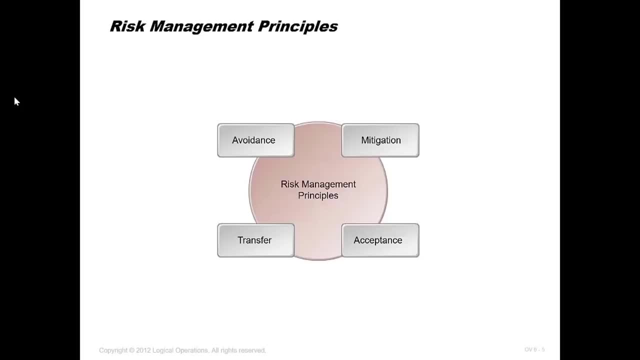 And finally, we have transferring, and transferring mean we are remote, transferring the risk to someone else, like insurance. Instead of buying fire equipment and so on, I'm going to buy insurance policy. If fire happen, they will be paying for the risk, Not me. 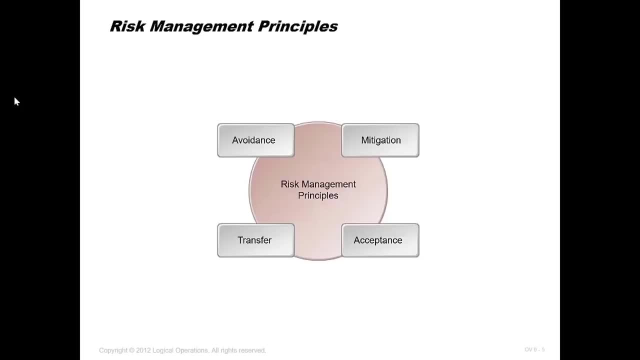 This is called transferring risk. Very, very important to understand the strategy, The fourth strategy. So not all risk can be mitigated because after all, it will cost you a huge amount of money. So some risk will be accepted, some risk will be transferred somewhere else. 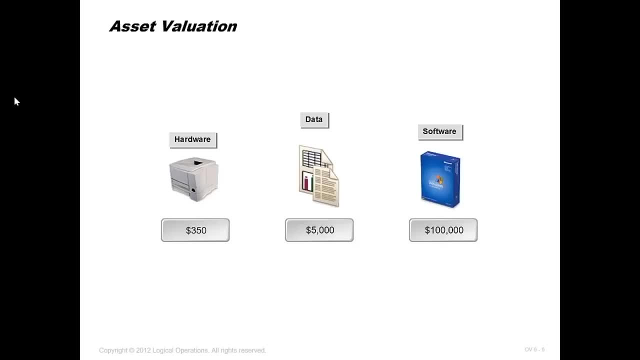 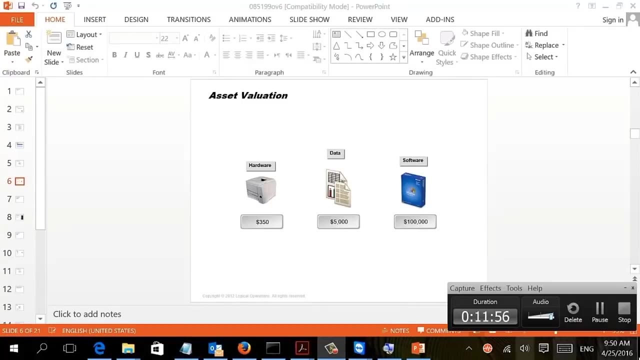 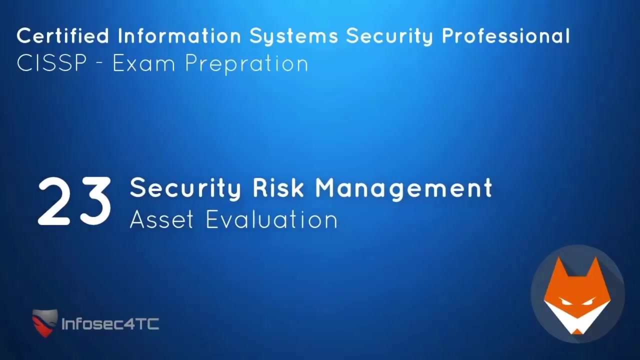 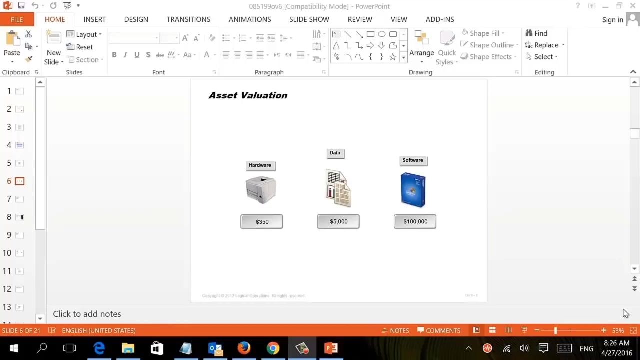 Some risk may be avoiding. So it's very important to understand the different risk methodology. This lecture, It's very important inside this domain, which is assets evaluation, And we're going to also explain some formula to calculate the risk and to calculate or to evaluate the effectiveness. 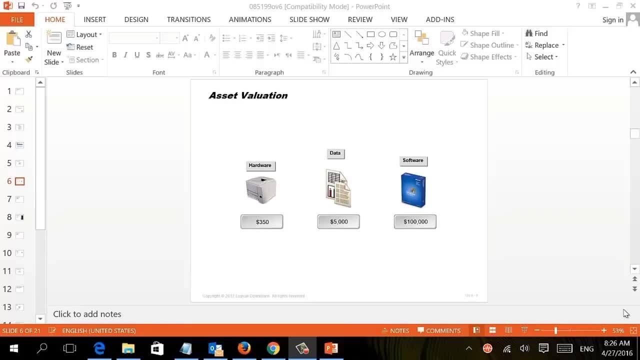 Of the control. So this is the only part inside the course that has some formulas that you need to memorize for the exam. Now, on the previous lecture, we explain the risk: What is the risk, How to identify the risk, How to manage risk- risk principle. 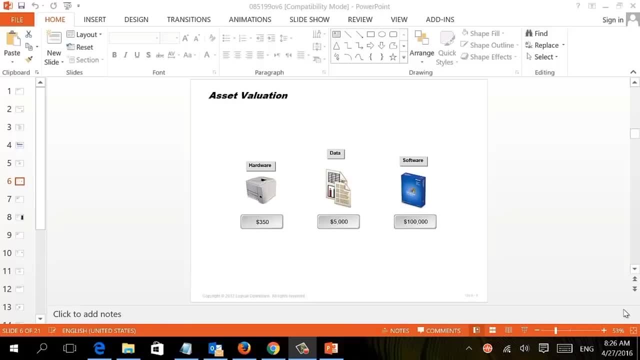 How to mitigate and avoid or accept, and what is, what is the definition of those principle or transfer? Now, this was just an Introduction. the previous lecture was just an introduction. Now on real life: How do we implement risk? from where should we start? 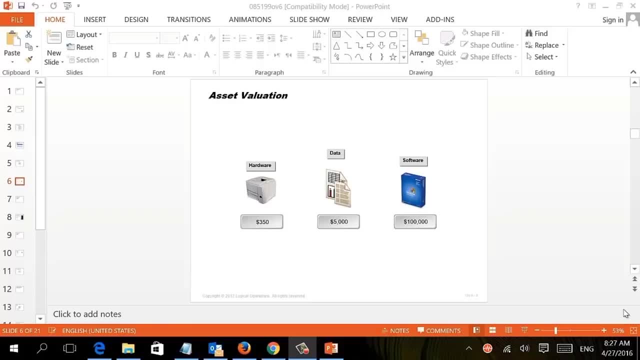 So to be able to identify or to do a risk assessment or to choose some counter measure to reduce the amount of risk, We need to start with evaluating our assets. So the first thing we need to do inside The risk management, It's to identify the value of our assets. 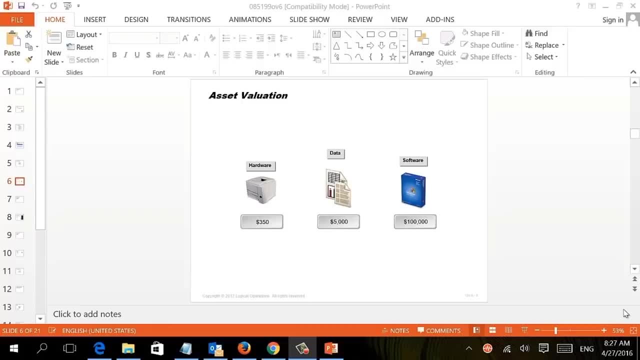 Now, in assets, we have two different type. We have the physical assets, like hardware, like shares, like tables- And this is actually it's not the main assets that we are looking for, but it should be considered- computers, hardware, printers and so on, But the really important assets that you need to evaluate will be the data asset. 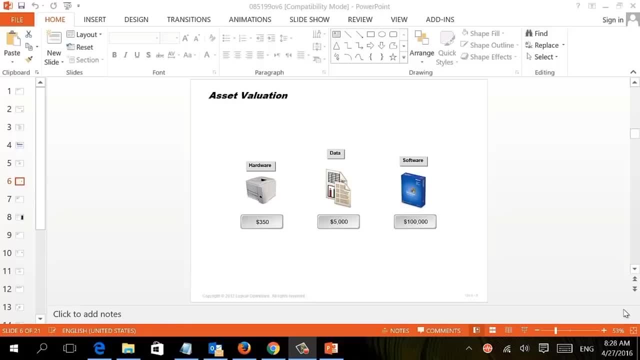 So data or information assets. This is the important part. Imagine that you are working in a bank. The bank has some devices or some physical assets. He got some computers and some printers and some scanner. fine, Those are easy to identify their value. 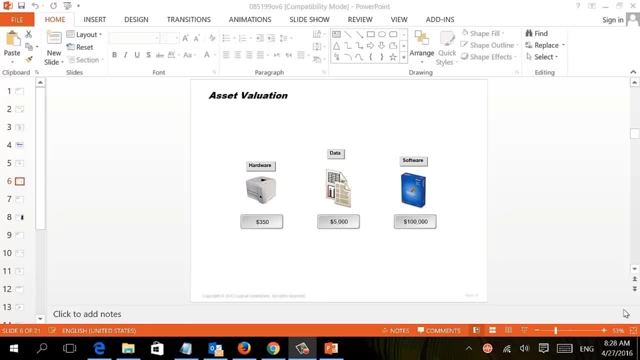 I can tell you We have 1,000 computer or 100 computer. Each computer has been bought with $1,000.. So our physical assets worth $100,000.. But can you tell me how to identify the assets, The information assets? 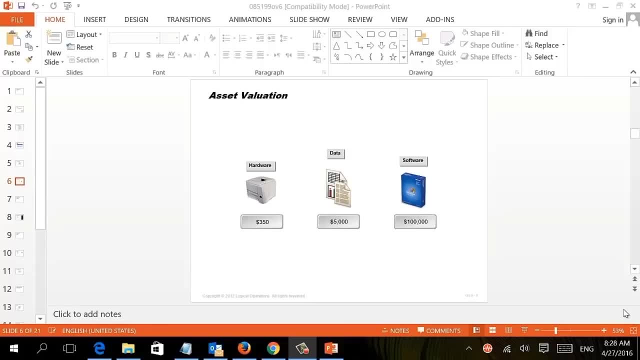 What is the value of the bank information? If it the bank lost those information, How can you consider the last of the bank Or how much Would be The loss of the bank? I mean, it's easy to calculate that if we are talking about. 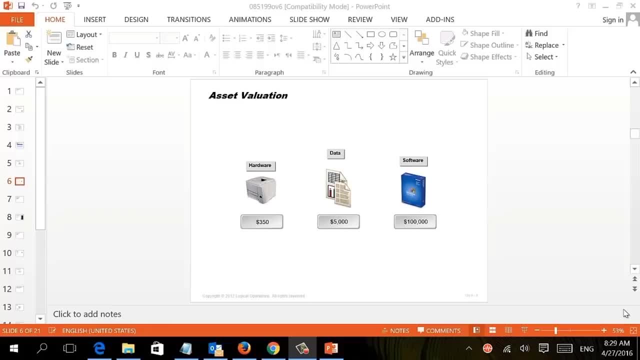 Hardware. So the information and the data, those are the assets. that's taking some effort to evaluate their value. We also have software, but also software is easy to identify the value. Now, before go, before start explaining the formula, I'm going to talk to you about some different techniques. 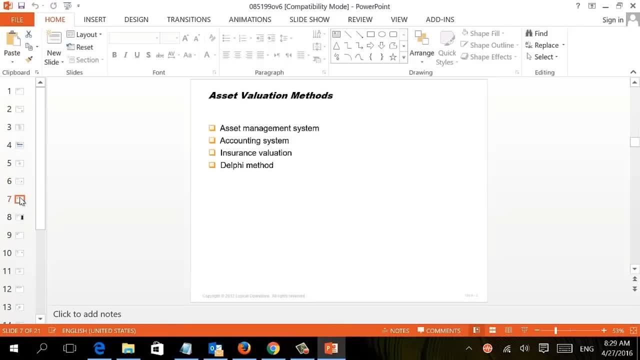 That is used for assets evaluation. So we have different way. We have the inventory. If any organization has an inventory system, we can refer to that. We have assets management system or accounting system. This will help the first three. one will help in evaluating the physical assets because inventory will include 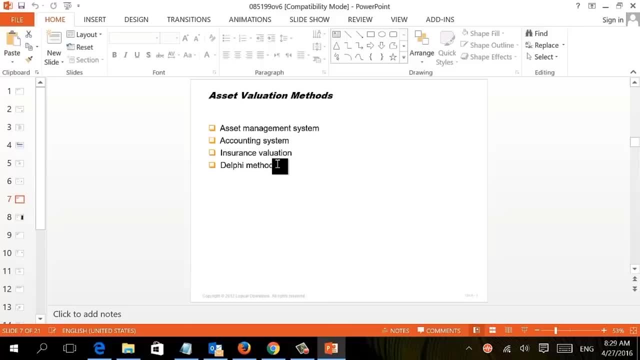 all the hardware and their prices, or the accounting system. While this one- please take a note about this one- Delphi technique, It's a technique used to evaluate the information assets And it depends about expert opinion and survey. So the key word here is expert opinion and survey. 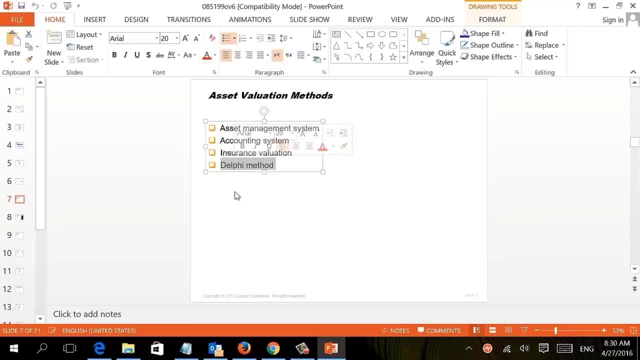 We are doing survey to expert people to be able to identify the value, So you are not requested to understand how it work, but you need to know what is Delphi technique. It's a technique that is used for assets evaluation and it depends about expert opinion and survey. 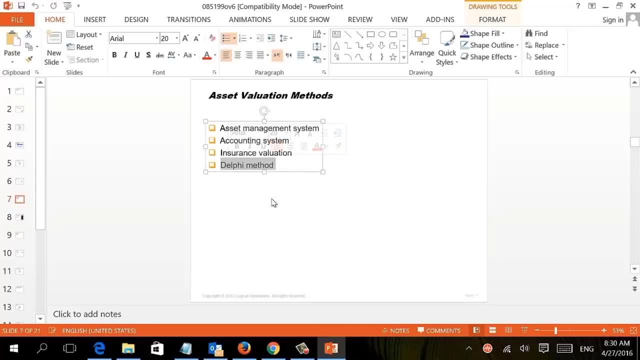 anonymous survey. So if you got any questions, as the exam was a stick keyword: what technique is used for evaluating assets based on expert opinion or survey? it should be Delphi technique. Now, here is the important part in this course. I am sorry in this domain. 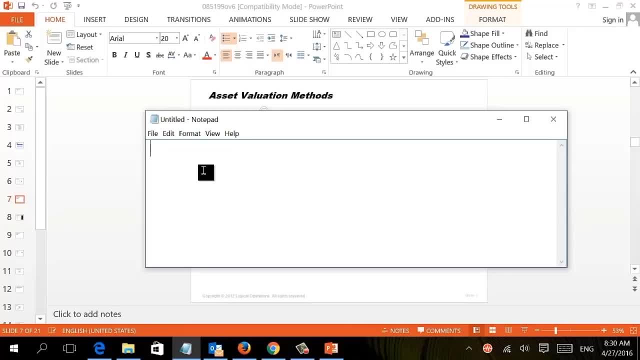 Assume that I was able to calculate all the assets values that I have: the tangible assets, things like the hardware, the computer, things like the printers, tangible- and the untangible, the assets like information and that, and I end up that my assets value both of them equal 100,000. 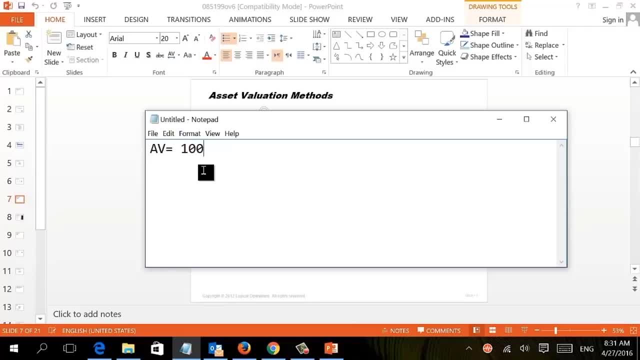 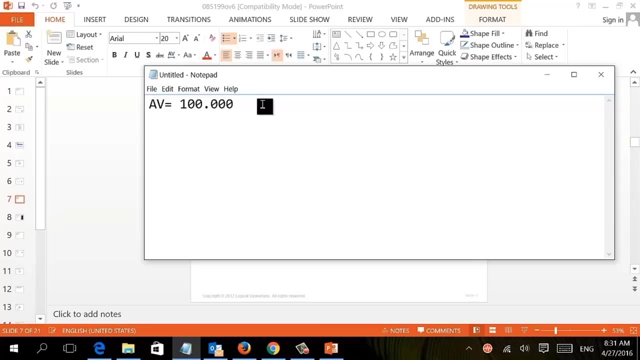 I'm going to put simple number for simplifying: 100,000.. So my assets value will be 100,000.. The second part of the formula Will be: And whatever I'm doing right now, it need to be done for each threat or for each vulnerability. 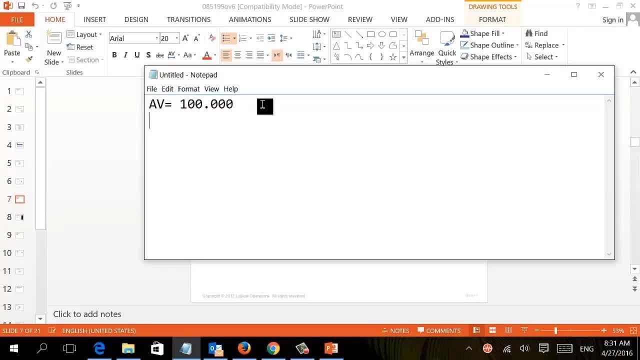 So, assuming that we are talking about fire. So first I did calculate all my assets, Who's at 100,000. the second values that will be given to you inside The exam is something called the exposure X Poser Factor. 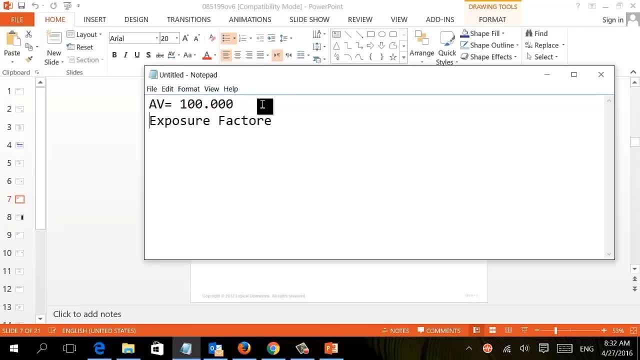 An exposure factor is usually a percentage. So exposure factor it's a percentage and it represent the amount of lost that will happen if a specific Vulnerability or threat has been exploited. So if you are talking about fire, to calculate the file, we are saying, okay, we have our assets, tangible and non-tangible are worth 100,000. 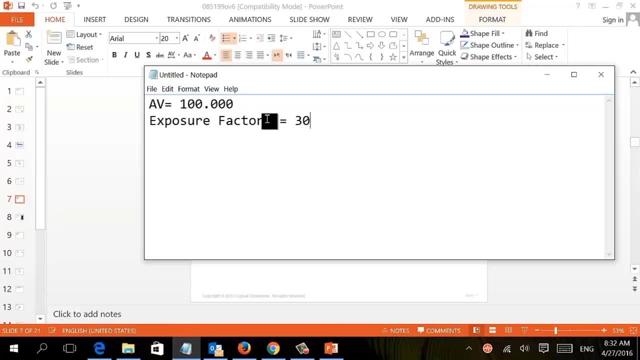 The exposure factor of the fire of the fire will be 30%, meaning that if a fire happen, my lost will be 30% of the assets value. from where they are getting those values? From where they are getting those values? There is different way for getting that. 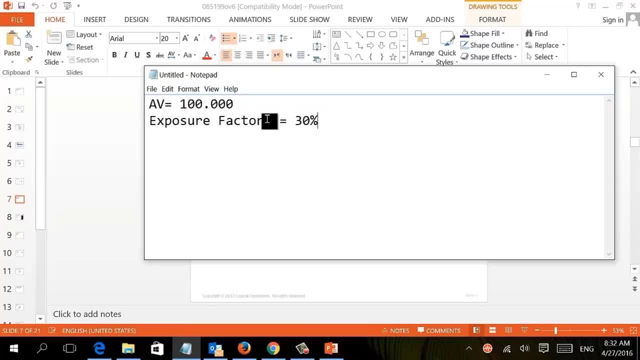 There is some standards, There is historical information, But actually inside the exam, you will be giving those information. You have one vulnerabilities that we are analyzing and he will give you the assets Value is that much? the exposure vector is that much then? 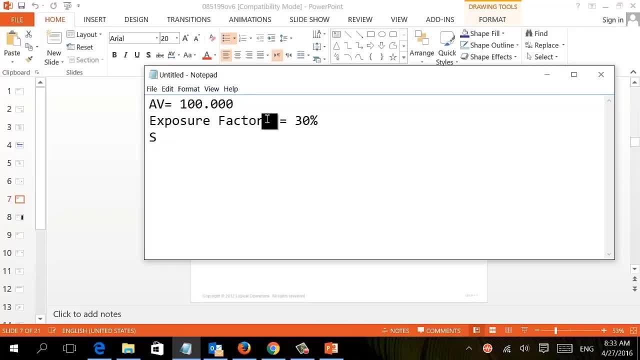 You need to calculate something called S, L, E or single lost expectancy, which is equal to a V Multiply E, F. that's mean every time the fire happen, how much we're going to lose. So it should be 30% multiply 100,000, right? 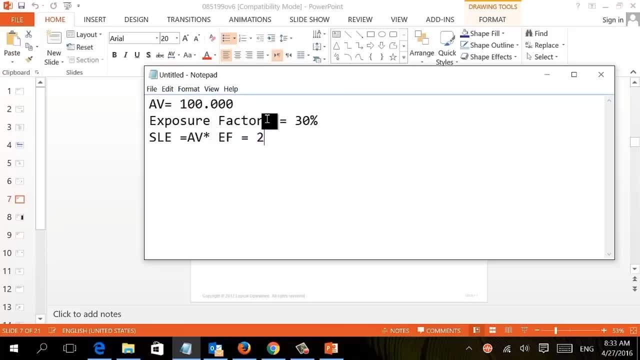 So it will be 30,000.. So the first formula that you need to memorize will be the single lost expectancy, which in our case will be 30,000.. Then he will give you another, So three input you should have inside the question and you need to calculate two formula. 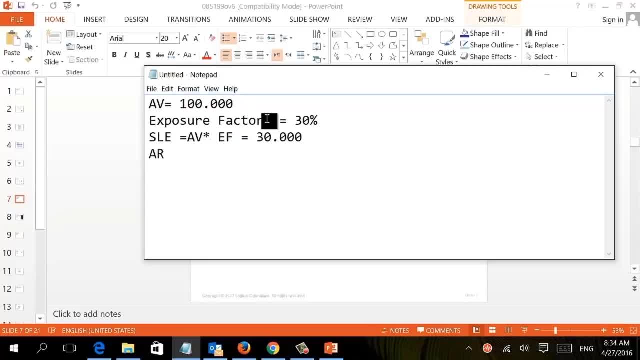 The third input. It's called a- are all sorry- or annual rate of currency. This means this: vulnerabilities that we are talking about, how many time It happened per year, and it's usually an integer: I, A, A, A, A. 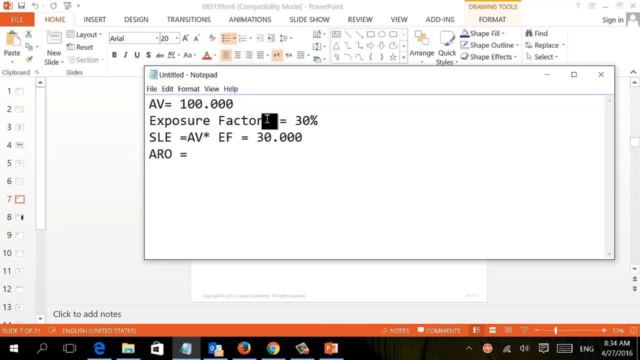 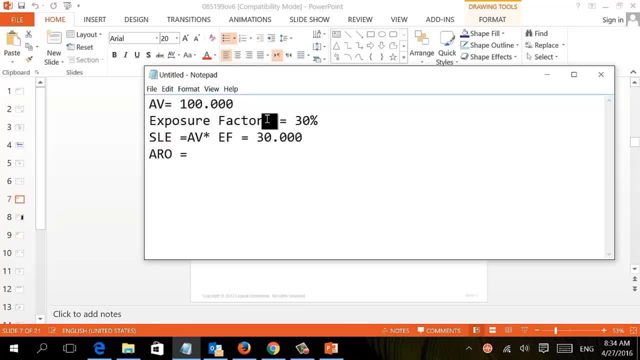 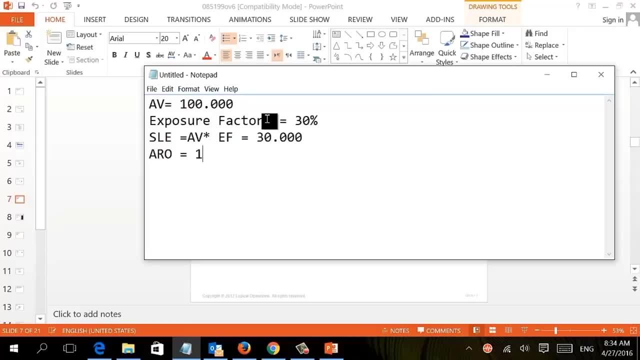 1. I mean it should be 1 over and the formula should be 1 over n, where n is the number of Occurrence of this event. So if we are talking that this event happen one every year, so it should be one. what if it was one every three? 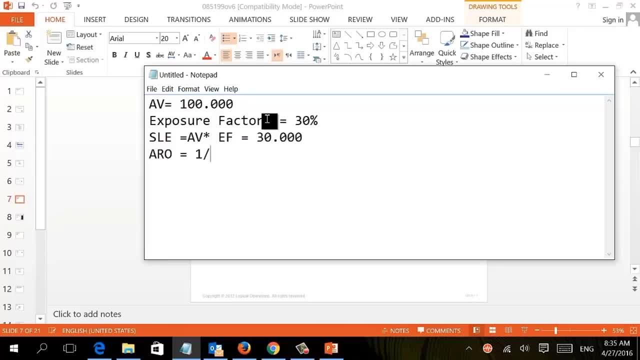 year, I'm sorry, and its number of here. so it will be one over three. so we are talking about 0.3, so the arrow will be 0.3. so arrow is the annual rate of currency. now the last formulas that you need to calculate. so you have three. 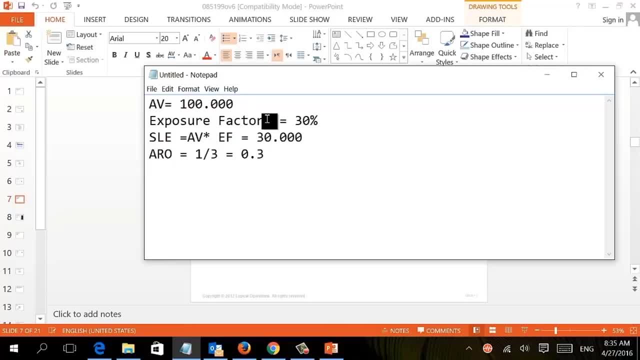 input and you have two formula you need to memorize. the input that will be giving to you will be the AV assets value, will be the exposure factor, which is the amount of damage that will happen if any vulnerability took place, and will be the arrow, which is the annual lost expectancy, and we should end up with a 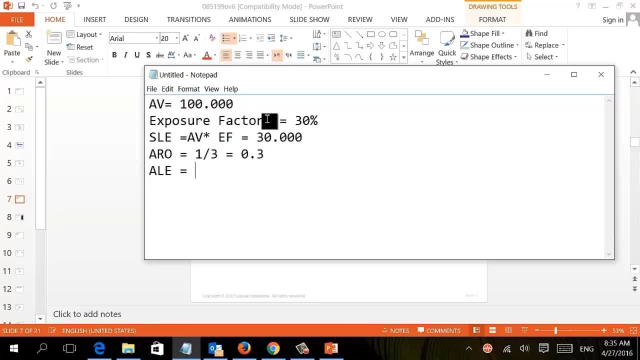 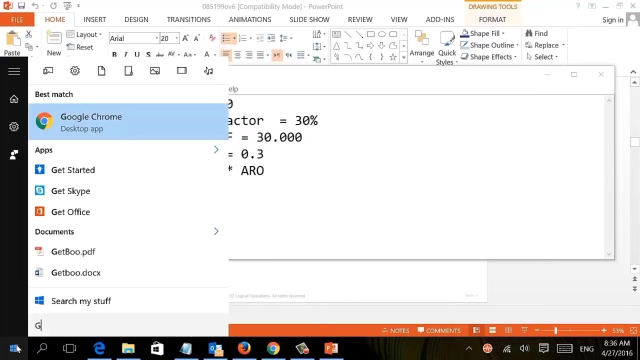 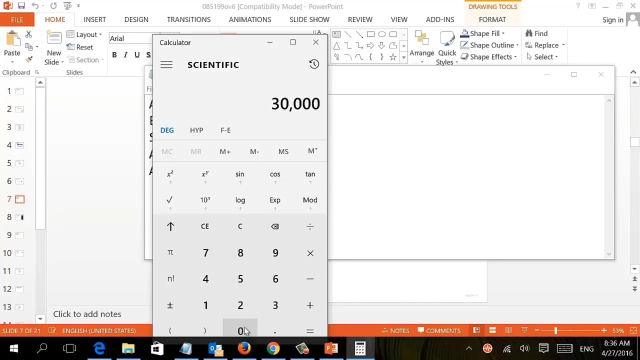 le annual lost expectancy. according to that, what is my annual lost expectancy from the fire should be SLE multiply a I A R? O, so it should be thirty percent as thirty thousand multiply 0.3. let's open the calculator. so we are talking about thirty percent, thirty thousand, one, two, three multiplied. 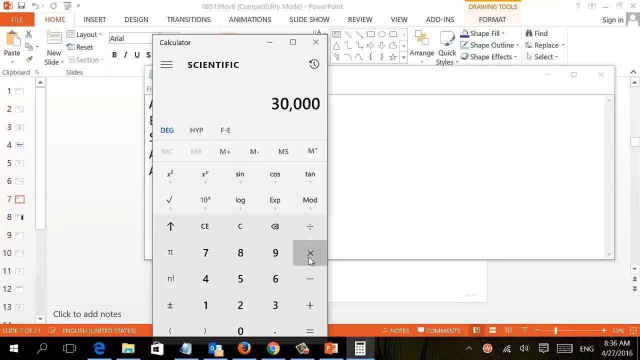 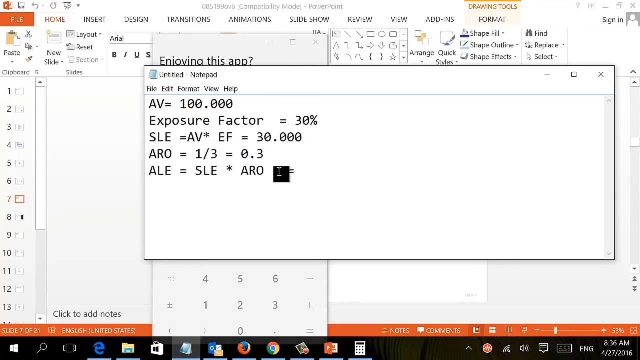 what exactly suppose that? I suppose this performing table: no, zero point. then I will be allowed to calculate inside in writing all variables. so nine out of two thirds will be nine and I will be able and I can change the list, you know. then we just leave them and okay, I finally 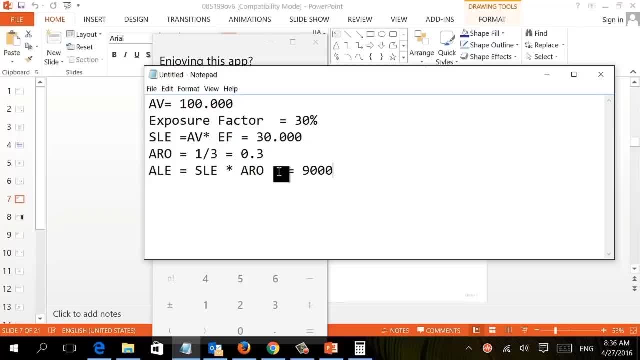 know, students, degree my body and workSTL. here you'll be able to apply to negative and the value should be nine thousand, so our ALE will be nine thousand. okay, so what? because the amount that will the lost from fire will be 9,000, so it doesn't. 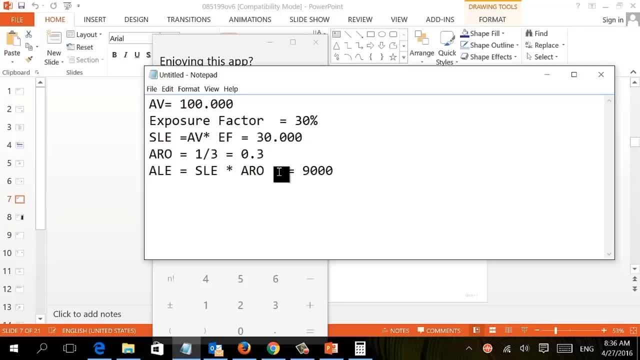 make any sense that my lost will be 9,000 and I'm gonna spend 20,000 on fire equipment. so this is a very important part inside risk, the cost effectiveness. it's not about just implementing the latest and the greatest technology to reduce the risk. it should be cost effective and actually sometimes inside. 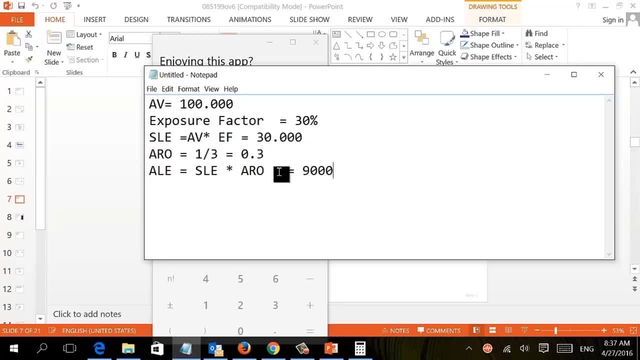 the exam. you will not get the questions that straightforward, but he will give you a scenario. he gonna say is that a team is working on risk in an organization and they found that the assets value is that much. they found the exposure factor. therefore, this is the ARO and they will give you how much the 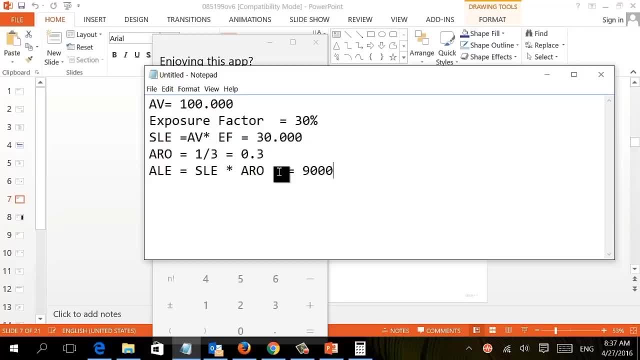 company spent. so he will tell you: the company has spent 14,000. is it cost-effective, plus or minus? so you need to calculate to be to understand how much the company has spent. so you need to calculate to be to understand how much the company has spent. so you need to calculate to be to. 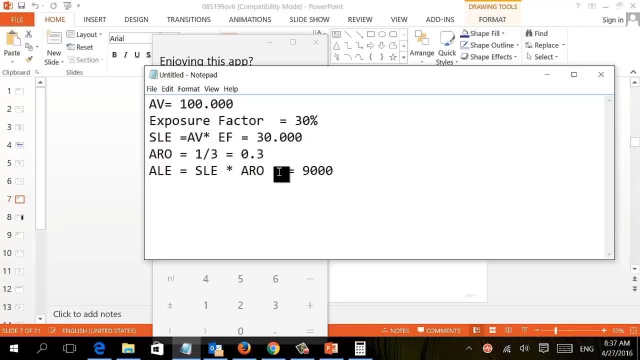 understand how- how much- they actually should be spending and how really they spend according to the question and you give your opinion. this is not cost-effective. this is minus 6,000: they spend more than should be expected. so this is very, very important- formulas that you're gonna need to memorize and 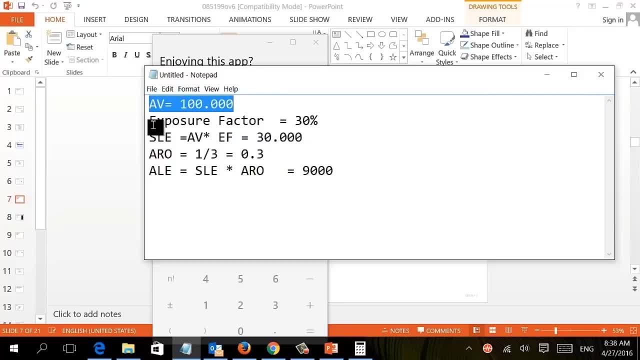 as I told you, the inputs that you'll be having- size exam is that, and the SS values, exposure factor. they are all and you're going to calculate SLE and you know they need to calculate early and your objective is to understand the how much you should spend on each thread, because you do that for each thread: fire hacking. 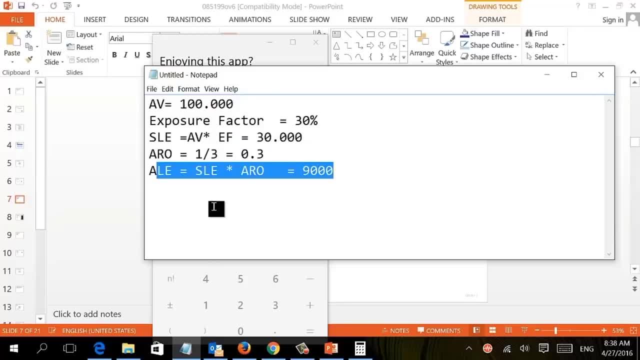 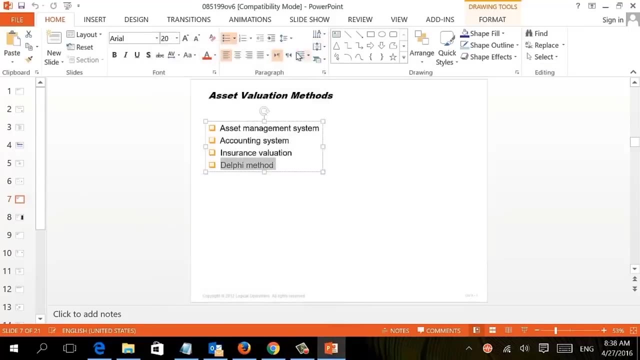 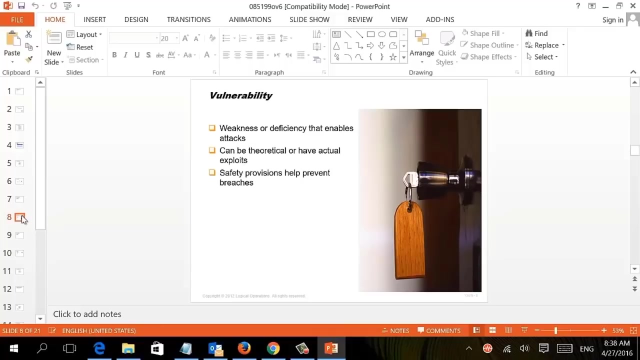 physical secure any threads that you should expect. you should do this calculation to be aware how much we need to spend on this specific control. so very, very important formula. please write them down, okay. then the part or the vulnerability usually is coming from different places, so it could be theoretical, it could be actual exploitation safety. so 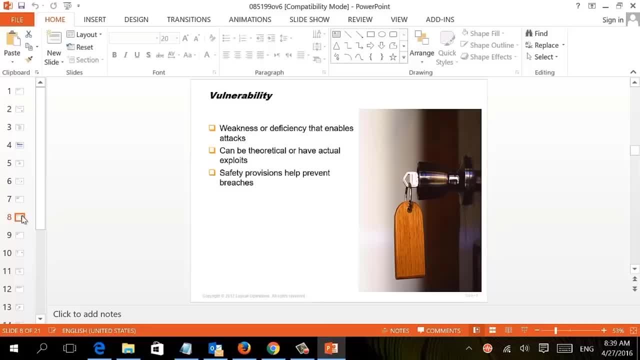 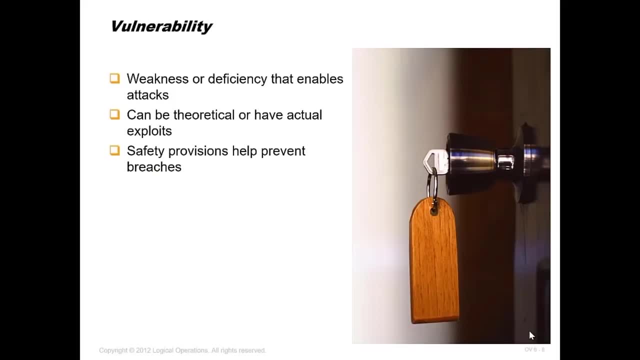 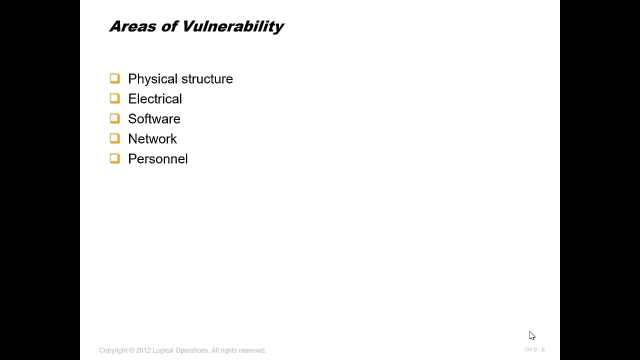 vulnerability could be different kind of vulnerability: physical in technical. we should consider all kind of vulnerability and do the formulas that I should. I just show you of vulnerability, also physical security: people who's working in operation should be analyzing the physical security vulnerability. electrical software, network, personal risk type. we have the man-made risk, which is something like: 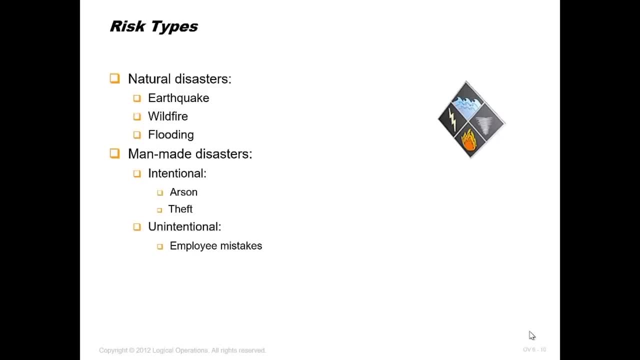 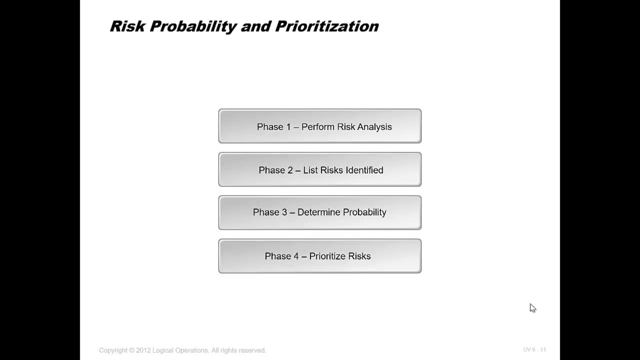 internal risk, theft, employee mistakes or natural disaster risk things that you can do nothing about it. so if you are in an area where there is a lot of tornado and flood, you have to work with that. I mean, you can not say you can do nothing about it. so when we are doing risk, we need to identify all the risks that we 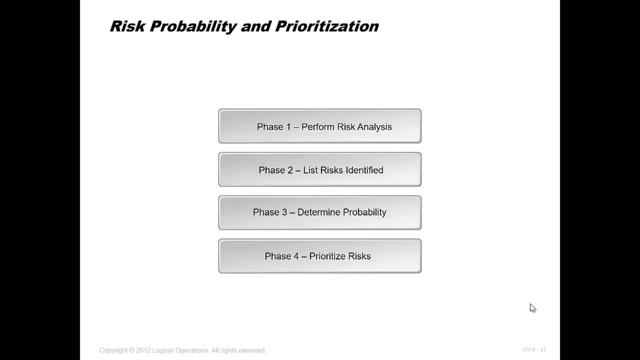 are expected, right. but when you do that, when you start sitting- and you should, because actually this is not easy- to the sit and to start thinking about everything bad that may happen in different area- in physical security, in technical security, in personal, in hr- it's not easy but you'll end up with a huge 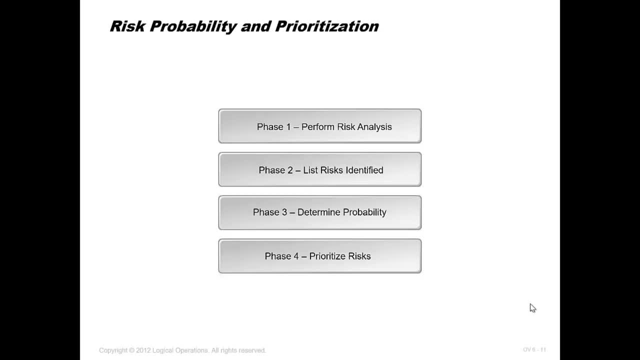 amount of risk. so i cannot assign or put a counter measure for each one of them. it will be endless because you know sometimes you have thousands of risks, not just hundreds. so after doing, after identifying your risk, we need to identify the term, to determine the probability and to put some priority on the some priority need to be taken into consideration. 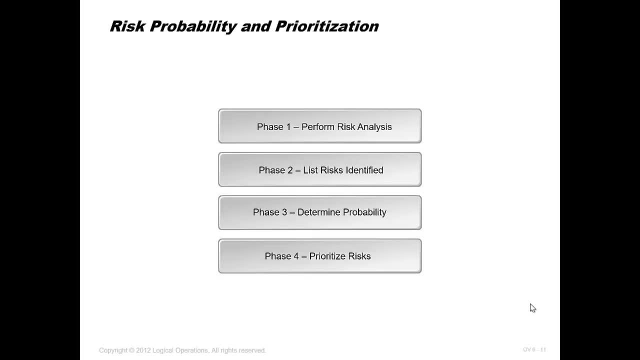 let me give you an example. assume that we are in an organization that and we are doing risk assessment, so we start identifying the risk. now this specifically organization exists in a city where there is a lot of tornado and flood, so this has been considered as a risk because it may happen and it may end up with closing our business. 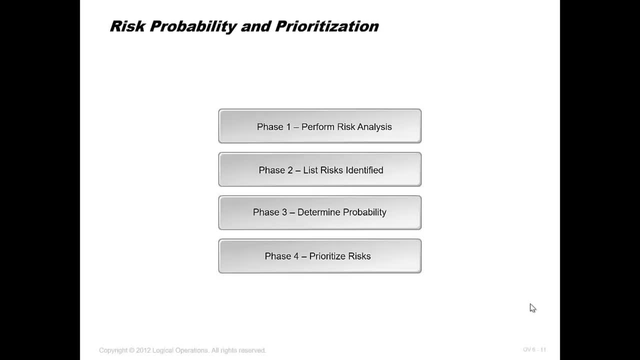 for few days until the problem losing some customer. i need to consider that. but also we have a risk, for instance, for earthquake, but this is very, very rare that happened. i mean it happened every like 20, 30 years now. if i have a budget to buy some control, should i divide the budget? 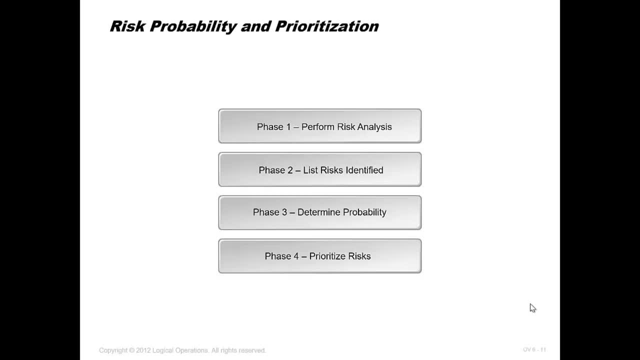 equally on those two specific risk? definitely not. i need to give one of them more priority than other because, according to that, the tornado is happening every year, so the probability of happening is very high. so i have to assign a budget for that. well, the other one need to be considered, but since it's a 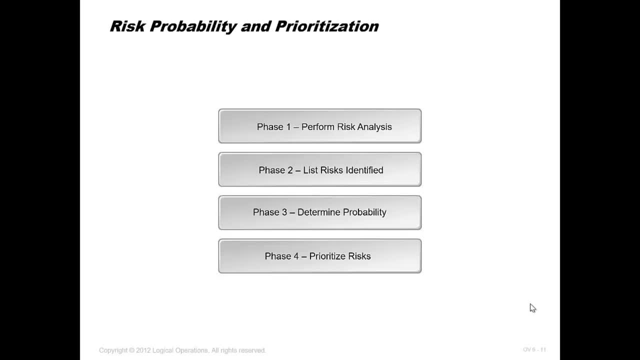 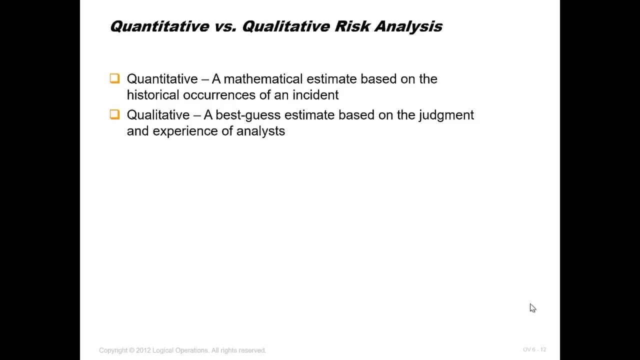 rare threat so I need to allocate lower budget. so when we are doing that- the identifying risk- you need to put priority, because you will not be able to mitigate all kind of risk. in doing priority. we have a qualitative and quantitative analysis. quantitative mean I'm giving a priority, according to some 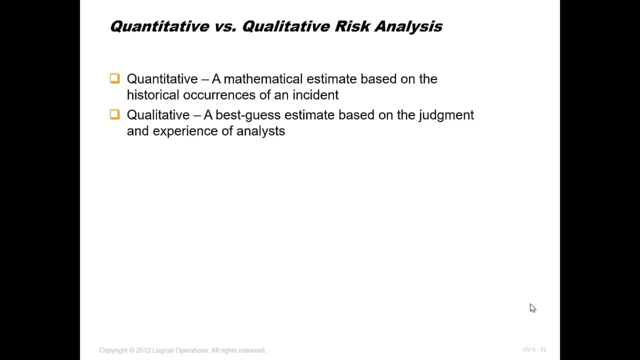 number. I have the last 10 year. a fire happen every year. I know this is very- I mean- pessimistic, but for instance, so I have. I'm putting priority according to number, while qualitative risk analysis mean identifying the probability of the risk, but based on the best practice, like I'm saying, this most likely to happen. I. 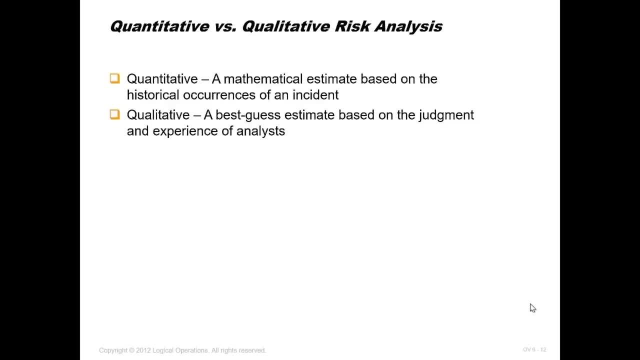 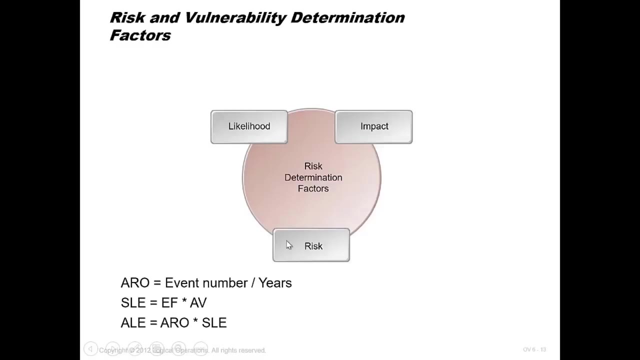 cannot put the figures, but I'm putting: most likely or will not happen. so I'm giving names but I cannot give numbers. so this is how to identify the qualitative analysis likelihood. we need to know the risk, we need to know the impact. this is the formula I was telling. 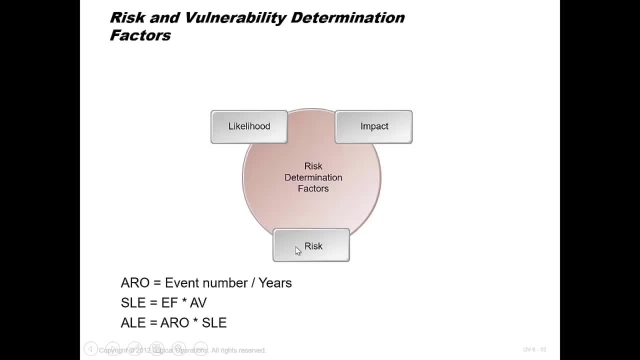 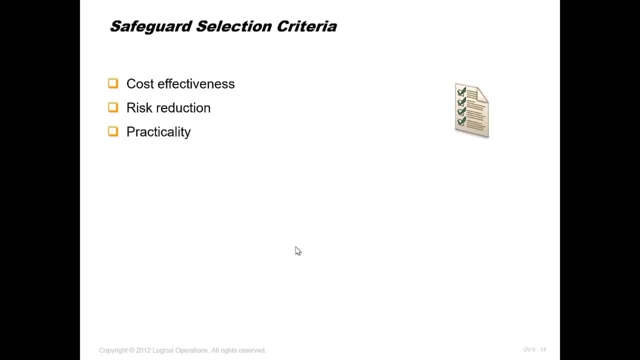 you about extremely important and you should understand what is a qualitative analysis and quantitative analysis. very important thing about the safeguard or about the countermeasure? it should be cost effectiveness. you will be required to evaluate the effectiveness of the cost from the question. it should reduce the risk. you should not implement a control that will increase the risk and 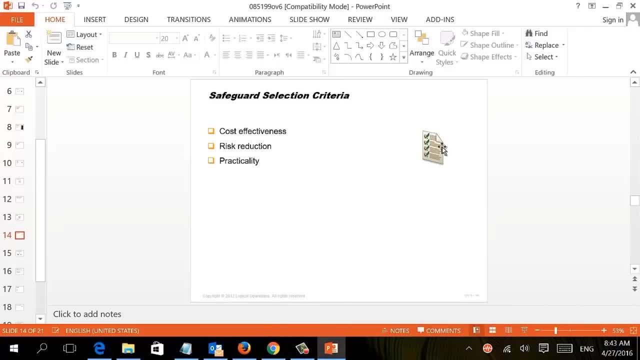 it should be practical, not a theoretical part. so when you implement the control it should match those point. so should not suggest theoretical things that cannot be implemented, but the first one, cost, effective and this is what he may ask you inside the exam and, as I said, told you to not be straightforward question, he will give you scenario. he. 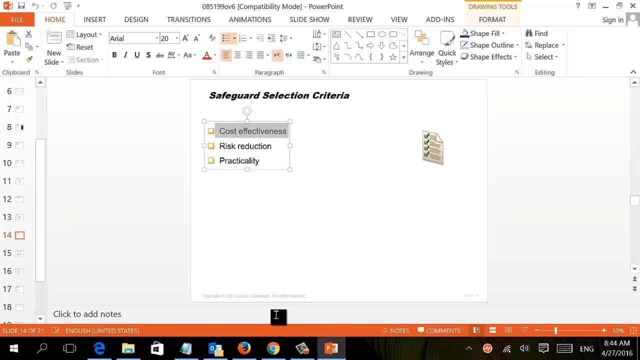 will tell you how much they spend on countermeasure and he will ask your opinion. so you need to calculate and you need to get the annual lost expectancy and to figure out what is the better amount to be or the best amount to be spent on this specific risk. 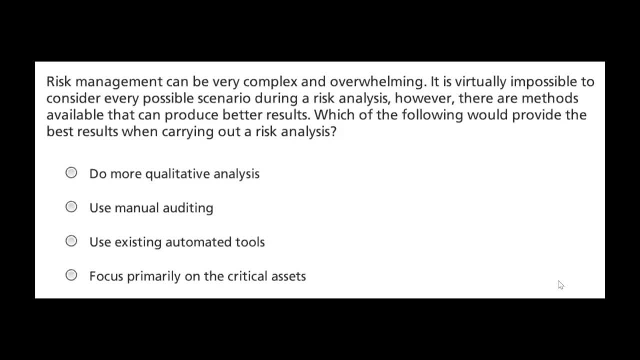 let's take an exam question related to risk management. risk management can be very complex and overwhelming. it's virtually impossible to consider every possible scenario during a risk analysis, which is true, very hard to analyze all different scenario or all possible scenario. however, threats are methods available that can be. 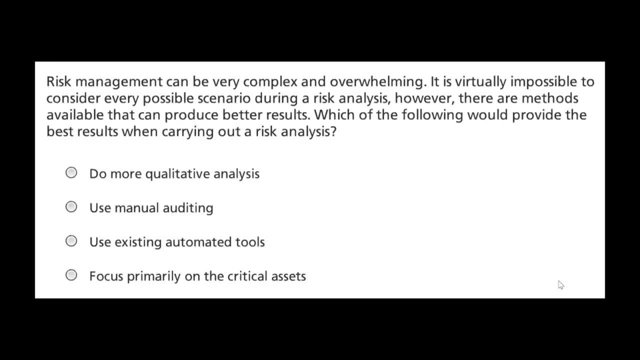 used to produce better results. which of the following would provide the best results when carrying out risk analysis? do more quality analysis, more qualitative analysis, which we explained before. use manual audit, use existing automated tools or focus primarily on the critical assets. so which one is the best way for doing risk analysis? what do you think? 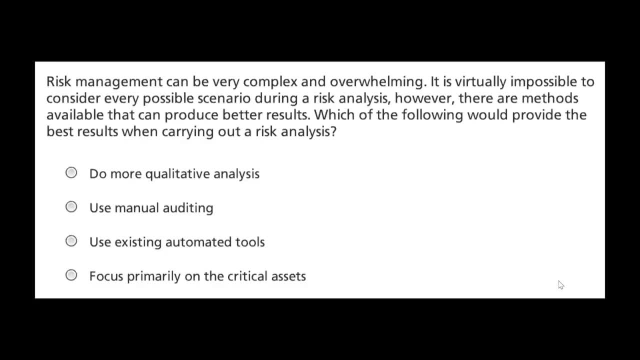 which one is the best way for doing risk analysis. what do you think doing a qualitative analysis? you remember that qualitative analysis it's a part of the risk analysis, it's not the full process. so definitely this is not the right one. use a manual audit, and manually mean it's not precise or it will not be effective. focus primarily on the critical. 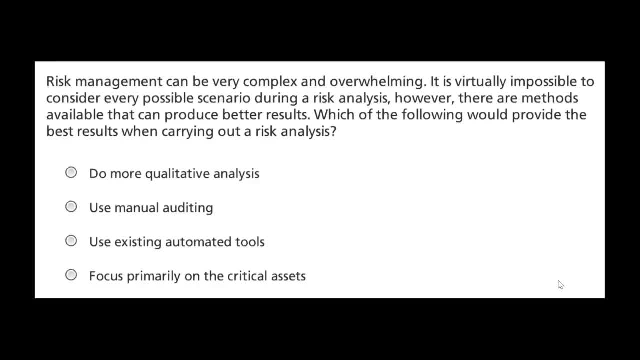 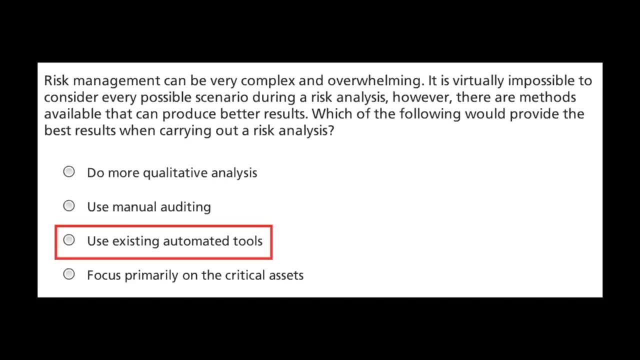 i said, this is also a part of the risk analysis, but it's not the full risk analysis. so the right answer will be using an existing automated tool, because the automated tool will have a lot of scenarios, will have a lot of built-in capabilities, surveys and so on, so it will give you better 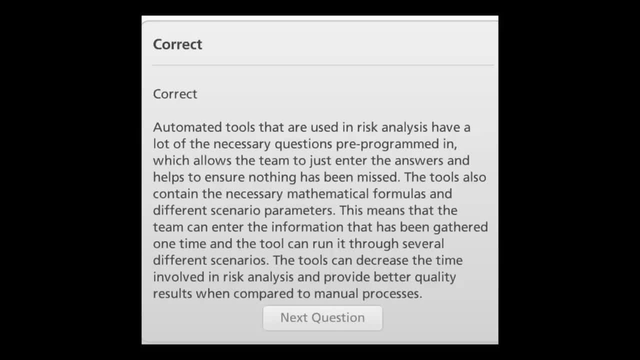 results and the explanation of this question. as you can see that using an automated tools, which is you, usually has a lot of information in their database that can be used right away and instead, instead of figuring those information out, will give you a better result. so the points that i'm trying to raise here, 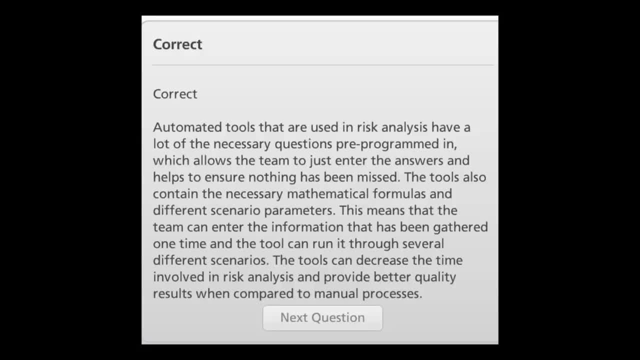 first is that, when it comes to things like risk analysis or risk assessment using an automated tool, it's much more effective and will give you better results. that's why, in the next lectures, i will forward to two of the major automated tools that we usually use in risk assessment. 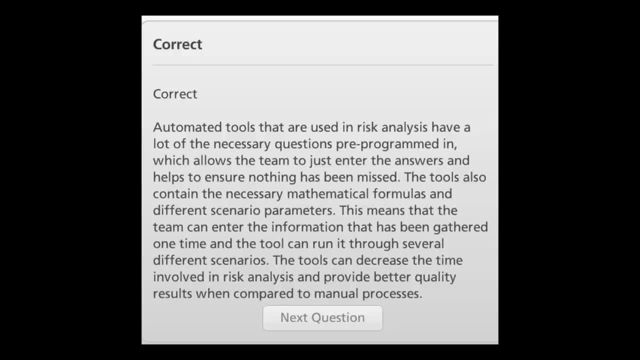 those are expensive tools, by the way, but you should be aware of them because, as we agreed at the beginning, it's not about the concept, but also you need to know what is in the market today in case you set for an interview or you join a job where they are using these tools. 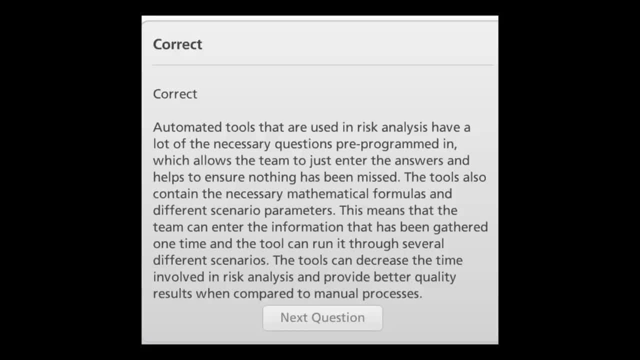 alwaysận, but just showing you a couple of tools like Archer, for instance, from RSA, which is a very effective risk assessment tool, or ARIS. they also have a GRC and so on, but I believe Archer is most common and used in different entity. so I just want to show you one of those automated tool for your. 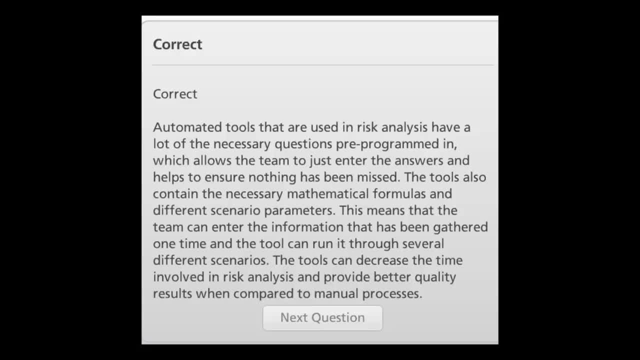 own knowledge, not for the exam purpose. another point that I would like to clarify is that a very important factor that you need to consider to pass the exam is to think like IC square. this is quite important because sometimes you may find one of those answer more realistic to you. 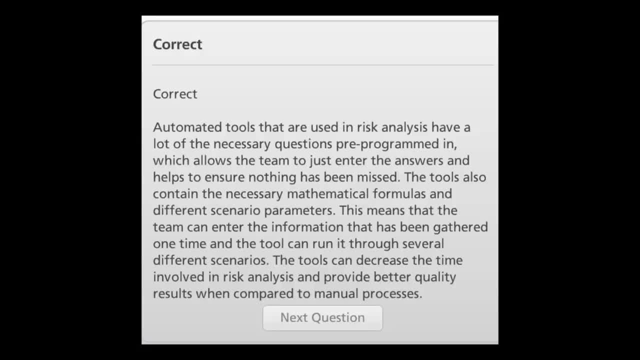 it's not about what is realistic to you. it's what about IC square is thinking. it's very, very important to get their mentality to be able to pass the exam and you'll get that by time. you don't have to worry about that. you're going to take a lot of exam questions and you start. 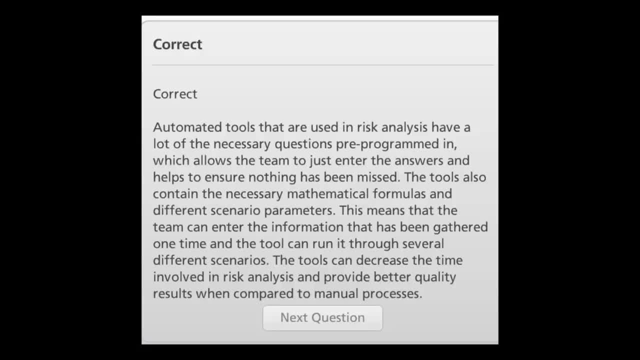 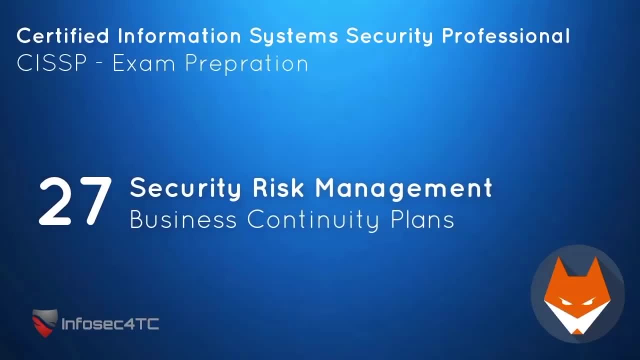 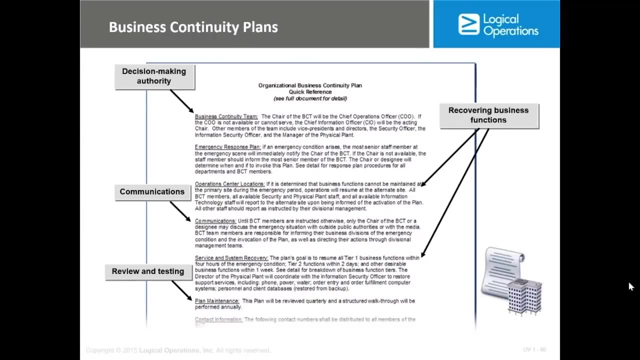 you will know how IC square are thinking and you're going to get the same mentality. after finishing the risk management, we're going to move to the business continuity planning and disaster recovery planning. now, risk management in the previous version of CISSP was a domain by 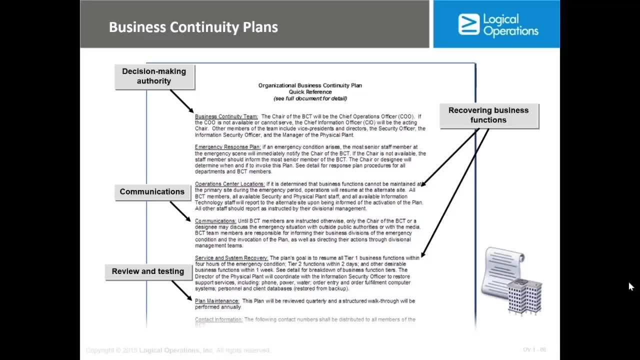 itself, and business and disaster recovery was a different domain, so by combining them together, they make the first domain one of the biggest domain in the course. business continuity planning is a very important topic and it has a lot of terminology that you need to be aware of, and you will find good amount of question inside. 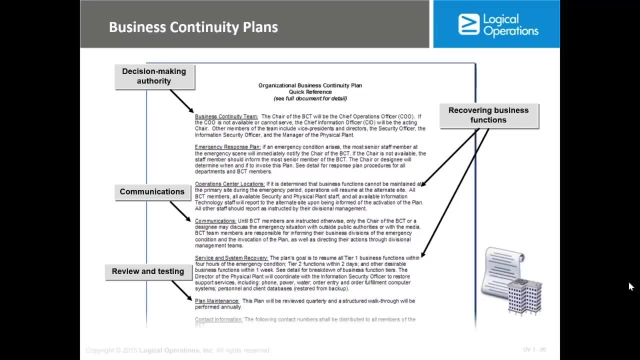 the exam about the BCP and DRP, so please study this part of the domain very well, take notes and after finishing the domain, I'm going to show you the best way to practice the exam question related to those domain. so let's start defining the business continuity planning and disaster recovery and 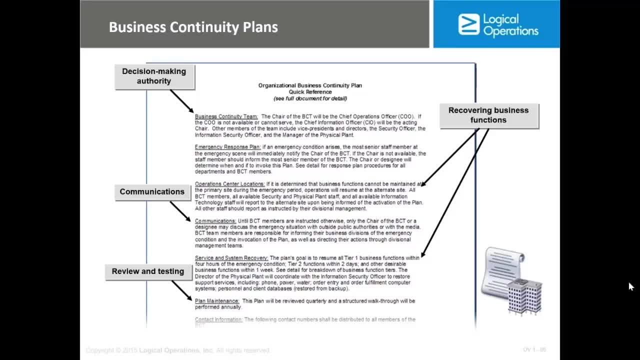 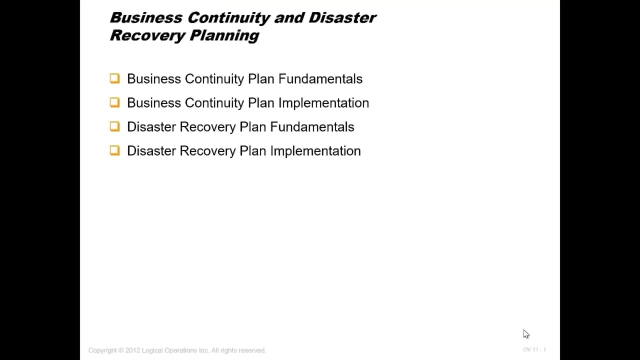 different terminology related to them and how to create them, besides the different document that is included in the BCP and DRP. now our first objective will be to explain what is the difference between business continuity, or BCP, and disaster recovery plan, or DRP: business continuity: 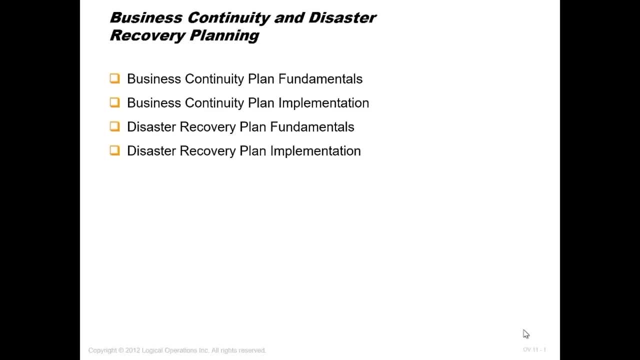 it's mainly a business document and we try in such document to identify all our business function and to give them priority to see how to recover the business. what is the most important business function to recover first? so business continuity. it's a business document, it's not a. 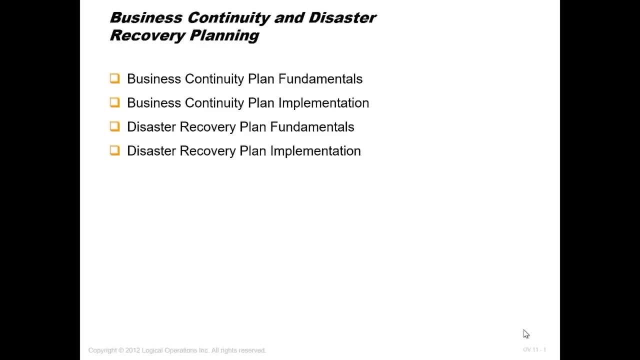 technical document, while disaster recovery. it's a technical document and once we finish this part, we're gonna see the sunflower document and see how to improve itデوا conseguir آيرفığا ما- the definition for both of them in the in the sunflower document. so let me. 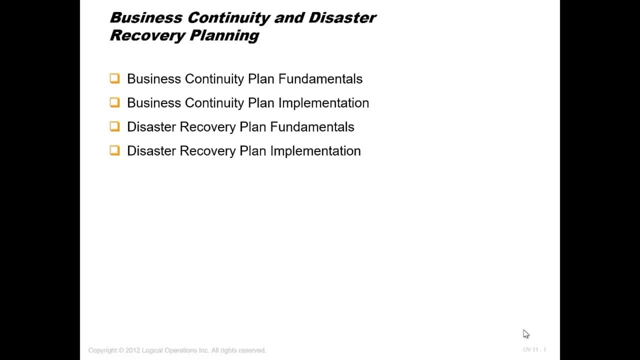 give you a small example. assume that you are a training center. okay, so training Center, what exactly is the type of server is providing? it's providing it, it provides training and to be able to run the business. what do you need? I need equipment, I need a location. I 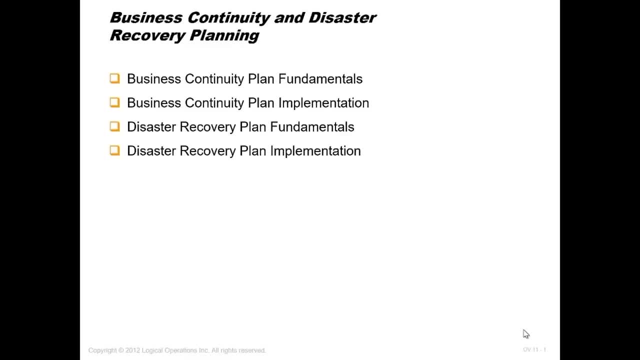 need desks, I need computers, I need instructor, I need operation reception. so those are the requirement that allows the business to running. now, in the training center we may have different departments, so we have the sales department, we have the training department, we have the operation department. right now, when we analyze the 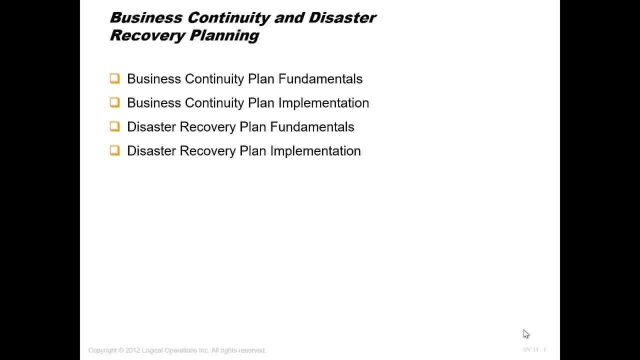 business. what is the most important department or business function that is needed for the business? it should be the training department. I mean, if you have a training, you have a course running and you don't have an instructor for instant, how can you run the training? you have the sales team, you have the HR team. you 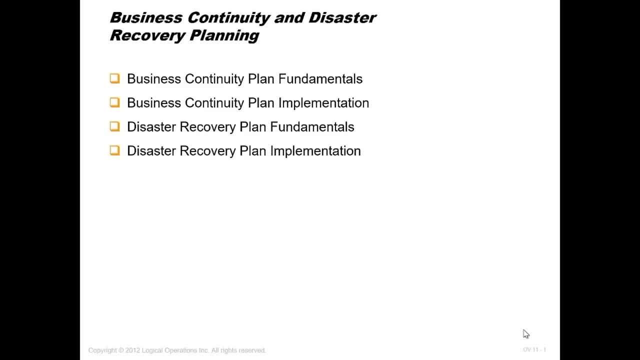 have the finance team, but you don't have an instructor from the training department team, so the business will not be running. so, according to that, maybe I need to get another instructor to become a backup. this is the business continuity. I'm analyzing the business, I'm identifying the business continuity and I'm 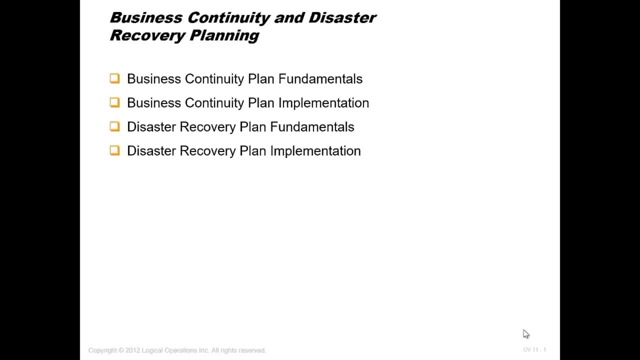 identifying the important business function and I'll try to find some option in case any problem happen. I'll be able to run my business. so it's a business document and, as you can see, it doesn't have any. it doesn't have anything technical so far. disaster recovery will be the technical document I mean for the 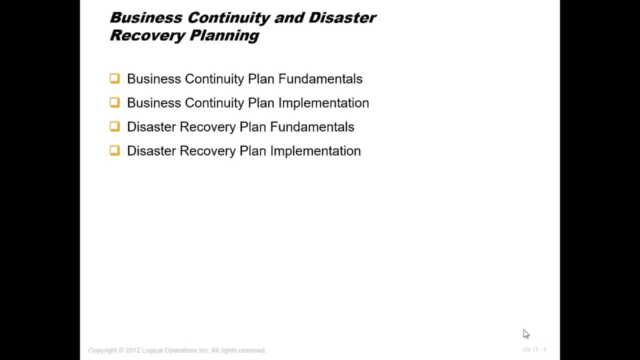 same examples that we are talking about training. maybe you need to have computers. what if a problem happen on the computer? we will not be able to run the business. so now I need to figure out a technical document that how can we recover if a failure happen to any computer. to take a backup from the 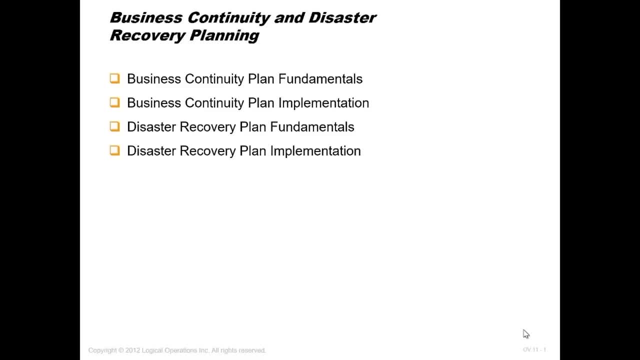 software, something like that. so business business continuity planning it's all about identifying the business, knowing what business function is inside, giving priorities to the business and then the business continuity planning. it's all priority to business function and to identify what is most important business function that you need to recover first, then second and third to be able to run. 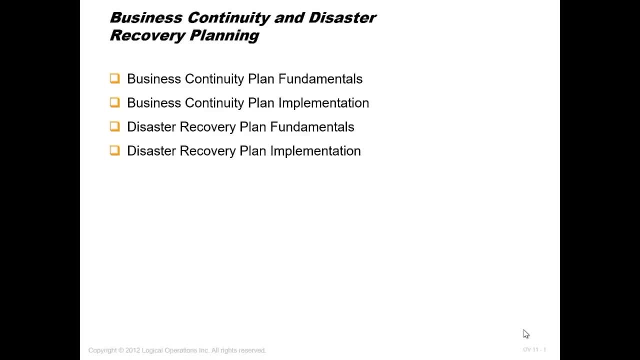 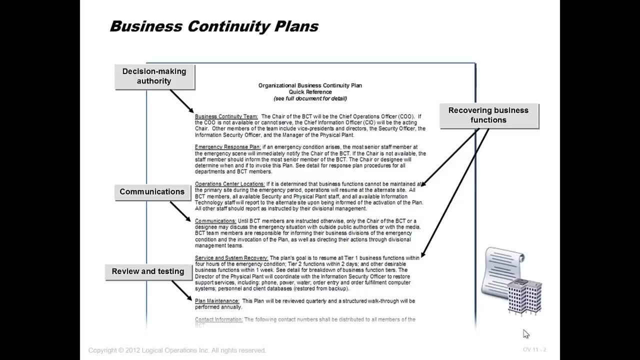 the business. well, the disaster recovery. it's a technical document and actually disaster recovery it's part of the business continuity planning, so a part of it will be the disaster recovery. this is an example of business continuity planning and I'm going to add some template to this lecture, but it's very 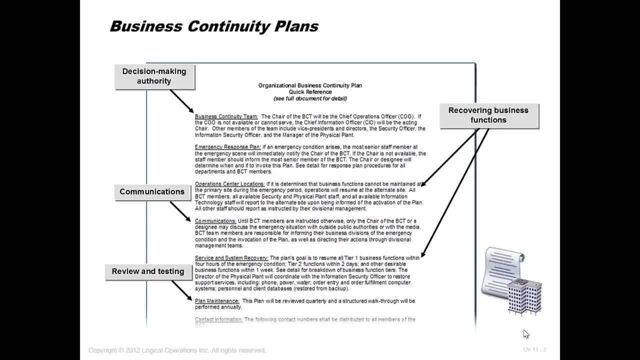 to go through it, because actually it's not easy to implement a bzp. you need, as i told you need- to understand very, very well the business and what is the critical business function. so, for instance, when we were talking about the training center, i told you that we have different department. 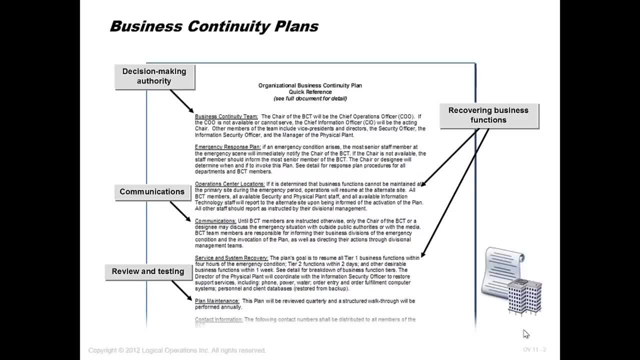 so, when you analyze the business, what is the important department is- or let's simplify the question- if i have a trainer and i have a reception guy, that uh sitting at the reception area for the all, for all new student who is coming for training, which one is most more important? 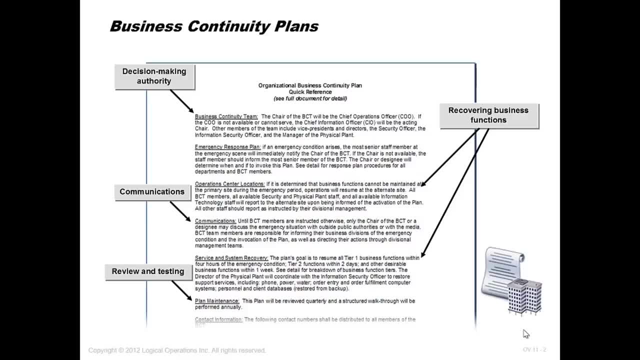 the instructor or the reception. most of them are important, but instructor are more important than the reception guy. the business can be running without someone staying in the reception area, while it cannot be running without an instructor. so now i need to have another instructor, but no need to have another reception, because i can run few days without. this is an idea about. 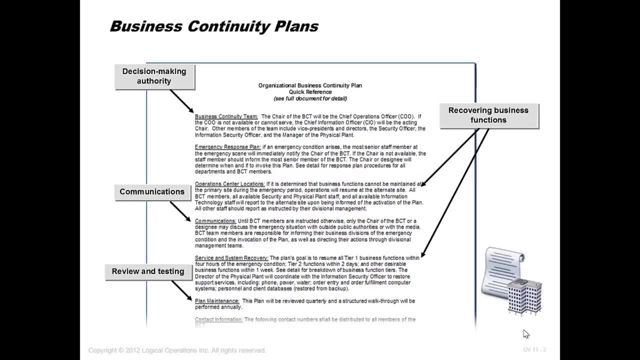 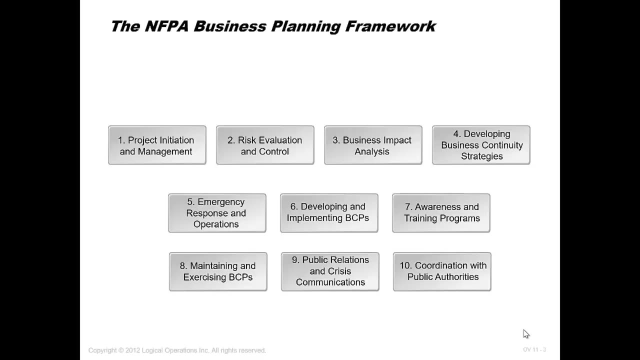 analyzing the business and the factors or the requirement needed for the business. so it's not a technical document, it's a business document. we have different kind of framework but you're going to need to know about mainly nest. this is related to a fire department business plan. 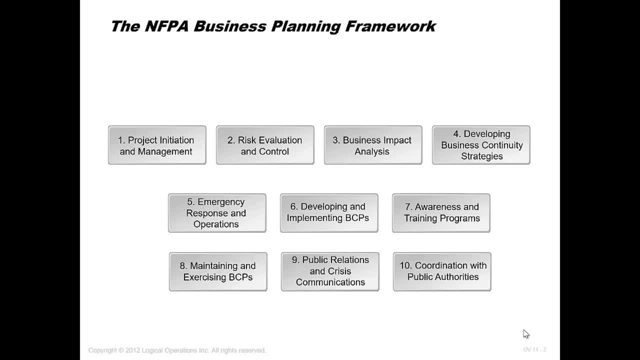 planning framework. they are all the same idea, but let's, let's go through it and let's talk about the step. so the first thing that you need to do if you are implementing a business impact, a business planning- uh, business continuity planning- is first, you need to have a 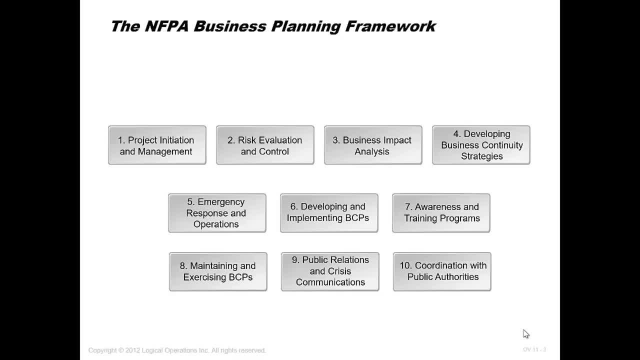 project initiation before doing the process itself. you need to do that as a project. what do we mean project project has a start date and end date. so you need to do, you need to say: i'm going to do a business continuity planning that will start on this specific date and 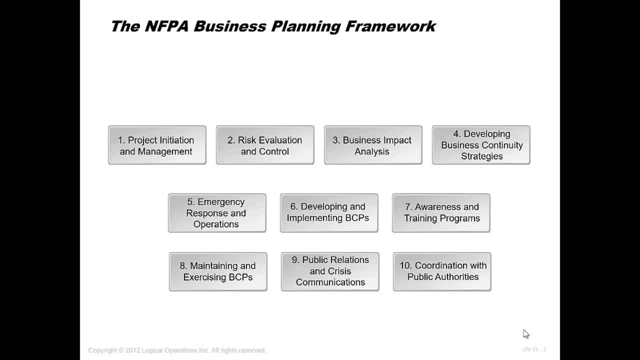 will end on that date and i'm going to need those resources and this will be my deliverable. so it needs to be clear. and also, this would be the project manager or the program manager. this needs to be identified at the beginning because actually this is a long process and 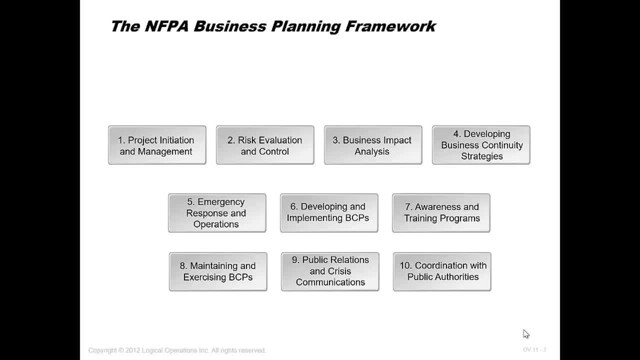 unless you put an end date and you assign resources, it will not never end and you're going to do a lot of meetings and a lot of interview, a lot of survey. it's not an easy process, so you need first to identify your resources and identify the length of your project and who will be. 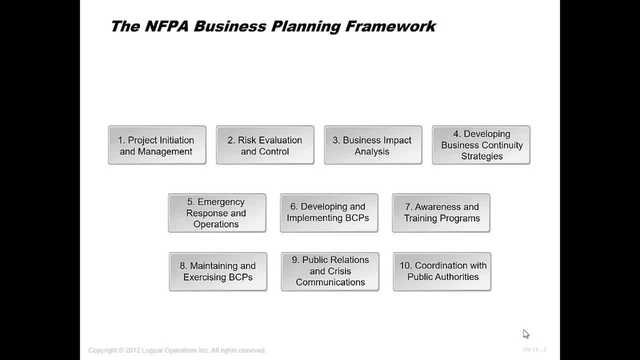 responsible? who will be in charge once we agree about that, when a second step will be starting the business continuity planning and how to start by risk evaluation and control. we need to start first the risk: identify our risk and identifies the controls that need to be done or put inside the 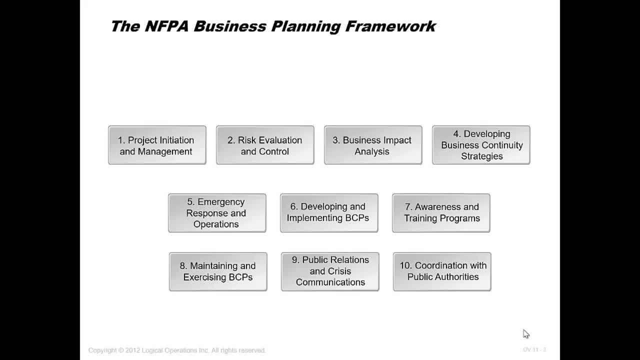 place the third part, which I believe it's the most important part in this BCP. it's called the business impact analysis I need, after identifying all the risk and all the threats I need to identify, is if this specific threat or vulnerability took place, it will affect my business, with numbers, the most. 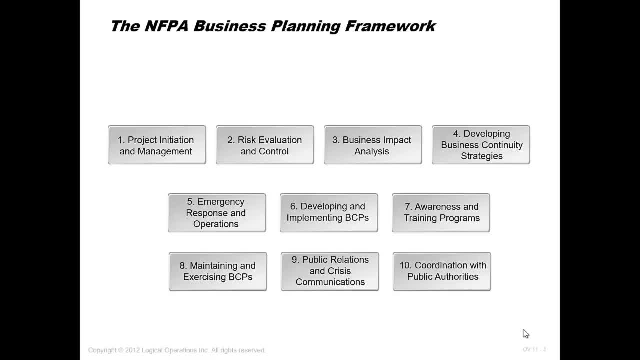 important thing I need to identify is if this specific threat or vulnerability took place, it will affect my business with numbers, the most important part in the BIA or business impact analysis. it should have figures because according to that, the management will agree or disagree to do this. 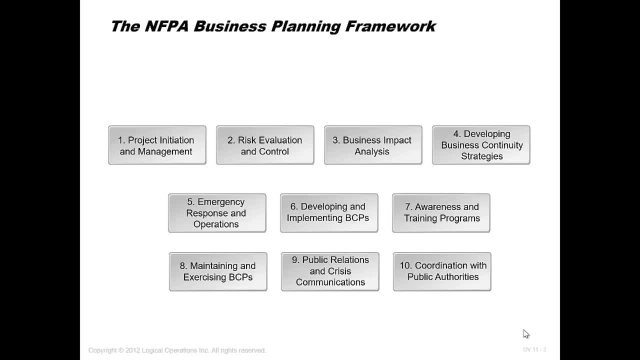 planning. so it should say okay if my, our system get compromised- and I get that from the risk evaluation and control. I know that we had a lot of bad experience and our system are not the latest, do not provide the latest protection software and hardware and we have some old operating systems. 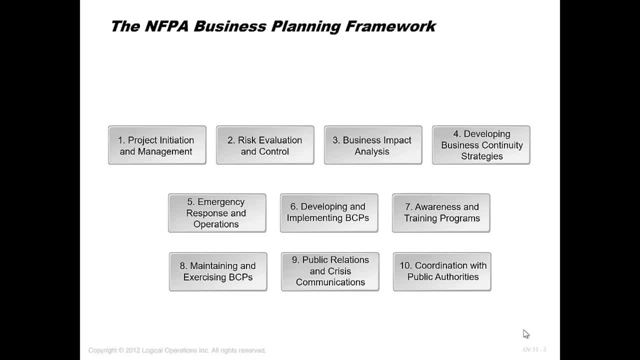 so one of the risk is we may get compromised on the business impact analysis and we're going to see a sample during this course. you're going to say, okay, if it happened, if we get compromised, we're going to lose one million dollar and according to that, we need to have a for instant. another. 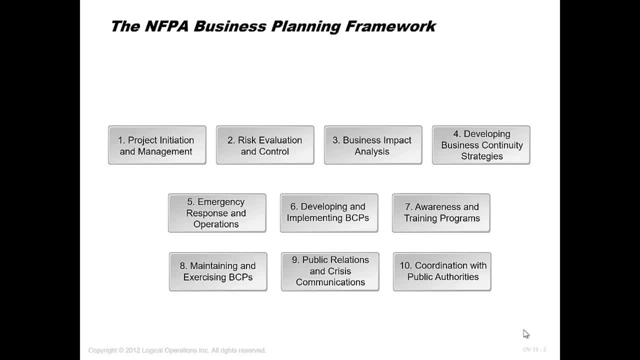 server or we need to buy some security appliance. so the BIA, this has figures. it will translate the threats and the risk and the compromisation into numbers and it will show the how our business will be affected. okay, now, once we created the business impact analysis- by the way, a very important- 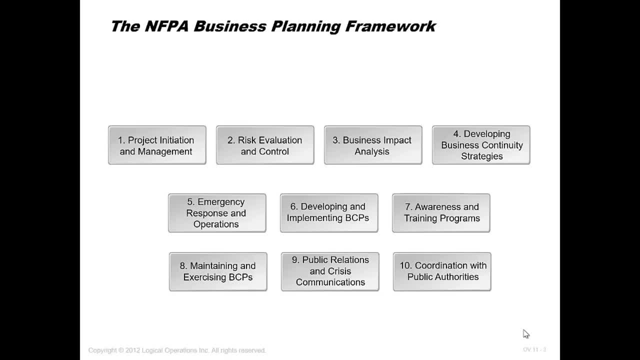 point is the sequence of the steps going to need to be memorized so you you may get asked inside the question, inside the exam: what is the third step to be done in the business planning or the business continuity planning? what is the second step? but actually I'm gonna point out that this is the content that I'm going to. 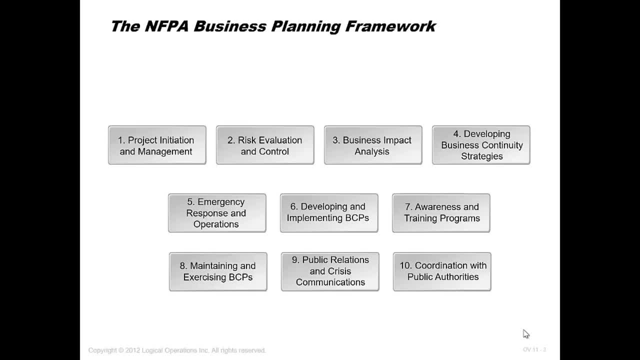 point to that from the sunflower once we finish this domain. after that we start developing our business continuity strategy. okay, so now I know if a problem happened, this would be affected, money wise or time wise. so I can say, okay, if a tornado happen, we will be off for few days, but we are a multinational company. 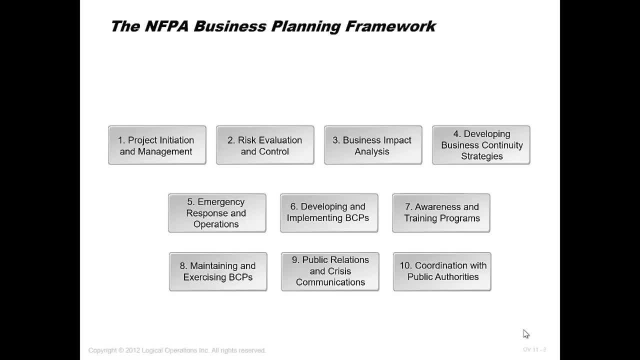 we cannot be off for few days, gonna lose a lot of customer. so our business continuity strategy will be to take another site in a different location and that doesn't have doesn't have this kind of problem and this would be stand on standby site. so my people will be moving here, but if a tornado happen I'll 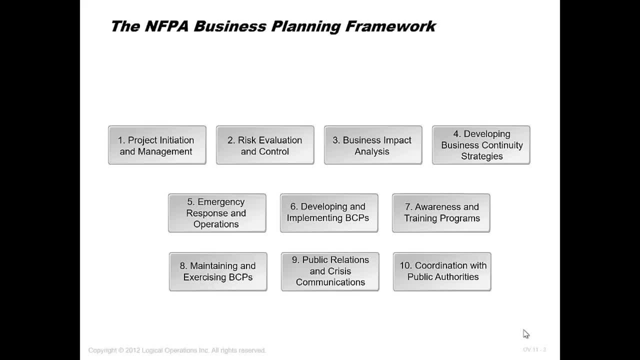 be moving my people there. this is a business continuity strategy. fifth step will be emergency response and operation. this is considered a very, very important step in this business continuity strategy. business continuity planning- because they consider the most valuable assets inside your organization- is people. it's not hardware, it's not information, it's 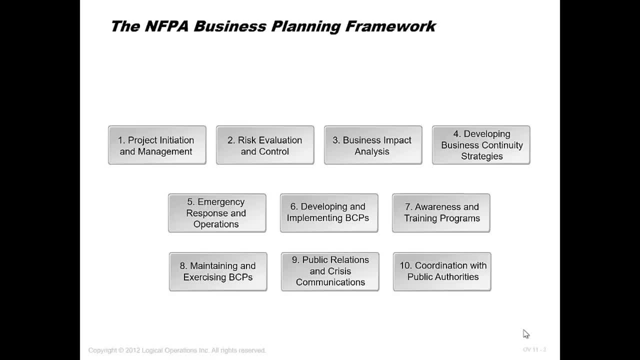 people. so the first thing that you need to do in the business impact analysis is to have an emergency response and operation. okay, how to evacuate people, how to tell them the assembly point after any kind of major disaster or problem. doing that, we gonna. after doing all the business continuity. 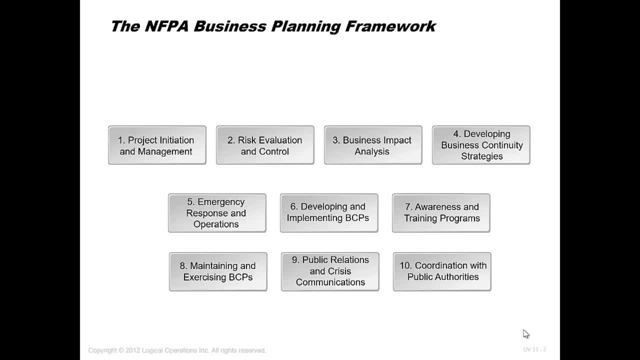 and emergency. you're gonna end up with a BCP or business continuity planning. now, after doing the business continuity planning, and how can we continue our business in case of any problem happen, and where should be the list of problem and the effect of problem? it will be in the risk evaluation and in the business impact analysis. 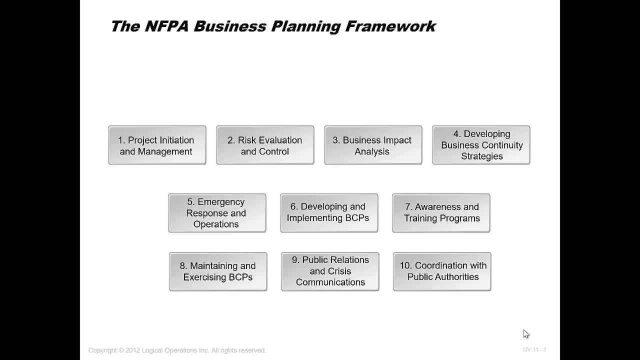 after doing that and have the plan, you should not put just write the plan down and put it in your draw. you have to do an awareness training program. people need to be aware of this planning so if a disaster happen, they know who to call or they know where to move. 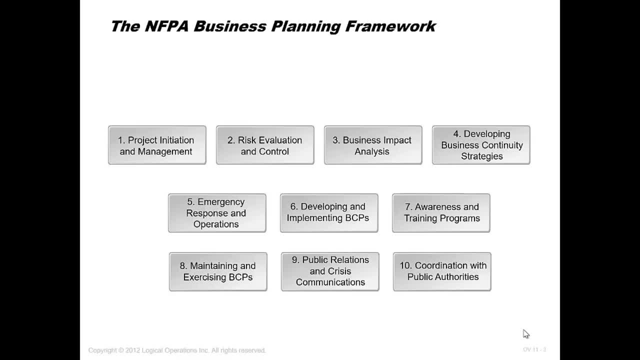 or say no, but if you do, the planning- even if it was in perfect planning and no one is all aware of it's- useless. so you need to implement awareness and training. program number eight it's to maintain that you have to check your planning at least one year. by the way, all the planning that we are talking about in the 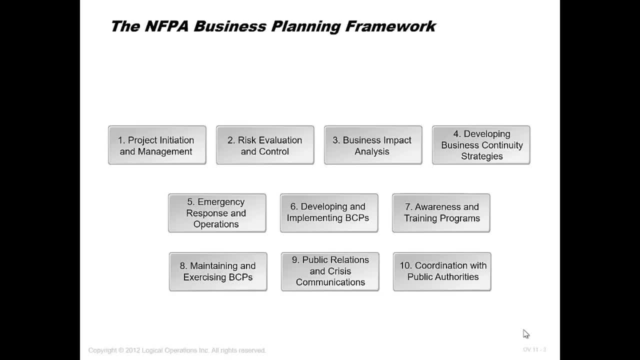 domain need to be reviewed one year, at least one time per year. why is that? because sometimes the factor or the parameters that you depend on- your planning does not exist anymore. for instance, assume that you planned that if a disaster happen, you gonna move your company. you're gonna move your. 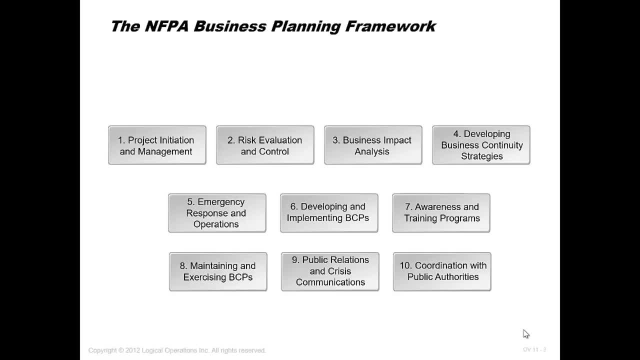 another location that you arranged and you can use a specific transportation company. what if this transportation company went after out of business and you you were not aware of? so if a disaster happen, you try to call them. they are not there, they went out of business. that's why you need to. 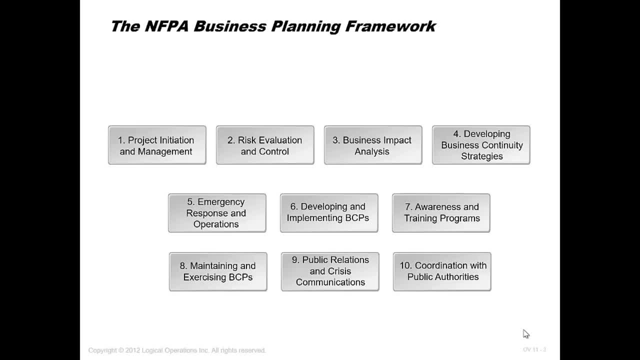 maintain. you need to review that at least one period to make sure that it's still applicable and nothing has been changed. number nine it's to inform the public relation and number ten it's to communicate with public authority. this is, you know. in case for major things- fire department, police department- you need to let them aware by 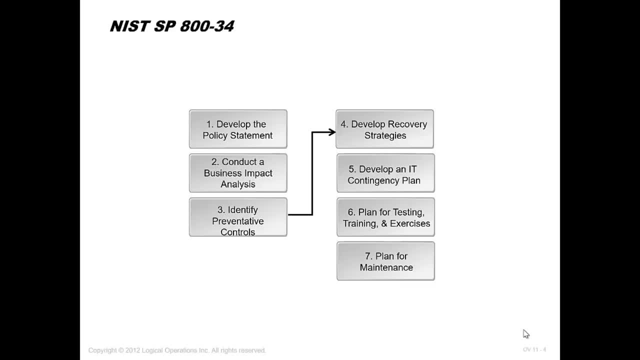 your planning if a problem happen. this is another framework and I believe this is the one that you need to memorize. the number nest publication 834, and it's similar to what we explained, maybe less, but it's similar. you are developing a pilot statement, you are conducting a business impact. 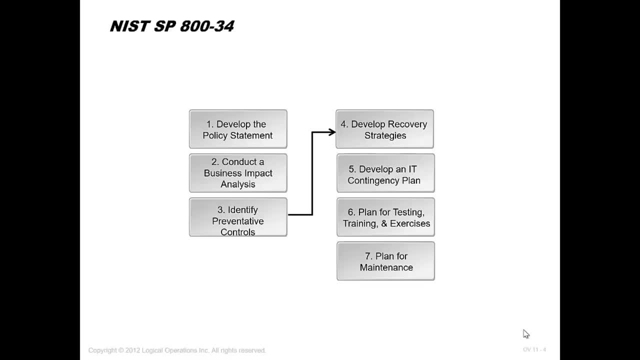 analysis and if you need to memorize steps, it should be from the nest, not from the first one. so don't forget that. the second step it's to conduct a business impact analysis and then identifies a preventive control, develop recovery strategy, develop an IT contingency plan on step. 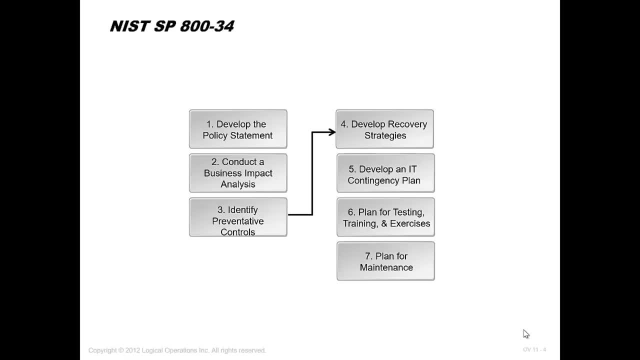 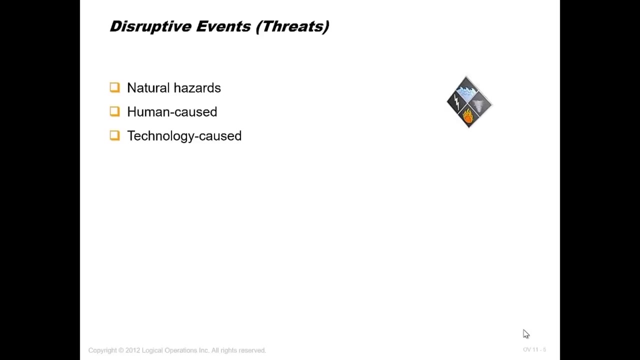 number five: this is where the disaster recovery planning will come: plan and test and training and plan for maintenance. so this is the ones that you need to memorize, but I explained the first one because it was more detailed and I want you to be aware of such details. 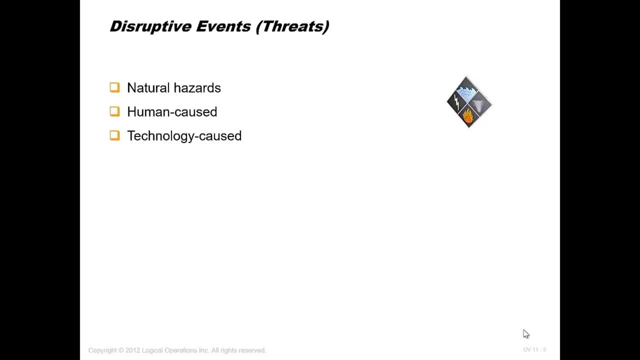 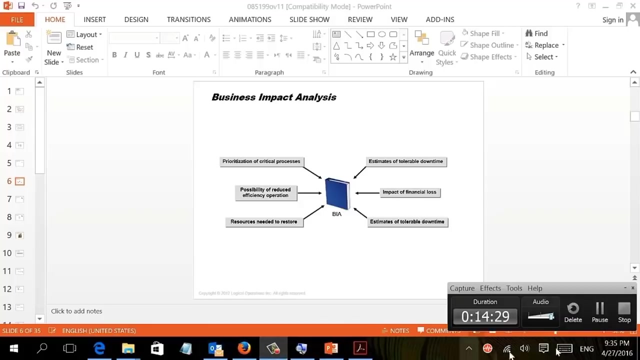 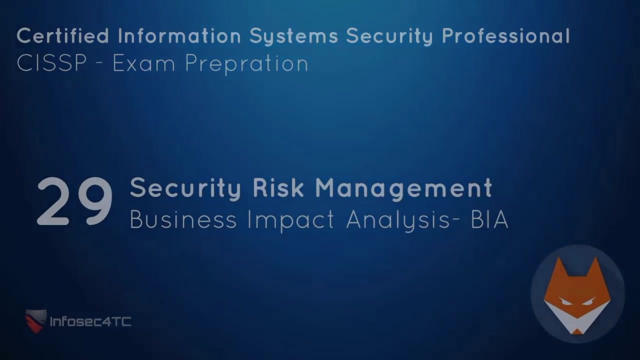 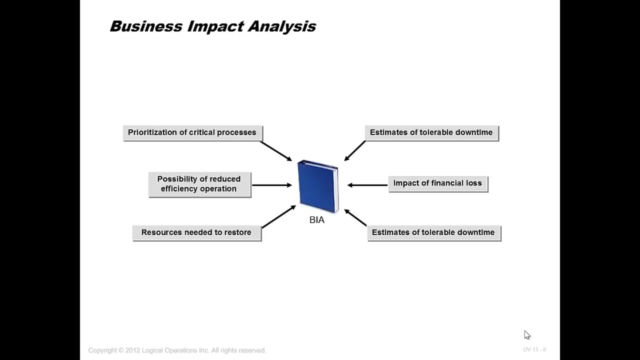 the threats that we may expect could be natural threat, could you could be human caused, could be technology caused. so you consider, while we are doing the risk assessment, all kind of threats in a sense. so, as we agree on the previous lecture, what is the most important document inside the BCP is: 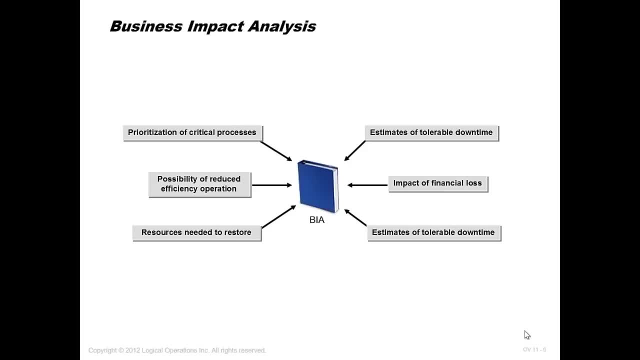 the PIA or the business impact analysis, what exactly you should find, size the PIA, you should find and list of all the business function inside this organization. so it will explain how's a business is going first: if it's a finance organization, if it's a broker, a stock exchange. 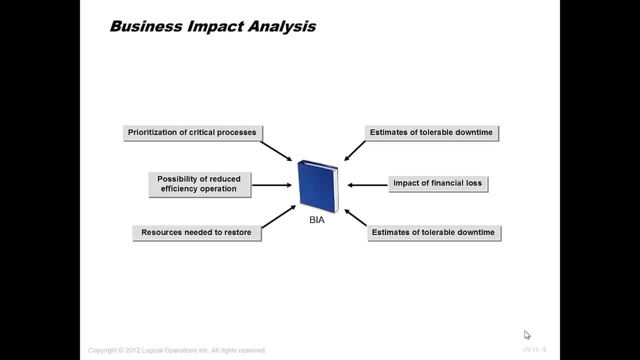 broker- if it's a training center- how the business is working, how the process related to the business is working. so it will first explain the business and this is not easy to do. i mean, you have to understand very well how the business is running and in real life you have to do a lot of meetings. 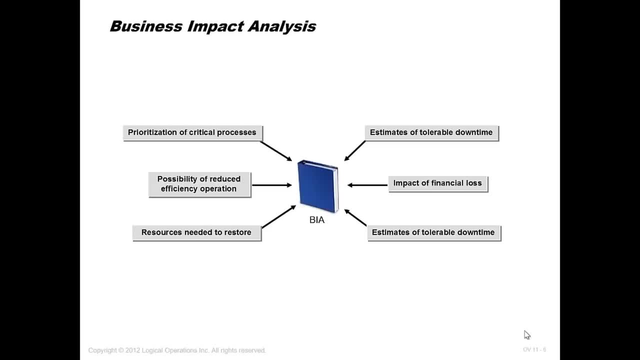 with different department to understand if you are coming outside the business, if you want to understand how the business is going and what is the important function of the business. so you need to identify the business function of the business. like the previous example we explained on the previous video, if it's a training center, you're going to need to know how the training is going. 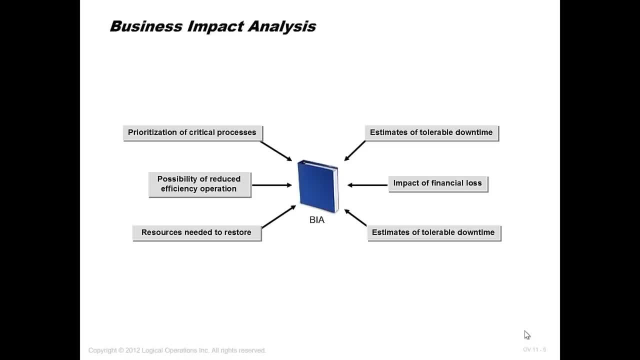 from the start. student came for registration- where they register, and then those information- how they will be saved and to how they will be creating a course and inform the instructor and request the material. according to that, you'll be knowing the main business function and then you start giving them priority. what is the most critical? 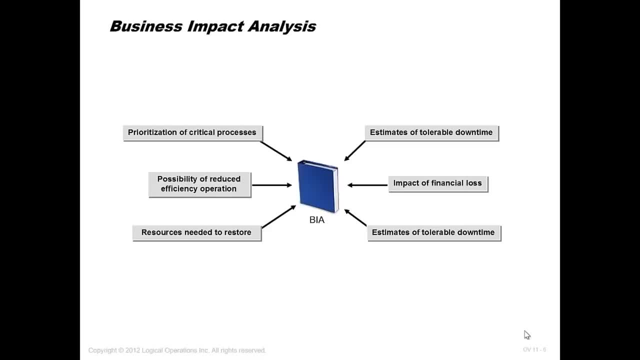 business function. what is the business function? that if it doesn't exist, it will stop the business. but you need to put that with figure, with numbers. so, as you can see, you need to have a list of business function and you need to give them priority. you need to possibility of reduce the efficiency of 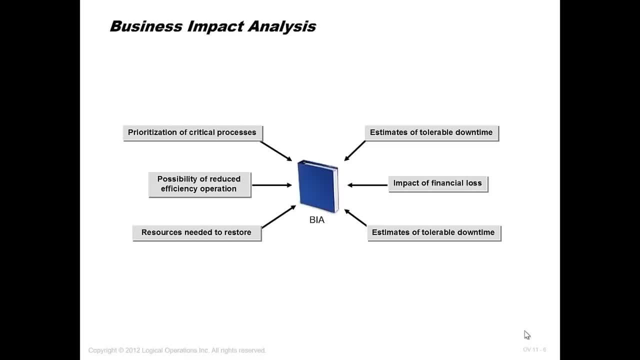 operation. we're going to see an example in a few slide. you need to identify the resources needed to restore if a problem happened. to restore the business function or our business, what resources is needed- technical resources, human resources and so on. you need to know the estimated tolerance. 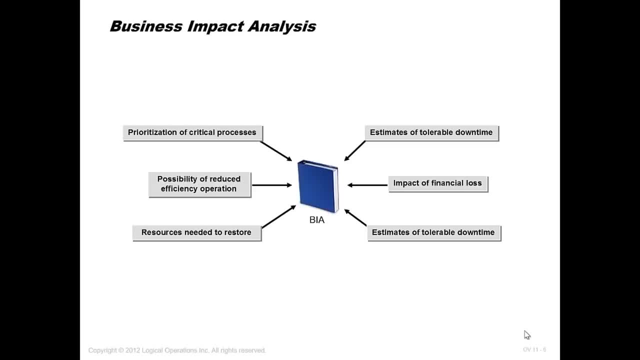 time. we're going to explain this concept on the next lecture. this has some numbers, but the most important thing for management is the impact of the finance impact. so this need to be very, very clear. if this problem happened, how much the company will lose. because you can identify a 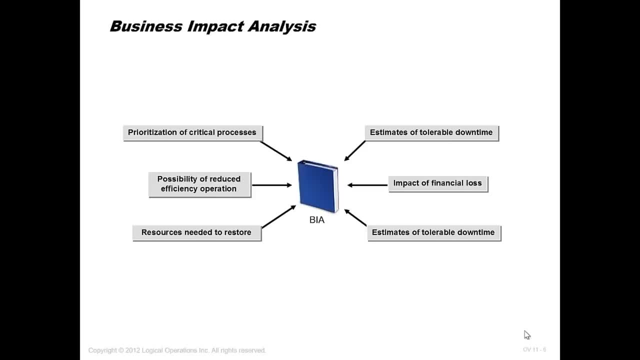 budget according to that, if you're going to lose 1 million, if, for any disaster happened, so maybe you need to allocate eight hundred thousand dollars to restore the business. so you need to know the amount, or maybe you need to look at less than 1 million. but i cannot allocate 2 million from my 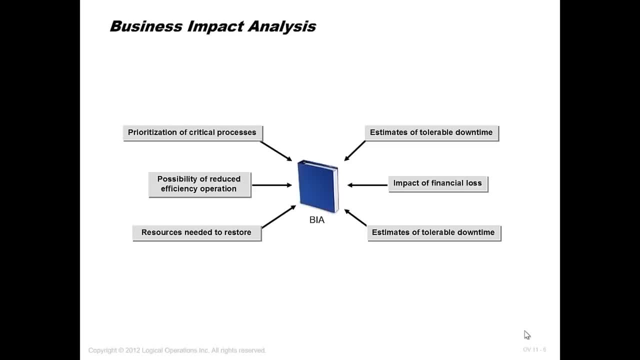 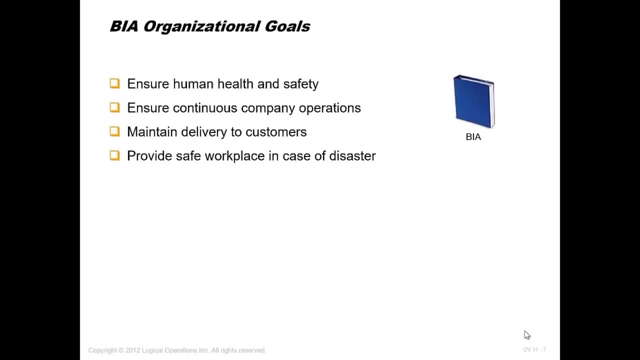 budget for some things that will have an 1 million finance impact. so the business impact analysis is very, very important. it show, as i told you, how the business is running, where is the weak point and how to recover the business and what is the resources needed. don't forget that human is considered number. 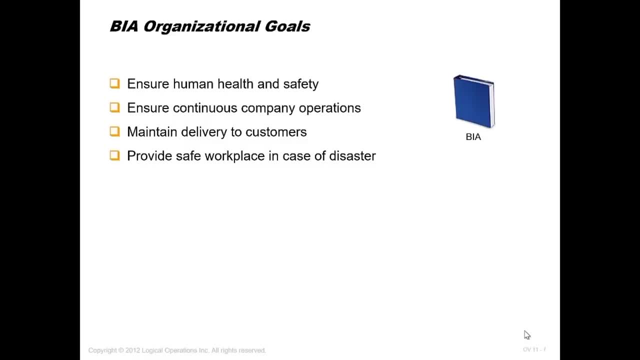 one. so inside the bia, you should also consider a human factor: how to make sure that they will be safe for any disaster and it make as a goal of bia. it ensures that your business will continue. according to this document, you're gonna plan for the bcp and you're gonna make sure that if any disaster happen, you will still run your business. 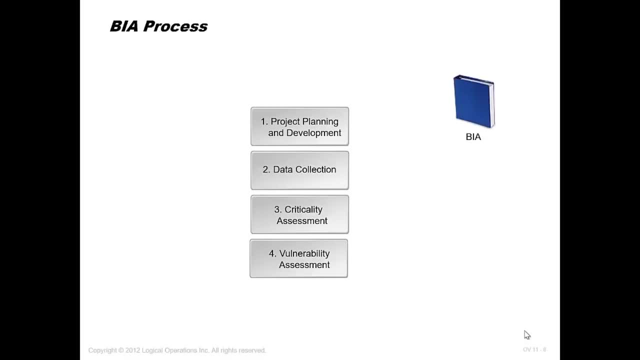 so this is actually a very, very important document. the process of doing that number one again it should be project planning. so you should start by planning, for the bia has a start date and end. it should not be an endless process, because you know i work with 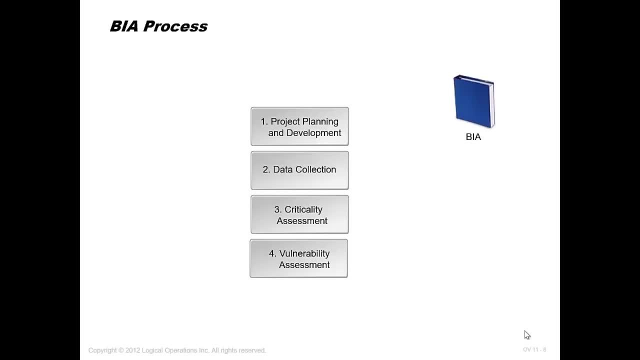 couple of those process- and, by the way, i'm going to share some template with those lectures- and unless you have a plan, it will end up meeting with meeting, with meeting with different department. so planning need to be done, done and project planning: it should be done as a project you have. 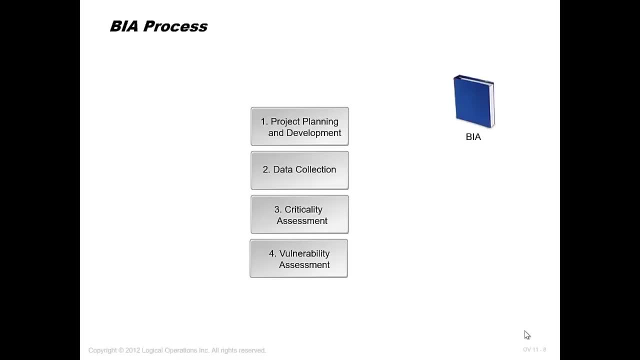 someone responsible for this project and you have a timeline. this project should start on date and end on date, and before that you should have a management support. unless you have a management support, no one will obey, no one will give you any information. you'll have very, very hard time then you need to collect. 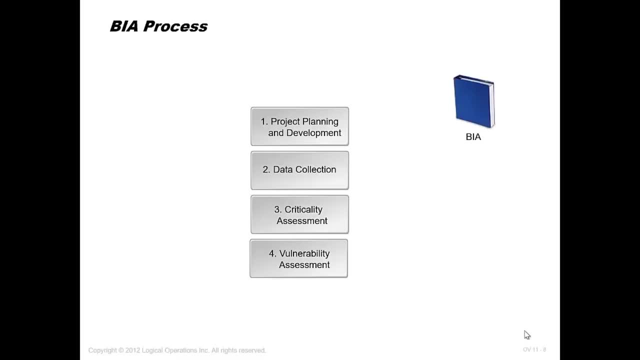 data. I mean, how can I know? you know how the business is running, what is the income if the problem happen, how much you're going to lose? so you need to collect data. you can do that by interview, you can do that by survey, you can do that by observation. but you need to collect information. do not 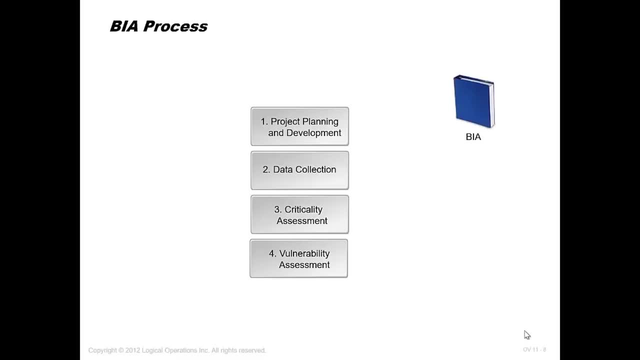 take only from one source, sitting with someone who will give you some information, so you build on that. you have to take from different resources and compare between them because, realistically, whenever you sit with some departments, they will give you the impression that they are the most important departments. 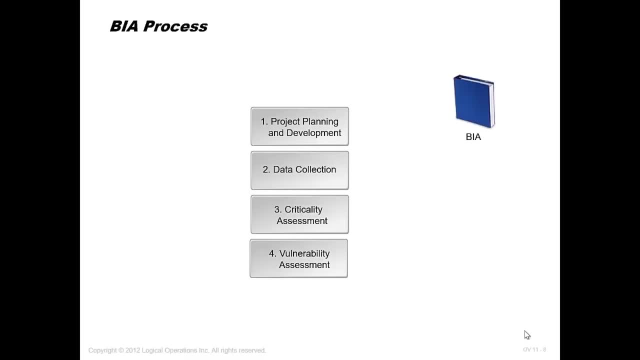 in the organization and without them the business will not be running. even you know departments that is not that important. they're going to do that, so you have to do your own observation. you have to collect information from different area and you have to analyze it, and they usually 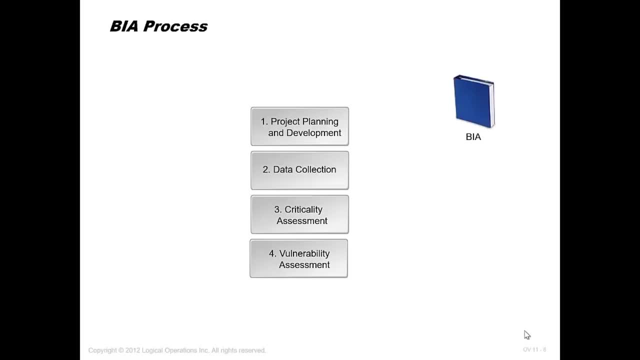 say, if you need to work on this field- business continuity and disaster recovery, which is well, well, well in demand today, has high demand today- it's better to start with an expert. I mean, do not take a course or read a book and then go and do a business. 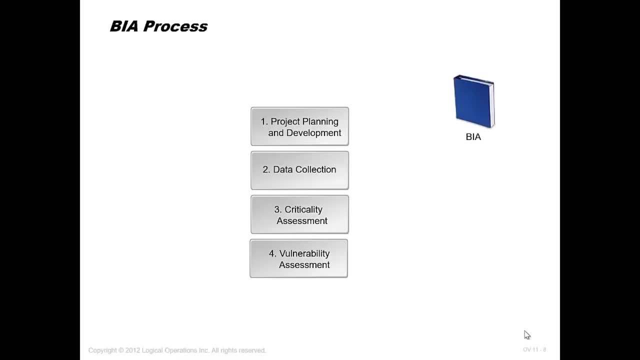 continuity planning for any organization because it's a little bit complicated process, realistically and you don't to take any risk there. I mean, I don't have experience. I go to organization, I'm gonna tell them that I'm gonna do for you a BCP and then you start going through what you read inside the book. 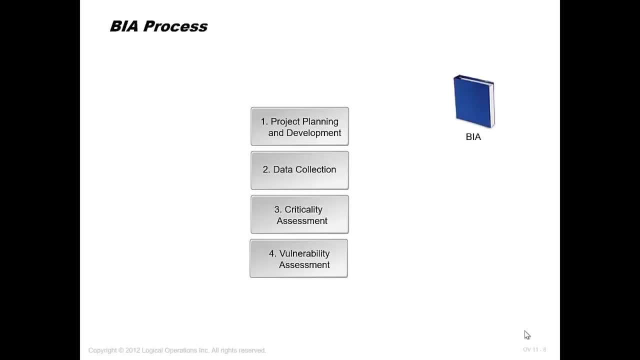 and a disaster happens they try to implement. this plan is not working, they will take some legal action against you. so if you need to work on this field, that it's as I told you. it's a well demand field or high demand field, it's better to start with an expert. so we 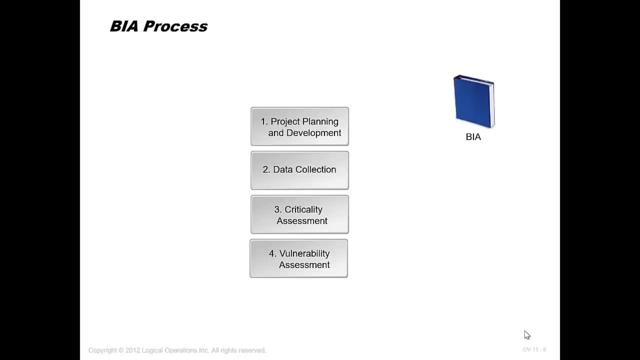 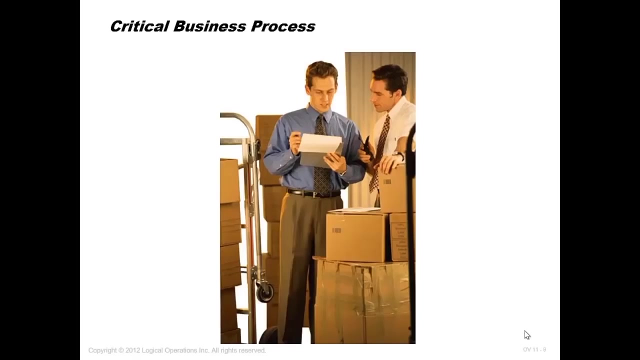 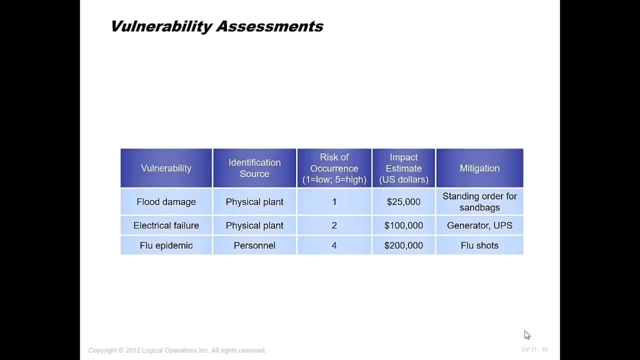 are talking about data collection, the critical assessment and vulnerability assessment as well. so we are identifying what is the important assets that we have and what vulnerability you are expecting. this is the BIA critical business process. this is actually one of the vulnerability assessment model or example. so, for instance, as in several the vulnerability 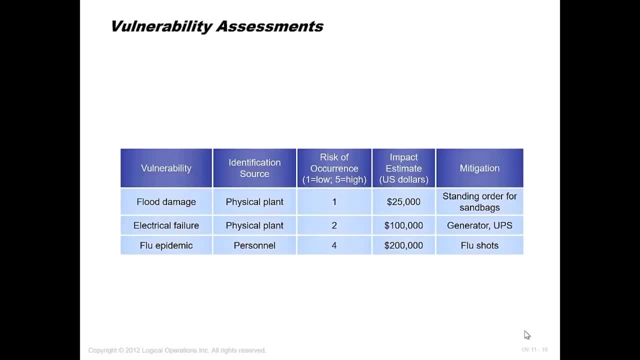 could be a float damage, damage happen for floating. this is what this is: a physical vulnerability. okay, the risk of occurrence? this is, as you can see, qualitative and they are giving from one to five. look where one is low and five is higher because this happened every 10, 15 years. so the probability of happening, 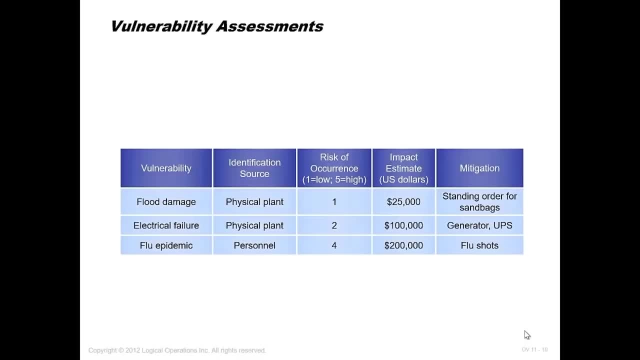 is one. okay, if it happened, what is will be the impact on our business? it will be 25,000. and how to mitigate that, how to reduce this risk? it's to standing order or, you know, sandboard or sandbag or whatever control you're gonna put okay. 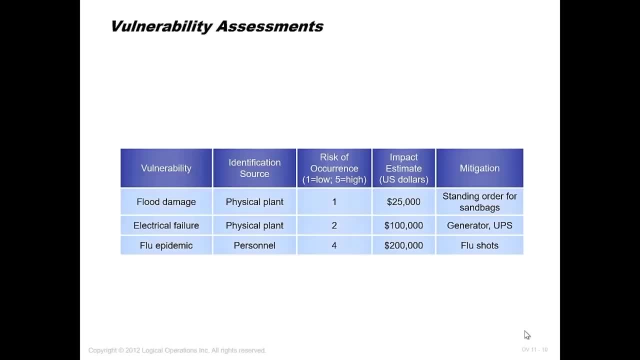 second one, electrical failure. this is a physical and it happened from time to time, so I'm gonna give them a risk occurrence of two and if it happen, what will be? the impact will be one hundred thousand and how to mitigate that in the generation. when you give them to management, maybe they will accept some. 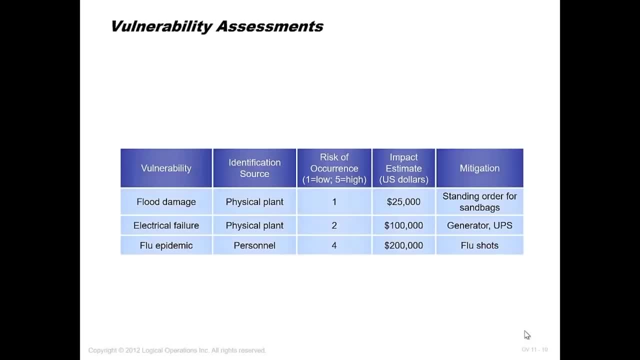 and do not accept them. so they may. for the second one may mitigate. they spend 100,000, but the first one because the risk is so low so they can. we're gonna accept that, if it happened you're gonna find a workaround, and so on and so forth. 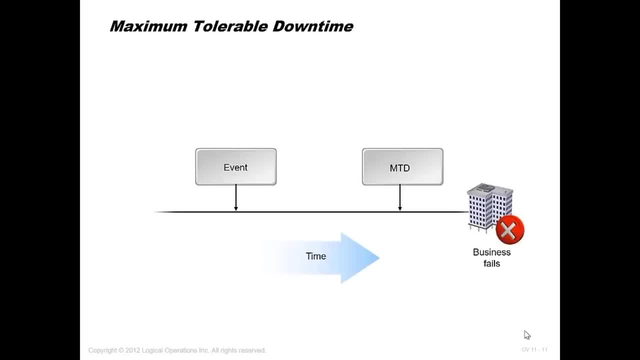 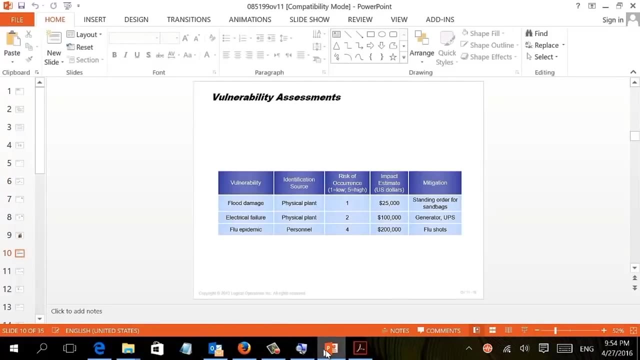 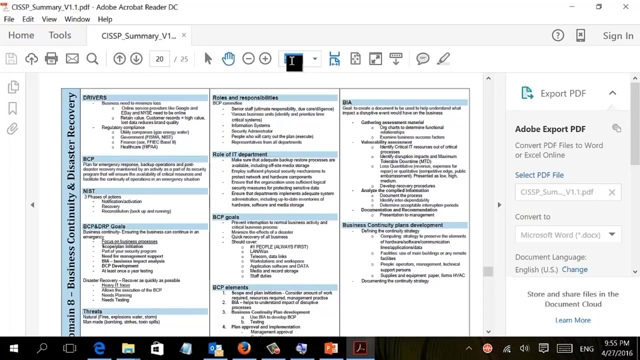 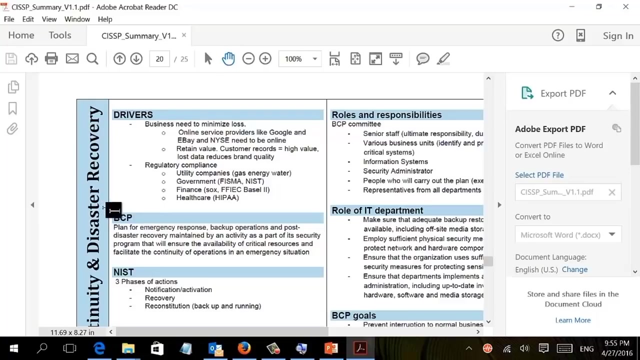 so this is an example of a vulnerability assessment. now, before going to the next lecture, I just want to show you the BCP from the sunflower and what exactly need to be memorized from them. so let me just increase the size a little bit. so the business how, why we are doing that to. 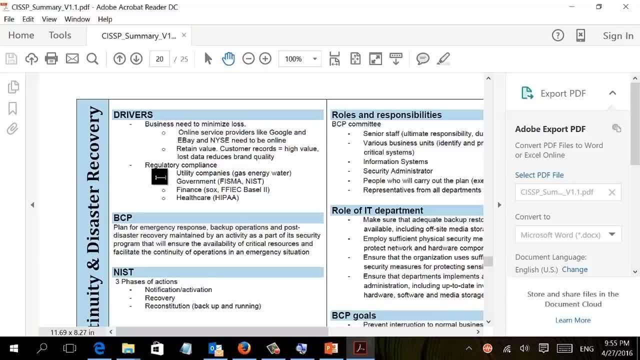 have lit to reduce the downtime of our business, to make the business working. the BCP is now government requirement in some country. I mean, if you are a supplier for government, they will tell you before we work with you as a government, we work with your private organization. you have to show our, show us our business. 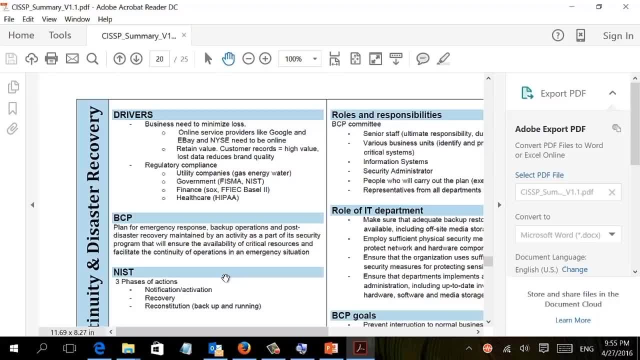 continue your business continuity planning because if something happened to your business and you don't have a plan to recover, you're gonna affect our business. so now it become more as a government requirement and major company requirement. so it became very, very important. that's why I told you it's in. 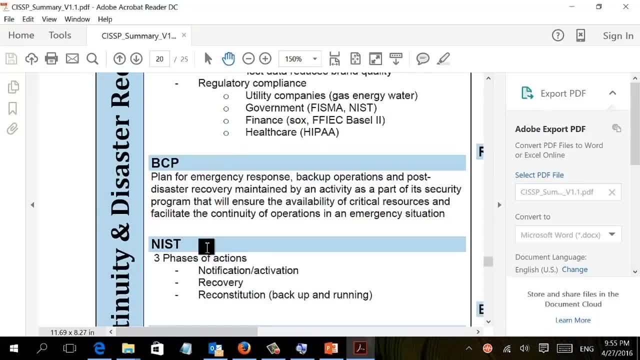 high demand in the market. so we are doing that, for it's a business document, and don't forget that the first thing that you need to do inside the business is the emergency response planning. so first thing inside the BCP is not how to recover the business, is how to make sure. 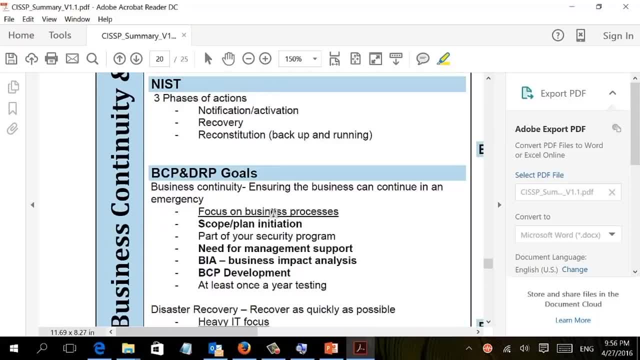 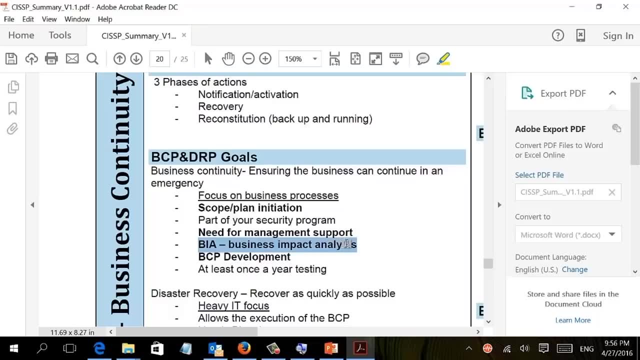 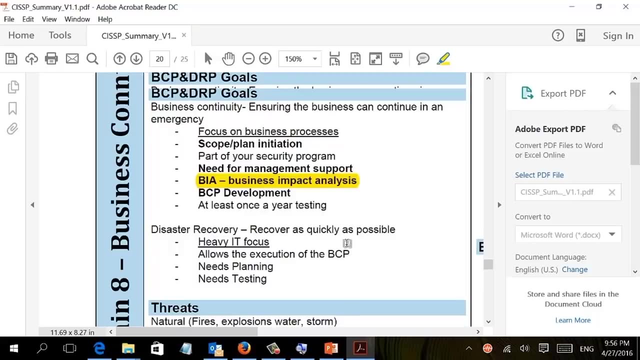 that people are safe. what is the scope? the BIA: it's a very, very important document. you should know what is inside the BIA. okay, business impact analysis has risk and it has business functions or priorities lost. so the BCP, as you can see, it's a business document, while the disaster recovery it's a technical. 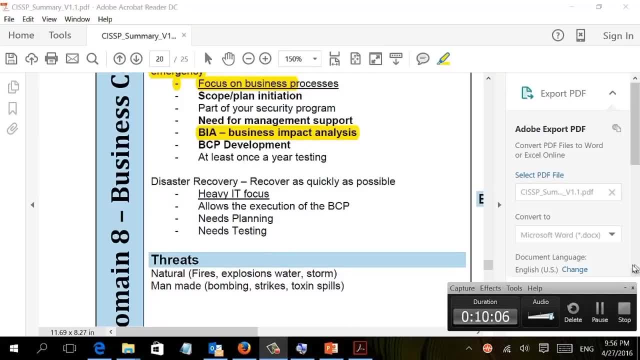 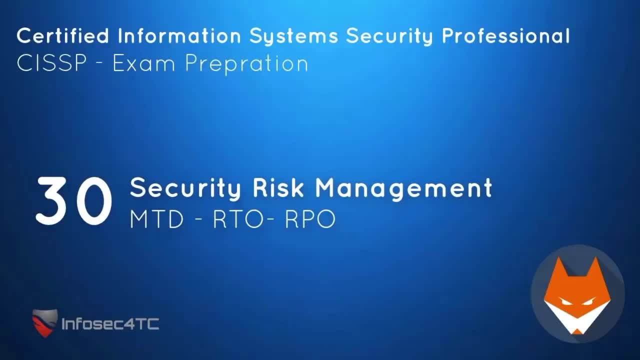 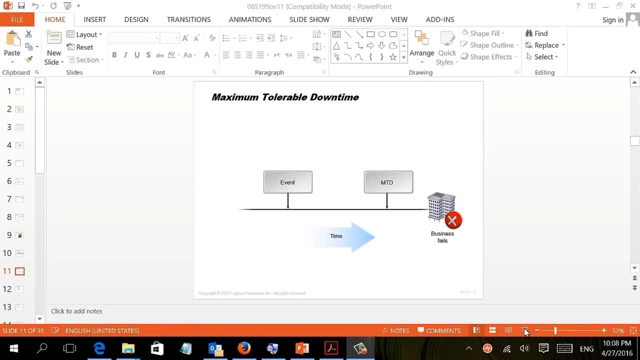 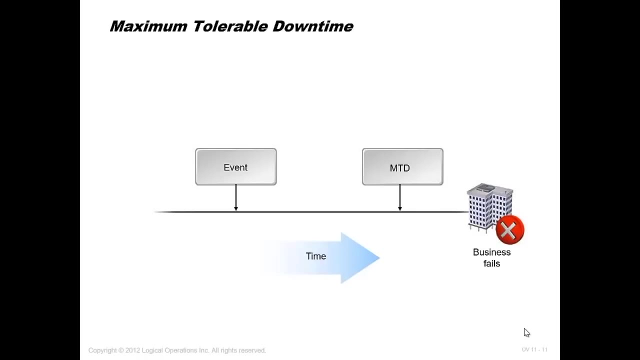 document. you can do it online. what do you need to do to recover your business continuity plan? what is the first question? you ask for management before starting to work on a planning and collecting information. so MTD, it's a maximum acceptable downtime for any organization and this number should be coming from the management. so 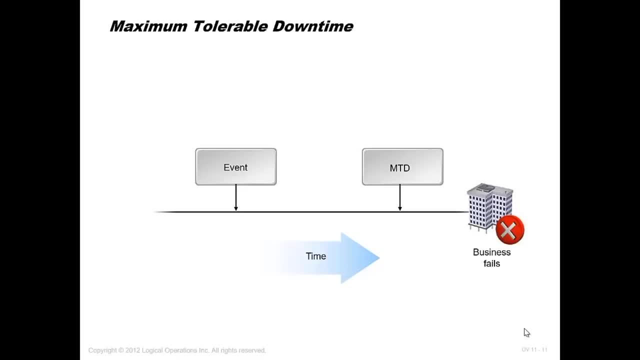 you're gonna sit with the management at the first meeting and he is, they, gonna tell you: okay, our organization, MTD, is going to recover its business continuity planning from any organization. and then another thing: you should know that when mtd it's five hour means that we can be down. we will accept to be down for maximum five hour. 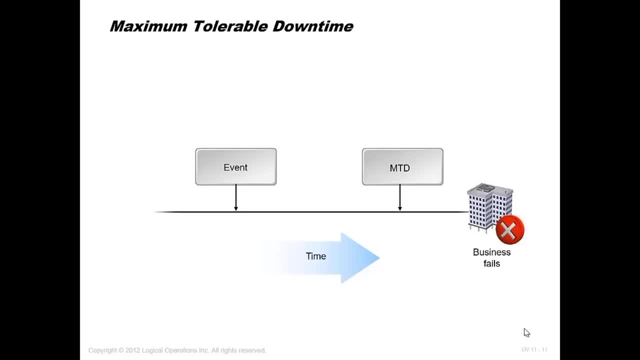 but we cannot be down for six or seven hour. our downtime, acceptable downtime, it's five hour and, as i told you, that should be coming from management. this, this is called the mtd. so which is the maximum acceptable? uh, maximum tolerant downtime accepted, accepted by management and they will tell you: do whatever it take to make sure that we will not be down more than. 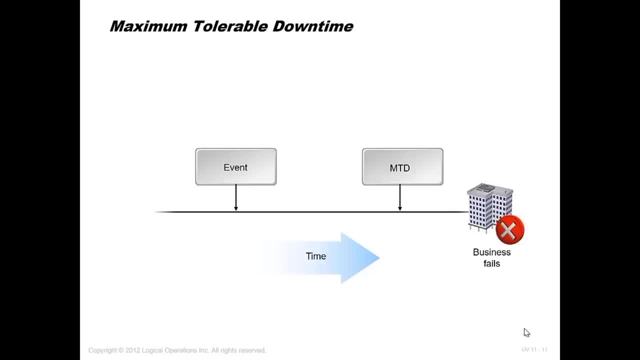 five hours. so whatever problem happen, we can afford to be down for this amount of time. some of them will be lower. like you know, government or law enforcement they cannot be down for like six, seven hour. they will tell you we can be our down for 30 minutes, for instance. 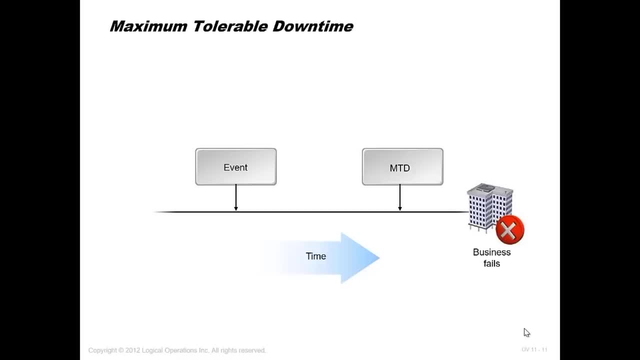 so the maximum tolerant downtime, or the mtd, it's acceptable downtime by management. now let me first go to this one. so assume that, okay, you sit with management and they told you that the acceptable downtime it's, or the mtd is five hour. so you said: okay, let me test, let me see. 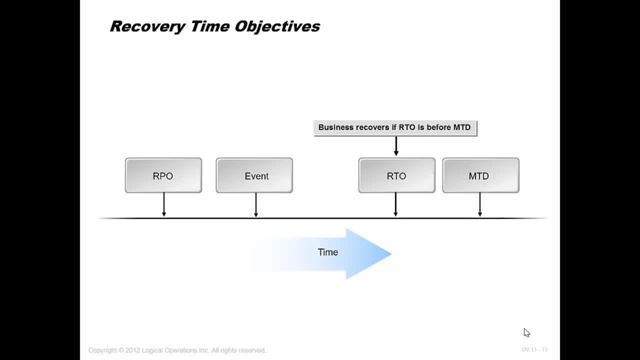 how can i recover the system? so you start doing a scenario, you crash the system or you do whatever scenario, and then you try to restore the business and to get functional again and then you try to recover the system again. it take you seven hour. so the realistic values that you are testing it. 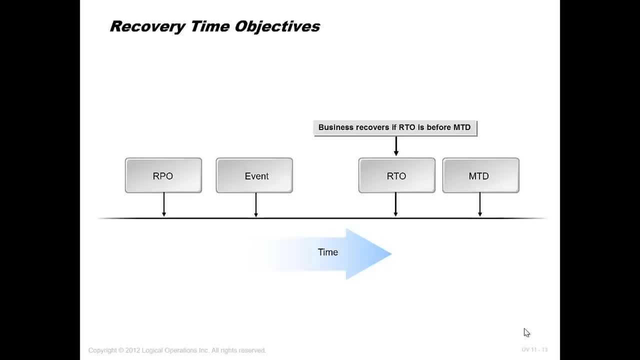 take you seven hour. what do we call that? it's called the rto or recovery time objective. so rto it's the values that you are giving based on the testing. so management told you it i need to. uh, the maximum amount of time i can be down is five hour. you did your test and you tried everything. 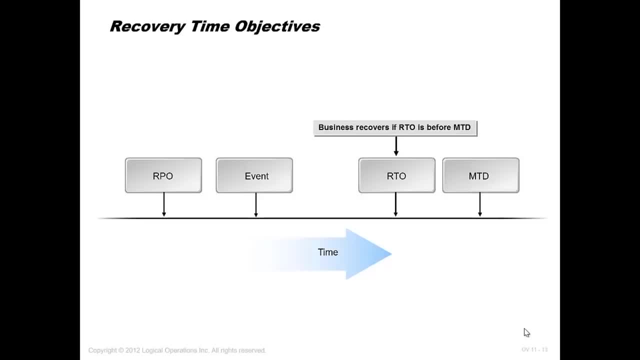 and you cannot be up before seven hours. so you go to management. you said i did according to the resources i have, i cannot be up before seven hours. this is called the rto. definitely, definitely. what will be your objective? to make the rto equal the mtd or to make the difference between them zero. so this: 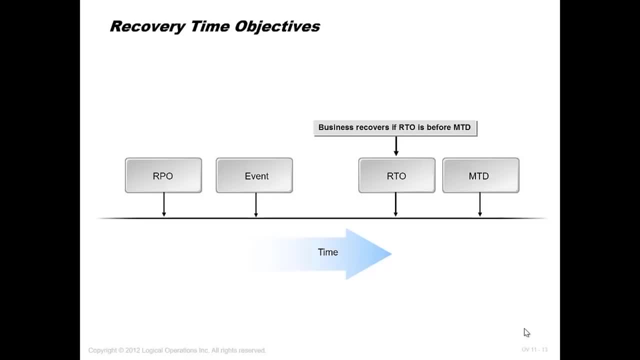 will be your objective so you can tell the management: okay, if we need to decrease those seven hour to five hour, maybe we need to spend more money because you requested to be down five hour. so first terminology is mtd. second terminology is rto. we have a third terminology. 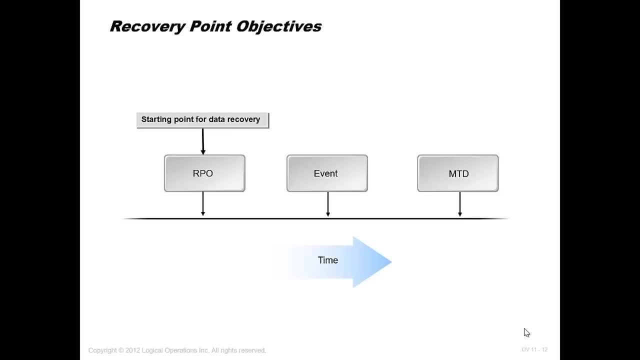 it's called the recovery time, recovery point objective, and this is related to backup. how frequently should we taking a backup? if the question came asking about a value related with backups, the keyword with backup is the rpo. this is related to the amount of time where we need to. 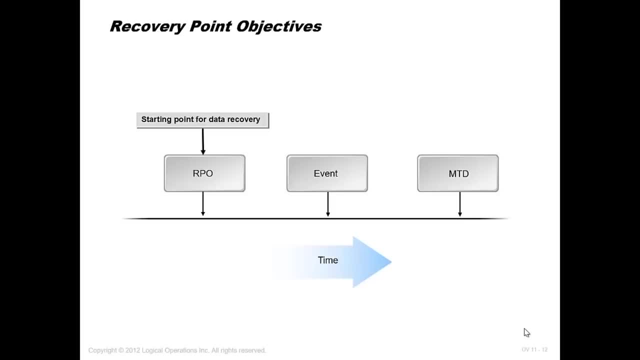 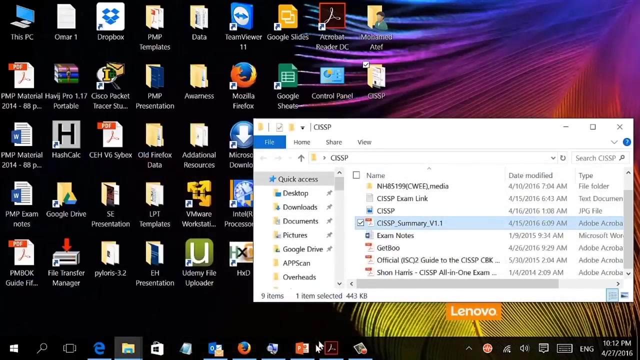 take backup every hour, every two hour, because according to that i can afford to lose the data for one hour or 30 minutes depend about how frequently i'm taking backup. those are three important terminology, but i need to add two more terminology from the sunflower, which is mean time between failure and mean time. 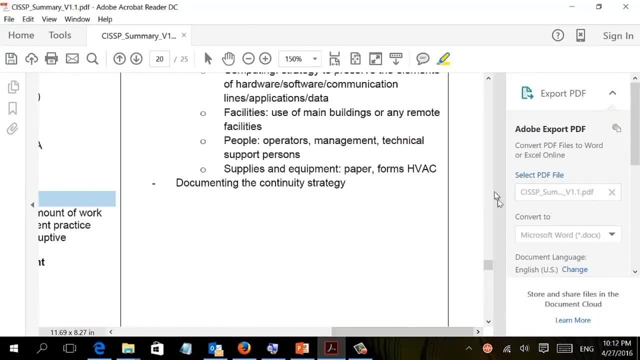 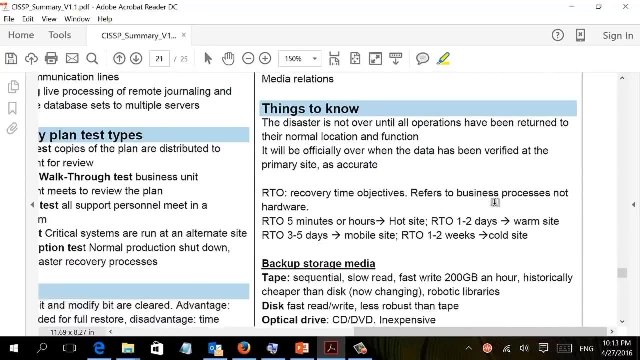 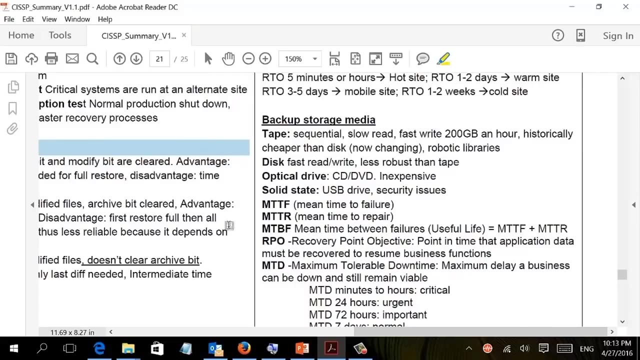 between repair. so let's go here and let's go to the last section. here those value are very, very important. definitely you get question about set inside the exam. so we spoke about the mtd, the rto, the rpo. now, those time we are those concept, which is mean time between 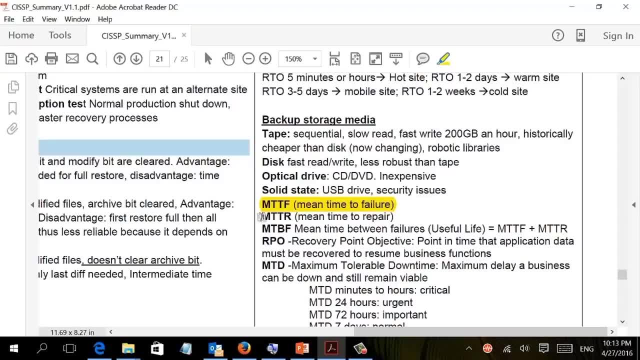 failure. and mean time between repair- what exactly does mean and what need to be increased and what need to be, because most probably he will not ask about definition or this is stand for what, but he will ask you: what do you need to increase and decrease? now, mean time between failure. it's the time between a failure in any system- for instance- assume that i have a server- and from the previous experience and for the previous, from the previous. 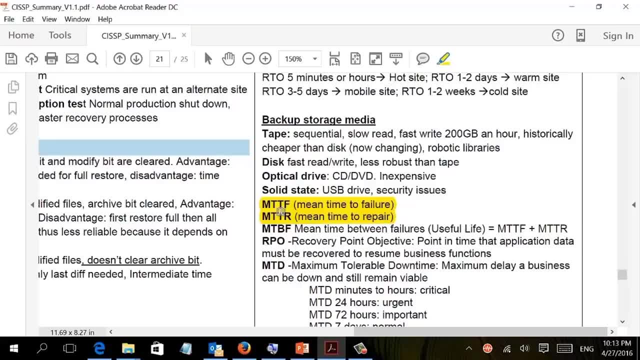 history, i know that this server fail every six months, so the mean time between failure is six months for this server. okay, now, what will be my objective? definitely, my objective will be to reduce- i'm sorry, to increase- the mean time between failure. so i need to have the 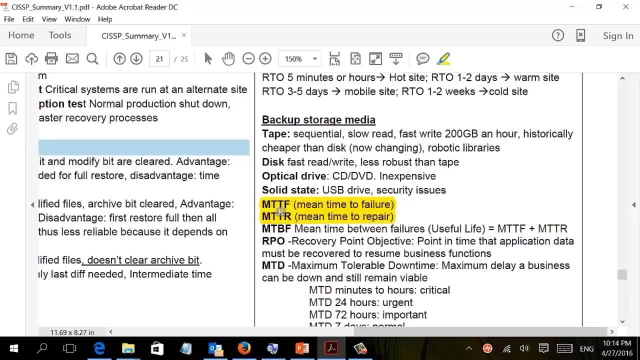 failure every one year, every two year, but not every six months. i need to increase the mtcf while mean time, uh, to repair its amount is take you to repair the server. so assume that i know that the server will fail every six months or seven months frequently, but it take me one hour three hours. 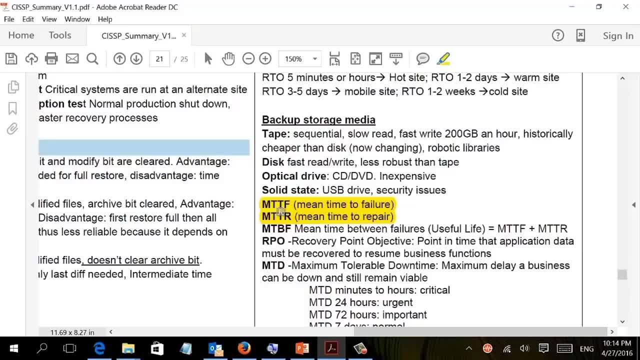 to repair it. so I need to decrease this amount. so MTTF need to be increased, while MTTR, which is the time needed for repairing the system, need to be decreased. don't get confused about that. take notes about that, because it's very, very important those terminology for. 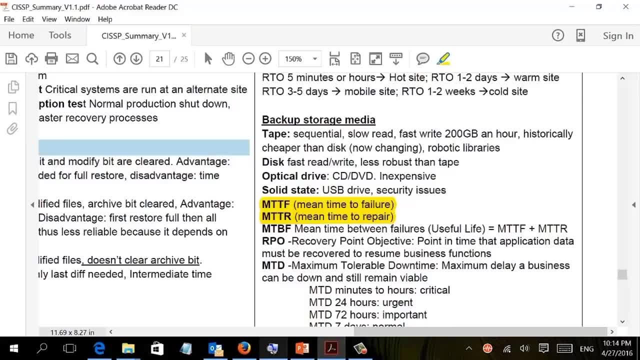 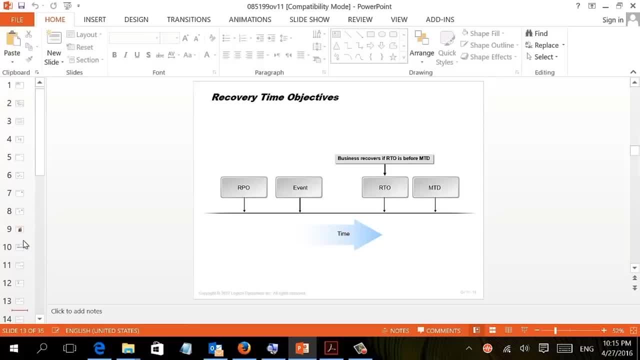 the BCP. so the terminology are very, very important when it come to the business continuity. when we are doing a BCP, you need to have someone in charge, because you'll be doing a lot of work, you'll be sitting with a lot of people, so someone need to be in charge. we do not call it a project manager. 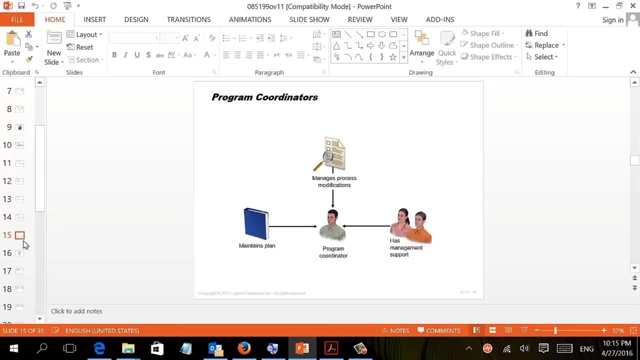 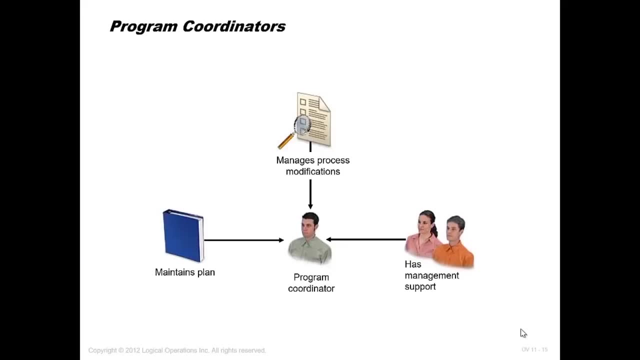 it's called the program coordinator. so program coordinator is the one in charge for the BCP and he is the one who is planning and who's assigning assignment to the team and doing the resources, and he will be the one accountable. so if a problem happened and the plan is not working fine, he will be the one responsible for. 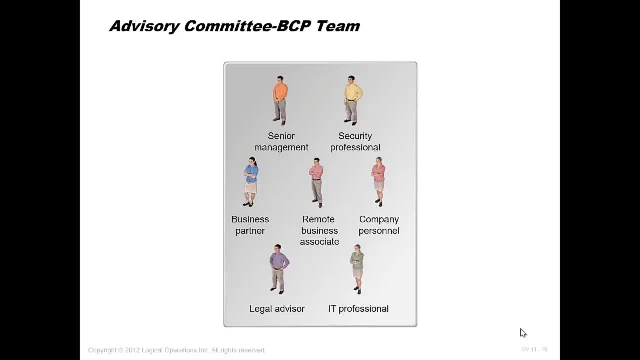 that this is the BCP team and it should be have people from senior management, from security, from business partner for remote businesses, from IT, from legal and I think, if it's a government sector, they should also have someone from PR, because if a government, a disaster happen, of the 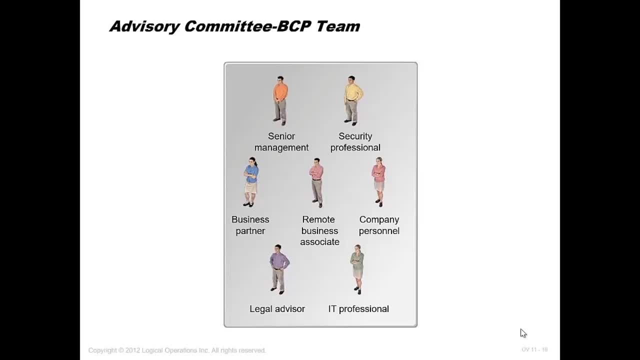 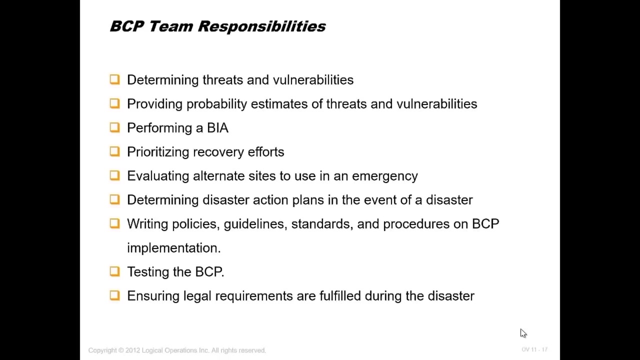 government. someone need to go to the media public and explain what is the situation, but if you keep everything secret, this is definitely will affect their business and people will start losing trust in that. okay, this is their responsibility, the ones that we explained. and one more time, do not. 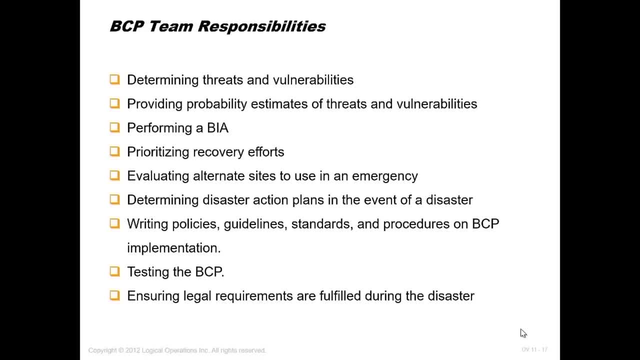 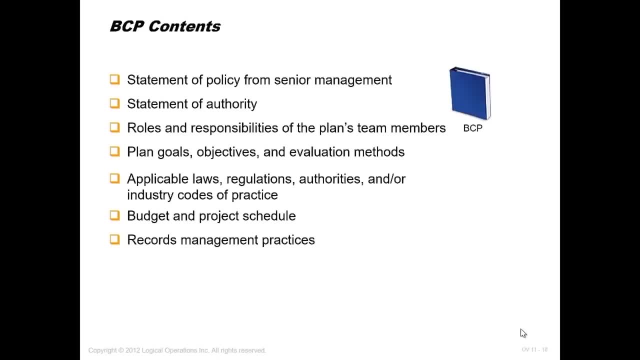 forget that people come first. so, whatever BCP need to be implemented, the first thing to be done is people planning now. this is the content of the BCP: is a statement, statement of austerity, role and responsibility, plan, goal and objective, applicable law, regulation, everything it need to be. 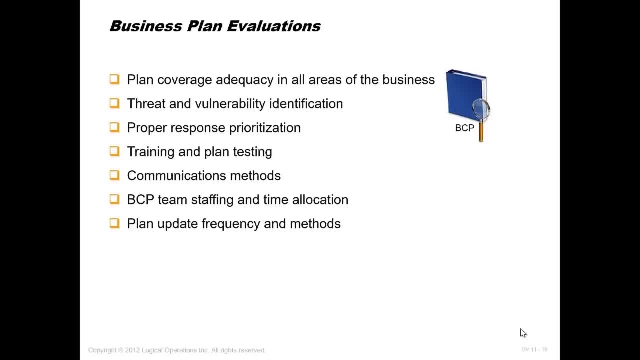 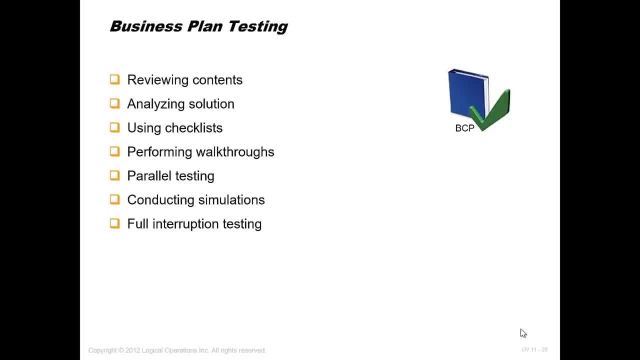 applicable and that all is the resources that are depend on it still applicable and that all is the resources that are depend on it still okay. now, when you do a BCP or DR, it need to be tested, otherwise it will be something academic. so we need to test and we have different way for testing. so 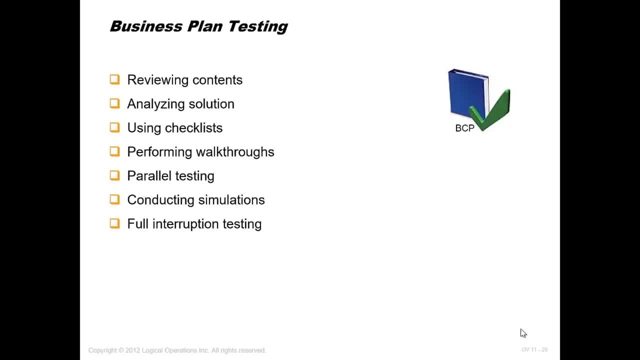 for instance, we have a full interrupt test, that we are simulating a real disaster and do a full interrupt. this will involve transporting people to other places and recovering and it will take time, but you have to do that. we have another kind of testing is called the walking through testing, which is just 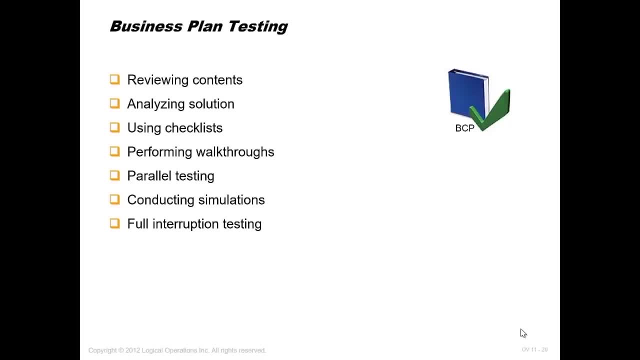 sending this plan to different department and they will check if it's applicable or not and sign. we have a parallel testing. you are keeping your business running but you are doing a parallel testing on a similar side. so there is different kind of testing for the planning and you need to implement. 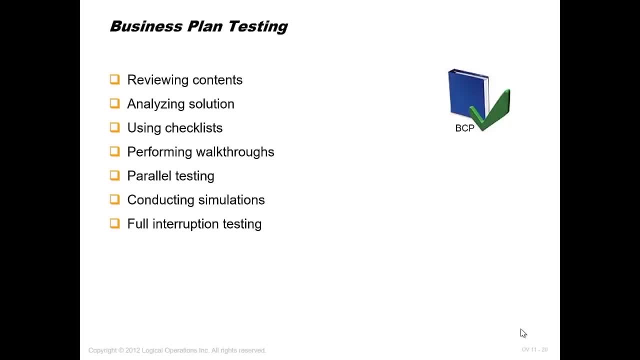 most of them, especially the full interrupt, because you need to see if this plan is realistically or not and it need to be maintained, one per year at least. okay, so before going to disaster recovery, to close the BCP, as I told you, the business continuity planning should have some plan inside and one of the important plan is called 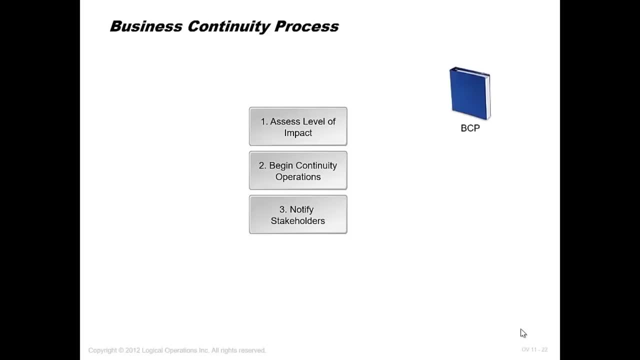 the emergency planning. so the emergency planning will explain it's a sub plan planning. so the emergency planning will explain it's a sub plan. the bcp will explain what should be done for evacuation and for making sure that people will leave or will will be evacuated in a proper way. now here is the question i saw inside the exam. 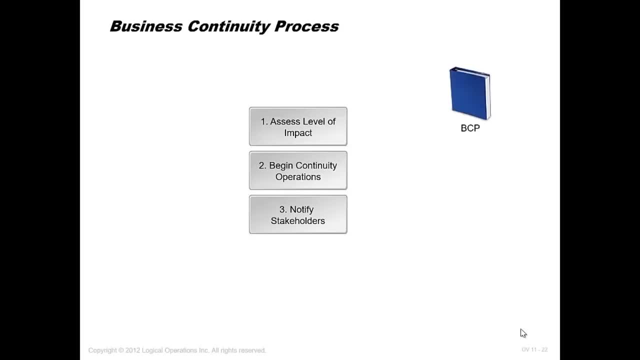 they are telling you, if a disaster happened, what should be done first? first, number one: evacuate people. number two: implement the bcp. number three: uh, implement. whatever. i mean. let's talk about one or two- evacuate people or implement the bcp. what do you think? i believe some of you may think: evacuate people because people come first, but actually you should. 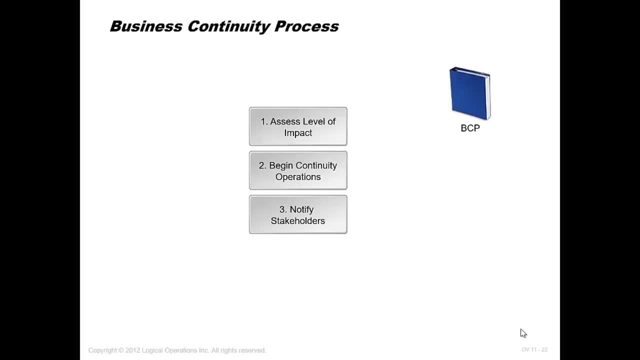 first do the bcp, because inside the bcp it will have the plan for evacuation, because you cannot keep screaming to people: evacuate the place, they will. you're gonna have a lot of uh damage and people will will hurt themselves. it should be done according to the. 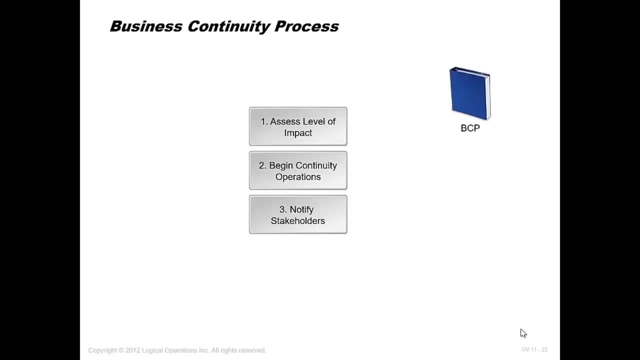 plan. so the evacuation plan is a part of the bcp, so it should be done according to bcp. it should not be done randomly evacuating people because unless it's planned, it will do a lot of damage. so don't get confused about this kind of question. everything should be- should be going according 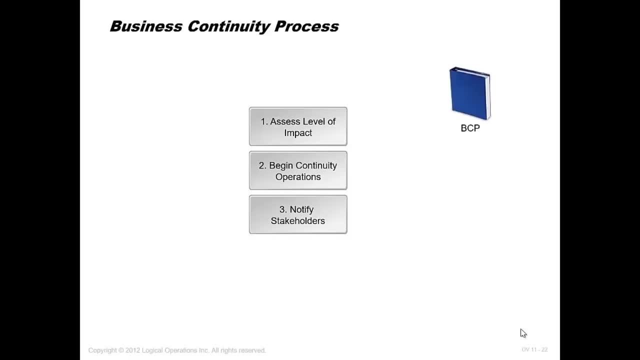 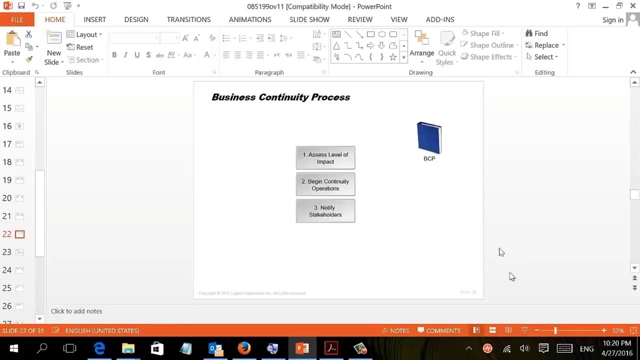 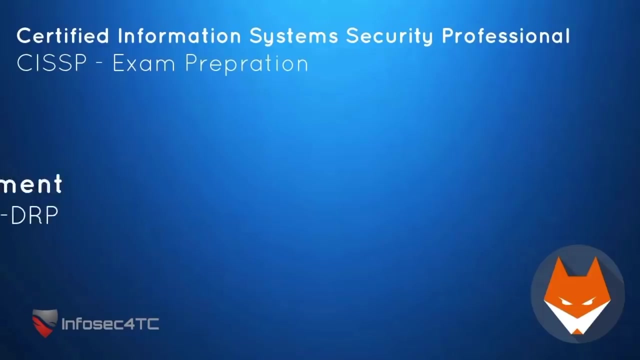 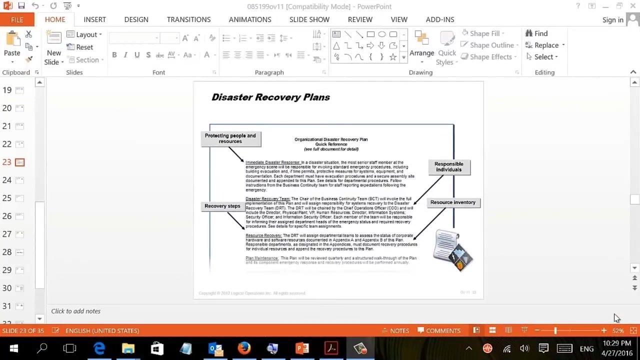 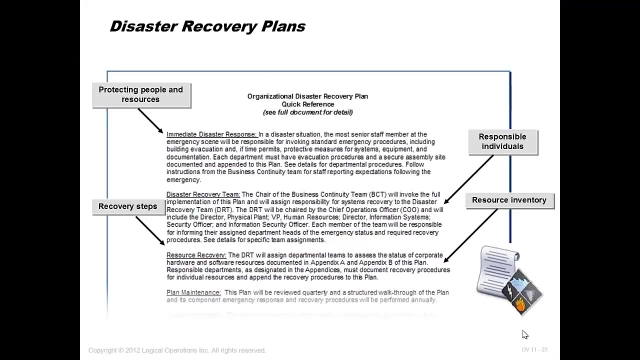 to plan in any domain. the objective is square is that you should have plan for everything and everything should be going according to plan. second part will be the disaster recovery planning, or drp, and i think the drp it's the sub plan for the bcp, because the business continuity is a generic plan while the drp it's a. 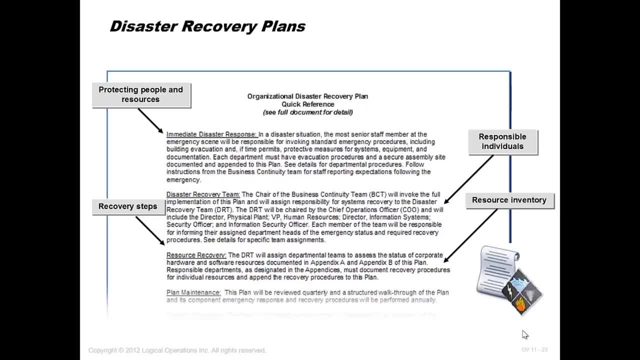 technical plan for recovering the system. but not all business are only depending on the technical part. some business have some operations, some sales, some training. so the drp it's only focused on the technical part and on this lecture we're going to see the same terminologies that we went. 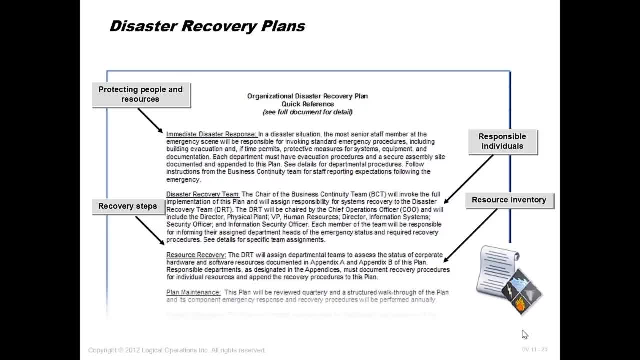 through the last time on on lecture and on the network domain where they will be repeating the type of backup, type of rate, redundancy and so on. so the disaster recovery plan, it's about how to recover the technical document, a technical part of the business, and i'm gonna add some template to be aware or to check how it. 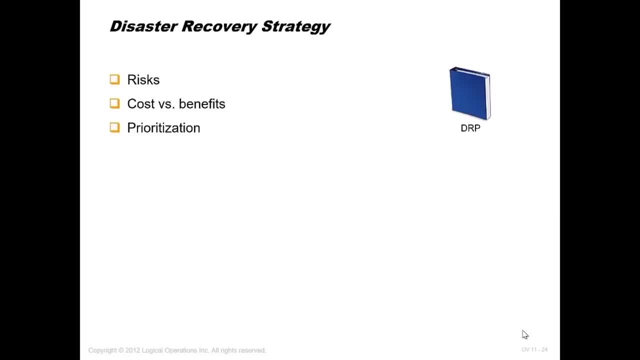 look like now in the disaster recovery plan you're gonna find the risk, what risk may affect the infrastructure, the cost and benefit, and the priority should be cost effective in disaster recovery. you have things that need to be recovered on short term, midterm, long term. by the way, when 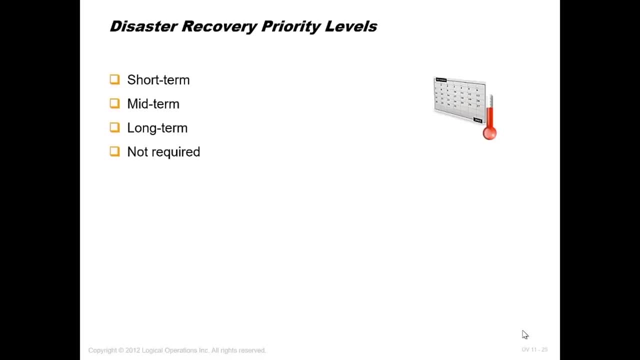 we are talking about long term. usually, especially in planning, it means more than five years, so things should not be recovered all of them at the same time. i mean no, unless your business needs that, but you need to identify what needs to be done- done on short term and what need to be done on midterm and what need to be done on long term. 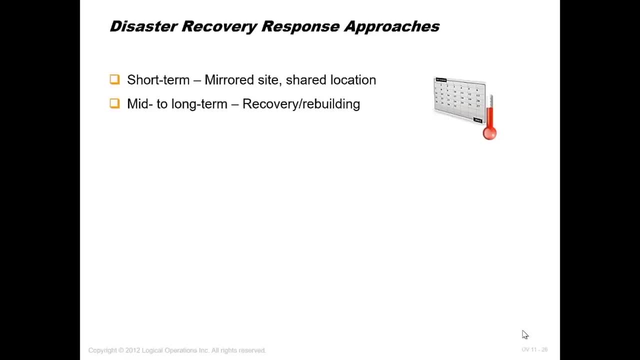 So if you need to recover on short term, you're going to need to do mirroring site. We're going to re-explain that again. on midterm, you need to do a rebuilding. So One of the things that we are going to re-explain one more time. it was explained in. 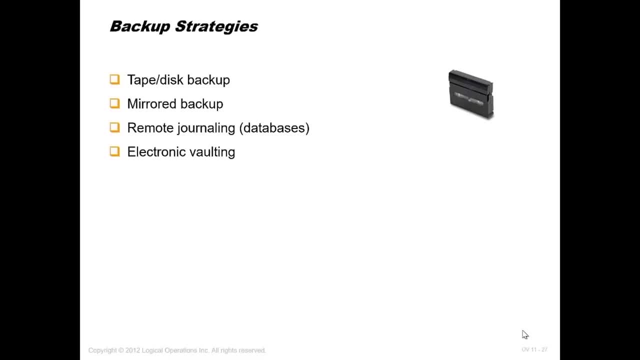 details in the Network and telecommunication is a type of backup. first, before talking about type of backup, how backup will be taking, Are you going to take on tape or disk? Are you going to do a mirroring backup? mirroring mean a alternative backup. 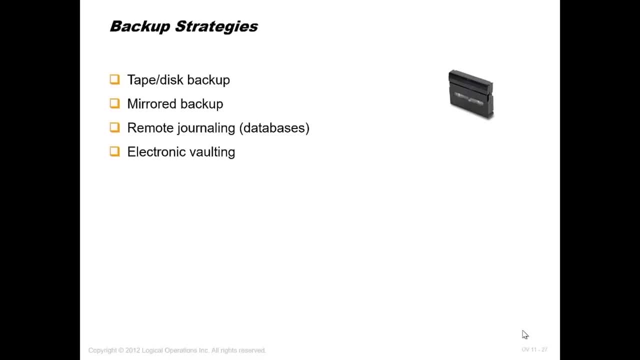 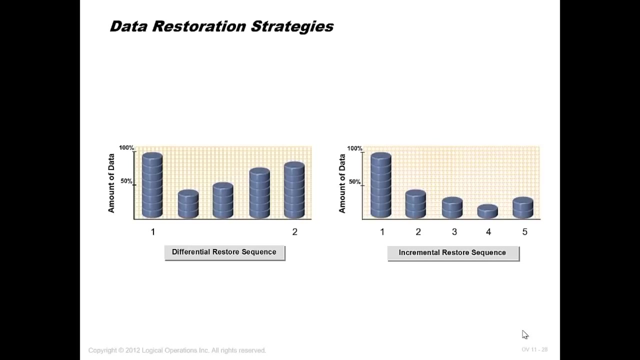 Are you going to do a remote journaling, electronic voting? Do you remember what is remote journaling and electronic voting? backup, which is a site? remote sites that take transaction by transaction, like banks, or remote sites that take bulk backup. So just to memorize what is a full backup and differential backup and incremental backup, full backup are taking a. 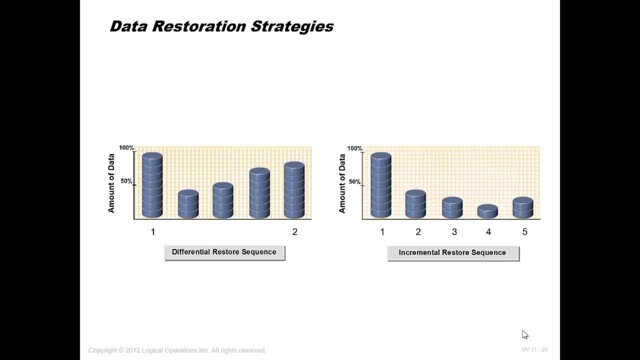 full backup increment and are taking the last change as a change from the last taking backup, and differential are taking the change from the last full backup. If you don't memorize that, please refer to the backup lecture Inside the network. Well, this part has been explained. the difference between differential and incremental and mainly the difference will be while. 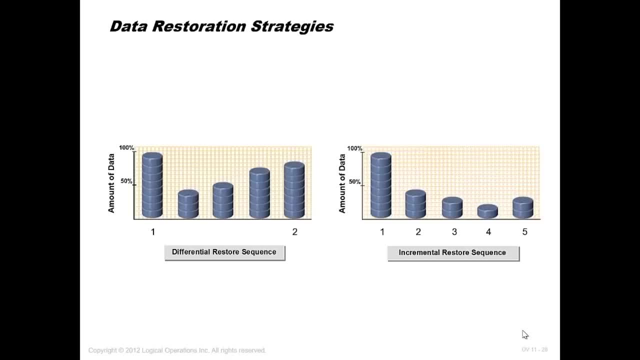 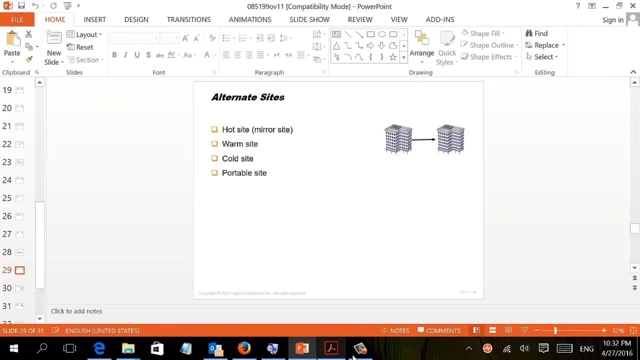 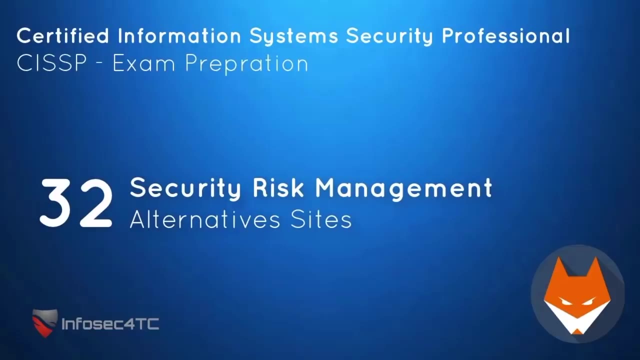 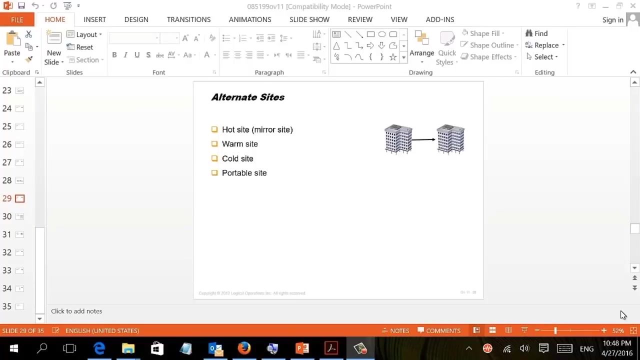 you are restoring, You need less amount of tape if you're going to do a differential backup. Is this lecture We will be talking? Talking about alternative sites. sometimes in your plan for major disaster and for critical business, you may need to have an alternative site. 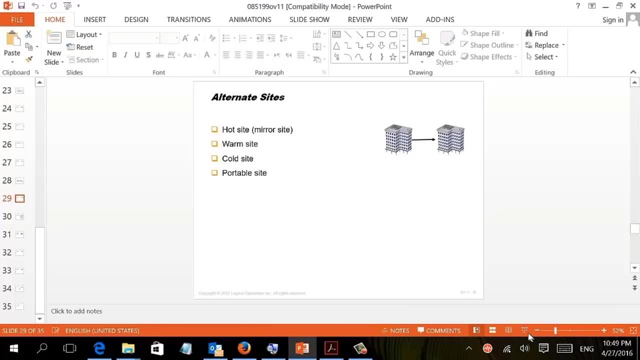 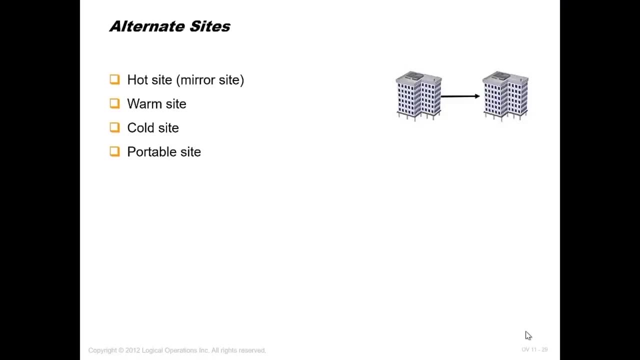 So if a disaster happened and you are not able to run your business from your present sites, you may need to another site, you may need to move to another site. So in alternative sites we have let's see five, not just for first site. 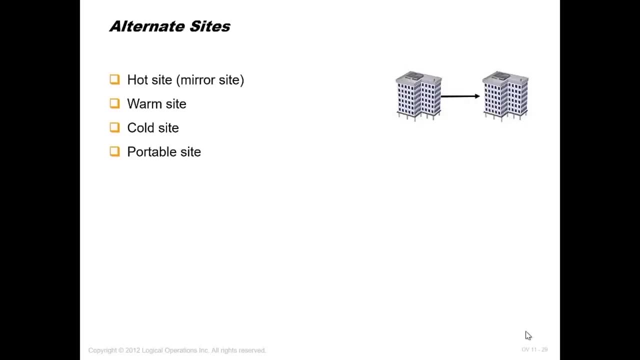 It's called the Hot Site and another name for it is Mirroring site, And this will be a site that is fully equipped with furniture and machines and even data, and the information are synchronizing from your primary site to the mirroring site, So if a problem happened or a disaster occur, you just need to move your people from your current site to the mirroring site and they will be able to be up and 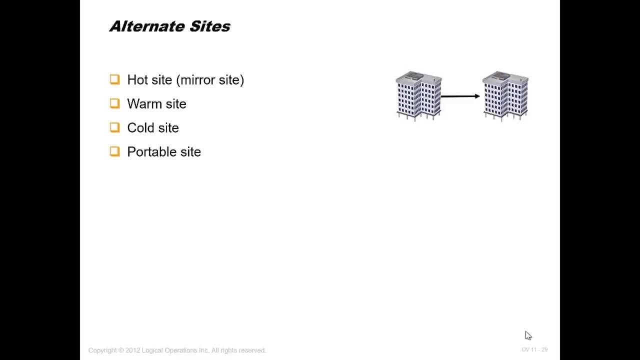 running within hours. so the definition of hot site or measuring site is the site that can be up and running within hour. you'll be having your business up and running. then we have the warm side, and warm side it's a site that has equipment and has computers and has communication, except it doesn't have 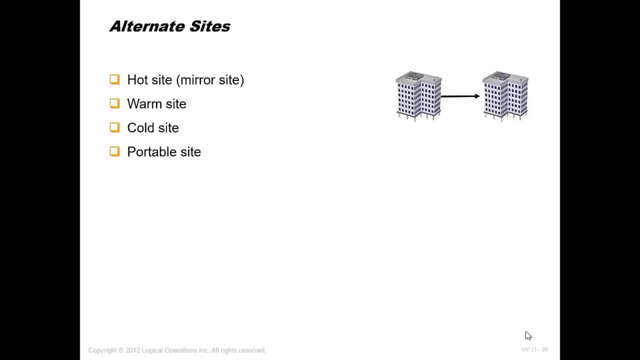 data. so if a disaster happen, you gonna need to move your people and you're gonna need to get the information tapes and recover or restore them so it will be up and running within days. so, as a definition, a warm site is the site that can be up and running within days. then we have the cold side, just a place with 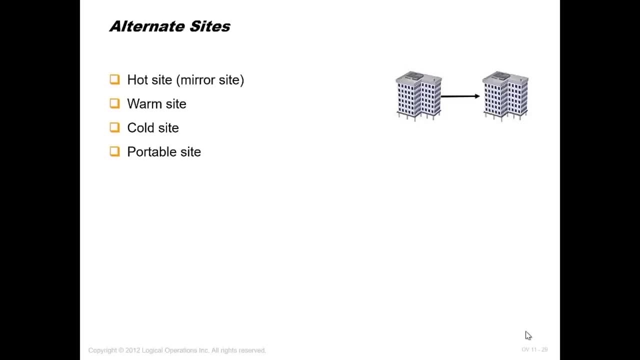 light and communication, you need to have furniture, you need to have machines, you need to have data, and this is can be or can recover the business or can be up and running within weeks. we also have a site called portable site, or sometimes it's called site on wheel. it's like a van where it's, like you know, has some main. 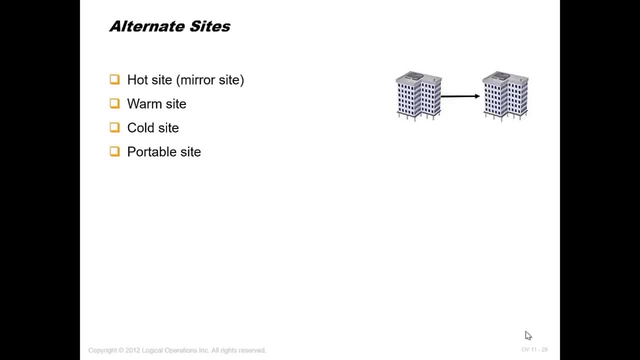 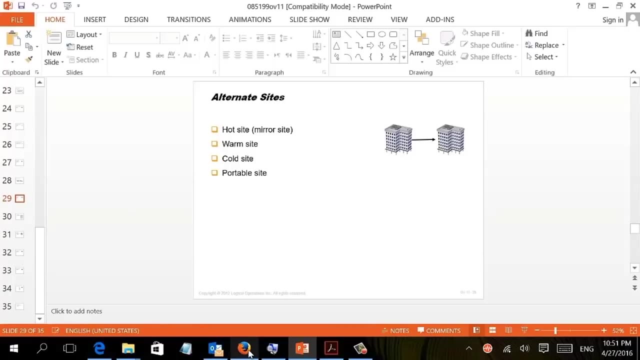 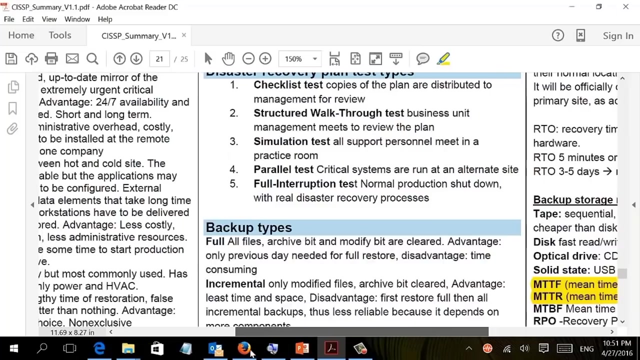 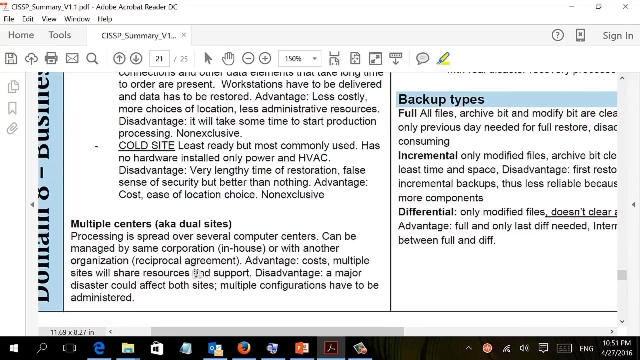 devices that allow you to run the business from the van. now, besides those alternative sites, there is a very important site and quite interesting also. it's called the mutual site. so this site also you need to be aware of. so let's see the. so we have the hot side, the warm side, the cold side. 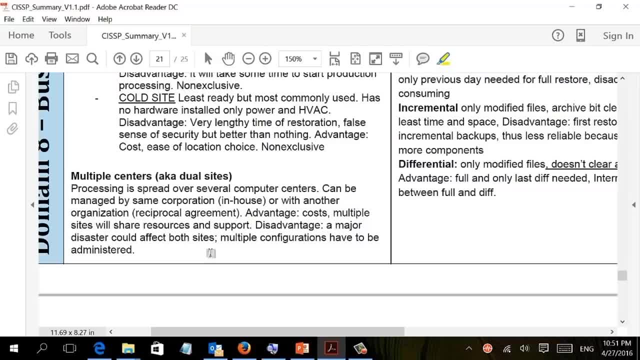 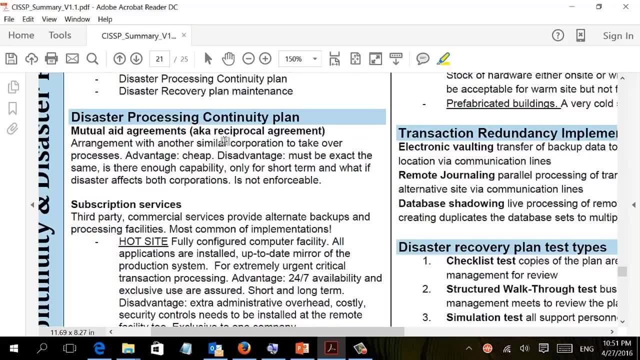 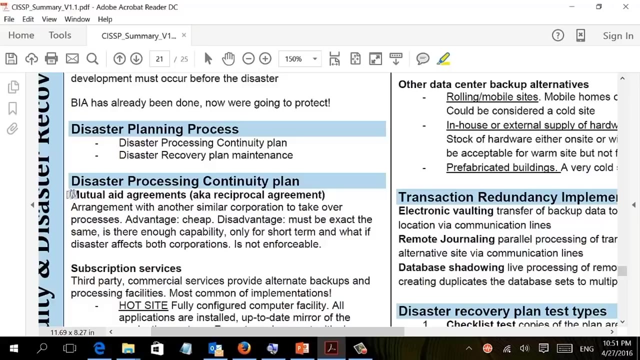 the mutual, or multiple- uh, this is the one- or, yeah, mutual aid agreement side, or a reception agreement. what is that exactly? now, some business cannot afford to have two different sites with equipped with all equipment and, after all, it's a site that you may never use. i mean, maybe the 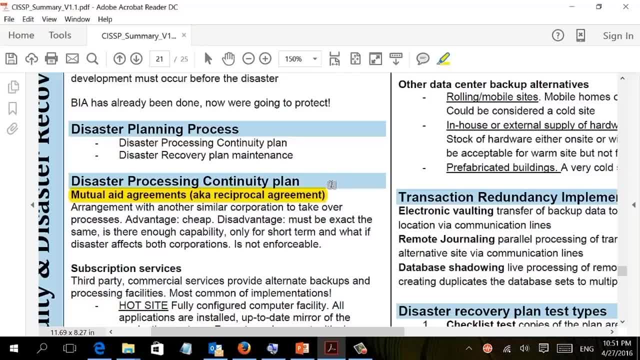 disaster will never, would never occur, and you may have never to move to the alternative side. so, uh, you are paying rent and you are getting furniture and you are testing people, but you may have not to able to use it and besides, as i told you, some business. uh, it's very hard to have replicate site, for instance newspaper. 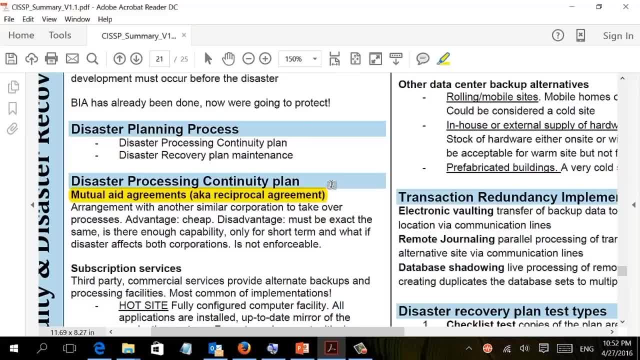 companies that publish news. you know those equipments that they they have are very, very expensive and they cannot have an application of that. so another way for for alternative site is that assumes that i have a newspaper, i can check for someone that has the same business but are located on different. 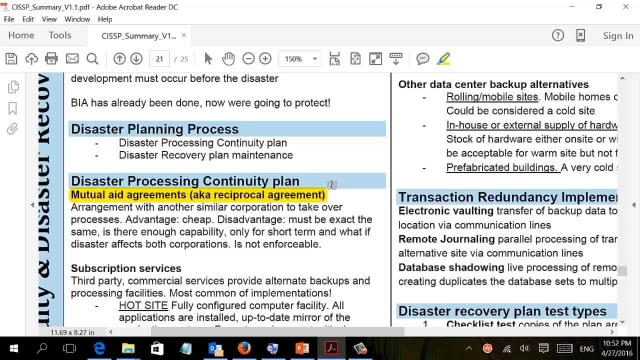 city or on different places, and we can have an agreement together- it's called the mutual mutual aid agreement- saying okay, if a disaster happen on my site, since you already have the same equipment because we are on the same business- i'm gonna go move my people from my site to your site and they will be working on your site and if a disaster happen to, you can. 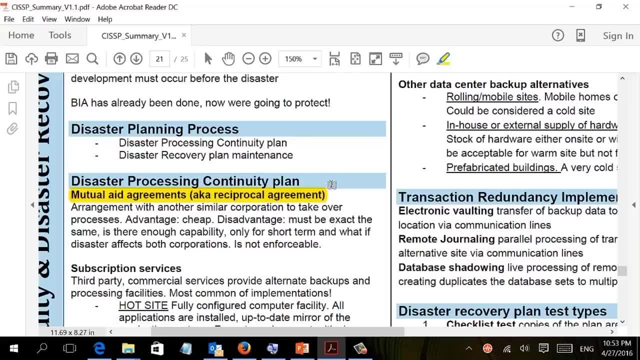 move your people from your side to my side and they will be able to resume working using my same, the same equipment I have. so this is, theoretically, it's actually very effective, except practically it's very hard to enforce. so disaster, for instance, happen, you take your people there, they are quite busy. 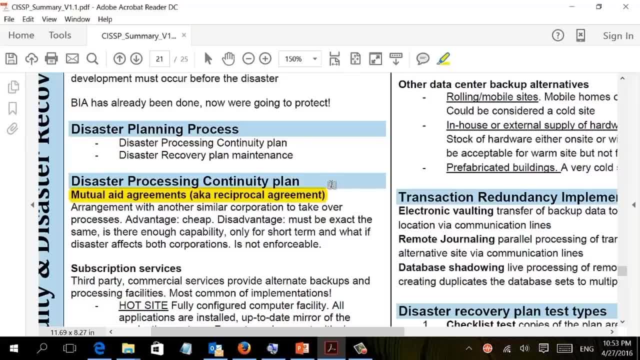 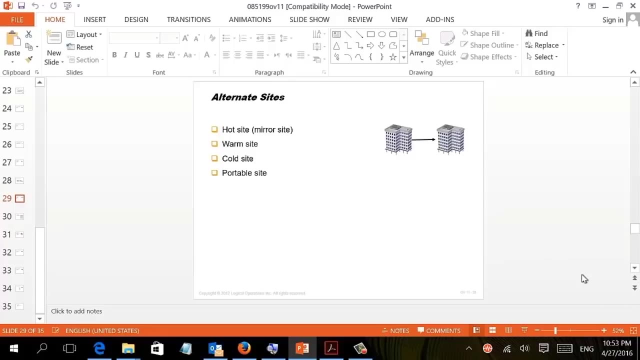 they don't have. so you cannot enforce that, but theoretically it seemed very realistic idea. so those are the different kind of site and you should know the definition: what should be up and running within hours or days or weeks and so on. so getting back to our presentation, so type of site is also. 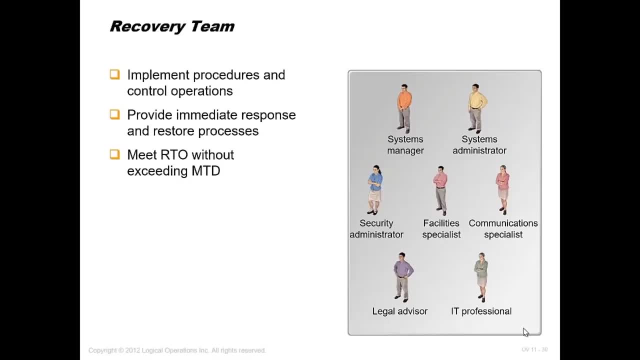 important now. recovery team should be: man is similar to the. the recovery team should be: man is similar to the. the recovery team should be: man is similar to the BCP team has every member of the team and those are the people that, whenever a disaster happens, they know exactly what to do and they know where to start. 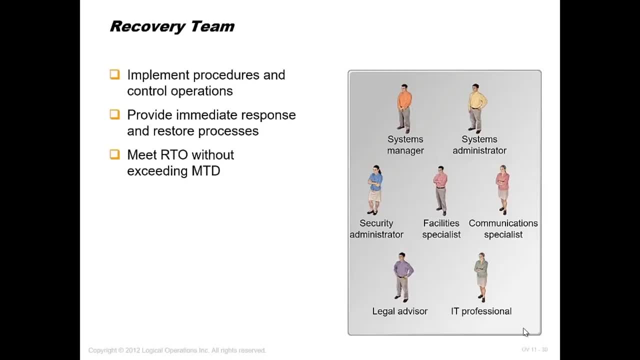 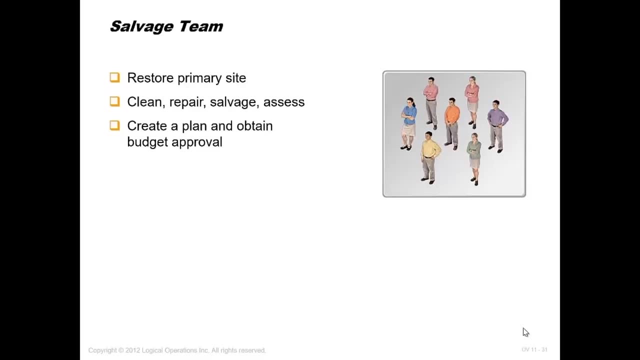 and they have all the process and don't forget those terminology, which is the RTO and MTD and so on, and we have also a team called the salvage team. what is the salvage team? is the team that is responsible that, once the disaster is finished, he need. 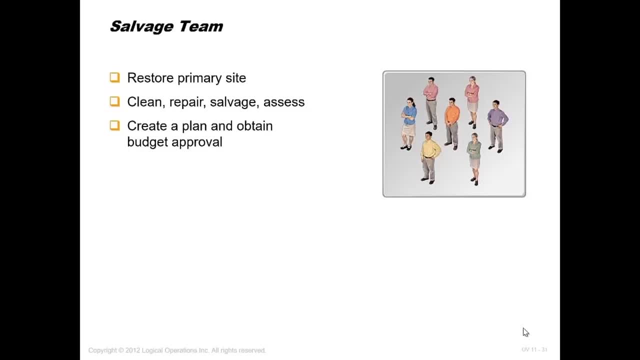 or his responsibility. start- I mean recovery, recovery team- start when the disaster start. they start working, they have the plans, they do everything. now the disaster is finished. people has been moving to the alternative side. now they are working fine and disaster is finished. so I need to get people back to the 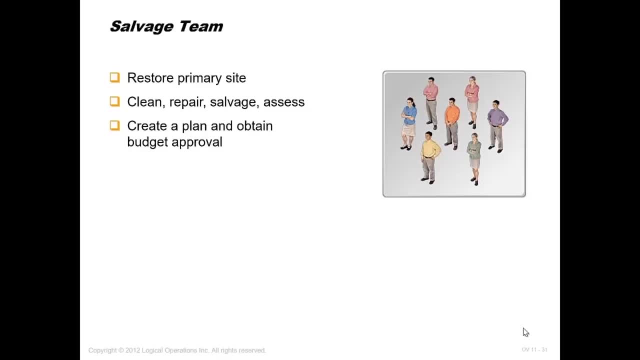 original side. who's doing that? the salvage team. so salvage team start once the disaster finish and their responsibility is to retrieve the people, to get the people back to the original location once it's clear and once the location are ready to be used one more time. so those are two different team when. 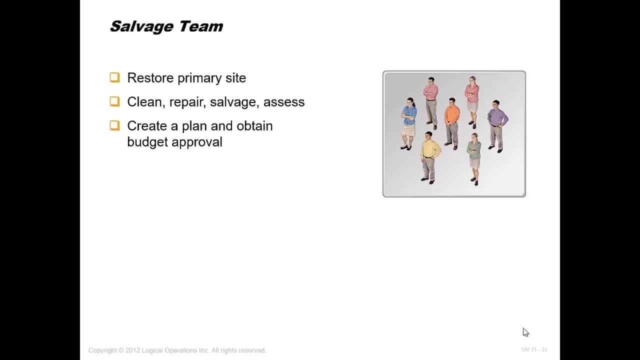 a disaster happens, the recovery team start first. once everything is settled and every people and everyone has been moved to the other side and they are working fine, you need to get them back. who's doing that? the salvage team. the plan also need to be evaluated periodically, one per year, and to make sure that still valid. nothing has been. 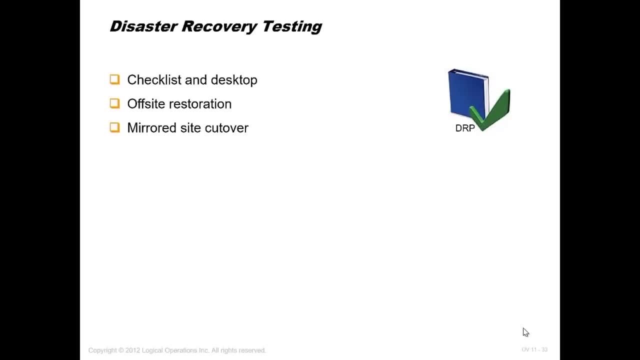 changed and also we have some kind of test- checklist test or also called walking through. we have a mirroring site test, we have a off-site test, so it need to be tested as well. so this was the part or domain related to disaster recovery and business continuity. it's very important and 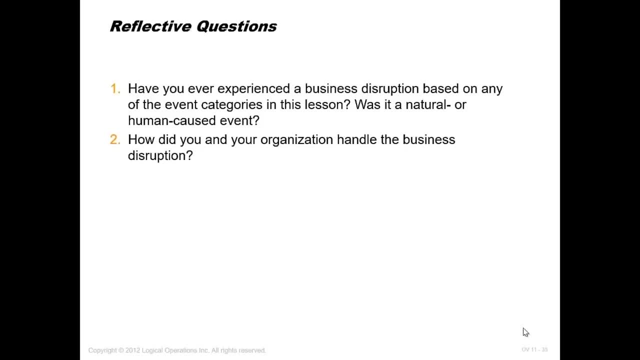 in today market. this is actually extremely important and most of the framework- like if you need to implement ISO 67, if you need to implement ISO 27001 or any type of framework in your organization- you can see that one of their main requirements that your organization should have a business continuity planning and a disaster. 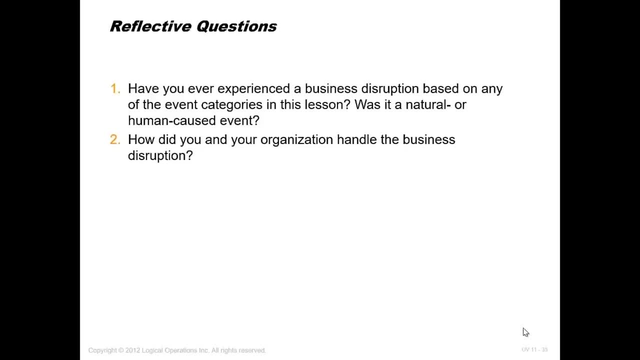 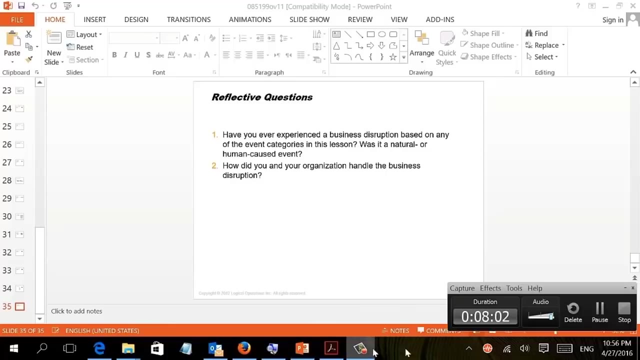 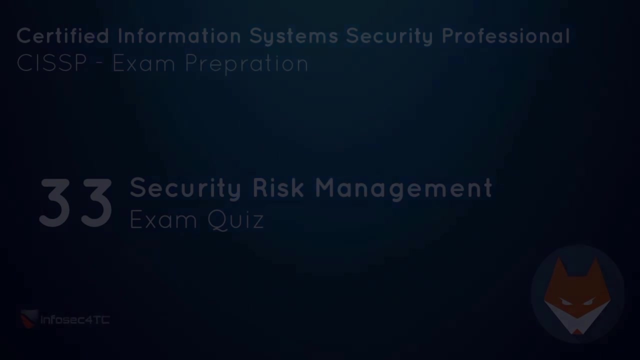 recovery plan so realistic is very, very important. that's why I added a lot of template to this domain. let me know if you have any question, and I hope the domain was clear enough. thank you. we already cover a lot of topic in this domain and we still have like couple of 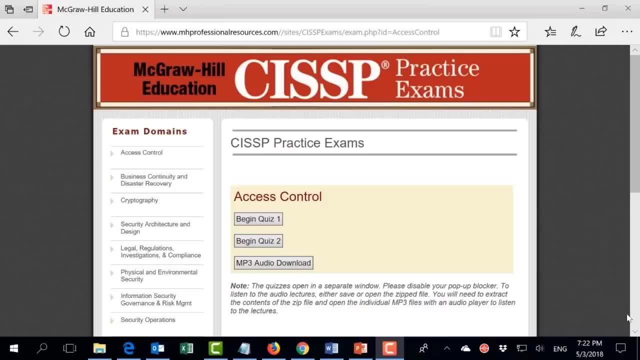 topic remaining. that's why, besides the exam practice questions that I will be sharing with you, I will also would like to refer you to a very good website for questions for taking different quiz related to some of the topics that we covered so far. this website, which is MacroHealth Education. 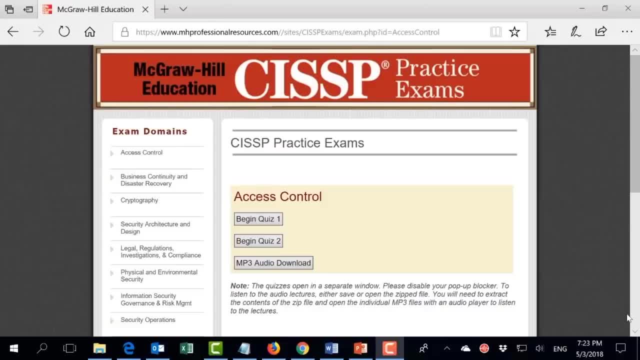 website. it's one of the best website from where you can find a lot of questions that has the same idea or the same kind of tricks that you may find inside the exam. the only problem with this website is that it's categorized based on the old. 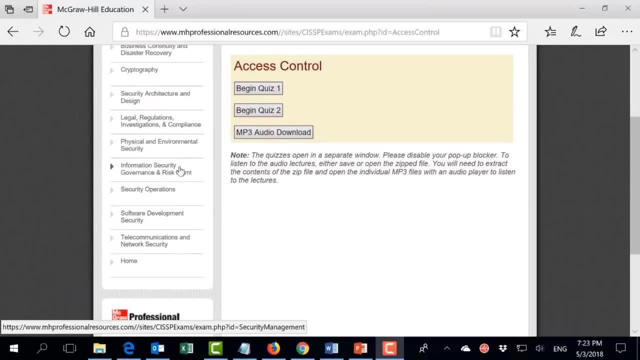 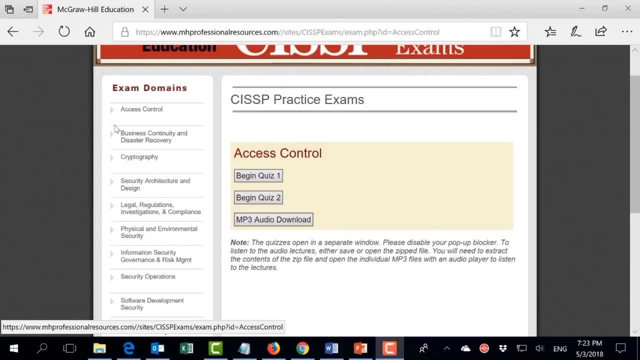 format, so you will find them as 10 domains, like the 3rd edition, not as 4 domains. I'm sorry, 8 domains. so according to that, you can work on this website, practice those topics, but based on subject, not. 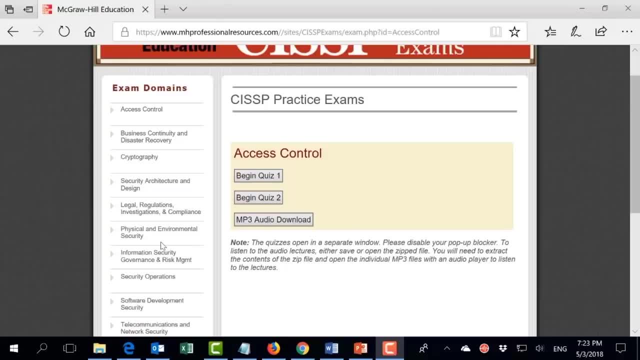 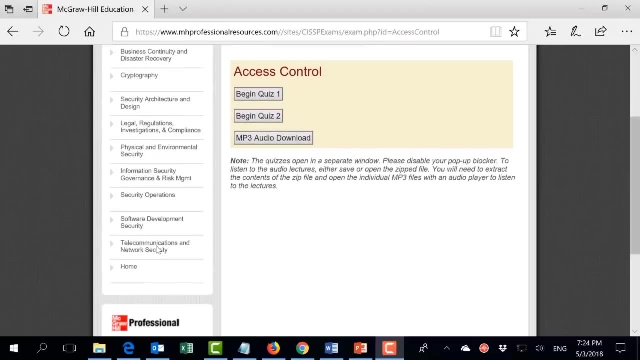 on the domain. you will not be able to map them as domain names with the new curriculum. so, for instance, business continuity and disaster recovery, you will find it here, while risk, you will find it here, and both of them are in the same domain, and so on and so forth. 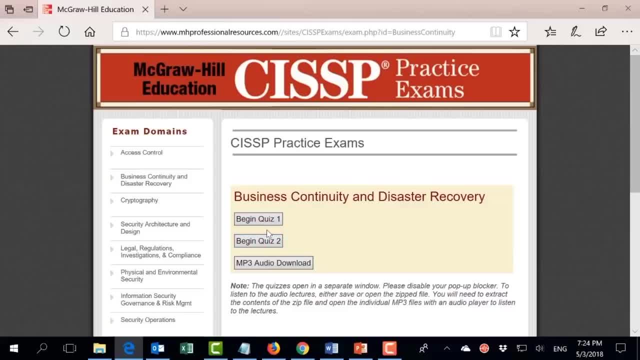 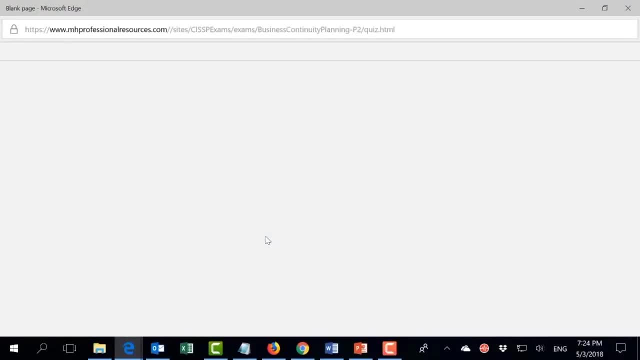 those domains you will find two different quizzes. each one has around 50 or like 52 questions, but they are quite good and very similar to the real exam practice. I want to tell you two points. first, you will not be able to run those exam practice questions on your mobile. you have to run the exam practice. 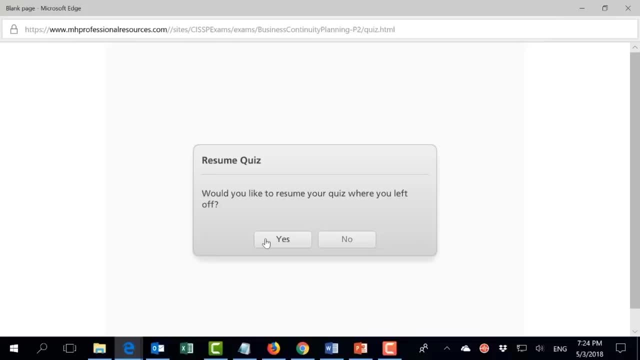 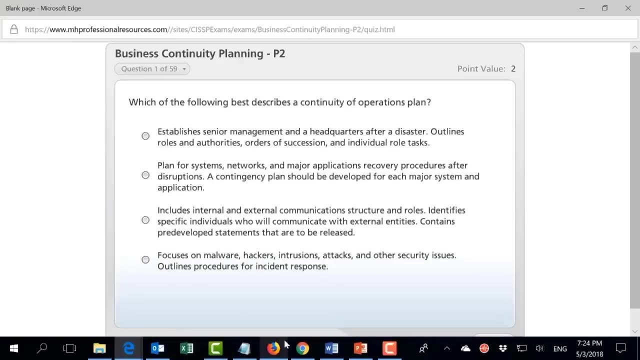 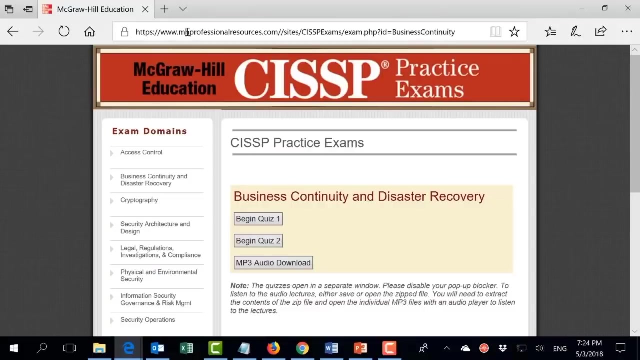 question on your computer because they request flyers. So this is one point. the second point, that regarding the URL. let me show it to you. I will add this URL inside as an additional resources in this lecture, but be aware that it's case sensitive, so it's better to copy and paste it from the notepad. 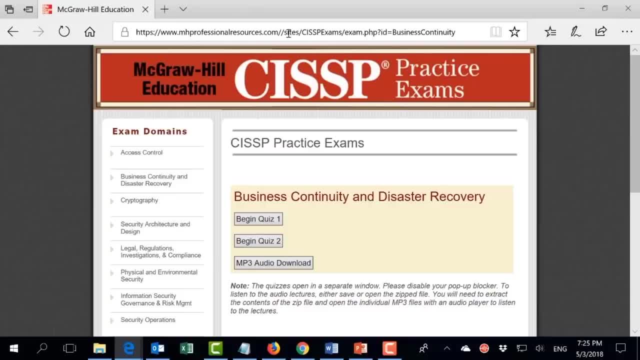 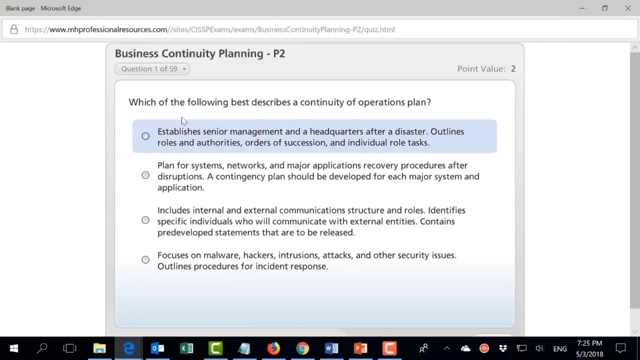 files that I will attach it. so it's URL is a case sensitive URL. so let's see you know how the exam look like and let me tell you a very important point. so this is, for instance, which of the following best describe continuity of? 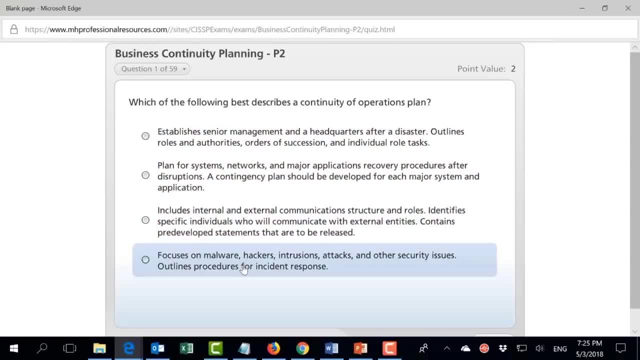 operation plan, and you will find different kind of answer. now, the point here is that when it come to reading the question and answer, the most important part is reading the explanation, even if you select the right answer. so let's read the questions and let's 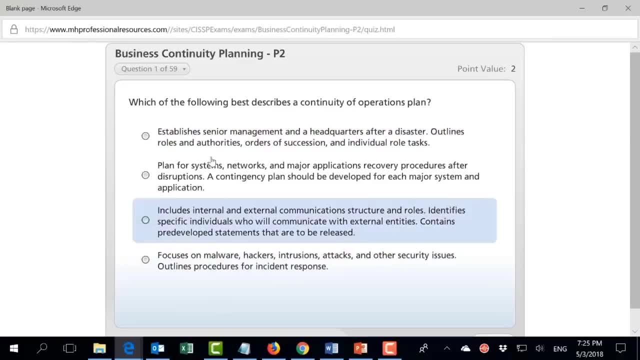 discuss. you know how you should analyze the question. so what is the following? what of the following best describe the continuity of operation? plan: it establish senior management and headquarter after a disaster. outline rules and authority. order of succession and individual role of task make sense. plan: the system, the network, the measures, the 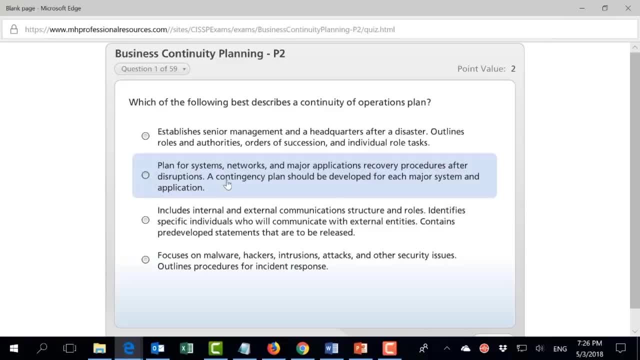 application recovery procedures after disruption. a contingency plan should be developed for each major system and application. I think this more into the disaster recovery area include internal and external communication structure role: identify a specific individual who will be communicating with external entity? yes, of course, inside the continuity planning communication plan should. 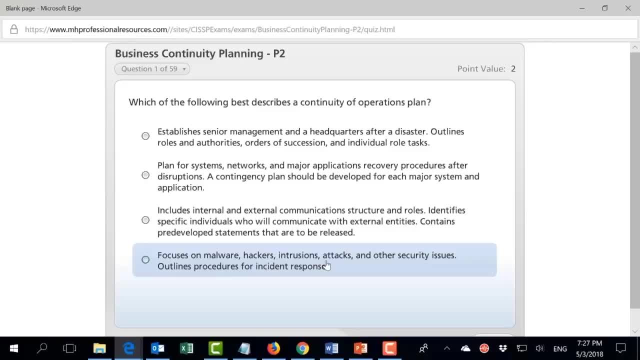 be there, focus on the malware, hackers, intrusion, attack and other security issues. now let's, let's do a specific technique, Let's remove the answers that do not apply at all, which I believe it's two and four, because this one only focus about malware and hackers and, as I told you in the business, continuity. 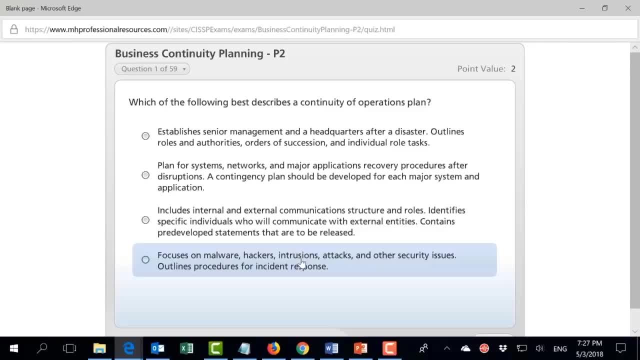 maybe something else happening, maybe like an earthquake or a tornado, or maybe someone left the company and you know, like the know-how of specific technology or something like that. so number four, it's very limited. it's not about, it's only about technical and number. 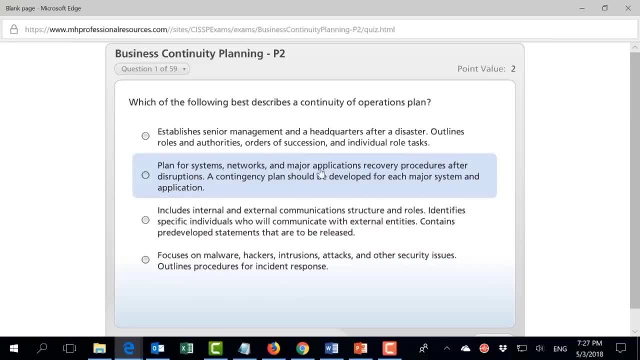 two the same. We are talking about system and network and application. but as we saw in the business continuity it's not just about the business. maybe it need technology and it need equipment and application to be running, but also it need people and process and so on. 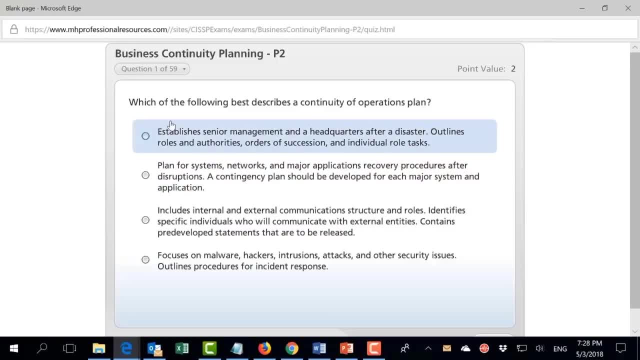 So we are between one and two. establish a senior management and headquarter after disaster outlines role and security. This is the order of success and individual role task. This could make sense by eliminating two answer. you're going to have a 50-50 chance to answer. 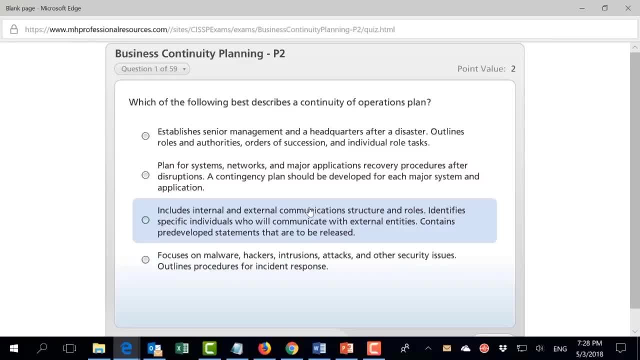 the right one. Number four: number four include internal and external communication. structure and role. identify specific individual who will be communicating with external entity. So if you see the right answer, you can do it, You can do it, You can do it. 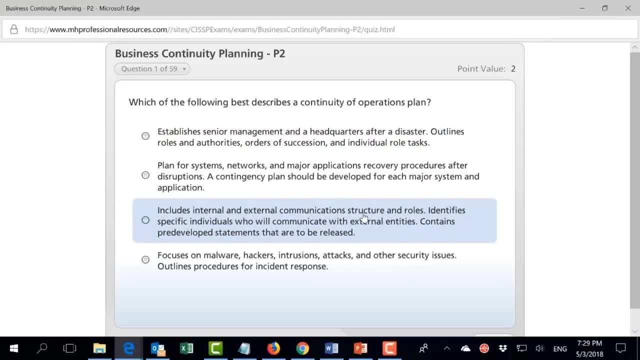 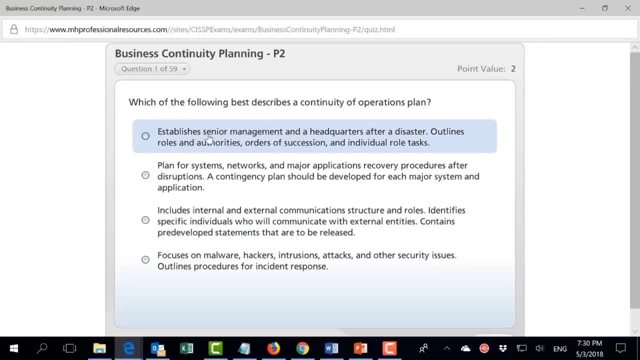 not the full operational plan, But number two, which is having a senior management headquarter. people will be knowing the role and responsibility. I think this more into the right answer. So sometimes you cannot find the full, convincing answer, but you need to select, you know. 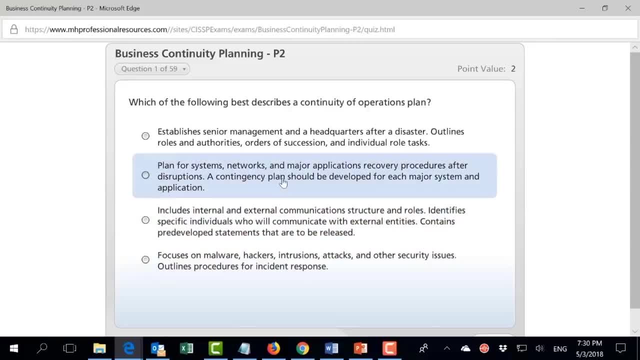 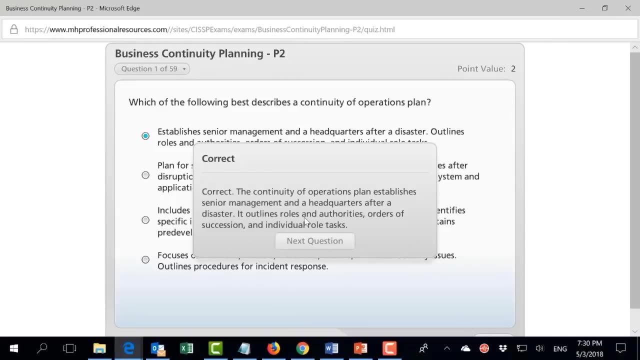 what could be the best one. so, according to that, I eliminate two of them. this doesn't make any sense, so I have a 50- 50 percent to choose the right one. I would go with number one and let's see. and, as you can see, he is giving you the explanation of the answer, is it? 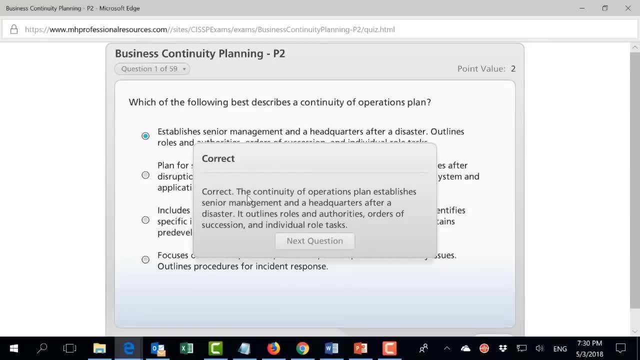 right or wrong and the explanation. it's quite important to read that, even if you did the right answer, because, as I mentioned before, it's quite important to understand how I see square is thinking. this is what we are trying to teach you. it's not about the knowledge because, as you can see, it's not that deep, but it's. 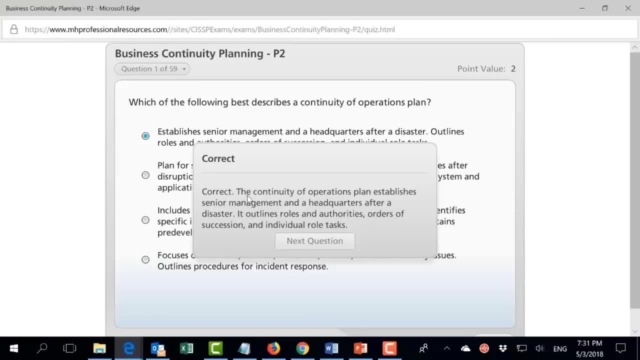 about how I see square is thinking. what is their mentality. this is quite important, so you need to understand if you got this right answer by coincidence or you really thought the same way. I see square is thinking about the operational plan. so this is very, very important and this is one of the very effective website. so 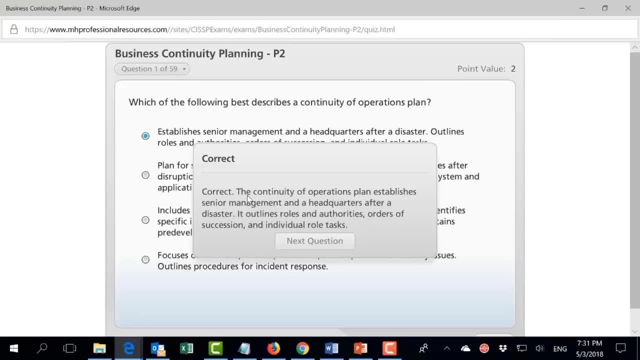 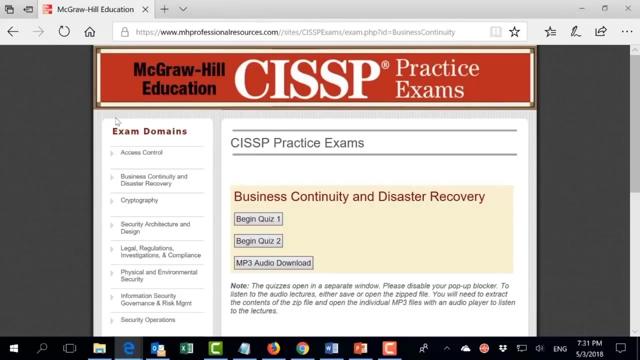 besides exam practice questions, this is also one of the websites that, whenever you finish a topic and you find a quiz about this topic in this website, I strongly recommend that you use it. it will be very, very useful for you. so the website is there. I'm going to attach the text document that includes a URL. it's: 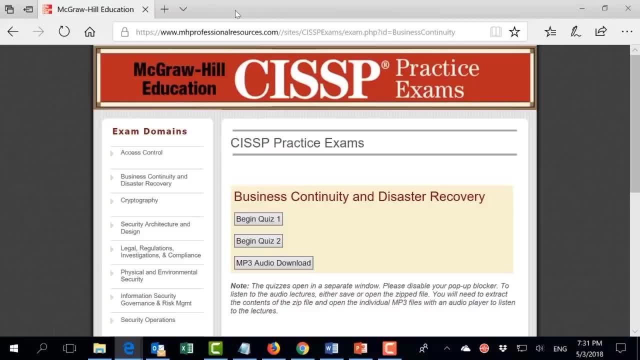 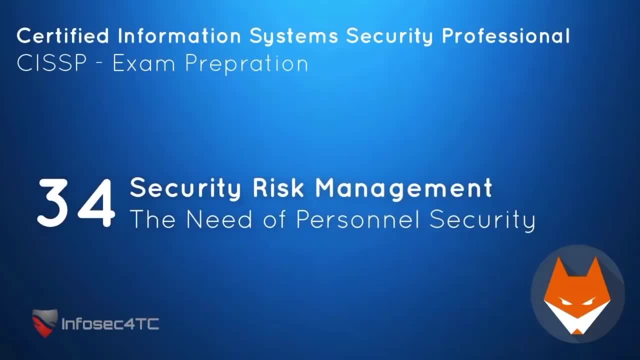 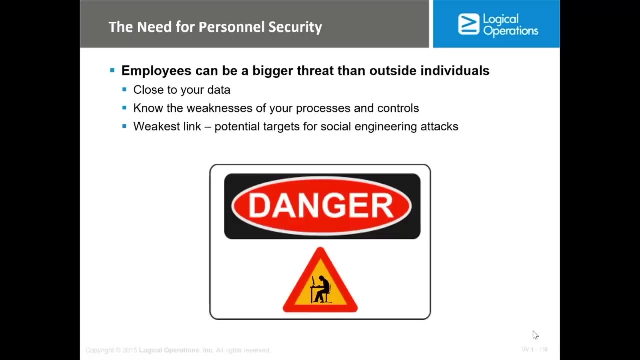 an excellent title website, but it's not a replacement from the exam practice questions that I'm going to send to you now. we're going to talk about a serious threat to any organization which is employee. if you noticed that the last few years- maybe the last 10 years most- 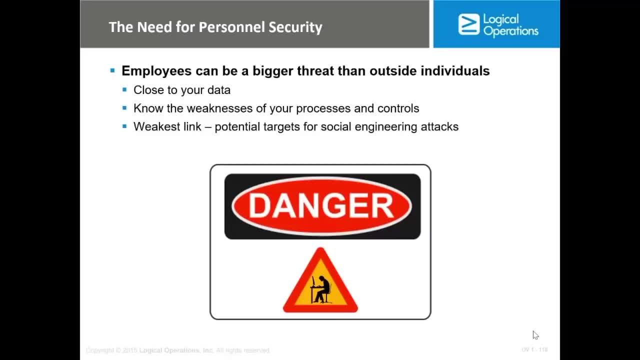 of the major incidents that happen to company or most of the company and organization who get compromised. the main reason for that with the internal employees and actually I believe that more than 70% of the majors attacks that happen because of internal employee. and think about it: employee in any. 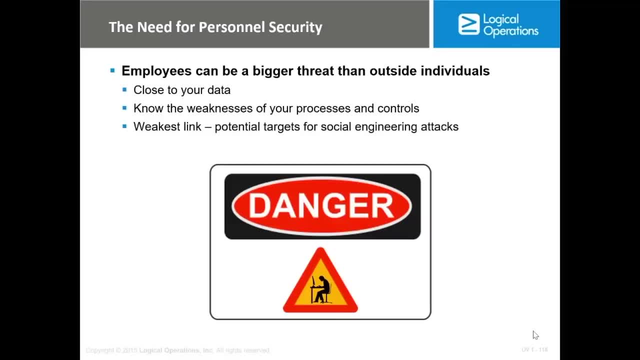 organization have close access to the data. they know the weakness of your system and your process and your control and they are the weakest link. I mean they can do harm to your company, intentionally or unintentionally. sometimes an employee may be, steal information from the company and sell it. 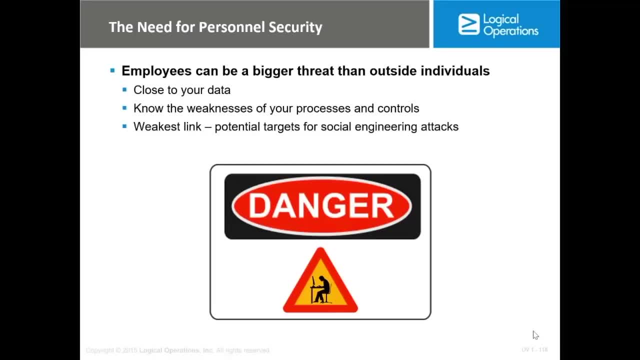 to another company or maybe they get fired. so he need to do damage to the company so he delete some critical data. or maybe unintentionally he, you know, receive an email with a link. he don't care, he don't follow the company policy, he click on the link and that's it. company get compromised. so usually 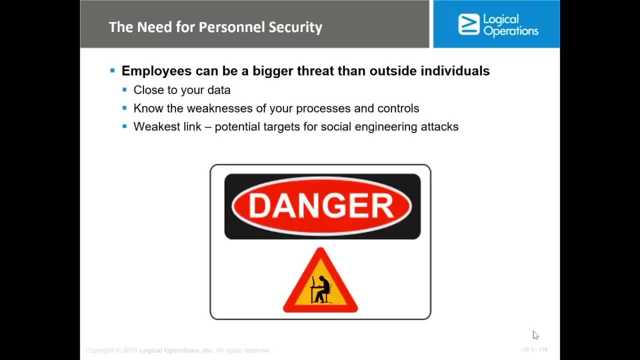 the employee represents the weakest link because they can do like damage intangible, intentionally or unintentionally. that's why, as an information security specialist, or or or information security officer, you should give a lot of attention regarding controls that you need to apply for employees. you need to do some process when you hire people. you need to do some. 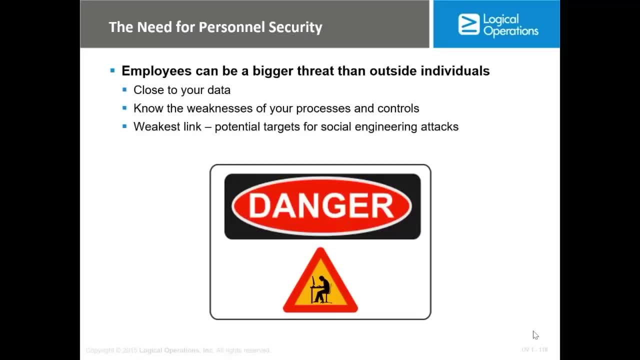 process. when you fire people, you need to do some process. when you hire people, you need to do some process. do some process, like awareness, to people saying that you need to be aware of the policy and if they break the policy, it's not. there is no, not an excuse saying 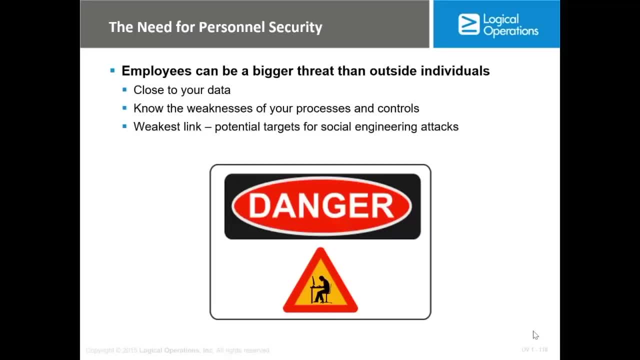 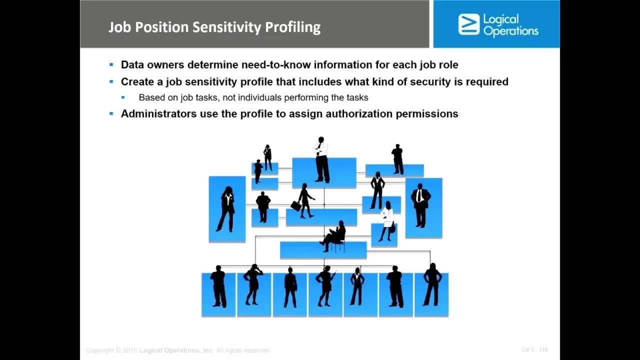 that I don't know. it's not an excuse, so we're gonna talk about that in this and the upcoming lecture. so it's quite important to understand the threads that come from the employee. so how should it start? what control I can implement to secure my data against employee mistakes and, as I mentioned, intentionally or 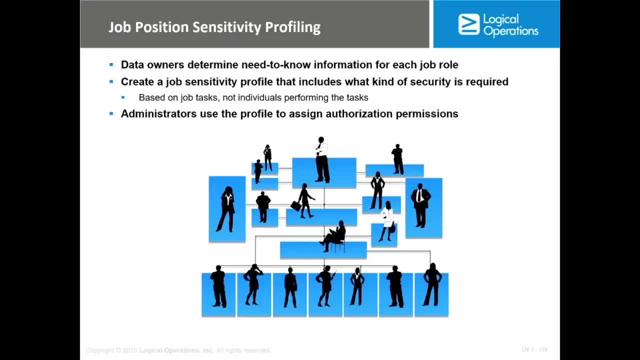 unintentionally. first thing, there is a terminology that you can use in different places, which is called need to know the data owner. he's the ones that need to specify or determine the need to know the information. so, for instance, if you are a functional manager, you are the HR manager or you are the finance manager- right, you are the one. 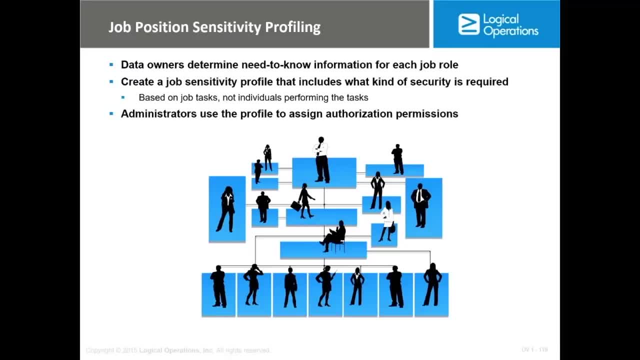 who can say that this guy Jack, for instance, he should have access to those file, while this guy Bob, he should have access to other file according to his functionality, according to his job description. right, it's not right to actually like give all your people all kind of access. this is actually quite risky and this is what may lead. 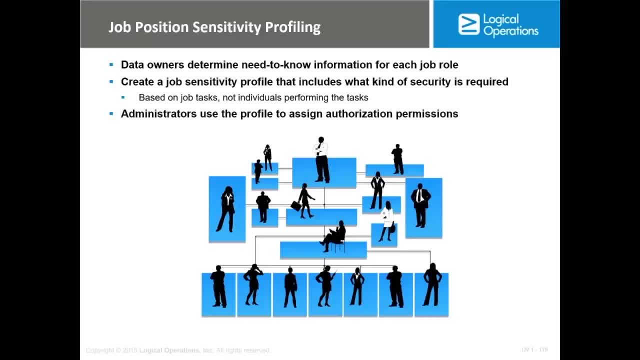 to problems and what may lead to a lot of issues and compromising of system. so you- you are giving- not yourself, but i'm talking about data owner- will determine the need to know information to each job role. this is, as i told you, quite important. so we saw in some organization. 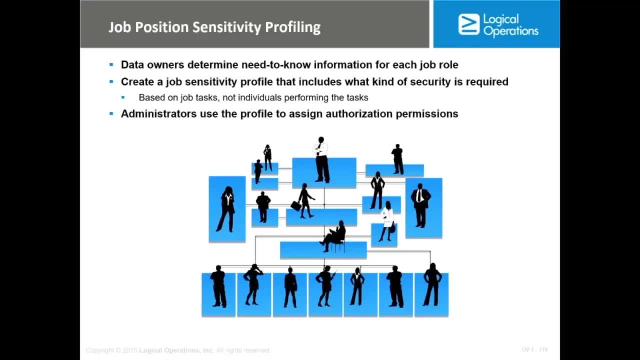 that it's done. it's not done this way. people get hired. so me i will inform the technical team to. if this guy get hired in hr, give him access to the hr folder that include all the file of hr, or give him access to all hr application. it's not done this way. you should have a list. 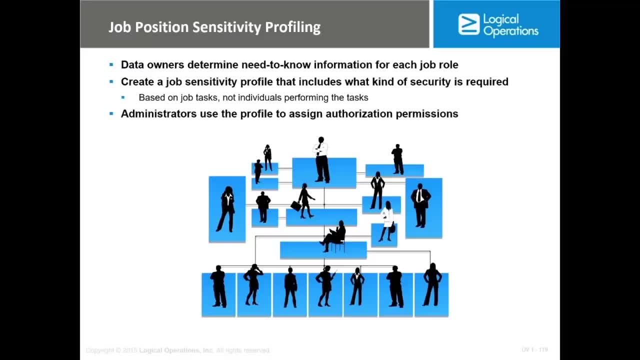 of the people that has access to different system and different files from the data owner and you should follow that. it's maybe like common sense but realistically it's not done this way. i saw some company when people get hired, you know, just to save themselves effort and planning and writing down different. 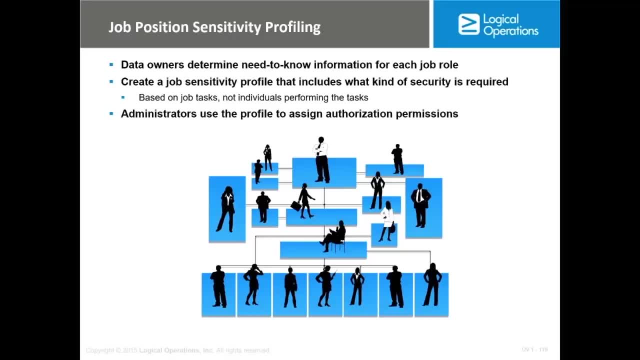 access according to their job description. they will give any new employee access to everything, which is very, very risky. another control that you can implement it's to create a job sensitive profile that include what kind of security is required. so, for each job, and actually also this thing to be done from the functional manager, we need to have a security profile regarding the 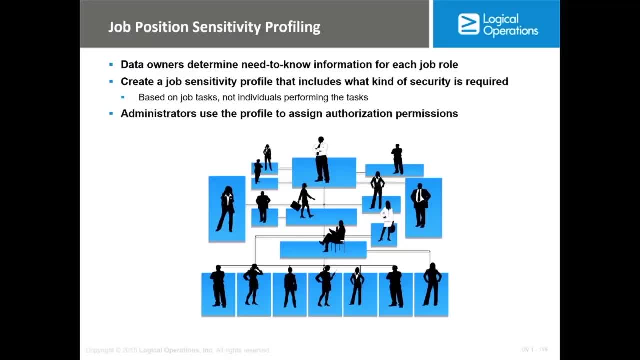 level of security or level of information security he can access and according to that, the administration will use this profile to assign authorization permission. so it need to be designed, it need to be like planned and data owner need to be. by the way, data owner it doesn't mean necessarily the 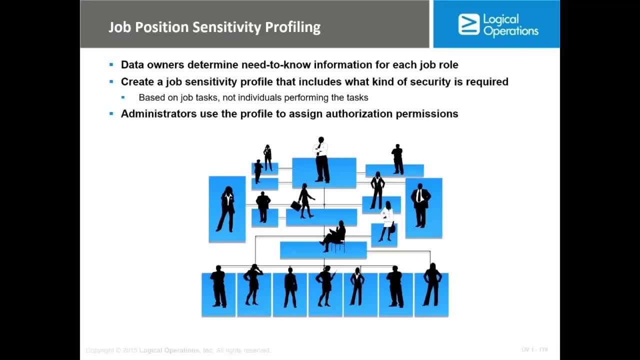 guy who created the file or he created the program. it means the owner, who is responsible of the file, and on the next lecture we're gonna talk about the difference between the data owner and the basic data, and소�jän, which is quite important and you should expect a question about. 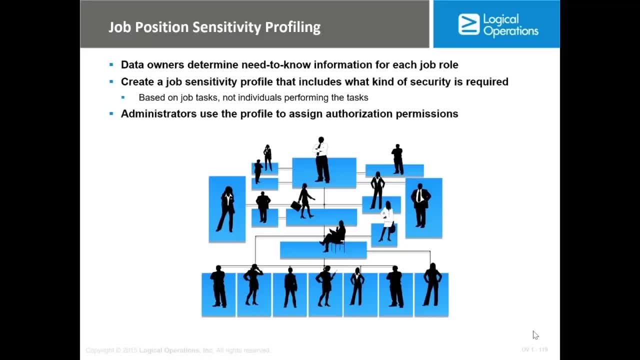 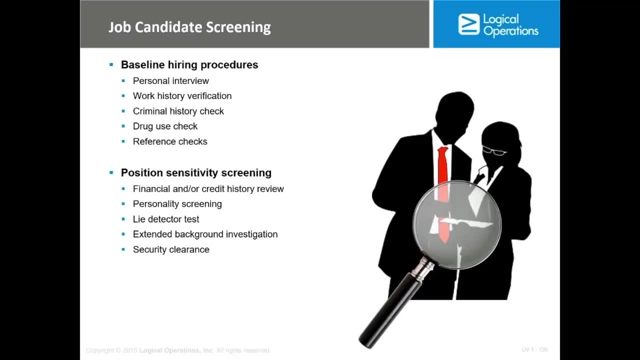 cert inside the exam, but this will be covered in the asset management in the next domain. so some of the controls that you can implement. maybe it's related to HR, but just as an information security officer, you need to be aware of things like background check when you get. 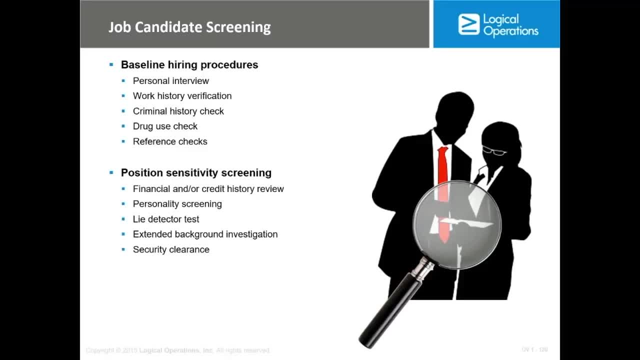 hired. when you hire someone, you have, according to the job, sensitivity, propertyリOur job. but you have to do a personal interview. you have to check the history verification, work history verification. you have to do a criminal background check, drug use check, reference check and it depends about the 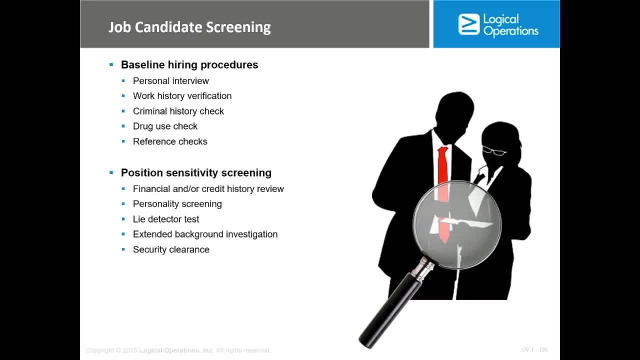 sensitivity of his job. maybe you have to do all of them or some of them. so the verification before hiring it's quite important. Also, things like financial and history review, personal screening, lie detector in some like law enforcement or army, they are doing that- security clearance. so those 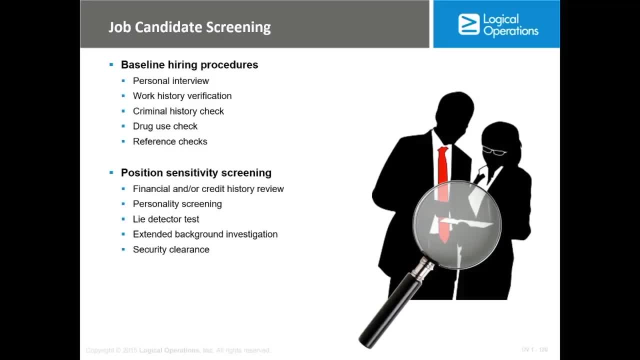 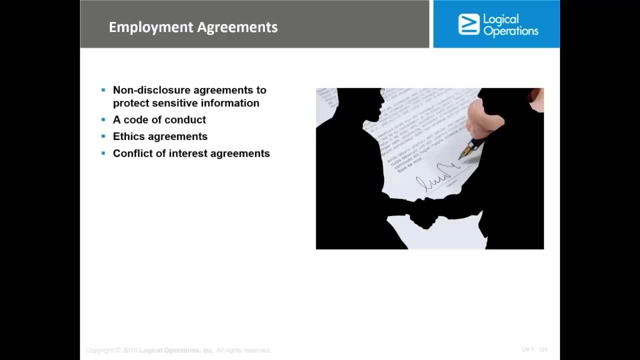 are some of the control that should be in place, especially by HR, but you need to make sure that they are in place. Another important topic that you need to do, or another important control, which is the NDA or the non-disclosure agreement. Each employee need to sign an NDA because he can have. 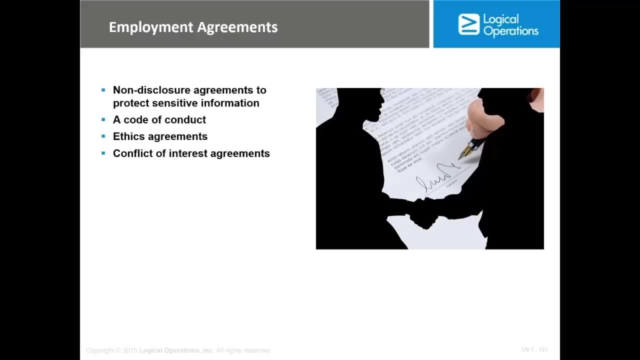 access to the information he can have access to data. so he you need to make sure that he will not leak those data out. so he need to sign this form and I will attach with this lecture couple of like template about NDA. but this is quite 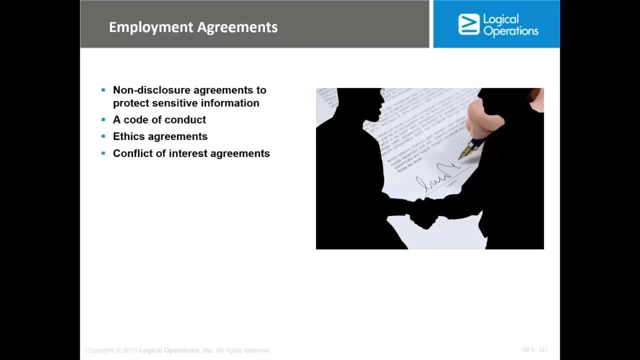 important NDA non-disclosure agreement maybe will not prevent the employee for leaking the data, but if it happened, you have a legal document that you can take action using this document. so, how it look like, I will attach a document, but it's a very, very important document that. 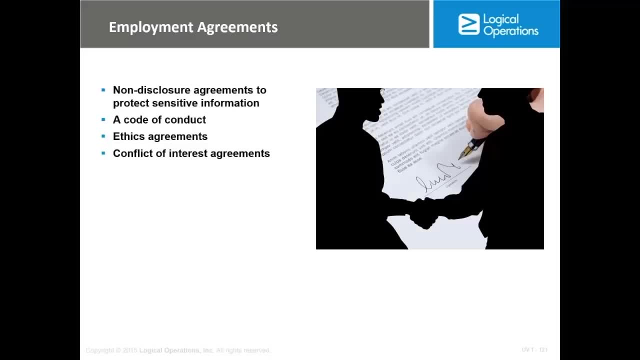 you need to make sure that all employees has signed before they get there, before they get hired. Besides NDA, also depending on the sensitivity of the data that they can have access to or sensitivity of the information, you may change in the content of the NDA. 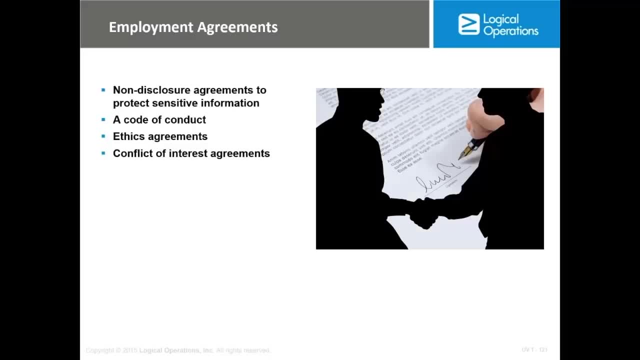 Sometimes you may make this NDA valid till after, even after they leave the work for like five years- People who are working in places like intelligence agency or armies. they are signing a lifetime NDA that whatever they have, they will not have access to disclosure, even after long time. 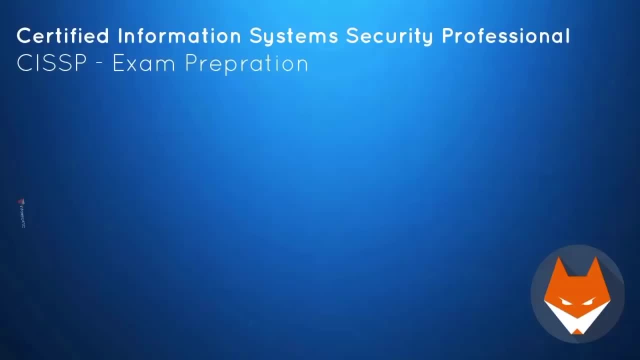 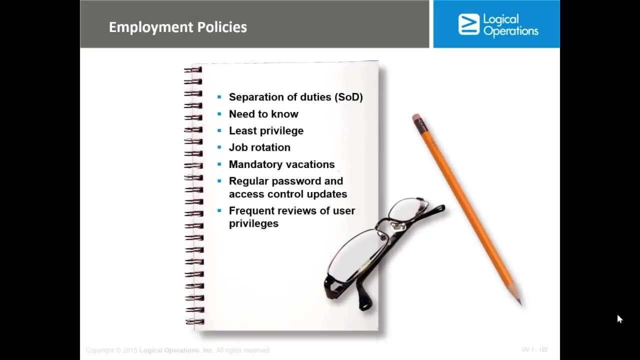 Now we're going to talk about some employment policies that you can implement in your organization to mitigate the risk of employees, the threats that's coming from employees, and to be able to use this employment policy, you need to understand their job responsibility. So to maintain your job responsibility very well- and those are the policy is the most common one, but you'll not be able to implement them unless you know what they are doing. and also, you need to identify the critical business function in any organization. 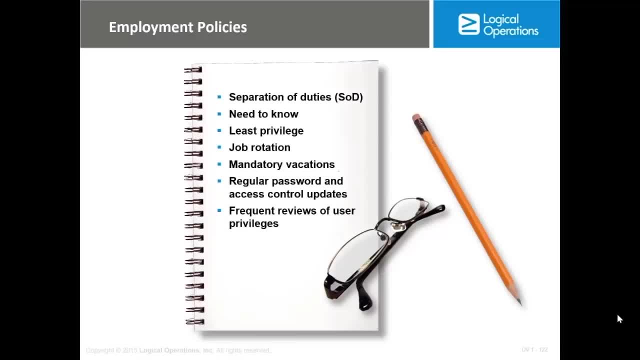 Those policy used to be a part of the operation security. I mean, if you are doing the exam quiz that I show you in before, in one of the lectures you can find question related to those policy in the operational security part. but in the next lecture i'm going to go briefly about. 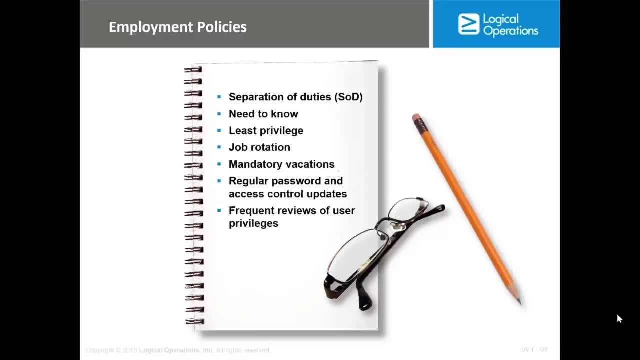 each one of those what exactly they meant. we already spoke about the need to know policy least privilege, which also means that people by default should have least privilege unless they need additional privilege. so someone get hired. i should not give him access to everything and privilege to everything. i'm just going to give him the minimum privilege and then 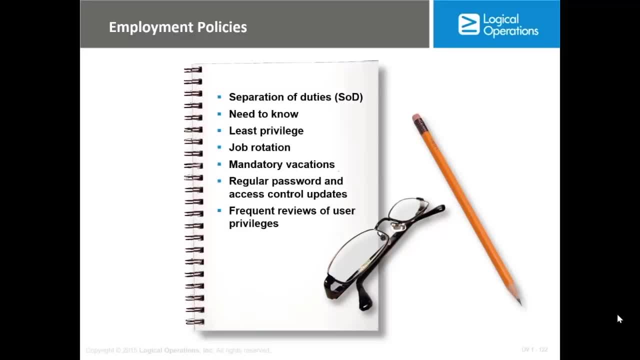 according to their role and responsibility and maybe new assignment or new tasks that get assigned to them. maybe i need to raise their privilege according to that, but by default they should go. they should get the least privilege. so what i'm going to do in the next lecture we're going to 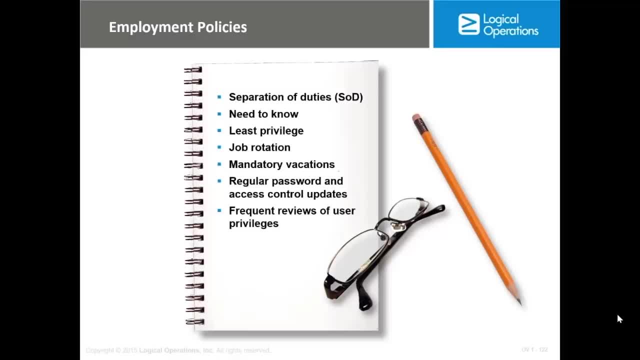 talk about each one of those policy in a very brief way, from sunflower, because actually sunflower covered those very well and i suggest that you do some once you finish this part, that you go to the exam practice questions, or actually the, the quiz website that i showed you, and to solve some question from 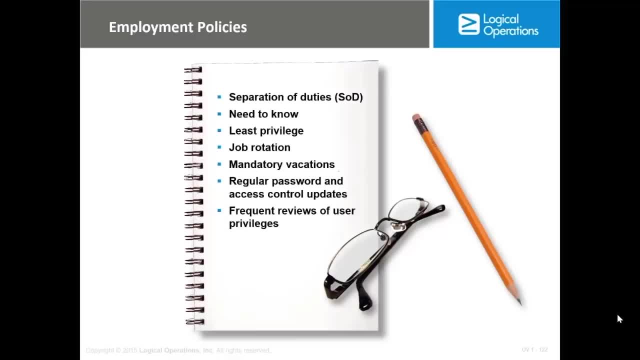 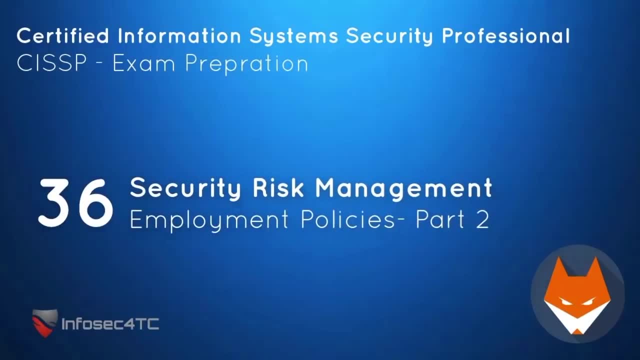 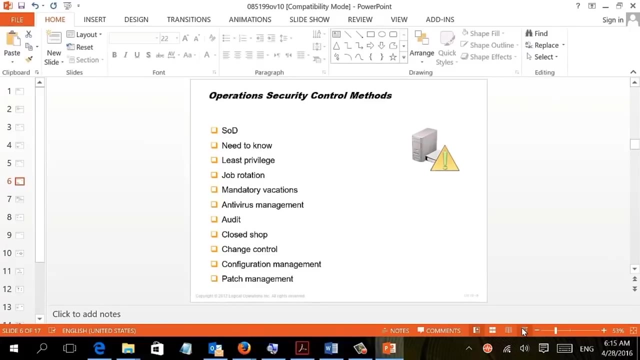 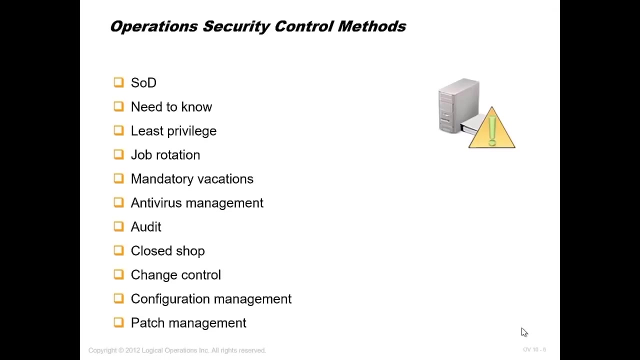 operational security related to the policy. but first let's discuss those policies step by step. so in this lecture we'll be talking about some of the administrative security policies- a major one, and most of them has been covered, as i told you before. so we have the separation of duties that 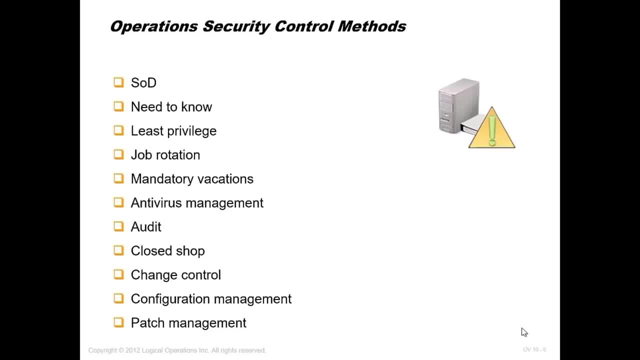 critical tasks need to be uh or the. the role and responsibility need to be separated depending on the criticality of the task. need to know: no one should be able to check or to see the information unless they have a need to know uh permission or have to need to know least privilege. people by default should have least privilege. 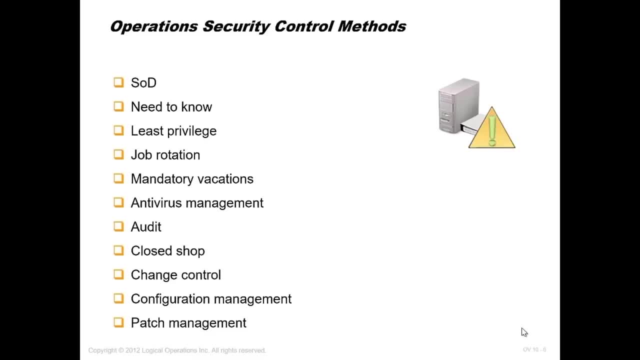 i know it make a lot of sense, but in real life this is not what's happening, because i saw some places where, because people keep asking for more privilege, the administrator will give everyone the full privilege and you know, just to make himself comfortable and no one will call him. so a lot of. 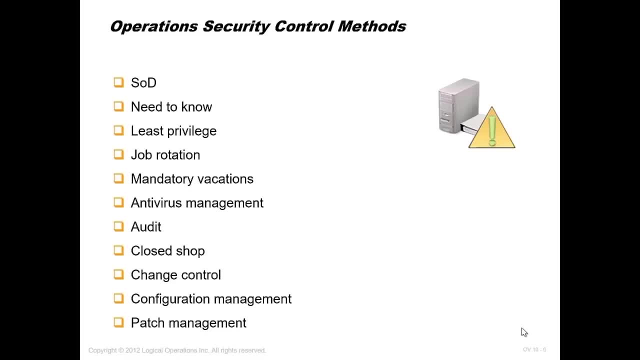 those uh uh policy or a lot of those best practice are not really the best practices for the administrator implemented. they are making a lot of sense but are not implemented. job rotation this is. this is actually mainly into the financials department where you need to move people, so around, so people. 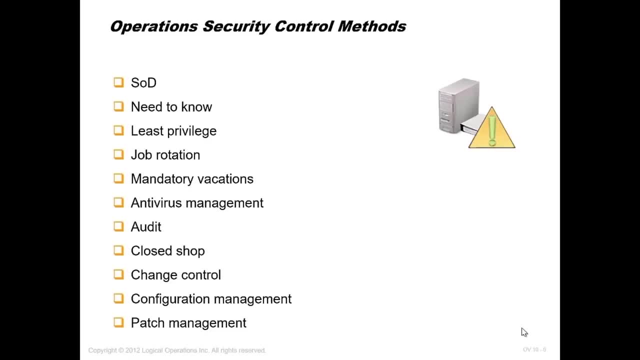 that working on a payroll should be moving to, for instance, uh expenses and people on expenses, because if any fraud is there and you are moving people from their position to other position, fraud will be uh discovered, Mend and Torification. this is also uh in most of the financial department and it's usually targeting 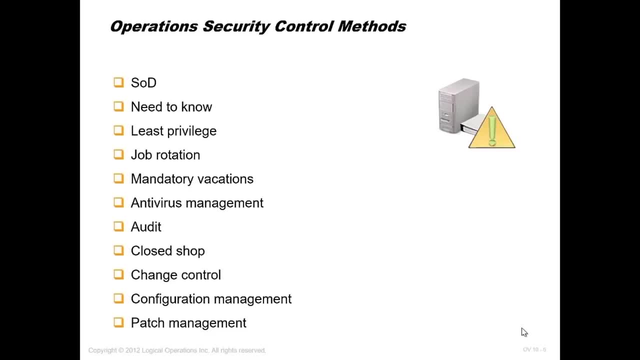 the head of the department. so mandatory vacations that people should take a mandatory vacation. that should not be less than 10 days because they can take couple of days and still no one will be able to figure out any uh fraud or anything like that. but if you leave for 10, 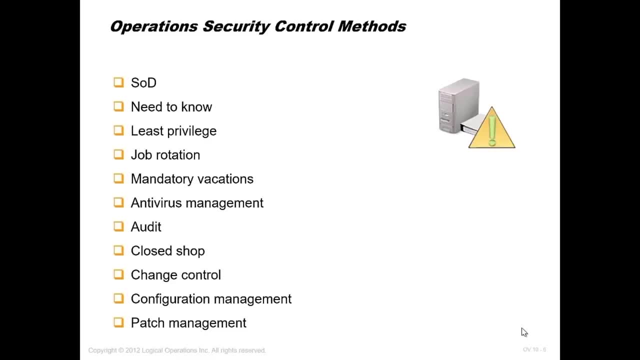 days and someone will be replacing him during the vacation. he will be able to discover any fraud and then he will be able to figure out any potential frauds. so you do have to make sure that you have all the information that you have, and then the next step is to manage antivirus management. so 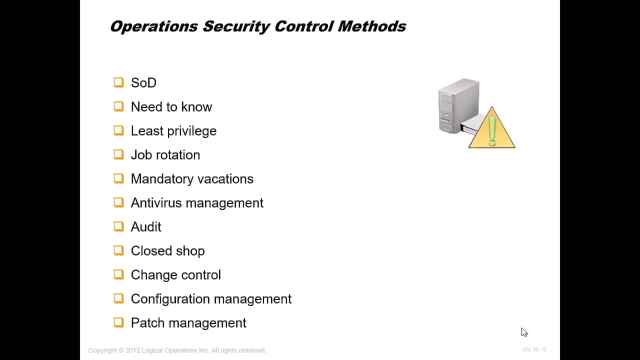 if you have a good antivirus management and you have a good antivirus management, you can go to management and manage antivirus. so I cannot keep people. I cannot let people install whatever antivirus they want and manage in the way they wanted. no, we can do that in a centralized way. 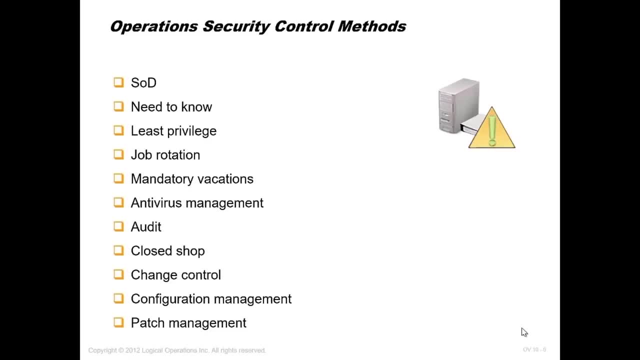 where we can update the antivirus, we can verify the activity, we can check the malicious behavior and so on. other thing should be done frequently: closed shop change control and change control that some change it more. it's more into the application part or software part, but assumes that someone requested a firewall change you have a developer. 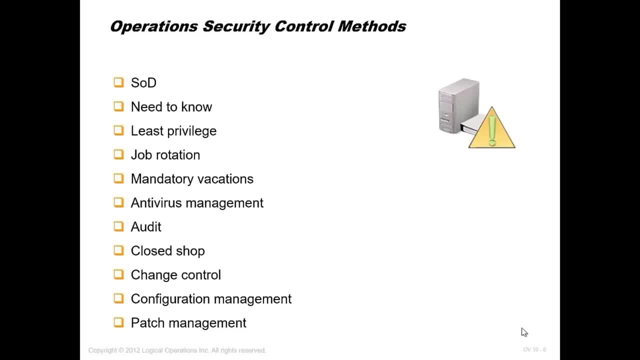 team and they requested to open a port on the firewall. do you have a process for that? or you just let those people call the network administrator and he will open the port for him? it's not like that. it should be written in a form and and it should be assessed. I mean it should be validated by opening this port. 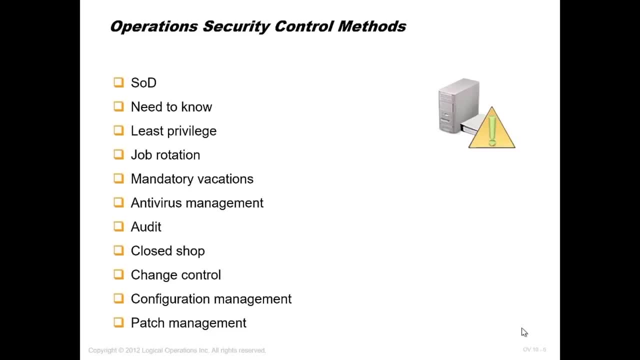 are we going to have any problem. what is the reason for having this port open and then it should be approved? so you should have a process for change, control, configuration management. same issue: if you need to change any configuration, are you doing that through procedures or it just someone? 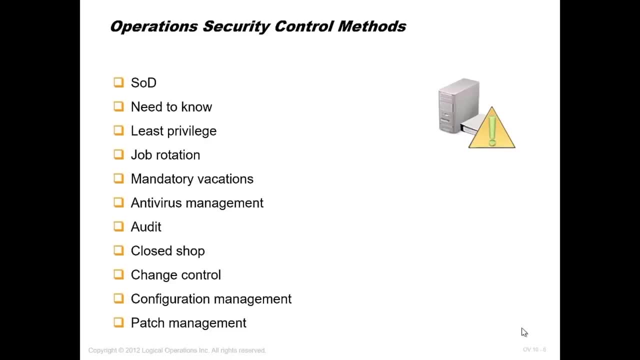 calling someone and asking to change any configuration and patch management. patch is very, very important in any organization. you checking the update and patching the application. but it should not be done individually. everyone should update or not update. it should be done centralized and most of the organization has some software that manage that. so if we are 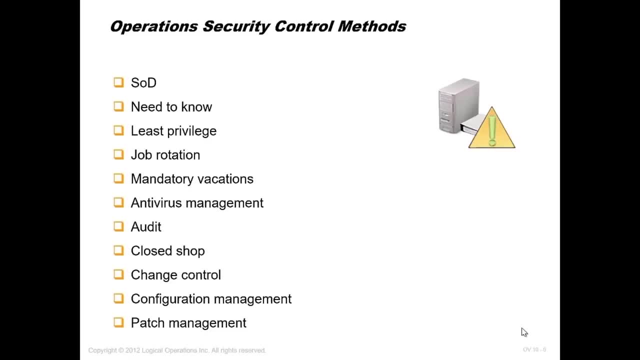 talking about Microsoft Windows. there is a service called WSource that do the centralization, do this updating centralized. they have a server that has this role, WSource, and he will test the patches and then it will be distributed on the machine. so it should be done in a 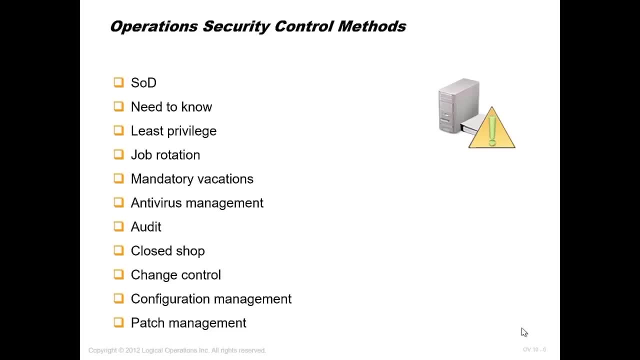 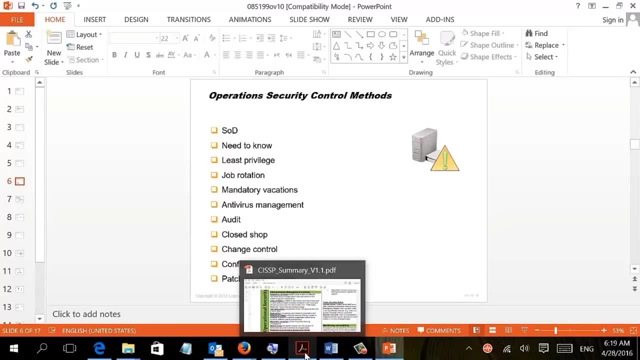 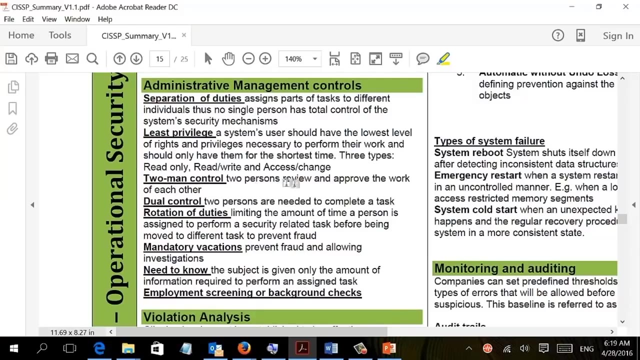 centralized with Microsoft Windows or any other product. also, I would like to show you a couple of extra policy inside the sunflower which I believe is quite important. separation of duty already spoke about list privilege to man control, which is two-person review and approve the work for each other. this is 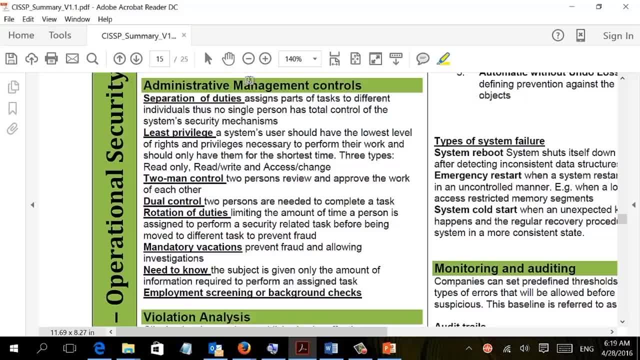 one way for controlling the security. it's an administrative technology need dual controls that two person are needed to complete the task. it's like movie: when people try to launch a missile, the two people need to open, like or use their own key together. this is called dual control. rotation of duty. who? 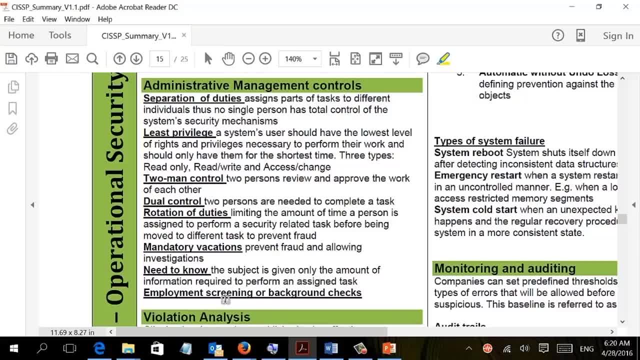 spoke about mandatory vacation, need to know employment and employment screaming or background. it's mainly into the HR part where if you are hiring someone especially sensitive position, you need to do a background check just to make sure that you know he's suitable for such position. so those policy you have to read, you have to. 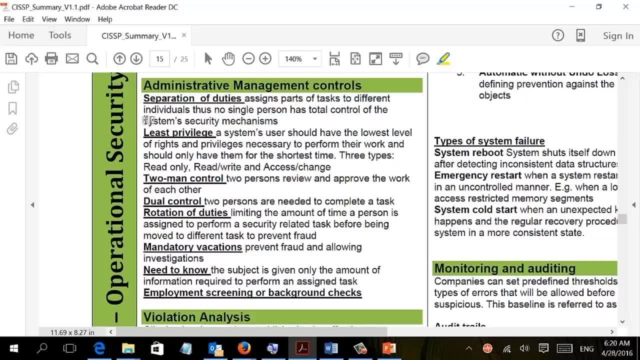 memorize them, you'll be able to know the regular one. I mean, if I'm telling you list privilege, it makes sense. but what about two-man control or dual control? sometimes you get confused about it. so this need to be written, the administrative policy or administrative management control, and to be memorized. 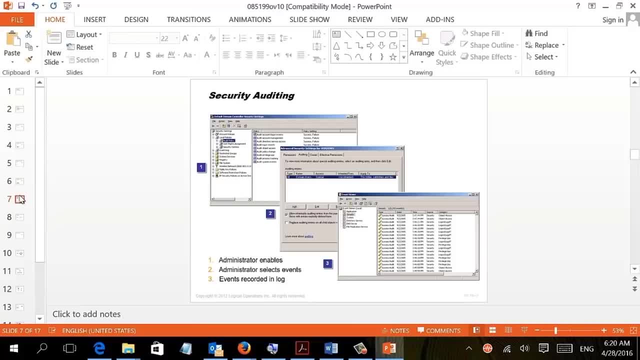 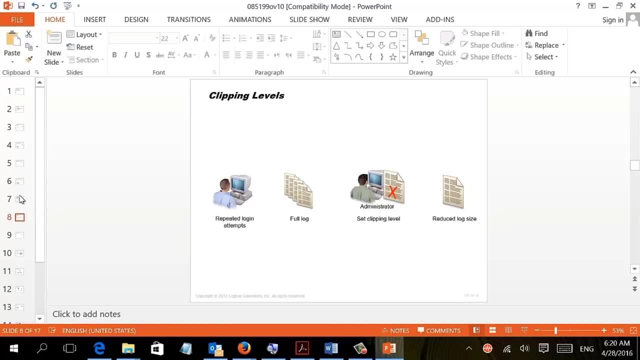 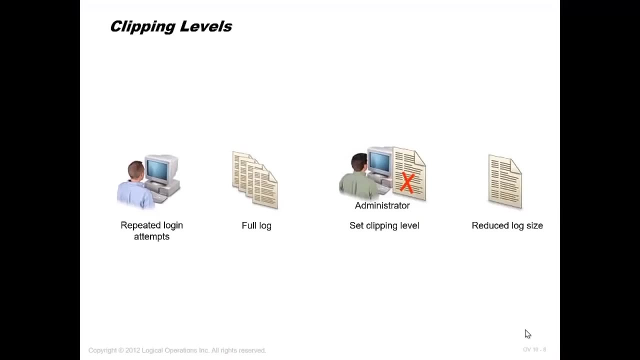 then. so those was a policy, security management, control and to be able to manage the security of the thing. yeah, this also, it's important terminology: clipping level. what is a clipping level? clipping level is to identify the level of error where you should expect something malicious. let me give you an. 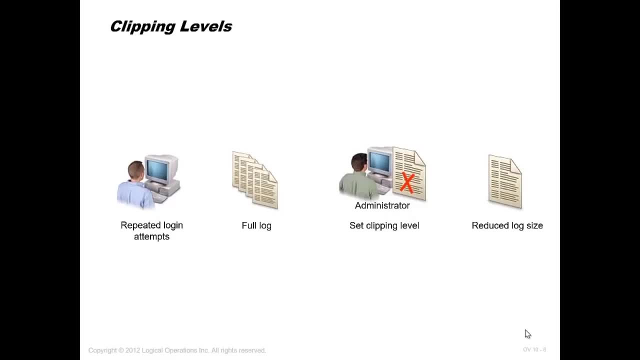 example, some system will allow users to login three time. try to login three time, but if you fail to login three times successfully, it will be blocked for like one day and you have to call the service desk to allow the service, like banks. but some other service give a chance for five. attempt. other service: give two. 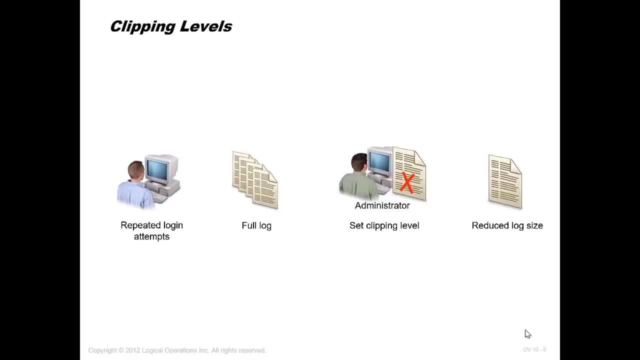 attempt. this is called the clipping level. how many attempt I should allow the user to try to login and after that I should block it because it seems suspicious. there is no like a standard that it depends about how complex your system is. so if you are giving user passwords, that 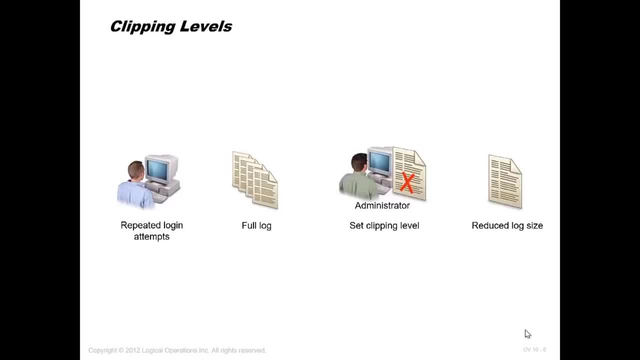 is 15 character, capital and small, and, and, and letters and number and so on. most probably, you know, he may need like four or five attempt. well, if you are giving user a pen number of four, number three attempt will be enough. so clipping level it's to identify the number of unsuccessful attempt that the user try. 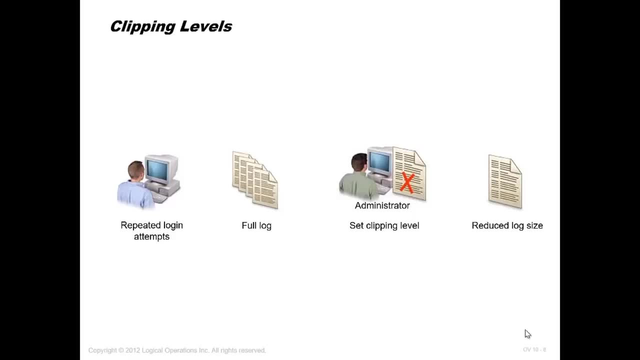 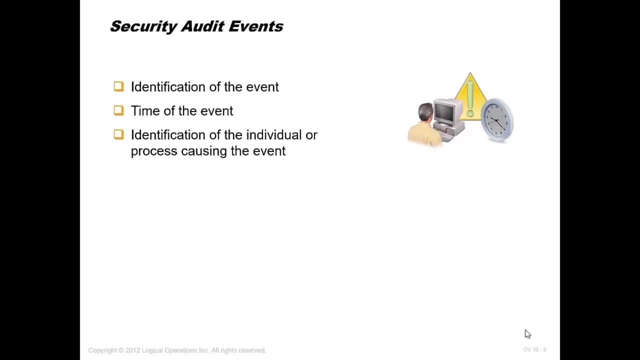 and after that you block him because this is seem malicious. so please write it down is quite important. you should audit the event from time to time because a lot of people are just checking the logs and event just in case there is a problem. but I've actually you. 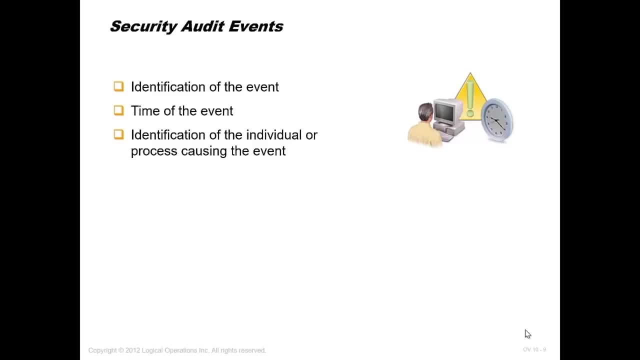 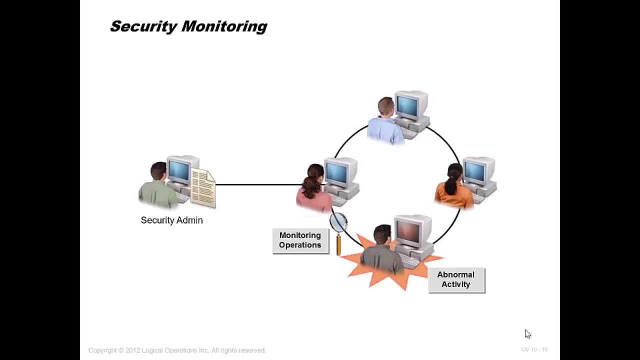 have to do that periodically just to identify your baseline, what is normal and what is not normal. so you need to do that from time to time. you need to identify the event, the time of the event, who did that event and so on. now also the security monitoring and evaluating any kind of violations- very important some. 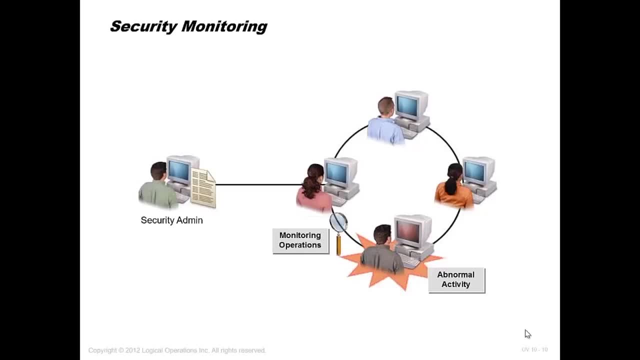 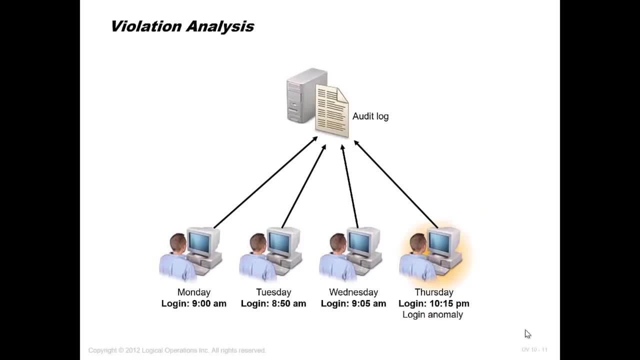 people are doing that unintentionally- zero value violating their policy- and some people are doing that intentionally. so it's very important to monitor people and to analysis the violations that they are doing. maybe someone is doing something wrong because they are not aware of the company policy about that. 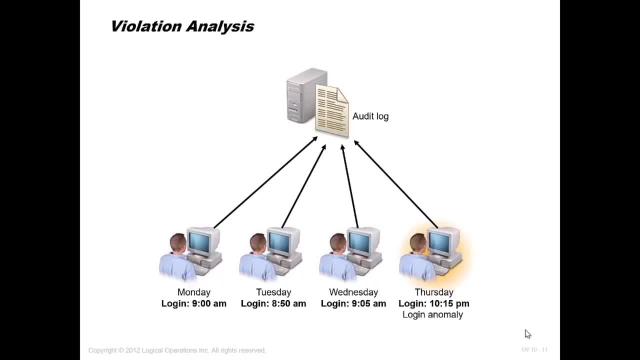 but maybe someone is doing something wrong because tensionally you need to do something- the computer- so I cannot give the same penalty for both of them. if someone is doing that unintentionally, he's not aware that he should. our company policy regarding email that mail, company mail, should not be used for private reason. he was not aware of that so I just need. 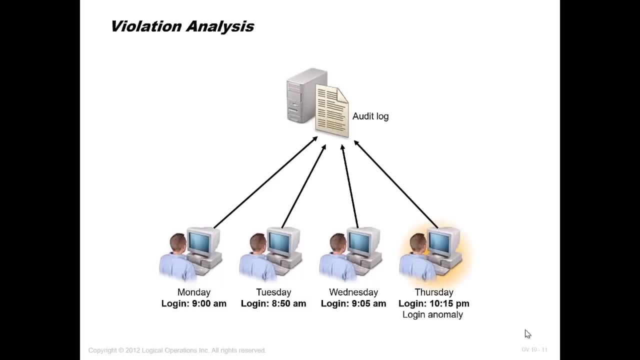 to inform him. well, if someone is trying to like some company confidential information using the email, this need to be taking in consideration and a hard action need to be taking against this guy because this is a malicious activity. so I cannot give the same kind of punishment for both people. they are both misused the email, but in a different way. 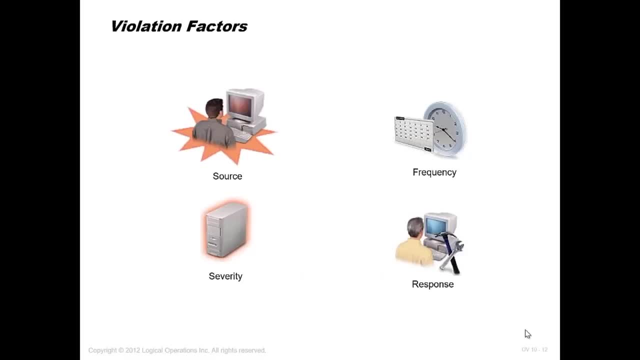 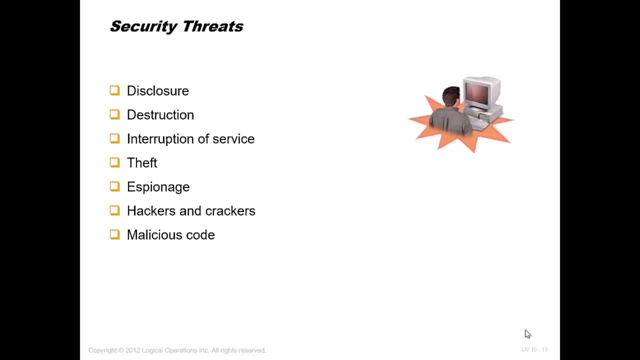 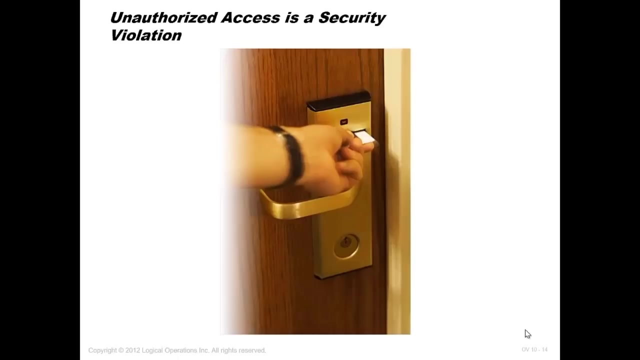 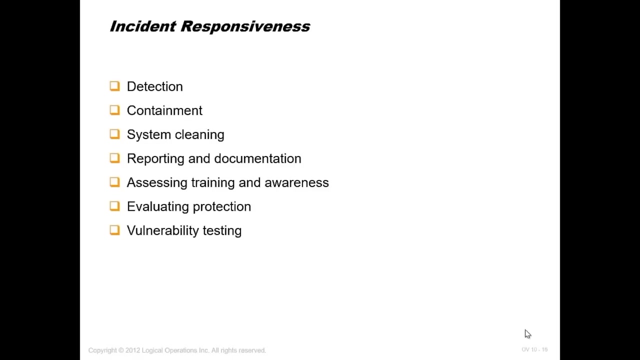 so you have to analysis the violation security team. I'm sorry, security threats, disclosure, disclosure destruction, theft, esponage, hacker and cracker. we went through that before. unauthorized access is a security violation. there is a physical violation type, logical. I mean, it's quite, you know, quite clear what we are talking about: incident response. this is actually a big 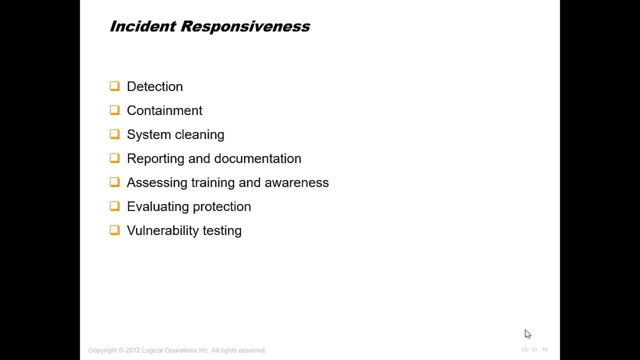 a big subject and instant response. it's the proper action to be taking in case of any incident. so incident could be small incident, big incident, but you should have a procedures: what should be done first and what should be done next. so the first thing you should detect: 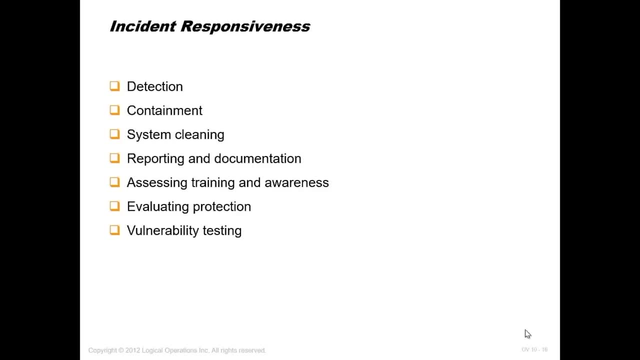 that this is an incident. a virus has been spreaded inside network. I should first detect, then content mean I try to stop the bleeding. then I should start system cleaning, remove the virus, then reporting and documenting that so in future I can prevent that, then assess training and 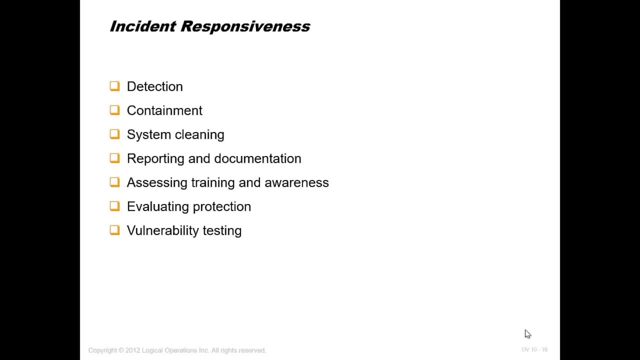 awareness. I should do some lesson learn and start training my team: what happened, how, what was the best actions that was taking, what was taking and can be taking in a better way next time, and so on, and then evaluating our protection and then vulnerability testing. so those are the step in. 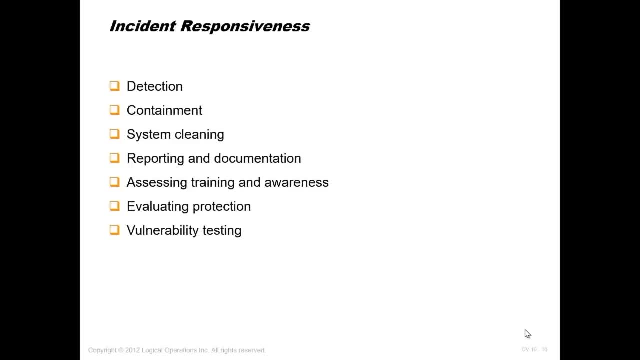 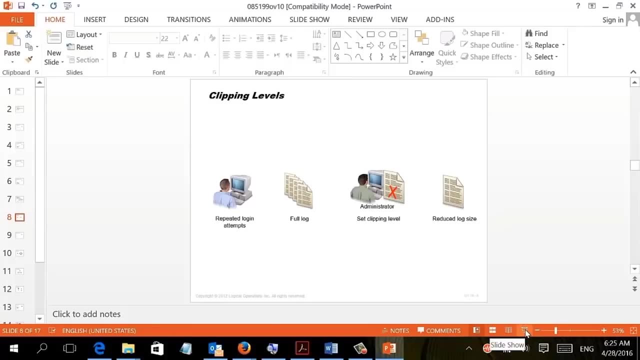 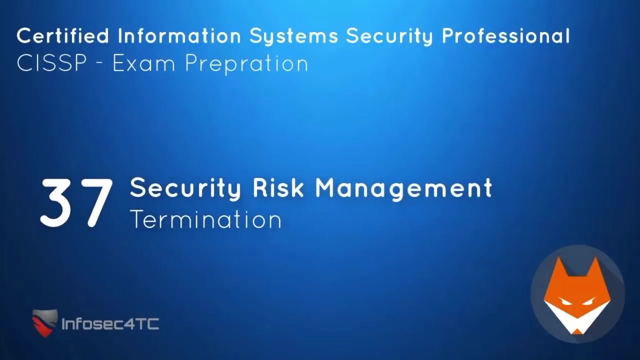 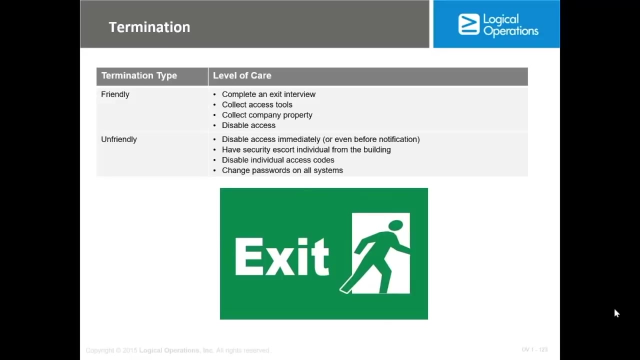 incident response, just to make sure things enhanced so people will be aware later on what to do. this is the operation security quite small module and the only importance is the policy is the best practice, the control and this terminology, clipping level and stuff like that. even in case of employee termination, there is a proper way for doing it from a security. 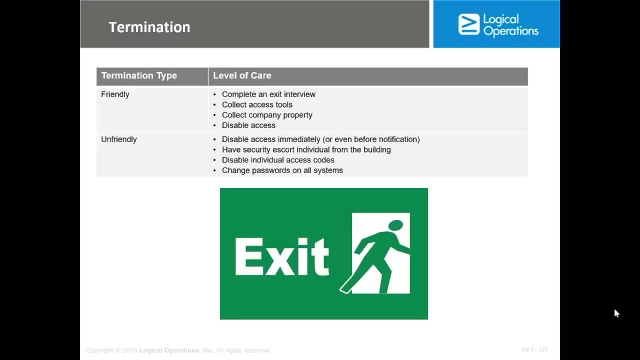 perspective. so if an employee get terminated, first you should disable his account immediately and then you should inform him and give him around 15 minutes to take all his belonging and why. we are not giving war. we are just giving him 15 minutes to not allow him, allowing him to do any. 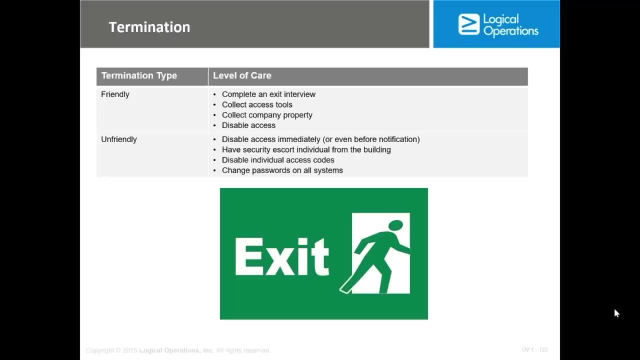 kind of damage. so if you inform an employee that he was fired and you left him till the end of the day, Imagine the amount of damage Demage The can do. he may delete a lot of file because you know, after all he is so. 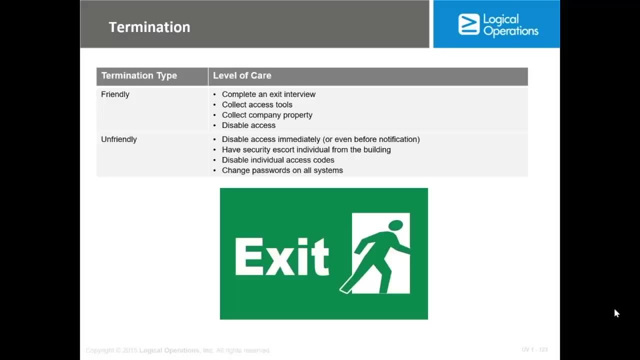 upset. so you need to inform him and you need to give him 15 minutes to to collect all his belonging and then you need to escort him to the door. I know it seemed very mean, but this is how things is going. so terminated employee is also a big threat to any business. so from this discussion, this lecture in the 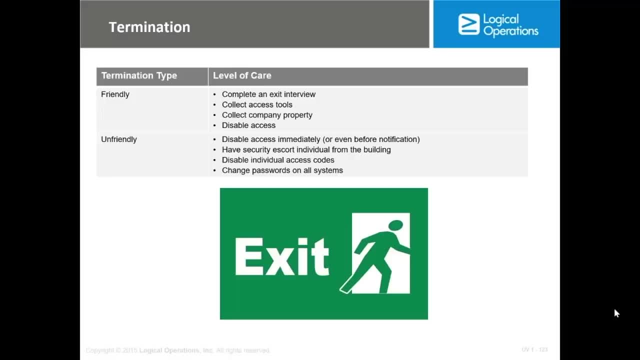 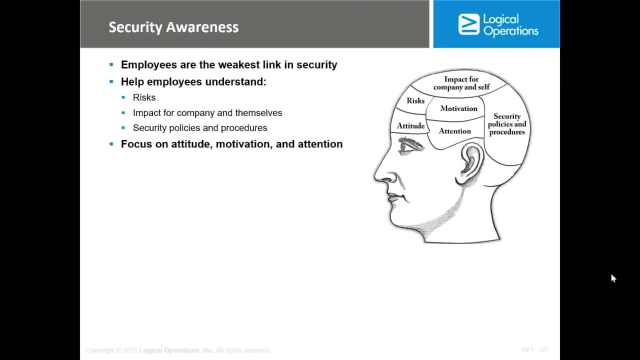 previous lecture. those are some of the controls that you can implement to reduce this kind of threats and to put controls on the employee, which is considered the weakest link in any organization. we have two point remaining in this domain. I know this is a very big domain actually and it combined a lot of previous domains, but we still have two. 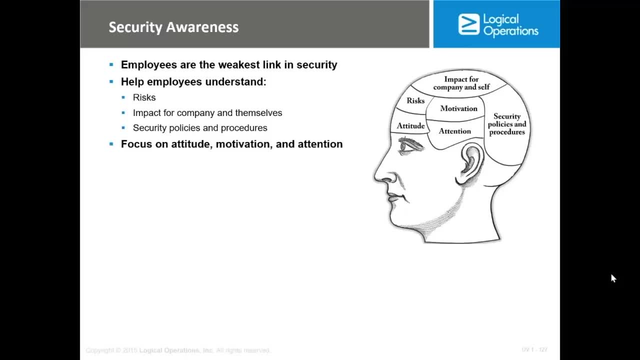 point remaining. we're going to talk about security awareness and then we're going to talk about security testing. now, security awareness- it's a topic related to the previous lectures. for employees and and and I. actually, this is a very, very important topic. maybe you're going to. 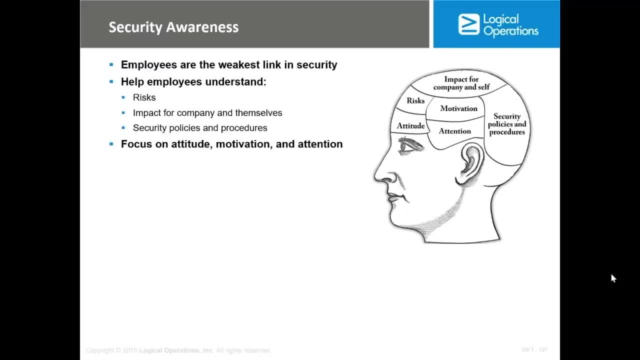 explain what is security awareness and why we are doing it, but actually it's a main requirement for any compliance. I mean, if you are ISO 27001 certified or if you are following any kind of standard or compliance, you're going to find that one of the main requirement it's to do a security awareness for all. 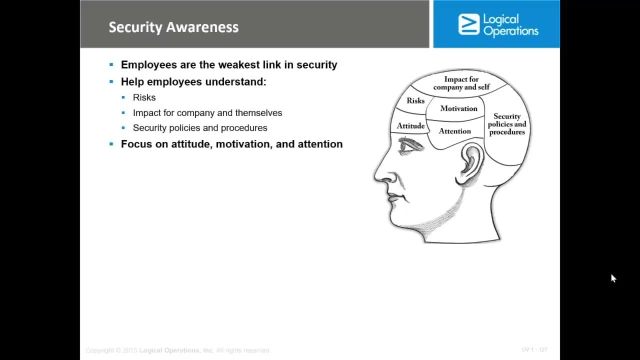 your, your employee, frequently. it's not a one-time process. you have to do that once per year and I saw myself any audit that was related to ISO 27001 or any other kind of compliance. one of the things that they will always ask about: show us the attendance or an 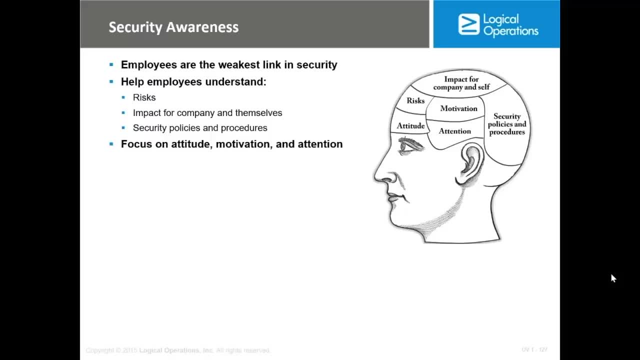 evidence that people attend the security awareness in your company and why they are doing that? because, as I mentioned earlier that most of the incident and compromising system was because of people, not because of technology. so, as we keep saying the last few lectures that employees are the weakest link in any organization, they may do damage. 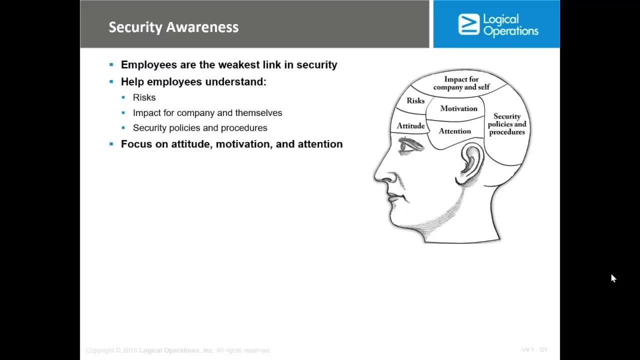 intentionally or unintentionally. so you have to provide them with a security awareness session once per year. it shouldn't be like a full five day training or even a full day training. it could be like one session, couple of hour and you start explain to them the threats, the, their role and 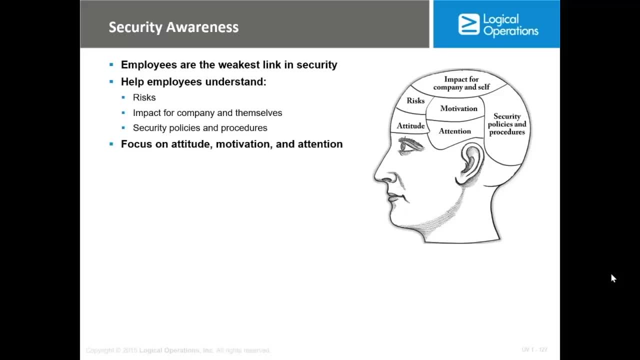 responsibility, which is very, very important, because the the concept here that you should eliminate: i didn't know. so if someone did something wrong he should not say i didn't know, because if he's attending the awareness and he knows that he should not click on the links, that 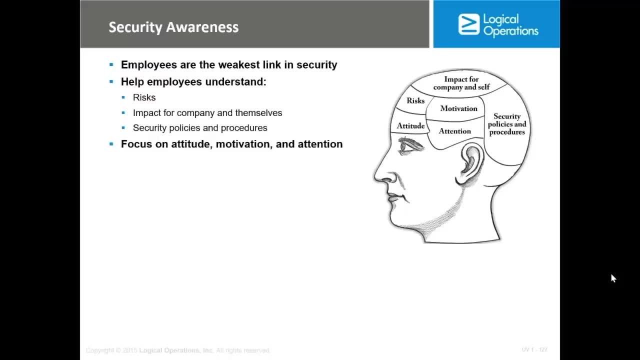 are there to prevent any suspicion email or or any suspicious uh sms. so he will tell you- i didn't know, but if he attends awareness and he will be aware of the new threats- what is the ransomware? what is a virus? what is uh? what is the best practice when it come to uh mails or sms that will 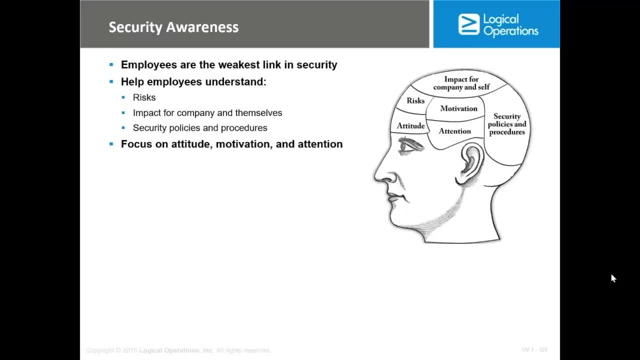 prevent any problem with the company network or data or information. he will be more responsible because by attending the awareness he cannot say i didn't know. beside he will know that he is responsible. if he did something wrong, he will take responsibility for that and we saw that in a lot of companies that if people didn't attend, 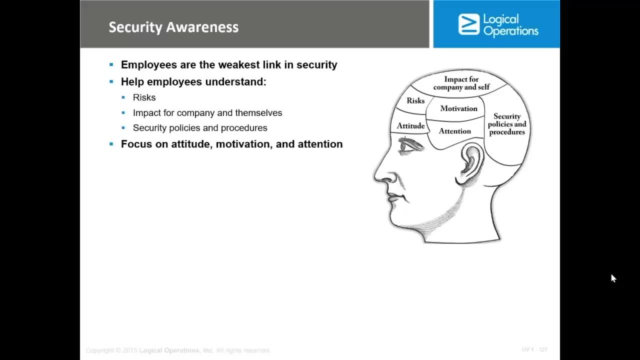 awareness. they don't care. whenever they receive an email, they will open it, they will download the attachments, they will click on the link because people think you know what could go wrong. but when they attend the awareness and they know that there is a threat and if something went wrong, 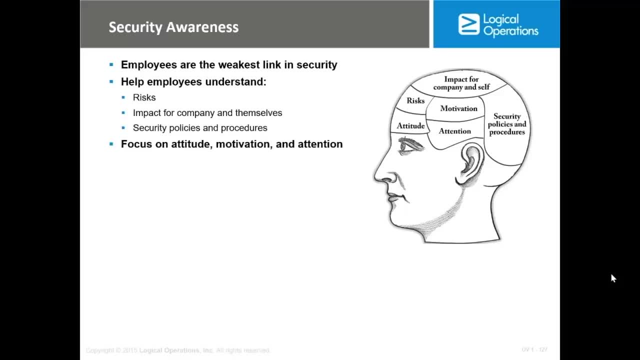 because of their behavior or because they are like not giving attention to that. they will face problem. could be legal problem, could be business problem, but they will face problems. they will be more careful. so it's very, very important to arrange those security awareness station and actually i can share with you 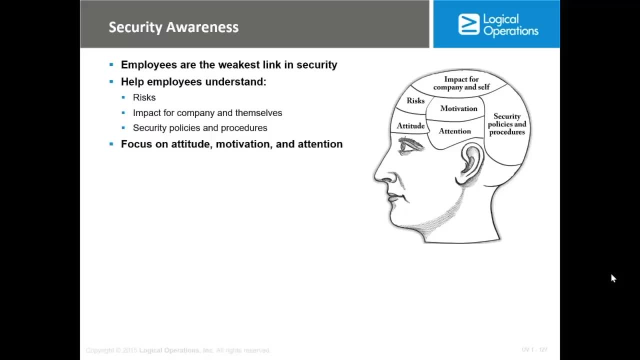 uh, some of the presentations that i did for security awareness is that you can do to your company or your organization or your department. and, by the way, security awareness should not be done only for it stuff or it department, but it should be done for all the company employees. 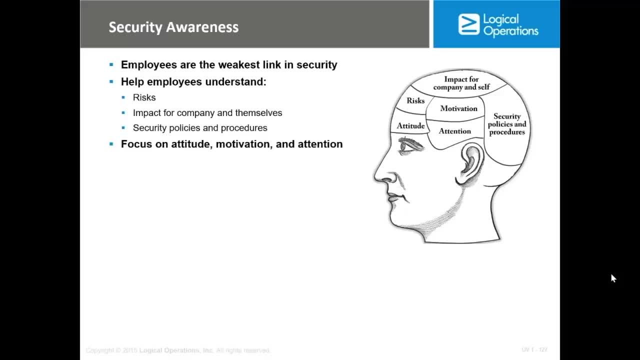 from hr for from finance, from operation. everyone should attend this awareness session. it's a main requirement and, as i was saying, whenever you have any audit, one of the main things that they are asking about and evidence that people attended this employee- and they will go and ask some random employee: did you attend the awareness? do you know your? 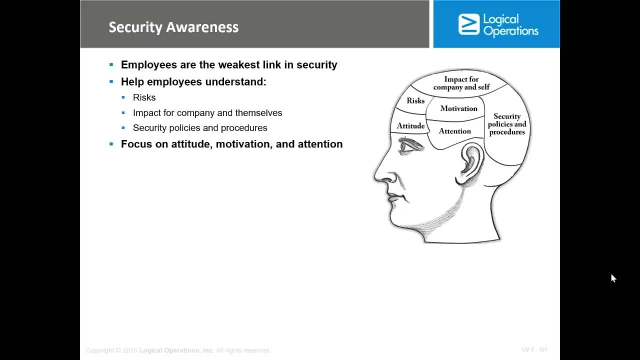 role and responsibility. another objective or scope for this security awareness is to tell people that we, as a company, we have a security policy and you need to be aware of those policy and their location. this is quite important because if the employee is using any company assets or service, there should be a policy, which we already explained at the beginning of 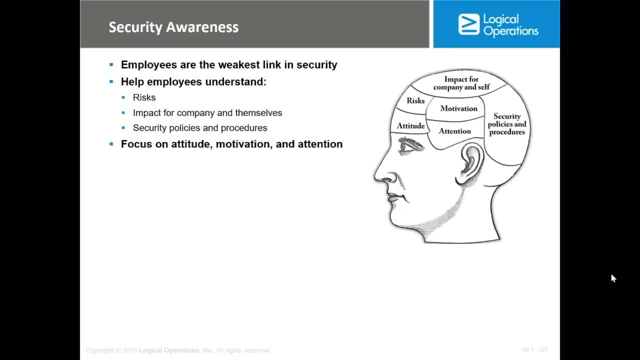 this lecture. so, for instance, he has a laptop from the company. you should have a policy related to portable device or laptop. that's saying what he should do to secure this laptop if he's using the internet in your company. you should have an internet policy, so he should treat this policy. 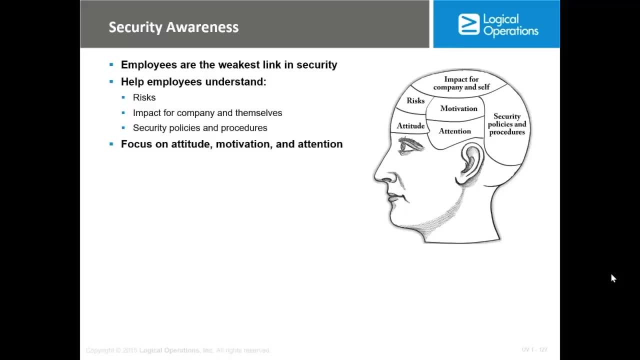 before start using the internet. by reading the policy, he will know what should, what can be done and what couldn't. he couldn't do it or should not be done. if you are giving people an email from your company domain, you should have an email policy saying what is the best practice and what should be done and what is not allowed to. 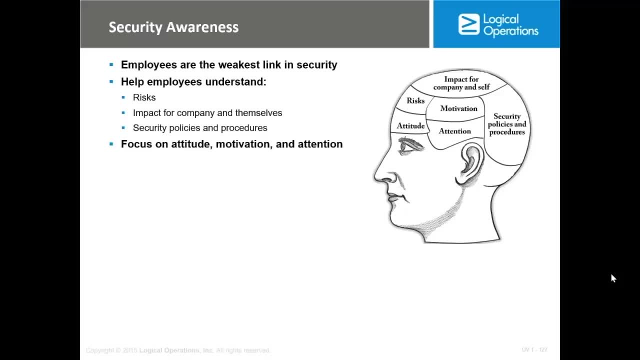 be done and we already spoke about policy. but if you are doing those policy and employee are not aware that there is any policy in this company or in your organization, they are useless. the point is you doing the policies. then you have to inform the employee about the policy and their location. 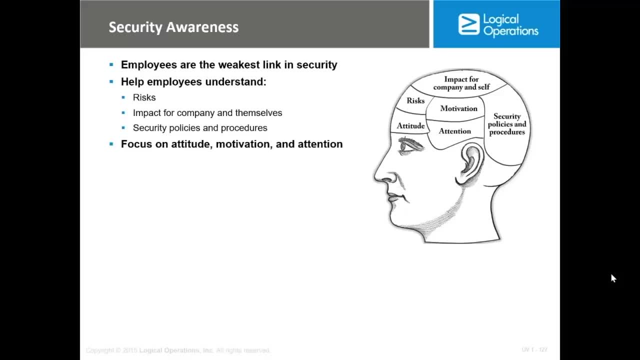 they. they don't need to memorize all the policy at, but at least they should know where they can get those policy. and they should know that if they are not aware of the policy, it will not prevent them from any punishment if they did something wrong. so you are saying, okay, fine, if you are using any service, just have a look about the policy related. 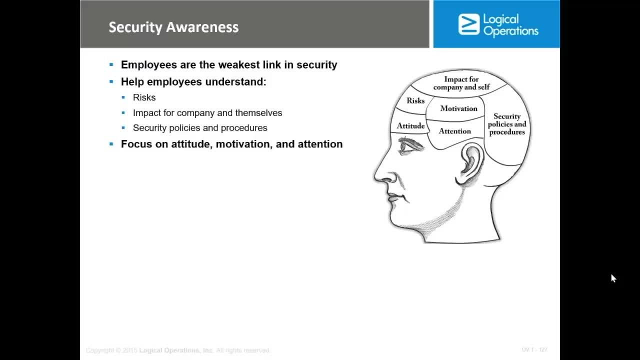 to the service because by not knowing the policy, it's not an excuse. so security organization is quite important and one more time, i'm offering some of the free presentations that i did for employees for security awareness, if it's going to help you improve the security in your organization. 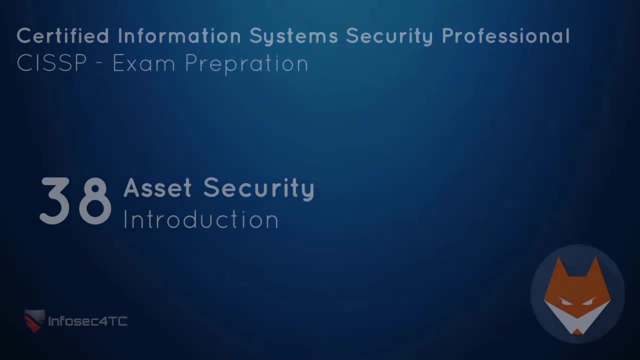 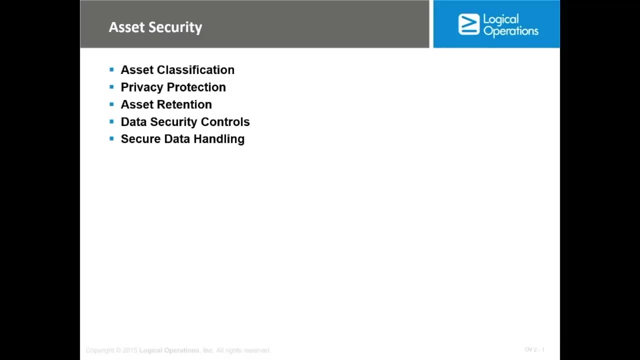 let's start with the second domain, which about asset security. this is actually a short domain. it's not like the previous one, where we covered a lot of topics. here we only going to talk about asset security. it's maybe a short domain but actually and realistically is very important. 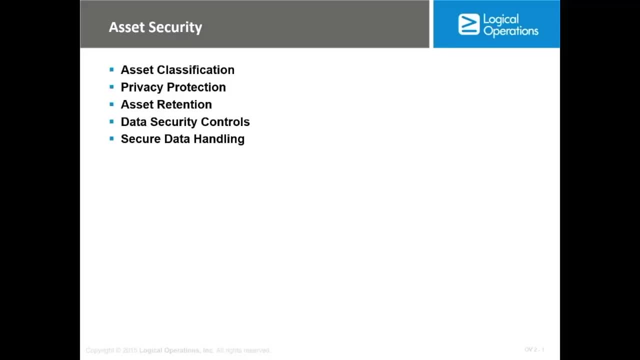 so, if you plan to start an information security implementation in any organization, from where should you start? and let me simplify the question: at your house, and i believe i already gave you this example before, but at your house. if you plan to secure your house based on what you're going to decide, 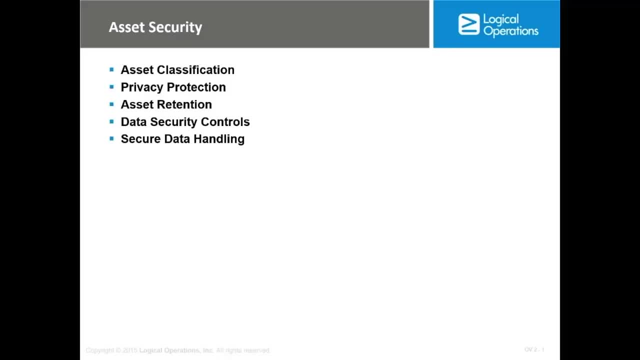 what to secure and how much you're going to spend, usually based on the value of the assets that you have. you may have a lot of assets, you may have a lot of assets, and you may have a lot of assets. have a computer, you may have a laptop. you may have money, you may have assets. 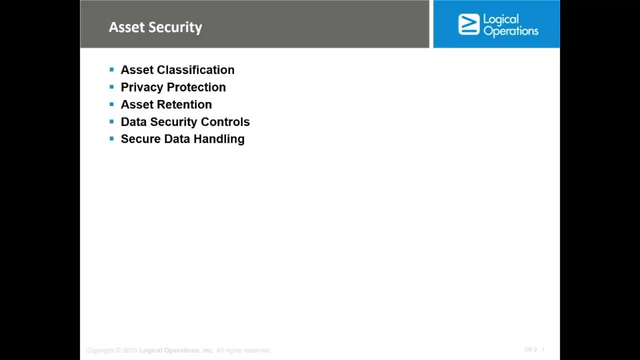 in your house that you need to secure, and based on the risk. so if you are in secure area, you will not spend that much, like if you are in in an unsecure area, right? so two factors usually let you decide about how are you going to implement security and how much you're gonna spend to secure. same concept. 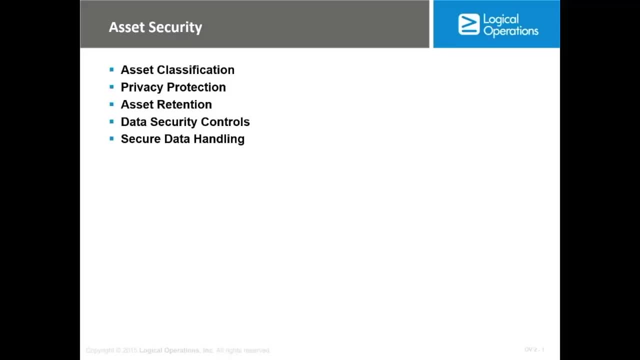 apply in any business: according to what we're gonna secure our organization, according to the value of the assets that we have and the risks that we are facing. and, to take an example, let's talk about the bank. what assets the bank have? they have physical assets and they have. 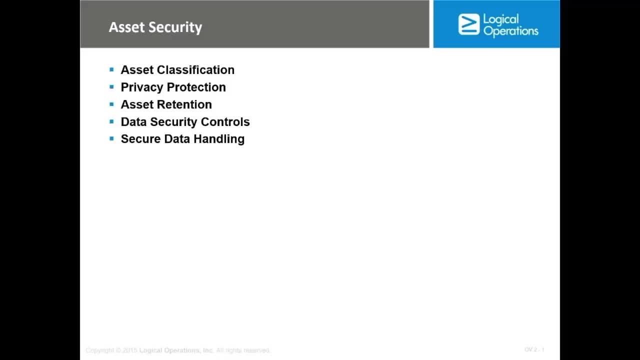 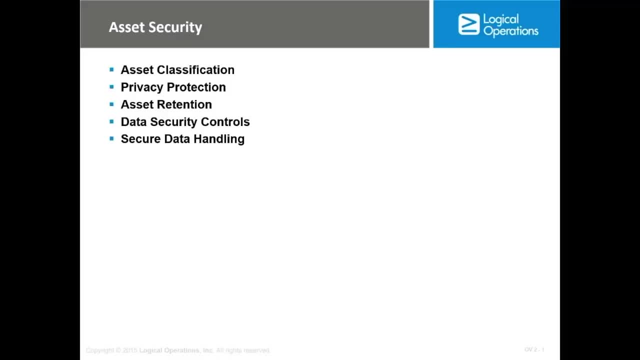 information asset. I mean, if the bank is a bank, lost a couple of chair, couple of table get broken or something like that, how much would be his lost? well, if the bank lost some customer information with the fight with their financial transaction, how much this will last? right, so usually the information. 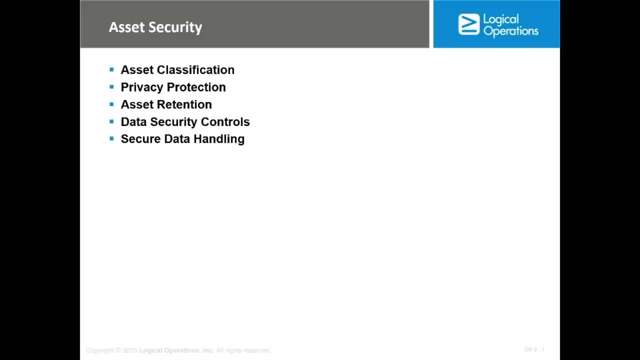 assets is the most valuable assets to any business and in any business they used to have like an inventory with all the physical assets but the they don't have any information assets, and this is what we're going to start with: how to create an information asset register. so, before showing you how to do, 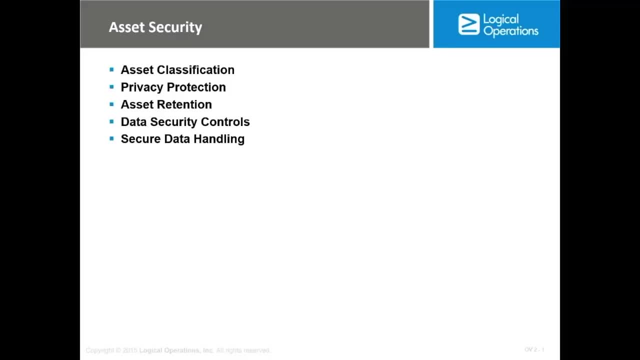 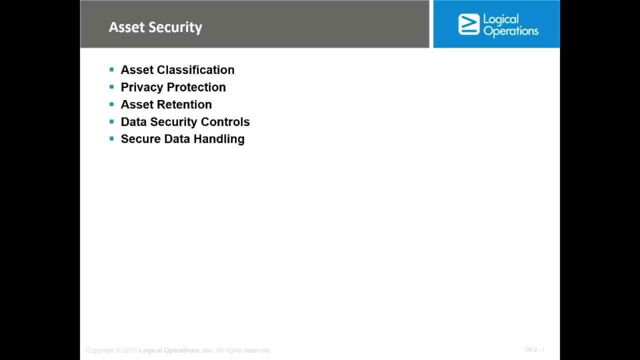 your smartphone as an example. your smartphone as an example, your smartphone or something. you maybe spend five hundred or one thousand to buy it, but you save on on this phone a lot of information. you have contacts, you have email, you have personal photo, you have personal video. so if you lost your, 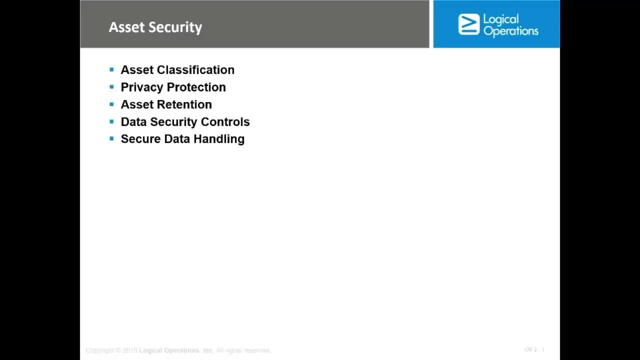 smartphone. what would be your real lost? would it be the phone itself, the price of the phone? definitely you will be upset about those five hundred dollar or one thousand dollars that you lost, but most probably you'll be more upset about the information on the phone. how much time 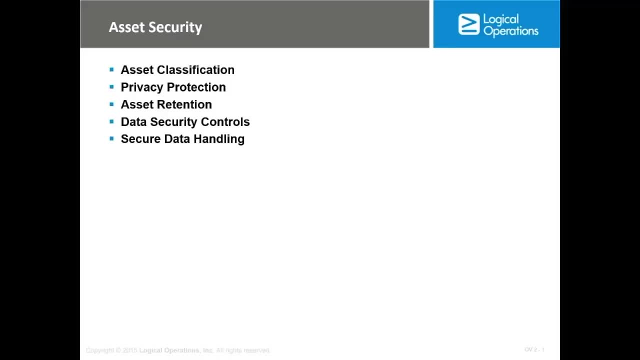 you're going to need to recover all those contact, how much time you need what if someone reset your password still still your information on this phone. so usually the information is the real assets that we need to configure. so in this domain, I'm going to show you how to create an information asset register. 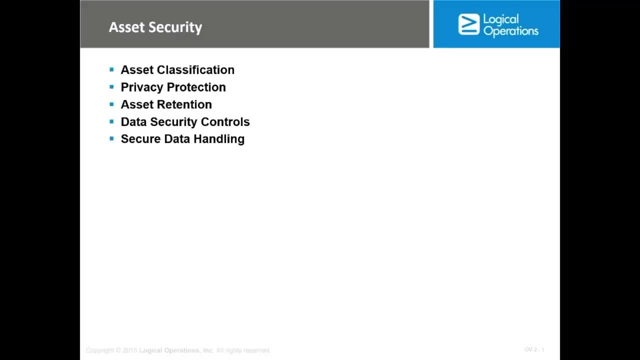 which is very important, and usually any information security framework like ISO 27001 or PCI DSS or even any other ISO like the business continuity ISO, one of the first requirement whenever they come for an audit, they will check: do you have an information asset list? because if you, 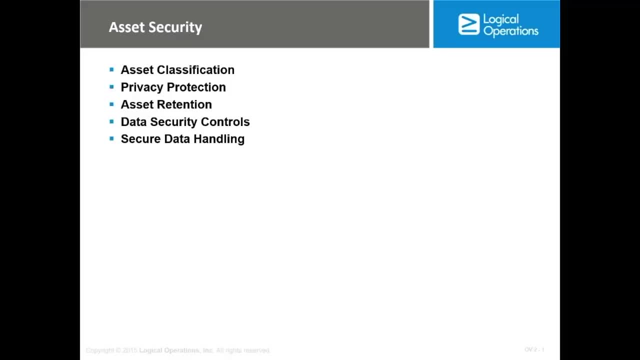 don't have. how can you secure them? if I don't know the value of the information that I have and they are not written in one list, how can I secure them? how can I decide what need to be secure or not? so what we're gonna learn in this domain. 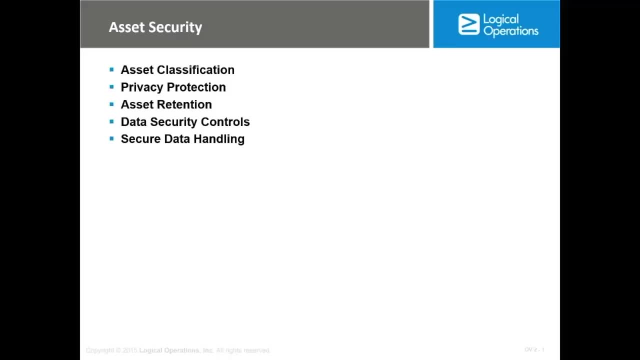 will be: first, how to create an information asset register and what is the information asset register in the first place. then the asset classification, and here you're gonna about the classification, the asset owner, the custodian. then I'm going to talk about privacy protection, I'm going 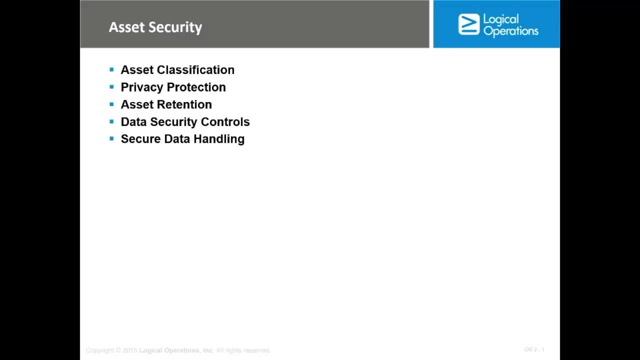 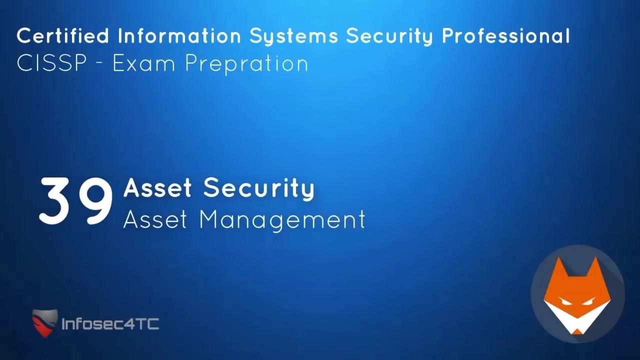 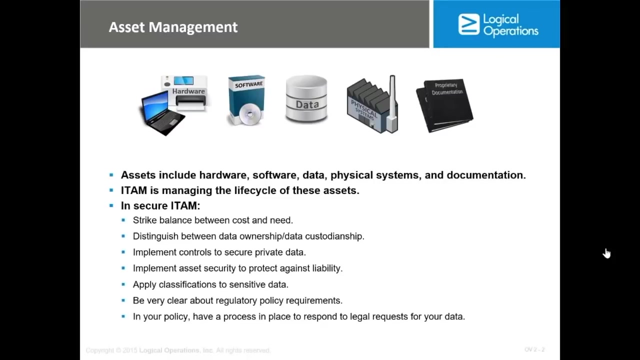 to talk about asset retention: how long should I keep an asset and what is a policy when it come to management or depreciation? attention, then data security, controls and finally, secure data handling. So let's start with the first lecture. From our previous discussion, we agreed that, as a business, you need to have a 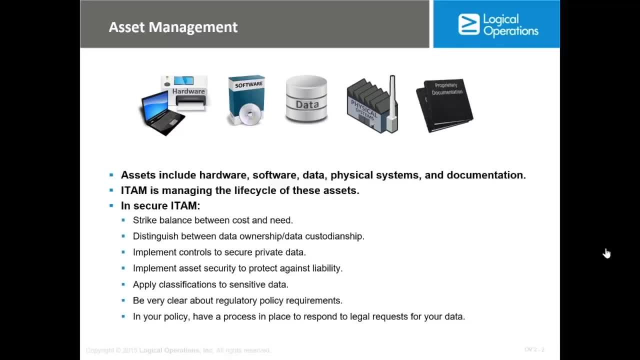 list of all your assets. Now, what are those assets and what are the assets that is usually available and what is the assets that you need to do it yourself? So if you go to any organization, you will find that they usually have a list of. 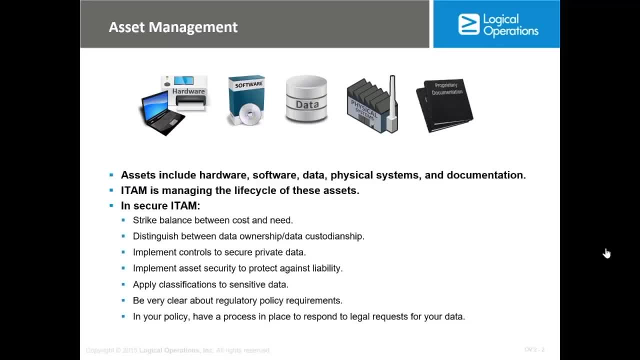 all the physical assets, things like computers or laptop shares, table cables, switches- All those are listed in assets and sometimes it's under the. it's managed by the finance department because they need to know how much they spend on that. Sometimes They have. 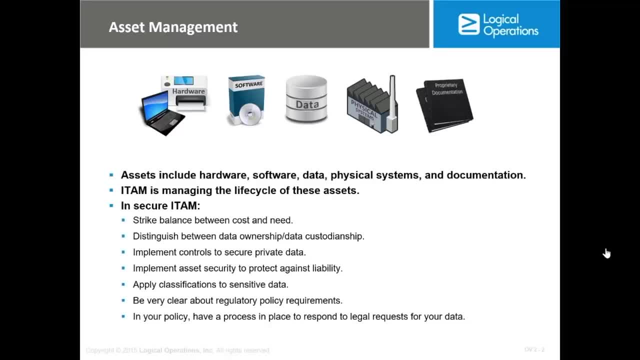 An asset department and so on, But the weakness is usually in organizations. They don't have an information asset list, And this is what I'm going to show you in the next lecture, And if you go to any or if you get hired anywhere, this is one of the main lists. 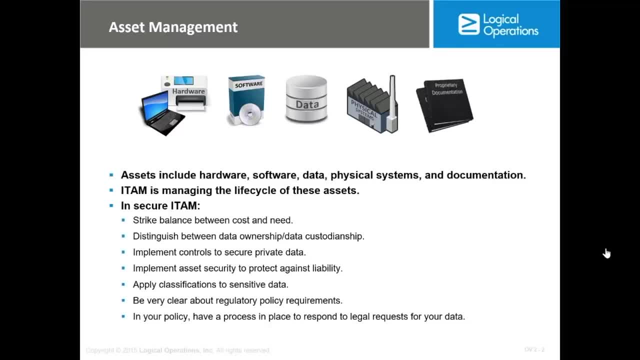 that you need to make sure is there, because if you get any audit or any compliance audit or legal audit, they will ask you for that, Because the information, as I explained in the previous lecture, is your main assets as a business right. 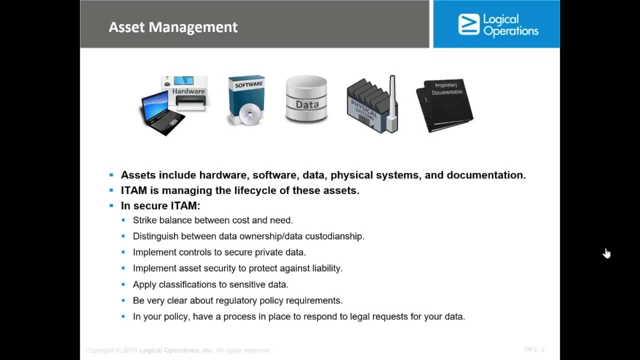 Think about banks, For instance, how much their information was. Can they afford to lose any of those information? If you have a bank account and you lost it, is it acceptable? Can you take a legal action against the bank because of that? 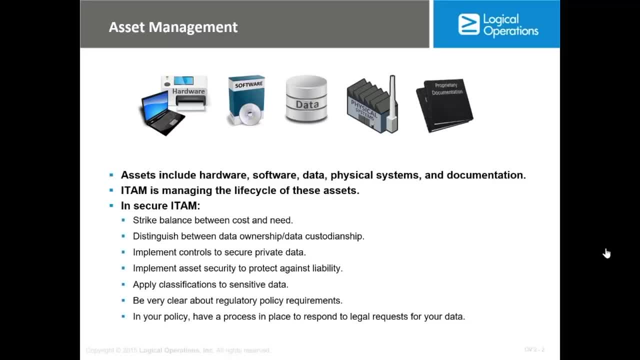 Is anyone going to trust the bank to open an account if you lose one customer information? It's quite important: Right, Military or government, What is their information and how much it was, and so on. So, in general, before showing you how to create the asset list, which is a very important, 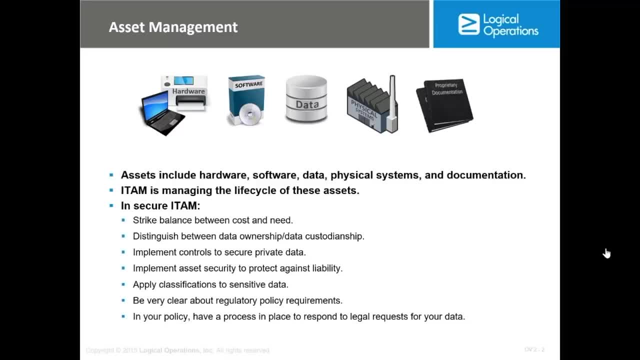 document in the organization and you are not the one who is filling it. by the way, the information asset list or the information asset register is usually filled by department. You are just making sure that they are filling it right. So if anything get lost, you will be. 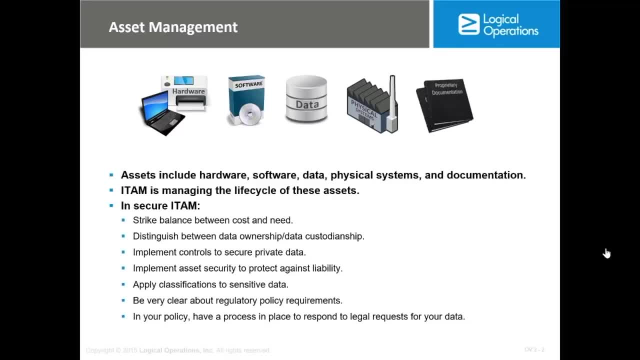 Knowing who's responsible and who is not. So in any organization, what kind of assets they have. They have hardware, They have software, They have data asset, physical system documentation, ITM or IT asset management is to manage the life cycle of those assets, to have the list where you are writing down all. 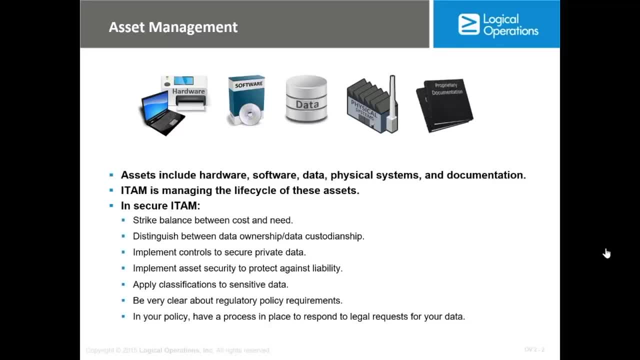 this information. By the way, here we are talking about anything that hold assets. So if you have an external hard Drive that include a lot of files and document, this is an asset. If you have an application or a database that hold customer information, it's an asset, and so on and so forth. 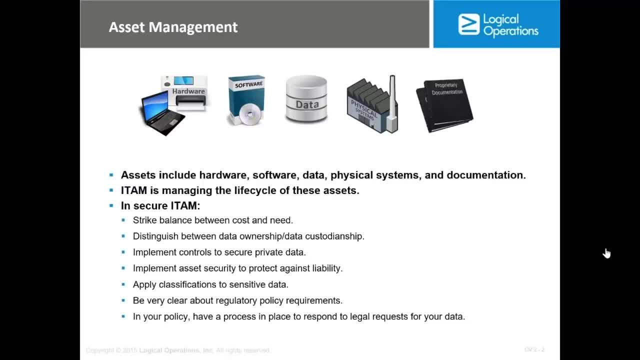 So you need to have a list that have all those asset information which I'm going to show you in the next lecture, And you need to write down the cost And also you need to identify the ownership of the asset. Now This point is very important. 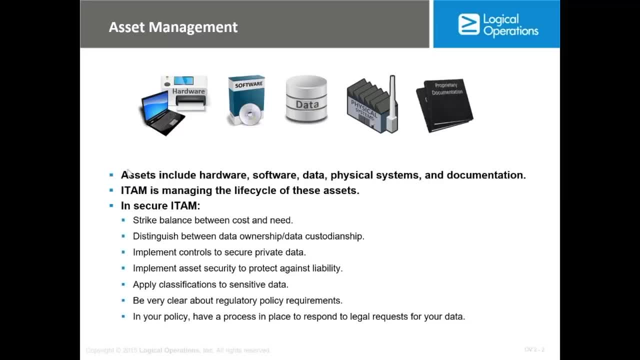 And let me have your attention on that: Any asset list, as we're going to see, will have the name of the asset, But also you should include the owner of the asset and the custodian of the asset. What's it? What is the difference between owner and custodian? 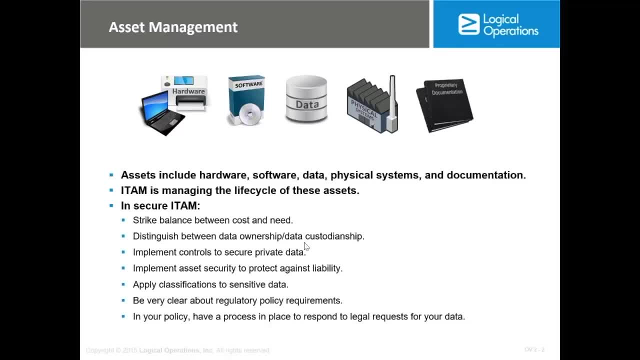 So, for instance, If you are working in an insurance company and you have a list of all this customer information, or all the customer information of this company, okay, which is very important, because if someone was able to steal this list and sell it to a competitor, he will know your customer and what deal you are giving them. 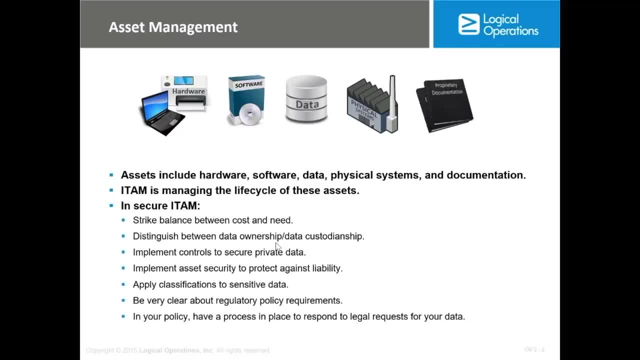 And maybe he can give better deal and steal all your customer. So, as an asset is quite important. Just Excel sheet that include all their contacts and financial details: finance details, their contact information and so on. Okay, who's the owner of this file? 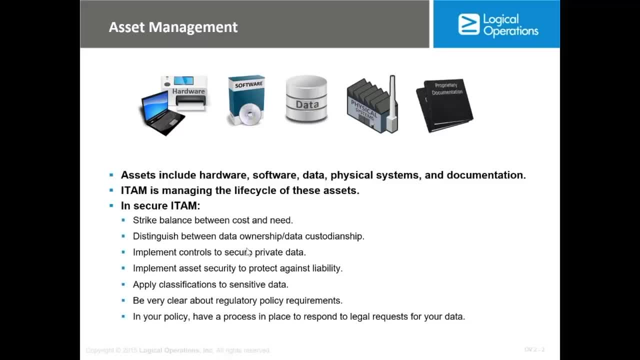 It's an Excel sheet, Is it you? Maybe you are the one who created it, But are you The owner? Let me ask you this question: If you leave the company, do you have the right to take this file with you? 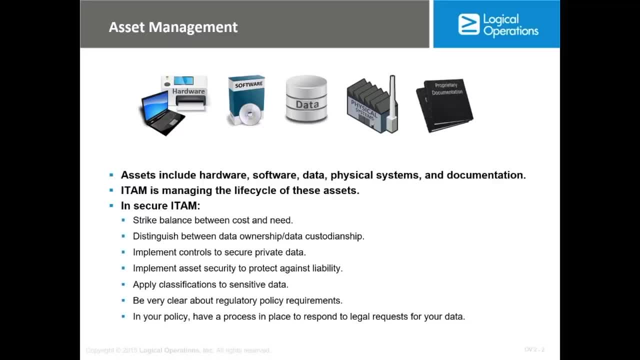 Definitely not. That means the owner. It's not you, Even if you are not. if you are the one who are creating the who created this file, you still are not the owner. The owner in most of the cases is a company right. 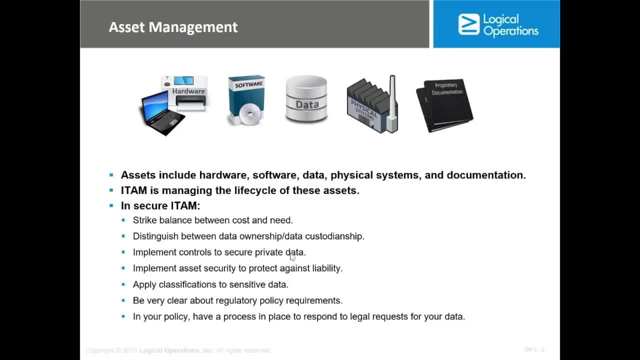 While what do you call yourself? You are the custodian, You are the one who are managing this file. So, most of the times, the owner will be, the department, Will be the company, But the custodian is one who is managing this file, who modifying, who decides the importance of the file, who decides the classification. 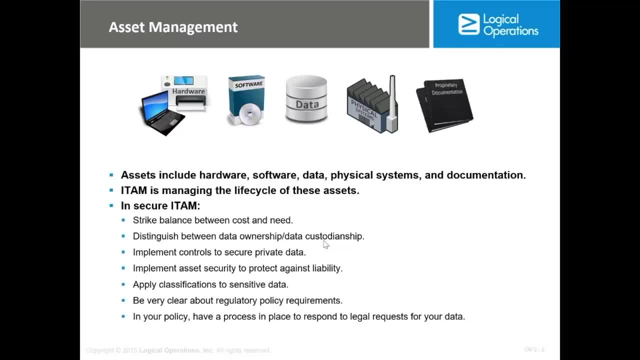 But he's not the owner in the, in a sense that he do not have the right To take the file if he leaves this company and go to another company. So very important to understand between the difference between owner and custodian and it will be very useful if in the sheet that we're going to create in the next, 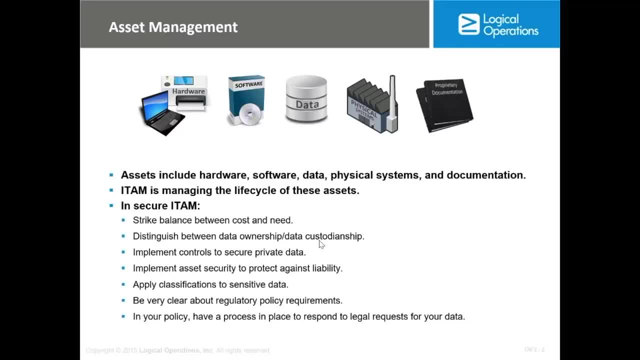 Lecture. beside identifying or writing down all the assets that you have. Also, you need to identify the owner of the assets, and the custodian Custodian means a person who is managing the asset. in case something went wrong or a file get lost, Who you gonna call or who you gonna like talk to who's responsible? while the owner- most of the time, it will be the department or it will be the company. 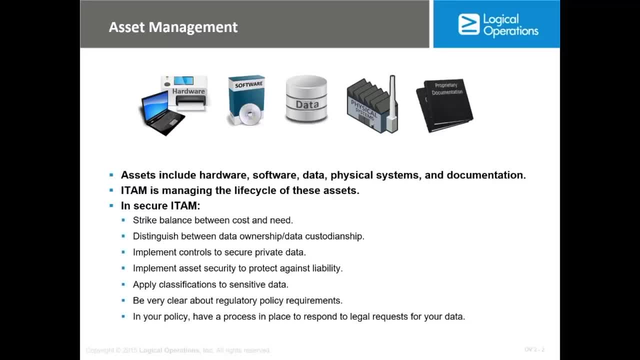 Or it could be the CEO, the senior management and so on. Also, according to the list, you're going to implement the security control to protect those data. So, for instance, if you have a list of all important file that represent report or a budget or a payroll, 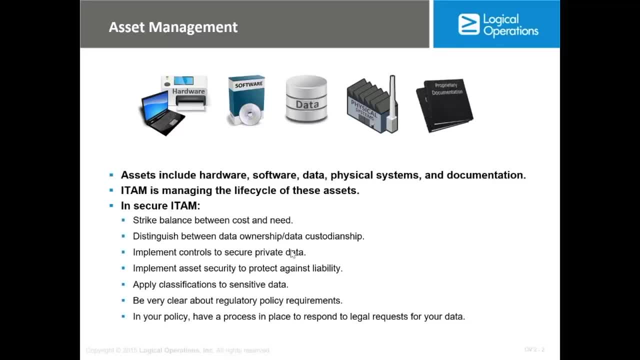 Okay, according to that, because it's written in the file that those are confidential data, You're going to decide how I'm going to secure them. Do I need to encrypt the drive? Do I need to assign a password on them? So having an information asset register will help you. 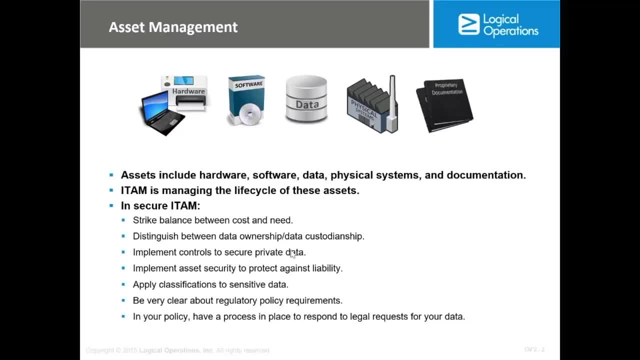 Identify what need to have security and what not. maybe in the list You have a document like a brochure. you have like a brochure template on your computer or maybe some some advertising document. They are not that quite important. If you lost them it will not affect your business. 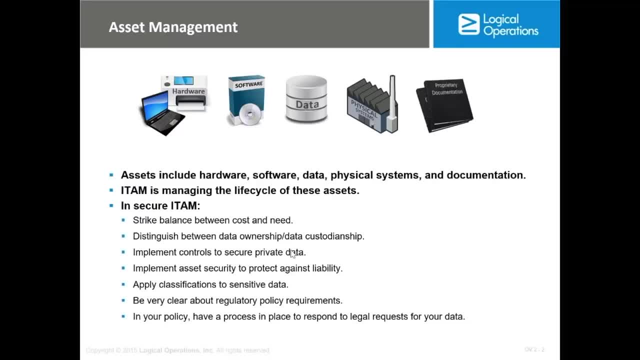 It will not affect your reputation, and so on. Okay, So Having this list Will help you to do that. So I want you not just to take the knowledge from this domain, but I want you to create an information asset list yourself. 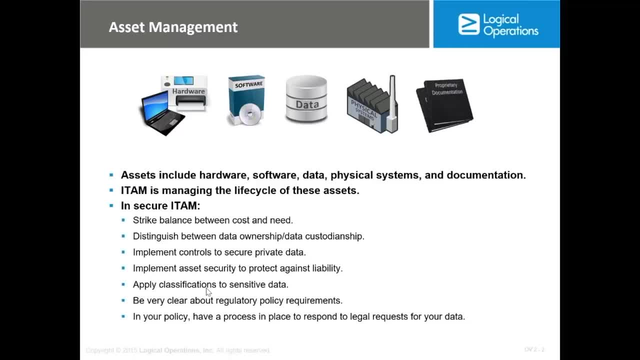 Okay, it's important to apply classification, as you're going to see, according to the sensitivity of data. So it's not just just writing down the list of information and list of software and list of data that you have in a list, But also you need to classify them. 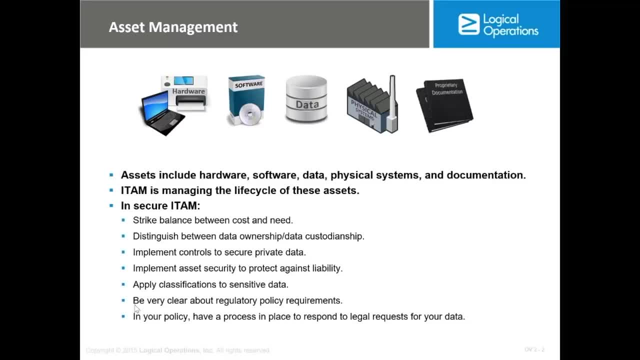 You need to identify the owner and custodian Very be very clear about the regulation policy requirement and about the legal as well. What do we mean by that? Let me give you a small example which is very, very important: right logs any application or any software or any computer. 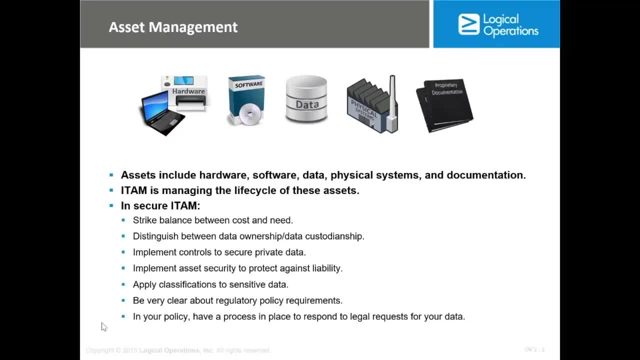 They have logs right And in one of the lecture I'm going to show you how to check the computer logs. If you have a surveillance cam, for instance in your company, they are keeping videos, They are recording video right. 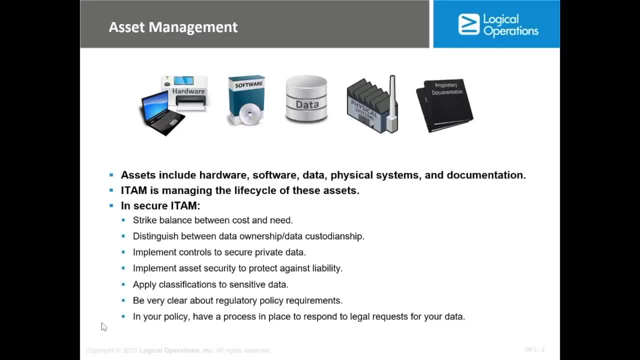 How long those logs or those video you should keep them. Should I keep them for one month? Should I keep them for one day? I mean, I'm recording those surveillance video and I keep them in some storage in my company. or I'm capturing logs from my system and I keep them. 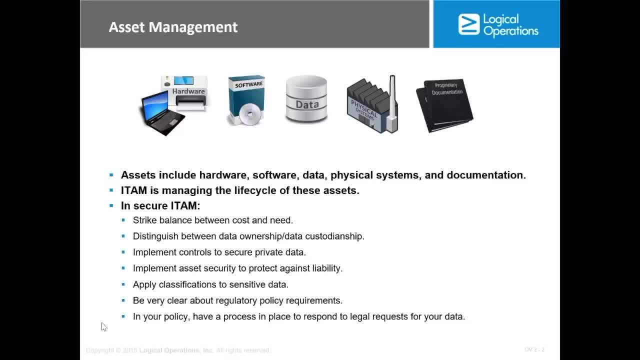 How long should I keep them? What do you think? Should I keep them for two days, for one week, for one year? because I cannot say I will keep them forever, because it will take storage And by keeping all those recording or all the slugs, you know, it's an endless process. 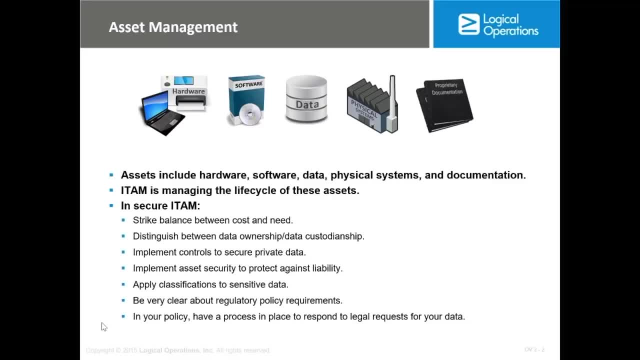 So you have to keep them for a time or for like a period of time, and then get rid of them. Okay, let's assume that you decided to keep them from for one week Because you checked and you don't have enough storage. So you decided to keep all those recording and all those logs for one week and then 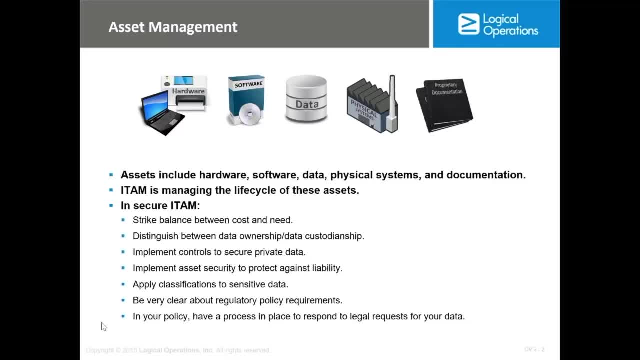 A robbery happened to your bank or someone steal something or someone like hack to the company network and steal critical information. You're going to inform law enforcement and then law enforcement will come and ask you: what is the video recording? Okay, it happened after two or three weeks. 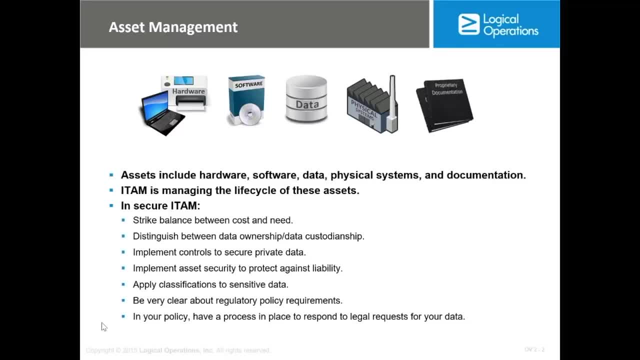 What you're going to tell them. I only kept them for one week, Or the logs. I used to override the logs every one week. This is not right. You're going to face Legal problem because of that. Okay, so we need to know about the legal, because it's different from one country to another and it's different that if you are working in a government, different than if you are working in a private sector. 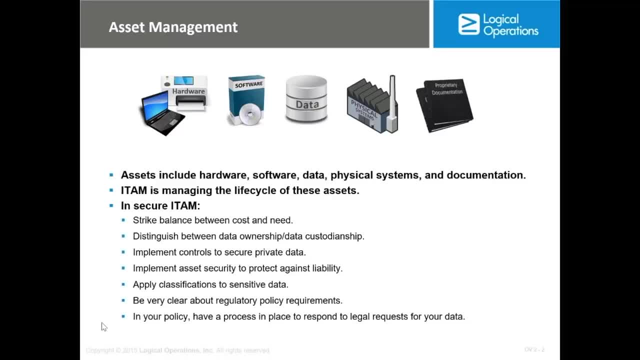 So one thing you need to do before starting creating those asset list and starting managing them is to contact the legal department. guys, Could you let me know How long should I keep the logs? How long should I keep the information? How long should I keep even the information? 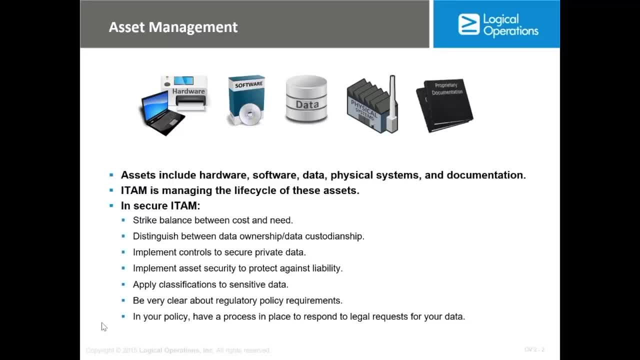 Of this organization, The document, the list, how long should I keep it? according to the law, And you should follow that. but saying that I didn't knew this is not an excuse. Usually this kind of jobs- information security officer or consulting or specialist- They are getting paid very well but they have a legal responsibility. 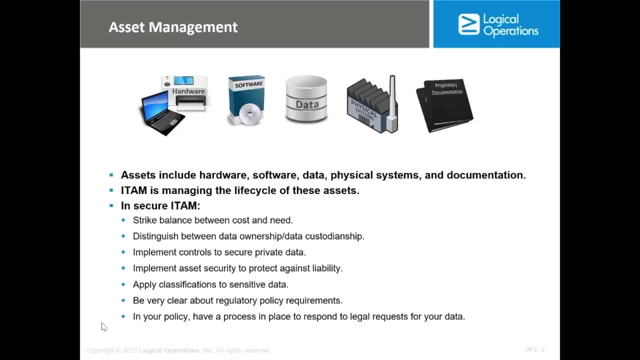 So we need to check with legal department first: What is the regulation, How long should I keep the assets, And so on. Now, after having this discussion about the information asset list or asset management, Let me show you how to create one, and I'm going to ask you for small practice: to create your own information assets and then 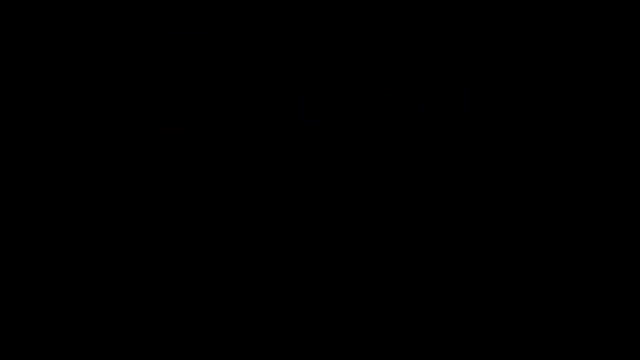 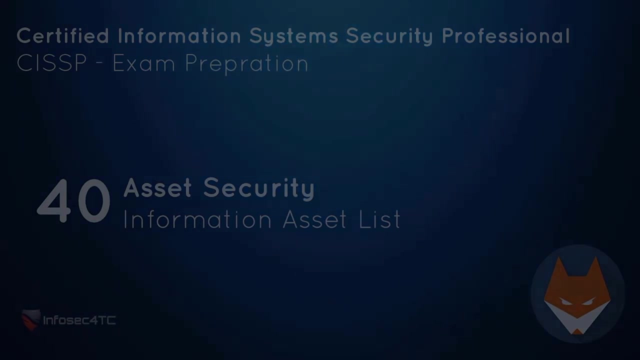 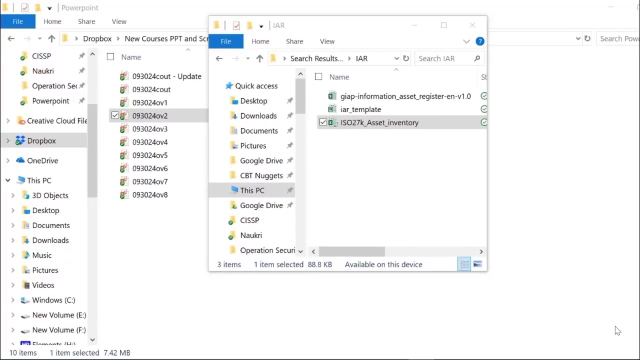 We're going to evaluate it together. Now Let me show you how to create an information asset list, also known information asset register. You may find different name related to the information assets. Some of them would be IAR or ITAM, whatever the name is, but the concept is having a list that include all your information assets and their classification and their owner and custodian. 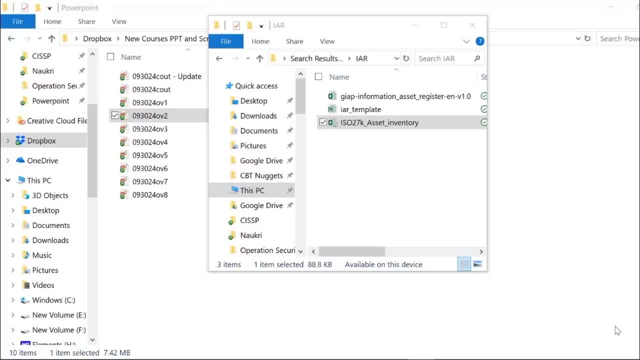 Don't forget those terminology: owner and custodian. So I have some of the templates which I'm going to share with you. But actually if you search online you can find beside. you can modify in the template. It's not like you have to use this specific template, but you can modify. 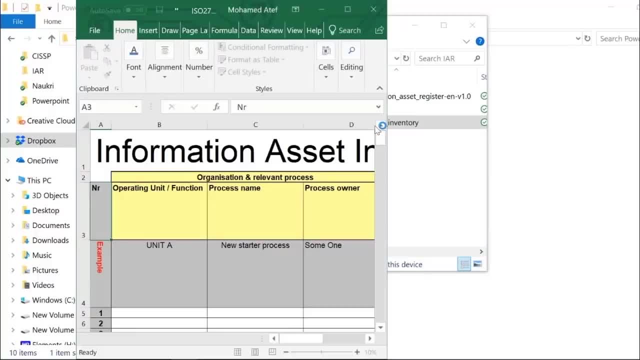 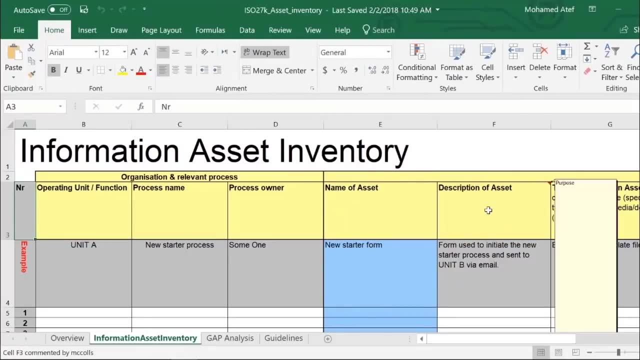 So let me open one of them and let's discuss what should be inside the asset list. Now, before showing you the different item in the asset list, Let me just tell you that who should like write down all the information that you have, Because this is not an easy task. you have here in this list to write all the software that you have, all the computer that has information, that all the document, digital document and hard copy document. 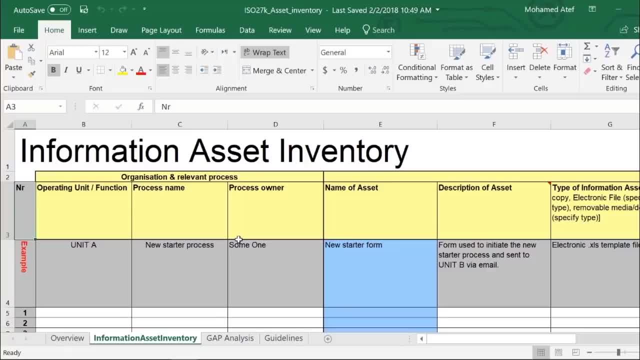 So you have some Excel sheets, You have some reports on PowerPoint. You have to write down all those information, their classification, where they are located, how important they are, and so on and so forth. Who's in charge of that? Is it You? definitely not, because you need to have a list of all the information asset. 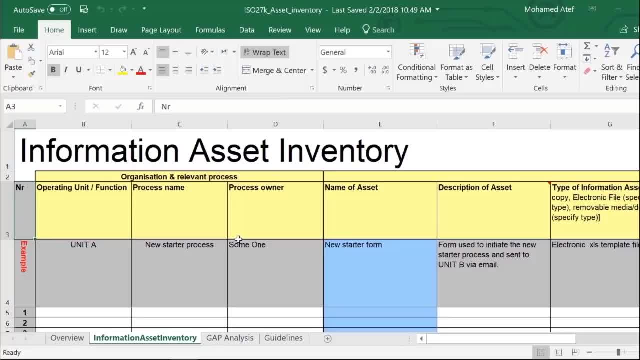 For all your organization, not just IT, HR. They have important information, finance. They have important information. So you have to give each of those department a list and you need to ask them to fill it. Your responsibility is to show them how it need to be filled, and this is very important for. 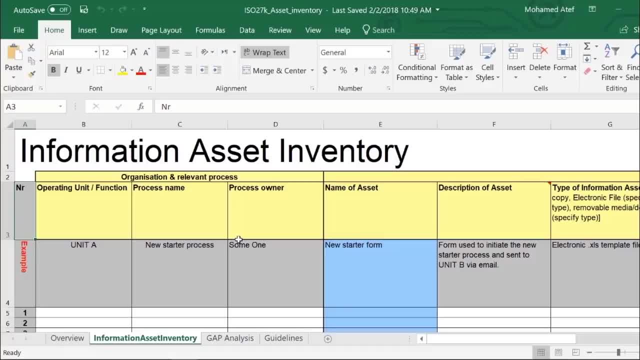 The exam, because you can find many questions inside the exam related to the information asset management, about classification, about labeling and so on, But also for a business, because Any audit that will come will first ask you about that and if you go to any interview, this is one of the points that you need to raise- show them that you know that you should start by having an information asset list. 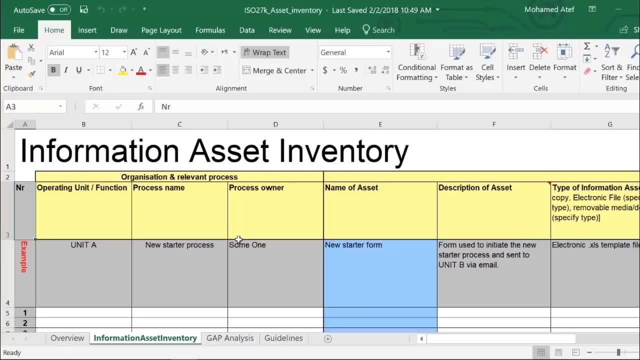 Because if I don't have a list Of all the valuable asset in my company, how can I know what to protect? right, So what should be in this asset? So, again, your responsibility is to make sure each department are filling that and are updating them as well. 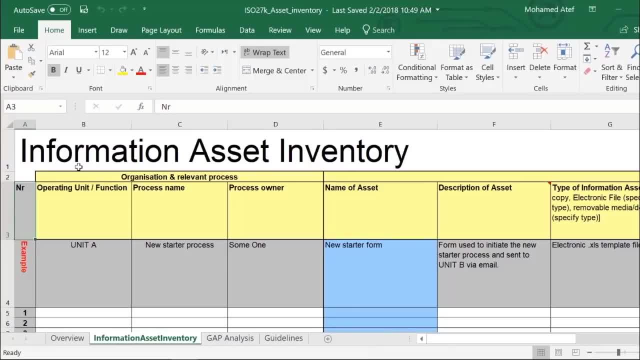 Because, as you know, that information keep changing, some new information is there, some other information will be written under retention, So it need to be updated frequently. So we're going to talk about Update later on, but let me show you first the list. 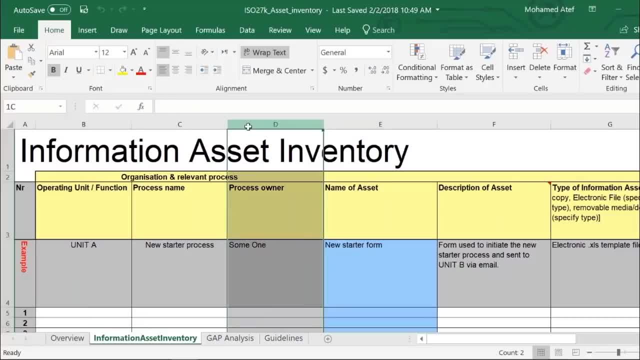 And, as I told you, you can change that. I will leave the process right now. We don't need to talk about the process. This will be covered in a different topic and we're going to start from here. name of this. What is the name of this? could be a document. 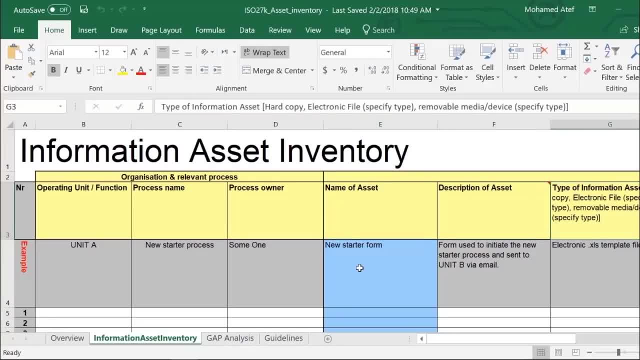 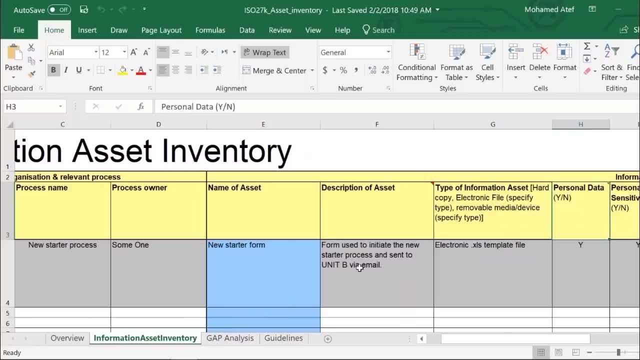 It could be a full digital document, It could be a hard copy document, It could be a software database, whatever the name then. So I'm going to assume that you're going to start from the name of this. You can even give a number, the description of this. 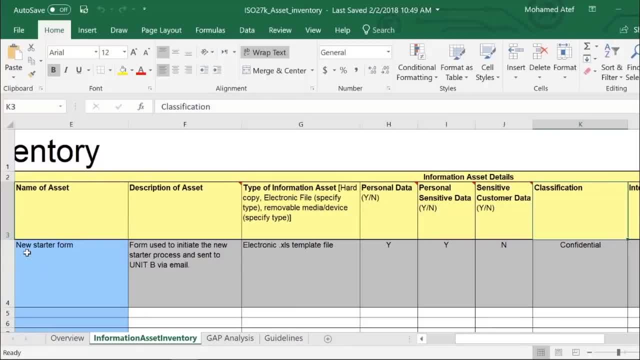 So, for instance, if the name of the asset it's like a document name, Now what is inside this document? Just a brief description. This is a list of all the company customer. What type of information? is it hard copy? Is it an electronic copy? 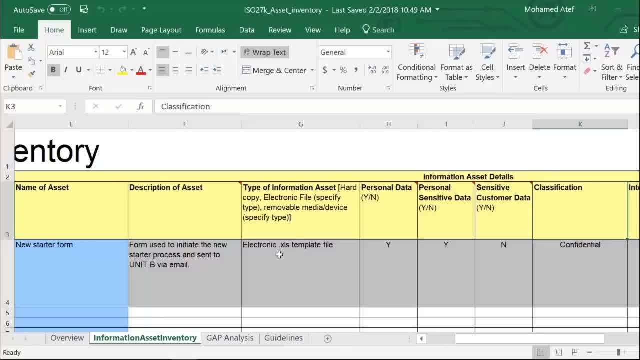 You can choose from here or you can create a drop list where you can specify what kind of assets is that? Is it a personal data, Yes or not? This is not very common. Some of the document will not have this. Is it personal, sensitive data? 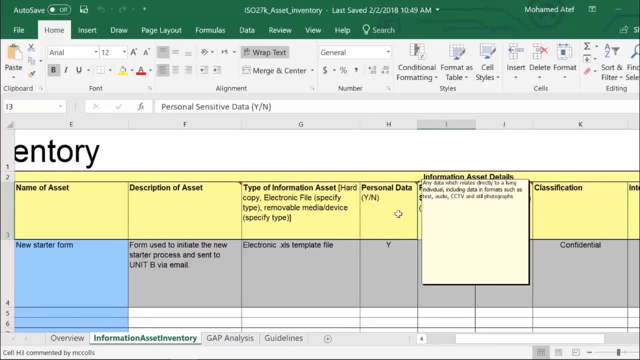 Also, this is in case you know, we are talking about privacy. So the information asset details sensitive? Yeah, customer data. So the data is it related to the business, related to the customer? but still, I saw a lot of document where they didn't categorize them. 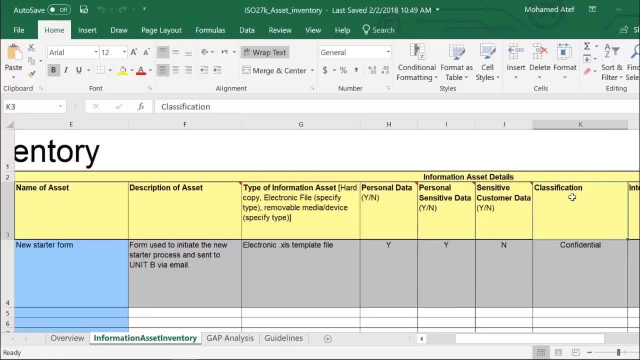 If it's a personal customer, but it's up to you. here We're going to talk About classification. This is very important. You need to classify the data according to a, according to the classification level that you have in your organization. So, in your organization. 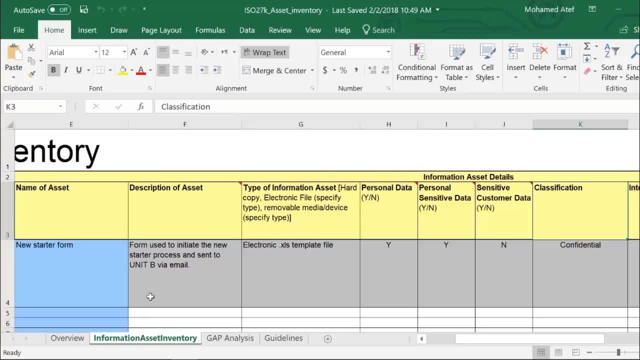 You should have a classification level. How much level of classification you have? Is it 4532?? Do you have secret and public? Do you have confidential secret? So you should not invent the classification level here, but you should have your own classification level. 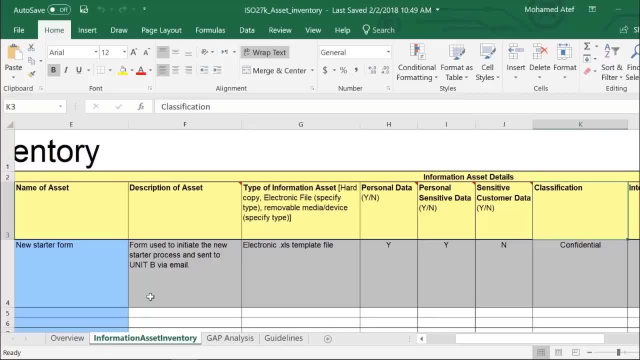 In your business and you should apply. This is a confidential, This is a prior internal document, This is a public document. So you need to write down- here is the type of the classification- Because according to that you will know which document or which assets, because actually, as I told you do not just talk about document. 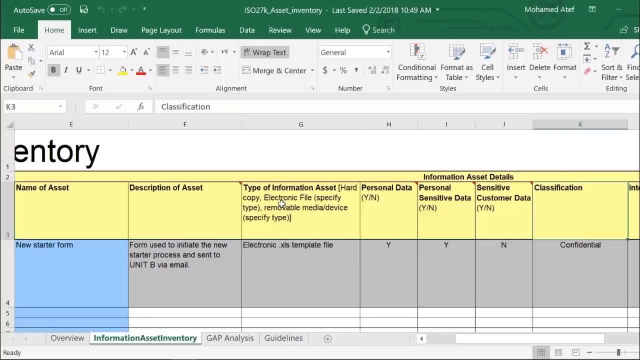 We talk about? we talk about document, electronic data, software databases, removable media like CD Or like a flash drive and so on. So according to the type of classification you're going to decide what kind of protection you're going to use. again, Who should assign that? 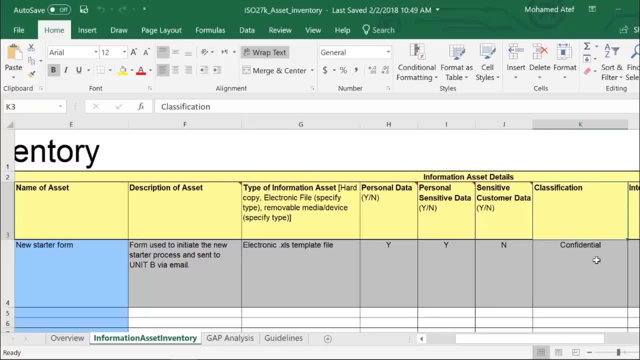 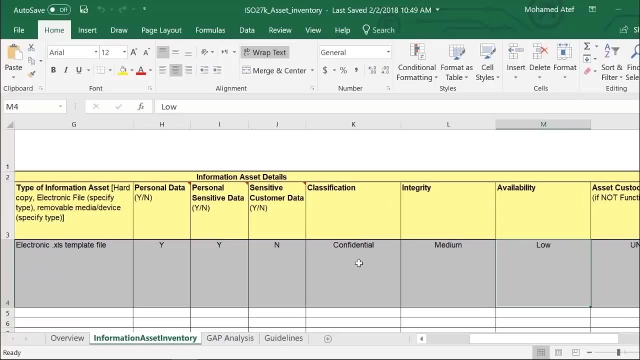 Is it? you know, is the one who's filling this information, which is data custodian. He's the one who specifies the classification here. It could be the data owner If the owner is a personal, but if the owner is like a business or department. 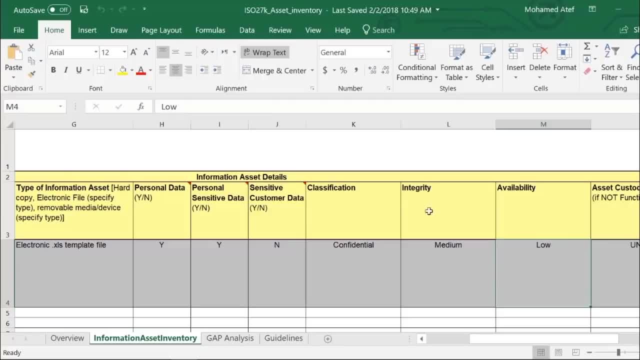 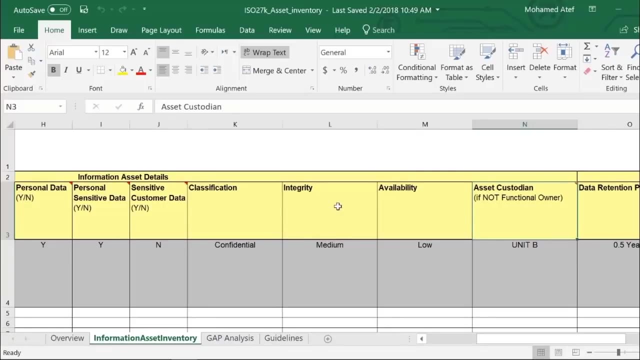 It could be the custodian or the one who's managing it now for the security CIA. It's recommended to write down the classification of this asset when it comes to integrity, availability and confidentiality. So you can say, for instance, for confidentiality is very sacred, but availability also. 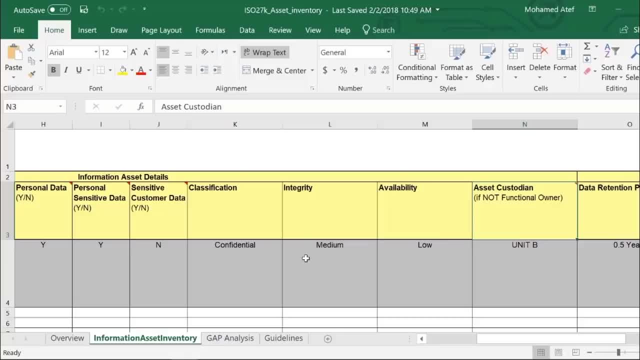 I'm sorry, is very high or integrity Medium, So you can choose based on it need to be classified and the importance of that. What about integrity? Are you going to allow people to modify in this document or you're going to put some control to? 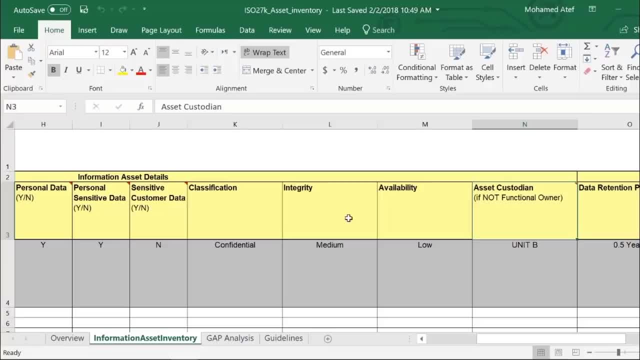 Prevent any modification to protect the integrity. is the document need to be available all the time? Not any asset need to be available. Is it the website? Is it the database? Maybe it need to be available 24: 7 because it has critical. 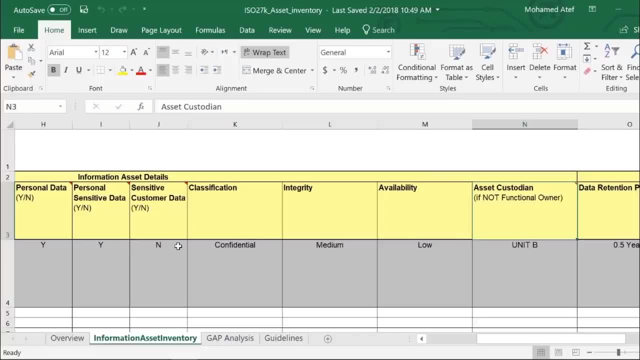 So you need to put like the classification or the level of each one of those: integrity, confidentiality and availability, Two important fields that you know. I saw some comment in some audit because of that That you should have that the asset owner and the asset custodian. 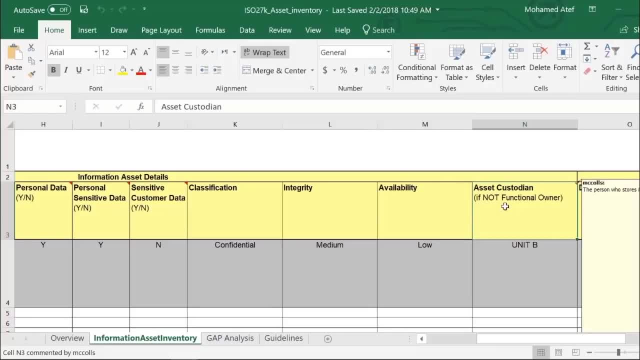 I keep saying that because I don't want you to lose this question size exam. Some people get confused between what is the difference between the owner and custodian? And, as I mentioned, owner is the one who are like Own this assets, like the company, and the custodian is one who's managing it, like the employee. 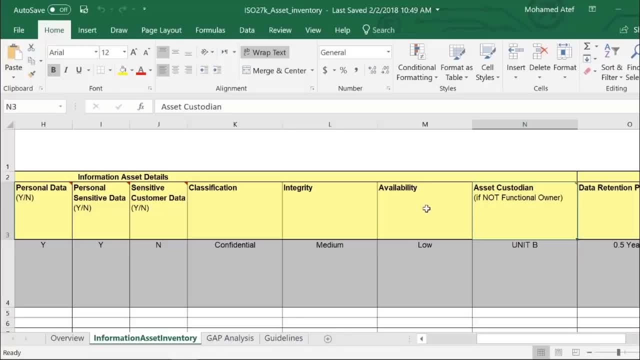 Okay, owner could be the manager or senior management, as I told you, but after all, think about it This way: who got the right to take this asset If he leaves the company? this is the owner and this, since those are assets to the company. 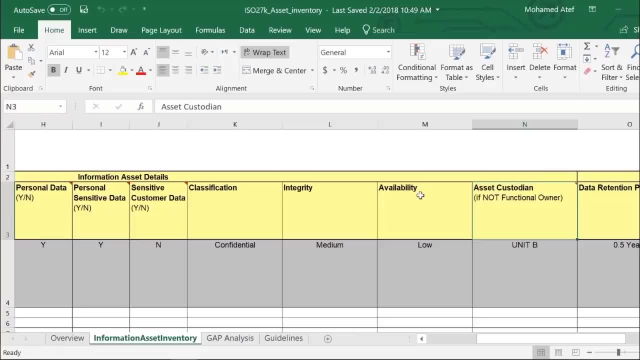 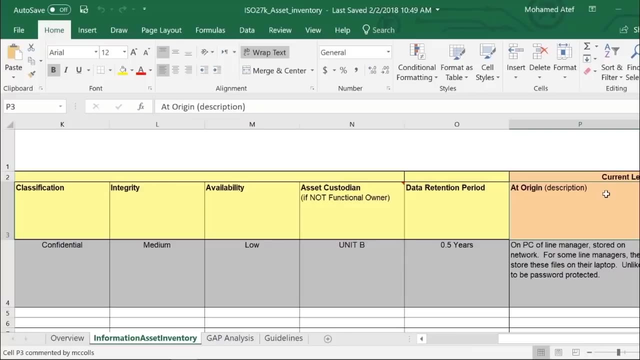 That's mean you don't have the right, even if you are working there, to take it while leaving the company. Here we have the data retention now. data retention because each assets has like a life cycle. after a while, You will not keep all the assets located somewhere for long time. 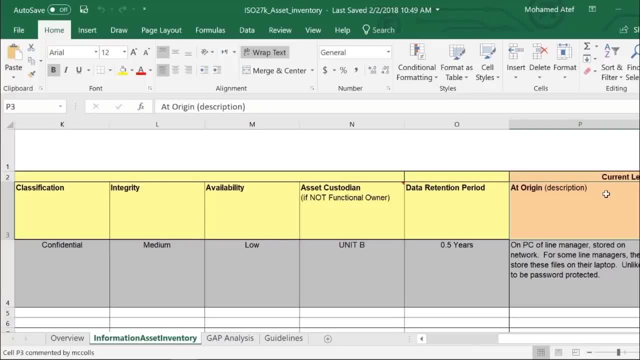 Think about the documents that you have, Even the Hard copy document. If you are working, like in a hospital, or where you have a lot of document and patient information and blood test and a lot of document, Are you going to keep them in the same place lifetime? 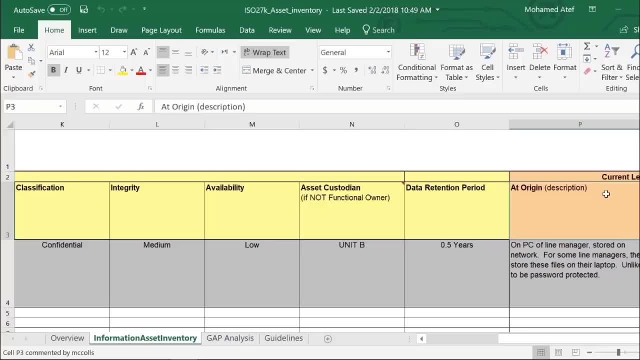 Definitely, from time to time, You need to take those assets and keep them in an archive or maybe in a warehouse or something like that. How long you need to do that is the data retention. Now, this could have some legal reference. according to The data that you need to, it need to be retained every how long? 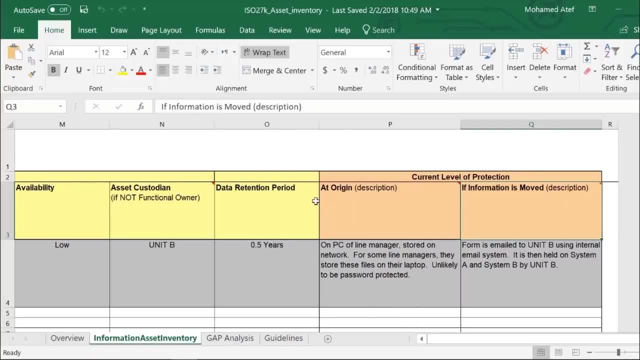 What else again? You can customize it according to your business. but I'm just showing you an example for a information asset register. And guys, Your work is an information security specialist or custodian. I'm sorry, information security officer are working in this field. 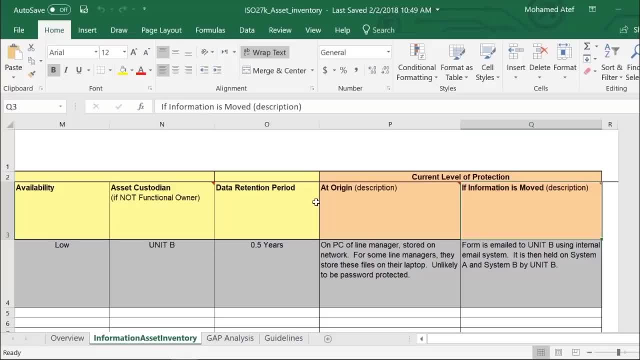 We have a lot of documentation. I mean you will be involved in documentation like policy procedures planning, disaster recovery planning, asset list. So whenever we are talking about a specific document or specific, take that very seriously, Because you may face a question about that inside your interview, not just in the exam. 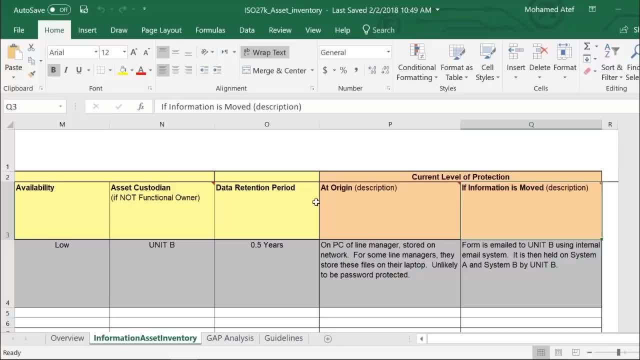 But when you go inside the interview they will ask you what documents you should have. What is the information asset document? Because those are the assets, Those are the things that when you have an audit, they will ask you about that And if you fail to prove an evidence or show them this document, that's mean you are not doing your job. 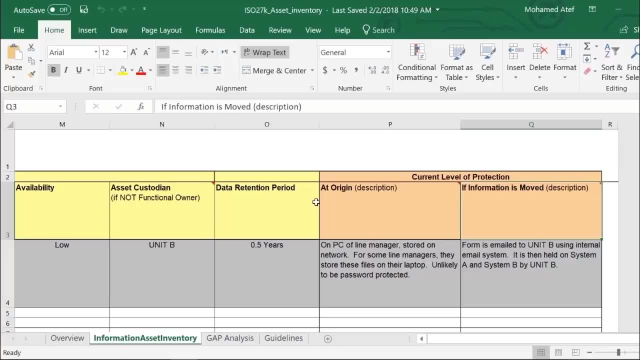 So it's quite important that when we are talking about talking about the document like a policy, like an ISR- I'm sorry, information asset register- IAR Or any other document, It's important to download them, check them, modify them, create template or create a demo. 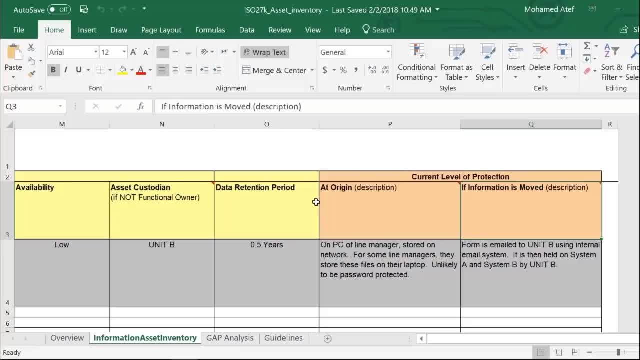 Get familiar with such document, analyze each field, Because once you Get hired you can have to take those document to different department and to explain to them What is this document is all about. So it's important to take especially the things that has practical or documentation quite serious. 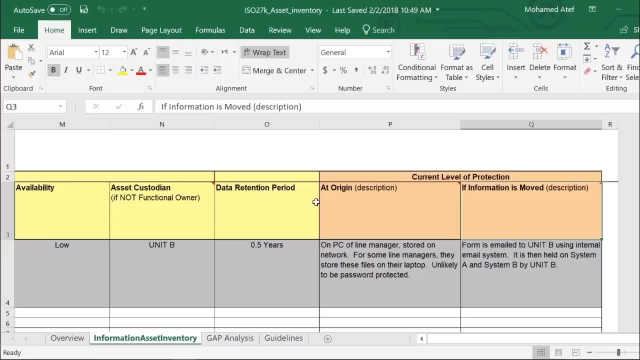 Because, besides the exam, it's important for the exam, It's also important for your job. One last point before moving to the next lecture, which is this document need to be updated frequently, And we're going to, When we are going to talk about document control, where we are writing all the information about this document. 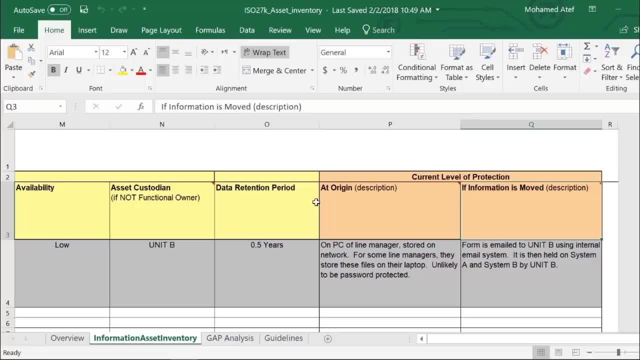 You need to show when was the last update. It's not a one-time process So it need to be updated frequently. Usually, most of the company are doing that once per year, So every year you need to update it and you need to write on the document controls that it has been updated on this specific date and time by this person. 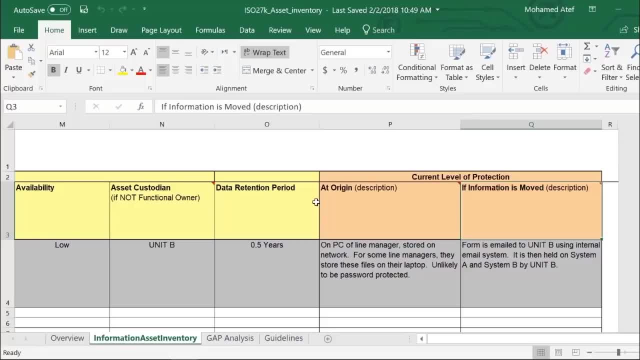 So this is quite important. Another point, which is Management support. Okay, as you can see, many of the document will need some input from other department and some of them will need A full input from the department. in a sense, like a document like that: 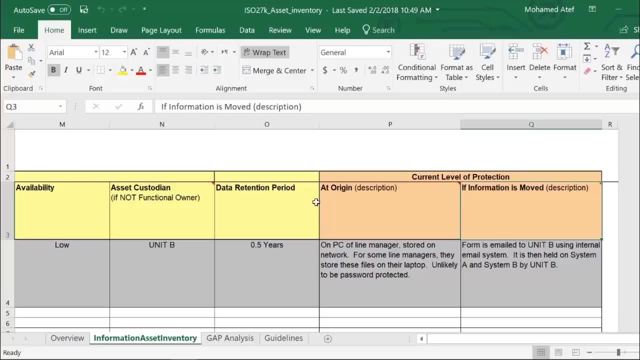 It would be fully done by the department, business department or functional department. So unless you have a management support, no one will like leave What they are doing And start filling such document and this is a critical document for any business. So you need to have a management support in a sense that if you are not getting any kind of cooperation from department you can report back to management. 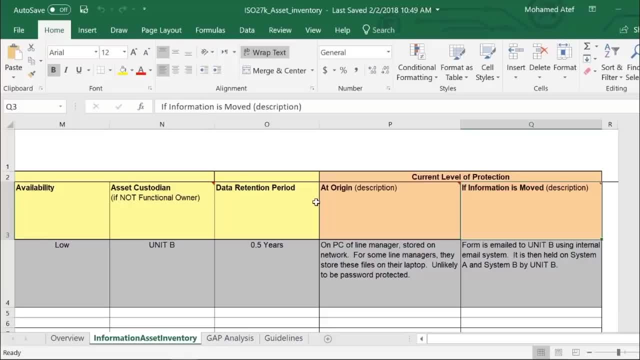 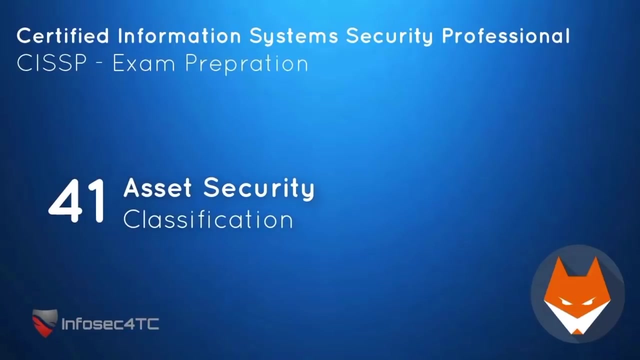 Because, after all, you are taking responsibility of the information security of this organization. So that's why, in the first domain, we explain the importance of the management support to be able to implement The right information security system implementation. In this lecture, we're going to talk about classification and labeling. 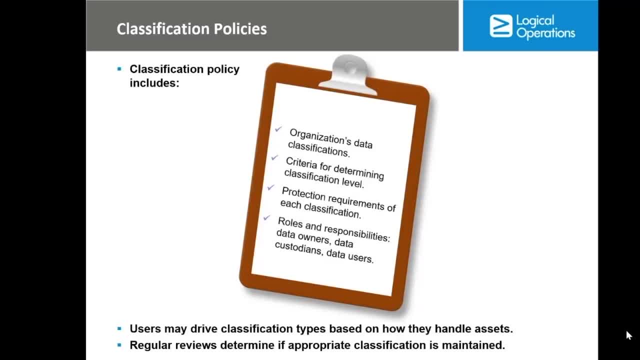 Classification. It's one of the main requirement when you identify your assets, but it shouldn't be done randomly. You should have a classification policy that identify First how many level of classification do you have? Some organization will have three. some organization will have four. 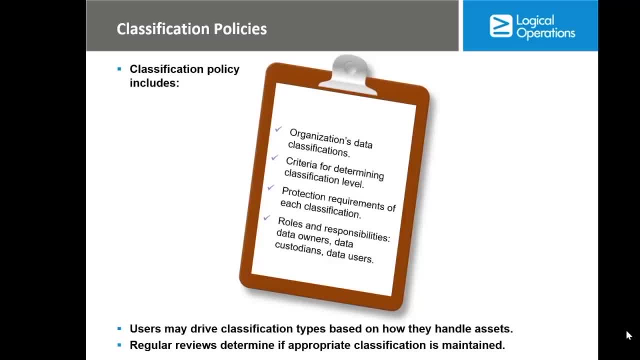 So you need to follow the policy from the level of classification you have. Second, the policy will include the criteria that you should use to classify the information. So, based on what, you will identify this asset as confidential Or confidential, and restricted or internal. 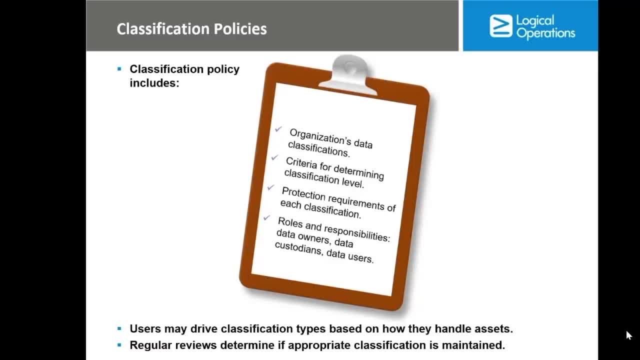 So it shouldn't be done randomly, It should be done according to a policy. Now the first question will be: who should classify the information? Should it be you, as an information security specialist, or the information security officer, Or it should be the information owner? 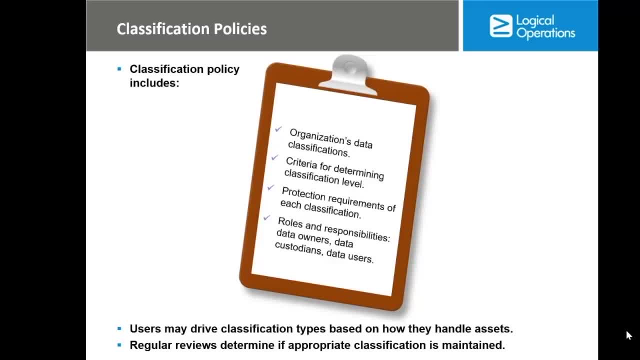 Most actually, it should be the information owner, Because he's the one who can identify the value of the information or the value of the asset And, according to that, he can say that this information is confidential or internal, or public, and so on. 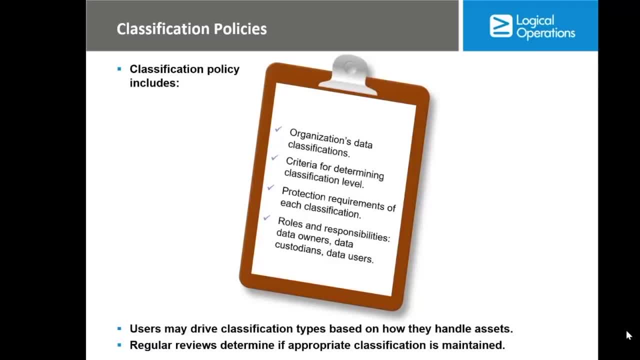 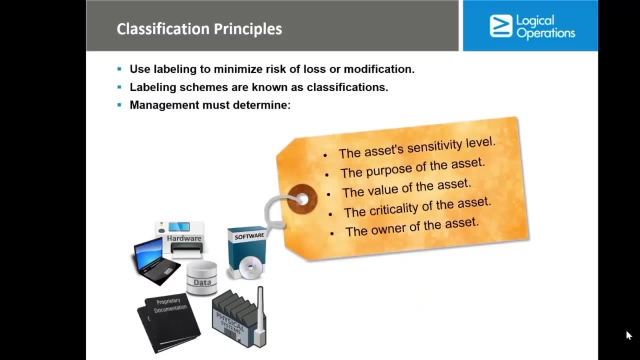 Classification should be written inside the information asset register, as we saw in the previous lecture, But also it should be written on the assets itself, Which we called labeling. So labeling, it's to identify the asset From the level of the classification, And I'm going to show you a couple of example. 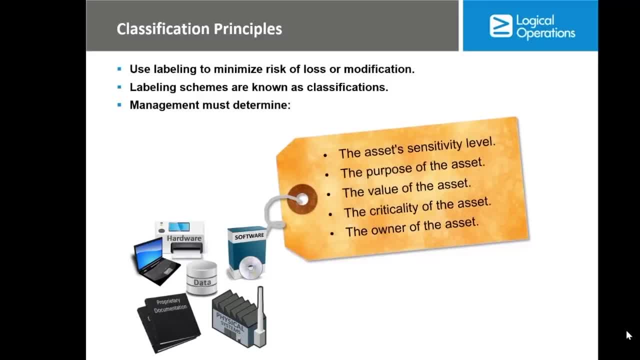 In the next lecture on how to do labeling on the assets, But why we are labeling the asset. First, to be obvious that this is a classified document or internal document, But actually, most important, that some of the software and some of the application that is used for preventing the leakage or the loss of data can only be working in case you have labeling on the assets itself. 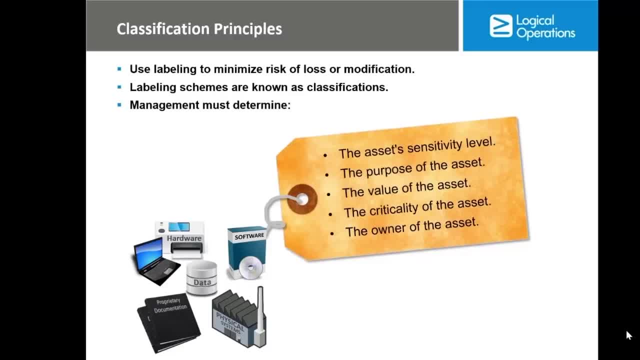 And we're going to see that in the next lecture, And I'm going to show you a couple of product who's doing that, which is the DLP. So some of the software, like DLP software, will not be working Unless you have your information. 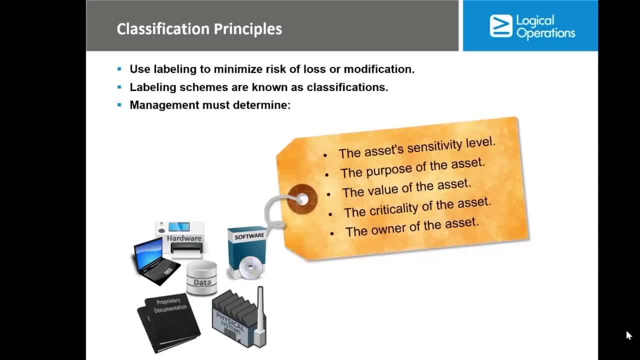 Classified. So labeling, which you should expect a question about it inside the exam- The classification in general. and labeling: You should expect many questions about them inside the exam. We need to understand the difference between classification and labeling. So in this lecture I'm going to go through the common classification levels. 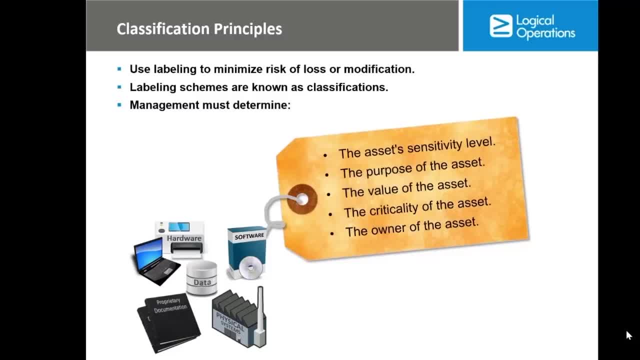 And in the second lecture or the upcoming lecture, I'm going to explain the labeling process with showing you few of the samples, And then we're going to talk why we are doing labeling and how it can be effective or how it can be useful when we are using some software for leakage prevention. 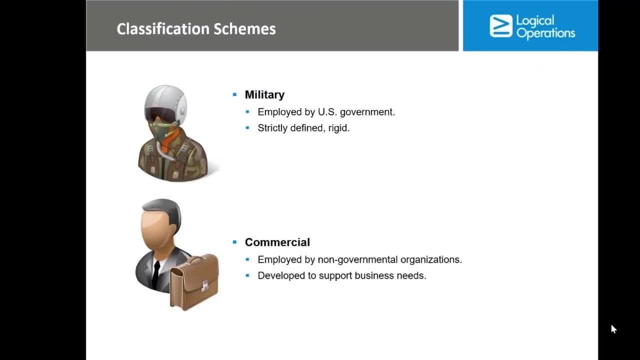 So, in general, there is two different kind of classification. There is a military or government classification and there is a commercial classification, Military, which is applicable to military or US government or any government in general, And it's More restricted, While commercial has different level of classification, like, as you can see right now, things related to copyright, things related 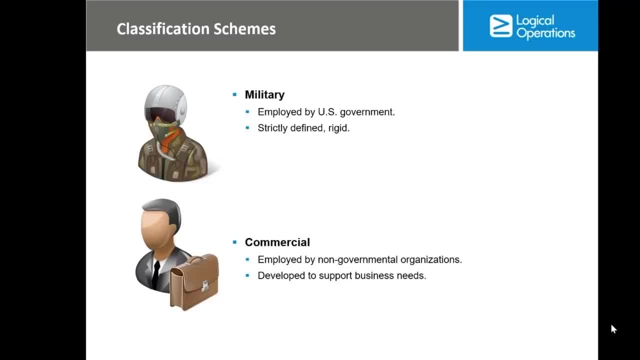 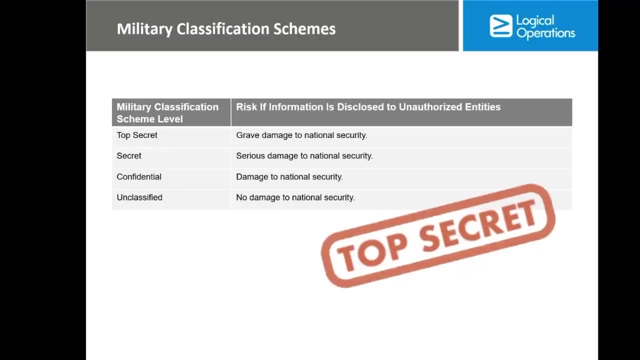 So in to the know-how for a product or something like that. So usually you have two different kind of classification. Let's go through them as an general idea about the classification. So the military In general could be more or less. We have different four level of classification. 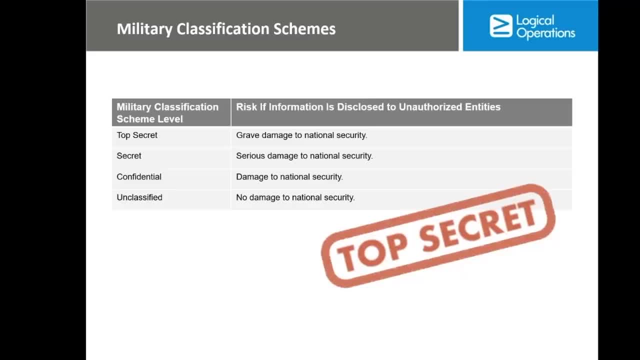 We have the top secret And to define it's the information that if it gets disclosed, a great or grave damage to national security. We have the secret, Which is like serious damage, and we have confidential, which is damage to the national security, and we have the unclassified, which no damage will happen in case of disclosure. 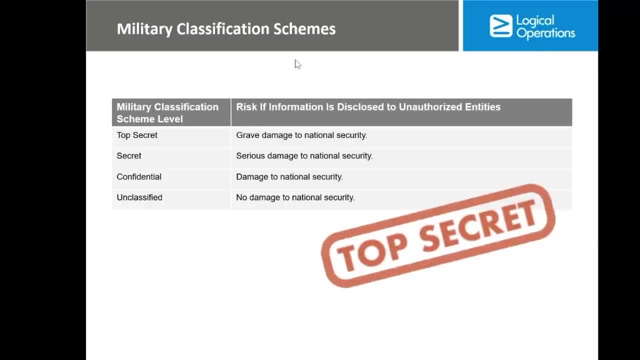 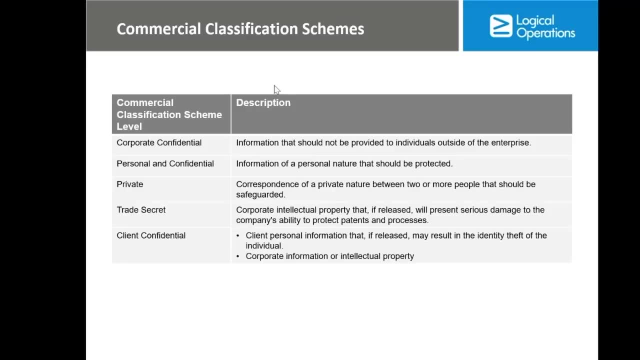 This is the most common military classification. As I mentioned, it could be more or less, while commercial classification is kind of different. So we have the corporate confidential, which is the information that need to be protected, provided to individual outside the enterprise. We have the personal and confidential, like the employee information or the customer information. 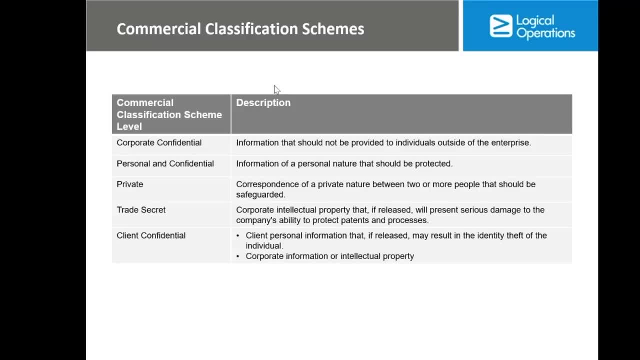 We have the private, We have the trade secret. You know things like the know-how of specific product, how it's done- and we have the client confidential. So those are the common type of classification in the commercial section. But again, How many level you can use it depends on your business or it depends on your organization. 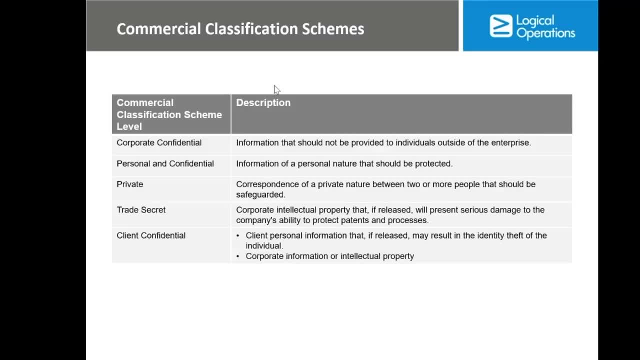 Besides, you should also check if there is any. Especially If you are working in government, you need to check if there is any kind of law or regulation regarding classification. So in some country they are enforcing all government to follow a specific classification schemes. So before you start identifying the level of classification, 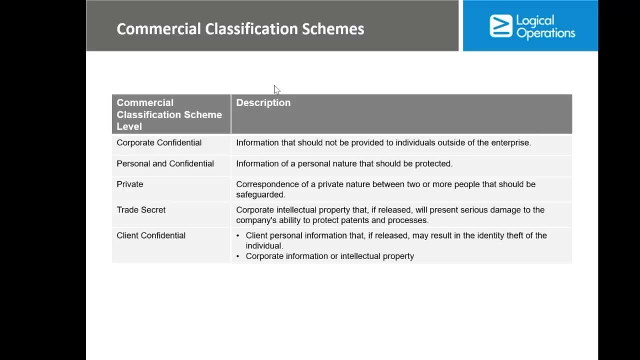 And start explaining it to the functional manager so they can explain it to their employee. you need first to check if there is any Requirement, No requirement when it comes to the classification- and here I'm talking about government specially- Let me remind you that you are not the one who's doing the classification. 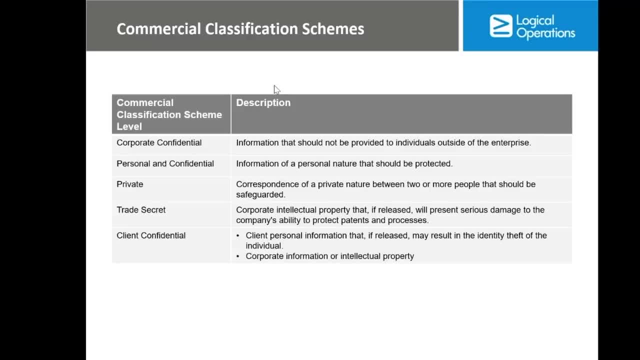 You are just enforcing the policy to be implemented, the classification policy to be to be implemented, and you are explaining to different department What is the criteria that based on They're going to do the classification And according to their output, Regarding asset classification. 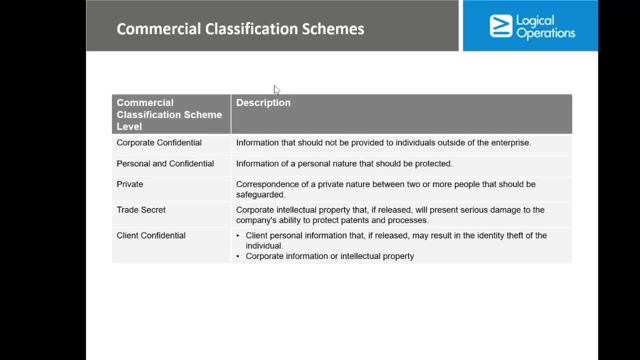 You will be implementing the proper control to protect those assets according to their level of sensitivity, and the classification as well. Now, as we explain the importance of classification, And classification is not an option, It's a must in any Information. if you are implementing an isms, you should classify your information. 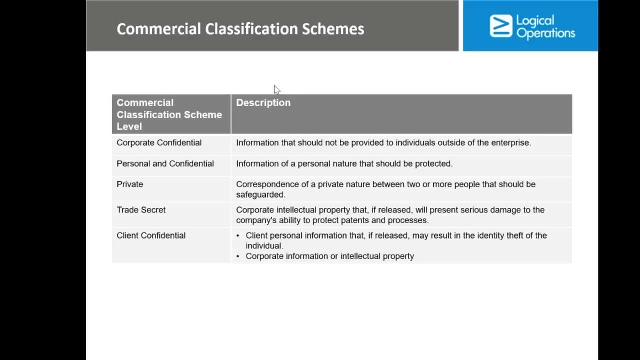 They will not accept to approve your as isms unless you classify all your assets. Next step will be labeling, and labeling is to write down the level of classification on your document. So it could be a stamp on your document or it could be if you are using digital document, like Microsoft Word or Excel or PowerPoint- any other document. 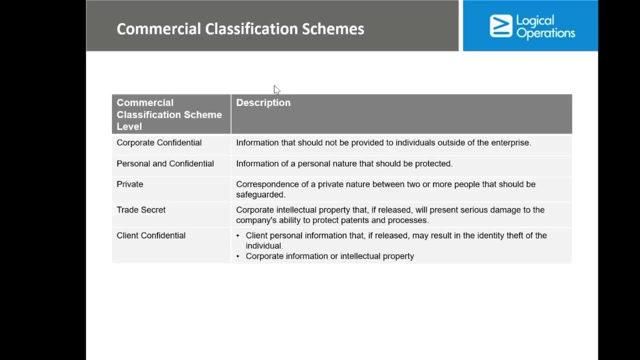 You should have write on the document, on the header or footer, the type of classification And on the document control. Why are we doing that? You can see on the next lecture some samples, and then I'm going to tell you why. we are labeling the assets with their classification. 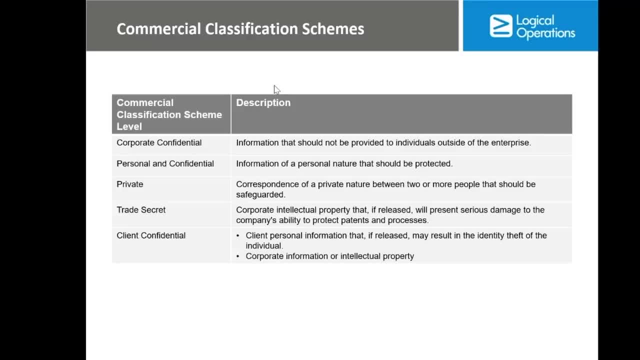 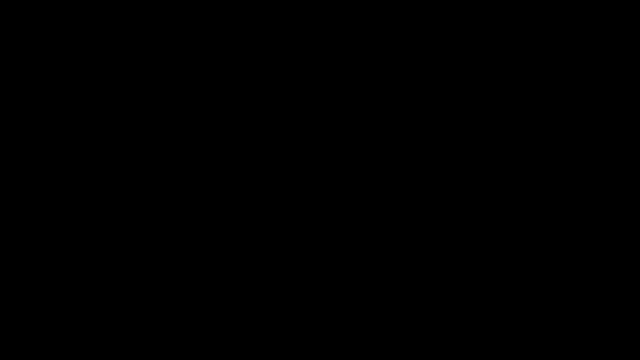 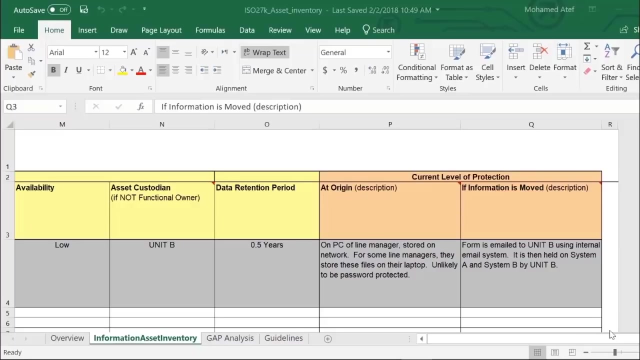 In previous lecture We spoke about classification and different classification schema. in this lecture We're going to talk about the labeling, which is I adding the classification to any assets and, to give you a small example, We're going to take the information asset list, which is one of the security document. 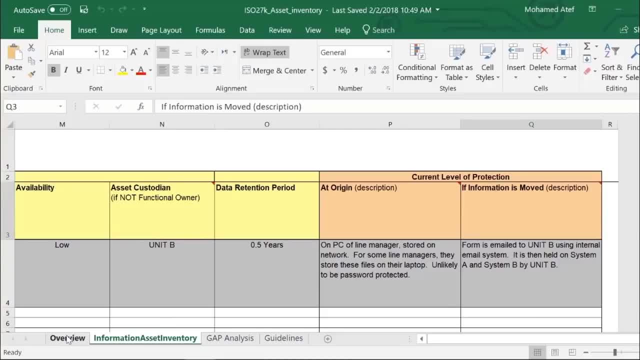 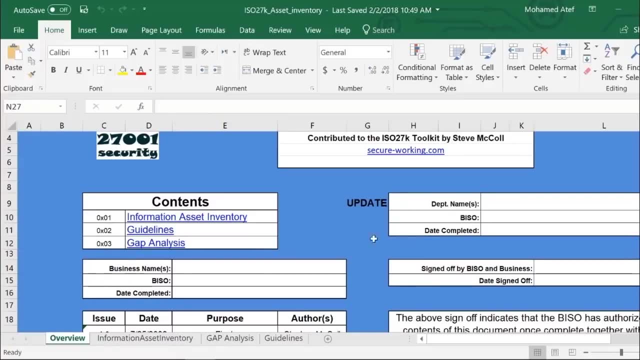 If you go to the first sheet here you will find all the document control information: This document has been introduced or has been written, by whom, and when it has been Updated. and don't forget that most of the information security document need to be updated at least once per year. 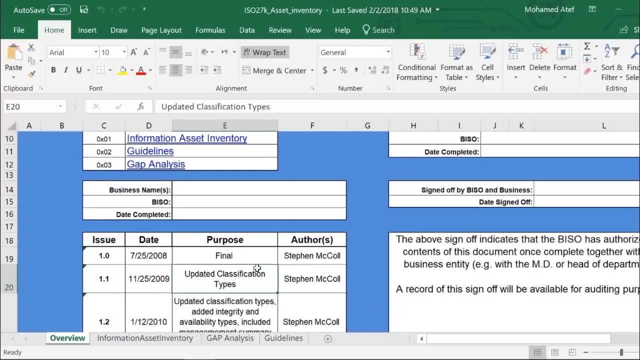 And, as you can see, here there is a classification. You need to add here the classification type. What do you consider this document? Is it the top secret secret confidential? Again, it should follow the classification policies that you are following in your organization. 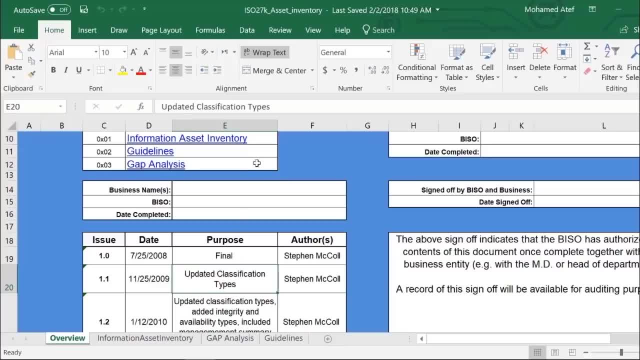 Now here is a point: Why are we adding labeling? Some people will add that in the like header or footer writing down: If it's hard documents they will put that in like a stamp. But let's talk about the soft copy document. 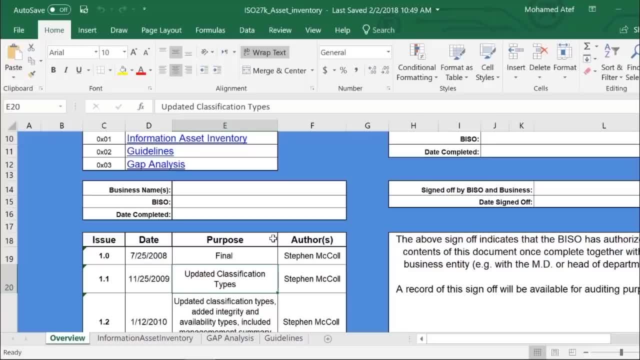 Why it's important to do that? for many reasons. First, it's one of the requirements, one of the compliance requirements. But second, which is quite important, is that some of the software That you may use to prevent leakage will depend on that. 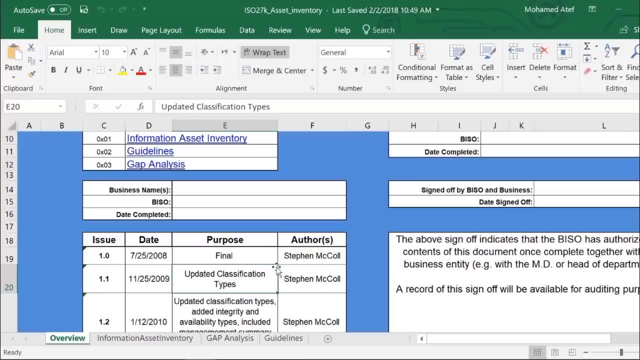 And let me clarify. We have a very common software that we are using right now. It's called DLP or data loss prevention. Some people are calling it data leakage prevent, prevention. The DLP is a software That monitor any information, like sending email or copying a document from from your computer to an external hard drive or send an attachment. 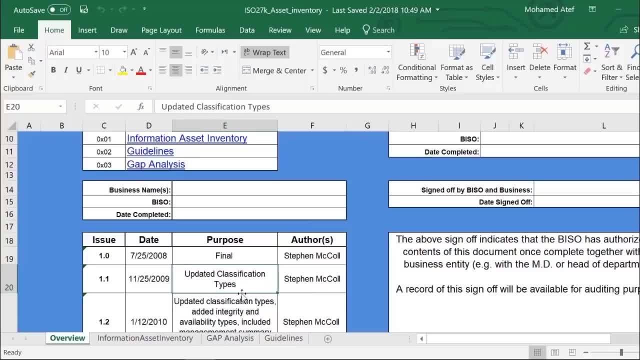 And, according to the classification level that the document has and according to the policies that you should implement, It can prevent that. Last few years, we heard a lot, especially from military. We heard a lot, a lot of leakage happen in different organizations. 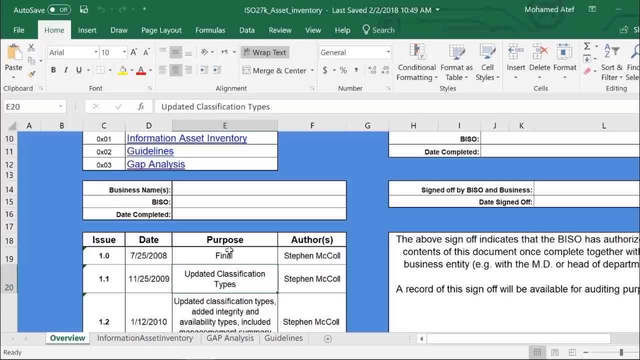 That's why a lot of company right now are considering using DLP and there is a lot of product- and I'm going to show you a couple of product in the upcoming lecture. But those product, when you install them on your network, What happened is you can assign a policy that please do not allow, for instance, the confidential document or this top secret document to be exchanged. 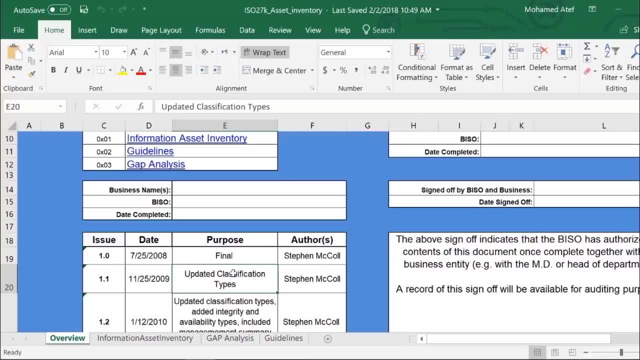 So, according to that, if you try to send an email, if you have a DLP installed on your company and you try to send an email and this email has a top secret label on it, the policy will apply and then you'll not be able to send it. 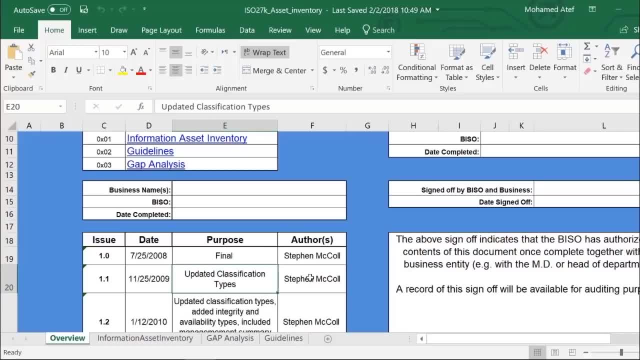 So you try to send it by email, It will tell you that you are not allowed to send it. You try to send it by Or copying using a USB drive or hard drive, because there is like a top secret word on it: It will not be copied, and so on. 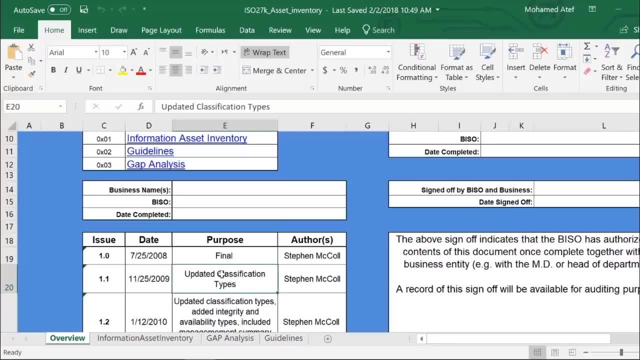 But to be able to use a DLP you need to have a labeling system, Because what if the user didn't write down anything here or he removed what was here? So you need to have another software that do this labeling part that whenever you create a document he will not save. 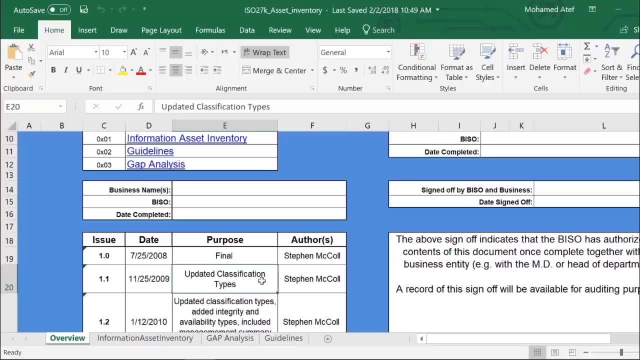 It unless It has a label on it. So it's like two different software that you need to be able to prevent any leakage of data or to be able to prevent any lost of that. first We need to have a classification, Then we need some software or even some policies that each document need to be classified or need to have a label, and then you can use a DLP that will prevent the leakage of that. 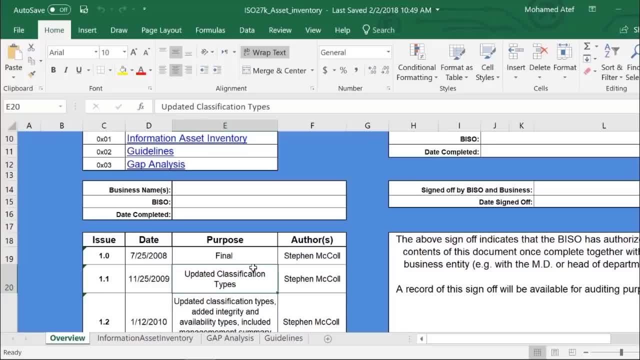 So it's a very important approach that you should consider, especially if you are working in a government or a finance entity or any place where they have very critical information that you need to prevent against leakage of data or lost of data. So let me show you a couple of product and how exactly they are working. 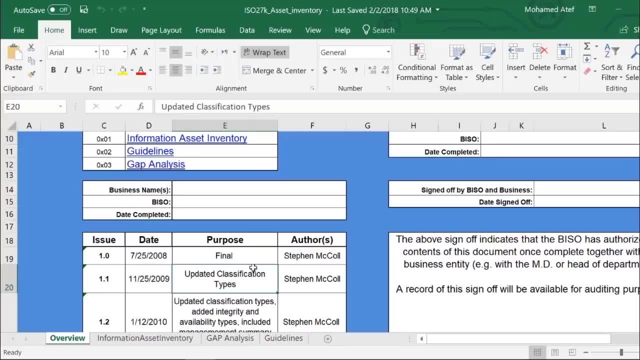 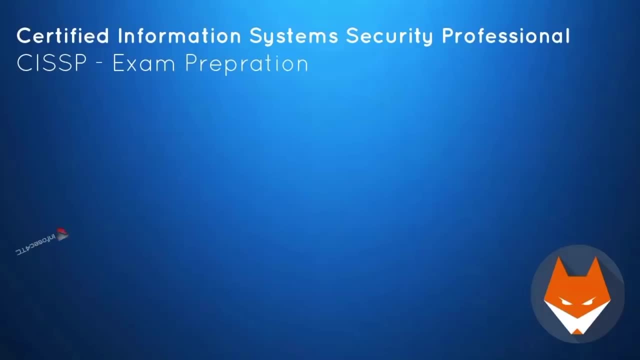 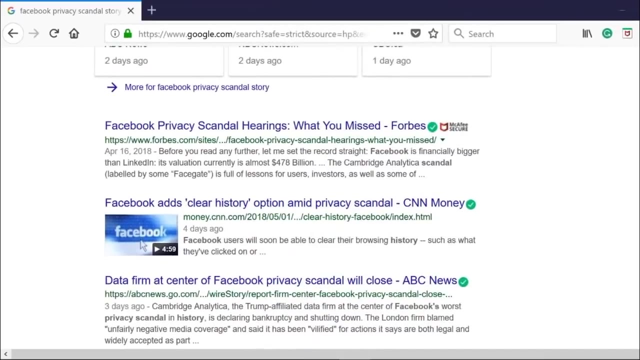 And then you can relate what we are seeing To the, The DLP And the importance of labeling for preventing the leakage. So let's see a couple of product as a proof of concept. In this lecture we're going to talk about privacy. 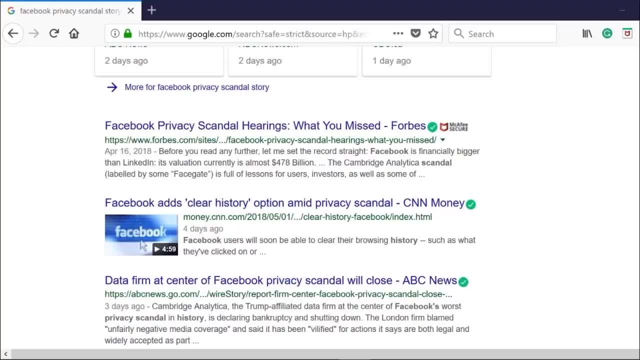 If your business are maintaining or are collecting customer information- For instance, you are a hospital- You need to keep your patient Information, such as their name, their social security numbers or health history and so on. Or you are keeping customer credit card information or you are keeping any kind of personal information for customer. 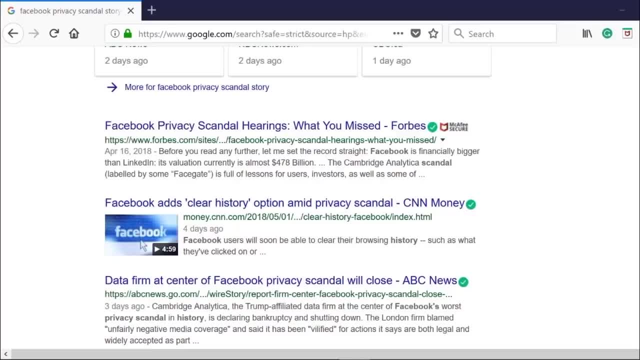 You need to follow a lot of flow and regulations, But first you need to be aware of them. So there is a lot of compliance- or actually low- That will enforce you as a business to maintain the privacy of this information, And a very good example to explain what could go wrong because of that will be Facebook. 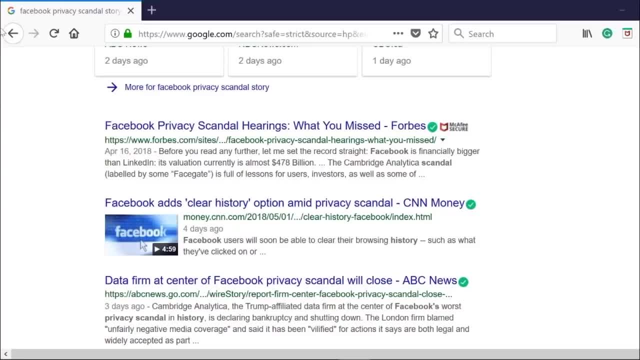 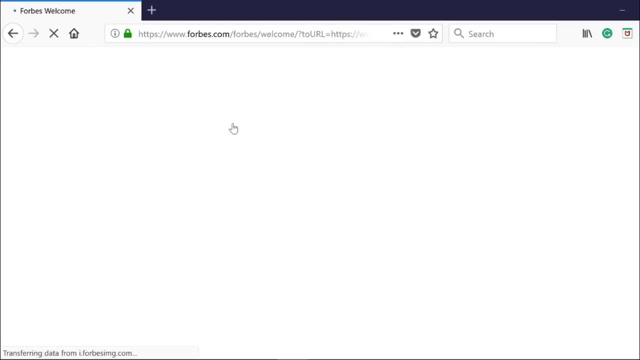 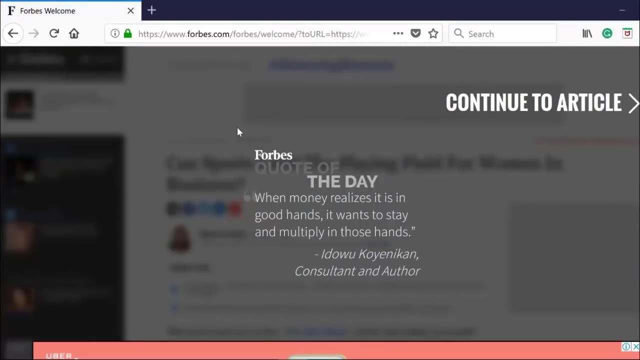 Facebook. the last few weeks There was a big incident in Facebook: The privacy scandal. Facebook are collecting information, And they are not just collecting personal information, such as name and email And an information like that, But also they are collecting behavior information. 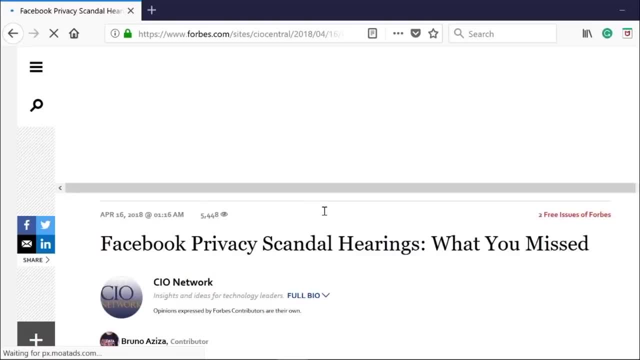 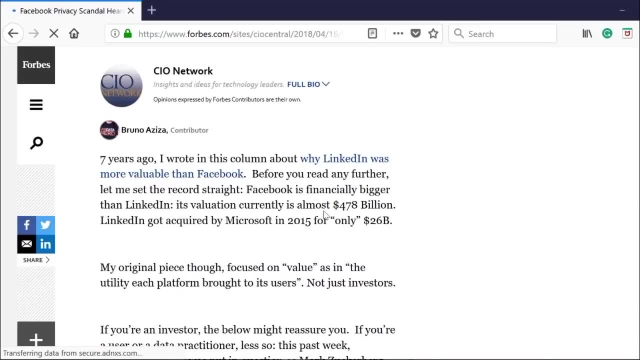 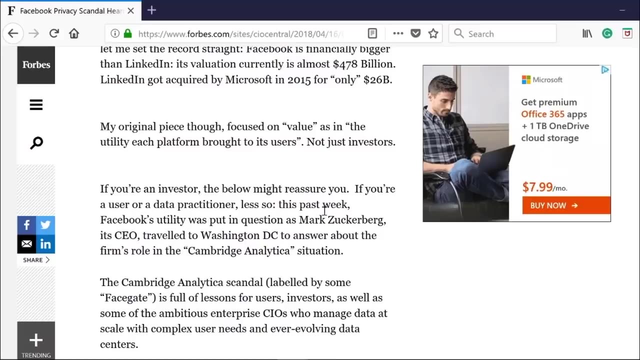 They are checking, what kind of ads we are clicking on, What kind of groups we are joining. They try to get or to analyze Your interest and according to that They start- or this is what you know- the legal issues that raised the last few months. 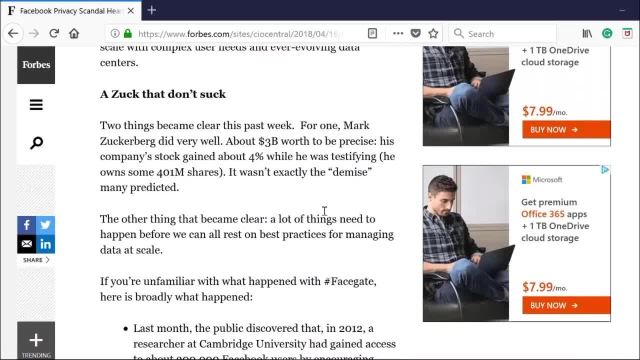 Related to Facebook that they are taking such information and sells them to vendor. So people who are interested in traveling They may send sell that to traveling agency because they know that from your behavior You are, you have interest in such activity. So this is considered private information. 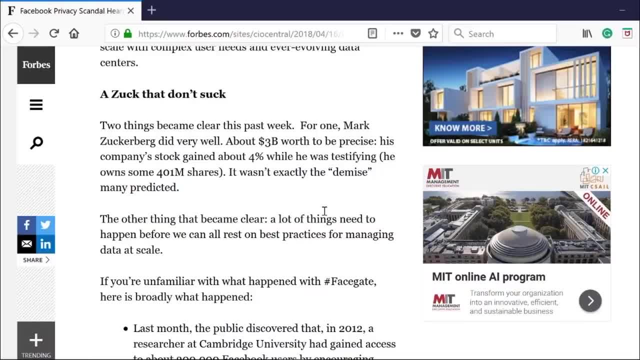 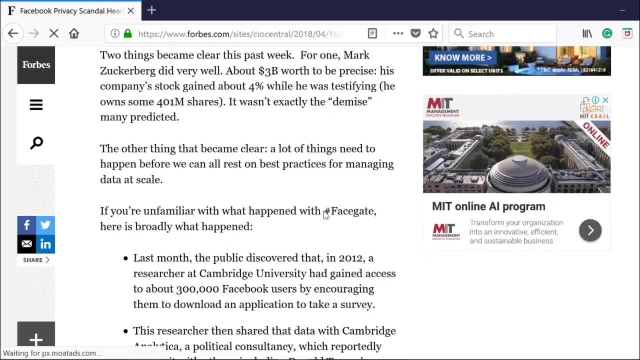 They are collecting your private information and, without taking permission, They are selling that to other, also Third party or other kind of vendors. This is a very good example about privacy breach And, as you can see, you know the problem has been raised. 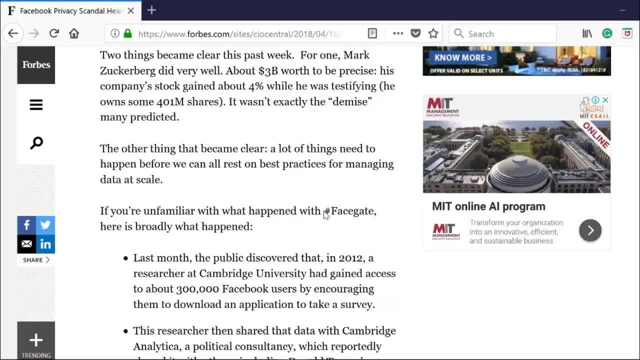 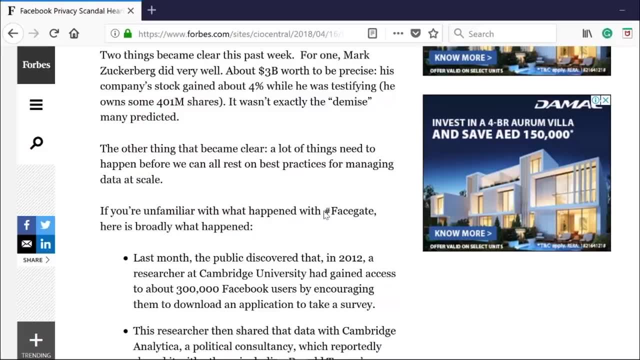 And it went to the Congress and there is a lot of legal consequences to that, Because Facebook didn't take permission from you to sell your information. Even if the service was free, it's not giving the right to sell the information to any other entity. 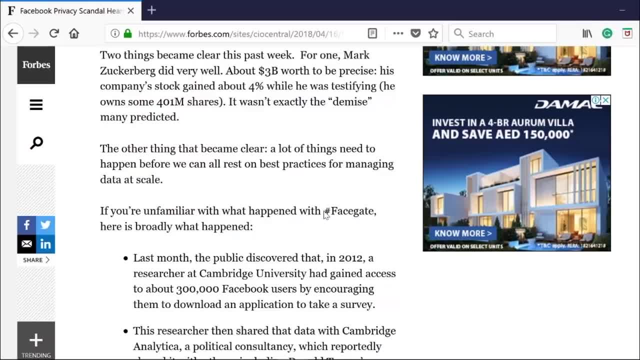 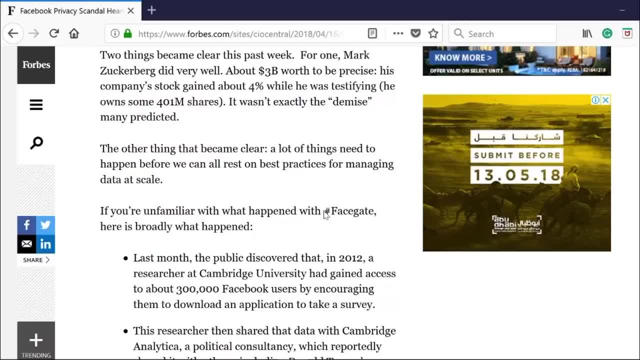 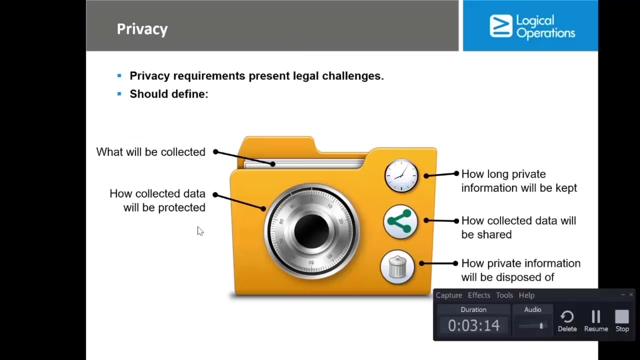 So this is an excellent Example about the privacy that, if you are maintaining private information, You should follow the PII, or the personally identifiable Information PII. So What should you do when it comes to maintaining the privacy of the information, As we agreed? privacy which is collecting personal information, such as. 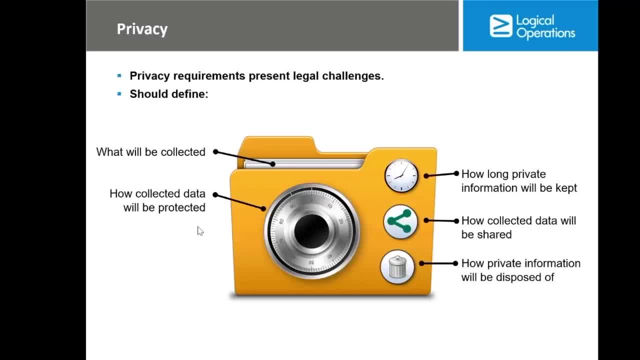 Social security contact information, names, email and so on. This is a legal channel challenge because if you misuse that in any way, there will be a lot of legal consequences, And I already gave you an example is Facebook. So you need to first identify what will be collected. 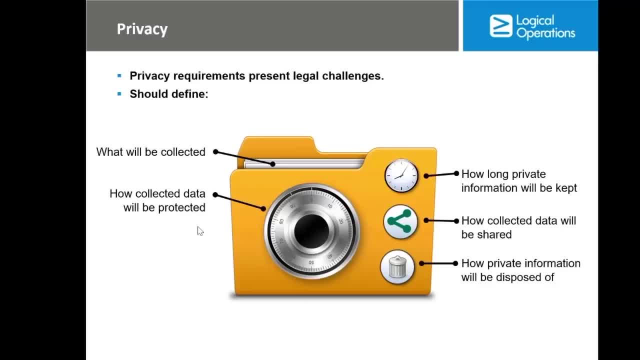 I should not collect information That doesn't have need for my business, How it will be collected, how it will be collected and protected, Because, again, if it any breach happen, you will take responsibility And those legal requirements are very hard. 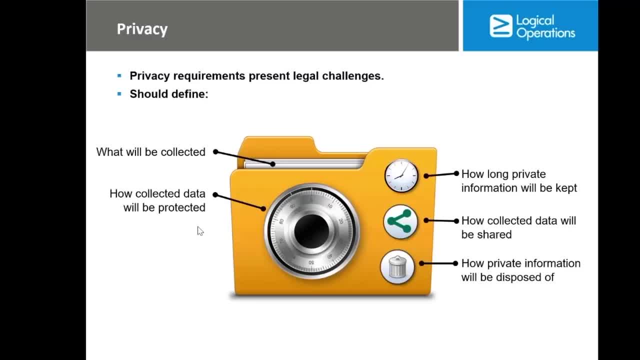 How long private information will be kept? Are those information private for for for lifetime or it has, like, a retention time? How collected information will be shared? Are you going to share them with other entity? Did you take permission for that? What about the other entity? 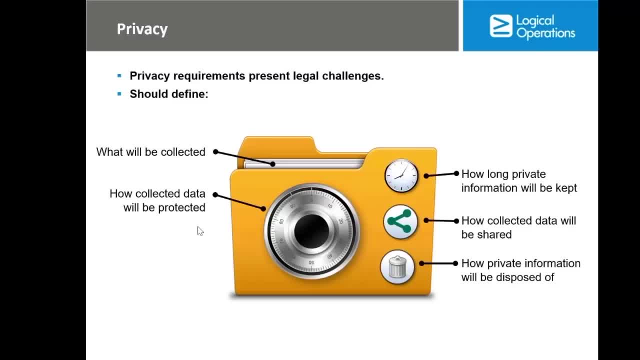 May. do you have any guarantees that they will not be shared with other entity? We keep hearing about credit card information gets stolen. You keep hearing about personal information with social security number And I believe few years back it happened to Sony, where a lot of personal information has been stolen and sold. 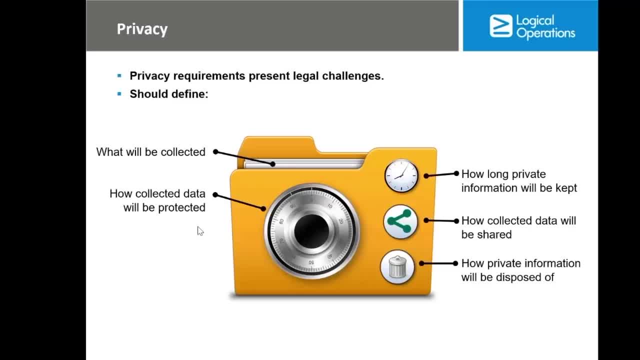 In the dark web How private information will be disposed. As we spoke at the beginning of this section that the information has a life cycle, So after a while you're going to need to dispose that. you will not keep them forever right. So what is the proper way for disposing this information? 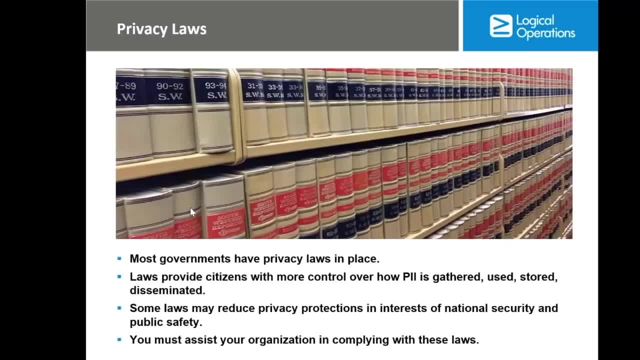 All those factors need to be considered when it comes to maintaining the private information. Don't forget that there is a lot of privacy law. It's different From one country to another another, But in US and Europe they are very strict and in US, you know, like HEPA law. 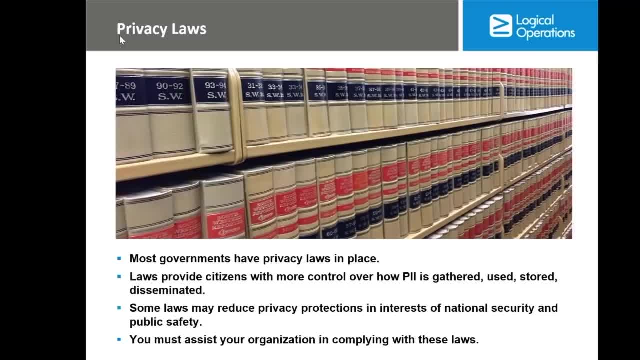 For instance, if you lost- intentionally or unintentionally, like patient information. according to HEPA law, this is a big issue. You're going to pay a fine with millions and maybe some jail time for senior management. It's, it's, it's very serious topic. 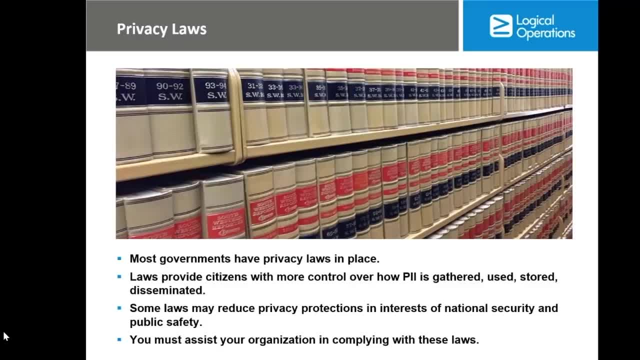 So what you need to do- as I keep saying that- is that if you join a business That depend on or keep customer information, You need to sit with the legal department and you need to ask them what legal or what laws they are following And, according to that, because you're going to need to put more control on those private information. 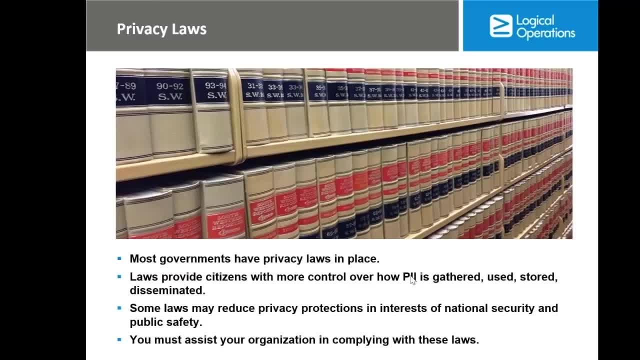 And don't forget the terminology with the PII, which is stand for personally identifiable information. What is the personally identifiable information could be name, social security number, credit card Number, address, phone number. All those are considered private information. So it's quite important to start by knowing the privacy laws that you are following, because they are different. 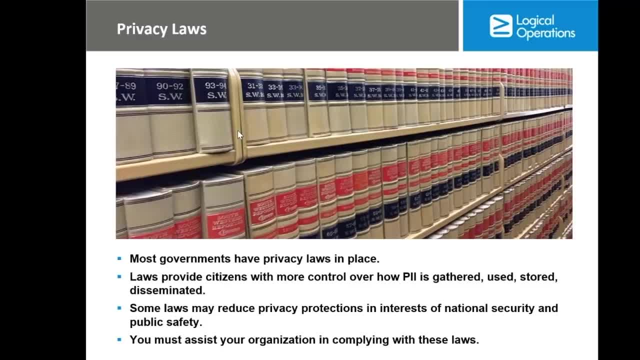 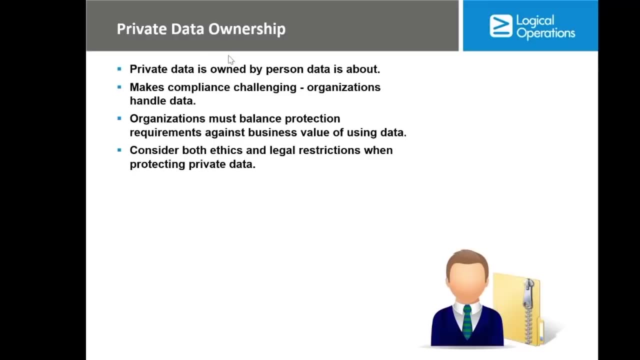 If you are, us is different than UK or Europe, and which law? also according to the business. So it's important to start by knowing what is required according to law. This is an important point because before we spoke about the difference between the owner of the data and the custodian of the data. 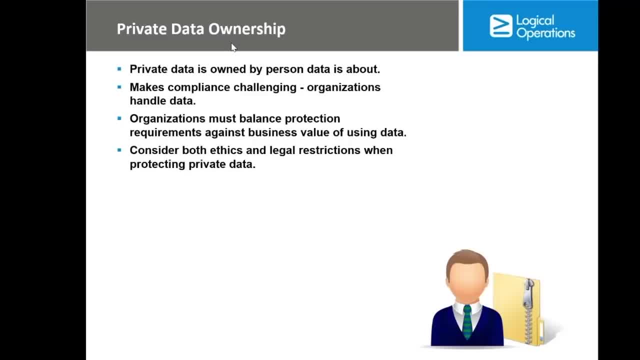 And, if you remember, we mentioned that the owner usually is a business. It's not a person, unless is the business owner, or it could be. the senior management is the owner of the data. This is in general, and custodian is one who's managing it. in private information or in PII, the owner is a person. 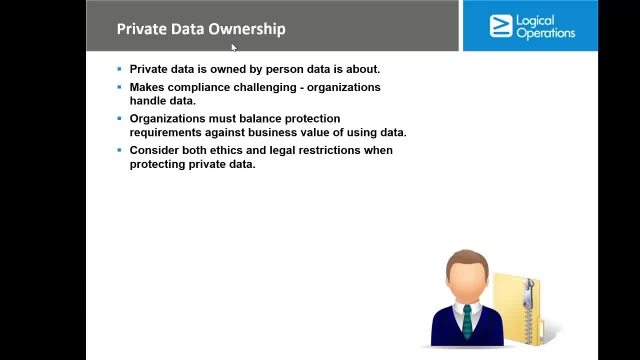 Who gave you this data? So if I'm logging to a website and I'm writing down or I'm filling an application to your company website and I'm writing down all my personal information and you are keeping them, Who's the owner right now? 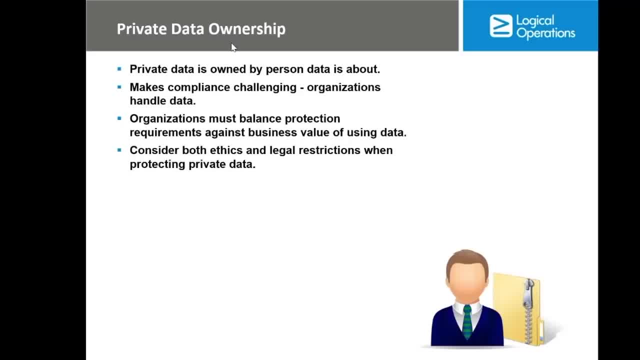 It's not you as a business or as a as a company, It's me, still me. So the owner here is different. It's not like previous lecture, where the owner used to be the senior management or used to be the department and so on. 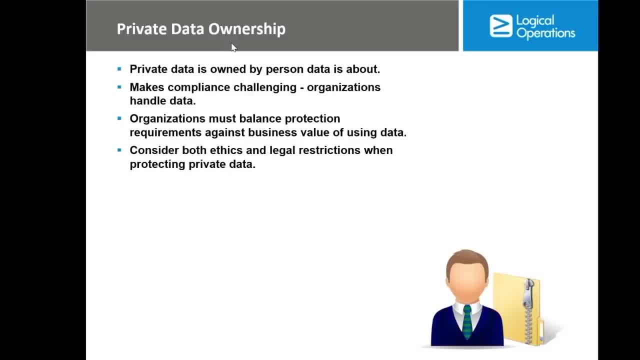 So it's important to know the Clients, the organization, how they are handling this data. It's important as well to try to balance between the protection and the effective of the business. You have some customer information. Definitely you're going to need to use them in your business. 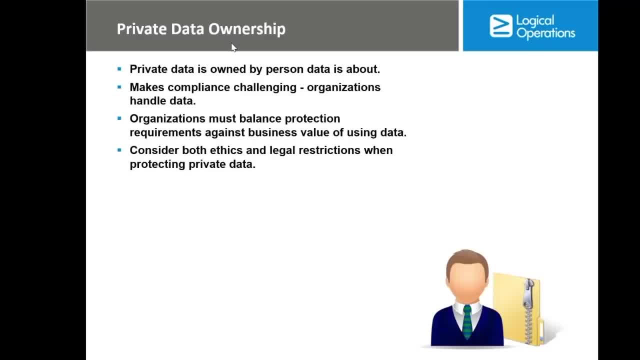 But how can you know that it will not be leaked in any way? So if you are dealing with a third party, for instance, and you need to share with them some personal information to your business, Not to be shared for any advertising purpose or something like that, 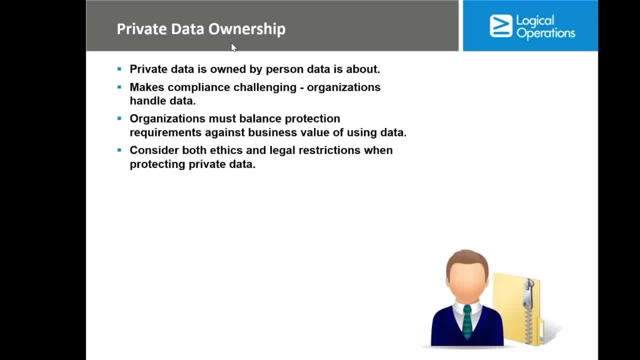 How can you know that he will not keep it and then sell it to a third party or another kind of advertising business? So there is a lot of challenge when it comes to managing the private information, So I don't want to keep it Not to be used. 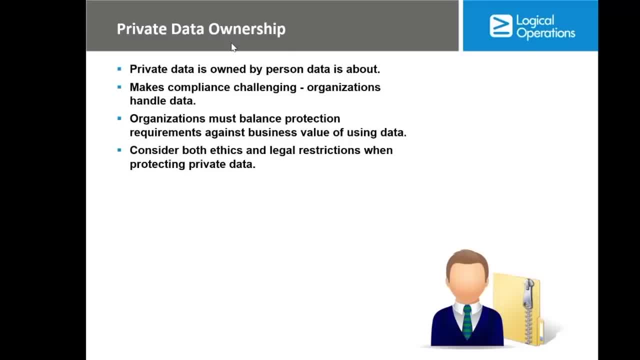 Which will affect my business and if I'm using that in my business, I need to make sure it will Only be used for the purpose of the business, Not for any advertising on anything else. You need to consider the ethics and legal restriction. 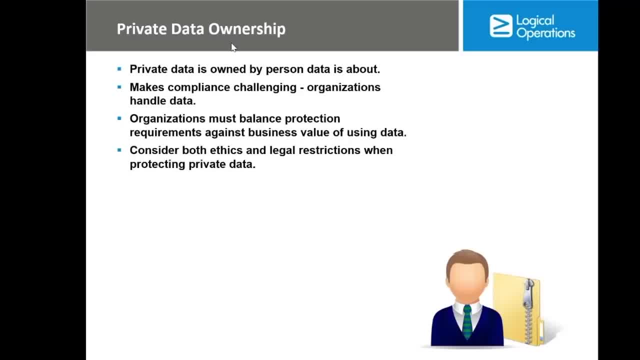 When protecting private data, It's quite important not to get someone number and try to misuse that, or get someone information and try. This is a sick part, but the legal part actually is very strict. So the first approach to the privacy if you are collecting private information is too low. 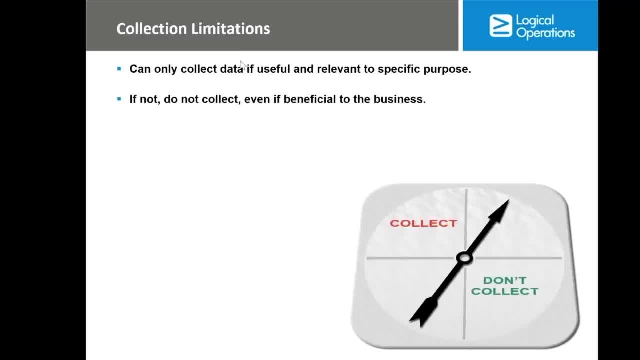 It's to know which law you are Following. Also, you need only to collect the information that it's needed for your business. So, for instance, If you are allowing people to make purchase online, where you are getting the name and the address, shipping address and getting the credit card information. 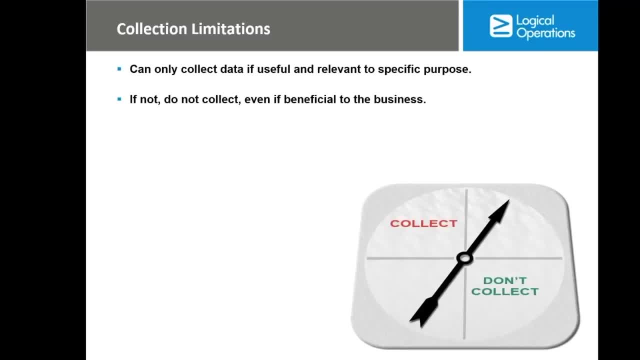 You should not ask for information that is not used for transaction. like you know where are you located, What kind of Car you are driving, is your house rented or this information has nothing to do with the information. Do you need to make the transaction? 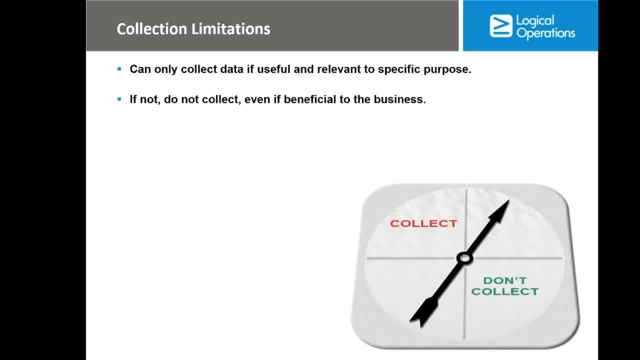 So you need to make sure to limit the collection Now. maybe you don't plan to misuse it, but getting a lot of information will raise the risk of losing it. So if I have a huge amount of information and I'm only using 30% of them, 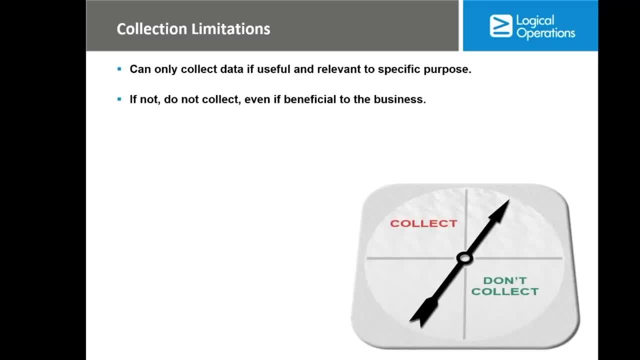 I need to double my effort to secure All of those amount. What if I only collect the information that I need? I will reduce the amount of control that will be implemented to secure. So it's not an advantage to get information and saying maybe I'm going to use it later. 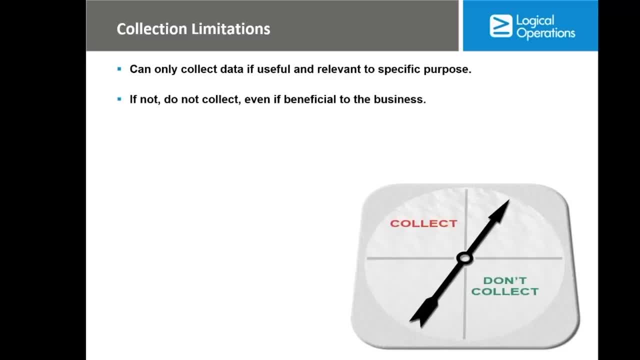 It's not like that, because it will take you time to secure them And if you break, if it get breached for somehow, you will take responsibility. So you are raising the risk of that. So, if not, do not collect Any information if it's not needed. 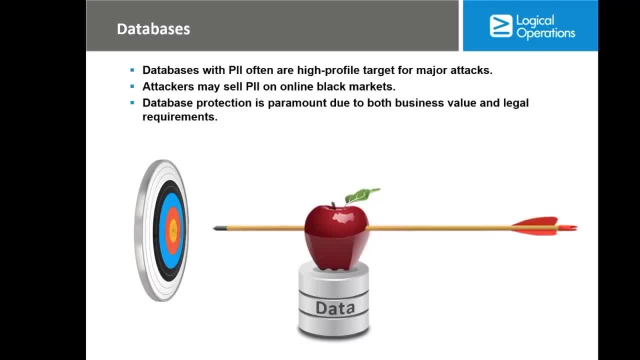 Databases. Most of the information will be saved. private information- We still talking about private information- will be saved in database And just by doing small research, online checking, like the last few years breaches. actually just few days back, Twitter has been compromised And I published that on my Facebook page and actually it has been everywhere online that a lot of account has been stolen and Twitter. 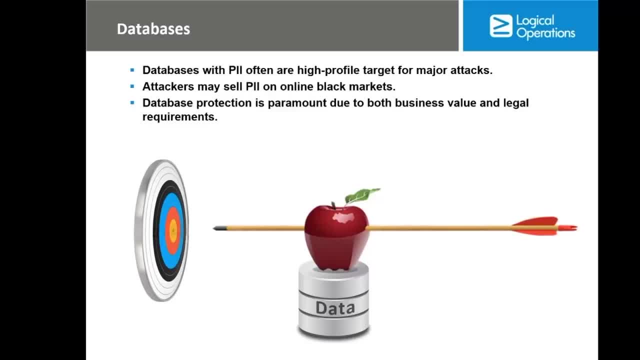 Request user to change their information. Now this is a privacy breach, right, Because Twitter collect our information and they should secure them. So by getting breached and the information gets stolen, this will be an issue. Also special is a credit card information, which is all also kept in databases. 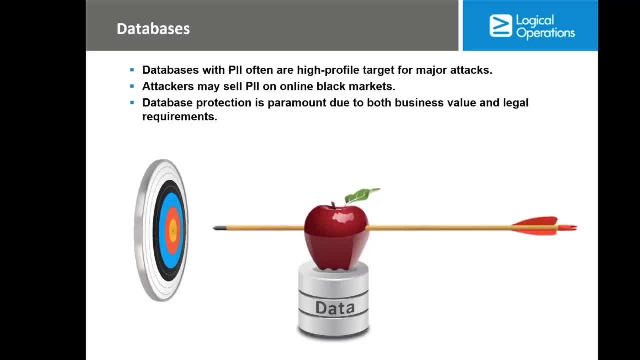 It gets compromised. Usually, attackers are looking for this kind of database. It got compromised And they took this credit card Information. what they are doing with. by the way, do you know what attackers are doing when they steal a credit card? They are not using it online to like buy something, because it's traceable. They will sell it on the dark web, on the internet, Some of the website you can go and not yourself. Of course, any malicious hacker can steal those credit card and offer them online. They are selling each credit card with $1.. So that's it. 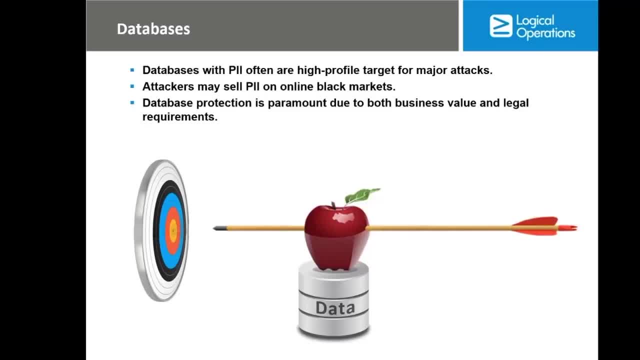 He's breaching database. It has 1000 or it has 10,000 or 100,000 credit card and then sell this credit card online and getting 100,000 and it's untraceable. So those databases that hold the PII. your responsibility is to provide the best or the most secure control that you can have. 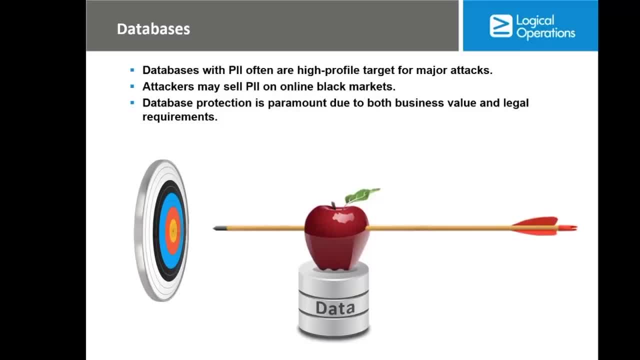 So if you have a regular database but you have other database that has a PII, Both of them need to get your secure attention, But the PII database going to need to do twice the effort to secure them, monitoring them, putting access, control, encryption. 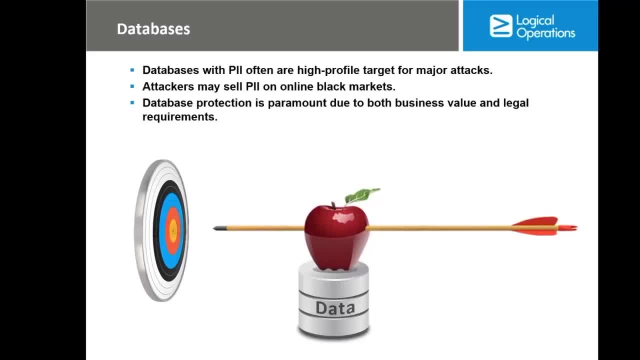 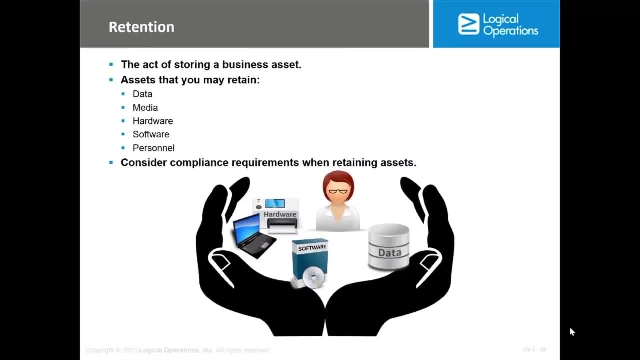 We're going to talk about the controls that can be implemented. In this lecture, we're going to talk about asset retention. Any kind of assets- It could be data, could be media, could be hardware or software, or even people- need to be kept for a specific period of time. 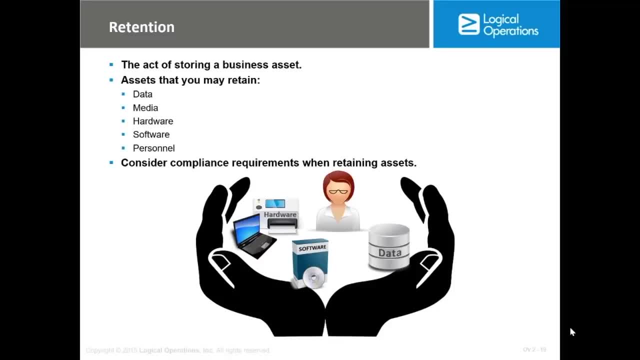 I cannot keep all the business and ongoing business information for lifetime Right, So you need to have a policy that are mentioning how long we are keeping our assets- different kind of assets- because this will be considered your internal rule, But this should not be interfering. 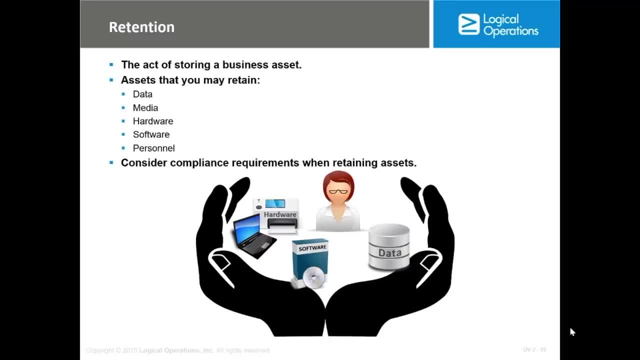 With the government law and regulations. So, for instance, In some government they ask you to keep all the logs or the surveillance cam for 90 days, surveillance cam recording for 90 days. I cannot have my policy saying I'm going to keep it only for 60 days. 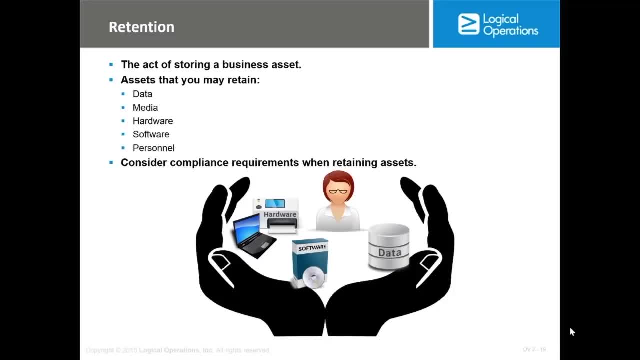 So whatever policy you are doing to for data retention, it should match or it should be. it should not be interfering with the government Law and regulation. So the assets that we're going to cover here will be different kind of us data. How long are you going to keep data media- saying media, which is the device, the device that hold data, like CD or DVD or external hard drive or USB hardware software people? 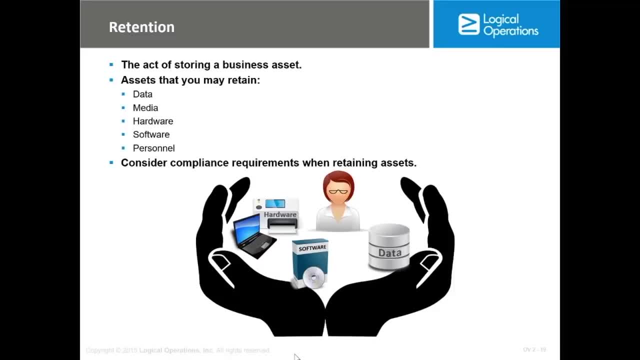 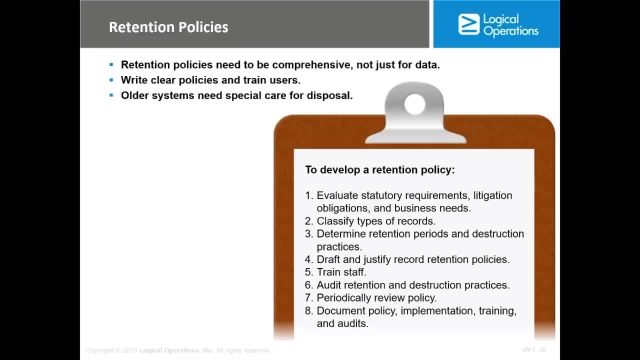 We're going to talk about each one of them, But, as you can see here, you should first check the compliance. Then you should have a policy. I cannot do that based on what I think. Okay, let me this year decide to retain the data for six months, while next year? 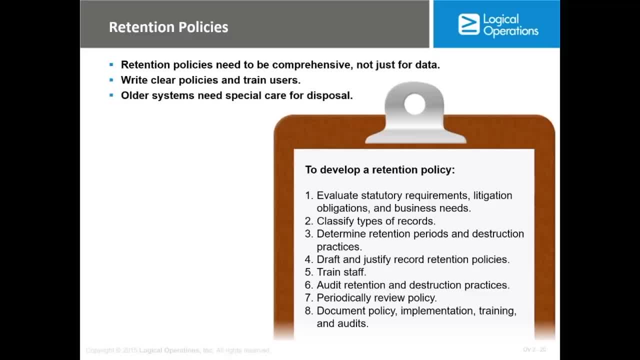 I'm going to do it in a different way. It shouldn't be done this way. You should have a policy. in case of any audit, You're going to say that I'm retaining the assets according to our company policy And again, you should consider the legal requirement in this policy, that how long you are keeping according to the legal requirement and 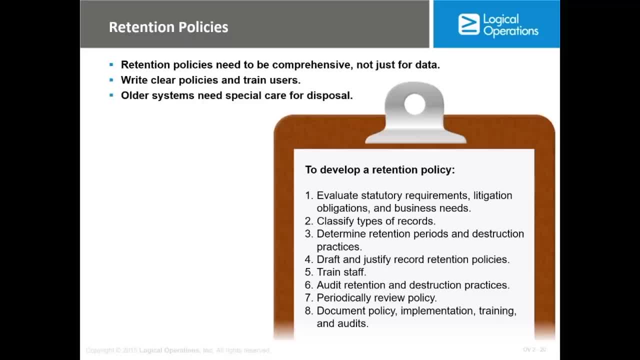 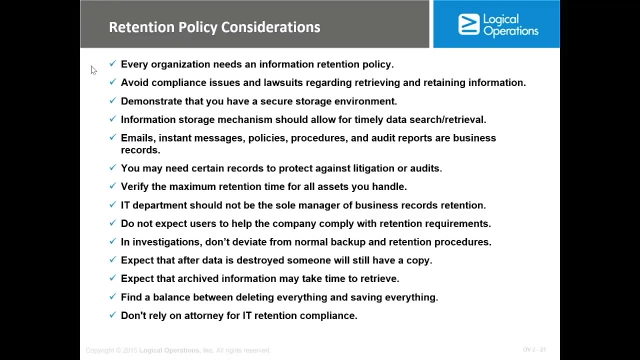 Sometimes also, we need to consider the disposal. So maybe I'm keeping the information for 10 years and after 10 years I have a secure policy for the disposal of the assets. So what are the consideration when it come to the retention? What should you consider first? 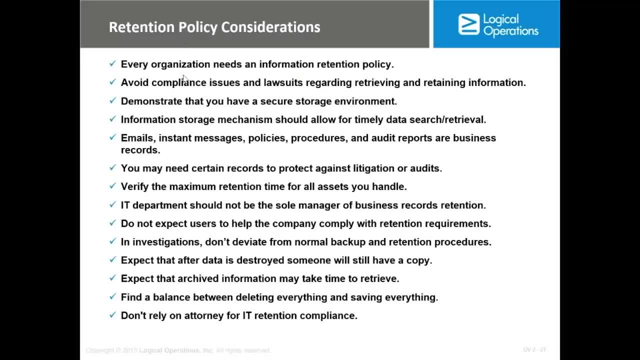 As I told you, you need to consider the law and regulation first. You need to make sure, if you are in government, you need to see what kind of flow and regulation Regarding the keeping the information If you are a private military, each entity have their own law and regulation. 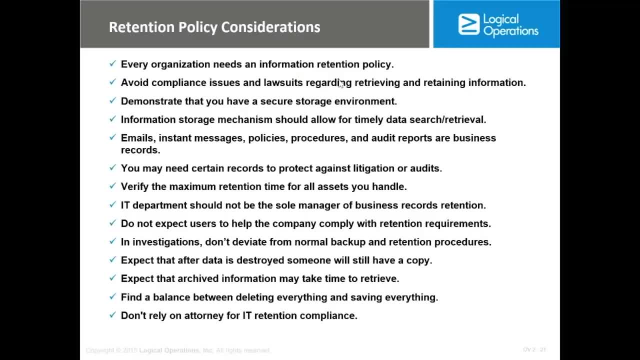 Then you should write the policies that map this law and regulation and you add to it How long I'm going to keep different kind of assets, Because you're going to find that it's not specific period of time Like usually financial information. It usually kept for seven years, while surveillance cam recording is usually for 90 days. 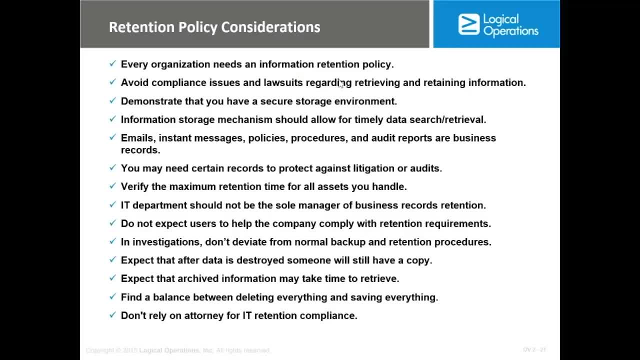 So it's not like it will be one specific time Or duration for all your assets- It depends. So, second one: it's extremely important: Avoid compliance issue and lawsuits regarding retrieving and retaining the information. So you are an information security officer in any business. 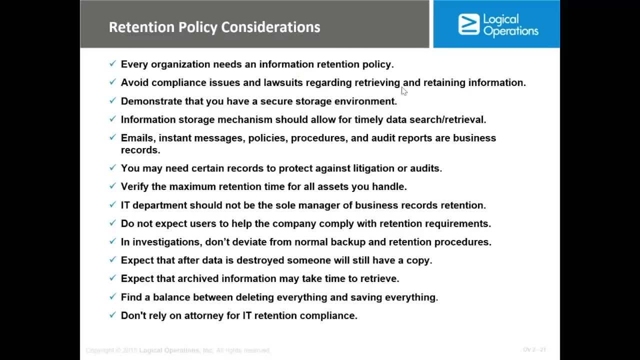 You decided to keep the information only for three days. Sorry, three years, The financial information. now, for some reason, government or any entity requested information that was Before four or five years and you told them I don't keep them anymore, I just written them for five years and in the laws, 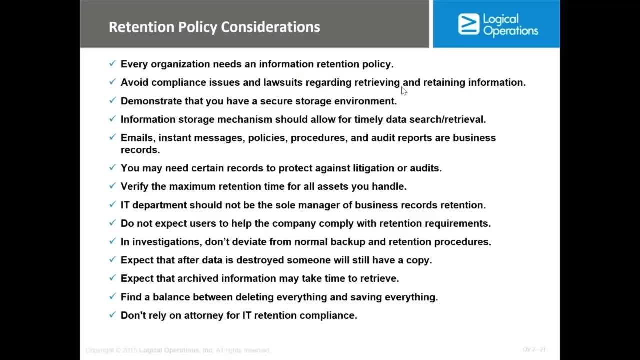 They are saying it should be seven years. You're going to take the whole party, So you're going to take all the legal consequences for that. So it's quite important to understand that it may lead to lawsuits and legal problem Demonstrates that you have a secure store environment. also, when it comes to securing 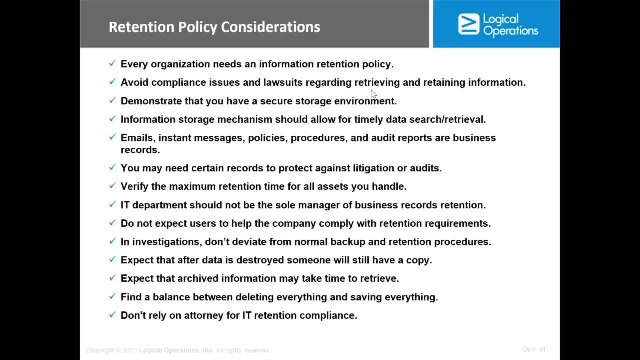 Decide in the policy writing down the duration. Also, you need to make sure that you are secure them in your saving them or storing them in a secure environment. Okay, information storage Machine Should allow for timely data search or retrieval, So you're going to keep them somewhere. 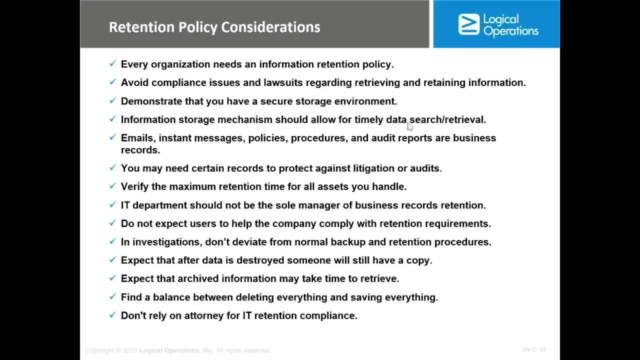 How are you going to retrieve Them if it's needed? Is it an easy way for doing it? or you are keeping it somewhere where it's hard to retrieve, or it will take time? Everything like emails, instant messaging, policy procedures, audit report- All of them should be retained for a specific period of time. 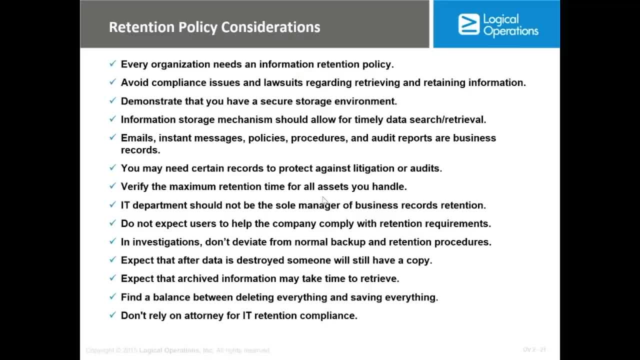 Legal is a big issue. as we explain, IT department should not be Sole manager of business record retention, So it's not just the IT department responsibility, but it's all department or department. in specifying the duration, Maybe IT department need to provide the infrastructure needed. 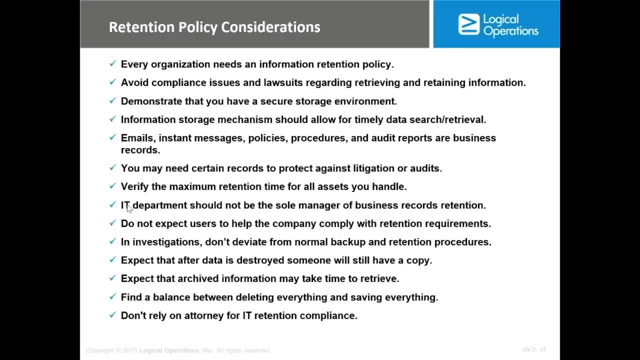 But after all, it's all department responsibility. Do not expect user to help the company while retention requirement. We, as an information security people, we are always facing this kind of resistance. You know people are not cooperating that much, So you need first to have a management support and then you need to follow up with your requirement until it's fulfilled. 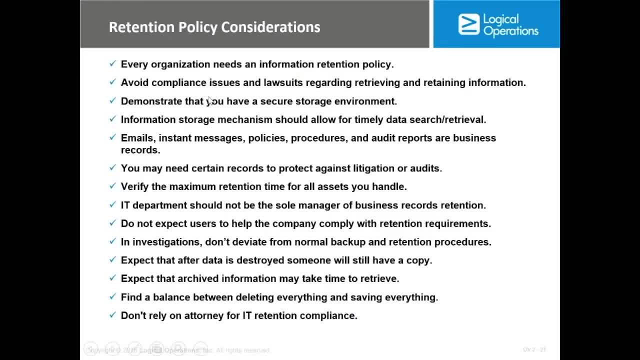 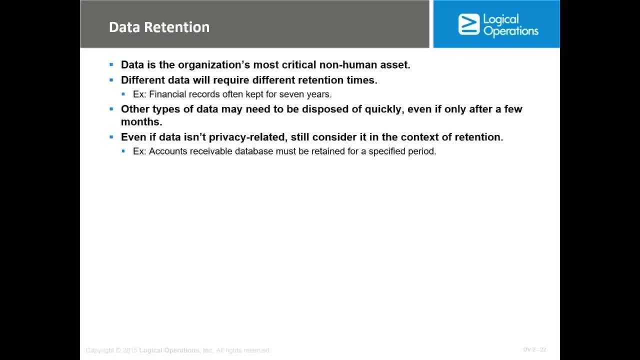 This is about What you need to consider when you decide About the retention policy. I think SANS has a very good retention policy. You can read it and if you need one, just let me know that. the retention, as I told you, it depends. 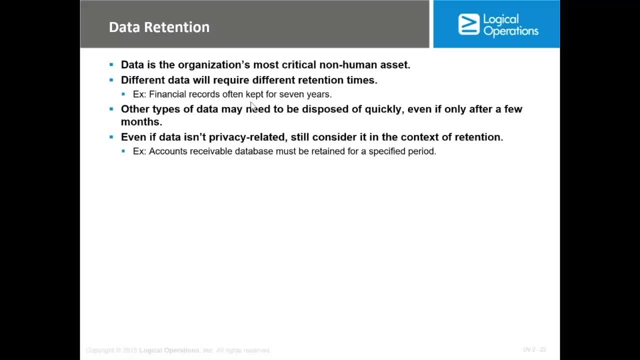 And, by the way, I think this is one of the questions that you may face Inside interviews: How long do you need to retain Data? So what if you get a question like that in an interview? They ask you: you're going to be hired here? 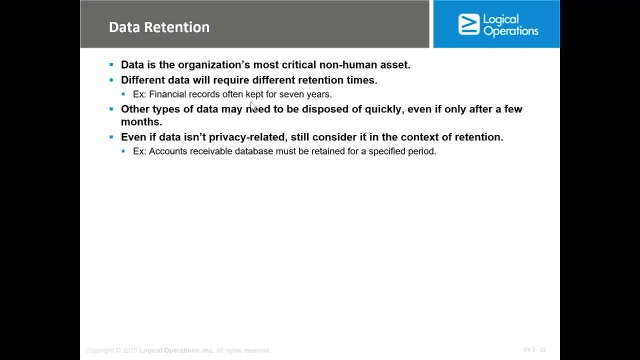 How long are you going to keep the data? What will be your answer? A very good, like mythology when it comes to interview. Okay, it always depends. Always start your answer with it depends, because this is really the right answer. We don't have a solution that fit for any kind of business or organization. 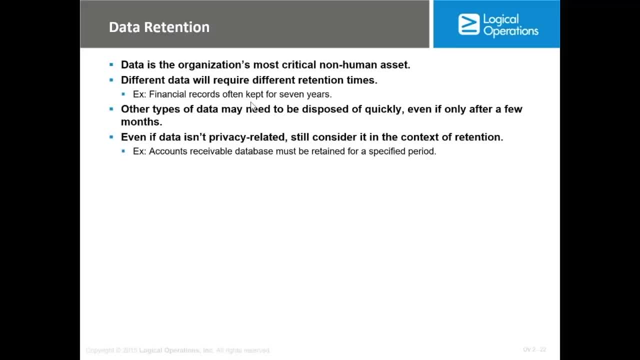 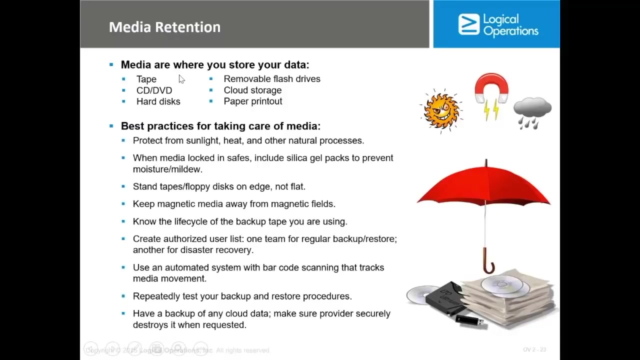 It always depends on something. It depends on the storage that you have, It depends on The law and regulation, It depends on many factors, but it always depends Media retention, media, which is the media that keep or store the information, like the tape, backup tape, CD and DVD, hard disk, removable flash drive, cloud storage paper. 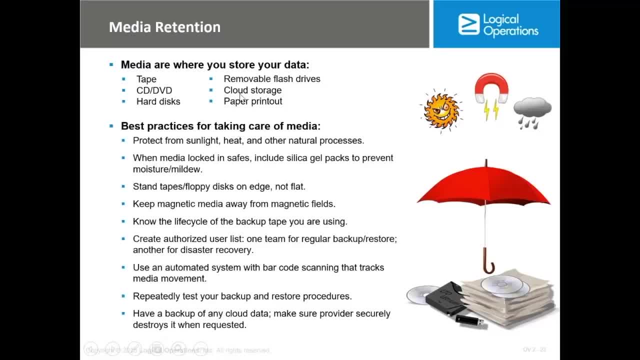 Okay and the best practice just to keep them in a secure place. If you are retaining them, Do not put them in a place where no good or it has heating or sunlighting because, as you may know, the sunlight are affecting the CD and DVD. anything that may affect those detention. 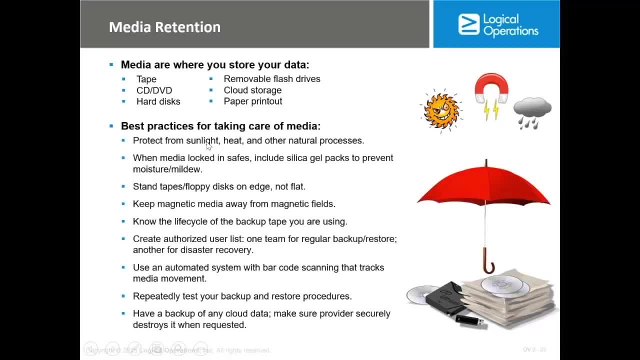 It should be locked in a safe place and you should have an inventory about them. I cannot keep like storing the backup tape and they don't have a list about how many backup tape do I have, So you should have an inventory for that. Make sure that any magnetic media should be away for magnetic field and there was a story about the company. 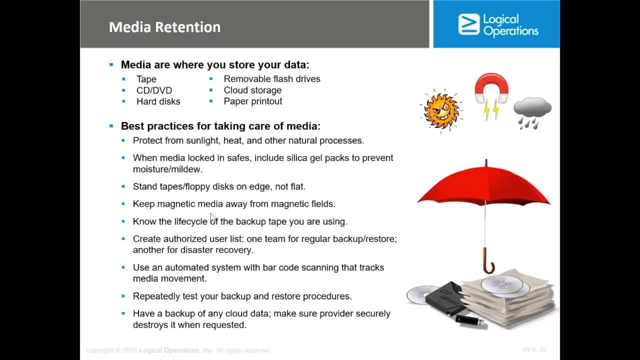 This is actually a real story- that they were following the best practice when it comes to backup, but they used to keep the backup tape in a place near, like a power station or something like that, And because they didn't do any kind of restoration testing, which we're going to talk about later on. that. 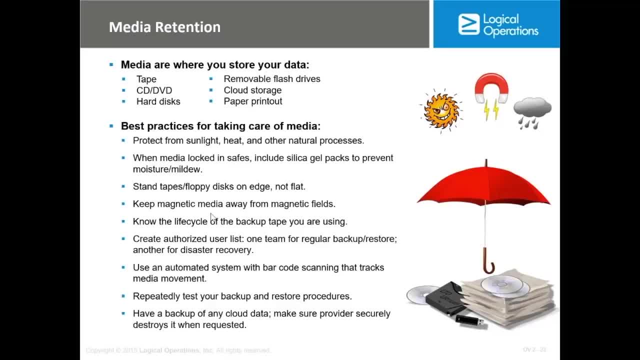 It's not just taking a backup, but you have to do a restoration testing. I don't have to wait until something went wrong and then I restore the information, But I need to do that from time to time. So this company used to keep the backup tape. 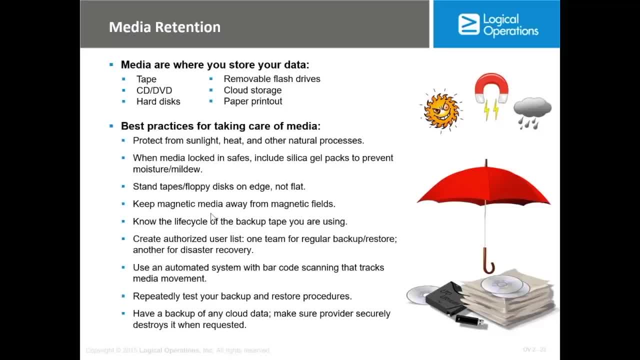 They were taking backup daily and keep it in a place, but the place was near a magnetic field, So when a problem happened and the information get destroyed and they try to restore, all the backup tape was useless. So it's quite important to keep them in a secure place. 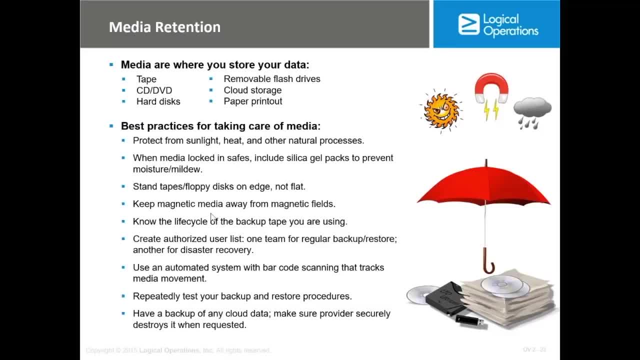 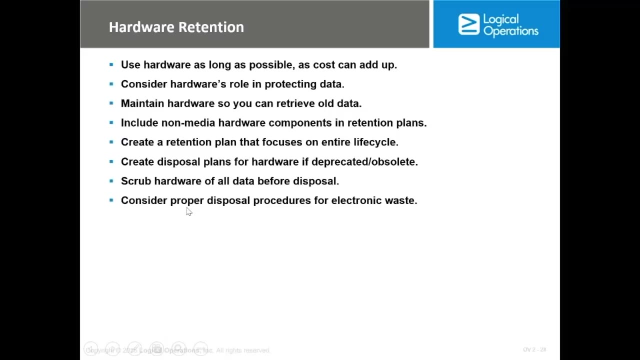 Far from A magnetic field, but it's more most important to test them from time to time. Automated system for inventory, as I explained. Don't forget the restoration testing. It's quite important. Hardware retention for the hardware Also. I need to keep them as long as possible to utilize the cost. 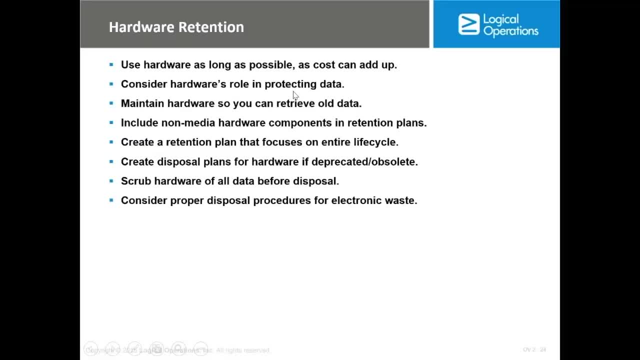 I need to consider hardware role in the protecting the data. Maintain hardware so you can retrieve all data. Include no media hardware. It's important that if you are getting rid of hardware, That to make sure that no information can be retrieved from the hardware. 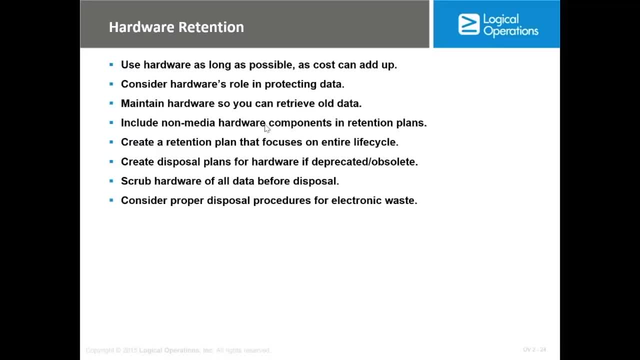 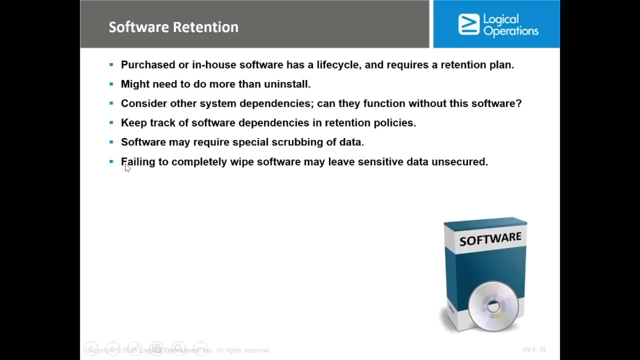 So even the disposal of the hardware. they need to be according to a policy and using a proper tool that prevent data for getting retrieved. Software retention Also, same rules apply. What do you need to consider when it comes to how long I'm going to keep, because the software has a life cycle as well? 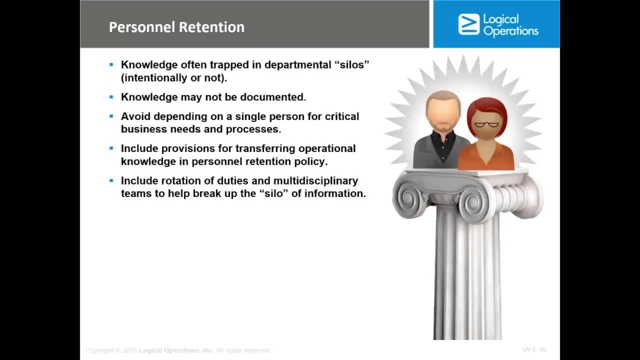 So after a while it gets retired. So the retention. finally, the personal retention. Now, this is a hard one. What you going to do about it? You are keeping someone for working in your company for a long time. He start to get the secret of work. 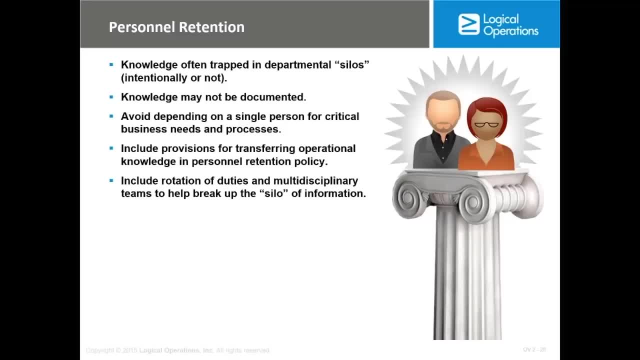 He start to know about the know-how. How can you protect your business when it come to this? because it's not really an asset that you can keep. So, for instance, I'll give you a good example- What about people who are working in Pepsi or Coca-Cola and they know the secret of how Pepsi it's done? or Coca-Cola right? 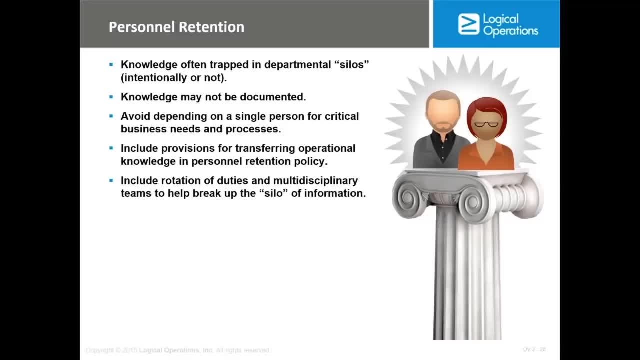 This is a big asset because actually this is their main assets. If those people like left the company or sell the secret to another competitor, Pepsi will lose their business, or Coca-Cola right, What do you think they are doing to protect against that? 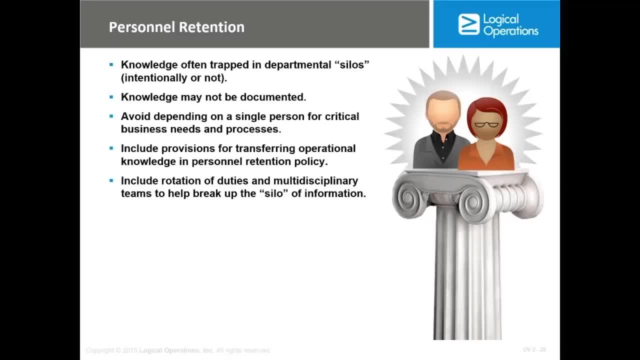 Many things. first, they will not give the full secret to only one guy. Secret will be divided between different people. So, regarding the recipe of doing Pepsi or Coca-Cola, usually four or five people. I'm just assuming. I don't know exactly how it works, but the way that I think it should be managed, that this secret should be between different people and no. 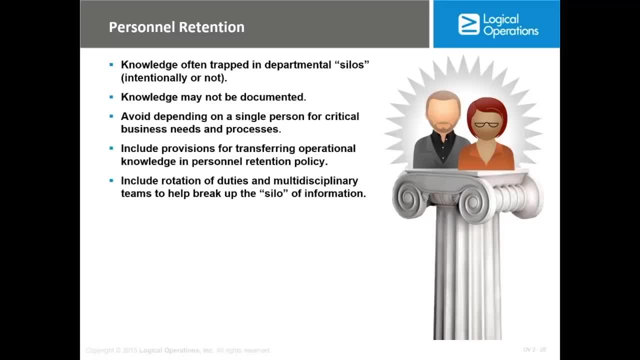 One should know about the other one in a way that if someone left the part that he know will not allow him to sell it to any competitor, I should let him sign a non NDA Even after he is leaving the company. He don't have the right to sell the secret or to sell whatever information here, and according to that, if it happened, I can take a legal action against him. 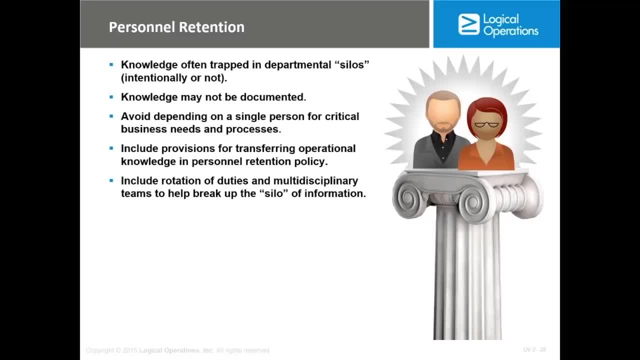 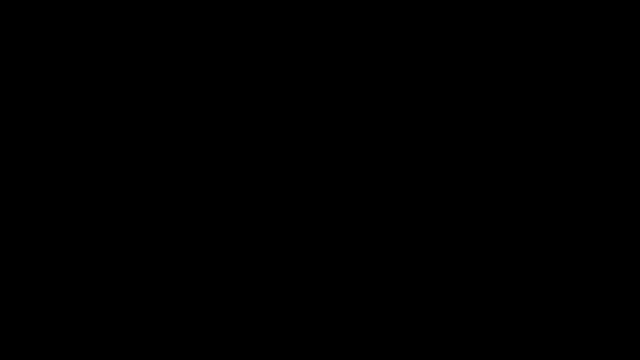 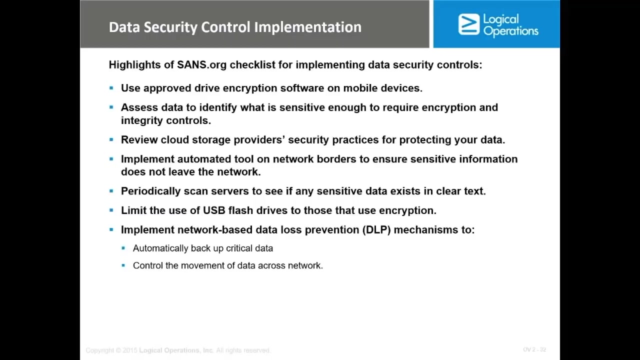 So personal retention. This is actually the challenge. How can I make sure that the information that people Is keeping in their mind get not leaked or get not misused? We're going to close this domain by talking about data security control implementation. As you may know that I may have different state. data could be at rest, in a sense that data could be stored somewhere or on a media, or data could be in. 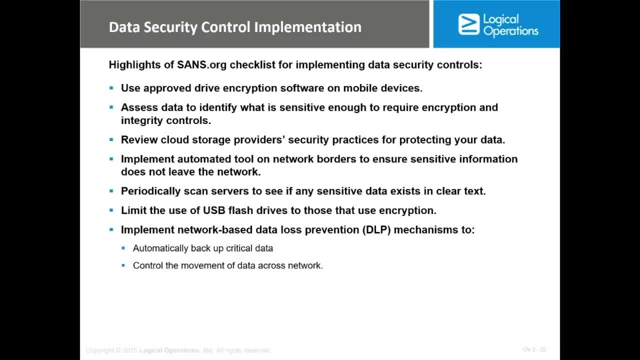 transmit, moving From one place to another, how to secure data in different state. Before going through some of the best practice regarding data security control implementation, I would like to refer you to a very important document. It's not really a document. It's more as a checklist that you can use in your business to check if your data is secure or not. 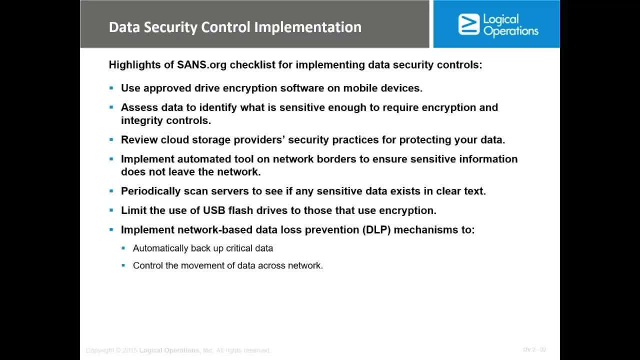 This document can be downloaded from free from sans website. You'll notice In this course that IC square is referring to sans in many location, So it's one of the good sites that you can use for downloading policy and procedures or downloading a lot of templates like checklist. 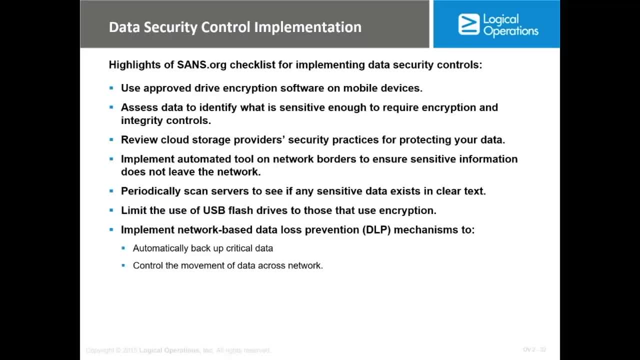 So, before going through some of the best practice, let me show you the documents that I'm referring to, and kindly be aware that I'm going to attach this document to the lecture, So, in case you fail to find it, It's a free document. 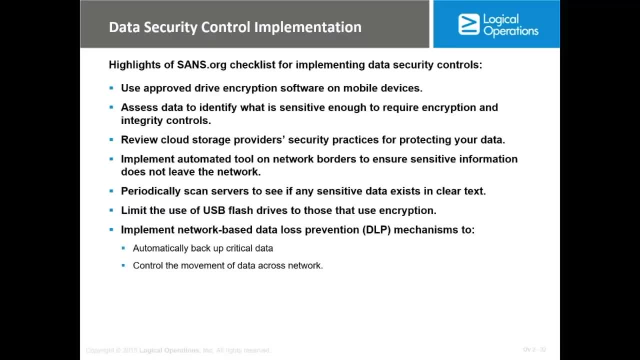 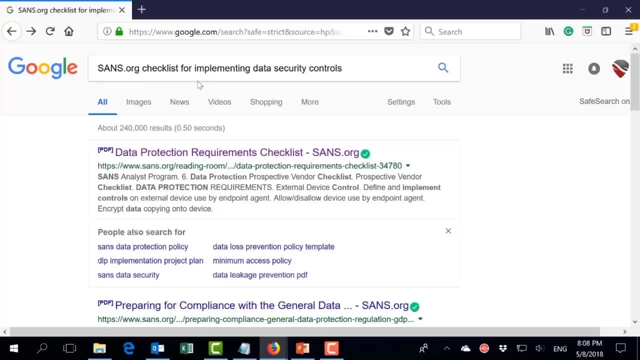 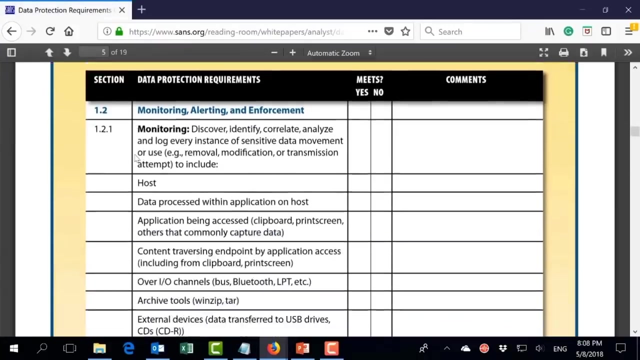 I will attach it to this lecture, So let me show you how the document look like. So to get the document, just Google it, search for sansorg checklist for implementing data security controls and you're going to find this checklist. It's a PDF file, but it's actually quite impressive because, instead of like implementing those control randomly, it will give you this checklist. 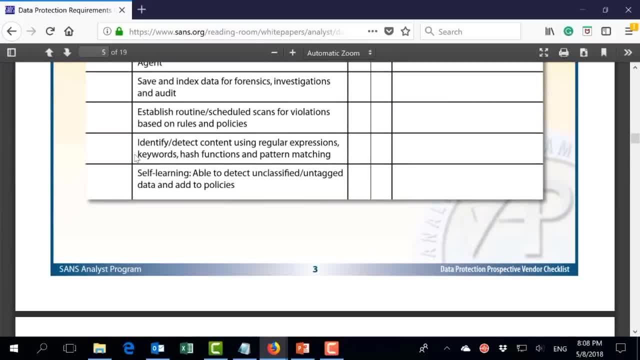 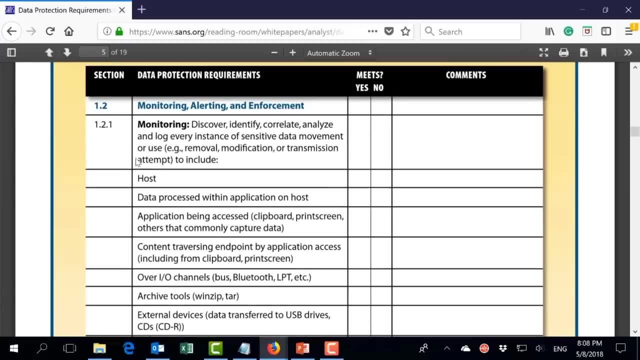 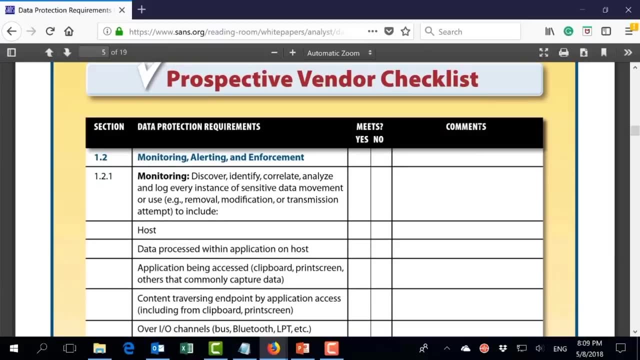 It's very long- actually It's 19 page- but you don't have to To implement all this control, only the ones that apply or it's applicable to your business. So, for instance, this is the data protection and here you can write if it's met or not and the comment is here like it will be implemented as a future or we are working on a solution, or something like that. 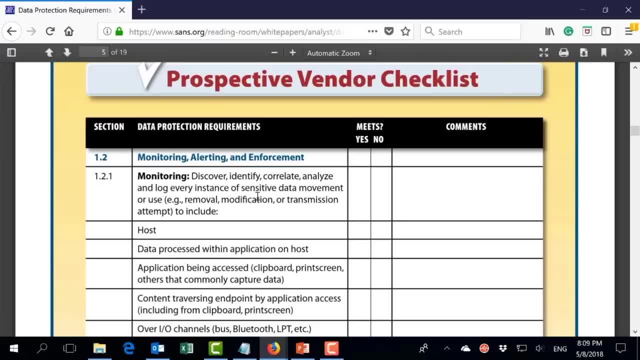 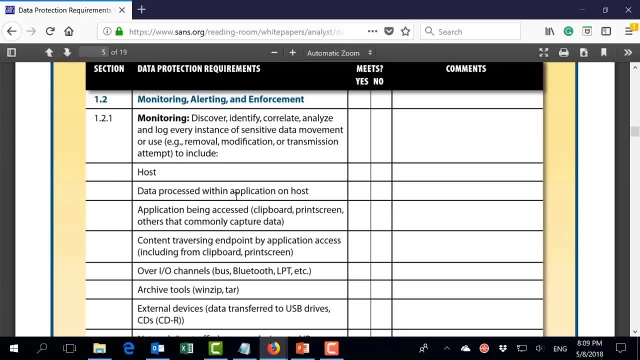 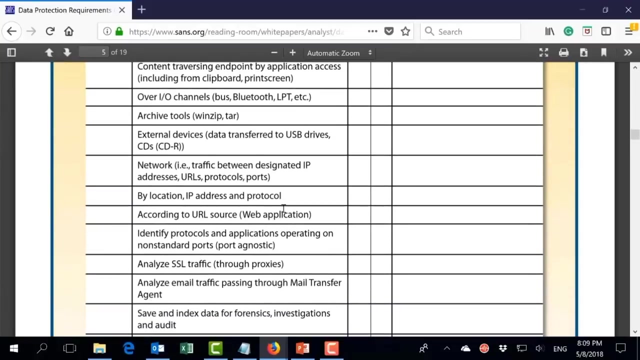 So do you have a solution for monitoring, discovering, identifying, Analyzing and log every instance, Yes or no? Do you have for instant data process with an application on host- Yes or no- application being accessed like clipboard or print screen? Are you are allowing that or not, because someone can misuse that? yes or no, and so on and so forth. again, you can choose whatever you see. 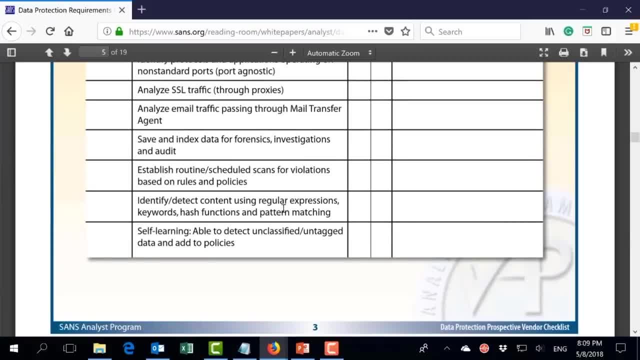 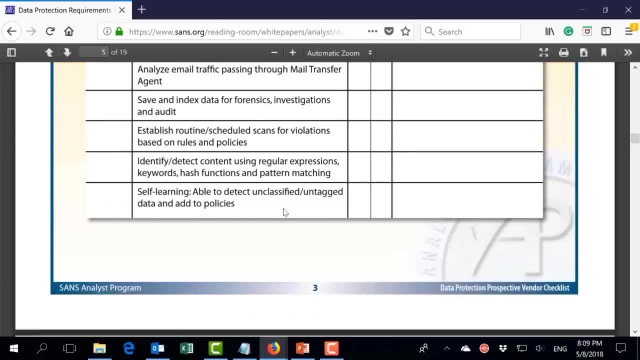 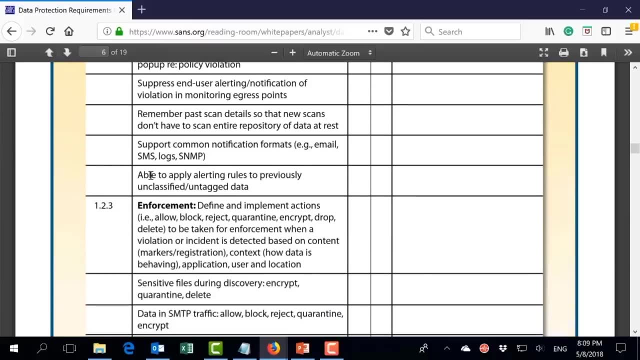 It's more applicable to your business, but this will be a checklist and those are the controls that need to be implemented, based On the type of business that you are running, and here you can choose if it's done or not And, as you can see, it's divided by section: monitoring, alerting. 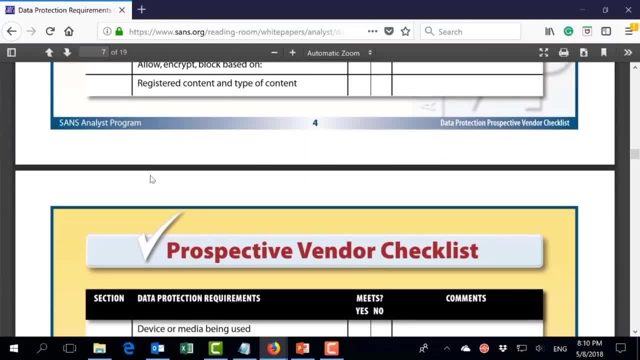 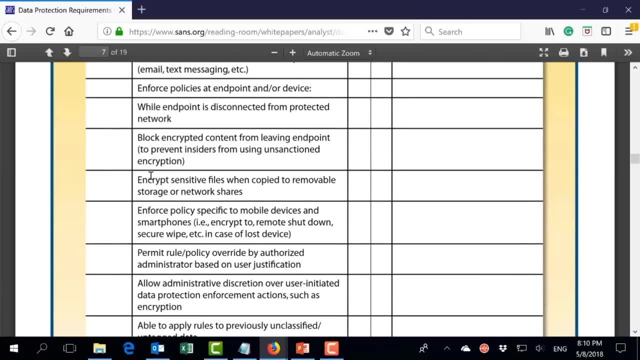 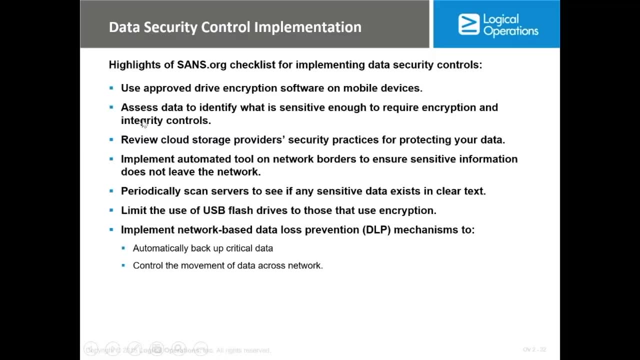 If you have a DLP solution, it will give you question If the DLP solution is fulfilled- some of the requirement- or not. So it's an excellent document that you can use. Now let's get back to our slide. So, after going through this document, from sense, as you can see, there is some options. 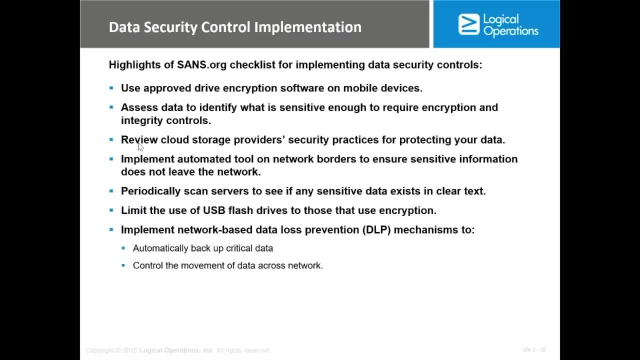 That you can use in general for data security control, like use an approved drive Encryption. encryption is very important topic and it will be covered in depth in the next domain, Identifying the sensitivity of the data, which is a part of that will be classifying the information. 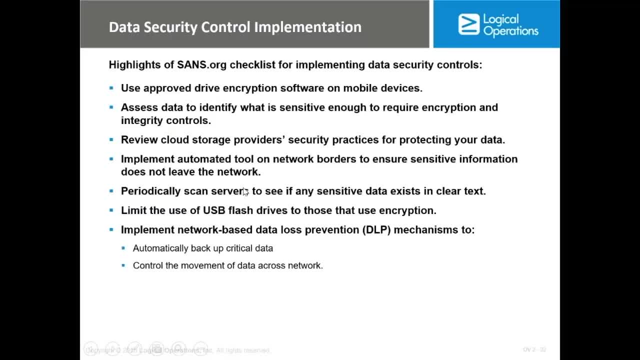 If you are using a cloud storage, you have to check if you know it's, it's is a secure cloud and you're going to discuss in the Cloud how to verify if this cloud is a secure solution or not. A lot of government has a concern when it comes to using the cloud. 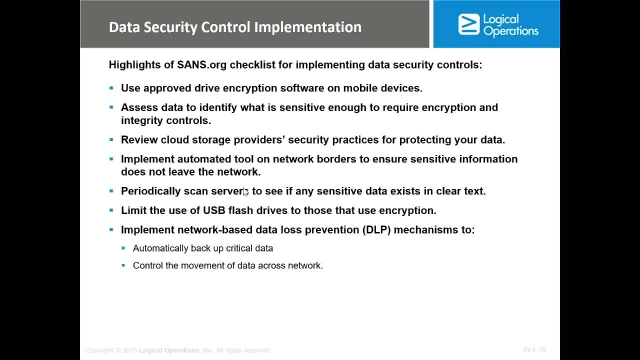 So I will share with you an excellent cloud checklist- security checklist- that you can go step by step and accordingly decide if this is a secure cloud solution or not. This is very important actually, which is implementing an automated tool on a network border To ensure sensitive information does not leave the network. 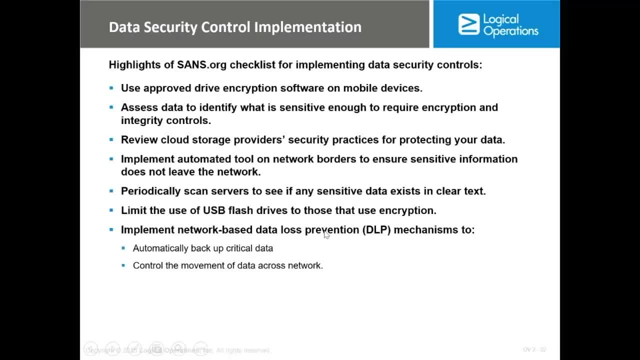 And, as you can see, it was quite clear here then that they recommend to use DLP. We already explained the DLP solution and I showed you some some of the DLP and like product as a proof of concept. But the point is the DLP, or data loss prevented prevention, and some people call it data leakage prevention- should be implemented. 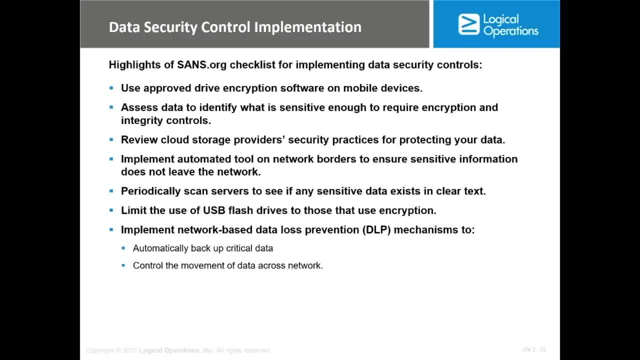 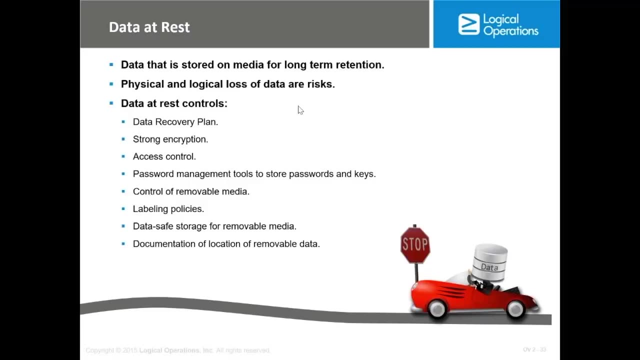 If you need to secure your data and it will put a very tough Control on data in a way to not be copied or moved or emailed and so on. So this is in general: let's divide them to data at rest and data in transmit that at rest. 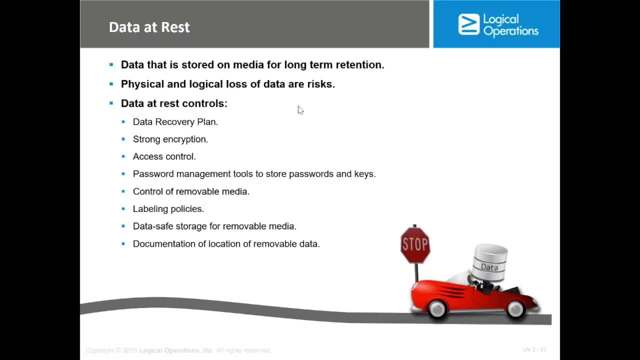 It mean it's stored somewhere, So the place where you are storing this data should be encrypted. and, by the way, This should not be done for all data, because encryption is not easy, as you can see in next domain. when you decide to use encryption, it mean you need to generate. 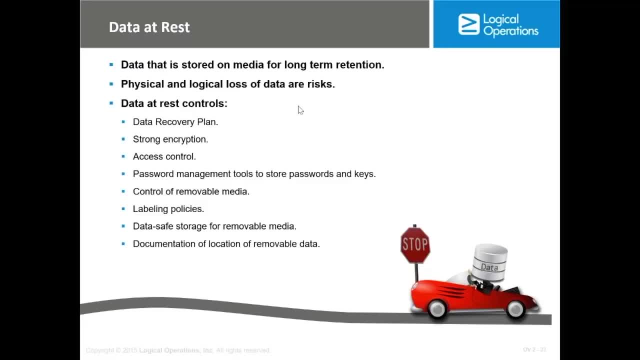 Key. you need to maintain key. This is a big overheads in a bit organization So it's not really a best practice to encrypt everything. You just need to encrypt the sensitive. that but you, if you have some data that is considered public or is not like sensitive. 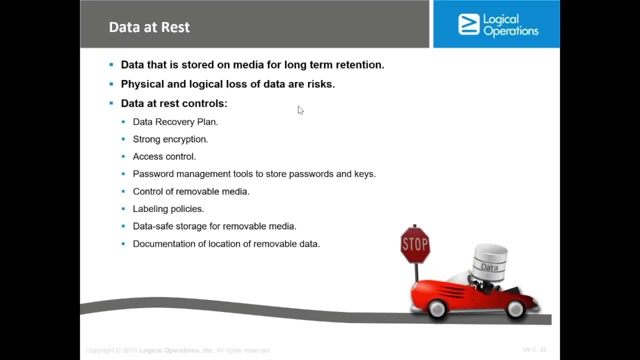 You don't have to encrypt the drive where those data are stored. But again, that encryption will be explained as a concept in depth in the next domain. Access control- allowing to be data to be accessed through a password using permission and access control will be also, as a topic, explained in a different domain. 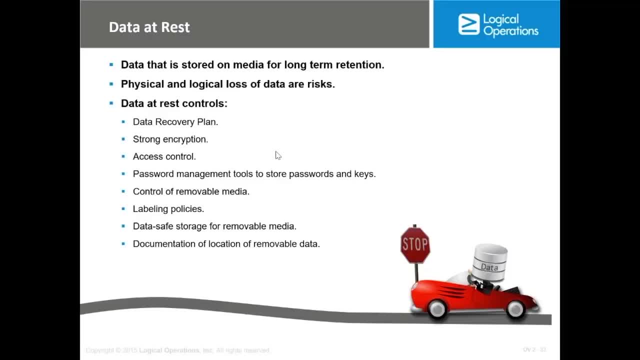 Password management control to removable media. Removable media need to be secure in a safe place where it cannot have like a physical damage because, as we keep saying that we do not prevent only against malicious hacker, but we also prevent Against any circumstances that may lead to losing the information. 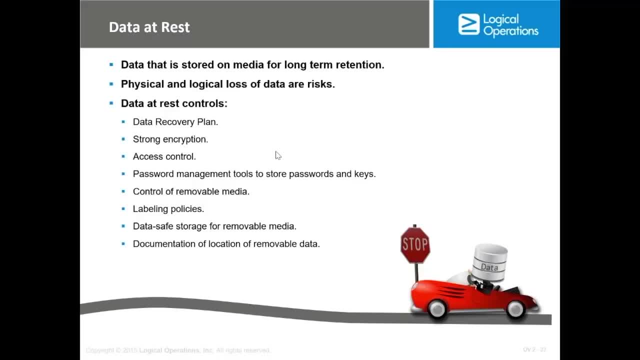 So if you are storing those removable media in a place where they can be like damage or something like that is the same result that will be lost. Labeling, which is quite important. Documentation: very, very important: to have a documentation about all your data. Data in transmit. 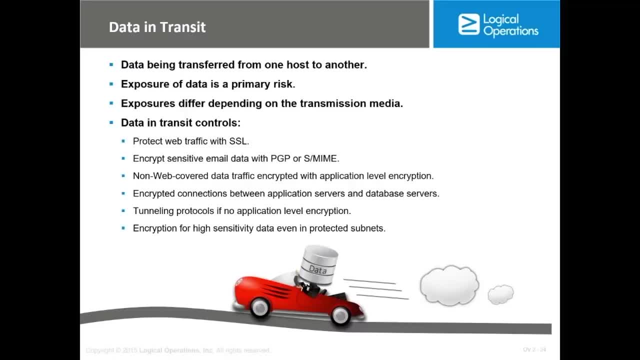 Which means that how to secure data while it's moving. If I'm providing like web services for my customer, Now the customer will be writing down their credit card information and it will be transmitted from their site to the web server, or vice versa. I'm using email with confidential information. 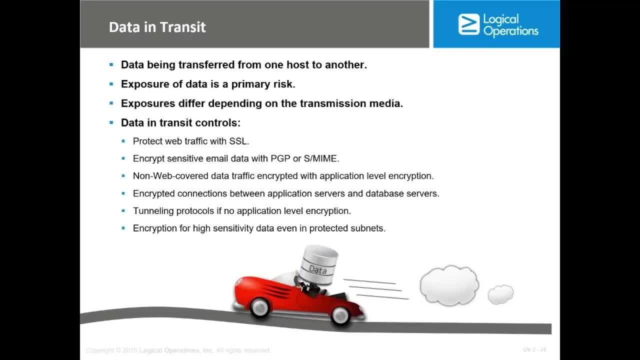 Concept apply, which is using encryption, but we have different kind of encryption for the data and transmit. so we can use a secure connection like SSL. We can use encryption for emails. There is specific protocol for encrypting email like pgp or smine. 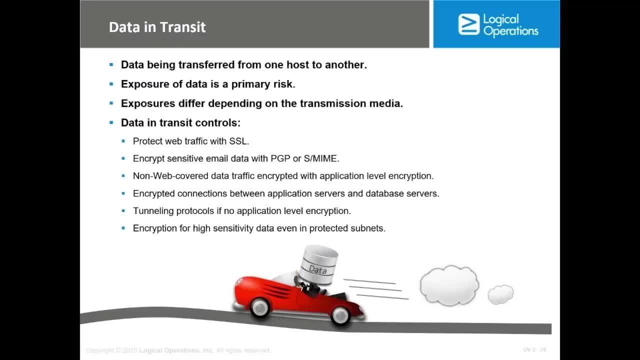 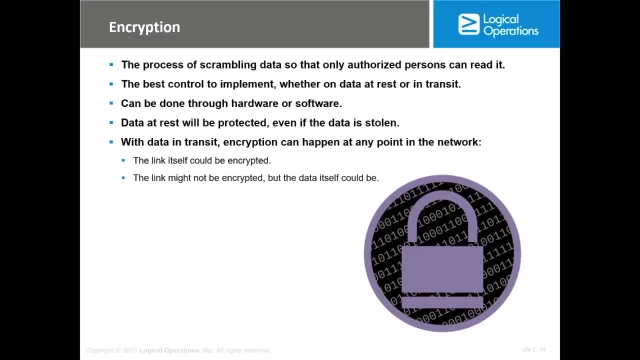 So it's all about encryption, but choosing the encryption according to the state of the data. So, to summarize, we need to implement encryption for all kind of data at rest or in transmit, and we need to have some control. and one One more time: using the SAN checklist will help you a lot to identify if you are implementing the best data security control or not. 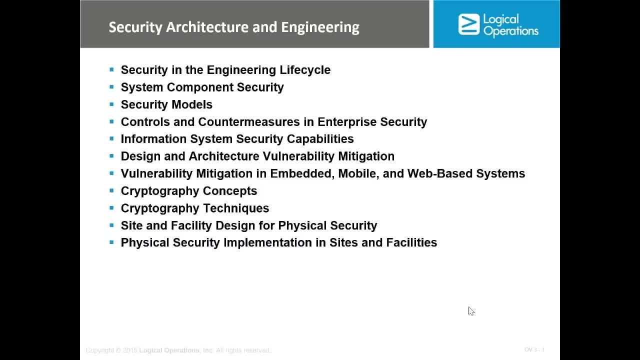 Security, architecture and engineering is the third domain in our course. This is a big domain because it cover many topics that used to be separate domain in the third edition. So, for instance, Physical security, which is one of the topic in this domain, used to be a separate domain by itself in the third edition, cryptography with a separate domain, and we usually get good amount of question about cryptography, security architecture with separate domain. 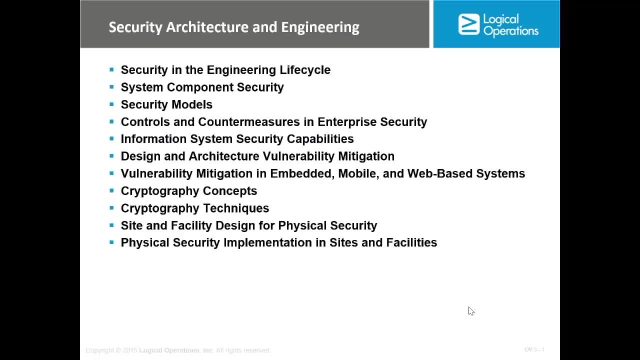 So you're going to notice that they combine many domains together in one subject, which is security, architecture and engineering. in this topic We're going to talk about some or an introduction part that includes security And engineering, Engineering, life cycle, the system component. then we're going to move to very important topic, which is the security models. 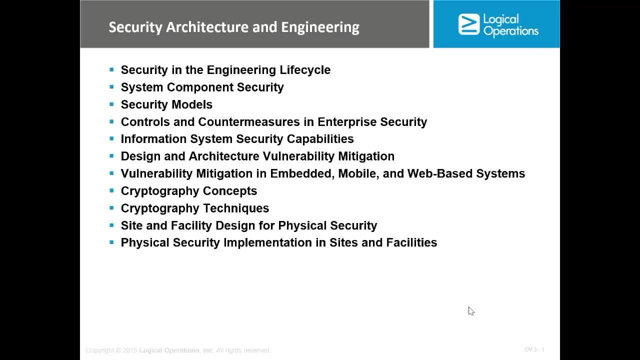 This is actually a very important topic. It's a little bit academic, but I will try to be as simplified as I can to let you know about the concept. We're going to talk about control and countermeasure in an enterprise security. We're going to talk about information security capability, design and architecture. 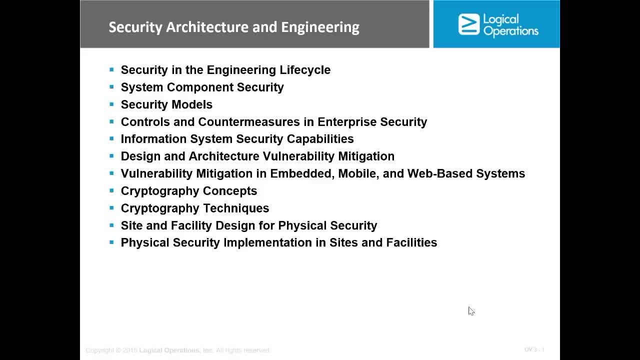 Vulnerability mitigation. We're going to talk about mobile security web-based system. We're going to talk about cryptography, and cryptography is a very important topic And, as I told you for the exam purpose, you will get some good amount of question about cryptography. 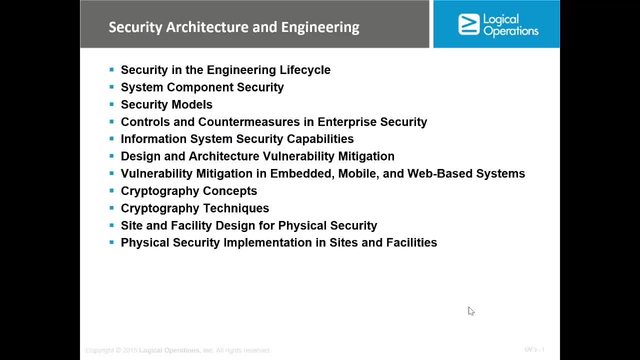 You don't need to dive very deep into cryptography. You're going to talk about the basic terminology or definitions related with it: What is symmetric, What is asymmetric, What is a block cipher? What is so? we're going to cover Everything that you need to know for the exam purpose. 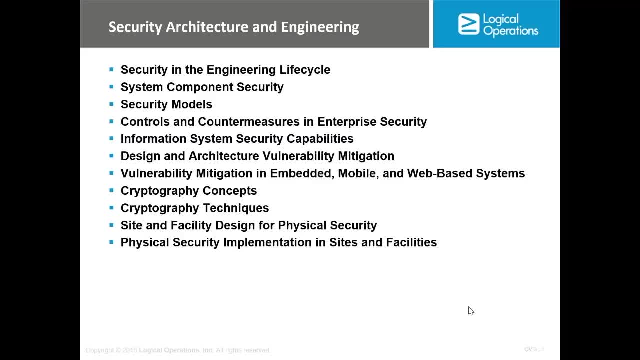 Then we're going to talk about physical security And I will point- because actually physical security is a very big topic, But I'm going to point- to: what do you need to know for the exam purpose And, realistically also, what do you need to know? 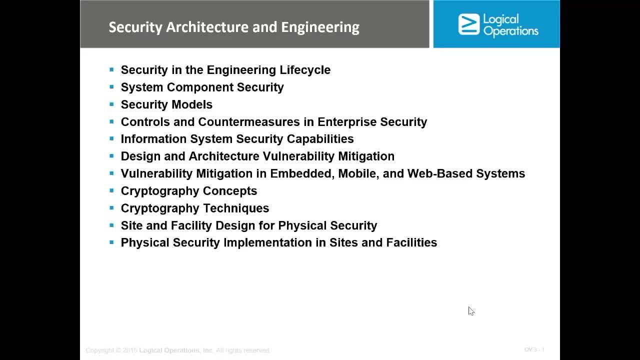 But I don't you to lose the question related to physical security, because they are quite straightforward. Some points they always ask about cryptography also. Also, you get very good Amount of question about cryptography that you should not lose. So while I'm explaining this domain, I'm going to focus about what do you need to know for the exam purpose? 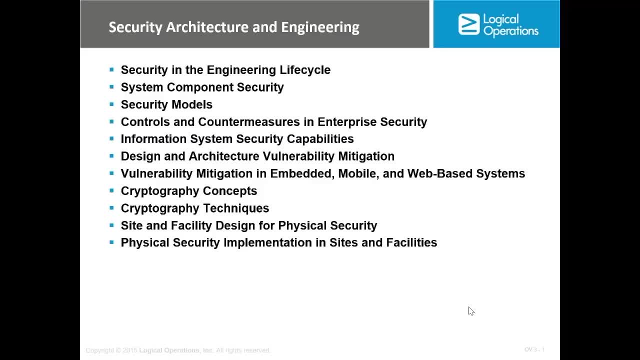 Now kindly be aware is that you're going to need to take some notes from this domain, and it will need some memorizing. I know that some people are not comfortable with that, but still, you're going to need some memorizing when it come to this specific domain. 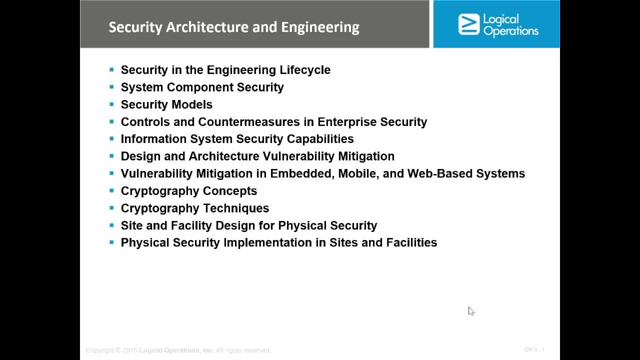 Also one of the good points That we're going to learn about this domain, which is measuring. How can I measure security in a computer environment If I have two different machines that I need to use in my work? which one should I choose? 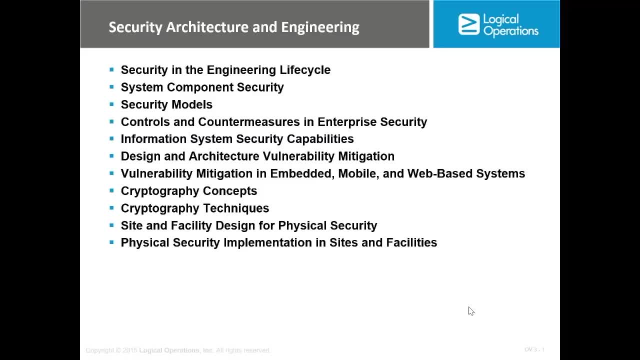 Should I choose the HP or should I choose the Dell, for instance? Is it measured this way, by the brand name, or do we have a way for measuring the security? if the following concept can be implemented, So it will be that great, or if not, it will be that great. 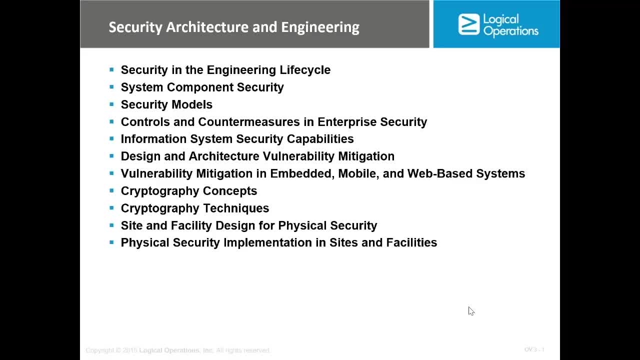 This is very important To understand a way for measuring the security in a computer environment. We can learn about that in a very simplified way. So let's start and let's take it step by step and let's see how can we get to understand the security architecture and engineering. 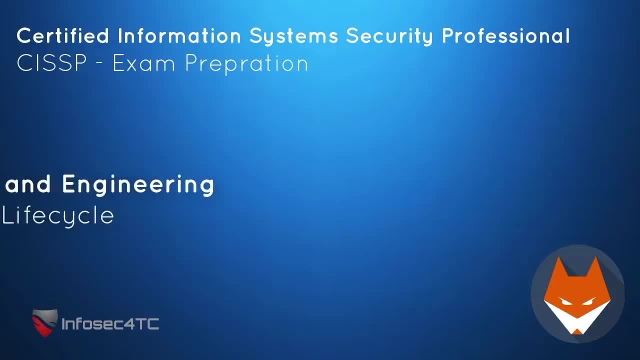 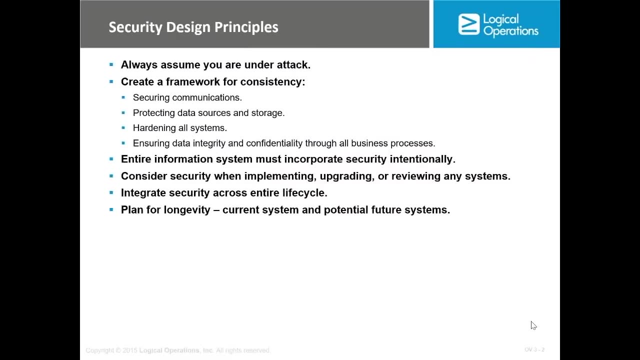 Very well. This domain is covering two main points: The security architecture, and this will focus about the different security models. It will focus about the way for measuring the computing system security and the different standard used for That, and the security engineering life cycle. 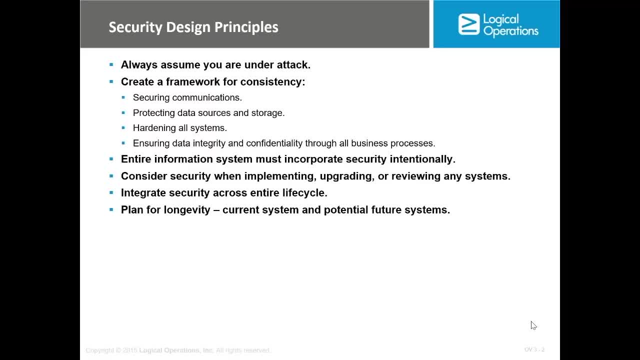 As you're going to notice or as you're going to learn in this platform, that we have a security engineering life cycle. So point is that you should, or you need, to consider security In all phases, as you can see in a few seconds. So security is not just during the designing or it's only during the implementation. 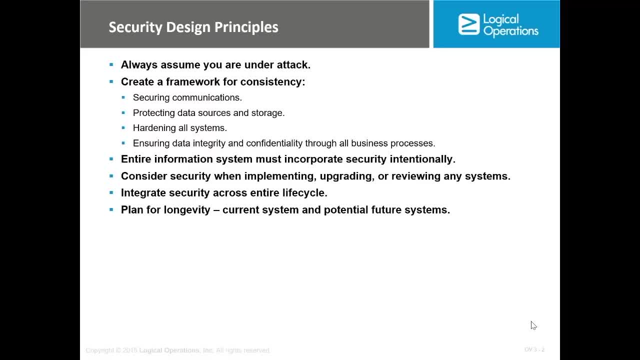 Or operation And so on. But you need to consider in all phases the security And in the next lecture we're going to introduce an excellent nest publication That will give you the major principle when it comes to security design. But before we start, you know there is some like security design principle, which is quite general. 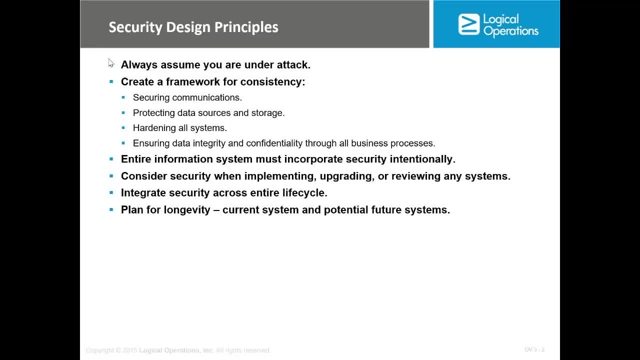 So always assume that you are Under attack, Do not like design your system in a basic way And then, according to the threats and according to the vulnerability, you start taking action. So, for instance, let's talk about patch management, which is an extremely important topic. 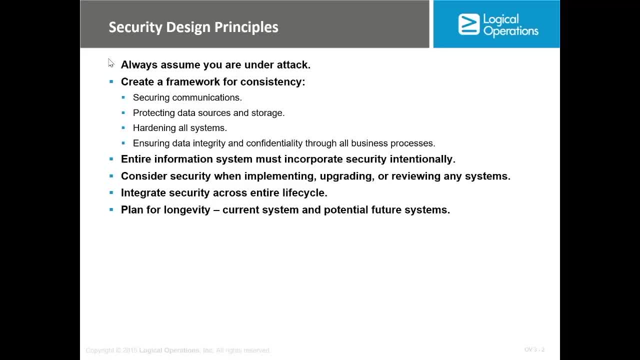 Should you manage all the update and patches to your system frequently, Or should I do that whenever a new threats has been introduced And they recommend specific Patch around it? You should be proactive in ways that this should be like regular or task to be done. 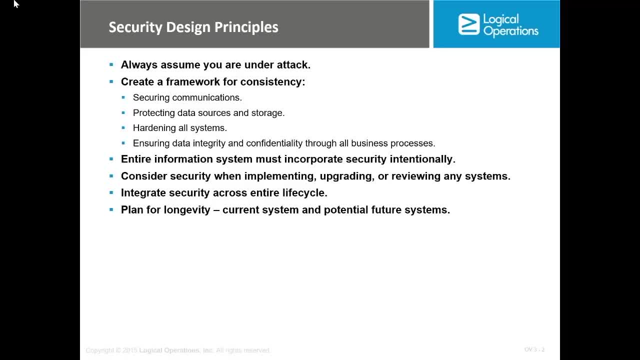 So you should always consider yourself under attack. You need to create a framework for consistency in a way that you need to secure the communication. You need to protect the storage resource. You need to hard in the system here Harding system in patching system. 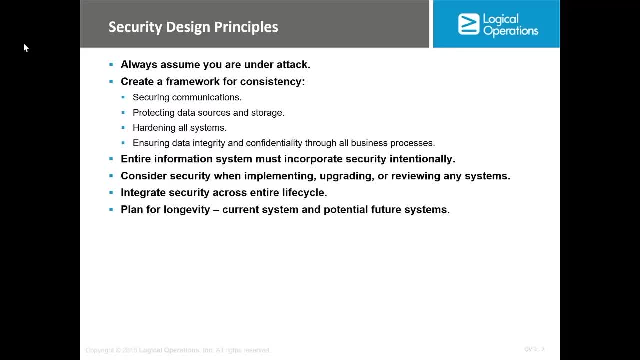 Managing the updates, Managing all application update, Ensure data integrity, confidentiality and, of course, availability. You should also ensure that the entire information system must be incomplete with security intentionally. So whatever information system that you are using, it should have security implemented in it. 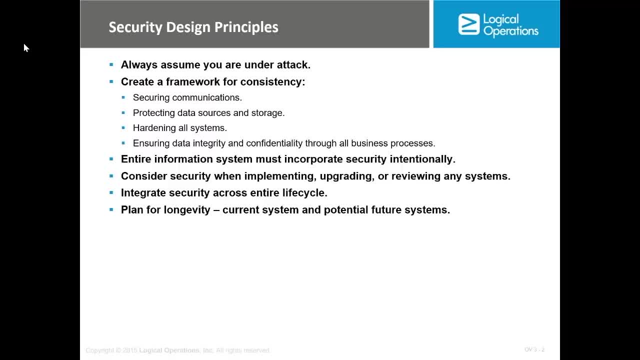 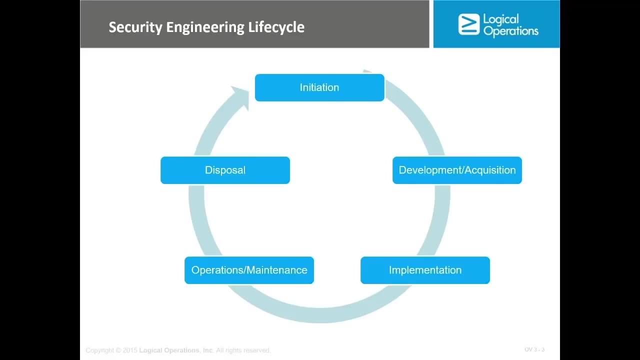 Security should be considered while Implementing, upgrading, reviewing During all phases. This is like a general design principle. but let's move to the security engineering life cycle. So, as you can see, we have five different phases in security engineering. It start by initiation. 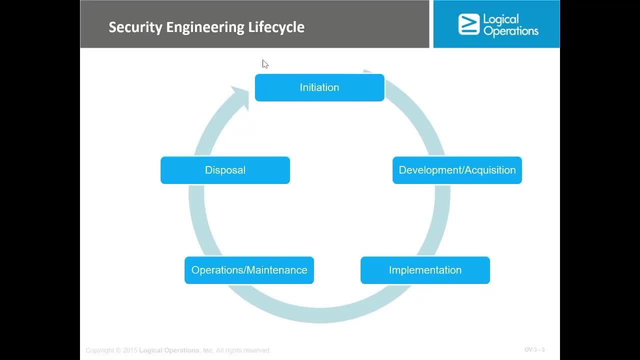 When you start the start deciding that you're going to implement security, Security in your organization- then development, An accusation, collecting information about what system do you have, What database you're going to use, all kind of applications that will be used in your business, and then implementation, and then operational and maintenance. 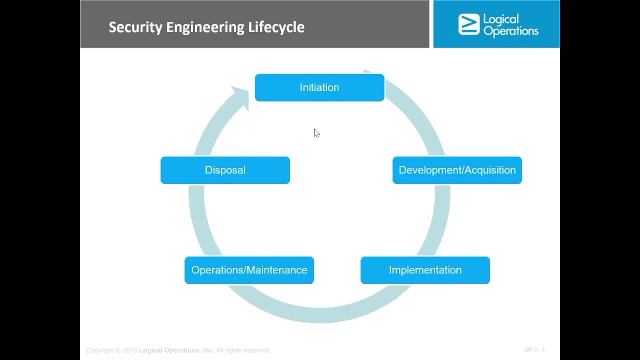 And finally disposal. We will go through them during this domain, but with different examples, so it will be quite clear. But So point here that this is considered the security engineering life cycle. Now let's see that in a like a checklist. 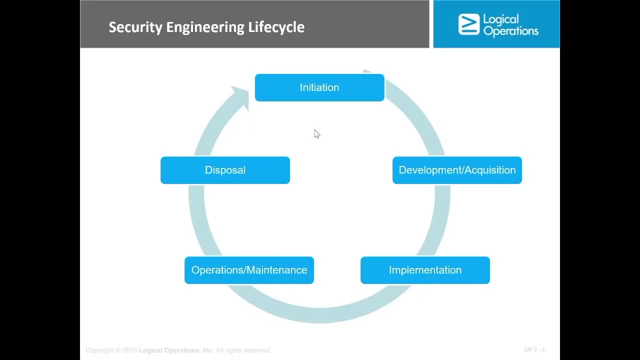 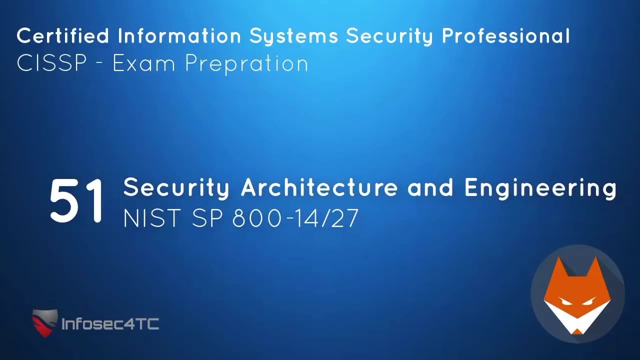 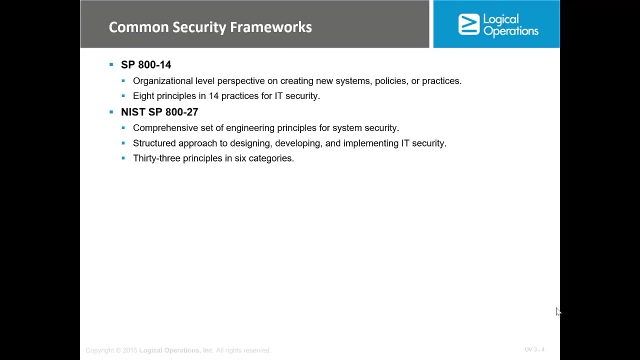 Or some best practice how security engineering should be implemented. I would like to refer you to two very important document That you should download from nest website. Nest, or National Institute for Standard and Technology, is a very important website in our course And you can download a lot of document from nest. 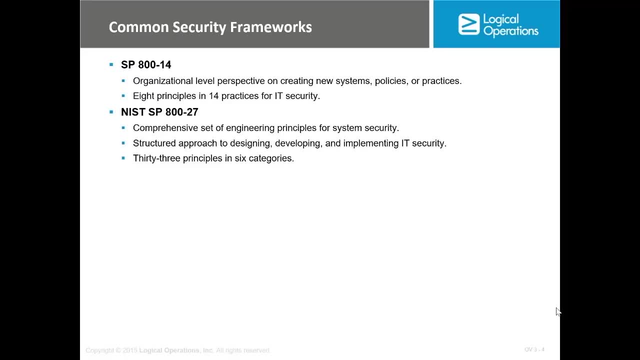 Sometimes they don't ask about the content of the document, but they may ask about the document name. Which nest special publication are covering common security framework? Which nest special publication Are related to risk assessment, log management and, by the end of this course, with the resources. 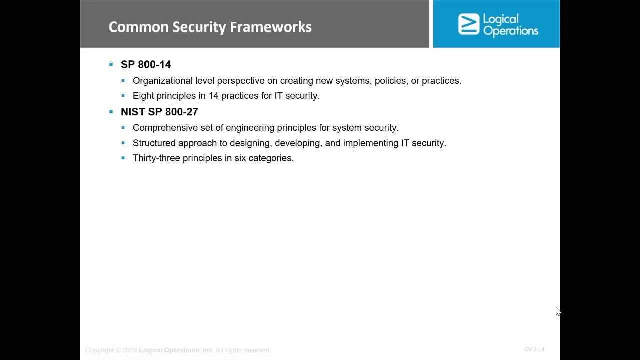 I'm going to give you a list of all the nest special publication numbers that you need to be aware of and what they are about. So here we're going to talk about two common security framework. We have nest special publication 814 and nest special publication 827.. 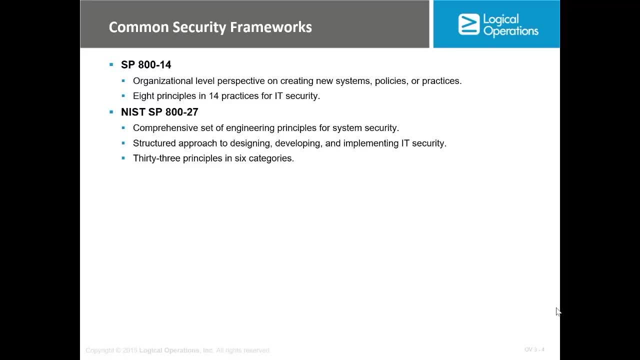 And we're going to Cover more the 827, because actually it's a big document. but you should expect a question about that inside the exam. It's all common sense. I mean, it's not really physics, but it's common sense. 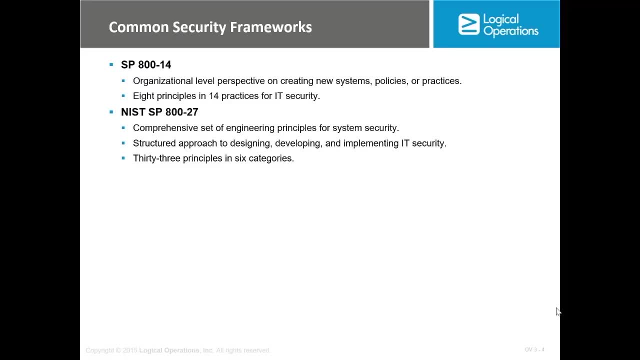 But still you need to go through them briefly and to understand what is the security framework according to nest. So nest special publication 814 are talking about the organization Organizational level perspective on creating a new system or policy or practice. What should be considered when you implement a new system or a policy or procedures? 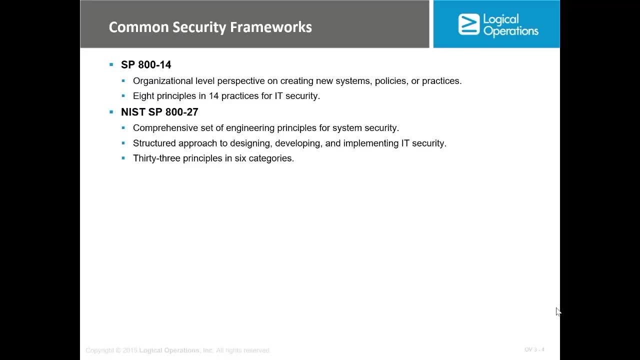 And there is eight principle in 14 practice for IT security, But the major one is the nest, special publication 827.. And this one is giving like a set of engineering principle for system security And it's giving a structured approach for designing, developing and implementing IT security. 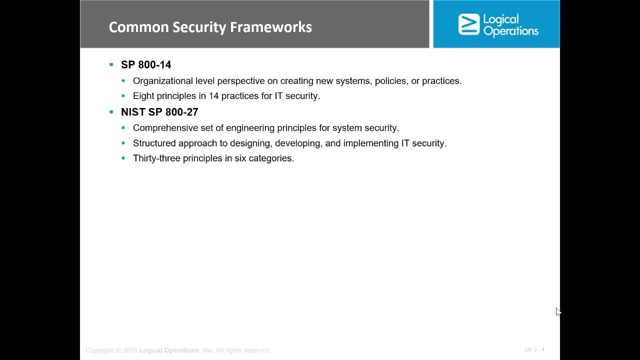 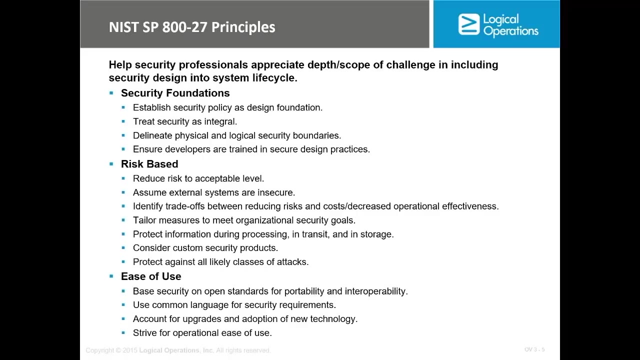 which map to the security engineering life cycle. It has 33 principle in six categories. Let's have an idea about it. Nest 827 principle. Now I will go in general about them, but I will let you read them And take notes about whatever like you need to memorize in the nest 827. 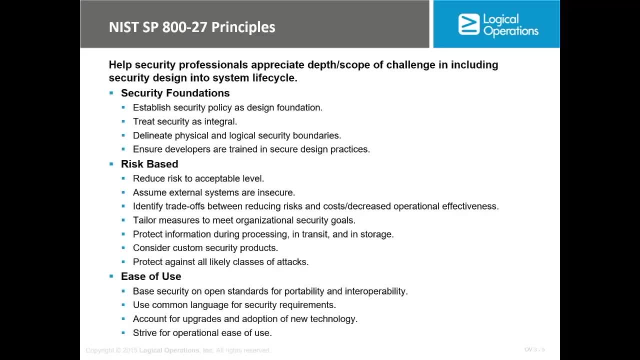 So first category is about security foundation. Now, in this category is focusing about security, is not just the technical security. And this is quite important And I have been saying that since the start of this course, that when we are talking about security, we are not just talking about the technical security. 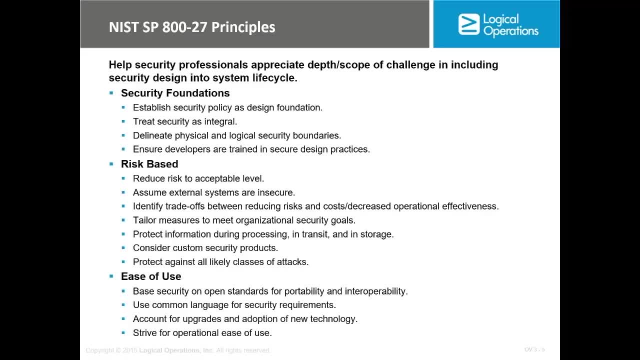 If you have a good technical security but you don't have a physical security. It may lead to the same result If you have a technical security and physical security but you don't have an administrator security- same issue. By the way, logical security are referring to the IT security. 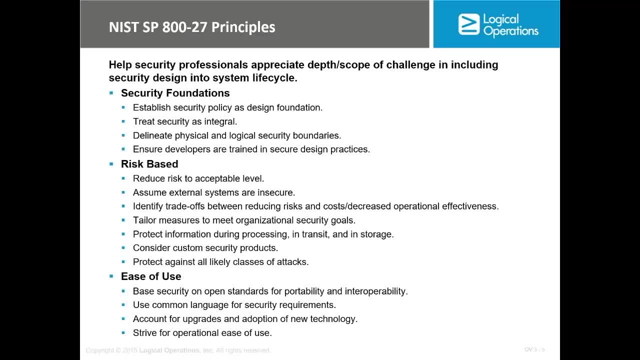 So sometimes, when they ask you about logical security, they meant IT security. So here is talking about that. the foundation of security should be not just on the logical or technical part, but on the physical and on the administrative as well At the beginning- and we already covered that in the previous section- which is you need to establish security policy as design foundation. 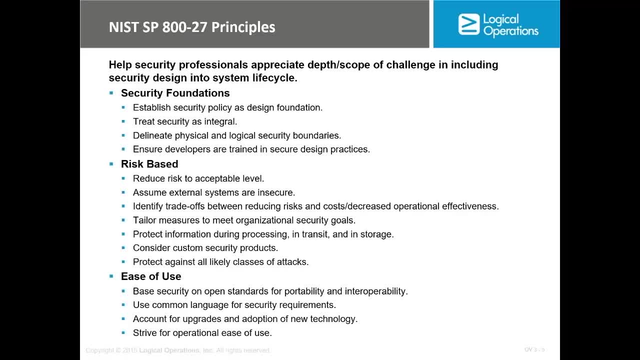 The document you know are explaining each point, but I'm going through the critical ones, ones that you may find inside, As example. second category is about risk, risk based, and we already talk about the importance of risk and that the security implementation are initiated by the asset value and the risk. 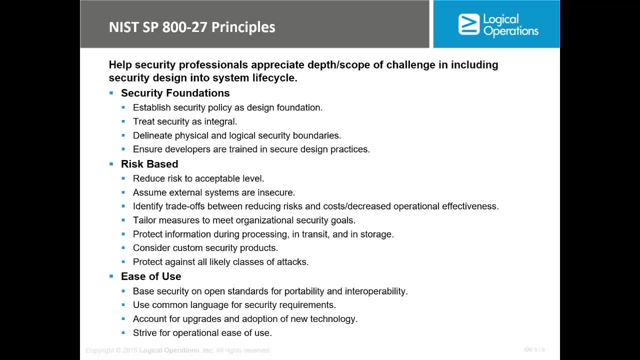 So the risk actually is one of the big challenge in any business, For instance you. first you need to understand that we cannot eliminate risk. We will always have a risk, Which we call the residual risk. So whatever you are doing, you are reducing the risk, but you cannot reach zero risk. 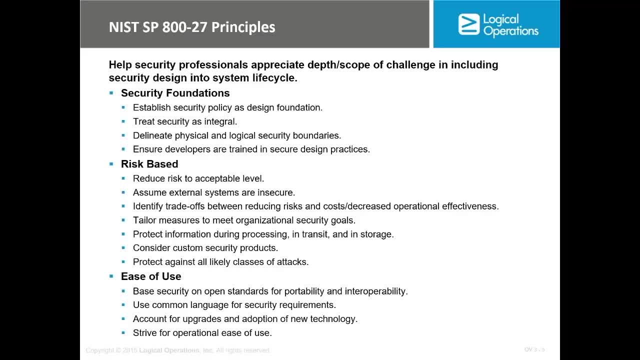 But sometimes- and this is quite important point, And this is the area where you can find questions inside the exam- We have something called the risk acceptance list. In a way, that assumes that you have a system. it's a legacy system, a very old system that your company depend on. but this old system, 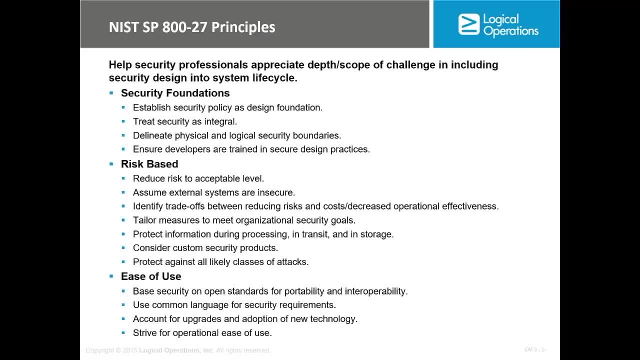 Can only work on an old operating system. So it can only work on Windows Server 2003 and we saw that in many company And, as you may know, Windows Server 2003 are a very, very vulnerable operating system. So your recommendation as security professional is to upgrade the Windows Server 2003 to the latest version, 2012 or 2016,. but they cannot do that. 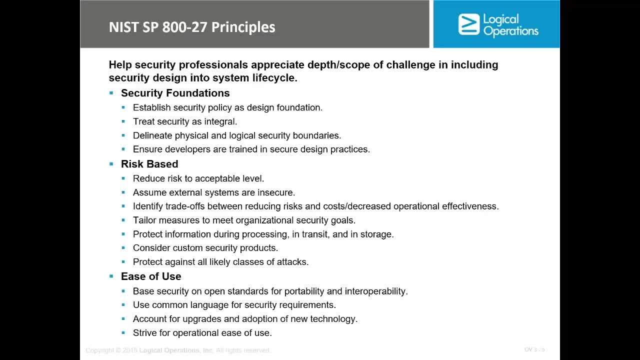 Because, if they do that, they were not able to run the system, which is very critical to the business. Now, what should you do in this case? In this case, Because we cannot enforce to stop the business because of security, but also we need to take some like countermeasure. 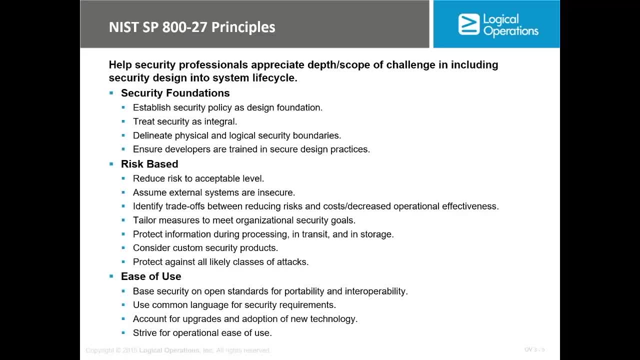 Now there is a technical solution for that, but this will be discussed in the network domain. But sometimes, what if you don't have a solution? You just need to accept the risk, the same way it is in this case if the business or the management 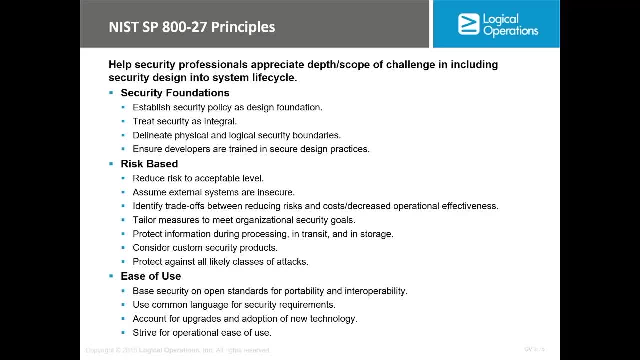 Did not accept. due to the business requirement to change some setting or to upgrade the operating system, You need to get from them risk acceptable acceptance list. So usually you have a form called the risk acceptance list. risk acceptance list in a way that if you are doing risk assessment, 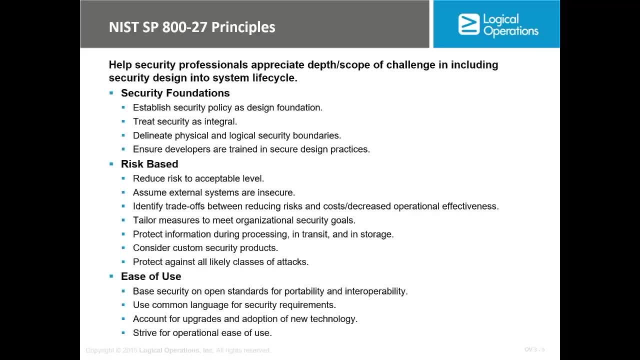 And you find some risk and you suggested some mitigation. But due to the business requirement or you due to some technology limitation, the management decided we will not do anything about it. What you going to do about it You cannot enforce right, but you can let the management take responsibility for that. 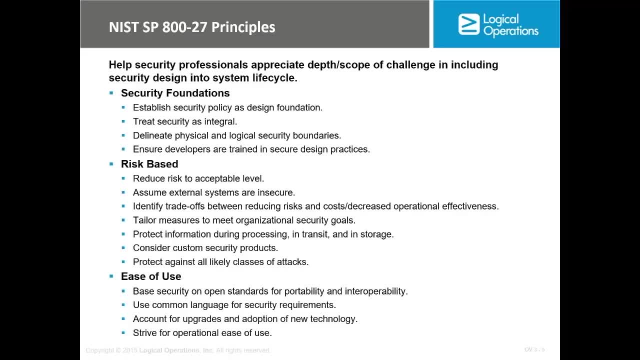 So you said, okay, you're going to need to keep those old operating system. You know that there is a risk for that. I have to clear my site. So please sign this Risk acceptance list that you are aware of the risk and you are accepting that because, after all, he's the one responsible for all security in there. 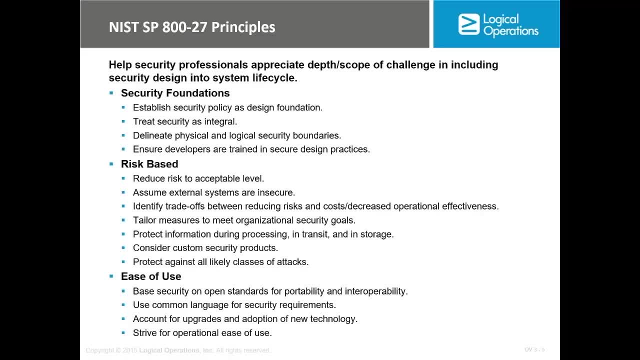 But you cannot keep it like verbal, like management request, because if something wrong happened, you know most probably he will deny that he suggested anything or he going to say that I don't know about technical stuff but we hired someone to deal with it. 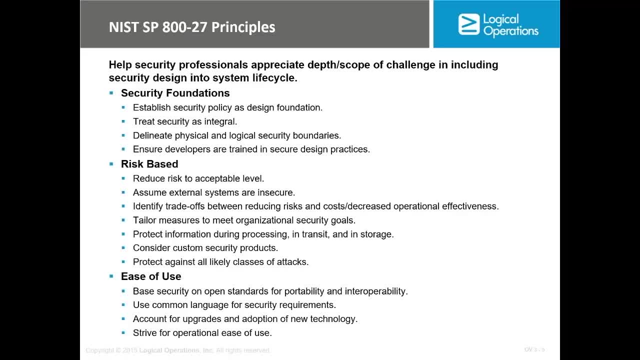 So you don't want to be in this situation. So this is very, very important point, which is the risk acceptance list. That is a document usually signed by management, saying that we accept the risk because of the business need, But according to nest 827, you need to reduce this risk acceptance in a way that you should not everything that mentioned and management disapprove, approve. 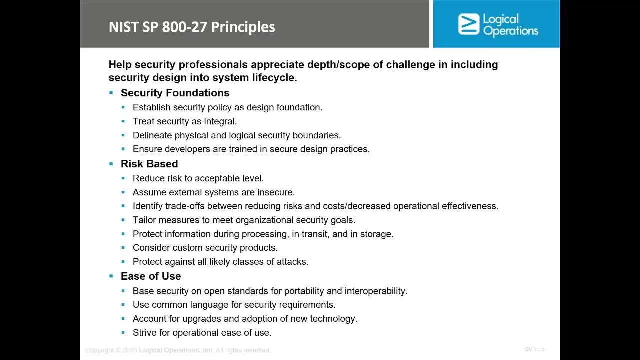 Okay, you should write it down in the risk acceptance list. It's not done this way. You need to try to convince the management, and when you reach to a dead end, then You need to let him sign the risk acceptance list. So it's a very, very important point. 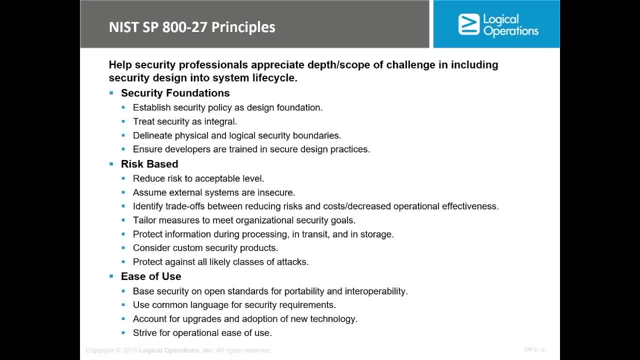 The second point also, it's important in ways that you should always assume that the external system are unsecure. Sometimes we are integrating our system with some third-party system, like some payment gateway or any other system, So we have our own system and then we are integrating this system. 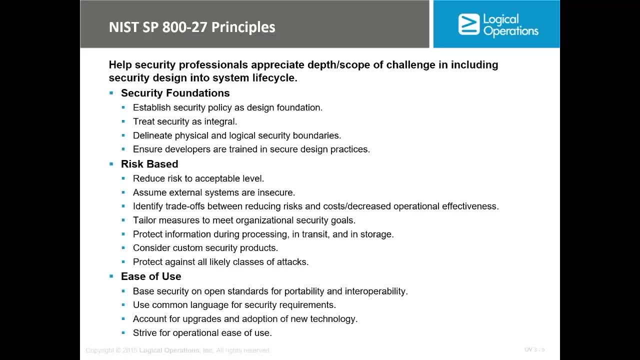 We use another system. So I should not say that, Yes, those people are very, very secure. I will not consider any security problem from their side. Let me work on my side. No, you have to make sure. whatever system you are integrated with, you have to assume that is not secure and you have to check all the control and you have to communicate with them and to see what security are in place. 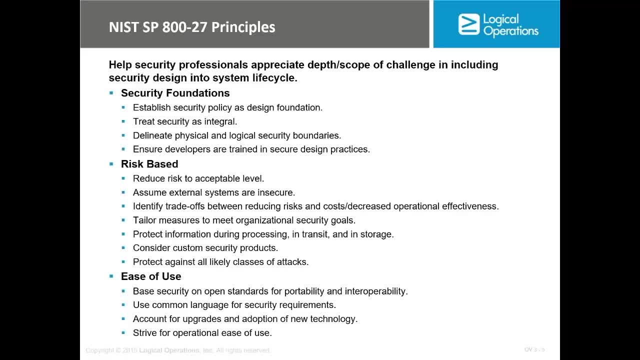 So always assumes that the external system are unsecure. Do not take anything for granted. Yes, this is a big name, So what could go wrong? I'm going to integrate my system with their side. No, no, you have to check what controls they are using, and so on. 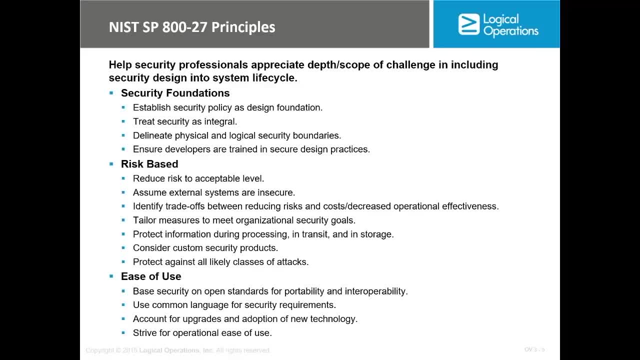 Cost effective hundred percent. You get the questions that about that inside the exam. It's not about getting the latest and greatest technology and secure. It's about the effectiveness, of course, And we already saw some example in the risk Assessment part. So before deciding how much you can spend on security, you need to decide how much it was. 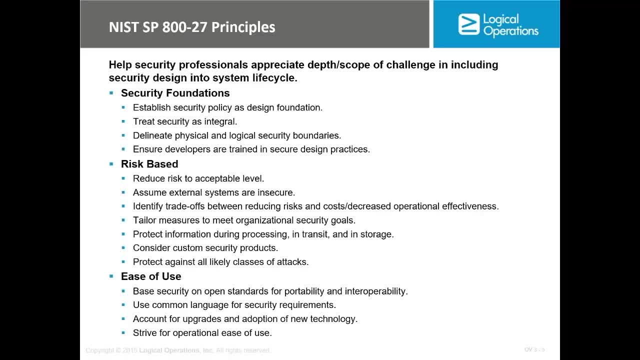 So this is quite important. So usually you can get question about that inside the example, but it would be in the risk part. Other point which is easy to use: that you know whatever standard you are following, whatever technology are for, do not get the complicated one. 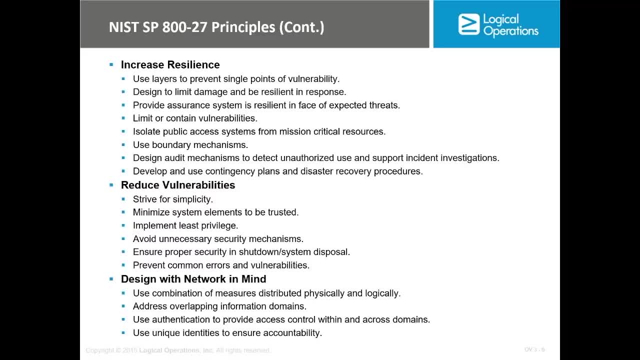 So, you know, try to make things easy to use, Increase resilient, reduce vulnerability. We're going to talk about this topic. Vulnerability is a very, very important topic, which is, you know, the vulnerability assessment, as that need to be done frequently, once every six months, for instance, and most of the problem related or vulnerability raised would be need to be solved by patch management. 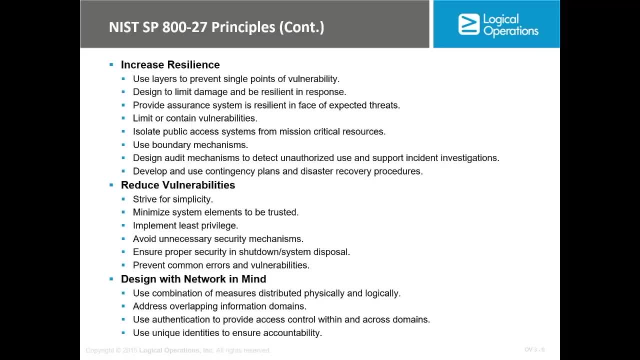 By updating the system, by retiring some old operating system. So it's it's a must task doing a vulnerability assessment frequently And we're going to see that later on- how we are doing vulnerability assessment And what is the purpose for that And what is the difference between vulnerability assessment and penetration testing. 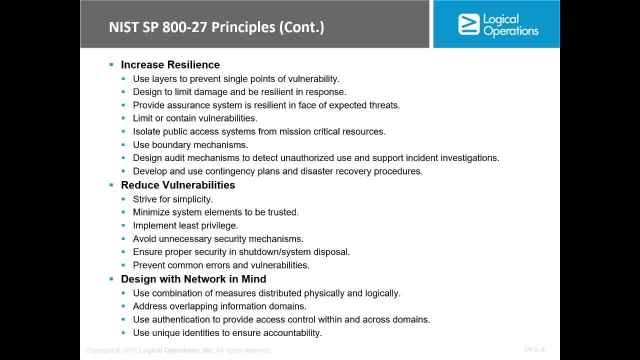 Okay, design with a network in mind, in a sense that, as we keep saying, security is not just technical security or logic Security. security is technical, logical and administrative. So those are some men of the main point in the next special publication, but I strongly recommend that you go through it and highlight some of the point printed and highlight some of the point because it's rich area for questions. 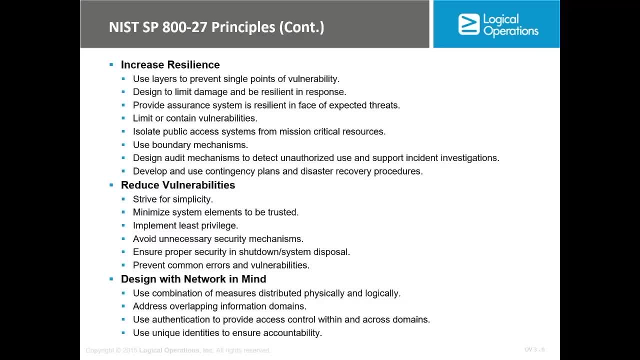 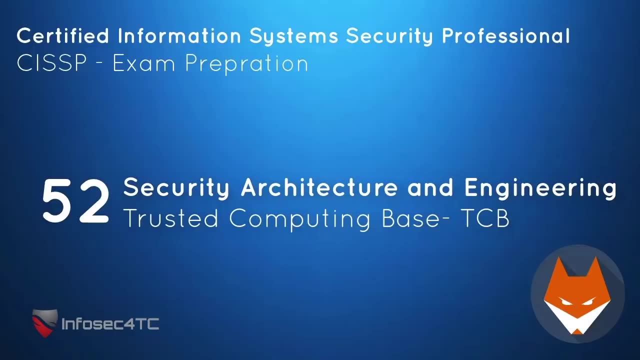 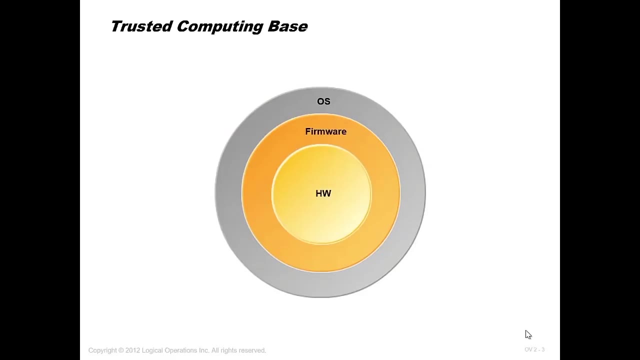 And, as I told you, this is maybe seem straightforward point, but when you're going to see them inside the exam, as you can see in the exam practice question, You can see house again Manipulate those point. So in this lecture will be defining a very important definition, which is the TCB or trusted computer based. if you remember from the previous lecture, 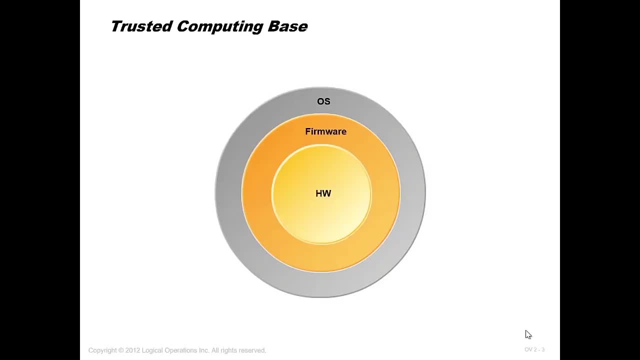 I told you that what we are looking for- trusted computer based. what we are looking for in this domain, It's how can we Measure the security in our system And we'll focus on the computer or not focus on the network. right now, My focus in the computer and I give you an example. 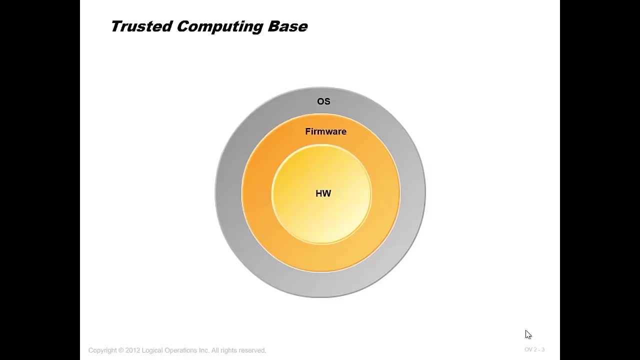 If you are buying some machine. how do you know that IBM machine with this kind of processor and this kind of hard drive How secure they are right? You cannot take a decision based on other people opinion. You need to have some standard to follow now, from now on, when we will be talking about system on computer. 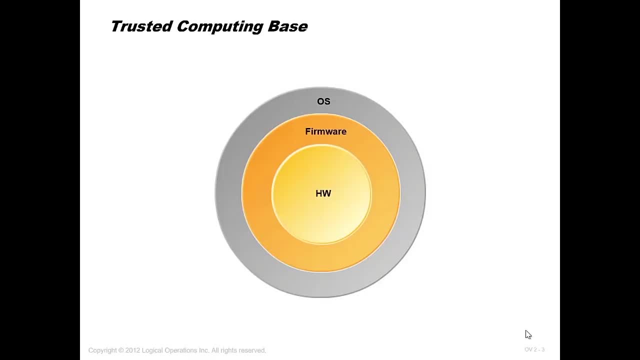 We're going to give them another name, Which is the trusted computer based trusted computing base. It's three different devices inside the system: The hardware, the framework and the operating system. So when we are evaluating now, we will not evaluate just the hardware. 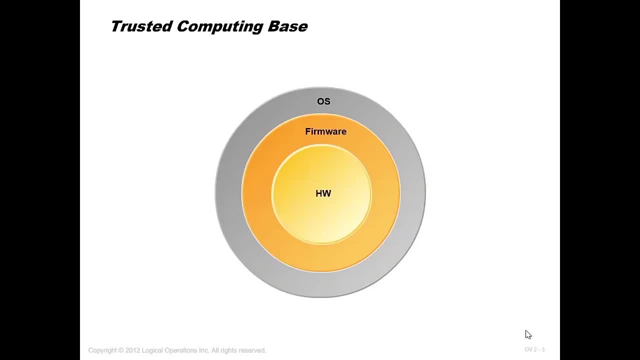 We will not evaluate the framework Only. framework is the software that installed on hardware, Like, for instance, the room. the room has a BIOS. This is software to manage the BIOS. This is called the framework And the operating system. So evaluating will not be based only on hardware, will not be with the owner and framework and will not be based on operating system. 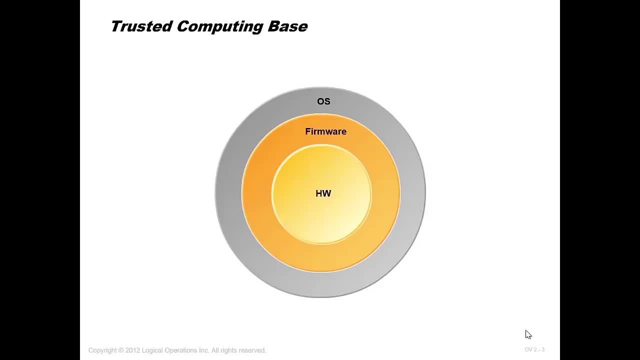 We will be evaluating our system based on those three of them. Instead of saying hardware and framework operating system, we're going to name them trusted computing base. So this is the evaluation areas that we will be talking about: the trusted computer based, or the abbreviation which will be the TCP. 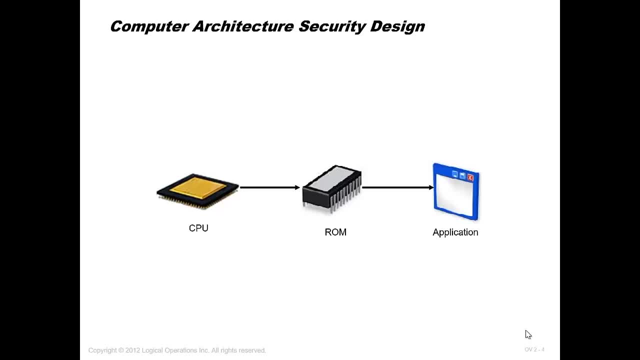 How can we evaluate the TCP? now We'll be talking about A little bit about the architecture of a computer, So let's talk about the hardware architecture In hardware. I'm going to talk about the processor and we will be talking about the storage and 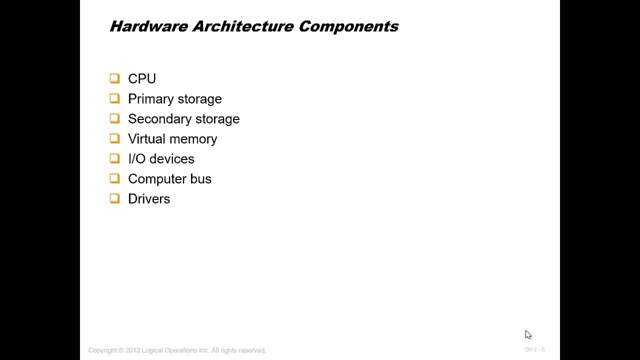 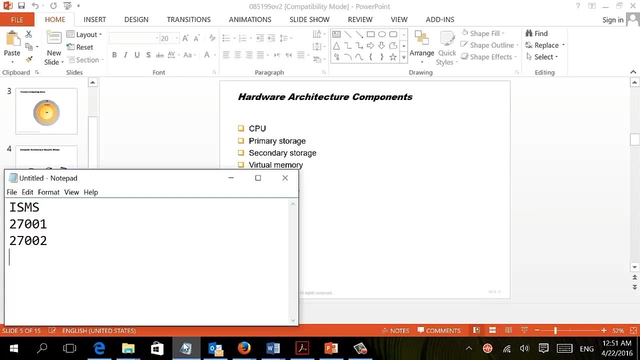 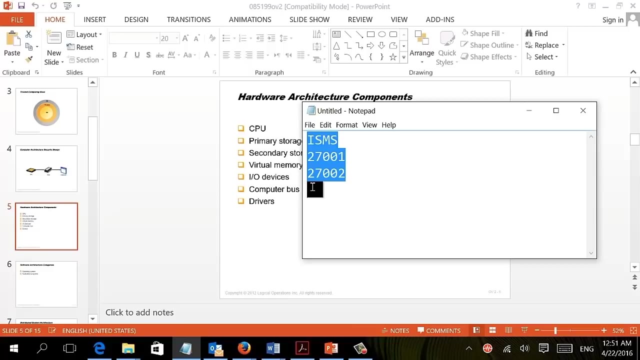 Some other definition. Some of them will seem very basic, but it's okay. Now let's talk about the CPU first. And CPU, it's a main Unit inside the computer where It's doing all of the processor. CPU it's divided logically to three different of three different. 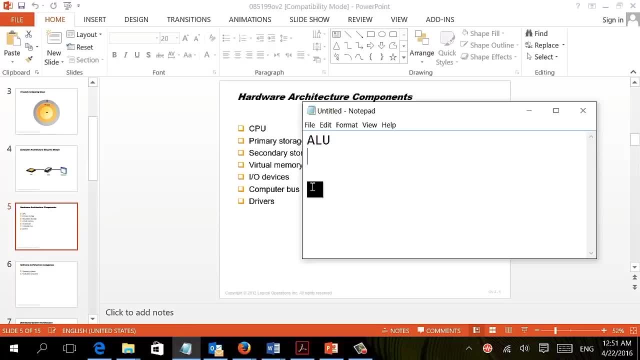 Part CPU, It's ALU, or as an arithmetic logic unit, MU, Which is memory unit. and see you, Those are the component of the CPU. The arithmetic logic unit is the one That doing all the processing is the brain. He's the one that analyze and calculate and do everything. the MU. 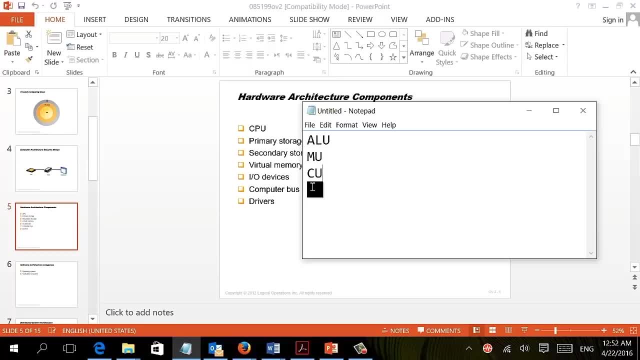 It's a memory unit and this is a part of the processor where it's used as a memory. You know, when you go to buy a computer and you're going to tell you that this computer has L1 hash- I'm sorry, L1 cache this amount. 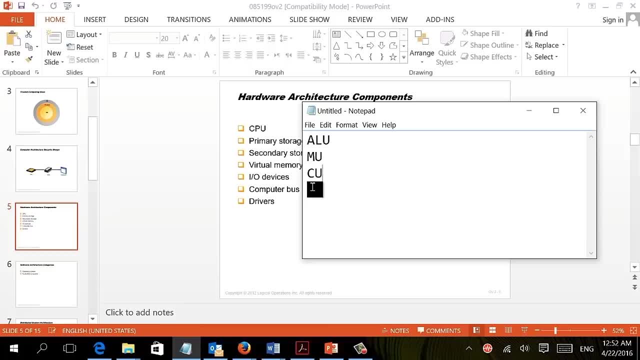 This is the amount of memory inside the processor, and This part is very, very fast. I mean, this is the most fast part of memory inside your system. Then we have the CU control unit When you run any program. let me show you some small example. 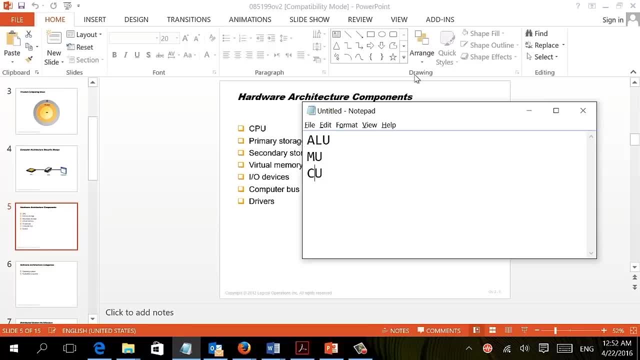 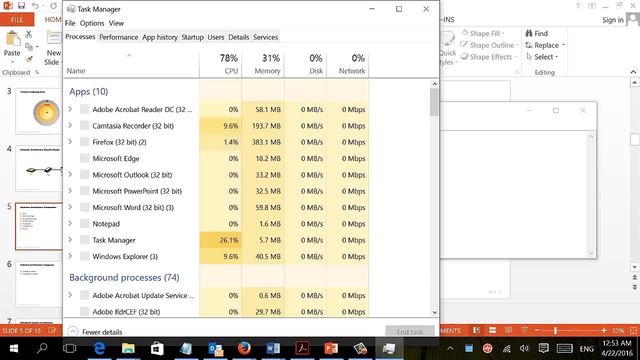 When you run any small program, any program, this program- Let's assume that you are running Excel or world or anything- This program will launch some process. So if we open the task manager And we go to details, you'll see that. 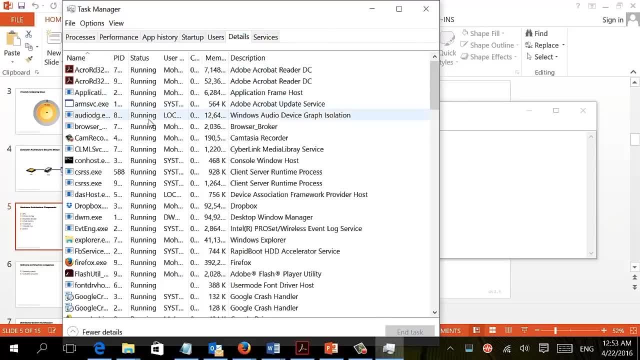 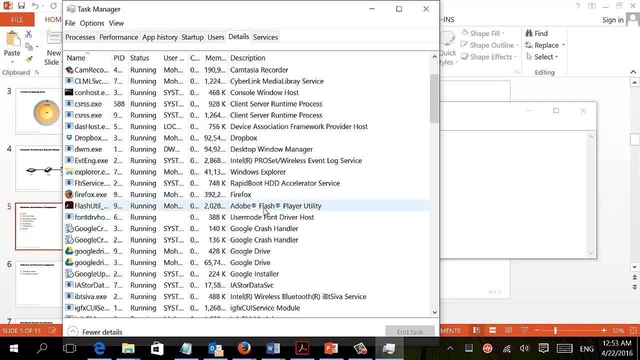 Each program I run, it's running some process. So Adobe, for instance, has to process a word, Maybe have more process, and each one of those process will launch with him Something called threats, which is the comment itself. So each process has many threats. 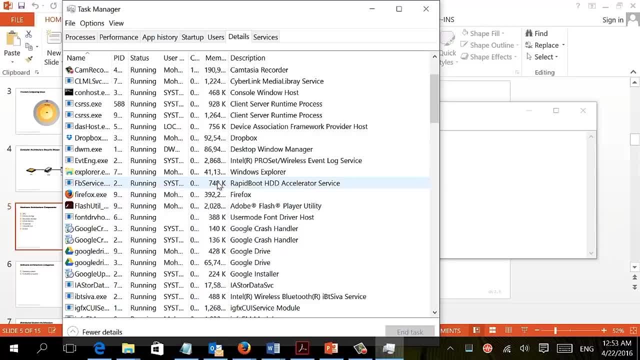 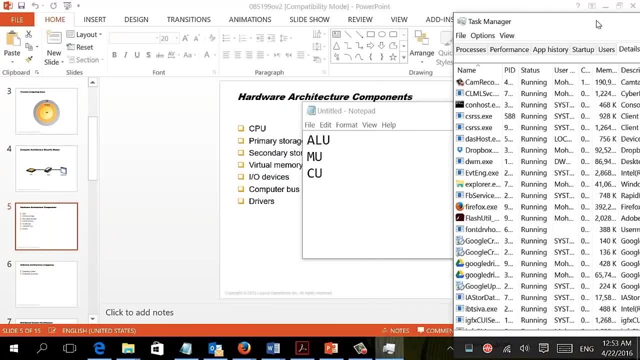 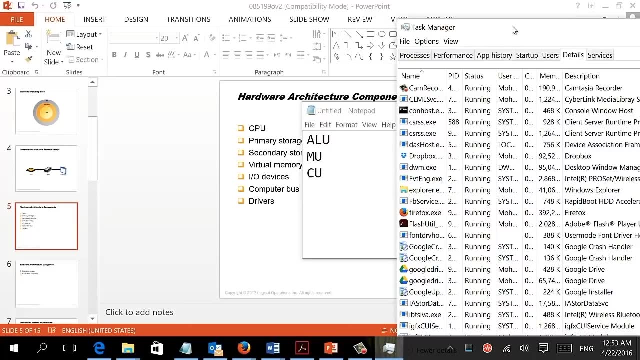 So each application has many process and each process has many threats, And Those threats will be sent to the CPU to be to get executed. The processor can only execute one thread per time. Maybe it seems slow, but this is how it go. 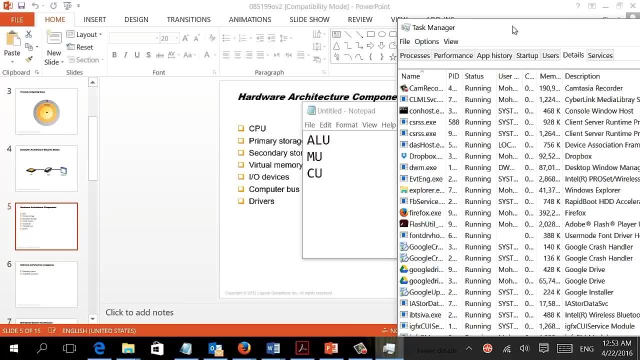 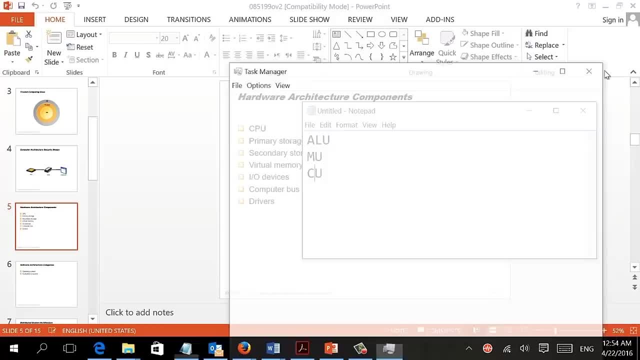 And who's responsible to do that? Who is responsible to send one thread per other, And he will not send two thread together. You have to set one by one until it get executed and he send another one. This is the control unit. This is what the control unit is doing. 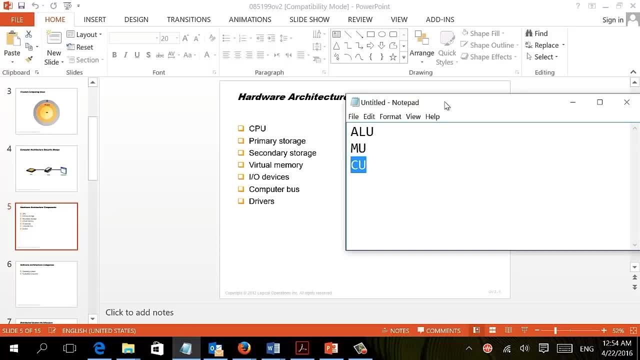 Okay, so control unit are managing the Thread. that is a part of the process, That is a part of the program going to the ALU to be executed. Now we'll be talking about primary storage- It's your hard drive- and secondary storage. 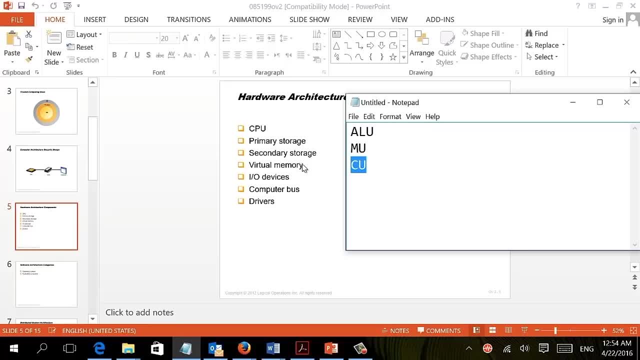 Is- I'm sorry, Yeah- the memory. I need to talk about virtual memory. I'm need to talk about memory in general. Okay, how many type of memory do we have? Okay, we have L1.. Cache- This is the first type of memory- and L1. 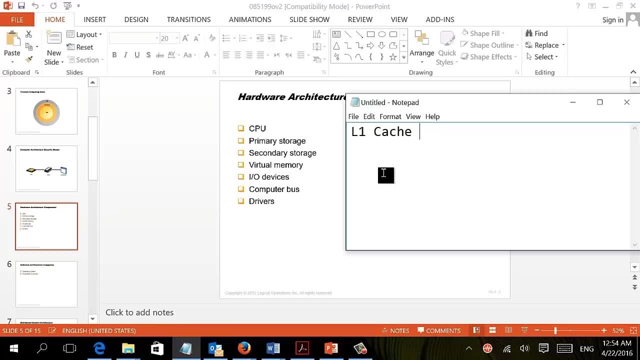 Cache is a very, very High-speed memory, So and usually located on the processor itself, the MU. So this is a very high-speed memory and it's located on memory. We have the L2 cache, Which is also very high speed, except it's lower than inward cache. 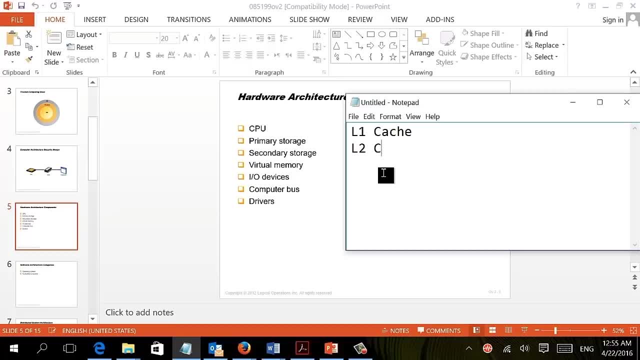 And this is will be located on the motherboard itself Cache, and we have the RAM, which is a slower one. Okay, Those are the amount of memory Now we have. another concept is called the virtual memory, VM And the virtual memory. do not get confused that with virtual machine. 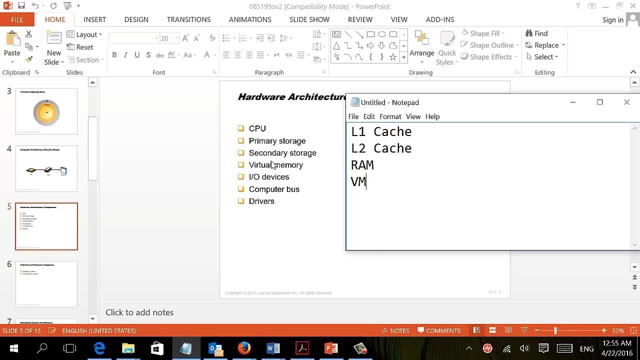 I'm talking about virtual memory. The virtual memory are a part of hard drives that you can are taking and it will be Acting as a memory. So you can take a part of hard drive. Let me show it to you. If we right click on, 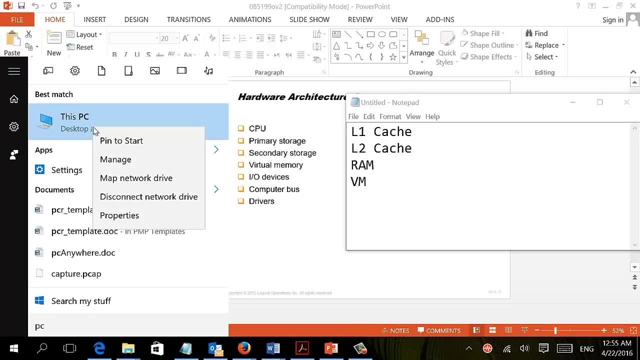 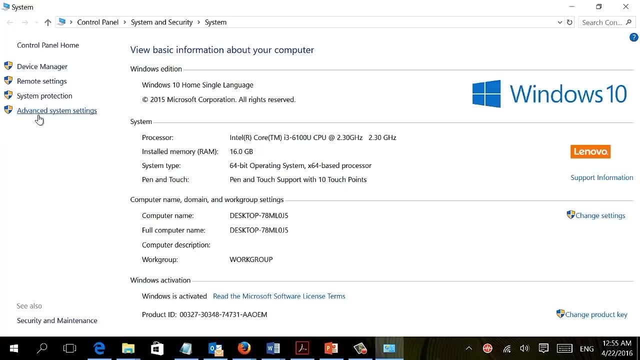 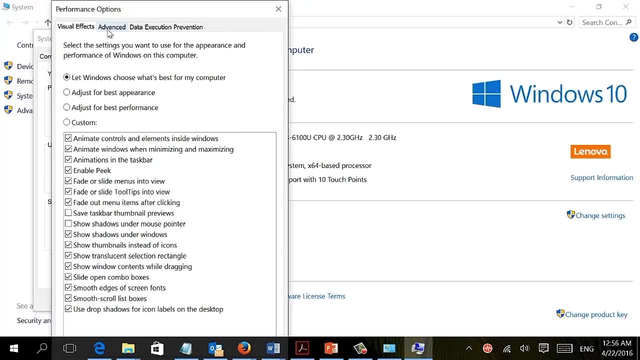 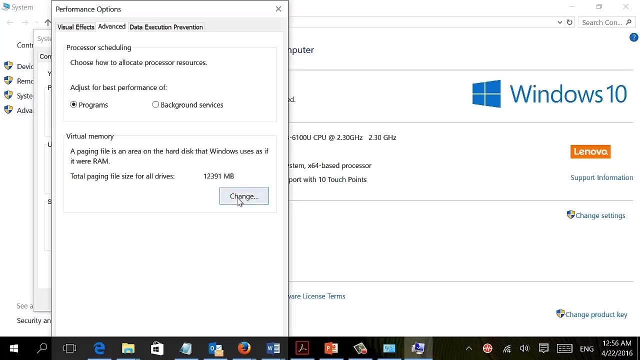 PC, You right click and you go to property, because you can change from here as well. And in property let's go to advanced setting. Should be in performance. Here you go setting and Here you go The virtual memory. the amount right now is that much and you can change it. 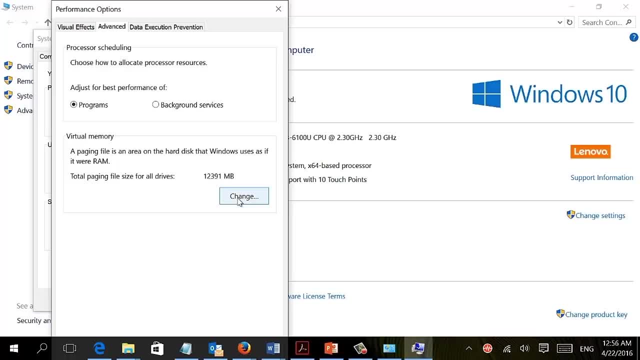 Now the question is If I take a part of her hard drive As a virtual memory. I mean it's acting as a memory. That's mean I can increase the memory of my computer without adding memory. So what I can get a computer with 2 GB and take from the hard drive, because the hard drive is usually much bigger than. 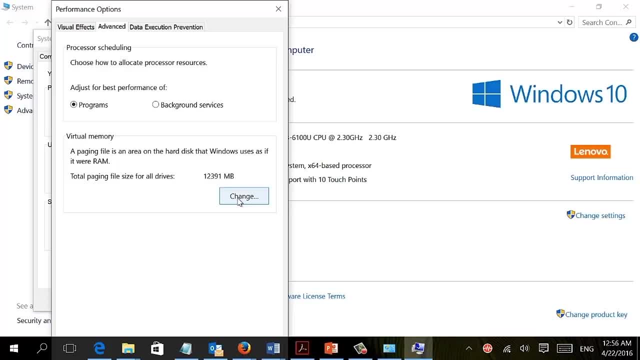 The memory so I can take whatever amount and my computer It will be extremely fast. Actually, this is not right, because the virtual memory It's not really a virtual memory, It's not really added to the hard disk, to the ram, because the point is there is a big difference in speed between the ram and the hard drive. 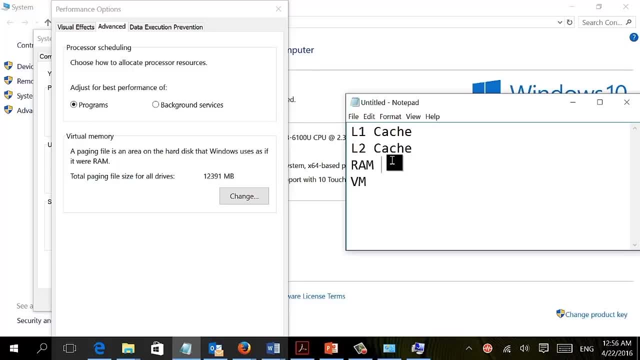 So ram. usually the speed is with nanosecond. This means 1 and 9- 0.. While the hard Drive speed is with millisecond, Mean 1 and 3- 0. Millisecond. Okay, so there is a very, very big difference in speed. 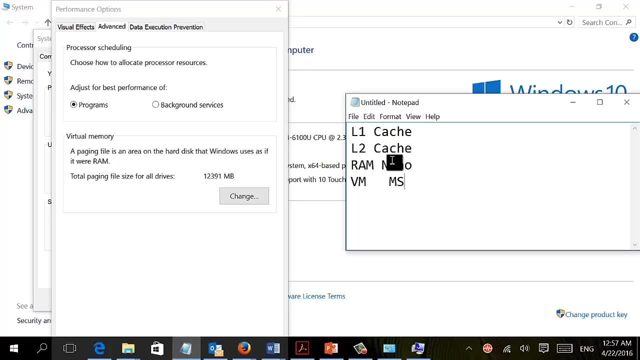 Don't forget that, Please. ram is with nanosecond, while virtual memory is, or hard drive is, memory second. But what will happen is when you take a virtual memory from your hard drive, it will act like a temporary storage. So, for instance, 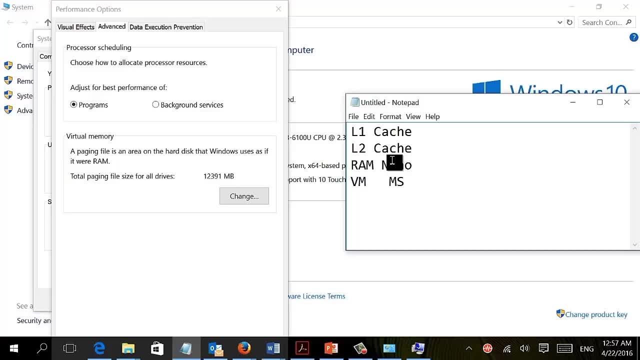 You are open a lot of program and now we need to open another program. inside the memory You don't have any space. He will check inside the ram What is the program that is less used and he will take that inside the virtual memory. 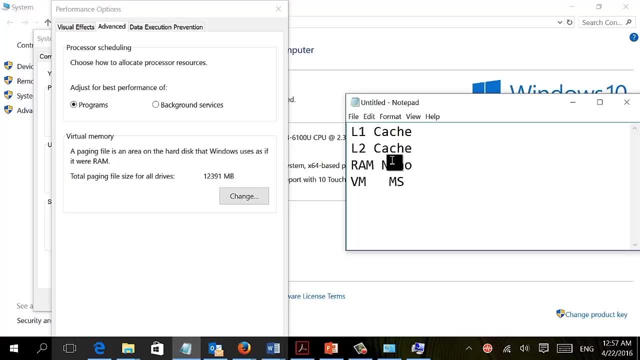 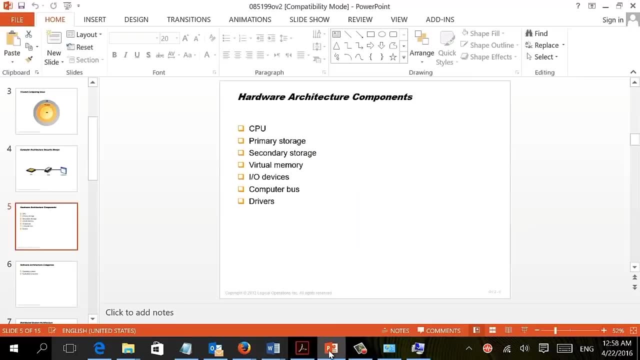 So it's like a storage between the hard drive and the ram. So don't get confused about that. and you know, don't let this question trick you. We have the input output device, things like keyboard Mouse, you know, any input output. 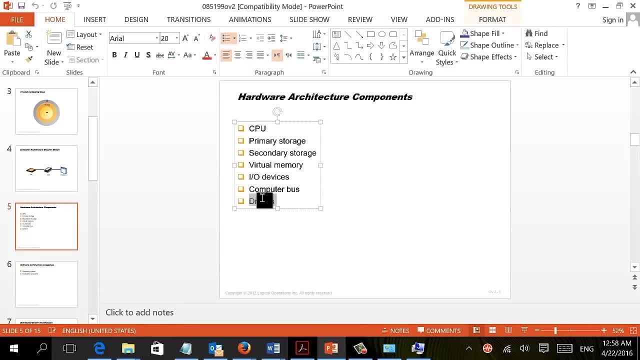 We have the driver, which is software that identifies the hardware to the computer, and we have the computer bus, which is just some passes inside the computer. You know we have the 32 by a bit and we have the 64. It's how many buses or how many paths of information are inside this computer. 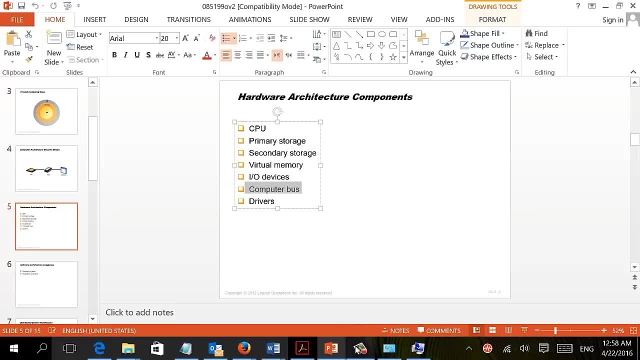 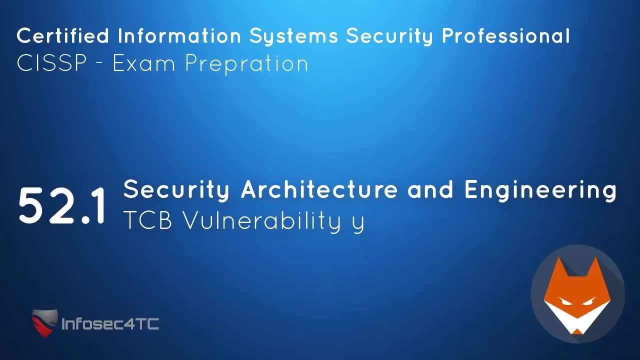 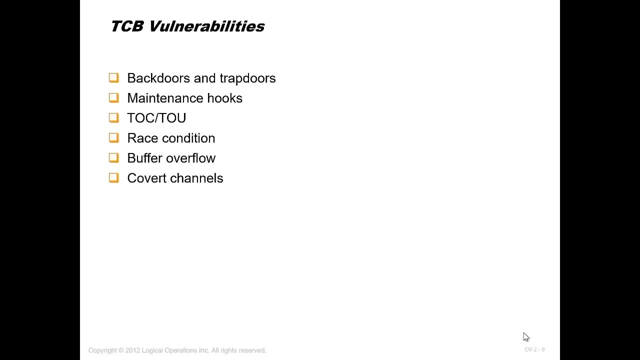 So those are the hardware architectures that you need to be aware of As we agree on the beginning of this course. a very important area in each domain that you should be aware and some good amount of question will be coming from there is the vulnerabilities and attack. 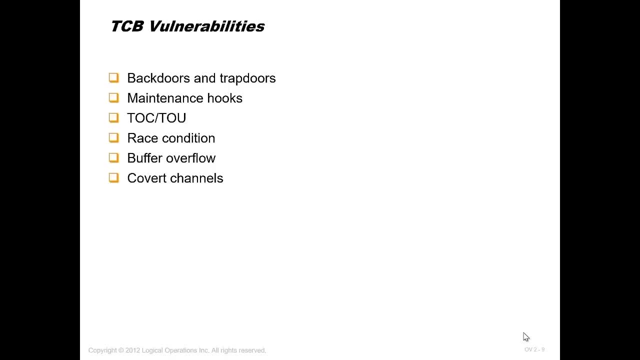 So whenever we are talking about the domain access control, physical network, anything- you're going to find that there is a slide that Talk about the vulnerability and the attacks And you should be aware of the definition of the attack and some attack of are quite clear. 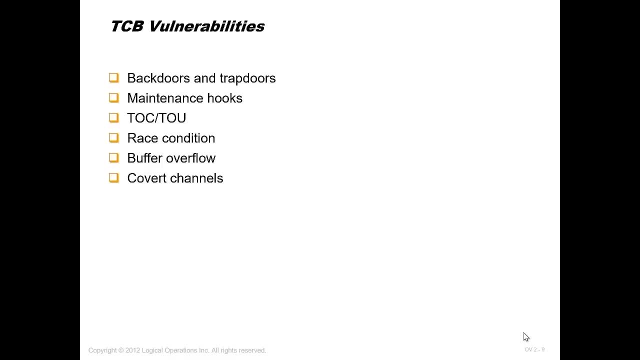 But some attacks. you may need to write down some like definition or some keyword about this attack. So now we'll be talking about the TCP vulnerability. Now let me remind you What is the TCP: the trusted computer base, which includes the hardware, the framework and the operating system. 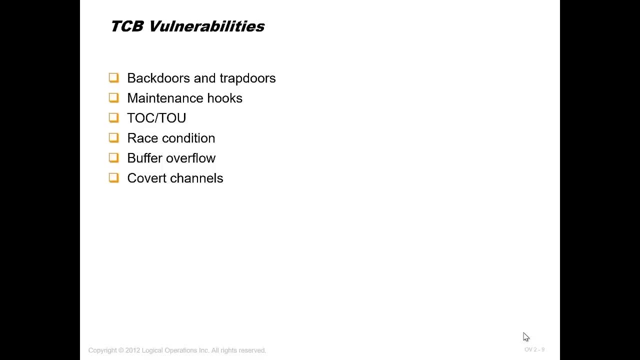 The good thing about attacks that some of the attack will be repeated in most of the domain, which will make things more easy, But some of the attack will be new. So, for instance, back door and trap door. We are aware of that back door, which is things like software that open a back door on a system like Trojan, or this kind of malicious software that allows someone to connect hiddenly. 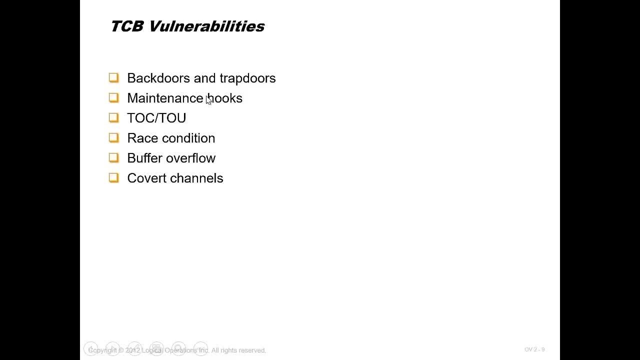 This is called bread, or do you remember what is a maintenance hook? Because it's very, very important. maintenance hook act as a back door, But actually it has been implemented for a good use and has been misused. So some developers and some programmers, when they create a program for any organization, 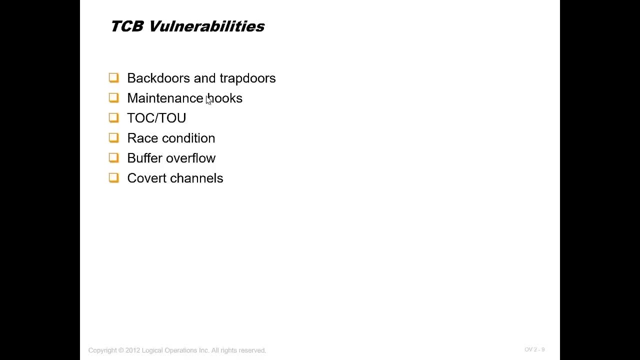 They know that after delivering this program, a lot of support will be required, especially at the beginning, as that people are not aware of the program, problems start showing up and so on. So, developers, to make things More easy for him, He will open a back door that allow him to connect remotely to the system and do whatever support is needed. 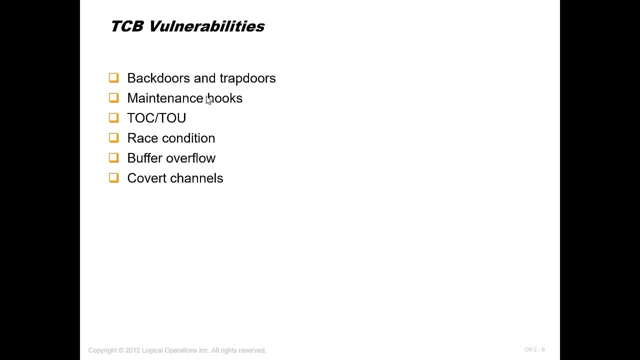 But sometimes they are doing that without taking a permission from the business. So I'm doing a program or an application for any organization, I will open a maintenance hook and whenever they call me for support, instead of moving there and leaving my job and everything, I can remotely login from my location and try to solve this problem. 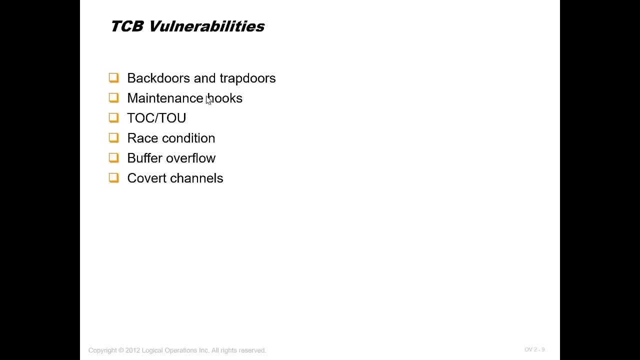 It look fine But actually it Can be misused. So if anyone else will be a or any malicious hacker will be aware of this maintenance hook or this back door, He will try to compromise it and try to get access to the system. 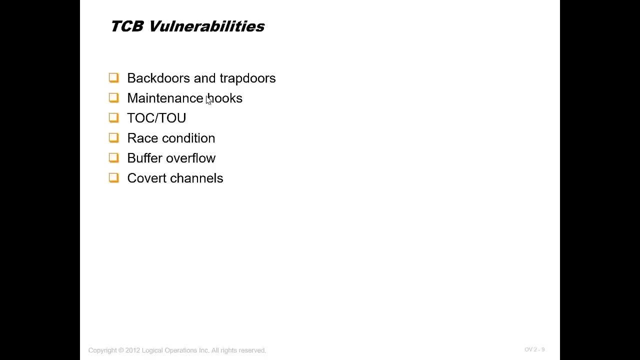 That's why we always say that when you do an application, when you are getting a developer developer to do an application for your organization, You have to let him sign that he didn't left any maintenance hook inside the application. This is very important from a security perspective. 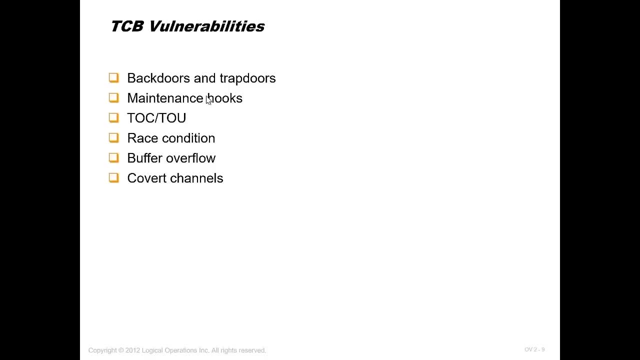 Because We agree. Maybe it has been used for a good reason, but it has been misused as well. We have the TOC, TOU and I don't recall this is stand for what, but this is an attack that try to get advantage from the traffic going between the client and the back end server. 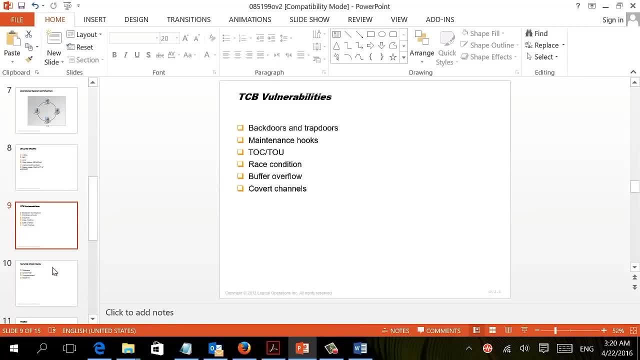 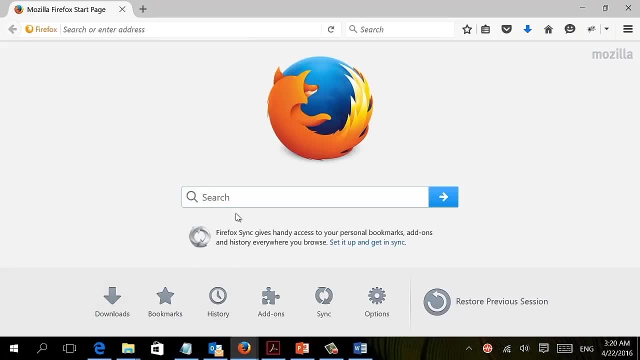 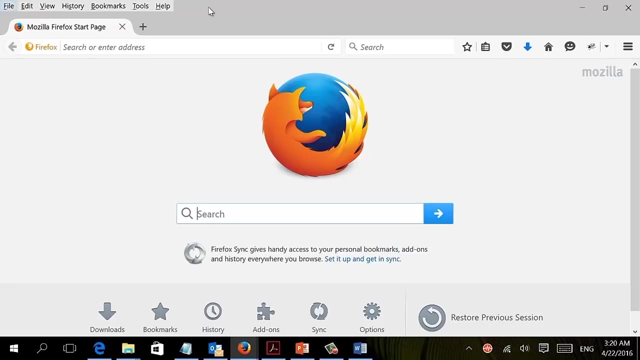 Let me show you a small example. So if we open Firefox for instant Firefox, It has a very nice feature called- sometimes- actually it's nice for malicious hacker and nice for people who's testing as well- It's called tempered data. So if I open the menu and you go to tools- actually it's an add-on that you have to install it for free and you're going to find tempered data. 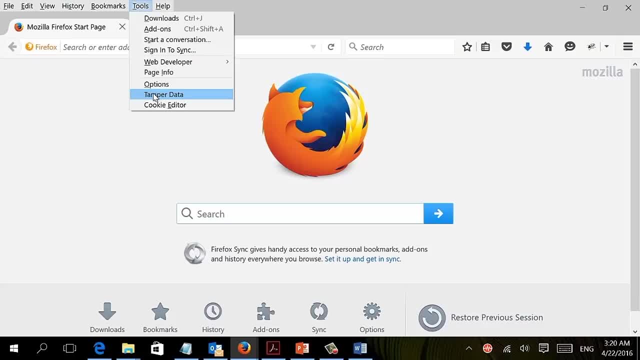 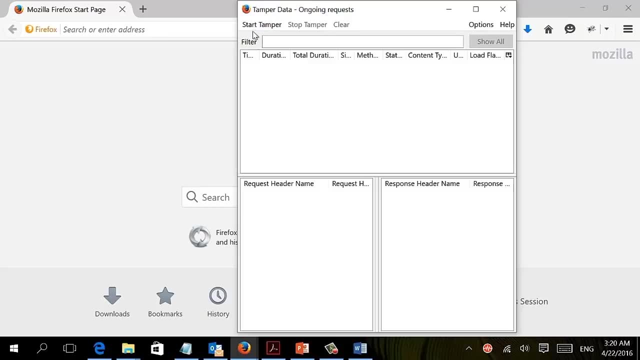 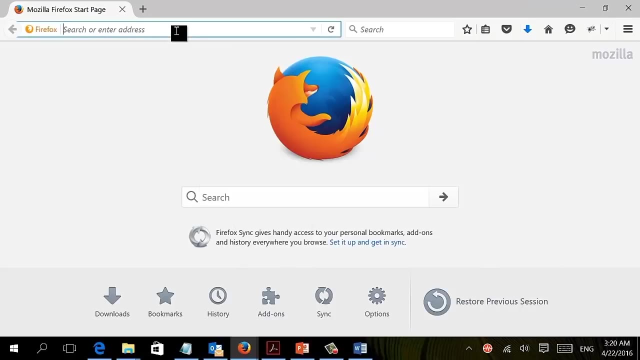 What's tempered data is doing? it just intercepting the traffic going out from your computer and change it. So, as a proof of concept, If I go here And I go start them permanently, mean whatever is going now I want you to intercept it and I try to go to Google. 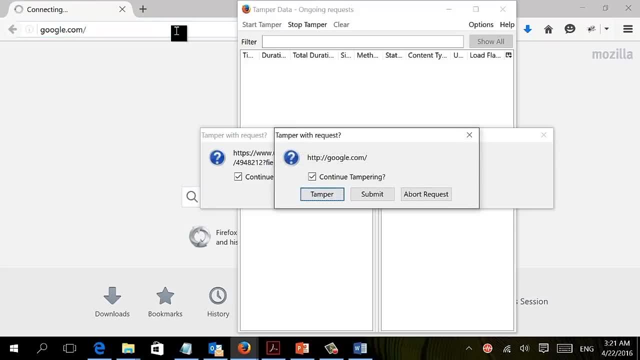 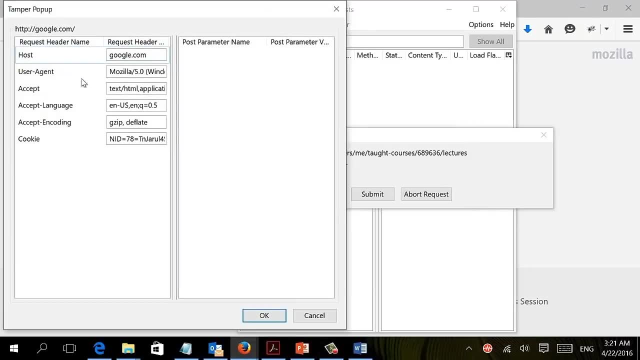 So the request is going from my machine to Google to get the page. that request will be intercepted by this program And you will be allowed to change. I can ask him to go to Yahoo Now- how that can be useful for any hackers. don't think about the scenarios that I just gave. assume that you are buying something from the internet. 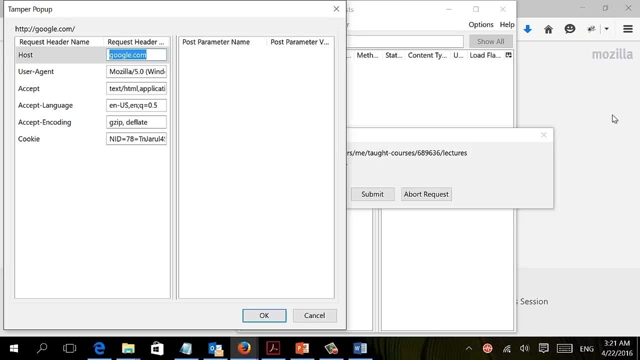 And the developers has create a very good e-commerce website for this company. Now for a user: he went and he bought something and this thing was costing one thousand. now, while he's writing his information and think he's buying an item with one thousand, and before clicking on submit, he can temper the data and change the one thousand to one dollar. 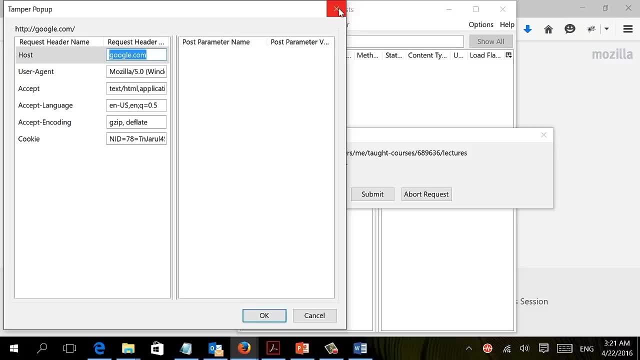 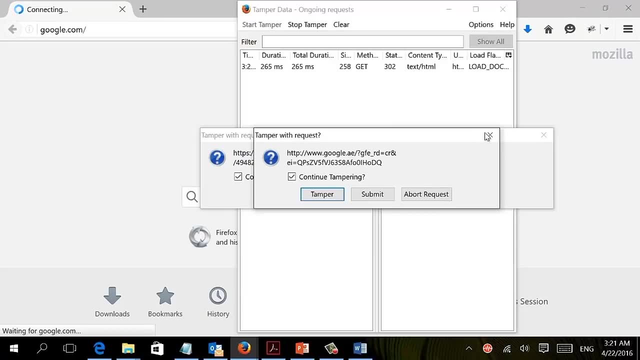 So now he'll be buying something with one thousand with that worth one thousand with one dollar. So this is my Plating: the traffic between the back end server and between the client, or maybe I can try to reset the password and send the reset link to my email, instead of going to the right minutes, and so on. 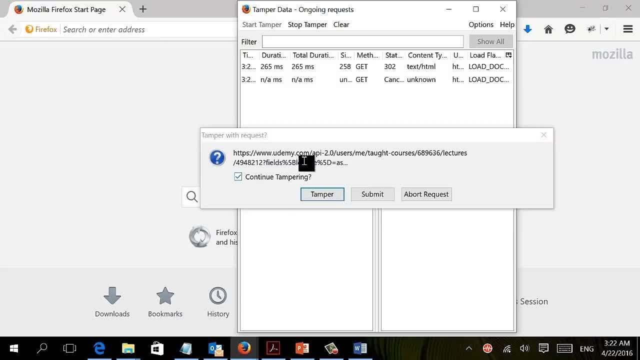 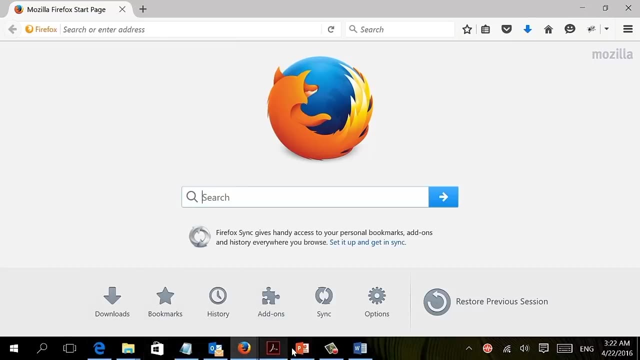 So intercepting the traffic between The. let me just about the request between the client and the server. This is called to you to see. you just like the keyword, or maybe if you try that yourself, you'll memorize it. Okay, another attack which is a buffer over. 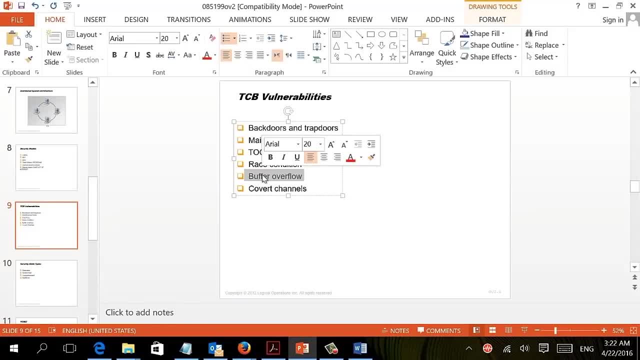 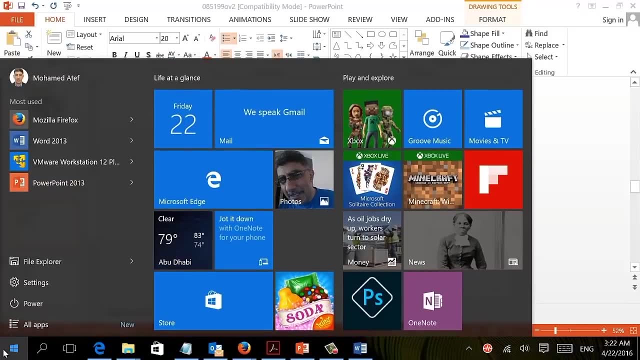 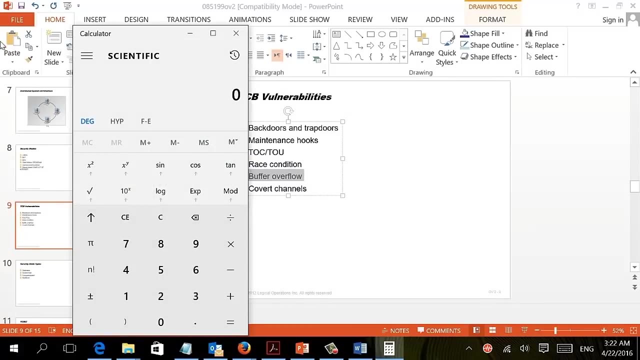 Flow, buffer over flow. It's a very advanced attack but very, very effective as well. buffer over flow, adjust, manipulating the memory. So, for instance, Let's take any program like the calculator, for instance. So the calculator, the way it work, that when you are writing down some number, those number will be saved inside the memory. 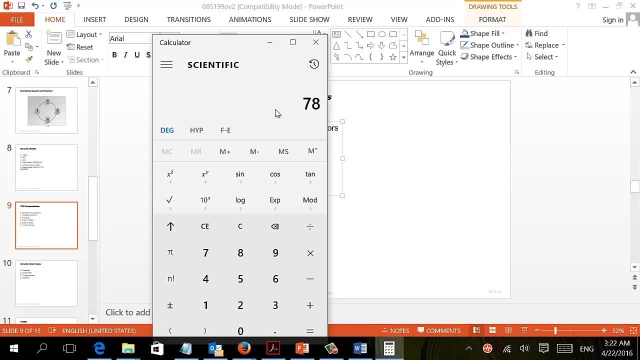 So I'm writing a number and the number will be saved inside memory Inside one specific location inside memory where the programmer who did the calculator has assigned the location inside memory to save this number. And then you put another numbers and you do some formulas. 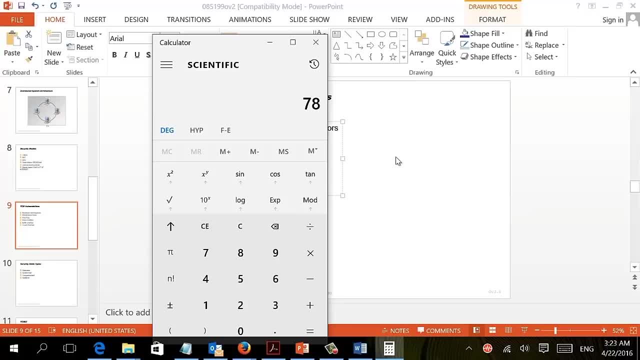 So everything will be done inside memory. Nothing will be saved on your hard drive. The question is: whoever created this Program? while he was developing or creating this program, he was assigning some location inside memory where all those information Will be saved and then some processing will be done on them. while he's doing that and assigning some location inside memory. 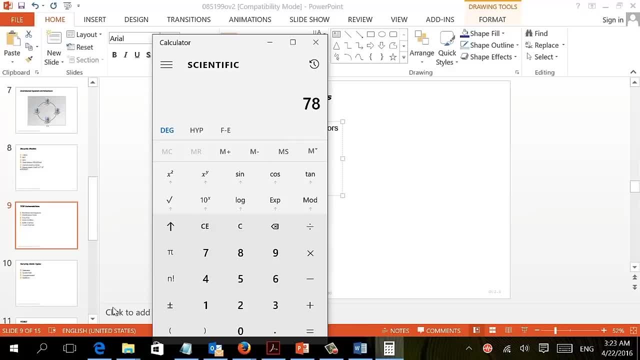 You have to put a size. what will be the maximum size? that say why you notice in calculators that it has a maximum. You cannot keep writing number because it has some limitation, which is very good. after a while it will stop taking number. So now he stopped taking number. 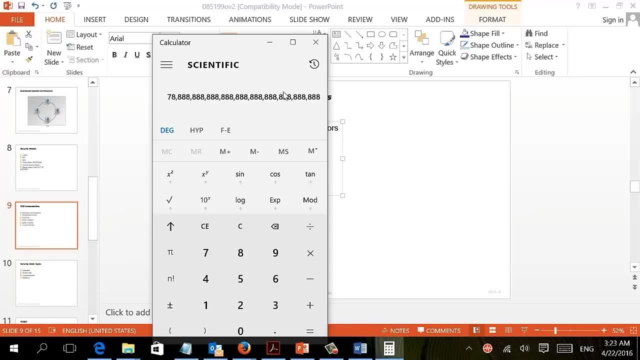 But what will happen if you have a program that do not validate the input? So you have a maximum 100, for instance, instead of 400.. You put 1000.. So if the program was not well made, like this calculator, he will keep, he will take all the 1000. 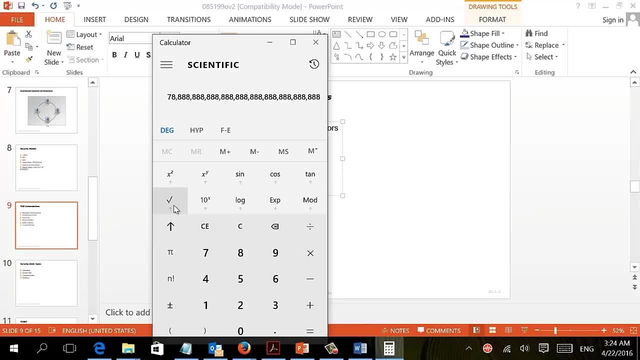 But the place where those 1000 need to be stored actually has a limitation on size, which is 100.. Now where are you going to put the remaining of those 1000. So those remaining will be saved inside randomly inside the memory. So now the hacker was able to reach inside the memory by the buffer overflow. 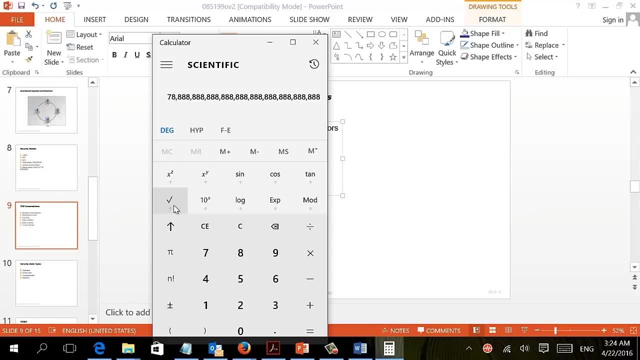 Now There is Some places inside memory that, if you reach them, You will be able to allow the computer to execute anything, And this is what exactly we are trying to do. We are getting an application when we are doing penetration testing and we check if it's affected with buffer overflow or not. 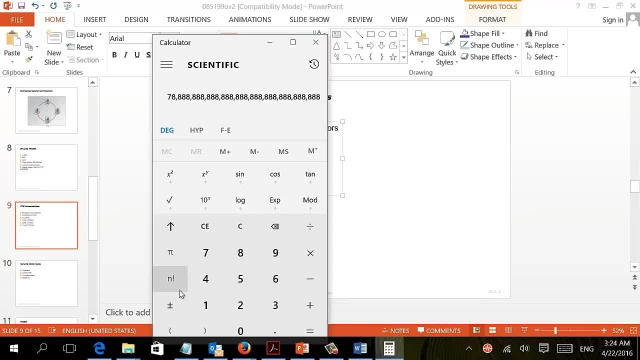 And then we try to send as much information as we can if it's affected. I'm going to send some payload, But I need to Make sure that it will go in a place inside the memory where whatever you send it will be executed. 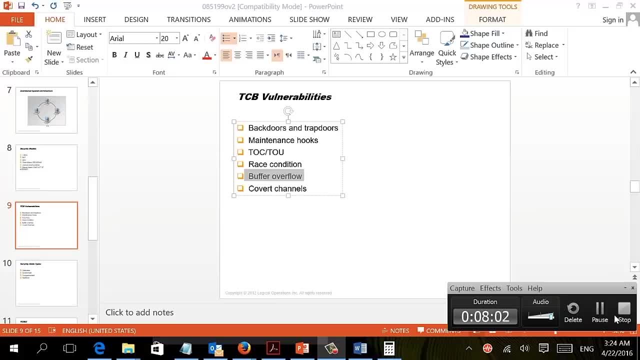 This is called the buffer overflow, The remaining attack. It's a covered channel attack And this is where the traffic has been manipulated. So you are assuming that your traffic is going from A to B, but actually is going from A to B through C. 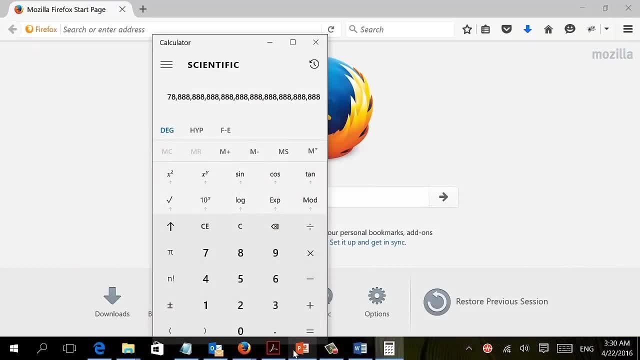 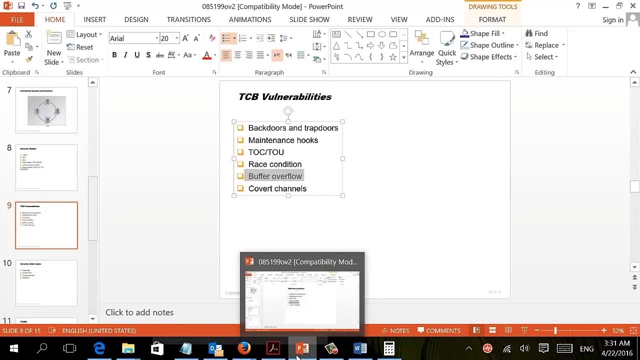 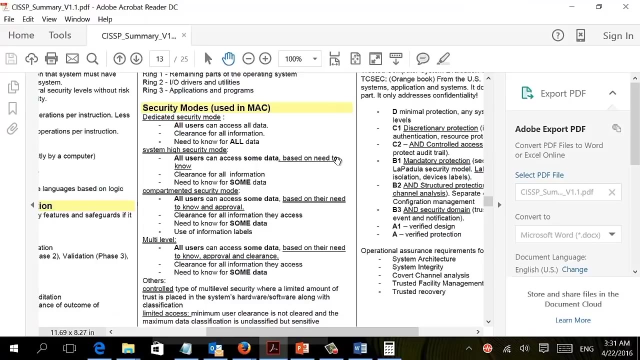 Okay, so attacks as we are very important And the Sunflower will help you with that. What is it? I think that I close it, So Sunflower will help. No, here you go Identifying the attack, But sometimes you will not find all attack in the same place. 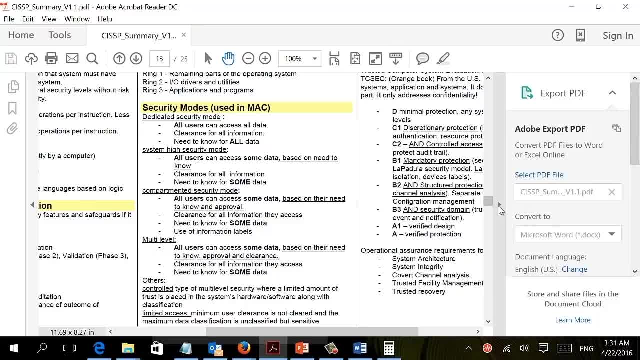 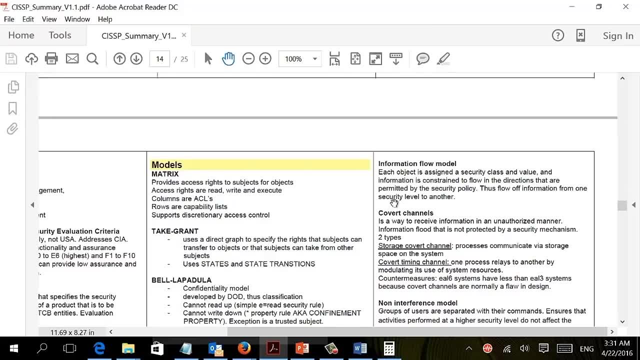 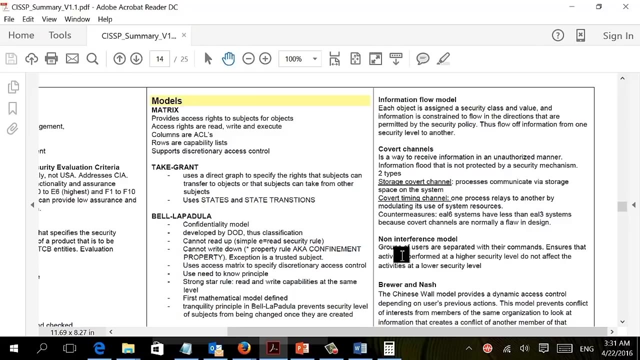 I mean It's usually Special- is a common one would be located in one area. So here you can see those attack cover channel. Even there is two type: storage cover channel cover channel cover cover, timing channel. We have the Here. they didn't mention anything about the other attack like the buffer overflow, because this was mentioned in the network. 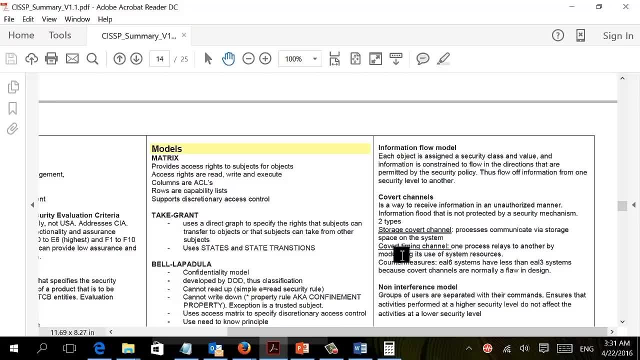 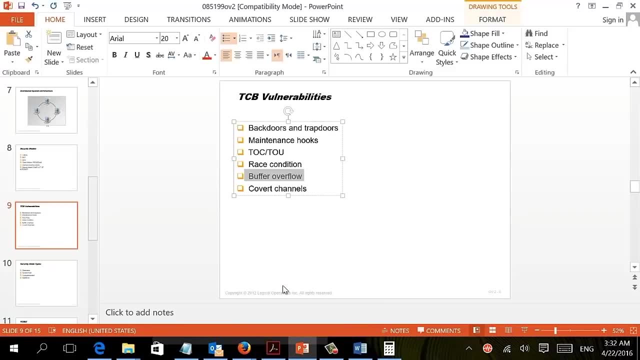 So you will find attack in different location. But after all, this need to be actually memorized and if any attack it's new to you, You have to write down how it works And you know. a good way for memorizing the attack will be to go through any YouTube video to get the concept how it work. 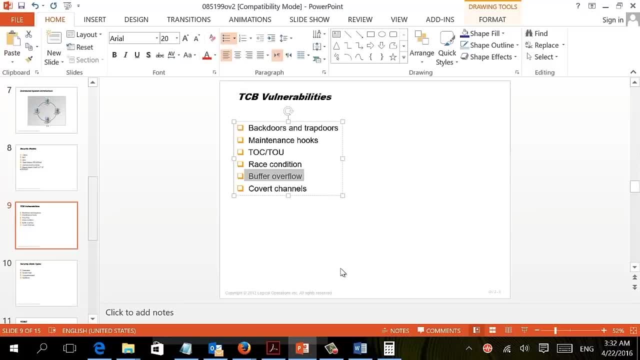 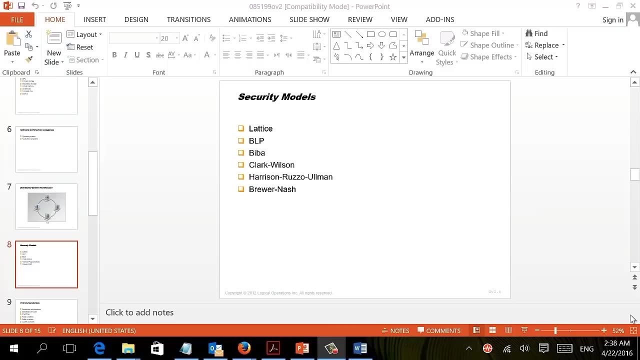 Okay, so attacks is very, very important for the exam purpose and understanding all the attacks. This lecture we will be talking about some things that confuse a lot Of student because it's little bit academic, Which is security model, And we're going to try to simplify that as much as we can. 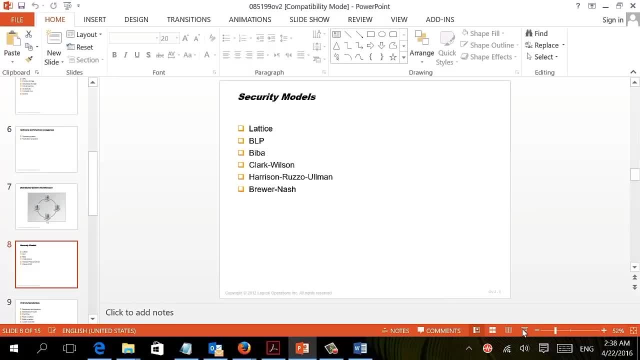 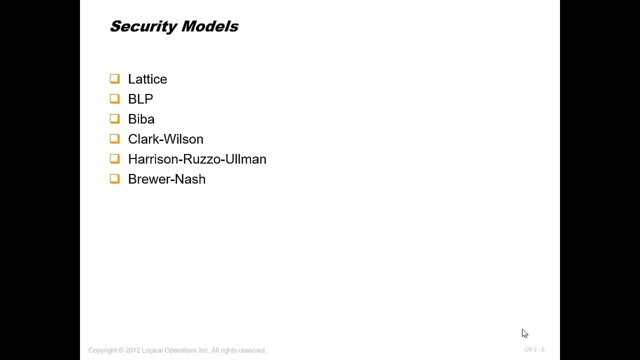 So we have some security models that we can implement in our organization, Except it's not implemented By their name. I mean, you will find that some appliance or some application or some software are working according to those models. So we will not Say that we're going to implement Beba or BLP or Clark Wilson. 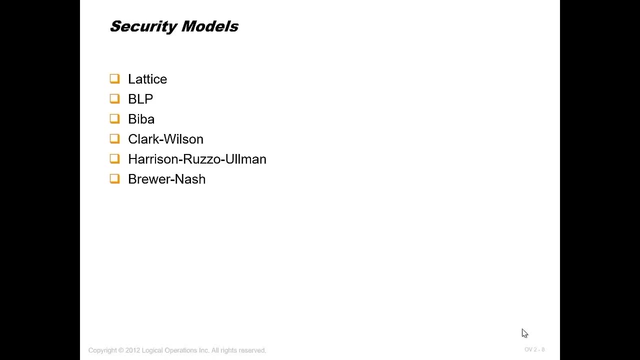 It's mainly into the concept of this implementation. Now, before explaining those implementation- and the major one of them, I just need to point to that- The first thing that you need to do, you need to know, is: this model are providing, what Are this model providing? confidentiality or integrity or availability? 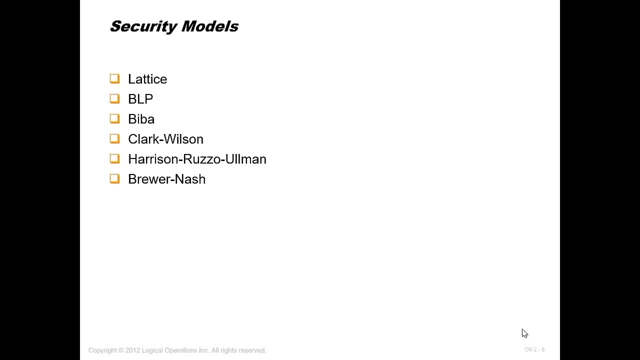 And this one of the questions that you should expect He will ask you: Beba is providing. what if you implement the Beba model? Is it about confidentiality or integrity, or availability and so on? And don't forget to write down the keywords that I'm going to mention during this lecture. 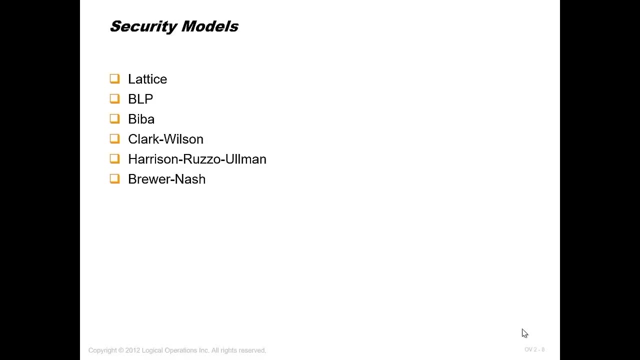 Because this is extremely important. So I'll take the first one: BLP or Bella la Padula and Bella la Padula. It's almost the first model, And the only model that provide confidentiality. Now let me clear to you and let me clarify to you. 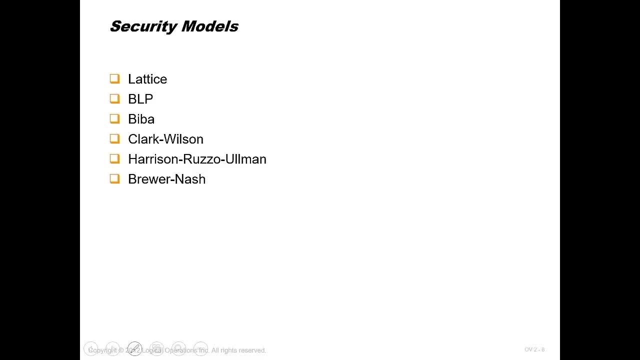 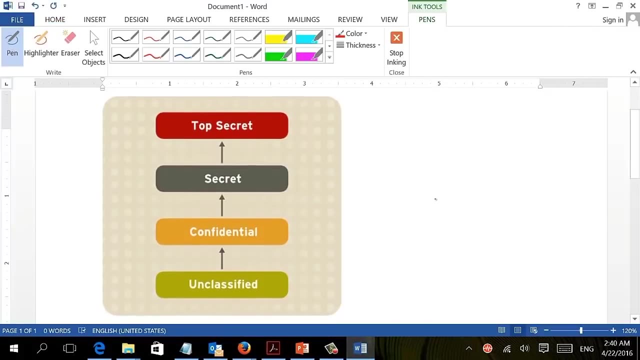 What is BLP model? So we're going to go to our Sheet And assume that I have A classification of information this way. So I'm using a Mac classification, mandatory access control and my own for the information that I have has been classified to top secret: secret, confidential and unclassified. 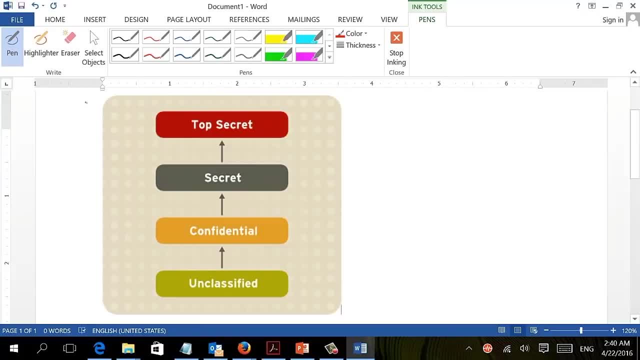 And you remember how the deck model is working. You can have, your information will be classified, They will have different security level and then each user will have A Clearance level. So assume that we have this type of classification and you, as user, has a. 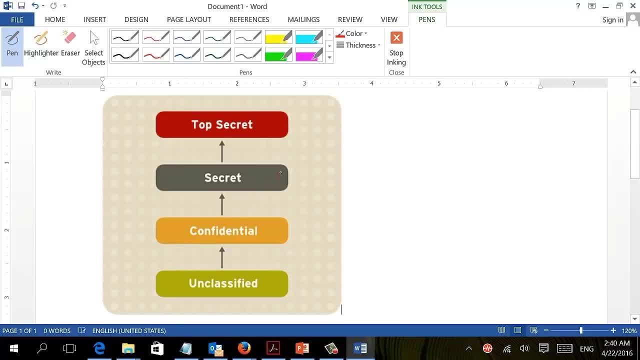 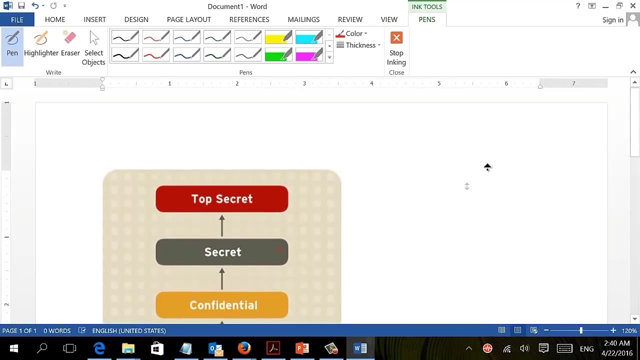 Secret level. Okay, so you are inside this level. You have a secret level. Now what is BLP is saying? Okay, and one more time, BLP, It's about the confidentiality. It's not about the integrity or availability. 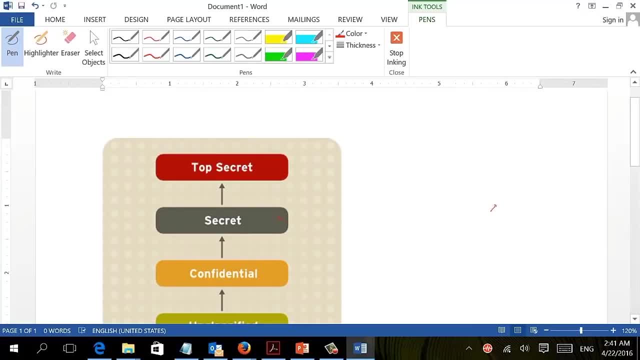 And actually this is as I told you. this is the only model that is about confidentiality. So what is BLP is saying? or Bella la Padula is saying: No, read up, Let me write it down for you. Yeah, sorry. So what is BLP saying? 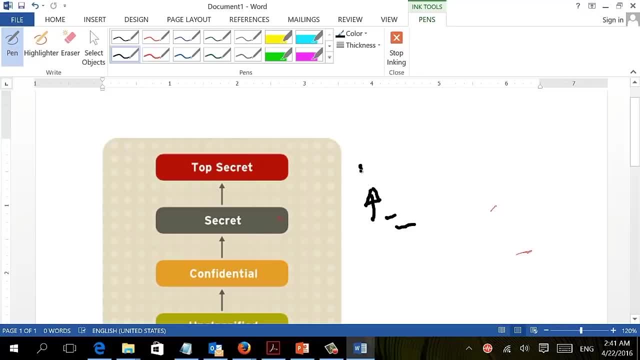 Let's put an error here: No Read Up and No Right Down. So if you are implementing BLP, that's mean No read up and no write down. Let me explain it to you, If you have a secret clearance. 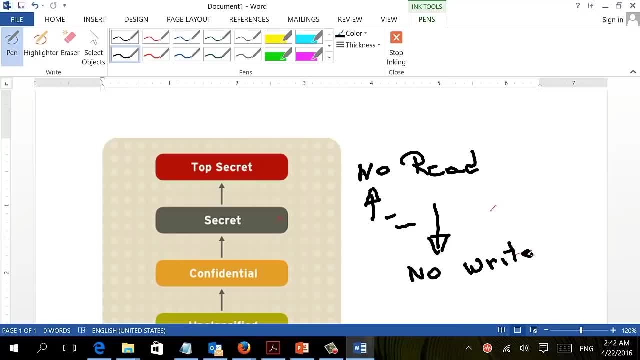 So you can only check the secret information, The information that is classified secret, in this case you will not be able to read up, right, as a secret Clearance user, You cannot read the top secret. So it makes sense, and you can also not allow to write down. 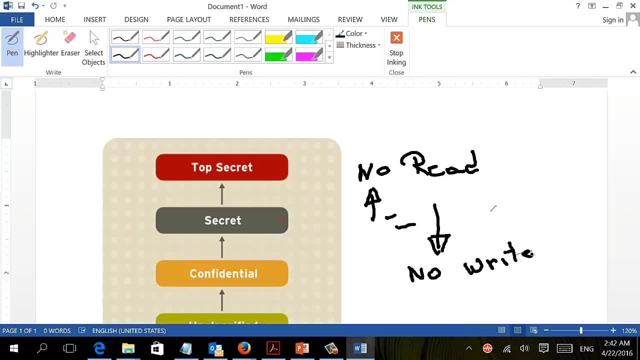 So you will not be allowed to write down. So you from the second level, you can write right inside the confidential level. And why is that? Because if I know secret information which is more important than confidential information, So if I'm allowed to write on the confidential I may, I may write something. 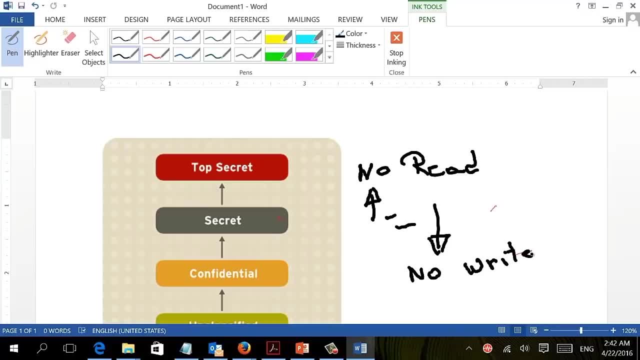 That should not be written. I may write some secret information into the confidential, which will affect the confidentiality. So you are not allowed to read up, and this is quite clear. but you are also not allowed to write down Because, as I told you, whatever you're going to wrote, or you can wrote something that should not be allowed or should not. 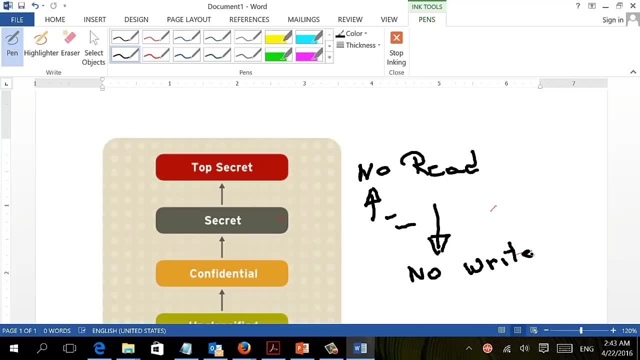 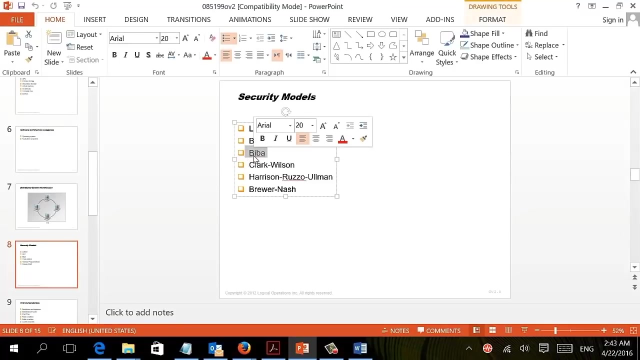 Be available for confidential user. So BLP number one it's a confidentiality model And it's saying no read up and no write down. Second model: it's called better and better model. It's the opposite of BLP number First thing that, Baba, it's providing integrity and not confidentiality. 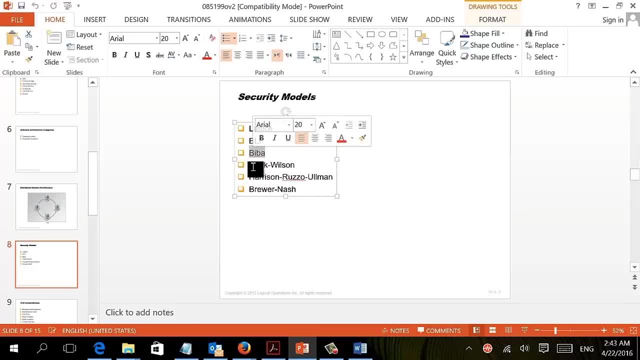 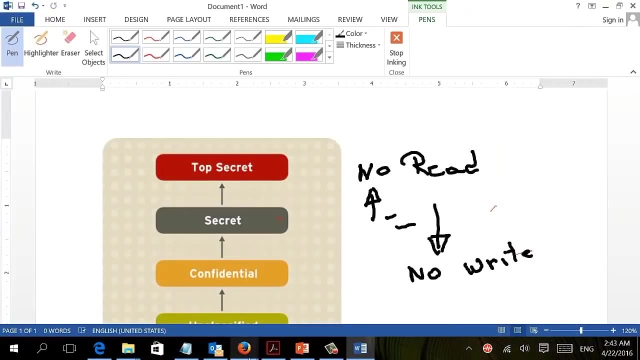 And Whatever remaining. it's about integrity. Only BLP It's about confidentiality. So Baba model is providing integrity. So if your organization need to provide integrity, you're going to need to work on Baba model. Baba is the opposite of BLP. 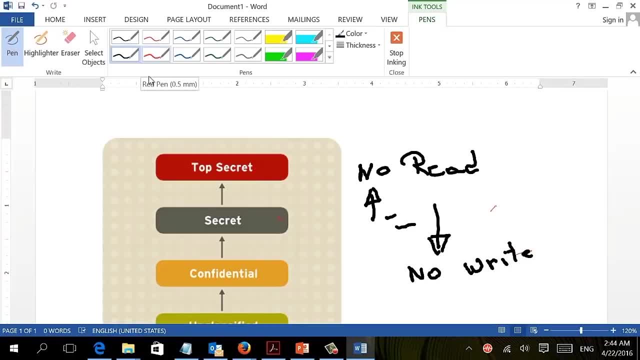 Okay, so BLP are saying no read up and no write down. Baba will say No write up and no Read down. So Baba is the opposite of BLP. So what? Baba is saying the opposite, which is no write up. 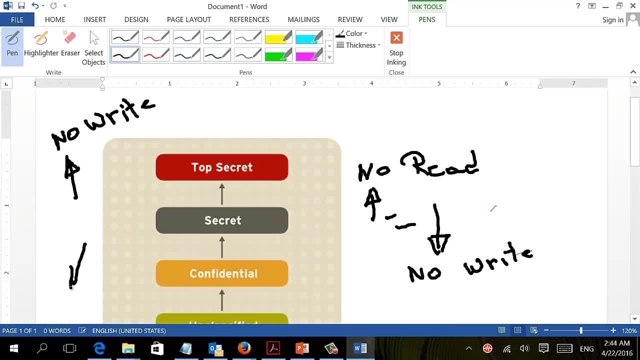 And no Read down. And it's not a confidentiality model, It's an integrity model. Now let me explain the concept. So Baba is the opposite of BLP. If we are on the same scenario where you have a secret, cleaners right. 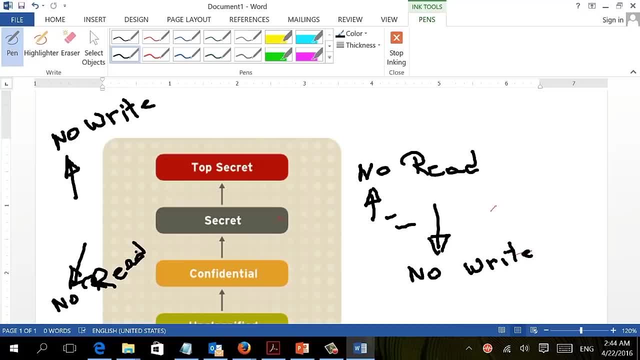 Now, If you are allowed to write up or read down, what will happen now? let's assume that we have some information, And the information with the confidential people are not hundred percent precise. They have some general information. Okay, for instance, let's assume that we are talking about financial information. 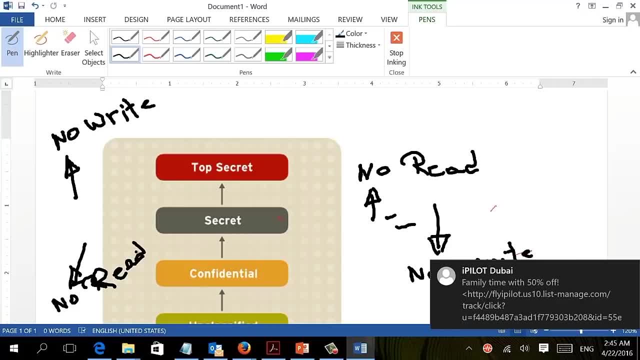 So people in confidential level knows that their organization are doing well And the organization are getting profit, but they don't know any numbers, They don't know any figures, right, They know that the company are doing well. People in secret level knows the figures. 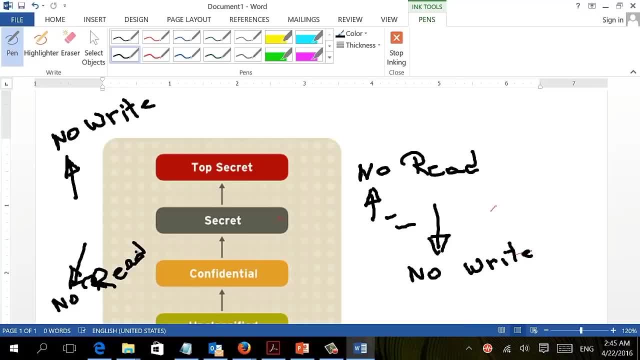 So know that the company are profiting two million, three million- They have number, So the information is a secret level- are more precise than the confidential. people in top secret know a lot of details So they know the bonus for this top management where people in secret don't know about it. 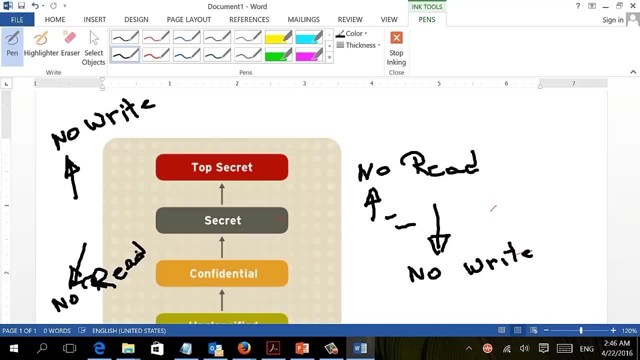 They know that there is a profit And they know the figure, but they don't know the bonus and they don't know the details And what deal has been sold with a good price and so on. Now, if you allow people from secret to write up, they may write something that affect the integrity. 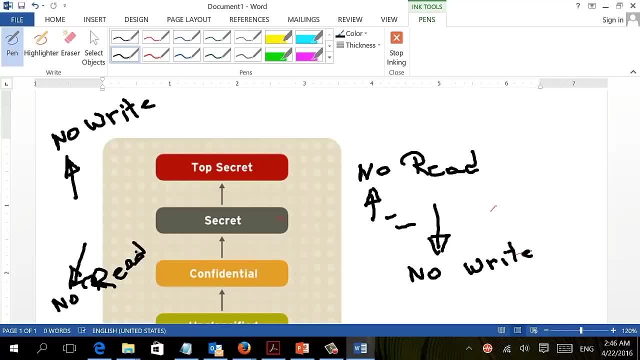 Okay, so I know that company are doing well, So but I don't know the details. So if I writing on the upper level, I may write that say that May lead to confusing people in top secret. So top secret people has more precise information. 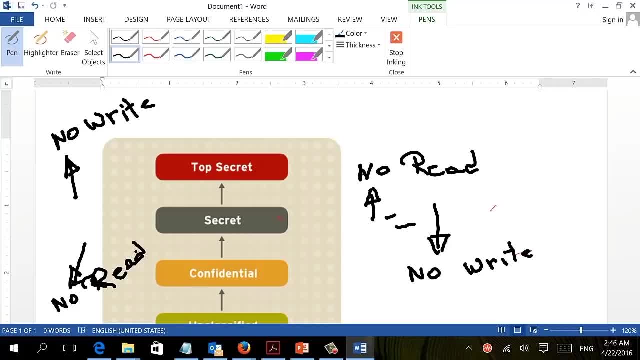 And maybe they get confused if you are allowing people from a lower level to write information, So maybe the lower level do not have this precise information, So they will write anything that will confuse what they know. So I'm affecting the integrity if I'm allowed to read down. 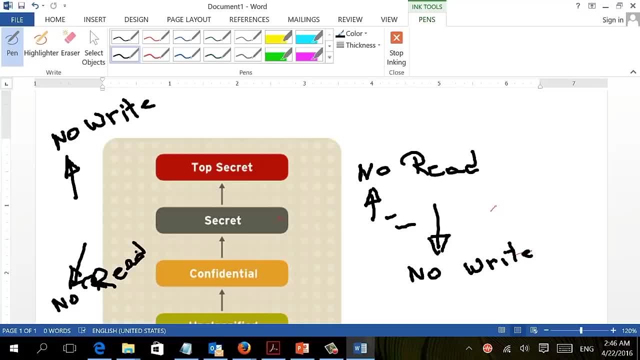 So, for instance, I'm in secret and I'm allowed to read down, So I'm reading the confidential. My information inside the secret level is more precise and more exactly, or the number are precise, than the confidential level. So I'll get confused myself. 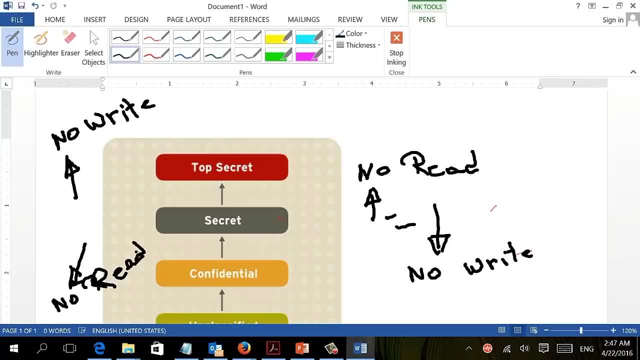 I don't know now who's whom to believe. I went to the confidential, confidential level and I wrote the information. It's different than mine, So now I'm affecting the integrity. So BLP it's about integrity And I'm sorry. BLP is about confidentiality. 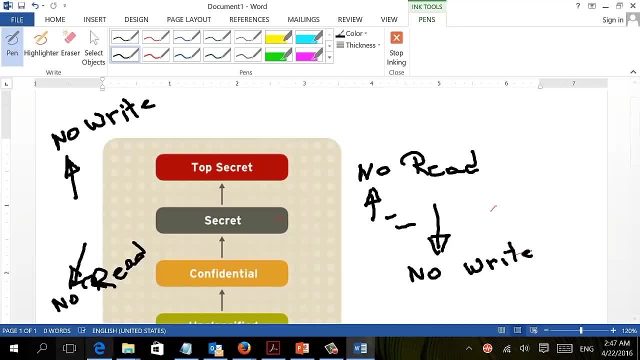 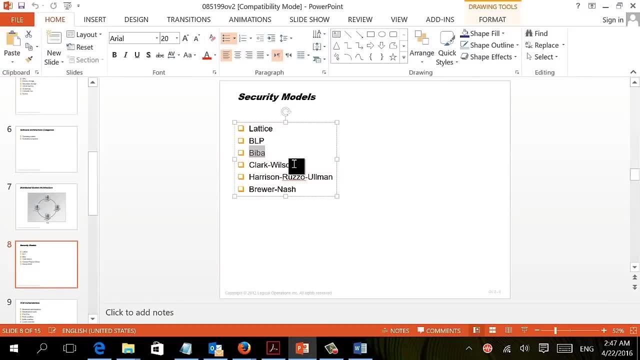 Biba is about integrity And don't forget that. no read up and no write down. Let's get to the other model. We have Clark-Wilson model and in Clark-Wilson some terminology are there. So Clark-Wilson model are saying two things and some keywords- very important keywords, are there. 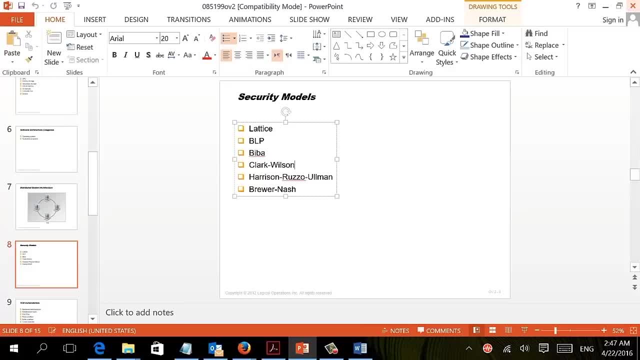 Number one, That user should use the information through program. So the first keyword here is a program. So what Clark will also. by the way, I'm sorry, Clark-Wilson is also about integrity, It's not about confidentiality. So what Clark-Wilson is saying? that user should be able to access information through. 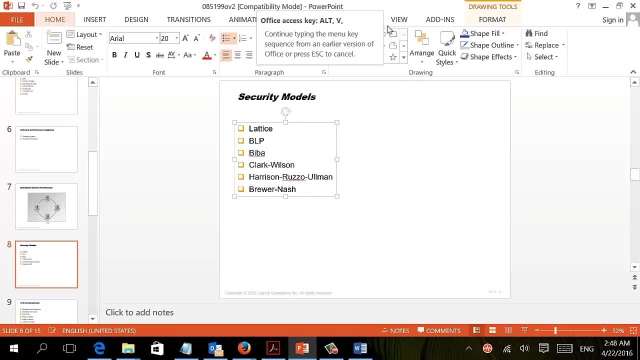 Application or through a program, right? So, for instance, if I have all my information written in Books and everyone who can access those book will be able to see whatever he want, This is against Clark-Wilson. Well, Clark-Wilson saying, which is: make a lot of sense, that you should put your information inside any program. assume for Excel sheet. 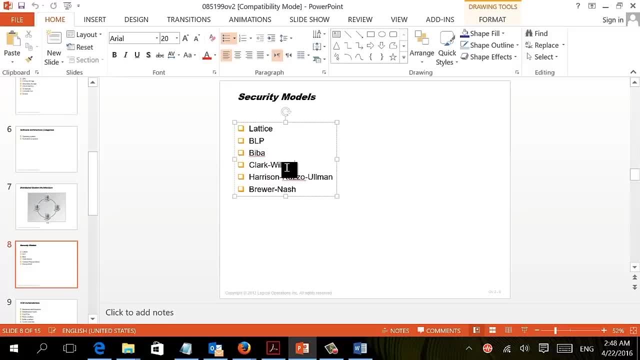 You are putting all the company data information in an Excel sheet And you are putting permission to user. So one user: when he login he will be able to see some column. as a loser, He'll be able to see another sheet. So a keyword here: 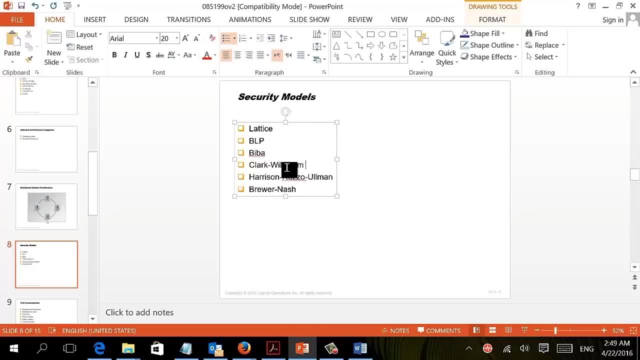 It's a program. user should access Program. Okay, user should access information or data through a program. The second concept- So the keyword here is a program. second concept in Clark-Wilson is- says that user Intersection interaction should not be interfering. 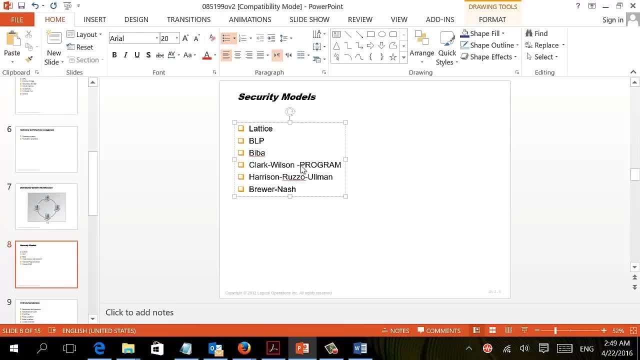 So if we are taking an Excel sheet and we are both writing on the same time on the same sheet and on the same cell, which one will be The updated one? actually, Excel is not allowing that, but as a concept, So user transaction should not be interfering. 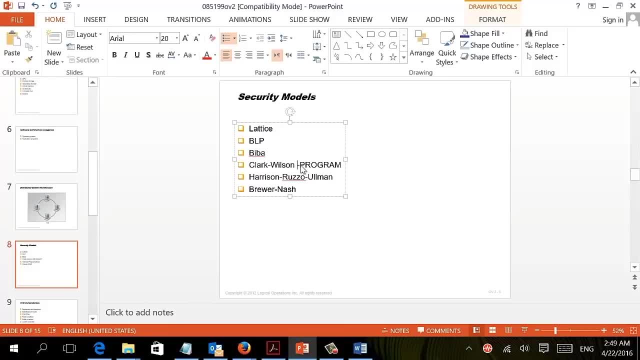 This is what Clark-Wilson is saying in his model And, as I told you, this is a Integrity model. The third one, which is very, very important, is called Brewer Nash. Brewer Nash has a very, very important terminology or keywords that definitely is asking about Brewer Nash. 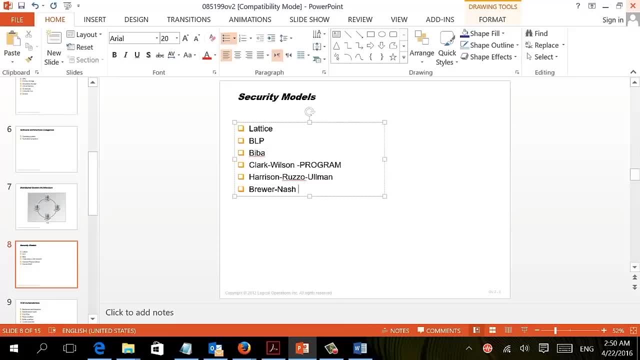 He will mention this one. It's called the conflict of interest- Very important terminology, conflict Of Interest. So if you got any questions that asking you about conflict of interest, it's Brewer Nash. Now let's explain Brewer Nash It's. it's how it to be implemented. 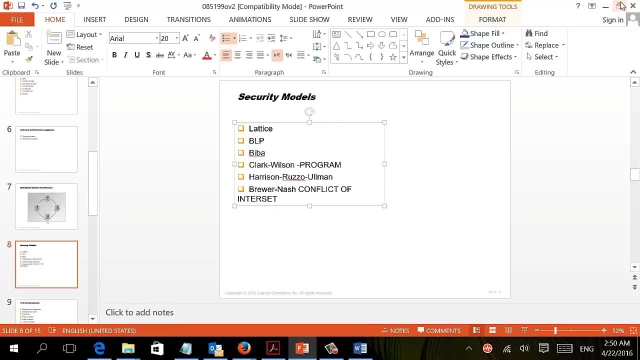 By the way, there is another name for Brewer Nash. It's called the Chinese wall and you'll understand the terminology from the explanation What Brewer Nash is saying: that sometimes the control will be taking based on The decision. Let me give you a small example and I hope I'll be able to explain it. 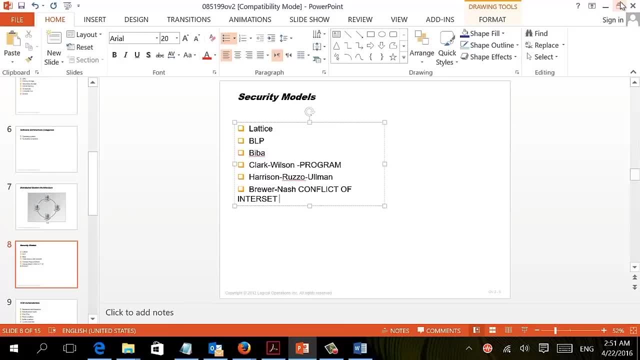 Well, assume that I am a lawyer and I have two client Against each other and I have to select one of those client to become my client against the other one. So I need to take a decision. So if I select client a And I'll be able to see all the information of client a- so my decision was client a- I should be prevented. 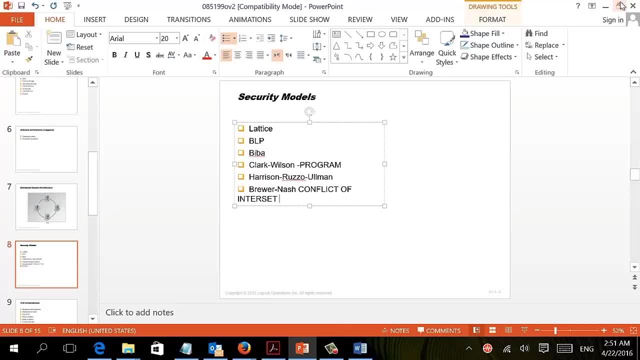 From seeing the information related to client B, because this would be a conflict of interest, because now he will be Against my client and I'm trying to take charge or I'm trying to suit him for anything if I took Client B to become my client. 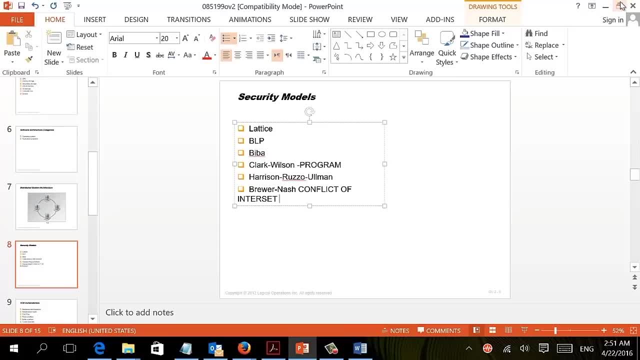 Now I should not be allowed to Check the information of client a, so The control has been implemented according to my decision. This is called the conflict The Brewer Nash. That's why they call that a Chinese wall. So, according to your decision, a Chinese wall will be built between 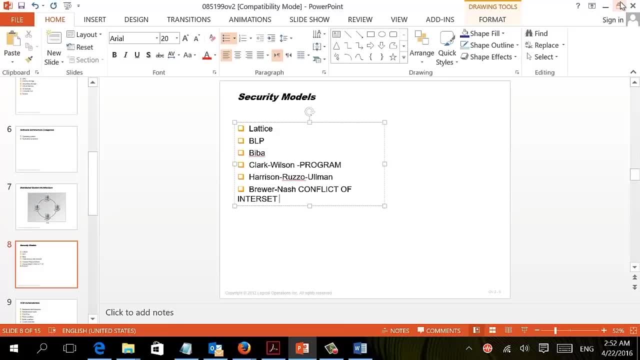 The information that you have access to and the other information. So it's a dynamic access control list According to your decision. So conflict of interest: It's a very, very important terminology that you should be aware of. Those are very important for models. 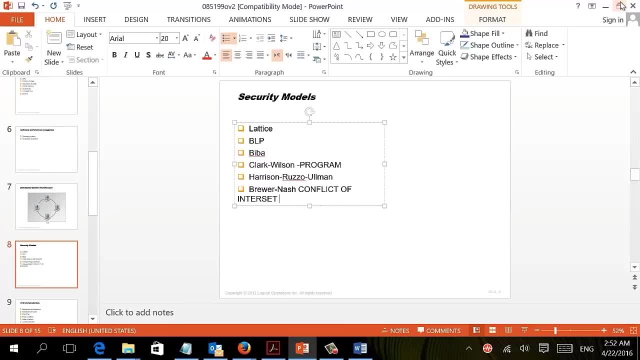 The remaining of model. just you can read the definition: latest means they are layers. But those are extremely important and hundred percent. You get a question about that inside the exam. now, before moving from this part, I want just to show you the details on that, on the Sunflower document, because, as I told you, it's easier to read this part from Sunflower. 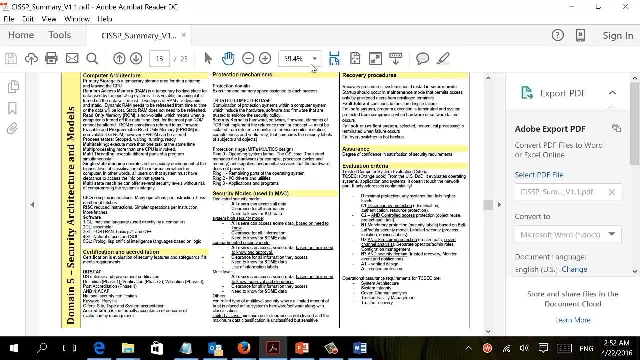 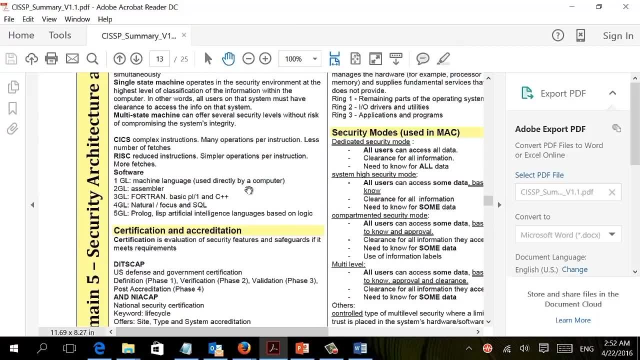 So from Sunflower document, let me just increase the size a little bit and let me show you how it has been explained, and then we're going to talk about the implementation of that. So let's see Where is the models BLP. 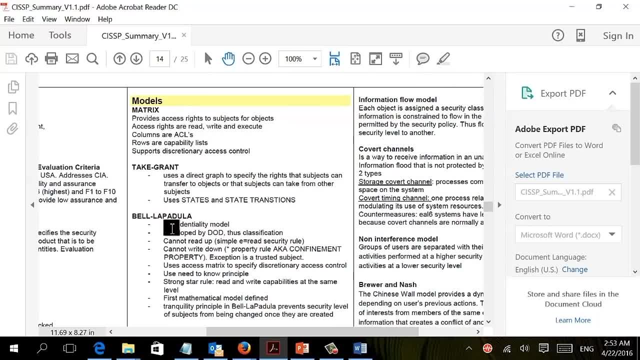 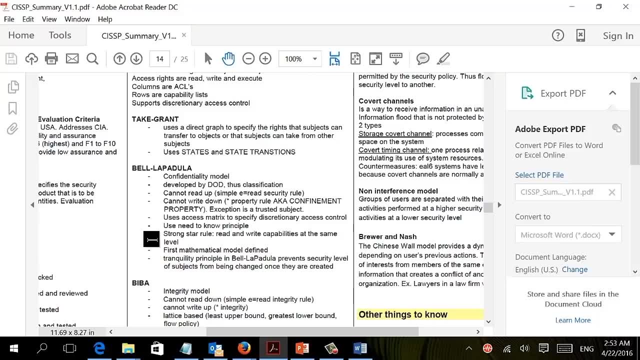 Here you go. So we have BLP. Don't forget, It's a confidentiality model, It has been developed by the Department of Defense, and so on. And what exactly it's saying: No read up, no write down, but they have names. 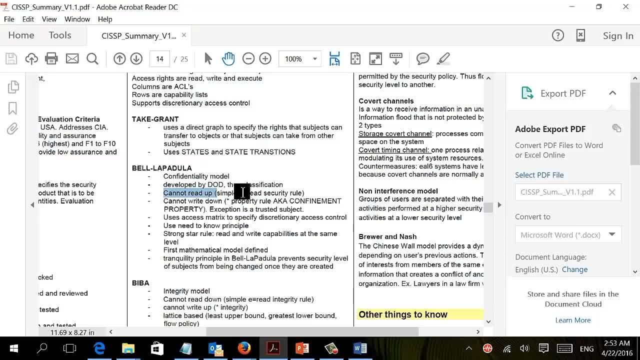 I mean cannot read up, has different as another name, simply E read. And, by the way, as I told you earlier in this course, that you should be aware of different name because you don't want to lose a question because you didn't know that this is a different name from the same. 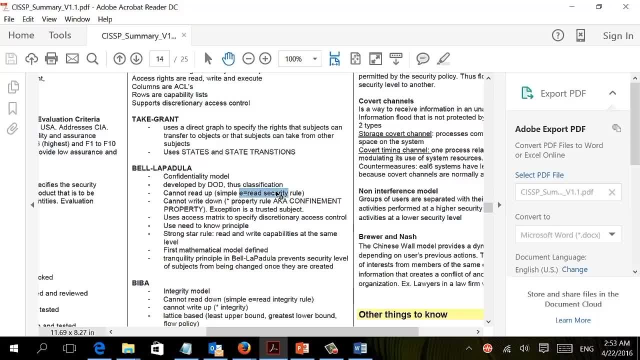 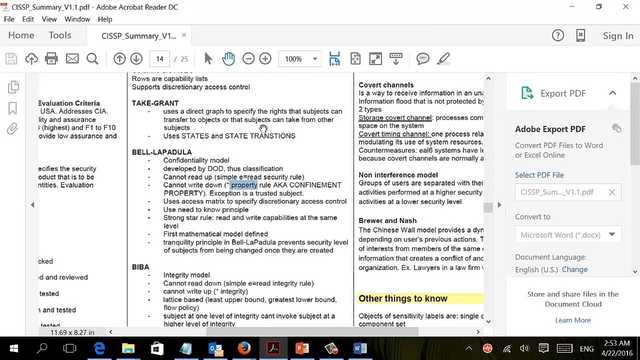 Terminology that you are aware of. So no, no read up- has a different name, which is the simple E and no write down. It's called the star property. Okay, so you should read about BLP and its confidentiality model and so on. 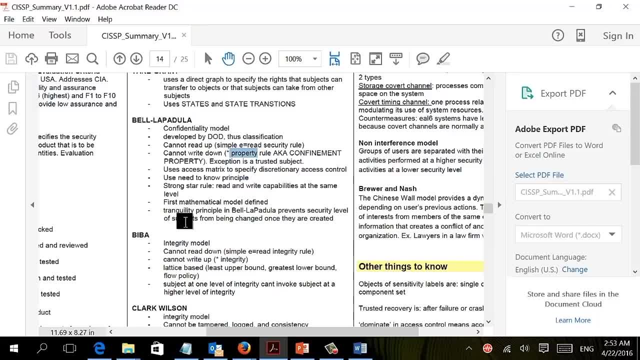 We have better. It's an integrity model and it's saying: cannot read up also simple E and cannot write down its star, Sorry, cannot read up, Cannot read down and write up. It's the opposite of BLP. We have the Clark Wilson and see the things. that is underlined. 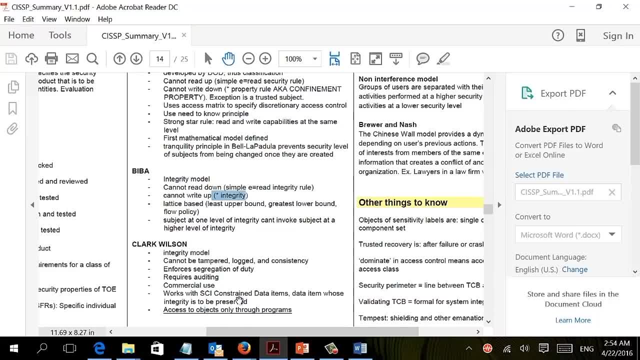 This is extremely important. This actually PDF file, anything that is in capital letter or underline. Be careful, This is, you know, a tricky part inside the exam, So access to the object should be only through a program. Okay, so those are the models. 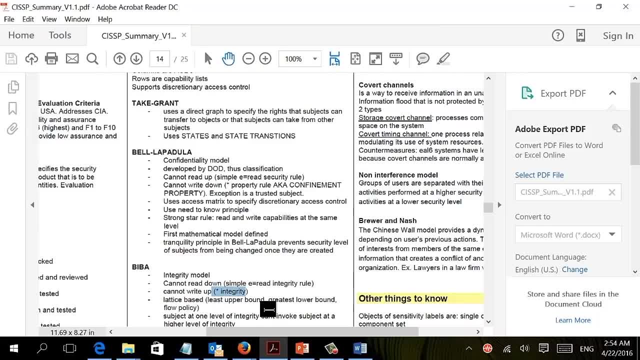 Now the question is how they are implemented in real life. They are not implemented the same way I explained. It's more into the concept of those models, So the concept that you'll be getting an application or software on a system that implement BLP or implement 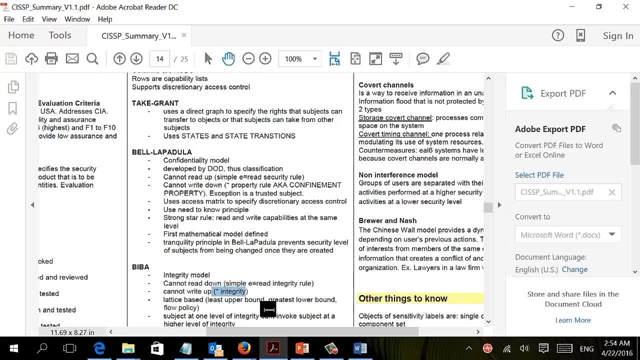 Beba or Brewer Nash and so on, and it could be a part of BMP or so it will be through something. It will not be implemented by their definitions this way. It's a very, very important part. security models and please feel free to post any question if 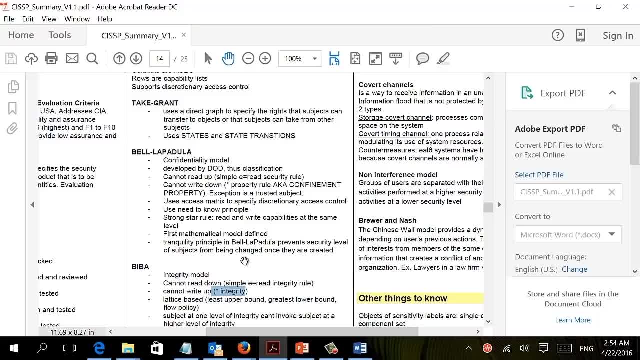 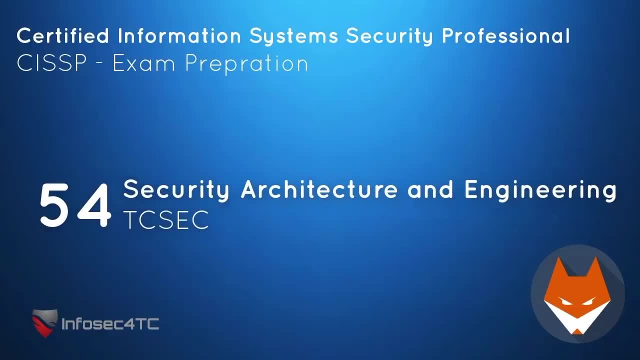 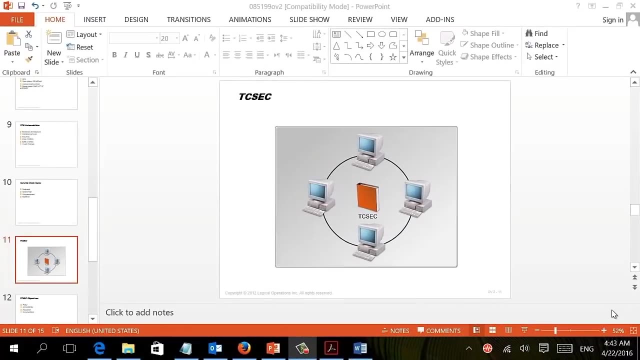 not clear and I believe if you want to study this part, it's easier to read it from here, quite simplified, because this is, you know, as far as you need to know for the exam purpose. Two remaining part in this domain, which will be the TC sec and IT sec and common criteria, and those are: 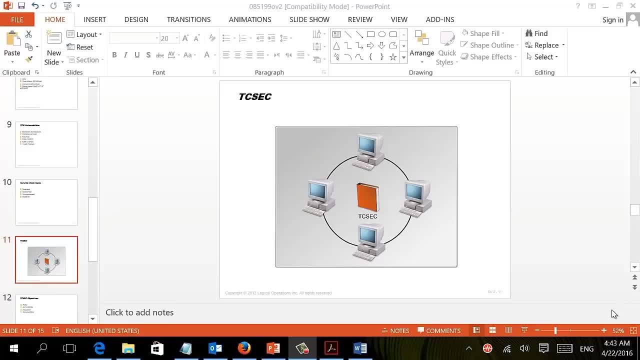 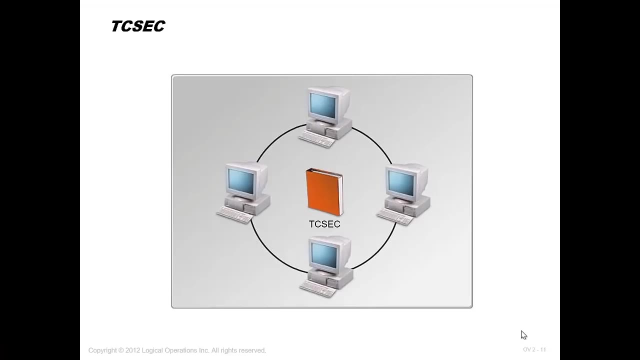 the main objective of this module. Actually, You remember the discussion we had at the beginning of this domain, where we spoke about how can we evaluate a system and we define a system as a trusted computer based which is the hardware, software and operating hardware framework and operating system. 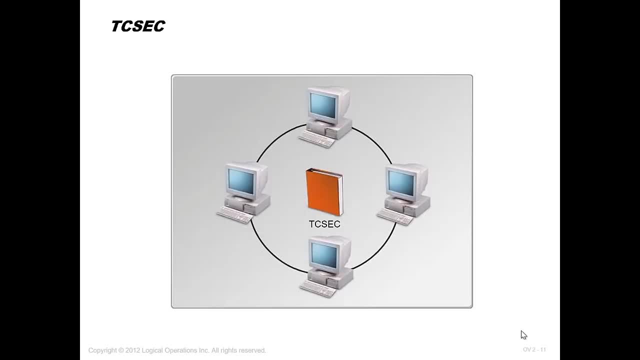 So when we started this domain, we agree. then, when it comes to getting computer, buying computer, how can we evaluate? Do we have a reference to refer to that? identify which machine? now I will not talk, I will not say machine or system. 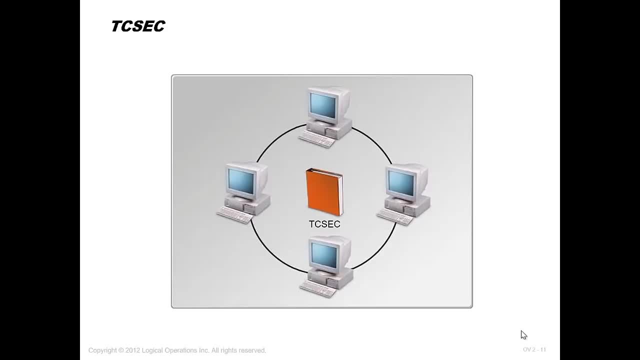 I will say the T- trusted computer-based TCB. So do we have something that we can measure or we can refer to, that will allow us to know what is more secure than other? the first approach for that, with something called the TC sec, and it has another name. 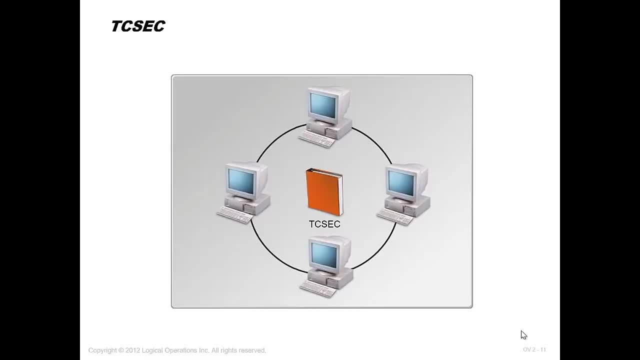 And please take a note for different name, which is the orange book. So TC, sec or orange book has been found from, has been introduced by nest, National Institute of standard and technology, and we had a discussion about nest at the beginning of this course. They introduce a book where they have been categorizing the system, or the TCB, and they are saying, if yours, 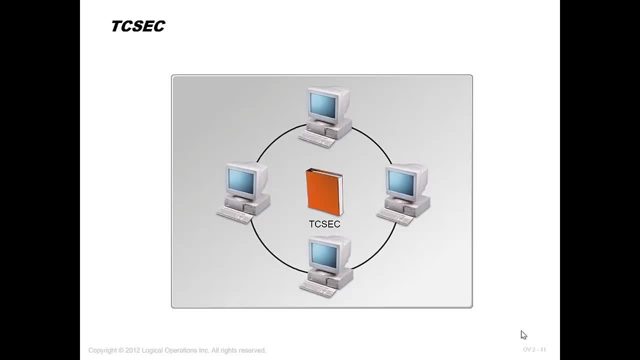 TCB are providing one, two, three, four, five. This is considered a or B or C. So nest has introduced an orange book and the nest actually didn't just introduce the orange book, They introduced a set of book called the rainbow book and they have different color. 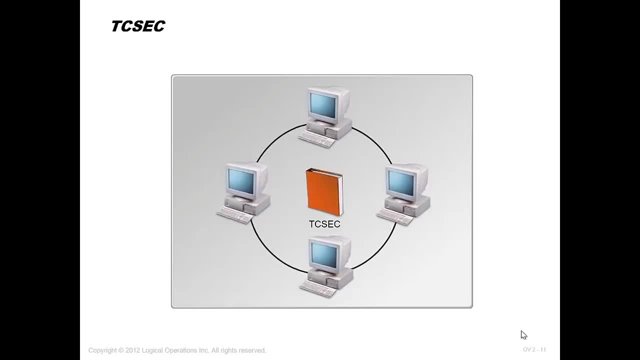 So the orange book has a way for evaluating computers or the trusted computer-based, while we have the red book. This was a book to evaluate the network. We have the green book for password and you're going to need to know the measures- one of them like four of them, but the details. 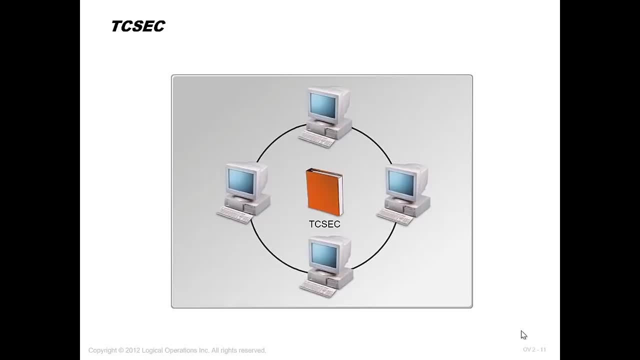 you're going to need to know The orange book or other name for that, the TC sec- and they put a table or schedule that start from A to D, where D is considered the lower security. If your system is D, if your TCB is D, this is considered the minimum security, while a is a higher one and they put some 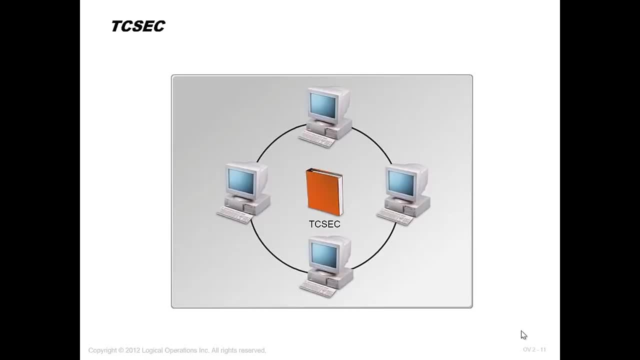 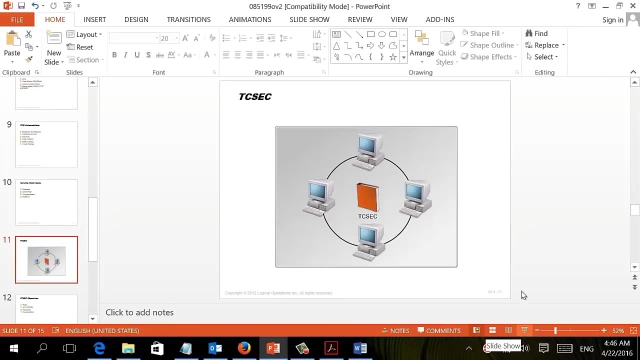 definition for that. If your system can provide, your trusted computer base can provide this and this and this, this is considered a or B or C only Now. this is the part where you're going to need to do some memorization. I know it's not easy, but if you keep reading them, you're going to memorize them after time. 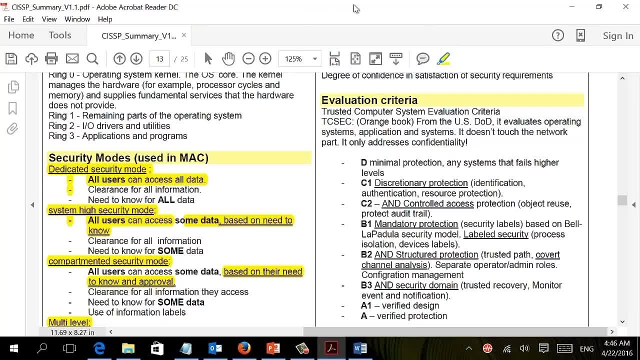 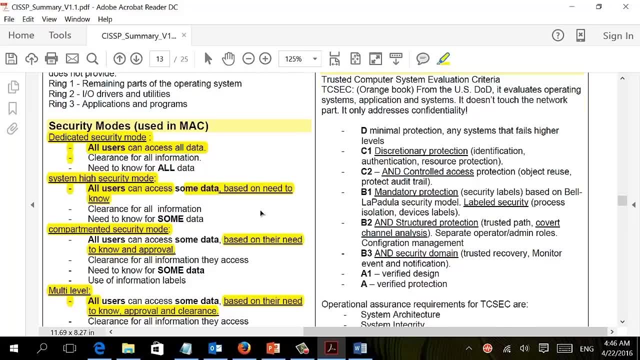 So, as you can see, the TC sec, which stand for trusted computer system evaluation criteria from nest, and another name for that is the orange book, has different category at start from D, where D it's considered the minimum security, and a, which is considered as a higher one. 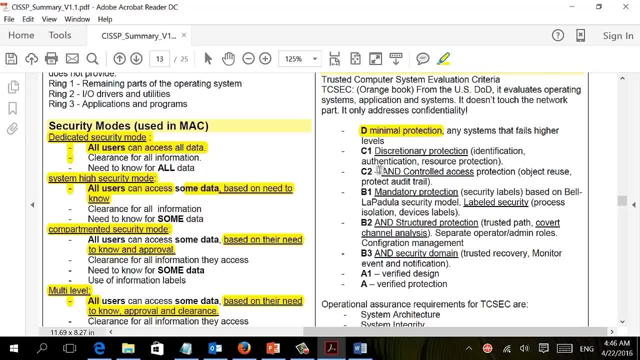 So let's start with the mean. It doesn't have any security at all. See mean: it implement deck Actually access control, So this is considered C1 if it implement that, this credential access controls that we are using in Windows, which is permission, read, write and ownership, and it also has identification, authentication and resource protection. 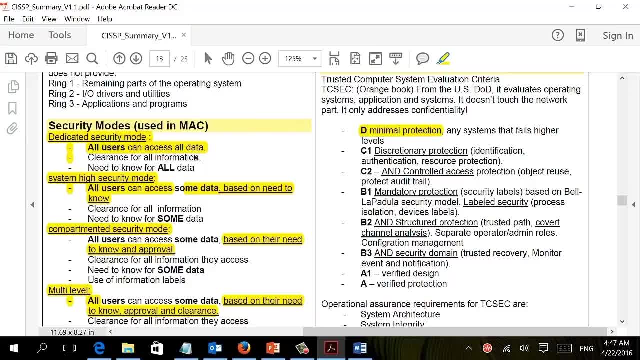 This is considered- I'm sorry, it implement the deck and also has control access protection or it prevent object reuse and has an audit trial. This is considered C2, like Windows, Windows It implemented deck and it has an event viewer. So we are considering computers that has Intel processor with Windows operating system. 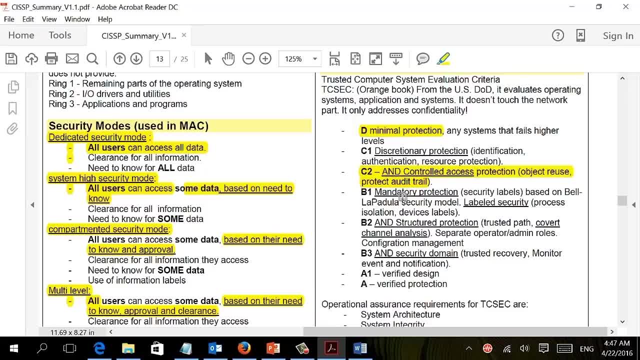 This is C2 and, as you can see, it's not very high. If it can implement Mac Windows, cannot implement in Mac mandatory access control and has, which is security label, and has and can implement the BLP, Bella Bella security model And the has. 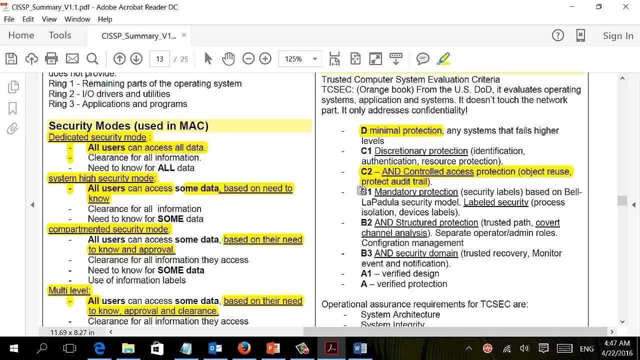 And has Davis device label. This is considered B1. if it has all of those and can structure protection- I mean trusted pass it, prevent, cover Channel and has the separation of operation or separation of beauty can provide that. this is considered B2 if it has all those feature beside security domain or trusted recovery. 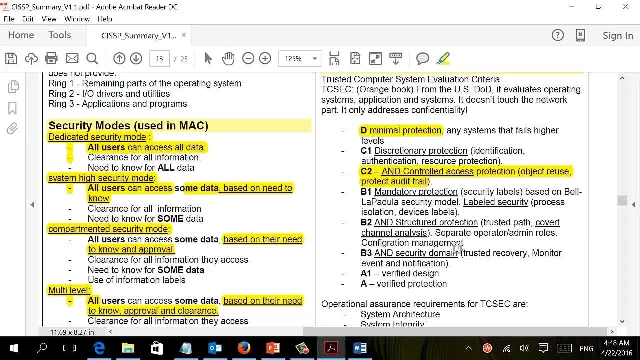 This is B3 and so on. So this part need to be memorized because this is very important, Important for the exam And you'll get the ask. Okay, according to TC sec, If you have a system that can provide Mac and has a labeling and so on, which one do you consider? 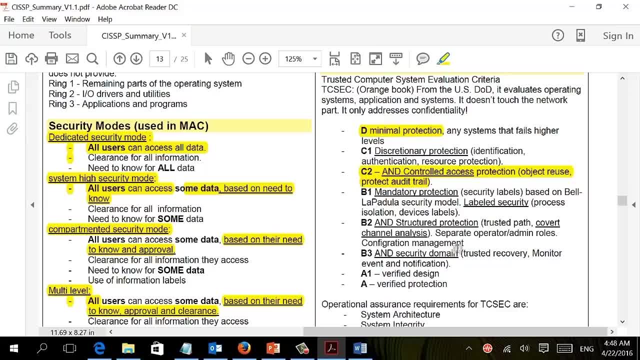 This is D or C1 or C2 and so on. So I'm afraid this part going to need a memorization and this is the only one where we're going to need a memorization. I mean later on or the next lecture will be talking about IT sec and an IT sec. 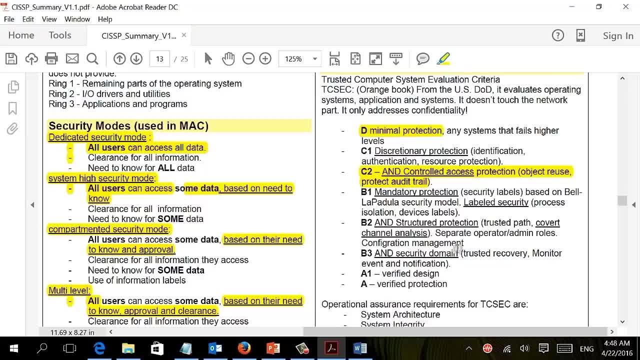 You'll notice that we have also some category, But you don't Need to memorize that much of detail. This actually was quite old. I mean, it was like maybe 20, 25 years ago. Now we are using different way for evaluating, but you still going to need to memorize that for the purpose of the exam. 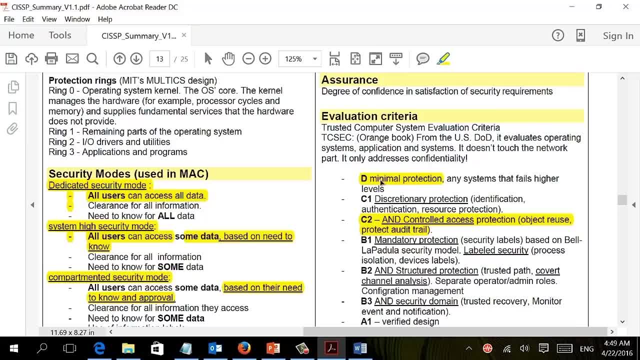 Don't forget the way of evaluation. This was an American way because the second one is the next one will be British, So this one was an American, introduced by nest. another name for it was the orange book. So he may ask you about the TC, sec or orange books. is same way and you're going to need to memorize those. 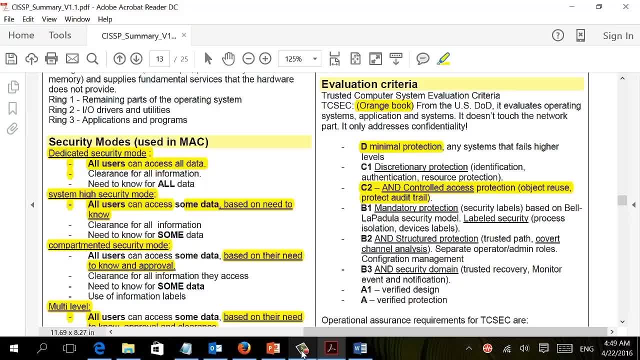 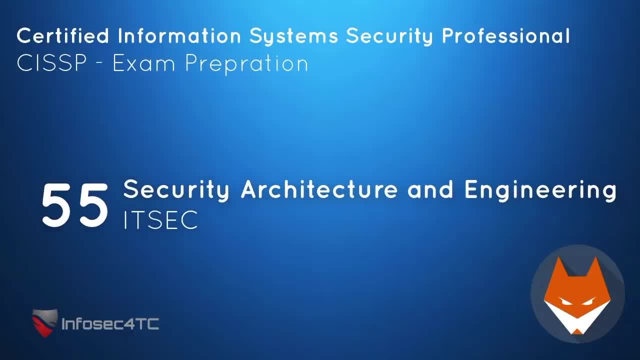 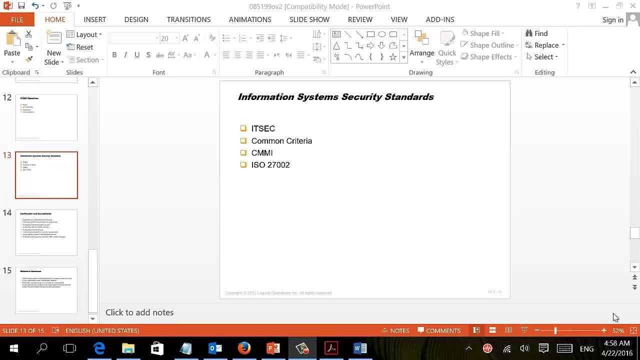 Categorization of the system. Last lecture on the security architecture where we will be talking about other kind of evaluation system. I mean on the previous lecture We spoke about the TC sec which came from nest and DoD and it Has another name, department orange book. 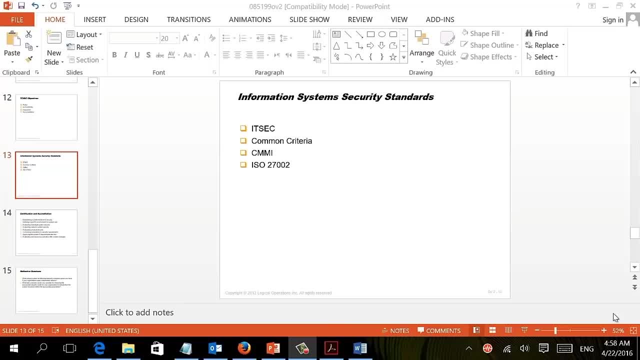 I told you, by the way, you have to, given you have to have some idea about the different books that nest have. They called the rainbow book, at least the major one, and this actually has been written inside the sunflower document, So you don't need to search for it. 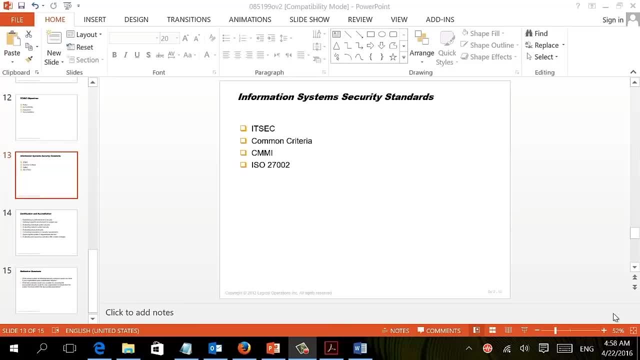 So the green- I'm sorry the orange- is about the trusted computer base, which is a hardware, software and operating system. the red is about the Network and I believe the green was about the password. That's mainly what you need to know about the rainbow book. 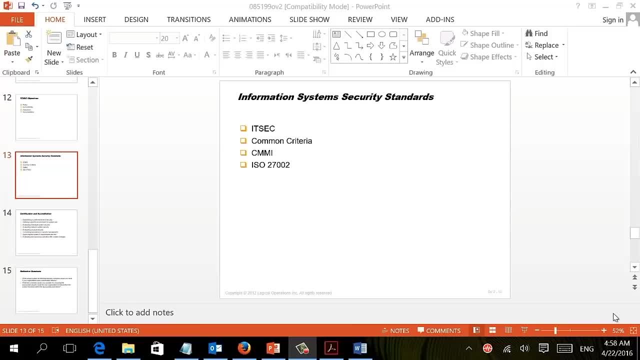 But the details you need to know, the details about the orange book, which is the category I showed you in the last, in the previous lecture, how they are categorizing and how they are able to measuring the efficient, the security of the system According to the features that it can provide. now the IT sec. 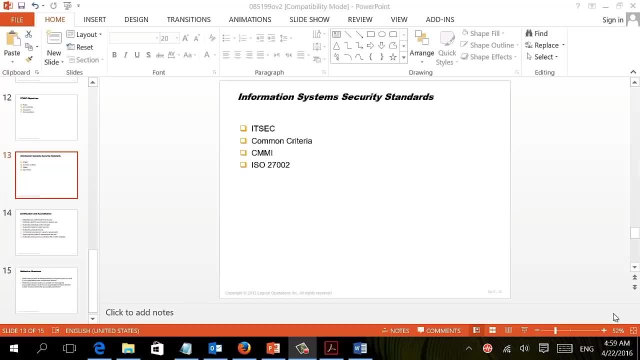 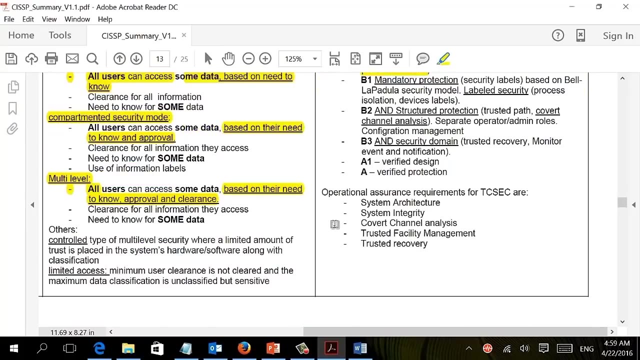 It's an American standard. There is another standard is called the IT sec, And this is actually. it's a European standard And it's similar. You don't need to memorize all the things that I asked you to do on the previous lecture, except you need to know what is the difference between the IT sec and the TC sec. 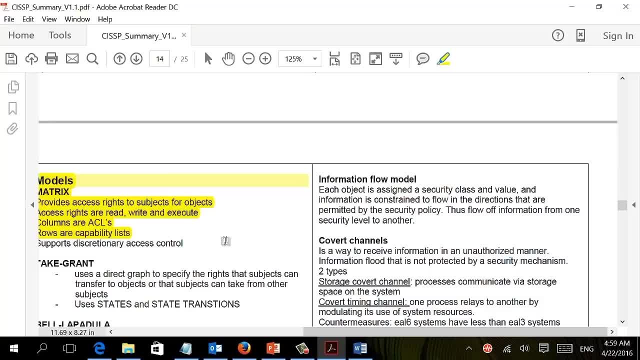 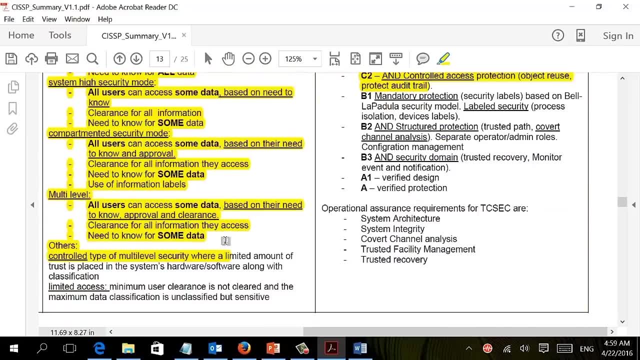 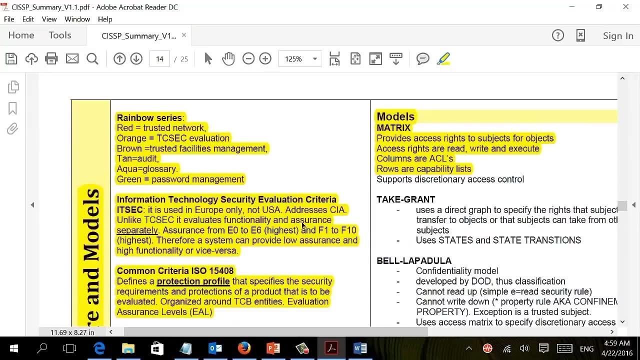 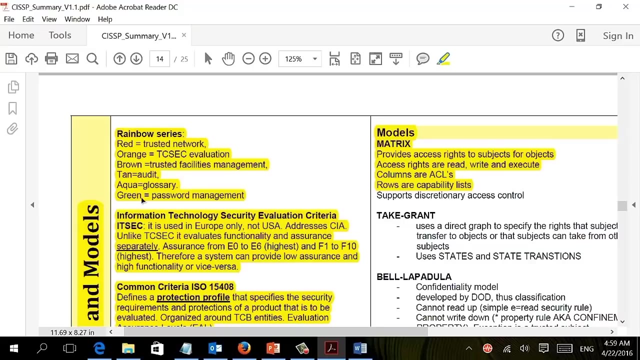 So let's see and get and check the IT sec. Now, the IT sec was different in a way that it was not just measuring one thing. Okay, let me show it to you. So in IT sec, Okay, Let me just. Those are the rainbow table books that you need to know, the red and trust and orange and brown. 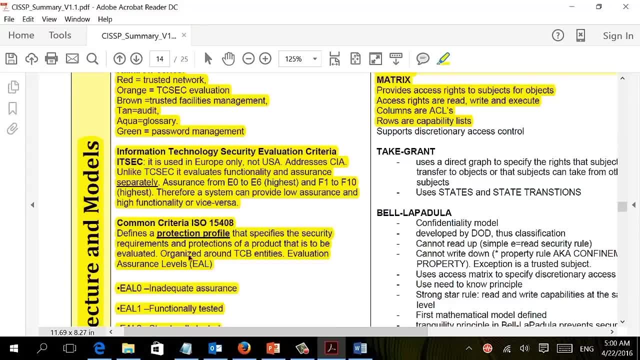 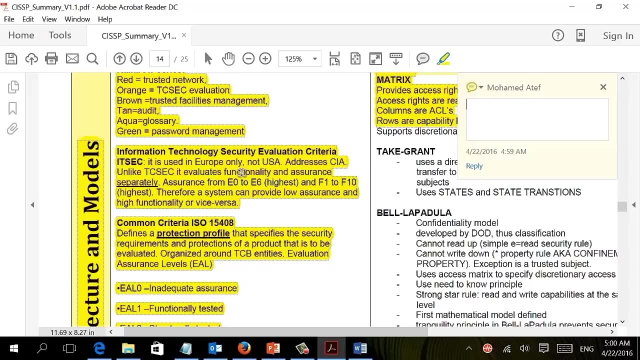 Just have a look about them. And let's talk about the IT sec. IT sec was different in a way that it was not just testing The security. it tests two things: the functionality and the assurance. It seems that I so here. you need to know this part that the IT sec tests the functionality and assurance. 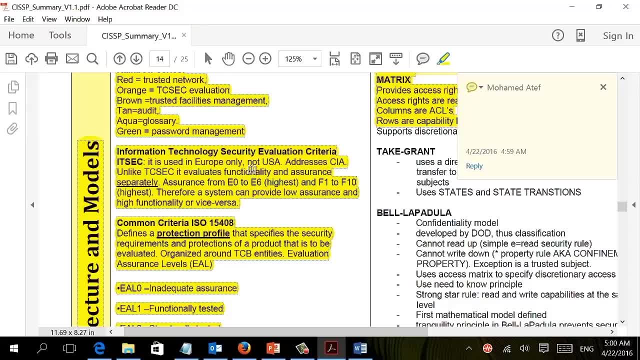 What is the difference between them? now, functionality- It's the assurance- has a scale from a to zero, from a zero to a six, where a zero is lower and a six is a higher, while functionality is from one to F10.. You don't need to know if one mean what and if two, you just need to know that we have two. 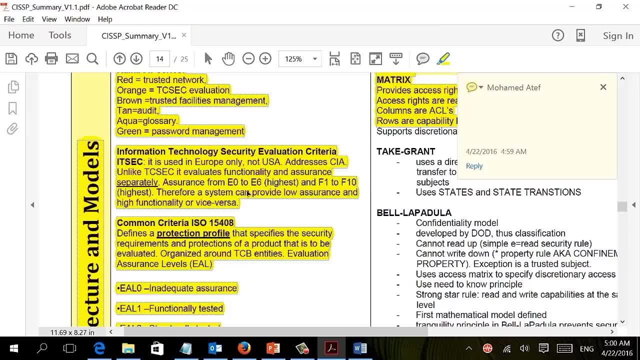 Two parameters that we are using for testing. Now, what is the difference between functionality and assurance? When we are talking about functionality mean they are testing if the system can do something or not. So, for instance, if the system are capturing log, this is a functionality inside the system. 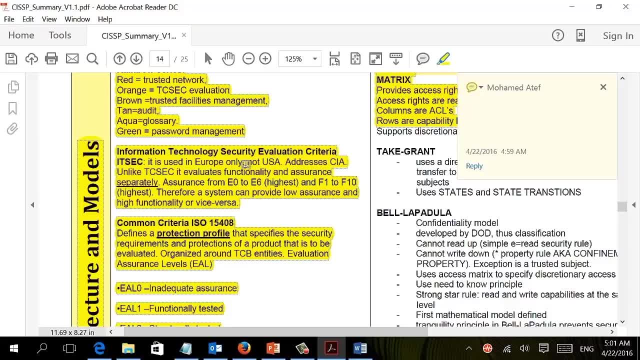 Assurance is to test if the system is doing that all the time or just sometimes it's do that or sometimes not. It's, it's Continuously of the functionality. So if the system is doing that all the time, this become assurance. So assurance it's to make sure that the functionality it's, it's done every time. 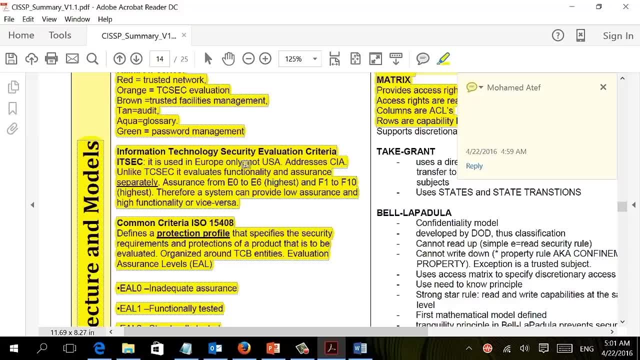 So the main things that you need to know about the IT sec Is that it evaluate the functionality and assurance, while on the TC sec It only evaluates the functionality, and the functionality has from F1. To F10, where F1 is lower and F10 is higher, and the assurances from E0 to E6, where R0 is slower and higher. 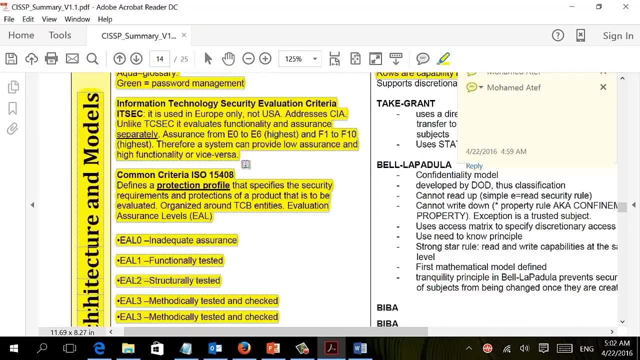 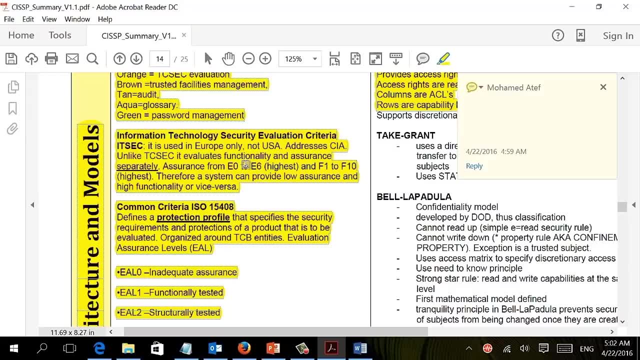 So those are two way for evaluating the system. Third one, because actually the problem with TC, sec and IT sec that it was main academic and besides it was very expensive to provide a high level of security. So they came up with a another way for evaluating system is called the common criteria or ISO. 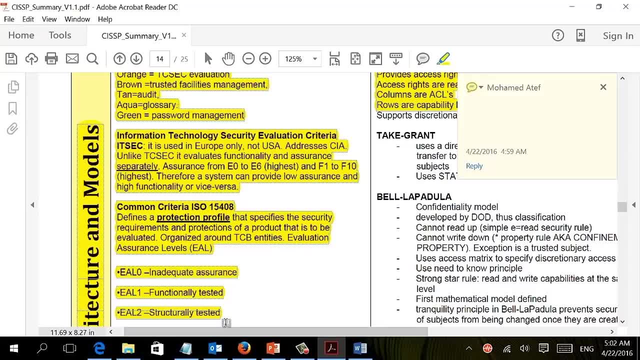 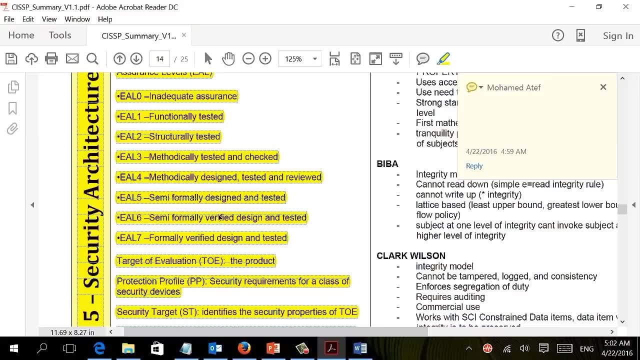 And it's quite different. It has AEL from 0 to 7, and it start by identifying what exactly you need to measure, because it's the target of evaluation, And then You're going to be sending or you'll be receiving a protection profile. 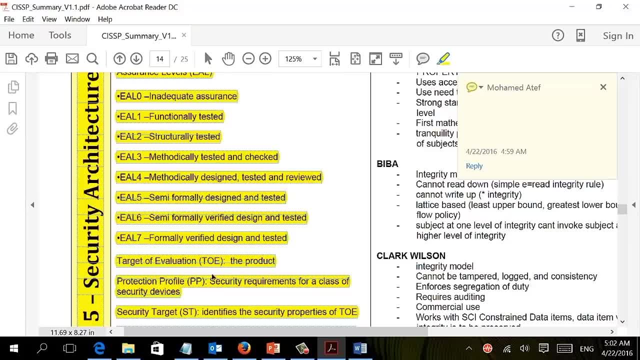 So ISO will send you what exactly need to Be Implemented on the TEO. So you said, okay, I have an organization I need to have implement ISO. They will send you the protection file. You need to implement those controls. You implement whatever you want to implement and then you send them the security target. 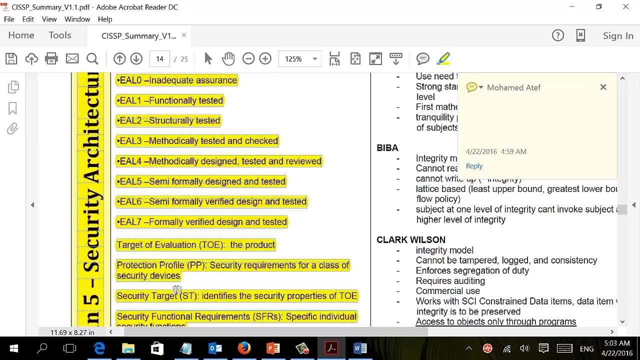 You tell them. this is what I did implement with a very big, heavy check. They'll come and they will audit you and you will check that your target of evaluation has a proper PPE. So what you are sending is ST security target and they are. 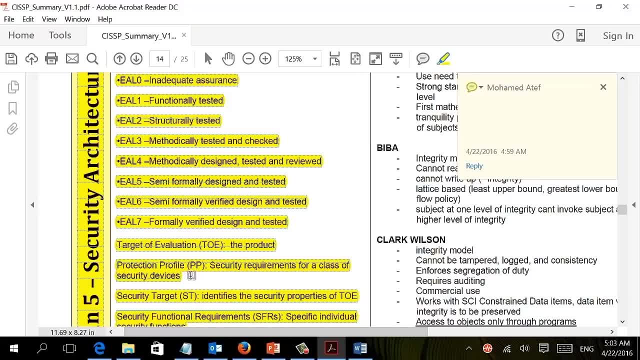 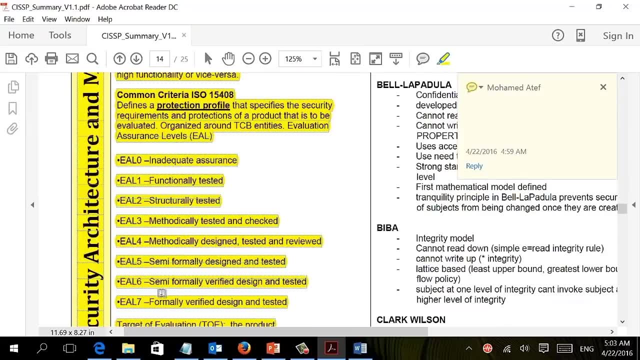 Comparing between the protection profile and that they send and the security targets that you send and make sure that you implement the security control and according to that you can certify. So you just need to know what is the common criteria and how they are measuring that also here. 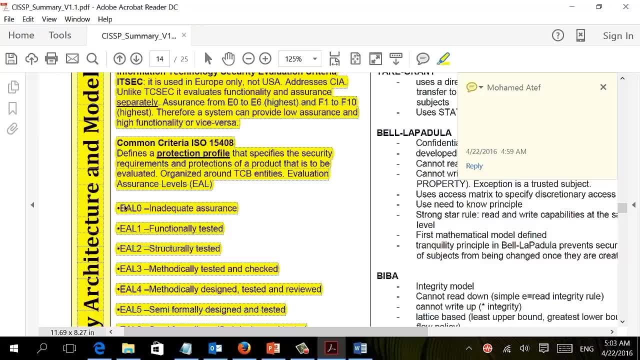 You don't need to know those definition, just the ways that they are evaluating and what is a 0 a, 1 a or how they are evaluating system. On the next lecture We're going to start by preparing for the exam. I mean it's kind of tricky module because a lot of terminology and academic, so we need to focus about some points and then we need to go and take some questions and see how I'll be getting question about this part inside the exam. 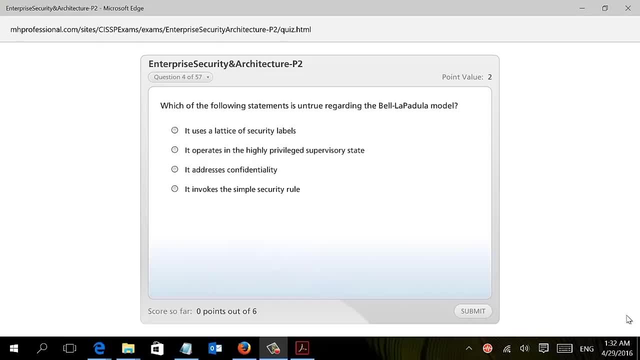 Now Let's take Some question about security architecture, just to get the idea about the type of questions that you may expect. So, for instance, which is the following statement is untrue regarding the Pella la Padula model. Don't forget: untrue. 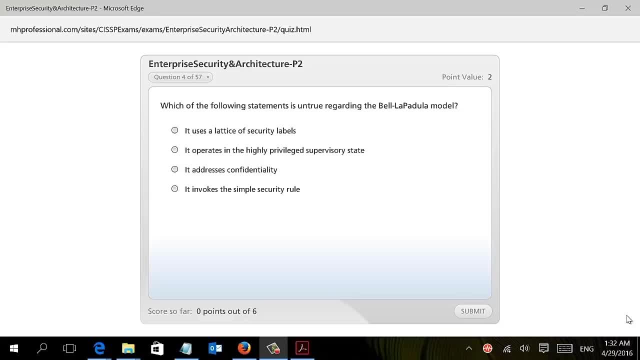 See, they usually do that untrue, which is not applicable, the least this kind of thing. but the good thing, as I told you, they put that in bold, So it will be quite clear. It's a latest security label. Yes, it is That it's open. 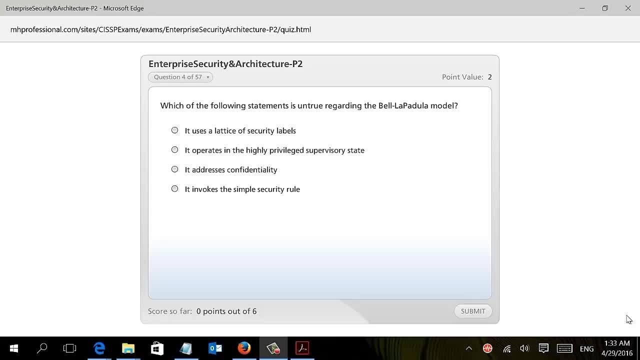 It operate. It is a highly privileged supervisor state. It addresses confidentiality: Yes, it address it. invokes the simple security rule: Yes, it invokes it. So the only one remaining that it's not true is the second one. Let's see. sometimes this technique work. 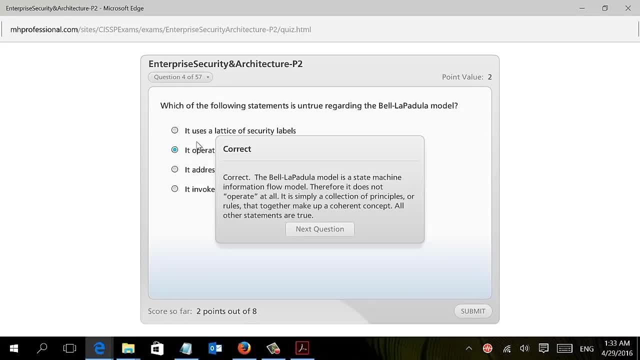 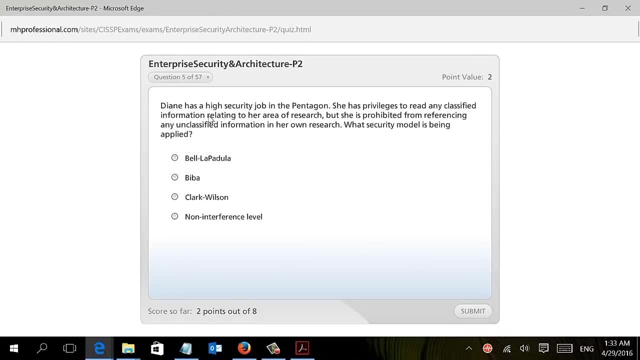 I mean sometimes one of the answer you are not aware of. so you can eliminate the ones that do not apply and if it end up with this answer, this will be fine. Next question: High security job in Pentagon. She has a privilege to read any classified information related to her area for research, but she's prohibited for 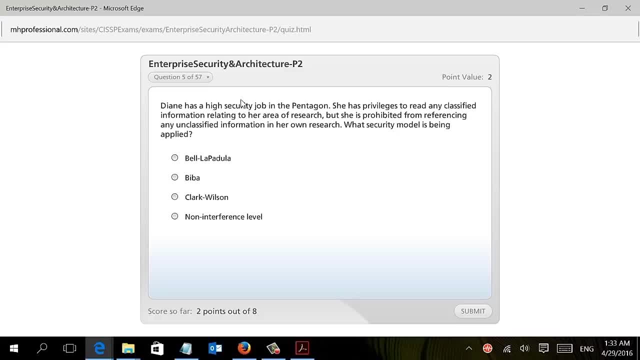 Referencing any unclassified. she has a classification clearance, but she cannot read the unclassified. which one is doing that cannot read down, Not read down or write up, It's a integrity model, Not confidentiality. and which one has an integrity model, It's Baba. 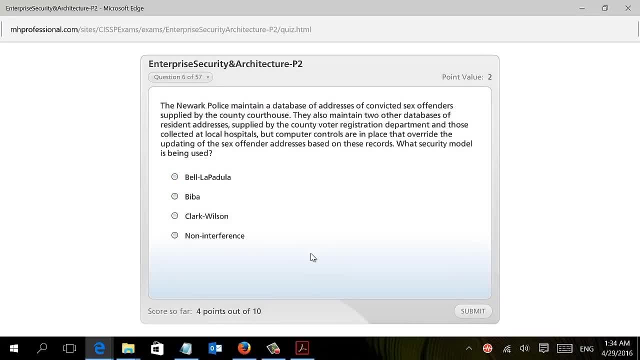 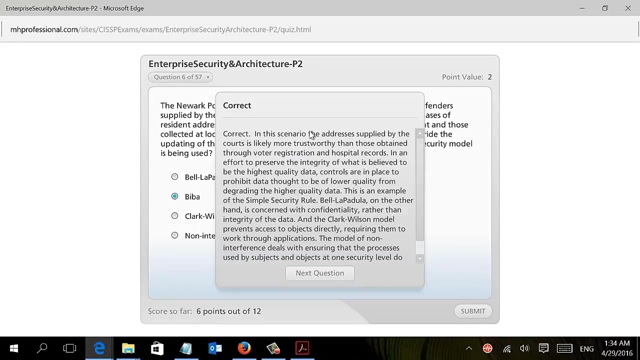 So this should be this one. Let's see this question. Maintain two other database? What security model? I think this one is very, very important to read the explanation Because, as I told you, one of the objective during this training is to get the mentality of ice square, and this will come by answering as much question as you can. 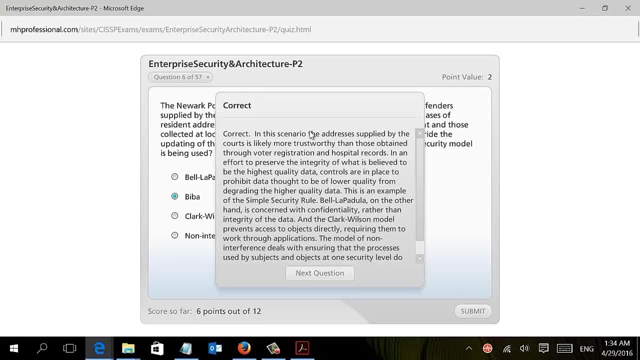 So it's very important to read the answer. Even if your answer was right, you need to know that you sought the same way. ice, ice, square are thinking, or it's just a coincidence? Okay, let's one see one more question: hacker gain access to a secure system. 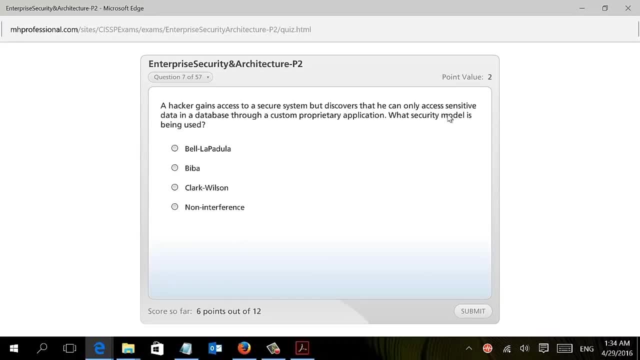 But discover that he cannot or he can only access sensitive data in the database through a customer proprietary application. Now, do you remember? we agree that when you see a keyword, application or software- which model is, it should be Clark Wilson. So Clark Wilson is a model related to you. 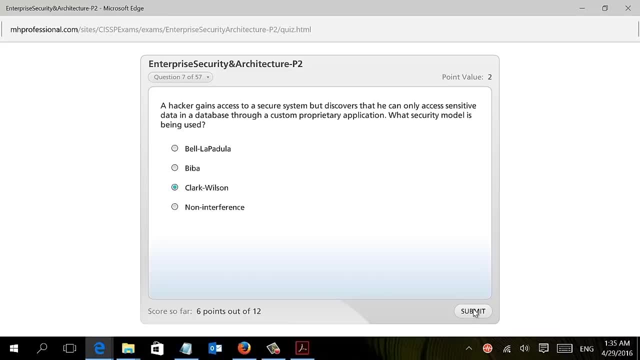 User access information through an application. So this is a Clark Wilson as well. So you are getting the idea, But the point is that you have to solve as much question as you can just to get those tricky point inside the question and also the get to get the mentality of ice square. 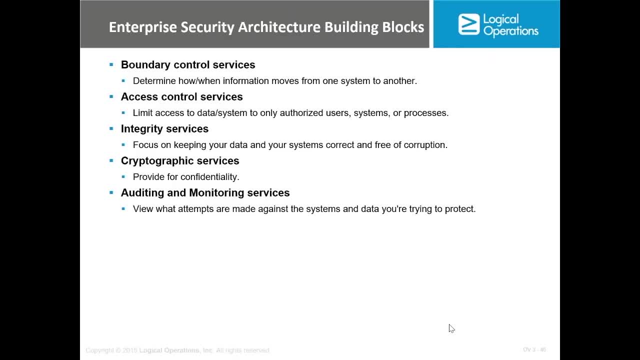 This is a very challenging domain. We still have a lot of topic to cover. I mean, we already covered The Security models. We're going to talk about cloud security. We're going to talk about physical security, cryptography- different topics- all under the name of security, architecture and engineering. 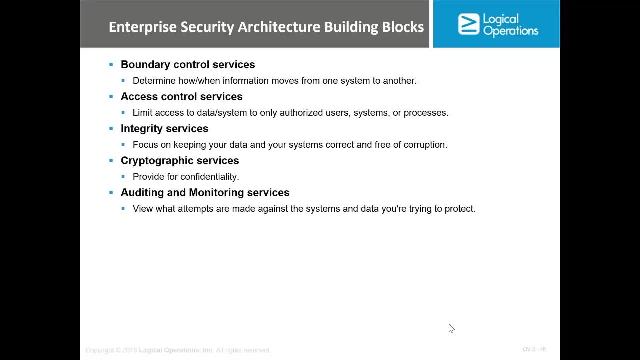 And you may face some problem. try to relate topic together. That's why, from time to time, I'm going to raise some guidelines. you know how we can implement so far What we explain in like some major guidelines, And this is one of the lecture where we're going to do that. 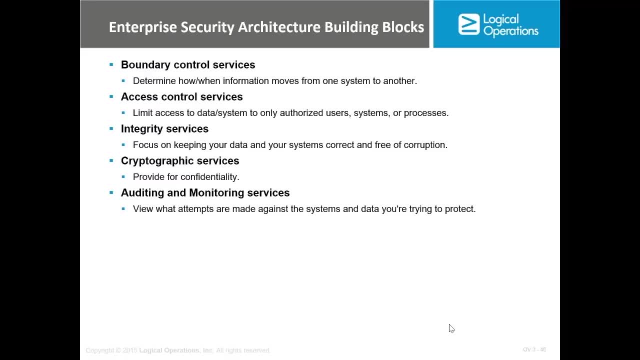 We're going to just show what is the enterprise security architecture- buildings, rock. If you consider your company or your organization security architecture, what should be the major item in the implementation in general, And then you can apply whatever we spoke about Or we're going to speak about. 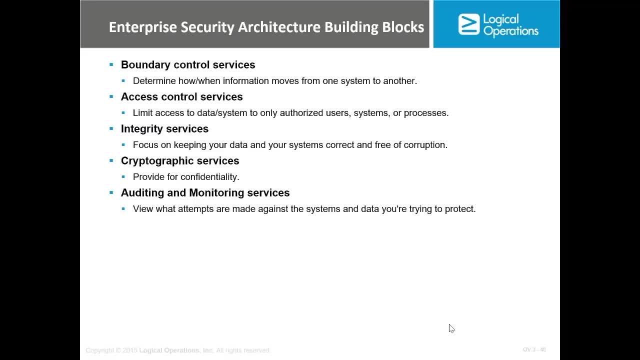 To those five guidelines. first, you need to have a boundary control services in a sense that, as you know, it's all about information. This is an information security courses, So you need to understand the information It's sitting where and it's moving from where to where and how. so, if you have like a web application, how the information are moving from one web application. 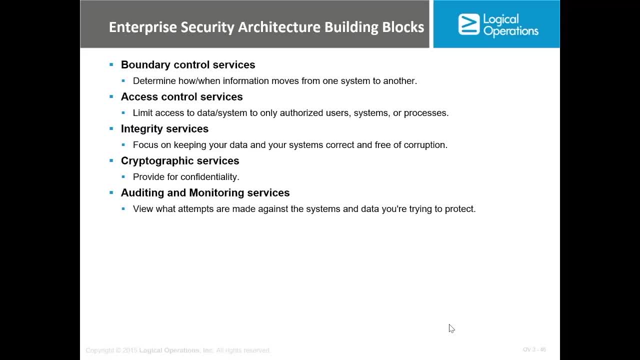 To another web application, If you have or you are exchanging information through emails, through media, How and when the information is moved from one system to another and according to that, you're going to decide which control you're going to implement. This is one point. second point, which is quite important, is access control services. access control will be explained in depth. 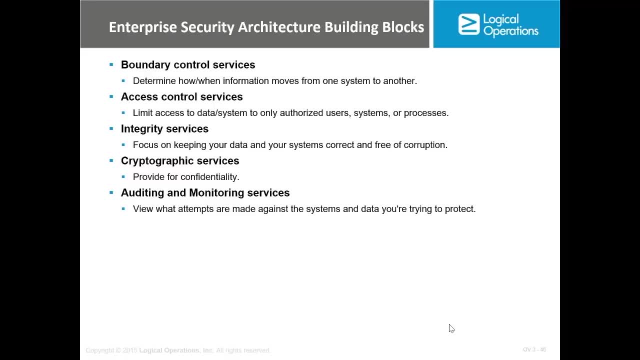 After two domain And One of the domain where you will get a lot of questions about. so still, you need to implement access control and, as you're going to see in the access control domain, It's not about assigning a password. access control also referred as the AAA- authentication, authorization and accounting. 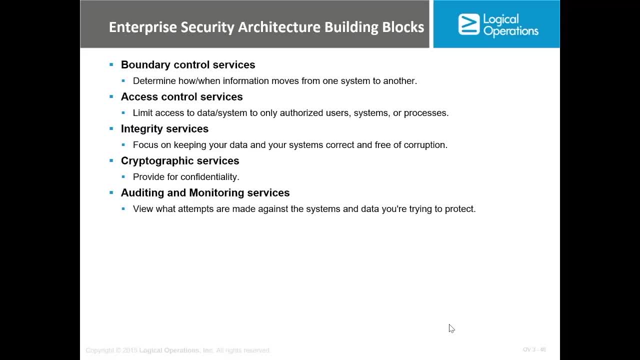 So this will be explained in depth in the access control, but it's one of the guidelines inside the enterprise security architecture: The limitation of Access to the data system. I should not allow everyone to access the data. I should only also allow authorized people. then integrity service. 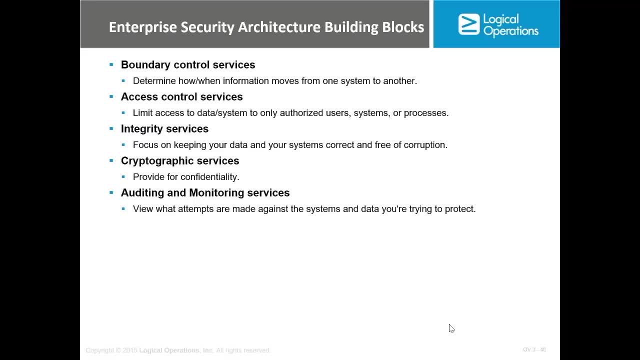 Very, very important. Maybe you have your information But you do not have some integrity control. Some information can be manipulated, intentionally or unintentionally. So you are working on it and, like in a bank, and people are writing down Customer transaction and customer. 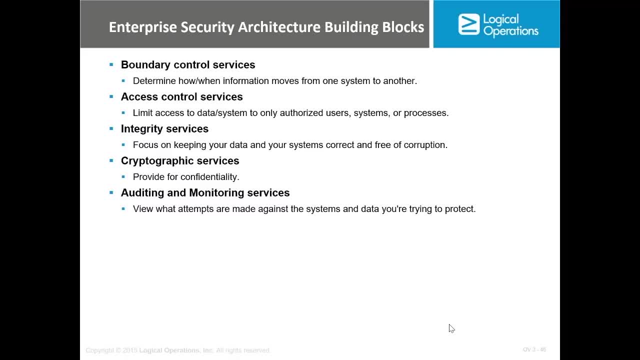 What if? unintentionally is the change your number? This is against the integrity right. I'm not talking about intentionally someone are- are men in the middle, attack and change the information. I'm talking. someone by mistake wrote something wrong. Do you have a control against it? 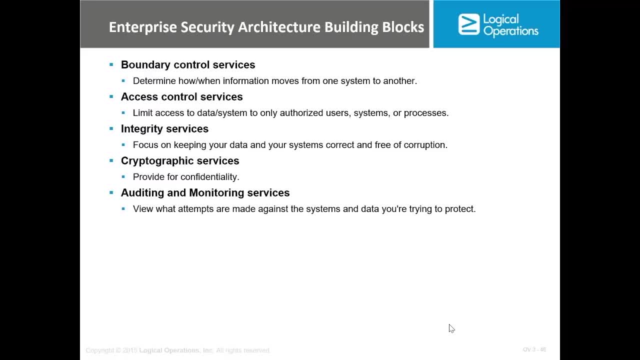 Yes, we do have a control and we're going to see in the operation security That we can Make people. We're going to see that we have a control where we can verify each other work in a way that even by mistake I did something, you know, someone will review it and will fix this mistake. 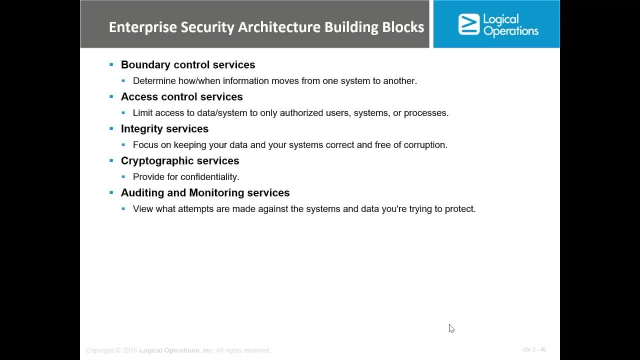 So integrity- it's for an intentional or unintentional modification of the information cryptography service. Also, this will be covered in depth in this domain We're going to talk about everything To cryptography and, most important, the auditing and monitoring service. Any information security implementation system will have a frequent audit. 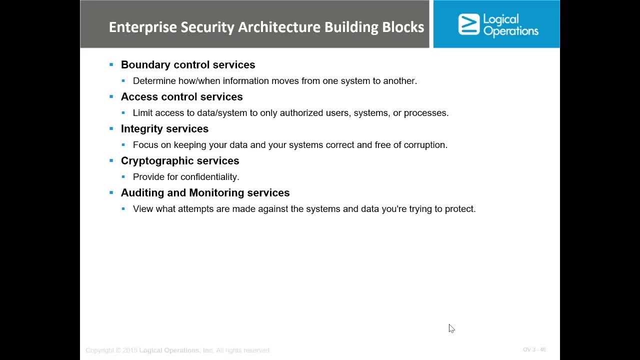 You need to make sure that everything is going according to the plan and you need to audit that frequently: Every one year, every three years to renew a certificate, and so on. So we do not just implement the control and that's it. We need to have an audit plan, and we have. we need to have a monitor. 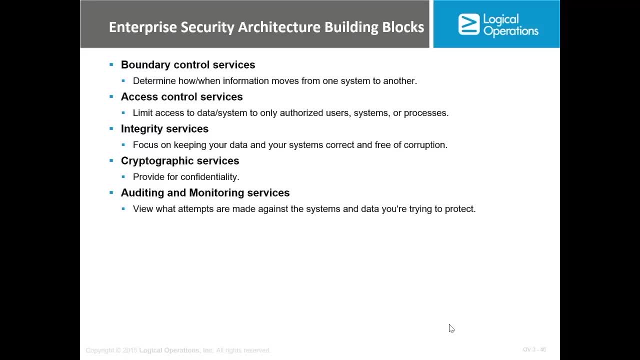 Your mythology. I should monitor how things is going and actually this is quite important. So those are some of the guidelines that will help you in general while you are building your enterprise security architecture, And you can apply whatever we spoke about so far and we're going to speak about in the same domain on those five different guidelines. 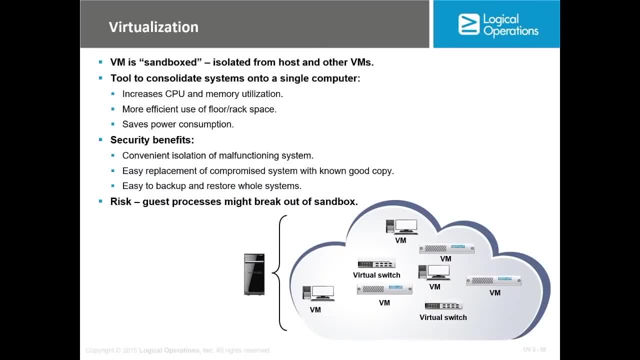 The upcoming few lectures will be about very small topics. Just in each lecture We're going to give you a brief about one of the service that maybe exist in your infrastructure or in your organization. You just need to be aware about it in a sense. 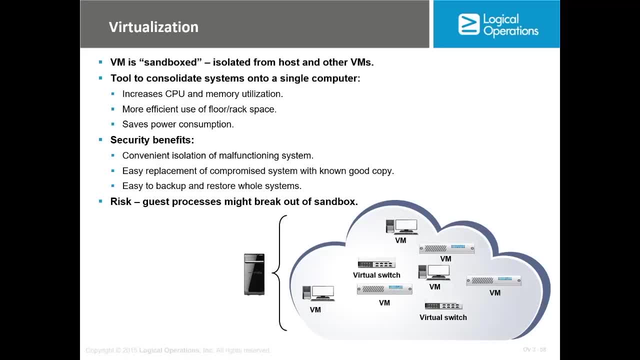 You need to know what is the benefit of having such services or technology and what is the disadvantage or of having that And some terminology related to it. Now, this part of the domain where we're going to talk about virtualization, We're going to talk about mobile security, cloud security, big data and so on. 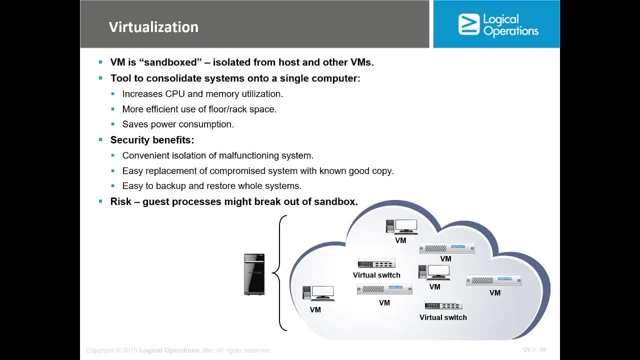 It. it map to the same concept, that just having a brief about it, in a sense that you don't need to dive deep into the subject. So when we are talking about virtualization, if you didn't use it before, you need to understand. 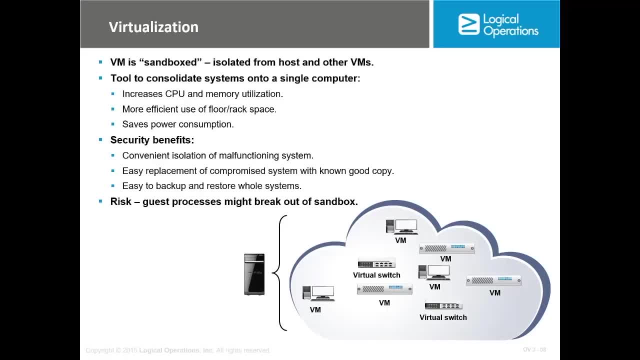 What is virtualization and why we should use it in our architecture, and what is the risk related to virtualization. When we will be talking about mobile security, We just need to know what is the benefit of using mobile in our architecture and what is the disadvantage of using it. 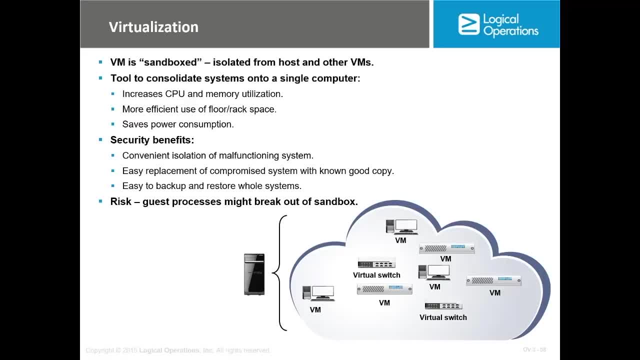 And so on and so forth. So it's not like we are talking about virtualization So we need to start studying virtualization set Very deep. You know that this course is not about that. The course is only about giving you like the definitions and always remember the saying about the CISSP. 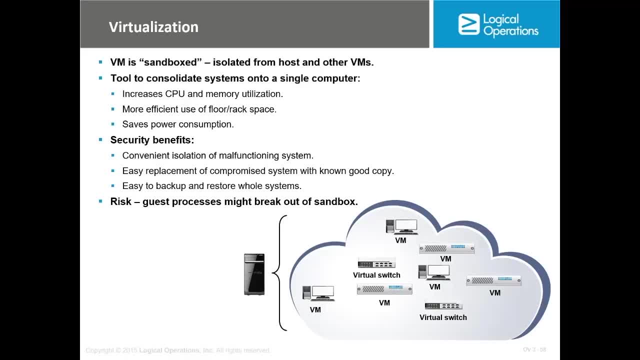 Which is it's one mile wide and one inch deep, in the sense that we're going to cover a lot of topics in this course, but you need to understand only the basic definition about that. So let's start with virtualization. Each lecture will be just one topic, but I think by getting those few lectures, just having an idea about it. 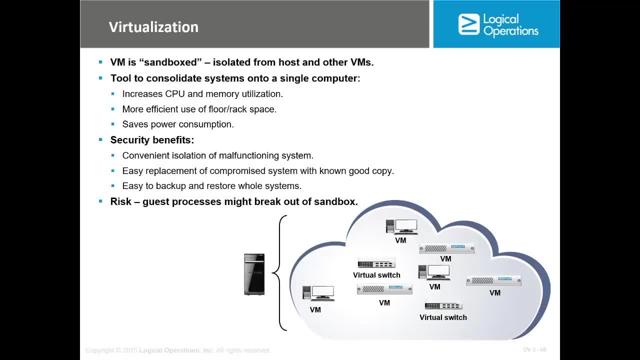 You don't need to go deeper than what I'm going to say regarding those specific topic. You will will guarantee like four or five questions inside the exam, because they usually ask about virtualization, They usually ask about mobile security. Just one question. You don't want to lose the questions. that has a couple of lines that you need just to have an idea about it. 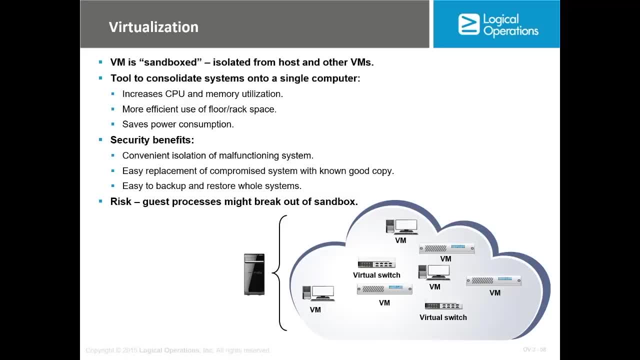 Besides, The only topic that you need to be familiar with- because recently there was some good amount of question about it inside The exam- is a cloud security, because cloud, you know it's start increasing in our business right now. So only cloud. you need to dive a little bit deeper. 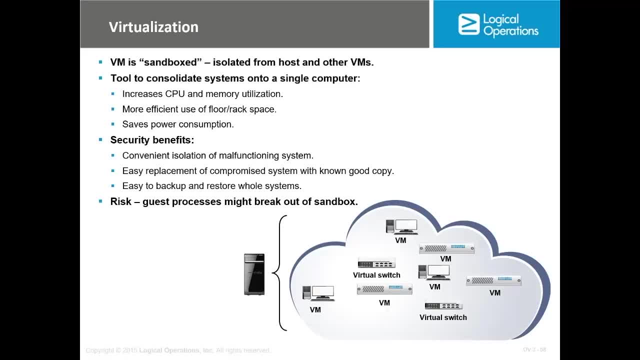 But actually I will not let you search here and there. I'm going to put for you few cloud lectures from my CISSP course. that will be more than enough to understand The different cloud services, to understand the cloud architecture and the cloud security. 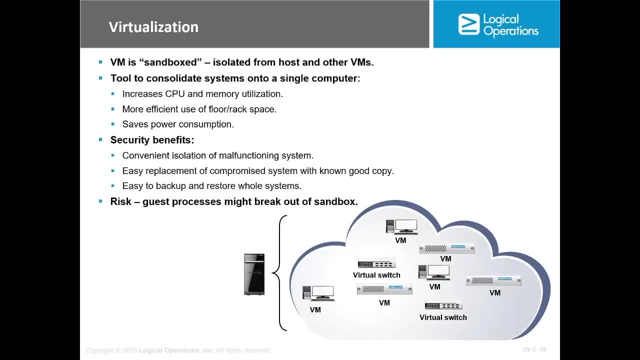 So I'm going to add more lecture about cloud in this domain, because it's all about not losing questions, So it's quite important to know the amount of questions that we get, usually related to topics. Let's start with virtualization. virtualization, as you may know it, just having a virtual. 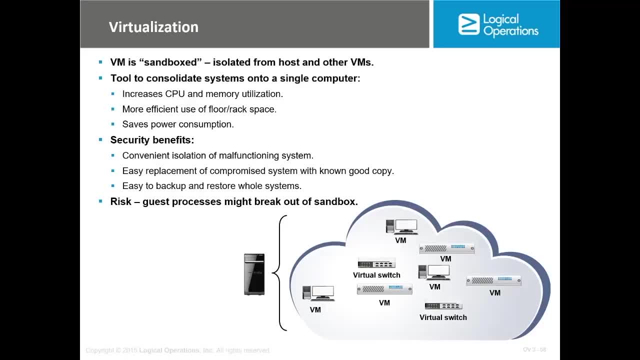 System on your physical system, So on my physical computer, on my PC here I can have a virtual machine, one or two or three, and they will be acting like a physical machine. What is the benefit of having that? definitely it's Cost effective because I can get one computer or one server and run on it four or five virtual machine, instead of firing or buying four or five. 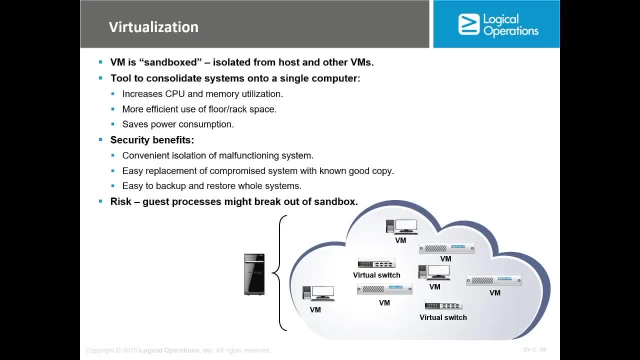 Computers. so definitely cost is quite a benefit here. We also have a security advantage, which is the system- the VM or the virtual machine, is usually isolated from the host in a sense that if it get affected with something or any breach happen, it will be Only the virtual machines that will be affected with that. it will not affect the host machine or the physical machine. 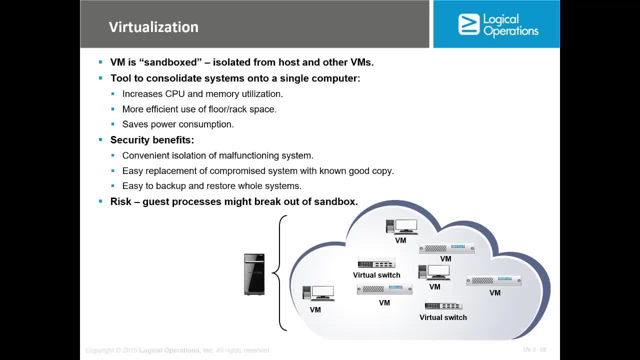 So from a security perspective also it has a benefit. We have some consideration like tool to consolidate the system onto a single computer. if you plan to have a virtual machine into your Single computer, What do you need to consider? you need to consider that this virtual machine, it will take resources from your physical machine, so it's not like having five. 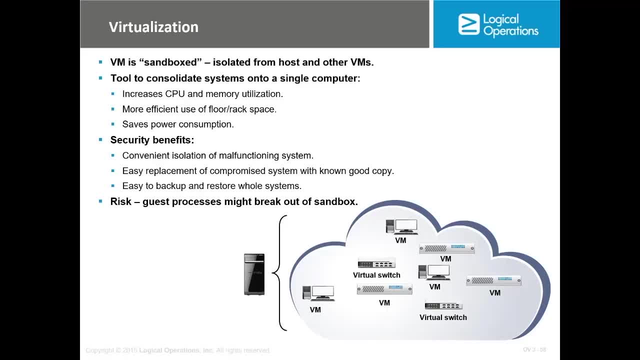 six, Seven, eight virtual machine on my physical machine. do you have, do I have, enough memory and enough storage to support this virtual machine? because they don't have a processor by themselves, they don't have a storage. they are taking from your local storage, from your local hard drive, they are taking from your memory. so you should consider that. 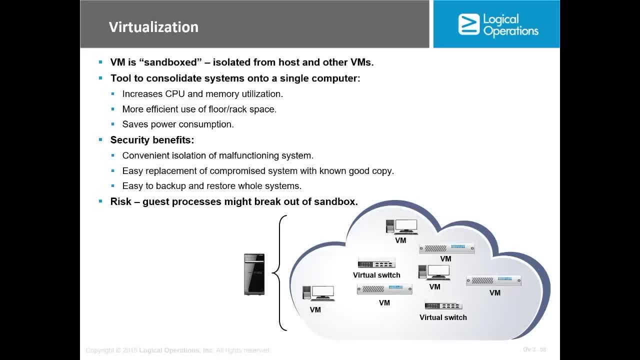 Security benefit, as we agree. it's completely isolated. It's easily replacement. The good thing about the virtual machine: it's like a file, which I'm going to show it to you in a few seconds, you know so it's. it's usually as a file. if you need to copy a virtual machine from my computer to your computer, I just can take this file, copy it on a flash disk or something and give it to you and then you can open it from your computer. so it's quite easier to move than a physical machine. 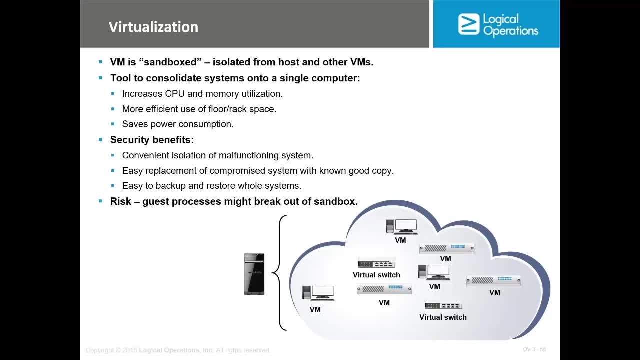 And I'm going to show you that in a few seconds, is easily backed up and restored in a whole system. This is the benefit. what is the disadvantage? usually it's related to availability. what if the system breakdown, crashed? So usually it's the risk that you have that the guest process might break out the sandbox. 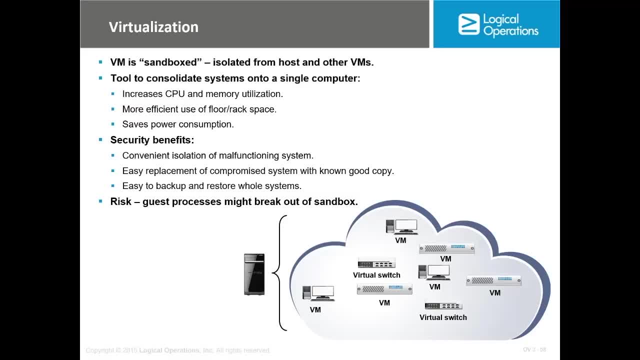 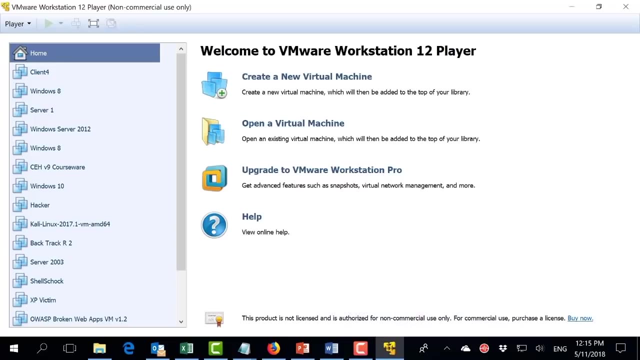 So if you have your physical computer crashed, all the virtual machine built on it would be crashed with it. and let me show you a small example about virtual machine and just To like clarify what we are saying. This is VMware player workstation. It's a free VM. 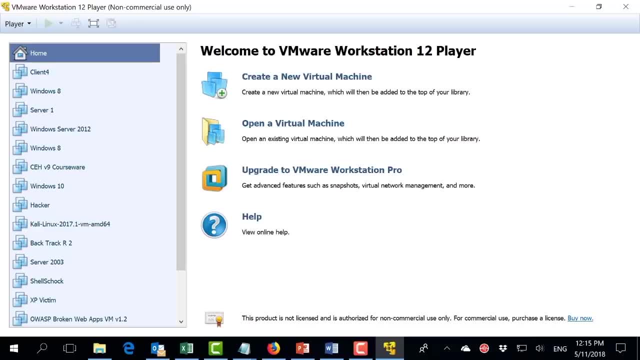 Application. you can download it from free for the for free from the internet, and there is different products. that is virtual box, There is the virtual PC, Hyper-V, different product, but this is a very common one and, as you can see, I have many, many virtual machine in a stool. 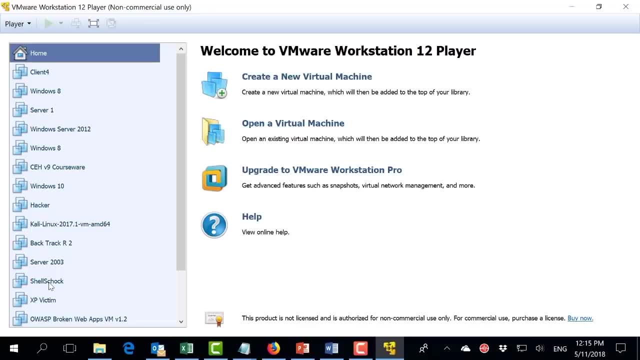 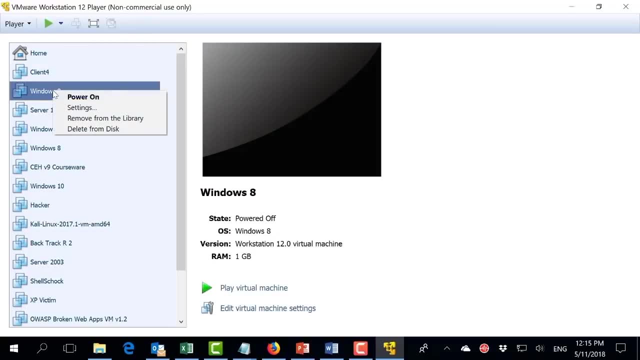 I have a Windows server, I have a Windows client, I have some Linux machine And so on and so forth, And if you go to any of those machine like Windows 8, this is already installed. I mean, if I right-click and power on, it will start the virtual machine into my physical machine. same concept to the server, and so on. 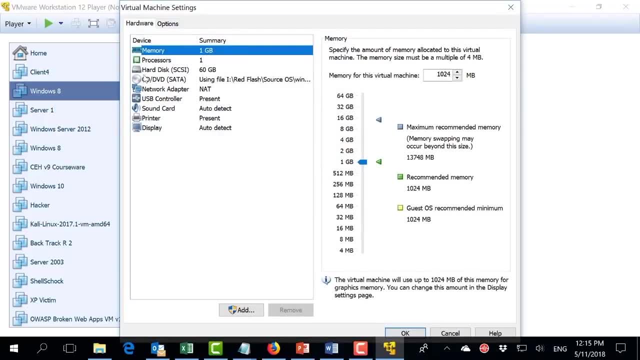 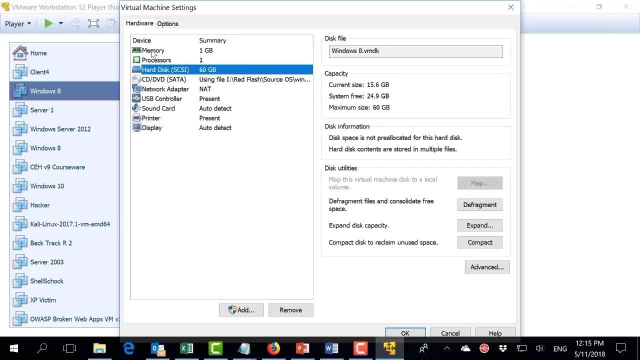 But let's go to the setting, as you can see this virtual machine. What is the hard drive space is 16 GB. from where it's getting the 60 GB from my physical computer? What is the memory? that it's taking one GP. So it's taking one GP and I can modify that. I can make it to, I can make it 512. 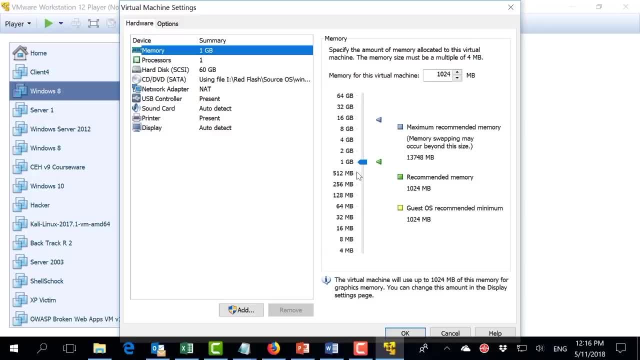 512 mgb, but it's taking from my physical machine and accordingly I cannot open many machines in the same like time. I have to make sure they are taking enough storage. and finally, or also you can check here, the location of my virtual machine. 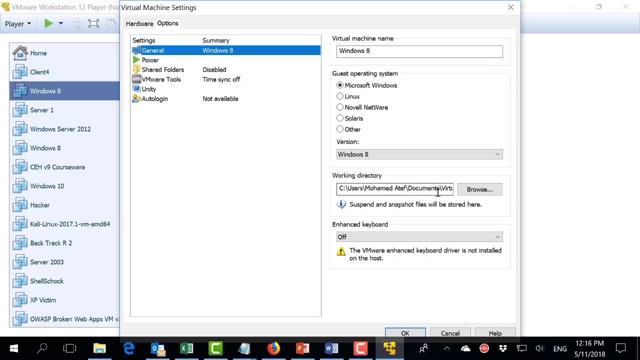 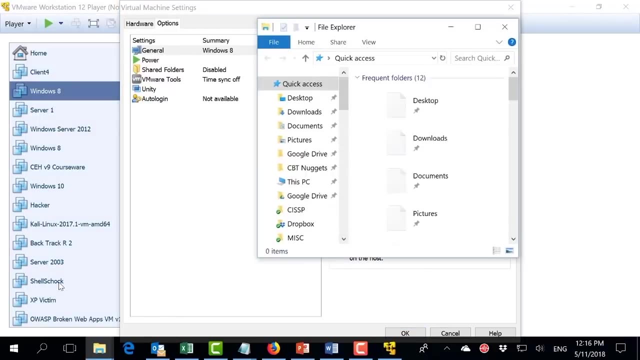 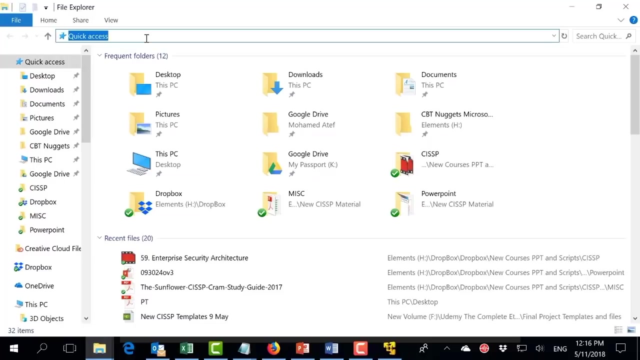 So, as you can see, this virtual machine are located in this storage. So, for instance, if we take this space, Okay, let's go to the space copy and open from an Explorer, And if you open from here File Explorer, just to see the location of this virtual machine. 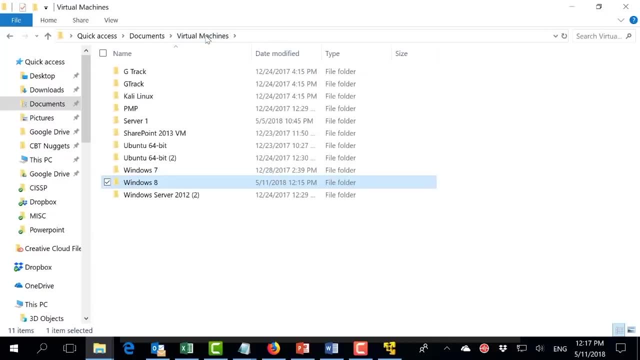 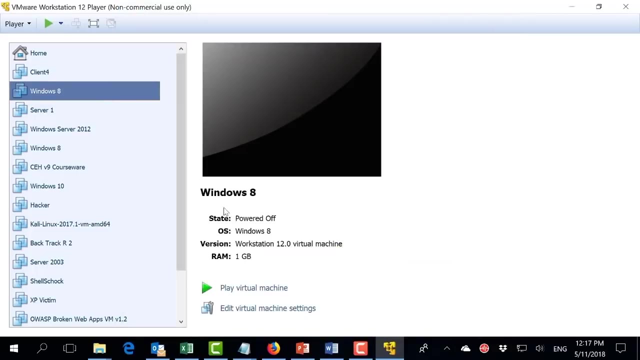 This is the virtual machine file And if I need to move this virtual machine from this computer to another computer, I'm just going to take this file And put it on another computer and install the same program, VMware player. Then I can go and to my home here and I can go to open virtual machine and I can point to this folder. 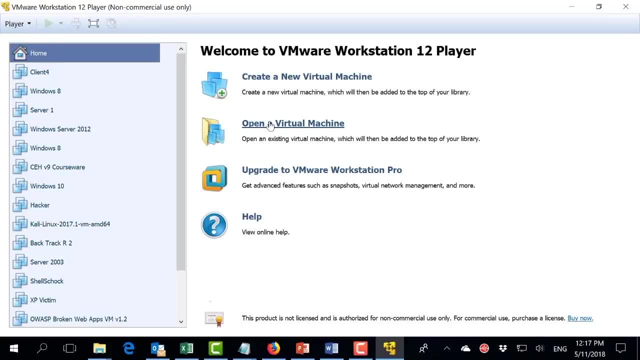 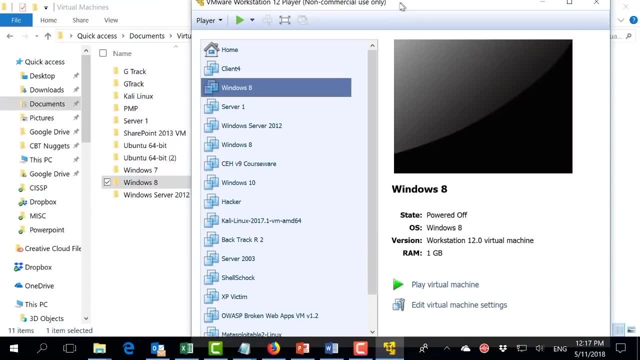 And this will open the same virtual machine but on a different guest machine. So it's quite easy to move that same way I was telling you and it's regular working as a regular machine. So, for instance, let me open a server for you here. 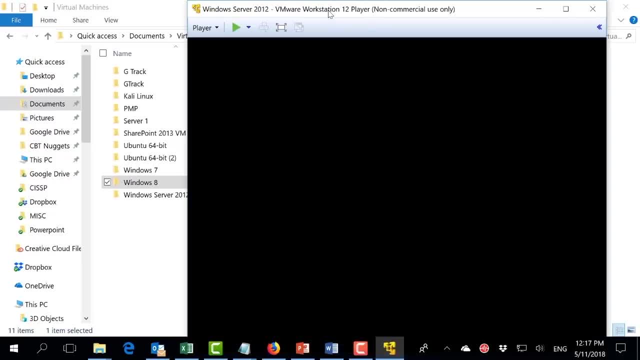 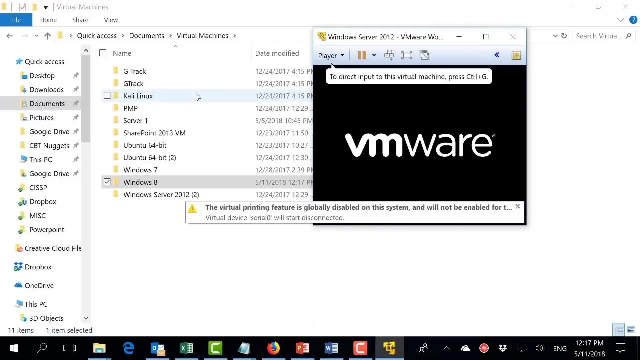 Just to show you, right click power on and, as you can see, I can have A server running on my same computer that has Windows 10.. And I can have more than one machine running in the same time. So this is the concept of virtualization. 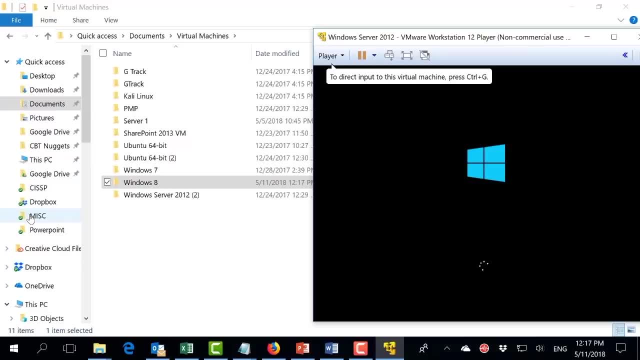 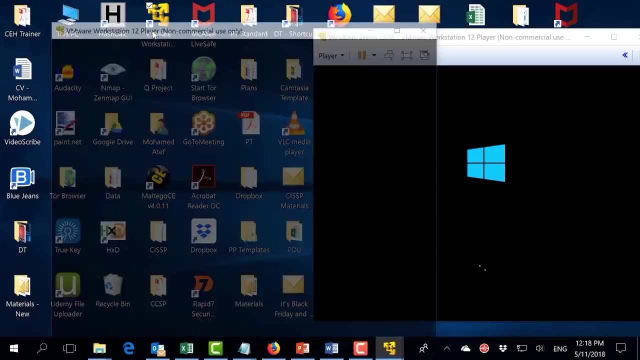 It's implemented in different enterprise right now because it's cost-effective, is secure. It has a lot of benefit, but you need to consider the concept that we explained earlier. If I need even to open one more machine, For instance, let me show you I can also open, for instance, Windows 8 machine. 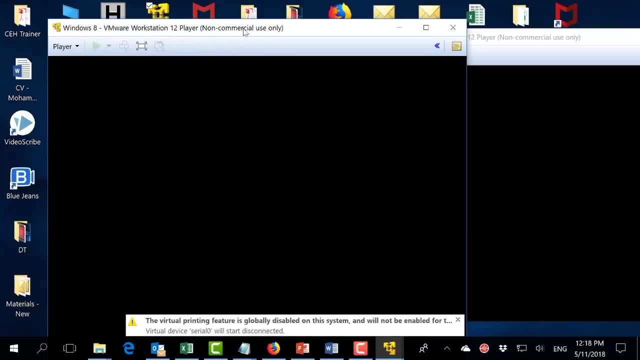 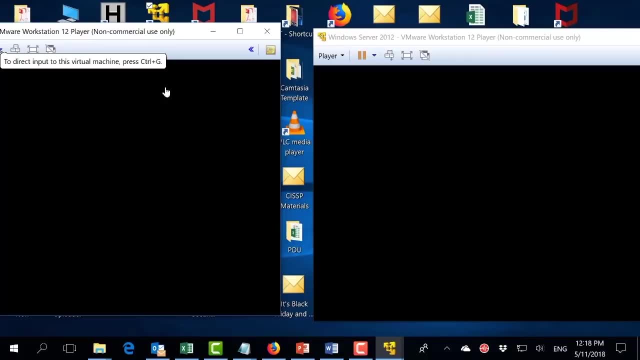 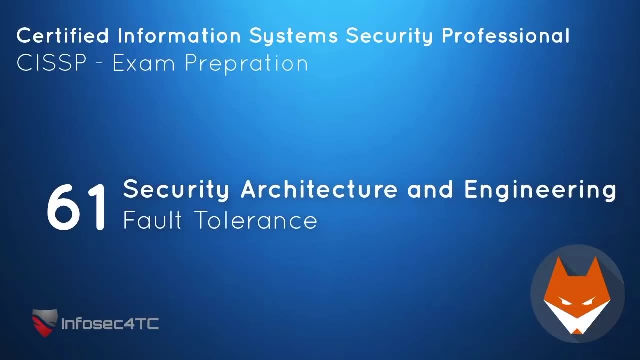 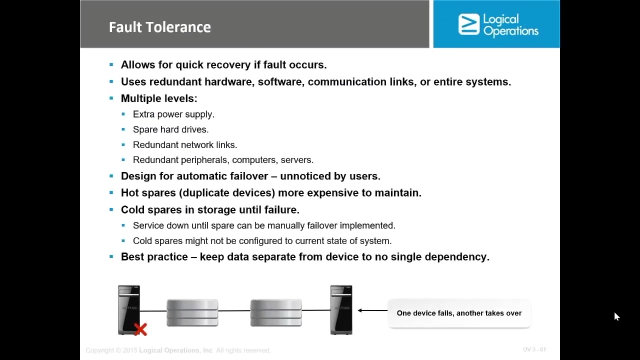 And by doing that, as you can see, I have two virtual machine up and running. I can have more. if I have enough memory and storage, I can have more. but the concept here, This is the virtualization concept. We spoke about virtualization. It was a very small topic, just to be aware about what is virtualization. 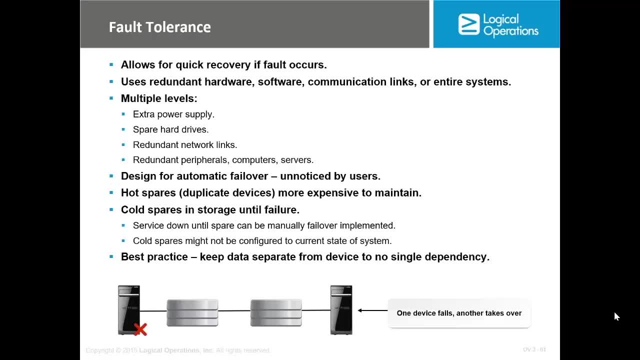 What is the advantage and disadvantage? next topic will be about full tolerance. Full tolerance is just to have a redundant system. So, for instance, if you have anything critical in your infrastructure or enterprise and you are worry Maybe it crash, I need to have an additional or it application for this resources. and I will give you a small example. 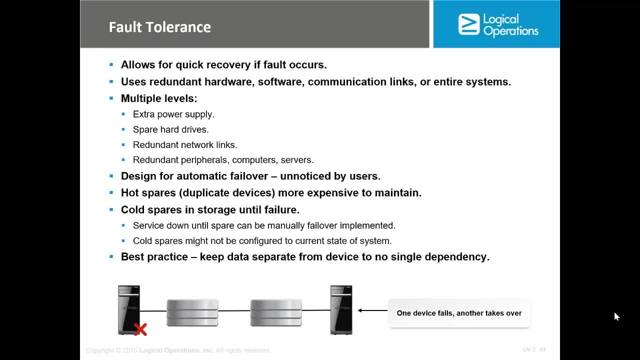 In your house You may have an access point where all your devices are connected to right. You have an access point or a wireless router and all your devices, like laptop, mobile, tablet, are connected to it. What if this hotspot or wireless router crashed for any reason? 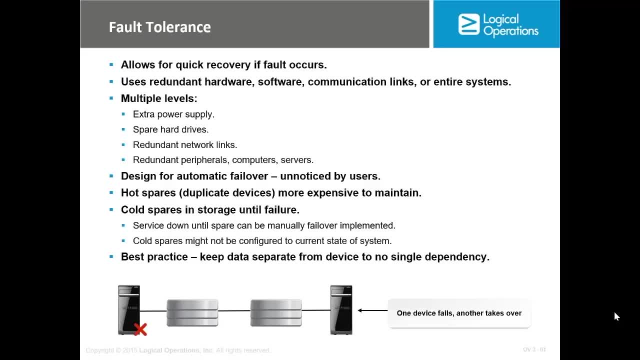 Your network, Your could be down. So for this device I need to have a redundant access point or another access point in a in a way that if this one fail, this one will take over and accordingly you should not have long Time, long downtime for your network. 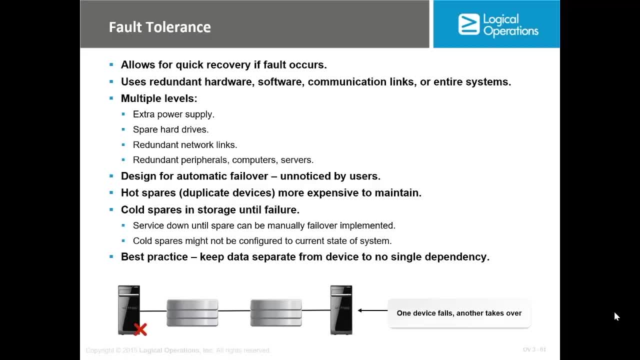 While your smartphone or your laptop. It's not considered a critical device because if it crash, You know, yes, it will be a small problem, but your network will be still up and running. So we need to identify what is your single point of failure. 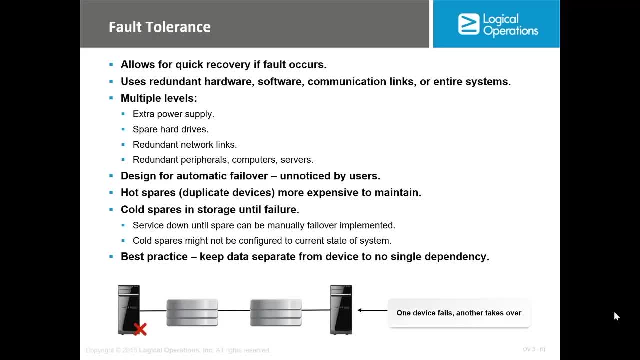 What are the devices that, if they fail, they will affect the full business, or they will affect your full infrastructure and have a redundant device for it. Okay, so this is quite important. What are the devices that you need to have a redundant or a replacement for? most of the time will be something like power. 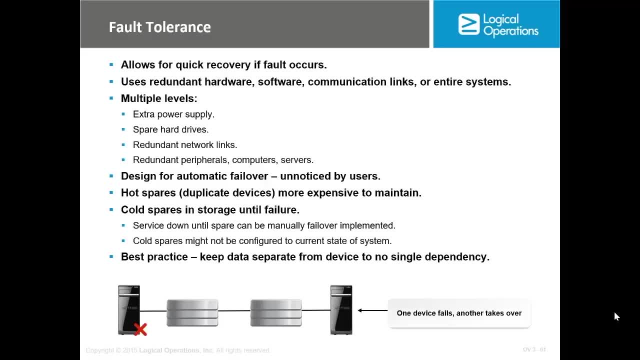 Because if the power crash, You will not be able to work on your device, So you need to have an additional power supply for your critical system. As I was saying, it's not like every device in your network. You can have redundant. 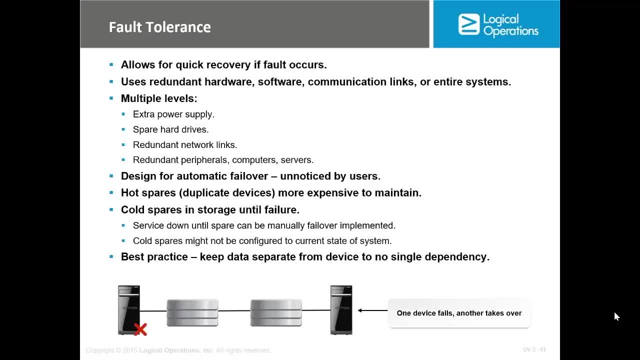 This is not cost-effective, but you need to understand which one is more important and which one will affect your infrastructure, Which one will give you long downtime and have another device for it. So, for instance, if you have In your company a lot of servers, you need to select which server are more critical to other server and then put a redundant server for it. 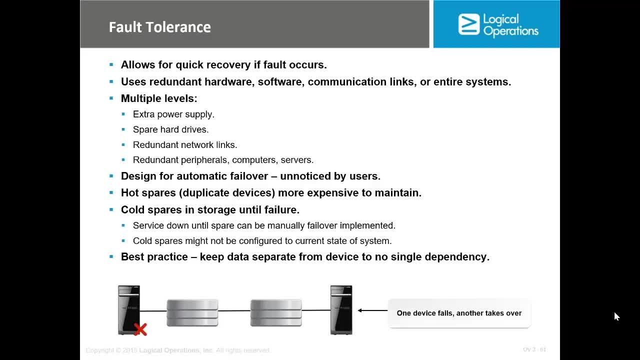 Client. same option also for network network link cables or switches. What if the switch crash it? all the network will be down. So you need to have a switch for that storage hard drive. You need to have a red 2 or red 5.. 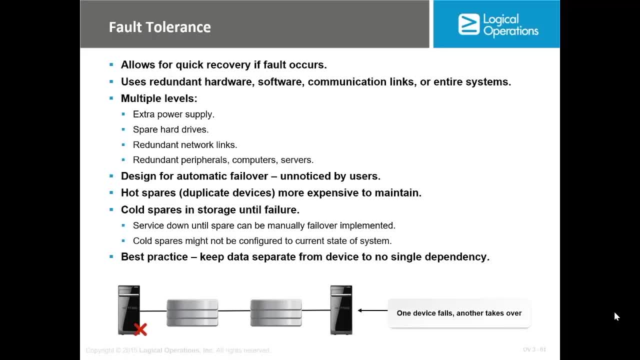 This is considered a redundant red one or red 5.. I'm sorry, It's considered a redundant storage in case something went wrong. So the concept of having a redundant because keep in your mind that security- I keep saying that because you don't need to forget that, for the example especially, security is not just about securing against malicious hacker. 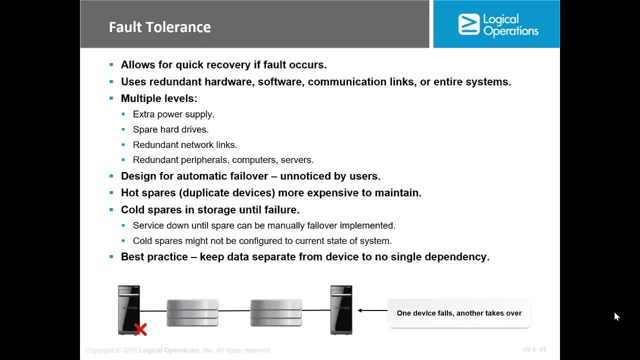 It's against against anything that may happen. hard drive crash, It happens. This is a physical device. It may crash. now It's not about the value of the hard drive, But it's about About the information that was stored on it. 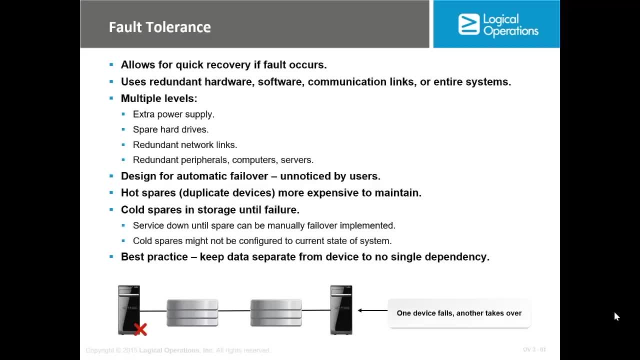 Did you have a backup? Did you have a redundancy in a way that if it crash, you will have another hard drive that will take over? So it's quite important to identify your critical assets or your critical devices and have a redundant for it. So those are some of the guidelines. as I told you, you need to have them as a multiply layer or a multiply levels in ways that, if you want, 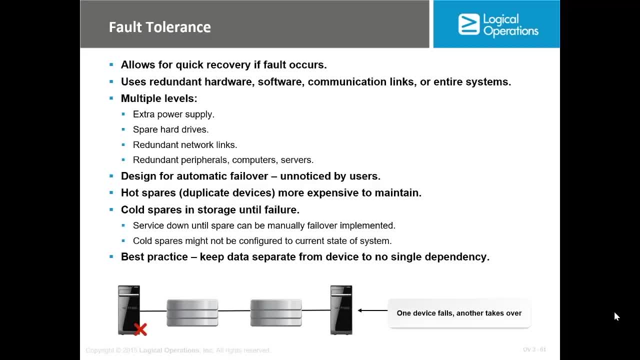 You can have a redundant, another crash You can have redundant. in this way, You need to have an automated failover process. So you have a for instant and another hard drive with all the information that are you going. if the first one crash, Are you going to remove it yourself and install the second one? 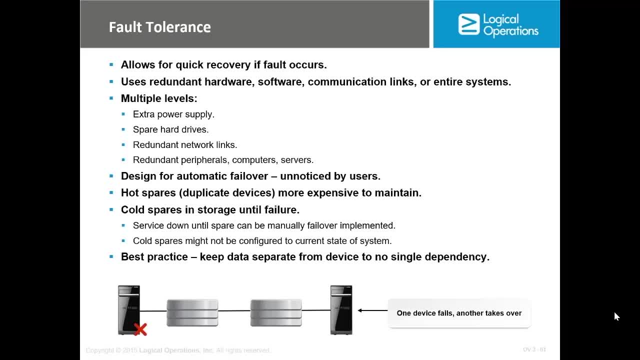 Or are you going to utilize for instant trade one which is a failover process to hard drive? You can do some windows Setting in ways that if one fail, automatically the second will take over and accordingly you will not feel any difference, You will not have any downtime. 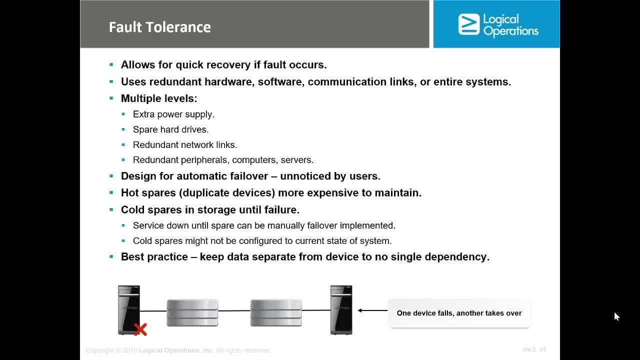 So you need to do the failover in ways that it should be done automated. You need to have a duplicate devices for the critical one. This is also related, as I told You, To the single point of failure, But It shouldn't be done randomly, in a way that I get there like a piece of paper and saying: this one, I'm going to replace this one. 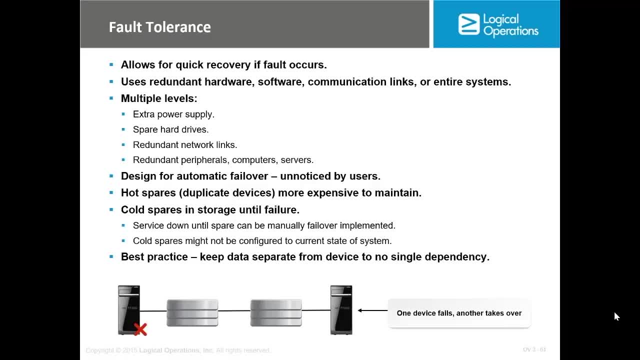 I'm going to replace. it shouldn't be done this way. There is some relation to topics that we already covered, like the MTD in the business continuity planning and the RTO and the RP. This point that was covered on the first domain, You need to be familiar. 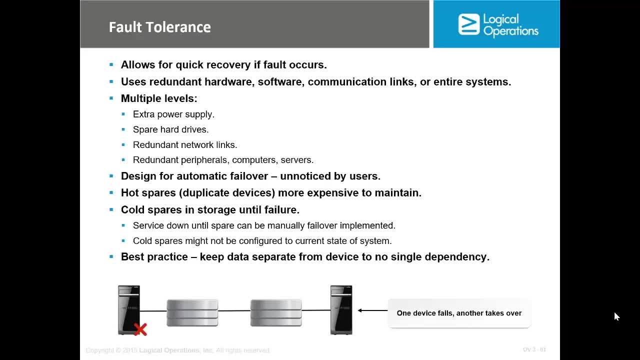 Which, In brief, How long the company can afford to have their network down, and according to that you're going to select which one is critical and which one will will- will help you get your system up and running in a shorter period of time. So the concept is clear. 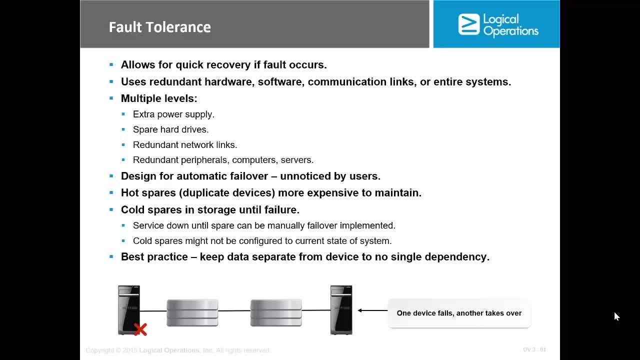 I believe. But the point is it should be based on the acceptable downtime And from where you are getting the acceptable downtime? from the management. You need to say to the management and ask them: Okay, how long can you afford to have your network downtime? 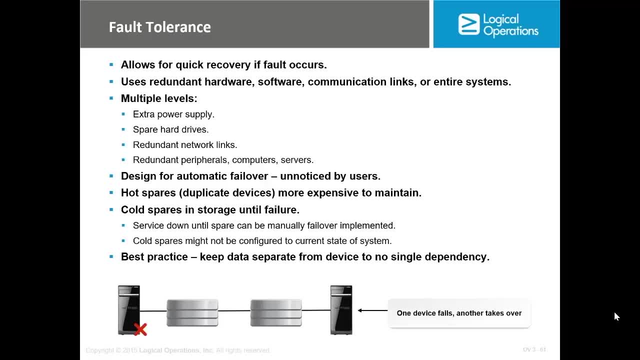 If they said we can have a downtime for a couple of days, no problem, I don't have to do any redundancy. I'm going to take backup for everything And if anything went wrong, I have enough time to restore and buy new equipment. 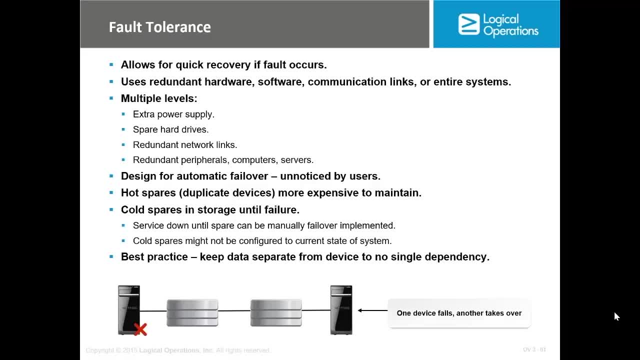 If they're going to say a couple of hours now, I need to think what can lead to more than two hours downtime and then I need to find the replacement for them. So the point is the full tolerance need to be built on values, Not a like random process to be done. 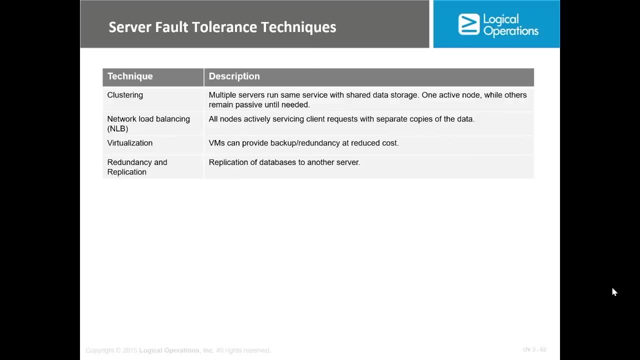 Some of the technique that can be used for the server- full tolerance. We are talking about the server level- will be something like clustering, which is very common right now, and clustering is just combining few machines together. could be two or more and they will be acting. 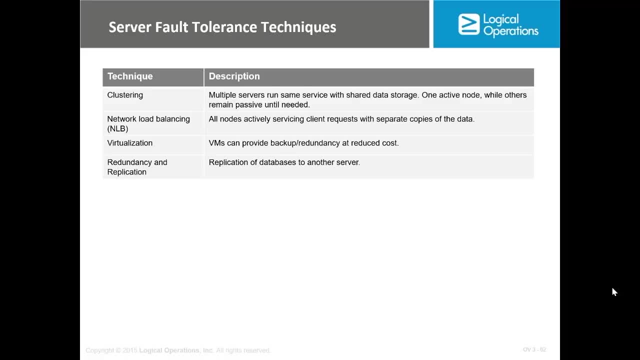 as one computer, so I can have two computers. They will have the same IP and they will be configured as a cluster in ways that whenever you install something on one computer, it will be automatically installed on the second one And according to that, if any computer went down, the second one will be up and running. is the same concept as RAID. 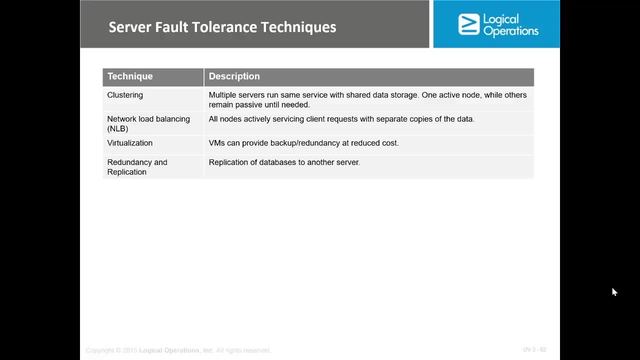 If you know about RAID 1, but on computer level We have the network load balancer or balancing, or NLP. This is not a really a full tolerant, but it's just dividing the load instead of having the load on one computer or one node. 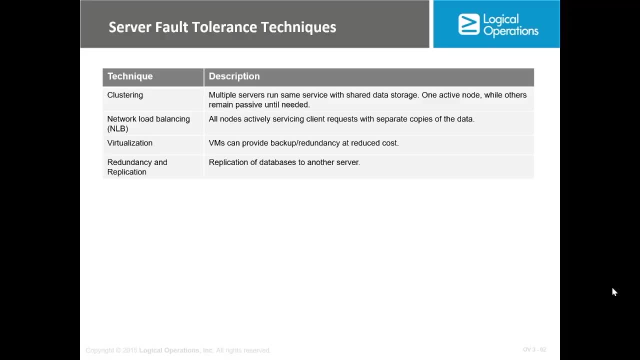 I can have it on more than one node, So each request coming to the server or each few requests will be divided between those two computer. I can use virtualization and we already saw about virtualization that it can be backed up. It can be redundant machine instead of having two physical machine. 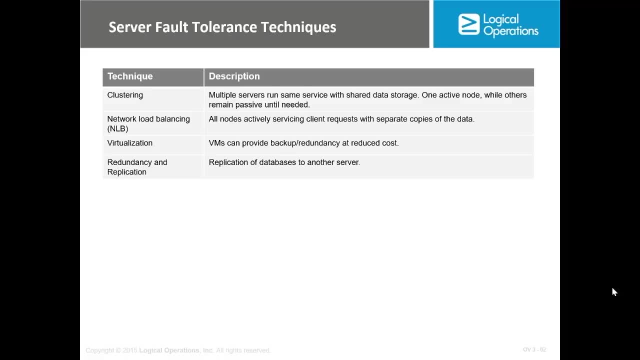 I can have one of them as a virtual machine. So if any Like server went down, I can replace it with a virtual machine, or I can have both of them as a virtual machine and work on a redundant solution. I also want to add RAID for storage, but actually in this slide he's just focused on the server, full tolerant techniques. 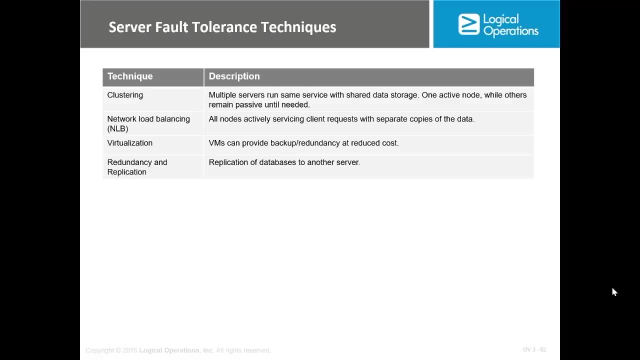 So especially the clustering is very common right now. when you install things like SQL Server, it's mostly recommended- because this is a database Most of your like to be very important to your business- Most of the process will be done on a cluster. So those are some of the server full tolerant technique. 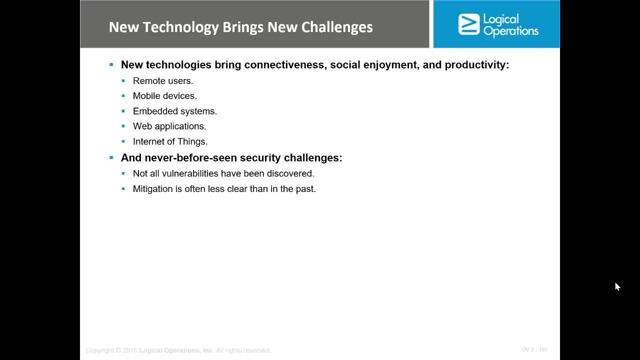 In general, new technology is very useful to the business, but also it raise new challenges. So right now we have things like IOT, artificial intelligence, embedded System, mobile devices. all those new technology have been helping in our business and it's make things more effective. 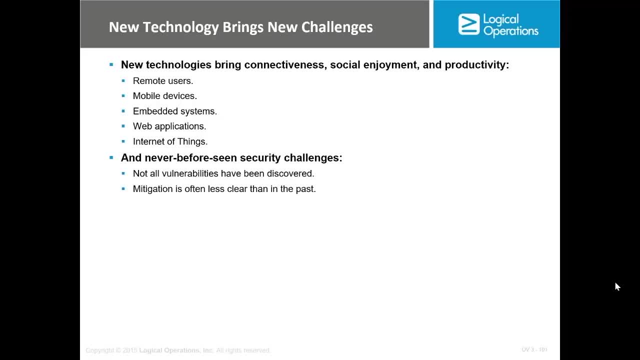 But on another hand, it raised new challenge and new security issue. So the point here: whenever you plan to implement a new technology in your business, you need also to understand what challenging is coming with. Let's take a couple of them. Let's start with remote. 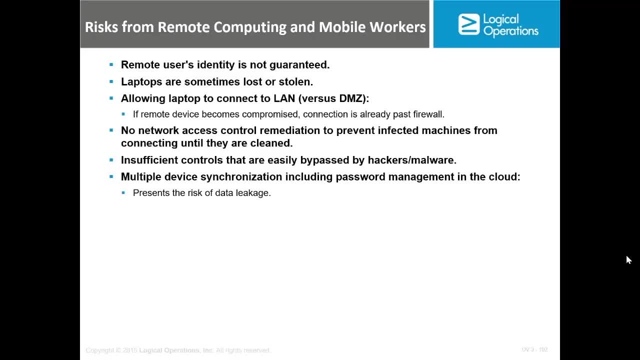 Remote computing And mobile worker. So in some cases and in some business, for the effectiveness of the business you need to allow people to work remotely. Maybe you have some of the project managers that keep moving around all the time and they are working from different side and you need to give them access to the company network to be able to access the resources and so on. 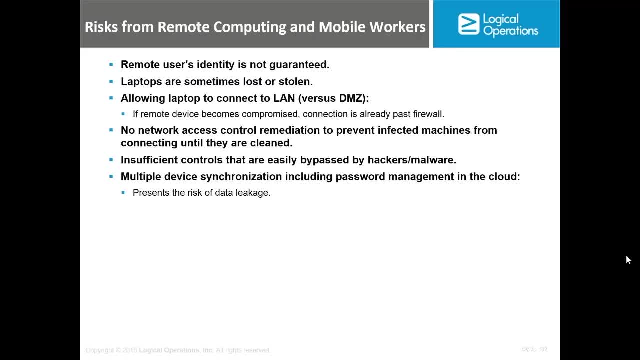 So from a business perspective this is actually quite good Because you are facilitating. Then they don't have to be on site on their desk to be able to access the resources, but they can do that from outside in case the business needs that. 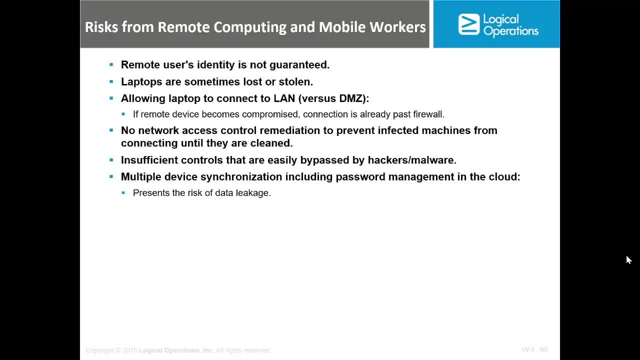 But on the other hand, maybe it can be manipulated in ways that: what if they lost the laptop and someone was able to get the laptop and access this remote connection? What if someone was able to get his credential and login remotely? So you need to have some justification for that. 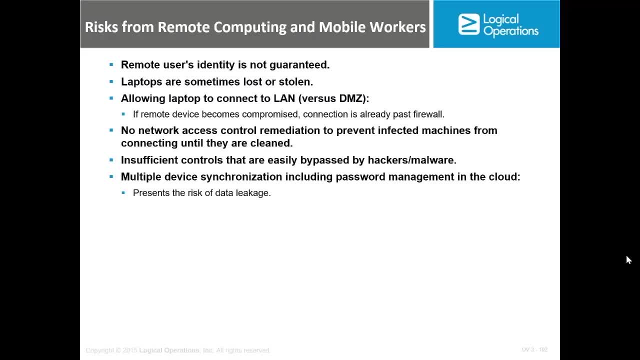 It's not that you need to allow everyone to be able to remote. First you need it need to be a part of his job description. So if one request some- you employee request a remote access, it need to be done through a specific process. 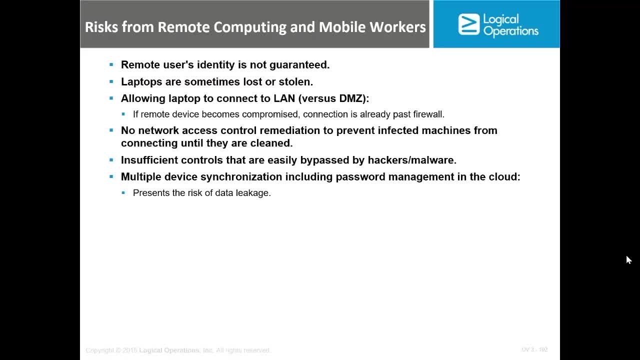 You need to take an approval from his management and you need to give him the control or the setting that will help to secure our network. For example, you should implement VPN, So if someone need to access the company from outside, I should not give him, like, any of those free tools that allow to connect to the network from remotely. 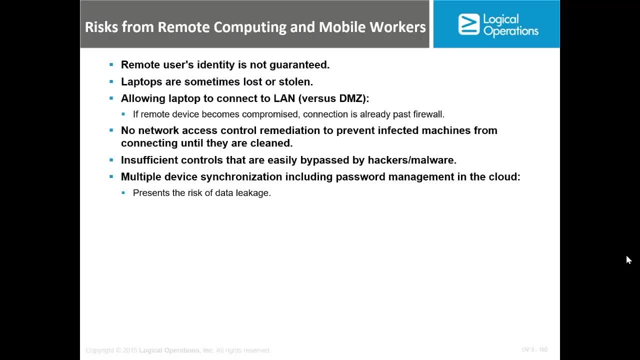 I should do that using a secure connection. Okay, so you are trying to like Harden the process. Do not keep it open for anyone. You should also have some Tools on the laptop in a way that, if you lost it, you can remotely delete whatever is on this laptop, and you should inform the employees that, in case he lost the laptop, his laptop. 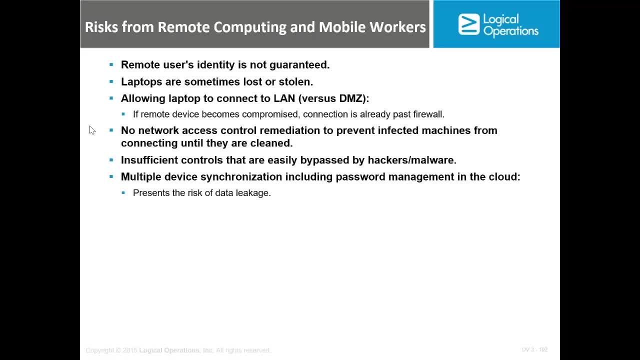 He need to inform the security team right away So you can take the action, You can block the account and so on and so forth. You should work or having a DMZ. DMZ is just like an area in your network where it's you. 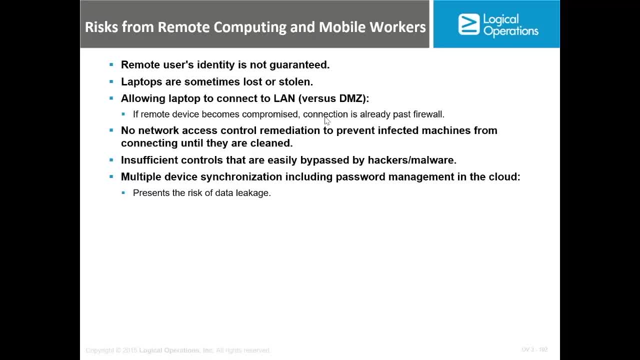 Are keeping all the machine that need to be accessed from the internet, instead of allowing people to connect to your local network right away. So you should have like a safe area or a safe domain. So this is called the DMZ. What else do we need to do? 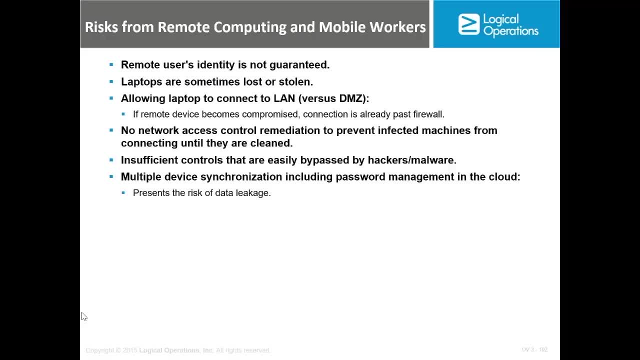 We don't have insufficient. I mean, whatever you are doing, you will not reach like a stage where you are hundred percent comfortable about that, But we are just following the best practice. and don't forget that you, as a security professional, It's all about following the standard and best practice, because if anything went wrong- because it may went wrong- 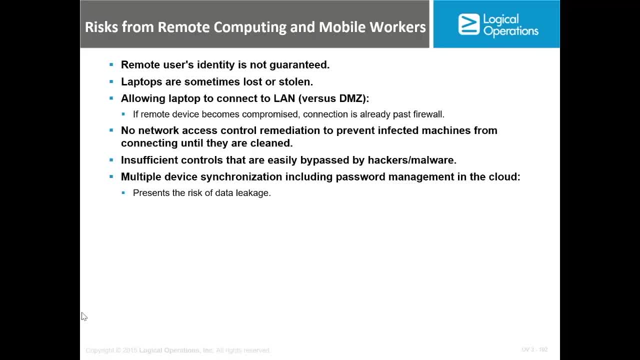 It may go wrong, by the way, because you know every day there is a new vulnerabilities, There is a new threat. So whatever you are doing, you know there is other challenge that will raise. but if a problem happened you can clear from. you can clear your site by saying: 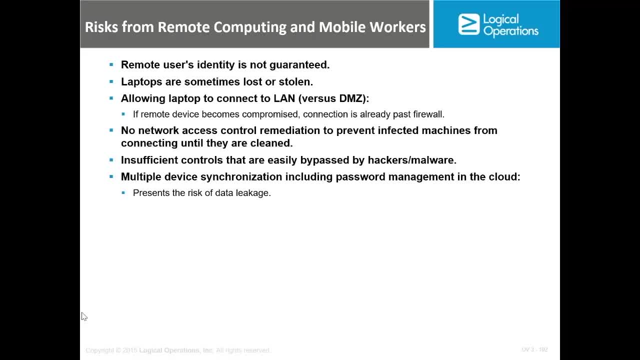 I was following the best practice, I was following the standard. This is quite important to do delegate and do care, which we spoke about in the first domain. In general- and I'm going to add this document with this lecture- You need to have a remote access policy in a way that if anyone need to have a remote access, he need to read about this policy. 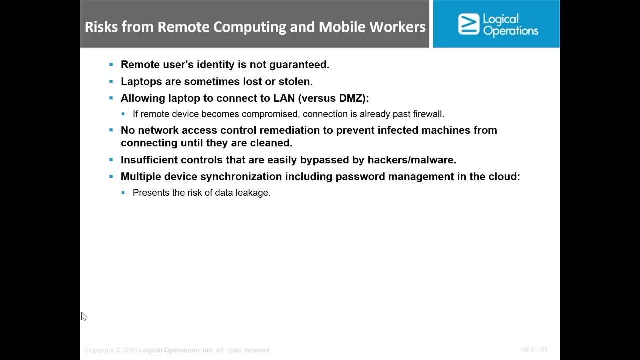 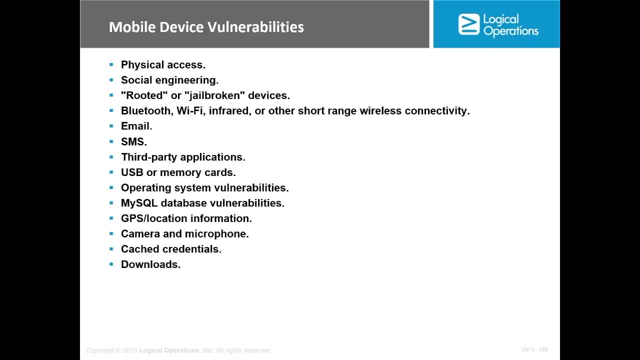 What is his obligation, What he should follow, what he should be preventing, and so on and so forth. The mobile device vulnerability or mobile security is common sense. What could go wrong with your mobile If you start using your mobile in the business, receiving email or using any messaging service for communicating with your client or communicating with your team? 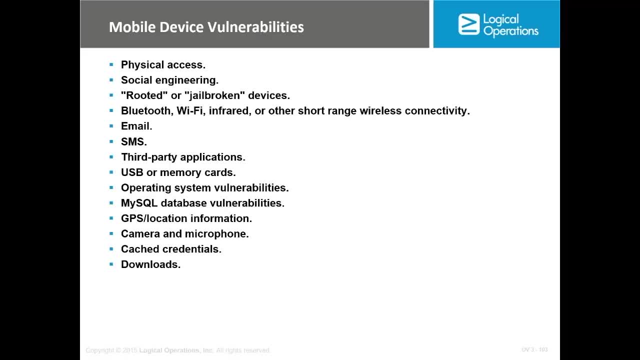 Okay, what could go wrong? first, You could lose a mobile. This is quite easy because it's a small device and you be maybe lose it somewhere. You may be a victim of a social Engineering, and in the next lecture I'm going to show you a small demonstration. 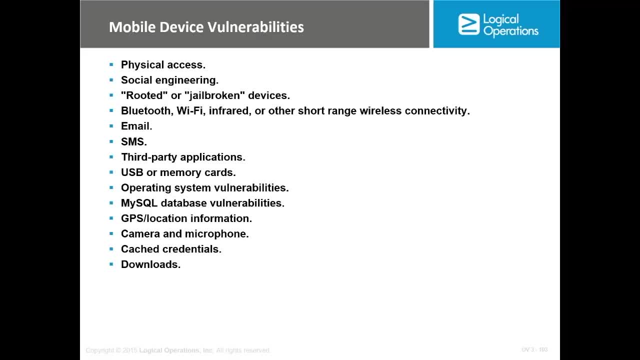 You are downloading a program, someone send you an SMS. You click on the link, That's it: SMS emails. So I'm going to show you different kind of, or I'm going to show you actually one demonstration that demonstrate how easy is it to compromise a mobile and get all the information just by sending you an email, fake email or SMS with the link inside. 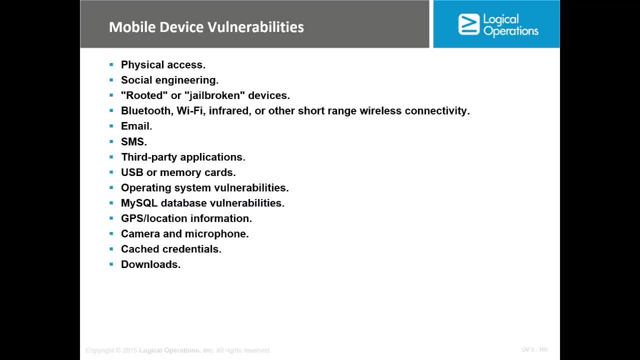 So those are some of the vulnerability inside the mobile and it's common sense. Malicious code, social engineering, lost of the physical asset, get rooted or jailbreaking. This is actually quite risky when you get your mobile and do a route for your mobile if it was an Android or jailbreaking. 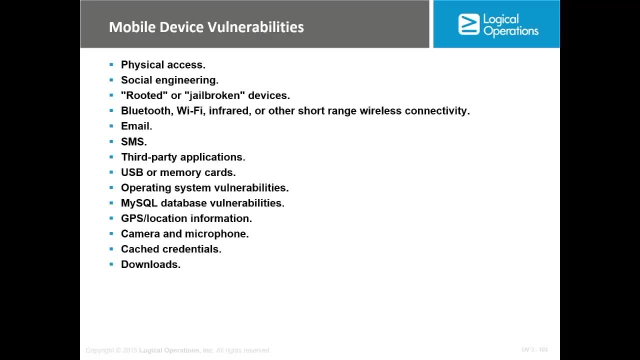 If it's an apple, quite serious, because you are breaking the security into the mobile and you are make it very vulnerable. So let me show you one or two demo about the mobile vulnerability, how it can be done, just as a proof of concept, and let's move to the next topic. 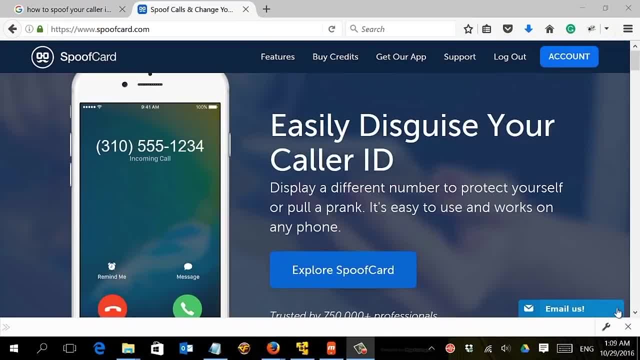 This lecture. it's under the subject of social engineering. It's not really an attack, but it will show you that you should not trust any phone call or any SMS Because, as we saw earlier, that email can be spoofed or can be faked on. also, phone call can be spoofed and text messages can be spoofed. 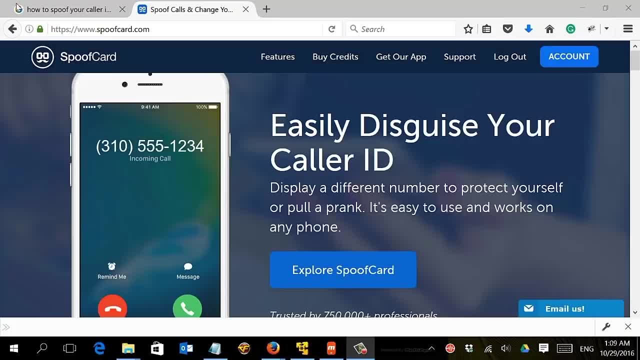 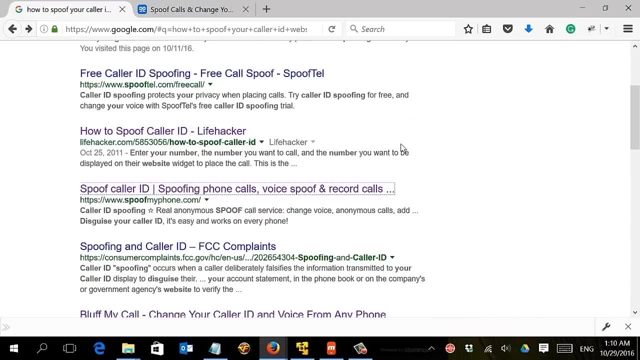 And this will be a small demonstration. If you search online, you will find a lot of websites- Some of them are free, Some of them are paid- that allow you to spoof your phone, call your phone number and to call someone- and it seem coming from one of his friend, coming from his bank, coming from. so you should not. 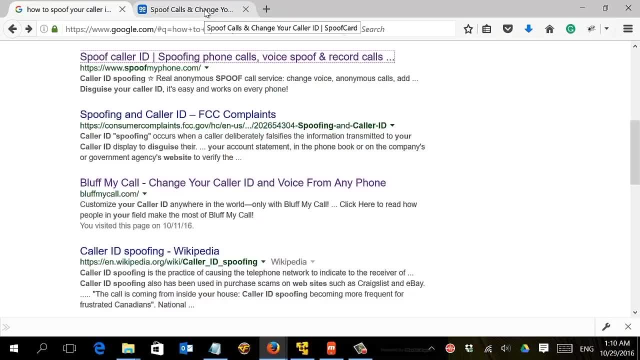 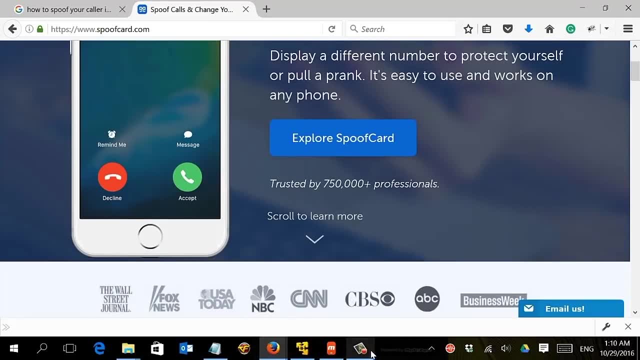 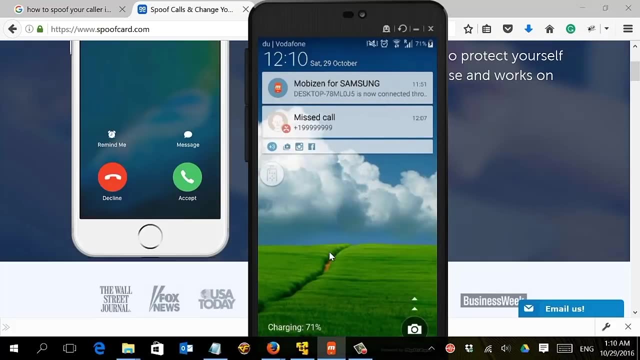 Trust the mobile number. if you're getting a phone from your bank, it could be spoofed call and let's see a small example about that. So this is my phone and what I'm going to do right now. I'm going to try to make a call, spoof call, and I'm going to choose any random number. 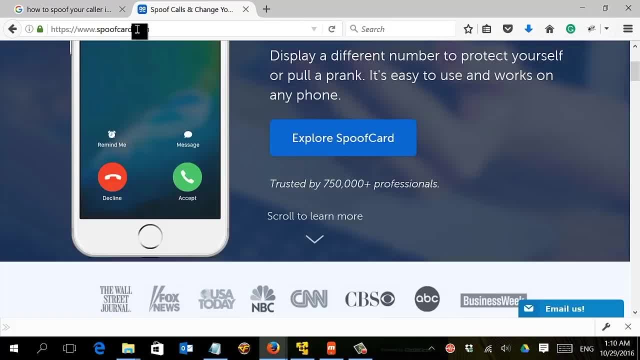 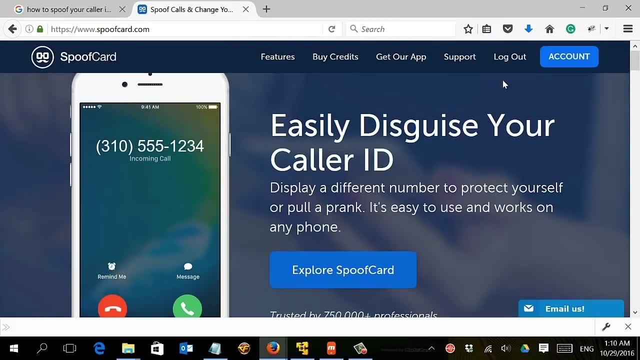 So let's see, I'm going to use this website spoof card. This is paid but, as I was saying, it's not about which site you are using. if you search, You'll find the site. There is some free side and some pay side. 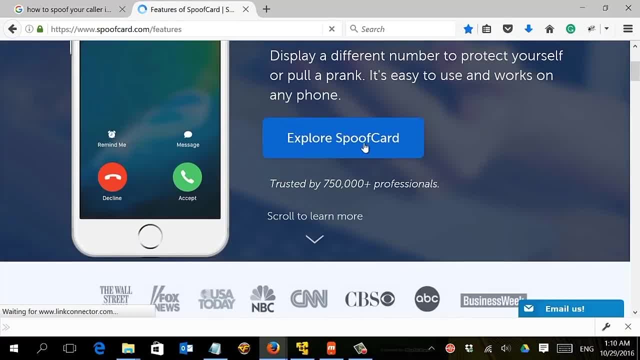 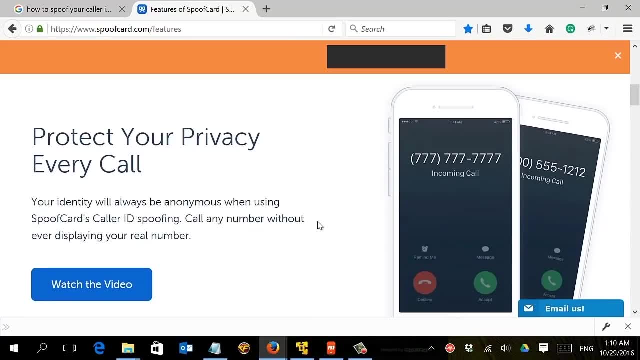 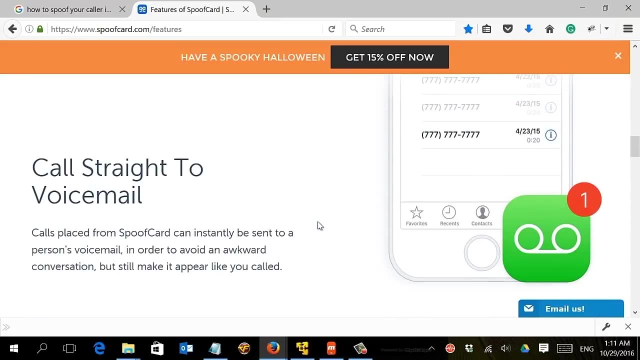 Let me go to this one and let me place a call Now. the good thing about this website that it's spoofing the number and it's spoofing the the text messages as well, So you can send someone an SMS that show is coming from like his work. 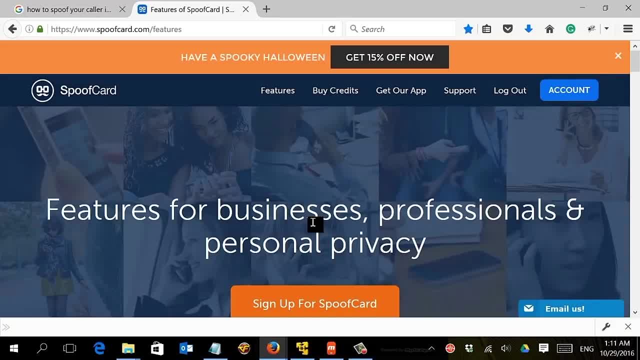 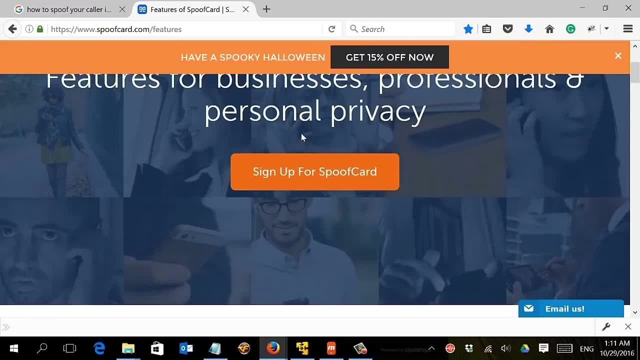 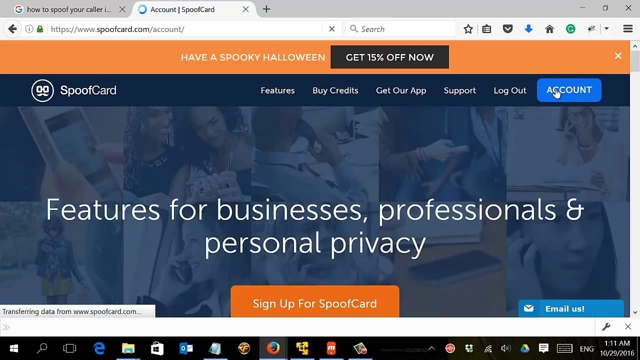 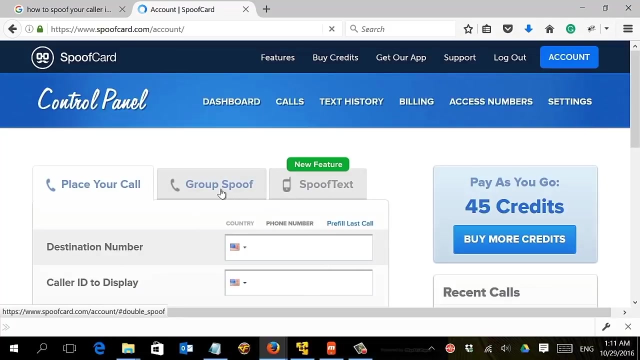 His Manager and by doing that, whatever link is inside, he will be comfortable clicking on it. So let's see, I just need to spoof a call. already sign up. Let me go to account Now. as you can see, I can spoof a call or I can spoof a text messages. I can record the. 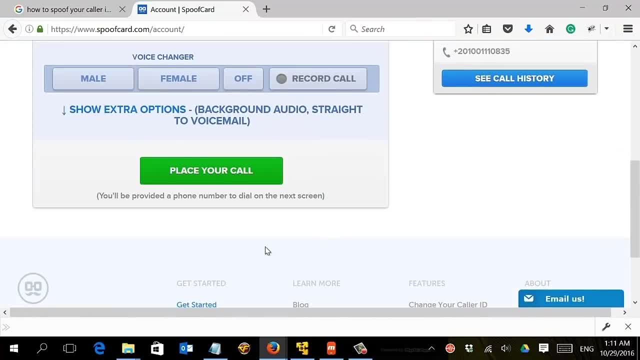 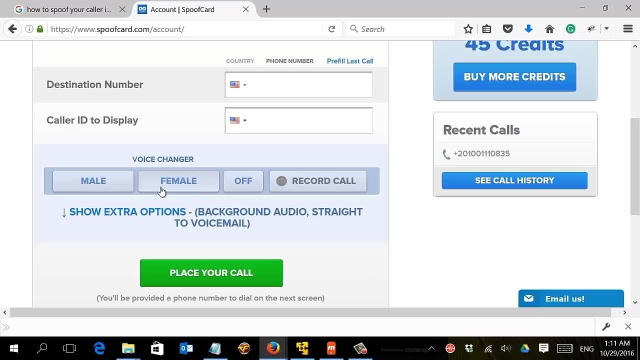 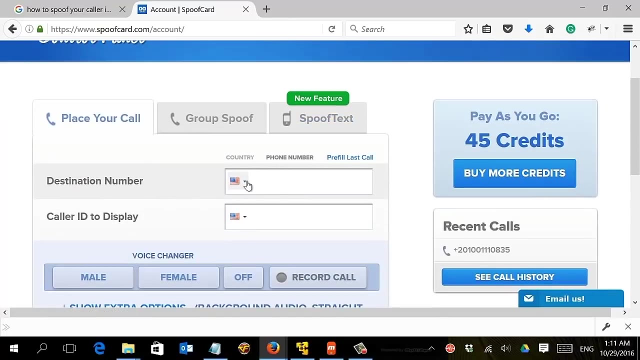 Call. I can change my voice, so it became male or female, or so you have different option here. You can choose different, like a voice, You can record the call and so on. So let's try. I'm going to put a destination number. 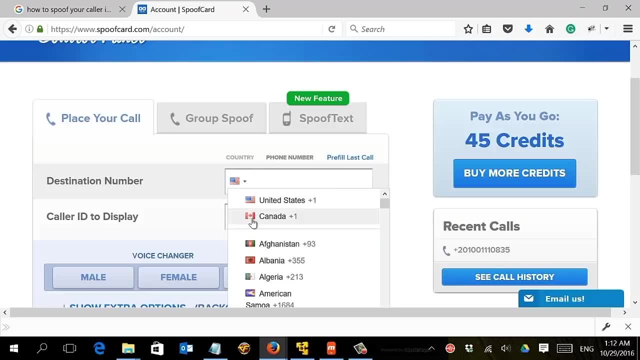 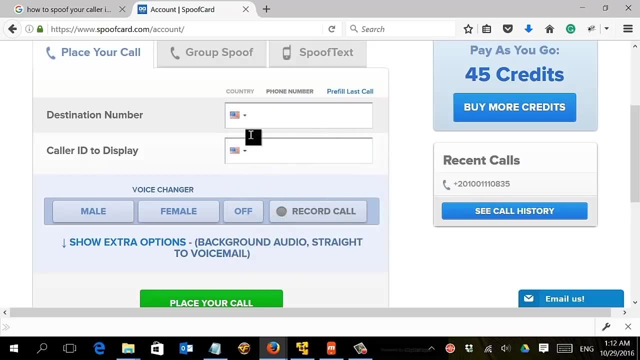 So let me put Number for testing: Destination number. I'm going to choose The mobile that I'm testing, Okay, And We will type the number And then the caller ID to be display. What number would you like to display? 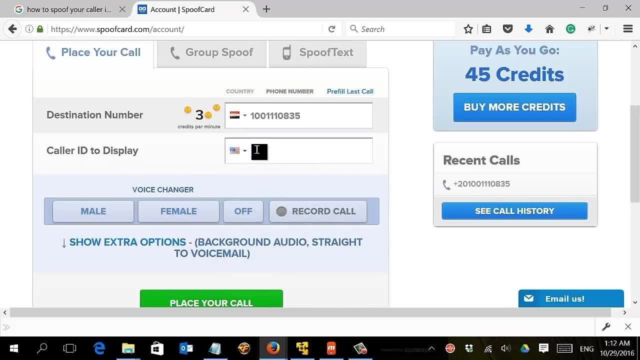 So I'm going to put it's coming from United States, For instance, and I'm going to put for instant all: six, one, two, three, four, five, six, seven, eight, nine, ten can put. any amount of number is not a problem, and you can make your voice, male or female, doesn't matter. record the voice. 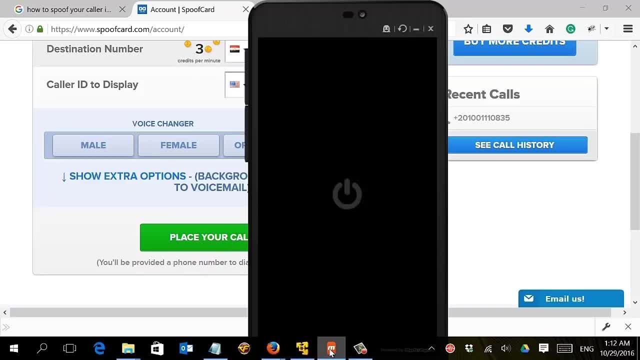 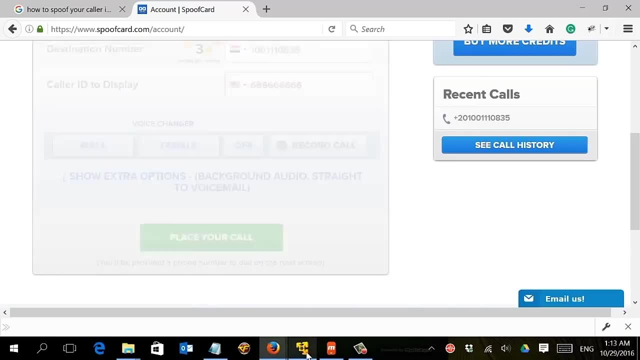 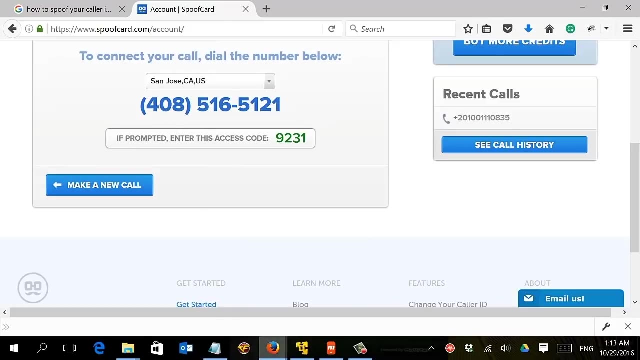 But let's test that first. So this is mine mobile, Okay, and let's place a call. Here you go And he can ask you to call a number In the United States, And once you call this number, let me it will activate the service. 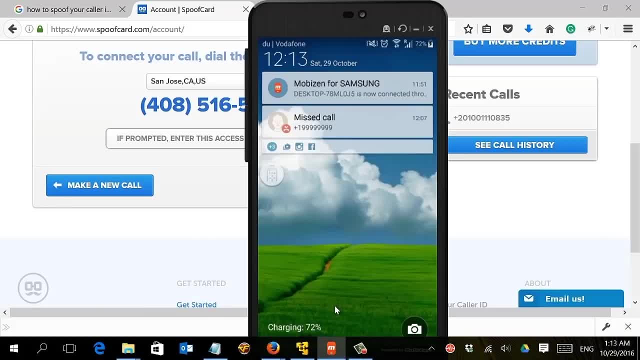 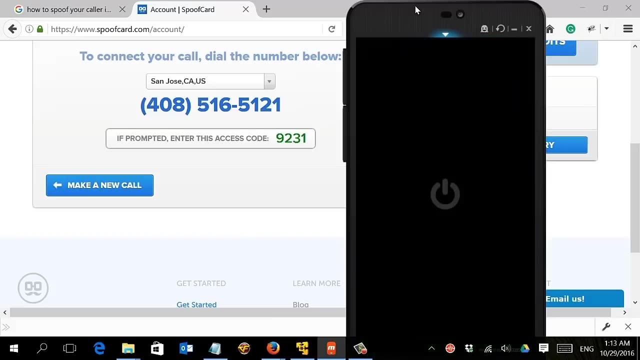 So let's see, Let's see, Let's worry, This is a mobile and let me call the number that he's saying and let's see what will happen. So just one second, Here you go. So I'm going to call the number four zero eight, from a different phone and four. 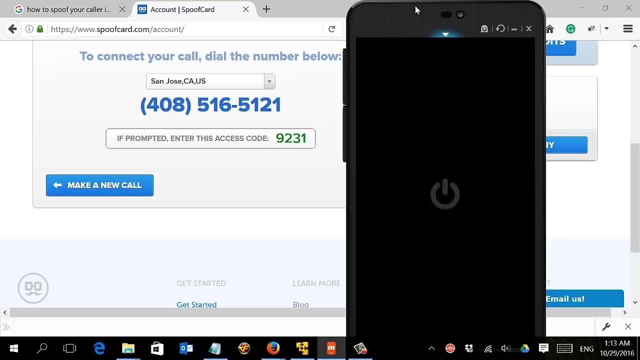 Zero, eight, five, one, six, five, one, two, one, And let's call I'm opening the speaker, because sometimes he's asking about a code. Sometimes it will run automatically or sometimes it some. opening the speaker. Oh, I'm sorry, I forget to put the US code. 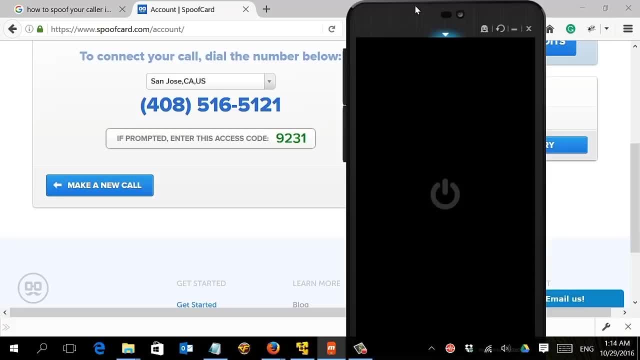 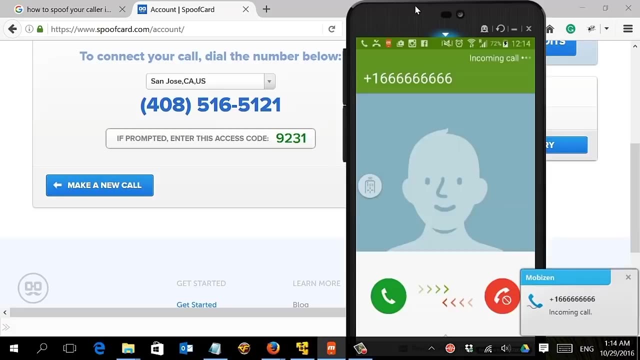 Because I'm not calling from us. So let's see. See, so I was able to spoof a phone call, so I can mix it. any phone call I want I can call someone seeming this coming from his office, or calling Someone's looking that it's coming from his manager or his bank. 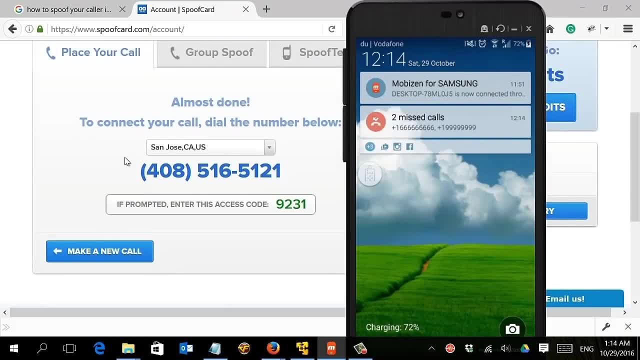 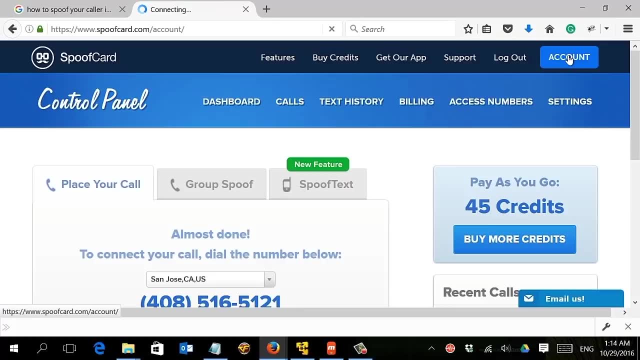 So this is very, very important and very, very critical. So do not test this kind of attack blindly. So you are getting a call from your bank, So definitely is the bank? No, not necessarily. So let's try this new feature if it's going to work or not, but let's try that on a different. 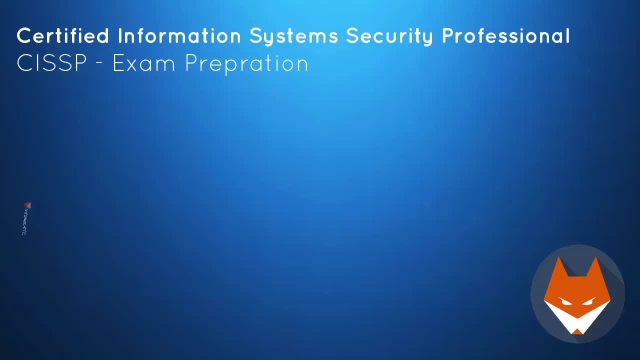 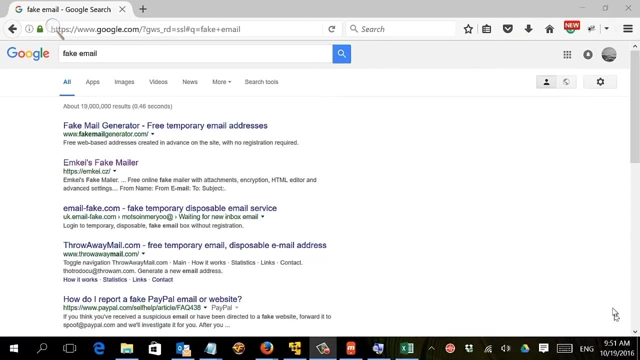 Let's see, Let's try this new feature. It's not really an attack section, but it will show you that you should not trust anything. Email can be spoofed, SMS can be spoofed, mobile or cellular number can be spoofed. So my point is: 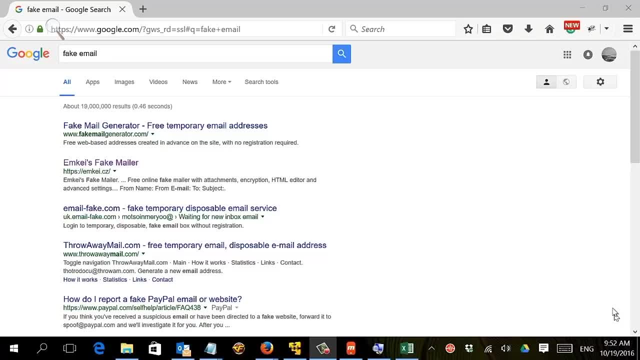 People trust email blindly. They receive an email coming from Their manager. They will execute whatever is inside. They will never think that mail can be spoofed or fake. same concept apply for SMS. You receive an SMS SMS from your bank. You think SMS cannot be fake. 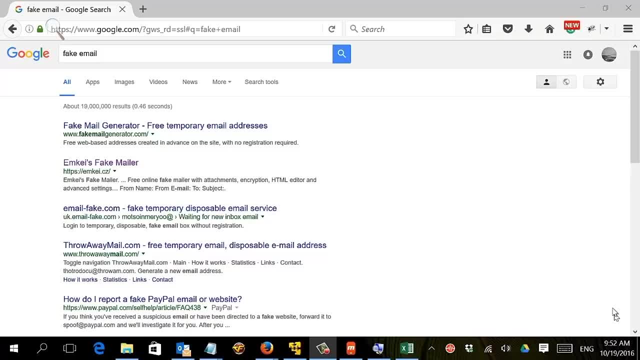 It can be faked mobile number. It can be fixed. So it's not really an attack session, a section. It's more into the tools that is used into the attack. So if a malicious hacker utilize such tools, it will be very 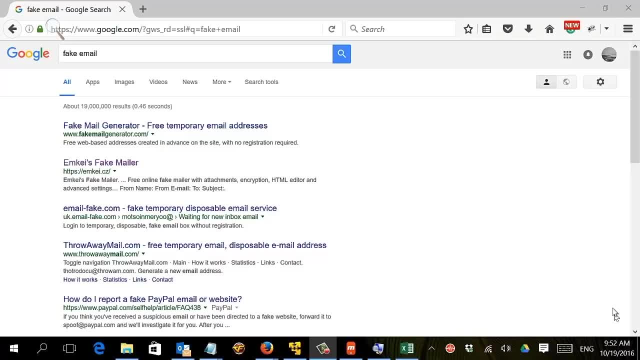 Easy for him to convince anyone to do anything that he want him to do. So if I send an email coming from your friend or from your manager, If you don't have enough background or you are not aware enough, you may be spoofed by this email and you will trust that the mail is coming from this sender. 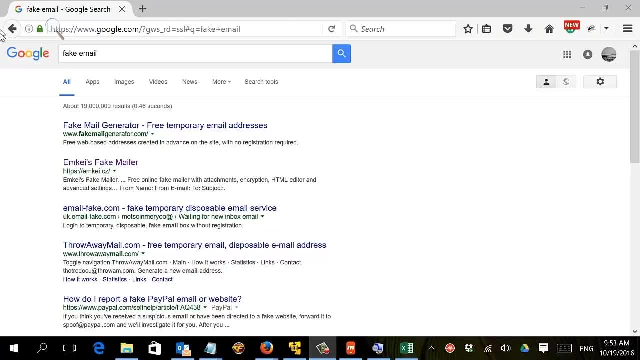 So the first demo I want to show you, It's the spoofed website or the fake, I'm sorry, the spoofed email or the fake email. If you search on Google for fake email, you will see this specific website. This is a quite interesting website. 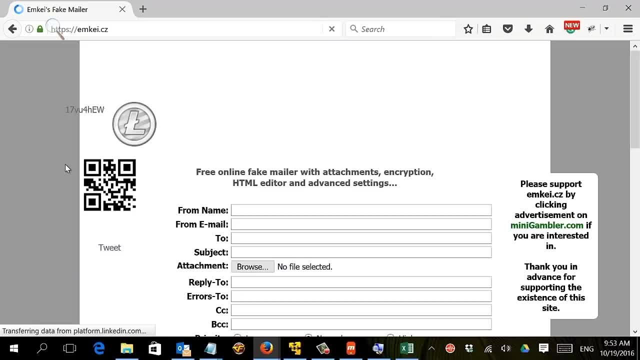 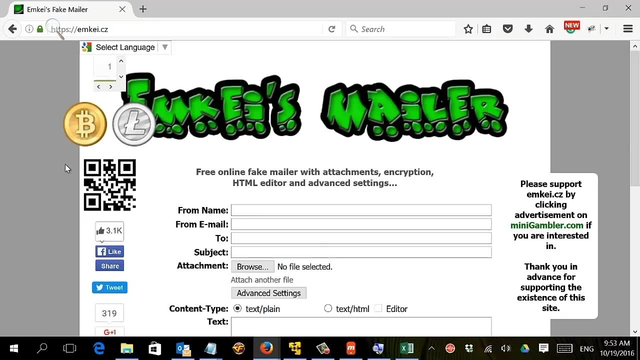 It's free, It's very effective. Most probably it will go to your inbox. If you don't have a proper mail setting, it may go to the junk, but it may go to the inbox. You can test it. You can fake an email showing. 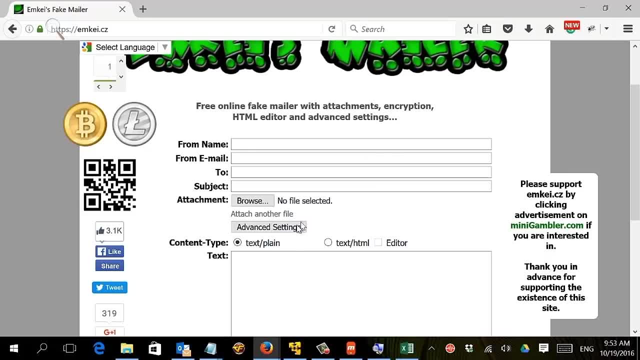 It's coming from Anyone to anyone and you can attach whatever you want. You can send it in a text or as an HTML, So it will shows like you know those message coming from LinkedIn or from Twitter's or this kind of thing. 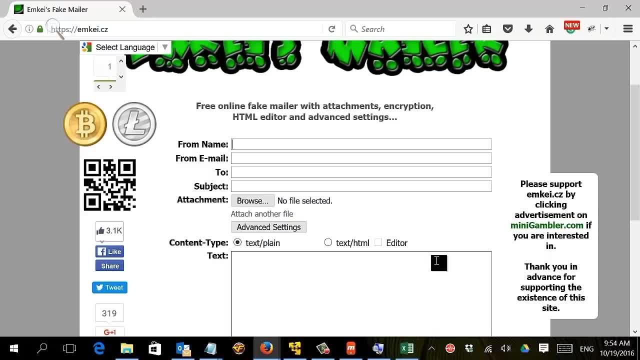 So, using such tool, It's very, very convenient, and I don't know why they are keeping such website up and running, because actually this is very dangerous. So let's try a demo here. I'm going to send the mail that show it's coming from. 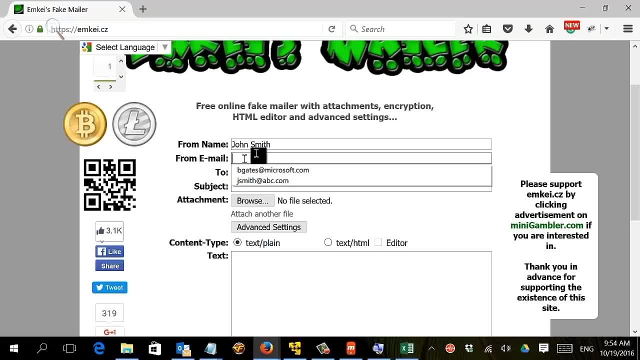 John Smith and I'm going to put an email, or let's make it. Oh yeah, let's make it, John Smith, and the mail will be coming from John Smith, abccom. You can put anything you want. I can type G Smith. 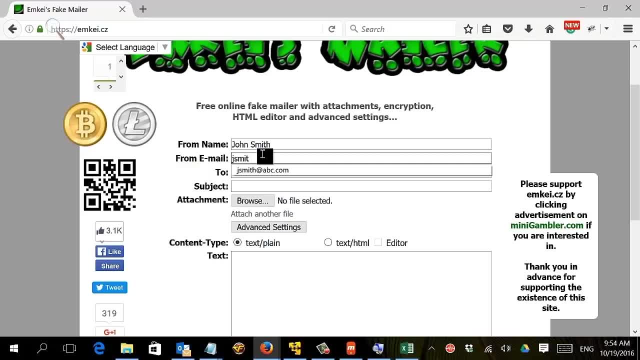 She Smith At for instant ms And dot-com And we're going to send this email to myself. I'm going to send it to different email, So let's try with the mail that I'm using on my testing mobile and the thought of at sorry. 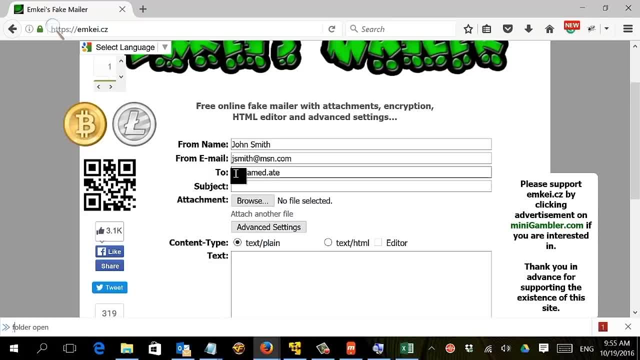 And the thought of At gmx, Dot-com. And let's type any subject: test email. Let me put any test email, Okay. So the point is that Can I fake an email or not? Let's see, And I'm not a robot. 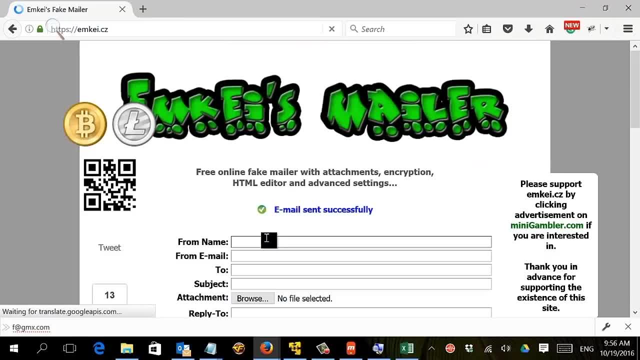 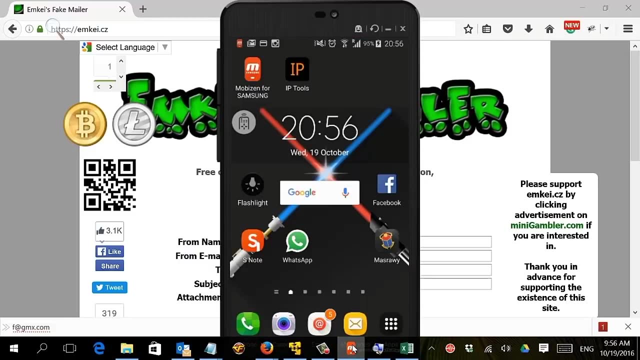 And let's send it. Now he's saying that the email has been successfully sent. Let's see if this is the case. So I'm going to get to my mobile now. This can be used on mobile or computer or whatever, And let's see. 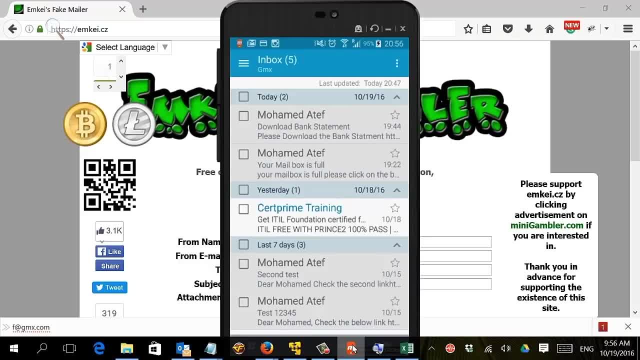 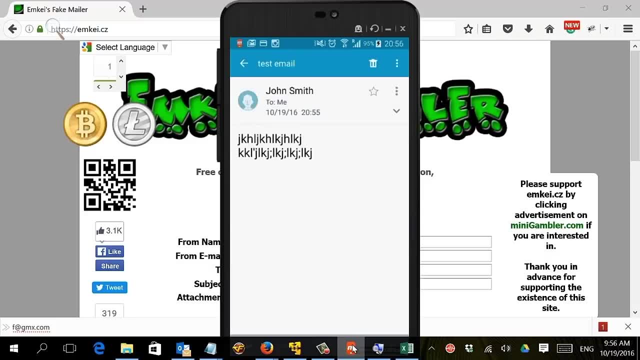 Are we going to get anything or not? Let me refresh. Here you go. It's coming from John Smith, which it's not an existing person, And, as you can see, it's showing that it came from John Smith. And this is his email to my email. 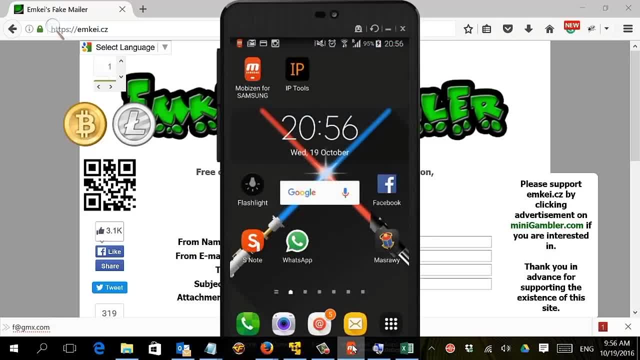 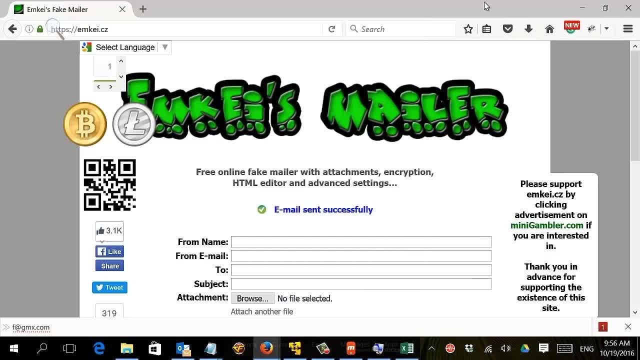 So imagine what can be done using this tool that you can like: Convince someone that an email He received coming from his manager or his wife or his girlfriend or whatever, was the case, And you try to convince him what was, whatever it may show. 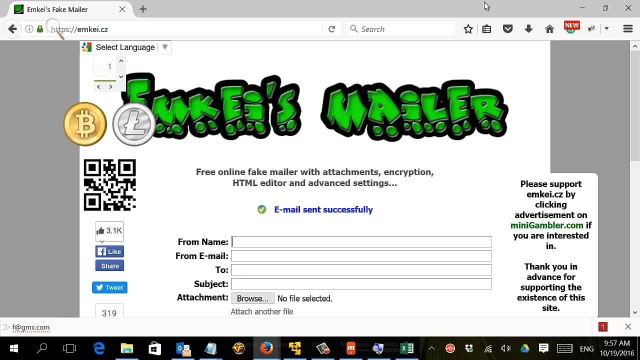 It's coming from Microsoft or is coming from their bank. But I have to tell you this is completely illegal And in some country it's a federal crime. So it's not something to play with. If you are doing a proper penetration testing in any organization and you see you need to check if people you know they have 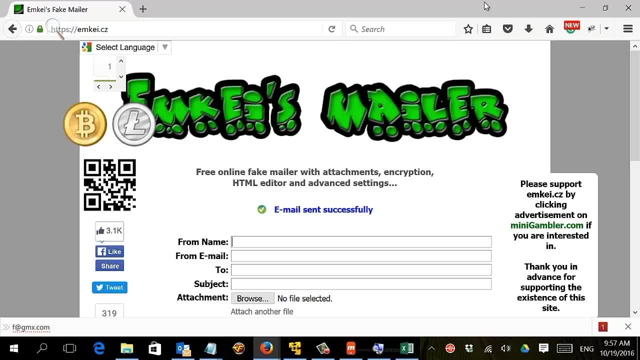 Enough awareness that if he's they receive a suspicion email, they will verify. You can use this tools now. only one weakness We have in such tools: It's one-way process. I mean you can send an email showing that it's it's coming from someone. 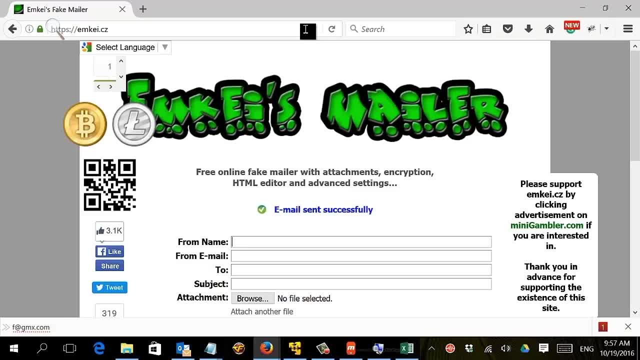 But what if the victim replied back? the reply will be going to the right person. That's why, when people use such tools, they will never ask you, They will never ask you to reply Back. They will usually ask you to do something inside the email. 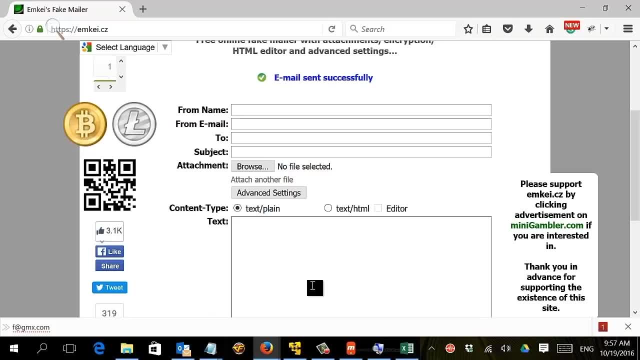 Please click on the link, Please download the attachment, but they will never ask you to reply back sending them your credential or any kind of information. So if you receive an email and you are sus, you are suspecting that this is a fake email. 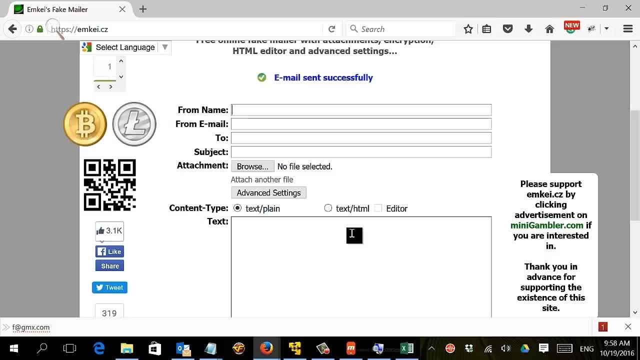 You can try to reply back, asking that you send me this email. This would be going to the website. and same concept apply for any spoof technique. If you received a fake mobile, A fake phone call from a fake number, You can try to disconnect and call them back. 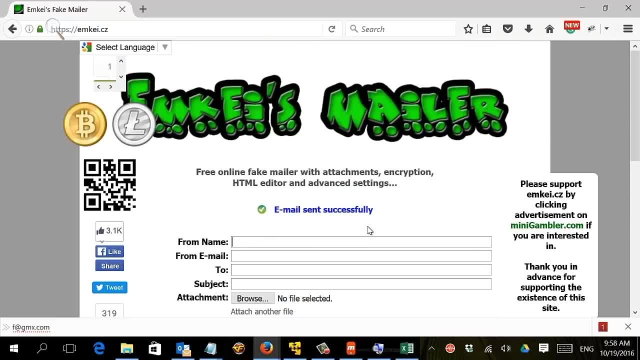 And so on. So this is one of the tool that if you use such tool with a technique that we explained in the previous lecture, it will give you an extremely good results. But one more time, this should be done in a proper frame If you are doing a penetration testing, with the right approver. 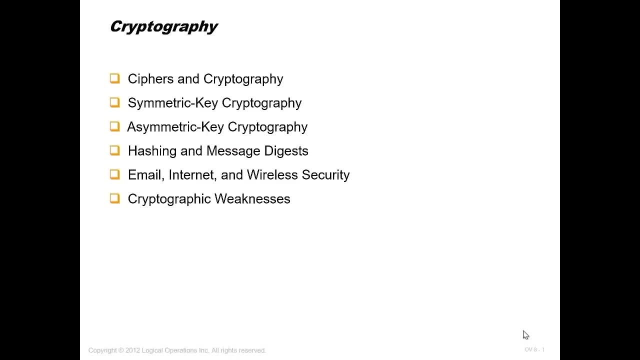 Cryptography. in this domain, We will be talking about cryptography. A lot of people have problem with cryptography and actually they should not have any problem because it's not that deep. You just need to know the basics about cryptography to be able to understand the concept and also solve the question related to cryptography inside the exam. 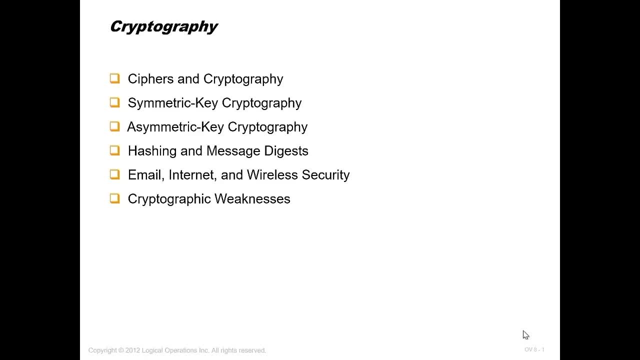 So I saw some people. they went and they bought some books that explain different mythology of cryptography. It's not that deep, It's really, really simple, and we'll try to simplify that as much as we can and because it's kind of academic Or it's kind of theoretical module. 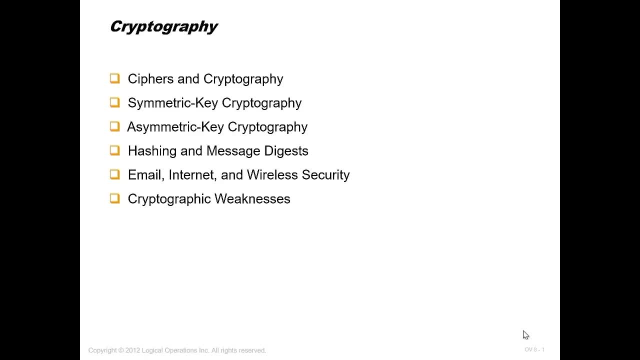 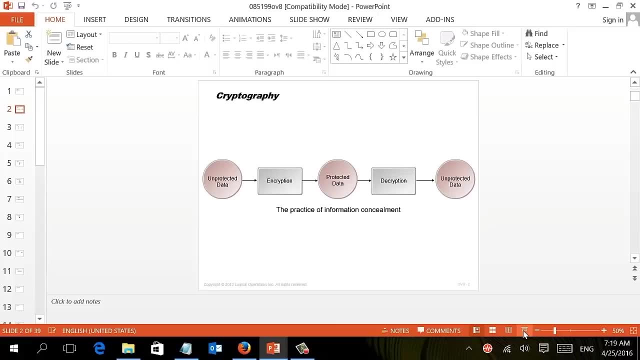 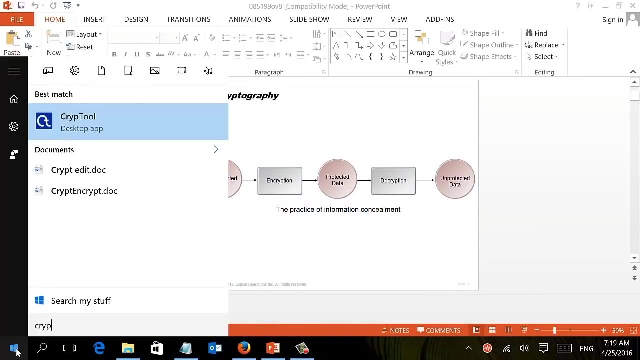 I'll be doing some demonstration while we are going inside the course. Now, what I want you to do to be able to practice cryptography, I want you to install one specific program called crypt tool. I already installed it. It's a free tool, but it's very, very handy when it comes to practicing cryptography. 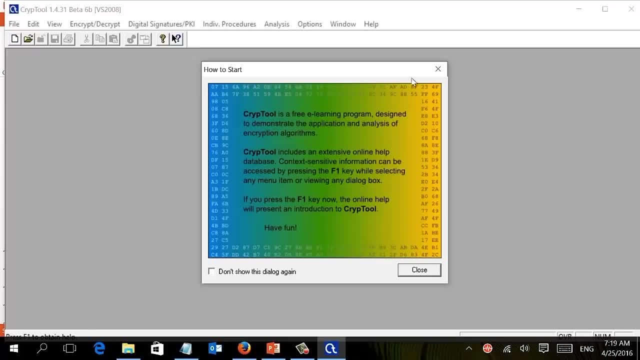 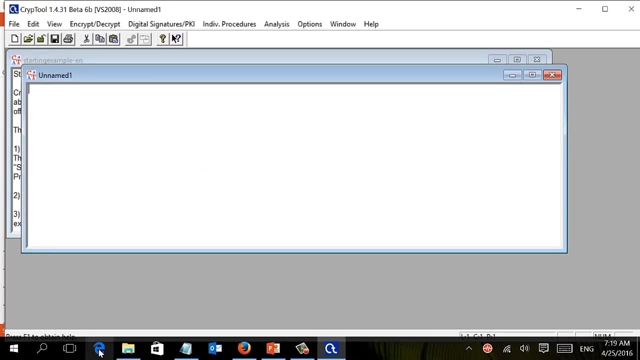 So it looks like a not bad. I mean, when you open it it will Start And the program with a file inside. so we close it and you can open a new one. so you can practice that. now I also want to show you from where you can download this. 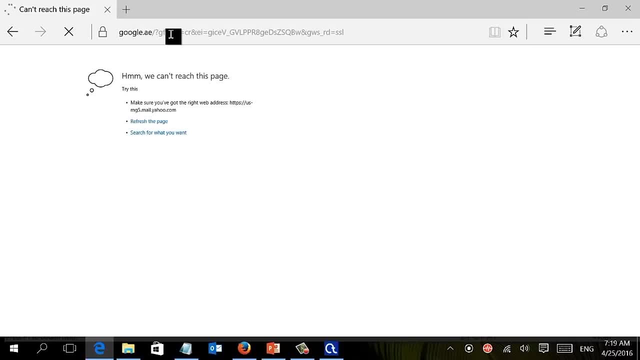 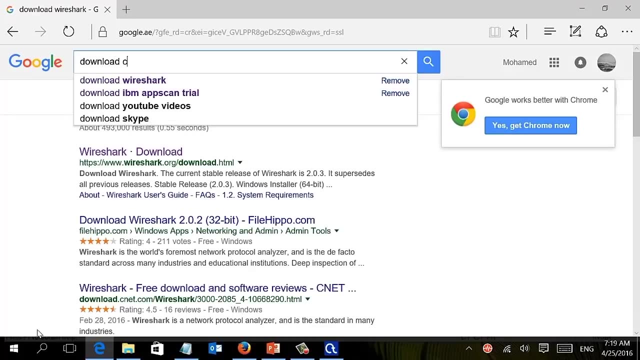 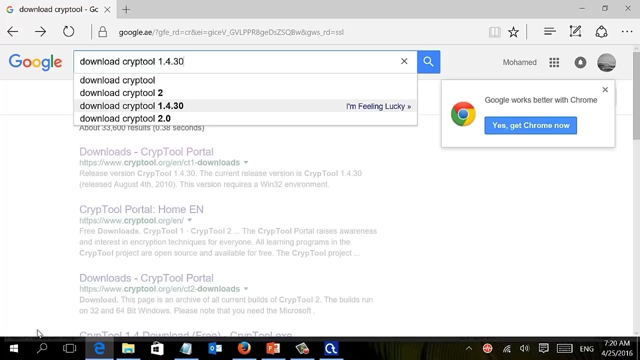 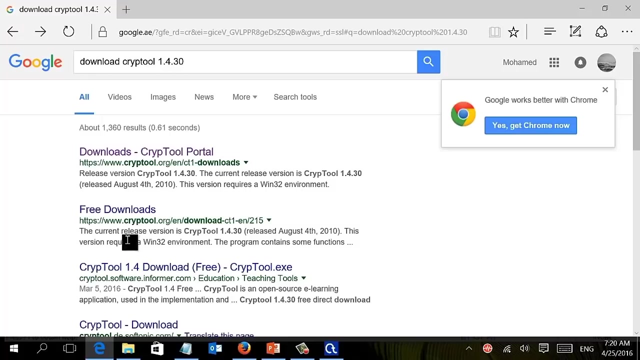 Application. So if you go to Google and you search for it, Down Load And you know it's better to get, for me I prefer 1.4 because it's quite easy. to use it too. It's also easy, but they added a lot of features there and I'm not very familiar with it. 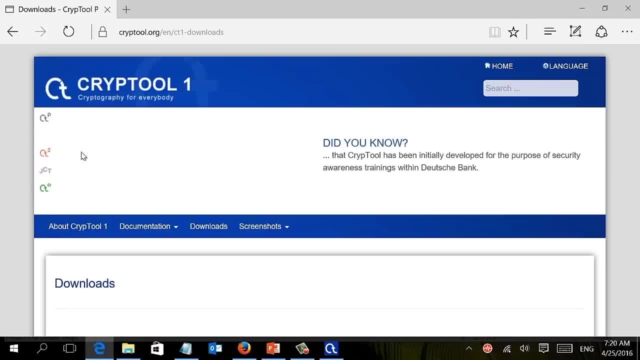 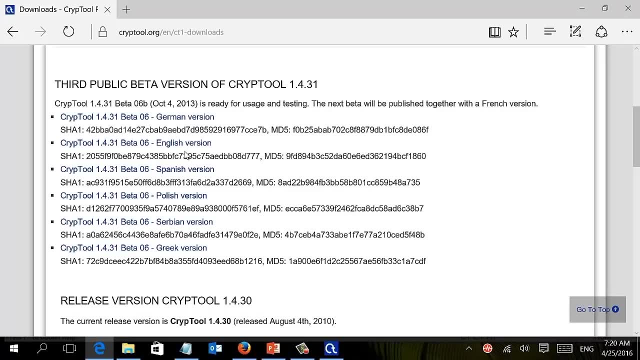 So, but you can download any of those. you know is there the same. so you can go and you can download. now You have to download the versions that match. I mean English or German. You have to be careful with it and I will. also, I want you to notice in: 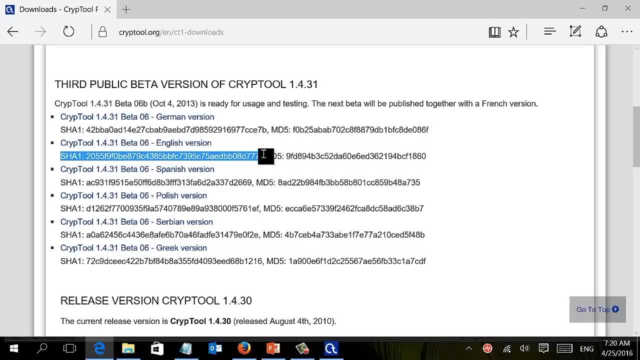 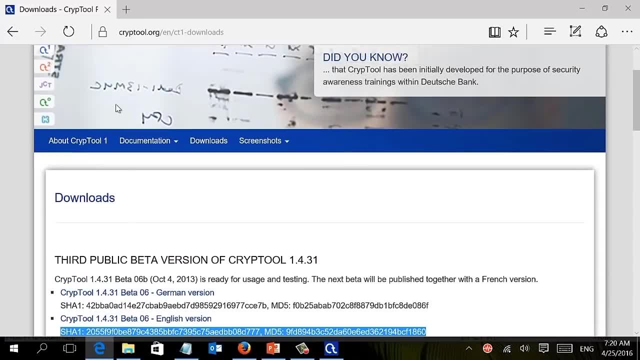 Below the download link, You can find something called the hash will be explaining that in cryptography, But anyway, my objective is that you have to download this program. It will help you while studying for cryptography. Now getting back to our subject: What is cryptography? 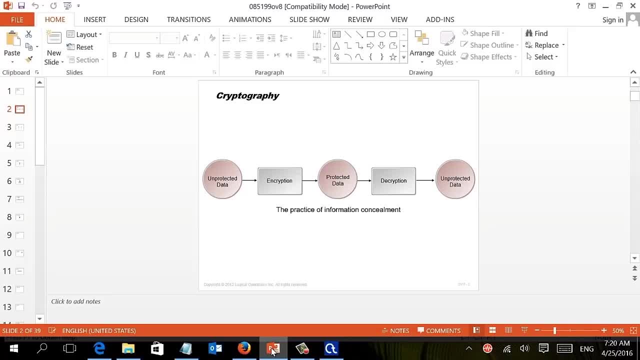 Cryptography. It's to encrypt a text So it become unreadable. Okay, sounds good. So I have a text, I'm going to encrypt it and it will become unreadable And people who need to read this text or he going to need to decrypt it to a readable format. 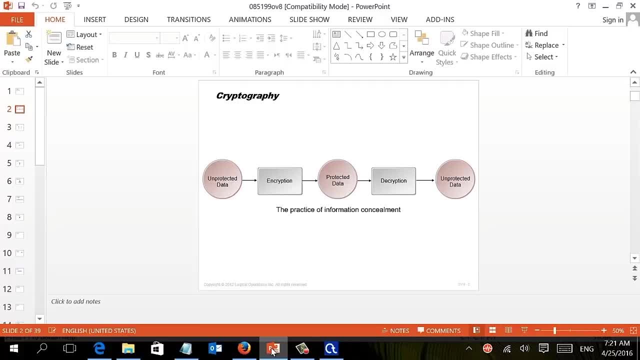 Now, this is this. come under which area in security? Is it a confidentiality feature or is it an integrity or is it an availability? I mean, when we are implementing cryptography in our organization, what exactly are we providing? Are we providing confidentiality or integrity or availability? cryptography will provide confidentiality. 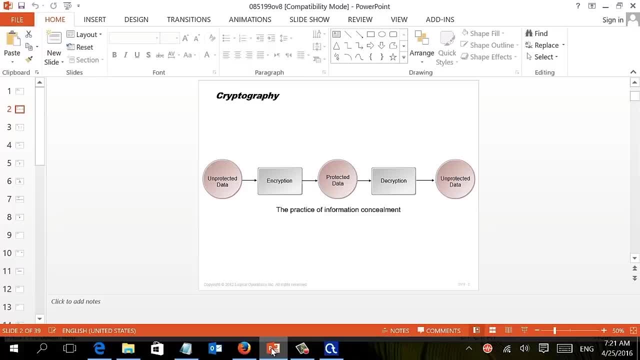 An integrity that has nothing to do with availability, confidentiality. It makes sense because I have some important information. I'm going to encrypt them and I'm going to send them someone to someone, and I will send him the key as well, So he will be able to decrypt it back and be able to read it. 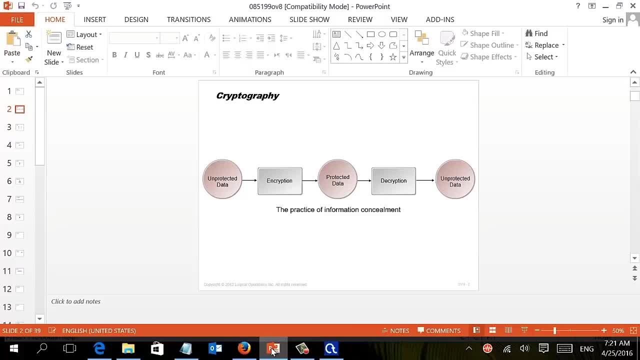 So by doing that, I'm providing confidentiality to my information. I'm sure who actually can access those information, because I'm sharing the key with authorized people. But what about integrity? How cryptography can implement integrity? You're going to see that during this domain, how cryptography can be used to confirm the integrity. 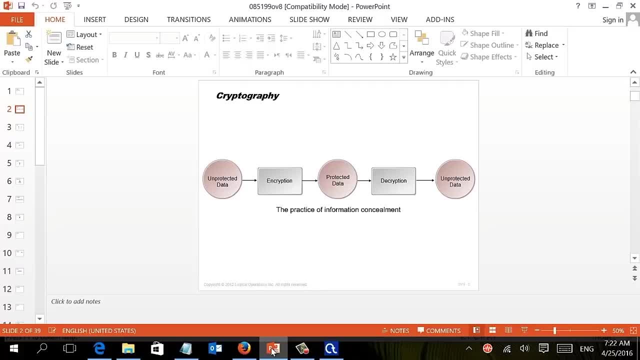 But cryptography has nothing to do with confidentiality. Now let's talk about the process and let's talk about two different definition. So we have a text, we will be run some algorithm on it and it become unreadable text. We have two concept here that we need to be aware of. 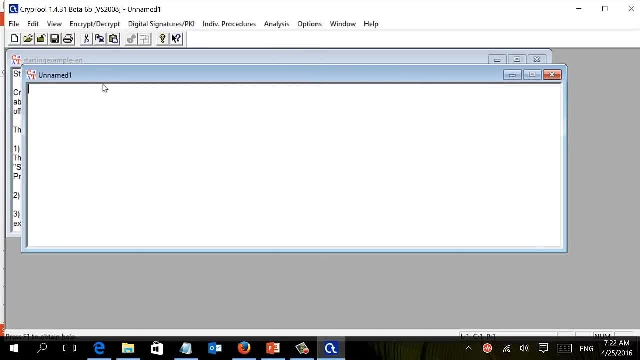 What is a key and what is an algorithm? Let's go to crypt tool and let me give you a small example. Let me close this file and I'm going to go work on this one. So if I write down, for instance, a sentence here: 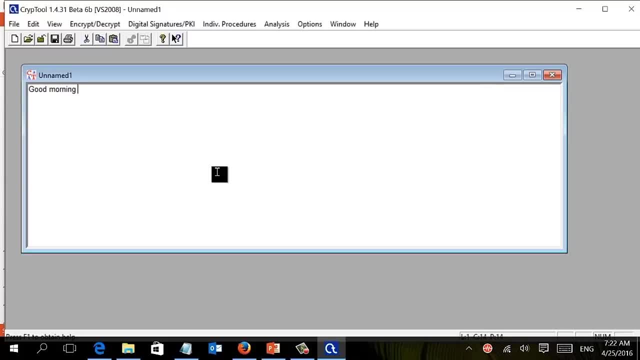 Good Morning. Plus, This is readable right. Then I can select this text. I'm going to go to encrypt or decrypt and I will find all kind of encryption protocol. I'm going to go to one very classic one, I'm going to go to symmetric classic and we're going to go to Caesar encryption. 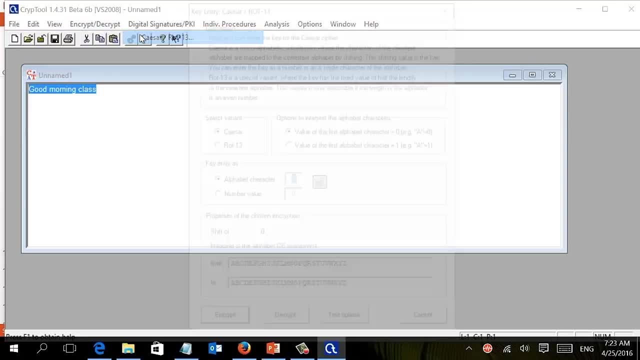 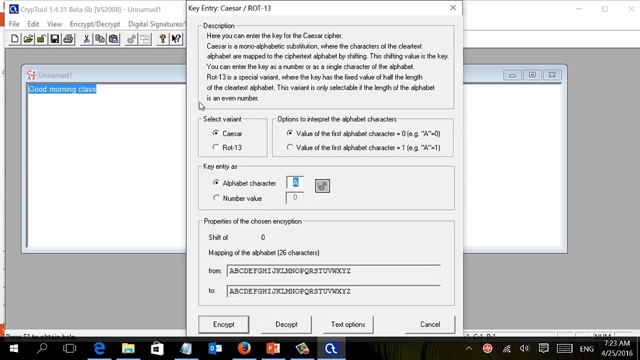 This is a very, very classic encryption, Caesar. and what is Caesar? encryption is doing it just moving the alphabet. I mean alphabet are starting from ABCDEF, So I'm going to ask him to start from E, So first letter, which is a, would be the would be. 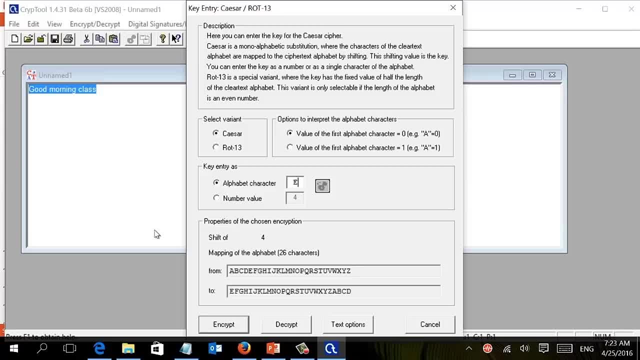 Transfer to E and B will be F and C will be G and so on. So I'm just moving the alphabetic. I can do that by name, by letters. I can tell him change from A to E, or I can tell him move the letter for letter. 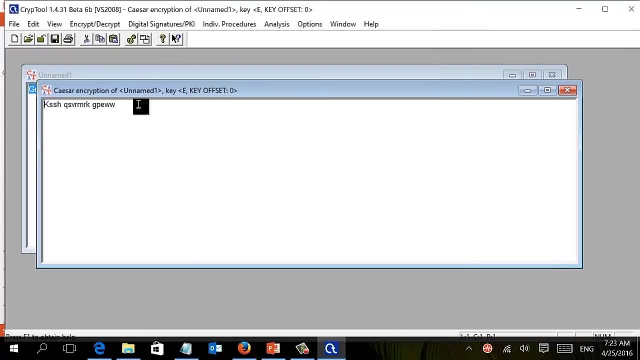 It will give the same result, and then I'm going to tell him encrypt, Then I'll be having another text That is also English letters, except it's unreadable. We call that. we call that the cipher, so cipher, It's unreadable. unreadable doesn't mean that it's a sign or a like, a symbol. 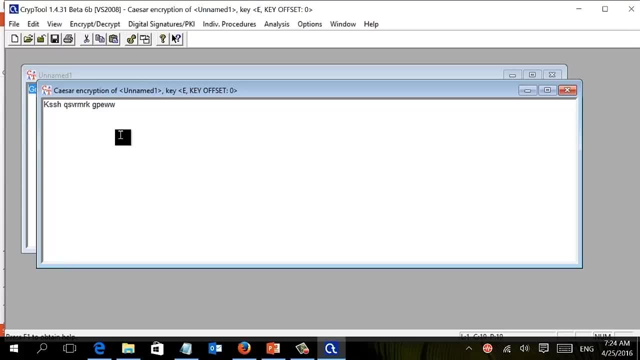 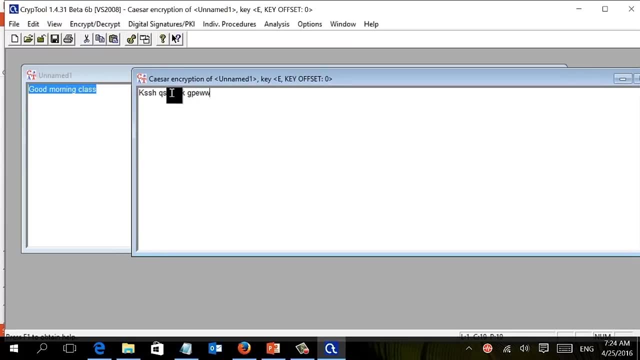 No, it could be an English letter, but it doesn't have any meaning. any meaning. So what happened is I did transfer Readable to unreadable text. Okay, Now here is a question: What is the algorithm here And what is the key? algorithm means the methods. the method here was shifting the letters. 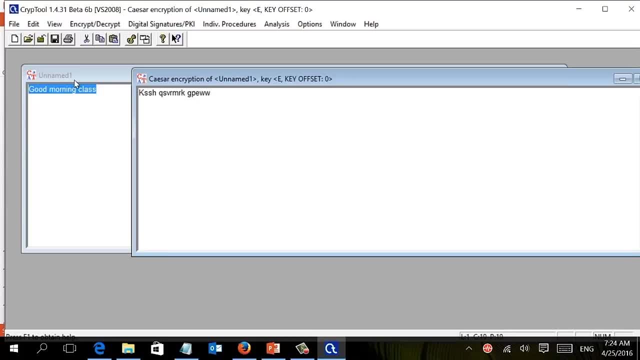 Another algorithm could be changing the letter to number- This is also an algorithm- or changing the letter to symbol. So the algorithm is the method that has been used. So what is the key? We are hearing that this encryption is 56 bit key. 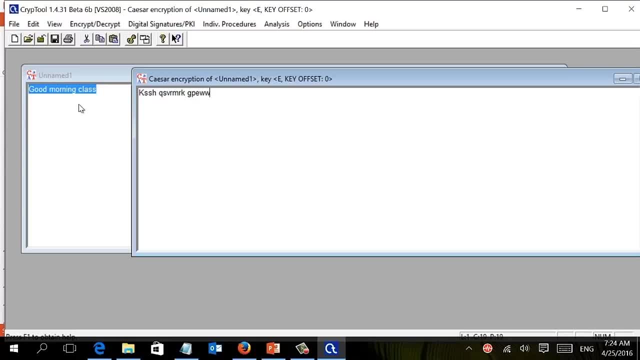 This one is 92 bit key. What is the key? the key It's the number of letters that has been moved. So this one, all alphabet, has been shift for four letter. So the key here is Four, and this is quite easy to decrypt because the key is very simple. 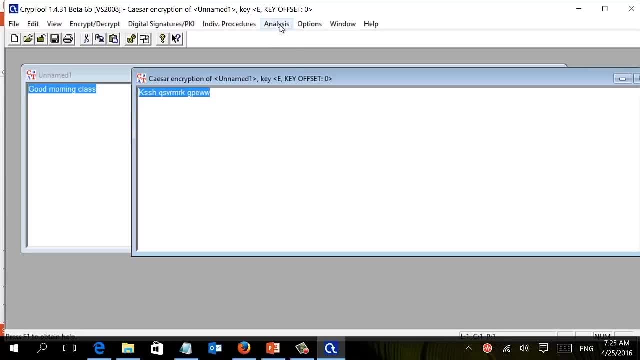 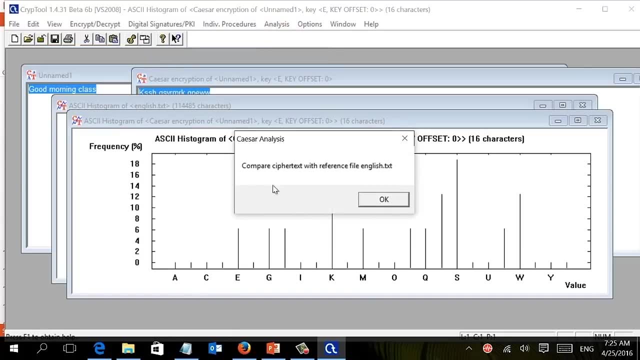 So if I just select an encrypted text and I go to analysis and we go to symmetric and cipher Caesar, he can start analyzing and he can tell you because he gave a dictionary file, He will keep moving letters and he until he get a readable text and he gonna tell you that. 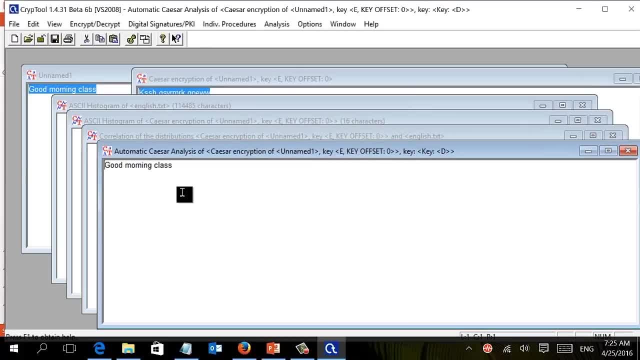 The last letter was D, So if I'm asking to decrypt, he can decrypt that. So the keys that we used right now was quite easy, because it was just moving all of them, the same amount of letter, which is four letter. Each one of those character has been moved for letter. 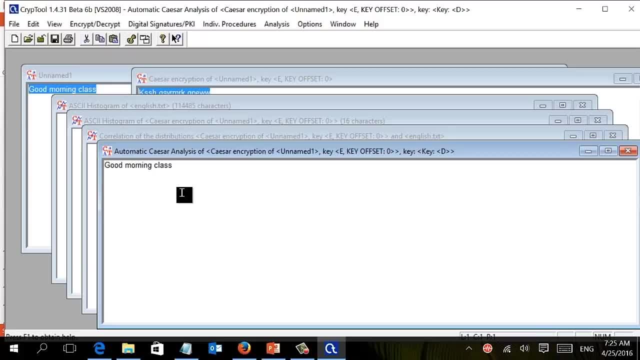 That's why it was quite easy. So algorithm is how to how the encryption is done, while the key is the number of letter. But what if the key was? has some randomization? So the first letter has been moved. for character Four letter. second letter has been moved. 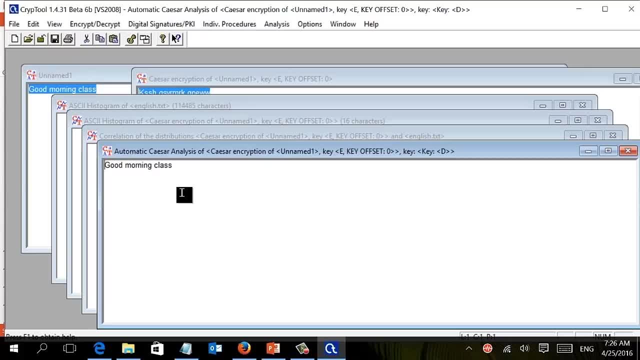 Six third has been moved to, force has been moved 11 and so on. This definitely will be harder to To decrypt. So when we are putting some randomization on the key, this is make the cipher more powerful and harder to decrypt. That's why, a very important thing that you should be aware of at the beginning of this domain- 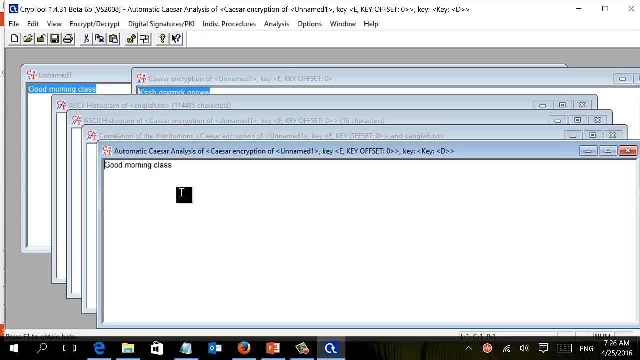 The rose Guy. His name was Kirchhoff and Kirchhoff said All encryption protocol should be public. Everyone should be aware of the public protocols. That's why we are all aware of how different encryption protocol are working. I can tell you how md5 are working, or LM hash are working or shower working. 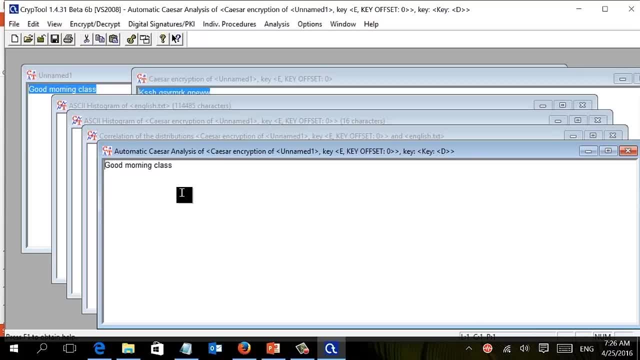 So it's it's public, while what is the secret part, It should be the key. So what should be kept secret, It should be the key. It's a very important saying that. we need to be aware of that. the encryption protocol should be in public. 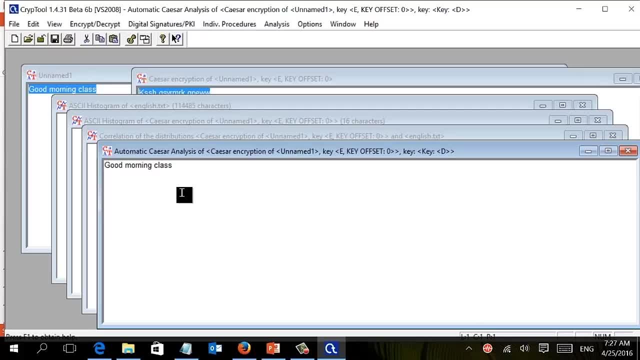 So all people that work in this field: they know how the md5 work and LM, hash and different kind of protocol, But where is the secret part that prevent people from decrypting? They know how the protocol is working. is the key? Okay, so the key should: 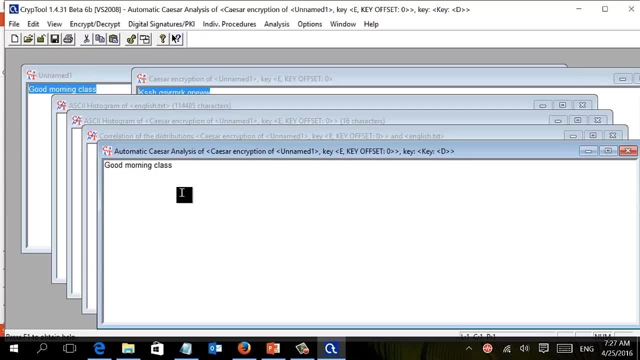 Should be kept secret and the protocol should be public. and why should the protocol should be public? because when you put something public to everyone, a lot of eyes will be reviewing it and a lot of flow will be found and it will be solved. So it will be more secure. 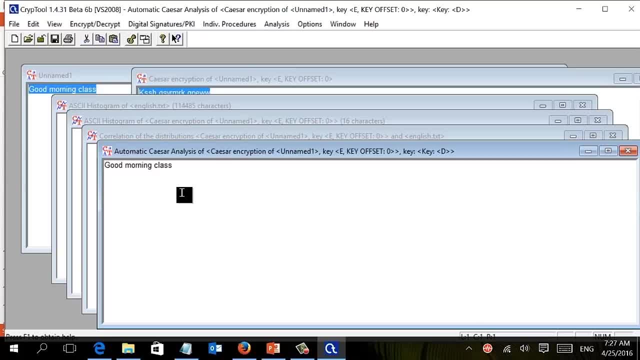 That's why, according to IC square, you should never suggest to create your own encryption protocol, because you know those protocols that we are taking during this domain has been Tested. but if you do your own, who will be testing and you keep it secret, and so route encryption protocol should be public. 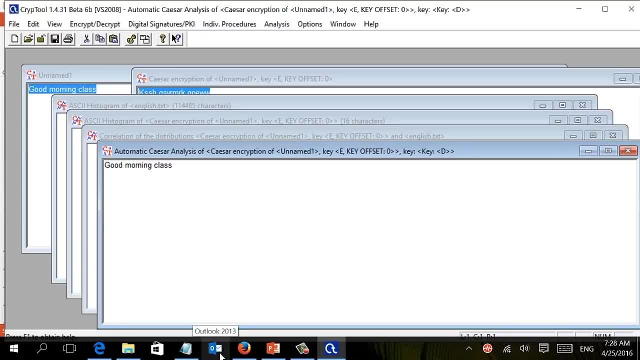 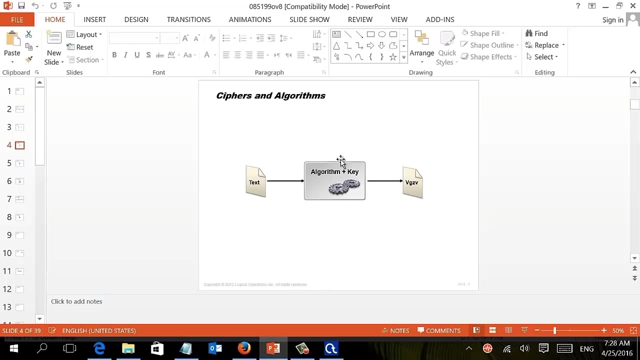 Well, private key should be kept secret. This is a secret part of encryption and also very important to know that it's not the guy who mentioned that or Who. His name was Kirchhoff, So this is also very important. So this is algorithm, different between algorithm, which is the way, and the key, which is a secret part, moving the letter four or six or two and so on. 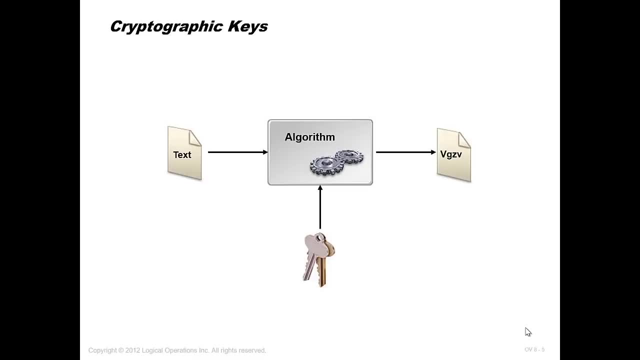 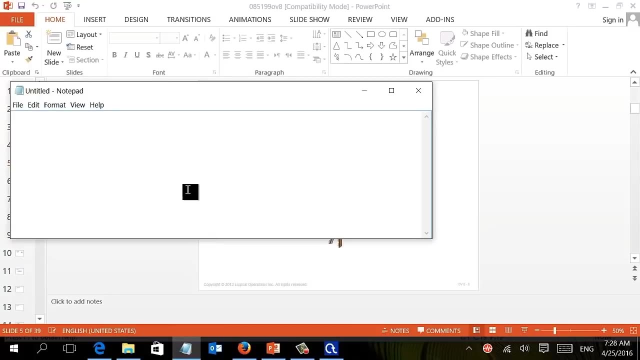 Okay, so we have a key, another. good, Now, this key has a meaning. I mean, when you see that we have a key, That is, this key is for instant One hundred twenty eight byte. What exactly does that mean? It means that this key has a number of randomization, which is two of the power of 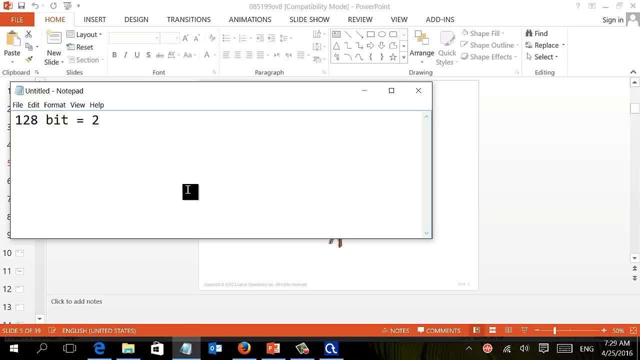 Can't find the power of, Okay, let me write it down. Power Of, sorry, One hundred and twenty eight. So when we are talking about a key, that is, the length of the key is one hundred twenty eight bit, It means that it has the number of randomization that it can generate. 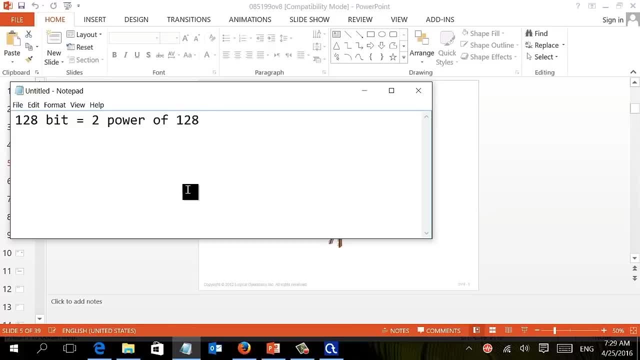 It's two of the power of one hundred twenty, eight, five, twelve, two of the power of five, twelve, and so on. That's why whenever the length of the key is bigger, the number of randomization that he can have is bigger. It would be harder to decrypt. 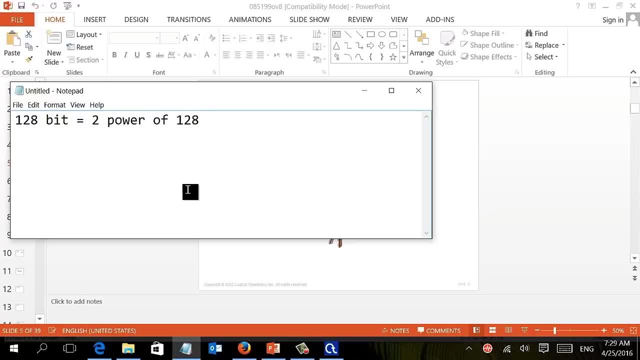 So why not making all the algorithm with A very big key? because it's taking a lot of processing. So it's not wise to use all your encryption with a power with with the keys, That is for instant one thousand twenty four, because this will kill your network. 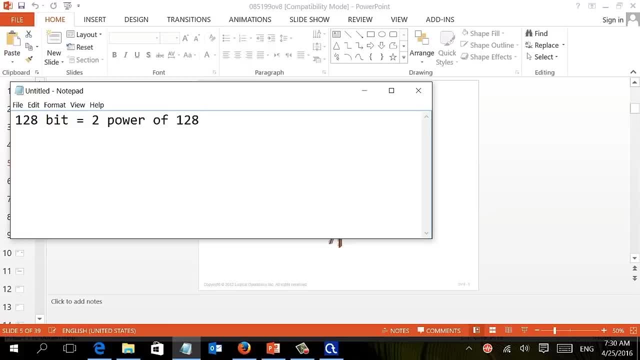 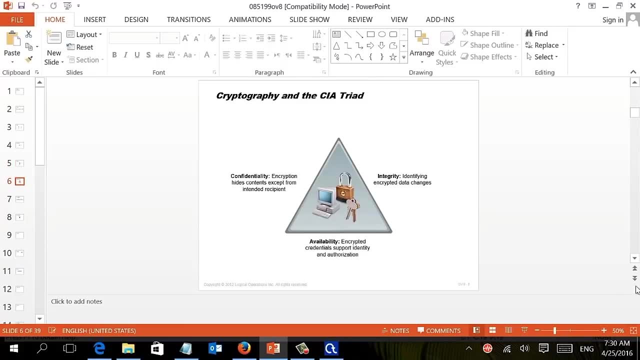 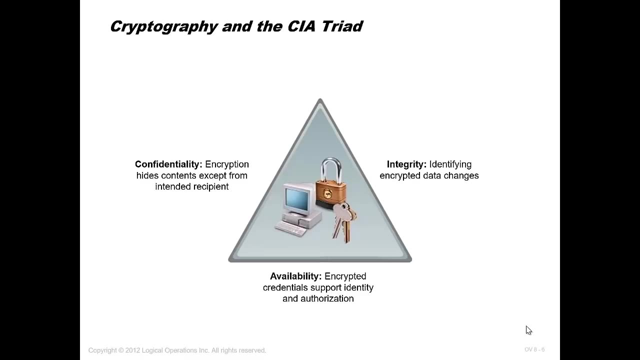 It will. it will generate a lot of processing, Okay, So don't forget that all the key are all the encryption, are well known how they are working And, as we spoke, that key are providing Cryptography, are providing confidentiality and integrity, but encryption has nothing to do with the availability. 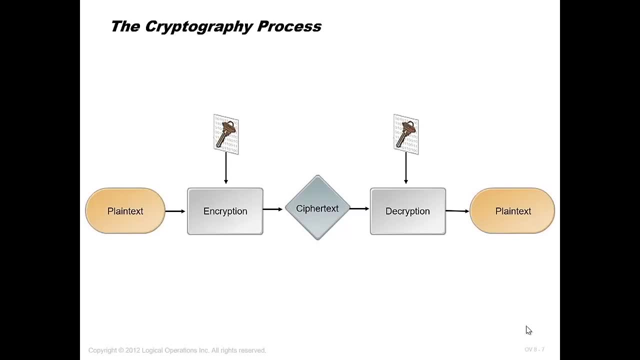 We are talking about confidentiality right now, but later on I'm going to show you how it provide integrity. So this is a process. We have a plain text using a key. It will be encrypted, Then it become a ciphertext and using the same key. 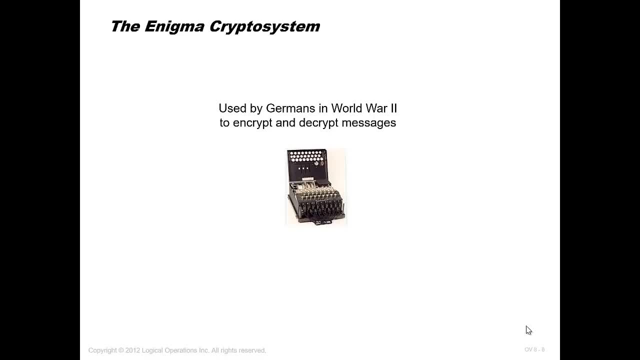 It will be decrypt and then a plain text. There is a small part in this course that talk about this History of cryptography. Who invented it was you know. they are talking about Julius Caesar and different ways that he using the cryptography He was shaving the messenger head and write on it and wait until his hair grow up. 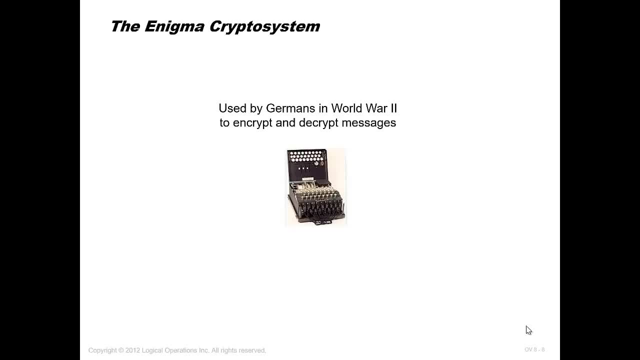 And again, this is one way for doing that. They were doing on a rope, writing on rope, and there was a method for doing that, And the first mechanic device was a device called Enigma And it was invented in World War Two and there was a movie about it. 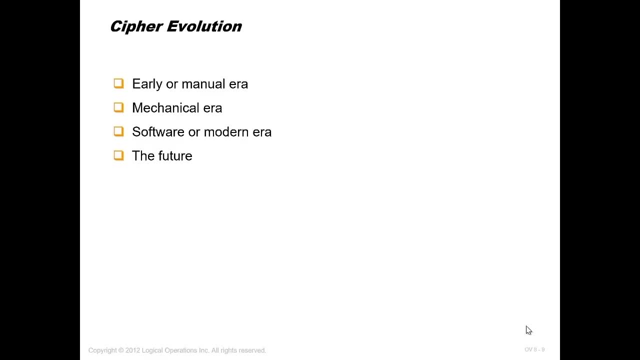 By the way, this was the first mechanic one, But right now you know there was an early area of encryption. There is a mechanic era. Now there is a software era. We are doing encryption by software- and there is a future. 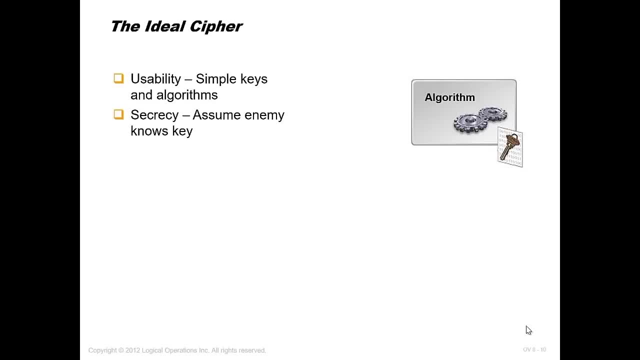 No one know how it will be done. The problem with cryptography, as we mentioned and as we're going to see inside this module, that we need something that is Simple, do not have a processing or do not need a lot of processing, and also need to have something secure. 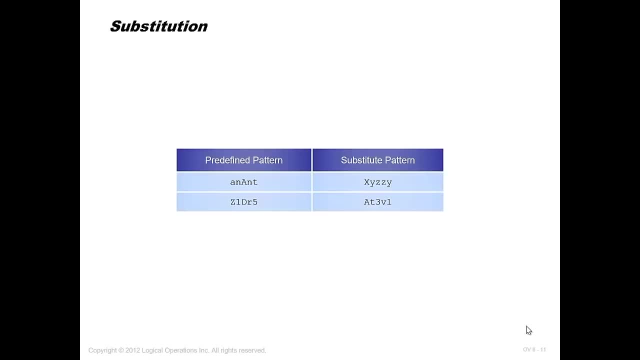 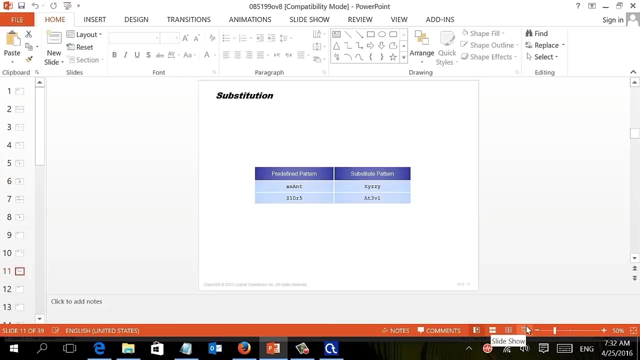 It's not easy to find something like that. Now, this is two terminologies that you should be aware of. Trump was a substitution and- sorry- substitution- and transposition. You should know that All the encryption protocols that we'll be talking about, they are all using the same or they are. 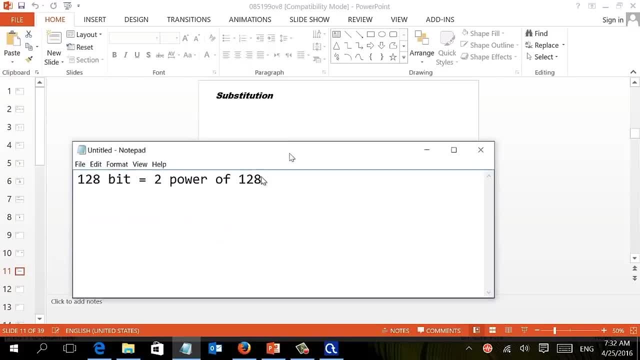 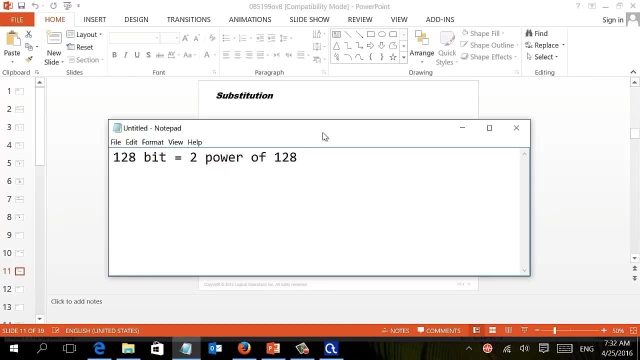 Depend on two different way. The first one, it's called the substitution, So all of them are done in using only two techniques: substitute. substitution and transposition. Substitution is the techniques that I just show you. encrypt tool few, second back, which is moving the letters. 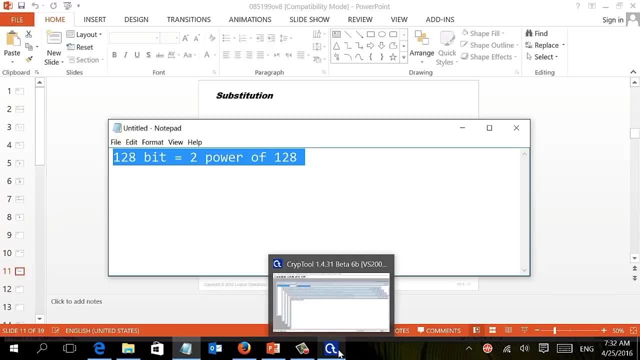 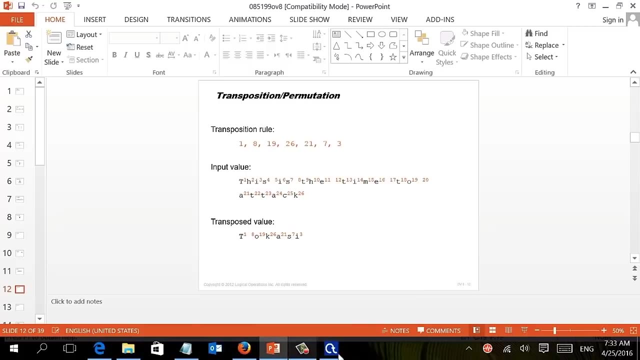 So one technique is used by most of the- maybe all of the encryption protocol Is a substitution, is shifting the letter. Okay, the same way Caesar encryption is doing transposition is to change their location horizontally and vertically. Let me show you how. I assume that I'm writing down something like that. 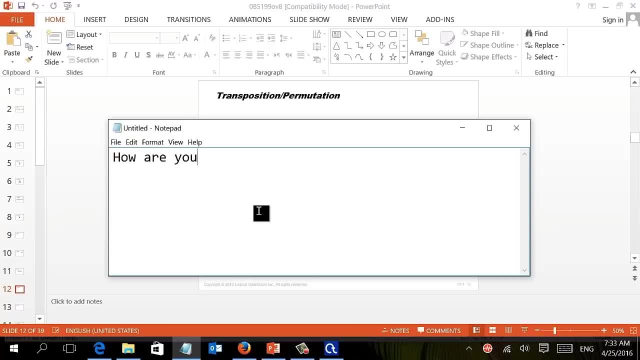 How are you Now? if I need to do a transposition, here's how it will look like I'm going to take them. How are you? And we'll write down. It's all The first. I'm taking the first one. 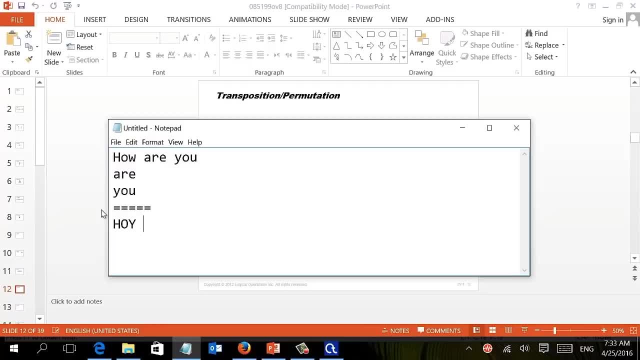 It's all why, and then All are all. and then W He you? This is called transposition. I change from vertical to horizontal, So the how are you became like this? So all the encryption protocols that we will be talking about are using transposition and substitution- substitution. 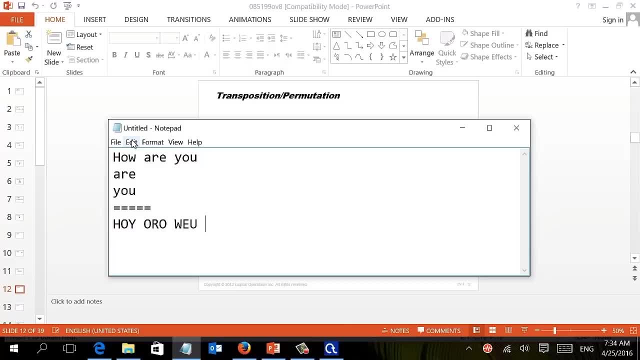 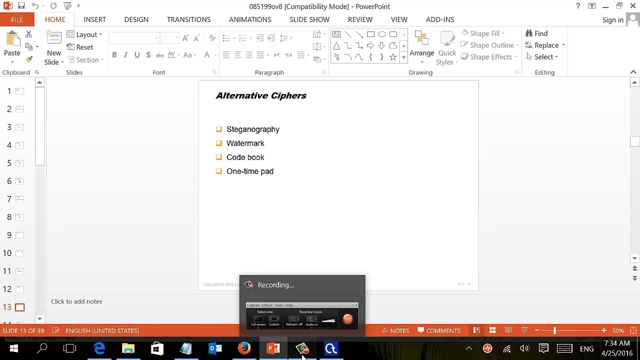 Just shifting. the letter and transposition are moving horizontal and vertical. Now, on the next lecture, We will be talking about some alternative cipher. I mean, do we have different format of the cipher, a different way for encrypting? Let's see a different encryption method. 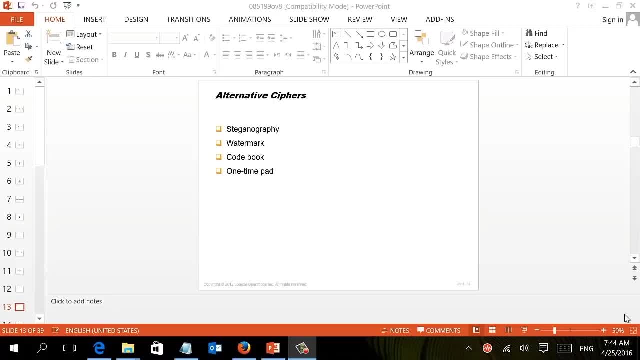 There is different type of cipher. Not all of them are unreadable text Like the one we saw on the previous lecture, but there is different format for hiding a text. One of the format I would like to talk about is called steganography, which is hiding a text, or hiding any information into a picture. 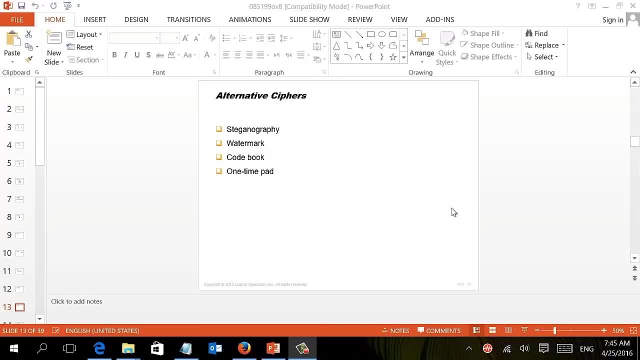 This is called steganography because it will lead to the same result: information. information will not be available or will not be accessible unless for authorized user. So I would like to do a small demonstration to show you about steganography, Just to try to hide any information could be a text, PDF file in Excel sheet, anything into a picture. 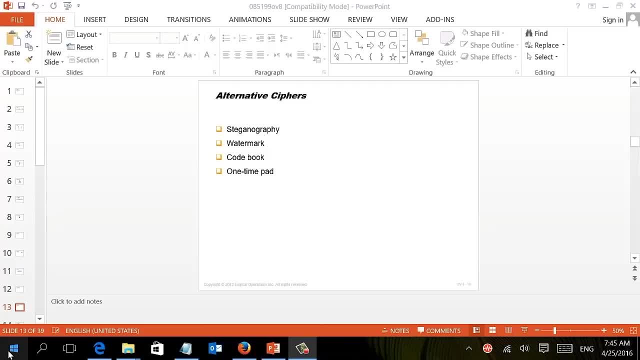 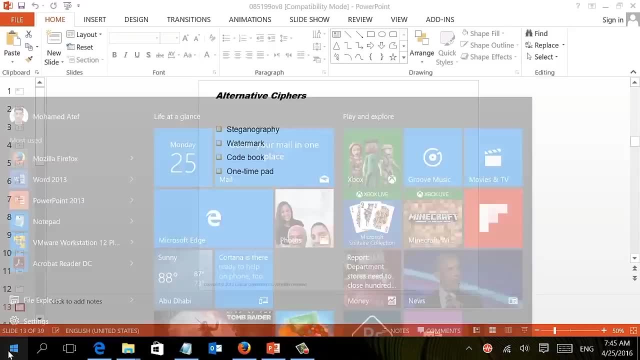 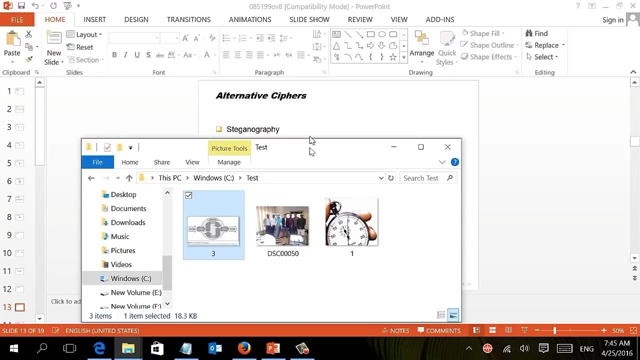 I'm going to show you how we can do that manually. Actually, there is a lot of application. who's doing that? like invisible secret is a very common application. but I want to show you how to do that manually. But before showing you, I want to show you the setting I prepared for that. 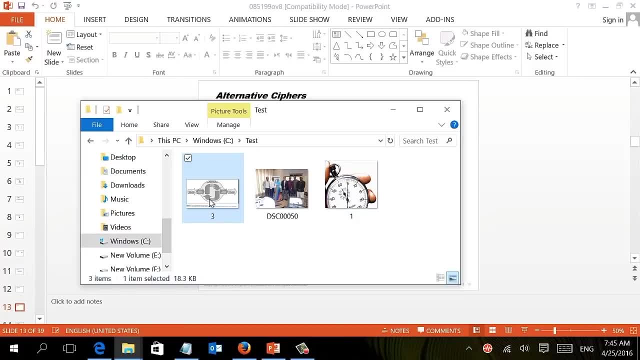 So I have a folder here that has two picture, picture number one and picture number three, And I would like to hide picture number three into picture number one. picture number three could be a picture, could be a text document, could be anything. now Let's check their size first. 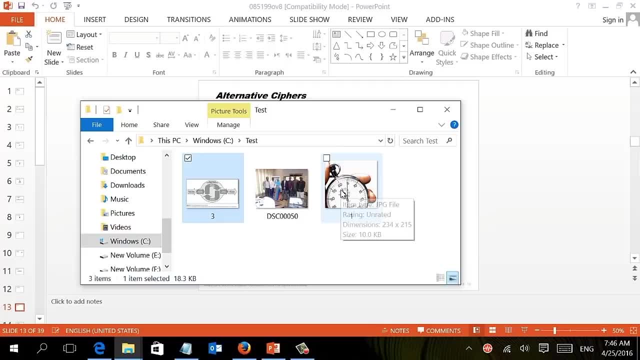 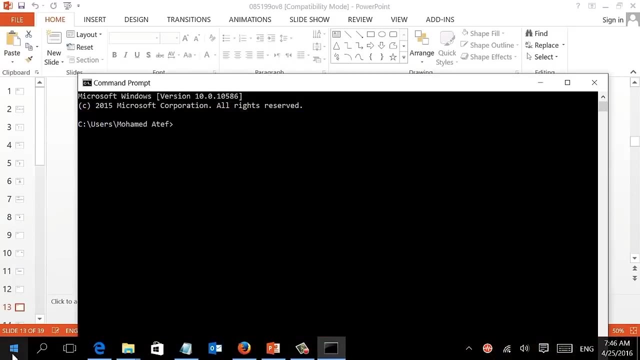 This file is 18 kilobytes, while this file is 10 kilobytes. Now let's go to the command line. This is in a folder called test on the C drive. So let me go to the command line And let's go to test. 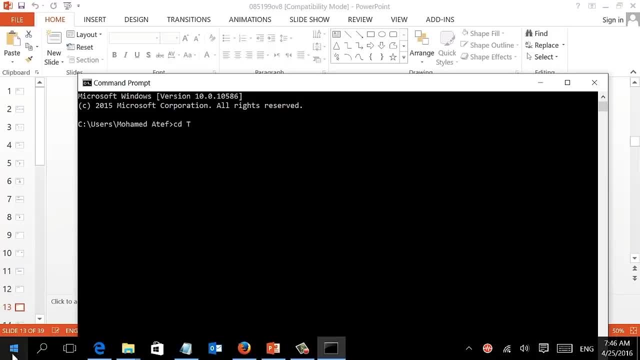 Oh sorry, go to the route first. Again, there is some application. who's doing that? But the reason I'm doing this demonstration, because I would like to introduce a new skills for you. Let me show it to you, But let's do the example first. 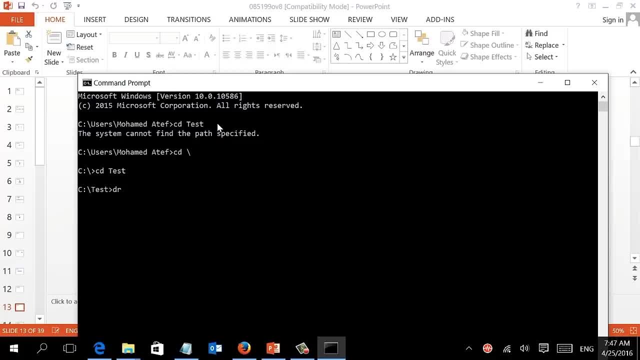 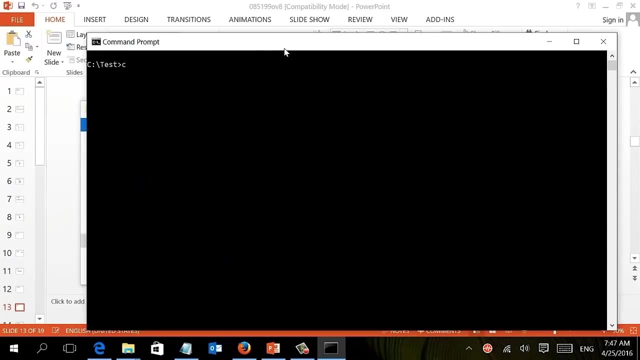 CD test And then we can check the file. We have a file called one- GPG- and a file called three, the GPG. So here is how to do that manually. Let me clear the screen And we're going to type copy. 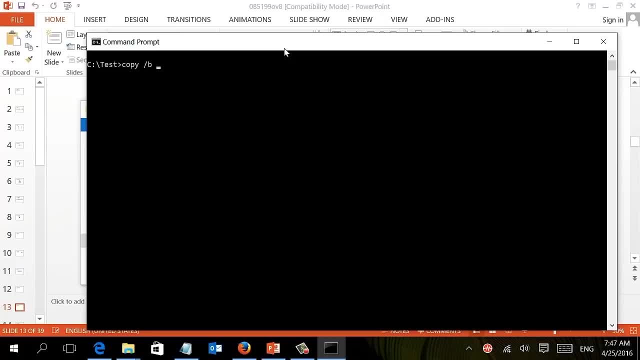 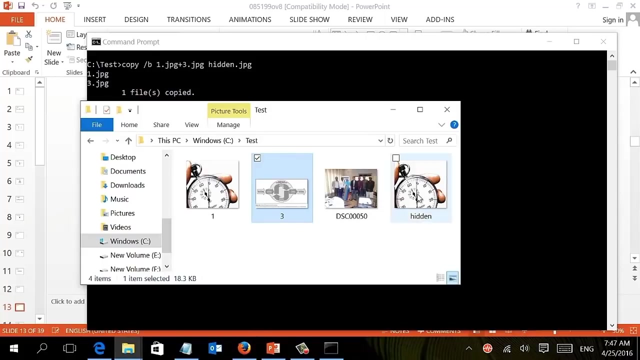 Then slash, be mean copy the binary of one dot GPG Plus three dot GPG into another file called hidden Dot GPG, And by doing that both file has been combined into a file called hidden. Let's see, So we have a file called hidden right now. 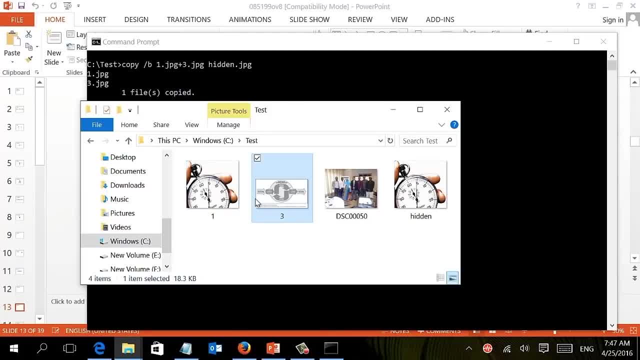 That should has those two file combined together. So this file it's hidden. now Another copy from this file Inside the hidden file And if you want to check, you can check the size. You notice that the size is 28, while this was 10 and this was 18.. 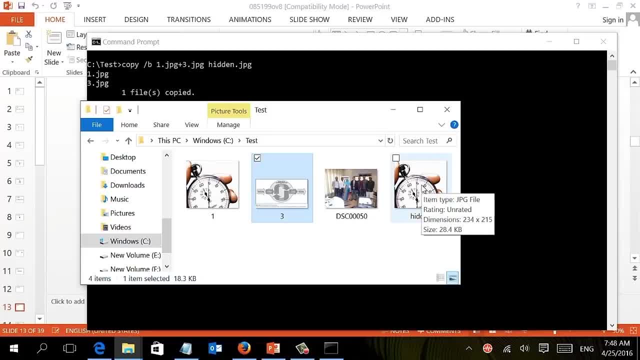 So This is the steganography concept. Now, what I want, what I want you to be aware of, or the skills that I would like you to learn, It's: how can we identify that? How can we know that this file hide another file? 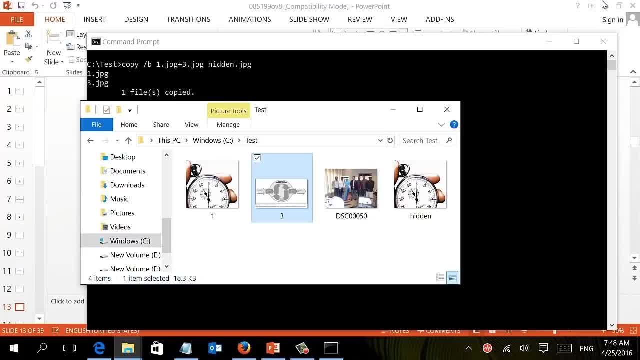 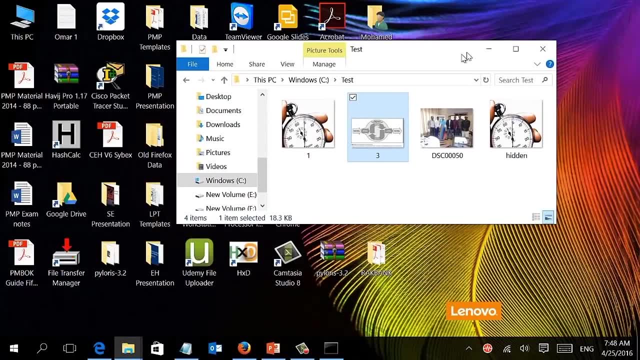 As I told you, it could be Image, could be a excel sheet, whatever. Okay, so I would like to introduce for you something called the hexa editor That allow you to see the file the same way The computer is reading it. 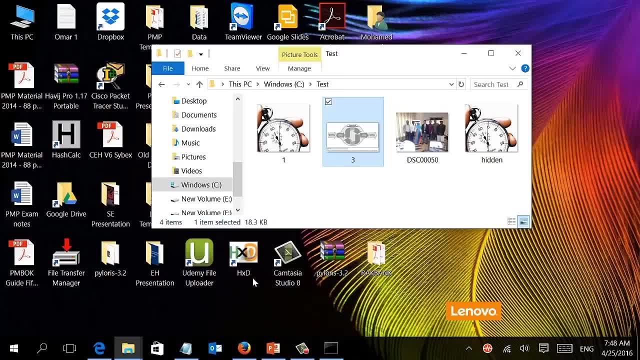 I mean, this is one of the applications called a HXD and you can download this one or any other application. Hexa editors, just Google it free. a hexa editor. Now, when you open this file, this program, I'm sorry, it will allow you to open any file, but you will. 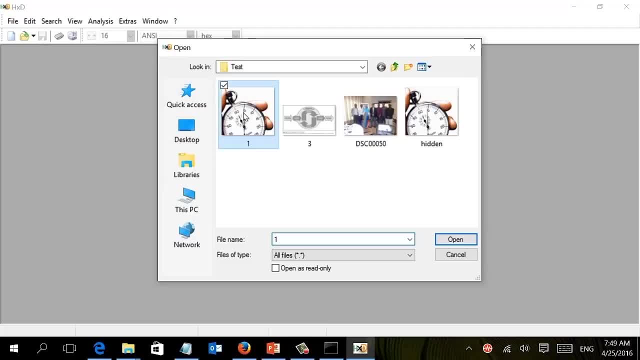 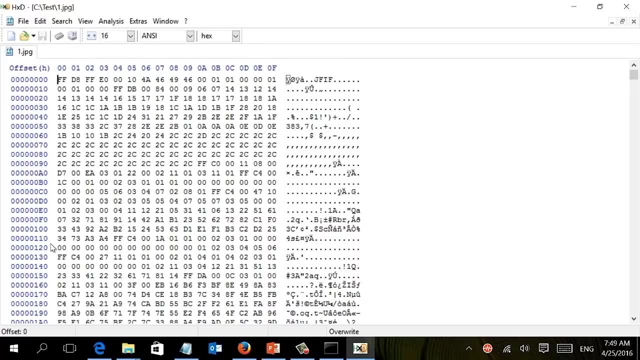 Open it the same way The computer is reading it. I mean, if I open this file, it will open in hexa format. Now what is the use of that? A very important use. Most of the file has some standard characteristic. 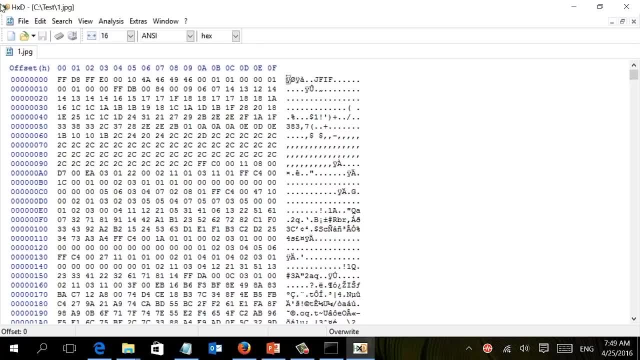 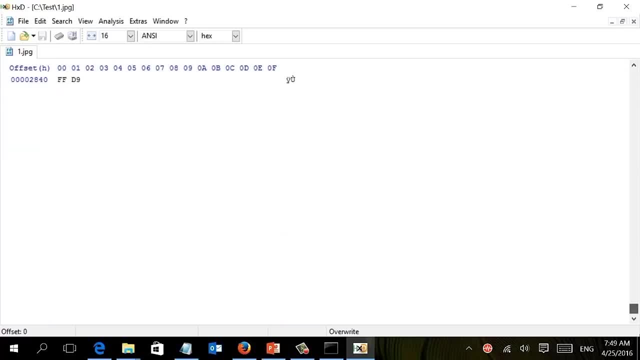 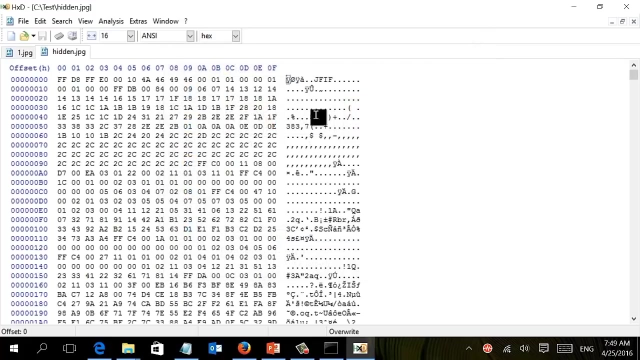 For instance, all GPG image start with FFD eight And end with FFD nine, While BMP has different start and different end, while TIFF has C. So it's Start with FFD eight and FFD nine. According to that, if I open the file that has been combined, this one, this one should include the two files together, right? 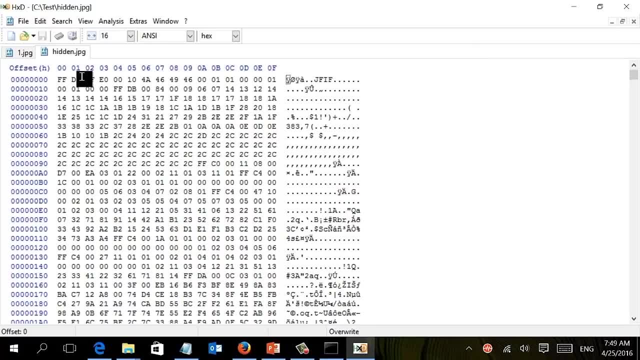 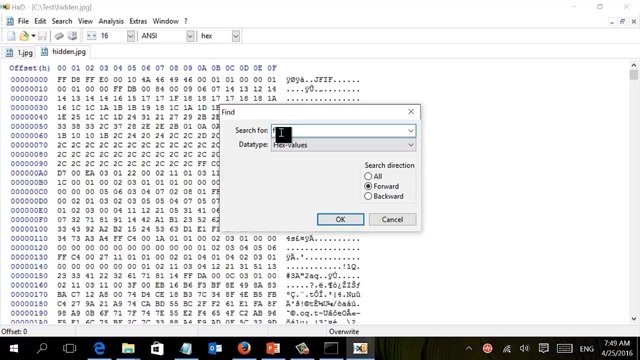 How many FFD eight. you should find Two, because it has two picture inside and how many FFD nine also to let's see. So if I go to search and ask him to find a hexa value Which is FFD eight, So you're going to show me the first one. 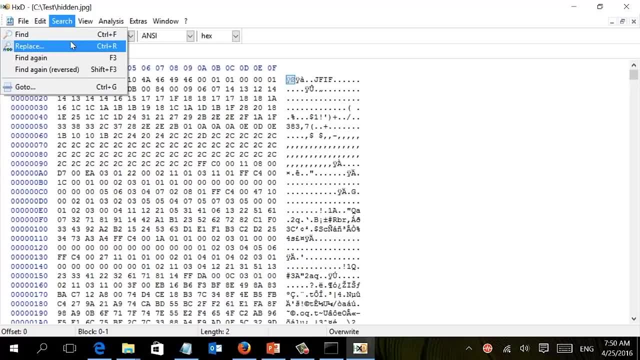 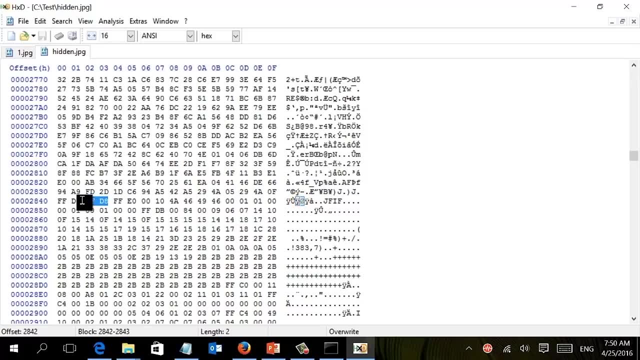 I can then go to search and tell him find again, Show me the second one, so he can show me the second one. And if you see the character before that was FFD nine. So this is look like the end of the first picture. 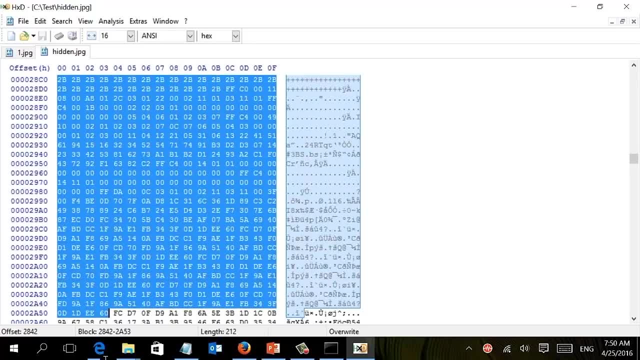 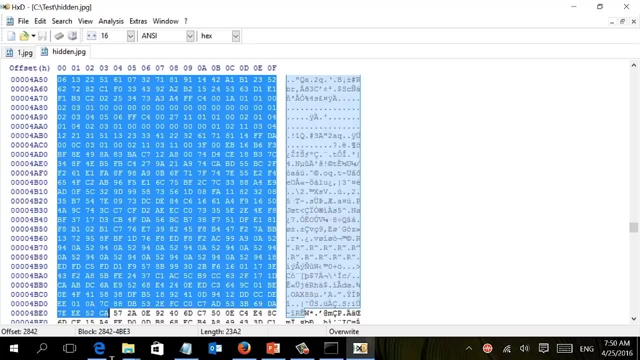 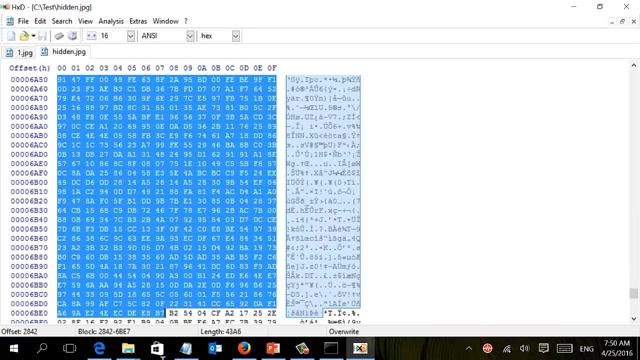 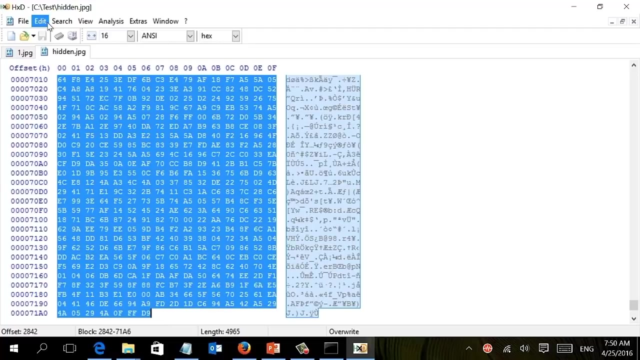 And this is the start of the second picture, and you can even extract it. You can right click on select set. It's a big one, but you know, Here you go, The end of the file and you can copy that, edit, Copy and go to a new file. 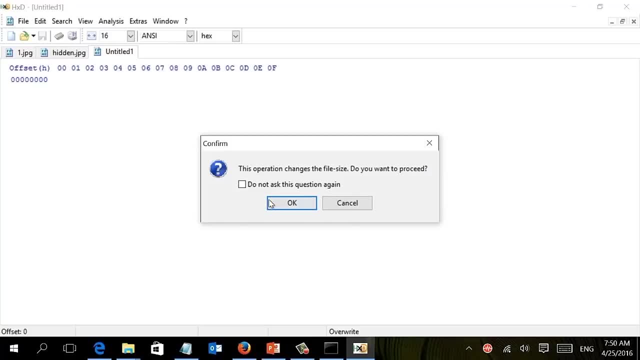 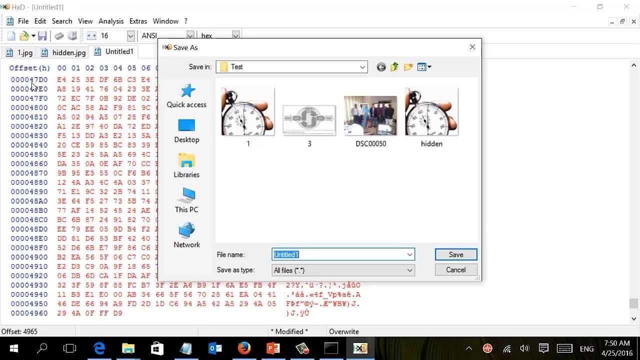 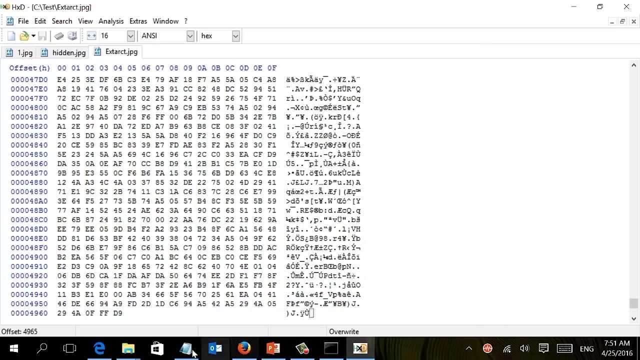 And paste, Okay, and then you can name it save as I'm going to name it for instant extract X track. It's It's Tracked Dot GPG And, as you can see, I was able to extract the file in the folder. 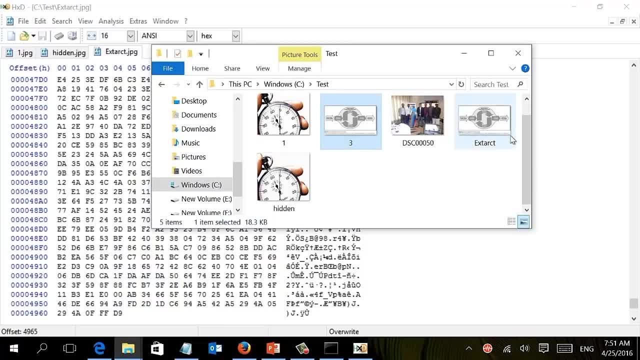 Let's get back to the folder so you can see the file has been extracted. Where is it? Here you go. So I know we are talking about forensic now- It's not The subject, But I just want to show you that file has different characteristic and it will be good. 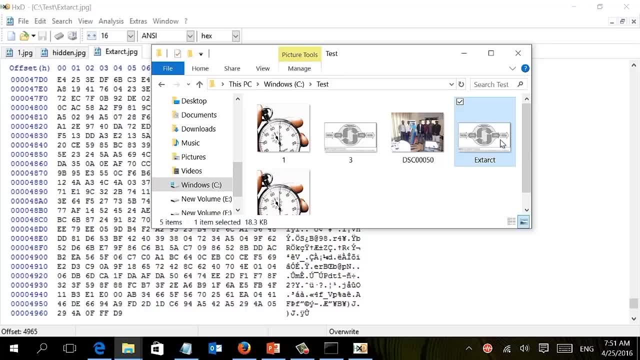 It will be good If you are aware of what is the GPG file start with and end with and you open this Hex editor in different file and check you know something similar between them. beside, Hex editor has another benefit. Do you see this part? 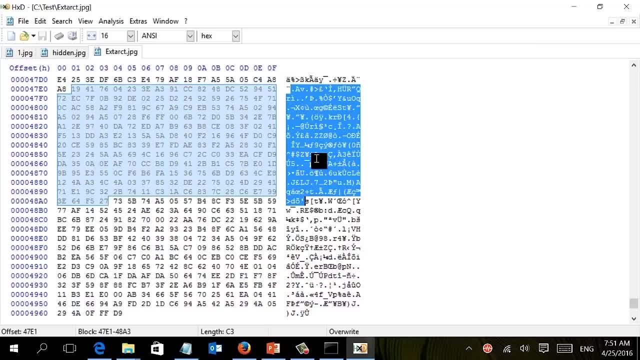 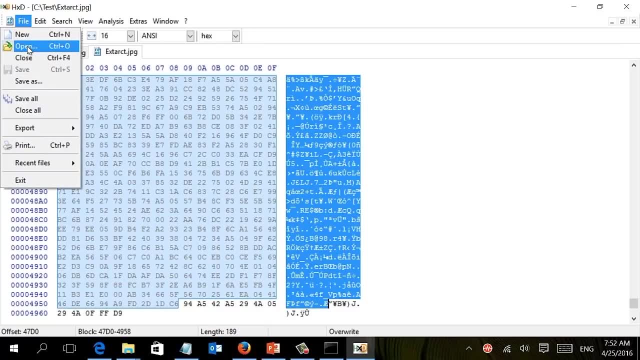 On the right side. This is called the metadata, Which is the information About the file. So if it's a picture, you can know from this metadata when this picture has been taking, like if I open this one, what kind of time camera. 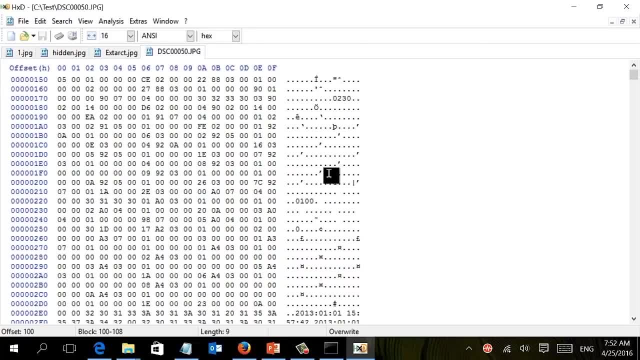 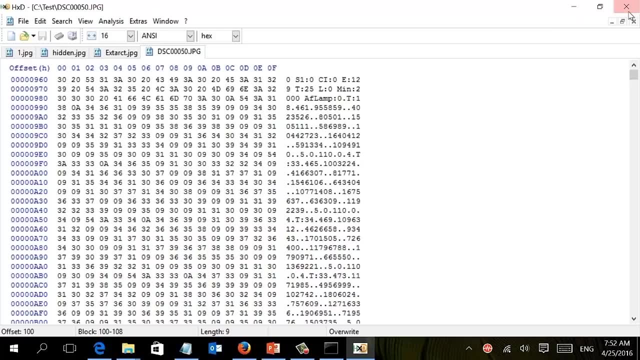 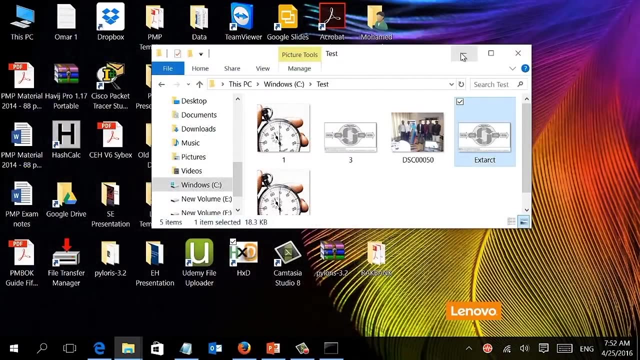 So here it shows you the date where the picture has been taking is a type of camera and it has the GPS location, So you can get a lot of information from the metadata. So I wanted to show you a small demonstration about steganography because just to let you, you know, getting a little bit. 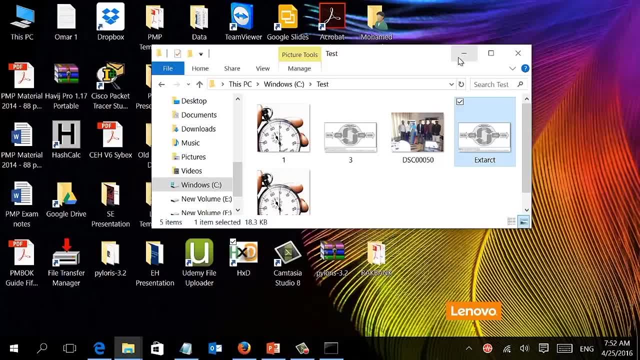 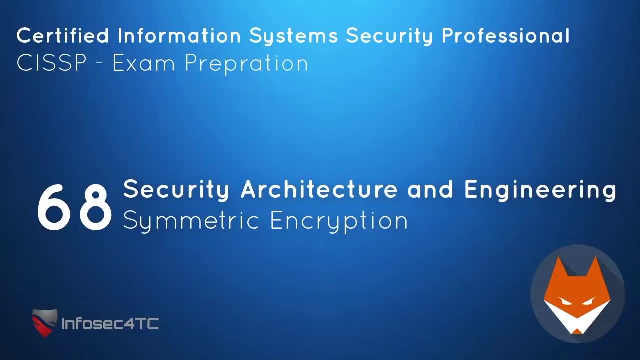 Deeper into file, not for the exam purpose, but for your own use, you know so Hex editor: It's a nice tool that lets you know a little bit about some characteristic of the file. In cryptography we have two method for encryption. 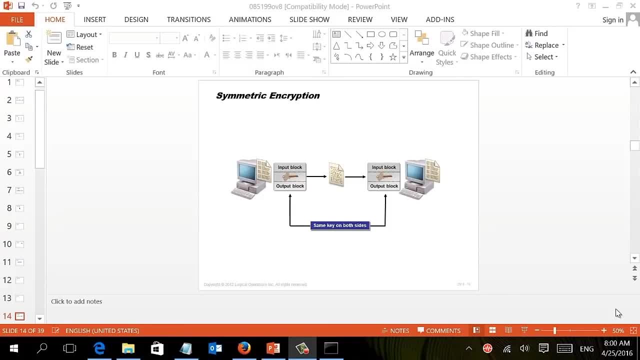 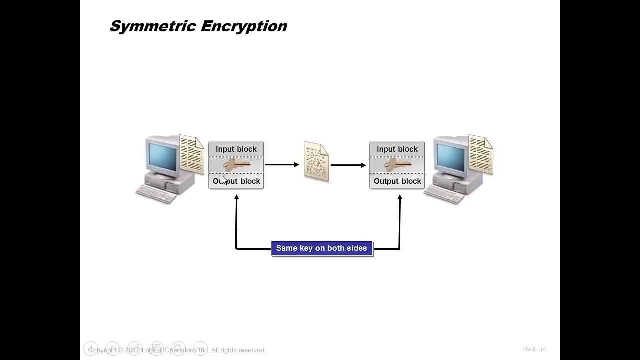 We have the symmetric encryption and we have the asymmetric encryption, So we're going to talk first about symmetric encryption, Because this is a commonly used one. Now, in symmetric encryption, We are using one key for encryption and the same key for decryption, The same way we did on the previous lecture in this domain. 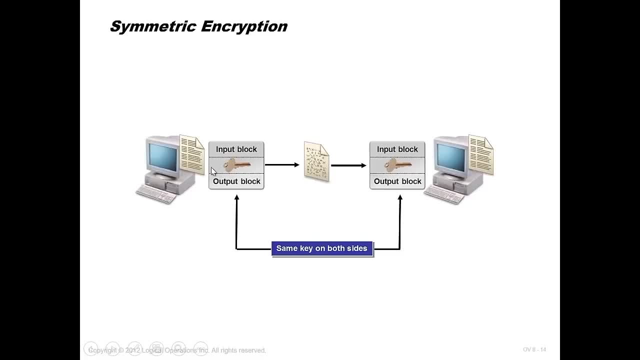 So you have a text you encrypt. that was a key- And then you send this key to the other side and with the text, and ask him to decrypt using the same key. So you are using one key For encryption and decryption. Now, before going and resuming, or before resuming the explanation, what could be the problem with that? 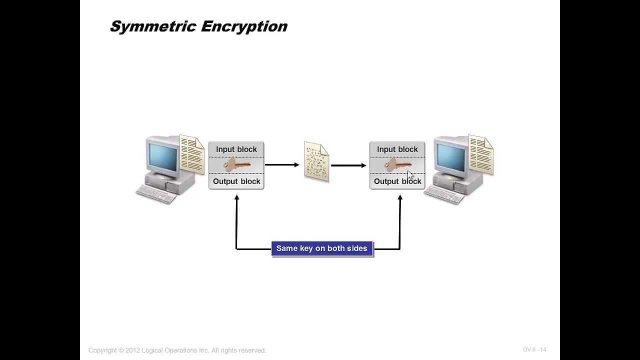 The problem with that is that now you need to think about different way for sending the key. I mean, you cannot be sending An email encrypted with the symmetric encryption And attach the key with it, because because whoever compromise the mail, he will get the key. 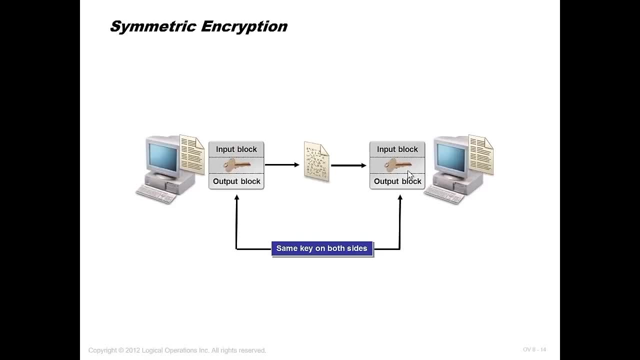 So now I need to send the email in one way and consider thing sending the key with a different way. It's called the out of band. I need to send it with a different way, So this become an overheads for me. I'm sending the mail by a method and then sending the key by another method. 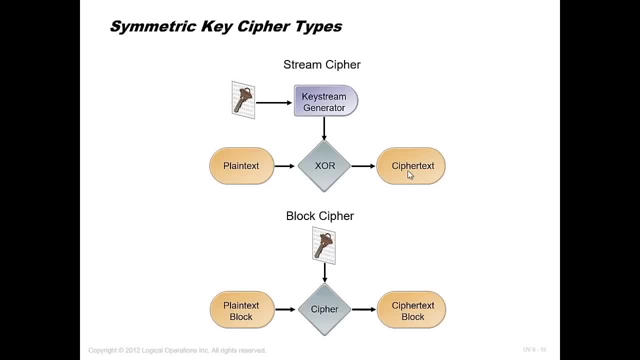 This is one of the problem, but it's not the main problem. Now, in symmetric encryption, We have two different way Or two different technique. The first technique that I need to discuss with you is the one below here, which is the block cipher. 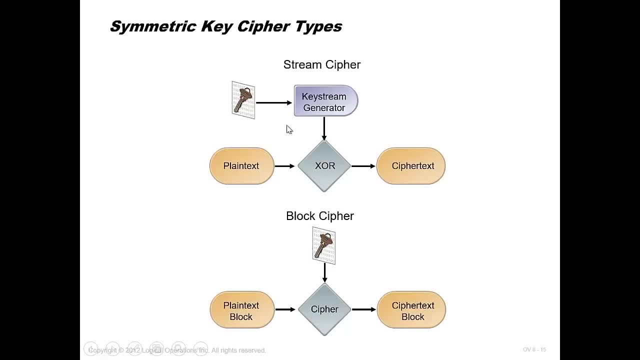 So symmetric has two type. We have the block cipher and the stream cipher. What is the block cipher? Block cipher is that, for instant, Assumes that you have a text or an Email that you can need to encrypt using a symmetric encryption, So he gonna take this email and he will divide it to different blocks. 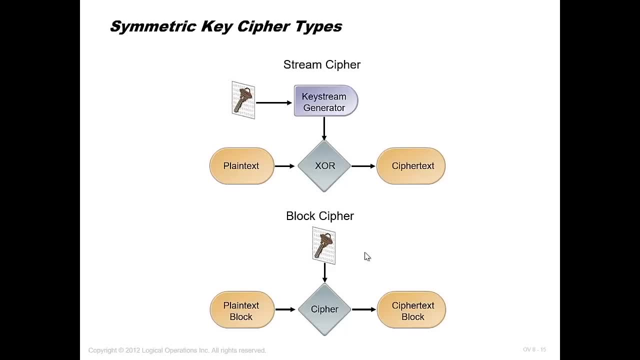 And with different, different block with a specific size, So you can have for instant. you are encrypting- forget about the email- You are encrypting an excel sheet, So he will take this excel sheet, divide that two blocks. Each block size could be 64 could be 32 could be. there is different size depending about. 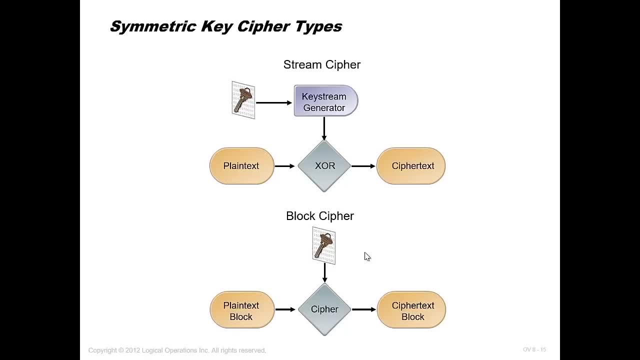 Which protocol, and then he will encrypt each block by itself. Then, after encrypting each block by itself, He will start moving them around. So now, to be able to recover, or to be able to decrypt the text, You need first to reorganize them the same way. 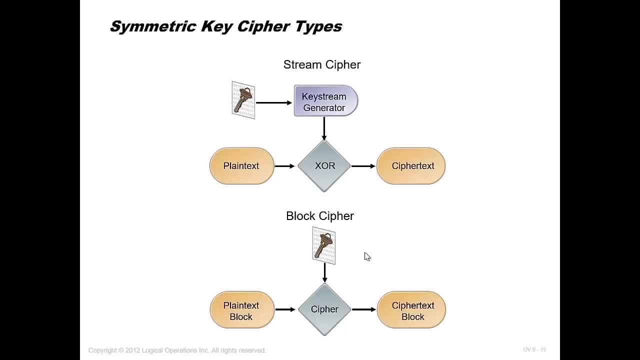 They are and then combine them together and then decrypt them. So block cipher is dividing the Text to different blocks. He's not taking the full text and encrypted. He divides them to blocks or pieces. the text to pieces and he will encrypt each. 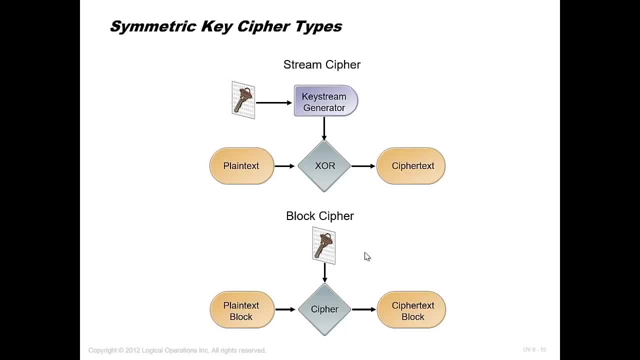 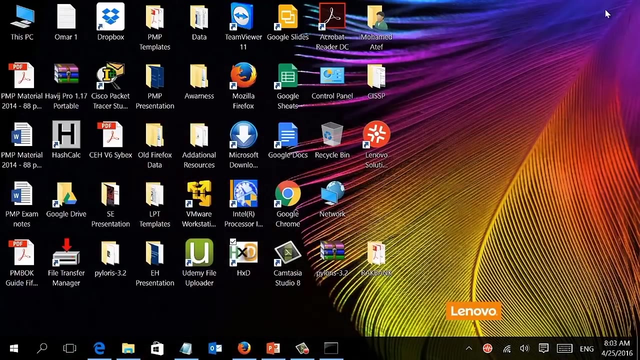 Pieces by itself and then He will start moving them around. Number of round. That's why one of the things that you're going to need to memorize- actually very few- protocol, You're going to need to memorize their characteristic, characteristic here. 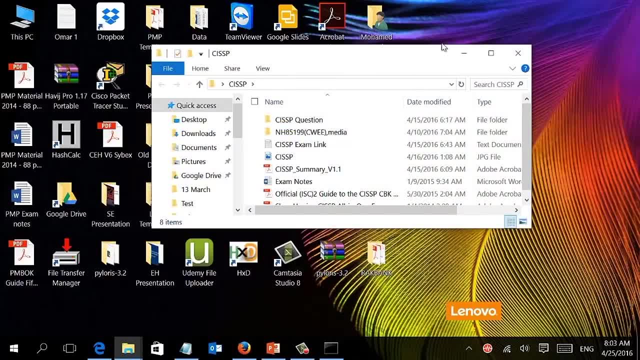 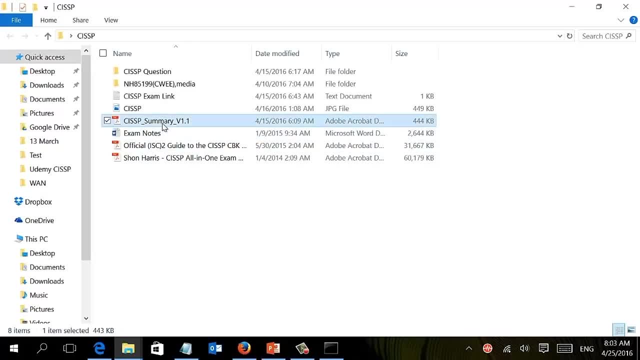 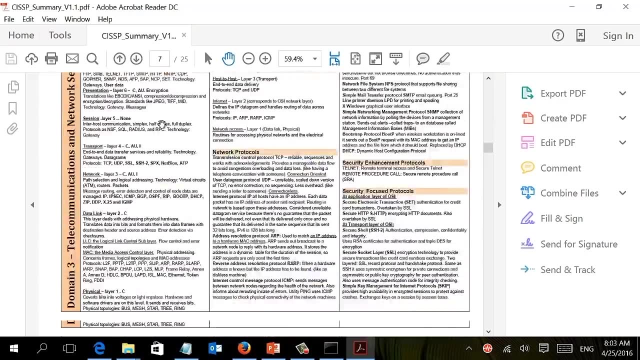 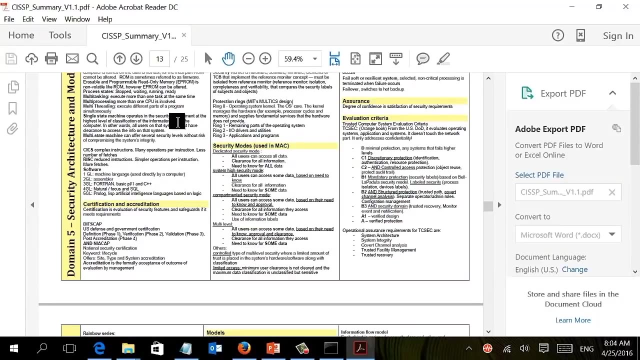 I don't mean just The key, because most people think I need to know the encryption and what is its key size. No, actually you have to memorize The key size, the block size. if we are talking about encryption, If we are talking about encryption protocol, block, cipher, encryption- 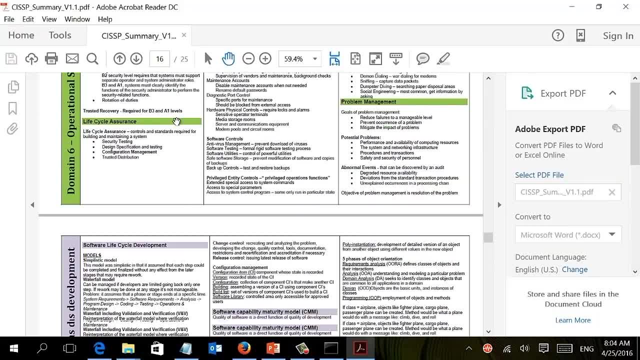 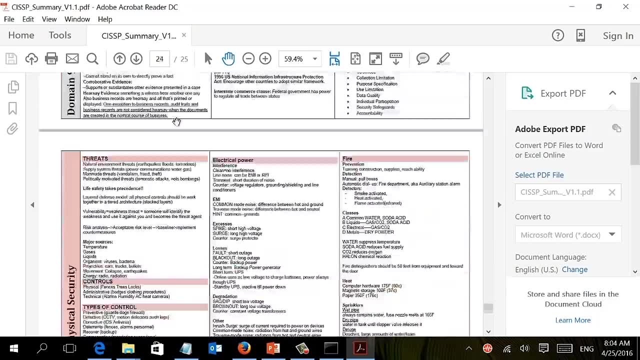 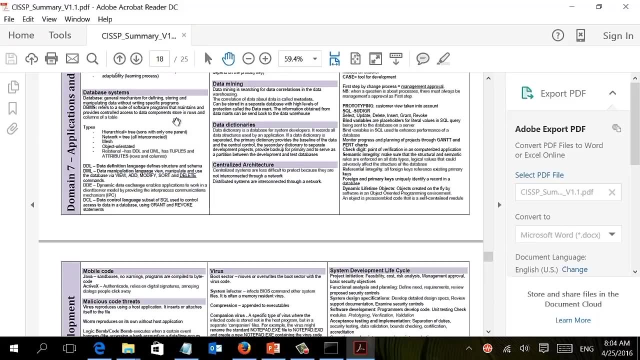 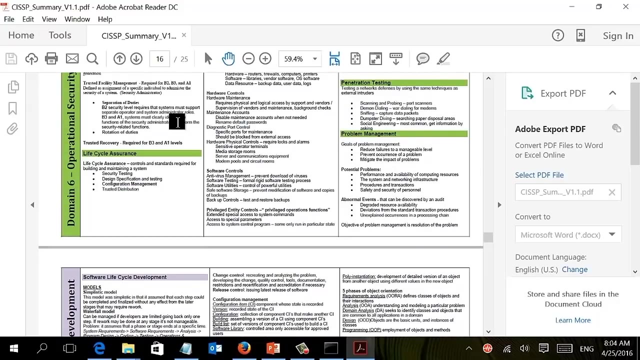 You need to know their, their. let me just get you the cryptography. It is continuity law and regulation- Think I missed it. So you're going to need to know their key, some of the protocol, their block size, their number of round. that will be moved. 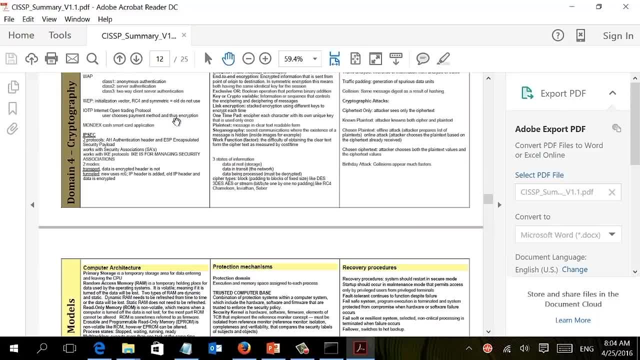 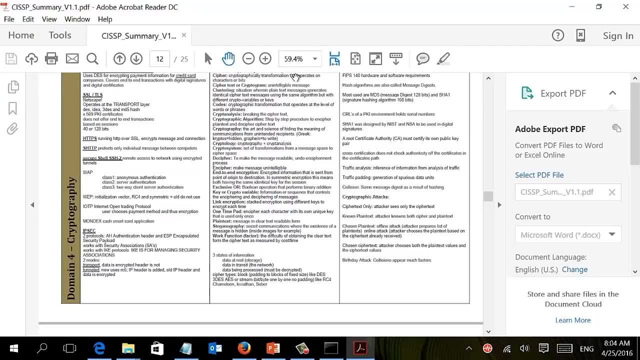 So you don't just need to know the key for those, but you need to know the specification, as this is one. So let's see, Let me just increase the size And don't get panic because, just like four or five protocol, You're going to need to know this kind of characteristic. 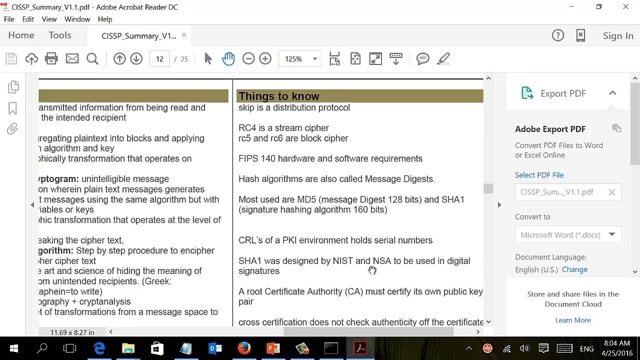 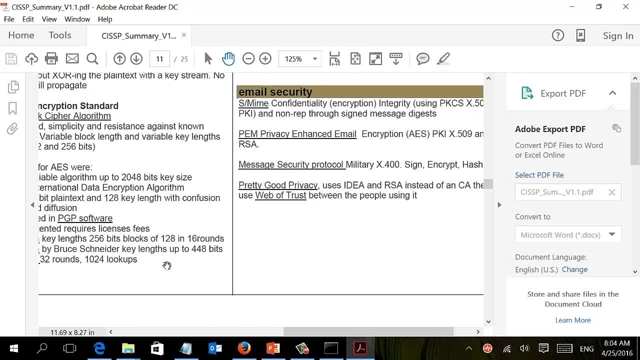 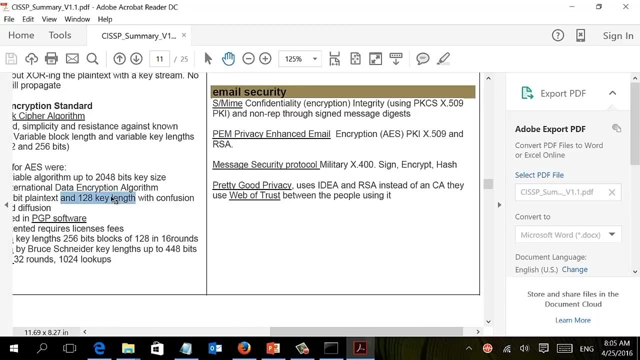 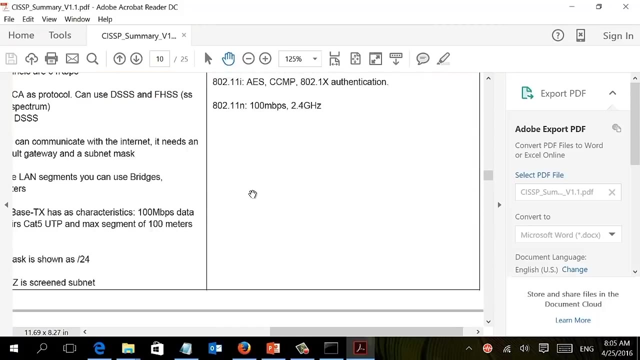 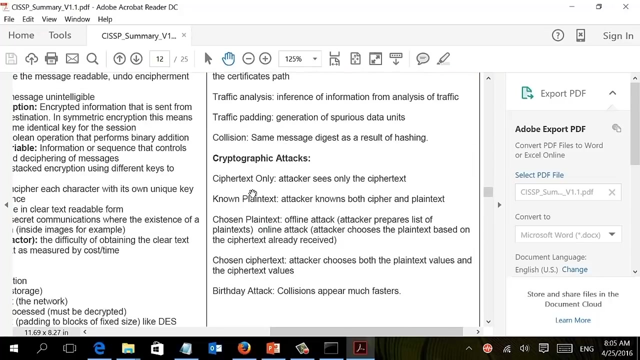 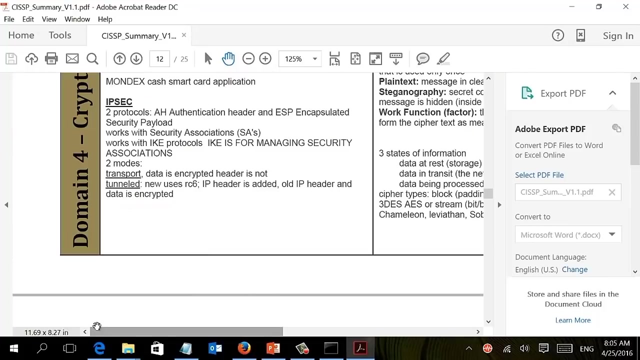 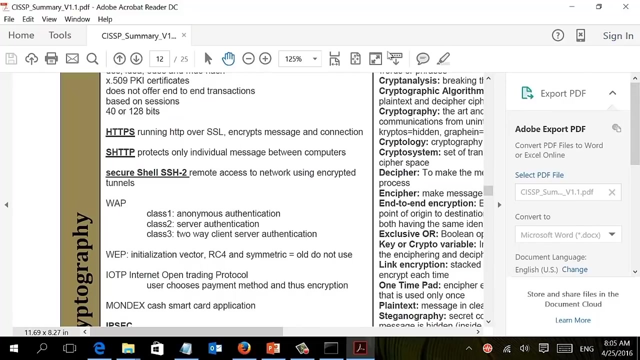 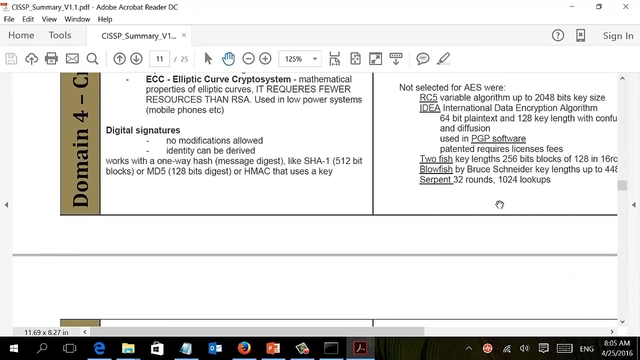 So let's see Where are they. I think here I'm just trying to show you what are you going to memorize for the exam. I'm just trying to show you what are you going to memorize for the exam. Block size. 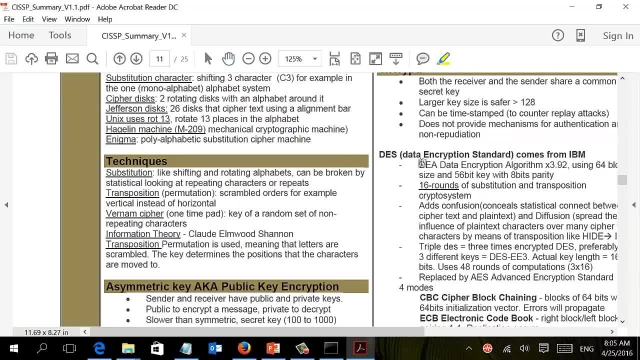 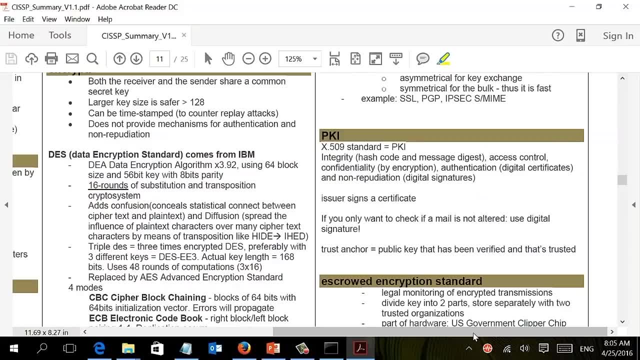 Yes, here you go. So, as you can see, those specific protocol you're going to need to know, for instance this: Okay, this is encryption protocol Using the key size is 46.. The size of the key is 56 bit key. 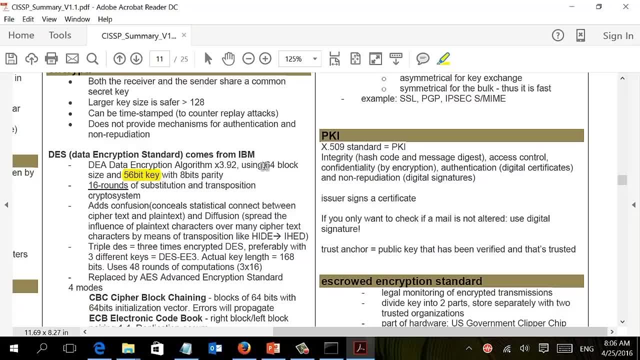 Okay, and it will divide the text to blocks. Each block size is 64 bit, as set. 64 block size and how many round he will do? 16 round. So only few protocol, actually, this section only that you're going to need to know for those protocols. 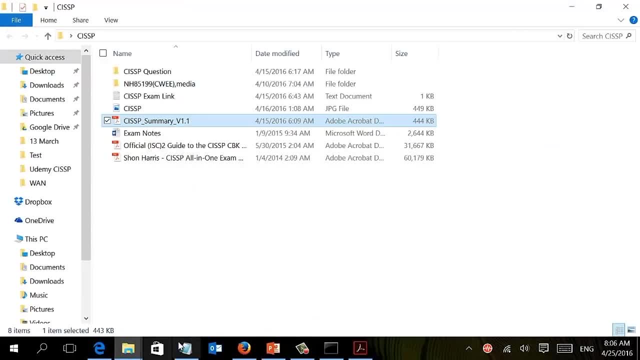 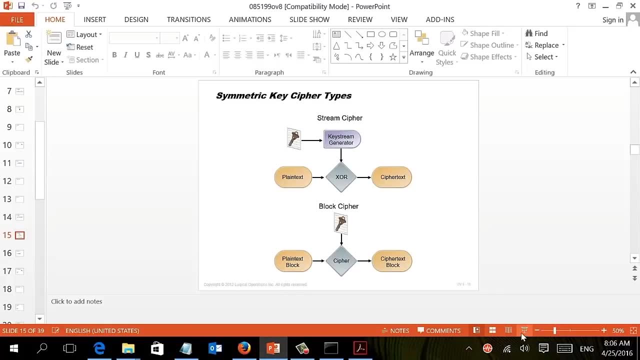 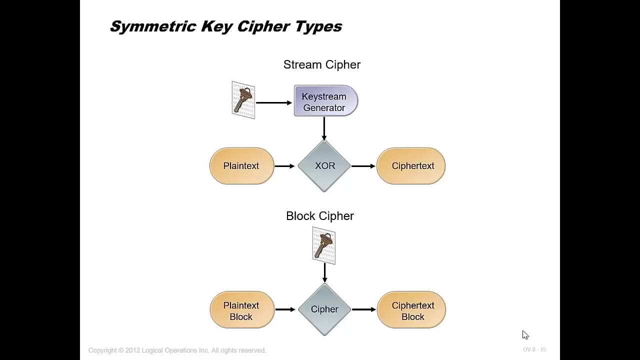 They're blocked: Block size, number of round and the size of the key Or length of the key. So this is the block cipher, while the stream cipher It's it's encrypting bite by bite And so it's not dividing them to block or pieces. 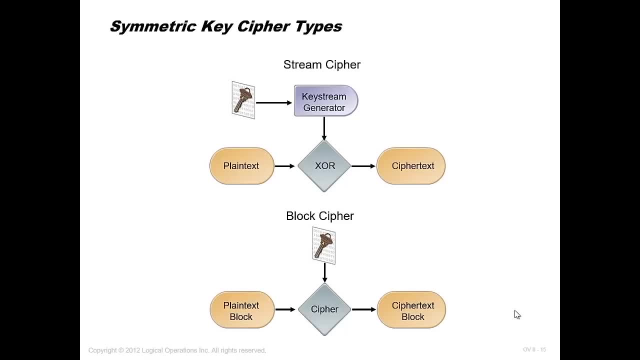 Just taking the text and encrypting them bite by bite, and they are using mathematically something called XOR And XOR, Just one on one, equals zero, zero and zero equal one. I mean, you know there is because after all it will be convert to binary. 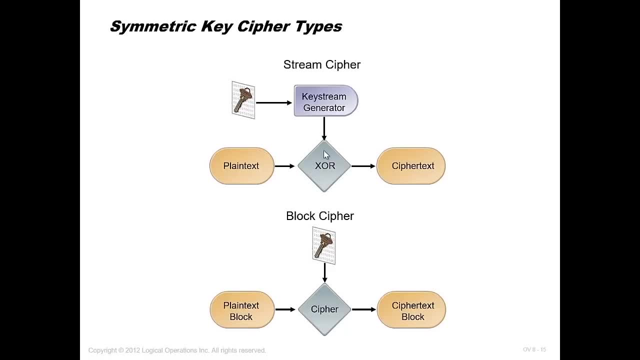 So they have different binary depending about zero and zero. You don't need to disturb about that, It's just a mathematic way. Just need to know what is difference between block cipher and stream cipher And what is the characteristics that you need to know about encryption protocol when we are talking about block side. 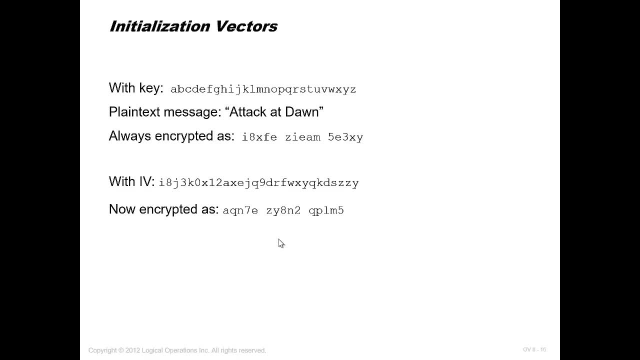 Now a very important concept here is called the initialization vector. What is an initialization vector? Here is the question. Assumes that now the definition, first initialization vector, It's one extra byte added to the key so it can put some randomization to the key. 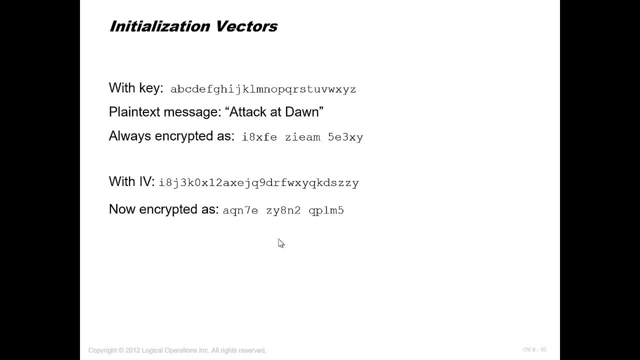 So let me give you an example. Assumes that Two people wrote the same word and it has been encrypted with the same encryption protocol, The result should be the same. right, Because the encryption protocol work is one specific way, So the result should be the same. 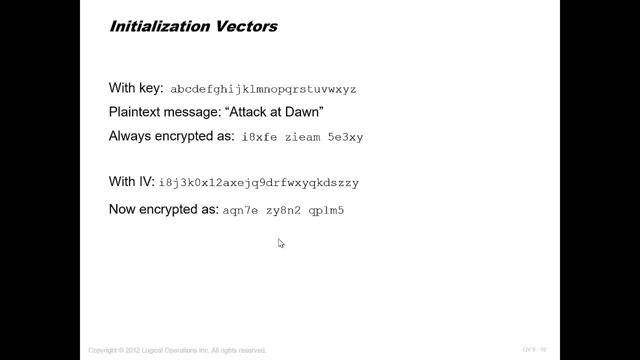 That's why in the, for instance in Windows, if you check the files that hold all the password is called the same file. If you check this file And this file is encrypted with LM hash, You will find that all users that has the same password has the same hash. 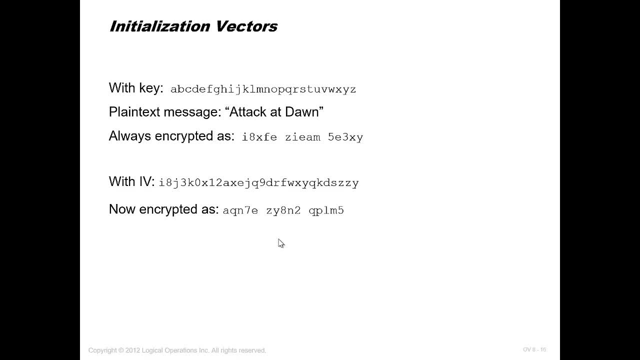 But When we add initialization vector, so we add in, each time we are using a protocol, one extra byte to the key, so it will get A different output. So by adding one extra key to the key, every one extra key to the protocol. 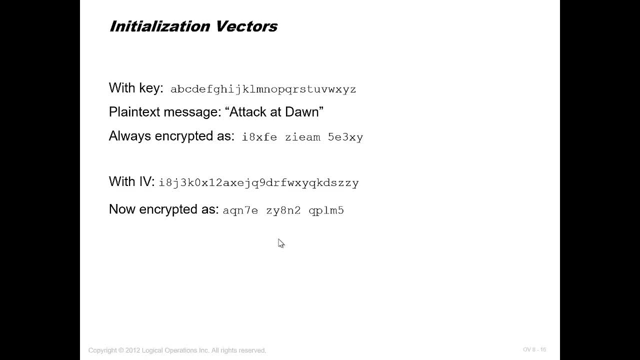 I'm sorry, one extra byte bit to the key. Every time it's used, same protocol are used, except every time you will have different output, Even if the text Text with the same. So IV. it's one extra bit added to the key. 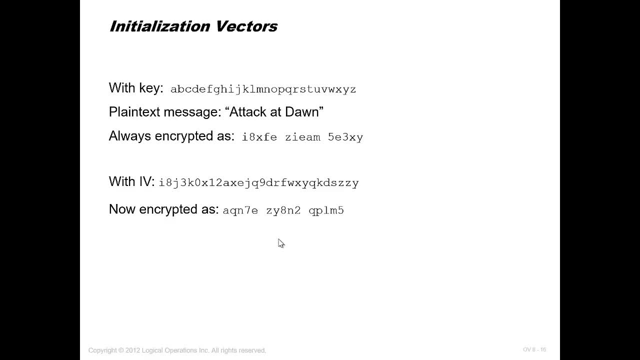 To put some randomization to the text. So two plain text. when you encrypt them with the same key, I'm sorry, with the same protocol, They will not get the same results. And this is implemented actually in Linux. in Linux We have something called sold. 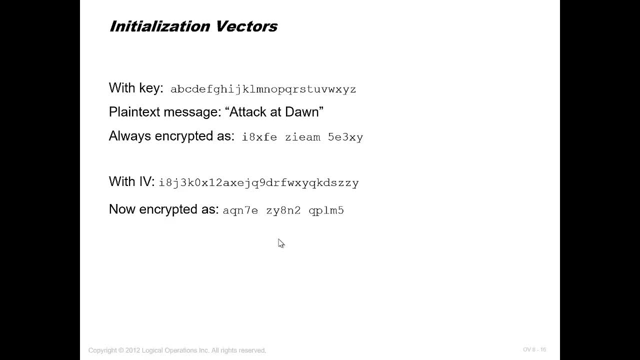 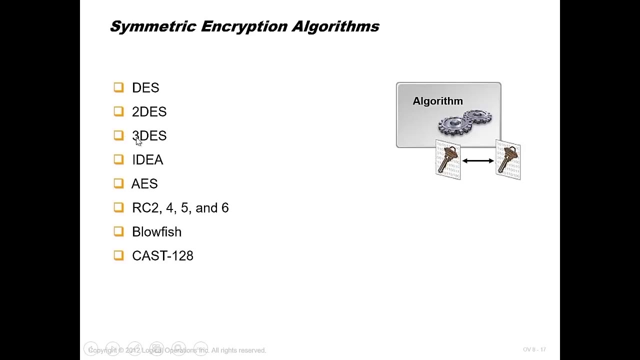 Salt, where it puts some randomization every time. So if two users Create an account with the same password because Linux are using sold, They will have a different hash. Those are some of the protocol, encryption protocol. This double this three. this ID is RC two, four, five and six blowfish. 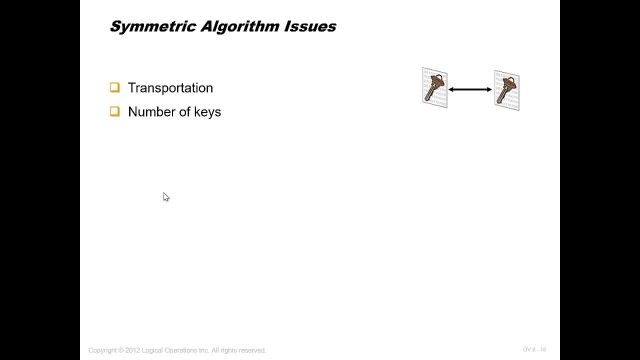 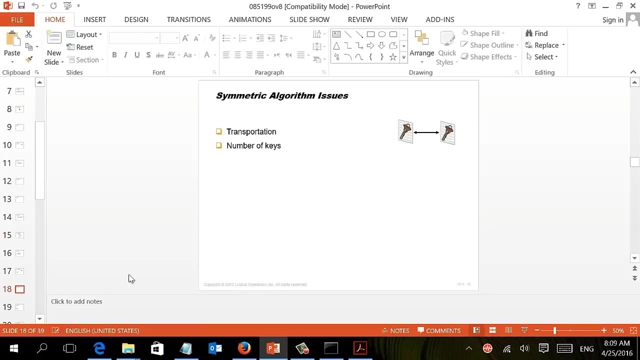 And what is the problem with symmetric? I told you about the transportation of the key, but actually this is not the main problem. The main problem is the number of key, and there is a formula that you're going to need to Memorize the symmetric encryption. 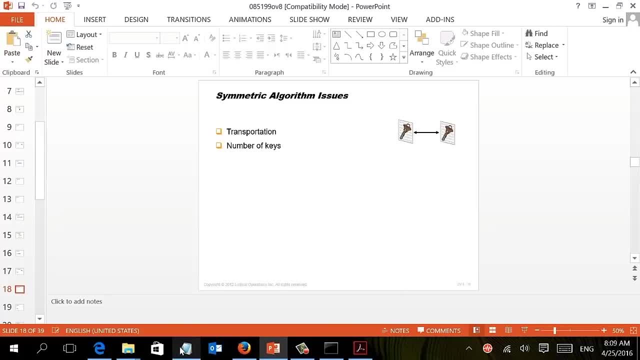 Has a huge amount of key. So, and it has a formula. Let me show it to you. So the formula is: It's an Multiply And minus one Divided by two, Where n is the number of user. So assume that you are an organization. 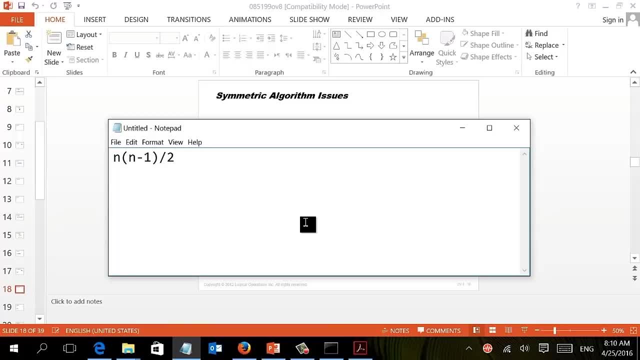 And you have, for instance, 10 user, How many key do you need? So it will be your place. and with 10. So it will be 10 multiply 9, divided by 2. It will be 45 key. assumes that you have 100 user going to find that you're going to need a huge amount of key and definitely key need to be managed. 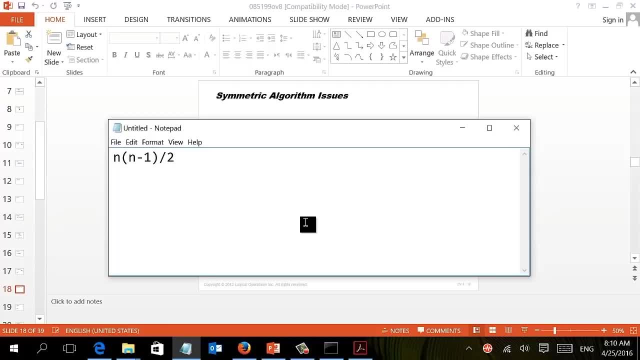 Key need to be transported, need to be issued, Need to be Disposed. There is a process in key management. So the main problem with the symmetric, we have two problem: We have the transportation and we have the number of key. But I believe the major problem is the number of key. 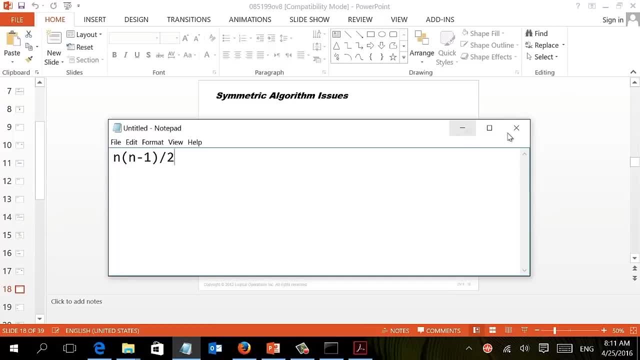 Now one more thing before we leave. the symmetric encryption: Yes, it's easy to use, But, as I told you, it has its own problem, which is this: This is a standard protocol used in US Government, But some flow has been found. 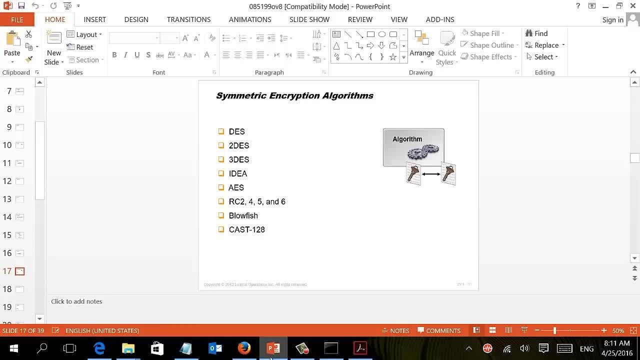 Those they created do this and three days. So you will find sometimes they give you some abbreviation for this that explain how it has been working. So, for instance, you may find in this they are giving you this format: E3. Mean That the text has been encrypted three times with three different key. 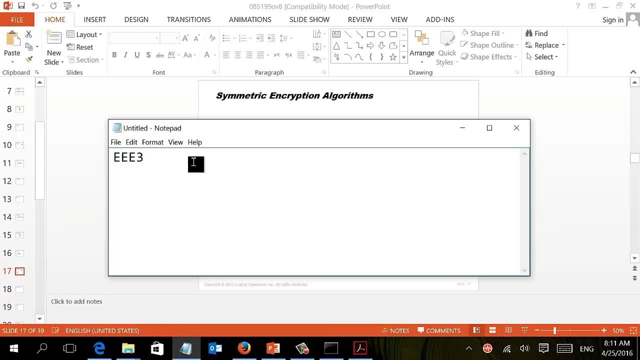 So they are taking the text encrypted one time with a key, Then encrypted another time with a key, Then encrypted with a another time with a third key. This is very so. it become very, very strong and very hard, Or it could be for instant. 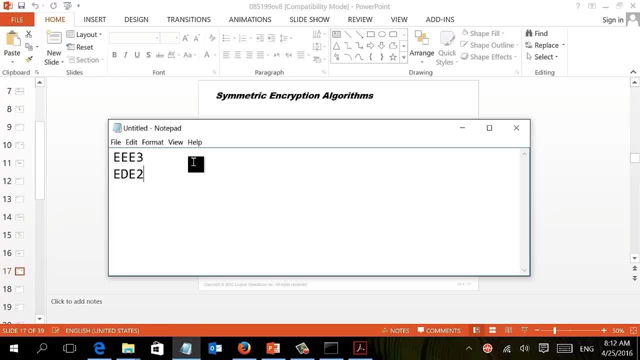 E, D, E2.. That's mean encrypted the crypt, encrypt using two key, So they encrypt using one key And then they decrypt the text using another key, So you can have a big mess. Then you encrypted one more time using 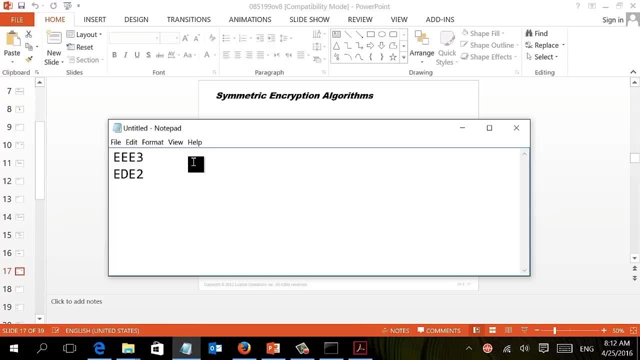 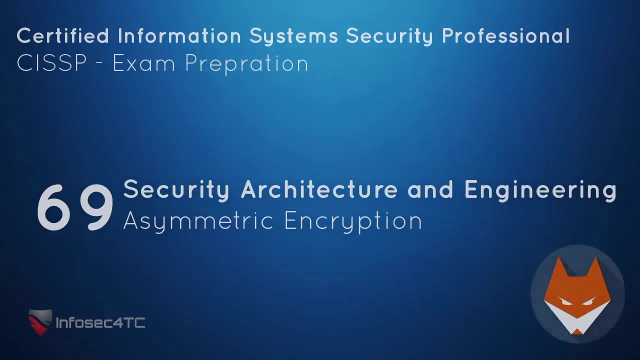 One another key, So it will be very, very hard to So. whenever you see this terminology related to the, Does you know it means how many encryption phase they done and using how many key. On the previous lecture, We explained the symmetric Cryptography. 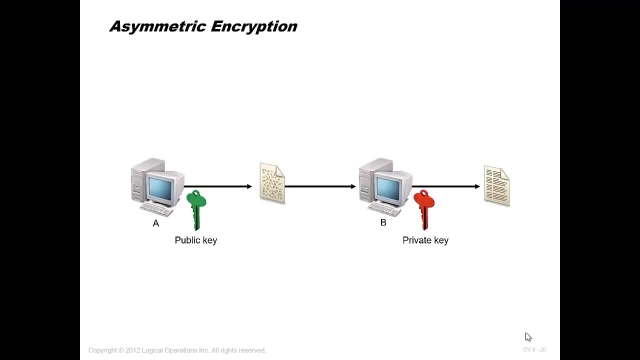 And what is the benefit of using it, which is the simplified Method of encryption- I mean, I'm using just one key is not complicated, But what is the disadvantage, which is the number of key- large number of key- And the transportation. Also explain what is the difference between a block cipher and a stream cipher. 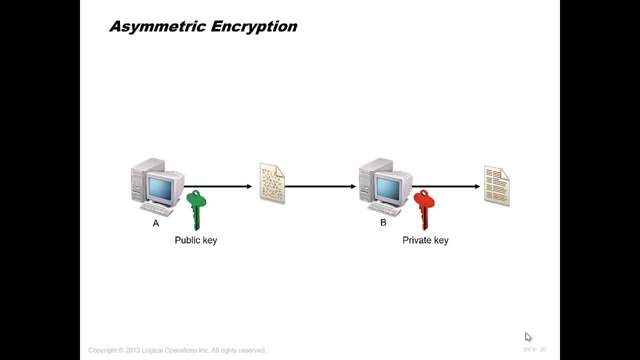 And I'm afraid you're going to need to memorize some of the abbreviation: What is AES stand for or this stand for what? But fortunately everything is written inside the sunflower in couple of pages. So the characteristic of protocol, which is their size and which protocol you need to memorize. 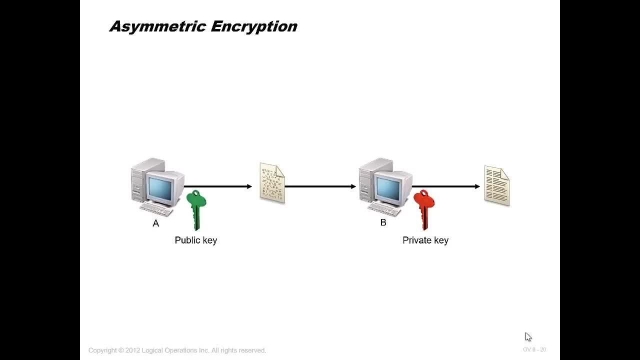 And those kind of information. you will find them in the symmetric in the sunflower document. Now let's talk about asymmetric encryption. asymmetric encryption- It's quite different than symmetric. In asymmetric, each user has two different key: Public key and private key. Each user has to keep public key and private key and they are mathematically related. 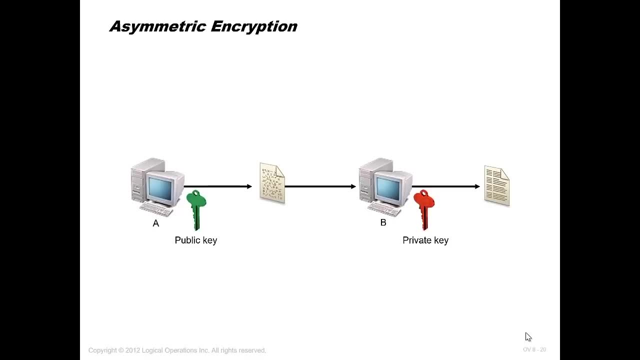 So whatever will be written in public key- I'm sorry- whatever will be encrypted with public key can only be decrypted with private key, And whatever will be encrypted with private key can only be decrypted with public key. So the key is just doing one function. 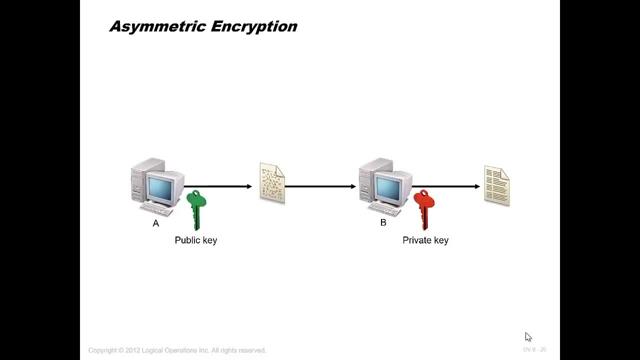 Encrypting or decrypting. Now here is how it go. assumes that we are working inside an organization that have 100 people, So each of those people, or each of those user, will have two key: One private key that is saved on his computer. 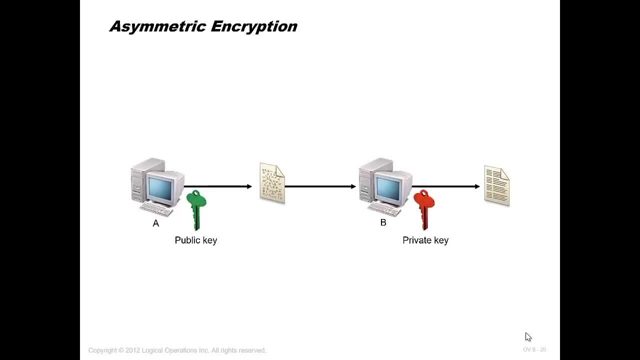 No one has access to it, And what public key that is hanging on the wall. I'm trying to simplify it. I mean, you know, this is everything is done behind the scene. I mean user will not notice anything, but this is how it go. 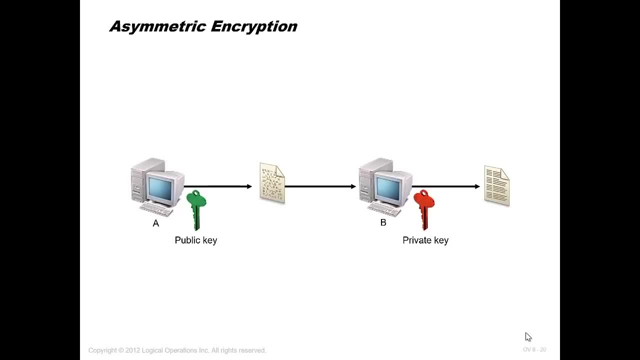 So I'm going to assume that each user has one key in his pocket- This is called the private key- and there is one hanging wall hang key for each user on the wall that is reachable to anyone. So what happened is: assumes that I need to send an email to Alice. 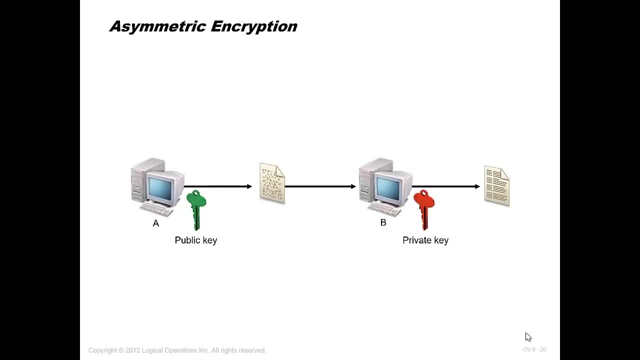 So what I'm going to do? I'm going to check for Alice public key That, as I told you, all public key are available for any user. So I'm going to check for Alice public key and I'm going to write the email. 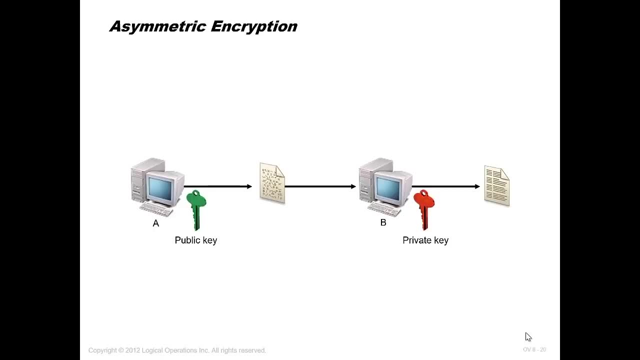 I'm going to encrypt that with Alice public key and I'm going to send her to. I'm going to send her the key. Sorry, I'm going to send her the message encrypted with her public key Now, now. now I'm comfortable that no one will be able to open this message except Alice using her private key, right. 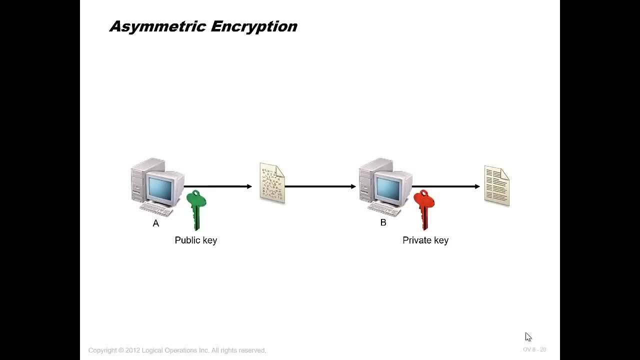 If Alice need to send me a encrypted message, she going to check for my public key that is available for anyone. write the message encrypted with my public key. And now she's. she knows that no one can encrypt this, decrypt this message, except myself, using my private keys that I have inside my pocket. 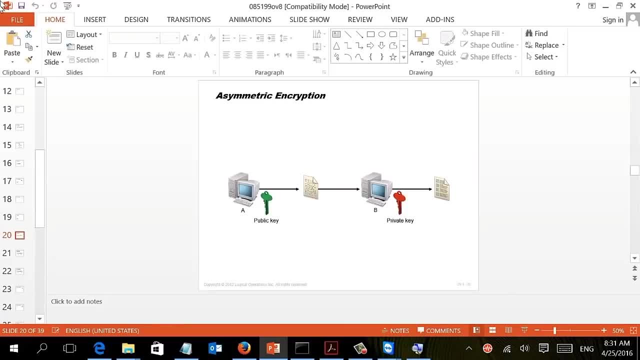 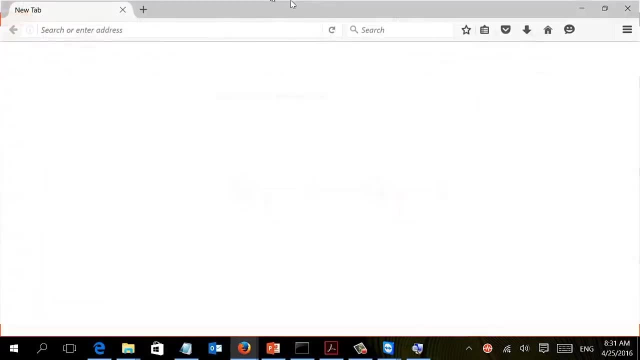 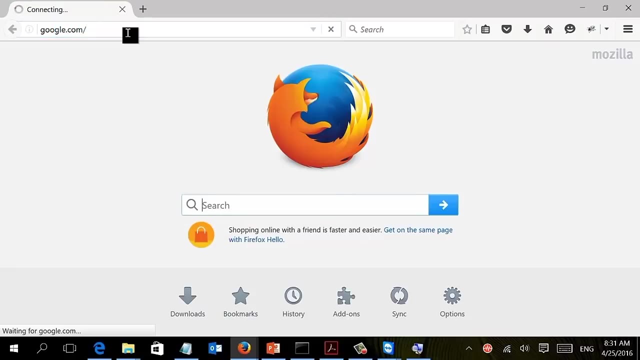 A good example of that will be the website, the digital certificate, Because when a website by a digital certificate, So you know some of the website has those HTTPS. So if you go for Google, for instance, let's go to Google. 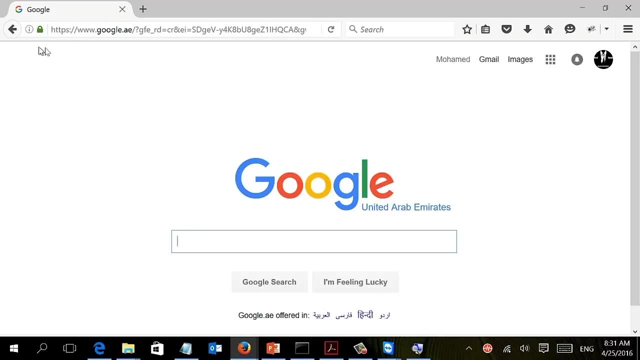 As you can see, Google it's HTTPS means this site has a digital certificate. What is a digital certificate? A digital certificate That any website can buy has two function. first function: It guarantee this site. If you have a website and you need to do some e-business on this website, you can try to buy a digital certificate from one of the major certificate authority like Verges sign or Google or GoDaddy. 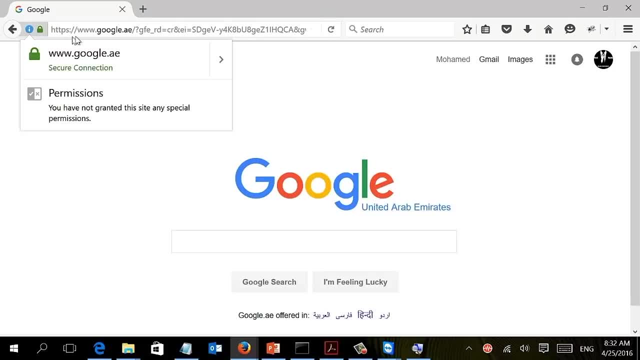 And they will not just give you the certificate and your site will be HTTPS right away. They're going to verify your existence, They're going to ask you for an ID and they're going to ask you for a credit card. So they make sure that you. 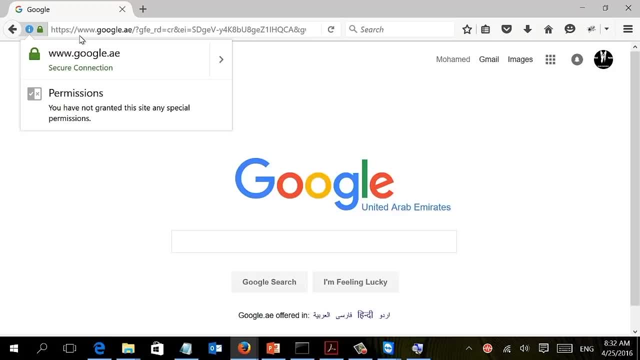 Are a real business. So the first benefit of certificate is that you guarantee this website. Someone is guaranteed this website for you. The second website is the second benefit of that. Let's open certificate. The second benefit of the certificate is so we can go, and we can go to more information. 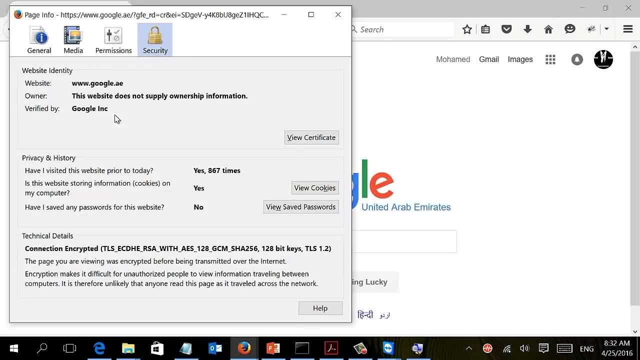 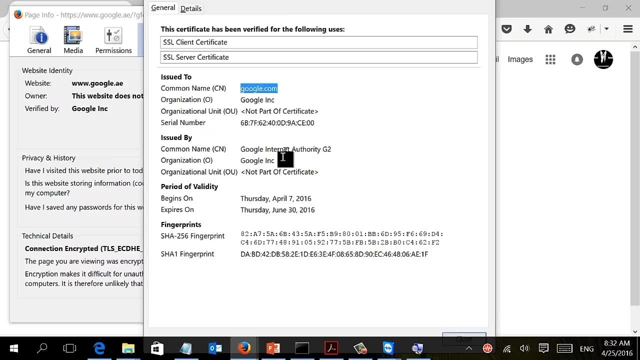 Whenever you buy a certificate, you got two different key. any website that has a certificate, He will buy two different key: a private key and a public key. The private key Let me see. I think It should buy. This will be kept on Google website. 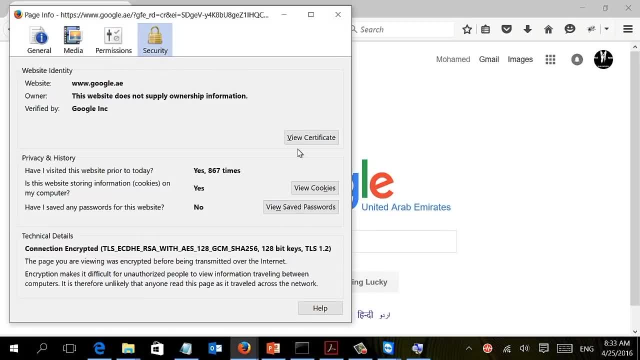 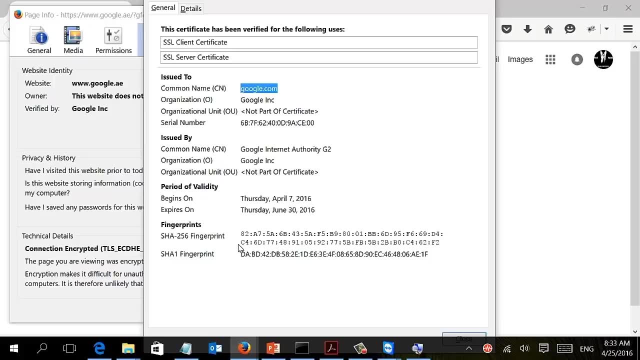 Let me see security You certificate. I think should be this Key, I believe, or one of those key, But anyway. So what happened is when you buy a certificate, you will get our Google. when they bought the certificate, They will get two different key: a private key and a public key. 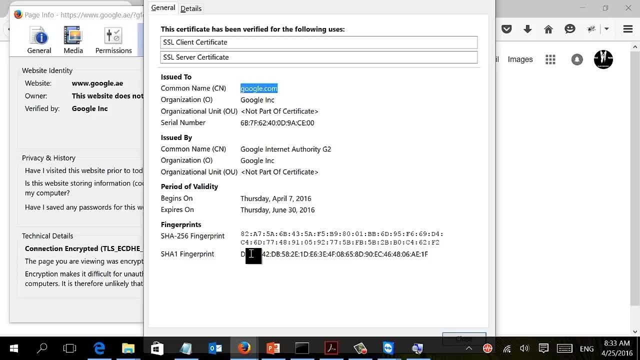 So when you open their website, they will send you to your computer a public key, their public key. So whatever you are writing, it will be encrypted with Google public key, and whatever is encrypted with Google public key can only be the crypt With Google private key that they have on their web servers. 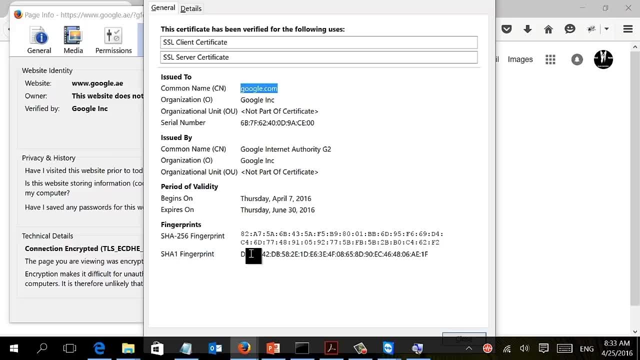 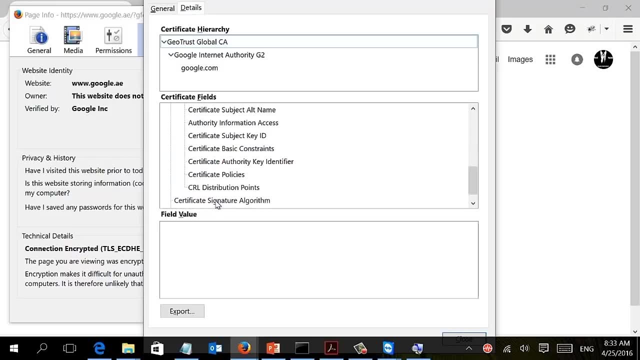 So this is one of implementation of the. I'm sorry, the publication should be here. I didn't saw that inside details and let's go down public key. It should be down here. Yeah, here you go, Here you go, Here you go. 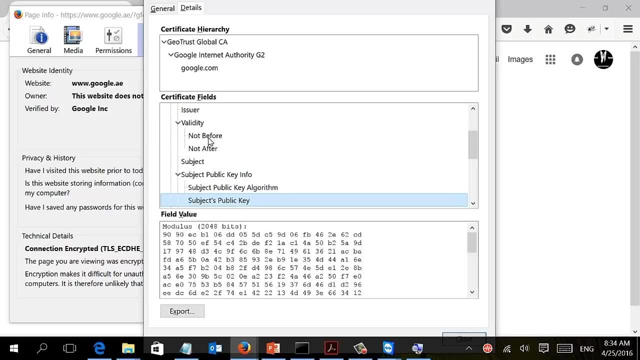 This is the public key for Google, and Whatever has been encrypted with public cannot be decrypted with public, has to be decrypted with a Google private key. So this is a very important implementation for the asymmetric encryption. So the first thing is The digital signature. 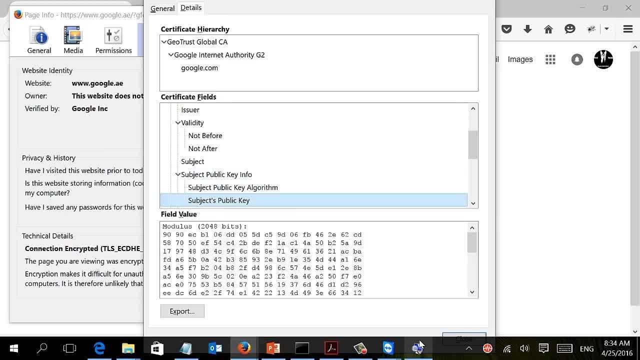 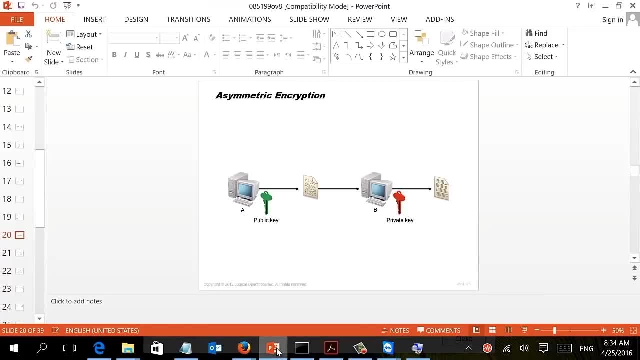 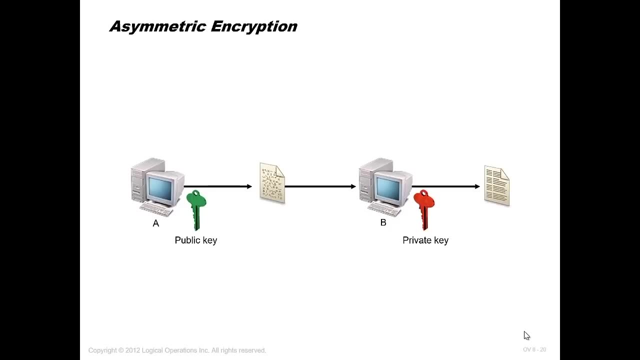 I'm sorry, digital. one of the implementation is the digital certificate. Now This can also be implemented inside organization where each user, so you can have inside your company something called the certificate of security. This is one of the role inside the domain controller: Microsoft Windows domain controller. 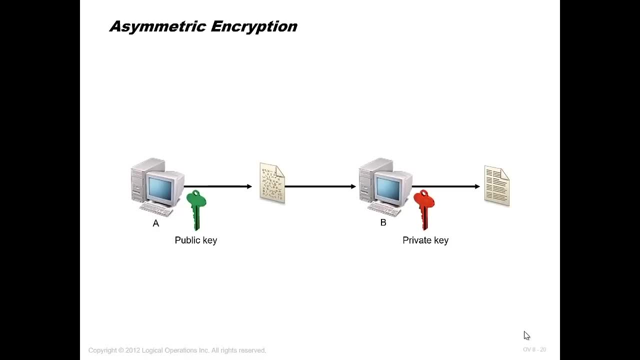 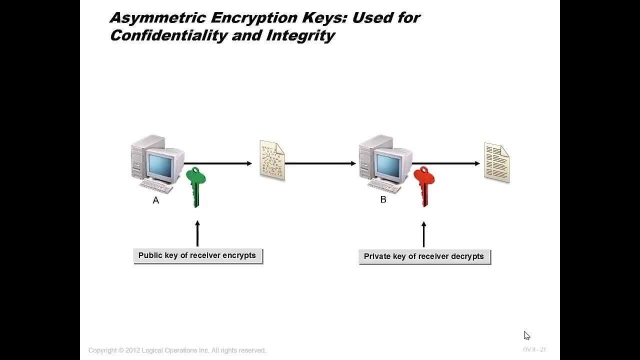 So you can implement that inside The network, where each user will have a public key and a private key. Now, This is private and public key, as we explain, and the mythology of using that. There is another way for using the asymmetric, So we saw how to use symmetric for. 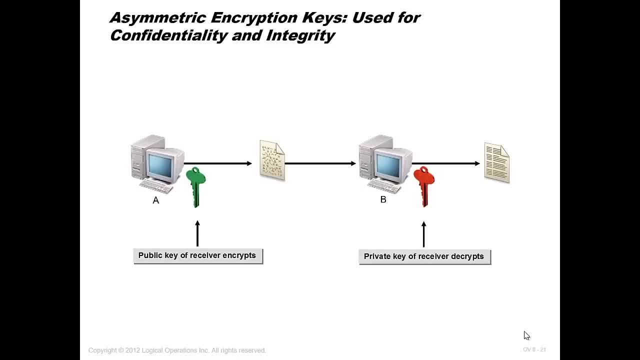 So we saw how to use symmetric for confidentiality, Okay, And integrity. But we can use asymmetric in a different way, which is: Assume that me and you, we are on a symmetric encryption environment. We have an asymmetric, So each one of us has a private key and a public key. private key are kept private in my pocket, while public key are available to anyone. 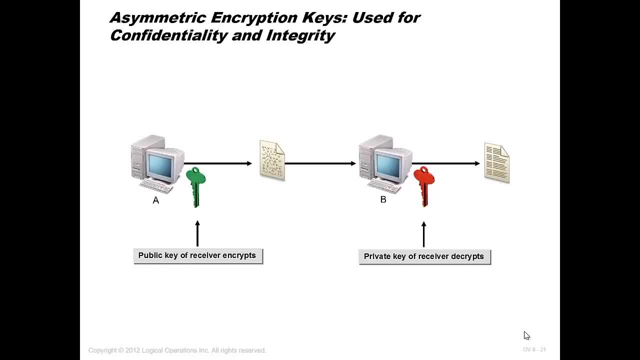 In the previous example we explained that I want to send you an email- and confidential email. I'm going to look for your public keys. that is available for anyone. I'm going to encrypt the text and send it to you. I can use that in an opposite way, so I can do the following. 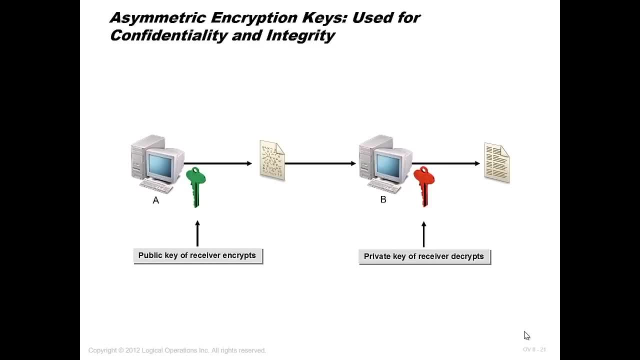 I'm going to write an email and encrypted with my private key. Now, if I encrypt that with my private key, it mean it can be decrypted with my Public key, right, But the public key is available to anyone. So what I? what did I provide by doing that? 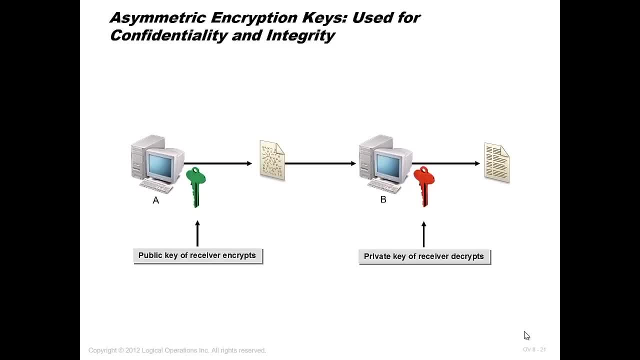 When we do that, We are providing something called non-repudiation. I mean, if I do this, this specific scenario, that I encrypt my message using my private key So anyone can open it using my public keys. that is available for anyone. I cannot deny that I send this email. 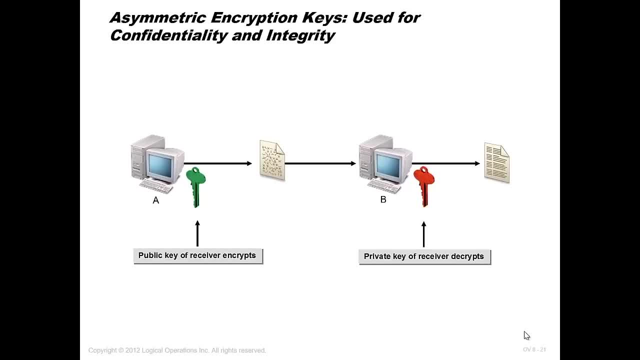 Okay, this is called the non-repudiation. So it's not for confidentiality, It just for confirming the identity And this is the Idea of digital signature, so I can send an email encrypted with my private key. If you are able to decrypt it using your public key, using my public key, that is available for everyone. 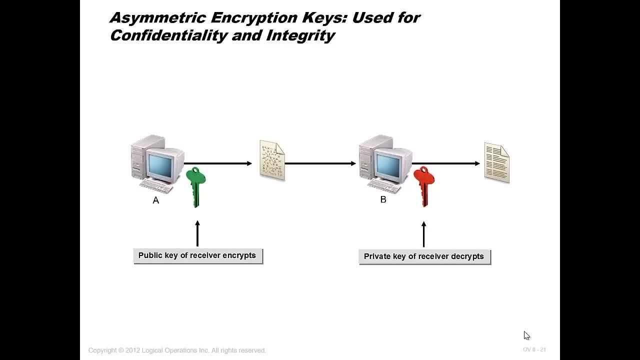 So definitely this mail come from myself so I cannot deny that I send it. This is called non-repudiation and this is the idea of Digital signature. in digital signature, What you are doing, that you are sending an email and you do not encrypt the email. 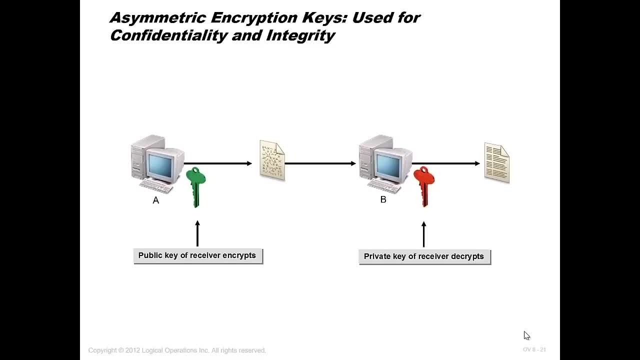 The full email, but you put an attachment that is encrypted using your private key And if the other side opens this email and he was able to decrypt the attachment using your public key, This means this mail came from this person. It's not a fake email. 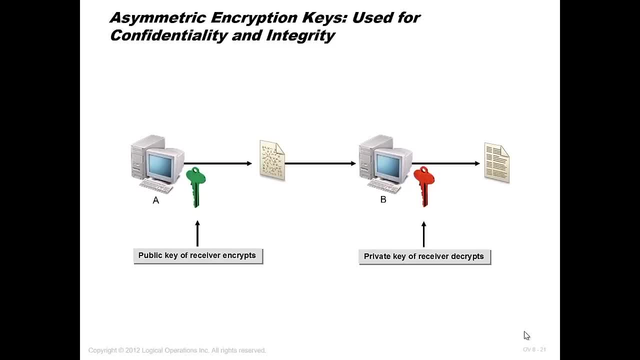 We usually see that in emails that you receive and below the email you find this disclaimer that if you cannot read, if you can read this text, This is came from this specific person. So this is The digital certificate as a digital signature idea. So some of the questions as exam, for instance, he will tell you and this was actually really question. 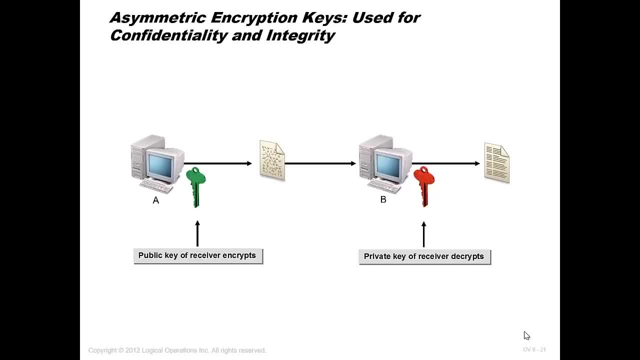 He asks the candidate the questions as exam. there is Bob and Alice. if Bob need to send Alice an email with a digital signature, What exactly he need? Bob, private key, Bob, public key. Alice, private key, Alice, public key. And there was like four question continuously related to the same scenario: Alice to be able to open the mail. 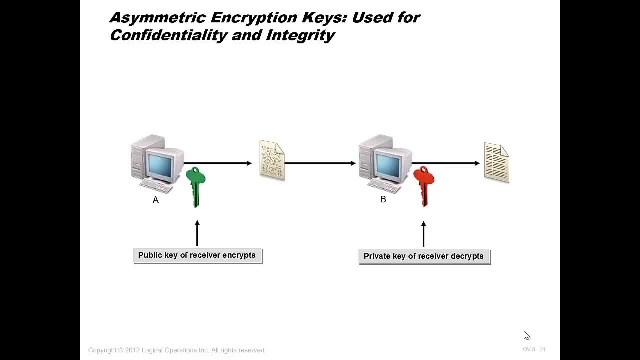 What exactly she need: Bob private key, Bob public key, Alice private key, and so on. So it's very important to understand digital certificate and digital signature And also to understand what is non-repudiation that can be implemented using asymmetric encryption. So a new terminology has been introduced here. 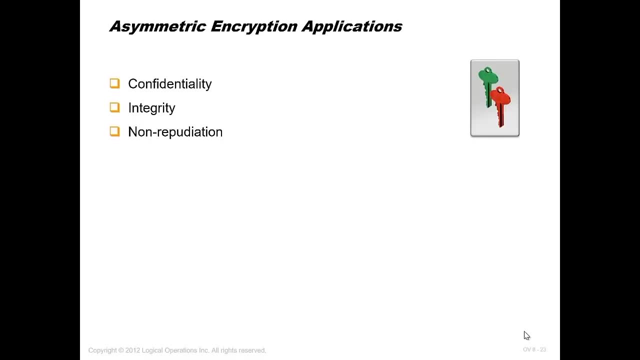 So asymmetric do not just provide Confidentiality and integrity, but also it provide a non-repudiation. Those are some of the protocol that is used in asymmetric RSA Aljamal. there is ECC. Now you need to know this specific protocol that has specific characteristic. 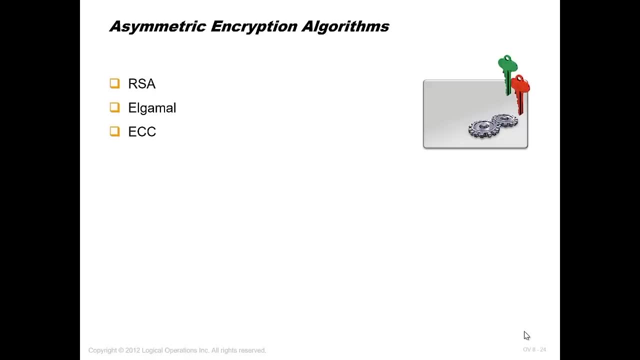 For instance, ECC: It's a protocol, because the problem with asymmetric is taking a lot of processing. So ECC, it's an asymmetric protocol designed for small devices Like smartphone and tablet, because they don't have the same processing power like computer and mainframe and so on. 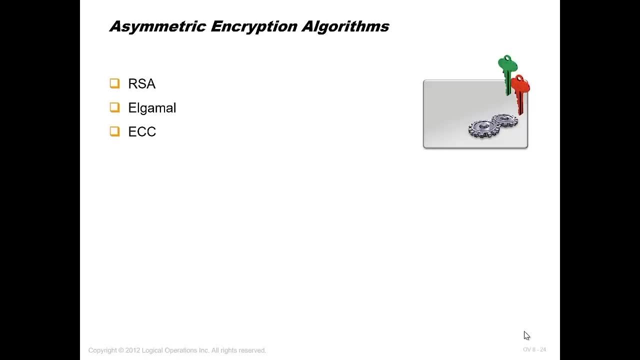 So this is an asymmetric protocol for specific device Like smartphone or tablet and so on. So this kind of notes you need to be aware of. you get the questions as exam which asymmetric protocol can be used for small devices or smartphone or something like that. 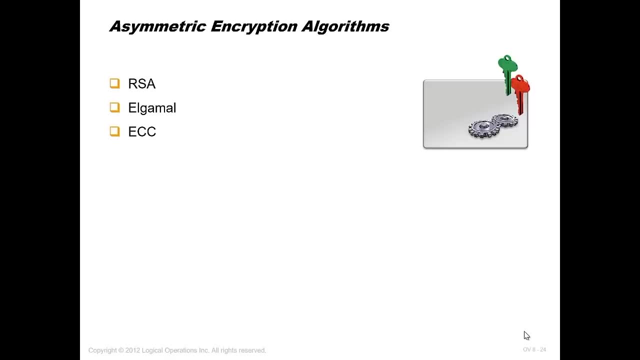 And they will give you some protocol. Okay, we'll go through that one more time when we will be reviewing the module and the important point, But I just want to point to that what protocol is used for credit card machines? You know those credit cards that you are using, that you are sweeping your card in. they are using their own protocols, called set. 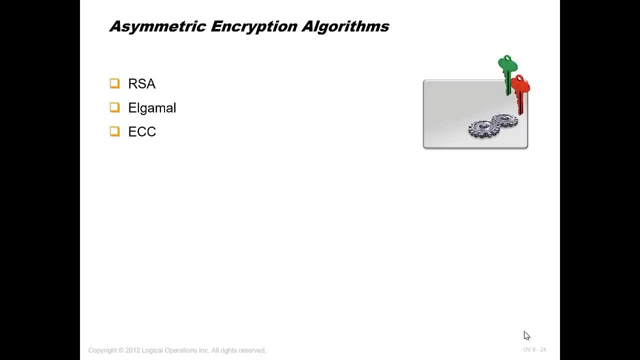 This is written in sunflower, So those notes are important. So not just to know the major one, but the things, that is, you know, different. So we spoke about the digital Certificate idea and how it look like and how it work. 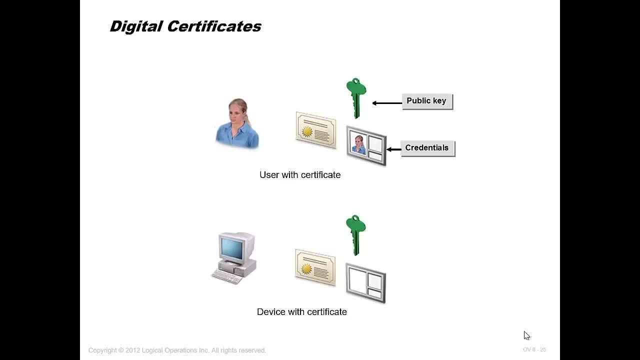 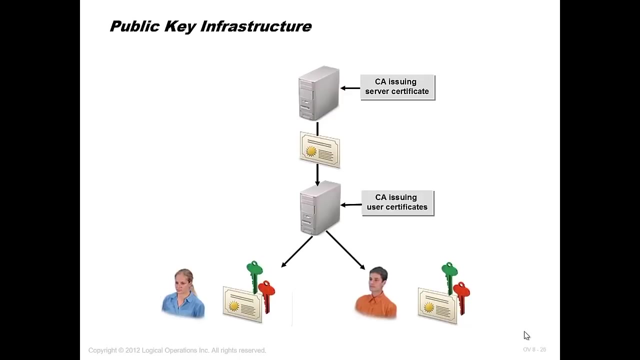 And we saw an example and you should know the digital certificate has different level. There is level 1, 0, 1, 2, 3.. Some of the level will request the personal meeting. So this is also will be mentioned in the sunflower document: public key infrastructure where you can have a certificate of security to a certificate and each user. 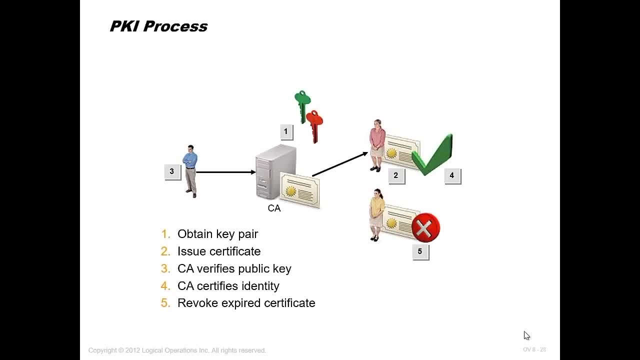 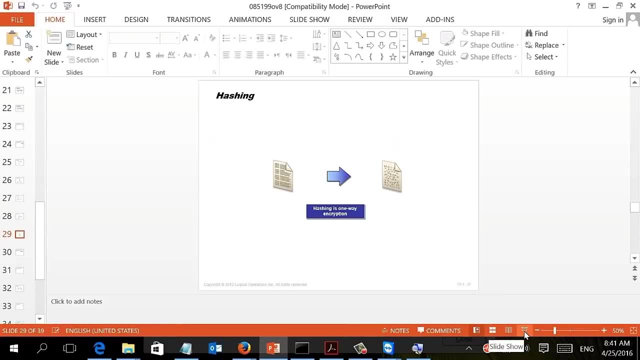 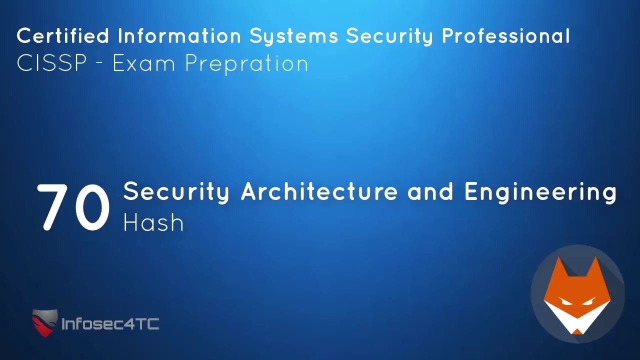 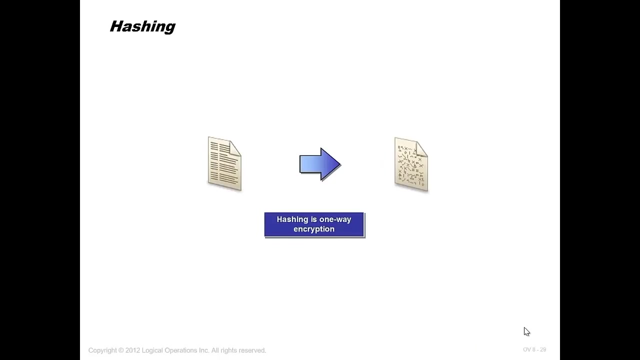 Also, we spoke about this implementation, PKI- same implementation. On the next lecture, We'll be talking about an important topic, which is hashing, which is using the encryption into the integrity, not the confidentiality. This lecture will be talking about using cryptography into Integrity. 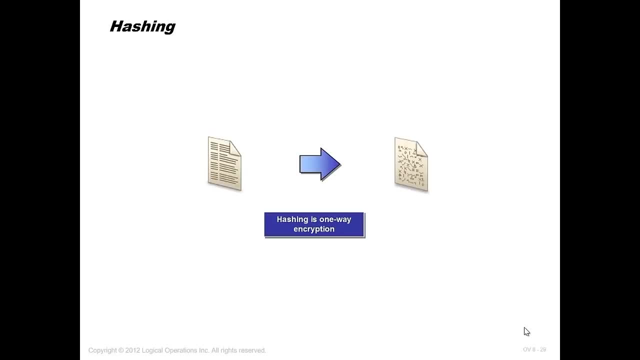 How can we use Cryptography for verifying the integrity of the file? Some of the protocol are used for what we call the hashing, and hashing will run a protocol or an algorithm on the file and it will get you a value And if any modification happened to this file, the value will be changed. 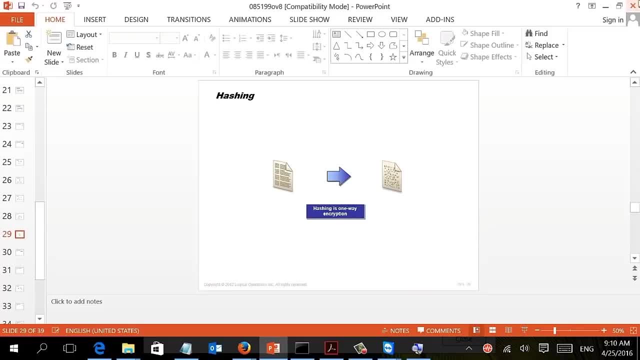 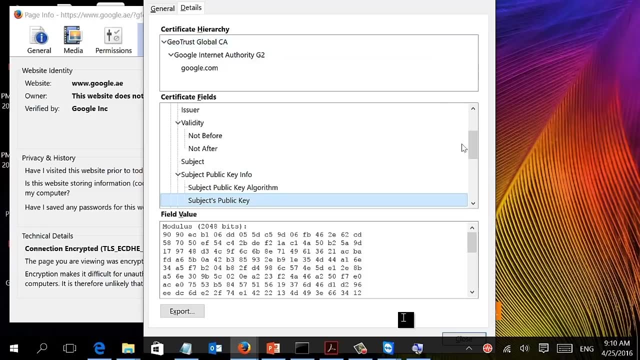 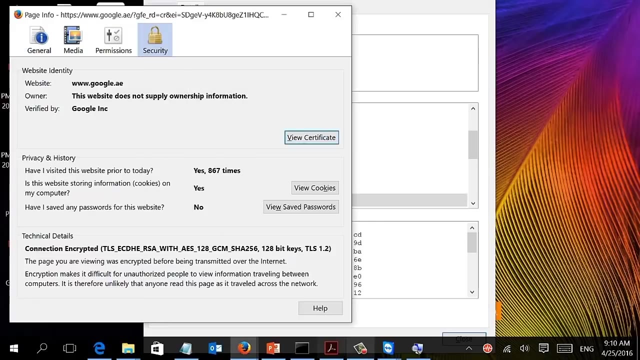 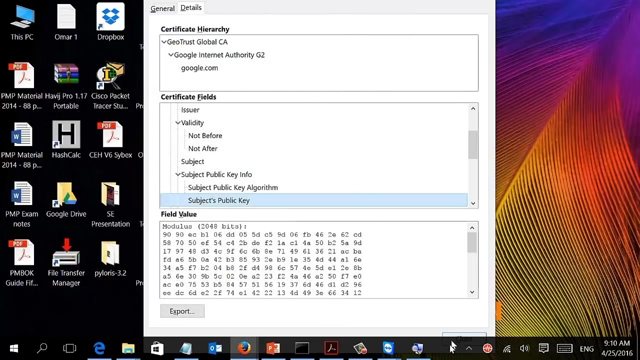 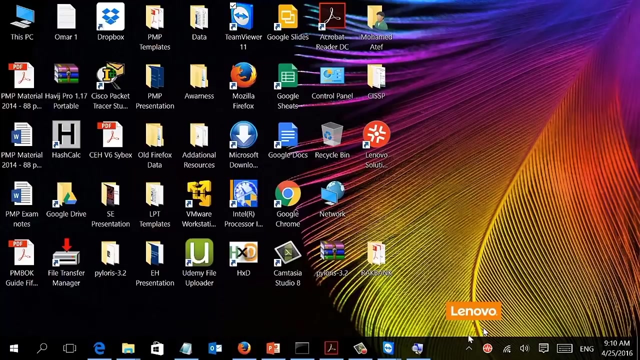 So let's see an example of hashing protocol and how it's used to confirm Integrity. So what are we going to do right now? We'll be opening the file. Let me close everything. Okay, so You need to have a hash calculator to be able to test or to do this demonstration, and you can find a lot of hash calculator for free. 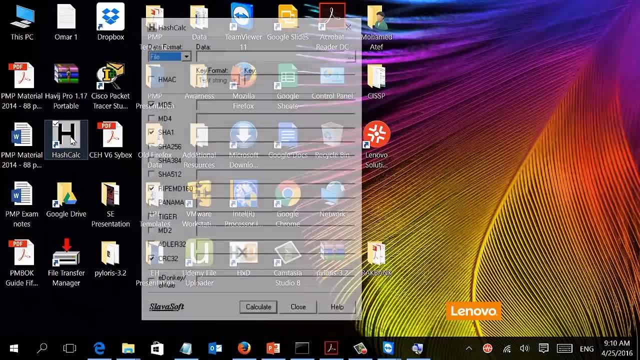 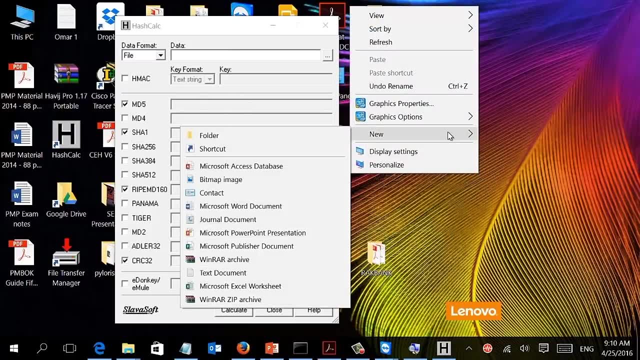 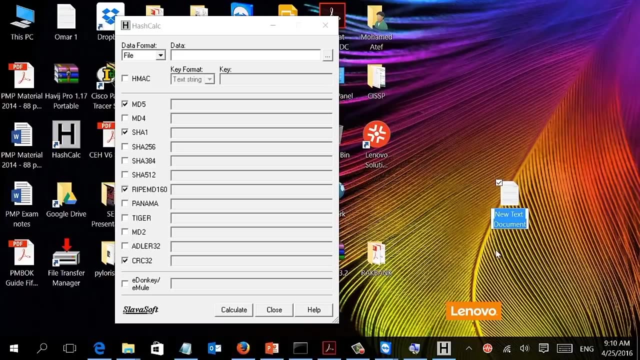 Just search online. This is a good one, hash calc, and let me show you how it works. So you open this program and let's create a file. So I'm going to create a file, text file, and I will name it for instant secret. 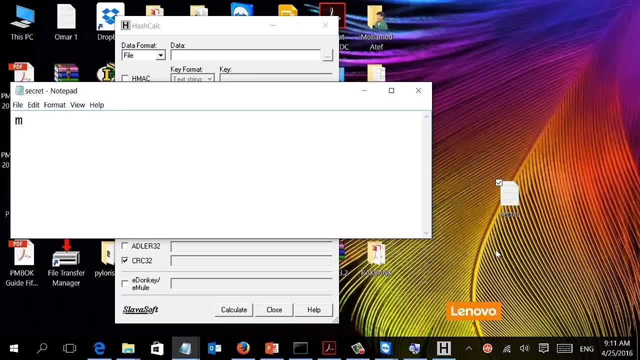 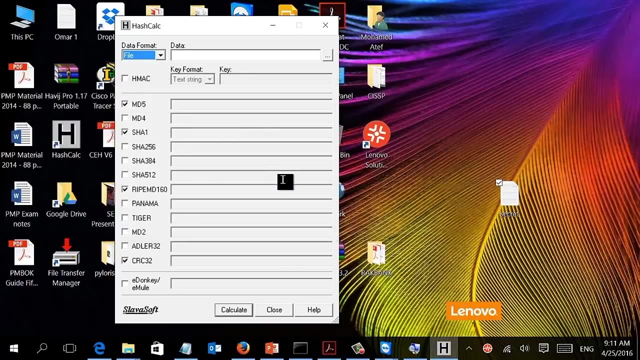 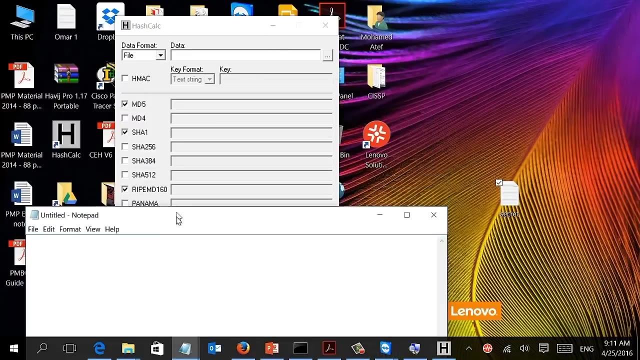 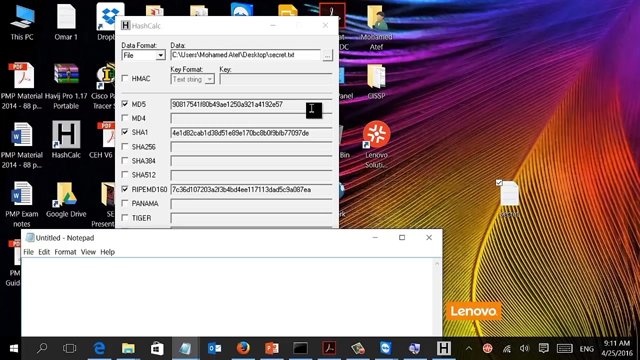 And let me put something inside, Good morning, Okay, And let me save it, See, And I'm going to open another file just to see the value and compare between them. So here is the situation: If I tweak, if I take this file and put it in the hash calculator, it will generate a value. 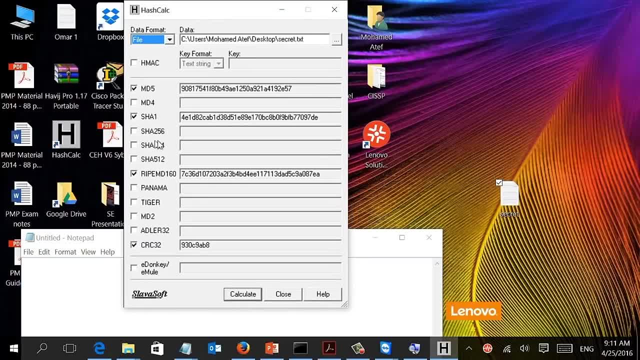 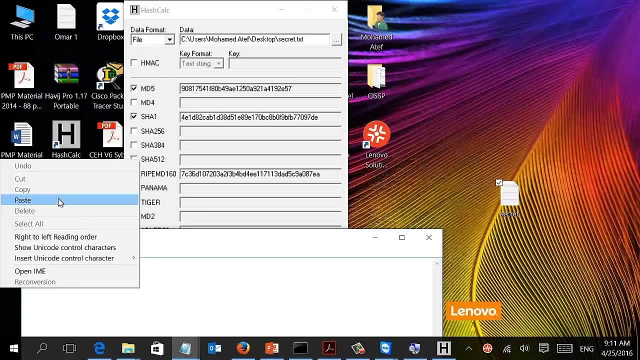 So those are some protocol like MD5. Shah. Those can be used for regular encryption and for hashing as well. So let's see this value. So this is a value that has been generated from the file. Okay, so I'm going to put it here, based. 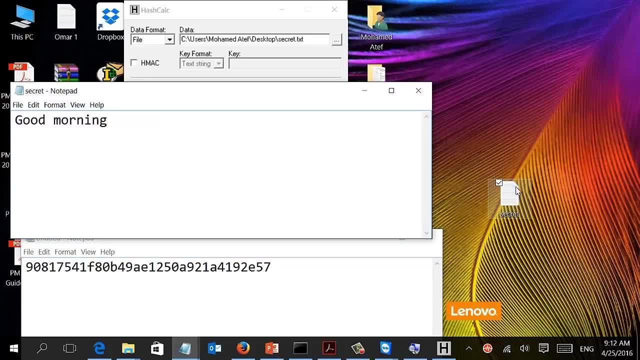 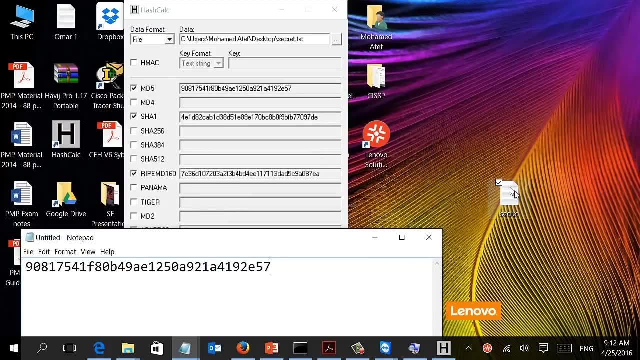 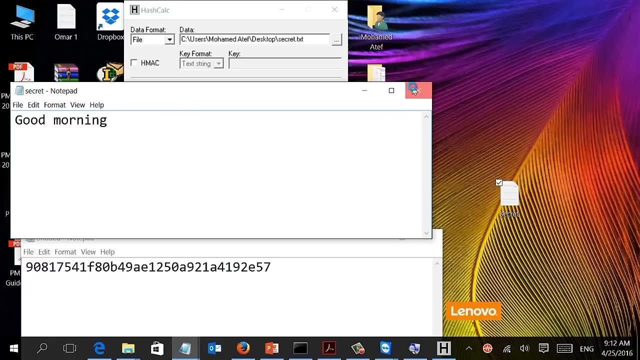 And you notice that the content of the file has not been encrypted. but he runs this protocol over the file and he got as a result, a value Now if any modification happened to this file. So, for instance, I add one space And I save that and I'll take it one more time. 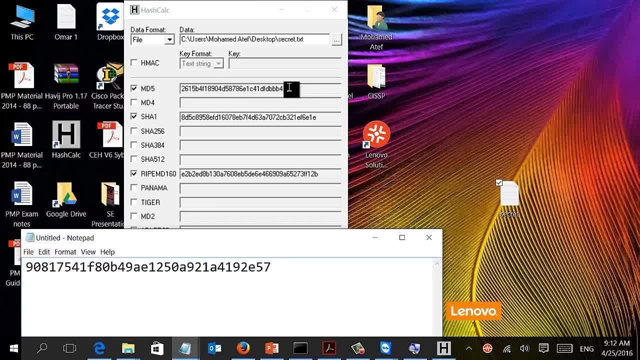 Let's see what will happen. Okay, you can see that the full hash has been changed. So if we check this one, this one, So any modification happened to the file. even if you add one space or you add one letter, the full hash will be changed. 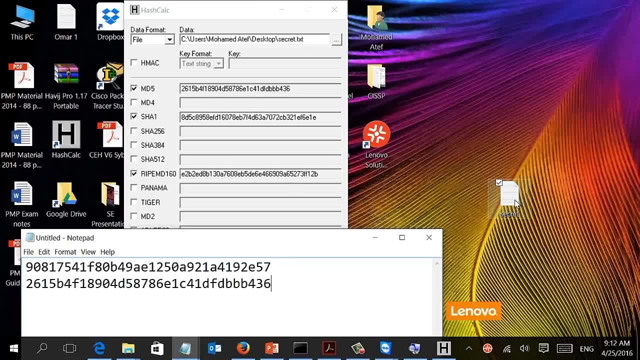 But this is has or it has nothing to do with the file contents. file content has not been changed, But it just showing if the file has been modified or not. So this is a way for confirming the integrity of the file. That's why I can send someone a file and I can send with him the hash of this file. 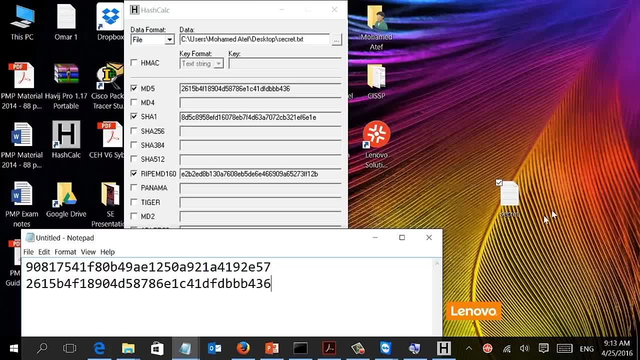 So if you got a file, he will run this hash calculator, And if you got the same values, that means that the file has not been changed. Now, an important point here is that number one. This has nothing to do with the file name. 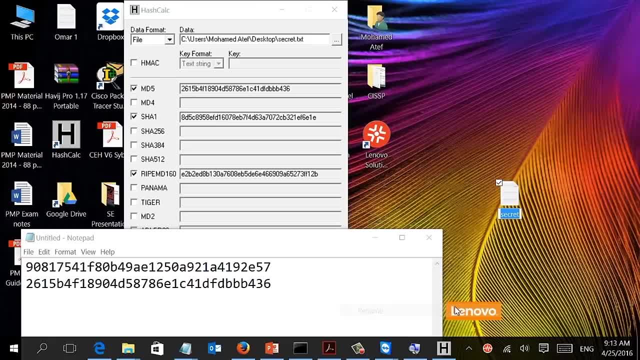 I mean, if I change the name To any other name, Do you think that the hash will be changed? No, because the content is still the same. So if I take this file here, you'll notice that it has the same hash. 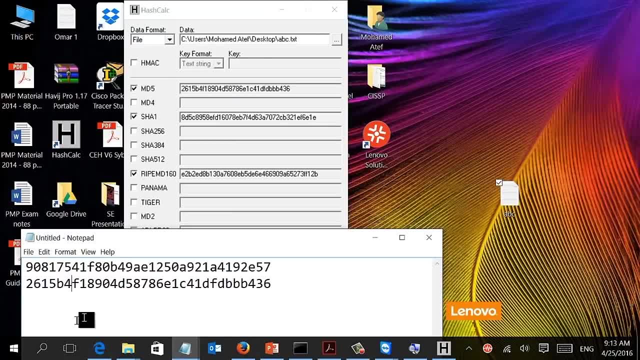 It has not been changed, So it's not related to the file name, It's related to the content of the file. Okay, number two, That this is a one-way process. I mean you got the file and you run the hash protocol. 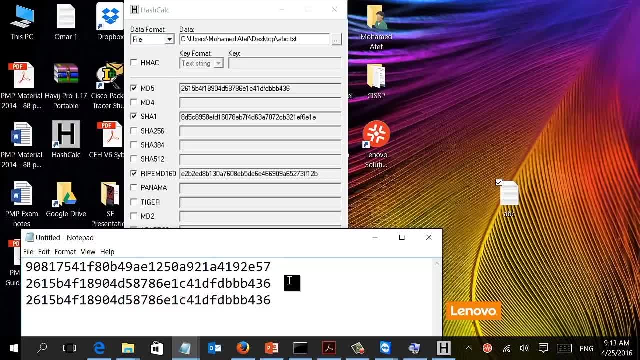 You get the value. any modification happens, The value will change. but you cannot do that in a different way, in opposite way. I mean I cannot have the hash and from the hash get the file. So hashing protocol It's a one-way process, while encryption protocol 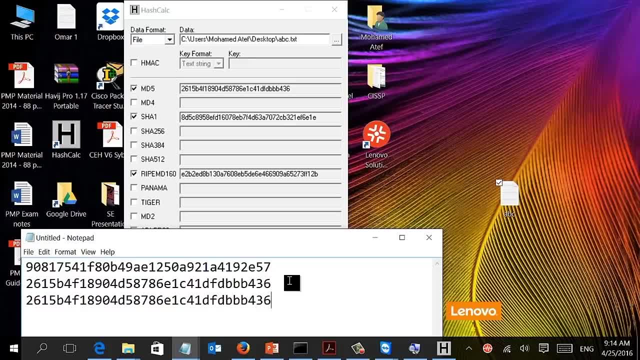 It's a two-way process. encryption: I can have the cipher and get back the text, or I can have the text and get the cipher. Now the hash is one-way process. Beside those protocol are hashing protocol, but they are also encryption protocol. 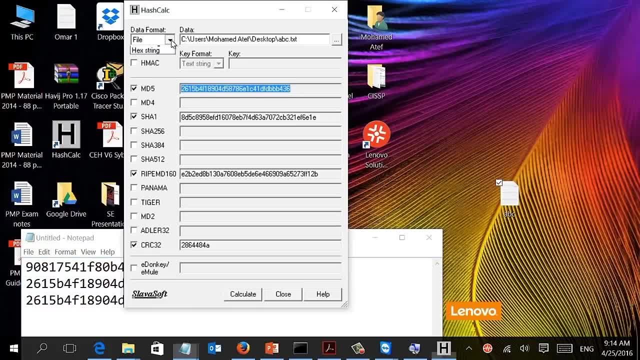 So I can ask him here. For instance, I need to change, I need to encrypt the text and I can write any text and he will encrypt it with md5.. Okay, so I can ask him to encrypt. So md5 or sha can be used for regular encryption or for hashing protocol for checking the integrity of the file. 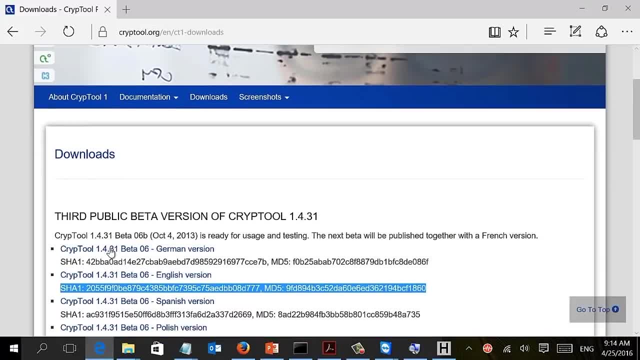 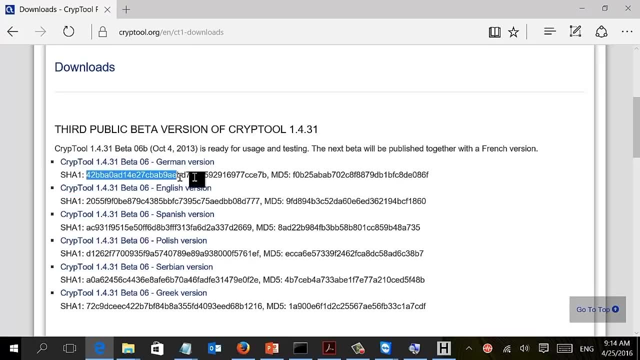 That's why, at the beginning of this domain, when we went and download the crypt tool, you notice that under each download link There is the hash Of this link and the reason they do that- especially professional websites- that when you download this program to make sure that it has not been modified or any malicious code has been added to this program. 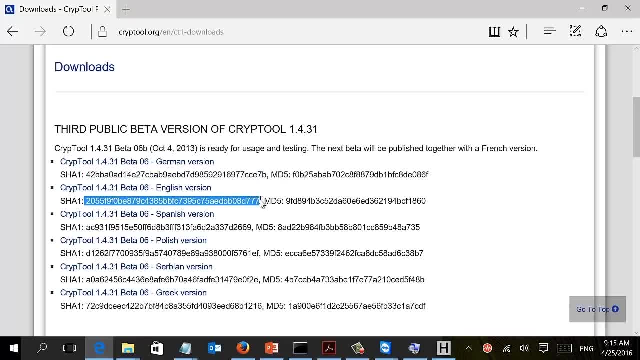 You can run the hash calculator and verify the hash with the one Mentioned on the website. If they are the same, It means that the site is a file has not been modified. So this is how to use the hash for integrity. So now encryption or cryptography can be used for confidentiality, which we explain, and integrity by using a hash protocol. 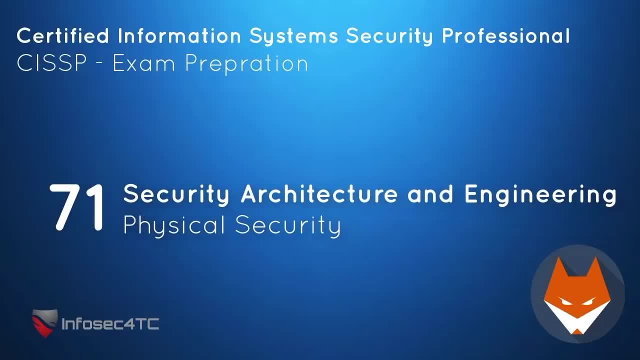 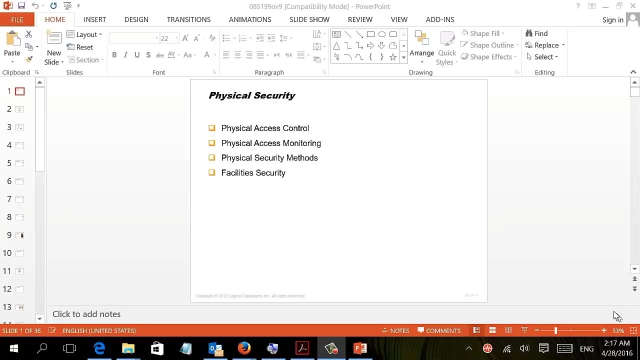 In this domain we will be talking about physical security and for many people this topic- Actually it's a new topic because most of us came from a technical background. So when we start talking about the type of fire and type of fences and type of luck, it's not really a very common subject for technical people- 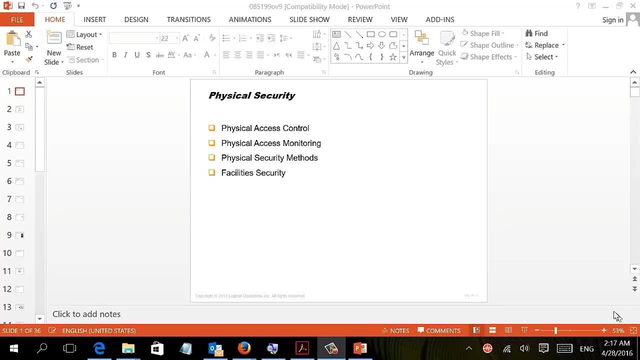 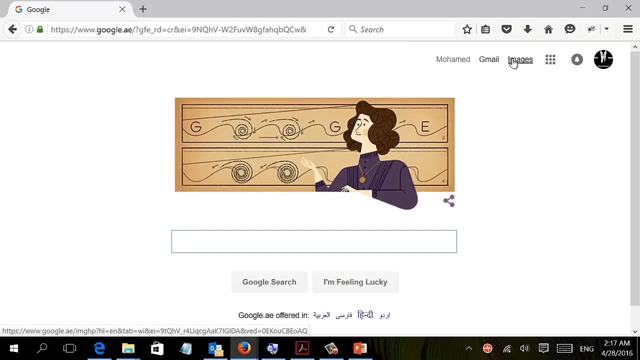 Now the problem or the challenge in this module is that you will be reading about say things that maybe you didn't see before. That's why I strongly suggest two things. Number one, to open Google image while you are reading inside this module, and whatever terminology are not aware of, just check. 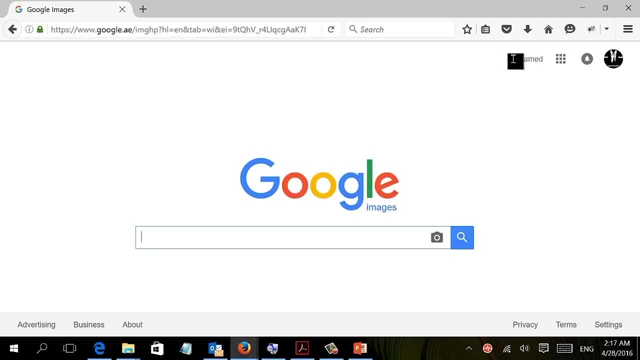 So when he's talking about a specific firefighting tool, maybe you didn't see that before, So search for the image. You'll be able to memorize that second point which is in this specific module. If you go through the book it will be kind of exhausting. 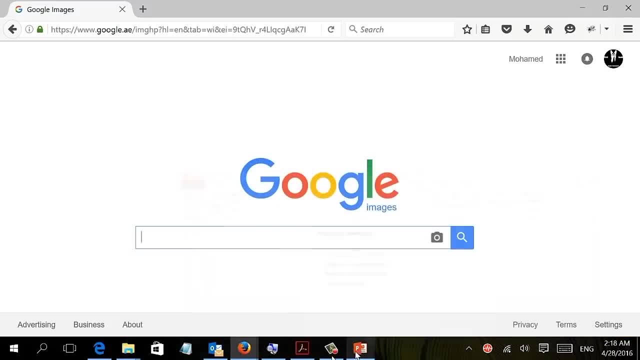 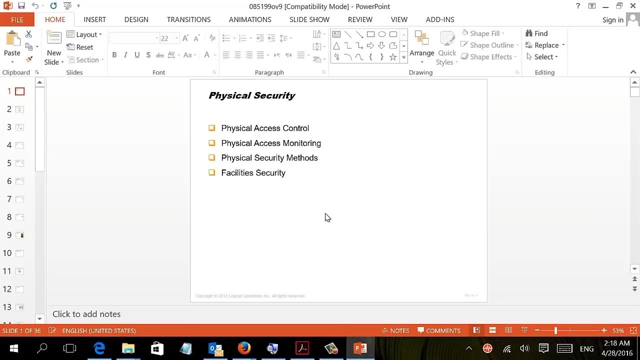 So it's much more better to go through sunflower, as we're going to do during this course. Now, there is three different topics that I want you to focus on when it comes to the exam in physical security. Number one is the power, the different power problem, because actually we always in real life 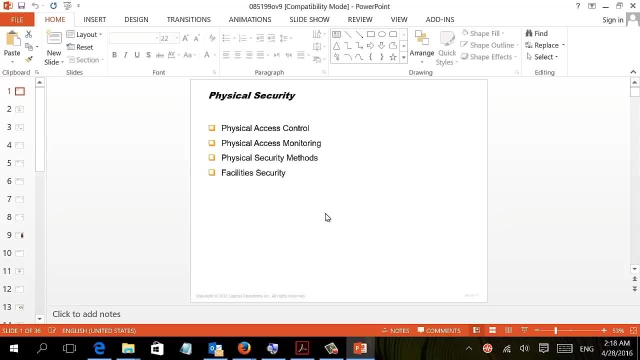 Focus about one power problem, which is the blackout or the power getting cut, But there is five other problems that you're going to need to know their name And what exactly do they mean. So number one is the power: Definitely, definitely get a question about that inside the exam, asking you: what is a surge? 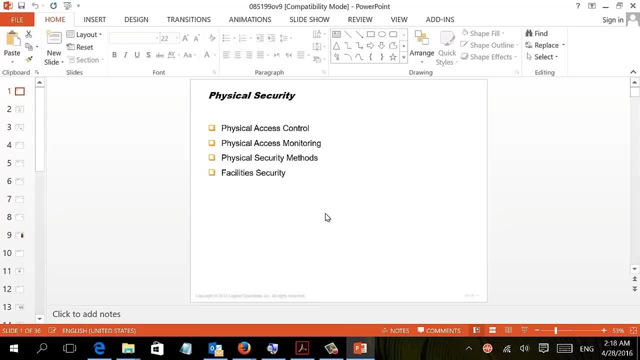 What is a spark? Those are all power problem. Second point is Fire. fire is extremely important topic and there is some memorization in fire. Like you need to know the fire table: What is class A or B or C or K? Because each class has some firefighting tools. 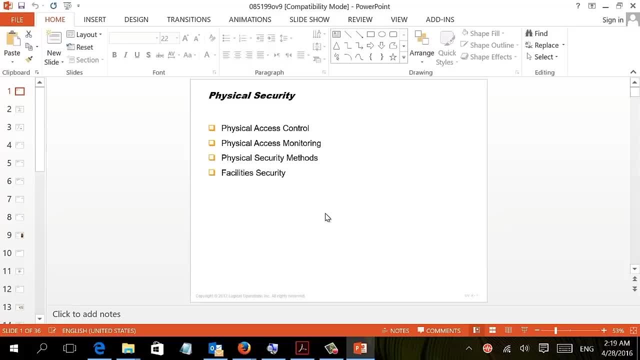 So you may get questions that if you get a class B fire, what should you use? co2 water soda. So the second point is the fire and type of fire and what should be used against fire in Firefighting tools, fire distinguish, fire sprinkles, and actually the sunflower document has helped a lot to categorize all of those just in one column. 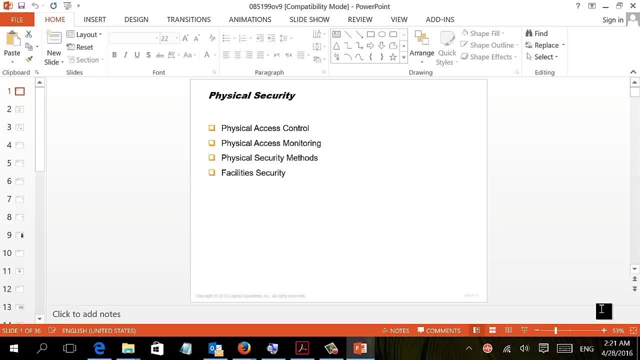 So it will be much more easier to read it from there, but you still going to need to memorize the image. the third point It's: Please write down those notes because if, when it comes to physical security, this is the major part that you may expect a question about inside the exam, 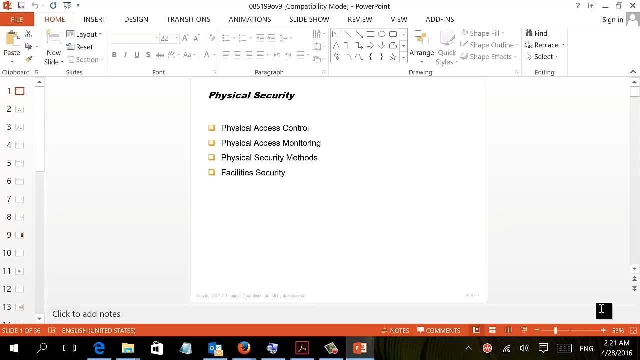 So data center where it should be located. What is the specification of data center? Like, some students get a question where they have been given a building and a data center and you need to drag the data center to the suitable pace, a place, so you cannot put the data center. 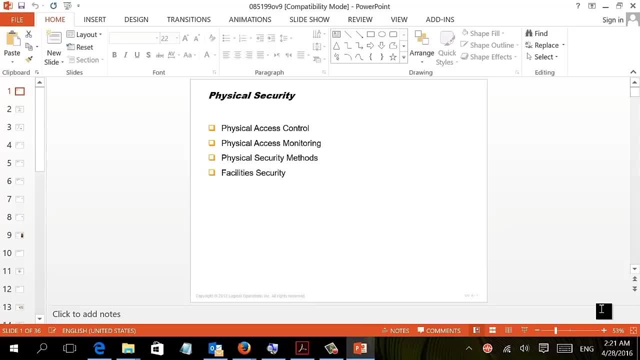 At the last floor because maybe there will be any leaking or something that or any under any bathroom or inside the basement, So in case they will be a float. also, data center should not have windows. This was quite clear inside the sunflower and it is a very common tricky questions. 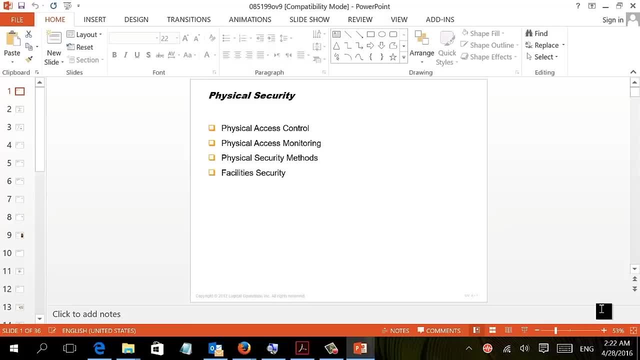 They will ask you: what type of window should the data center have, That the center should not have one. So those are the three point that is considered very important in the physical security, but we'll be going through all the topic and we're going to give special attention for those point. 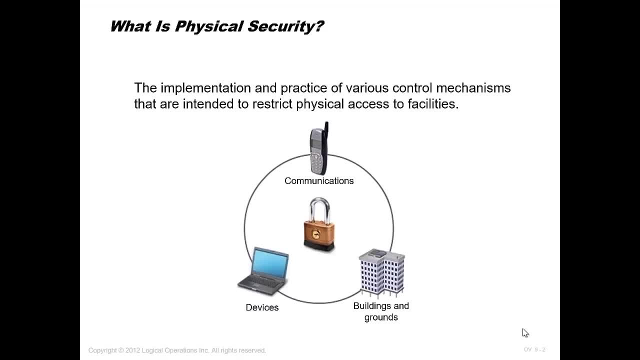 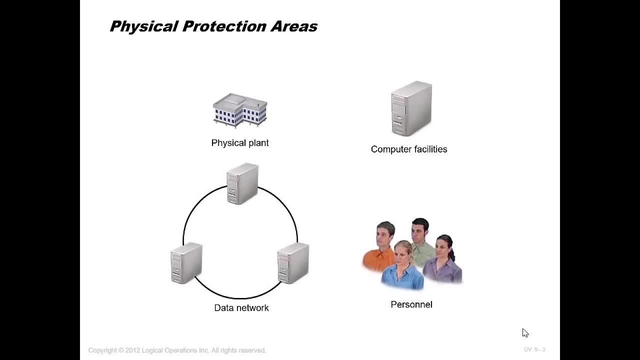 So physical security, It's to secure the place physically, secure the equipment, secure the communication and secure the building And even secure the people. So I'm not now talking about technical security. by the way, Another name for technical security Is logical security. 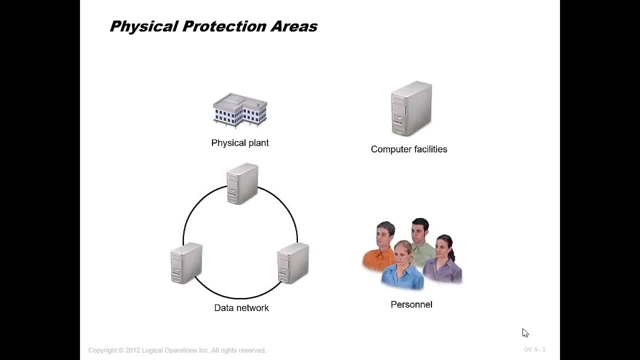 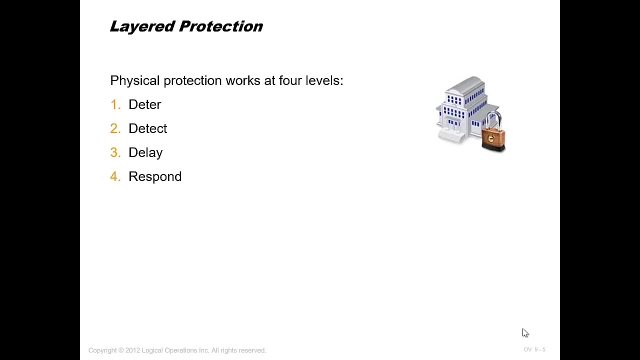 So We are securing, as we spoke, the communications and the data, the physical, the people, and we are securing them from different kind of threats: internal, external, natural threat, man's made threat. This is all just actually talking Now, when we are talking about the security. 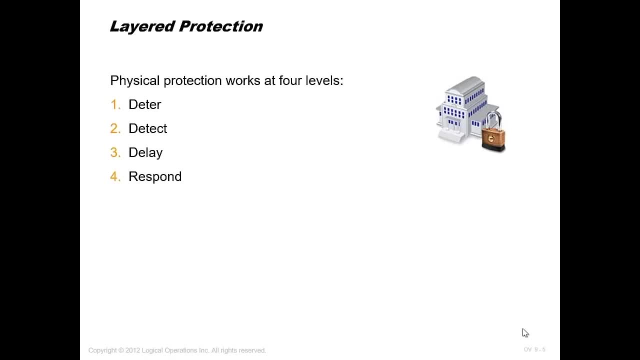 The physical security, The physical security implementation. We have category and this is a tricky part inside the exam. So we have the terror mean. it's like an indication. So for instant, a sign on a door that saying authorized people only. this is not a preventive. 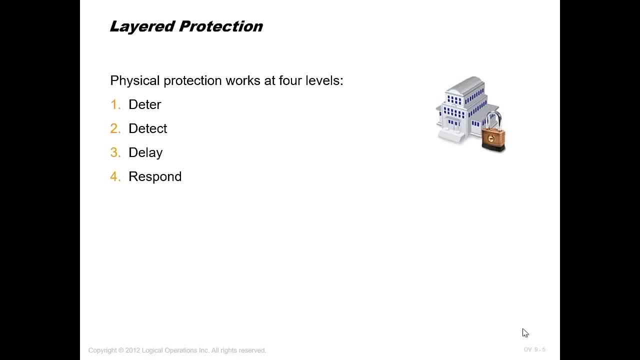 This is a deter. We have a detective like surveillance cam. We have a delay like some facility will have more than one door. when you go to entrance You have to go through two door. This is for to delay intruder And we have response like an alarm or something like that. 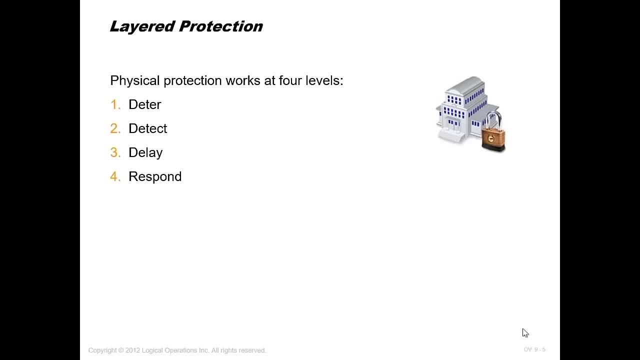 It's kind of confusing. I mean it seemed quite clear while while explaining. but let me tell you a question and exam questions that came. It was asking about the fences. What do you consider fences and actually going to give a small attention to fences on the next lecture- fences- 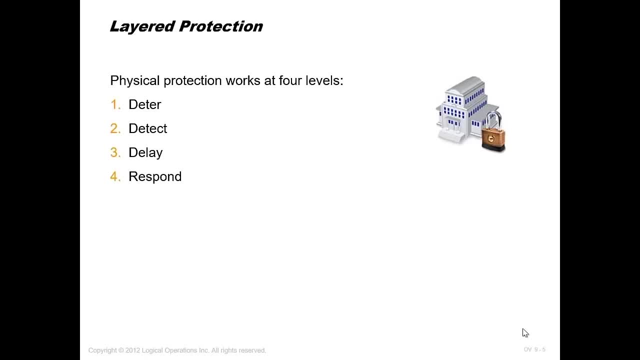 Do you consider that a preventive or a deter? So a lot of people think fences around the building It's a preventive, but actually no. According to I see square, It's a deter because no fences can stop an intruder. So it's a deter. 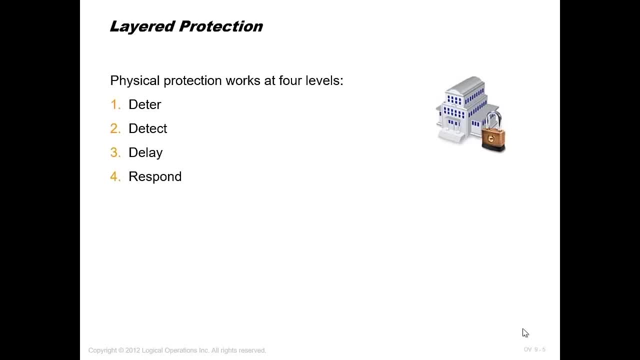 So what I'm saying is: maybe definition seem quite clear, but real implementation It's much more deeper than that. So you have to be careful while you are reading the question. I have to read the question more than one time, So we are protecting the premises. 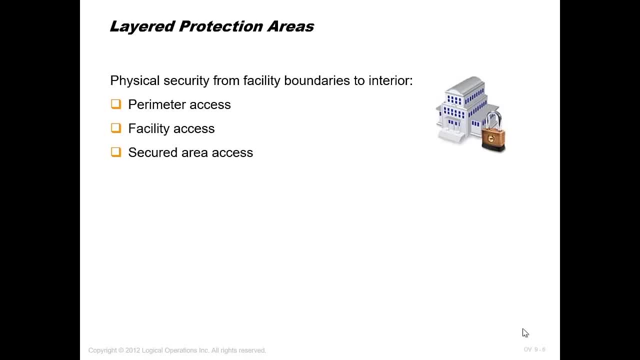 We are protecting the facility and we're protecting the secure area. From where should we start the physical security implementation? We should start from the physical security, should start from getting the blueprint of the building and starting and start checking Where is the vulnerable area. 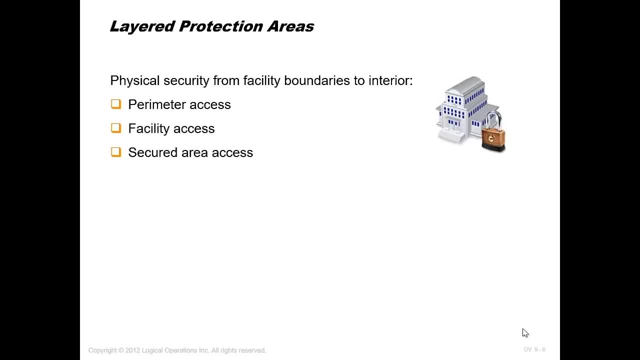 For instance, We do not consider the place where there is all the power switch Vulnerable, but actually it is very vulnerable because if someone was able to reach to this place and and disconnect the main switch, this will lead to a complete downtime. So this should be giving an attention, while the areas that has the washroom and the bathroom should not give that much of attention. 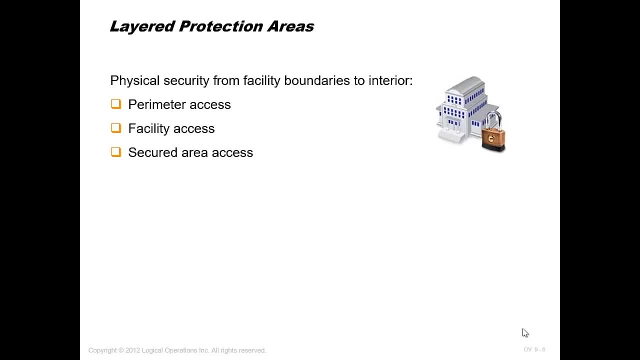 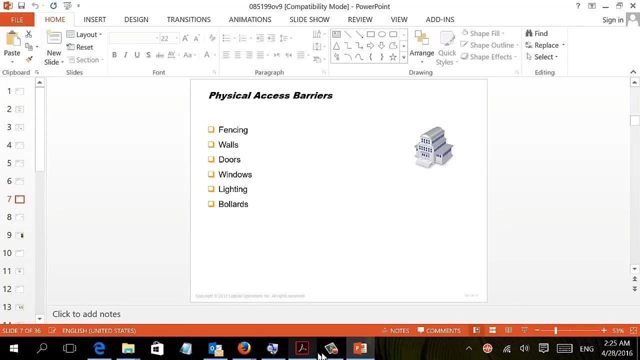 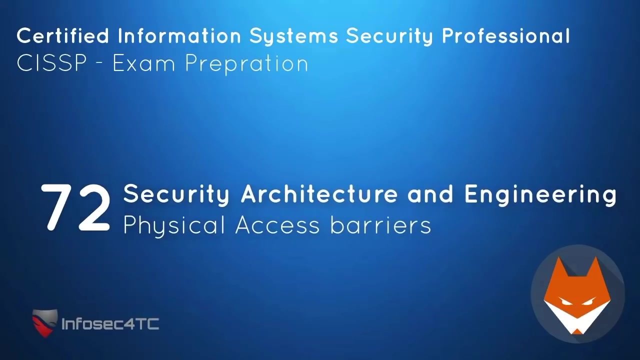 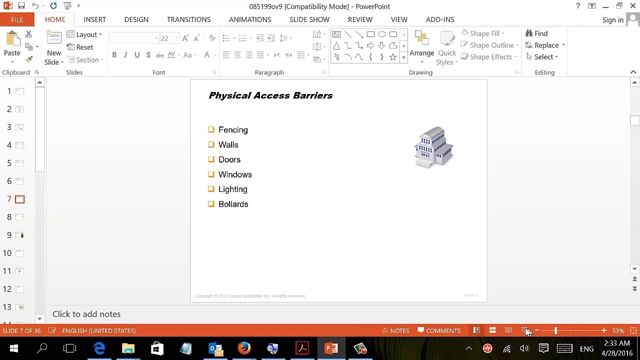 I should not put some like controls or some layer of security and so on. So you should identify where is the critical area inside your facility- data center, Power, communication, things like that. So it should start by identifying the critical area inside your facility. Now the first part in physical security implementation is to implement barrier, and barrier could be fences or wall or door. 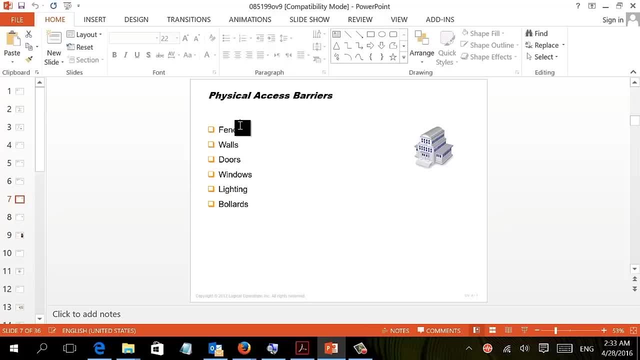 Or lighting and so on, and it's good to go through them, But I believe the most important part will be the fences and to know the different type of fences, and many of my students get a question related to fences inside the exam. Now I'll talk about some of the other technique and then I'm going to go about fences in more depth. 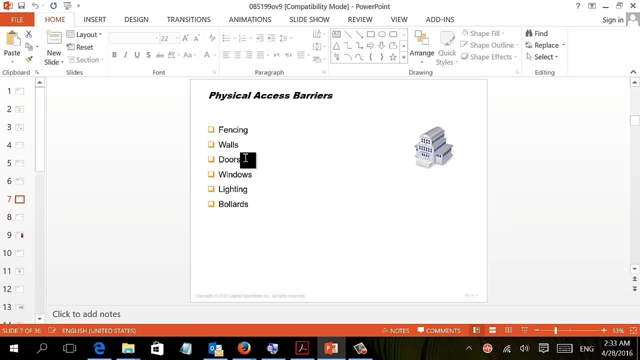 So, for instance, in doors we have different kind of door. We have the empty doors. that is very, very weak and can be broken easy. We have the bulletproof door. We have the hinge hidden hinge door, usually to make things more easy for yourself. 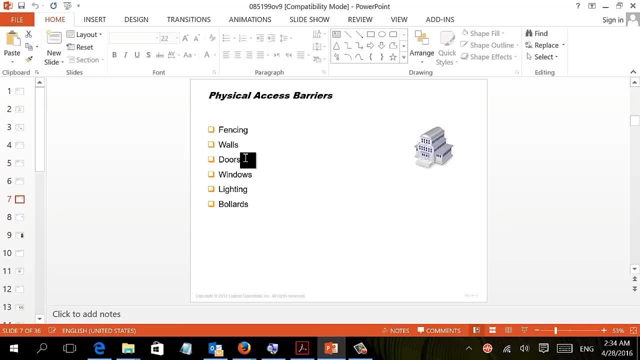 Whenever you have more than one type, just need to memorize the weakest type and the strongest type So he may ask you what is the best kind of door, but actually will not find that much of questions. as example, it come to everything except fences. 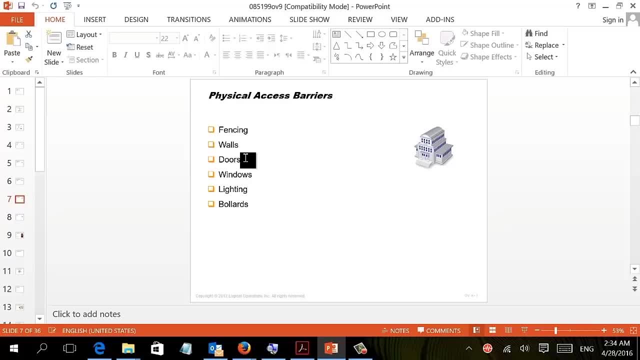 You may find the question about fences. So, as you can see, you have different kind of doors And wallet. we have a wallet. Usually we are choosing according to the ones that support the high temperature and we use that for data center room So if a fire happen or something you know, wall can support the high temperature doors. 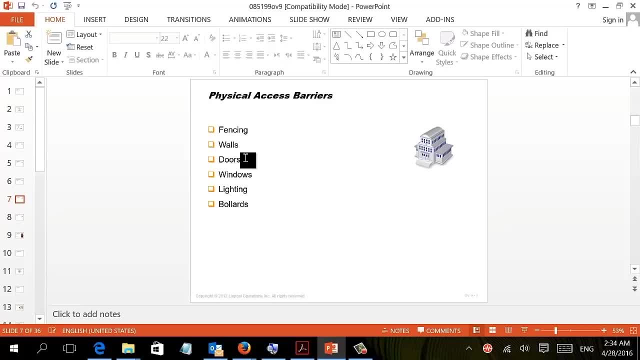 You should choose the door, depend on the location. I mean I mean the most expensive and most secure. It's waterproof door is waterproof door. is that means that I have to put to a bulletproof door everywhere? No, I cannot put a waterproof door on a well washroom. 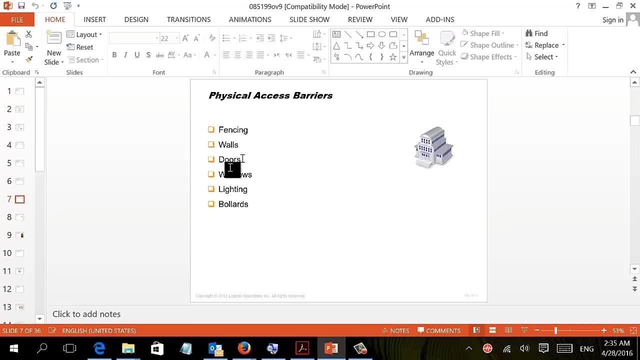 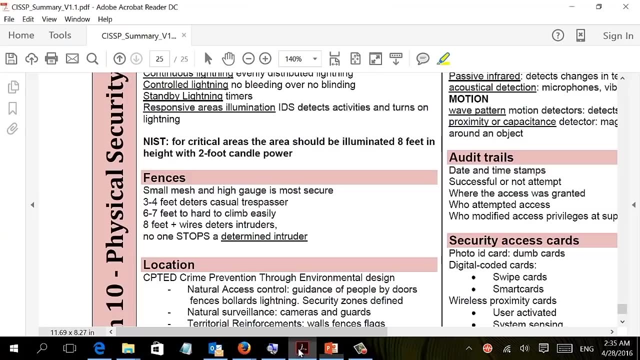 For instance, we have the lighting, we have the ball, But actually what I need to give a specific attention to is the fences, because it's very, very tricky inside the exam. So when we are talking about fences, you can see that here inside the sunflowers. 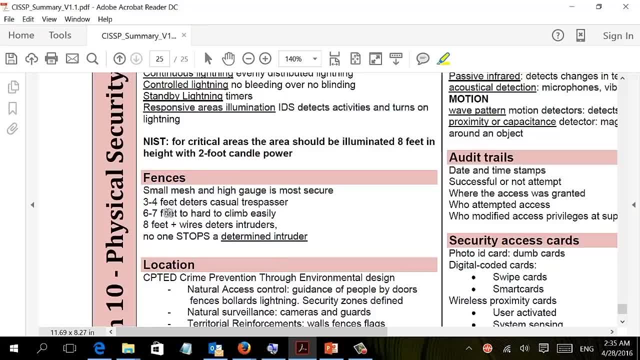 They put three different category for fences. Be careful with that. So for fences that has a lens from three to four, This is for the terror. It's not an, as I told you, it's not a preventive for the third thing: casual intruder or crunch. 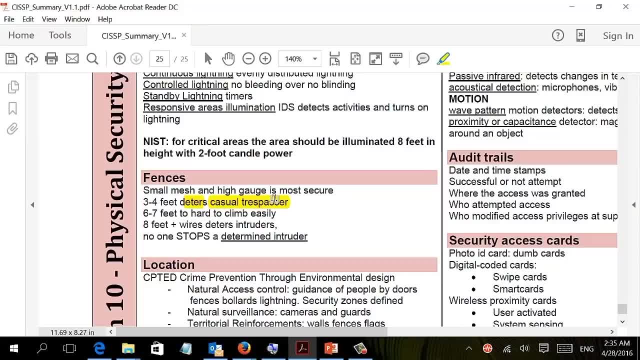 So someone who didn't have intention to break into the company when he find a very low fences, Maybe this will encourage him. six to seven- This is for- can be climbed easily, while the recommended one It's plus eight feet. So if you told you what is the recommended fence, less is eight feet, and don't forget this is the third, and please be given attention inside all sunflower document for anything that is underlined or is bold. 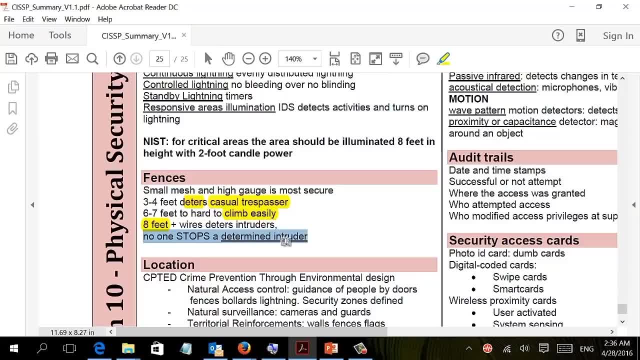 So no fences can stop a determined intruder. If someone need to break in, the fence will not prevent them, Whatever the lens is. So this part is very, very important, Especially this one. This is where the tricky- What will be coming inside the exam. 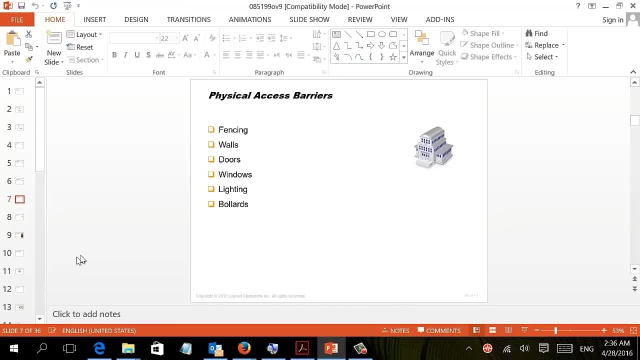 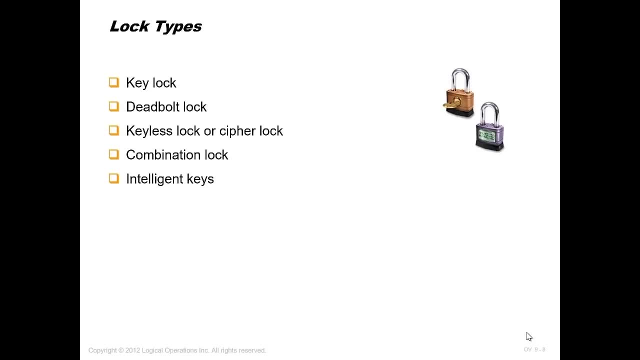 So this is the fences part. Now other technique will be pointing to, but they are not important for that, important for the exam. But it's good to know about them like type of look. We have the regular look, We have the pick resistant look. 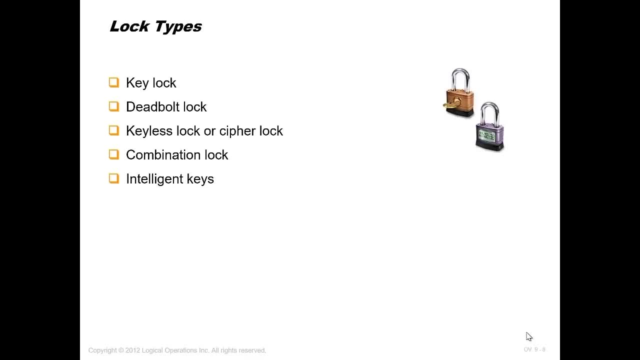 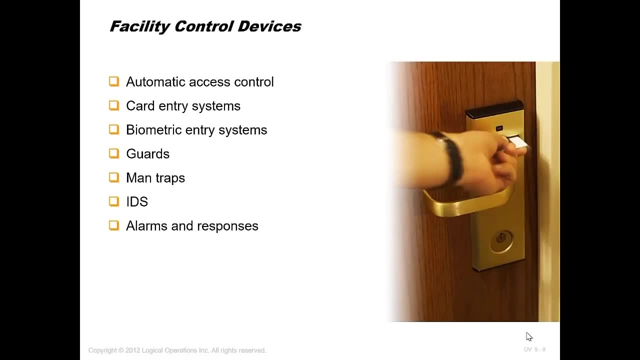 We have the combination look, the intelligent look. I mean you can search for anyone on Google image If you know. you don't know how it look like. the access control, We have the automatic access control biometric- went through that before. but I want to give an attention for guards, guards. 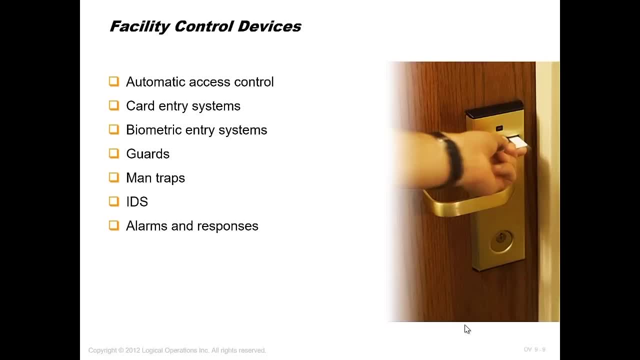 It's considered the most expensive physical security implementation. Why? maybe he's taking less salary, but actually is a guard, because when you are buying an equipment like an ideas, physical ideas- or you are buying or you are building a fences- You're going to make just one payment and that's it. 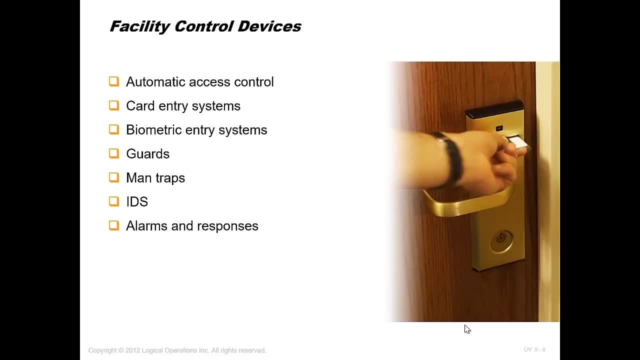 Whatever the payment was, it will be done one time. Well, guard is taking Monthly salary and medical insurance and so on. But what is the benefit of having guards? It has a judgment part so he can judge the situation. It will not be an automated situation. 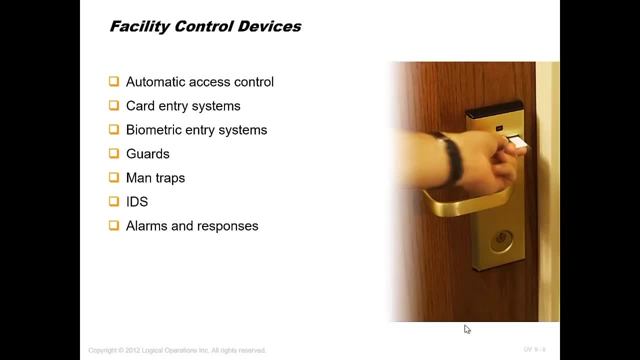 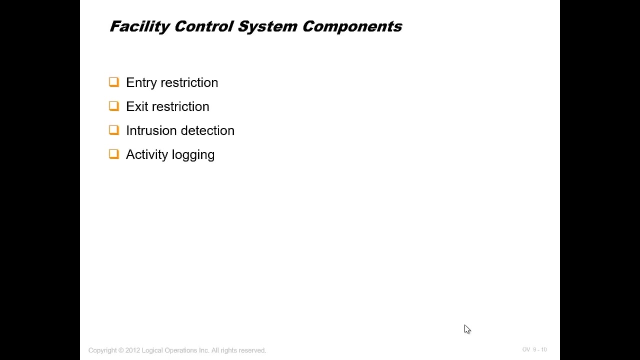 So you know, this is a careful man trap, which is a trap that like hold someone if he tried to steal or break through or something like that. This is some of the control. We can have entry restriction, We can have exit restriction, intrusion detection. 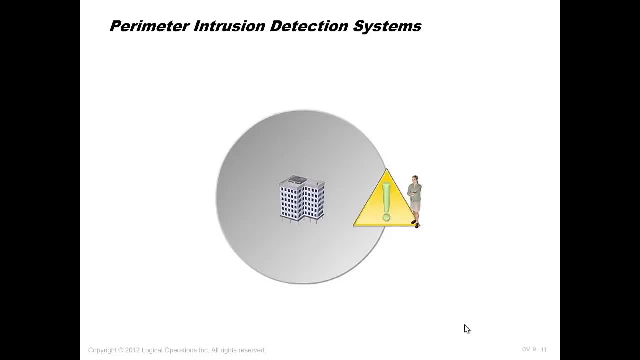 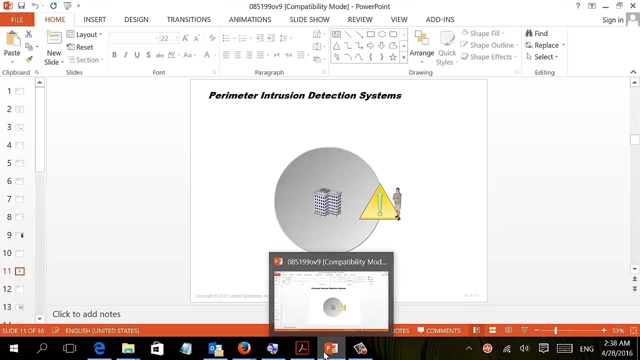 I mean, you know nothing here- need to be explained. Yes, regarding the ideas, not the technical ideas, but the physical ideas, the ones that can detect motion or can detect voice or electromagnetic ideas. in Sunflower You'll find the list of them. Let me show it to you. just have a brief about them. 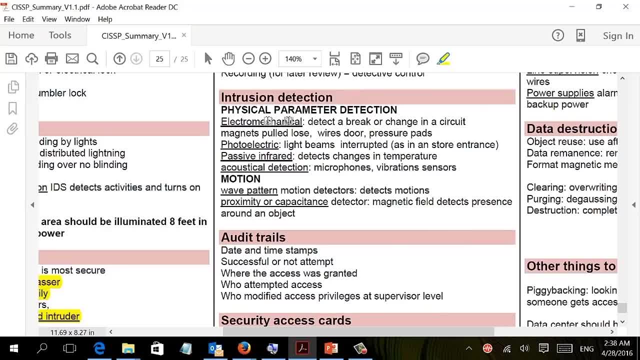 So those are the intrusion detection. You have the electromagnetic, You have the photoelectric ideas. Do you know what is a photoelectric? You know, when you try to like in big stores or malls, when you reach near the door it will open automatically. 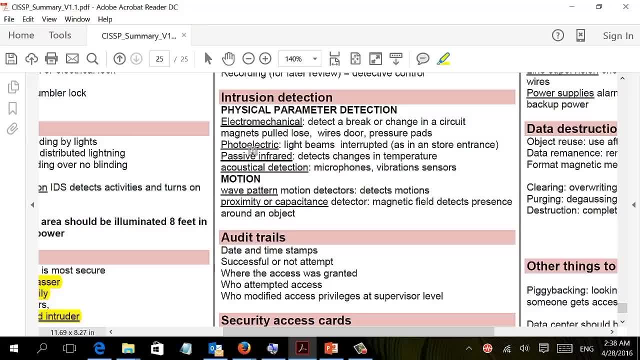 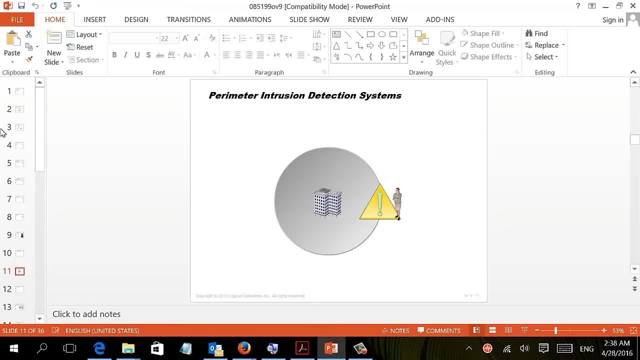 This is a photoelectric. It has a photon beam. When you break this photo, mean you'll be able to break automatically? I'm sorry. You'll be able to, he will. the door will open automatically. So there is different kind of IPS. 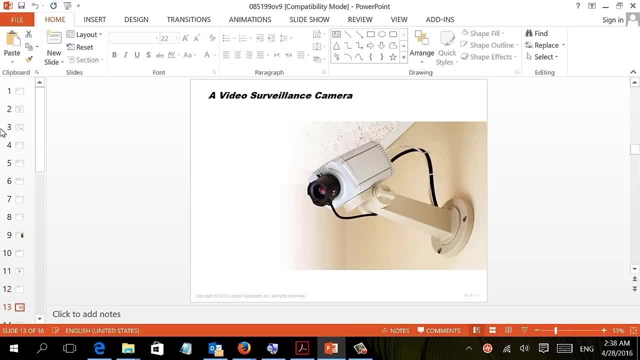 I'm just pointing to the important part. Those are the types that I just show you: surveillance cam. nothing is their type of surveillance. Nothing is there. This is an important part. logs- logs should be kept when it come to physical. So whoever access the facility, you should have his name, the time, the reason, a copy of the ID. 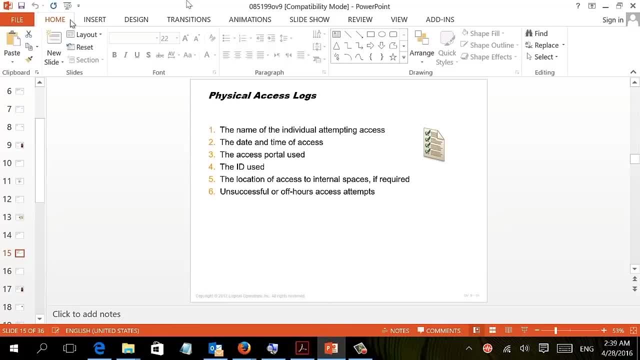 This should be kept and reviewed periodically. So in physical security, like access control, you should have authorization, authentication And accounting. So you should have a logging system and the log system should include such information and it should be reviewed periodically. The type of alarm: 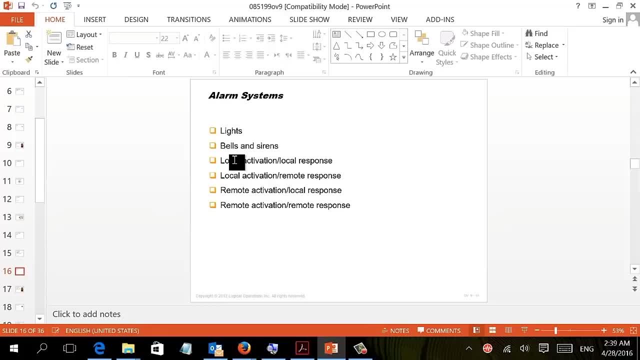 We have the line alarm and siren alarm, But actually those are the four type. Some of them is V. It's very common and some of them is very like local activation, local response. This is in case you have an alarm, that if something happened on this places, alarm will be triggered on the same place. 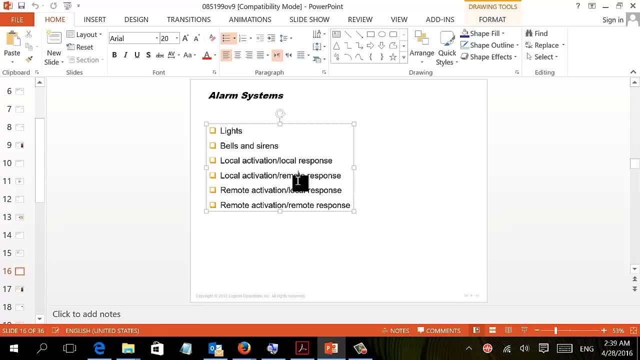 While local activation, remote response. This is like fire: a fire happen on the facility, the trigger, the alarm will be triggered on the fire department. The second is a certain force. actually, it's quite not common like remote activation, remote response or remote activation, local response. 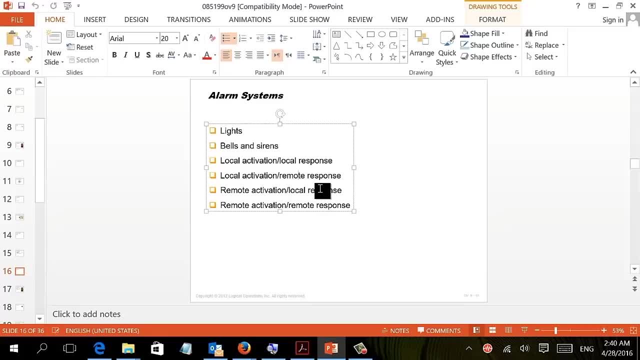 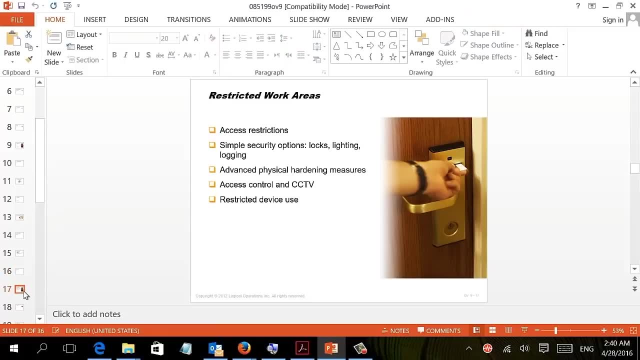 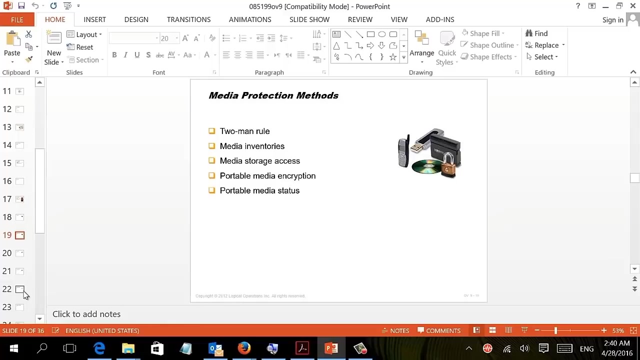 Actually this is like very theoretically- I don't have any example in my mind regarding that Restricted working area or Critical work idea- should be monitored, should be restricted Media risk to secure the digital media like external hard drive, CD drive, Those we will be covering during the operation: security, some of the policy, two-man rule and some other policies that can be used. 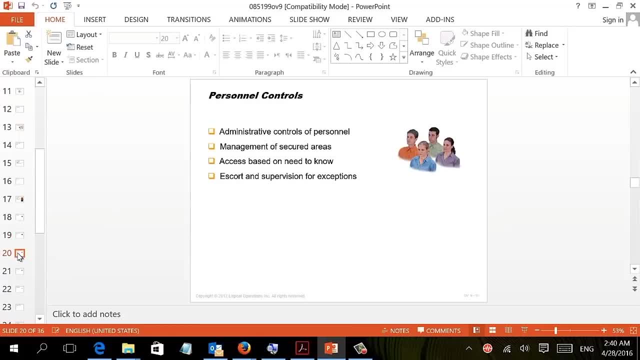 So he just explaining you know what should be implemented. but I'm need to point to the Important part for the exam perspective because, after all, In physical security It's usually done by HR people or operational people, but you, as an information security officer or someone managing the information security, you need to monitor that. 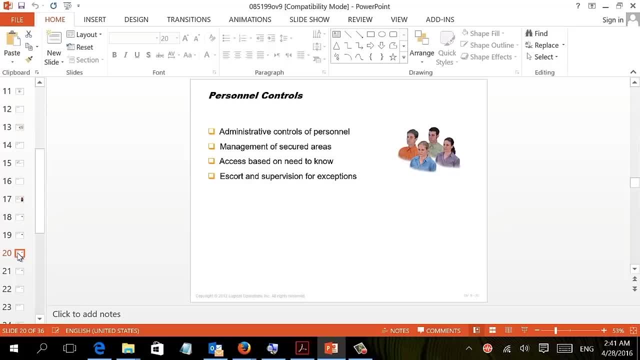 And you need to know the different options that you have. Okay, now let's go to, But before going, that don't forget. according to I see, square, personal safety come first. Any scenarios that you have that Problem happened, disaster happen. what should be done first? you should focus about people, so I call them twice a square. personal safety is the first thing to be considered. 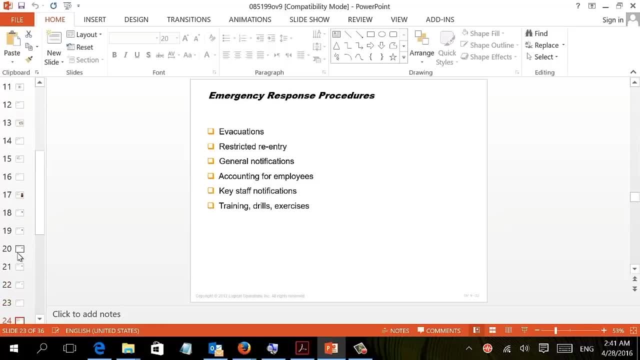 Okay now Also, facility design issue. here, One of the things that is related to information security, It's that choosing the design and the location is related to the physical security. I mean, if you are taking a site for your company that is outside the city and very 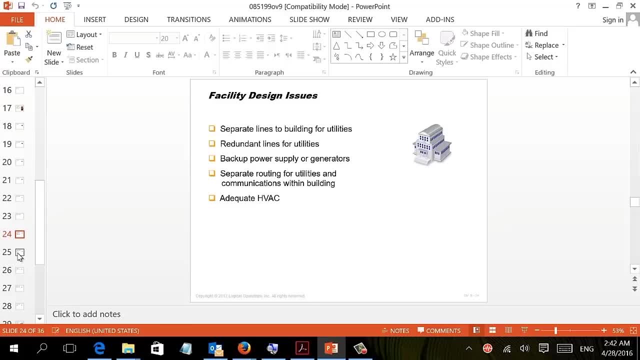 Dangerous area or is there is no transportation. you are increasing the risk. Also, you will find in some premises that they have like a long runway inside or with very high light, or maybe it's outside and maybe the reception area has a lot of glasses. This is a security design to make the intruder visible for a long time. so the design has a role inside the implementation of the security. 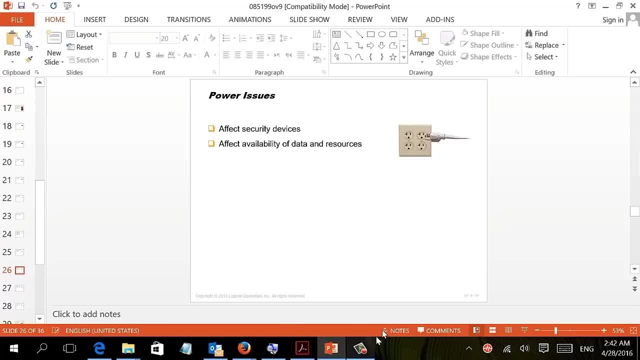 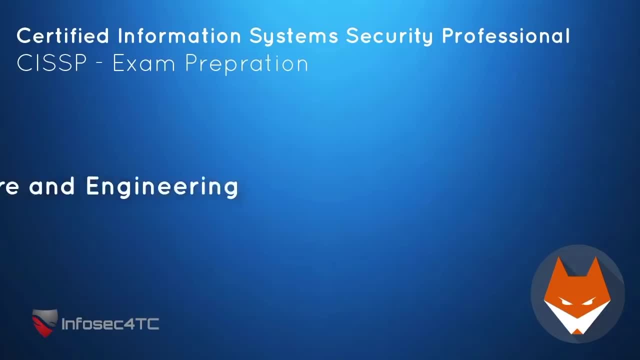 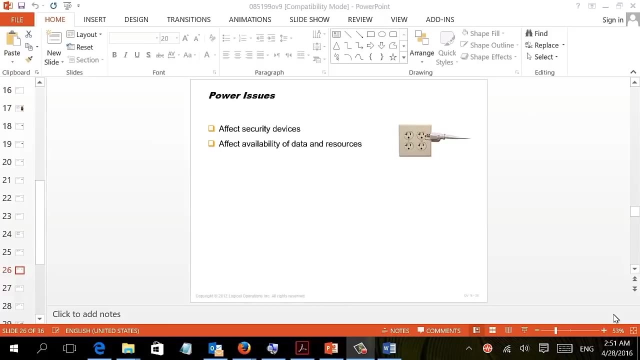 Now let's go to the power issue, which I think it's very, very important and most likely you will find the question about said inside the exam. In this lecture I'll be talking about power issue and, as I told you, because a lot of people focus on just one power problem, which is cutting the power or the blackout, 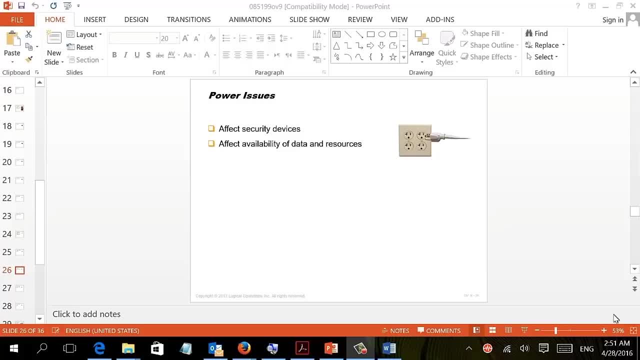 So they are putting all kind of countermeasures Again said, but actually there is six kind, six type of power problem and it will lead to the same result. I mean if you get exceeding of voltage it will damage the equipment, If the voltage is going low it will damage the equipment and those need different kind of equipment. 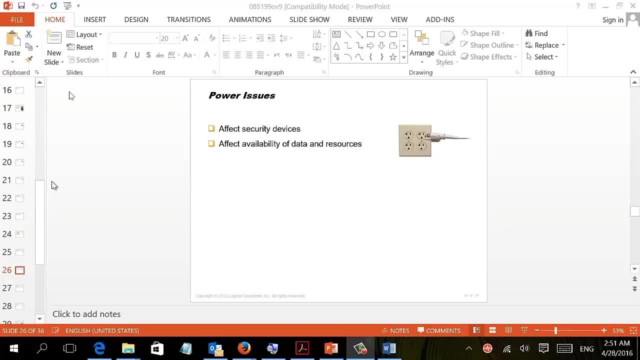 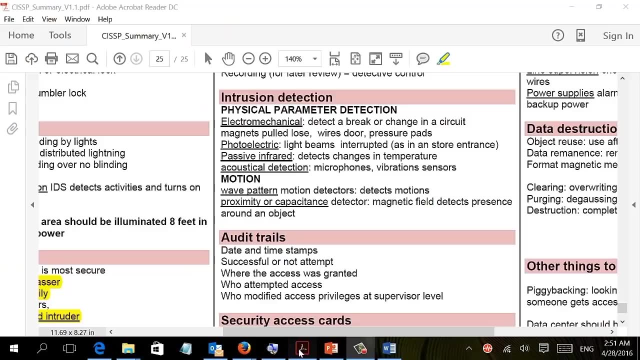 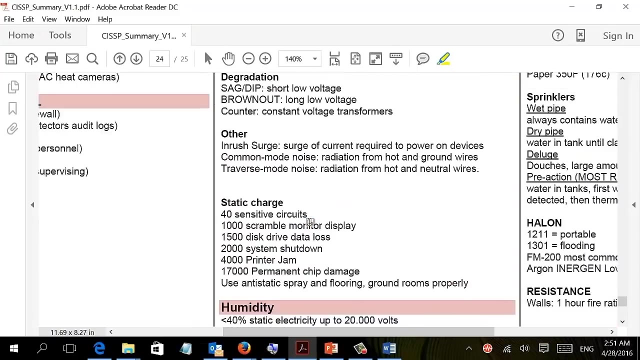 So not all the power problem will be solved by generator or UPS. So we have six type of power problems that you're going to need to memorize the name and their definition and the you may get the question about that. So here is the example asking you about what is a surge or what is a spark or what is other kind of power. 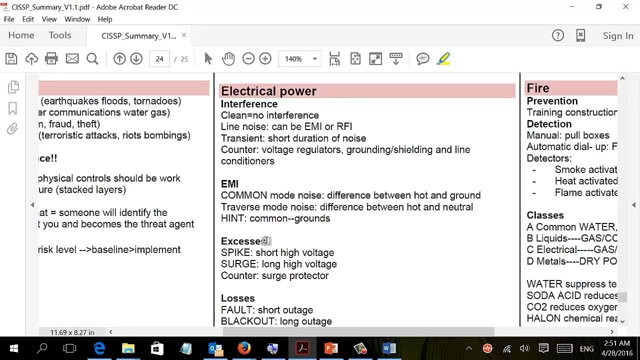 So the electrical problem, let's take first the exceed one if the voltage exceed. So if it exceed for a short voltage, for a short time, short voltage exceed, this is called the spike, while if it exceed for a long time this is called a surge. so spike and surge. 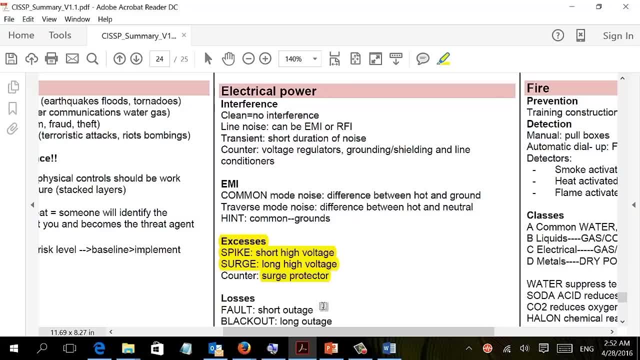 And what is the counter Tool to be used? surge protector. So he will ask you: what do you call the long, high voltage? is it surge? is it, sir spike? is it fault? is a blackout, and so on. Then the complete loss of power. if it's a short loss of power, 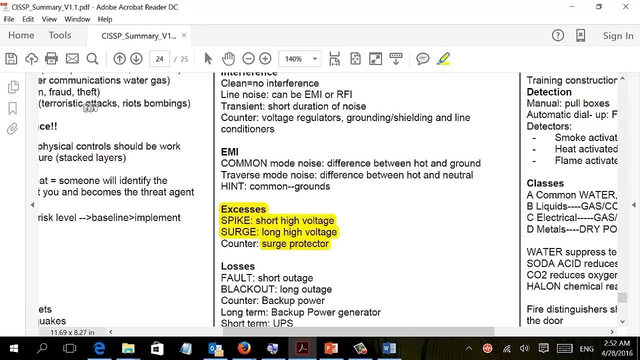 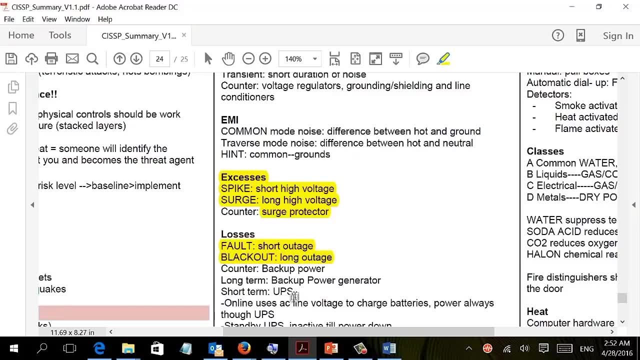 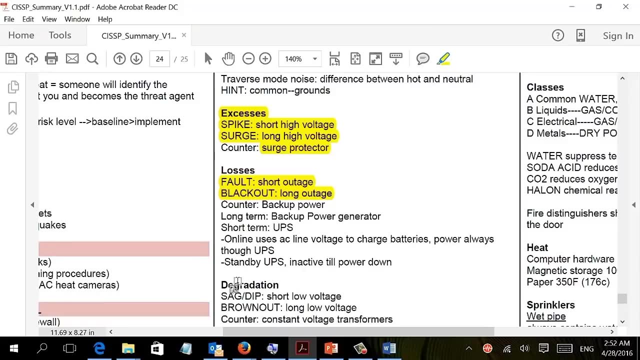 This is called fall, And if it's a long term, this is called blackout. And what is the counter for that? UPS? The third one, which is the degradation in decreasing of the voltage, if it's short term, is called sag or pit. if it's a long term, is called the brown out. 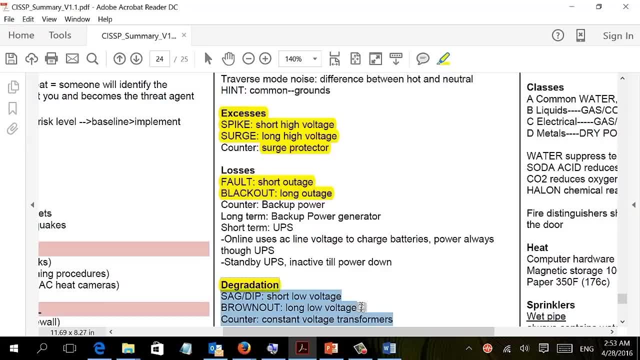 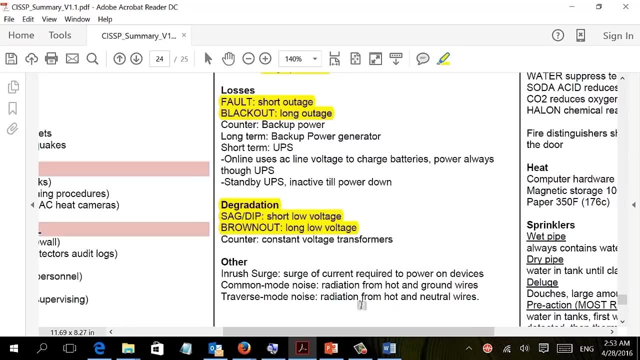 So those are very, very, very important terminology, as I told you some point here. I can guarantee you find the question about the exam fire power problem and most probably in the data center and the location of data center, other problems that we may face, things like 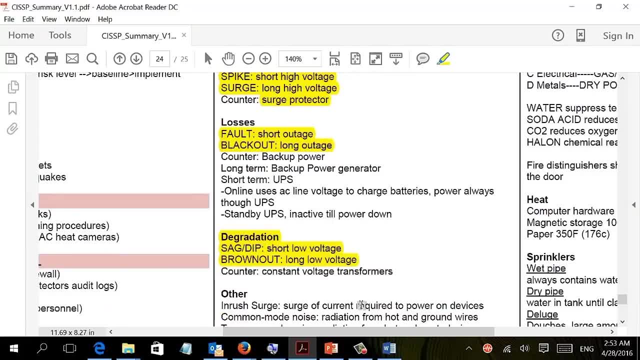 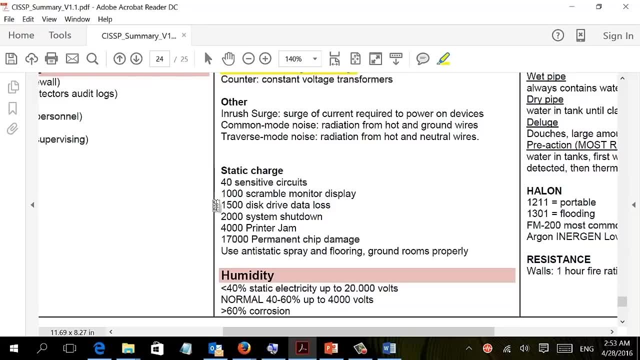 The static. you know some people has this problem with the static charge that so you may need to know about static. just to brief, about the charge: What could damage what if the static reach that much? it will damage what this amount, but I will. I won't recommend you to memorize all of them. 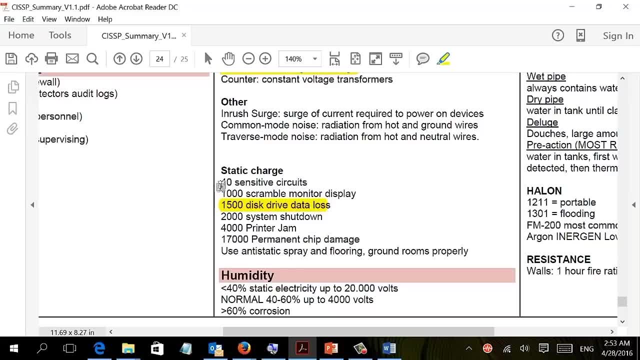 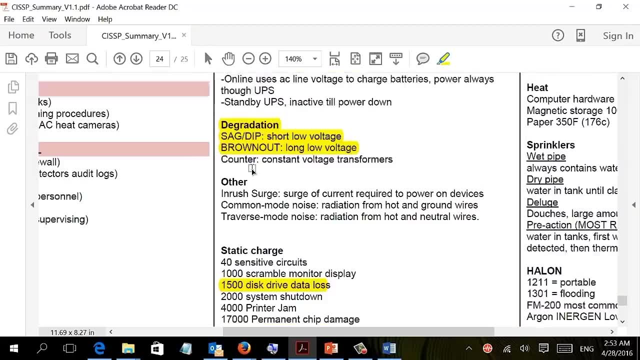 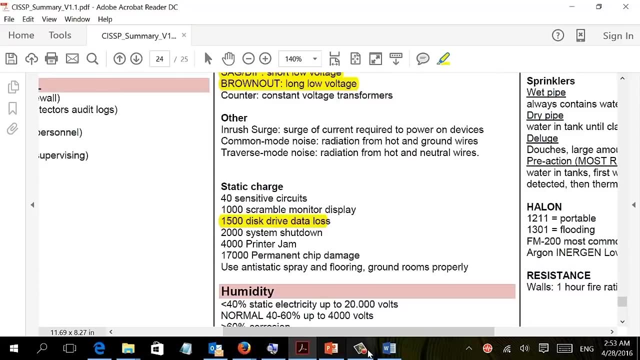 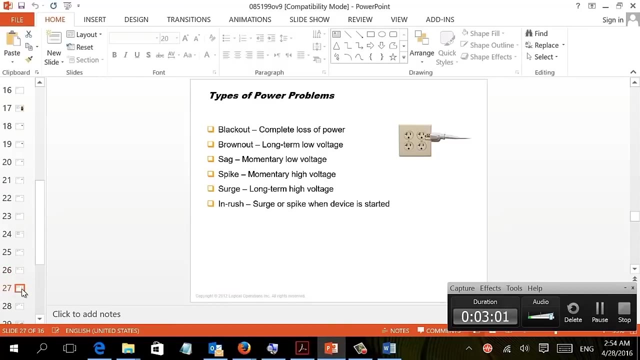 only the measure, one like what can really do damage? you know, like if you got more than seventeen hundred as a static, This can Really damage ships. So the this column, I believe, is very, very important regarding electrical and power problem. And here is the name: Eric are there, but it's not explained. but it's very important for us to know exactly what is the type of power problem and their definition. 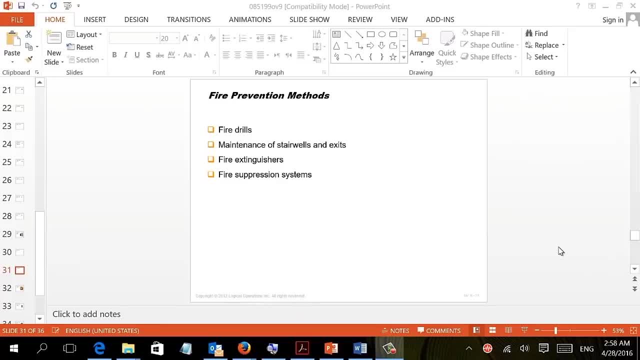 So the this lecture I'll be talking about the fire and, as I told you, this is the second important part. so you need to know the different type of fire, The different type of fire fighting tools, a different type of sprinkles, the different type of. 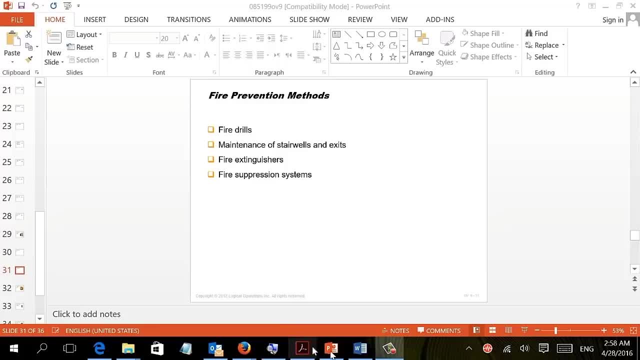 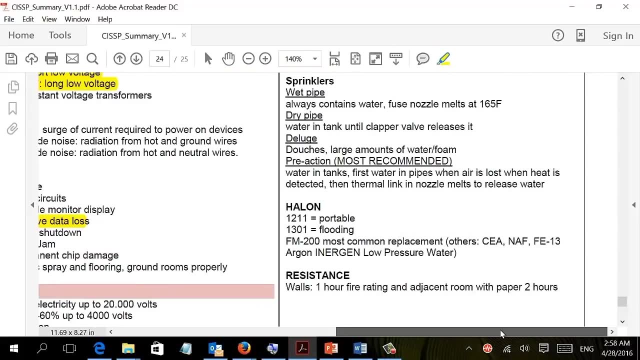 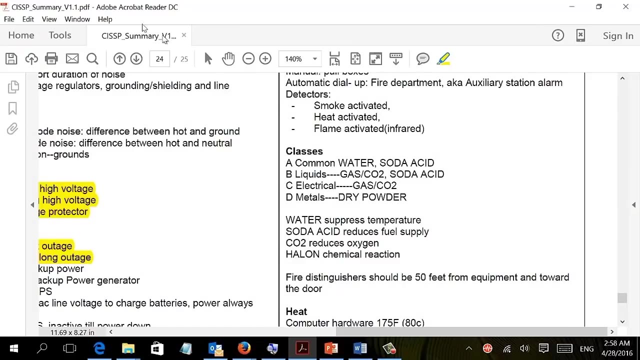 Tools used for for shutting down the fire. so this is a very critical part and, as I told you, it will be very, very good if you Open Open Google image while you are studying that. so the first table is that you need to study is this one: the classes. fire has been categorized, so we have 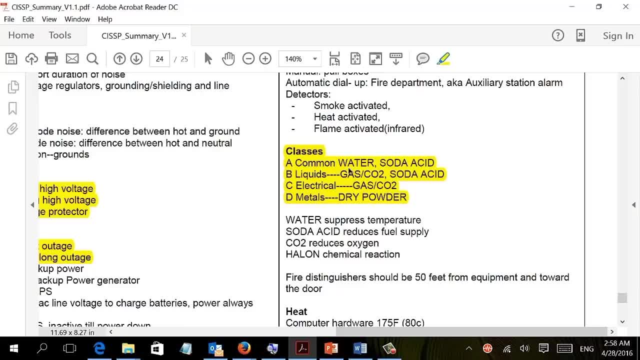 Class is. this is a common one- and what can be used to Deal with this: fire, water, soda and assets now below there. it explains the role of each one of our like: water is to reduce the temperature, while soda this is to reduce the fuel Supply. 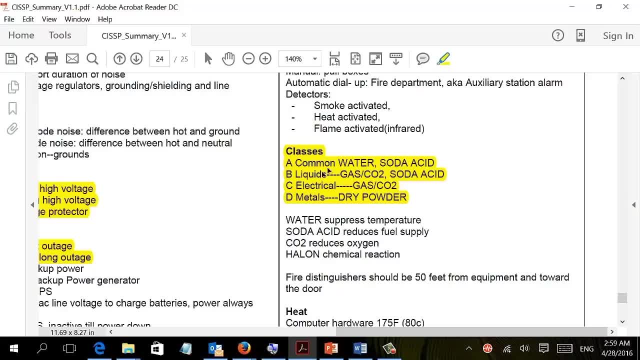 Okay, the B. it's usually from liquid. you cannot choose water in the B type of fire. so it could be liquid, it could be oil, it could be something. What should be used? gas, CO2, soda acid, and here you can see that CO2 has a, has a function of reducing the oxygen inside the fire. see- and this is usually the one related to us, because most of the fire got- 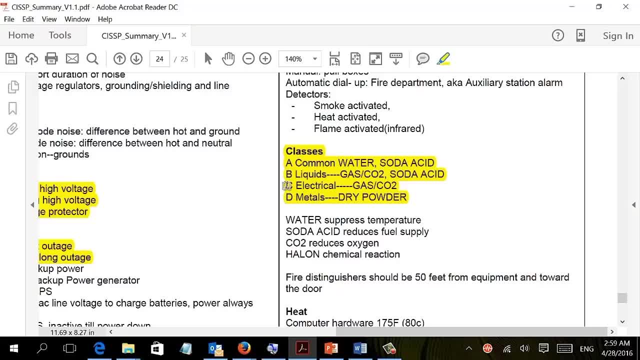 Forbidden. It's Related to electrical equipment. so what should we use in and see we should use gas or CO2. and finally, the worst one is it is one for on metals. this would be very, very high Temperature file. and what should you use? dry powder. so you need to know the staples. there is actually one more is called K. 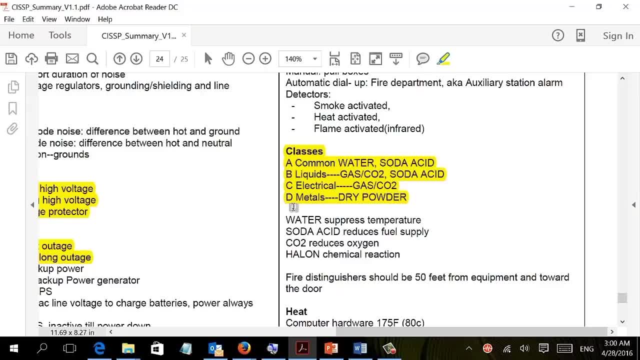 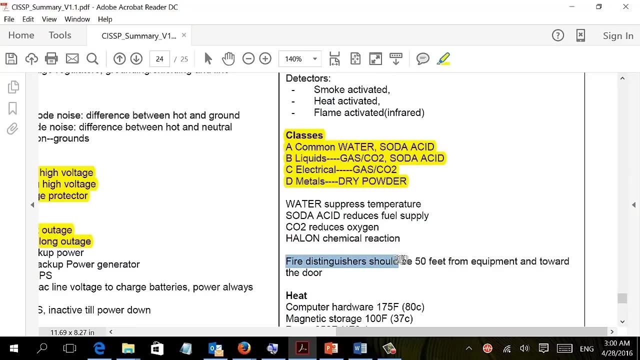 Which is for kitchens material, but it's not mentioning here so you don't need to memorize it. so classes need to be knowing the type of fire and what Should you use in any kind of class and the explanation of that. now, this is also an important point. that fire distinguish should be fifty feet from the equipment. 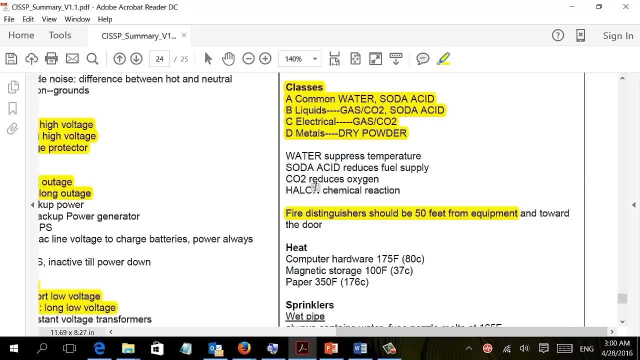 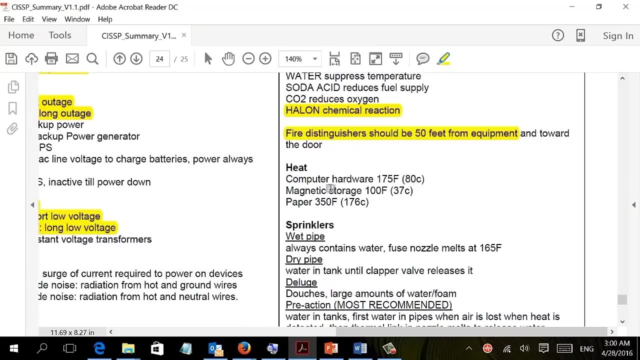 It's a rule. okay, now for Helen. there is one. notes that, if it's possible to take it down, that if they are not choosing that anymore because it was against environments, they are using something called FM two hundred. So please write it down. This is very important. it was. it was inside the the sheet somewhere, but I don't know where exactly. so we are not using Helen anymore now. sprinkle also is very important. 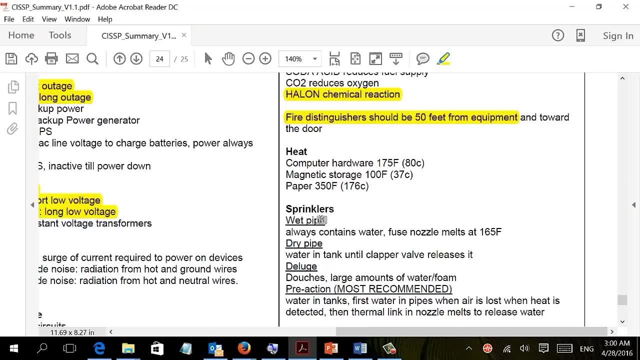 We have the wet pipe sprinkle and, as I told you, it's good that if you need to see how it look like, specially the rare one- I mean I know the wet one or the dry one- you can copy that And you can check on Google. so what is the problem? there is a wet and dry. 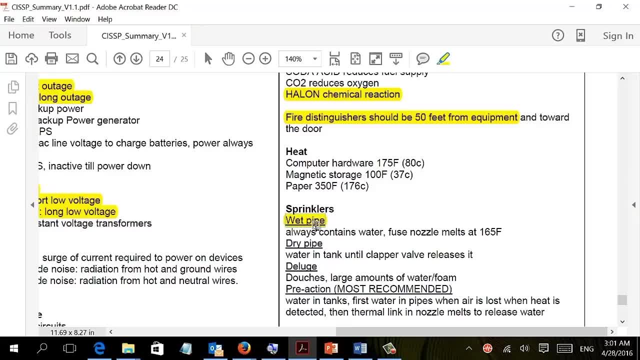 So The problem with wet pipe that the The water will be inside the pipe. so what happened is, if you are using that in one of the European country or the countries that has a very low temperature, the water will get freezing and it will prevent water from dealing with fire. so for country from this nature is a dry pipe is better. 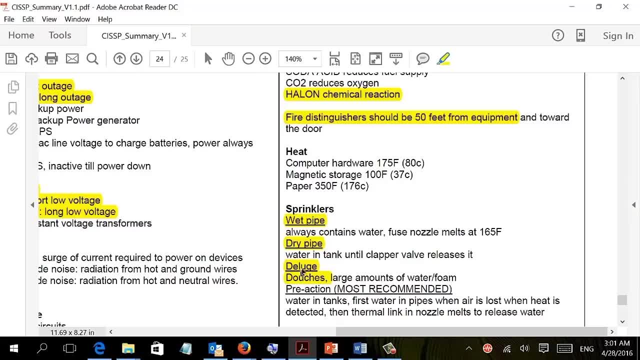 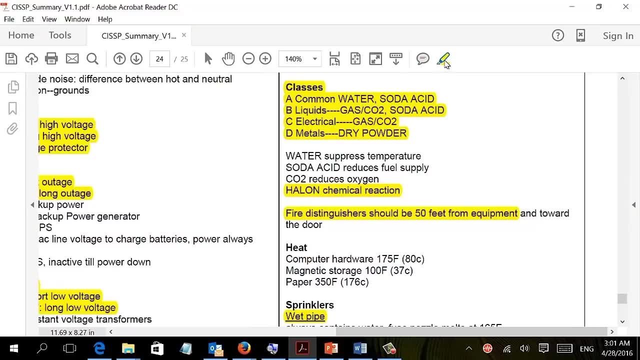 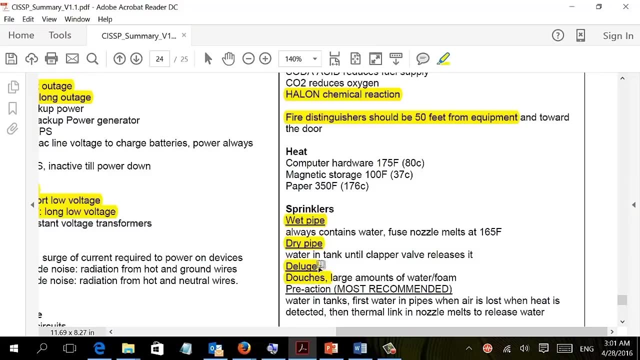 There is this one and this one. actually, I guess the question myself about this one. it's called the du, like Water pipe, let me just don't know how to- And this is actually. it's good it's doing or it's spreading a huge amount of a huge amount of water. so I don't know if you saw that before, I don't know why it's not selecting, but if you check on you, this one, Google, let me write it down, you'll see that it. 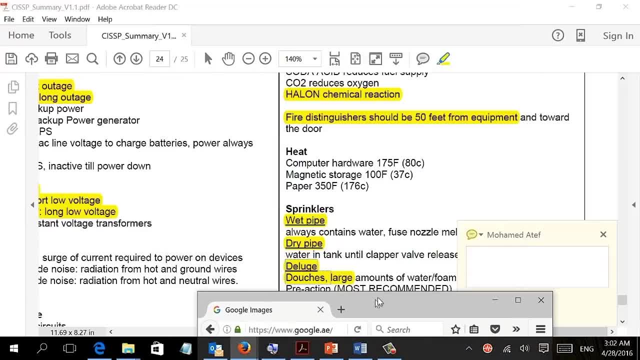 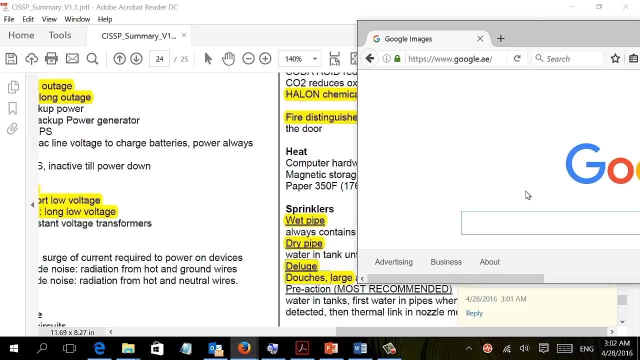 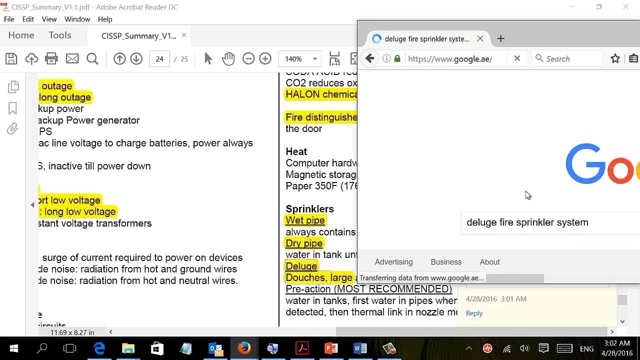 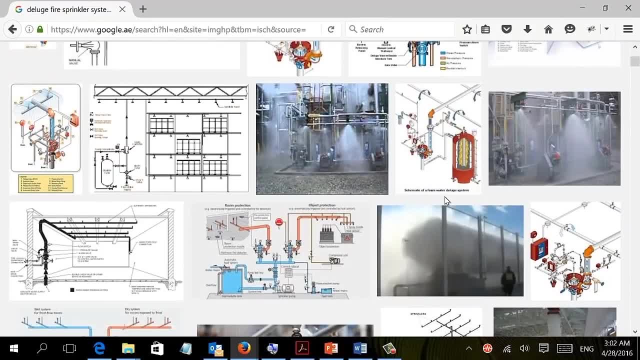 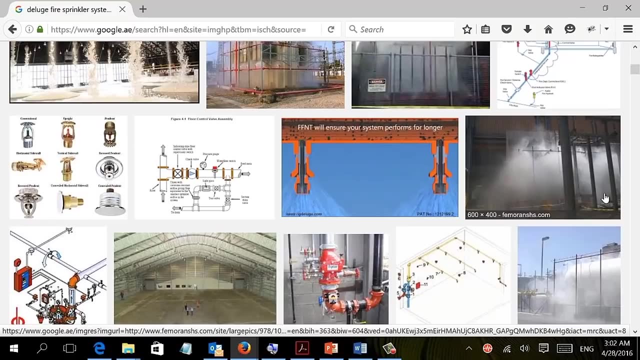 Sprinkled system. Okay, when it come to Fire, Different type, don't forget the best one. sometimes ask what is the best one to be used. so see, it look like that and it spread a huge amount of water if a fire happens. so it's good to take care of fire, except it's not. 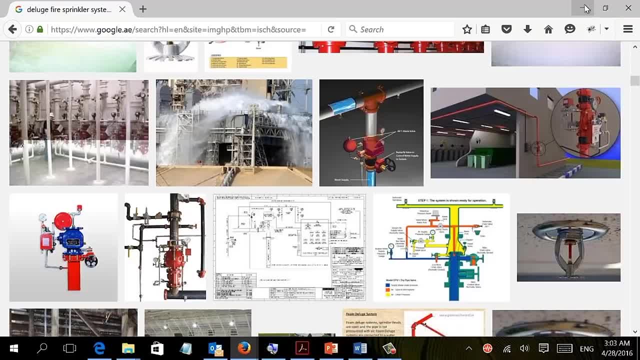 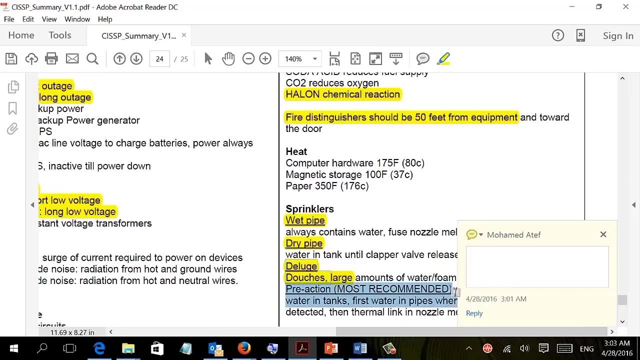 It do a lot of damage. okay, see the amount of water. So the best ones. that's why they are putting, see, a underline. it's called the pre-action because it's it has a automatic Part and it also allow people to interact. this is considered the best one. 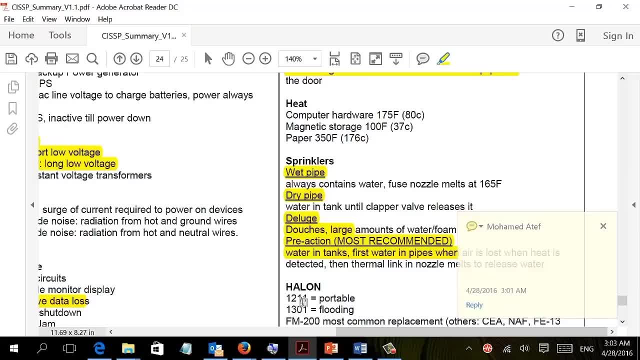 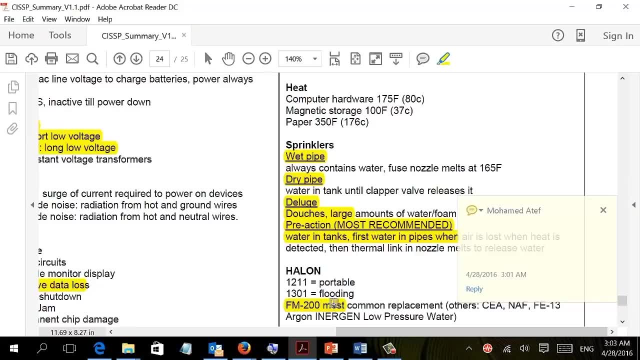 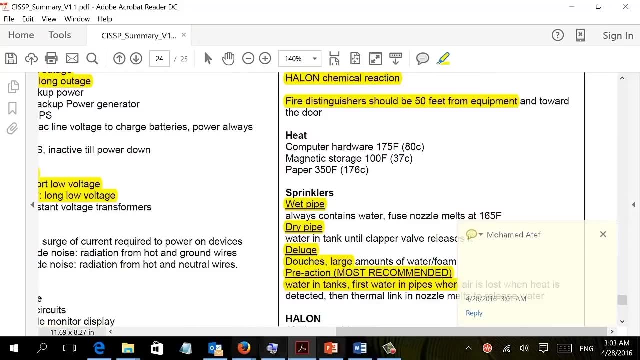 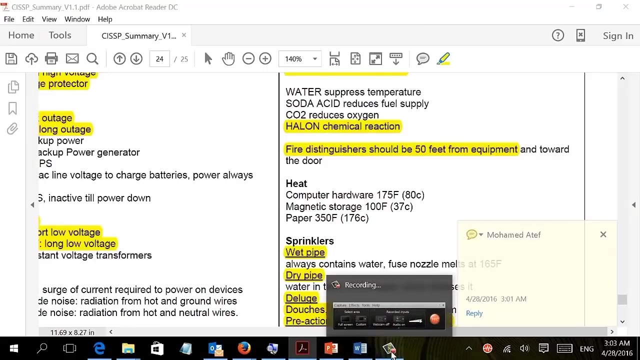 Okay, not this one, that one, the pre-action one, As I told you, here you go. Helen, is not recommended anymore. We are using instead of FM 200.. So this is what you need to know about fire. just one column. It's very important to know those terminology and the different type of fire and fire distinguish and where the fire distinguish should be and the fire sprinkle and so on. 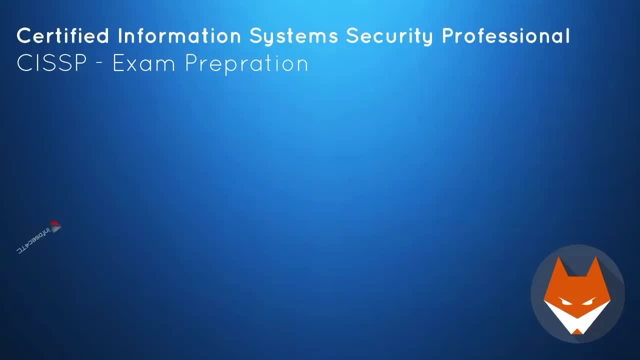 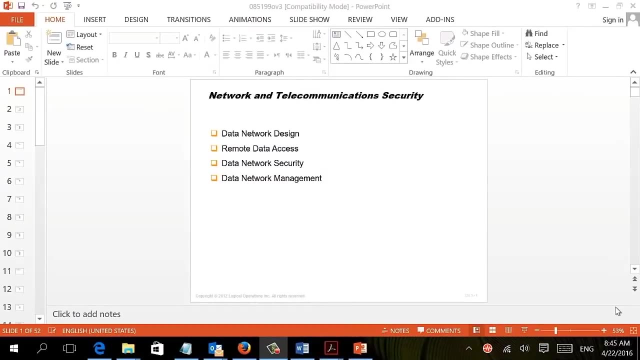 Okay, Third domain is network and telecommunication security, and this is one domain that has not been changed since the third edition, So it's almost the same domain in the third and fourth CISSP edition. Most people who are studying CISSP came from a network. 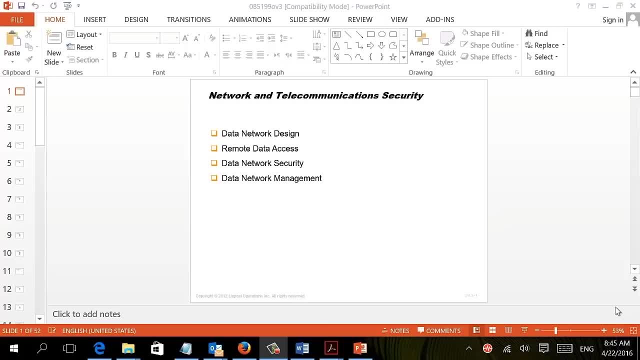 Background or technical background. So they will be feeling very comfortable going through this domain And you will not find any problem with this domain, except of the Amount of memorization that you need to do, and this will be not. this will not be a problem. 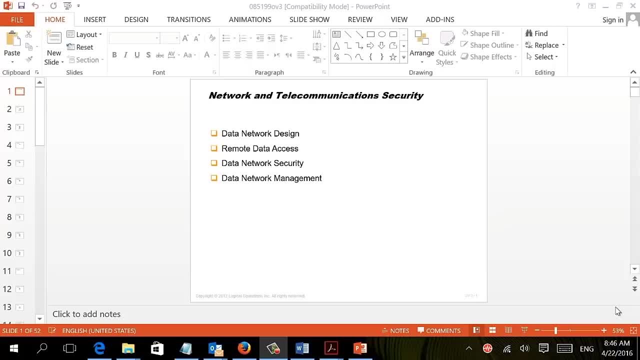 If you are using the sunflower document or the CISSP summary that gather everything together. So in this domain will be talking about almost Everything related to the network: network components: network protocol, network topology, network models, network attacks. So we it's considered like a crash course into the network. 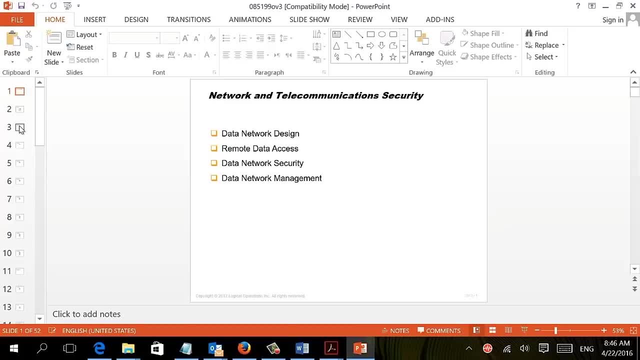 Now, usually in any network course, What is the first thing that you should study? So OSI model or open system internet. So the first thing in any network course that people study, Even if you are taking network plus or CCNA or Microsoft net, any network- 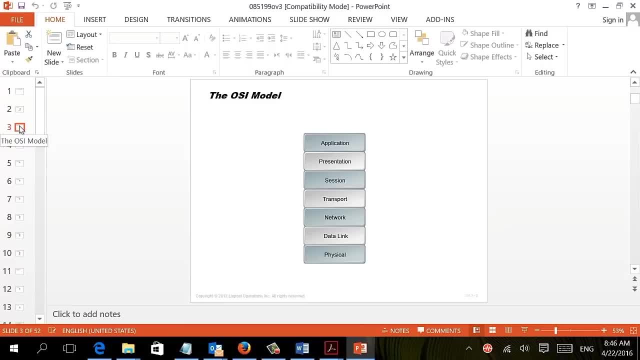 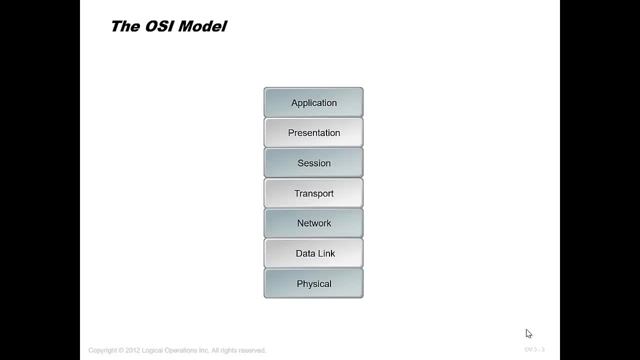 They used to start with OSI model as a standard use inside the network, So I'll be briefly going through that in case you are aware of that. But if you already are aware of OSI model with all its definition, you can skip this module except. 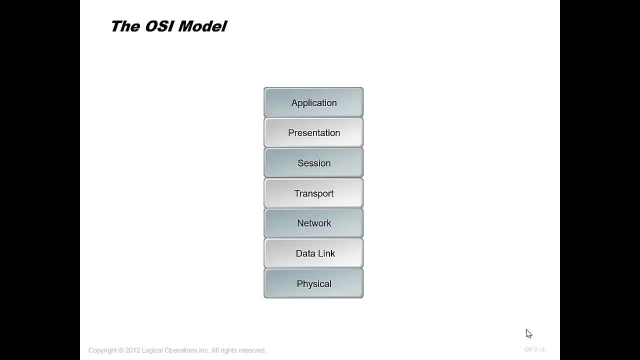 You need to know. what exactly do you need to know for the exam Regarding the OSI model, I mean, he will not ask you for the what is the application layer is doing or what is the presentation layer zone. He will be asking you about which protocol are working in which layer. 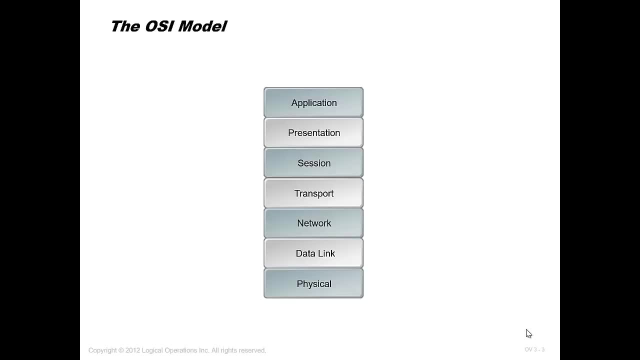 So he may ask you: DNS protocol is it's working on each layer, or TCP, UDP are working on which layer? They are working on the transport layer, or rep or EIGRP, which are routing protocols, They are working on which layer. So the only part that 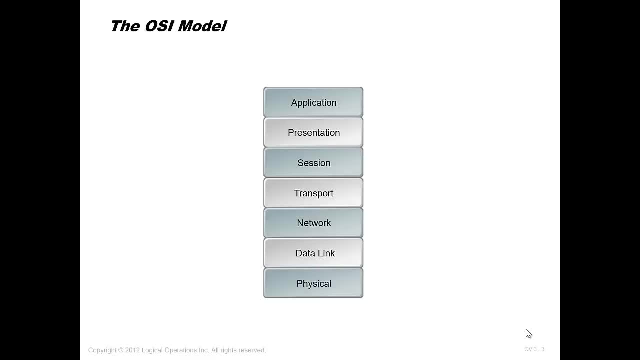 You have to make sure you are comfortable is not to understand the functionality of each module, but mainly to understand each module or each protocol are working on which layer. This is very, very important. So let me just briefly go through the model, the OSI model, for people who are not aware of that. 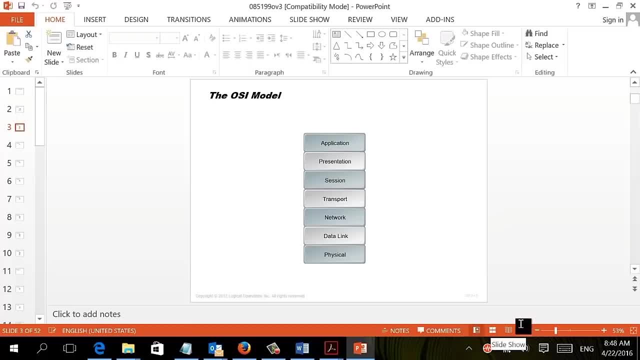 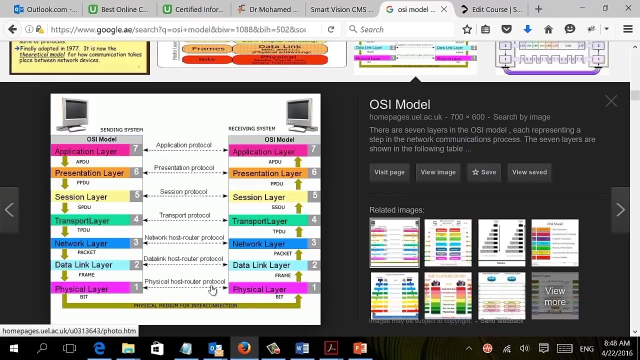 And then we will be talking about the protocol used in each of the layer. Now OSI model has been found, I believe in the late 70, to standardize the standardized the communication between the machine. So the point is that when two computer communicate together before the OSI model has been was introduced. 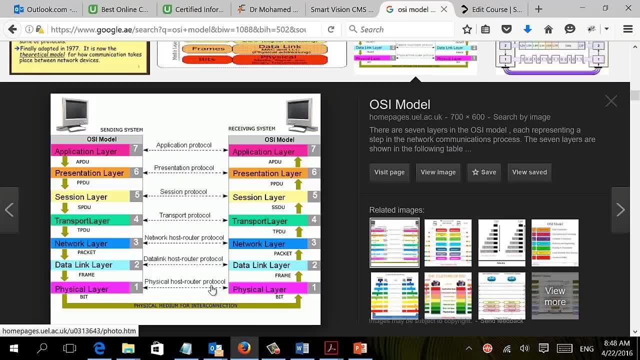 Different company used to make different systems that can only communicate with each other. So IBM was doing computer And they were. They were doing protocols that allows them to communicate together. HP was doing the same, Compact was doing the same. So we'll never find the network or you have IBM and HP and compact on simulator because they are communicated with different language. 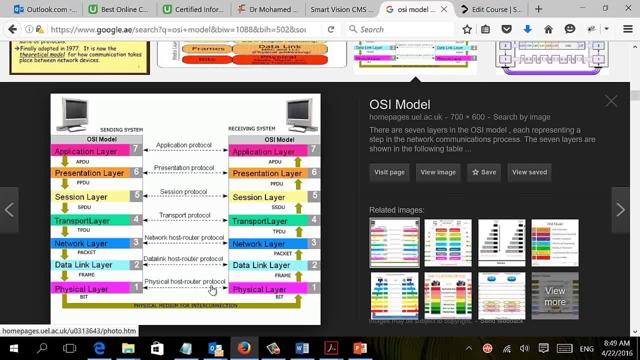 So OSI model is like standardization Of the communication. So everyone agreed to work with this model And according to that now IBM machine can communicate with. HP was compact with them because they are all, Because they are all communicating in the same way. 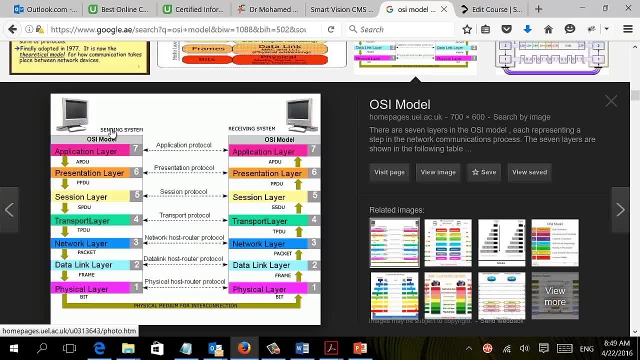 The objective of OSI model, or the aim of OSI model, It's to make one standard way inside communication. And to brief you about that, What happened is, if we have two computer here And computer on the left hand decided to send an email. 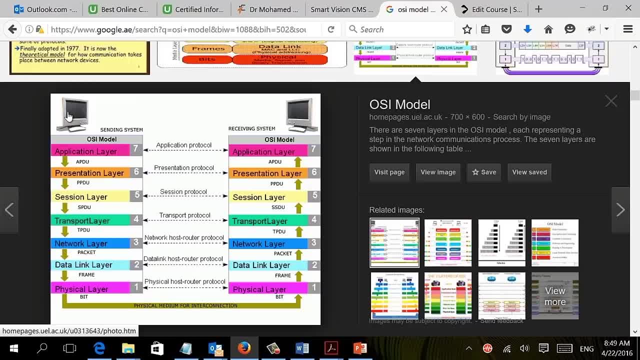 How this mail will be sent. So if he's sending an email to the other computer on the right side, He will write the mail And then click on send. Now the mail will not be sent the same way It's has been sent. 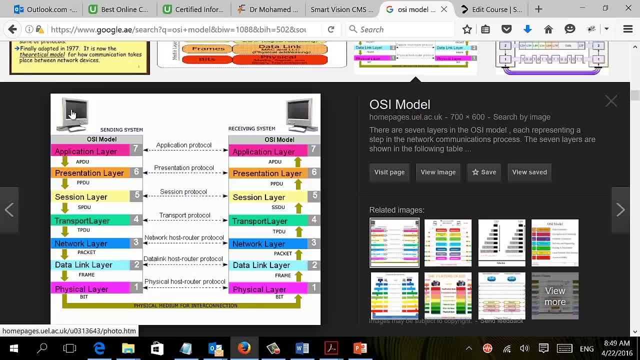 I mean it will be divided to something called packet And it will go through seven layer and each layer will do something to this packet. So the mail that I'm sending from the left- left side will be converted to a packet, And I'm going to show you how the packet look like. 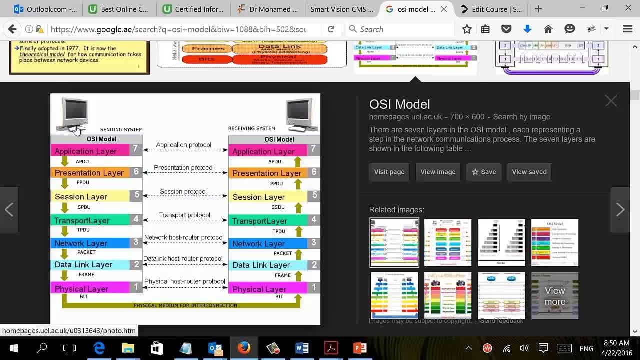 Just you know to be aware of what I'm talking about. And it will go through seven layer Before send to the other computer And each layer will do something. We have the application layer and the presentation layer. Both of them, mainly, are responsible to write on the packet. 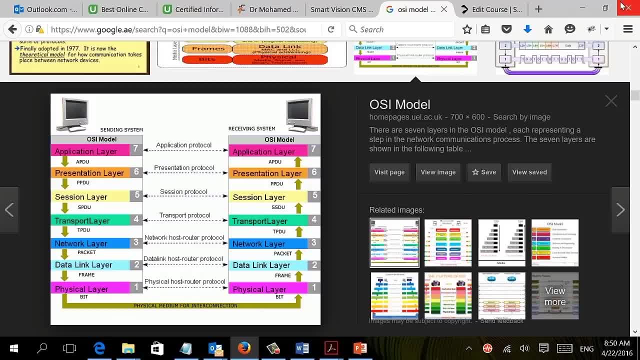 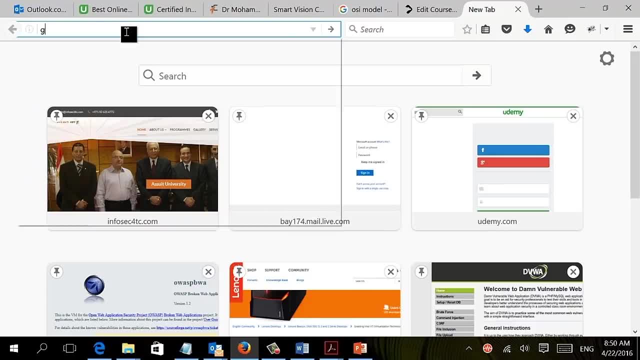 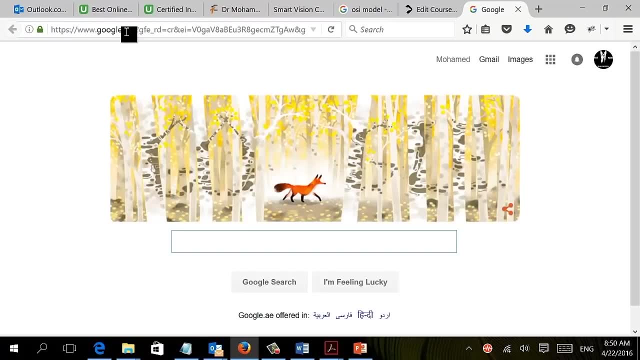 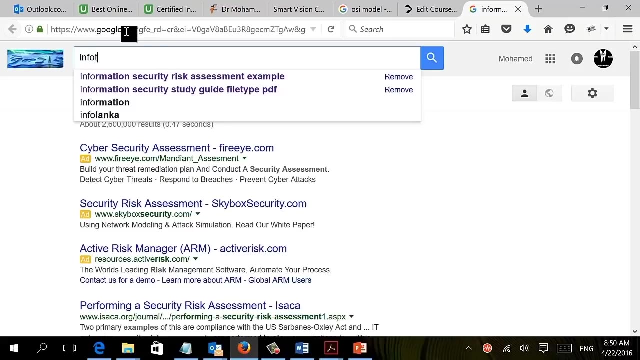 Because actually this packet of information is consist of two parts. Let me show you how it look like. It's consist of a payload and a header, So let's go to our main friend, Google, And let's see the information Once we finish this module. 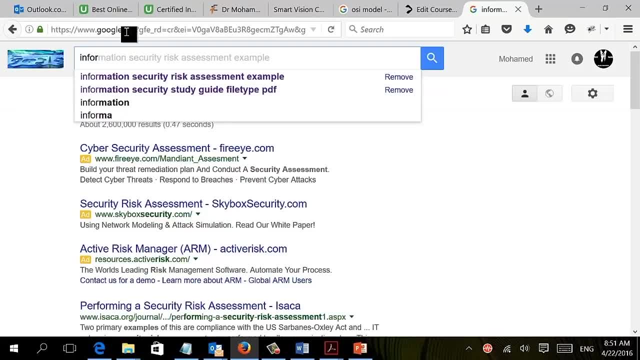 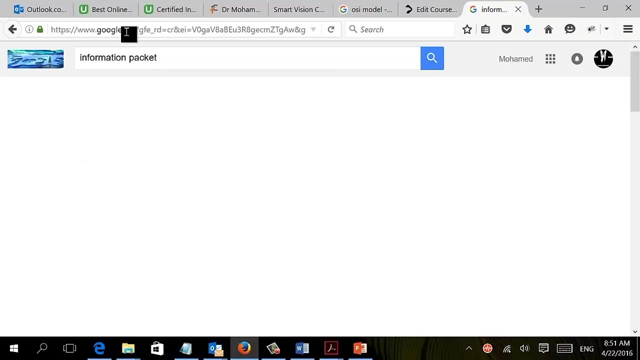 I'm going to open for you the Wireshark And I'm going to show you how the packet look like That are moving inside the network, So information packet. So the packet consist of two parts: The part that we call the payload and the header. 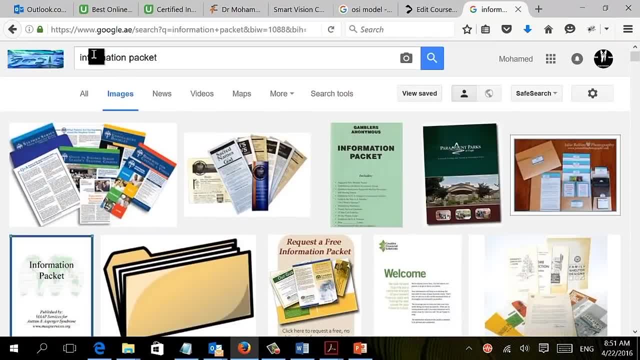 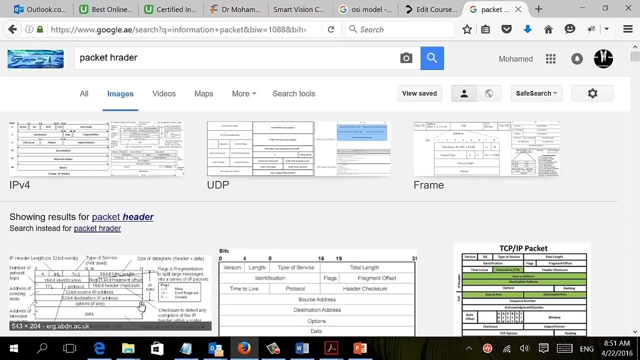 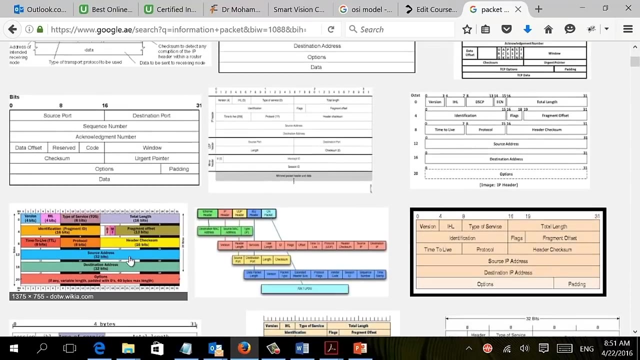 Oh, I got the wrong one. Ok, Packet header. Ok, So this is how the packet look like. Ok, We have a payload And we have the header. The payload is the information itself And the header is the inside or above the packet. 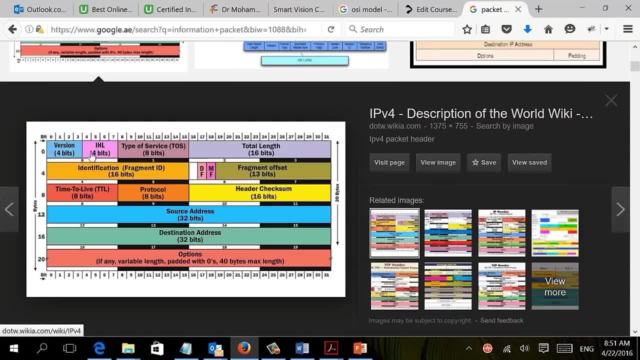 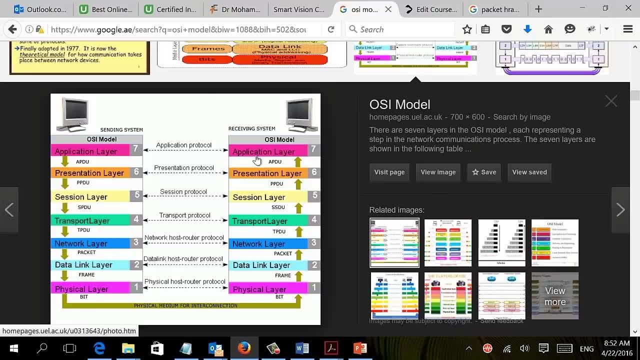 And has all the information for the sending and receiving. Ok, So the point is, As I was saying, I was explaining: Whenever someone is trying to send something, It will be transferred to the packet That consist of two parts: Header and payload. 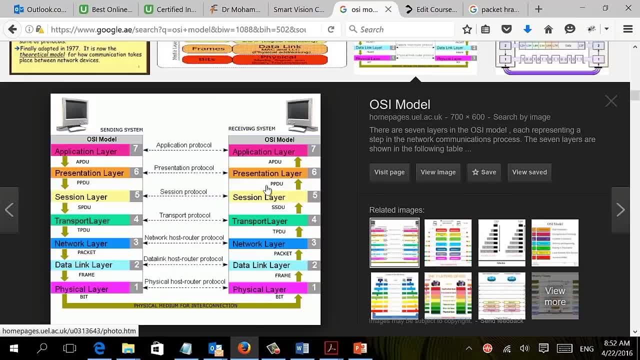 And you have to go through seven layers And each layer will write something inside the packet. So, for instance, Application layer and presentation layer, They will write inside the packet The type of information inside the payload, So when it sent to the other side. 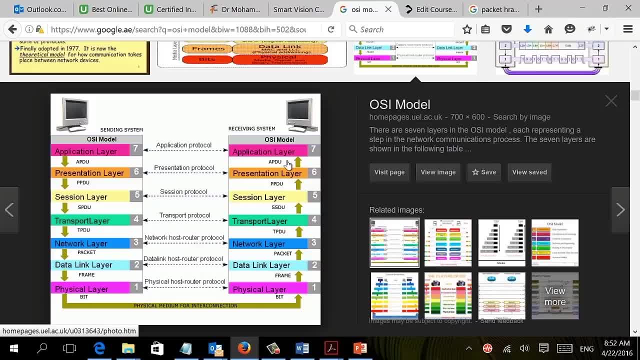 He will be able to recognize what was inside this packet. Was it a word document? Was it a picture? Something like that? We don't give that much attention about those layers, But we need to start, Or the important layer, Start from the session layer. 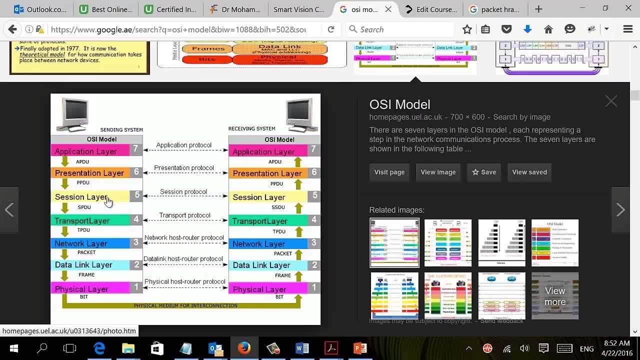 Session layer has full responsibility To Establish a session with the other side. He have to choose From on which port this information will be sent. And port, for people who is not aware of that, Is the logical communication channel Between the two computers. And how many ports do we have inside our system? Sixty, five thousand and five hundred and something. And you can check your port By going to the command line And type net state minus an. It will show you the open port on your machine. 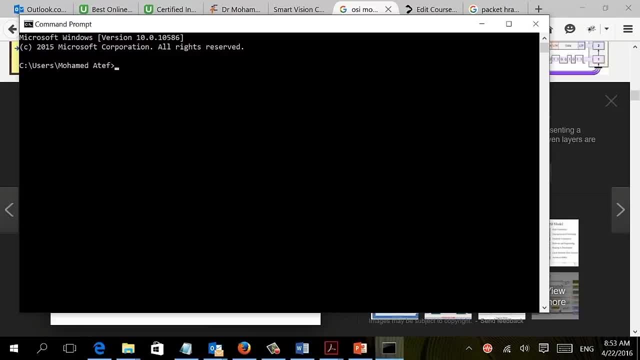 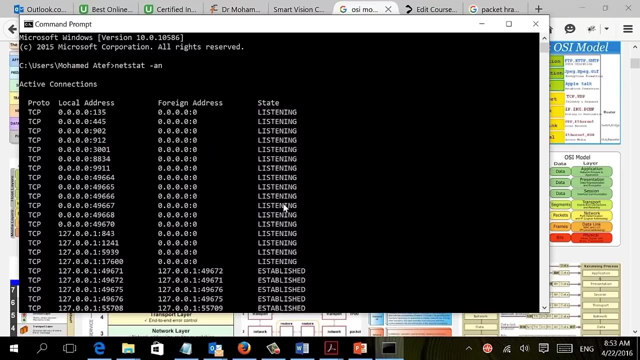 And each port is using which service, Or each service is using which port. So if you type net state minus an, It will show you all the ports That you have opened on your machine. Those ports are opening And if they are listening. 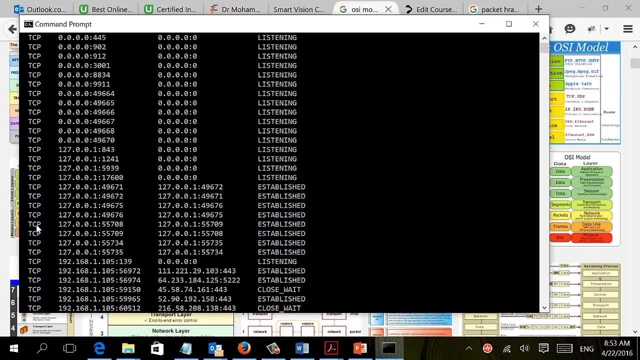 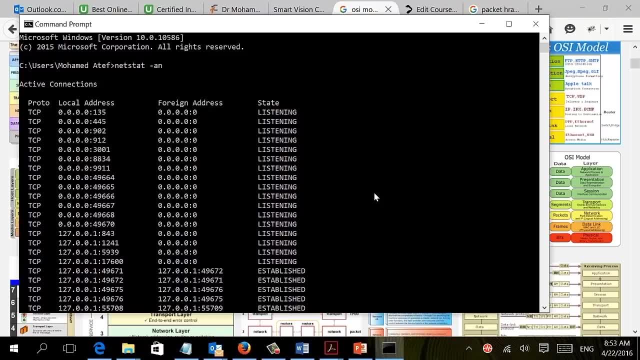 Or if they are connecting to someone, And it will give you the foreign address And so on. And ports usually are divided to different categories. By the way, This is a logical communication channel. It's not physical. I mean I cannot open the machine. 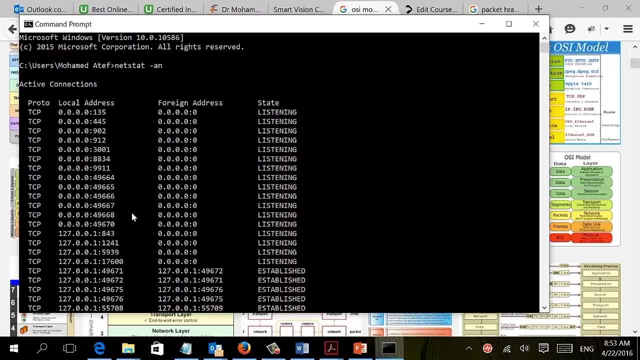 And show you where is port 80. Or port 21. Or port 23.. Those are logical communication channels. Who is responsible for establishing, Choosing the port And establishing the connection? And after finishing closing the connection, Is the session layer. 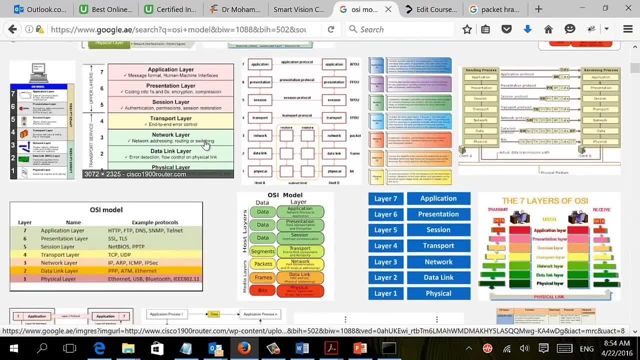 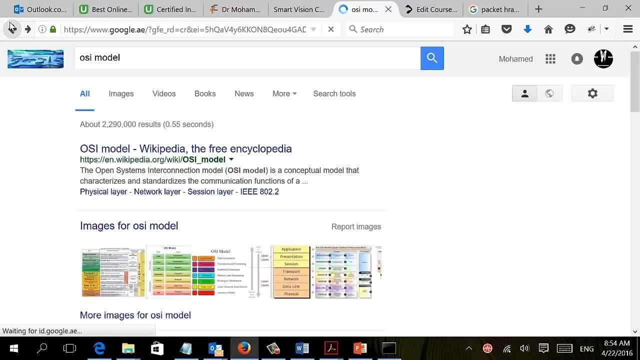 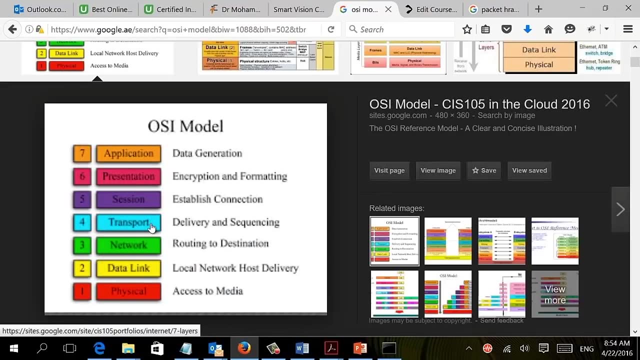 Then information will be sent. What is the Information will be sent to the Transport layer. Now the transport layer Has for function to decide This information will be sent. how We have two different ways for sending the information We have. 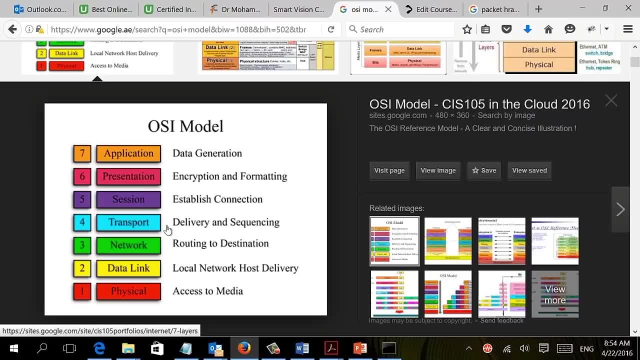 Connection oriented and connectionless. Connection oriented means Information needs to be sent And a confirmation needs to be made That the information has reached the destination. So you never received an email. That is missing some words, Right? Did you ever open an email? 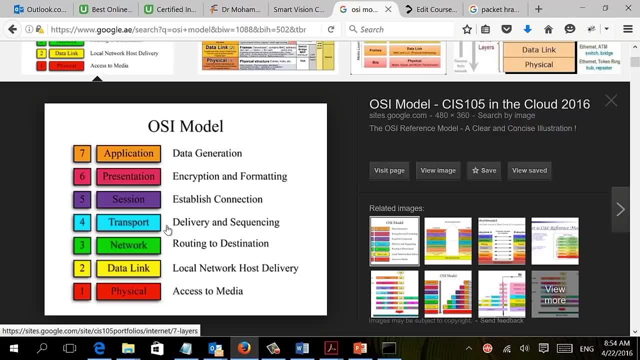 And it was missing some word, Because those words actually are Used to be backed And maybe they get lost During the During the way, But You never received an email That they are missing some word Or open a web page. 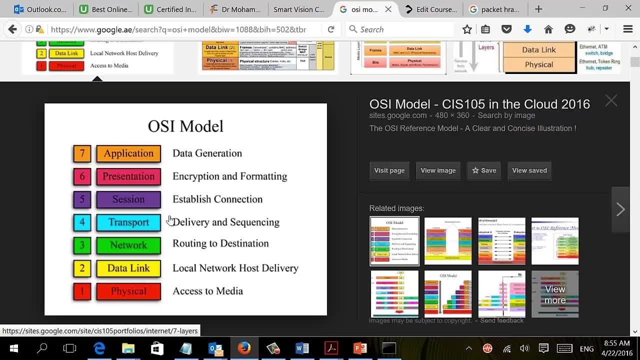 That is missing some word, Because the way The OSI model is sending the information That it guarantee That the packet will reach To the destination. And how can it do that? We do that using Two different protocol Protocol called TCP. 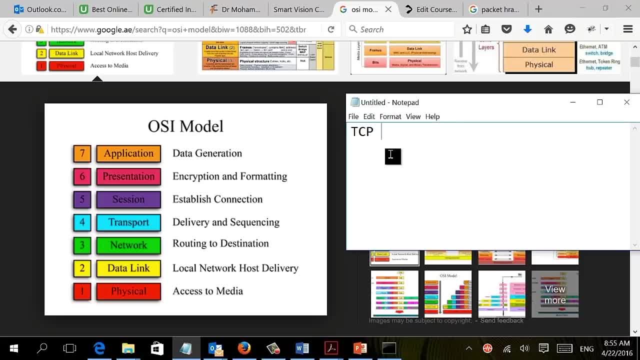 And another one called UTP, TCP and UDP And UTP. This is how it work. Assume that You are sending an email to someone, So once he Email will be going to the applications And presentations and sessions, Then it will reach the transport layer. 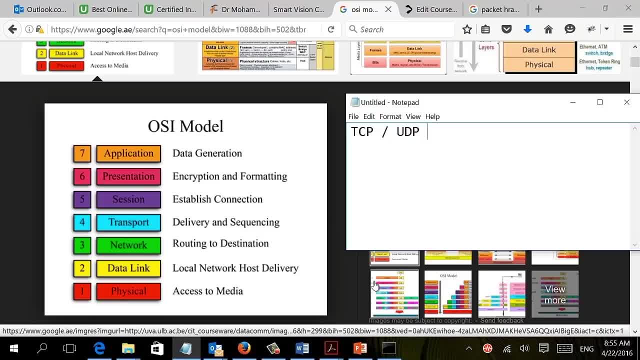 Transport layer will check the payload. The content of this packet, It's email. Email it's a TCP, I mean need to be sent With a guarantee To reach the destination. So what he gonna do, He gonna write on the header. 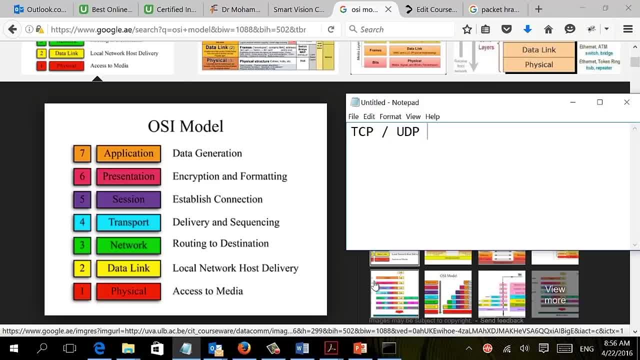 Of the packet, A sequence number. So assume that your email, When it has been converted to packet, It has been Converted to four different packet According to the size, So he will write on the header: This is one from four. 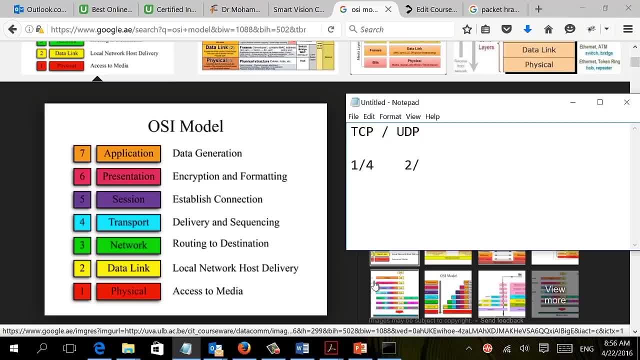 On the first packet, Then This is two from four On the third packet, Then this is three from four On the first packet, And so on, And then he will start sending A one packet And wait For confirmation from the other side. 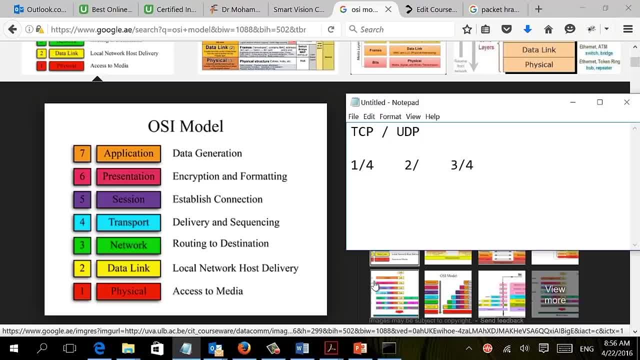 That he received one packet, Then he will send the second packet And wait the confirmation That he received the second And then you set the third. What if he didn't confirm The other side Didn't confirm that He received the third packet? 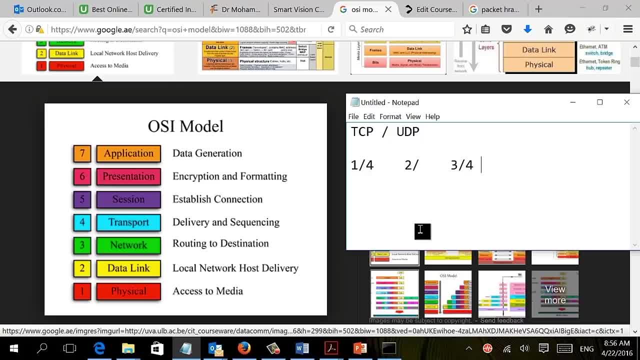 packet, he will send it one more time. that's why you never receive an email that is missing anything, because the email is sent by a tcp. so once the email reach the transport port, he will check the content and he gonna know that this is an email and he will flag this one with a protocol tcp. 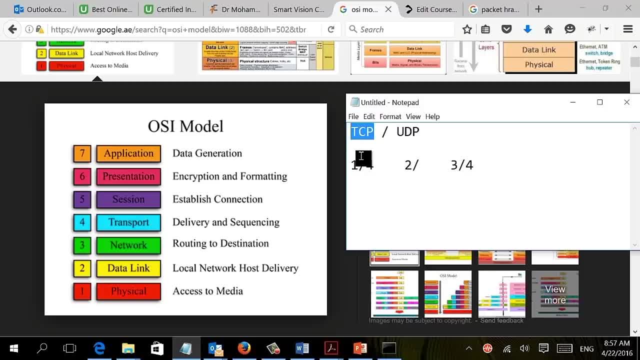 saying: could you please send this information using a tcp protocol, where all packet need to have a sequence number and you need to guarantee that it reach. on the other hand, some traffic cannot be done this way because of the amount of traffic, especially the streaming traffic. so voice. 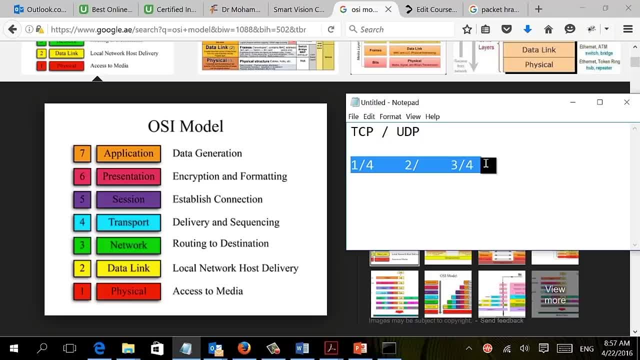 and videos. those are a huge amount of traffic. he cannot keep sending packet by packet and wait for confirmation. it will take like forever. so what will happen is if the information that was sent was a voice, i mean you are talking over the internet or video or something like that, and it. 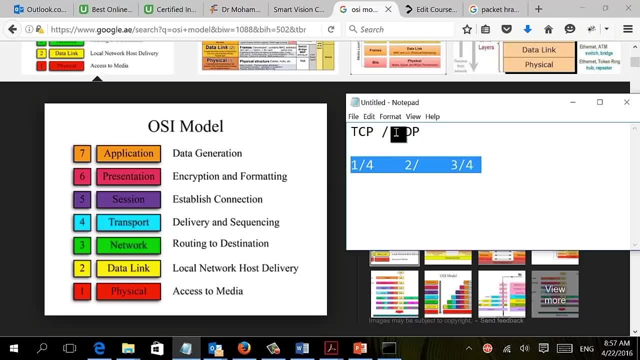 will reach the transport layer, he gonna see that this is streaming and he gonna decide: you let's send that by udp because it's too much packet and i cannot send it one by one. and what will happen is, once the transport layer decided that it will be sent by udp, the information will 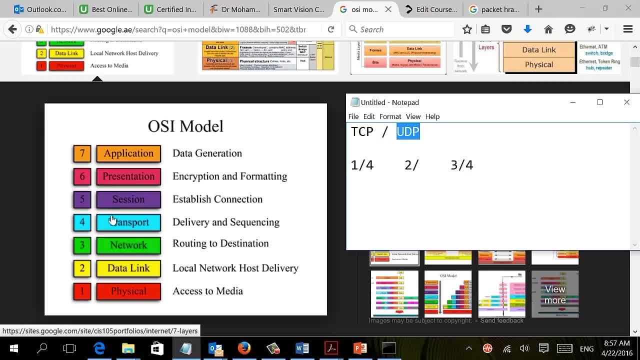 be sent, all the packet will be sent and whatever reach, destination reach and whatever will not reach, it doesn't matter. so you are sending and you don't follow up. that's why when you are doing a skype conversation or any voice over ip, sometimes you are, some word will be missing. those are packets. 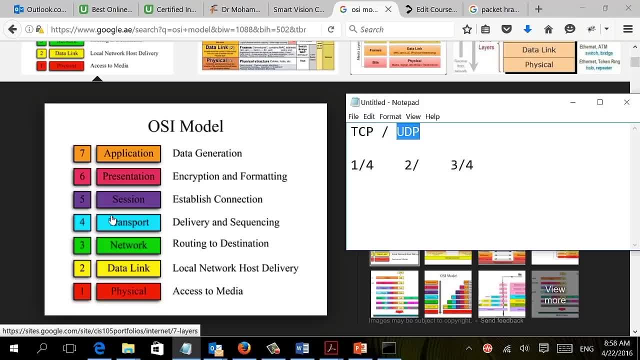 that has been dropped and not recovered. so the transport layer are the one deciding what to be sent by tcp, which is oriented, and what would be sent with udp, which is connection, uh, less. then the information will be sent to the raw network layer and this is actually, i mean, the 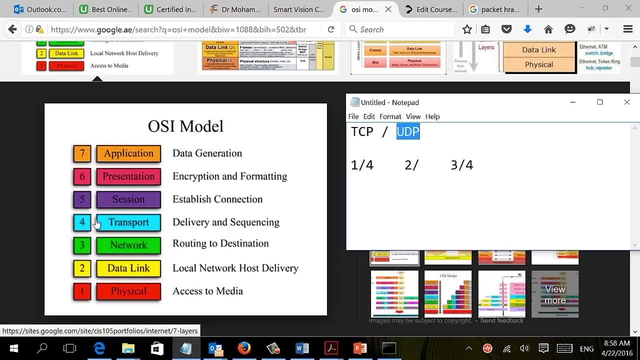 fourth layer, seven and six and five and four. those are inside the operating system. the operating system are the one who's doing that network layer has for functionality to addressing. i mean it will put in the pack header packets the ip of the center and the ip of the destination. so you're gonna say this packet is sent from this guy to. 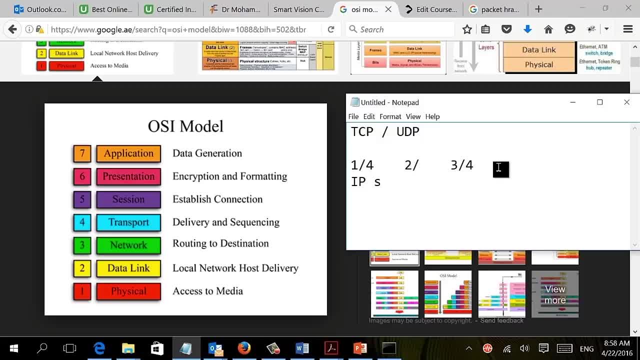 this guy. so it will be a sender and receiver ip and who is doing that? this is actually done inside the uh router. the router is the one who's putting the ip address for uh source and destination and router usually use protocol right: rip, eigrp. sorry, those are the protocol for addressing rip and 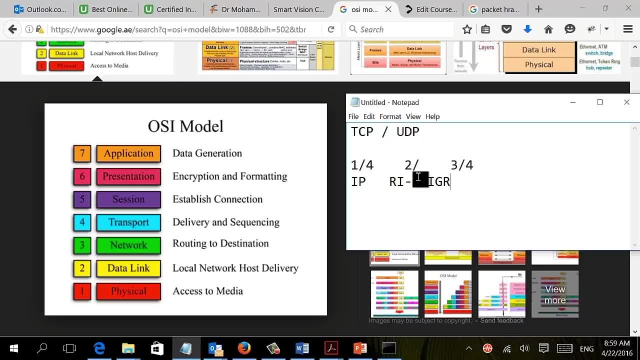 e i g r p and o s p f- all of those are routing protocol and, as i told you, sorry, sorry, as i told you that you need to memorize the those protocol on each layer. what protocol are working? sorry, e i g r p. then it will be sent. 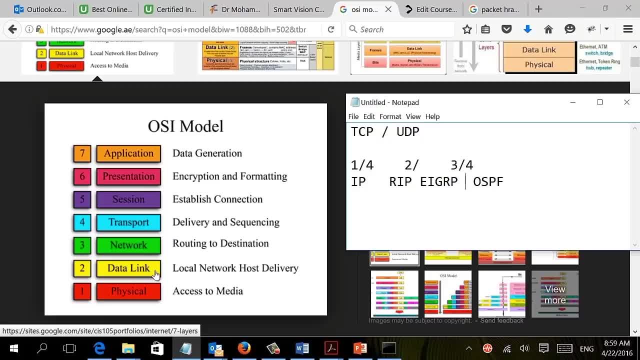 to the data link layer and data link layer. it's only one, also an addressing, but actually it's putting the address for the source and destination using the mac address and not the ip. so both network and data link are using the mac layer mac address. both of them are using the. 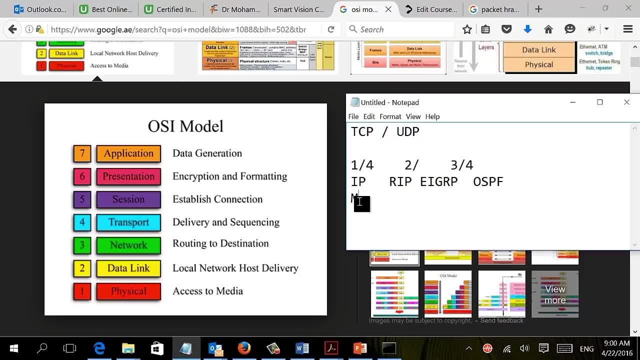 both of them are working as a addressing layer, but one of them is putting addressing using an ip and the second one is using mac address or physical address, and then everything will be sent to the physical, where it will be transferred to binary signals and it will be sent over the wire. so this is the osi model now. 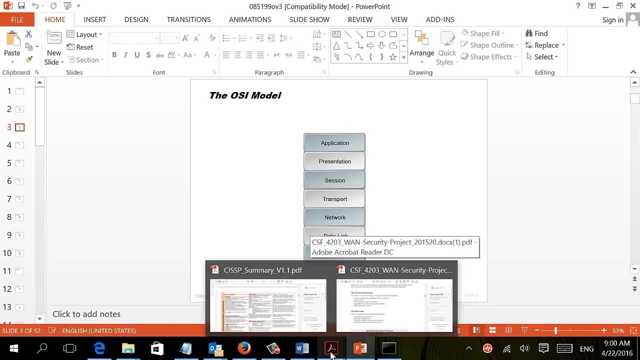 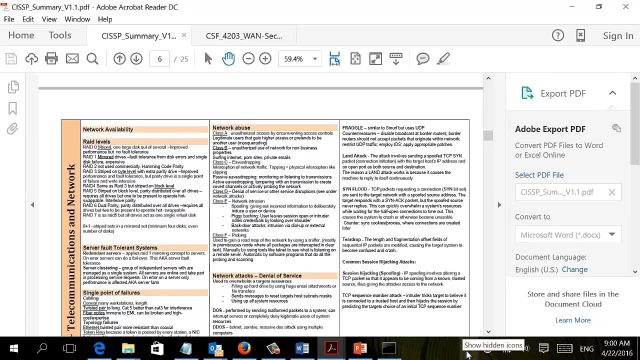 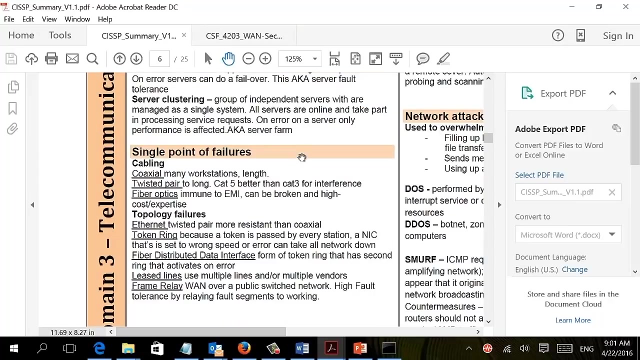 it's very, very important. i know that most people will be aware of this discussion, but i just need to point what exactly you need to be memorizing for this lecture. so if we just increase the size of this file, okay, so let's take the layer. i know the the sunflower is not going with same order. 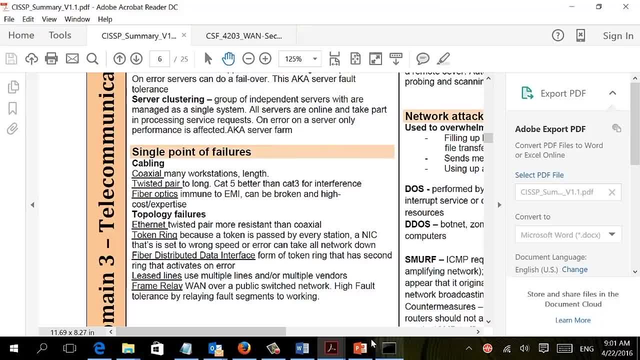 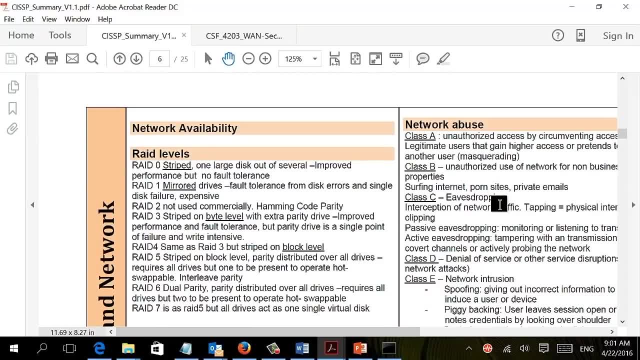 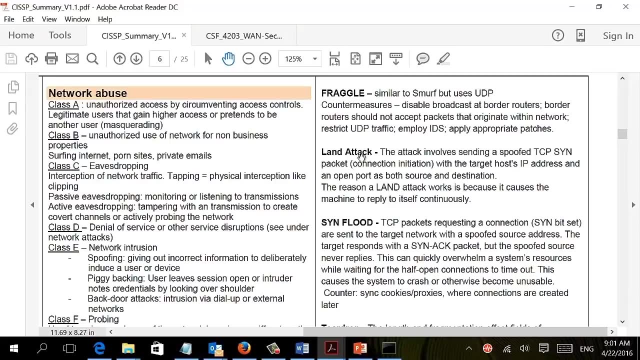 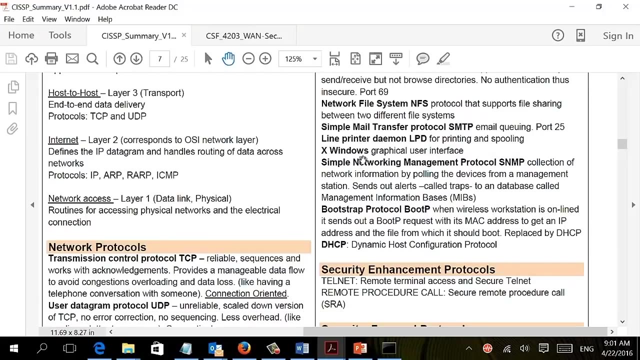 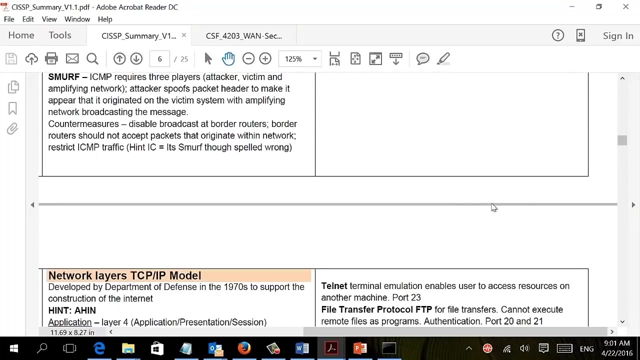 but i just need to point to the things that you need to consider for the exam: network radius: we'll talk about radius we already spoke about, but we'll talk about them one more time. text: yes, this is the layer. okay, but this is the ip layer. what about here? 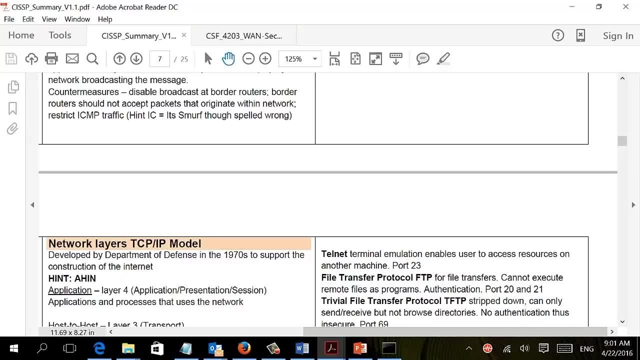 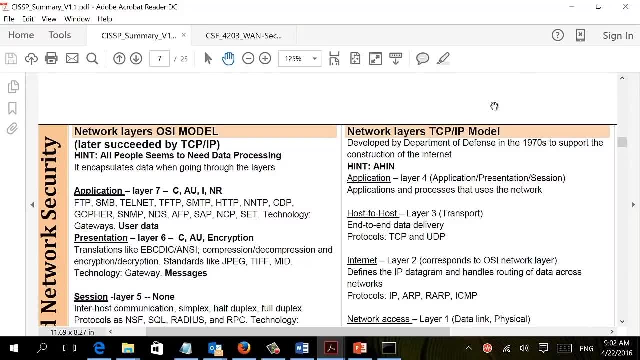 okay, even if i'm not able to find it almost probably to be here. yes, osi model. so, as you can see, it's explaining every part. but the point here is not the explanation, it's you need to know each one which protocol are working on. this one, okay, and he will not ask for those where protocol 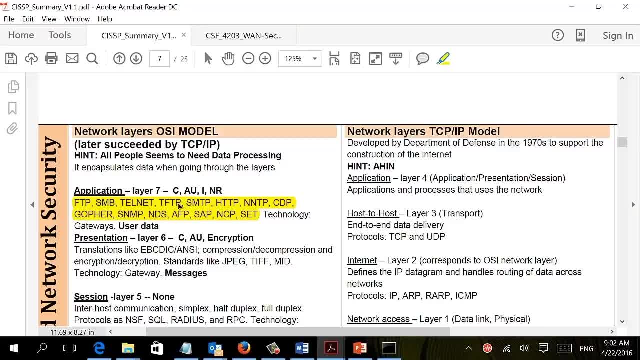 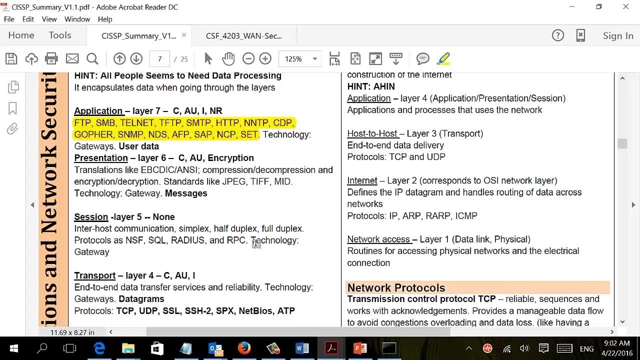 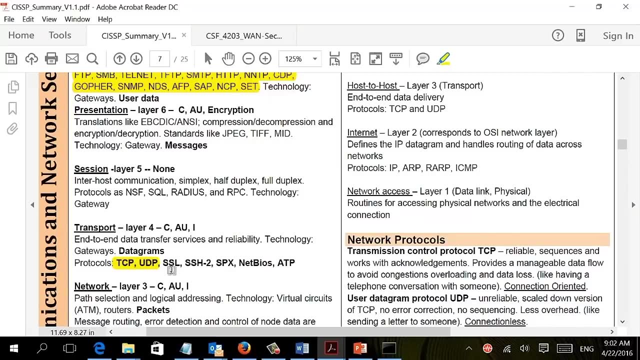 like cdp, sysco discovery protocol. he will ask about http, telnet. those are applications, so it's working the application layer, while for instance, the radius, the rpc, this is working on the station layer, while the tcp and udp is one we just explained inside the transport layer and including 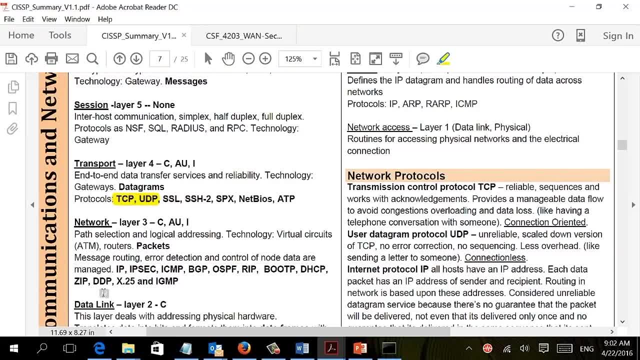 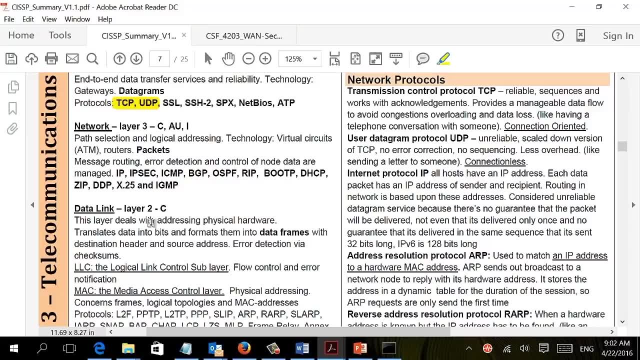 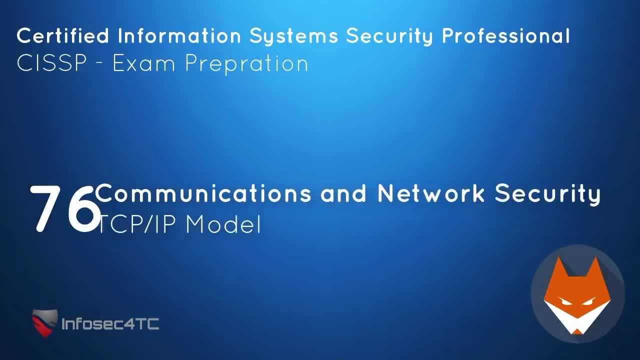 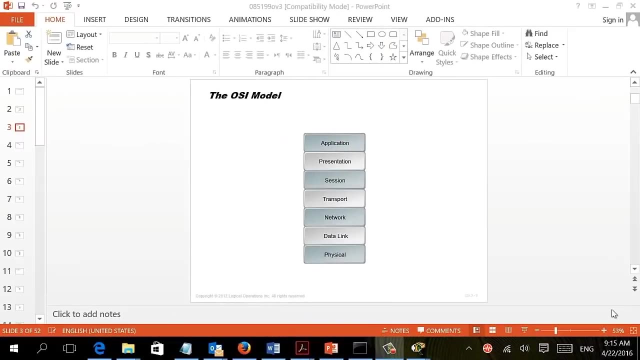 an ssh2, so for each one you're going to need to memorize the protocol which are working on this layer. so on the previous lecture we explained the osi model and different function for each layer and the protocol who's working on each layer, and you have to memorize this order. you know, and you have to put some like keywords that will help. 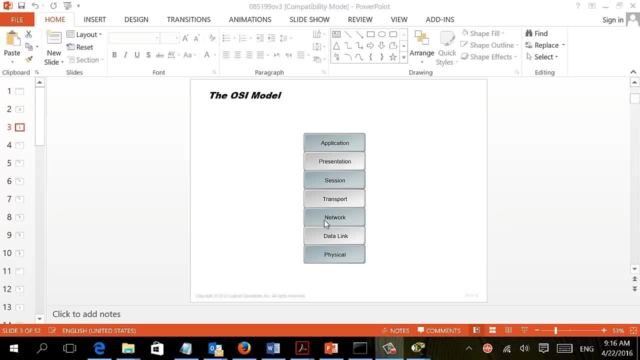 you, like all people seem to seem to like. i don't know actually what you can use here, but data processing. so you, you need to do something to memorize the steps. except i don't believe he will ask you about which layer is after which layer. now the reason, not an older model, that was. 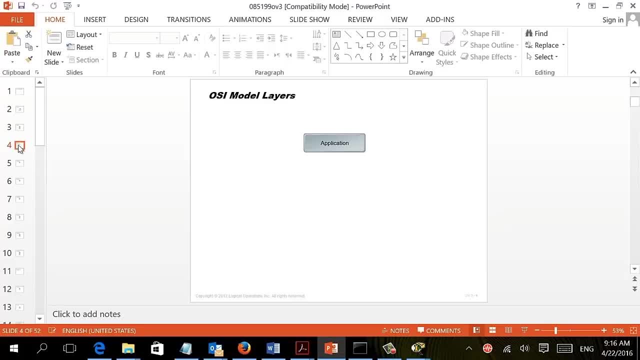 used on the internet and this layer actually was called the tcp ip stack and it's very similar tcp ip model, except it's only four layer and it matches the osi model. that's why you can use the osi model in our machine inside the uh tcp ip uh model. so the osi model, it's only four layer application. 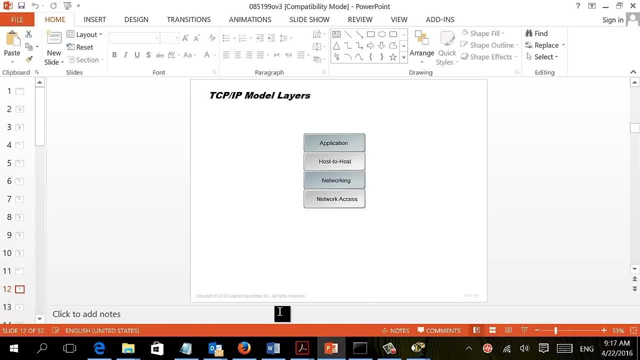 host to host network and network access and they are matching each other. i mean, you know, they are similar to each other and they can communicate. so you can communicate between osi model and tcp ip, and this is, i believe, the slides that you need to memorize, which is the protocolfort. 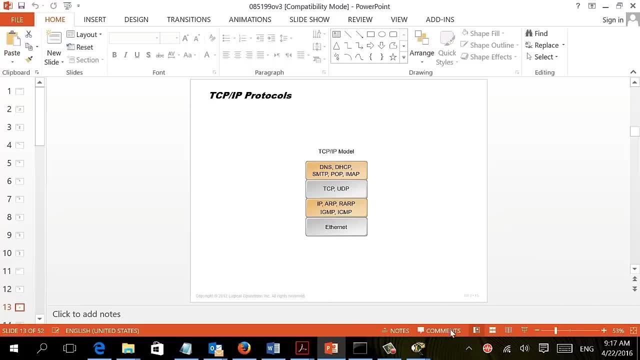 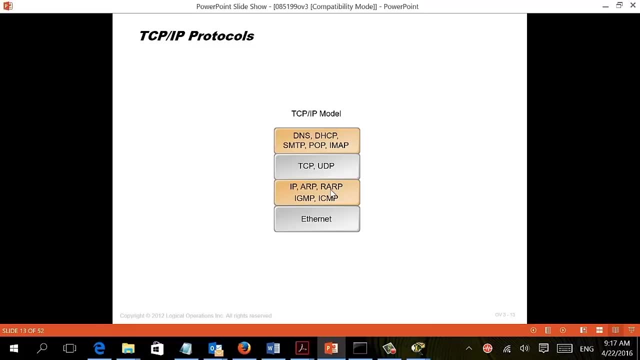 equals that working on which layer? similar to the previous one, except here it's in just one slide. so what is working on the first layer, or second or third offers? so this is how the protocol from the protocol works, for there each studies Eğer the layers. I'm sorry. the different models are explained, and what do we need? 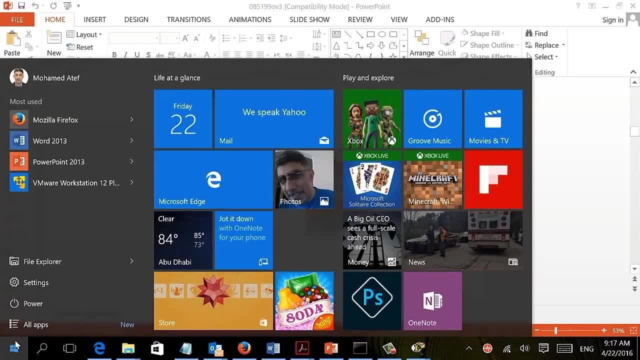 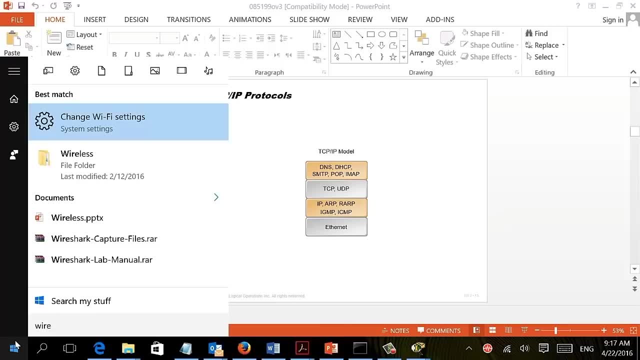 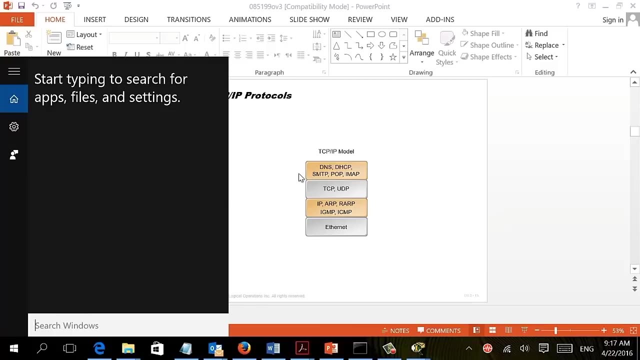 to know about them. so let me try something. I hope I have the program just to show you wire. I'm afraid I don't have, but you can download wireshark. it's a free application and wireshark- if you run it, you'll be able to see the packet. 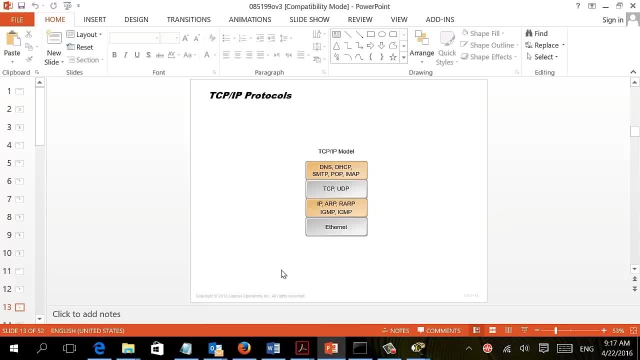 and the payload and the header as well. so this is the introduction part into the network. the next lecture we will be talking about the network architecture and different network devices. it will be a long lecture that we may have to divide it to two different part. so let's talk about network architecture and 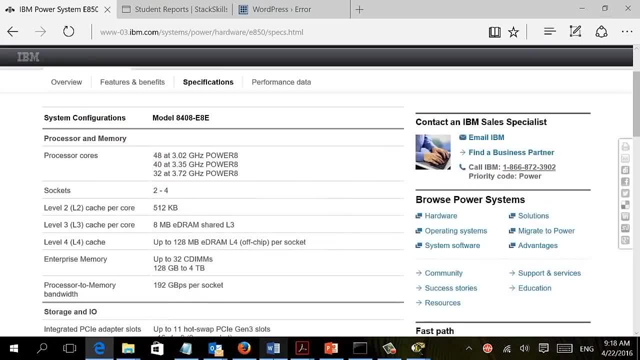 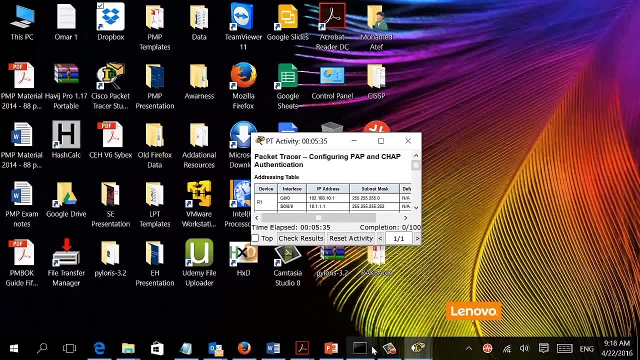 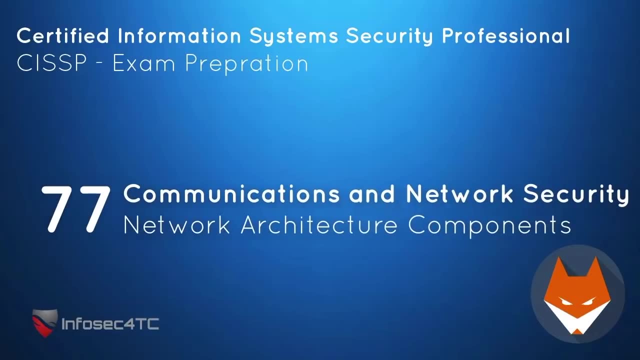 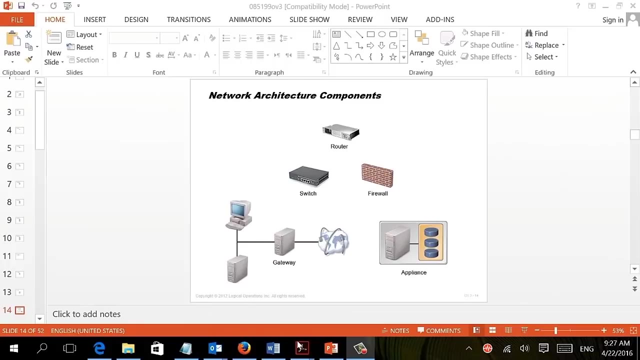 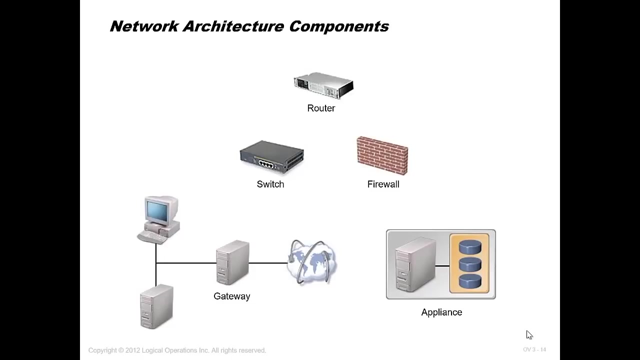 different kind of devices. you. this lecture will be a little bit long and maybe will be divided to two or more lecture, because we will be talking about the network architecture and network and network components and will be explained in the next lecture. so thank you for watching and see you in the next lecture. 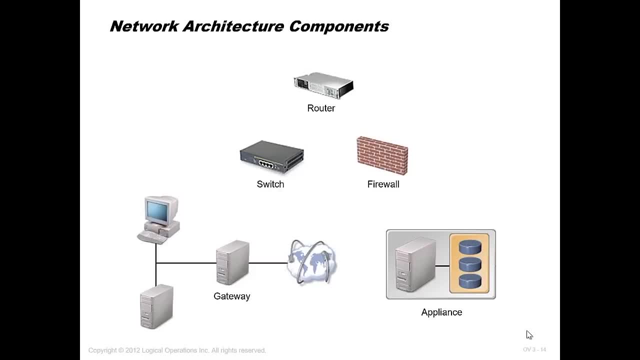 explaining how those different devices are working and the different terminology related to them. so please bear with me because actually this is an extremely important part now to be able to build the network. what do we need? we need clients- computer or smartphone or tablet or whatever client- to connect and 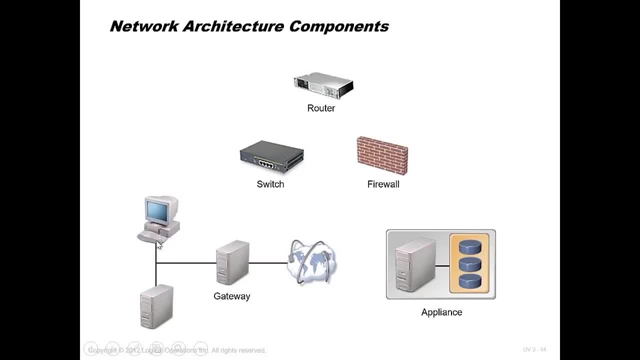 we need to have a media, which is a type of cable, and we need to have a switch switch. so let's start by switch the switch. what is the functionality of the switch? I mean, we are connecting all the machine with one central point. this is called the switch, and before the switch we used to have a device similar to the. 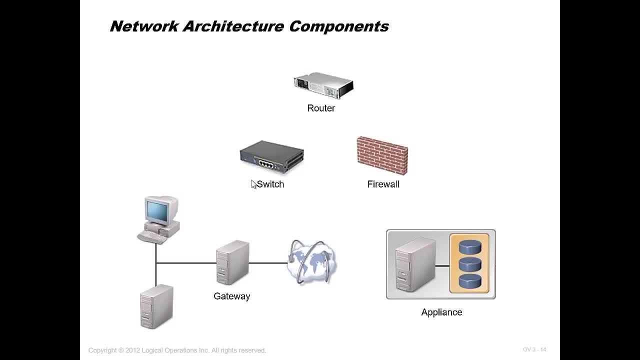 switch, but different in their functional functionalities. the device that exists before the switch used to call the hub. and what was the problem with that? I mean assumes that you are connecting five, six machine with the hub, how the hub used to work. so when computer a are sending information to any other, 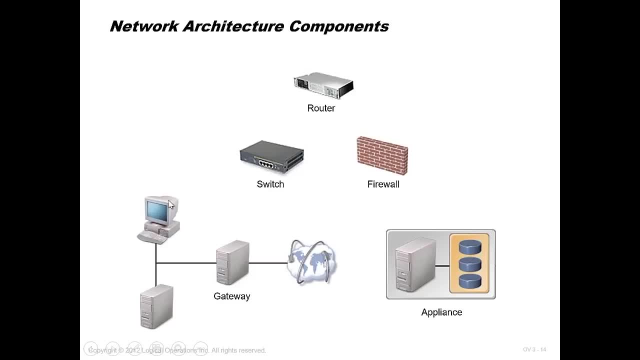 computer inside or connected to the same hub. this information will be sent to the switch and the switch will be sending them to all the machine connected to its port, because he cannot distinguish the machine from each other. so the problem with the hub was that it work based on broadcasting. he cannot distinguish which machine, so 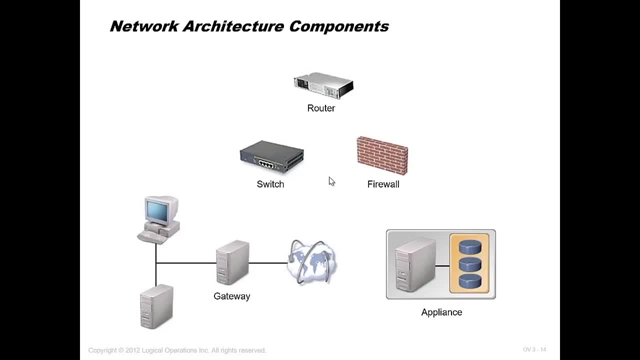 if one machine is connected need to send information to another machine. he will send to all the machine connected to the hub because he cannot know which machine are the destination. switch are more smarter than the hub, so switch actually had something called the MAC address table or sometimes called the cam. 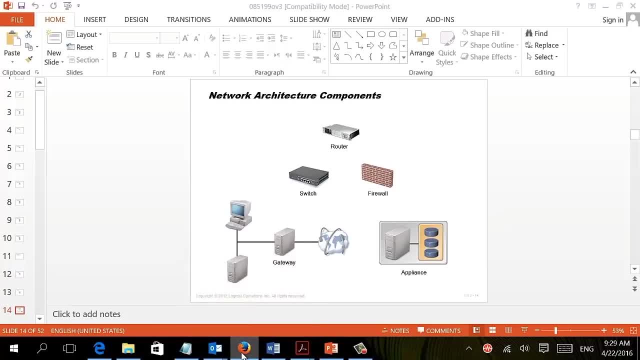 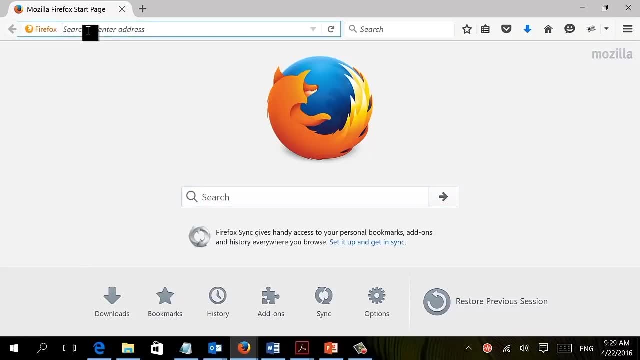 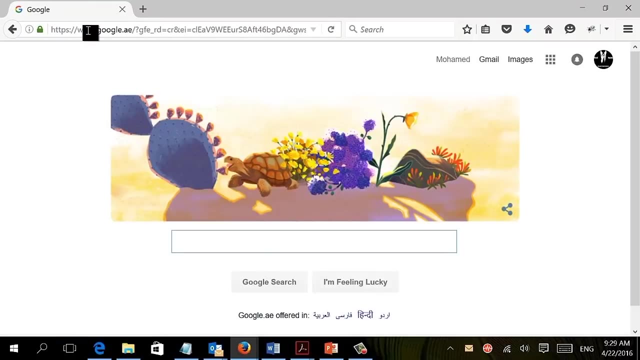 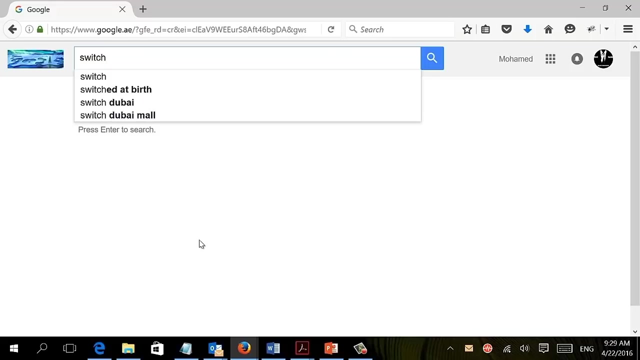 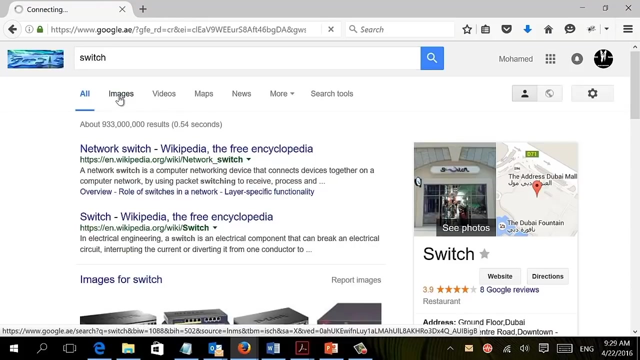 and the way the switch is working, let's see how it work. so now it's important to understand how it work, because if you know how it work, you will know where is the weakness of the device. so let's talk about the switch. switch and, as we agree, switch are a little bit different than the hub that he holds. 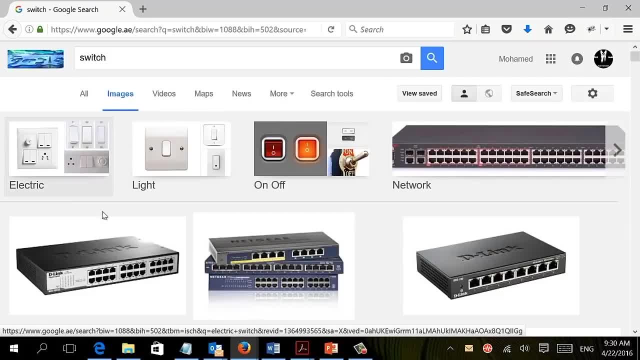 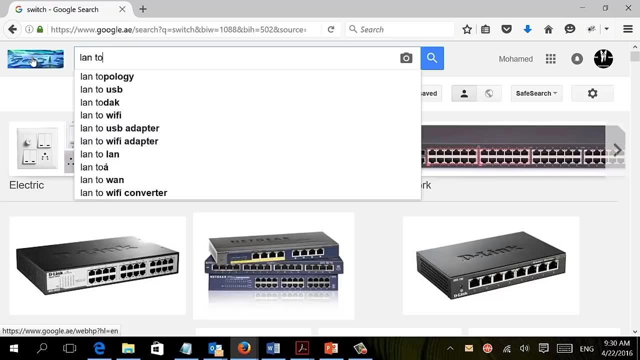 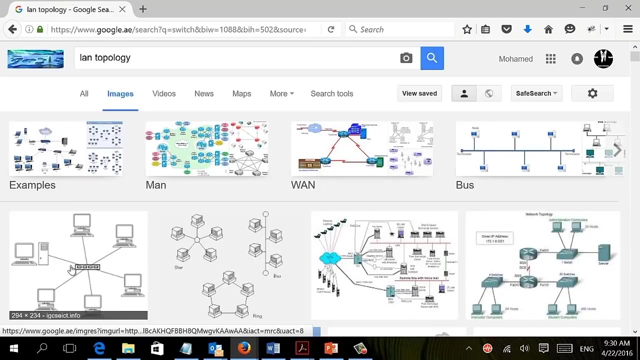 something called the MAC address table. so when you connect some machine to the switch, he will be, he will identify them based on their physical address or Mac address table. so let's open the land topology to be able to explain that in a better way. so we have some machine connected to a switch. now, as I told you earlier, if this was a hub, 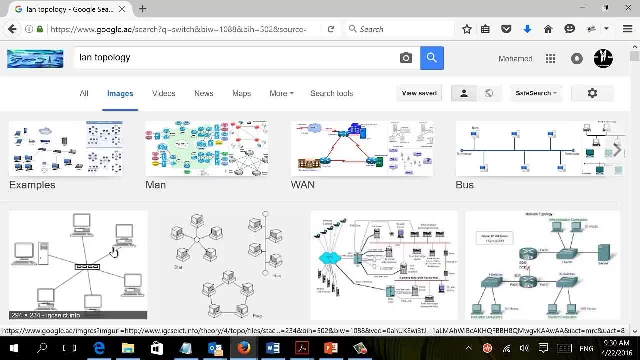 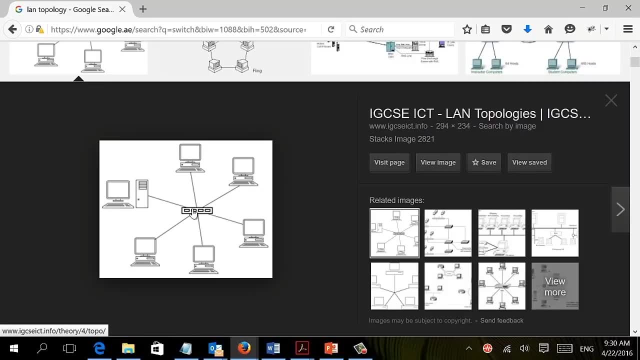 what happened is, when this computer needs to send information to this computer, he will send this information to the hub and hub will broadcast to everyone. while inside the switch things are a little bit different. so when you connect some machine to the switch, he will open or he will. 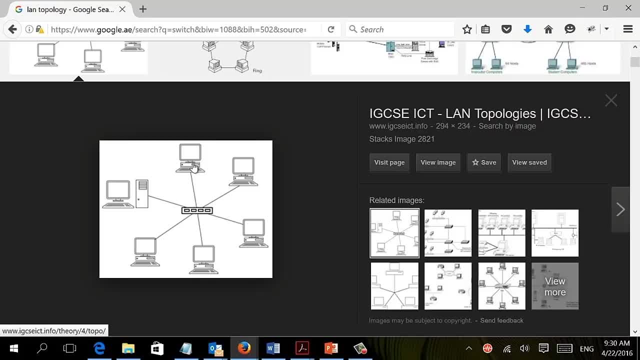 create something called the MAC address table or cam, and he will write down the each computer Mac address and to which port is connected. so if this computer need to connect to this or send information to this computer, it will be sent to the switch and switch will check the MAC address and he will. 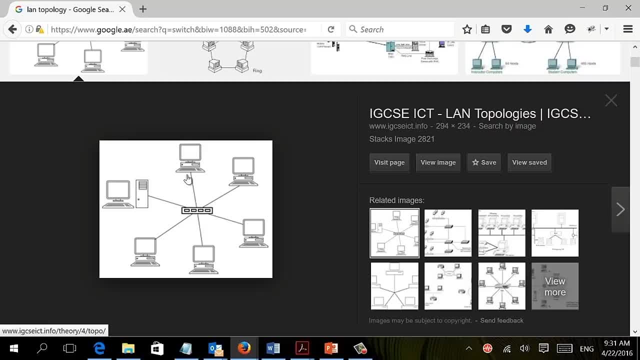 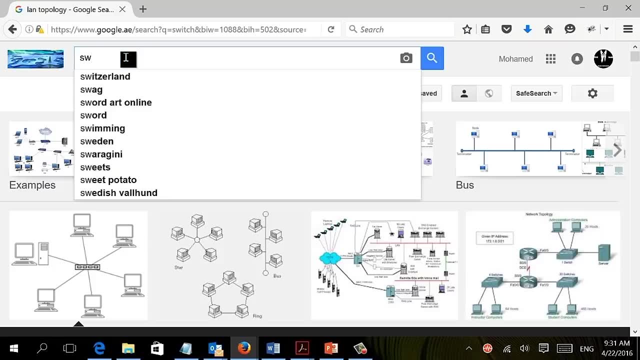 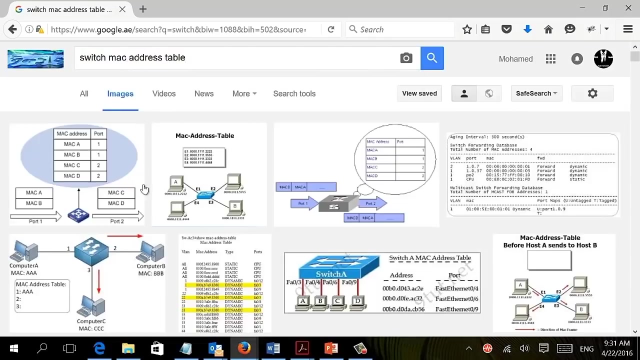 check on which port it's connected and he will send the information so it doesn't have the problem of the hub. let me show you how the MAC address look like: switch Mac address. okay, so it was actually more smarter than the hub. so this is how the Mac address look. 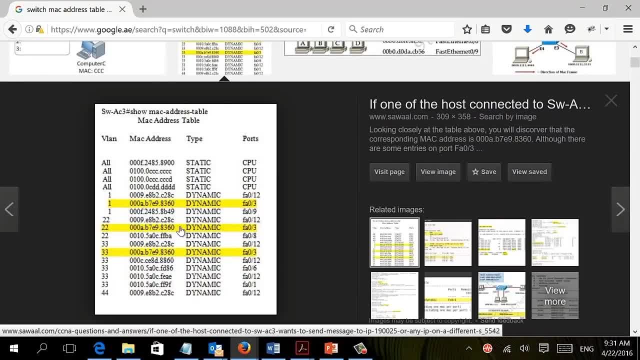 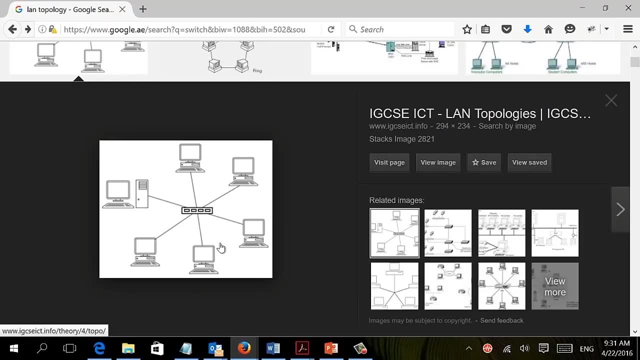 like you know, you have all the MAC address and on which port they are connected. so this one is connected on port f012 or f012. so by doing that switch are able to not prevent broadcasting, which is, you know, have its own problem in security, and so 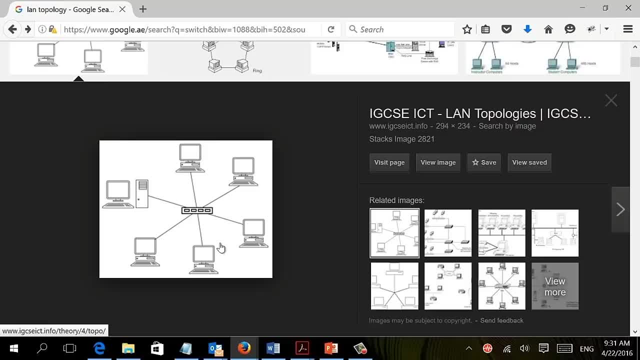 on now. what is the problem with the switch and why the switch, which is a layer 2 device, it's very easy to compromise. now, if you know how the switch is working, you'll be knowing where is the vulnerabilities are when you get a brand new switch. the MAC address or the cam has any information. 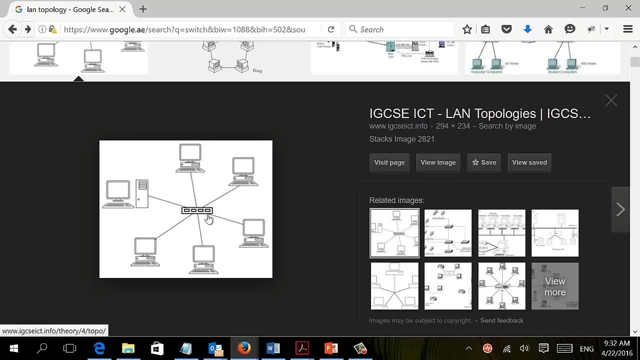 it will be blank how the switch are building the MAC address from the traffic. so if this computer send information to this computer, he will send to the switch and switch will send to everyone asking which one hold this MAC address and one of them will will be replying back and, to be more precise, 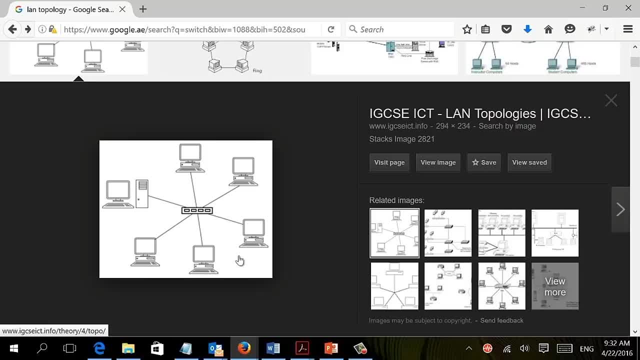 let's assume that this is a new network. I got five or six machine and I bought a switch and I connect them. so the switch right now are empty, doesn't have a MAC address there. now the thing is, the switch are a layer 2 device can only recognize machine by their MAC address, while 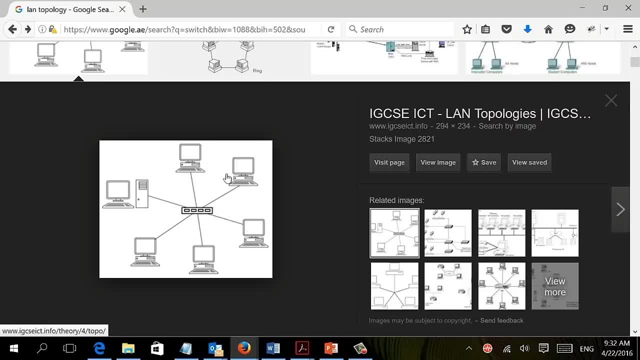 computers themselves. they are communicating using the IP. I mean if you try to ping from one machine to my machine, you are typing ping space, IP. so definitely there will be a problem here, because if you send the packet here and tell to the switch, could you please send it to this specific IP? he cannot. 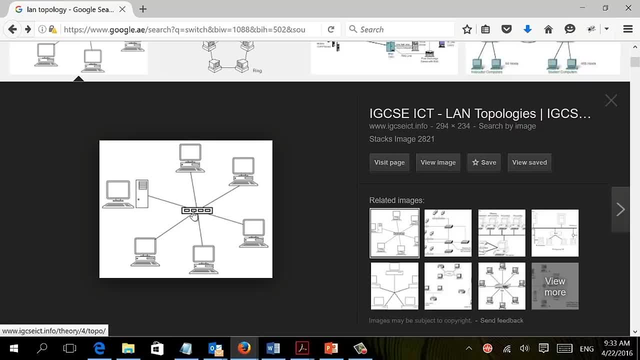 understand that even if you have some entry inside the MAC address table, he will not be able to understand, because switch are working according to MAC address and not IP. now, to be able to solve that, once the information on once the packet is a computer are send, a request to another. 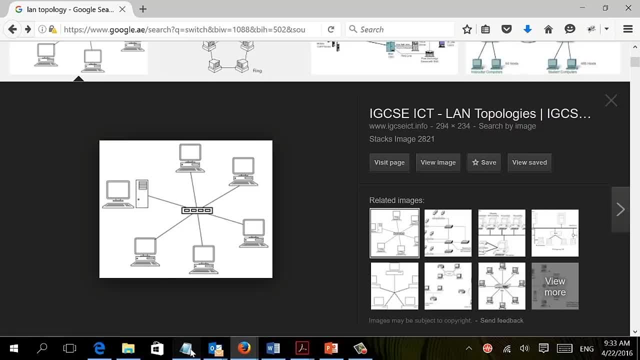 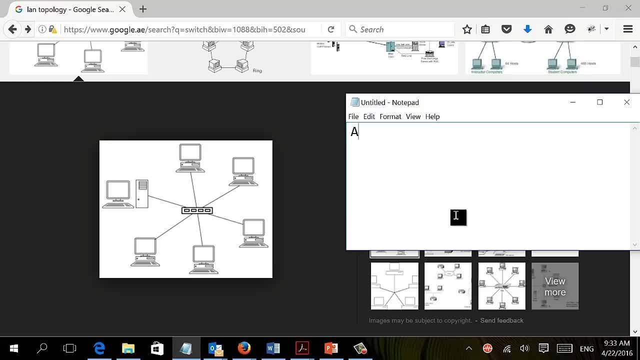 computer using the IP. the switch will. son will send, because this is new switch so the MAC address table doesn't have anything. he will send something called our request, our request, to all the computer except the one that he received the request from. so this computer wrote ping space 192.168.1.5. so the ping packet has been sent to the. 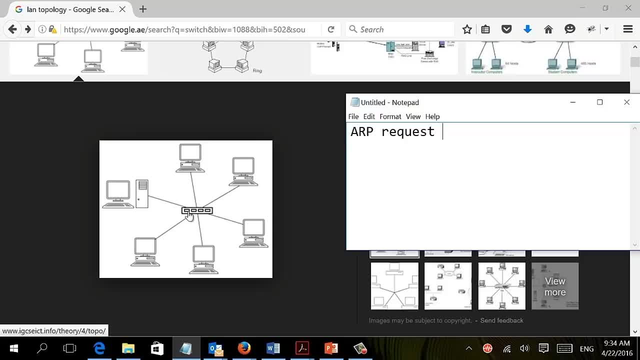 switch and the switch will. he don't know, actually, which machine holds this IP and he don't know even what is an IP. so he will send a request to all the remaining machine. it's called the ARP request, asking those machine guys which one of you have this IP and one of those machine. 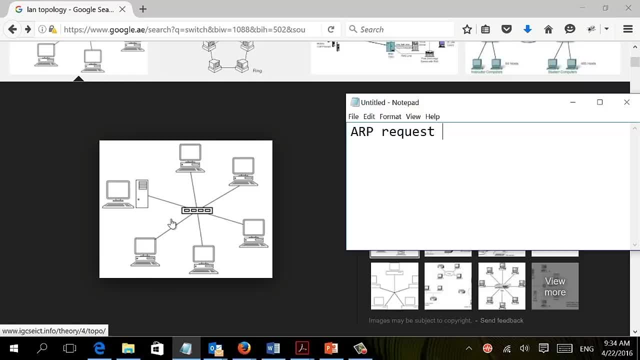 will reply back telling him I am the one who has this IP and this is my MAC address and based on that, he gonna put this MAC address inside he his MAC address table and next time when the computer send the request, he will know right away that this request need to be sent to this computer and the value or 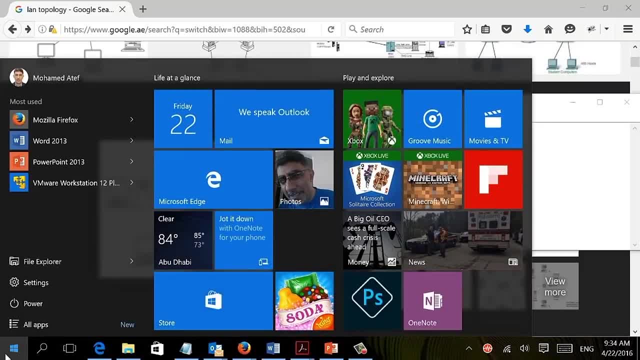 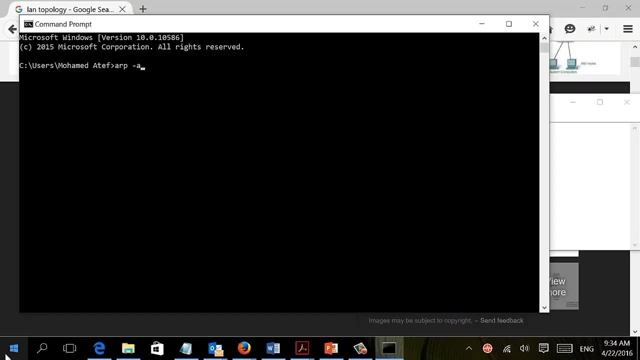 the MAC address of this IP will be kept on your computer. let me show you so. if you type cmd, for instance, ARP minus a, you will send all the ARP request that has been sent from the switch and what reply he received. so next time he can communicate. 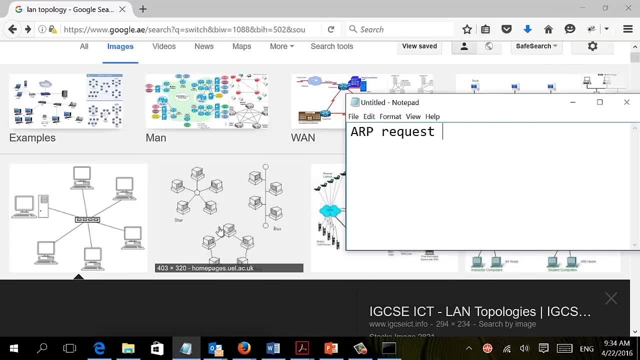 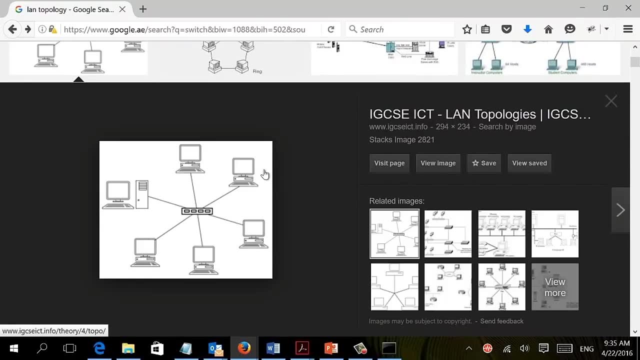 using the MAC address. the point is this: ARP reply or ARP request doesn't have any validation. so my point is: if this computer was a hacker computer and this one sent information to the switch going to an IP, and the switch will send the request to everyone, ARP request telling them, guys, which one holds this IP and if this is a hacker computer, sorry, the, it will reply back with something called the spoofed ARP reply telling them: yes, I am the one who has this IP. he's faking his MAC address, but no way that where you can check if this was a right ARP. 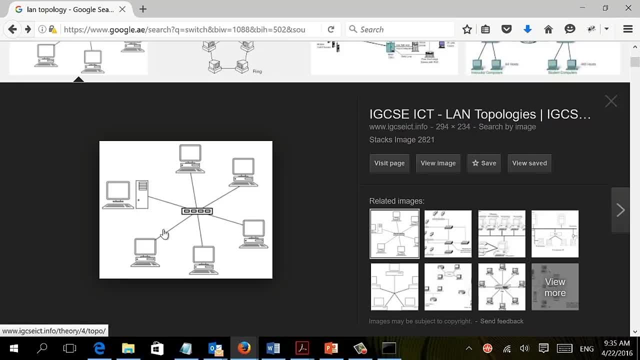 request or not. so the ARP can be manipulated. and you know those sniffing application are spoofing the ARP, are faking the ARP so they can fool the switch and they can redirect the traffic to them. that's why sniffing and man-in-the-middle attack 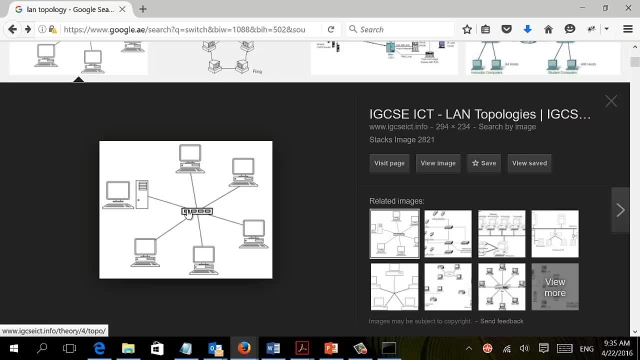 and those kind of attack are very easy to do because you are manipulating the switch, not the machine, even members. your machine is very, very secure than has all the layers needed, but you are working with a switch, are you, or you are manipulating the switch. so this is the problem with the switch: that the ARP or 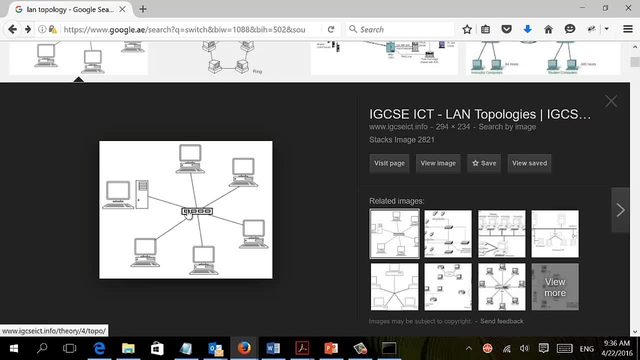 the MAC address table that is mainly based on ARP request and ARP reply can be manipulated in different way and you know, even if you put some static entry here, this would be hard to implement. it will affect some other appliance like IPS or traffic analyzer, so it's not easy to prevent this kind of attack. so this is how the switch is. 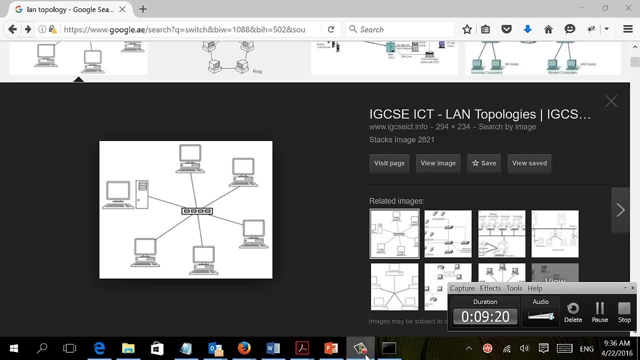 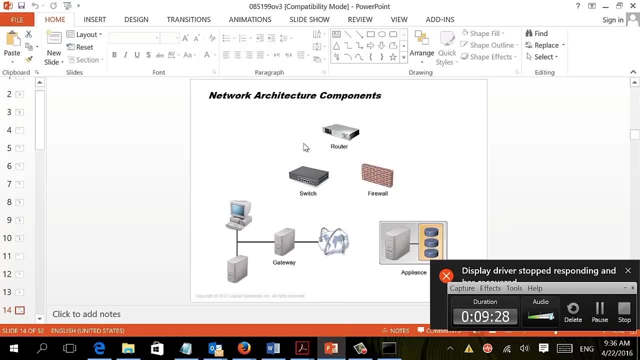 working and this is the weakness of the switch now getting back to a bigger layer or higher layer. now, if I need to connect this computer or this network in my building to another network located in a different facility, what do I need to do? that we will be needing for a router because 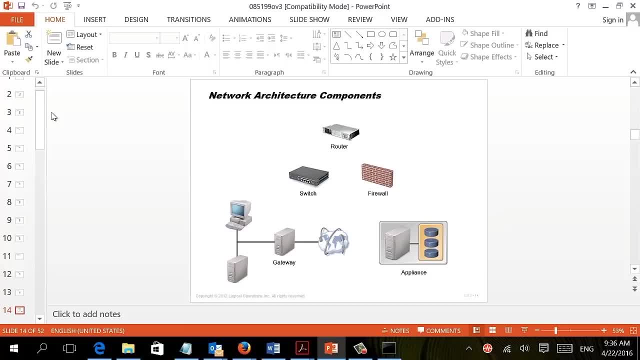 router are routing traffic between different networks so he can connect to different LAN together to become a one. so we're going to need a router. so what is the functionality of router? router as a functionality need to or has a function to the site. what is the best routing to a specific location for? 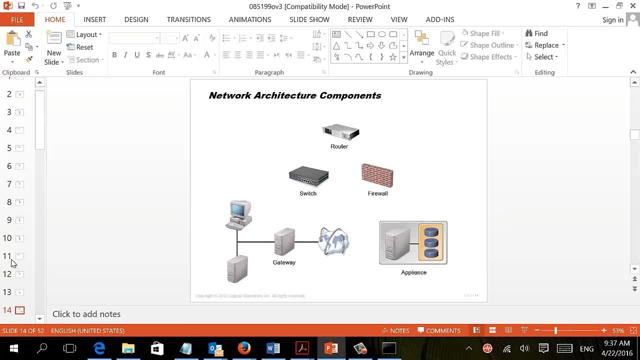 instant if you open a browser and type wwwyahoocom, so a request need to be sent to Yahoo to ask for the Yahoo page. do you think there is only one pass from your house or your office to Yahoo server? there is many passes and the router has to. 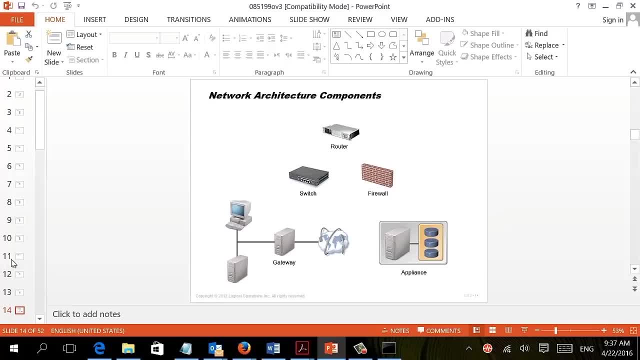 choose which pass he should use to get to Yahoo server the fast way he can. this is the routers. how's the router working? you know we spoke about switch switches. you're working according to the MAC address table, or sometime called the cam, while the router is working according to something called the routing table. he 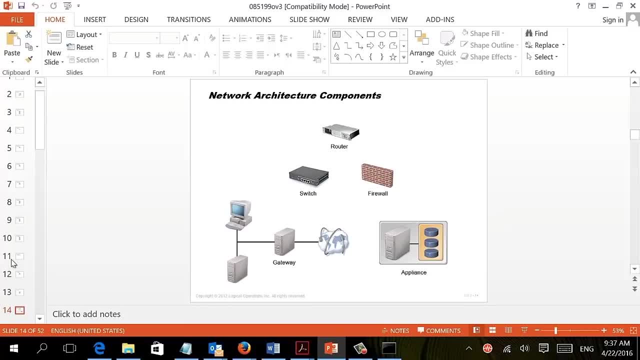 will have all the passes inside the table and whenever you send a request, he will open this routing table and check what is the best destination to this specific location. now here you need to know how can we do that. how can you make the router choose the best pass? we have two different. 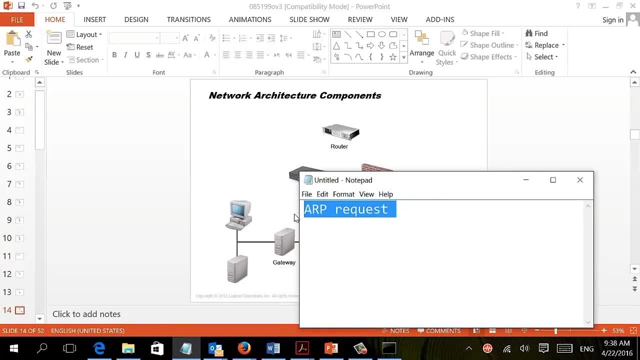 for doing that. we have the static routing and we have the dynamic routing. so static routing, which is not an effective way for doing that, it's that you specify the location yourself. static routing, so you can go to the router and tell him whenever someone need to go to. 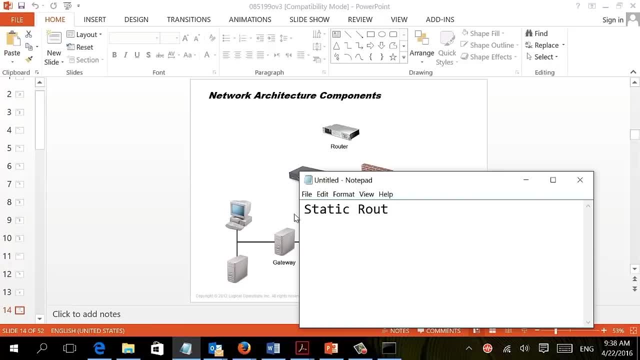 static routing. whenever someone need to go to the router inside or the location yahoo server, he have to go through this path. so you have to go to the network inside china's and the network inside europe, so you specify the path, and actually this is not an effective way because you're gonna have to specify every static routing now the better. 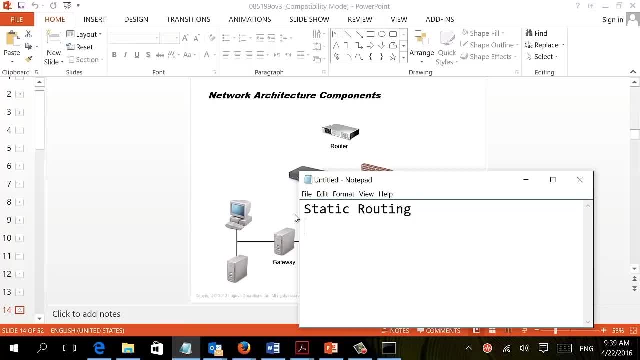 way is to let the router decide. do not tell him the path, but let him decide whenever he get the traffic to choose which path. and we are doing that by dynamic routing. and dynamic routing it's to let the router decide. now, how can we make the router decide? it's by assigning routing. 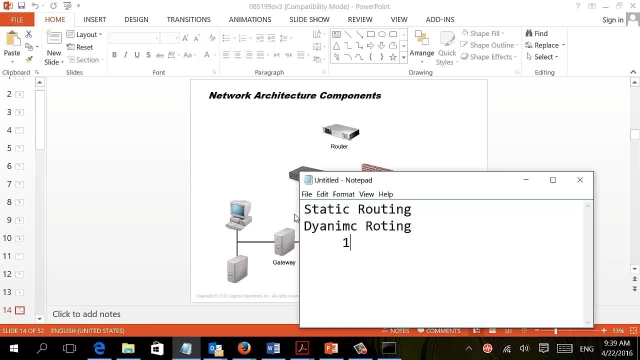 protocol. so by putting routing protocol on the router you make him decide himself which one, you, which path is the best path, and we usually we have two different kind of routing protocol- i'm sorry about those spelling mistakes, but i'm writing too fast- and the first one is called the 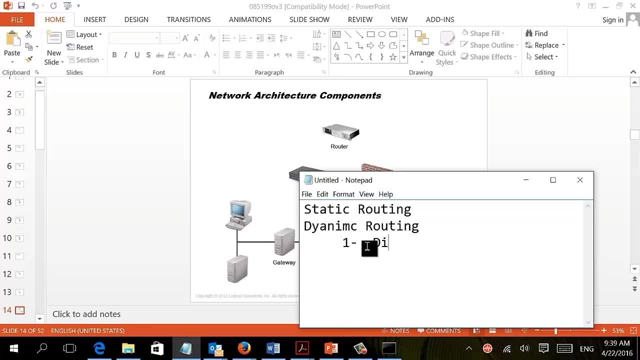 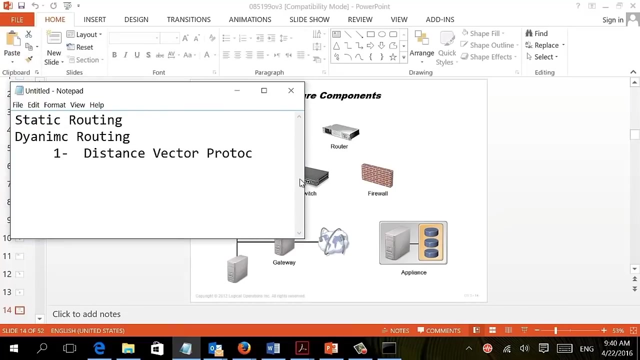 distance vector protocol. this is not the name of the protocol: distance vector, sorry, vector. distance vector protocol. and a good example about this protocol: it's a protocol called rep or rep version 2.. so the distance vector protocol, it's a protocol that depends on the distance, on something called proto. 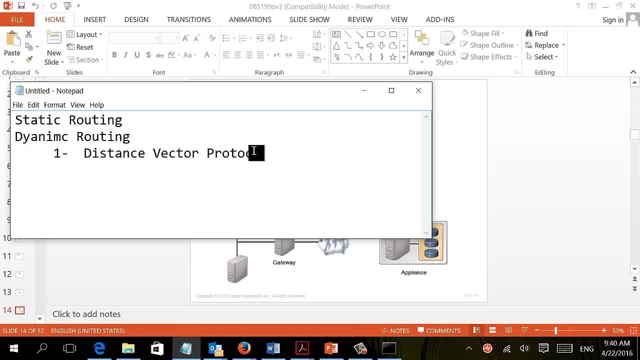 code and, as i told you, don't forget the example. an example of distance vector will be a protocol like rep or rep version 2. this is the distance, so the distance vector protocol depends on the hop count. so, for instance, if you have two different way or two different paths going to the same destination, 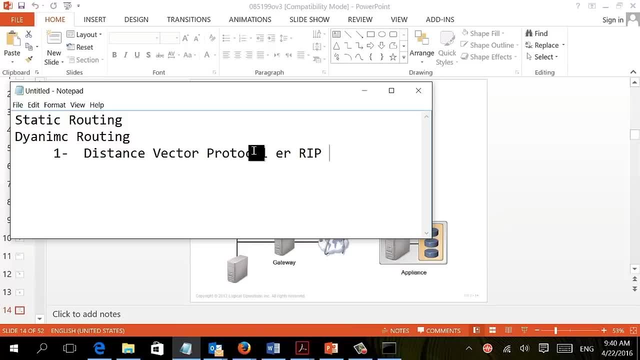 one of them has two router until you reach the final destination, and one of them has three router. he will choose the two router. so he's he's checking according to the less amount, or we are calling that the less hop count, less amount of router in the way. 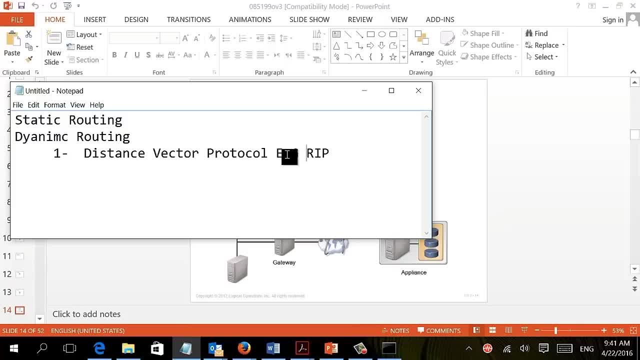 but this is not necessarily the right approach, because maybe you have two different ways that will take you to the same destination. one of them has two signal and one of them has five signal. if you choose the two signal, do you guarantee to reach earlier? definitely not. maybe it's two. 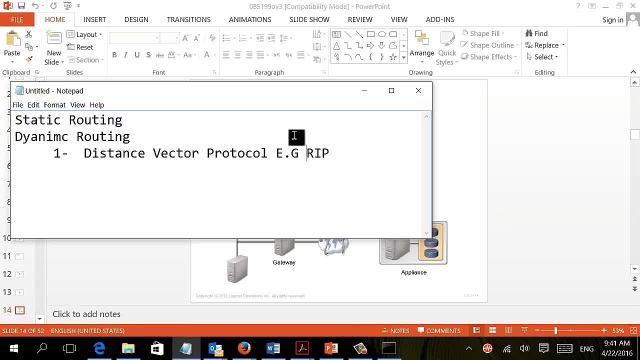 signal but it has a very high traffic. so distance vector, rep and rep version 2 are actually depend on the distance vector and, as i told you, it's not that effective. the second type of this is the one type of protocol. it's called the link state protocol. this is the type of 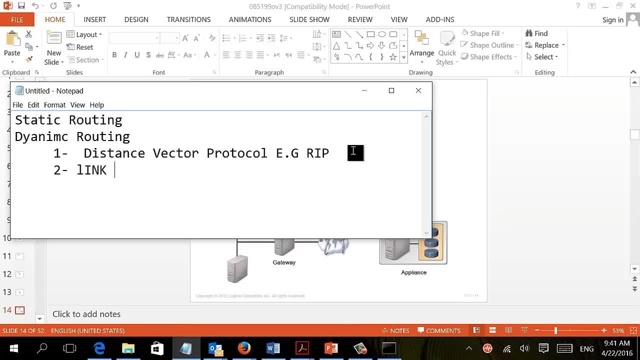 protocol link state link state protocol, and a good example of that will be a protocol called OSPF- open shortened passwords- and this is actually very, very effective because he will consider many things. I mean, when you give him or ask him to reach one destination and he got more than pass, he will consider the 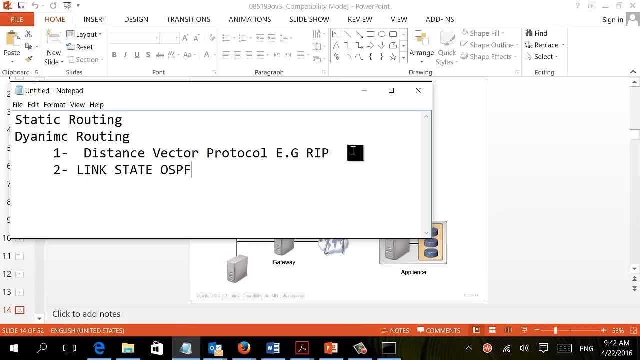 bandwidth, delay, the speed of the line and so on. so he's calculating many factor to take the right decision. so it seems that OSPF it's more effective than link state. I'm sorry, link set is more effective than distance vector, so why people are still using distance vector in some cases? 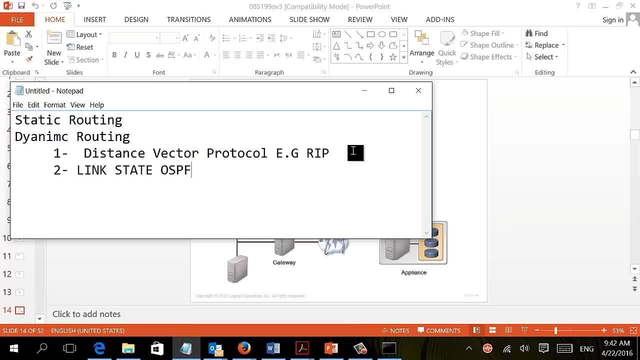 you can see that the distance vector is very effective in some cases because the problem with OSPF it was kind of complicated to configure. sunset easy to configure is hard while rep is very, very easy. so if you have a small network you can use rep. I mean it will not be that complicated. we have a third one we call 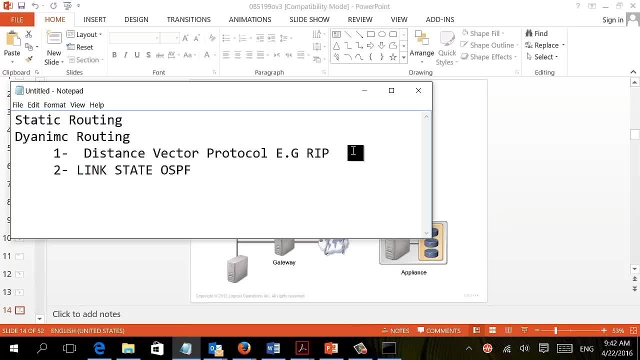 that the hybrid protocol, which is, you know, the best protocol, the one who's taking, sorry about that. so we were talking about protocol and we said in in routing. we were talking about protocol and we said in in routing. we were talking about protocol and we said in in routing. 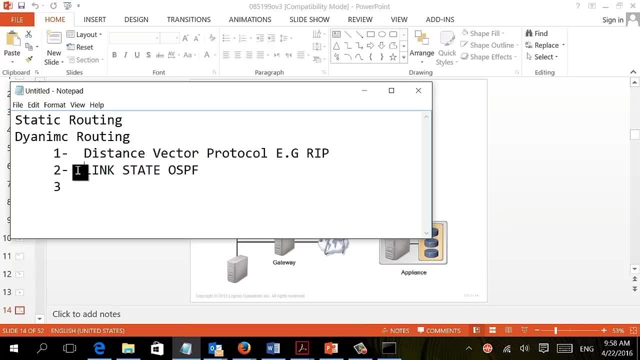 protocol. I have the distance vector, which is things like rep and rep version to link state like OSPF, and we have a third type that we call the hybrid protocol that have the both feature. it's the best protocol. it has a good feature from the distance vectors that is easy to configure and also it has the feature. 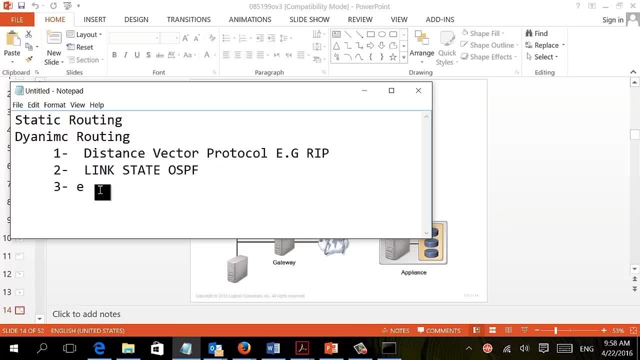 of the EIG of the OSPF, that it's checking the route based on many factor and it has its own feature as well. and one of the very well-known protocol is EIG RP protocol. this was one of the best routing protocol. it used to be Cisco. 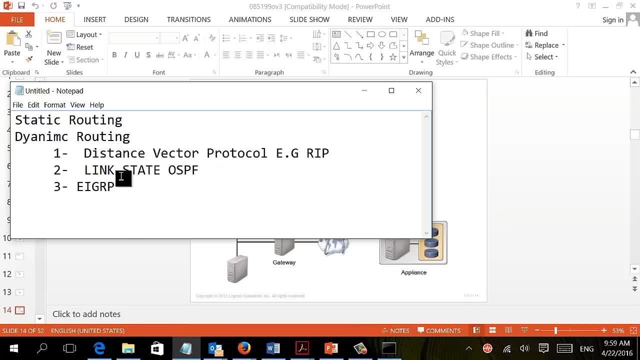 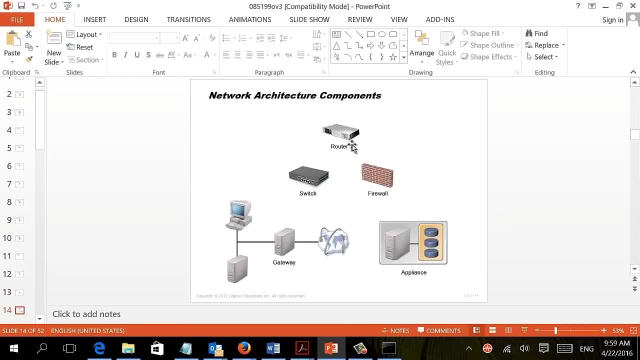 proprietary, I mean you can only use it on Cisco, but right now it's open standard. you can use it on any device. so this is the routing protocol. on the next video, we will be talking about the type of firewall and then we will be talking about the application, which is very, very important, where we'll be talking about 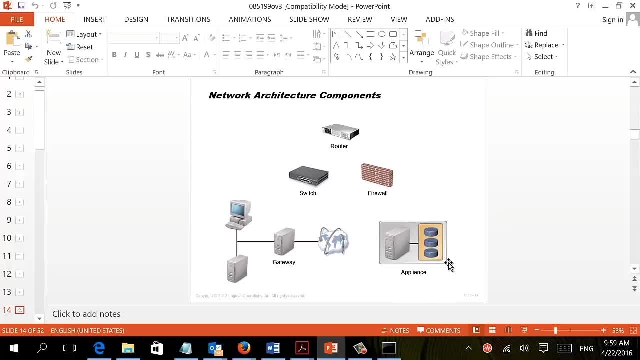 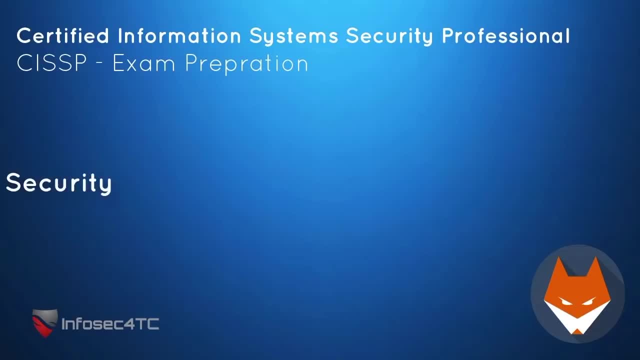 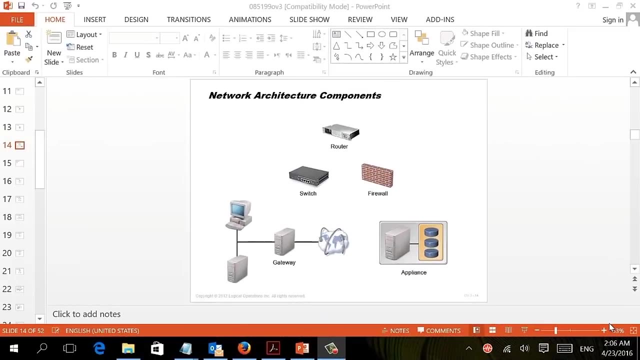 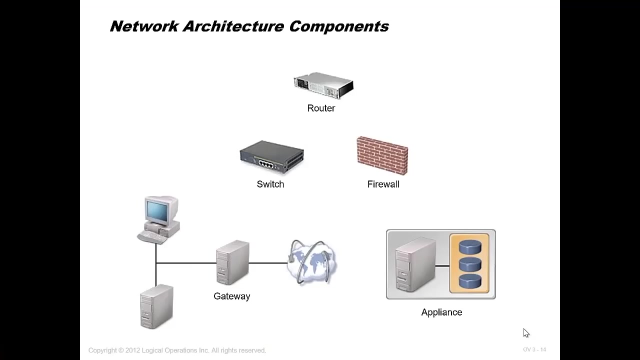 the type of backup, backup type of RAID. this will be a very, very important lecture. in this lecture, we will be going through firewall and explaining what is the functionality of firewall, different type of firewall and, finally, the different architecture of firewall, how firewall can be implemented inside your network- and I believe this is an important area as well. on the 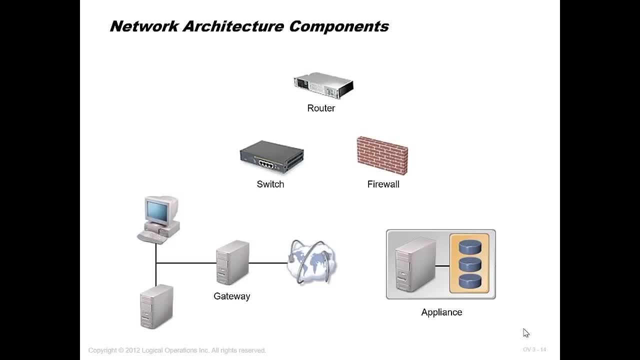 previous lecture we explained different component like switch, how it work and what is its weakness. we spoke about router: what is its functionality, what is routing protocol, what is static routing, dynamic routing, and now will be talking about firewall. and firewall it's a preventive technique layer, so what exactly firewall is doing? 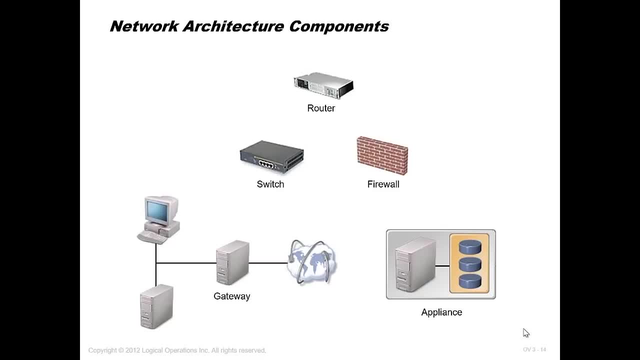 so what exactly firewall is doing in your network, whatever it is, if you are sónone, which I use, include firewall is doing. it's actually inspecting any traffic going in or out of the network and you can add some rules. so if the traffic matches the rule, he can allow or deny. so it's. 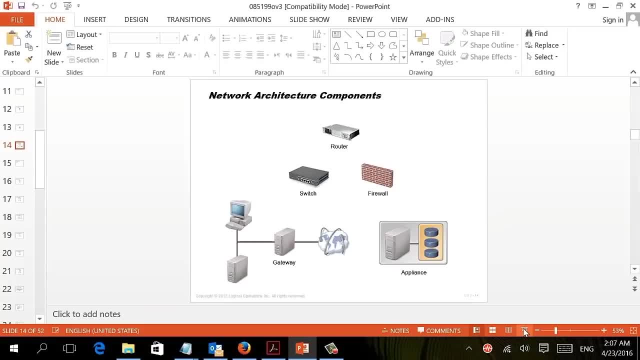 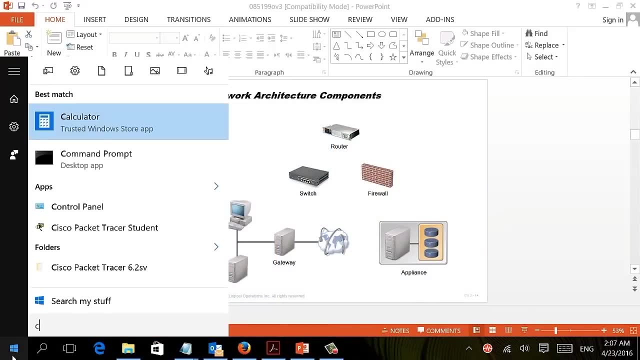 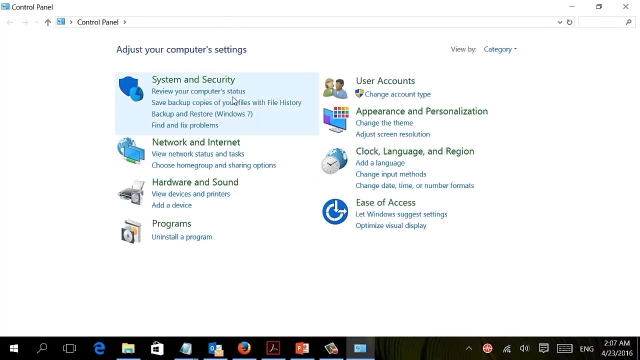 an inspection device could be an appliance or it could be software. let's see how it look like if you went and open control panel on your machine. let's see a simple fire rule which control. it's a host based firewall, because in firewall we have host based and we have the network based. 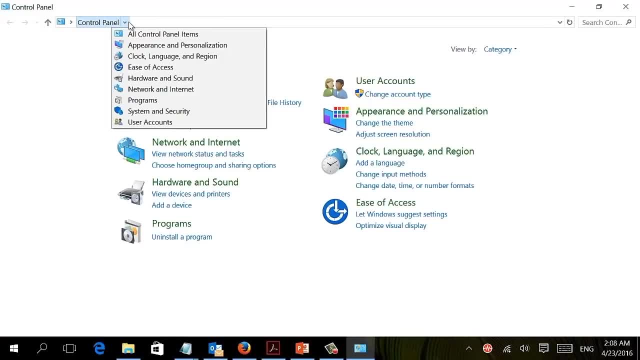 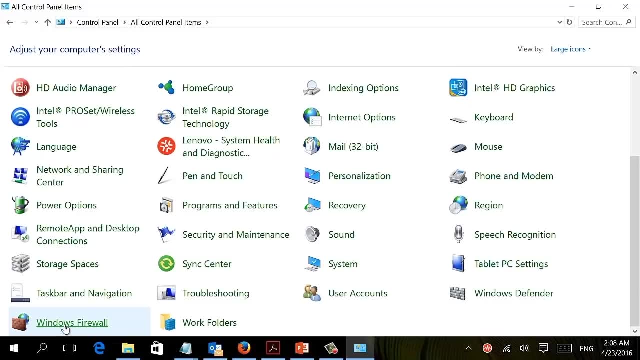 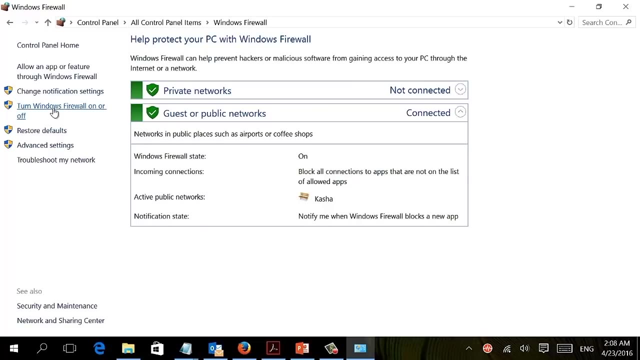 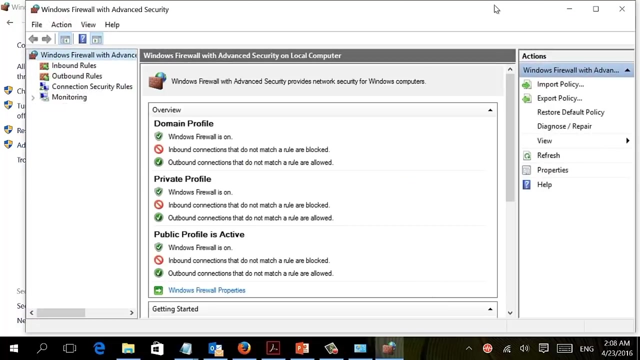 so let's see the ones that we have on our computer just to get the idea of firewall, all control panel and let's see here windows firewall and let's see the turn on advanced setting. you're going to see that this is how we are configuring the firewall. firewall usually have two different kind of rules: the inbound and the 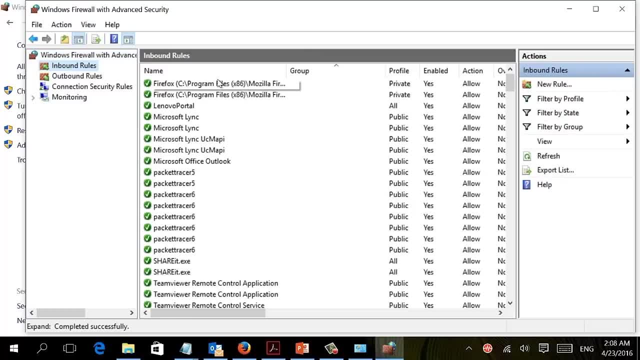 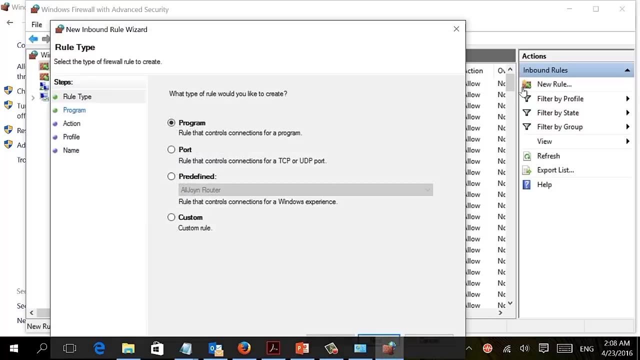 outbound. so the inbound are inspecting any traffic coming from outside into our network and you can put a rule here and according to this rule he can apply or deny and you can even create your own rules. so you go in on rule create and you choose which port and then you click on next and you 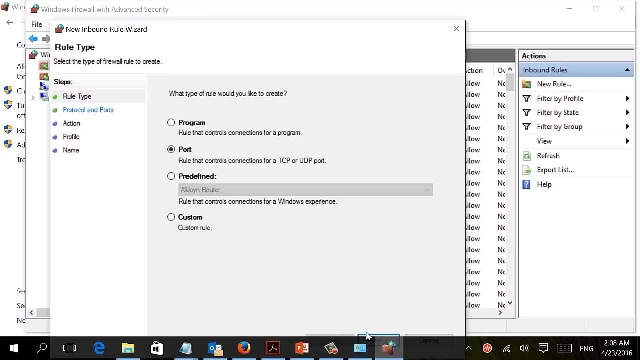 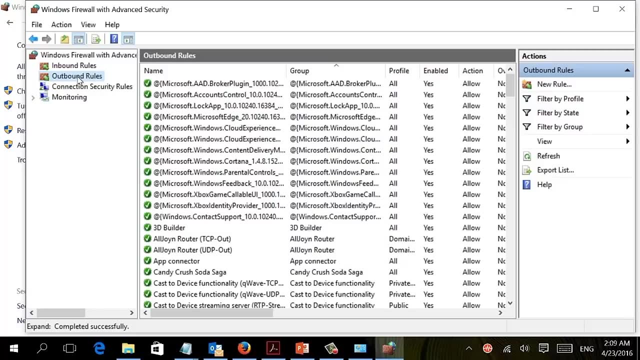 choose if it will be allowed or denied and the type of traffic. so this is how we are configuring in general, the firewall outbound rule. it's inspection of the traffic going from my network to outside. now, as i told you, it's an inspection tool, so it's a preventive. i mean it's like you are putting a security guard outside of. 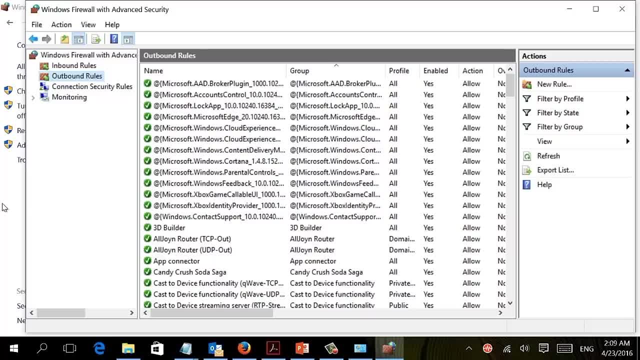 your house and he's checking everyone id before coming in. if the id match whatever you told him, he will let him in. otherwise he will not let him in. this is the idea of firewall, and i don't believe it's a very effective way for securing, because 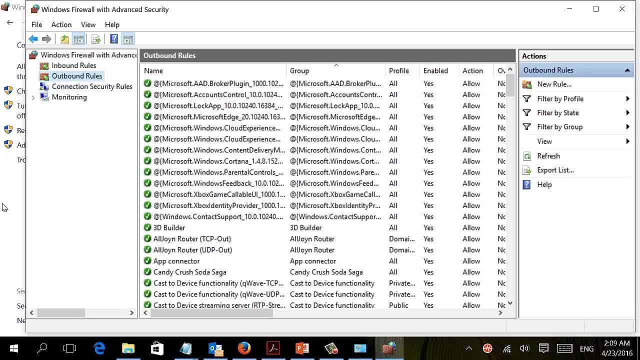 since it depends on inspecting the packet header, and packet header can be manipulated so it can be bypassed. it's not actually that i i consider the firewall more as a controlling tool than as a fire, as a protection tool. now, what i need you to be aware when it 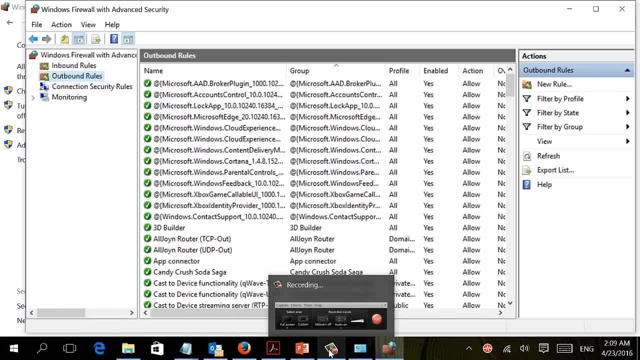 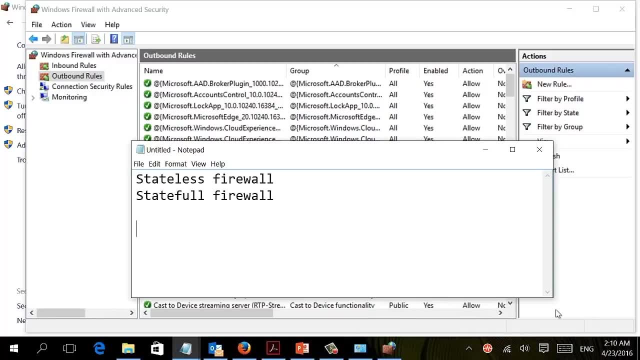 comes to firewall is two different type of firewall: stateless firewall and stateful firewall. there is like four different type of firewall- application firewall- but actually i want you to give a specific attention to those two, but you need to read the four definition which you're going to find inside the cssp summary. now, what is the difference? 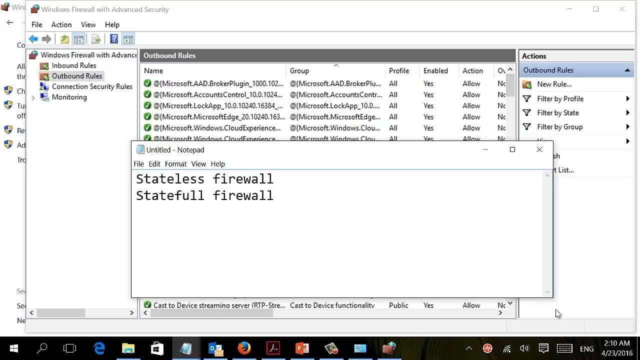 between stateless firewall, which is the old type of firewall, also known as filtering firewall, and the stateful firewall. here is the situation let's talk about about. first, about the old one, the stateless firewall. assuming that you need to allow people to browse the internet, it allows them to browse website from the internet. 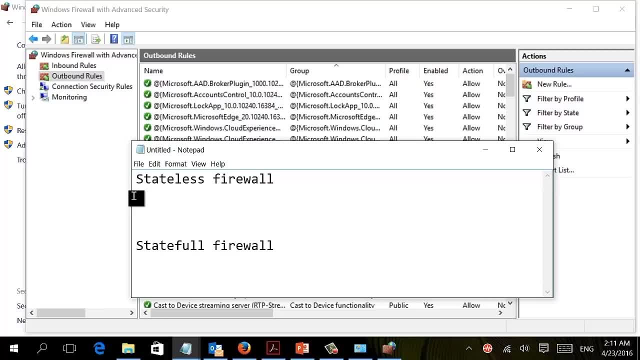 so you create a rule and you did allow: allow port 80.. so you put on your rule on your host based firewall and maybe on the network based firewall that please allow port 80, because you know that any requests that go into the internet browsing will be going through port 80. so any request going to yahoo, gmail, hotmail, 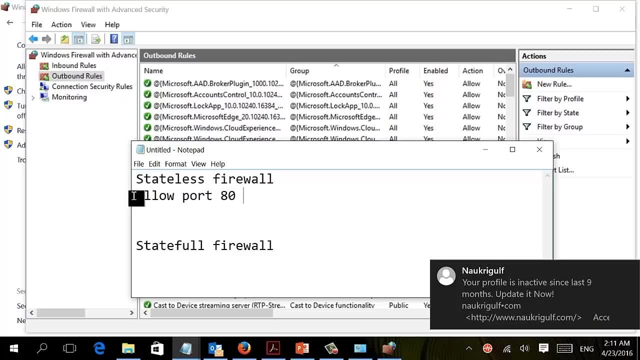 on the header here. it will have a power 80. it will allow only traffic to power 80. and the remaining of the port will be- uh, i'm sorry, it will allow traffic on port 80 and the remaining of the port will be closed. now here is the scenario. the request will be going from your machine to port 80, so the 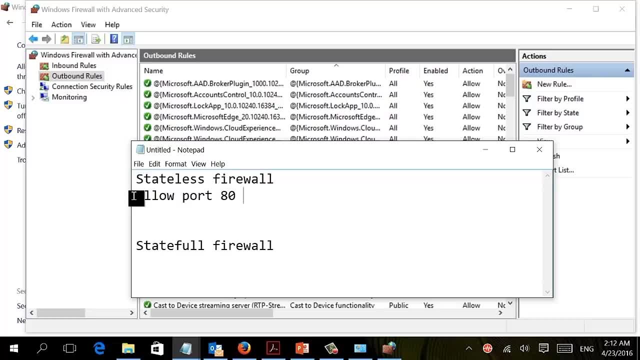 firewall will let him go out once this request reaches the web server- google or yahoo or whatever- and this web server is sending you back the reply. in this case, the reply is usually coming on a uh random port. it will not come on the same port, so he may come to port one, two, three, four, five or 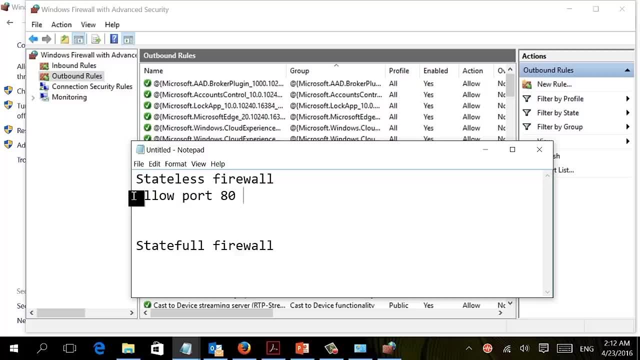 port five, five, five, five. so it will be coming on the port on a random port and since the firewall are closing- i'm not, i'm talking now about the stateless file- since the firewall are closing all the port- unless you allow it. so the reply of this request will be dropped. 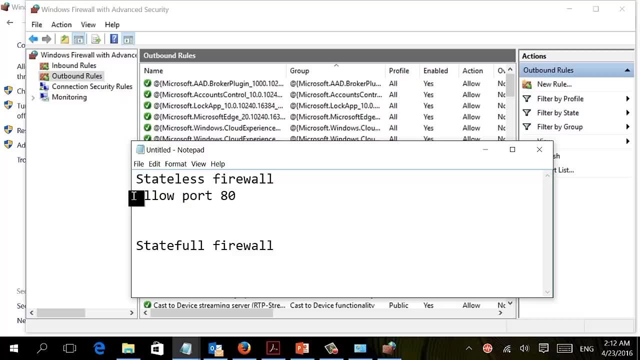 so now you will never try to browse any web page. it will not open because the reply, the, the, the request went successfully, but the reply, because it's coming to a random port, has been dropped. this was the problem with the stateless and you cannot. you cannot adjust that because 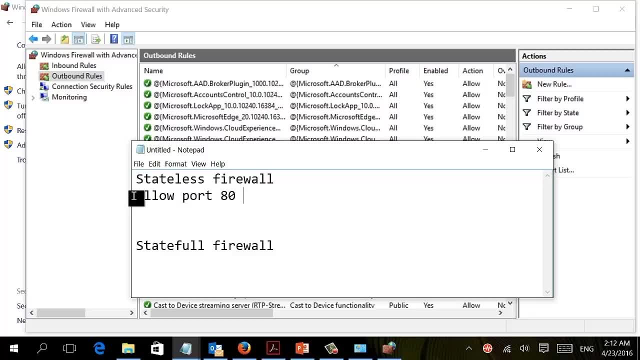 you will not able to understand or to know each website will send the replies through which port. so how can you configure that stateless? it's a little bit different that it's actually. it's it's solving this problem. stateful stateless has this problem. whatever you configure, he will stack with it, but he will not do anything else. the stateful uh. 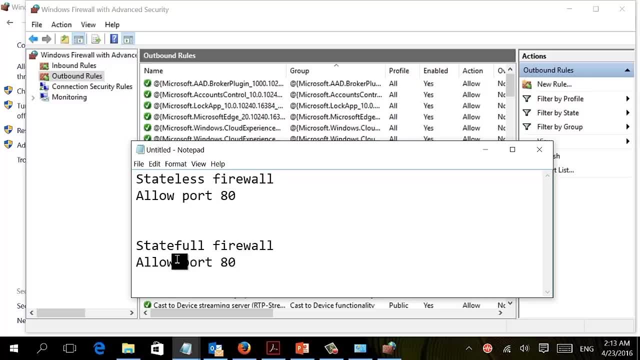 firewall. it's kind of different in a way that if you have the same scenario, you are sending requests through port 80 and you are allowing port 80 on your firewall, he will let him in, but the thing is he are tracing the request, so whatever reply is coming back, he will check the reply for. 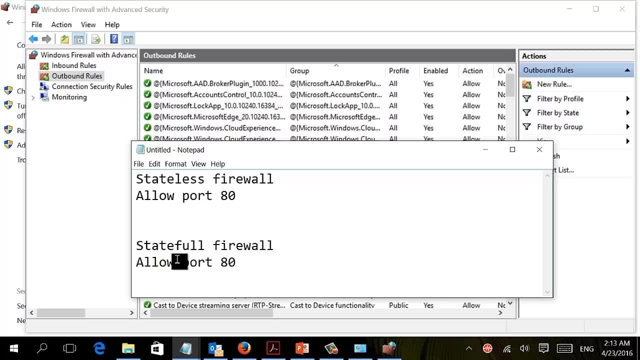 this specific request back on which port and according to that, he will dynamically open this port. so he's tracing or he's following the request to be able to open the port for the reply. so it's kind of dynamic. this is the stateful firewall. we have, as i told you, the application firewall, which work on application. 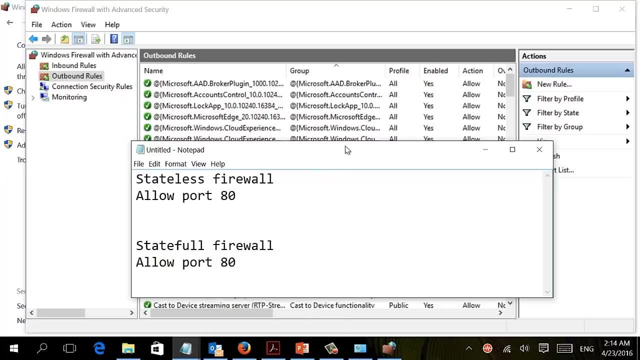 layer and, as i told you, you're going to find all the definition and you just need to know that deep about the different kind of firewall. the second important port point about firewalls that you need to be aware of is the structure. how are we going to implement firewall? are we just going to make a firewall or implement a firewall? 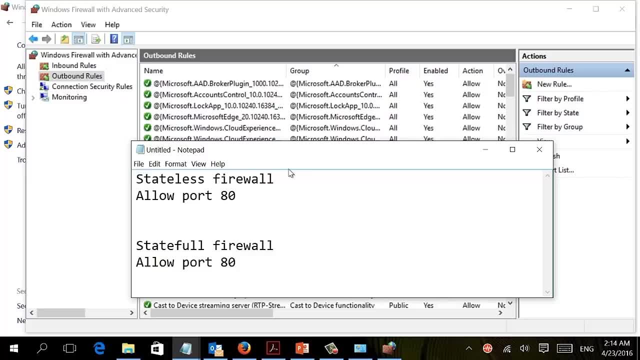 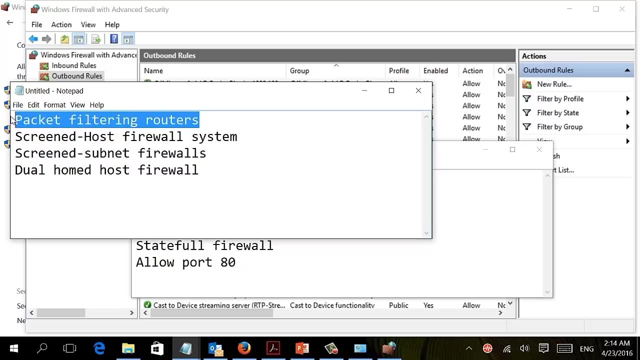 between the internal and external network. are we going to create a dmz with a firewall before and after. so we need to know those architecture and we have, like, mainly, three or four architecture. so for, for instance, we have this, the packet filtering routing, which is just putting a simple firewall between the two different network. this is called the packet, this. 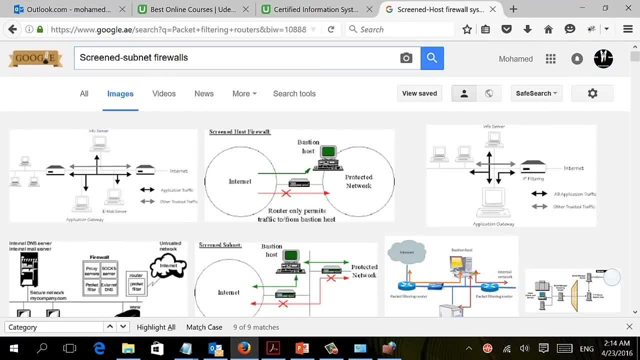 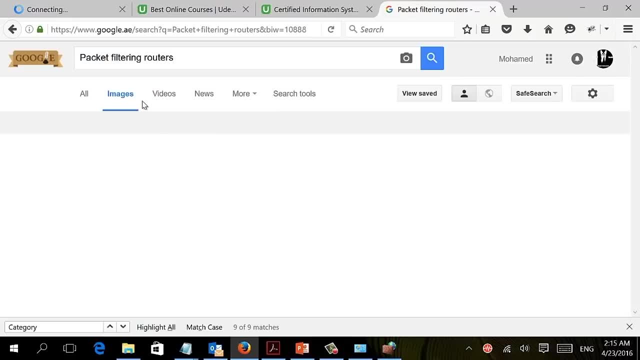 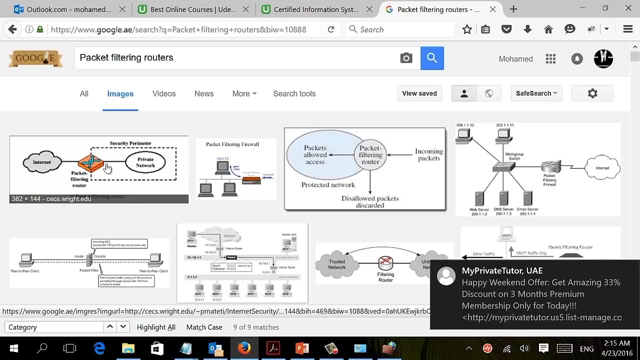 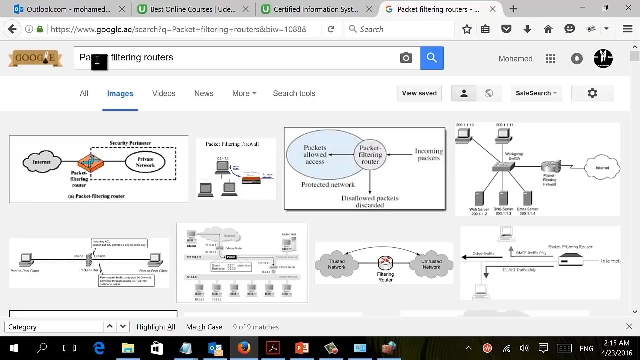 is the simple way of firewall. so if we go here and we create it or we check this kind of firewall paste, you will see just a simple way. you have two different network- internal network and external network- and you are putting just a firewall between them. this is one way for uh implementing. it's called the. 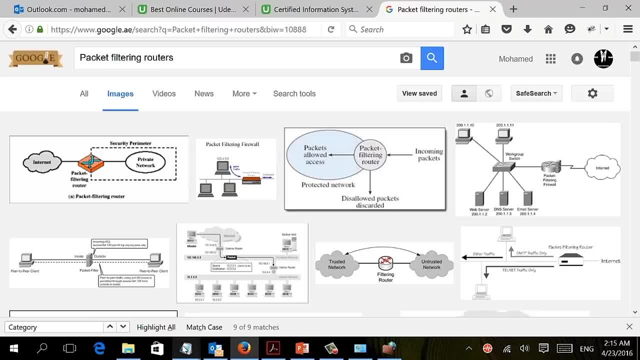 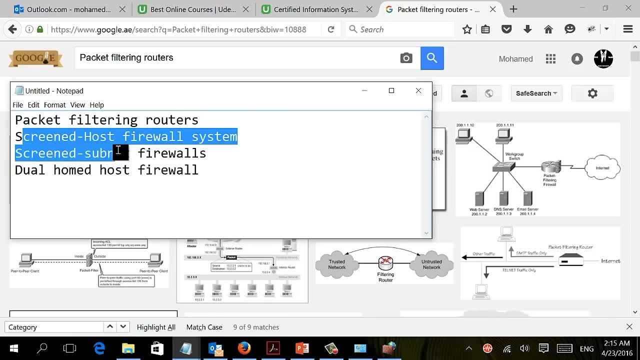 packet filtering. this is a simple implementation. we have another model or another architecture, which is a screen hosted file. do not be confused between those two, because actually those are quite important. screened host firewall system- it also the same way, except it work as a packet filter and application layer. write them, write this note down. it has two different function. it's. 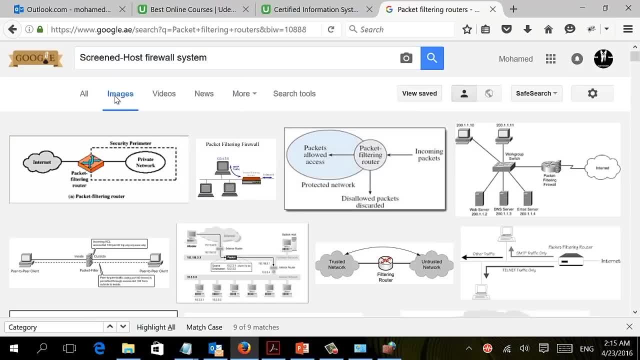 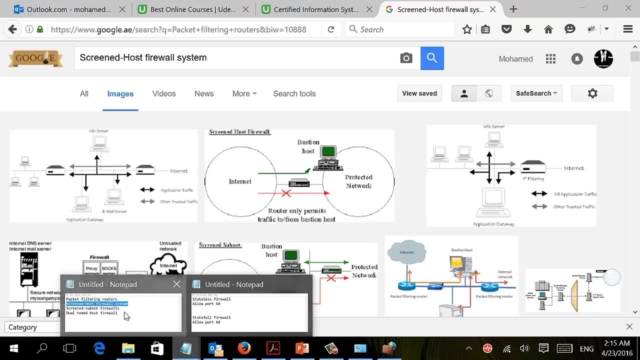 a packet filtering and also a application firewall. so it's similar, but it has two different function and we are going to demonstrate this one. in this case we have a specific network, to whom we have a virtual network, to where we are going to put the network we are going. 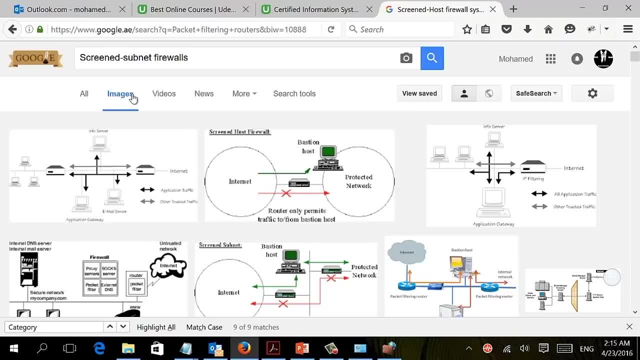 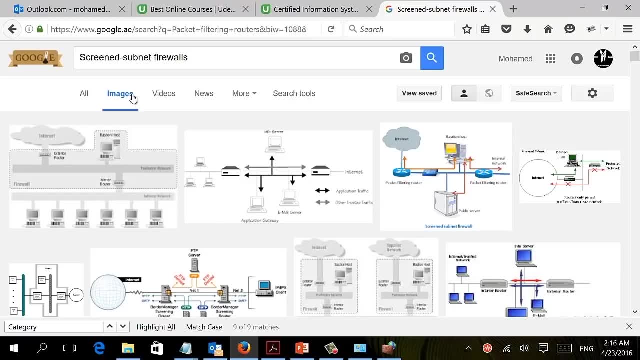 to put it, behavior. we are going to have user, user, and that's why we are calling it overview, in order to give you an idea of this process, because it is going to be a very simple project, but also it is very easy to do at a very simple basis. so this is a very simple way to do in this. 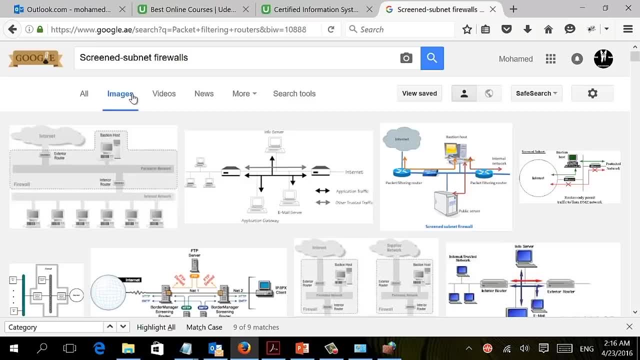 way in order to get the information to be available in our network. it's very easy because we start to exposed to the internet. like you have a web server where you're going to put the company website and people from the internet will be allowed to access, or you have a mail server, you have 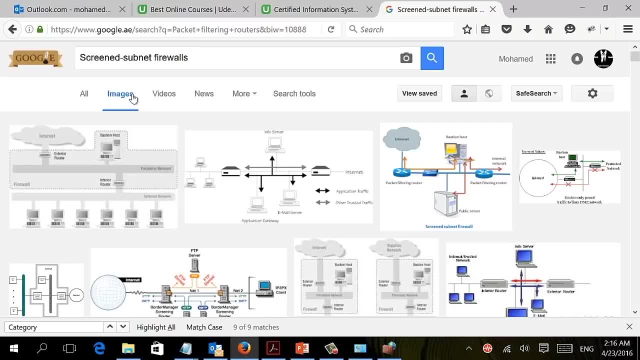 you cannot put those server that will be accessible from the internet within your internal network because by doing that anyone can compromise one of those server. he will be compromising the land. that's why we create a network that have those server and we separate this network from our network, from our internal network. this is actually- i believe it's- a good 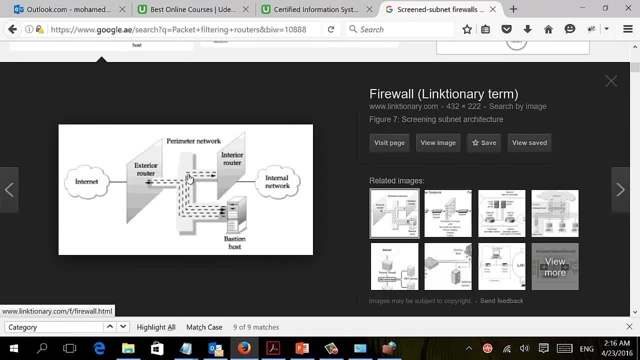 example. so this is the internet, and then you build a network here, you put all the server that need to be exposed to the internet and then you put your internal network here and you put two firewall: one between the internet and the dmz and one between the 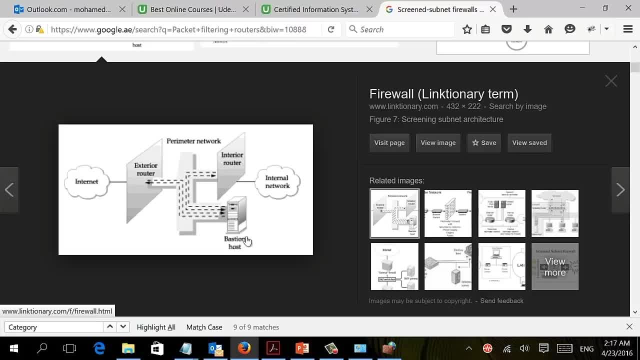 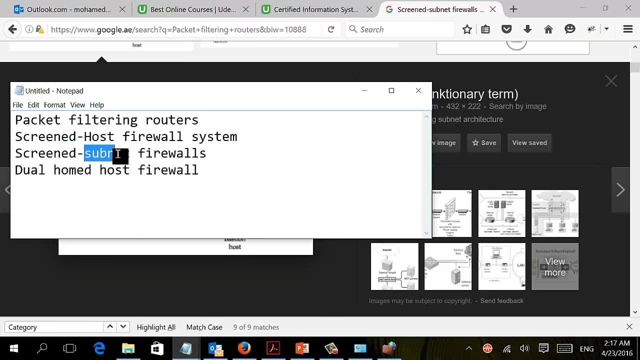 dmz and your. so you are trying to harden your system a little bit. so the screen subnet firewall: get the subnet as a keyword. i get the subnet as a keyword. subnet mean it's there is a third network between the internal and the external dual home hosted firewall. it's a specific firewall where we 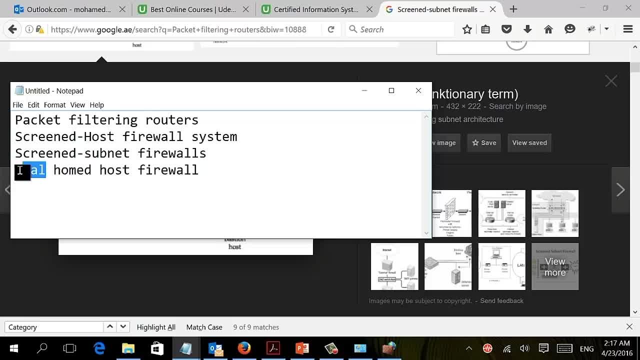 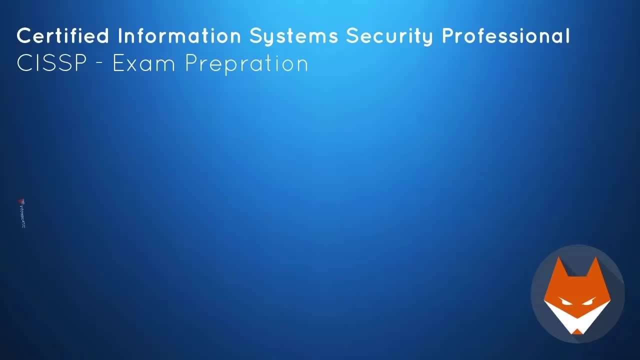 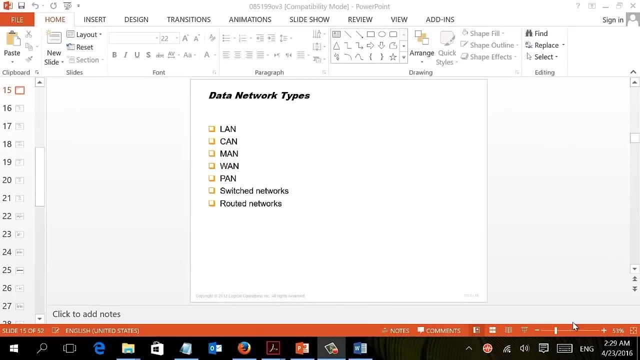 are putting two network adapters. that's why we call that the dual. at me it mean it has two different network adapter. so those are the architecture about for how to implement the firewall runtime. so i just have the data when we all apply, as you can see on our appliances. 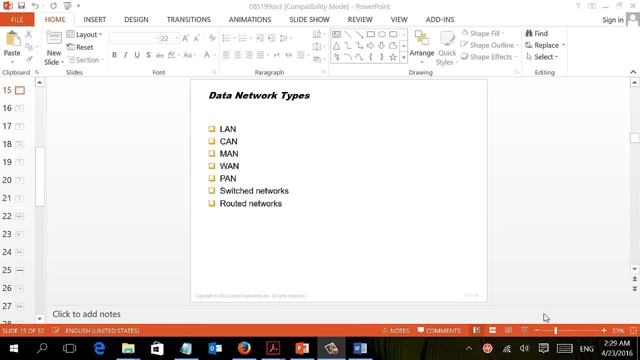 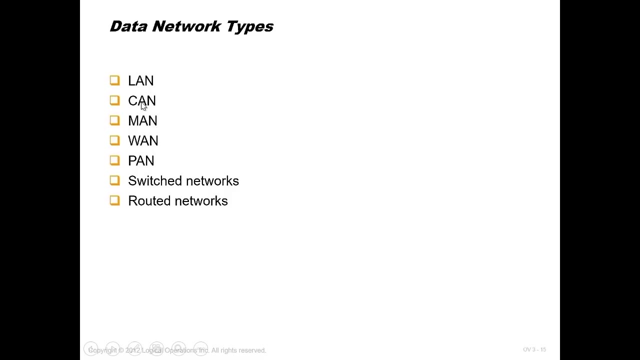 all, given that we are playing it, disappointed in the main computer. so we've open the PI, that is Intel sendiri. here we will enter the đi de entend litres. if you are initializing your construction, you are going to see that we are going to have the main metropolitan area network, which is a network that cover a city, for instance. 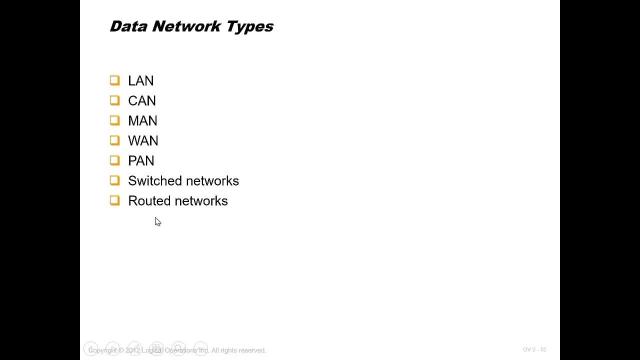 or a neighbor. we have a pen personal area network- this is like wireless mouse or a Bluetooth or something like that- and we have a switch network and we have the routing network. then the network topology. and topology mean how network could be connected together, so we used to have the start up all as a ring. 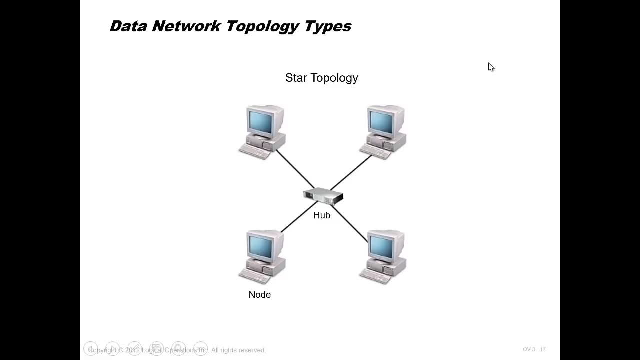 topology where we are connecting all the machine. oh, I'm sorry, let's start with the first one. first one is one we are using a star topology where we are putting one centralized device and all the machine is connected to this device. could be a hub, could be a switch, but this topology or this kind of 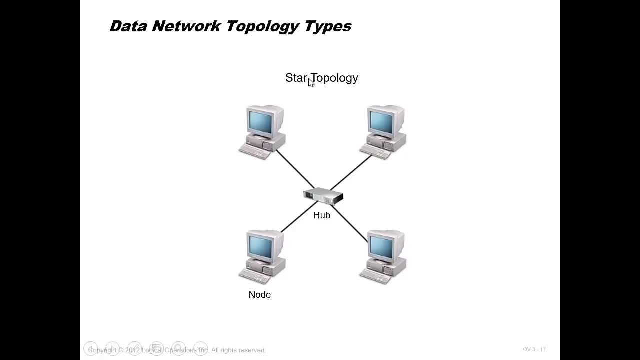 architecture is. this is called the star topology. what is the problem with star topology? single point of failure. this is very important terminology. please don't forget to like and subscribe to my channel. write down: for any network. to evaluate the network effectiveness, you have to check something called the single point of failure in such topology. do we have a? 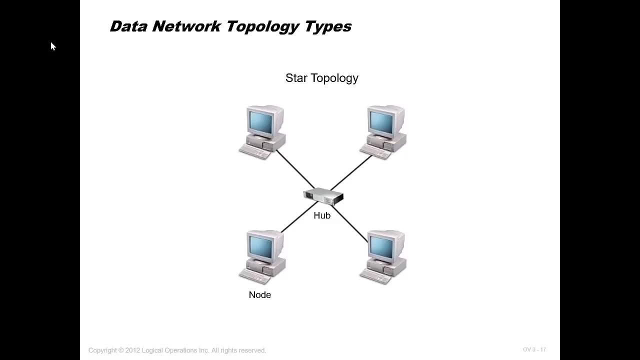 single point of failure. do we have one device? if it fail, it will drop down the network. yes, we have the hub. if the hub fail, all the network will not be able to communicate, because this is single point of failure, where the client or the computer are not single point of failure, because if this computer fail, it will affect. 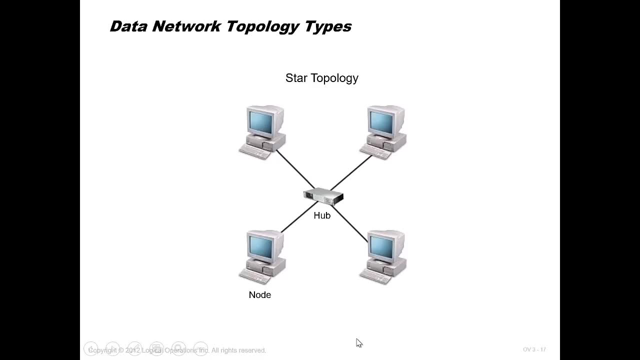 only the user who's working on this computer, but the remaining of people will be able to still communicate with the other users who are working on this computer, to still use the network. that's why we are adding two hub or two switch for redundancy. second topology is a bus topology and we used to do that, you know. 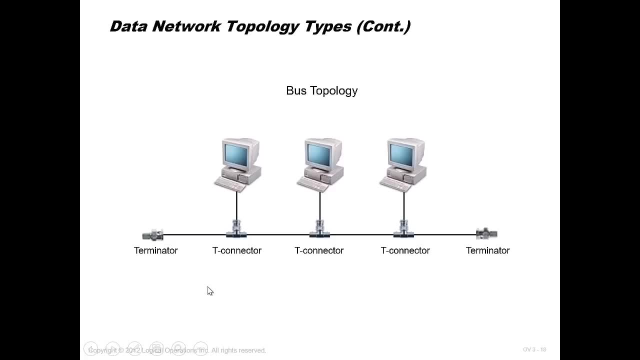 back in the early 90s that we have some specific network card with the T terminal and you connect all the machine on one segment. you don't have a route, you don't have a hub or a switch and you have to close the segment with something. 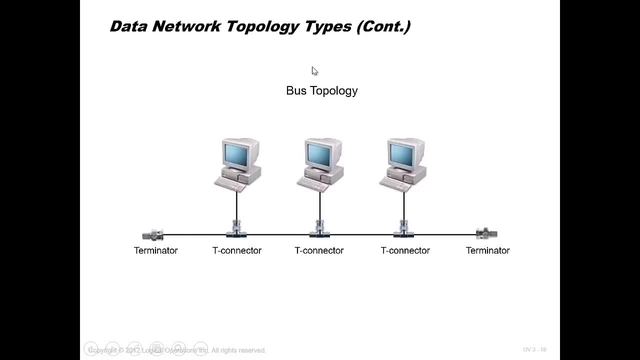 called the terminal and this is called the bus topology. the disadvantage of the bus topology is that any cut inside this wire will lead to the down of the whole network. we have the link topology, which also has some issue, for instance information, if you are sending information from the first computer here. 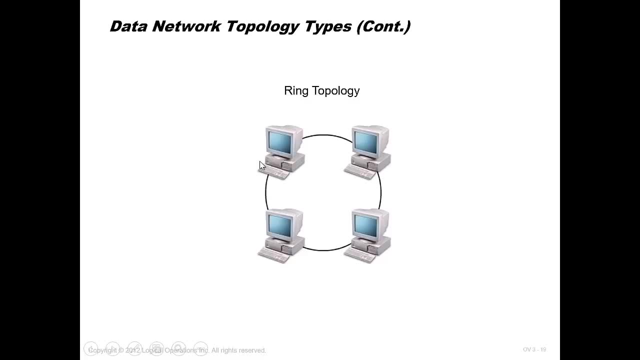 to this computer, there he has to go through all the computer. or from this one to this one he has to go to all the computer. this was one of the problem. beside, any cut in the wire will lead to the same results. but you should know that the ring topology is not just the legacy topology. we still using it, so fiber. 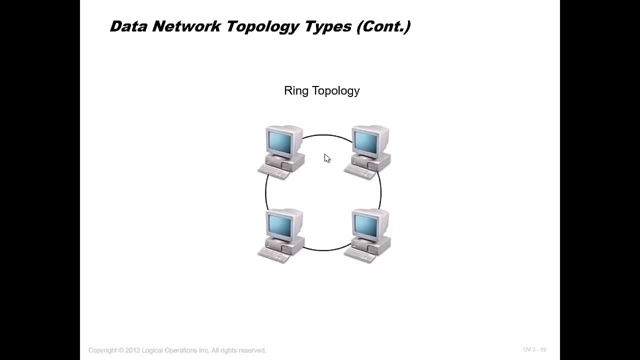 network that we are using in today, network in, you know, for high-speed internet. this is ring topology. they are using ring topology. they are not using stars, they are not using bus, they are using the ring topology, but they are doing some redundancy, as you can see later on, and so on. then, according to 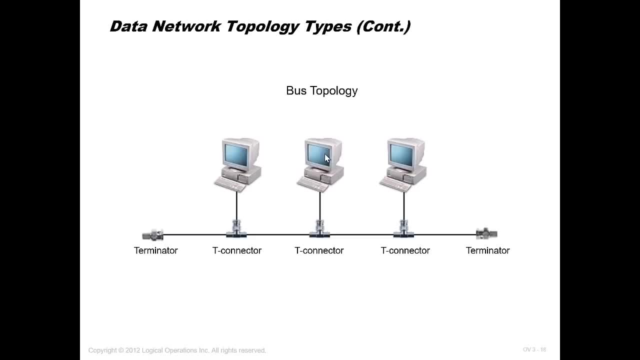 that each network has, or each topology has its own weakness. so which one do you consider the best topology? the mesh topology, i'm sorry, and mesh topology mean you are connecting all the machine to all the machine. so, as you can see over here some computers, they are all connected to each other. 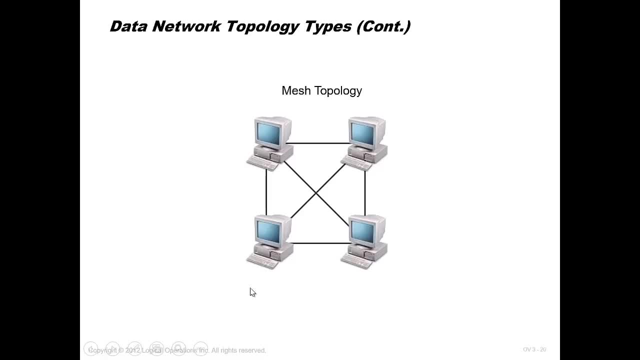 so if any wire you know get cut or any problem happen to any wire, you still can. network still is running because there is alternative path. but mesh topology, it's easy if you have a small network like this one, but what if you have a complicated network? i mean you have like 100. 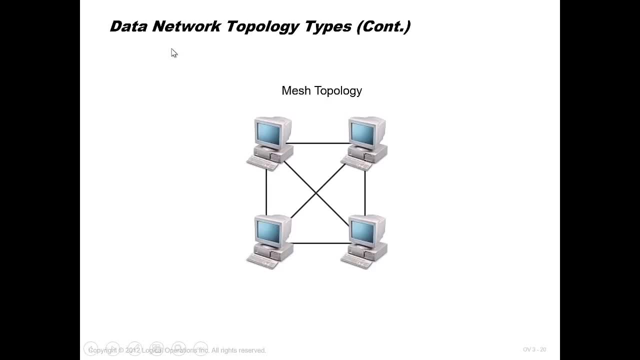 machine or 200. this would be very, very complicated. so we are using something called virtual mesh, looking for the machines that is more critical and then connect them together. so this is the part related to topology. now we'll give a brief about the media. network could be connected through wired or wireless. in wire we have different kind of 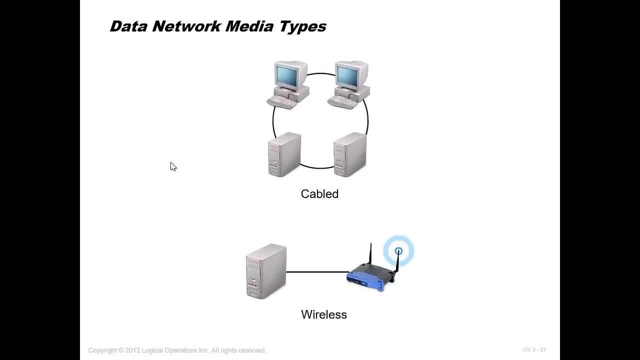 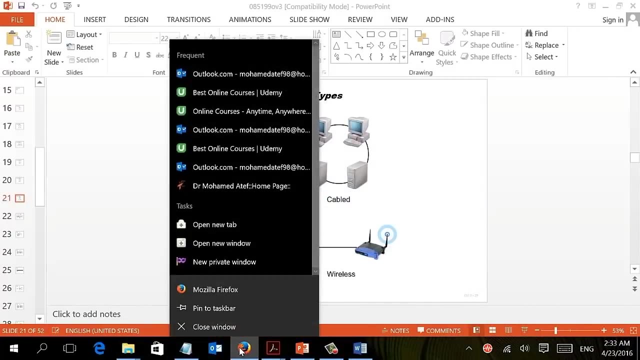 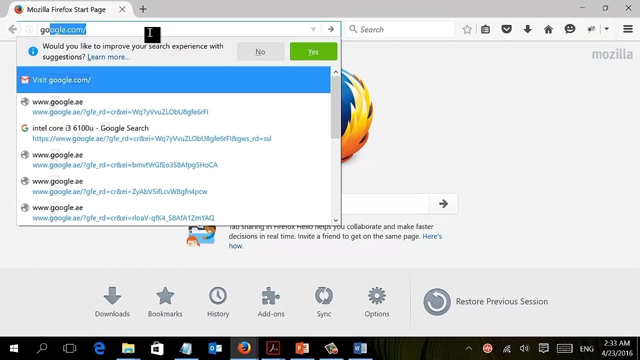 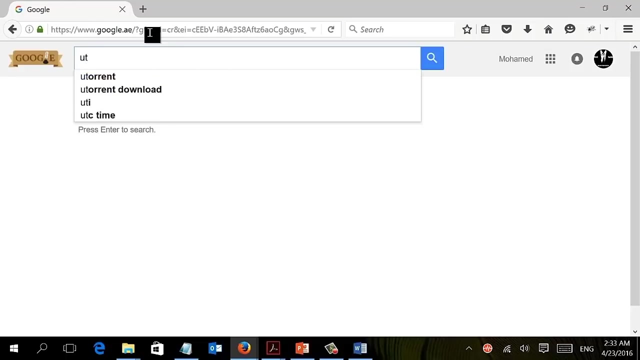 wires that you should have a brief about them. so wire we are using you, let me show it to you. so what kind of wire- i'm sorry, what kind of wire we are using inside the network. if it's lan, we are using utp cable or untwisted shield pair cable. 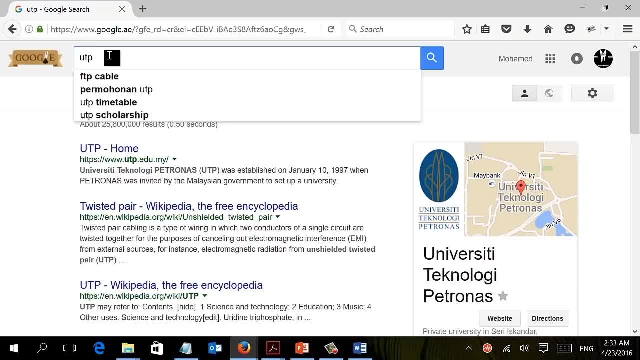 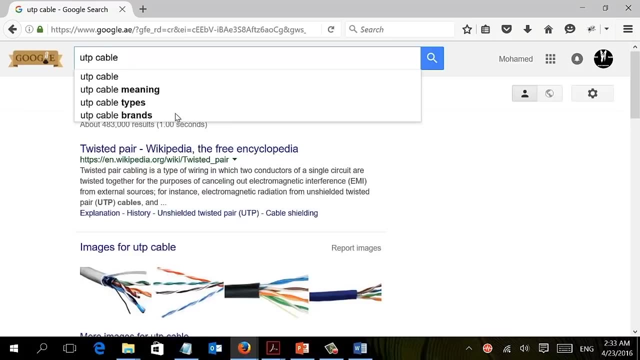 and utp cable. let me show you. it's just a cable that has eight wire utp- sorry, utp cable. by the way, google image will be very useful for you while you are studying in this course, especially things like physical security, because a lot of people do not have that. 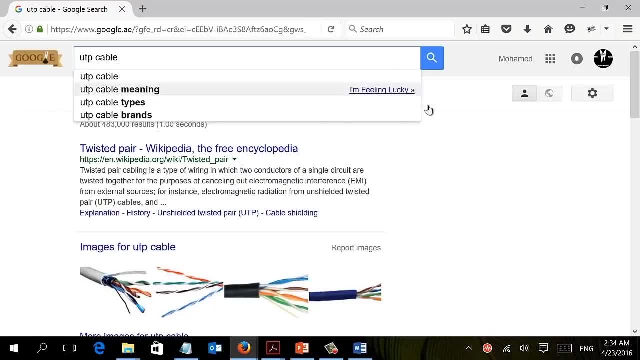 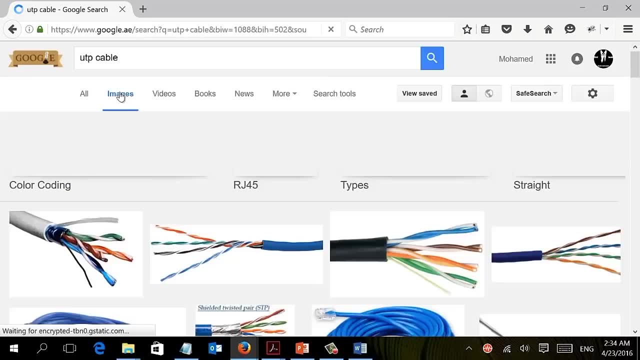 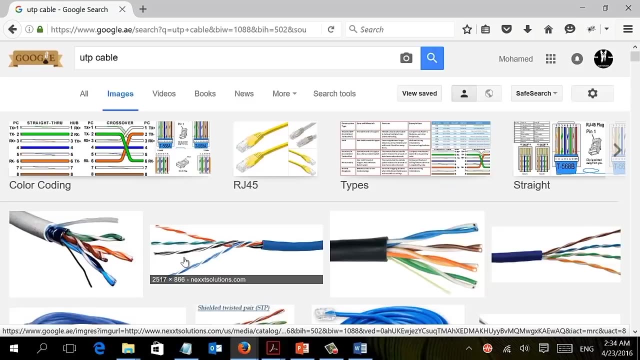 information about physical security, type of cam, type of firefighting tool, type of and this kind of thing. unless you saw it yourself, you will not be able to memorize it. so this is the utp cable and, as you can see, it has eight wire different color, and this is how we are connecting the UTP cable. there is a 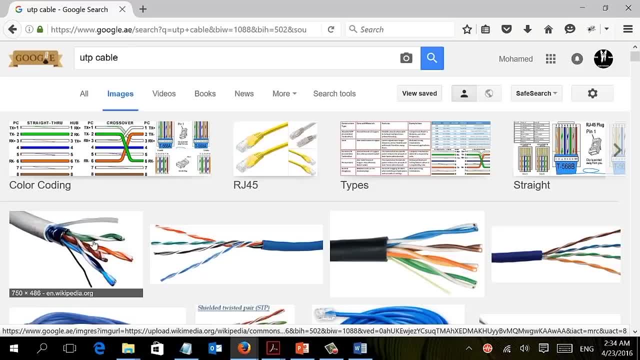 rose. a similar cable and actually UTP cable has different category of cat 3, cat 4, cat 5, cat 6 and each one has a speed. so cat 3: cat support up to 10 megabyte per second. cat 4 can support to 100 megabyte per second. cat 5: 1 gigabyte. 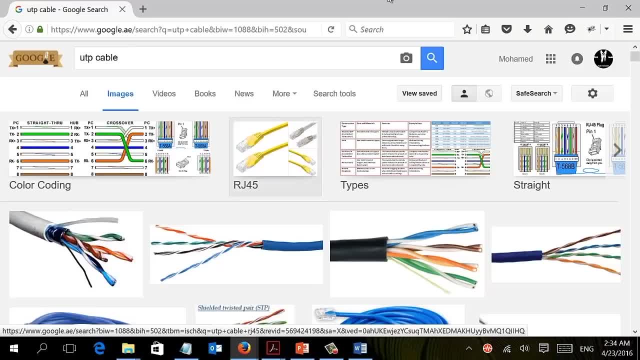 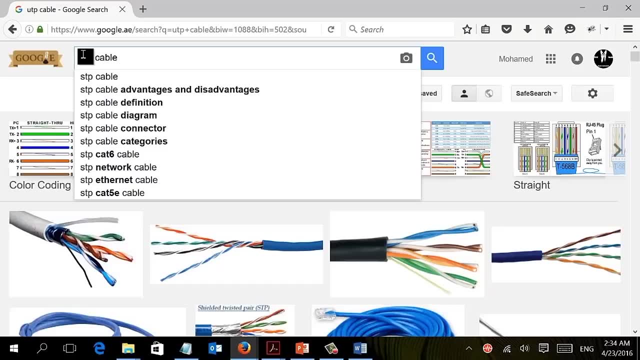 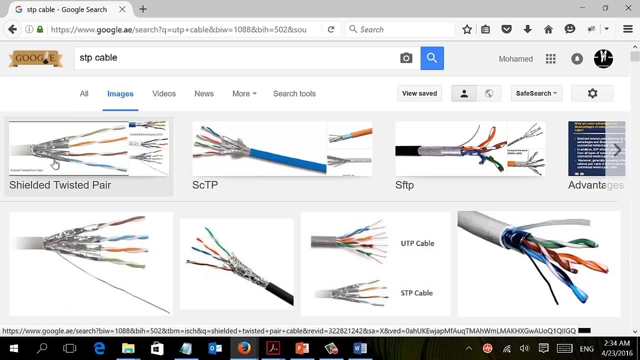 per second. you will find that in the sunflower. just have a small brief about them. we also have an STP. STP is a twisted shield pair and it has a shield on the outside, as you can see, which make it a little bit easier, or sometimes if 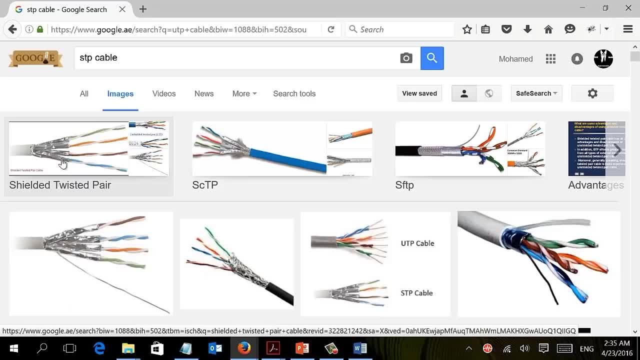 you are putting wire inside the place where there is electromagnetic field, it's better to have an STP, so this is the one used, in that there is some limitation for STP and UTP, which is that you can use the cable, which is that you can use the cable, which is the one used, in that there is some limitation for STP and UTP, which is that you can use the cable. 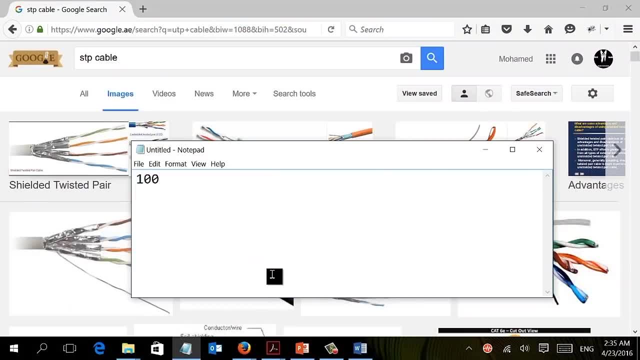 which is that you can use the cable for only 100 m meter, so you cannot have a for only 100 m meter. so you cannot have a cable long, as you know, one kilo or 200 cable long as you know, one kilo or 200 meters. limitation of that is distance you. 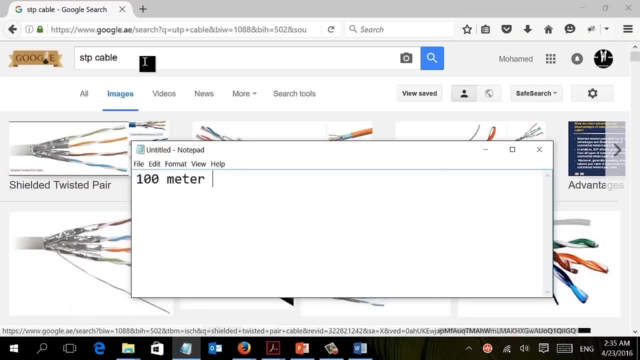 meters- limitation of that is distance. you meters- limitation of that is distance. you should have this cable between machine, should have this cable between machine, should have this cable between machine within 100 meter- okay. another type of within 100 meter: okay. another type of within 100 meter: okay. another type of cable is a fiber cable, and fiber we have. 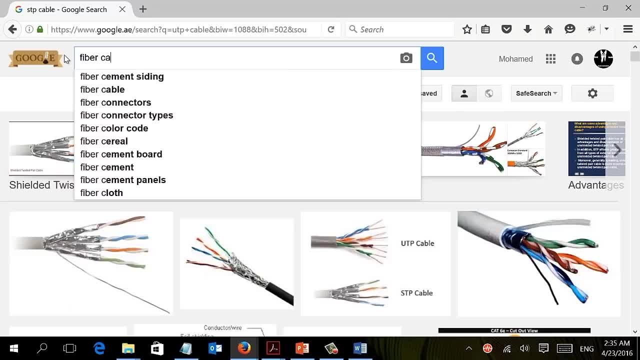 cable is a fiber cable and fiber we have. cable is a fiber cable and fiber. we have two different kind of fiber fiber cable, two different kind of fiber fiber cable, two different kind of fiber fiber cable. fiber is kind of complicated you, fiber is kind of complicated you. 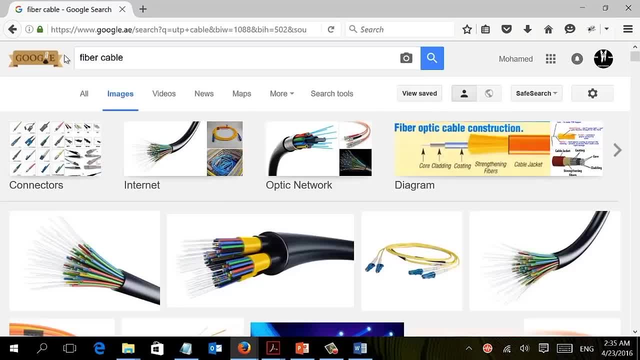 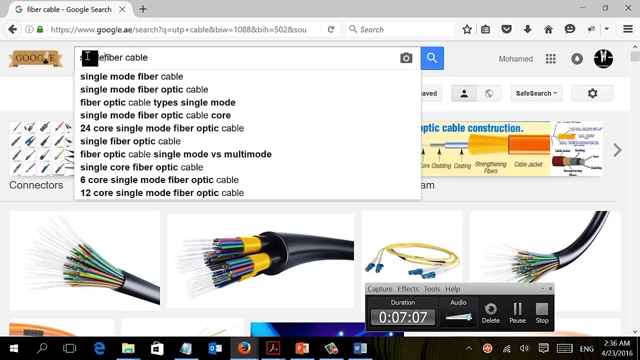 know it's, it has, you know, some specific devices and so on. but you should know that we have two different kinds of fiber. we have the single mode and we have the multi mode. so we have the single mode fiber cable and this is what ISP is using. I mean, this is a complicated one. single mode fiber. okay. 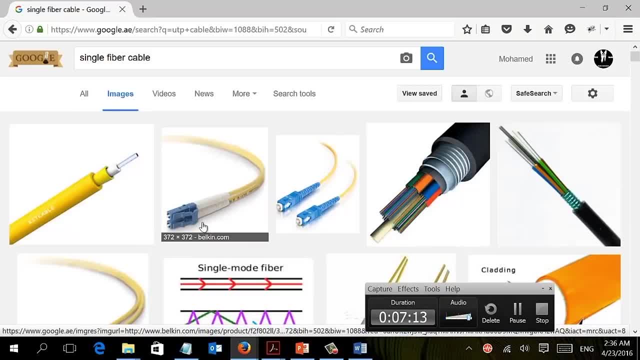 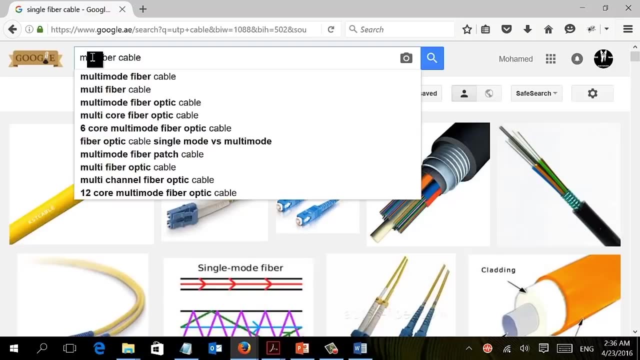 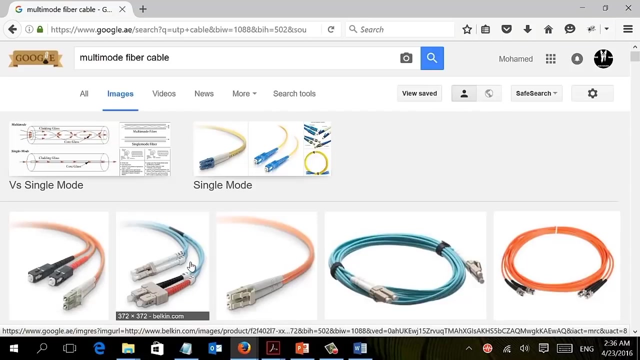 so this has to be done with an- I mean electrician need. to implement this kind of cable is very, very complicated, While we have another type- it's called Multi mode fiber cable, and this is actually can be used by users. I mean you can go and buy, it's very easy to implement and it just has some good. 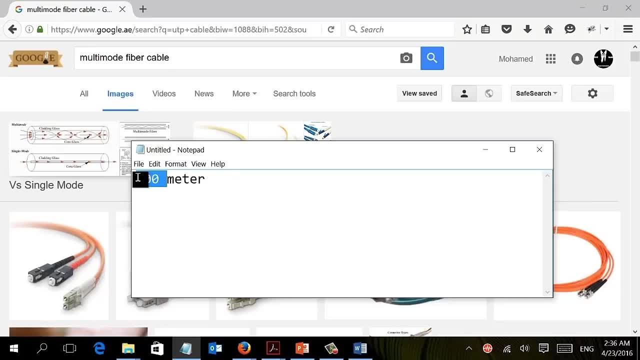 advantage- advantage over the UTP- that the limitation of this cable is 375.. So this is how far you need to know about the media. the cable Wireless will be explaining that by the end of this module, because wireless are using radio wave frequency and we have some discussion about that. So this is. 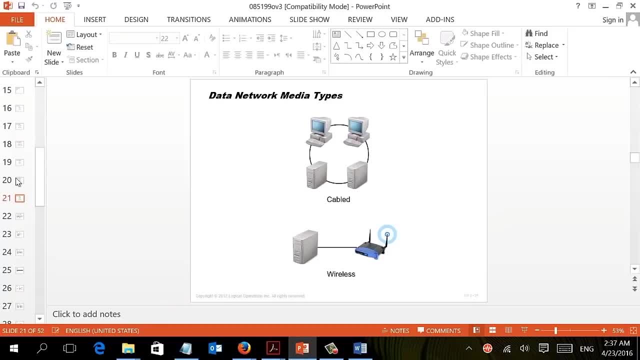 the medium part that you need to be aware, or the media that you need to be aware in the network. On this next lecture, we'll be talking about different type of transmission and I believe this one is going to need some attention because we'll be talking about 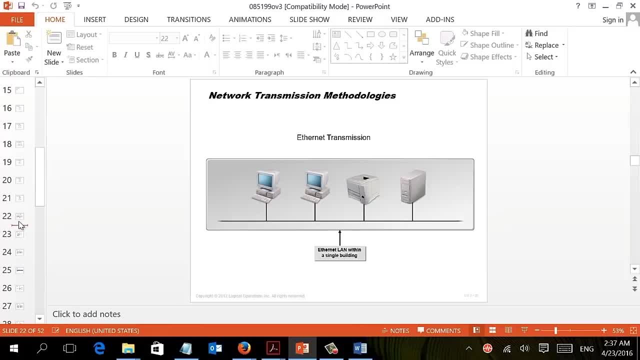 some protocols and you need to be a little bit focusing while we are talking about the way we are transmitting information between different devices. This will be a very important lecture in the network domain and I want you to give me some attention. Besides, please have a pen and paper and start taking notes about what I'm going to tell you in this part Now, because this part actually is confusing a lot of people when it comes to the exam. Here we will be talking about the remote access. 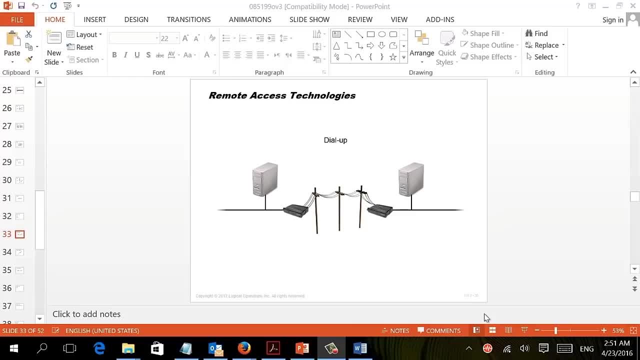 technology In the meaning of: assume that you have two different sites, Site A and site B, and you need to connect those two sites together because they are not physically located on the same place. You have one site in one city and another site in a different city. 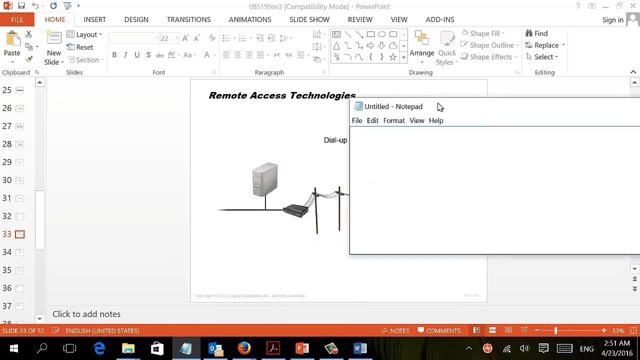 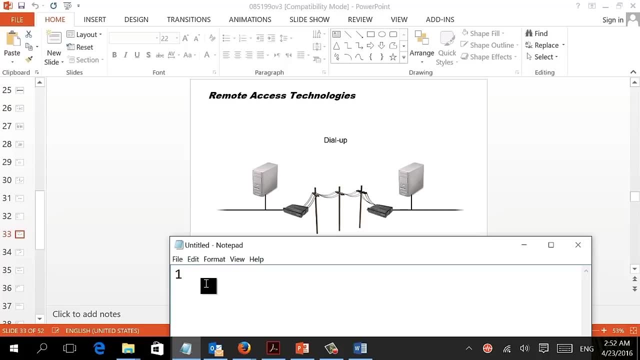 And you have been requested from your manager to connect those two sites. How many options do you have? Number one: We have this line, So we have a lease line Or a dedicated line. Now, the lease line is just a dedicated connection between those two sites. 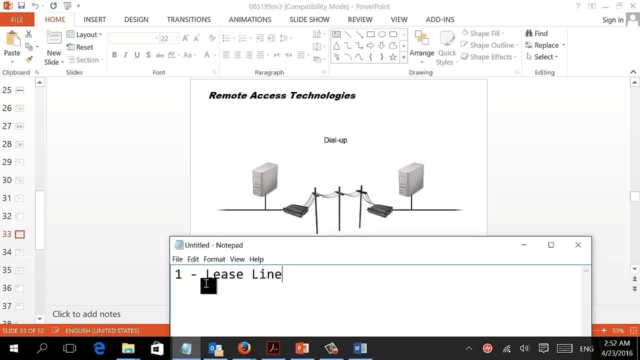 So you have one site in one state and another site in another state or city. You need to have one connection between them. You'll be going to your local ISP Or your telecommunication company. Tell them I need the connectivity between site A and site B. 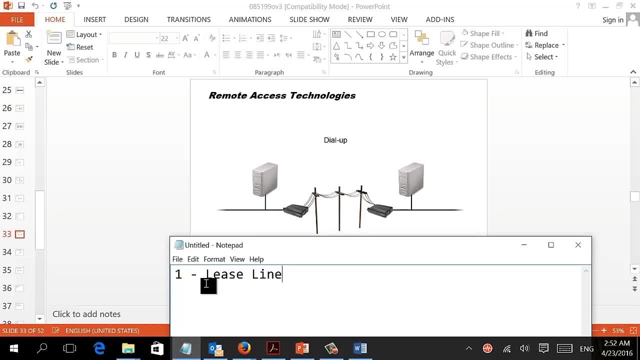 And they will give you a connection between those two sites. And actually they already have cables between cities, So they will give you a connection between those two sites and they will give you a plug inside the wall, inside your organization. We call that the demarcation point, where everything behind this wall is the telecommunication point. 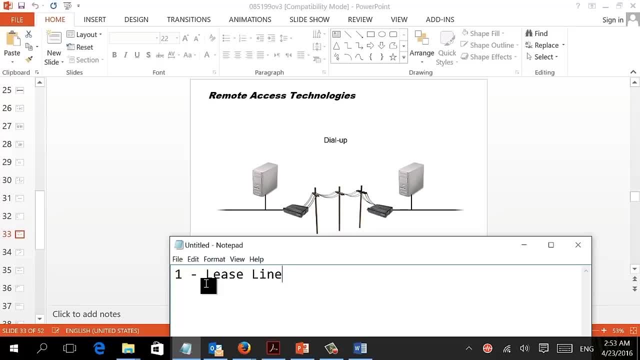 The telecommunication responsibility and everything after this wall which is inside your organization. It's your responsibility. Now, the good thing about the lease line is that it's a dedicated connection. I mean security is very, very high because it's just a dedicated connection between those two sites. 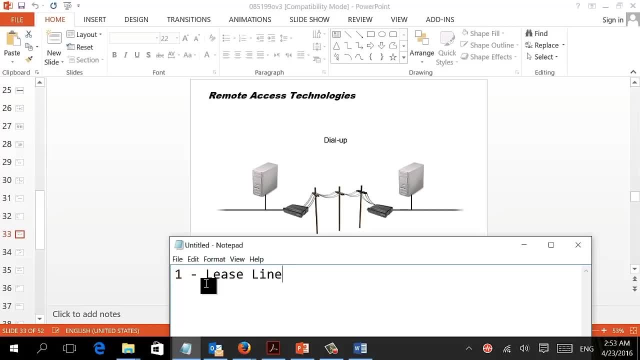 No one is there. It's not like the internet where everyone is connected worldwide. No, This is a dedicated connection between those two sites. But the problem with the lease line is that Cost. Lease line costs actually is very high. So if we have, we are talking about a couple of thousands of dollars per month around. 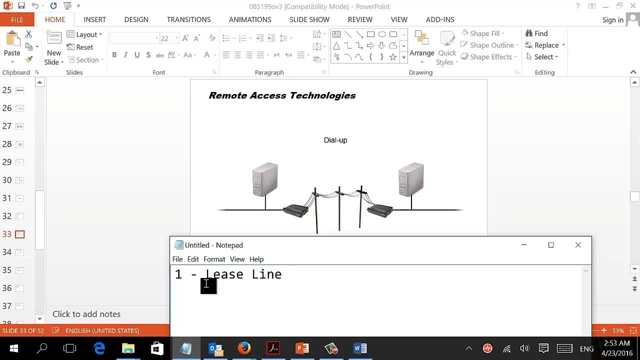 So if you have like five sites and you need to connect them together, This will cost you too much money. So the good thing is about the, The good thing about the lease line is about the dedication And security and the bad thing is about the cost. 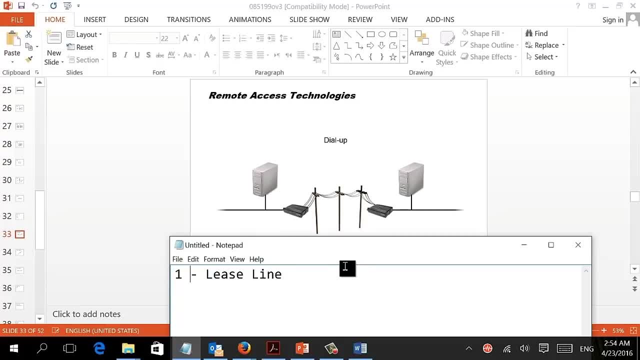 And we have different kind of lease line. We will be explaining the difference between them. I'm just going to give you an introduction. Then we'll be going and getting a brief about each one of them. So we have the T1 line. 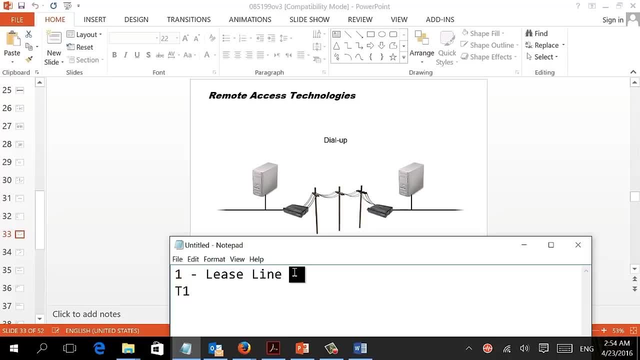 And we have the T3. And we have the E1.. E1 and T3. And E1.. You should know that T1 speed It's 1.44, I believe, megabyte per second. So it's not about the speed. 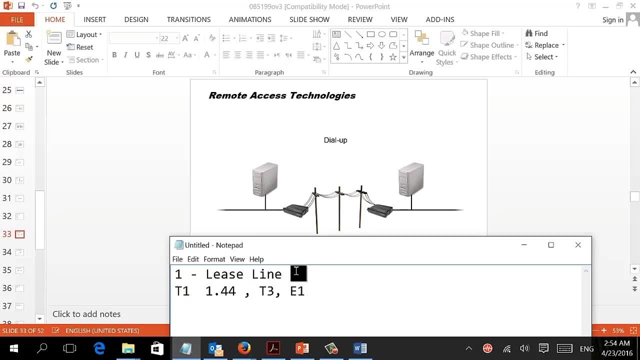 Lease line will not give you that high speed. It's about the security. So this will be the first option. Second option will be the internet. Now, if we are concerned about the cost- And this is actually kind of expensive to have those- 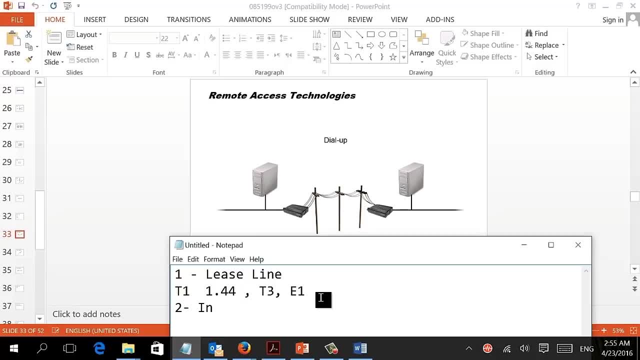 I need like 3 or 5 connectivity And I have to pay that amount every month. I can use the internet And the internet is a very good solution Because everyone has an internet connectivity. So we can connect those sites together through the internet. 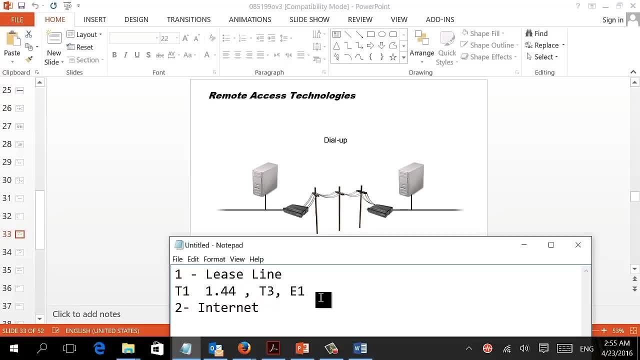 What is the advantage and disadvantage of the internet? Advantage is definitely the cost. It will not cost me anything. Everyone now have internet at their organization, So I just need to have a connection between the site. But the problem will be the security. 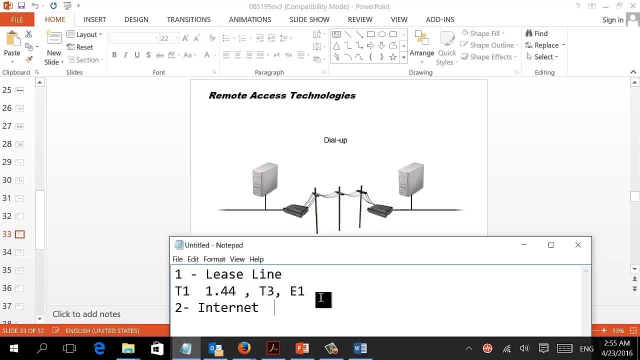 Because this is a public network. Yes, we can over like pass that, Or we can solve that by using a VPN connection, And VPN will be explained here as a brief, But it will be explained in more depth into the cryptography. So the problem is when I'm sending and receiving information through. 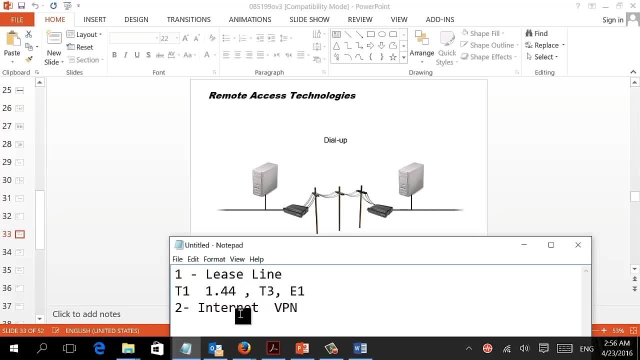 The internet. It's a public network. I mean it can be captured by anyone of this network. So I can solve that by implementing a VPN And VPN, which is a virtual private network. I can create a tunnel between the two sites through the internet. 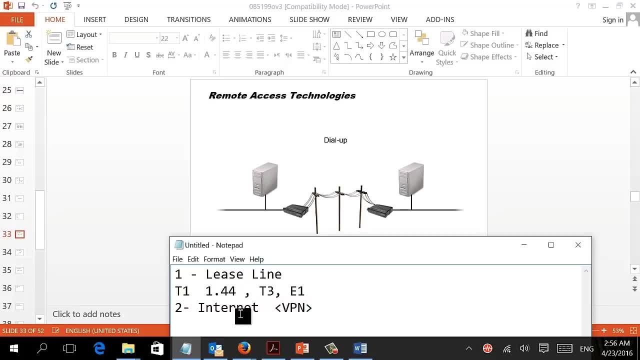 Where traffic will be encrypted between those two sites. So even if someone was able to capture this traffic, He will not be able to read it. So I can create an encrypted tunnel between the sites, But still security will be an issue there. Now there is actually one solution between those two solutions. 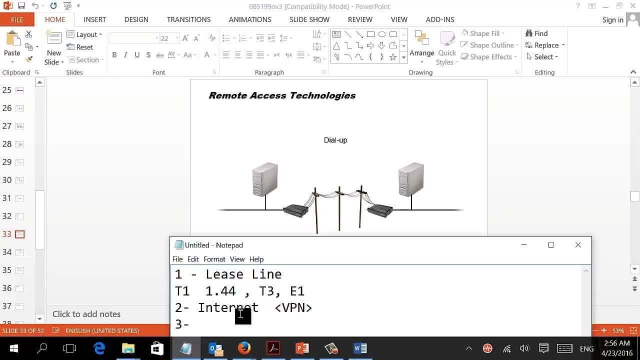 Which you know has been found in different name. It used to be frame relay, Frame Relay, Or another version was called ATM. I'm not talking about the ATM Banking ATM. There was a technology called ATM And now we are using. 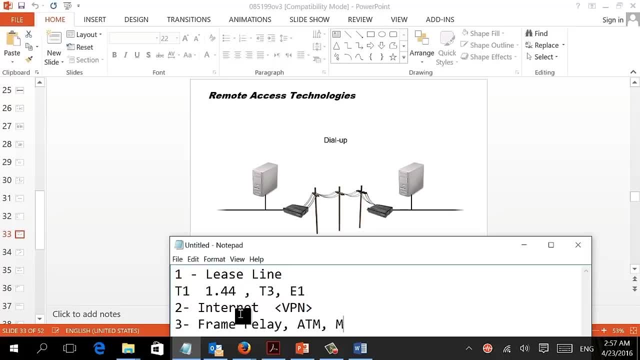 Today, technology, we are using MPLS. They are all MPLS, They are all on the same category. It's a category between the lease line And the internet connectivity, And using a VPN. Let me explain to you the concept of frame relay. 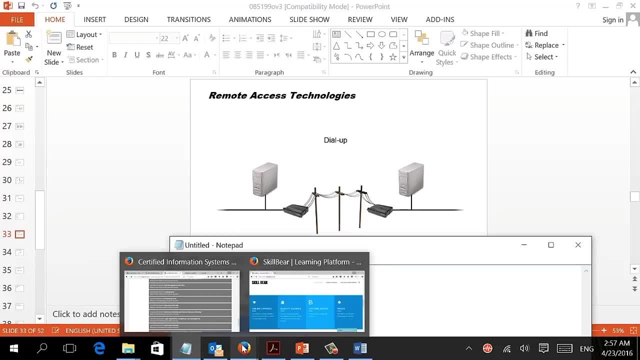 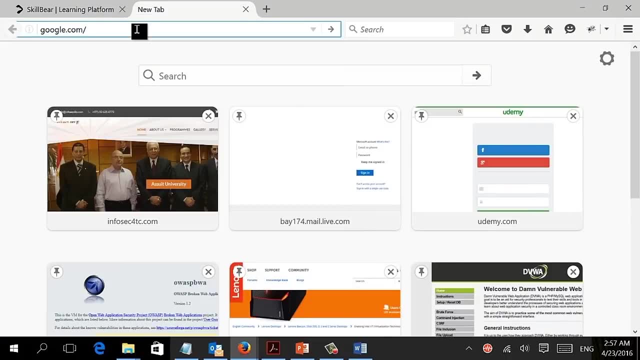 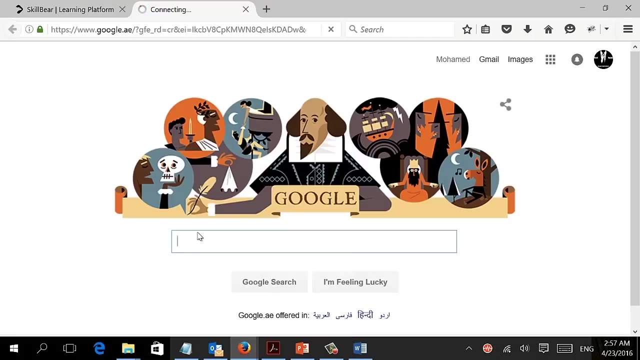 And MPLS and so on, Just open here. Let's go to Google And let me give you a brief about frame relay. Now, the thing with the lease line Paste, The thing with the lease line That no one is using. 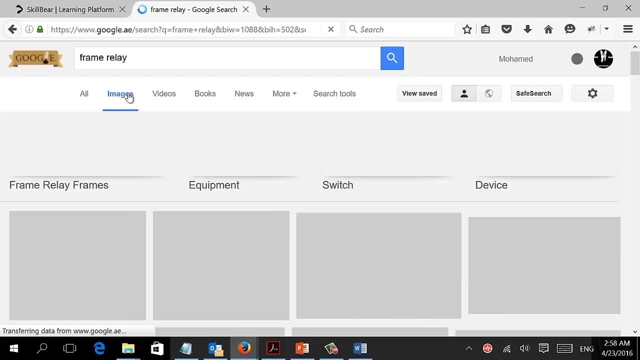 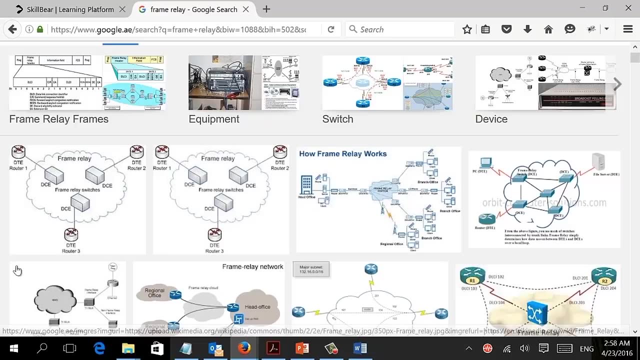 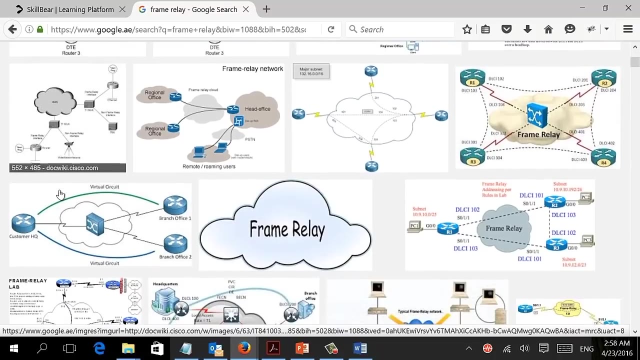 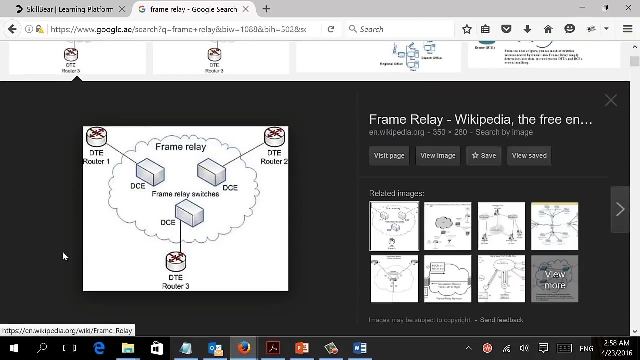 I mean, if you, as an organization, has a lease line, You'll notice that no one is using The full bandwidth All the time. Okay, Let's take this scenario, for instance. Or Yeah, This will do So. They take an advantage from that. 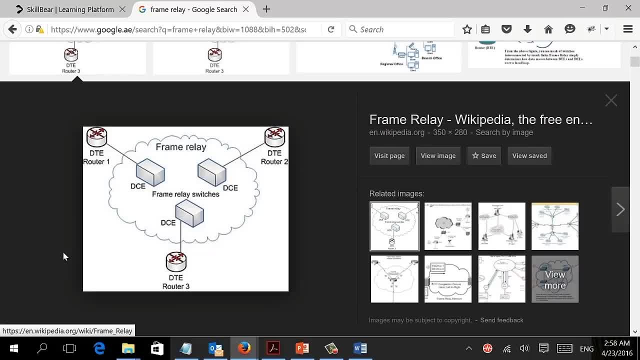 So if you have a lease line On your organization, You'll notice that you are not using The full bandwidth 24-7.. And also other customers are not using The full bandwidth 24-7.. So the idea of ATM, 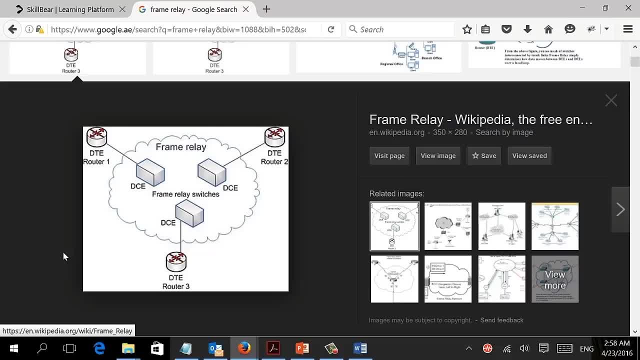 Or frame relay Or MPLS In the most of the concept That, okay, Let's do this Because no one is using The full bandwidth Full time. Let's have Three Lease line And give them Two. 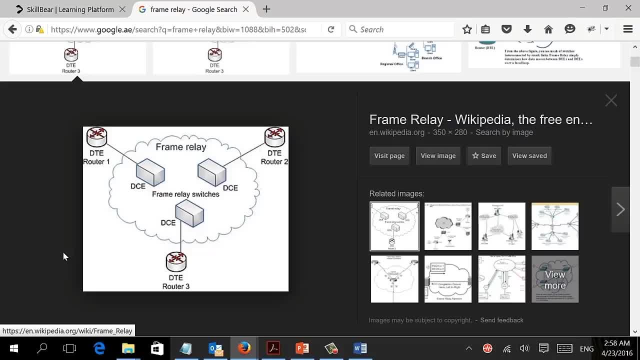 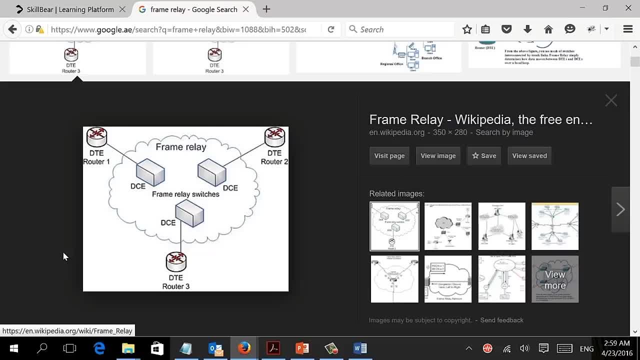 Six user Depends on That. no one is using The full bandwidth 24: 7.. And when you go to subscribe For a frame, Really You will be writing Your Or it will Be Giving to not have less than that amount. okay, so they are giving some lease line to more. 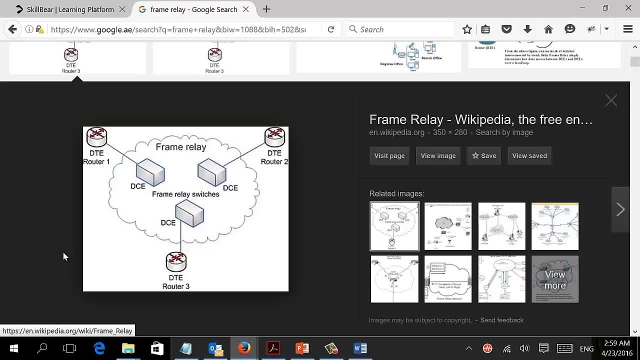 amount of customer and by doing that they are utilizing the bandwidth and the effectiveness of the lease line. so frame relay or ATM or MPLS, they have some difference but the concept is it's same idea of lease line. it's little bit public, I mean between different customer, but they are well-known customer. 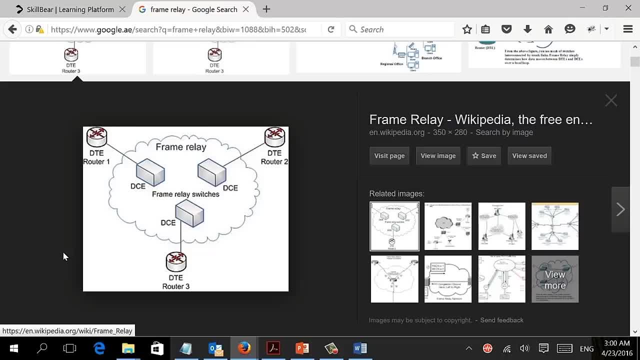 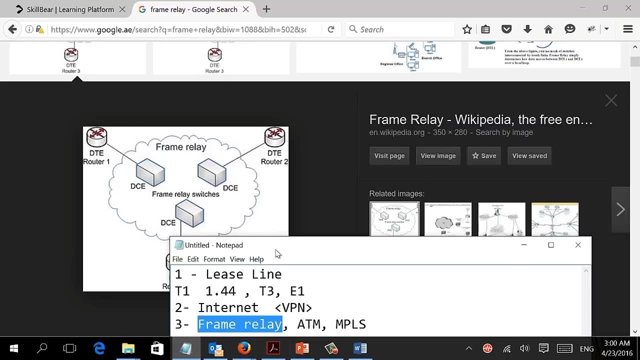 but it's not public as the internet. so you have the effectiveness of the cost and you have the security of the lease line. this is the idea of frame relay, MPLS, ATM and so on. now, what other methods remaining for the remote connection? do you remember on the old day how we used to connect together or to the internet? 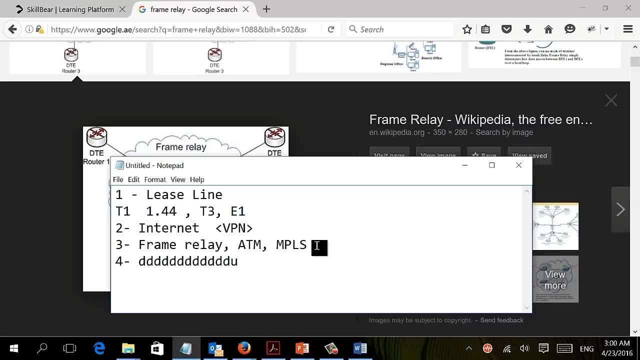 there was a dial-up connection- right dial- so the force or one of the remote connection method was dial-up. until now some people are using dial-up. I mean some places do not have internet, high speed internet. they will use the internet to connect to different sites, so still is used. now what do I need to know about those different kind of? 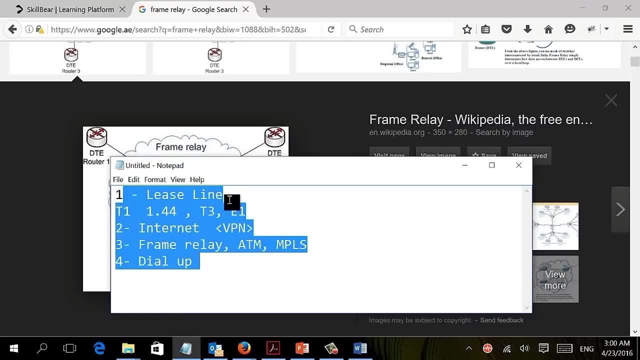 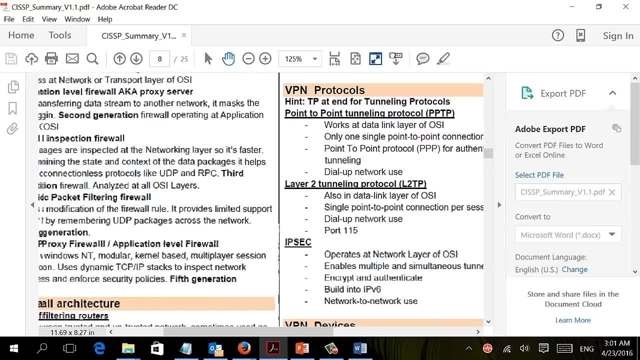 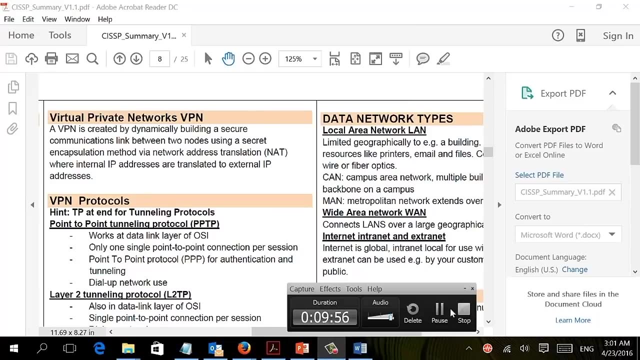 remote connection, for the example, is you need to know their definition and you need to know some details. how deep. let me show you. so if you go here and we go through the different protocol, so, for instance, let's take the VPN, or actually let's start with lease- 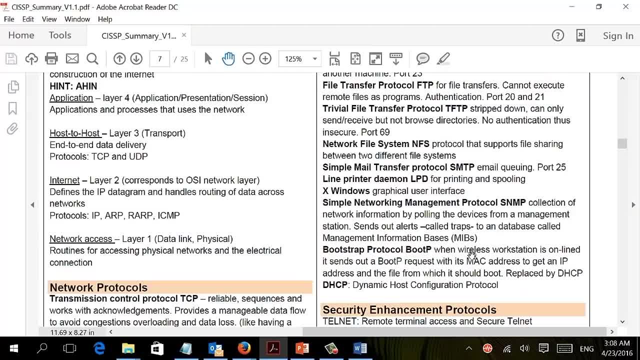 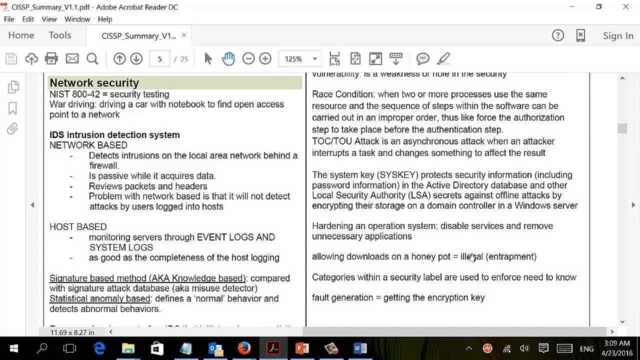 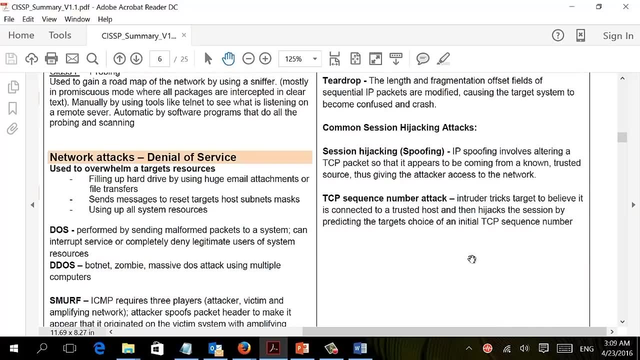 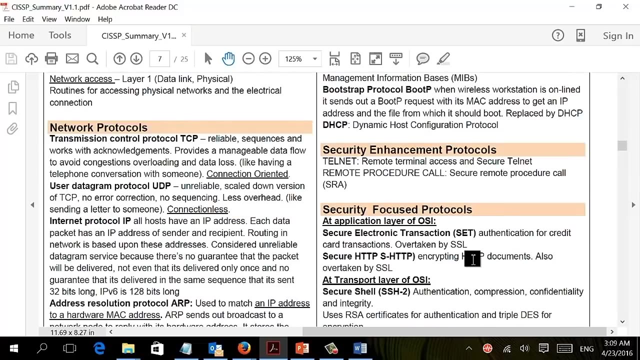 line. now this part. I want you to give some attention to that and I want you to highlight some of the important point, because it's quite important. so let's start with the different remote technology specification. and what exactly do you need to know when it come to remote technology transmission, we need the least line. this is it should. 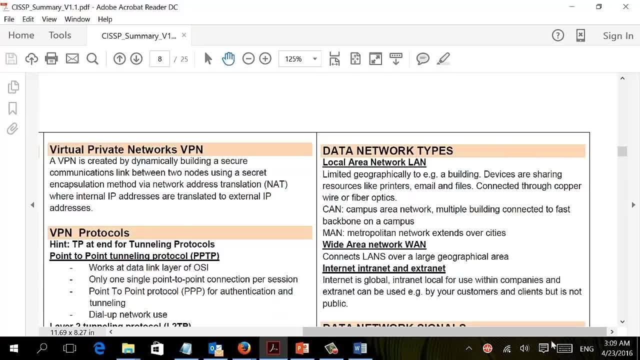 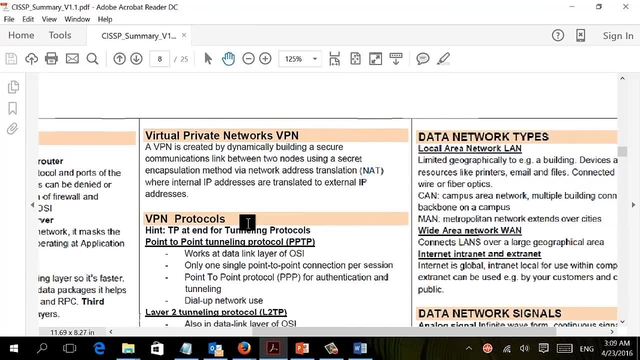 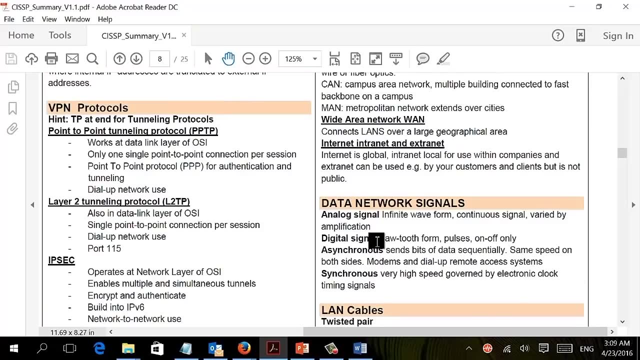 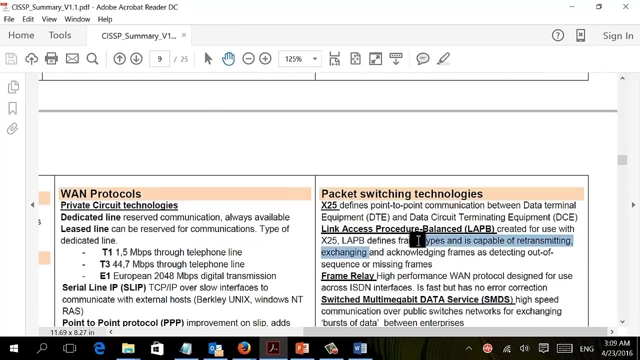 be here. yes, okay. so Firewall, VPN, VPN- We went through that Data network type. Yes, here you go. So we're going to start the same way. we had The discussion first with the lease line. What is a lease line? Okay, this is one dedicated communication. How many type? 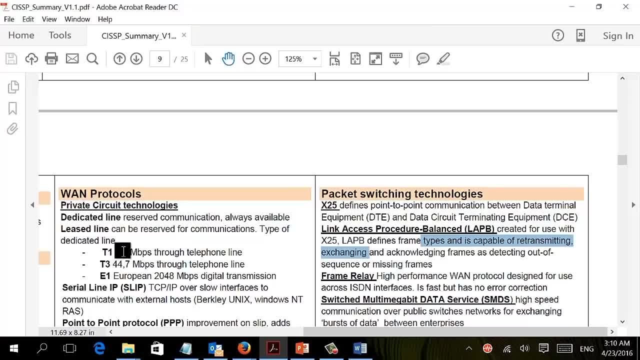 We have. you need to know the three different type. We have the t1, the speed Is 1.5 t3 for 4.7 and e1 European. This is up to 2048 megabyte per second. Okay, so the first part. 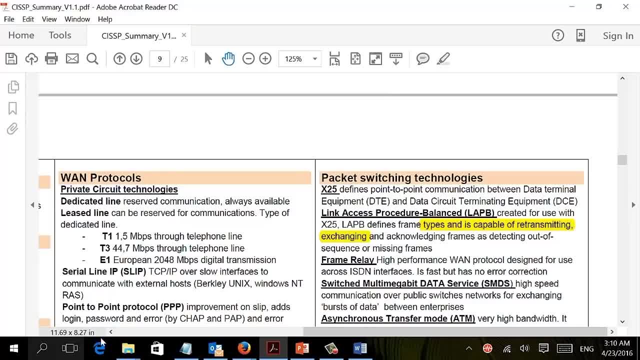 That you know. you need to know about the dedicated line or lease line. They are considered the same. actually, There is some difference between them, but they are considered the same. So the First point, which is the speed. you need to know this part. Let me just highlight it. 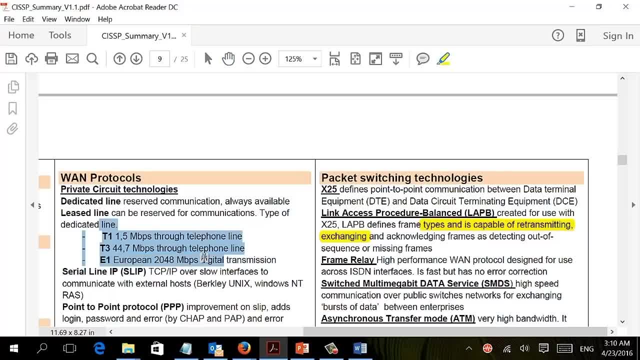 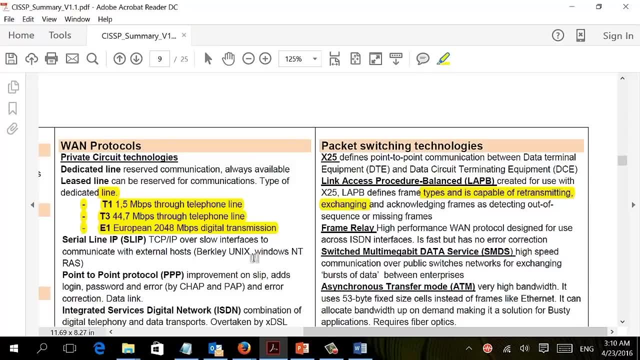 Just to point to the thing. Okay, this Is the first part. second, which is very, very important: protocol. What protocol are used in this line? We have the Major protocol, that the generic- I mean the one that is used everywhere- is called the PTPP. 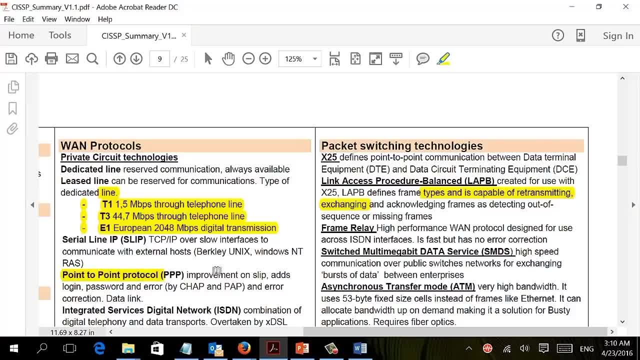 Point-to-point protocol, and this actually it's What we are using right now, but before that there was one called slip serial Line IP, And you need not just to know the name of the protocol used. but what is the Difference between them? What is the difference between slip and PPP? Both of 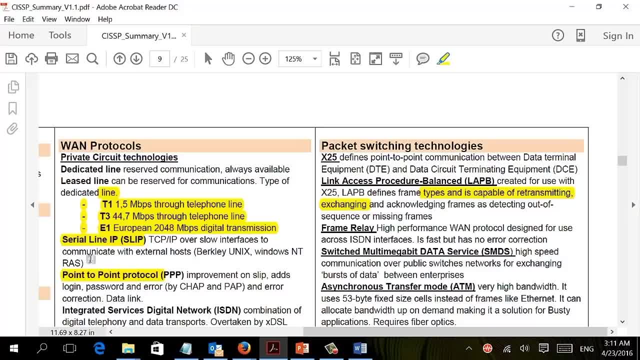 Them are this line protocol, So this one, for instance, Show interface to communicate with external host, can be used over remote Access server press, while the PPP- and this feature didn't exist in slip- can Use some authentication. This one didn't have An authentication and you can use the authentication sharp and PPP. This is a 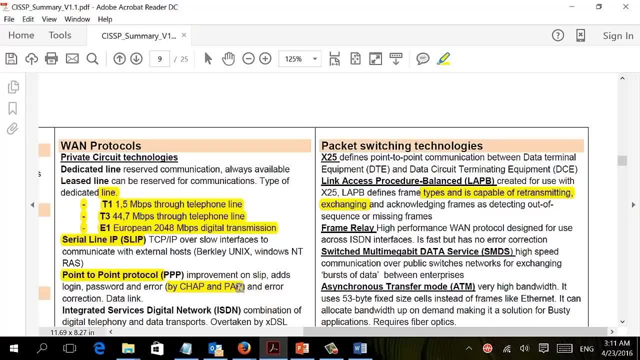 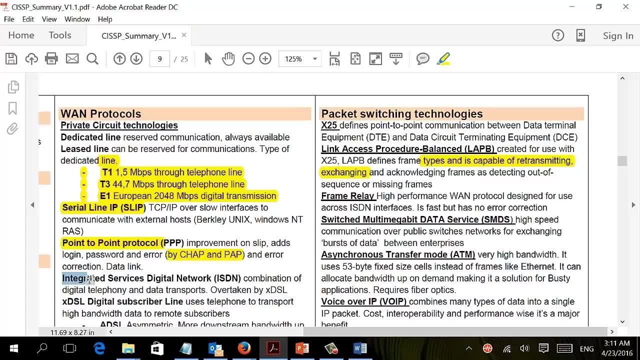 Method for authentication, sharp is a new one. PPP can send text in clear, can send Information in clear text. We have also ICND and, okay, this is also used. no, but Actually this is a different protocol. So for these lines, those are the two. 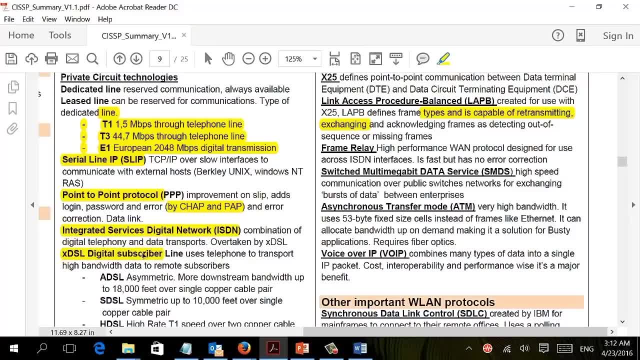 Protocols that you need to know. then we have the DSL one connectivity and we have the ADSL SDSL. Those are some major. what we have at home is usually a DSL- asynchronous DSL. why the- I'm sorry, asymmetric DSL, while the ones that businesses use is 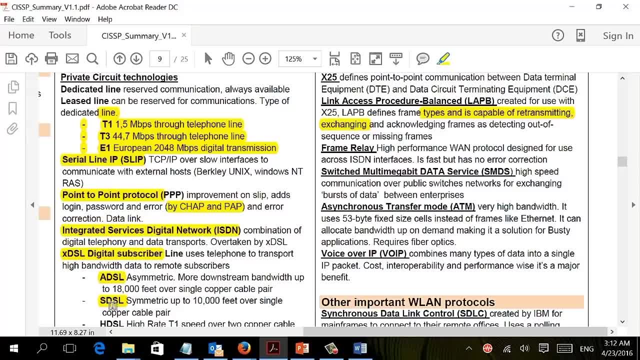 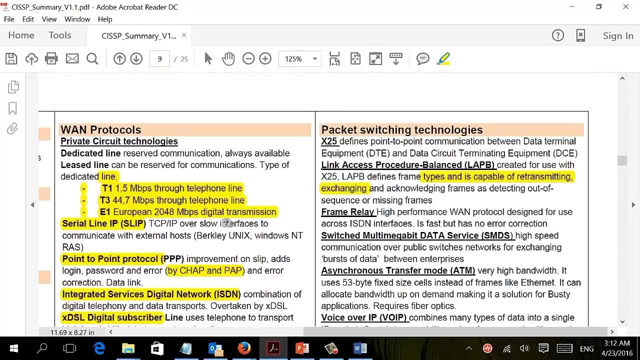 Symmetric DSL. What is the difference between them? The ADSL, the amount of Download. it's higher than the amount of upload, while the SDSL they are equal Amount. What else do we have? Yes, Now we're going to talk about the packet switch network, and this is the network. 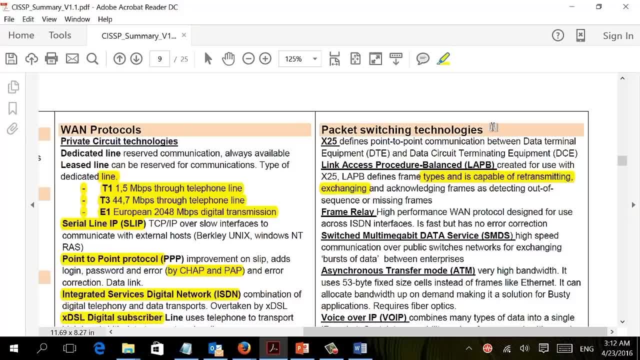 That was between the internet and between the lease line, which is the frame relay, and ATM and so on. So you need to know before it is lines or the x25. We have a frame relay and frame relay. So, as you can see, how far do I need to know? just a small introduction about that, like for 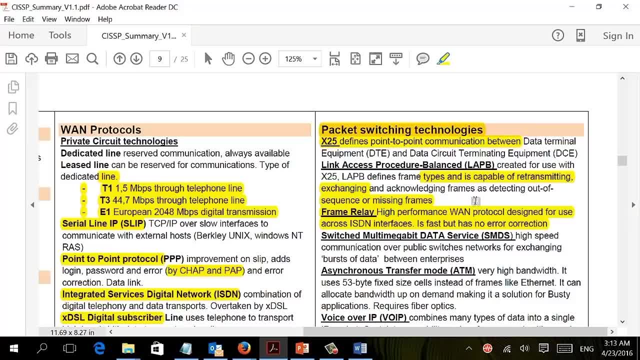 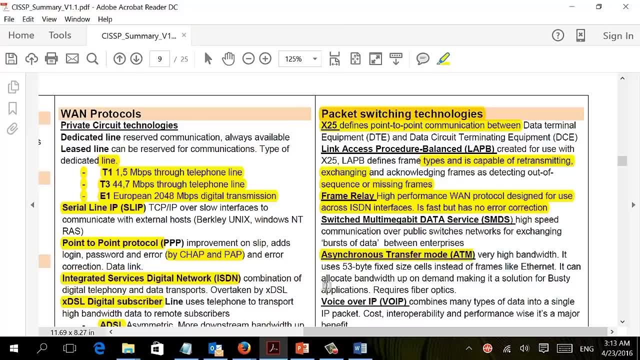 instance, you should know that we have the ATM, Yes, ATM. What is the specific about ATM that is used? a specific size, 35-byte fixed-site cell. So each cell is 35, 53 by. so you can see that small world are there. 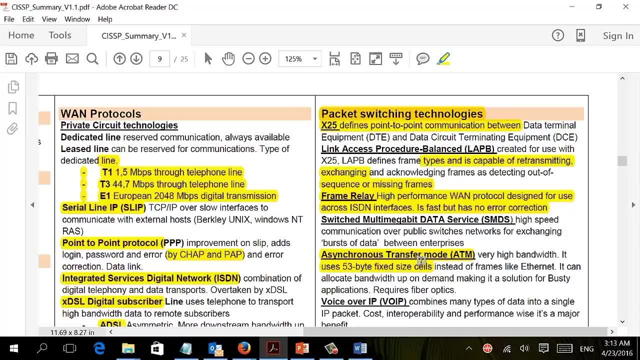 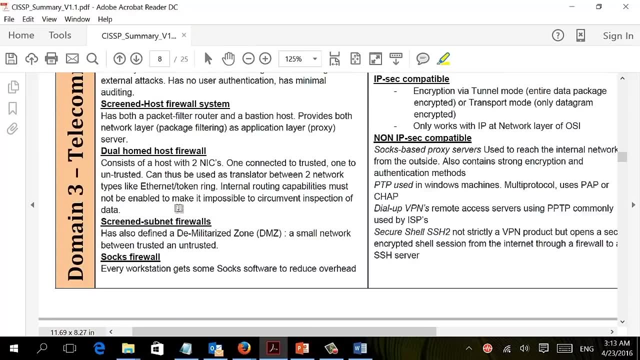 He will tell you, for instance, which packet switcher network has a fixed site: 50, 53 byte size. So this is how far you need to go. Now let's talk about VPN, VPN, As I told you, just going to give a brief right now, but our main discussion will be about VPN, will be. 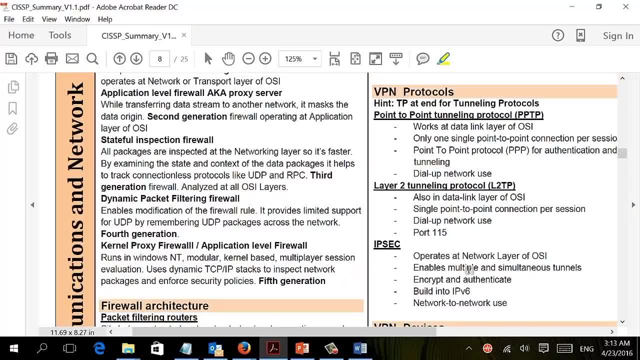 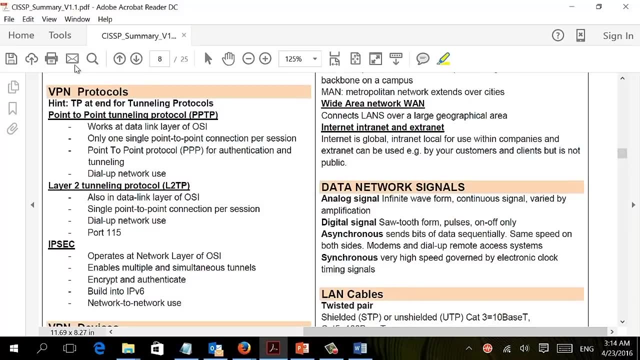 during the, during the cryptography, now VPN- We have two different protocols. We have the protocols that we are using over the internet and we have a VPN protocols that we are using over dial-up. So over dial-up we used to have point-to-point tunneling protocol called PPTP. 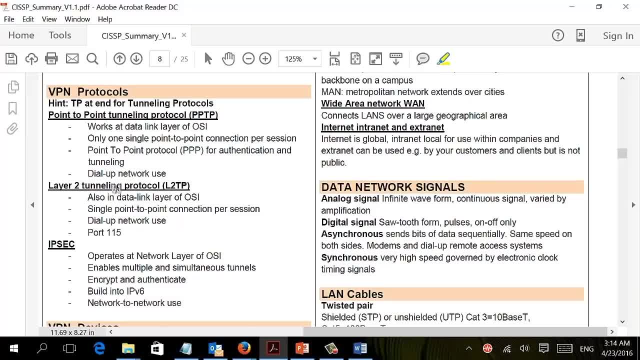 And, as I told you, check what is remarkable when it comes to definition. So, for instance, this is a point-to-point protocol, mean I cannot connect to one machine. too many machine should be one machine to one machine. It's a tunneling protocol and it's used in dial-up network only. 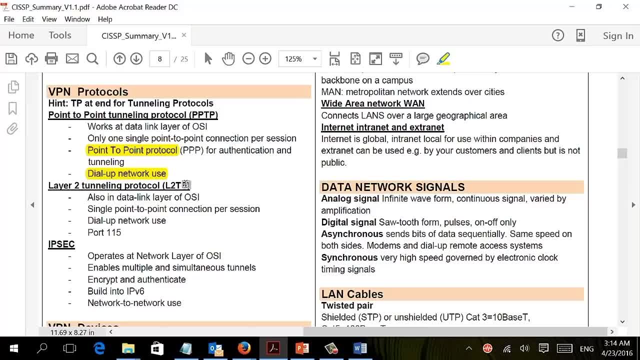 It's not used over the internet while L2TP, This is also a point-to-point, single, point-to-point, same and it work on port 15 and also on dial-up. Now on the internet to use on the internet, to use a protocol: IPsec, IPsec. 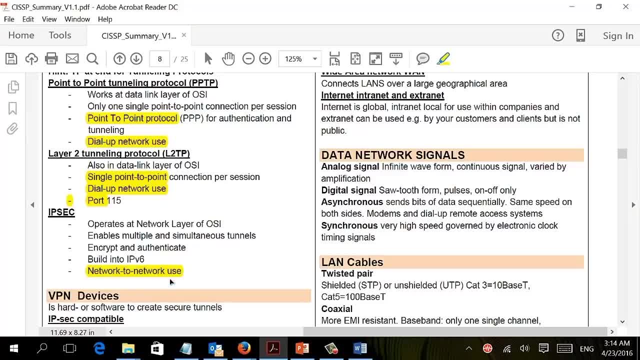 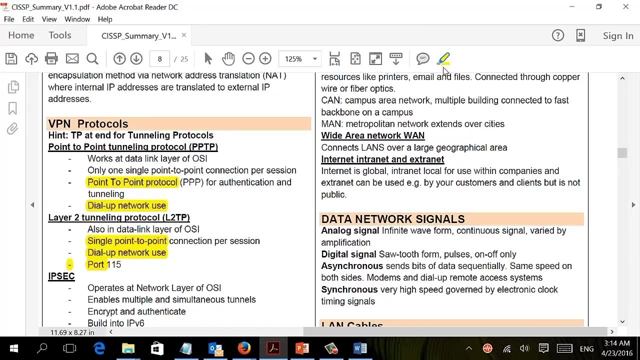 It's a network to network. So see, this is remarkable difference and it support IP version 6 and it's operate on network layer. So you just need to read those kind of definition to P2P. now, starting from here, You'll find that a lot of definitions is there and a lot of terminology is there. 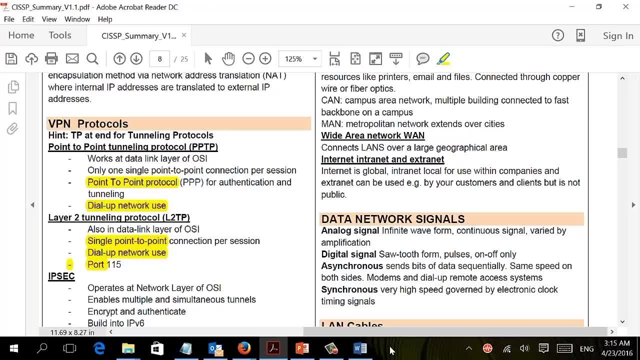 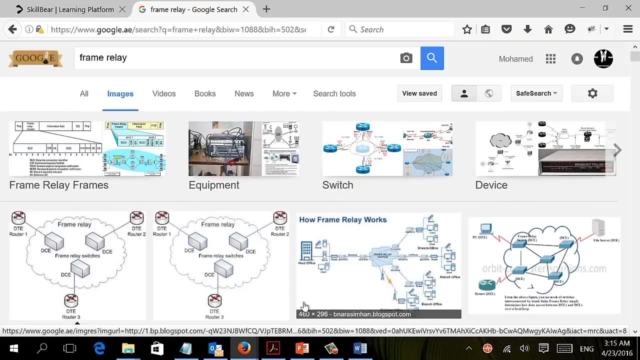 So I will suggest to you Some way for studying that I believe you will find it very effective to memorize when it come to big amount of information, and I tried that myself and I found it very, very effective way. Okay, this, this is a way for studying. method of studying is called mind mapping and I believe maybe 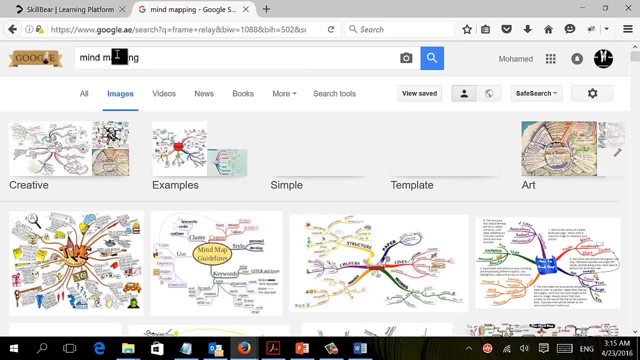 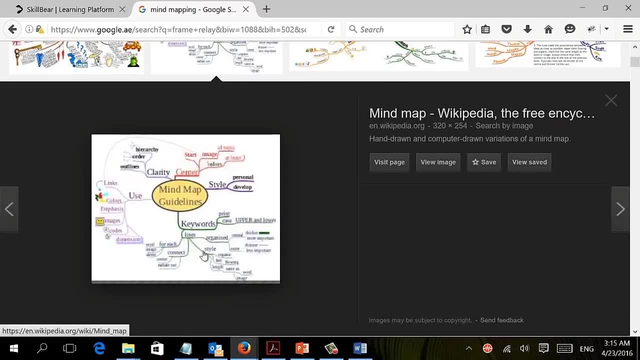 some of you are aware of the technique Where you are drawing the thing, So you start drawing the information. So for instant, Okay, you can put here Network, and then from the network We have the remote connection, We have the network types. 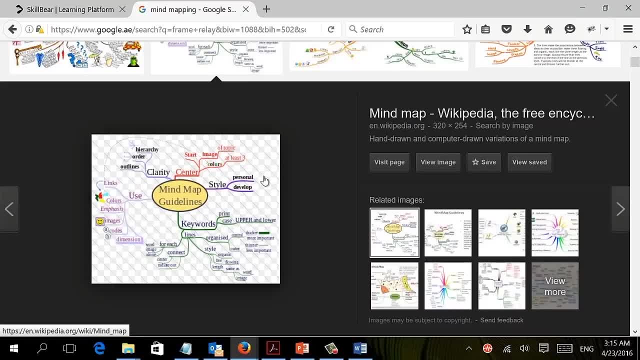 We have the and then you put from the network type, We have a remote connection, We have a VPN, We have a lease line, We have the internet and our frame relay or switch it Network and from this one we have those protocol and you put picture and smiley face. 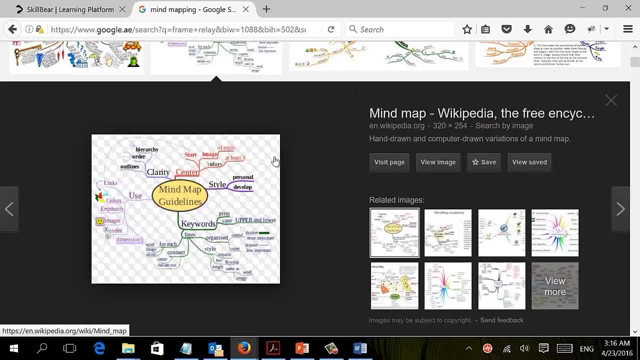 Then frame relay as a technique for studying. It's a very, very effective way- and I tried that myself- especially in those kind of topics where you have a lot of memorization and it has a scientific explanation, because they are saying that you it's easier to study or memorizing pictures and word. 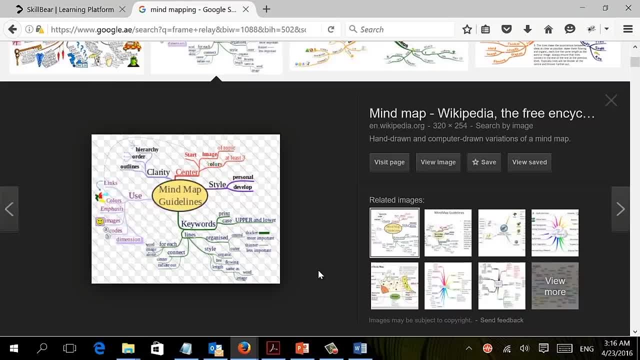 So according, or actually you will find with this specific lecture, You will find my mind mapping Implementation for the network. but you should not study mine. You have to do your, because this is how you can memorize that, and if you are not very good in drawing, you can do that using a computer application free. 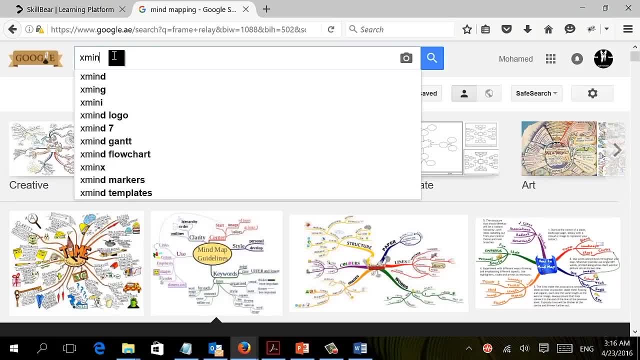 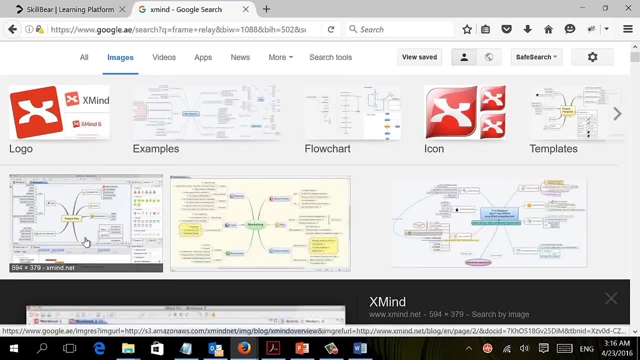 It's called X mine, X mine- This is what I'm using, but it's on my other computer- is not here- and X mind- It's a way for my mind mapping like this one, very easy to use and you can search on YouTube for any video. 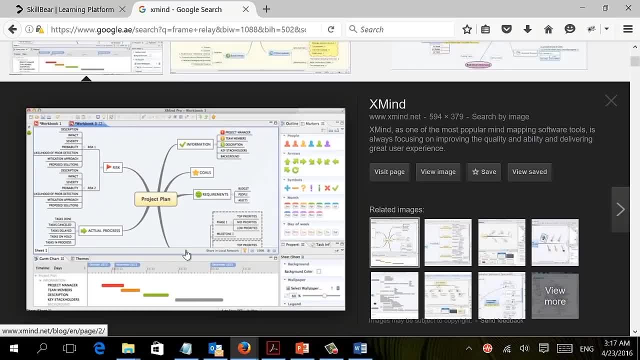 It's very easy To implement, but I believe this is very effective when you study a topic that has a lot of terminology. so this is a thing that I want to share with you, and I'm going to share with you some mind mapping document and- but you have to do your own. 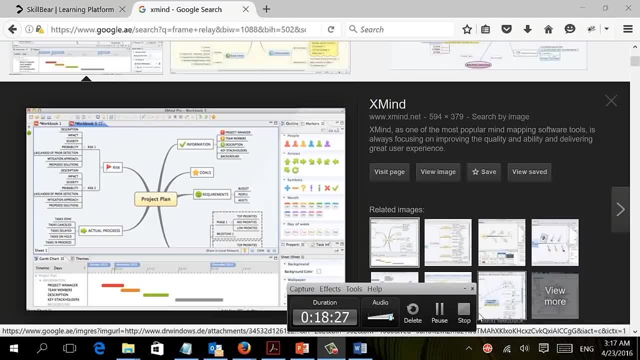 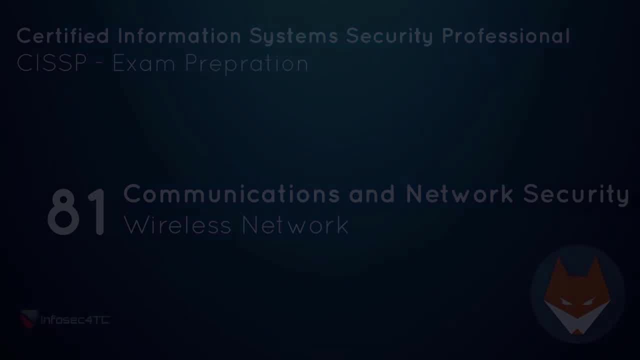 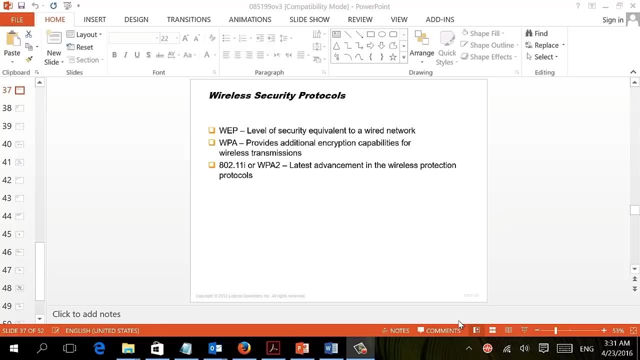 mind mapping This. we will be talking about wireless security protocol and I just need to give a brief about wireless, how it's working and what should you consider. now, wireless, it's a different kind of network and wireless, as you all know, are working on radio wave and the radio wave frequency. this is actually where all the 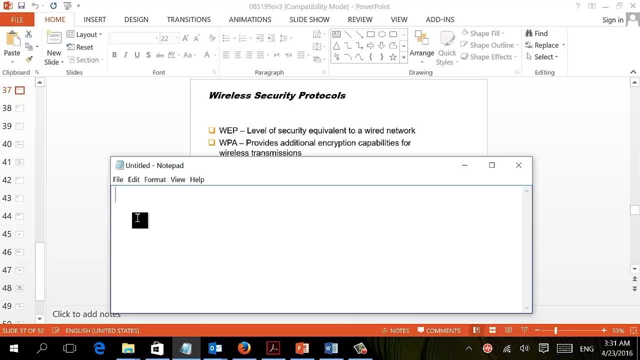 law enforcement and government and mobile and everything are using to connect. so when you are using a radio wave you need to have a license, except for a specific frequency, which we call the unlicensed frequency, and this is where all our device are working on the unlicensed frequency. these are 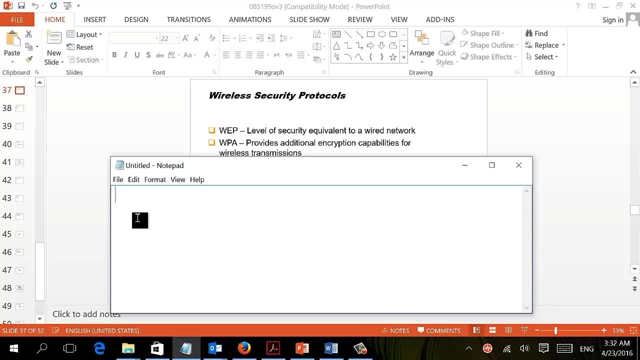 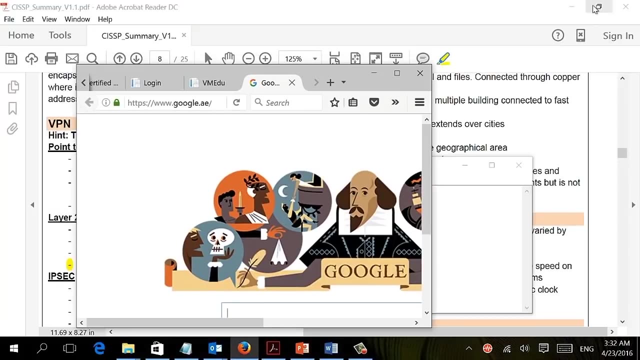 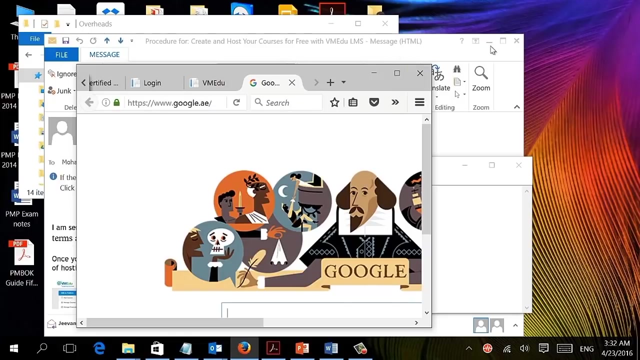 frequencies that we are using and do not request any license or permit. so in wireless, when you configure a wireless, what do you do when you configure a wireless network? let me just open a router and let's see how the wireless router is configured and what should you consider so a very good way. 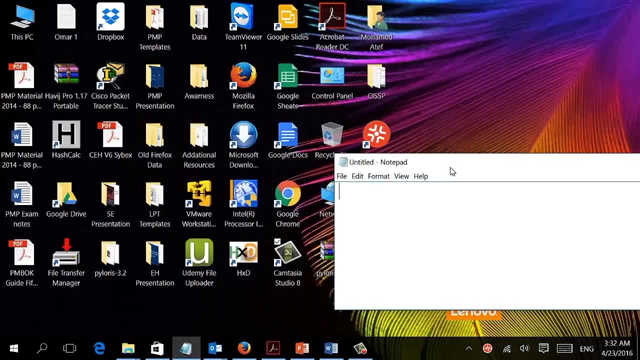 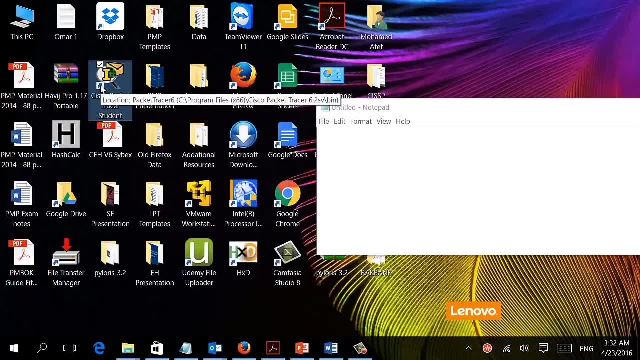 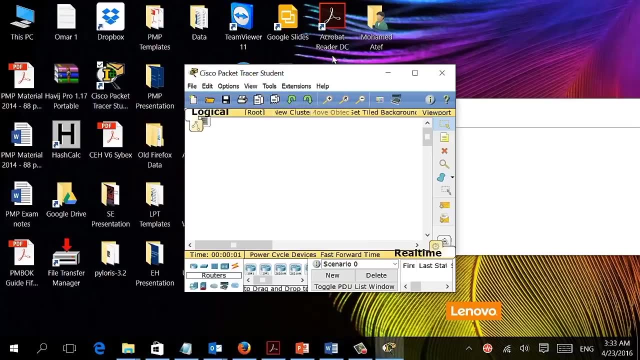 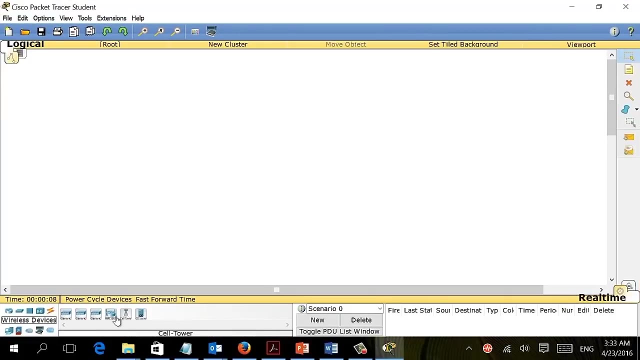 for testing. that will be a packet tracer software. they have a feature related to wireless. where is it? where is it? here you go. so let's assume that you are building a wireless network. what do you need to consider and what setting are you putting? so, assuming that I will build a wireless network, okay, this is my router and we're 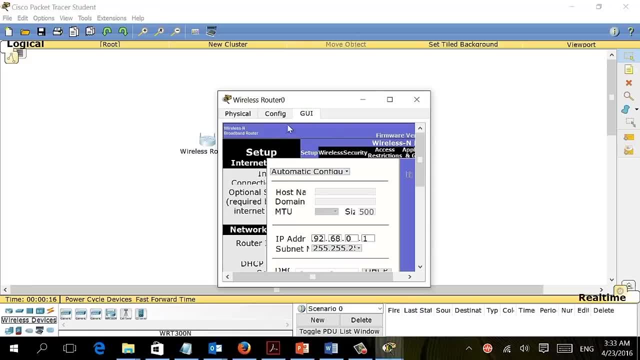 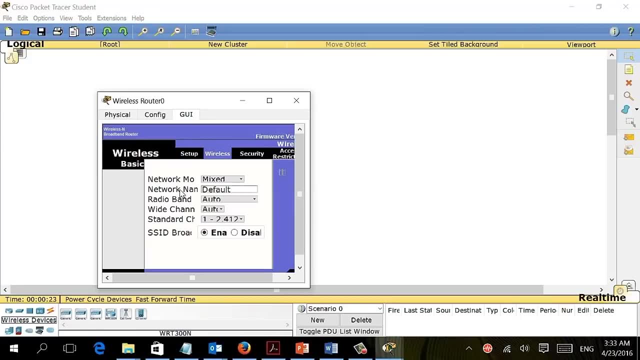 gonna go to GUI so it would be easier to configure and I'm sorry the size is a little bit small, but you know I'm going to configure it and I'm sorry the size is a little bit small, but you know, get the point. so let's go to wireless configuration. so what is fixing the 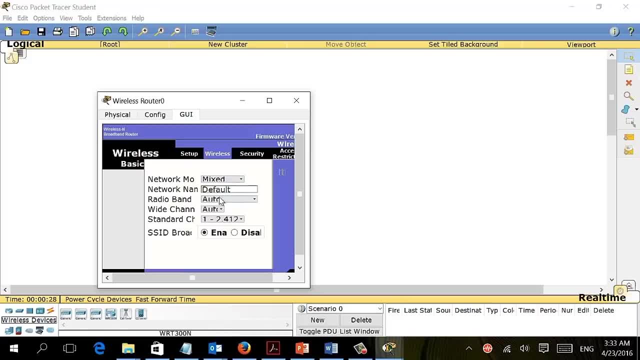 first I'm going to configure our wireless signal everyday most devices. first thing that we need to do is to configure an SSID. maybe it's not showing here because the size is too big, so we need to configure here the SSID, which is The name of the network. SS ID is the one. 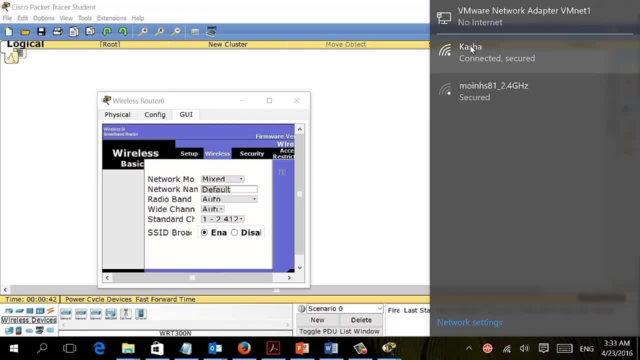 that showing which someone is scanning the network. I mean you click here and you find some network there. those are called SS ID. now SS ID is mandatory, except I mean mean, if you didn't write anything, it will keep the default one. so you should write something in. 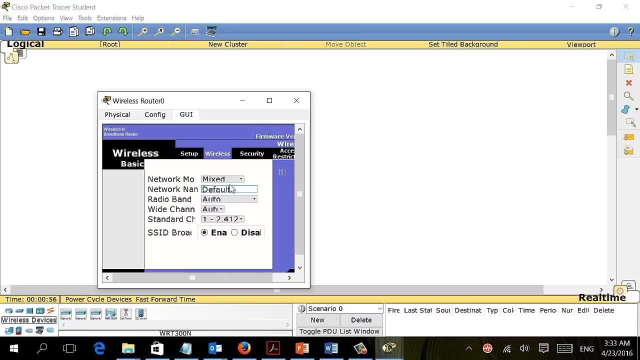 an ssd. now the first question is: when you have an access point or a wireless router and you put an ssid, is your and start you are and then start scanning using your laptop or smartphone to get access to this wireless. is your smartphone or laptop, who is the one? who's scanning, or is it? 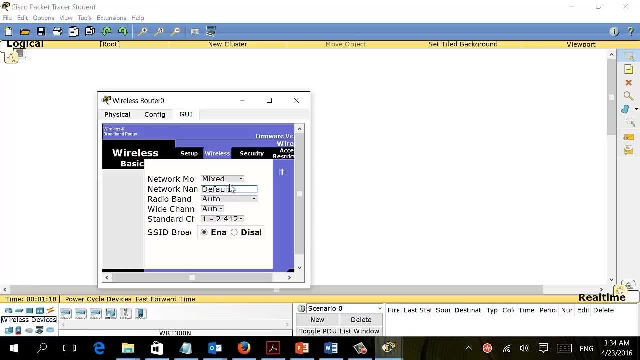 the access point, or wireless router, is one announcing about itself. actually is the second one. when we are assigning an ssid to any access point, he will start announcing about itself, telling: i am here and my name is sad and what happens is that your device will just capture this packet, so he will be knowing the smartphone or laptop that 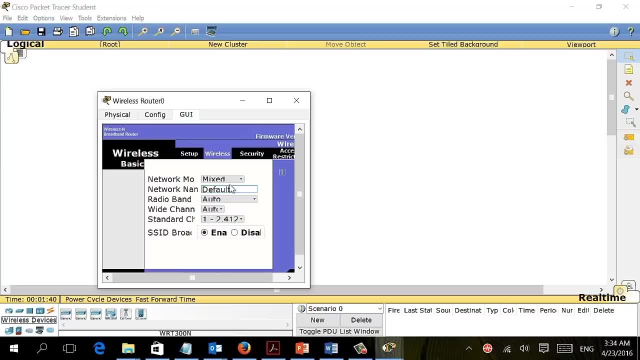 there is an access point by this name. that's why it's very recommended that once you configure your access point and then you make sure that all the device has been connected, to go and disable this feature instead of enable, make it disable. ssid broadcast. this may find under different name it. 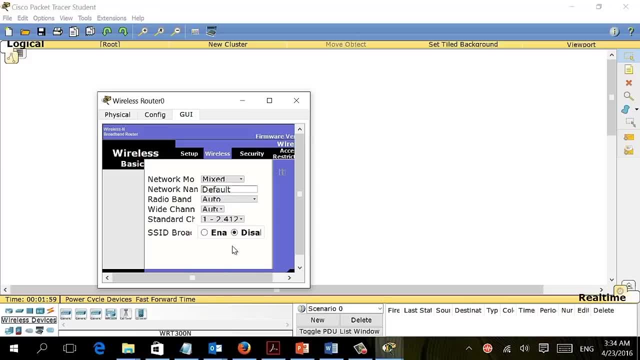 could be disable ssid broadcast. it could be, uh, disabled peaking. it could be this hide access point. they have the same function, which is you are preventing or you are stopping your access point to start announcing about itself. it's a good security mechanism because otherwise anyone can scan. he will know that there is an. 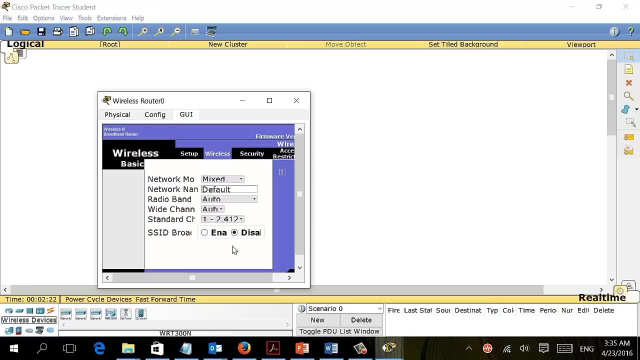 access point on this area and he will try to crack it. but if it's hidden or it's not announcing about itself, maybe you're going to make this thing a little bit more secure. the second, after assigning the ssid, is to assign a key. so when you go here we will find in the wireless security. 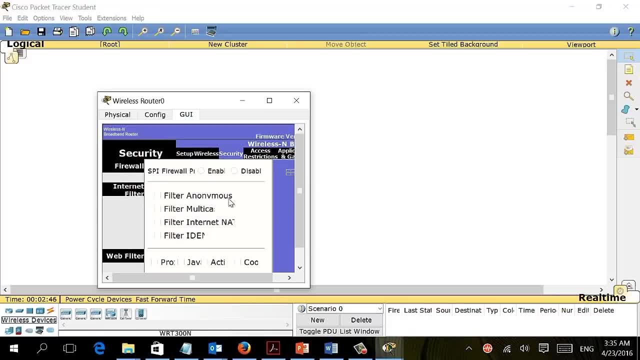 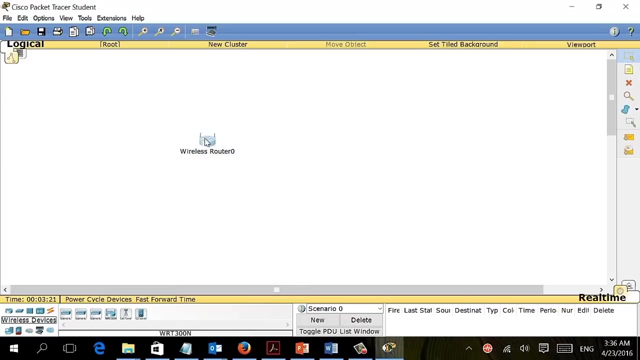 yeah, here we go: the- no, i'm sorry here- wireless and we can choose from here the security. i don't know how to decrease the size of the. okay anyway, so we you should found different key that you can assign to your wireless. so we have web and wpa and wpa2- let me try one more time. so let's go here: wireless, and 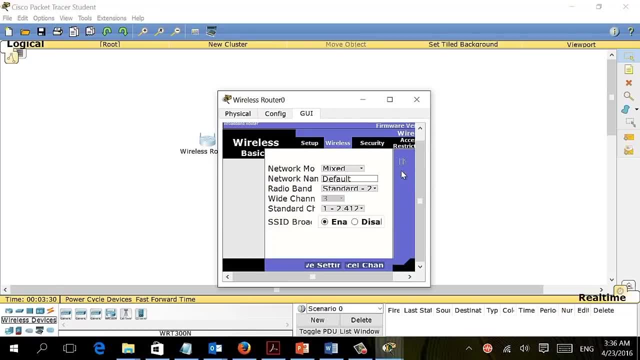 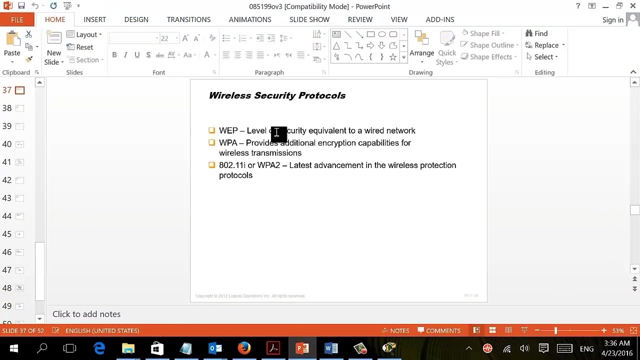 we should see the wireless security, but the theme is not working here. so under wireless security you should find three different key that you can assign to your access point, or you can keep it open, which is definitely not required now in wireless. as we saw in the slide, we have three different key. now the question is: what is? 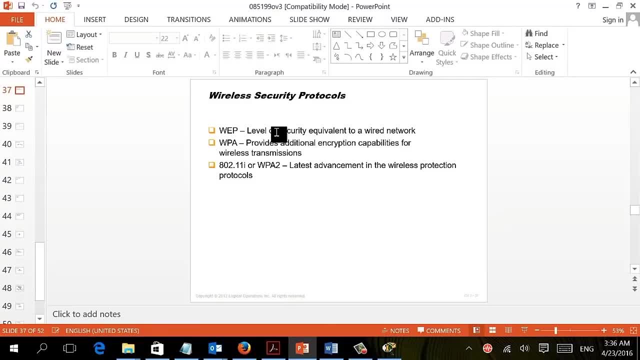 the key? is it a password? definitely not, because we are all using the same key and this is not a password. characteristic password should be unique. but when we put a key inside the access point to allow people to connect using this key, everyone will have the same key. so what happens usually? 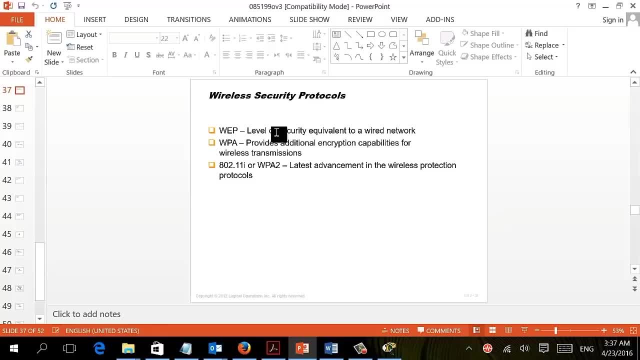 if you keep the access point open, it will send and receive in plain text, but when you put a key, it will encrypt the traffic coming and going and it will. these keys that you are giving to the user will be able to able to read the traffic, so they will be able to read the information. so it's an encryption. 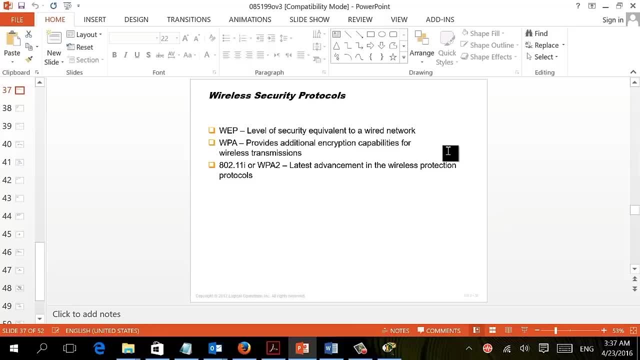 decryption key and because of that, you need to use one of the good encryption key. so there is different characteristics. the web key: it's considered the weakest one. it can be break in like 10 minutes or maybe less because it's using an encryption protocol called RC4 and RC4 is considered very, very easy to break. WPA are using RC4 also, but with a bigger key. RC4 with a bigger key, but it's also weak, While WPA2, which we are considering strongest, it's using an encryption protocol, is called AES, which is considered 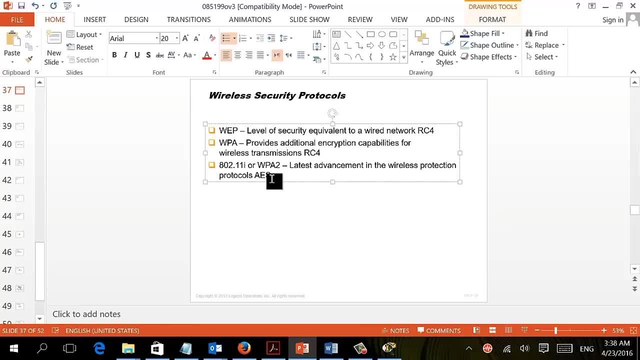 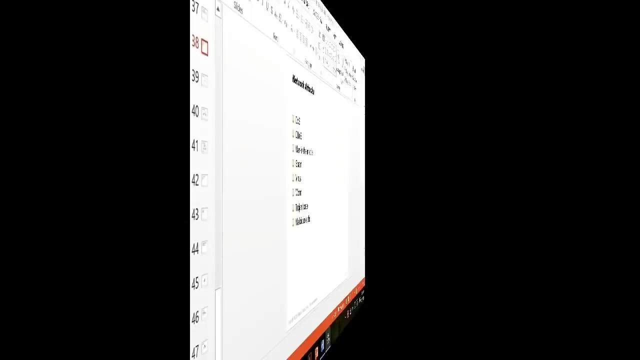 a very good encryption protocol. so when you are assigning a key to your access point, you should use WPA2 to make sure it will be secured and will be hard to crack. It can be cracked, by the way, but it will be hard to crack. Now we will be talking about attacks and we keep as we keep saying. 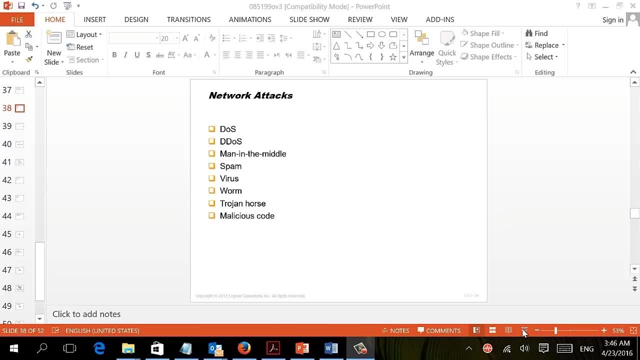 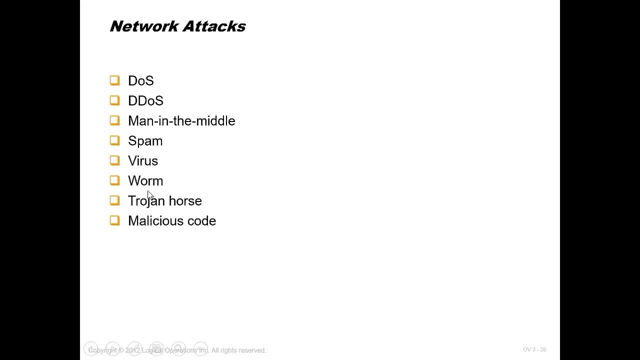 in each lecture. attack is very, very important, but the good thing is that you're going to find a lot of repeated attack in this module. so, for instance, we have the virus attack and worm and trojan. they are in the same category, malicious software- and you know that malicious or malware are divided. 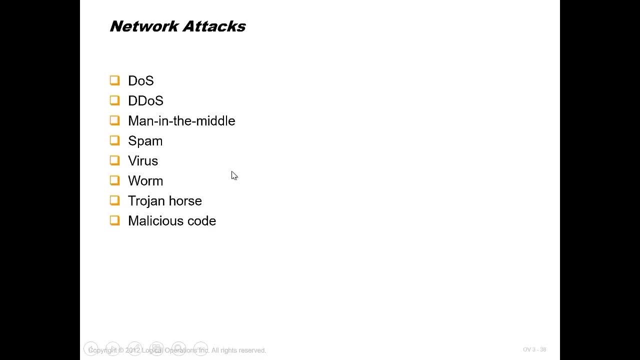 to two different parts. we have the spying things like trojan or keylogger, or we have the ones that are malicious. software and malicious code are the same, you know, because you can add to it the new type of malicious code like ransomware, and this kind of malicious code Man in the middle attack. 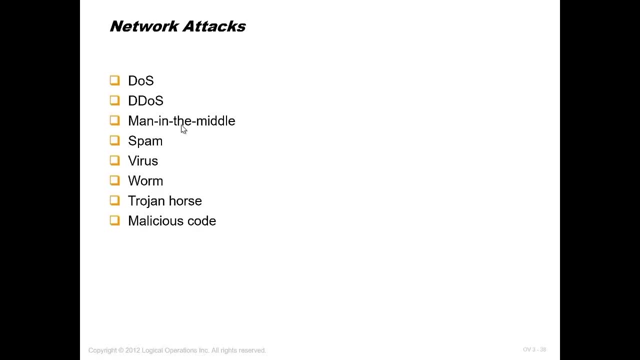 we spoke about that where you can manipulate the switch so he will send the traffic to you as a hacker instead of sending to the original location, and how people are using that based on ARP reply. if you don't remember the technique, just get back to the network architecture. 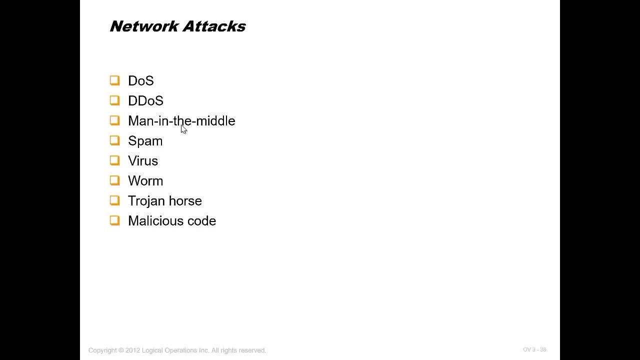 where we explained how the switch is working and how the how the switch is working and how we can our or how hackers are doing man in the middle attack or sniffering. now the important attack here that has some detail is the denial of service. denial of service, or distributed denial of service, is that you are trying to send a huge amount of 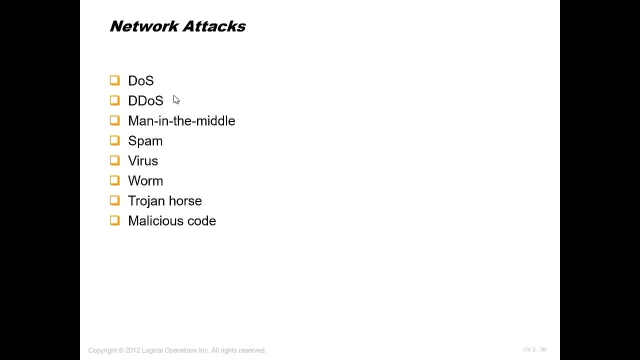 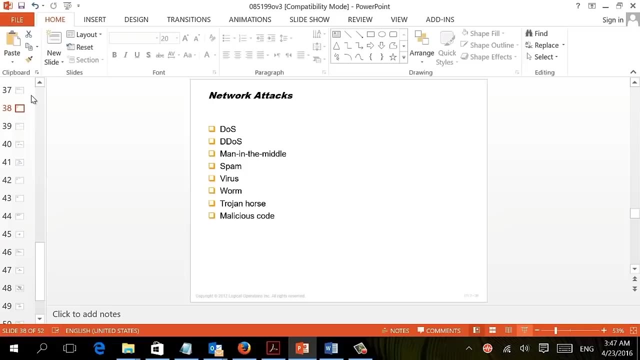 packet to a server or a service to crash it. we know that actually as a concept, but there is some details here in this module and it's important to know about that. so, for instance, let me give you a small example about how to how a denial of service. 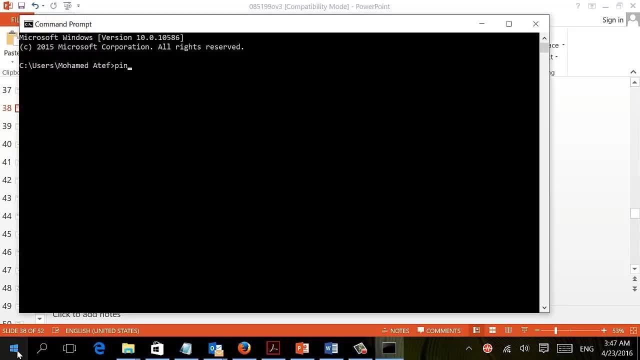 used to be implemented. if i'm do a ping on a web server like yahoo- wwwyahoocom- this exactly this serve yahoo. if you are doing ping on a website like yahoo, what is exactly will happen? my computer will send four packet with a very small size- 32 byte- to the yahoo server. and if yahoo has a ping, 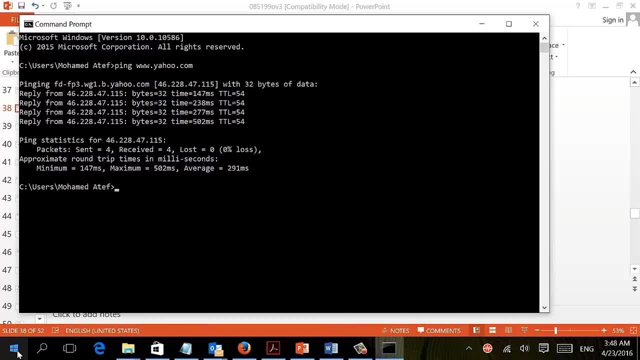 running and, i'm sorry, the icmp protocol running. he will reply back with the same amount and the same size. that's why you can see here that four packet has been sent and four packet has been received. now I can misuse that, I can type ping the same website, but minus T and minus T make me mean make it. 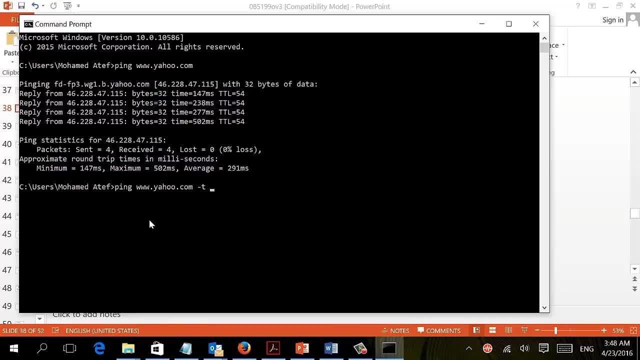 continuously. so he will keep sending ping and you have to reply back. and also I can type minus l which change the size of the packet, so I can put the maximum size. I believe it was 65,000, so I mean 65 MB. so now what I'm trying to do, it's. 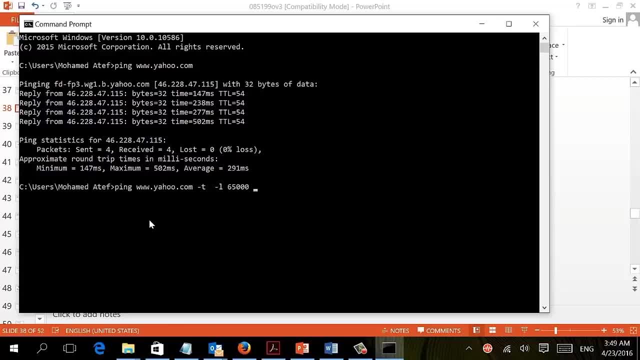 I'm trying to send the huge, continuously packet, very large packet to yahoo and yahoo has to reply back to me and I can do the same from three or four different machine and now yahoo has to reply to those three and four mailles machine, same amount and same size. definitely this attack will not get to. 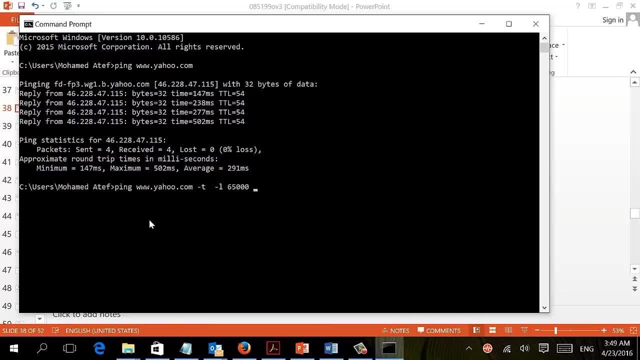 Yahoo. but if you do that on a single client machine it may affect its performance. so now Yahoo has to reply to those four, five machine with the same amount of packet and the same size. this attack is called the ICMP flow at the float attack. so you are sending a lot of traffic that we that will let to crash. 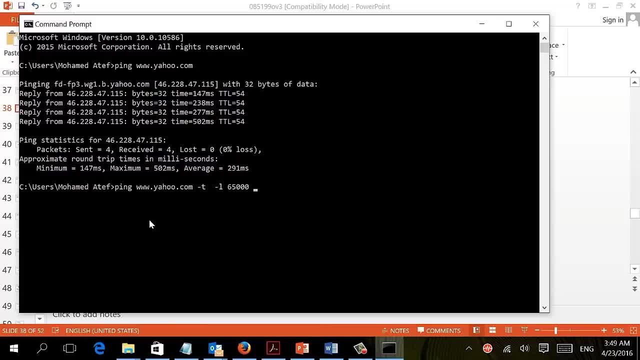 into system. you know reach not your any computer. if you are doing this attack against he, will reach a stage where he cannot reply because you know he keep replying to everyone with the same amount, continuously use the same size, so it will lead to crashing. so this is called the ICMP floating another attack. 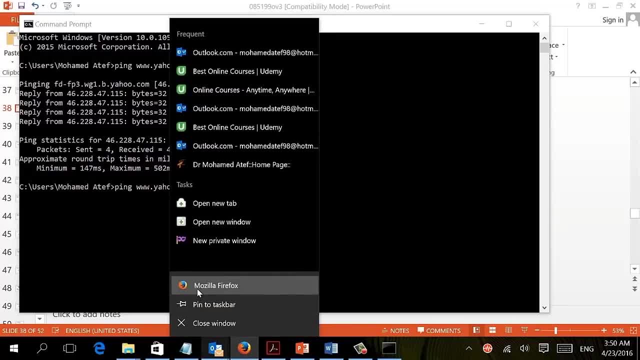 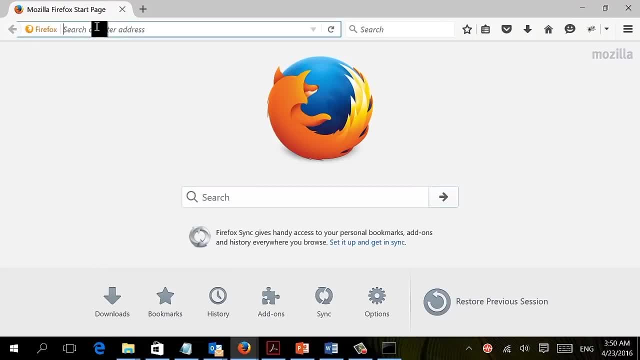 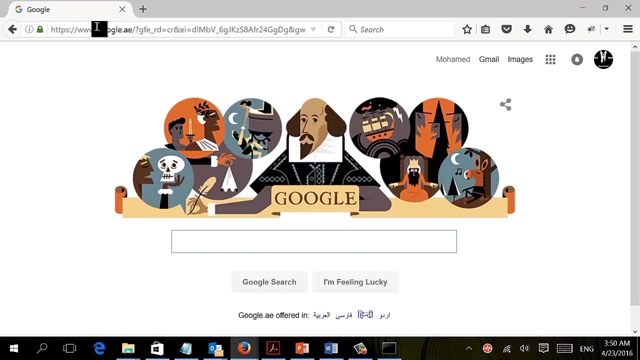 that I need to discuss with you. it's called the same float attack. so if we like search here, let's go to Google. so the line of service: it's important to know the different kind of attack, not just the definition of the attack. so let's talk. 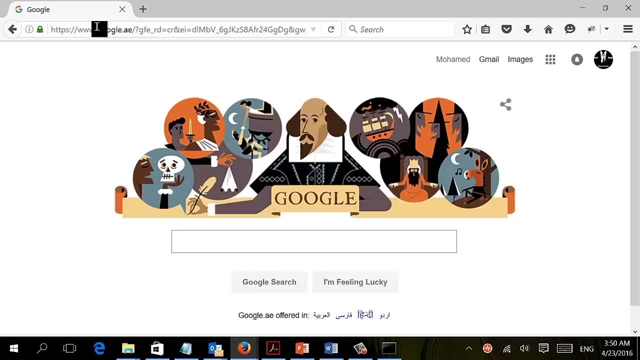 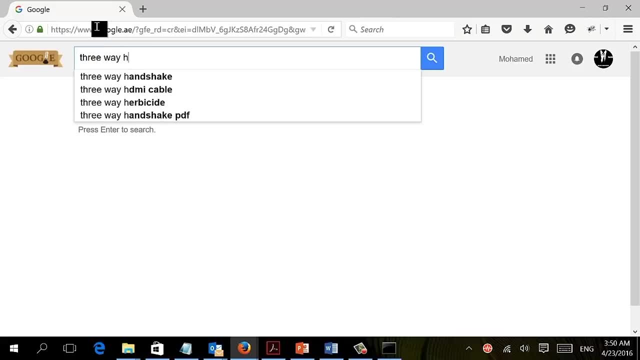 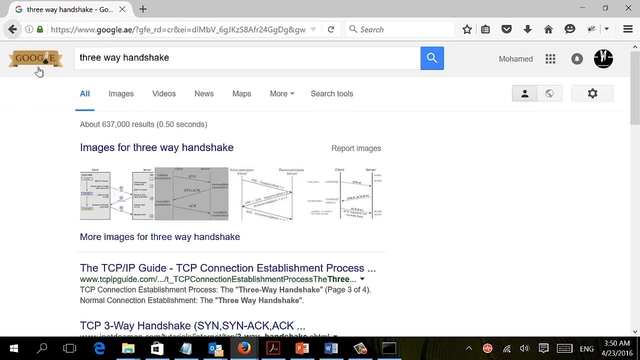 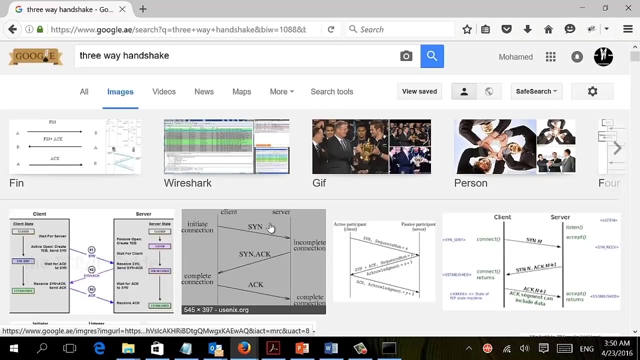 about something called a three-way handshake, because this is basic of this attack: three-way and check now in network, usually when two computer are communicating together. I mean, if you are communicating with Yahoo to open Yahoo page, okay, how it go. I mean three-way handshake, how things are starting. so assumes that we have let me. yeah, this one is okay. so 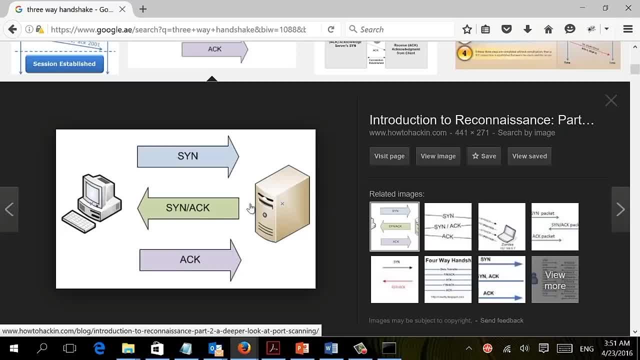 assume I have a computer and I have a server and this is my computer and this is Yahoo or Google website now to be able to communicate, I will not send requests for data right away. I'm gonna send something called sin and the server need to reply back with something called sin egg and I have to send an egg and 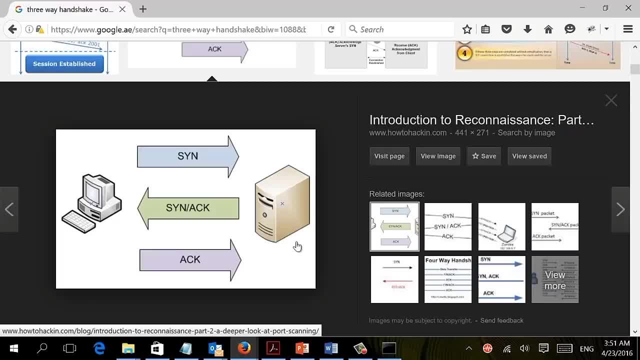 then the communication stuff. this is called the three-way handshake. so this is how the communication stuff it's like when you are calling someone over the phone. it's not like once he opens the line, you're gonna start talking right away. you're gonna say hello. this is the sins that you are. 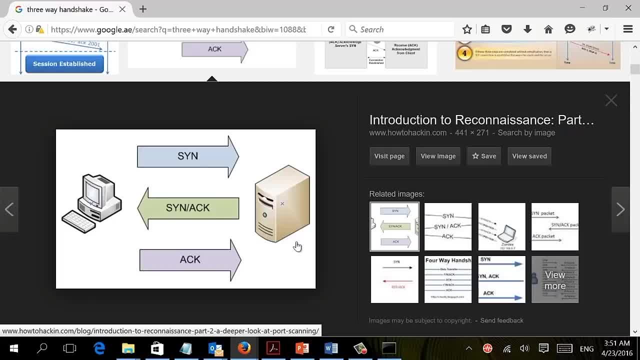 saying I'm on the line and he gonna say: hello, this is that you know. acknowledgement, I can hear you. yes, go ahead, and then you can tell me I speak to mister and then you can start the conversation. so there is some initiation process before starting the conversation. so one of the very 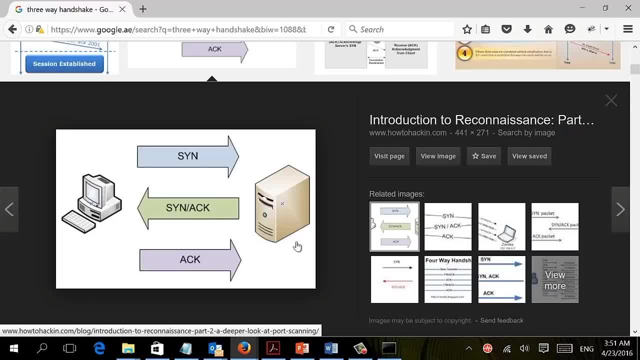 effective way for doing. actually, it was quite effective like soon or actually some early time. we used to do this for testing and it was very, very effective. so what happened is I can misuse it or any hacker can misuse it. I'm not a hacker, I'm just talking as an example. so what I'm saying is: let's 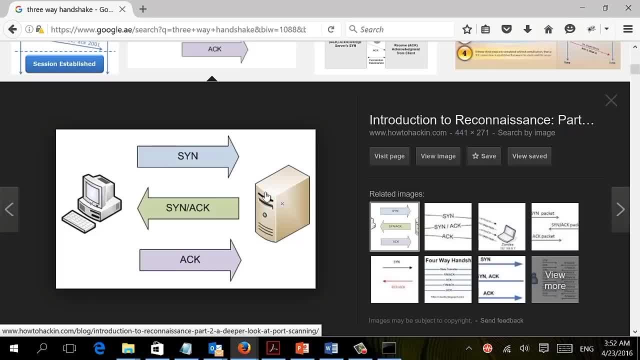 assume this is a hacker guy, he will send the sin to the server. the server will send the sin egg mean I got your sin and I'm acknowledged, yet I'm waiting for your management so we can start the conversation. the hacker will not send the hack and he will. 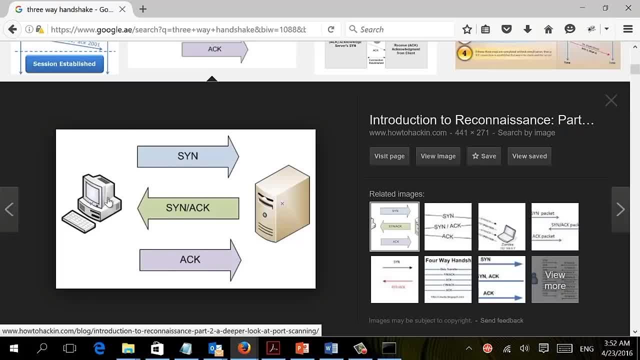 send another send. so by not sending the hack, he kept one session pending. the server is waiting to for the hack, and so he will establish the communication and start communicating. but he didn't send the hack, so the session is pending. now the hacker will send another send, then the server will send another send hack and waiting for the hack, he will send. 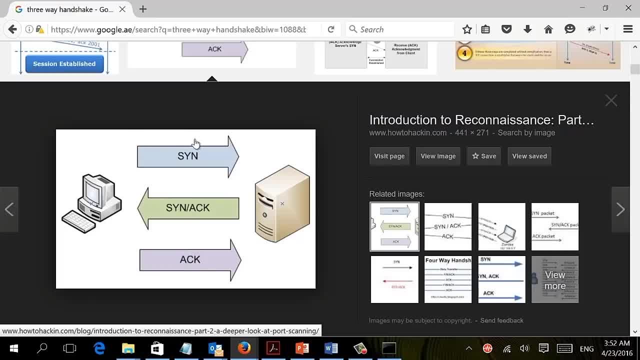 not send the hack. so now i have two session pending. he will send one more send and get send hack and he waiting for the hack. the hacker will not send the hack and if he keep doing that for a while, like 500 or 1000 session now, the server will not have any free session. 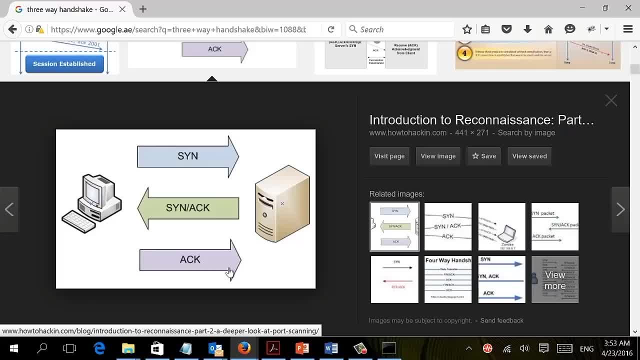 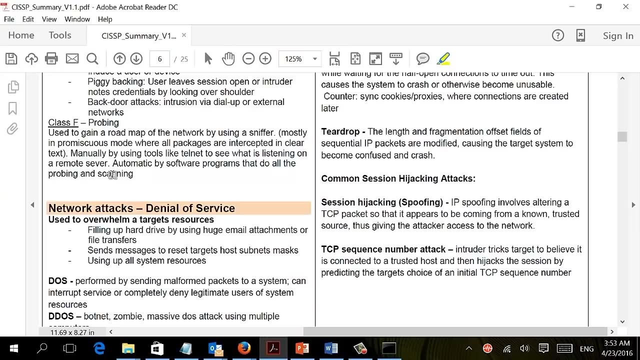 to give it for any other user. so you as a regular user you try to connect, you will not get a connection to this computer. this is called a send float attack. okay, also it will lead to denial of service. those are two major attack, but actually there is some more, like two or three more that you 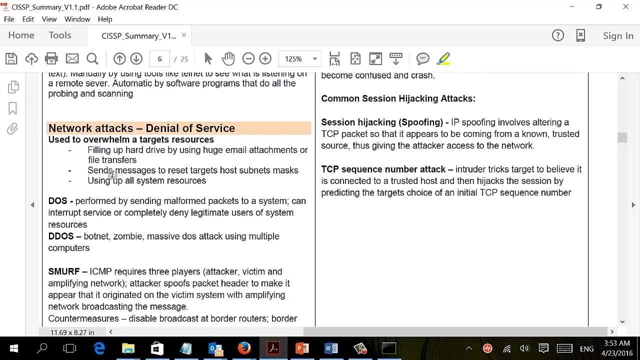 are going to need to memorize. so denial of service is very, very, very important to know the different kind of attack. so we have the dos. this is a definition. it's a. you are leading to crashing the system. ddos that you are using something called bootnet or zombie. it's a. 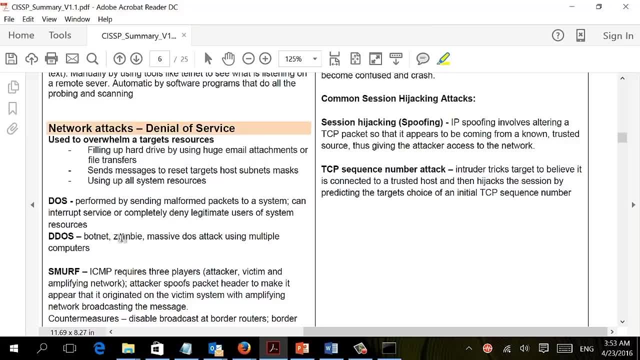 small malicious codes that you are spreading over the network and they are connected to something called command and control. someone sitting somewhere in the world he can see send requests to all those machines and it can lead to crashing systems. The one that we just explained is called Smurf. 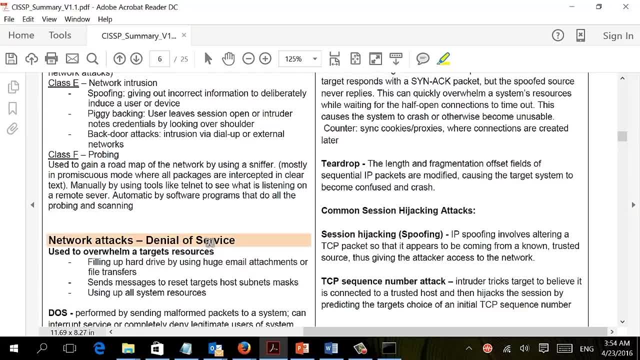 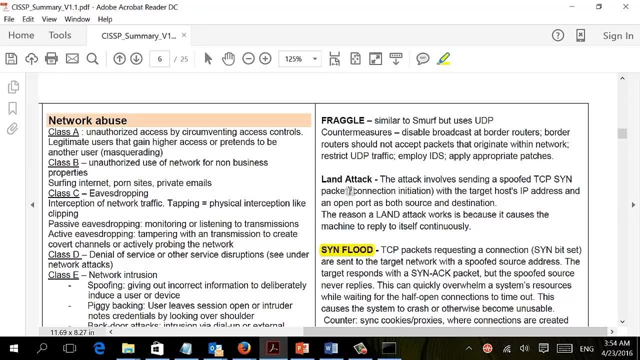 the attack that is dependent on ICMP. We have the SYN float. I just also explained this attack as well. We have the land attack where you are spoofing the TCIP SYN packet, So it depends about faking your packet connection. We have the fragile. 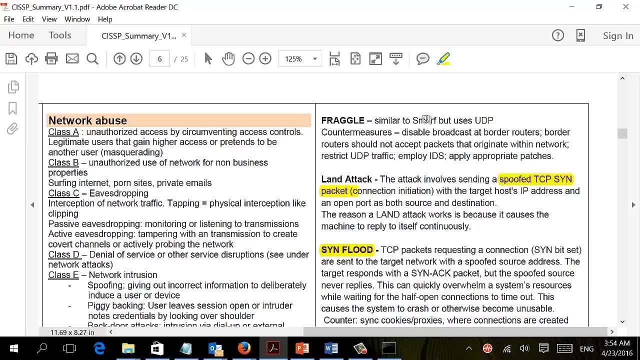 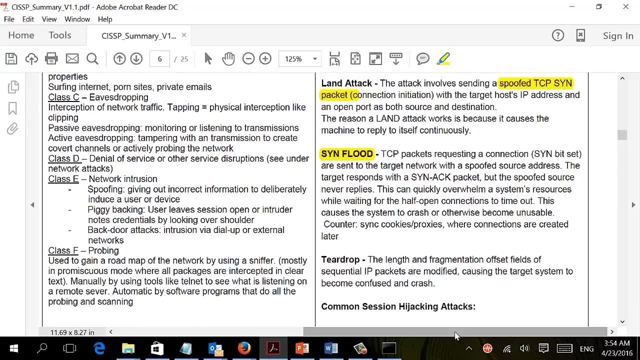 another attack that is, I believe, using UDP. just get the keyword. you know the major keyword, but you should memorize the teardrop where you are putting the source and destination. I believe the same. So those attack are very, very important in denial of service. You should expect one of those. So denial of service. 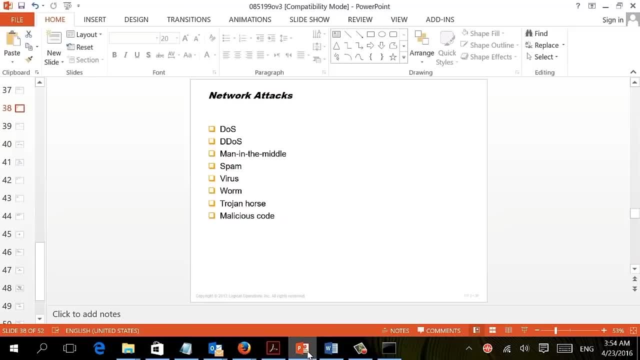 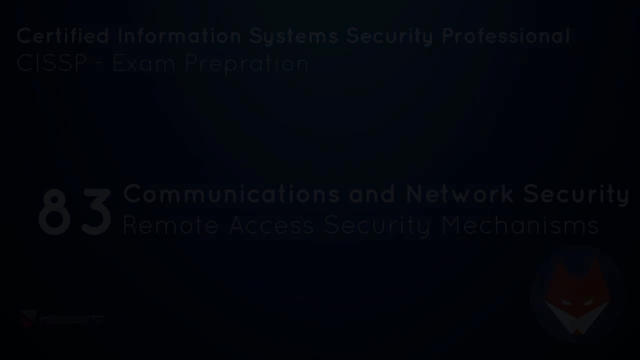 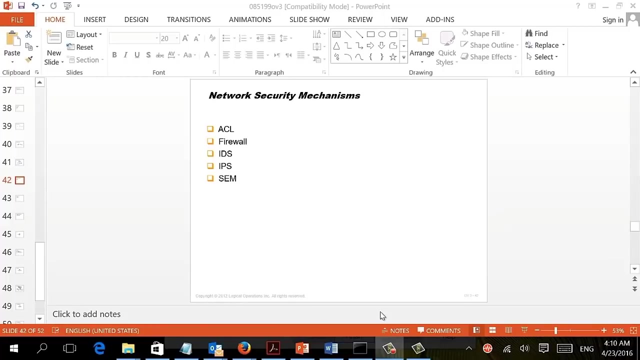 here in the network need more studying or need to know more details, not just to know that there is an attack called denial of service. This lecture will be talking about some security mechanism in the network. So we have the ACL or access control list. This can be used to put some 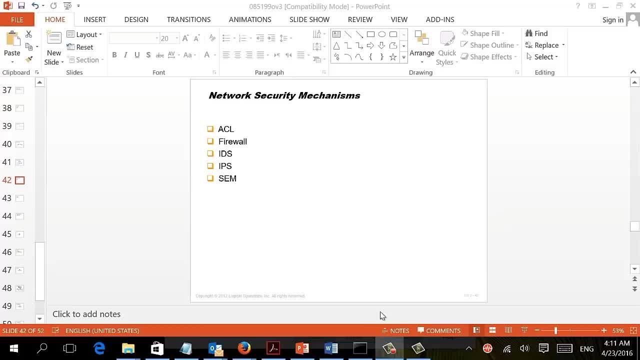 rules or allow some traffic or deny some traffic. Same concept of firewall. We already spoke about firewall and we create a video about it. We have something called the IDS and IPS that we explained on chapter one- intrusion detection system or intrusion prevention system- And we have the same solution, which is: 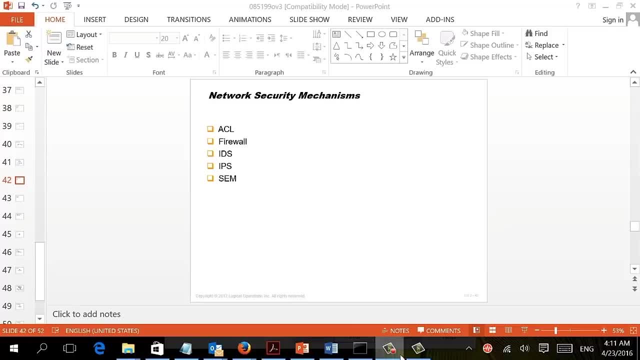 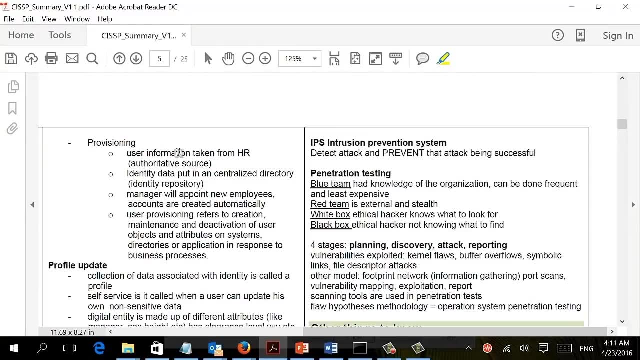 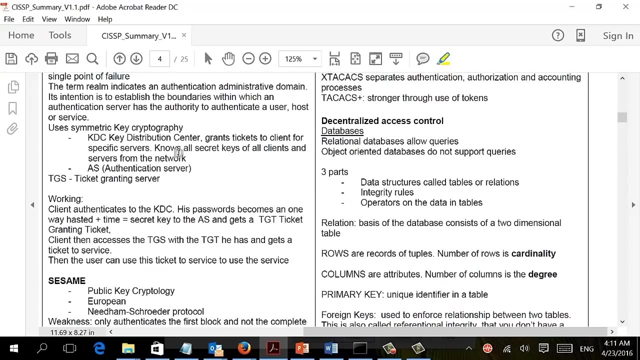 event management solution. But besides this technique also we have attack like caller ID attack, which is an attack that shows the caller in case of dial up. We have the not attack, I'm sorry, caller ID mechanism. We have the calling back some services when you try to call them, because number can be spoofed. So when 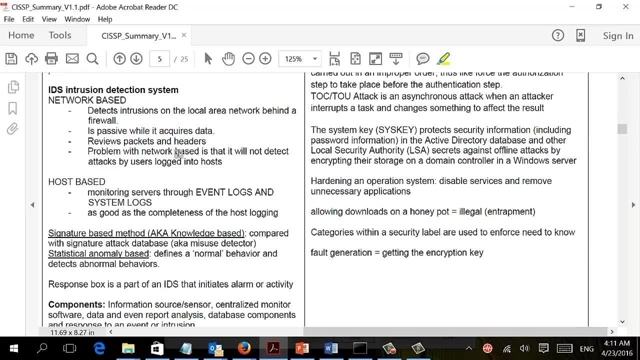 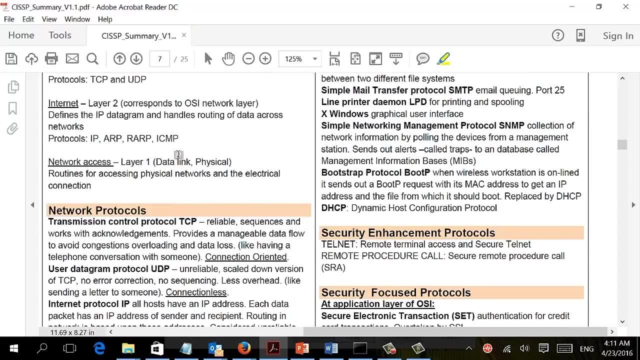 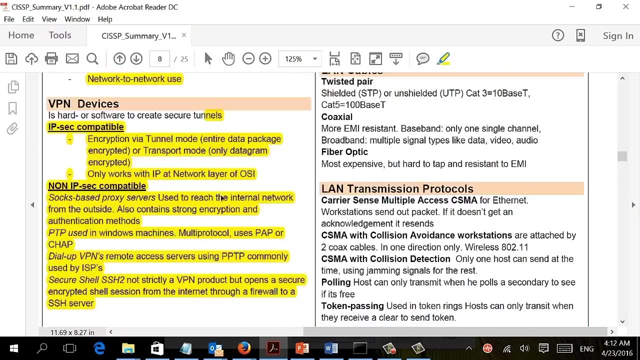 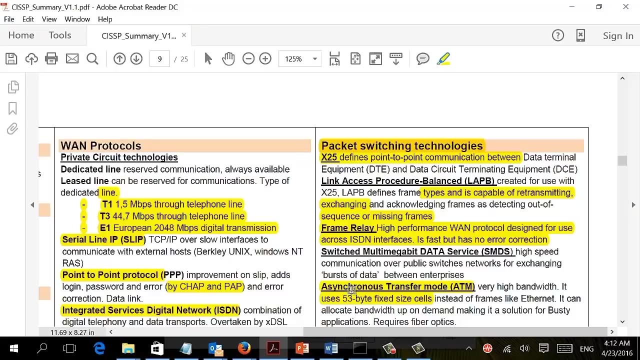 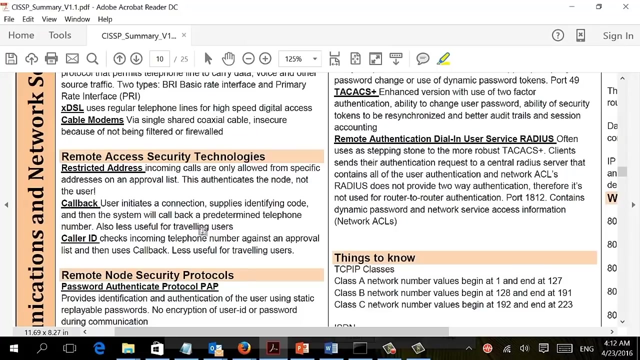 you try to call them, it will disconnect you and will let you, will call the, will call you themselves. I'm just checking user text. So we have different kind of security mechanisms that we can implement inside the network. It should be here, so definitely somewhere here. security, security, yes, this one. we have the restricted access. This is also considered. It's not in the slide, but it's very, very important that you can. 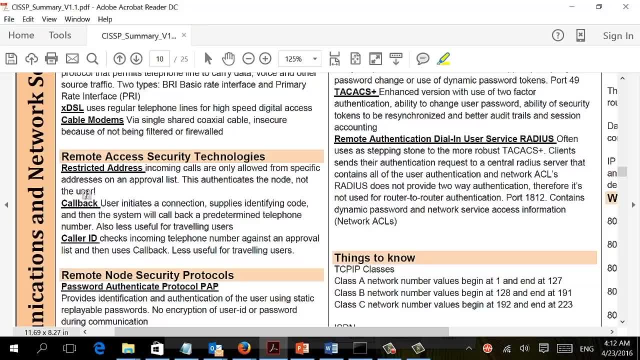 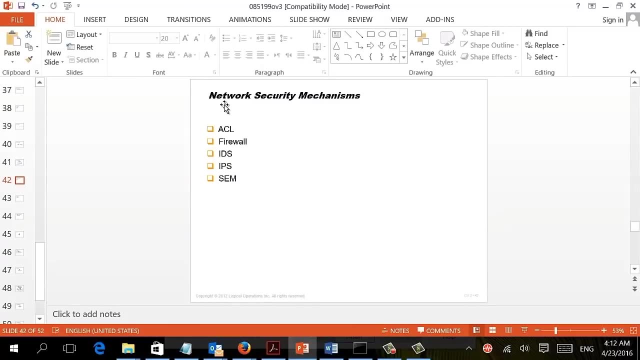 this one. we have the restricted access. This is also considered. It's not in the slide, but it's very, very important that you can restrict some access. You have the call back. when a user can call or user calling a place, you can disconnect him and call him back, And this is because if he's using a spoofed number or a fake number, you'll be knowing that you have the caller ID. This is also can be added to the security mechanisms that can we, that we can use to secure our network. 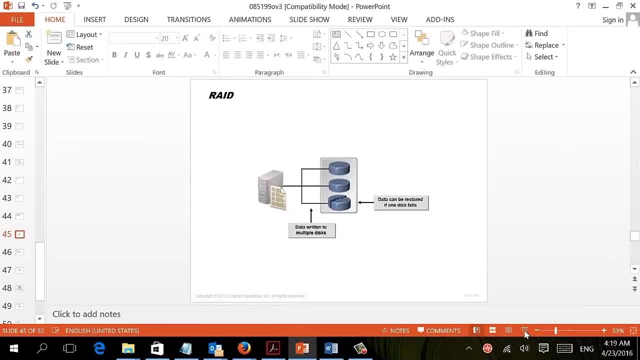 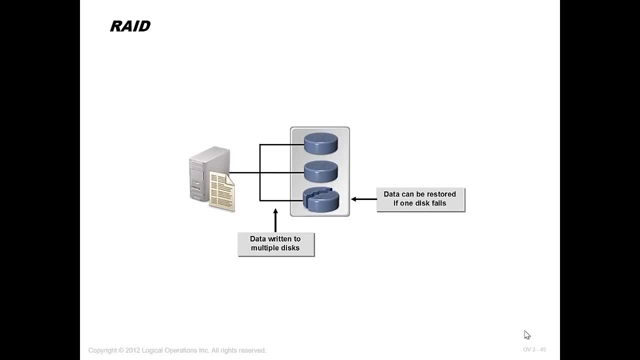 We spoke about different component of the network and one point remaining in this module, which is: We spoke about different component of the network and one point remaining in this module, which is Application and how to provide availability. I mean, whatever we spoke about was related to confidentiality and integrity and also availability, And when we spoke about the denial of service, on this focus inside the network will be focusing about 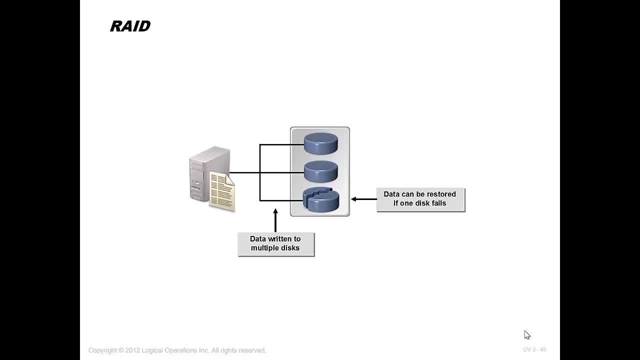 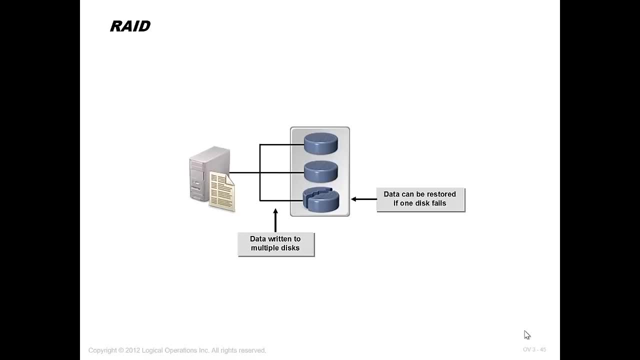 important server that has a very confidential type of information, and those information should be available all the time, 24: 7.. assume this is a bank, a huge bank, where customer can log in anytime from any place, draw money or check their account and so on, so you cannot have any downtime. 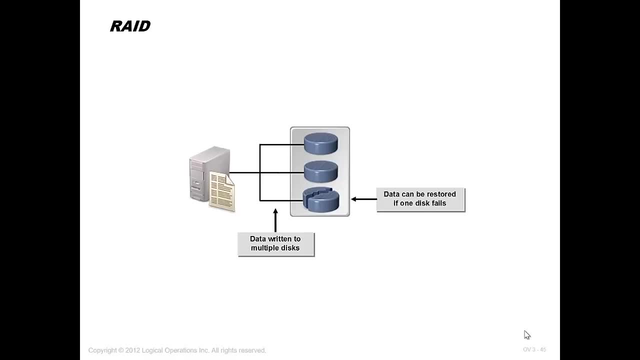 now where those, where all those information are saved- they are saved inside the hard drive or some hard drive or any kind of storage inside your network. now, this hard drive, as this hard drive may be a subject for any kind of damage, i mean, maybe the hard drive will crash, maybe 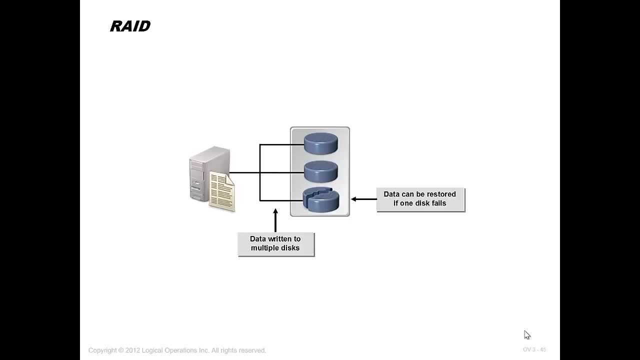 it will be affected with the virus problem happen all the time. so the question is: do we have anything to make sure that if any problem happen to the hard drive- physical or any kind of problem- we will not have any downtime? yes, we have something called raid implementation. 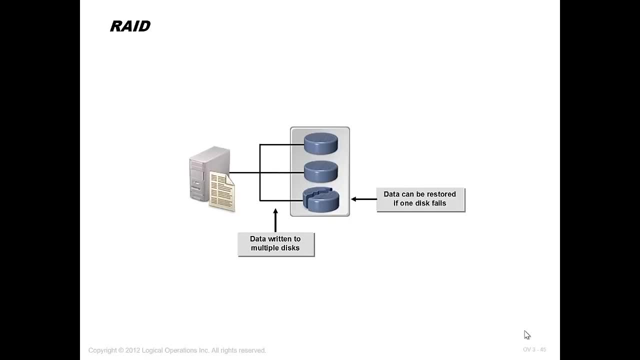 raid stand for redundant array of independent disk and the idea is that if i have a very important server like the one we have right here, we can add. instead of just having one hard drive, i will add two or three or four drive and i will combine them together so it will be showing to people. 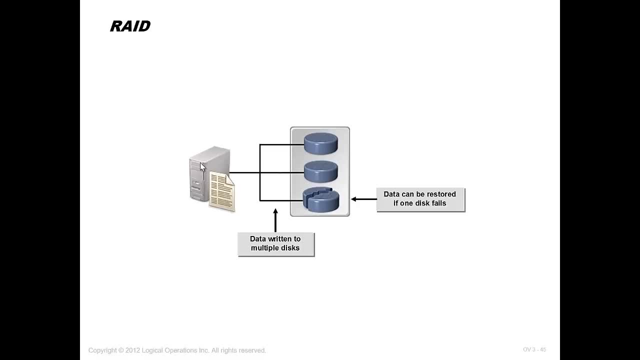 who's using this server as just one storage or one hard drive. and the thing is that if i do such implementation, whenever i'm saving a file in any of those disks, it will automatically be saved on the remaining disk, because for you it will show only one hard drive. this is called the raid. it's 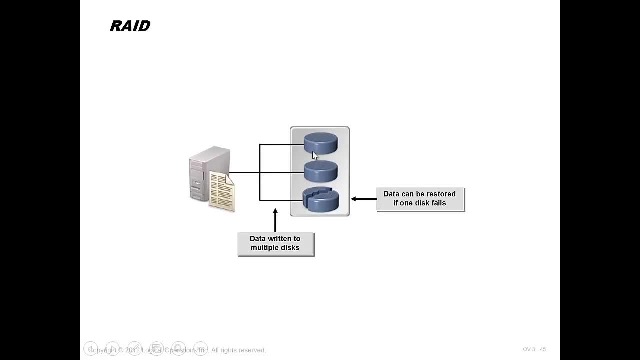 a physical hard drive. actually they have to be physical. you cannot combine logical partition. they should be physical hard drive with the same size. so by doing that, whenever you save a file, it will be saved, saved on the three or two or four drive and in case of any failure, the system will 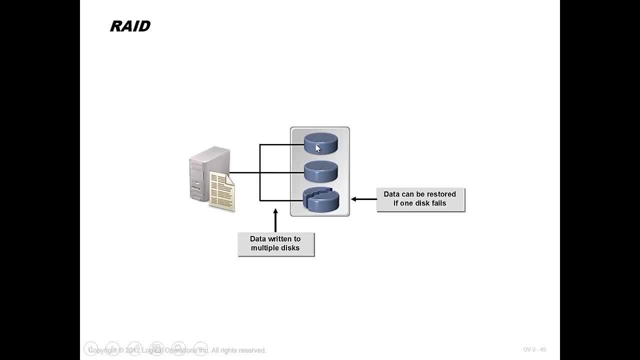 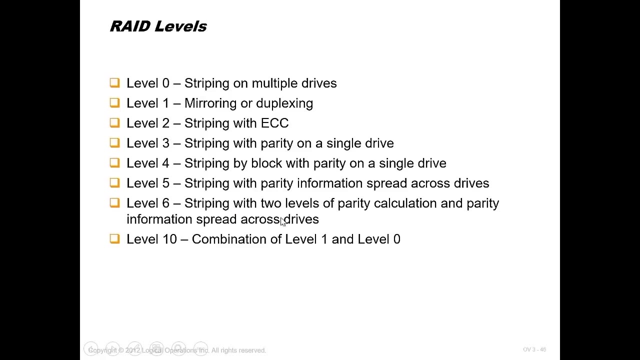 still be running and functional and you'll be able to retrieve the information for raid. we have different level, so i'll talk about the major one, which is red zero and red one and red five and red ten. those are the measures right now: red zero and it. 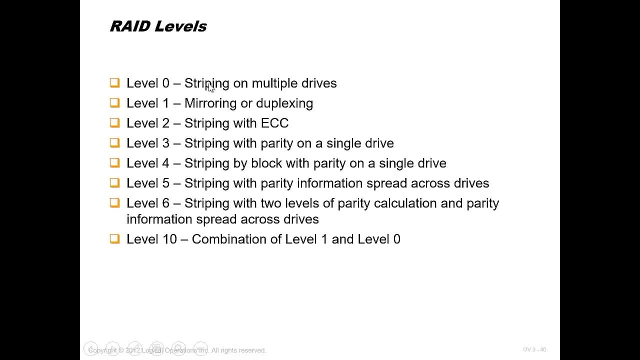 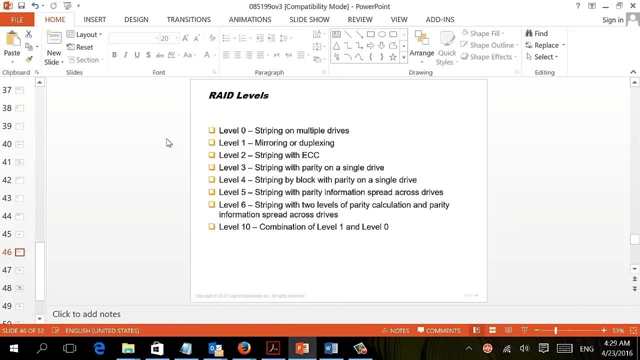 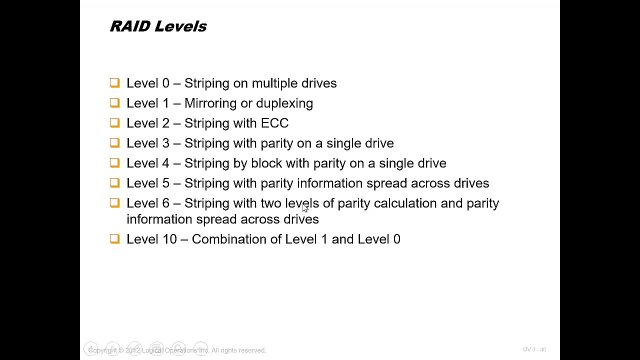 has another name, it's called stripping. uh, was working in a different way, so red zero, or also called stripping, was quite different than other rate. now red zero depend on or the way it was working, that you get two different hard drive should be physical, two physical hard drive and same storage. 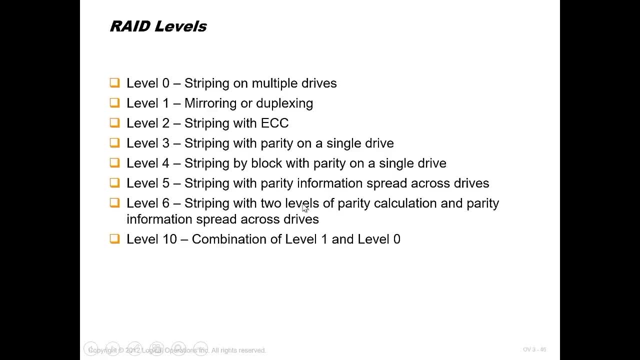 and you configure them to work as a level zero rate. now what happened is: whenever you create a file, it will be stripped, or it will be cut or divided to two different parts. one will be saved on disk one and the second will be saved on disk two. now, this will not be considered a redundant 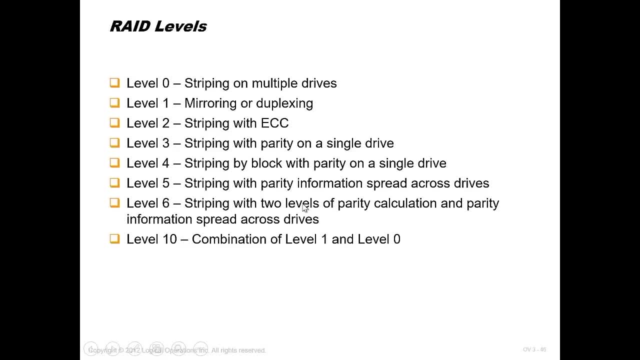 solution. i mean, if one hard drive failed, you cannot even use the second hard drive because the half of the half of those files are saved on the other drive that has been failed. so it was not used for redundancy or high availability, it was used for high performance. so when you do that, 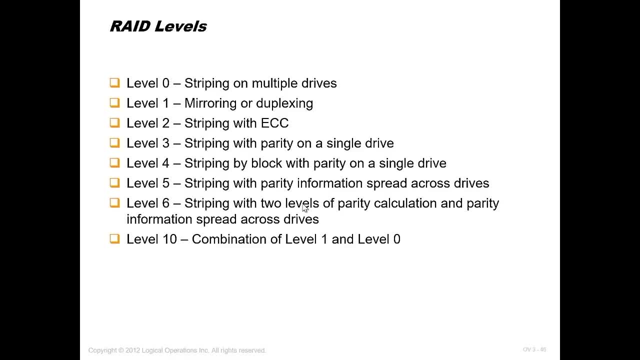 the performance of retrieving the file from the storage was high. so, strip, i'm sorry, uh, read zero is about the performance, not the redundancy. read one, which is also called mirroring, was different than that. you also have to add to hard drive physical hard drive same size, and whenever you save a file, it will be saved on the to. 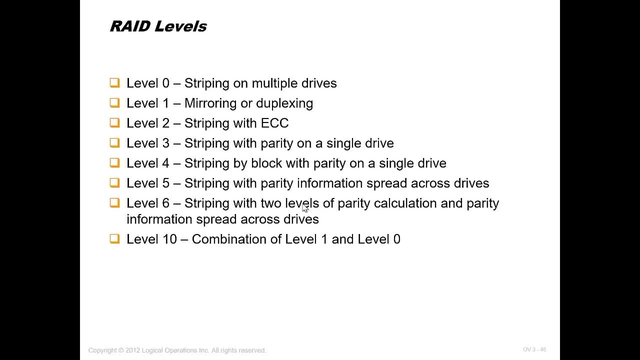 copy will be saved, each copy on one of the drive. so any files that you save will be copied on the to drive. so if you, if you have one failure- I mean if one of those two hard drive fail you still have- you'll be able to work. all the file will. 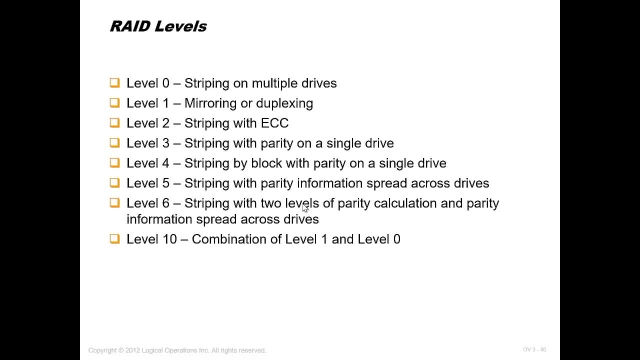 be there. you just gonna have a blinking on your screen that one of the file has failed and the only problem with read one was that it's waste 50% of the storage, in the meaning of assumes that I have to hard drive. each one is one tera. 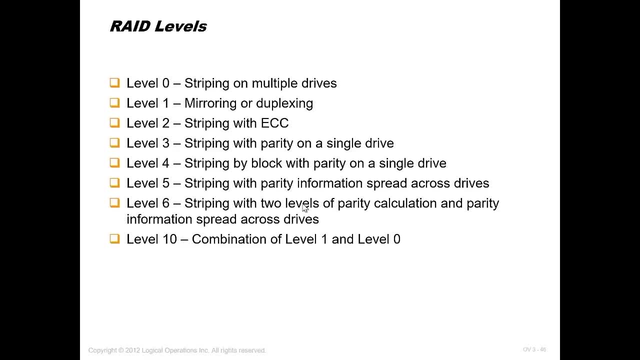 I combine them together and I create read one. so total should be two tera. but what will be showing to the user? one tera, only 50%, will not be showing because it will be used for redundancy. so the only disadvantage of read one was waste of storage. now let's 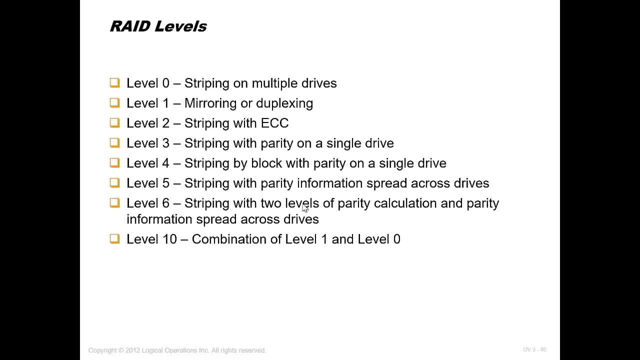 talk about rate 5. rate 5 is similar to rate 1, but you should use in red 5 at least three hard drive and the amount of storage that will be lost will be lower. I mean, depend about the number of drive if you have three hard drive, as 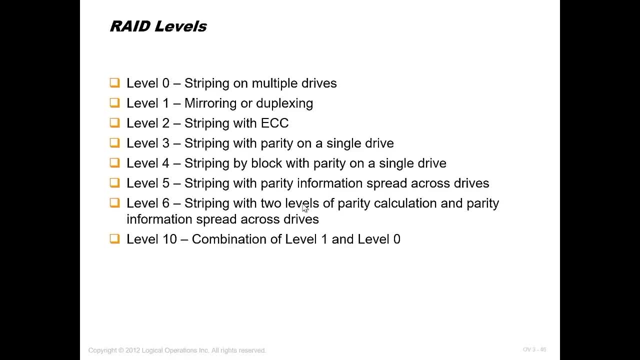 rate 5, you're gonna lose 30% cannot be used. this will be used on the for redundancy. well, if you have 4 hard drive, rate 5, 25% cannot be or will be wasted. if you are using 5 hard drive, it will be 20%. actually. it's 1 over n, where n is. 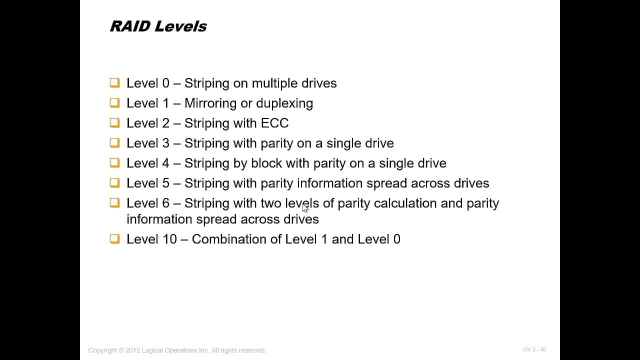 the number of drive. so whenever you add more hard drive, whenever this is will allow you to lose less amount of storage. finally, rate 10, which is combining grade 0 and read 1, actually actually scored read 1: 0, not 10, because it has the 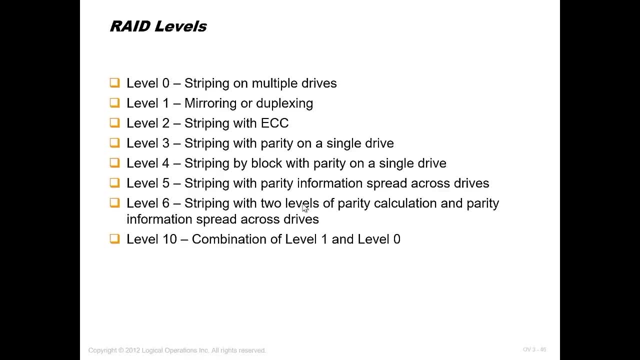 stripping and mirroring now how you'll be seeing those questions size exam. he will ask you your management request to implement rate for high performance. which one should you choose? 0 or 1 or 5 or 10, for instance, or for redundancy or something like that. so you should know the characteristic of each of those rate. 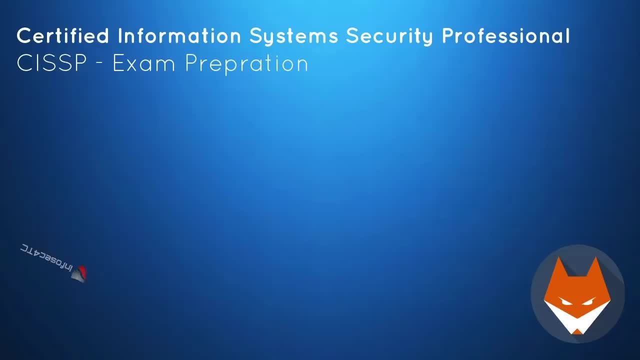 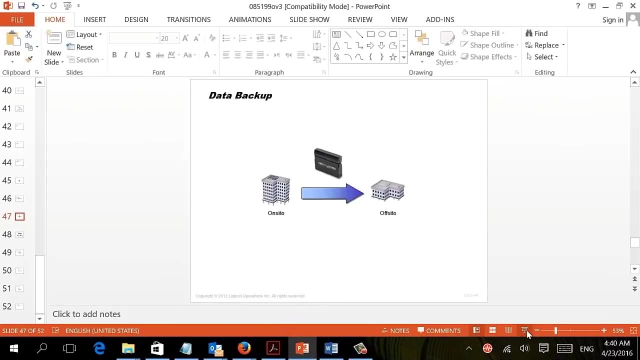 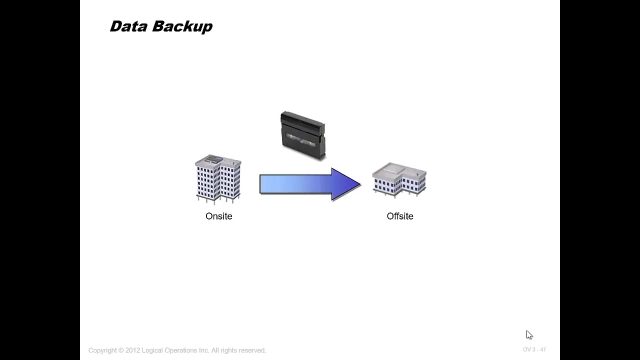 and you should know the characteristic of each of those rate. finally, in this domain, we'll be talking about backup, which is also providing availability. now, backup it's a very important topic in general and even in real life, but we should consider the backup best practice before going and 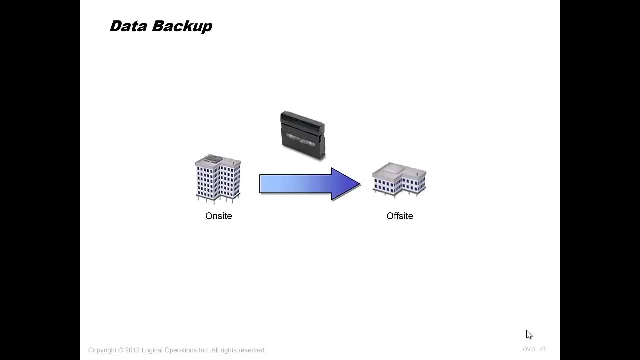 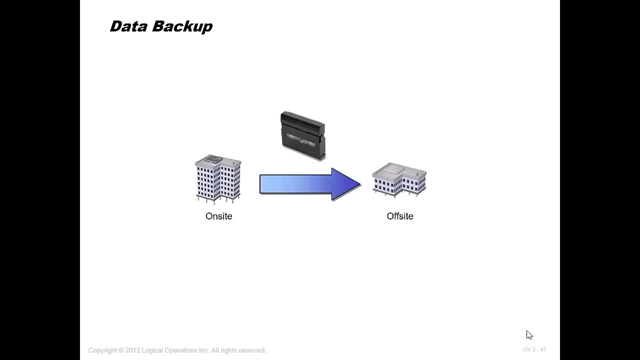 take backup. are you going to take that on an external hard drive? this is not recommended because actually anything that has mechanic can be damaged easily if it's failed or something. are you going to take that on optical media like a DVD or something? also it's not recommended because it has a lifetime. 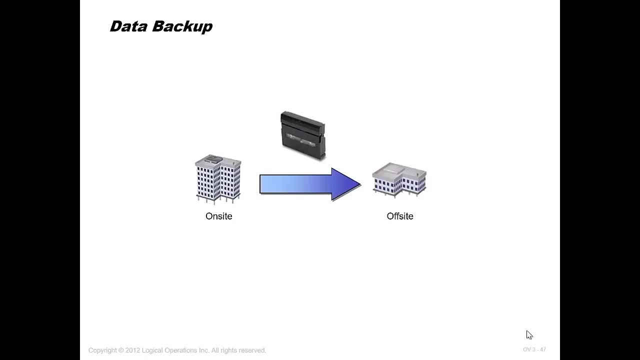 it's usually recommended to take backup on a tape drive. where are you be? where are you save the backup? backup should be saved somewhere remotely, not on the same premises and so on. but on this lecture we need to explain the different kind of backup. now, in backup we usually have three different kind of backup and a lot. 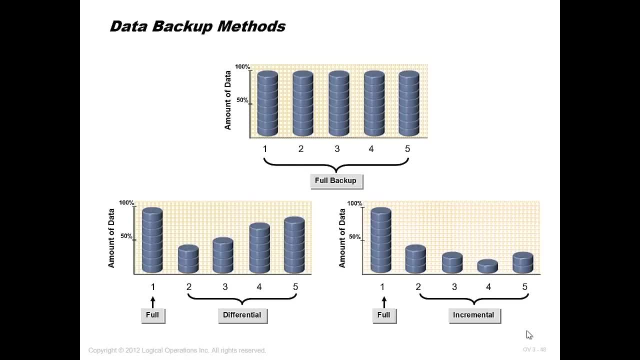 of people get confused about two specific type. so we have the full backup, which is taking full information, is quite clear- and we have the differential backup and we have the incremental backup. what is the difference between differential backup and incremental backup? let's take the differential backup first, which is the one on the incremental backup force, which is one on 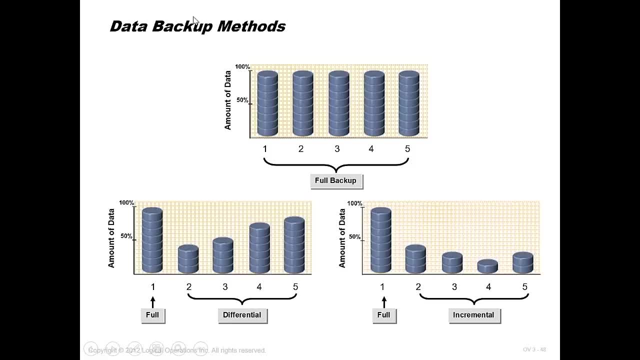 the right side. of course, most people will not be taking full backup every day because you know, some organization has a huge amount of information, so they are taking one full backup per week or per month, and the remaining of the week they may take incremental or differential backup. let me explain the. 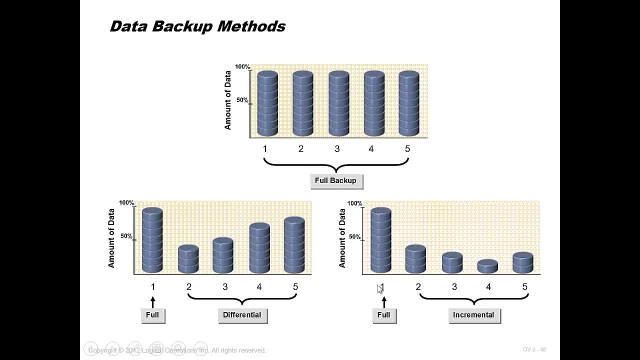 difference for you. for people who are not aware of that, assume that I am: on the first day, which is Sunday, I'm taking a full backup. the second day, I will just take the modifications that happen on the second day, so I will take the modification from the previous day. on the third day, Tuesday, I'm going to take 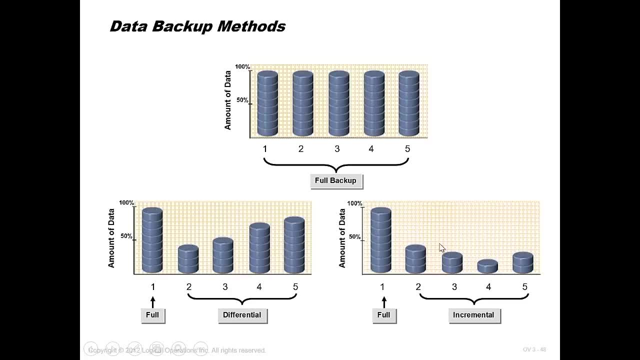 the modification that will happen. that happened from the previous day, from Monday on Wednesday. I'm just gonna take the modifications that happen since Tuesday and so on, while in differential I'm taking the modifications that happen from the last backup, meaning on Monday. on Sunday I took a full backup. 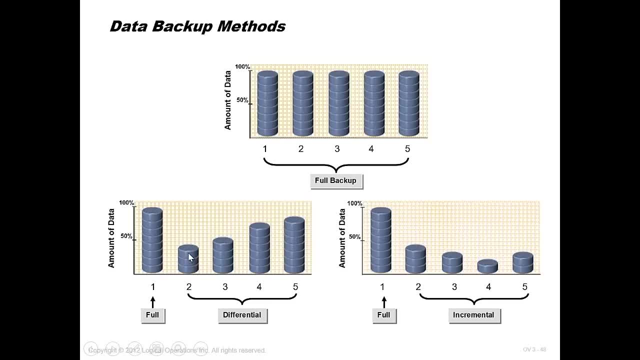 on Monday: the same: I took the modifications that happened since Sunday. on Tuesday: I took the modifications that happened since Sunday, not since Monday. So I'm taking the modifications that happened since the last full backup. On Tuesday: I'm taking the modifications that happened since the last full backup. 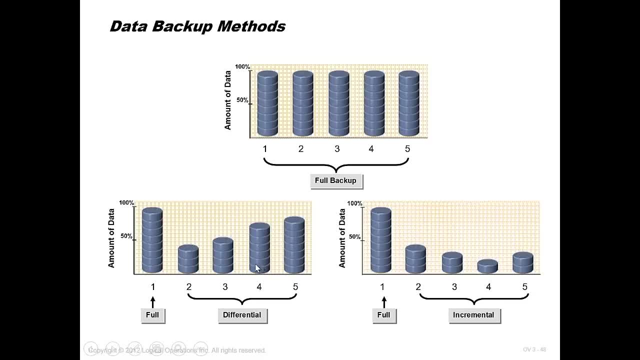 So it will include Sunday, Monday and I'm sorry- Monday, Tuesday and Wednesday, And on Thursday I'm taking the modifications that happened since the last full backup. How that is different than each other. They will be different when it comes to restoring. So in this case, like in the incremental case, 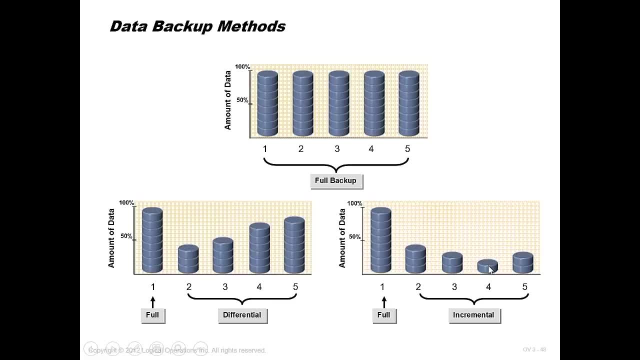 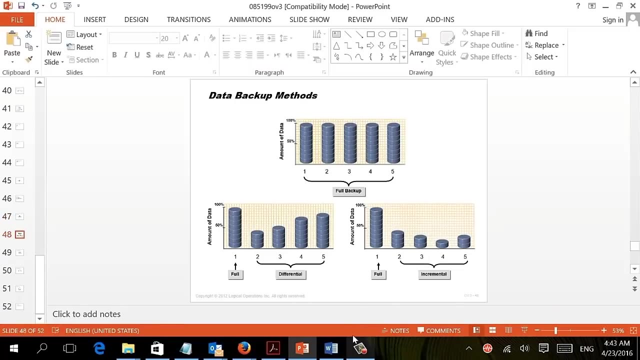 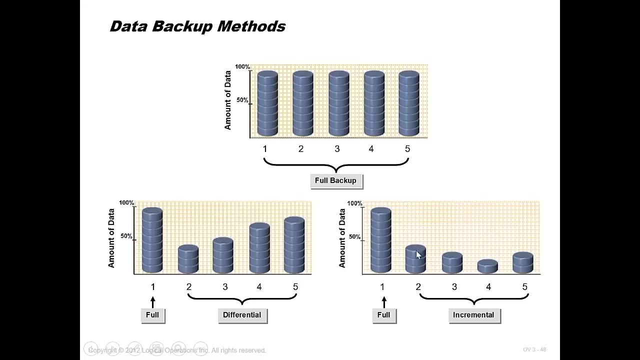 If a problem happened on Wednesday, How many tape? or on Thursday, how many tape do you need? We're going to need 4 tape: the full backup And 3 other tape While. So you need the full backup And you need The remaining tape for Monday, Tuesday, Wednesday. 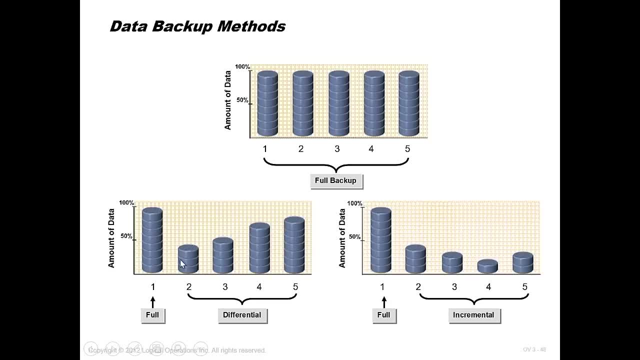 While if the same problem happened on Thursday, How many tape do you need? You're going to need only 2: The full backup and the previous day backup, So the difference will be in restoring The amount of tape that you're going to need while you are restoring your system. 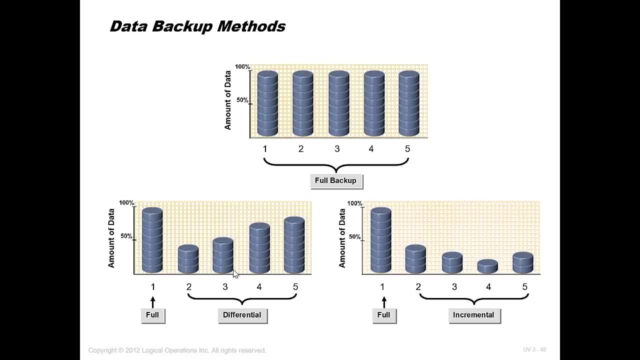 And if you are doing that per month, You are taking one full backup per month. If a problem happened by the end of the month, You're going to need like 29 Or 30 tape, While if you are doing differential you're going to just need 2 tape. 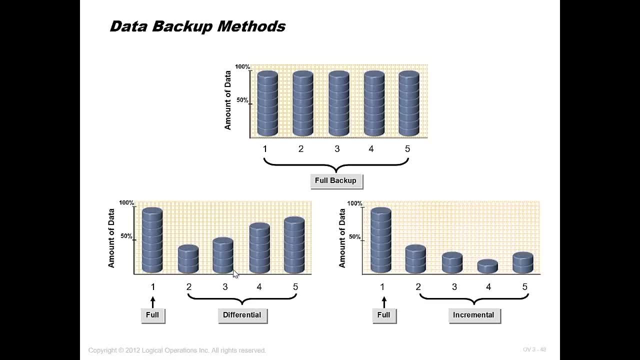 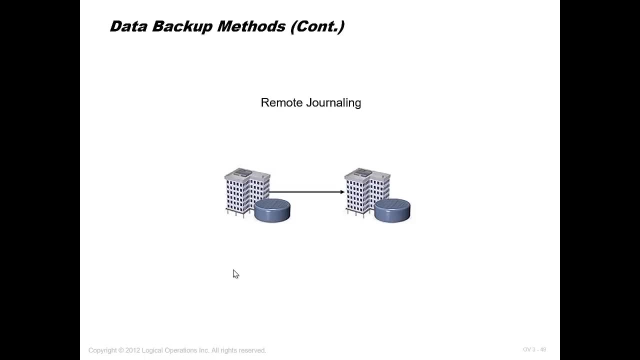 The full backup tape and the day before tape. So the difference will be inside the restoring. We have also some kind of backup like remote journaling backup, Where you are talking backup remotely, and electronic vaulting backup. But one of them is taking transaction by transaction remotely And the other one is taking bulk data. 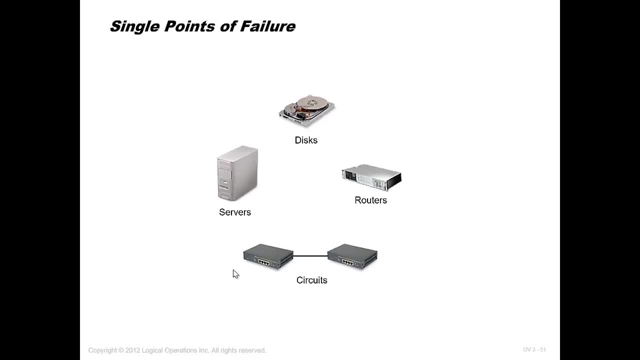 But all of them are remotely as well. And finally, the concept of single point of failure is very, very important inside our network, Where we need to identify where is the point device or equipment that, if it failed, It will lead to any kind of downtime to the network. 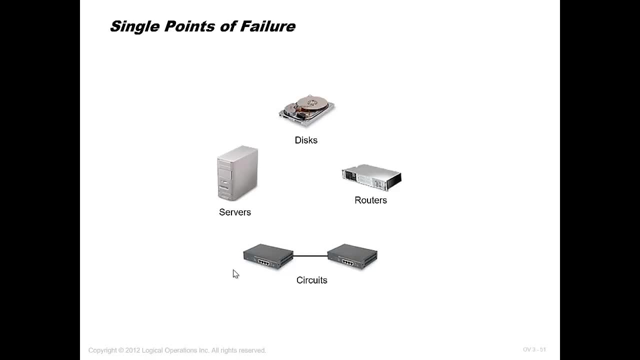 And I try to make some redundancy for that. So this was the Network domain. It's a big domain And I went brief as much as I was able to simplify that. It's very important to try to write down all the terminology. I believe sunflower will help you a lot when it comes to gathering everything in like three pages. 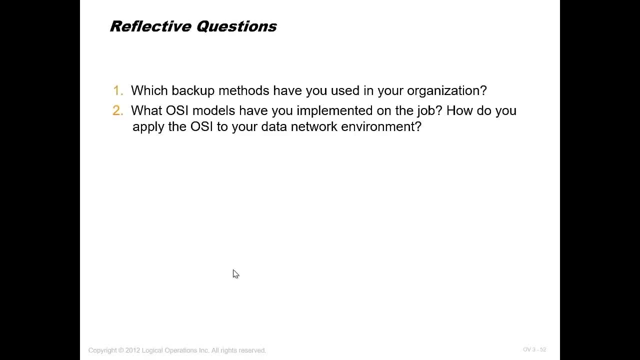 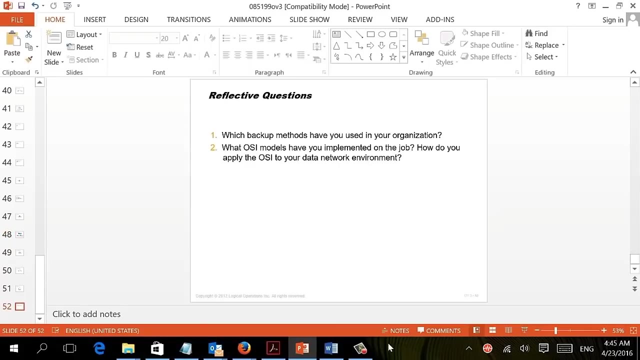 And starting from the next lecture, We're going to start going through the question and see how the question look like, And you have to answer all the domain question to be able to Be ready for the exam. So let's see how's the question for the network look like. 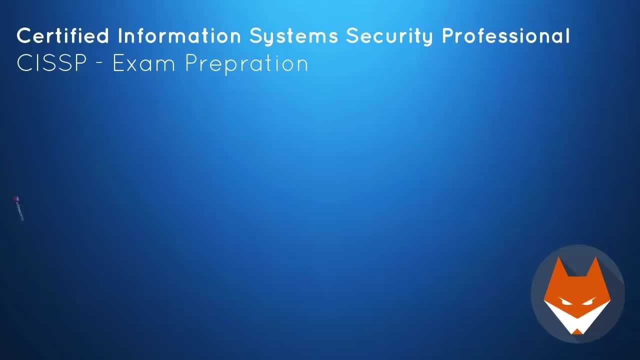 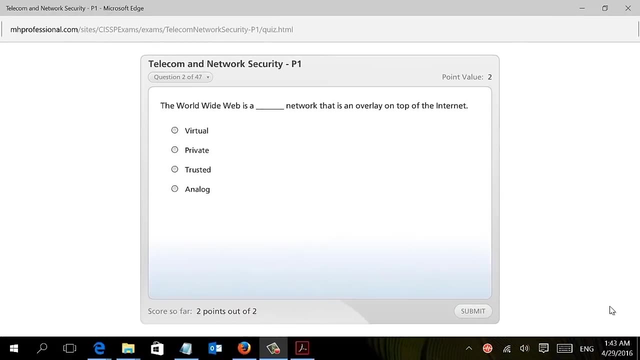 Now let's take some network questions. the worldwide webrebbeats Network in an overlay top of the internet. virtual, private, trusted an a lont, i think it's a virtual network. so an easy question: switch marries the technology of what and what. switch marries hub and bridge. 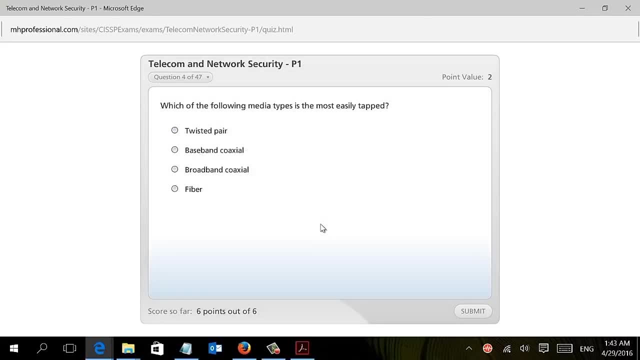 because habit was broadcasting, while bridge was not. which of the following media type is most easily to be tapped? most of the problem exists in everything except the fiber. so all this fiber is not inside the option. so twisted pair, for instance? actually, those are quite easy questions, but 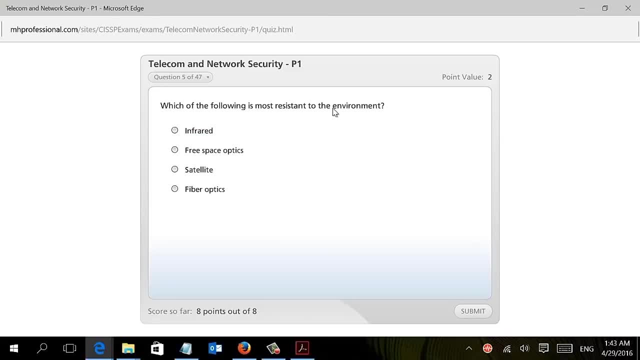 okay, which of the following most resistant to environment? anything that has a lot of feature will be the fiber optic. i mean, you know, it seems that whatever we got was kind of easy questions, but it show you that it's not that complicated about network. it will be more into the definition, or 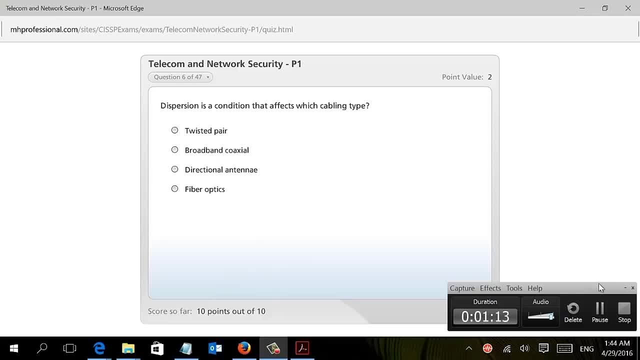 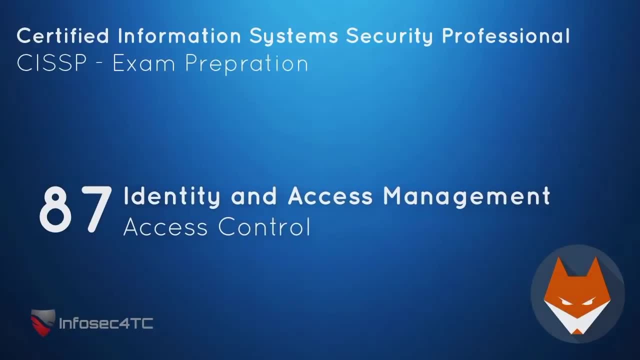 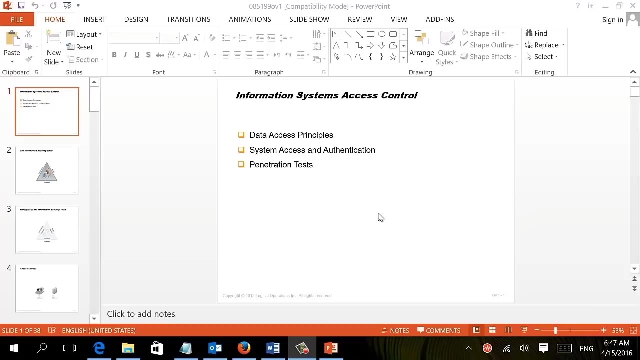 the characteristic of something that we're going to talk about in the next video. so let's get started. first domain that we are going to discuss will be the access control. now, before going through the domain and explaining the details and finally, before going through the exam questions. and what should you expect in the exam. 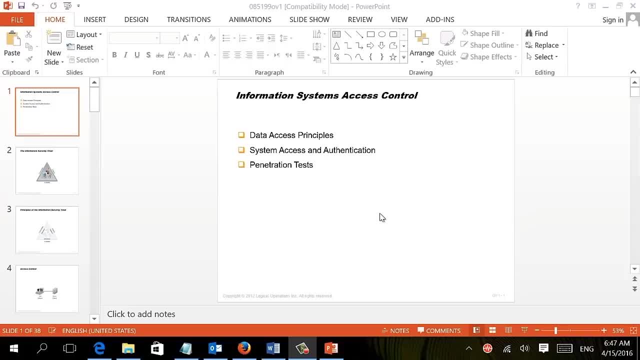 when it come to access control, we have some definitions that we need to explain. so, first of all, we need to explain the. so the first definition, which is extremely important. it may seem simple, but actually, when it come to exam preparation, this is kind of important, which is: how do you define security? 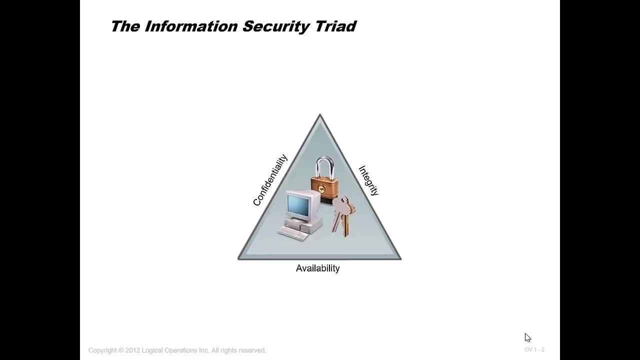 i think i mean before explaining any topic or any domain in this course. how can you define security? how can you say that your organization is secure? we have the security triangle, which is three factor. if you can implement them, you will consider yourself secure, which is confidentiality and integrity and availability, also known as 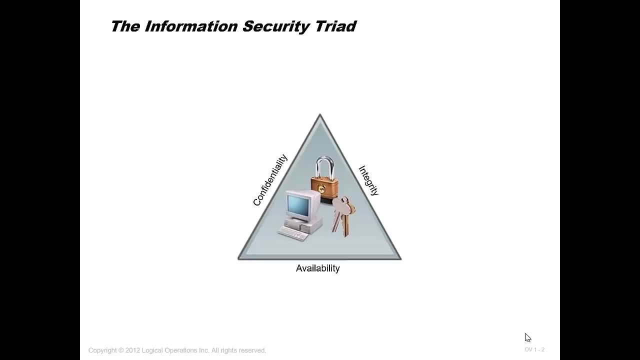 cia. so security is defined as confidentiality, integrity and availability. so whatever we're going to explain during this course should be under one of those category. so, for instance, if we are implementing password and access control, this is considered to provide confidentiality, because when i'm implementing a password, 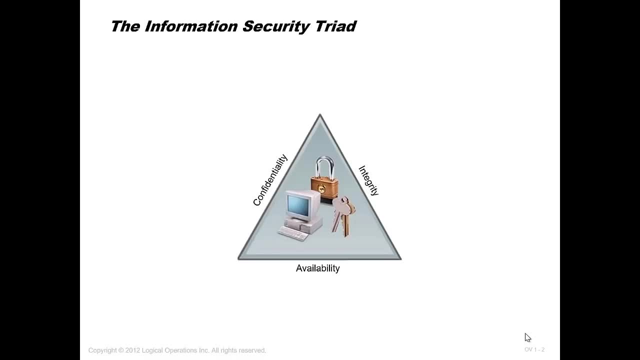 or an access control. i make sure that only authorized people will have access to the information. so now i can make sure that unauthorized people will not have access, so i can provide confidentiality. while if i'm talking about taking back your assets or assets from your account information, while if i'm talking about taking back the intellectual information, 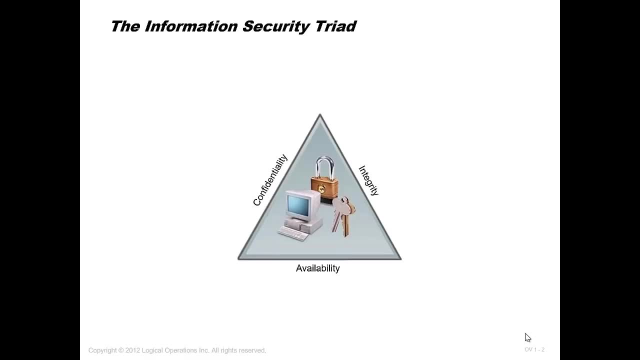 and doing redundancy to make sure that the information is available all the time. this is to provide availability, while if I'm doing something that will confirm that the information will not be manipulated, this is considered integrity. let me give you an example. assume that you are sitting somewhere and you are. 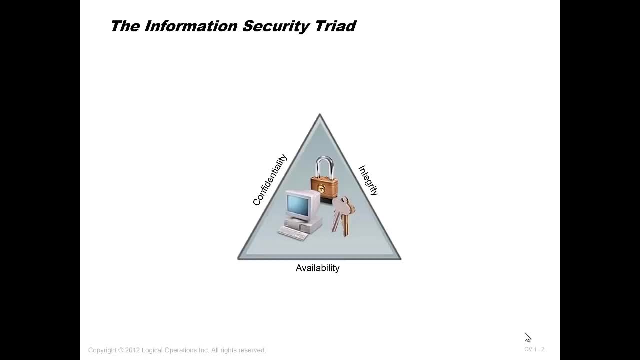 connecting to a website and you are writing. you are buying something from a website, so whatever you are writing, it will go from your client computer to the backend server that is located in another country. so, assuming someone is sitting on the same network, maybe you are in public place you are connected to- 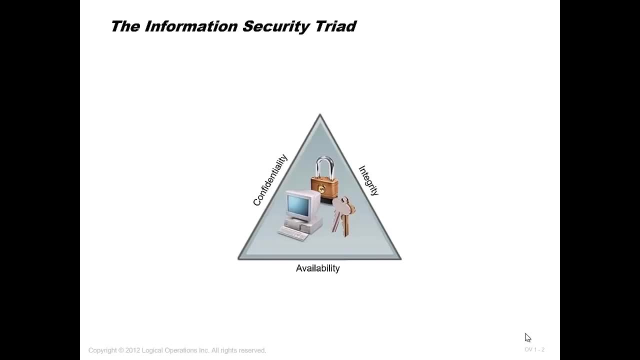 the public Wi-Fi. he's sitting on the same network and he's sniffing the network. will be talking about sniffing inside the attack, so he's sniffing the network and whatever you are writing, he's, he can see it. he can see your credit card information, your personal information. now, this is against. 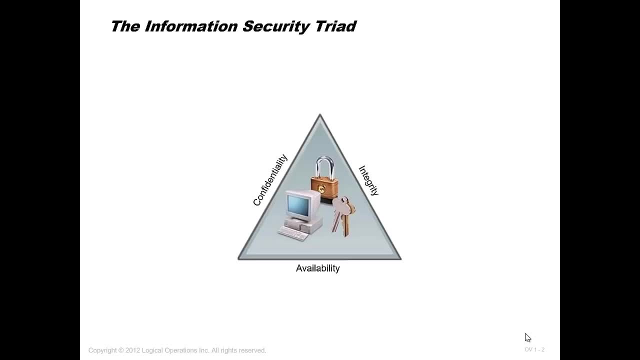 integrity. whoever designed this network didn't provide integrity, meaning that the information will not be sent from the place a to the place B without being manipulated. so someone can sniffer the network, he can see what you do, he can change. so this is against integrity. so any topics that we are covering during 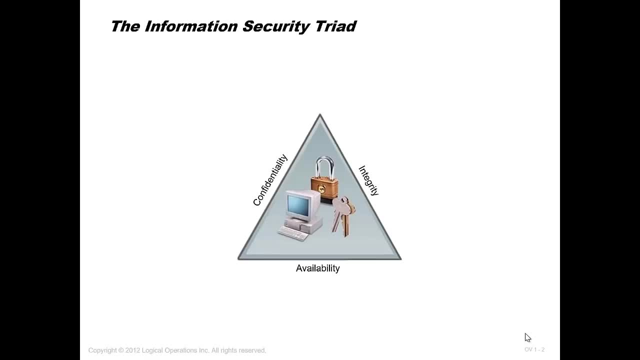 this course should be under one of those three category: confidentiality, integrity and availability- and actually you may find that inside the exam. so, for instance, he may ask you: cryptography, encryption and decryption- it's providing what? confidentiality or integrity or availability. cryptography provide confidentiality and integrity, but has nothing to do with availability: access control, provide what and so on. and 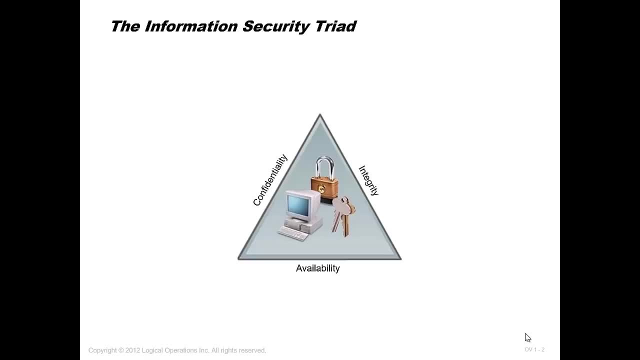 so forth. so anything that will be explaining during this course, before we start explaining you have to first think what exactly will be provided from that. so I can only say that I am secure if in my organization I can provide confidentiality, integrity and availability. this is the first. 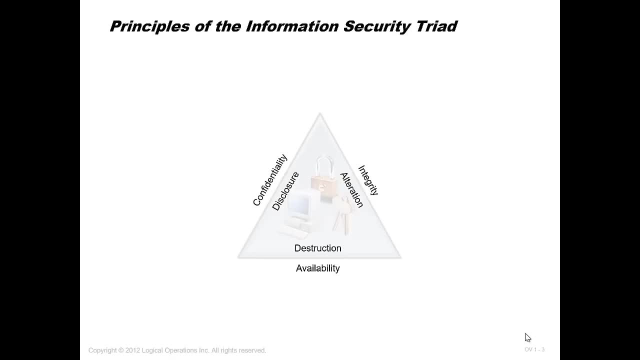 definition and, as we agree, you should always think about what is the benefit of implementing some control. is it for confidentiality, is it for integrity, is it for availability? this is extremely important as a basic definition. the second definition that we need to point to before we start our course is the. 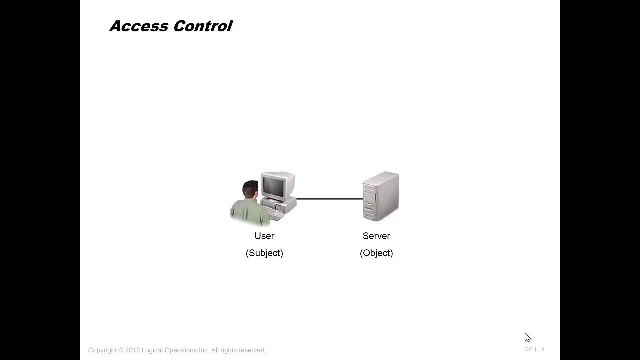 names. so usually when we have someone accessing computer, we call this a user and this is a server or computer. now we're going to use different name. during this course we'll be using subject for user, an object for the resources or computer or server. so now we have a subject who access an object. 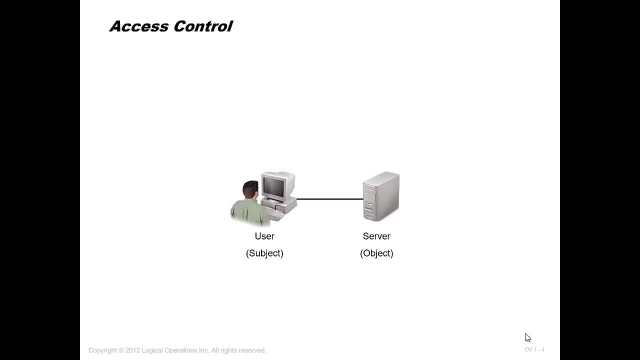 subject most necessarily is user. sometimes you are connecting to a website and then you need to buy something. so the webs- I mean when you are connected to the website- you are the subject and the server that holds the website is object. but the object is connected to another backend server from. 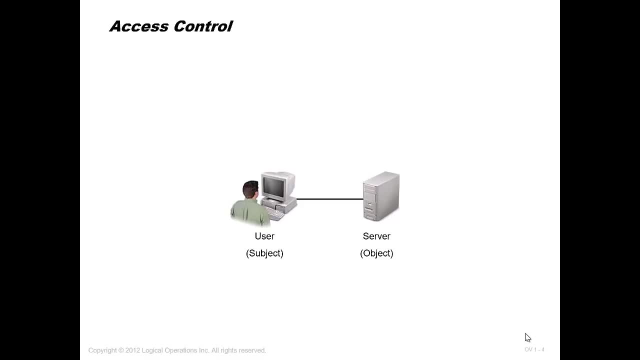 where he's retrieving information. so now the server becomes a subject and the backend server becomes object. so whoever access is called subject- people or a machines- and who ever get access to, I mean like a server, this is called an object. so the names that we'll be using during this training will be subject and 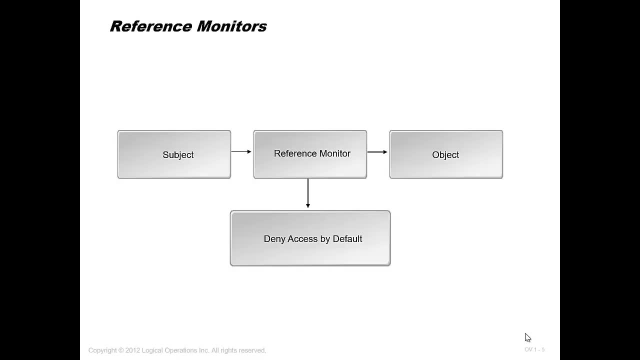 object, not user and server or client. so the subject are accessing object and getting information from object and the rule is saying that by default is denied. so the rule in access control or the rule that the subject cannot automatically access object, they should be some control and this is what will be. 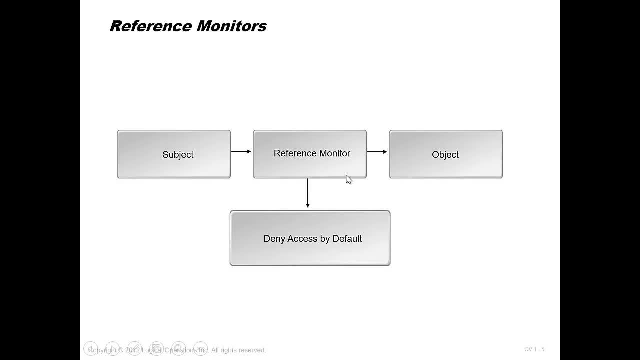 explaining inside the course, inside, I'm sorry, the access control, so they should be some control and this control. if no setting is done in this control, by default, subject is not allowed to access. object: you as user, by default you cannot access other people as our people account, bank account, unless you have a permission. 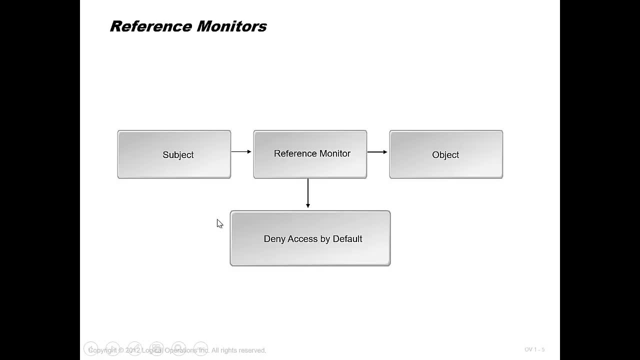 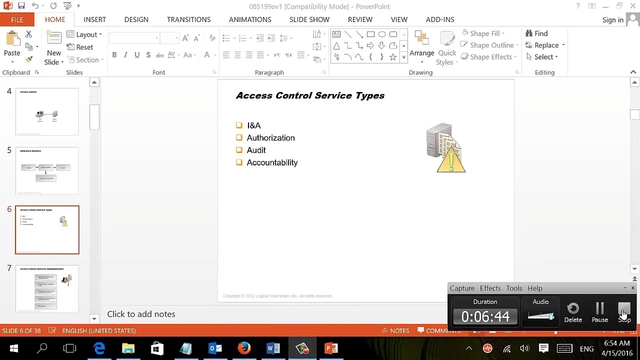 for doing that. so the default rule is: subject: it's denied to access object. okay, now on the next lecture, we're going to start talking about the access control, and what exactly do we mean by access control? before we start talking about access control, I just want to remind you with 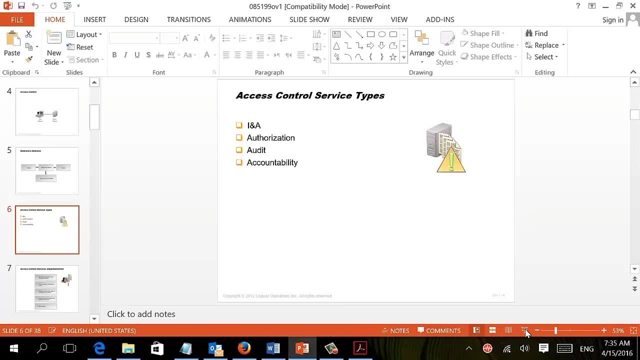 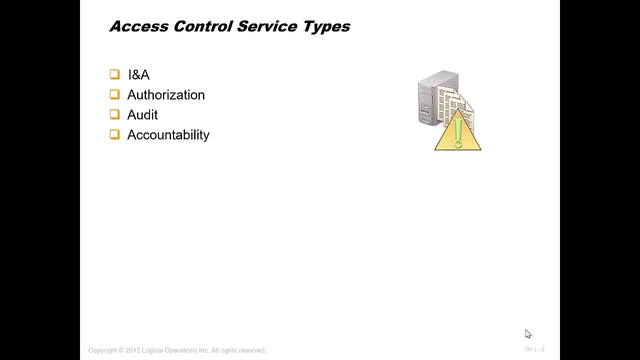 the introduction lecture, where we agreed that when we are talking about information security, it covers three different area: it cover physical security, cover technical security and it cover administrative security. so, from now on, whenever we are talking about any topic, do not just consider the technical security, Because, as we discussed earlier, most of us came from the same background, which is which is a technical security? 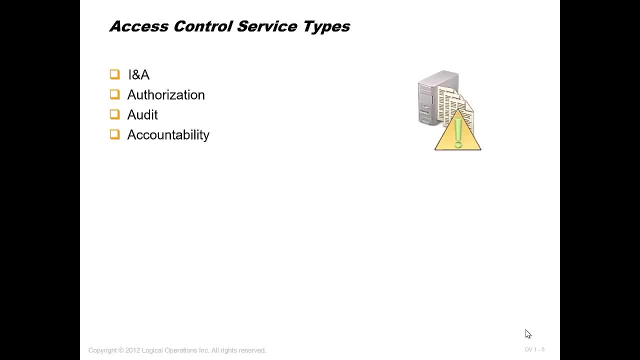 But now we'll be talking about technical security, also known as logical security, and physical security and administrative security, And we're going to start by defining what is an access control. Now, assume that you are doing a security implementation for any organization, A new company it's, you know, it's launching their business and they ask some experts to implement some security. 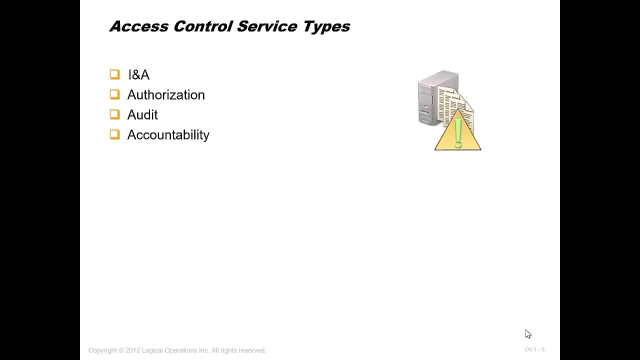 What is the first step that should be done in the security? What is the first implementation of security? It's usually the access control. Access control has another name, which is AAA: Authentication, authorization and accountability. So when we are talking about access control, we meant three different items should be implemented. 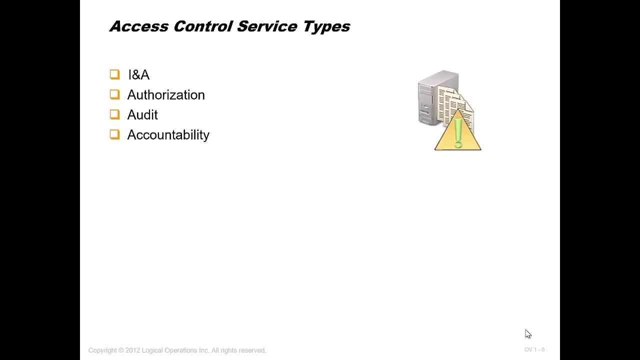 I mean when I'm saying we need to implement access control. it's not just to implement a password on the system or on the door or something like that. It's that we are implementing three different items- authorization, authentication and accounting- So that access control usually refer to authentication. 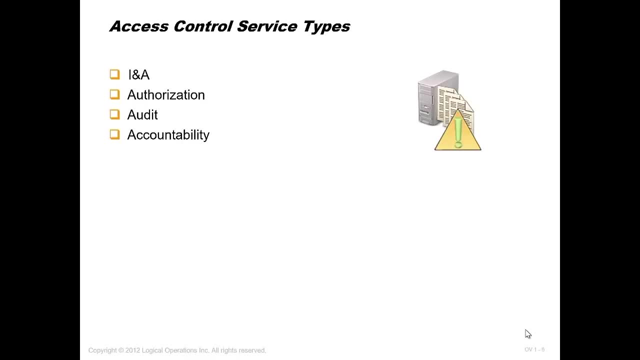 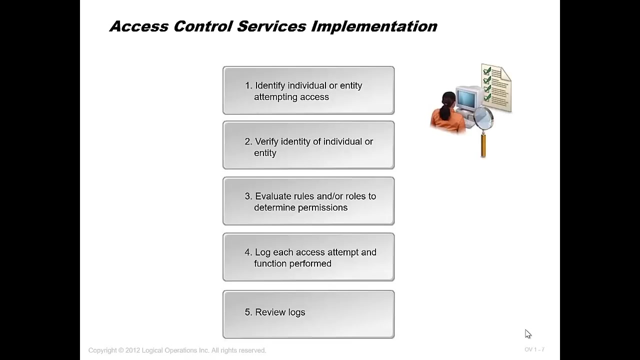 Authorization and accounting, And we add to that the I, which is identification. So we're going to explain each one of those: the identification, authentication, authorization and accounting. Now here is the proper way for implementing the access control. First, we need to identify the individual or entity attempting to access. 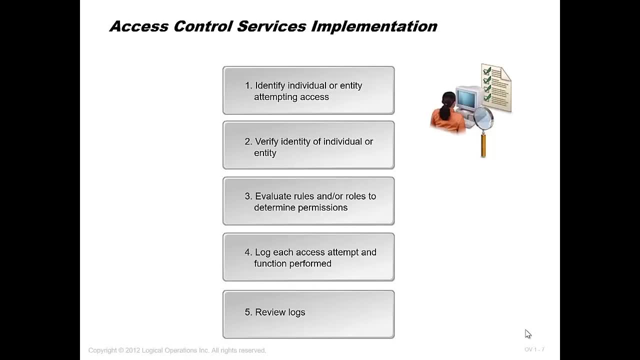 So we have a company And we have some employee. We need to know who will have to access the information, the premises, and we need to identify them. Are we going to allow only employee to access our information? Are we going to allow the contractor? 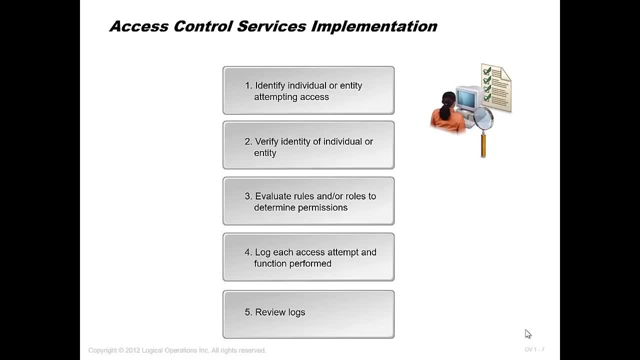 Are we going to allow our customer, who need to identify who will will access our information. So it started by identifying the people, The people who are going to access the information. Then we're going to verify the identity of the individual or entity. OK, so assume that we are in an organization and I'm going to give access to all my employee. 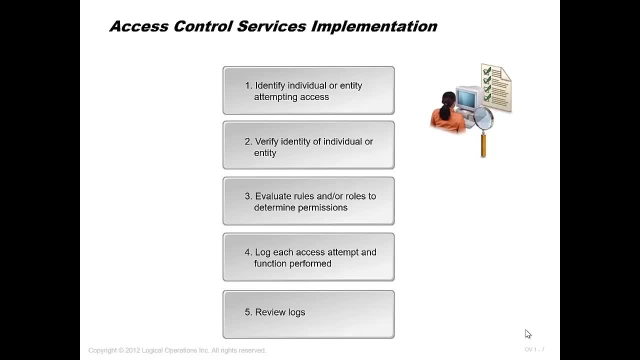 OK, this is the authentication part that people will have access, But definitely this access will be with different kind of permission, I mean definitely the CEO of this organization. We'll have different type of access than regular employee, then labor right, then the driver. 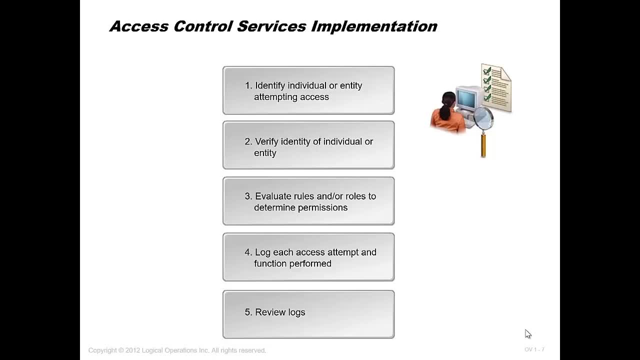 So different people that may have access should have different permission, And this is what we are calling authorization. So authentication is to identify the people that are going to have access to the system, where authorization is to give those people different kind of access, because it doesn't make sense if I give all the employees same kind of access. it will not make any sense. 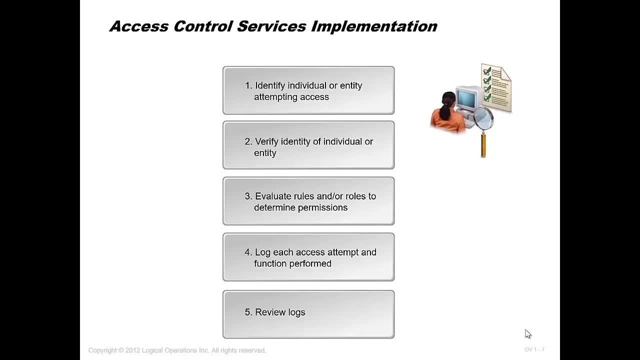 The third part of the access control, which is logging. So I have to whenever someone access to the system and the system one more time. I'm not just talking about technical system. It could be the technical system, It could be the physical premises. 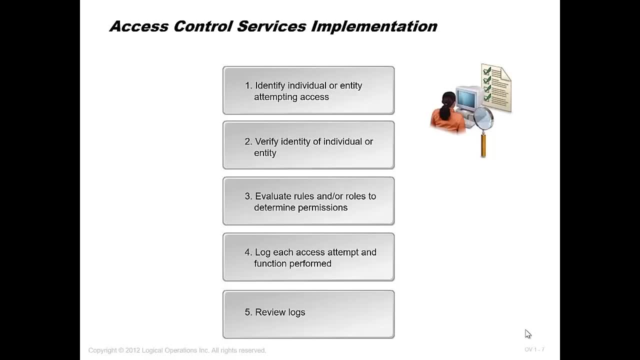 But to ever one of the employee access some resources, I should log that in a logging system so I can later on review them. if someone is telling me someone logged in Last, Last week at this time, I should have a record from where I can identify. this is called the logging or the accounting, and definitely this to be a need to be reviewed periodically. 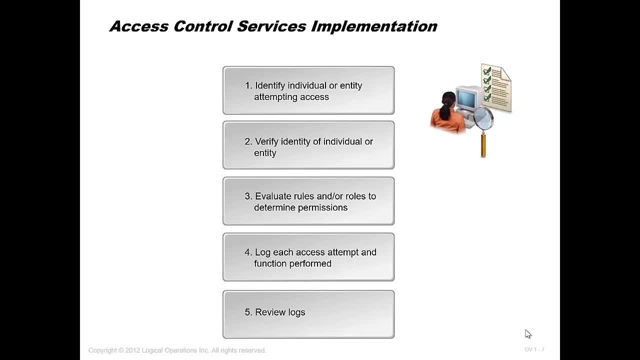 So the point is, implementing access control mean implementing authentication, implementing authorization and implementing accounting, And each one of those item will be explained during this domain And we're going to talk about different model. if we are talking about authentication, How many Models do we have? 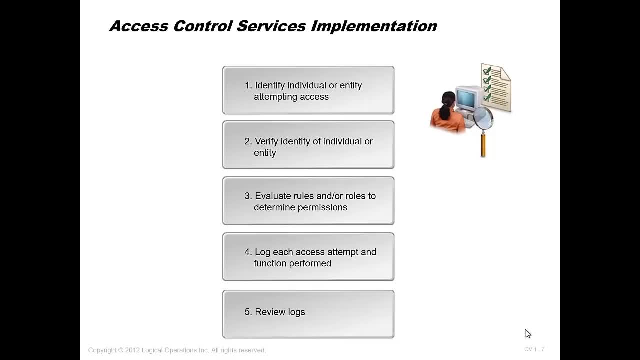 We have something, you know something, you have something. you are going to explain that in depth in a few minutes. If we are talking about authorization, how many model do we have and which model is more suitable to our business? We have the Mac. 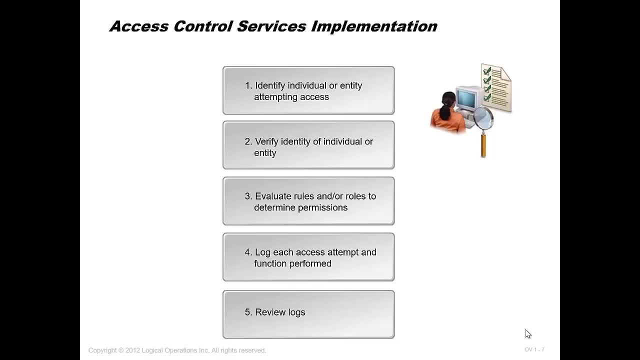 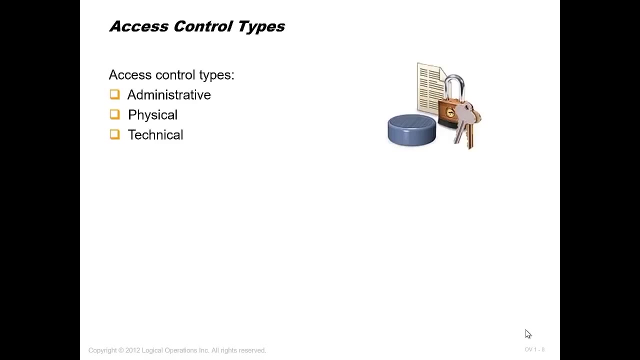 We have the deck, We have some on deck. So each of those category of the access control has different model and you have to select what is suitable to your business. As we agree, access control- it's administrative access control, physical access control, technical access control. 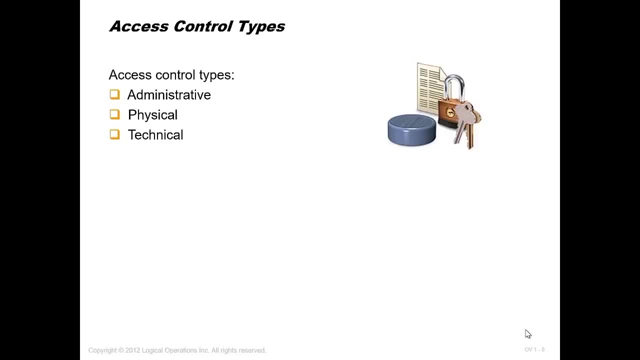 So, for instance, let's talk about technical, because most of us came from technical background- If we are assigning a username and password on our system, this is authentication right, While when we are assigned permission of on file and printers and resources, 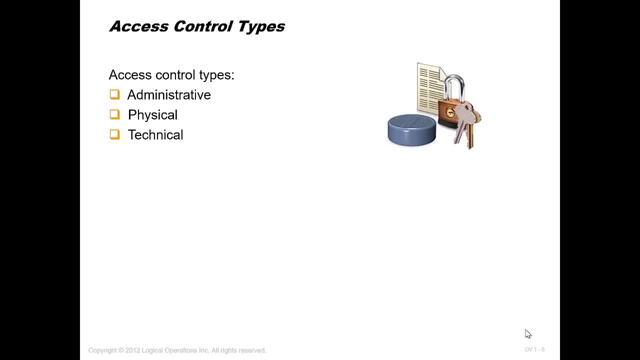 Different permission to a different user. This is authorization And when we are keeping the logs for all the user activity, this is the accounting part. physical security: When people have access to the facility or to the organization door or they have to the data center, they have access to it. 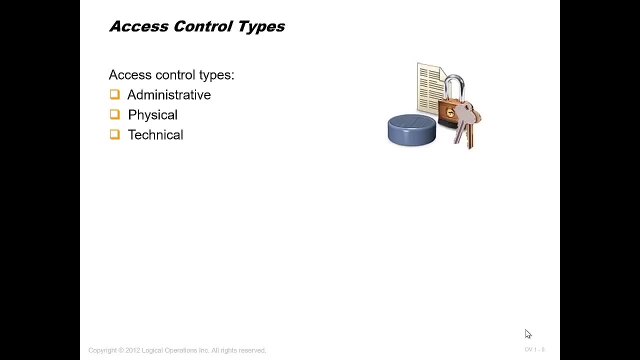 This is authentication. Maybe I have access cards that allow me to go to an organization, but this access card will not allow me to go to any place inside the organization. Maybe some places I'm not allowed to, like the technical room, like the data center, 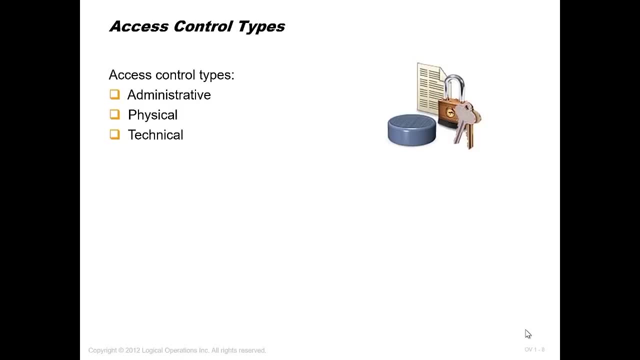 This is called authorization. And finally, definitely I'll be having logins that will allow me to trace if I need to get a specific record for a specific date. This is accounting, So access control is implemented not just on the technical, but technical, physical and administrative. 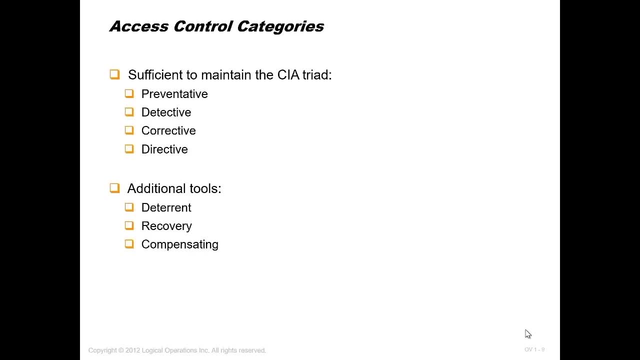 Now the category of access control, And I are actually let's. let's explain. Let's explain That in a more wide way or more generic way: in security, We have different kind of layer, Or when we implement security, we have different kind of layer. 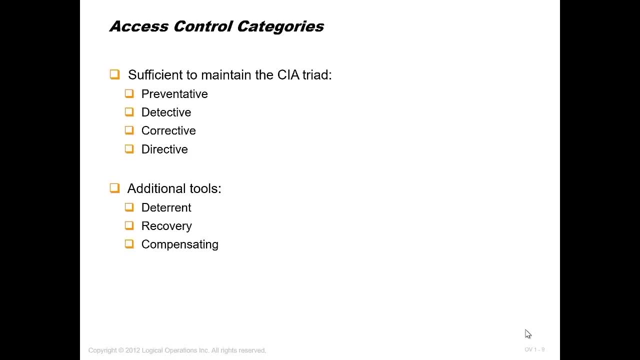 And please give attention to this slide because it's a little bit confused And I remember an exam question that was confusing about this part. So usually we have a preventive layer. So in security we have a preventive layer Like what? Like the firewall, for instance, in technical, like firewall, firewall prevent intruder to log into my network. right in physical, the door. door is a preventive layer that will not allow intruder to go to my facility, while detective layer could be something like surveillance scam. 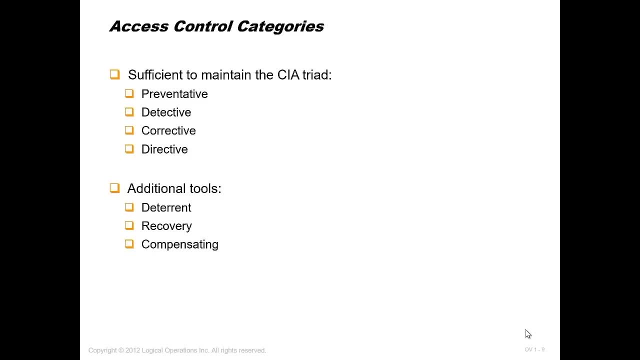 If you have a surveillance scamming inside your organization, it will not prevent an intruder but It will Detect. and then if an intruder in technical, what do we consider a detective layer in detect? in in in physical security, I'm sorry- in technical security? the ideas intrusion detection system. this is software for people who didn't work with ideas before. ideas is software that map or that sniffer the network and any suspicion behavior. 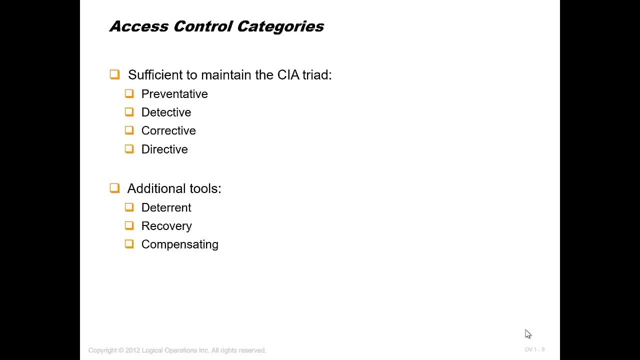 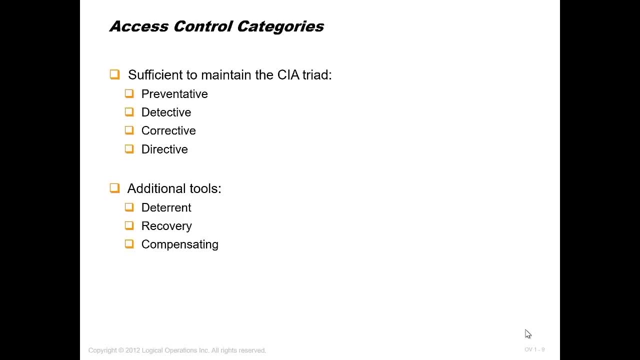 This is a corrective layer and directive, or sometimes called deter, So directive, and I believe they are the same, which is just an indication. If you have a sign on the door saying for authorized people only, This is a deter, Or also called directive. 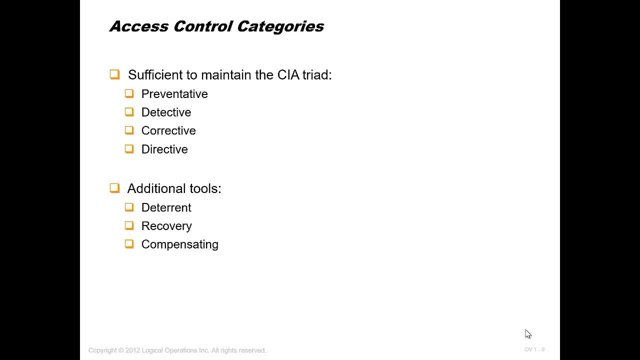 I mean it's, it's, let's. let's focus on the third right now. It tell people that you should not be allowed to go in. Why we are using that. Sometimes you find the sign and the door is not even closed. Why is it? 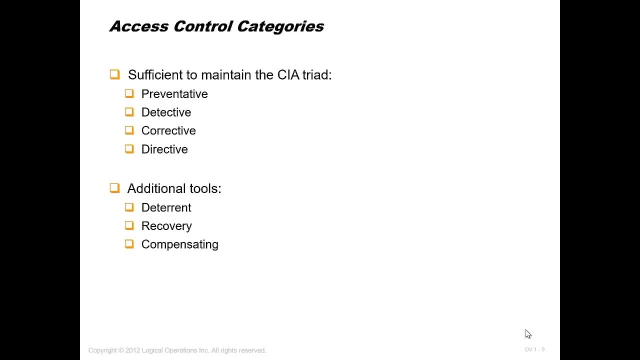 Is it important to have a sign telling you that it's deter? It's important from a legal perspective? I mean, if I find the sign on the doors that saying that this is for authorized people only And I ignore that And I enter the door. 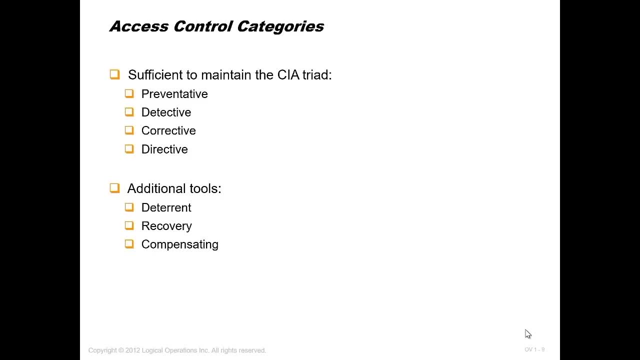 You know, those people hold will have some legal, as they can take some legal issue against me, because I knew that I should not be inside and I went inside. So the third is important. Here is a trick, Here is a tricky question. Exam question actually. 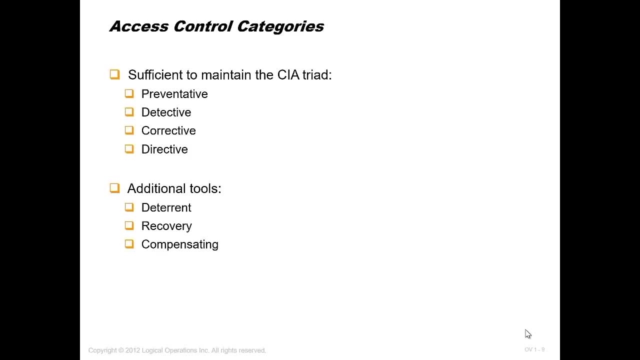 Fences around the facility. What do you consider them? Are they preventive, detective, corrective, deter? Actually, most people would think right away that fences is preventive, But actually- and we're going to see that in physical security fences according to IC square- is it's deter? 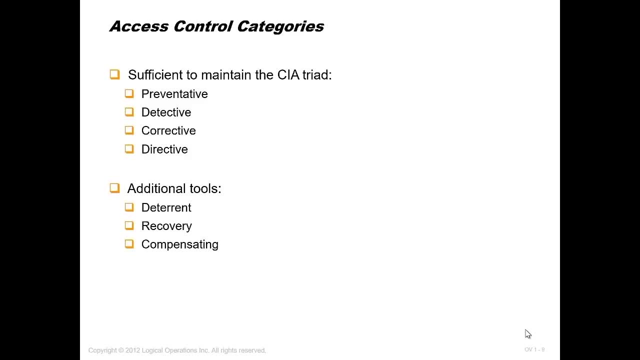 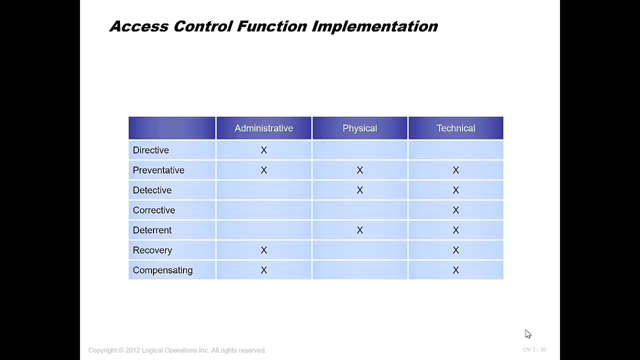 No fences will stop an intruder, So it's a deter, It's not a preventive, and this is showing you the kind of tricky questions that you may find inside the exam. So we're going to start with access control implementation. Okay, And I'll start with authorization. 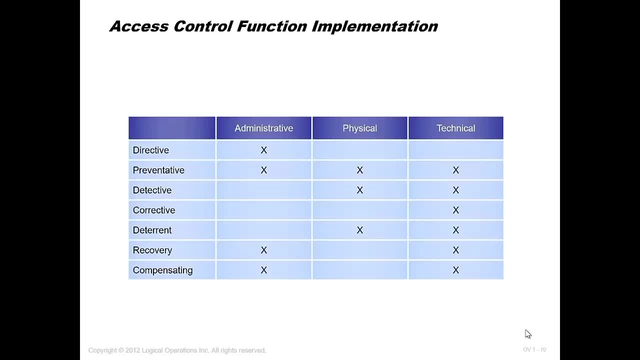 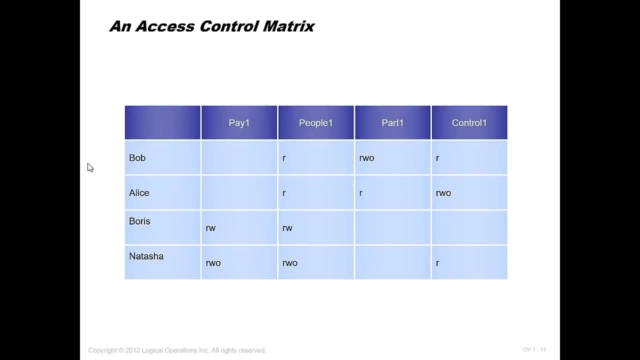 The different authorization mode. I mean, I know that we have three different items in the access control: We have the authentication, We have the authorization and we have the accounting. but I would like to start with the sorry. I would like to start with the authorization. 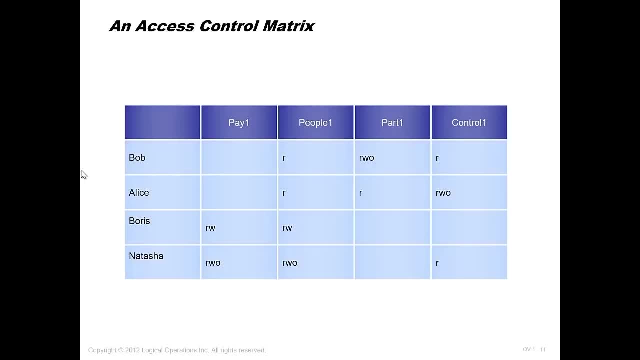 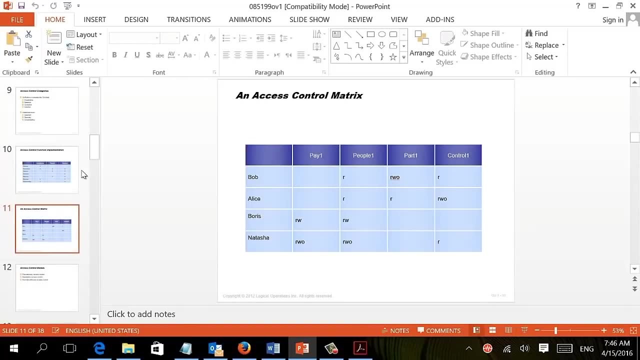 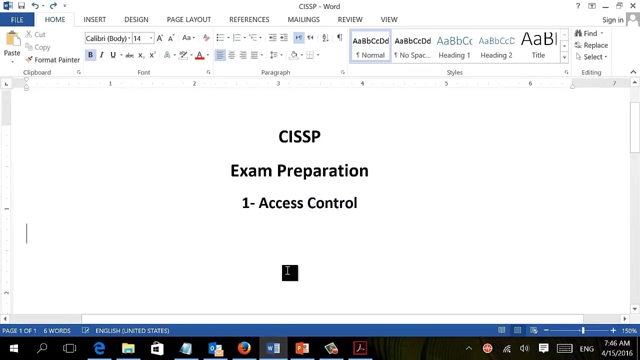 Second one, the type of permission. Now let me go to my board and let me explain this part. So in authorization, to make sure that we have enough time, Yes, So I'll talk a little bit about authorization right now. We have three different model that we can implement when it come to permission. 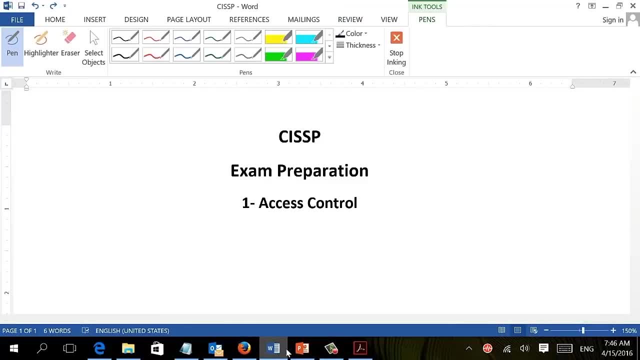 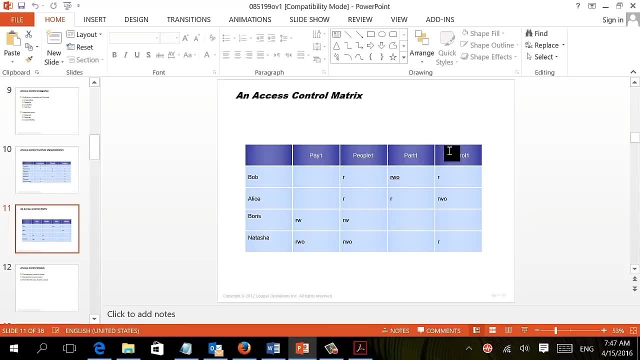 The first model. This is the model we are using in Windows. So in Windows, how do we provide permissions? We will get all the resources, file or printer or folder. So we have this file and this file and so on, and we will get all the user. 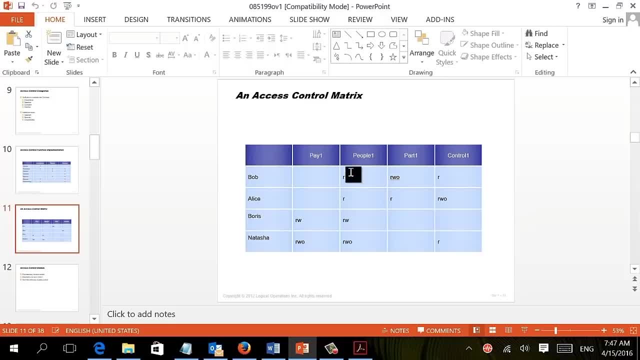 This is called a matrix, and then we're going to start assigning For each user some permission on those resources or on those file. So Bob has a read permission on payroll one, but he has no permission on pay one while he has a read. 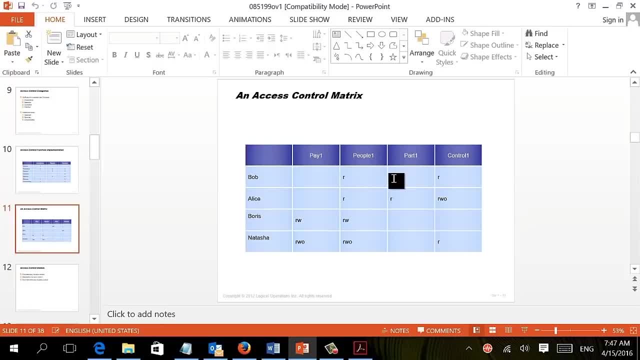 write ownership on part one. What is the difference between right and ownership? Ownership can delete and Alice has different permission on different file. This model is called the deck and this is what we are using in Windows, So the first model that we are referring to. this is the most common one and this is called 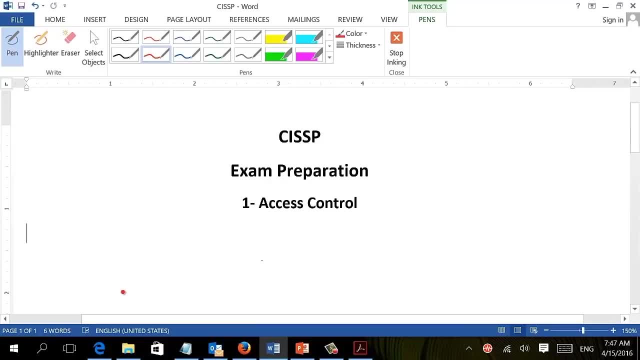 We just change the color. So this is called the deck model or the discretionary access control. So let me write it down. I'm sorry, It's hard to use those kind of Yeah, here we go. So the first model is: 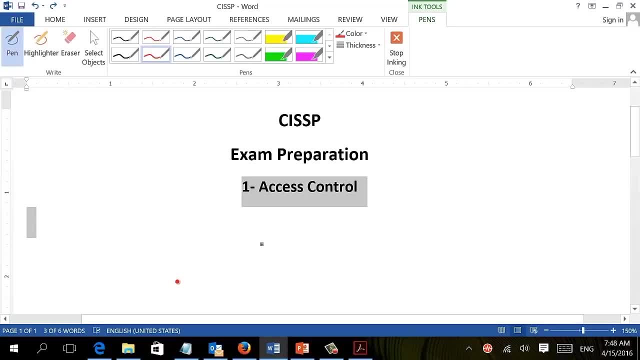 Deck Access control. The second model- It's actually so and this is what we are using in The noise Okay the screen truly access control. second one: It's called the Mac mandatory access control and this is usually used in Military and government, and this is quite different. 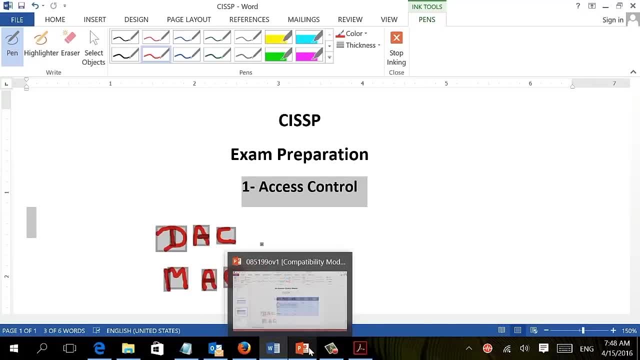 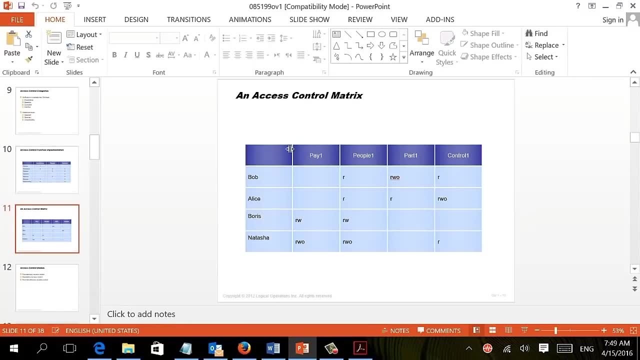 Okay, and you have to give attention to that because actually This is important for the exam. now, before going and explaining the deck, When it comes to assigning permission, who is the one who should say that? you know, Bob should have this permission and Alice should have this permission. 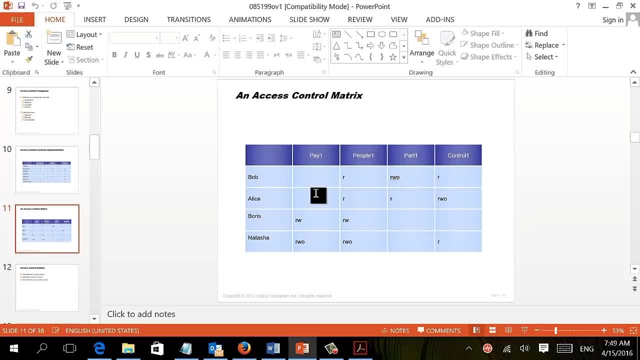 Is it the technical guy? Actually not the one who should say or should assign the permission. is the owner of the data owner? It's not necessarily the one who created the file, But maybe is the functional manager, I mean, I am the HR manager. 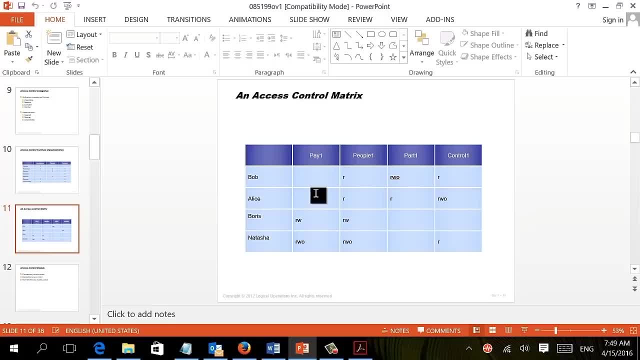 I know who should access what. so it's not the technical guy that should Assign the permission or decide about permission. It's a data owner. The technical guy should just implement those permission, but he's not the one who's deciding. now will be talking a little bit about the Mac. 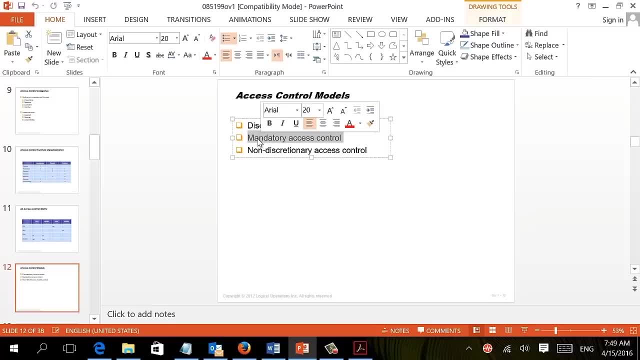 Access control, and I believe this is very, very important because it will be related to many subjects that will be talking about later on. So how the mandatory access control is working- mandatory, as I mentioned, it's different than the deck access control and this is usually implemented in military and in government. 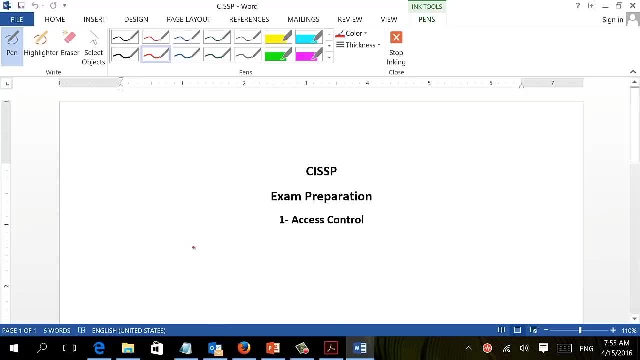 It start by data classification. So the first thing you need to do is one: you need to classify the information. I'm sorry about that. I think it's better to use the keyboard. So first thing we do, we get all the information inside this organization and we start giving them classification. 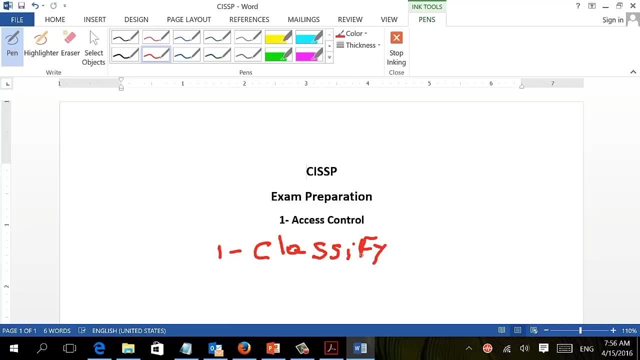 This is top secret, This is secret, This is confidential, and so on. number two: For each user, we are giving a clearance level, clearance Level. so this user maybe have a top secret clearance, This user maybe have a confidential clearance. So again, how is mandatory access control working? 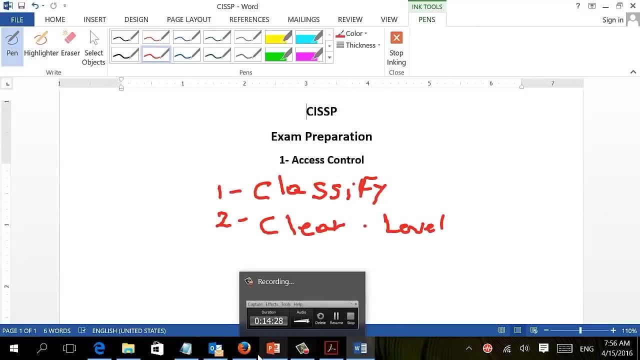 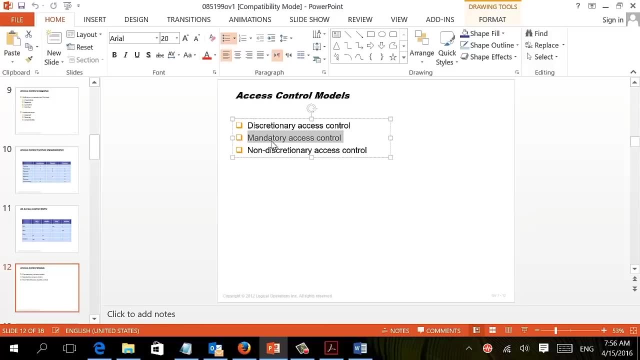 For each user, as I explained He will have. first you start by classifying your information, then, for each user, you are giving clearance level: top secret or secret or confidential, or now is that? by that do we mean that? Let me show you if I have an example for that. 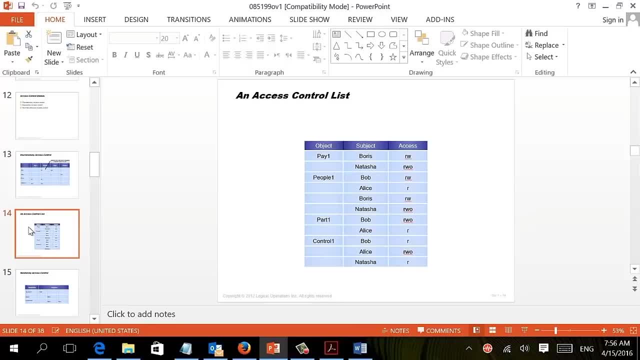 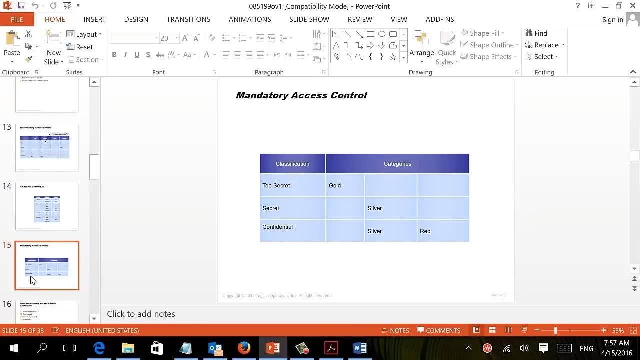 So by doing that, Does it mean that the one that has a top secret clearance can see any top secret? actually not. the another factor will be implemented is called need to know. So for me, as a user, I have a clearance level and I had a need to know that should match the clearance level or the classification level of the information and the information should have a need to know that. 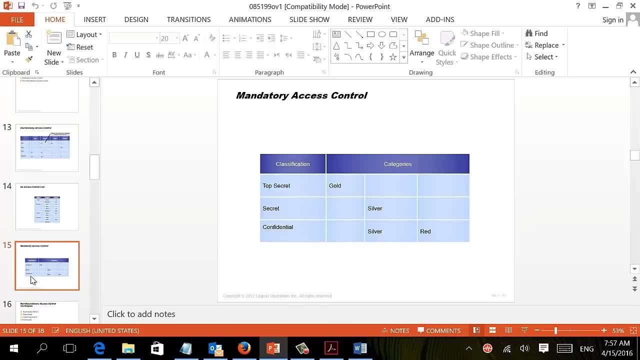 does not match mine. So, for instance, myself I have a need to know on, for instance, If I'm working in military, I have a top secret clearance, but I have need to know for only weapon information, so I can only check weapons information, and so on. so the implementation of mandatory access control is that we are classifying the information first. 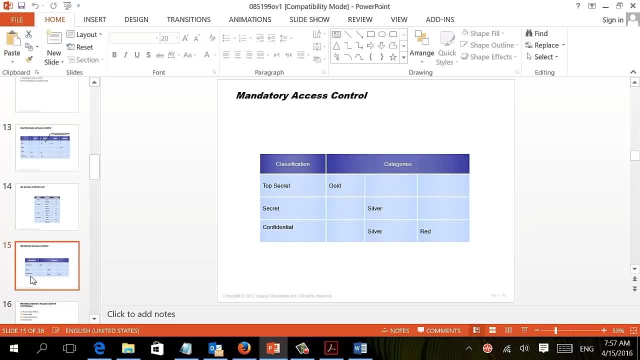 We have different classification and then we are giving for the user clearance level and we are giving them another factor called need to know, and their clearance level and need to know should match the data classification level and their need to know as well. so this is the mandatory access control. so 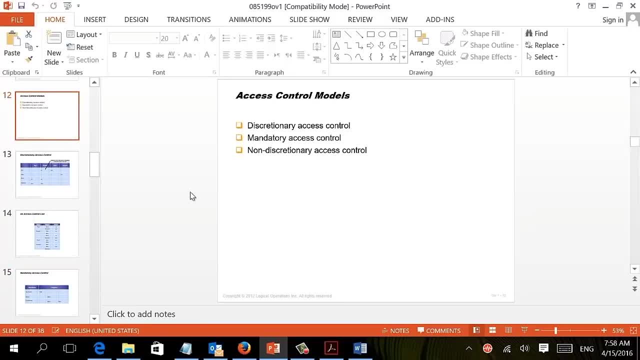 we have the Mac and we have the deck. we also have the nondescript- really access control. now other access control could be things like role-based access control. sometimes you are giving the access according to the role. so, for instance, assume that you have a department inside your organization that has a very high 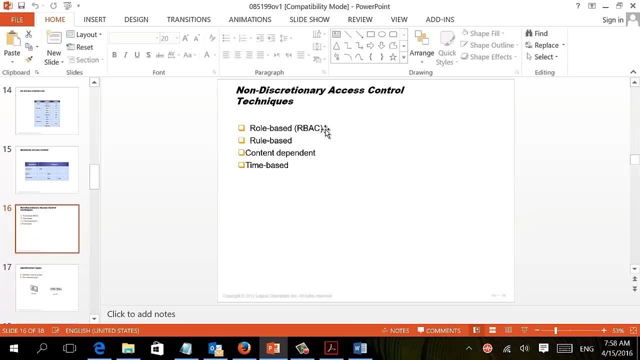 turnover. so people keep coming and going and resigning and hiring people. so whenever you have the company hire someone, you give him permission and then he will leave after a while. in this case is better to do that role-based. I'm gonna create an access control. I'm gonna create a group by the name of HR, for instance. I'm gonna give 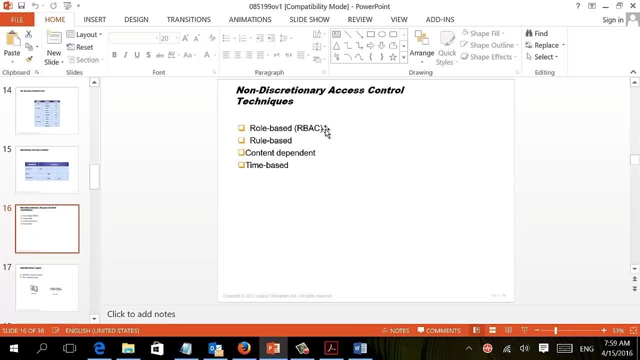 the permission for HR. I will not give permission for users. I'm gonna give them by role. so whoever is a member of HR will have those role applied to him. we have rule-based access control, like the firewall. firewall is a rule-based. you put some rules and any traffic coming in or out he will inspect those rule if it. 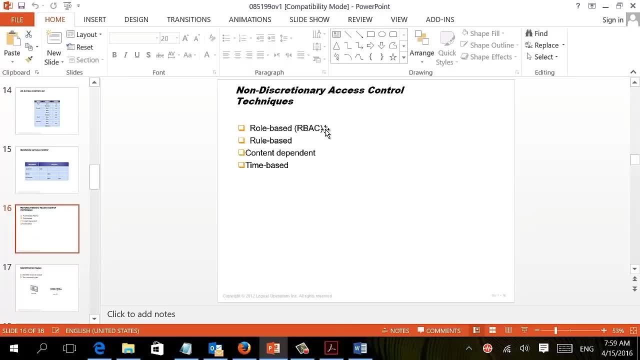 match, it will let him in. we have a content based. all of those is called nondescript, really access control. so access control based on the content and we have a time based. I can have an access controls that work from 9 to 5 through the working hour. so the point here is that we have three different. 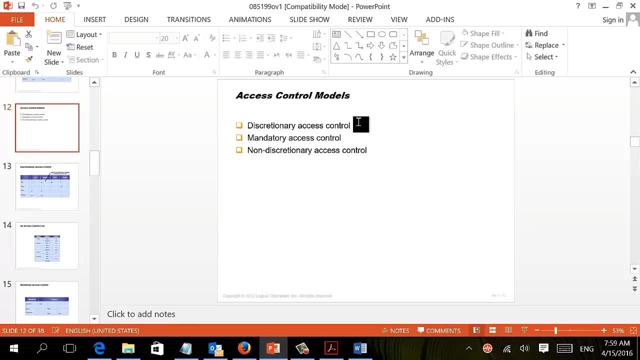 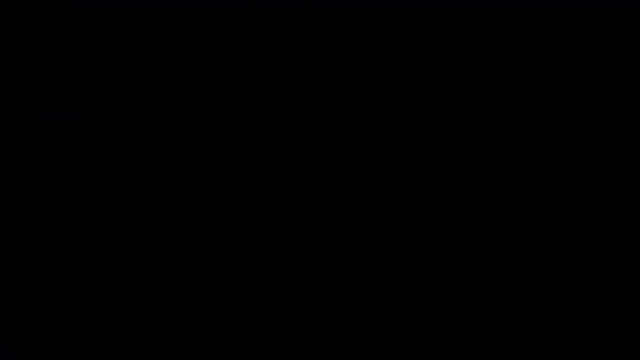 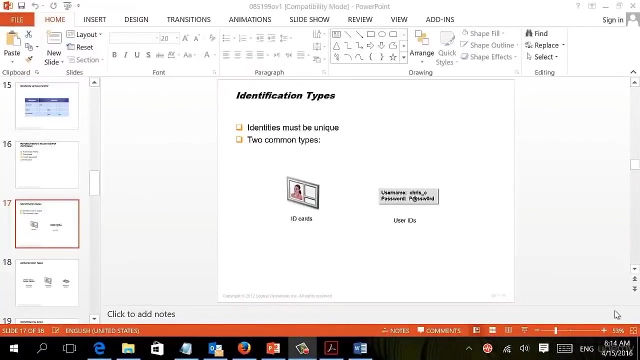 model when we are talking about authorization, the deck- this is one used in Windows, the Mac- this is the military or government models and nondescript is actually access control. on the previous lecture, we started by authorization, but actually authorization is the second step of the access control. first step is the identification and 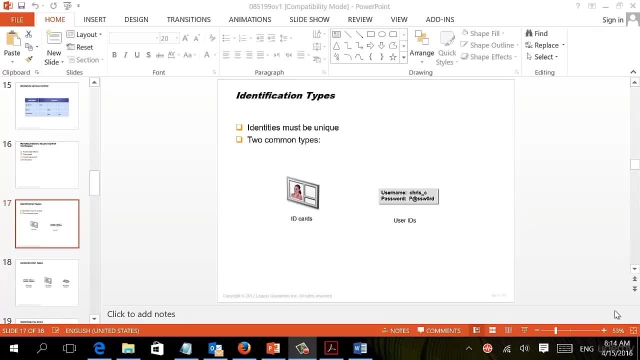 authentication identification is just to have username, so for instant. what do you think may make more sense when you are logging to a system just using a password? or you have to use a username and password, and username is not secret, i mean, it's written in a clear way, it's not hidden. why is important to have an identification part, not just a password? 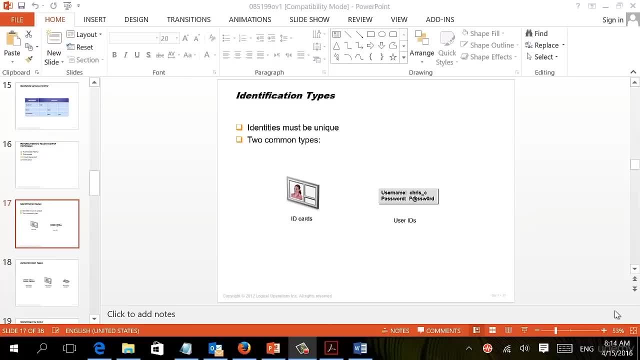 why do we use identification? why do we use username and password and not just the password? because it's helping for the accountability. i mean if all of us having only password, now if i'm checking some logs or tracing, how can i know which password belong to which user? so it's important. 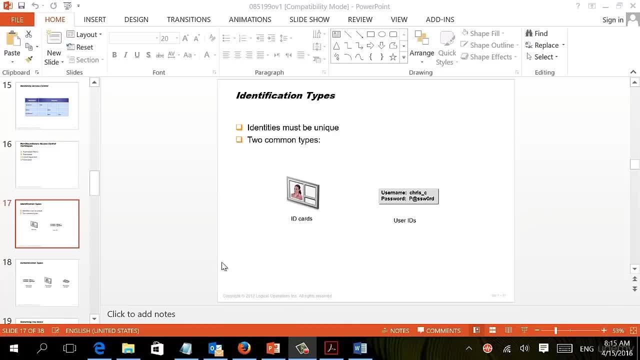 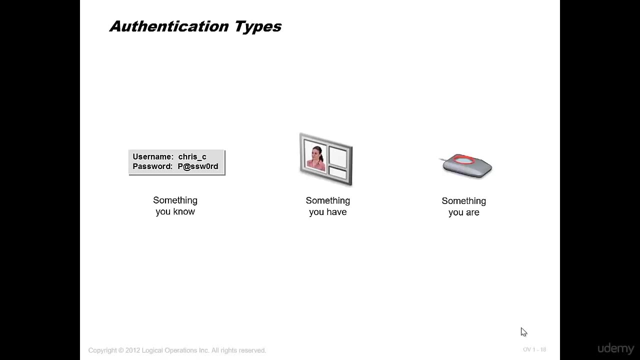 for identify, for logging. but the important part in this lecture will be the uh, authentication. okay, and authentication is the first step inside the access control and we have three different way of authentication. we have something you know, something you have and something you are. so the authentication could be: 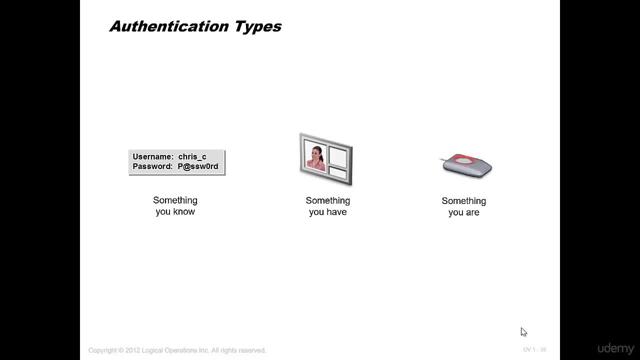 using three different model. i, as we explained, in authorization, we had three models: the mac and deck and non-deck. also, in authentication, we have three models that you can choose from based on the authentication. we have three models that you can choose from based on the type of your business and the sensitivity of your information. so we're going to start start. 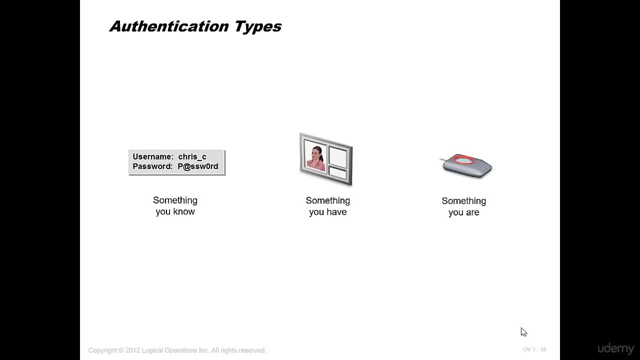 with something you know. something you know is the password part. so if you're going to make the authentication inside your network based on something you know, that's mean you're going to depend on people password. password is usually considered the cheapest and weakest authentication methods. i mean, it's very, very easy to crack a password. it's very, very easy to crack a password. 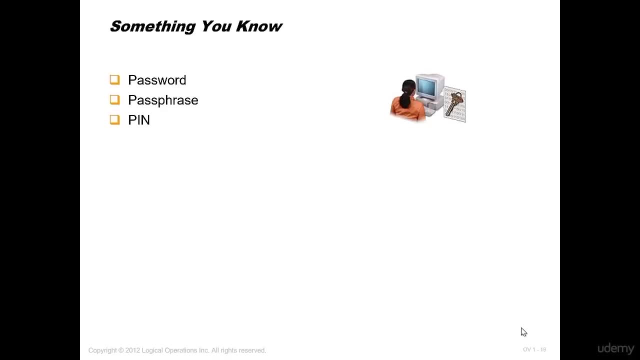 whatever the password was hard or complex, because password can be captured in different way. so that's why we always say that password is cheapest, because it will not cost us anything. i don't have to buy a reader for a fingerprint or a device for smart card. it's built-in inside the system. 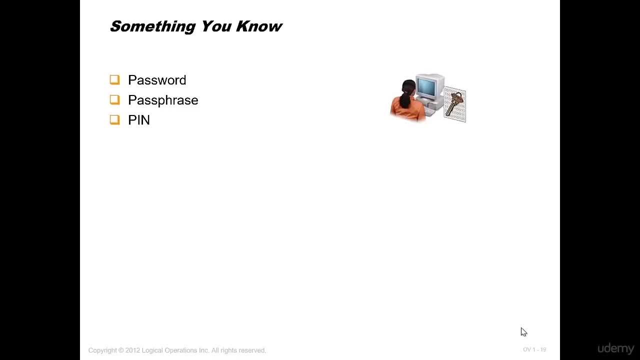 any system has a an option to allow a password on it, so it's cheapest but also is the weakest way. we have different way for assigning password. we have the password, which is a regular password. we have something called the passphrase, which is instead of password, and they are recommending. 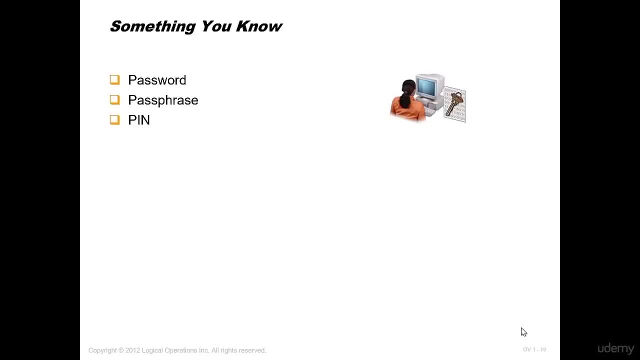 that right now you can write a full phrase. i like to do shopping on july- full phrase. so this will be a little bit harder to break, where to break and you have the pen, like you know, the ones that we are using on our atm machine and so on. so there is different format. 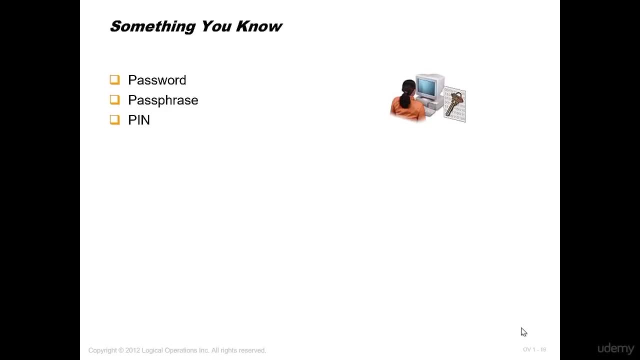 of the password, but they are all common. that it's all are something you know. i mean people need to memorize that and it's not easy. i mean now the best practice when we are talking about password, that user should have different password, all of them complex to different. 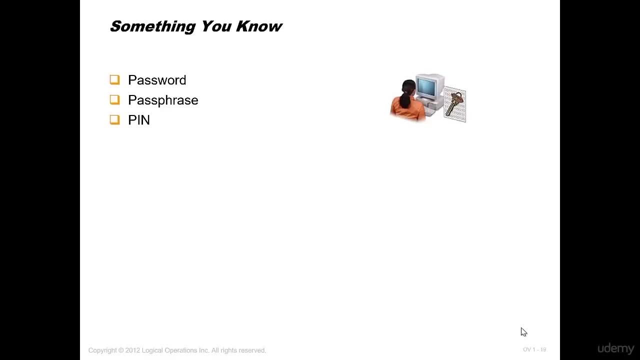 account. it's not easy to implement, that you know, because people will not memorize six, seven password. all of them are complex for different account. so it's not that easy to implement those different type of password, password, the passphrase pen. we have something called cognitive password which is like: what is your mother middle name? this is called cognitive. 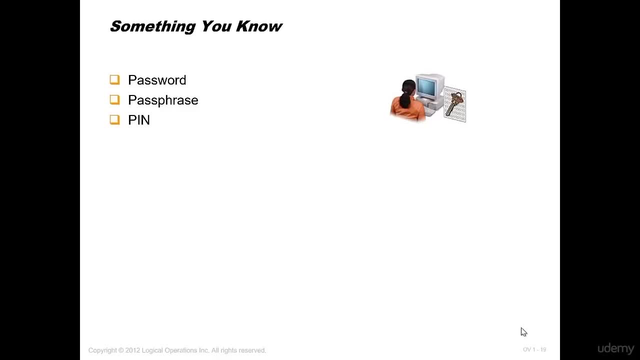 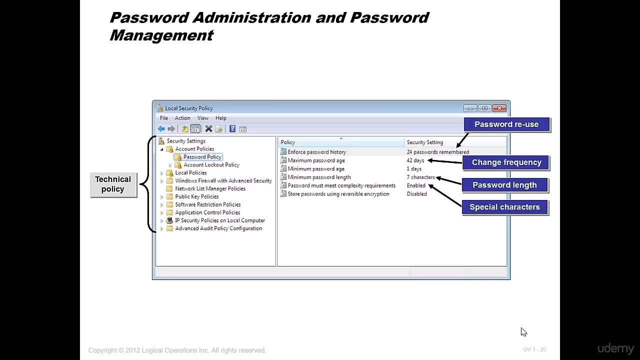 password and while we are doing a summarization by the end of this chapter, we'll be going through those different terminology related to the access control. so this is something you know. of course, if you decide to implement a password as a way for authentication- or this will be the model for authentication- you should have some control on it. 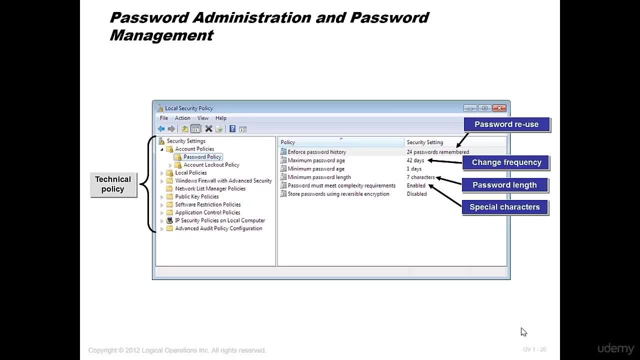 so you should implement some policies like what, like the one we are using in windows. password should be complex more than in character. it should be having capital and small, should have a lifetime, it should expire up to one and you have to enforce user to change their password, so you should have 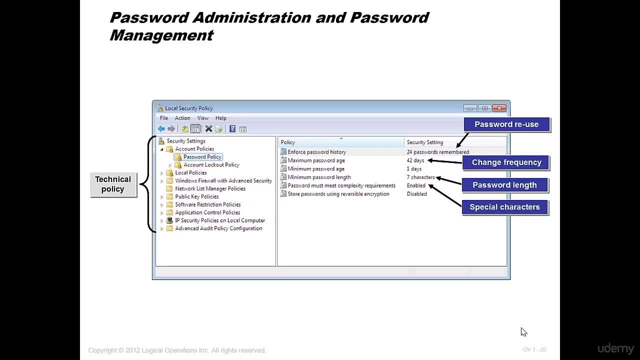 some control. at least you are hardening your password, but after all, i have to tell you that this is a very easy way, so i cannot guarantee 100, whatever policy i'm implementing, that this will make us comfortable. what kind of password we are talking about now? technical password, but what? 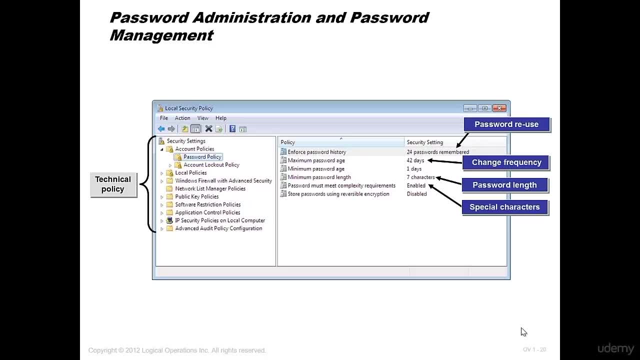 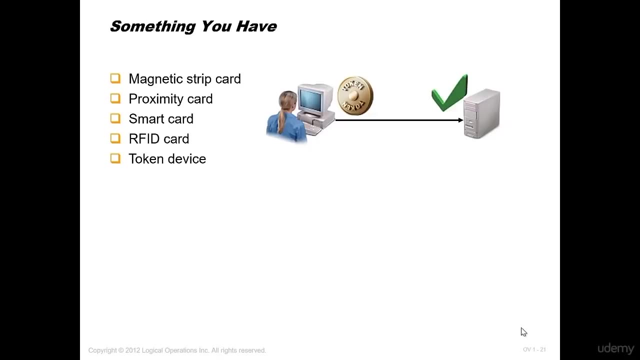 about the physical password. if i have a pen number on, like the doors, people access the door using a pen number. it's the same same concept as a password, but it's a physical password, sorry. so another model for authentication, something you have. it could be something like a smart car. 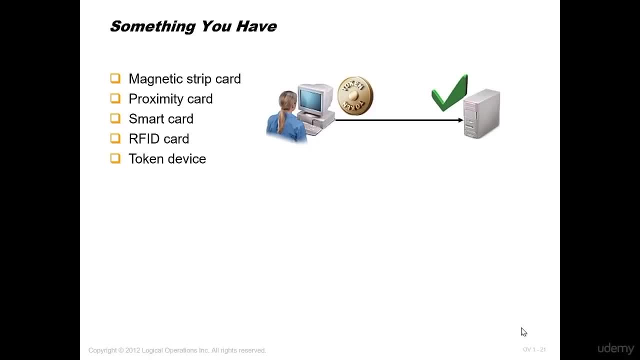 it could be a magnetic strip card that you can sweep and let you in, or sweep on yo or your smart, your laptop and login. it could be an rf id, radio frequency id that you know you just need to wave in front of the reader, and so on. it could be a talking device. 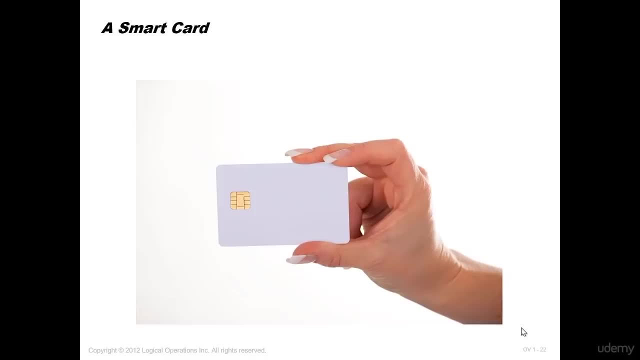 i'll just focus about the smart card and talking device card. you know it's a card that has a shape. this shape has some information. you can use that for authentication. now, what is the problem with with this kind or this model in general? what is the problem with something you have, the 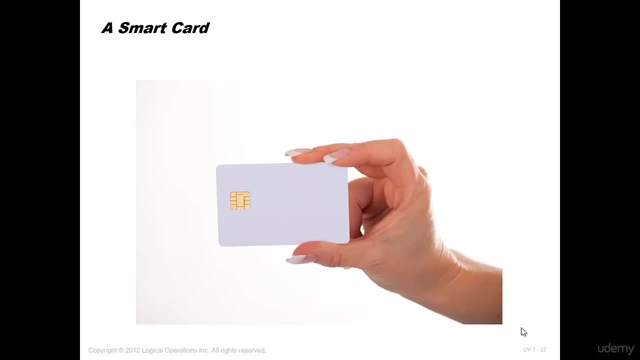 problem is it's it will cost. it will definitely be more expensive than using the password beside. people may lose those devices, so whenever they lose a card, you need to issue a new card or a token device and so on. there is one attack related to this kind of card. is called micro. actually gonna get that? 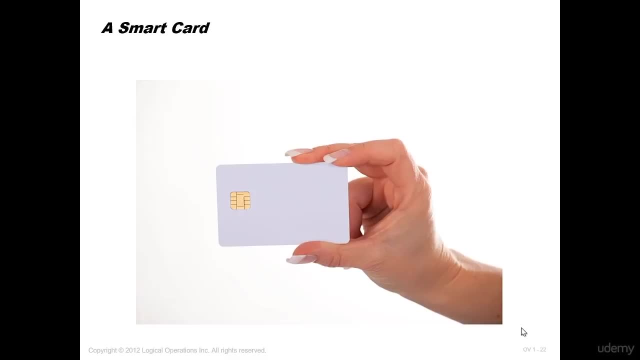 during the revision of the access control. after finishing, this domain, where we'll be explaining the attack related to the smart card attack, is very important for the exam. you'll get a lot of question asking you about attacks, so you have to write down whatever attack we are talking about. you have to write it down. 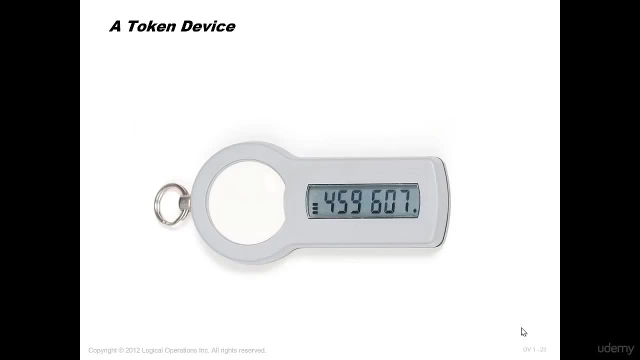 now, another type of something you have will be the talking device. and talking device- and a lot of people are aware of that- it's just a device that generate one-time password. it's considered very effective, actually. so whenever you are you are trying to syndicate, you push on one bottom, it will generate one time one. 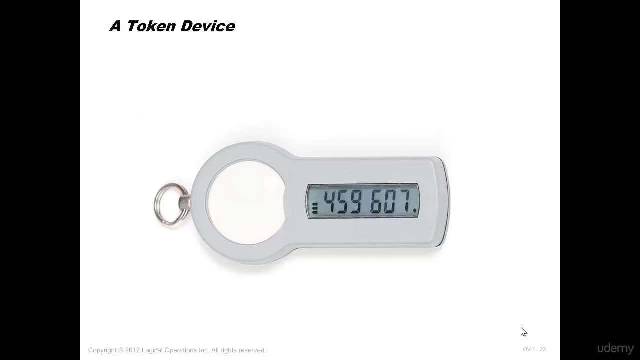 time password valid for like one hour and you have to use this pass. this is a very important important thing for authentication in talking device. we have two different type. we have synchronous and asynchronous talking device. the set when we are looking here. it's called synchronous and this 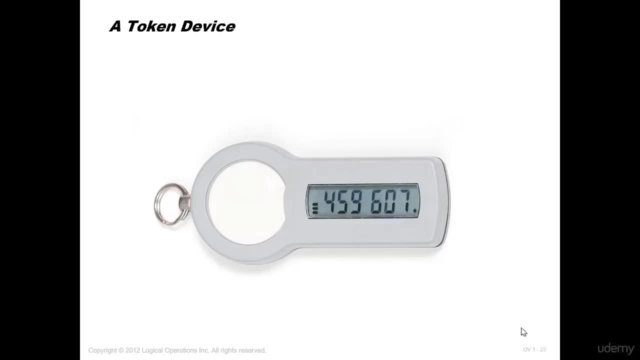 synchronous device depend on timing. I mean definitely. on the other side, I mean if this is a banking talking device that you are using to log into your bank account That generate a password on the same method or algorithm that match, I mean how they'll be knowing that this is the right password. Now, the password that this device, the synchronous device, is generating, depend on time. 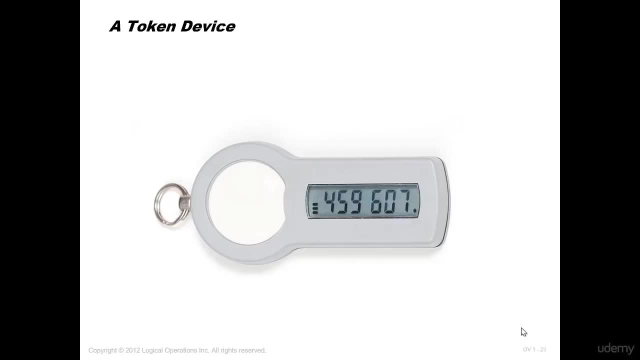 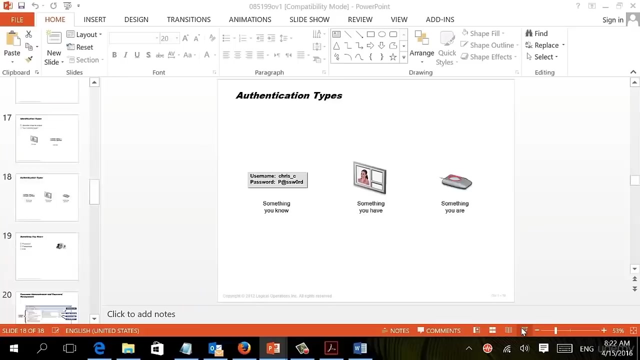 So the factor here it depends about when are you generating that And on the other hand, or on the other place, the bank or the organization. they have a server that has a formula, also depending on time, And when you click on it and you generate a password, it will be compared on the other side, based also on time. Let me show you the asynchronous that has like a pad on it. 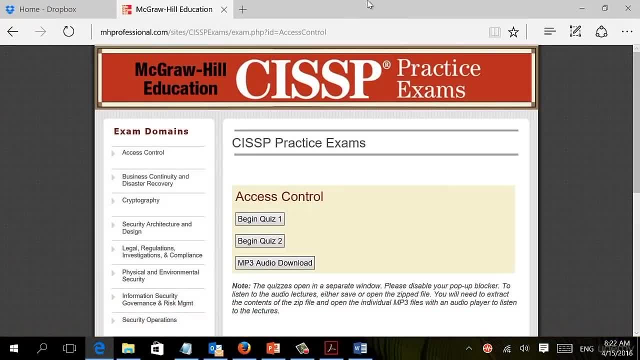 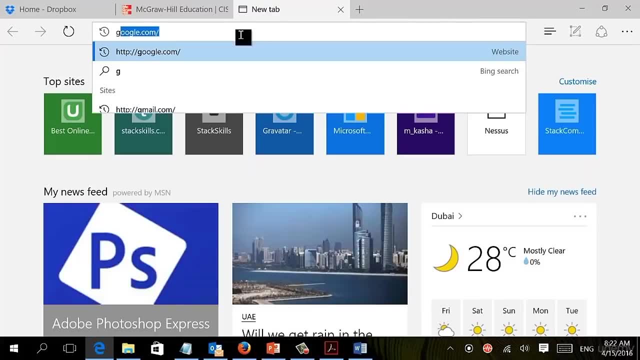 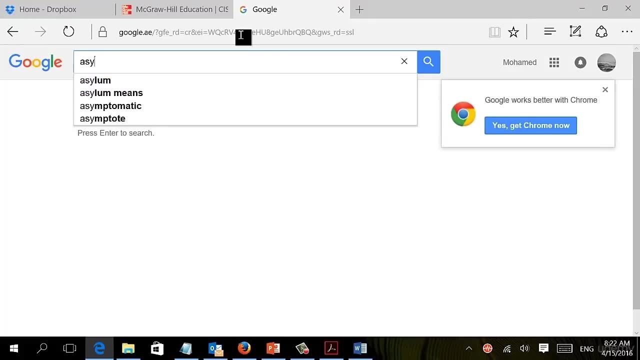 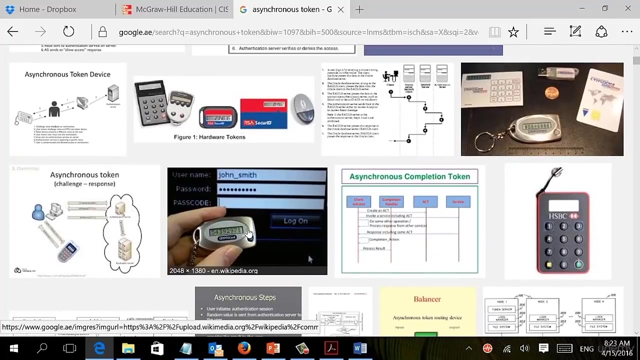 So asynchronous. let me Show it to you. Asynchronous token the asynchronous. it's similar to synchronous. Now, the synchronous device It just Synchronous talking device. It's like this one. It has a push button where you are clicking. click on it. 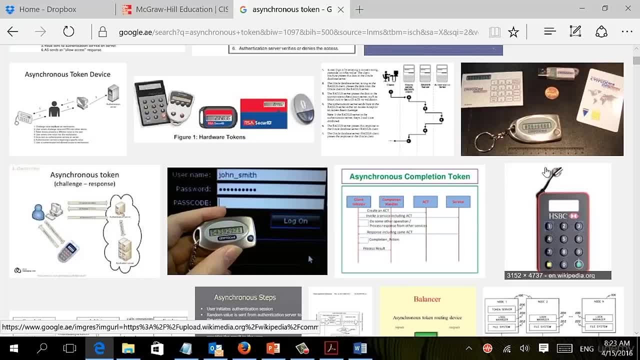 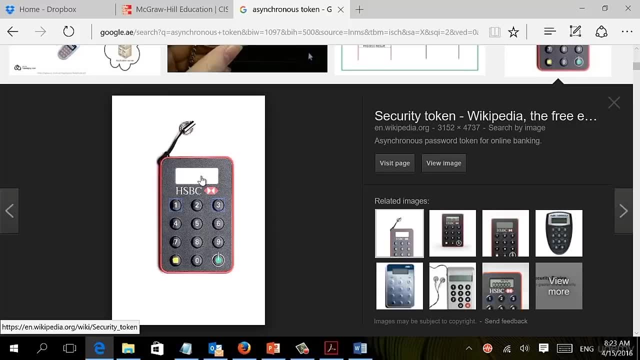 It will generate a password. So asynchronous, it's like this one: OK, it has a pad on it, You have to type a pen number and it will generate a password according to that. So the thing is the synchronous one. if you lost it and someone was able to find it and he know his account, he can generate the password. 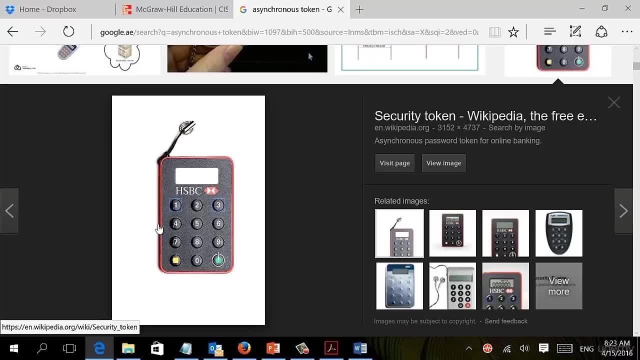 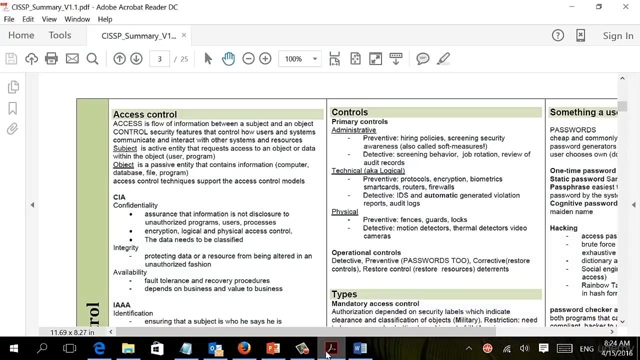 But if you have asynchronous, Asynchronous you know, even if you lost it and someone get it to be able to generate the password, you have to know a pen number. So we have a synchronous talking device and asynchronous talking device and you should know that the synchronous depend on timing. 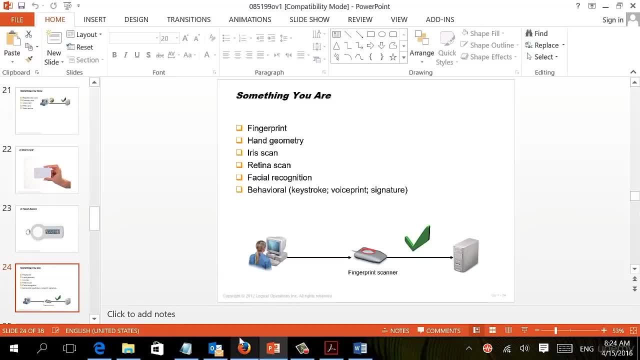 The third model that will be explaining is something you are- and I want you to give some attention here because I can guarantee that you may find the question About site insights, Ex. And Specially you have something you are, we are considering something you are the most. 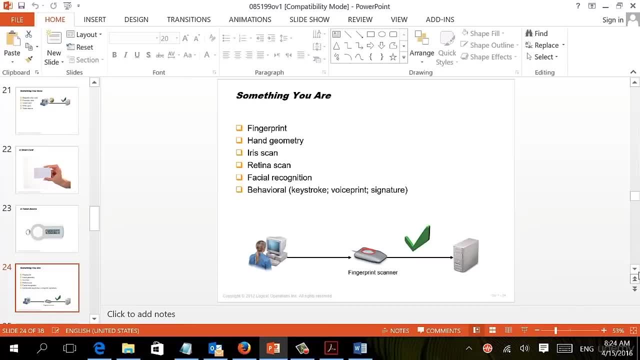 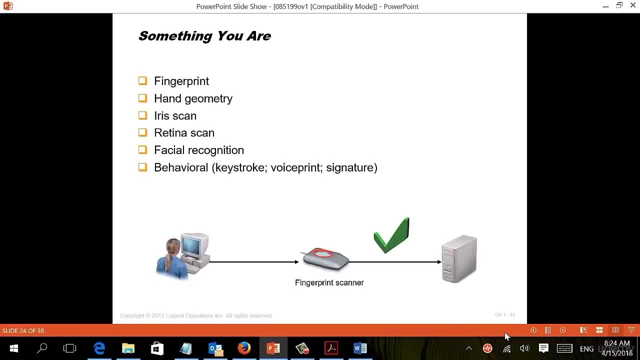 expensive but the most secure way for authentication something you are could be any biometric device: a fingerprint reader, a hand geometry, an iris scan, a face recognition, a voice recognition. also, we have some kind of devices that we consider behavior-based. I mean, in something you have, something you are which is a biometric device, it's 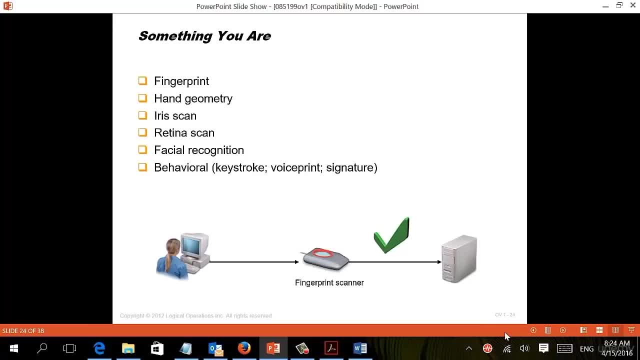 considered two different type. we have a physiology based and a behavior based. physiology based: it's like the fingerprint. something depend on your physiology, on your, you know, biometric, your eye, eye scan or voice recognition. behavior base: it's something like, for instant, the signature bed. you know some devices. you 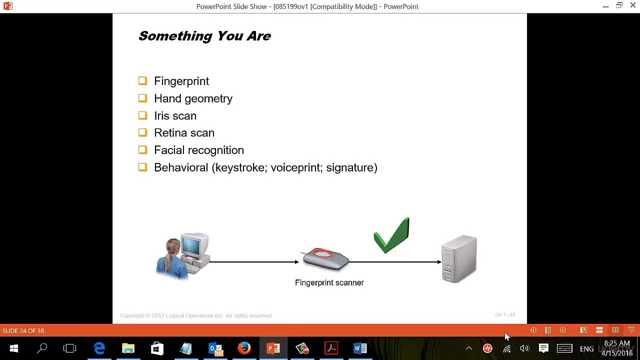 can write your signature on it and it will compare that to your real signature. this is called behavior based, or some keyboard that will check how the pressure when you are using the keyboard. this is called behavior based. this is considered, as I mentioned, very expensive, but also very secure and to be. 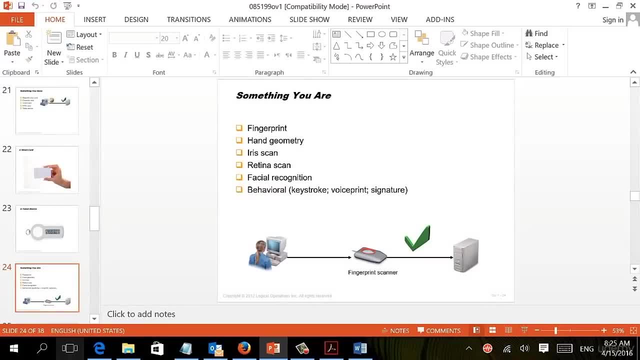 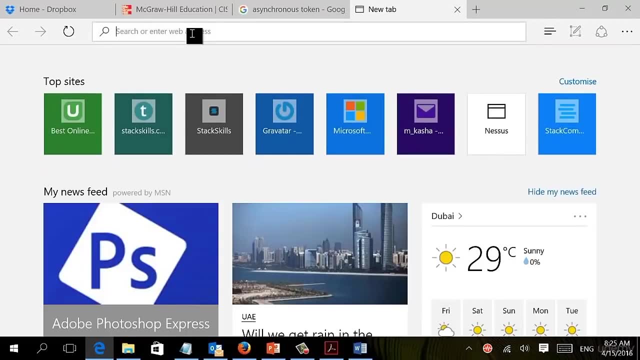 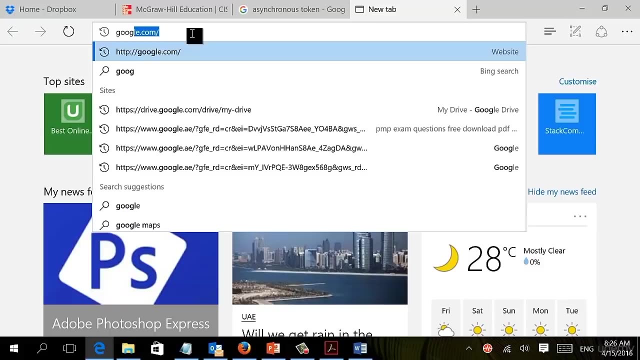 able to understand their characteristic. in general, ice rose strongly recommend this website. there is a website that show you how can you compare between different biometric device and what is the characteristic of each one. if you are going to buy any biometric device, how can you choose? so if we go to Google, and the site name is 3363 biometric device. Don't forget to subscribe. hit the bell regarding all the the video contents and we are working together visibleонь. the site data is in: 3 million examples of video that you are great viewers, I know from user materials in five special information wand and then video aerial coverage videos within a very good 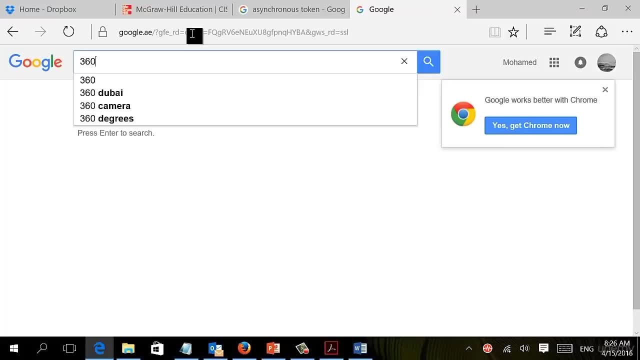 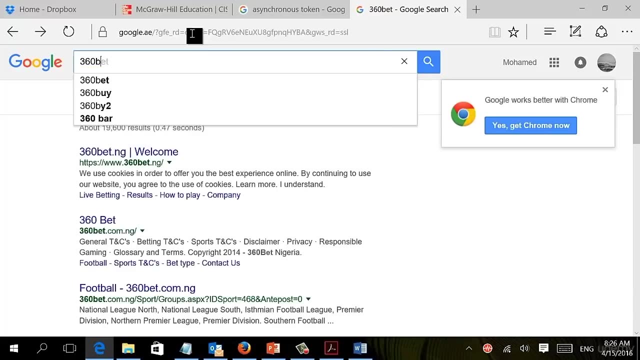 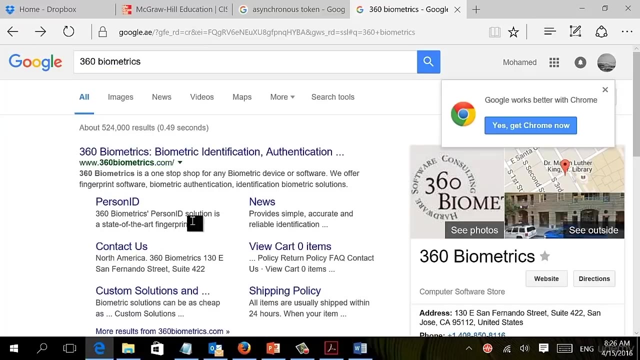 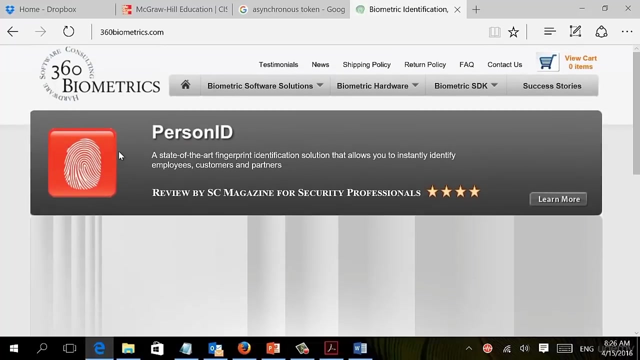 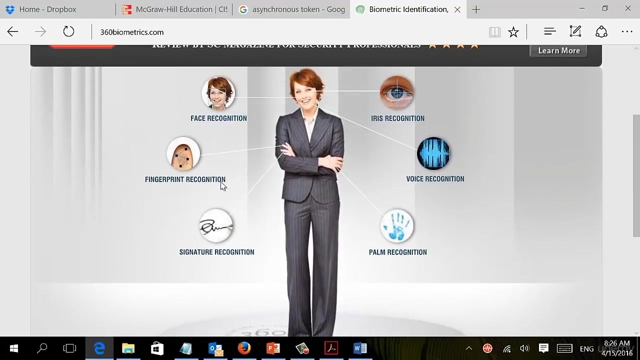 video, то что это 360 biometric 360, but you sorry, you metric, so 360 biometrics. excellent website from where you can go and you check the different kind of biometric device: the behavior based, physiology based, how can we compare between them, the different functionality in each one of them, and so on. so it's a very good. 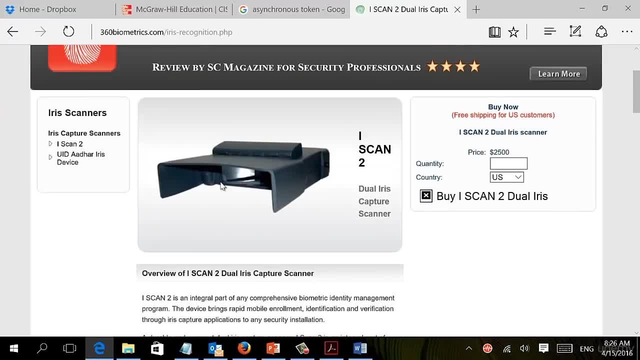 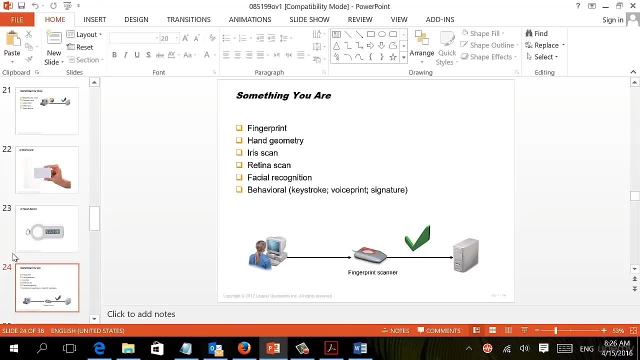 resources to understand more about those biometric device and how they are working and how can you evaluate between them. it's a very, very nice website. getting back to our presentation now, this actually is the most important slide in the something you are going to see in the next video. 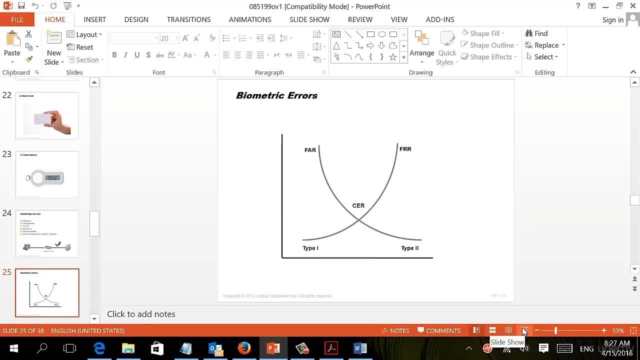 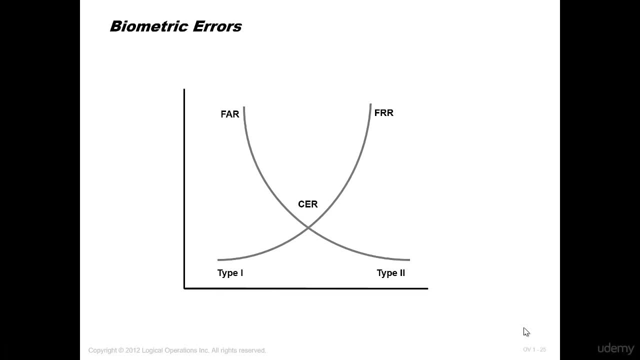 are and, as I told you, most probably you will find the question about set inside the exam. now we explain so far as a different problem in different kind of different problem in different kind of devices. I mean in something you have, you you know the password. the password can be break easily we'll be talking about 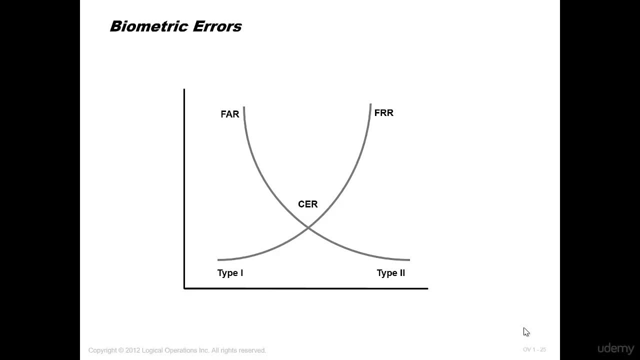 the attack after a few minutes. there is a lot of problem when it come to password. it can be break, it can be sniffer, it can be social engineering. I mean you can get the password very easily. something you have could be lost. it's not that it's very. it's better than the password, but also has its own. 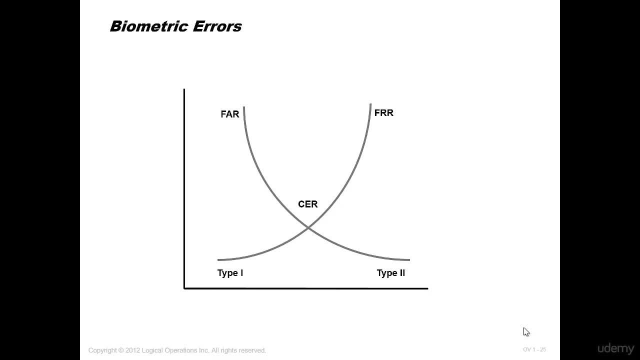 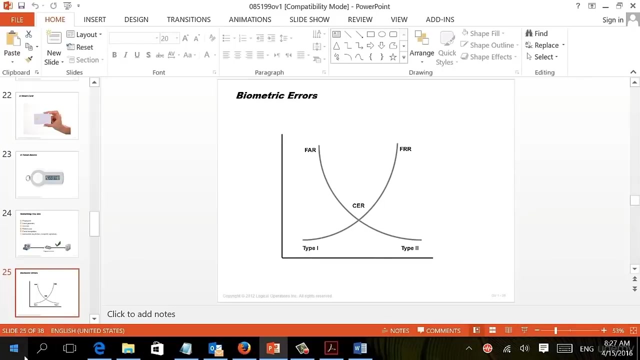 problem. what is the problem is biometric problem is a biometric, it's to adjust the sensitivity and this is actually is extremely important graph. let me explain to you when we are talking about a fingerprint scanning, let me get back here, to this website and let's talk about the fingerprint scanning. getting back here, 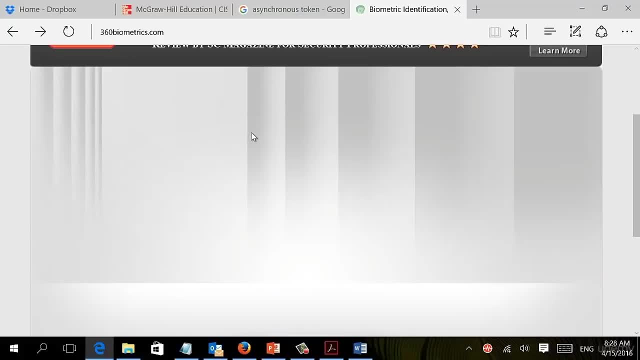 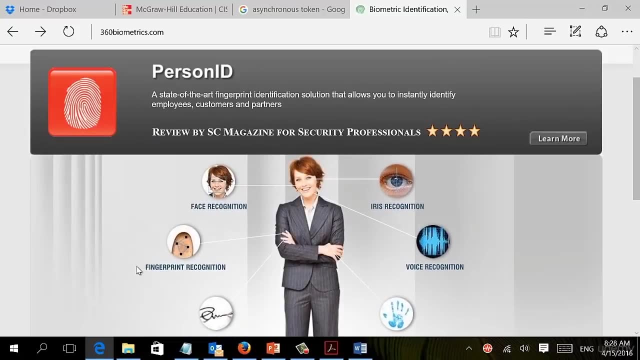 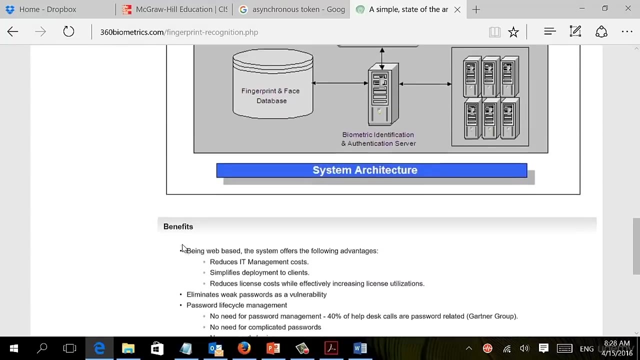 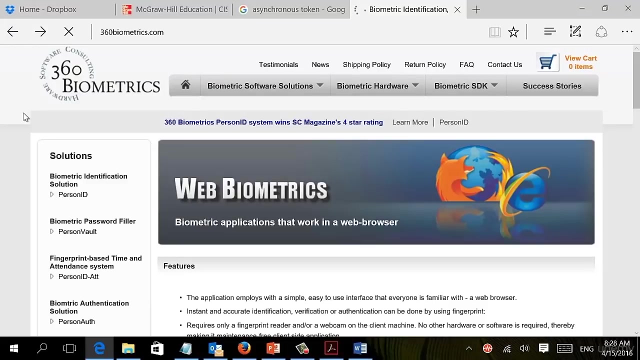 okay to fingerprint scanning: how the fingerprint is scanner are working okay, so let's take the fingerprint. as you can see when you have a fingerprint scanning how it work is that? and it's not here giving back when you. he's reading your fingerprint. he's not taking a picture of your fingerprint and later on he will compare. 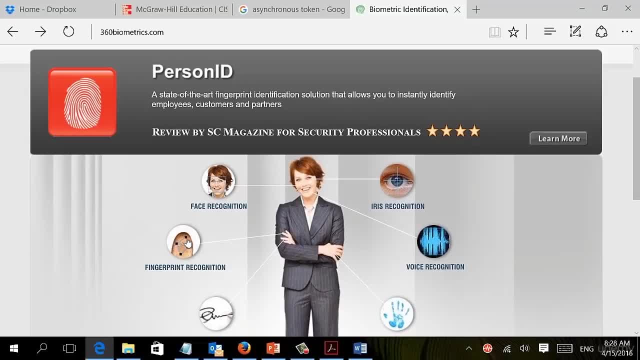 this picture with another picture. he's taking some point from your fingerprint, from your finger, and measure the distance between them and transfer them to value. then, whenever you try to authenticate and you put and you put your fingerprint, he will do the same and compare the picture with your fingerprint. 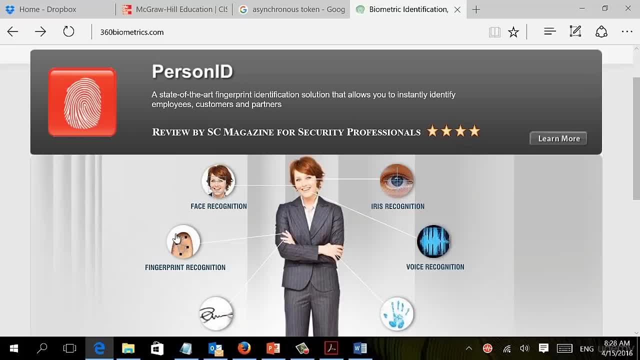 this value to that value. but maybe your finger is a little bit sweaty, maybe it's little bit in an angle, it's not on the same way they are putting, so you will not have the exact same value. now, what is the amount of error accepted? i mean, 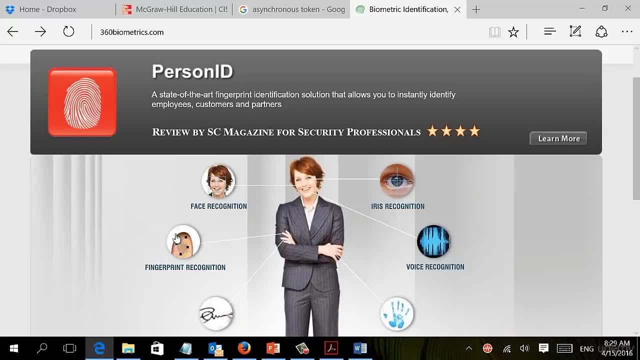 you know what is the error value that you can accept? maybe the value that has been taking while you are calibrating it was 100.. that means if i put my fingerprint one more time and the output was 80. should he accept that? should he accept 20 as an error? 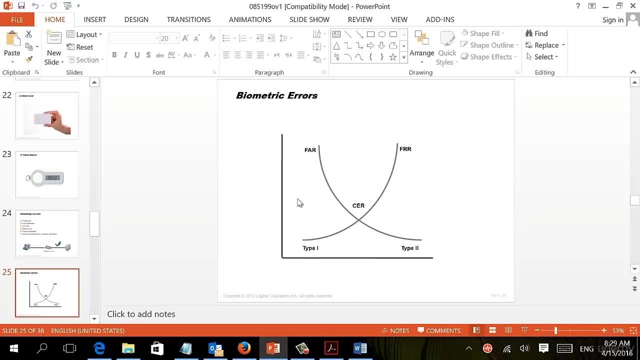 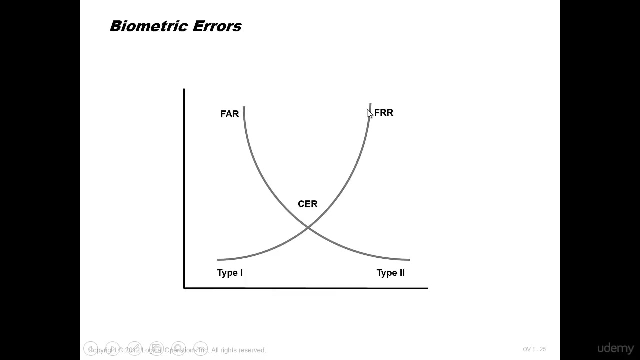 less or more. that's why, getting back to my graph here, the one down here, this x, this is considered the sensitivity and the one here, this is considered the failure attempt. okay, so let's explain that if you start increasing the sensitivity, like we are doing here, okay, meaning that he had to get the exact 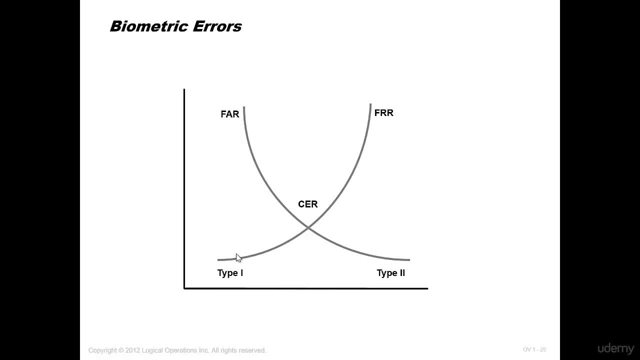 same value of my fingerprint. so if my fingerprint was a little bit sweaty, if my fingerprint was not put in this the exact same way i used it the first time. he will not accept that so but so by increasing the sensitivity i'm increasing the number of failure. so now, every time i try to syndicate, he 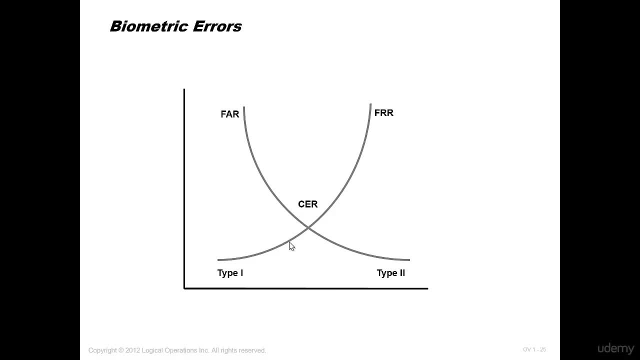 do not accept. i have to try one and two and three time until he's accepting because he has a very high sensitivity. so the high sensitivity will cause something called the frr false rejection error, which is: i have been rejected but i should not be rejected. this is called the false rejection. 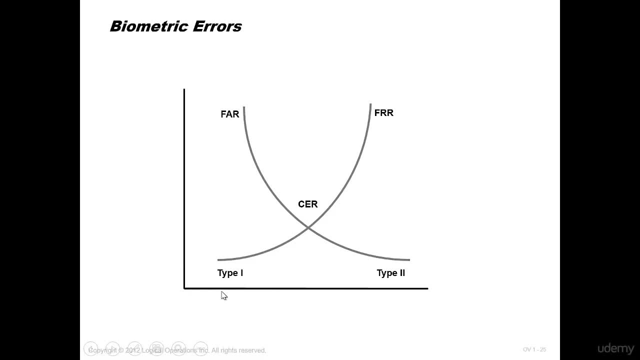 error or another name for it. it's type one error. if i do the opposite one, i decrease the sensitivity. what will happen is i have a big error rate. so whoever try to authenticate, he will authenticate. so by decreasing the failure, the number of failure will be less. 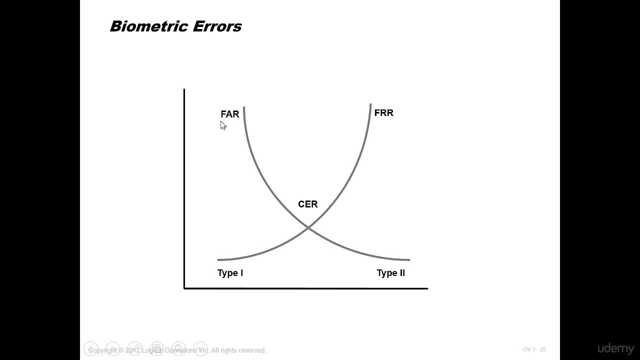 and this will cause another kind of error which is more dangerous. it's called the fr or false acceptance rate, meaning i should not be accepted, but i have been accepted. so it's more dangerous. and this is has a different name, it's type two, the intersection of those two curves. 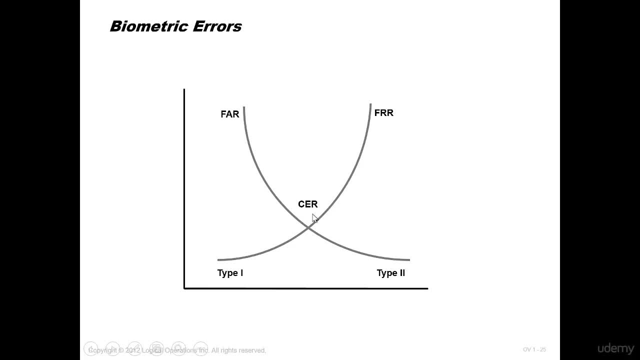 will introduce another terminology called cer- crossover error rate- and this is how we are evaluating the biometric device. i mean, if you have two different cer, i will look for the lower cr. this means it's more effective. so please give a big attention to this graph and understand what is type 1 error. 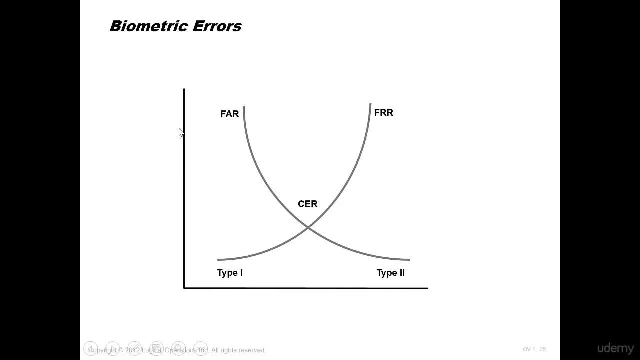 the false rejection rate, and what is type 2 error, the false acceptance rate, and which one is more dangerous than one? you may find the question asking you: what is type 1 error? is it far? if it is, it ser, is it frr and whatever name it? 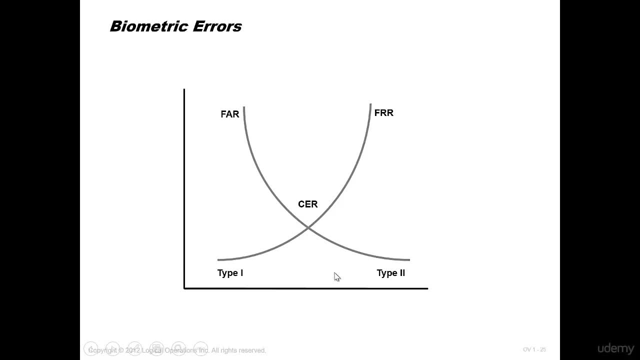 is so very, very important to understand this biometric. do not lose this question, please. what do we consider when it comes to authentication? i mean, should we consider using something you have, something you are? we should consider a multi-authentication factor and more than one authentication factor. 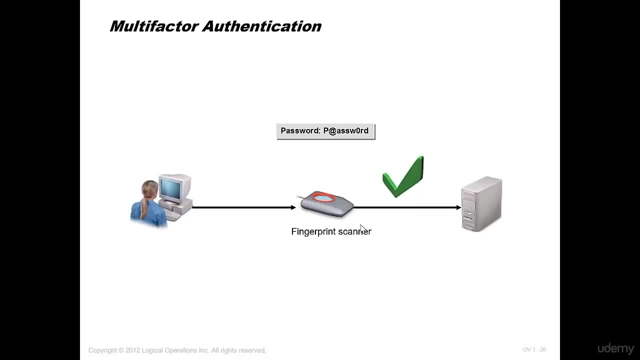 so if i'm using a fingerprint and a face recognition, do you consider that multi-authentication factor? no, this is single authentication factor because you are using two from the same methods. so when i'm saying multi-authentication factor, i mean a password and a fingerprint scan- one. 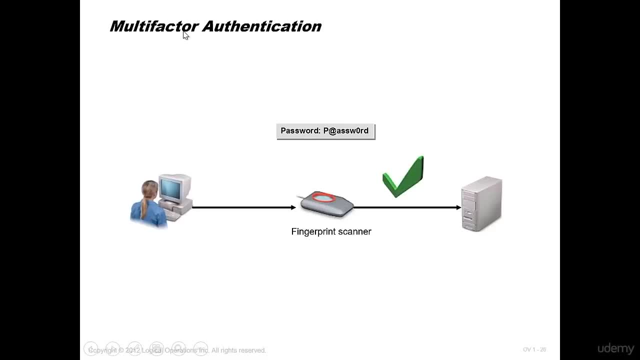 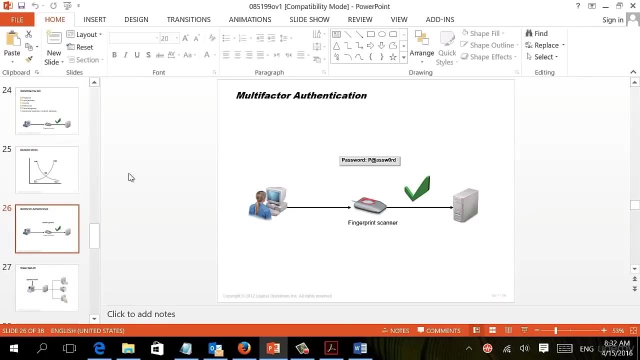 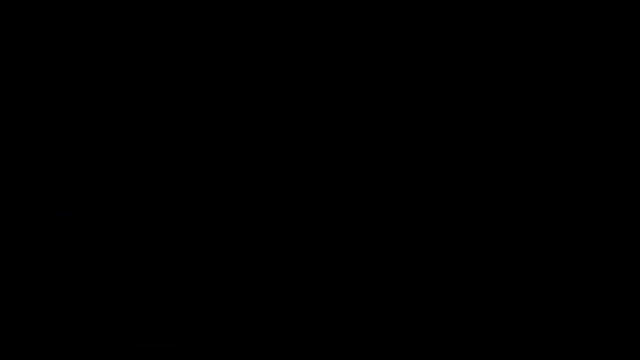 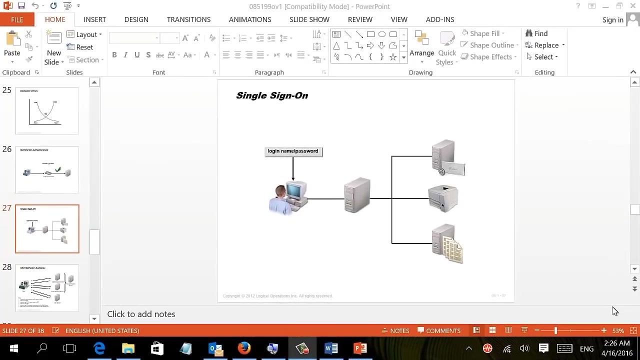 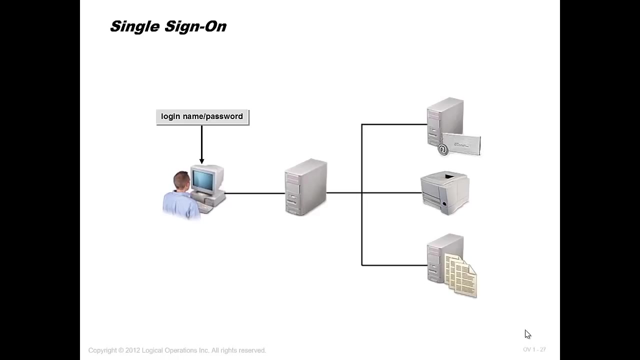 from each model. this is the recommended authentication models to be used: the multi-authentication factor. in this lecture, i will be talking about the single sign-on now. single sign-on, it's a very important topic in access control and later on during this domain. i want to distinguish between: 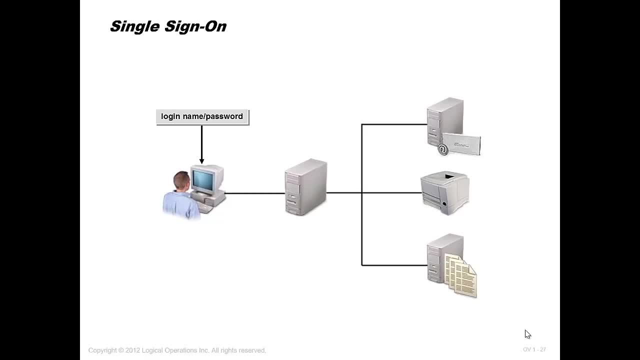 the single sign-on and the central access control. i want to distinguish between the single sign-on and the central access control administration. let's talk about single sign-on first. what is single sign-on? here is a scenario. assume that inside your network you have more than one server. 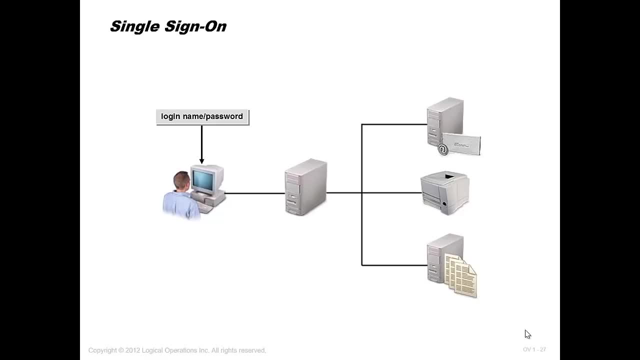 you have a sql server, you have an oracle server, you have a sharepoint server, you have a file server, you have a printer. now for each user you're going to need to assign different permission on different server. so user a going to need to have some permission on the sql server. maybe he have. 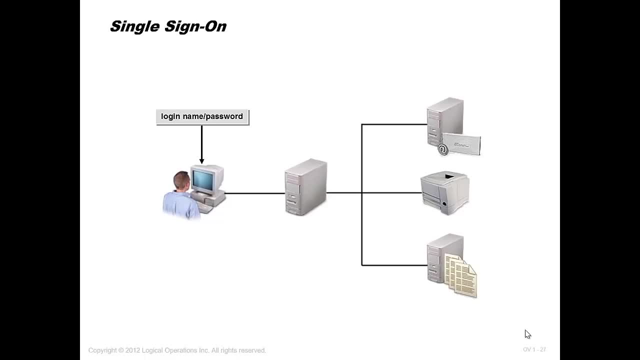 lower permission on oracle server, maybe have a higher permission on sharepoint and so on. so for each user he's going to need to memorize different account on different services and this is not very effective way for access control but, in opposite, in a better way for doing that. 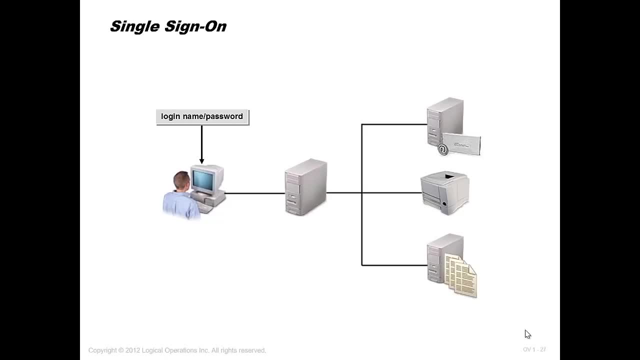 what if each user has one account only and once he logged in he can have access to all the server behind this network, so he don't have to log into the domain first, then log into the sharepoint and then log into the? no, he have one account. 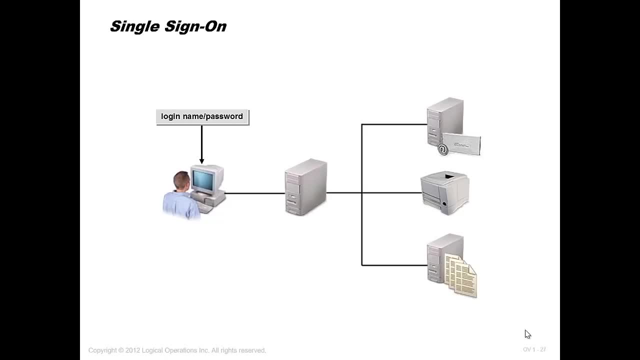 where i can assign the proper permission on the same account to different services seem very effective. but what is the side effect of that? if someone was able to compromise his account, he will be able to access all his resources, while if we have separate account on the sql server, he will not be able to access all his. 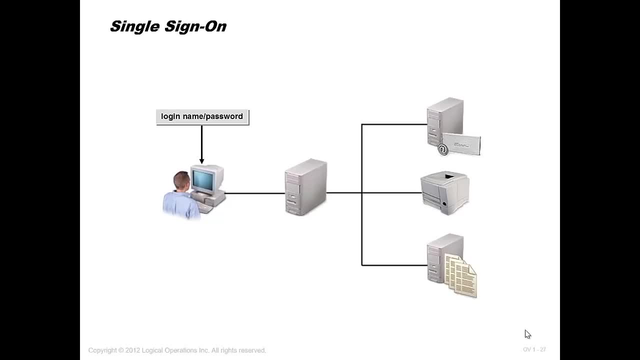 other resources. so single siren has its own advantage, but also this advantage and we already are using that. i don't know if you are you notice that or not, but when you log into microsoft windows domain, you notice that you can have access to all your resources resources one time. so using the same account, you can access. 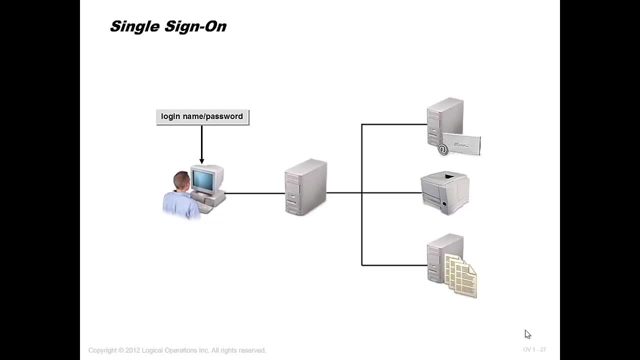 your file server, you can access your share folder, you can access, use the same account, you don't need to have similar account- and we're going to talk about one specific protocol that is implemented- and actually this is implemented in windows and in linux- is called kerberos. it's a single sign-on protocol. 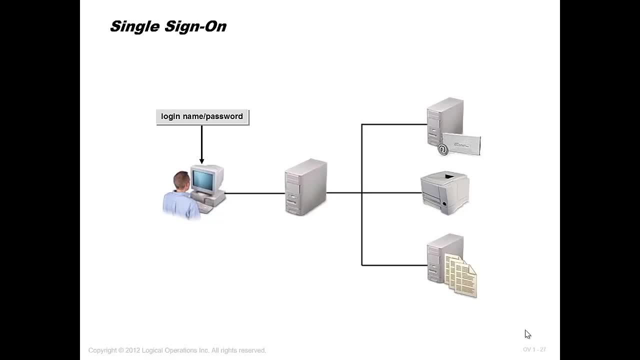 that can be used to allow people to log in just one time and access all the resources. so one more time. single sign-on allow user to log in one time and all the resources. permission will be assigned to one account and we call that the key to the kingdom. 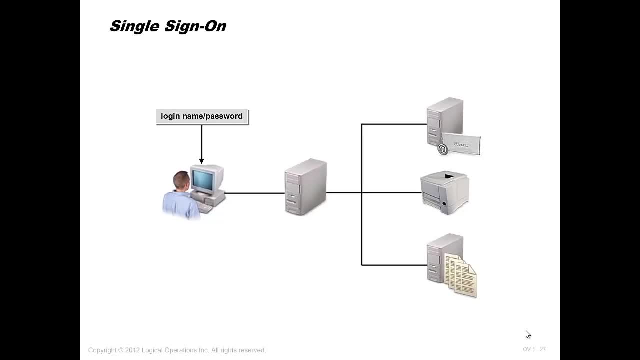 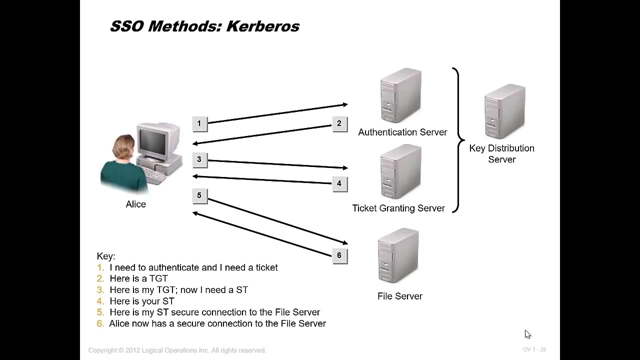 because if it, if the user lost it or someone else compromised it, he will be able to access all the account. now, what exactly do you need to learn for the exam? when it comes to single sign-on, you need to learn how it works, okay. so this is a very important slide and you need to understand the 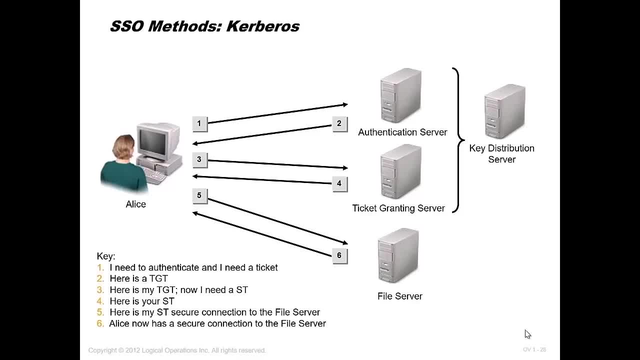 how the kerberos protocol single sign-on protocol work. now, to be able to have a single sign-on protocol, you need to have something called as you can see on your right key distribution server. so to implement kerberos you need to have kds or key distribution service. 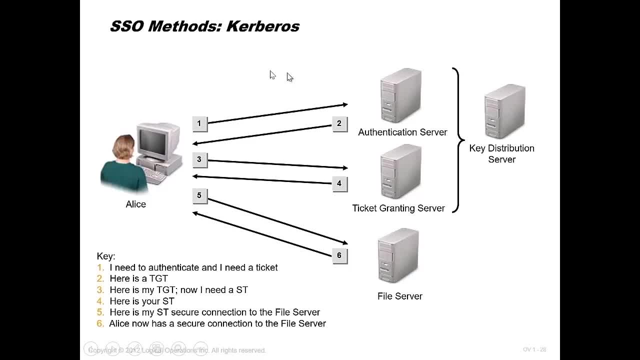 inside the server. you have two different server. you have an authentication server and you have a ticket granted server, and we're going to explain that. but it could be. one server has the two functions. it could be two separate functions, but after all, what do we call that? 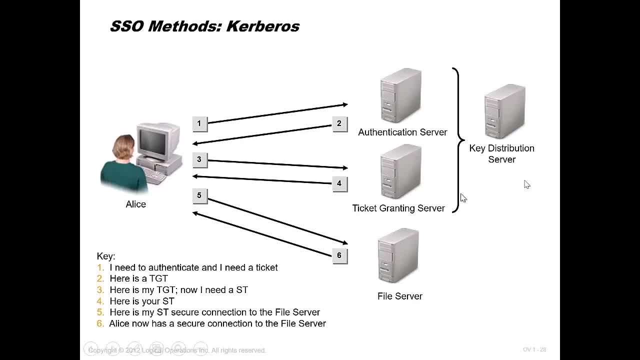 the key distribution server. so here is the scenario: we have one user and we have a network and the. this network has a file server and a print server and shortest servers have many server that we have and we need to implement the single sign-on saser there. login. 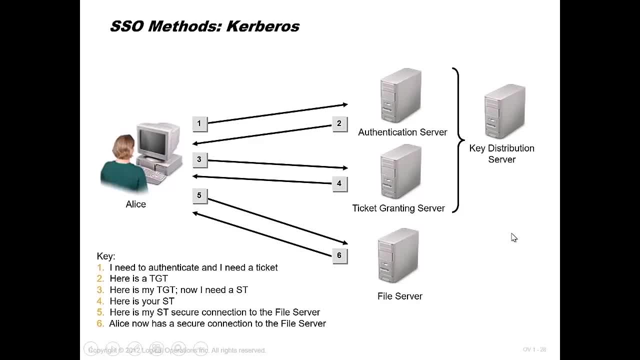 and automatically he will be able to access his account on the file server and shared point and so on. you don't need to memorize more than one account how it work. so here is how kerberos work. this is my user, alice. she's sitting and she's writing the. 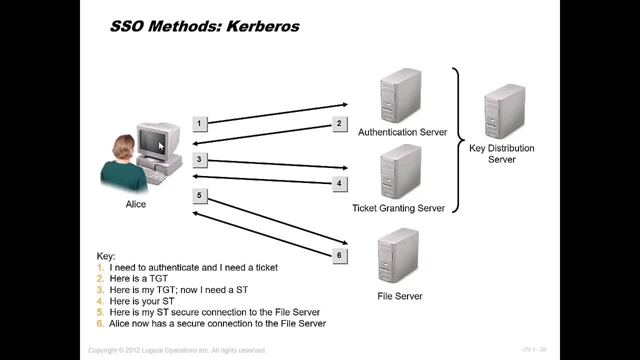 user name and password. where are the user name and password saved? are saved on the tracking eight. and how can you generate a password? where are the user name and password saved? are saved on the flow chart authentication server. so the first rule of the kds is working as an authentication server. 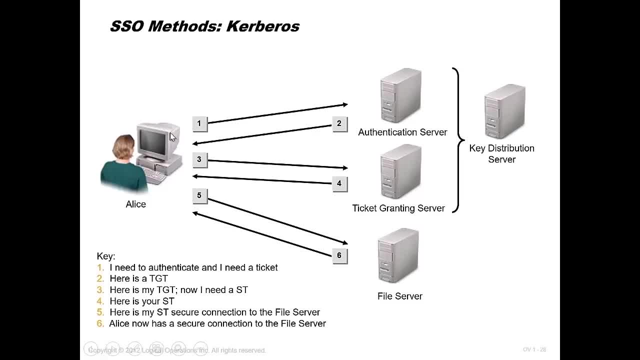 so she's writing the username and password and you click on enter. so the username and password will be sent to the authentication server to validate them. now here is the tricky part here, when alice are sending her username and password, only the username will be sent. password will not. 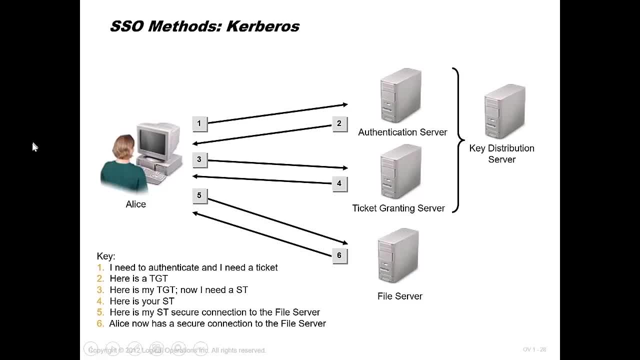 be sent to the authentication server, and this is to prevent sending the password over the wire. so if someone is sniffing or doing a man in the middle attack, you will get the password. so what happened is the way kerberos work: that alice will send his her username. she will type the username. 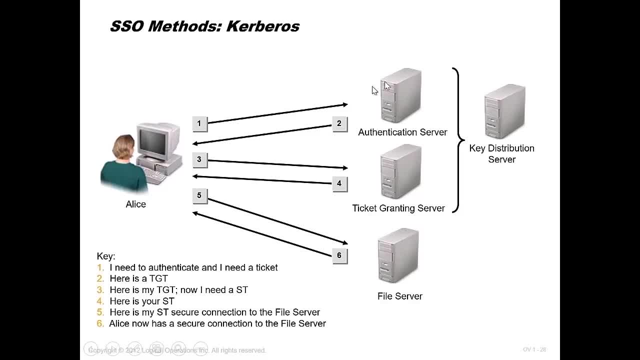 and password. the username will be sent to the authentication server, but the password will be kept on her computer inside the cache. so once the authentication server receive the username, he will only receive the username. he will not receive the password saying i am alice and i want to login. he said: okay, alice, you have your password and i also. 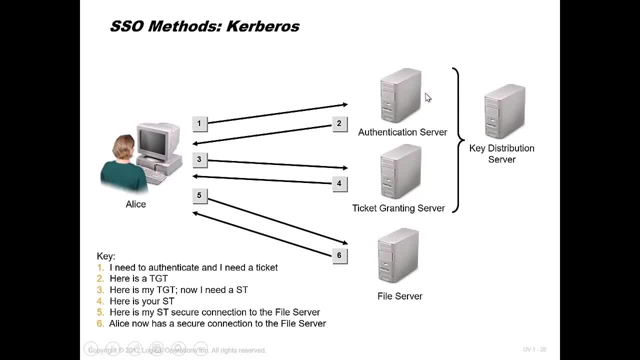 have your password saved, i'm going to send you a text that is encrypted with your password, and if you are able to decrypt using your password, that means you are alice. one more time, alice will send the username authentication server or will use the password as an encryption key. it will not be used for validation. 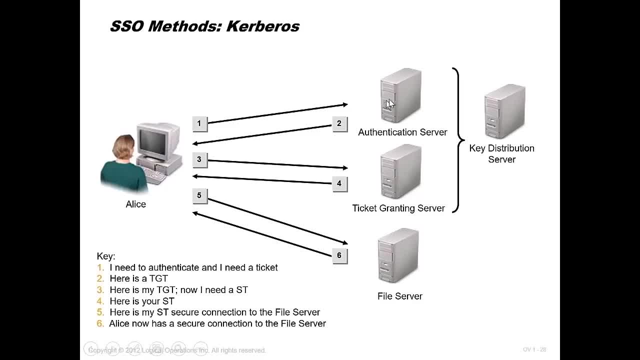 he will said: you are saying urls. fine, i'm going to send you a text and i'm going to encrypt this text using your password. and since you have your password cached inside your computer, if the password has been decrypted with your key, mean with your password, means this is the right password. so both of 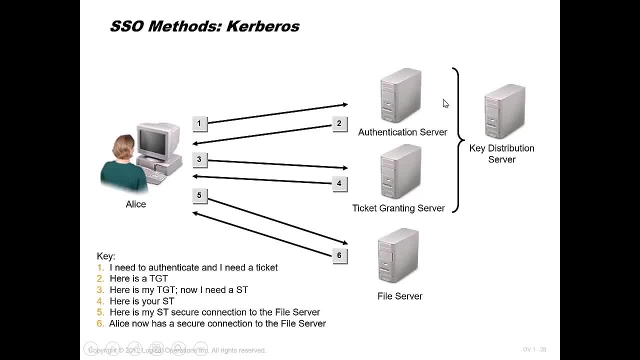 them will be using the password as an encryption and decryption key, and by doing that we are preventing for sending the password over the wire. so this is the very tricky part, or the first thing that you need to be about. you need to know about kerberos. they are 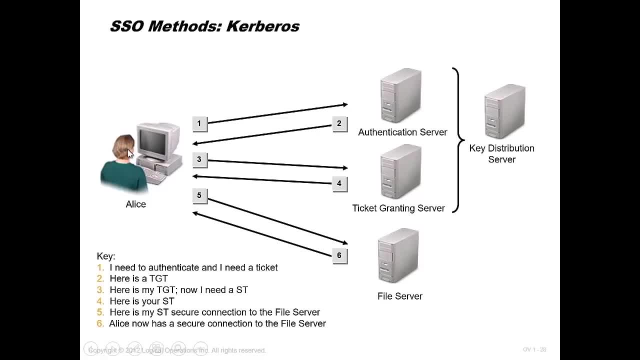 not sending the password over the wire actually, as alice will do nothing. everything will be done behind the scene. but this is how it works. only the username will be sent and the server will send a challenge for alice or a, a text that has been encrypted with alice password and he's waiting. if 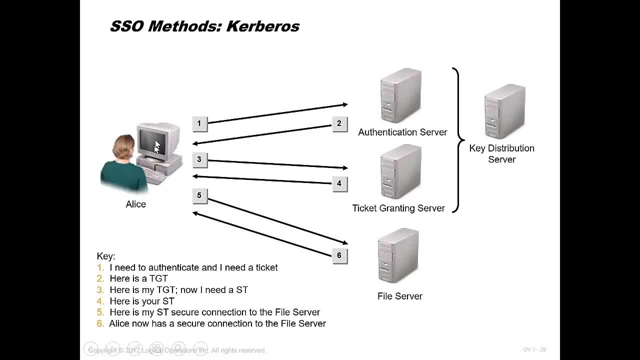 she is really alice, her password will be able to decrypt the text. this is the first step. now, once the authentication server confirms that this is alice, automatically the tgs or the ticket granted server will send to the asset. to to alice a tgt ticket. granted ticket. it will send to asset. 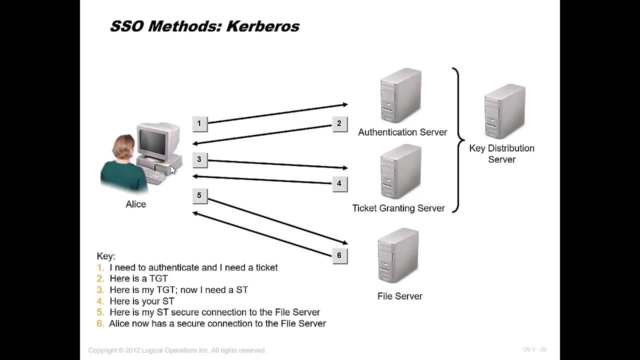 will send to alice a ticket. ticket granted, it's just a piece of code that we consider like an id, so the tgt will issue an id for alice. so next time alice need to authenticate, you don't need to send the username and receive this challenge and encrypted, you just need to show her id to the server. 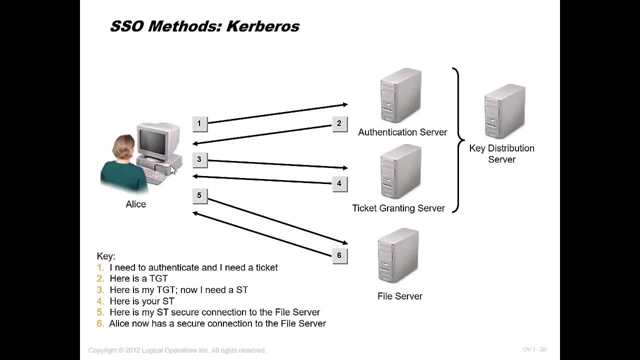 so, to make things more simple, the tgt will issue to alice a ticket which is considered like an id, and it will be issued based on the authentication server approval. okay, so now alice hold a tgt now. the tgt it's a piece of code, but it's kept inside. 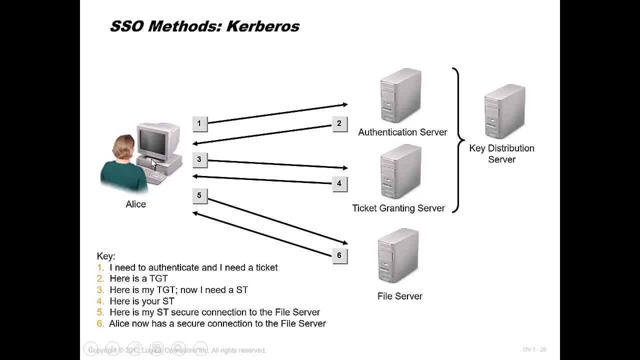 memory. it's not saved on her hard drive. i mean, if alice shut down her computer, she need to repeat this process one more time, sending the username and receiving this encrypted text and decrypt that with her password, and but whenever she's on this ticket it's inside the memory. it's not kept on site. the tgt is. 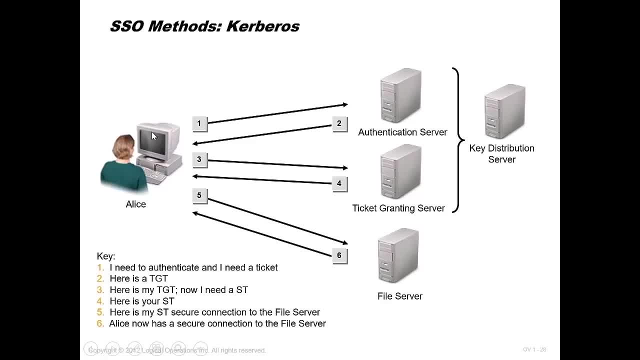 kept. it's kept inside her memory. then alice gonna say: okay, i have been authenticated and i received the ticket. now could you please allow me to access to the file server? and she's gonna show her ticket to the server and ask him to let him access to the file server. according to that, she will be having another ticket, so 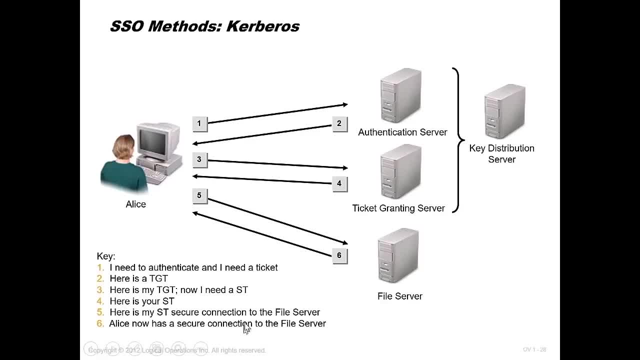 the server will issue for asset for alice another ticket called the session ticket st, and alice can only be access the file server using those two tickets: the tgt that has been received at the beginning and the st that has been, i'm sorry, the tgt that has been issued at the beginning. 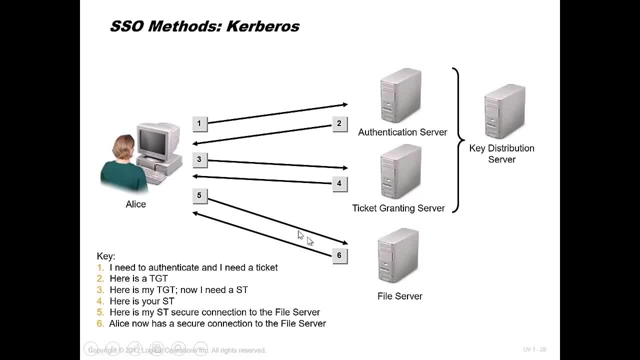 and the st that has been issued. once alice requested to access the file server and unless alice have those two tickets, she able to access file server. what about if there is another server- oracle server- she need to do the same. she gonna talk to the kds telling him i need to access the oracle server. he said: fine, show me your. 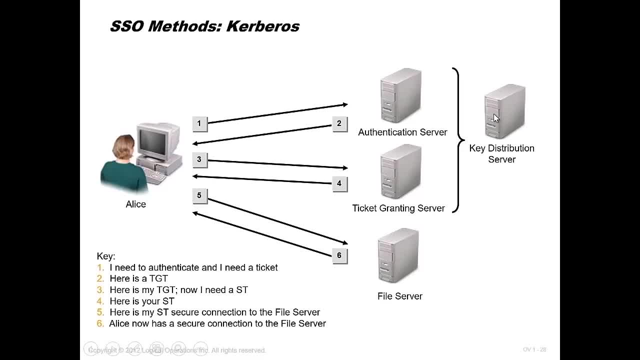 tgt. alice will show the tgt and the kds will issue another st that is valid for the oracle server. now alice to be able to access the oracle server, she needs the tgt and the st for this oracle server. so for alice to access any resources, how many tickets she needs. 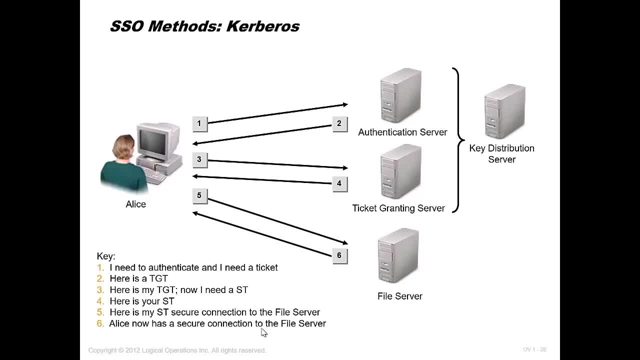 she needs two tickets. one of them has been issued at the beginning and it will be common in any connection to any devices. second one st. it's related to whatever service she's trying to connect, so she will be having an st for file servers that will be different than st for oracle server. 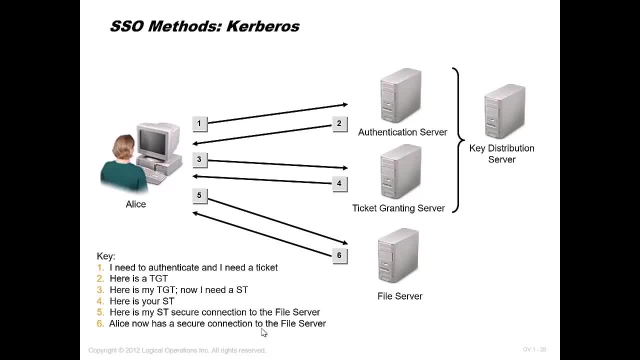 and will be different than st for sharepoint server or file server. so for each server she have one common ticket, tgt, and one very varying or variable ticket, which is st. this is how the sso- or, i'm sorry, how kerberos- as a single sign-on protocol is working. it's important to understand. 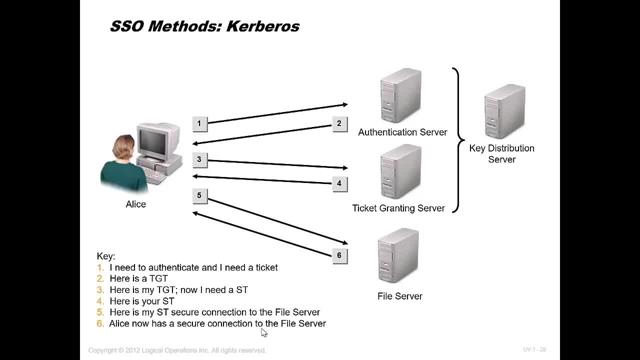 the steps. it's important to understand what is the kds. it act as a authentication server and ticket granted server. it's important to understand that in kerberos we are not sending the password over the wire and it's important to understand that alice to be able to access. 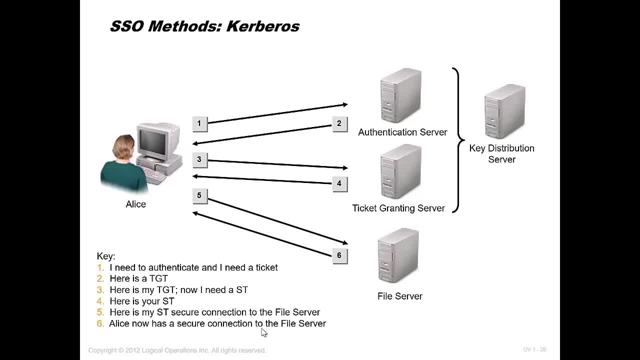 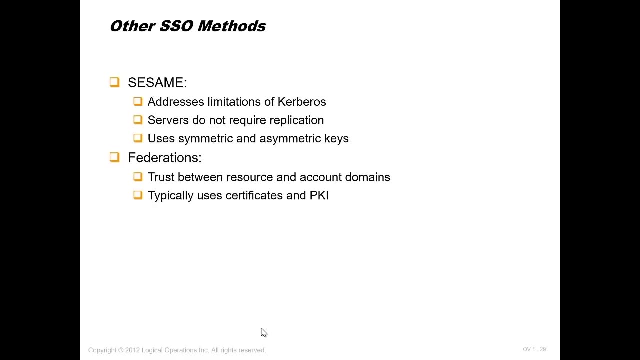 any device, i'm sorry, any resources behind the network. she need two different key: tgt- and this is it's not changing- and st. it depends from one service to another server. we have other ssl protocol. besides kerberos, we have sesame, we have federation. they are very from. you know like. 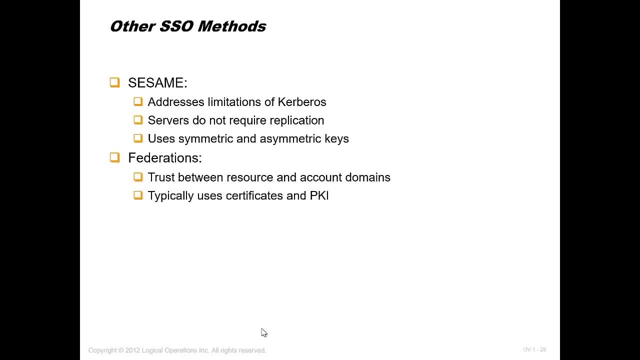 sesame. they are using asymmetric encryption, which is an asymmetric which is more powerful. but actually i want you to focus on federation. if you're going to ask you and say exam, it usually asks for the federation single sign-on. besides the kerberos, what is the federation single sign-on? 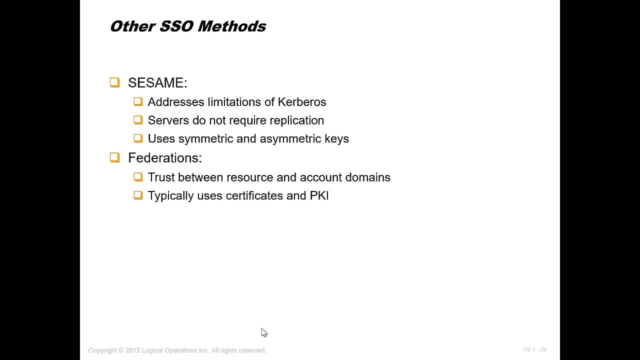 this is the single sign-on between website. i mean, if you saw inside the question website, he's asking about single sign-on related to website. it's a federation. what is federation or single single sign-on? it's when you- what can i say? when you authentic, assume that you are booking an airline ticket online. 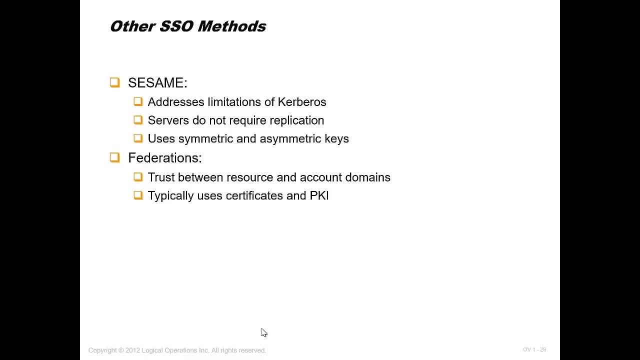 so you went to the page and you reserve your ticket and you made the payment. then he will ask you: would you like to reserve a hotel room or would you like to rent a car? and if you check, if you click on ok, he will redirect you to the uh renting car website, which could be a. 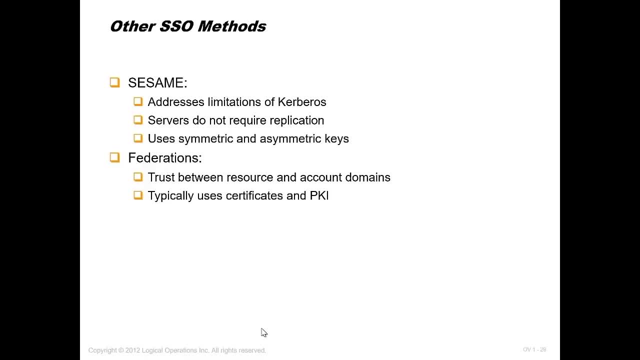 different website but you'll be logging with the same account and he will be using the same credit card information. so you did a single sign-on between different website. this is called federation. so federation is a single sign-on related to website. so if you got the question single sign-on and you find a key which is websites, it's a federation. 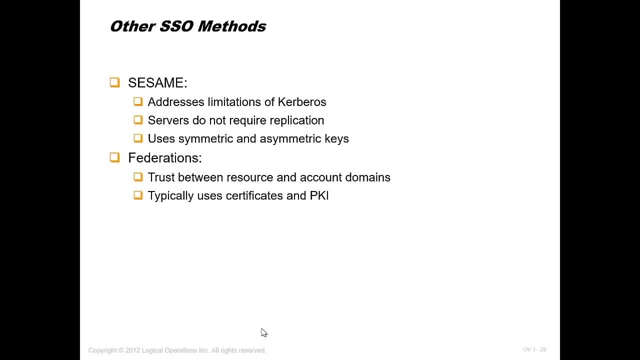 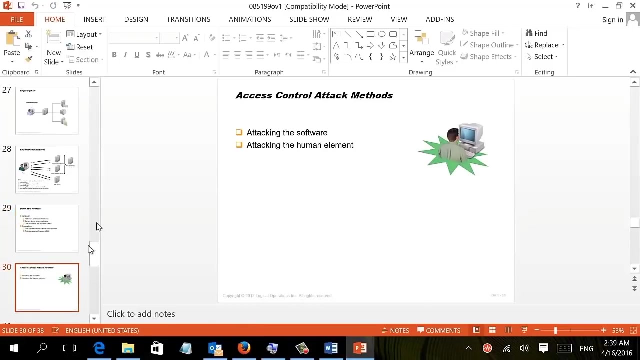 not kerberos be aware of those keywords, because usually this is what they are doing inside the exam. they will put a keyword that will change the option to choose. so the keyword for federation single sign-on is: uh, is a website. okay, now, before going through the attack, i just need to explain. 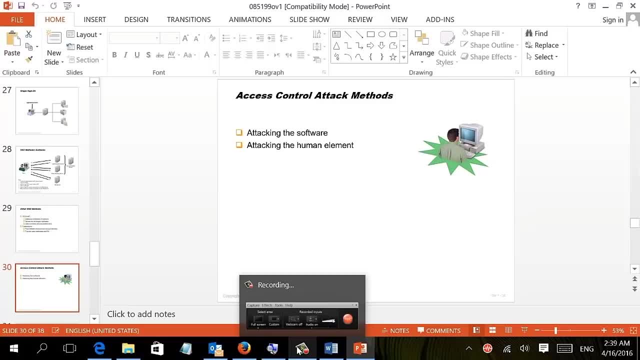 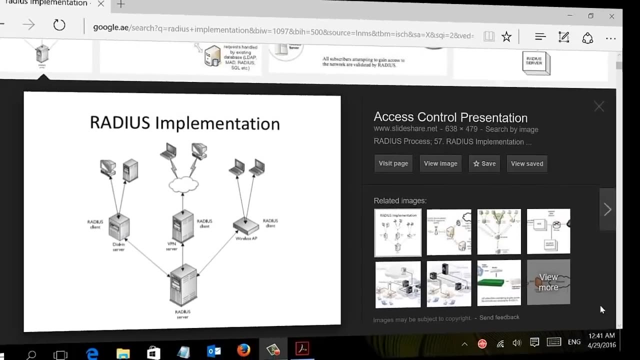 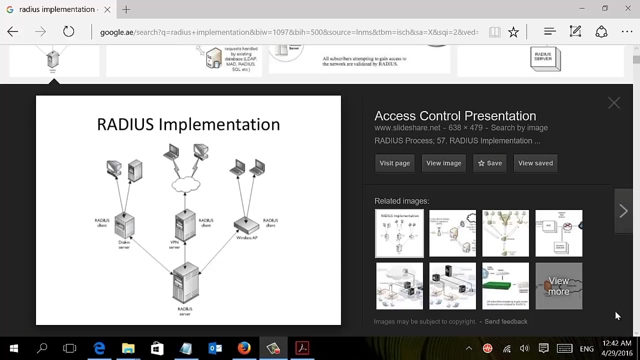 in the next lecture. what is the central administration and what is the difference between central administration and between the single sign-on? in this lecture, we will be talking about central administration, about a product called radius, and i want you to be able to distinguish between radius and between single sign-on. 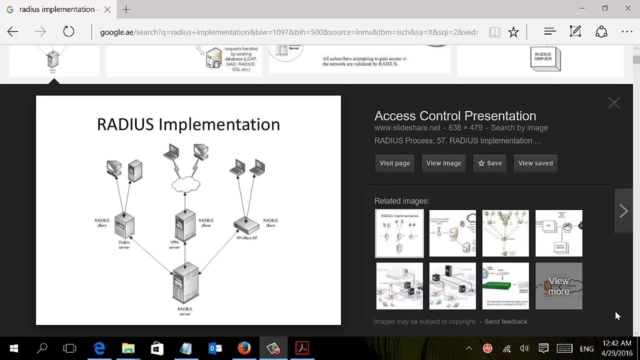 so single sign-on. it's a different story has been already explained. but what is radius exactly? now let me give you a small scenario. it will show you how it can be implemented. assume that you have a user that need different kind of login to the network, i mean if he's inside the 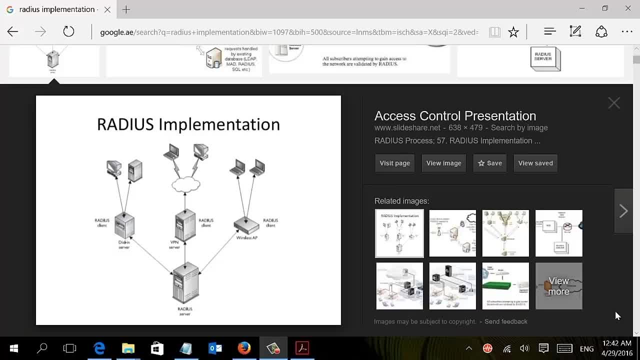 company- the company- he need to log in through the switch. if he's using his laptop or smartphone, he needs to log into the network using the wi-fi. if he's outside, he needs to connect to the company network using vpn and some places doesn't have internet. 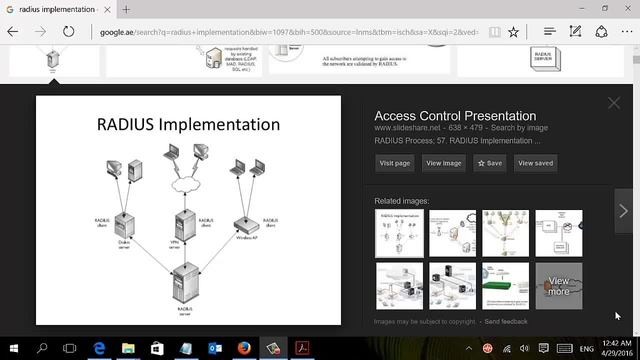 so he can need to log in using a dial-up. so for such user, how many account do you need? you need like four account, right and in a big organization for each user. you may need to give him four different account to be able to look into the network from the four different places. so you need to have a network on the vpn and another i'm 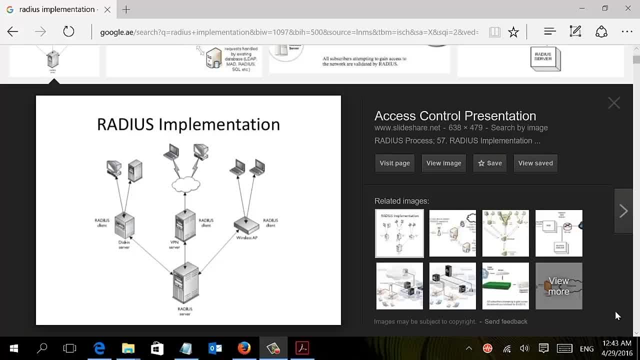 sorry, you need to have a password on the vpn server, you need to have a password on the remote access server, a password on the switch on wife, and so on. so to simplify this process, we can have the radius connected to the network, as you can see in the image in the screen, and this radius 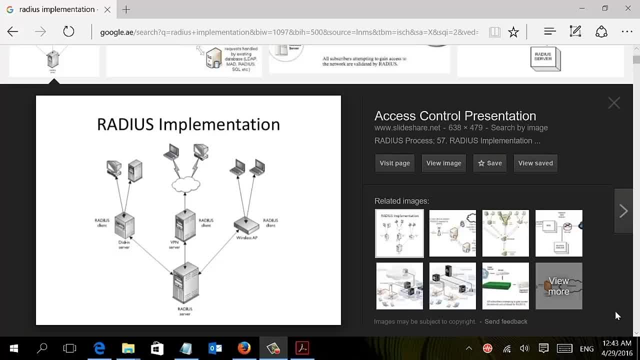 software will hold just one account. so he, radius, has a database that has all the username and password. now when one user try to login through a vpn, for instance, the vpn server will become a or will try to validate the account from the radius server. so vpn will not be keeping any. 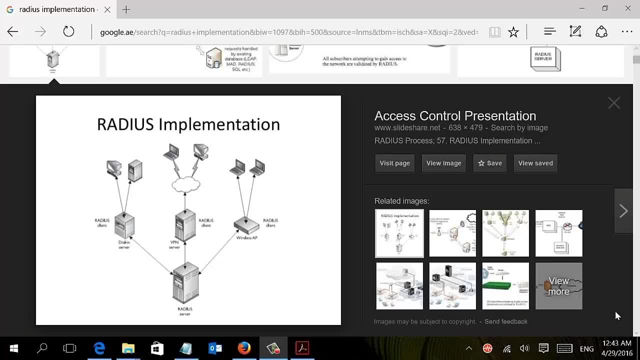 accounts. he will try to validate if this is a valid account from the radius server and according to that he will allow or deny. if the user try to login from the remote access server, the remote access server will try to validate the password from the radius server. same password. so now the 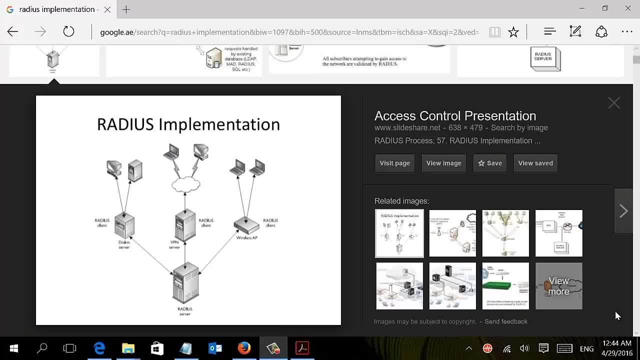 user can have only one password. he don't need to have different kind of password on the device. so this is a central administration scenario and this is the idea of using radius. now you need to know about a brief about radius and about different product that it's under the 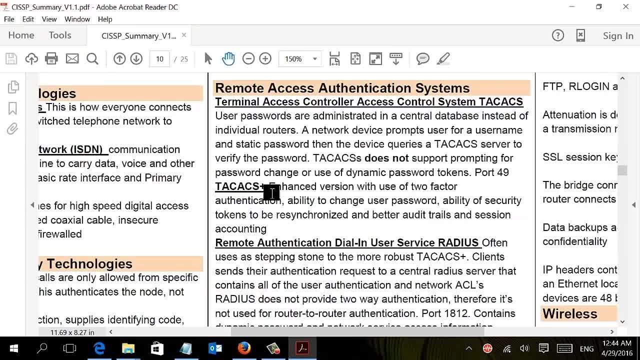 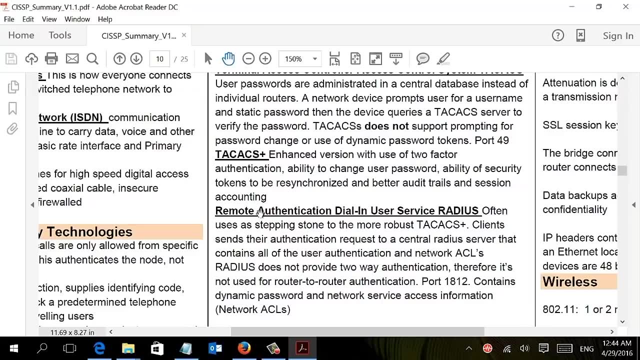 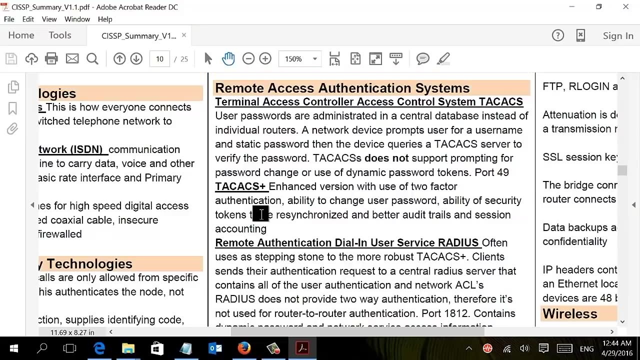 same category. i mean, we have radius, we have diameter, we have the taxi, we have the taxi plus and some of them support voice, some of them are encrypted traffic. so you just need to know a brief about radius and about this. you will find that in the small description about each one of them inside the sunflower document, so very important to 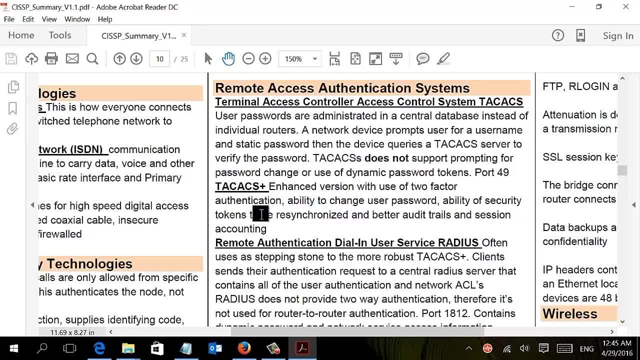 understand the central administration and to distinguish between the central administration and the single sign-on. single sign-on, it's authentication and authorization radius, it's mainly authentication. i mean now they have some products that do the same, but don't get confused to have one centralized place for all the devices to authenticate from. so it 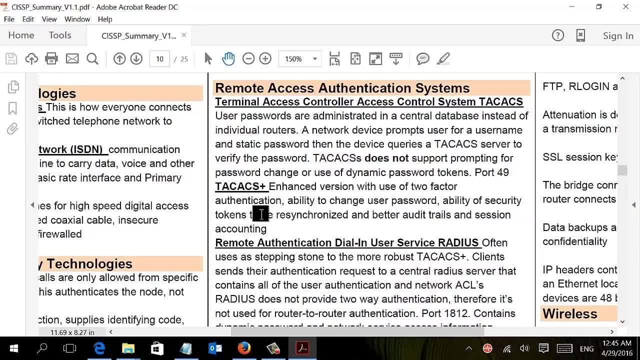 become an backend server, to be to syndicate for a VPN and dial up and any other server, so user can have only one account. so this is the idea of radius and, as I told you, you will find that in different location inside the sunflower, but, as I told you, you just need to know about the different product. 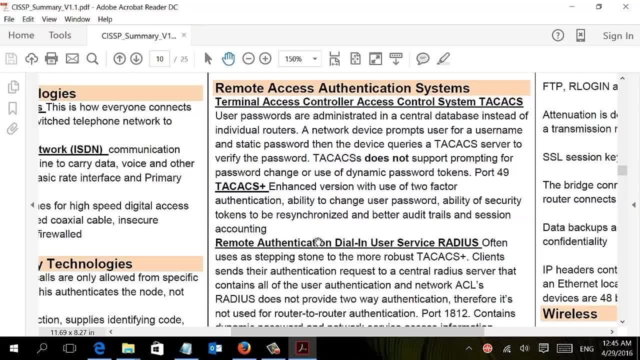 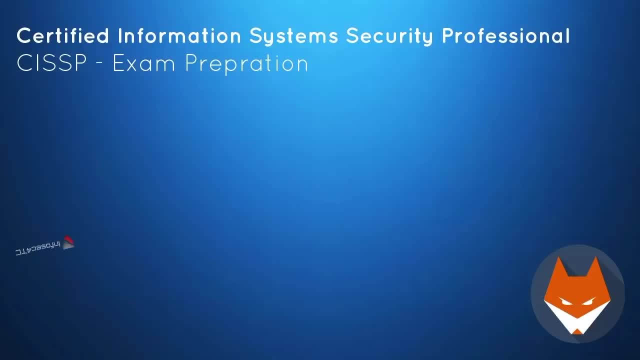 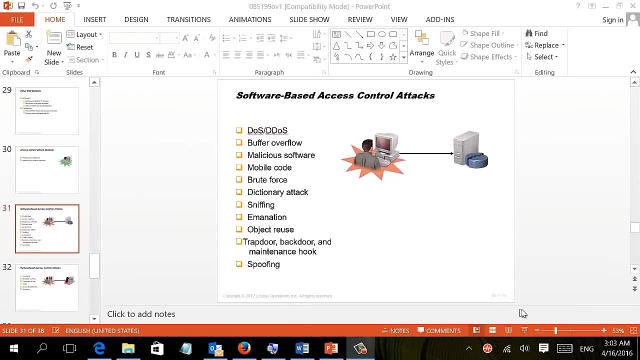 so I have like five product radius diameter: the taxi taxi taxi plus X taxi. just a brief about each one of those will be great, but you should know the idea. what exactly is the benefit of using that? in this lecture, we will be talking about access control. access control and how to use it. in this lecture, we will be talking about 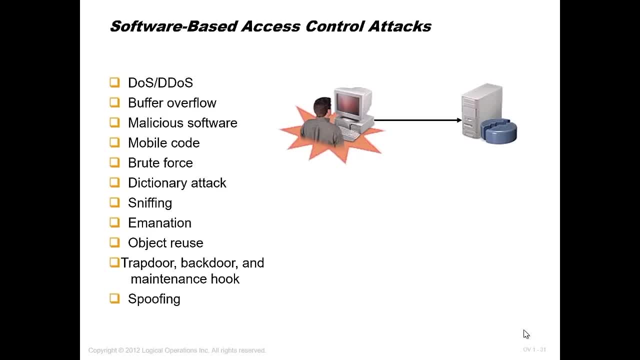 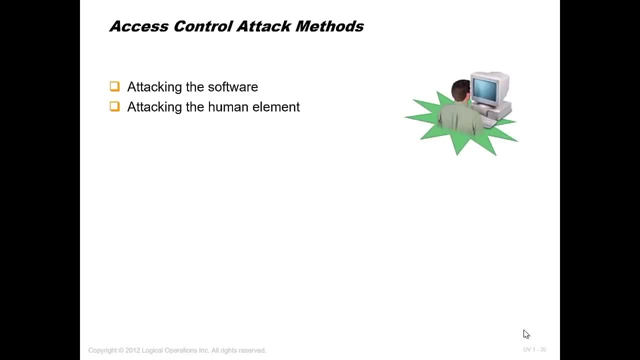 access control and how to use it. in this lecture we will be talking about attack and access control. attack- actually attack in general- is very important for the exam. many question will come inside the exam asking you about the definition of a specific attack, so we'll give some attention to. 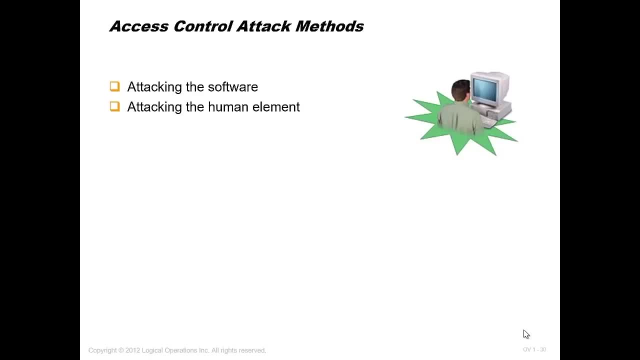 that, and there's a good point that many attack will be repeated in different domain, so you're gonna find some attack here that will be repeated on the upcoming domain, which will give us the chance to keep repeating the definition, so we will not forget about them. so please give attention to attack and I 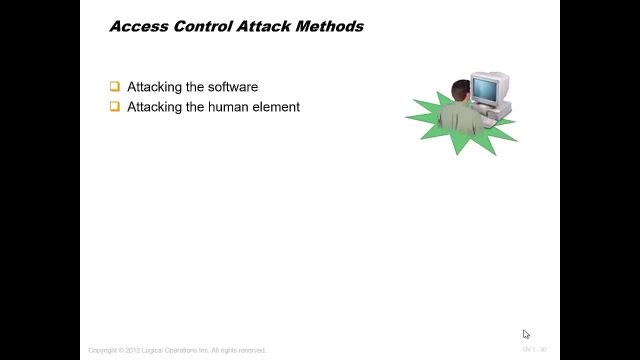 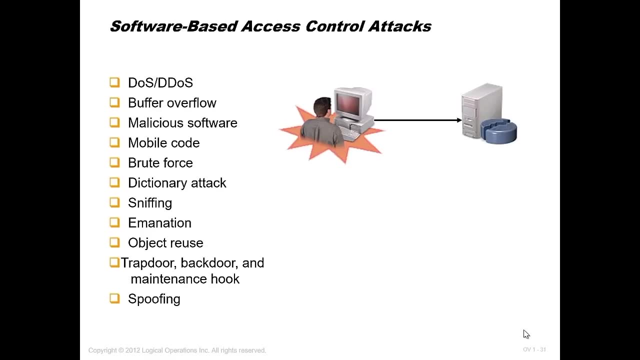 will strongly recommend to have a sheet or a document where you are writing down the attack and their definition. so here in access control attack, we have two different kind of attack. we have the software attack and we have we have the human element attack. let's start with the software attack. I'm gonna start with. 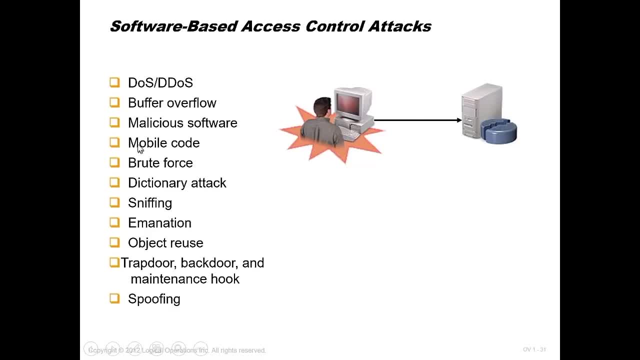 the similar attack. so, for instance, we have here an attack called the dictionary attack and brute force attack, which is kind of similar attack, and I would like to add to them, and please write it down, some attack called the rainbow table attack. so those three attack actually focusing about cracking. 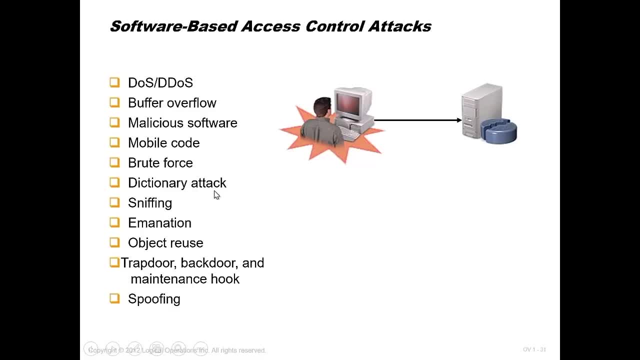 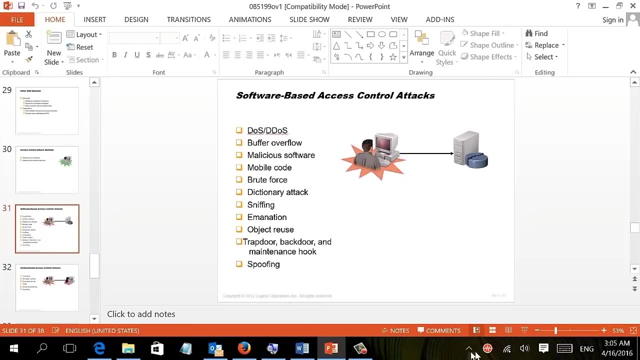 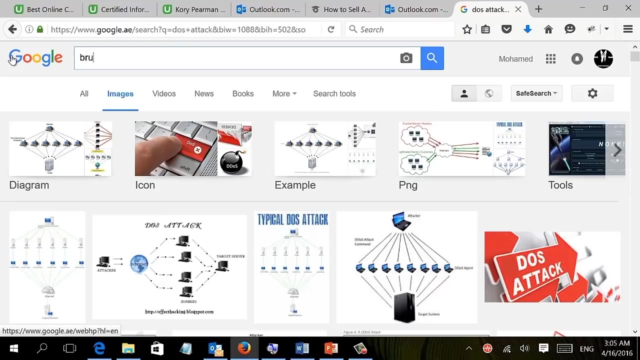 the password. let's talk about dictionary attack first, because it's kind of simple attack. dictionary attack it just you are using some program that keep trying the password. you know a lot of program are there. let me show you a proof of concept. so if we go to Google and go to, for instance, there is an application called Brutus. 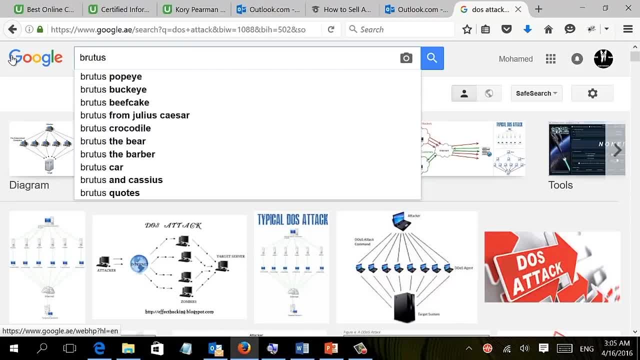 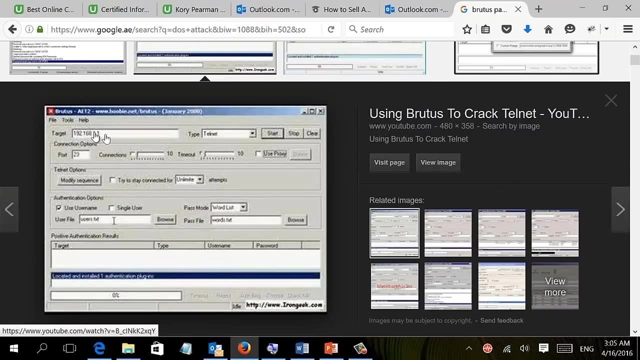 Brutus cracking Brutus password. okay, so this application for instant. this is how it look like: you are putting here the computer IP or name and you are putting here what service you need to crack the password- is it the HTTP or is it the telnet or whatever? and from here you are. 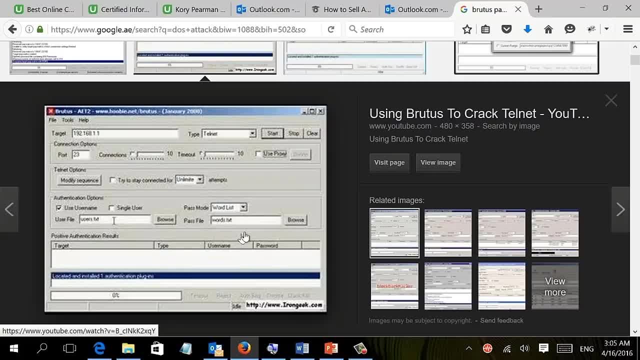 choosing a dictionary file. this is a text file that have all a lot of words, you know like the same type of file that is found in Microsoft Word. you know, when you are writing in Microsoft Word, how he is able to identify that you have a spelling mistake. 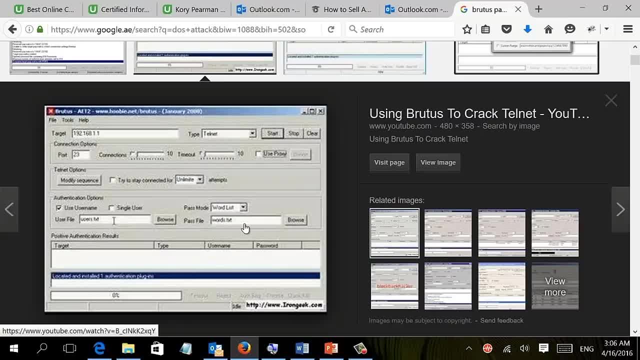 he got a dictionary fight that have all English word. so when you are writing a word that does not exist in this dictionary, he will put an unread red underline and tell you this is wrong spelling and you, when you right click on it, it will give you from the dictionary: oh, the similar word. this is a kind of 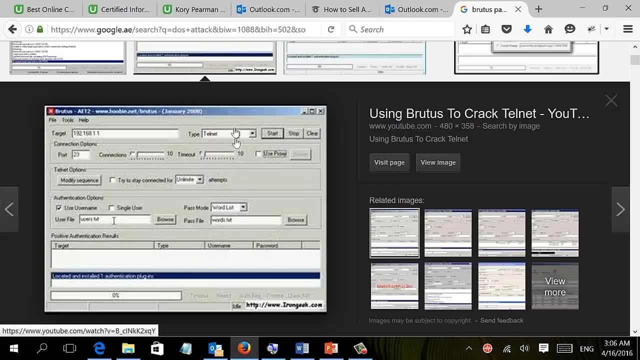 file is using to crack your password. so we're gonna try to crack the password using a dic and he's going to try word by word. this is called the dictionary attack, where you are using a dictionary file and an automated application. he's going to start cracking one by one. so point here. 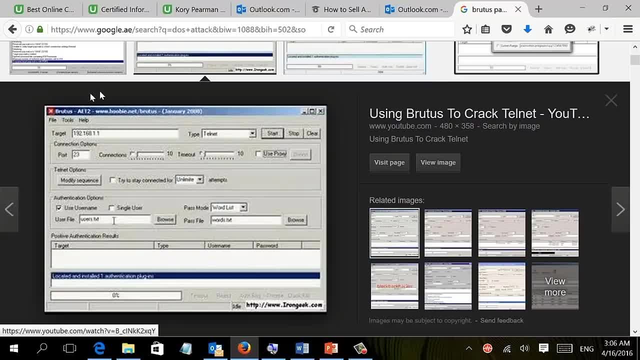 this will be effective. in case of that, your password is an english word. i mean, if you are writing your password, password or football or anything like that that can be found in the dictionary, this will be easy to crack using a dictionary. attack while brute force attack it's. 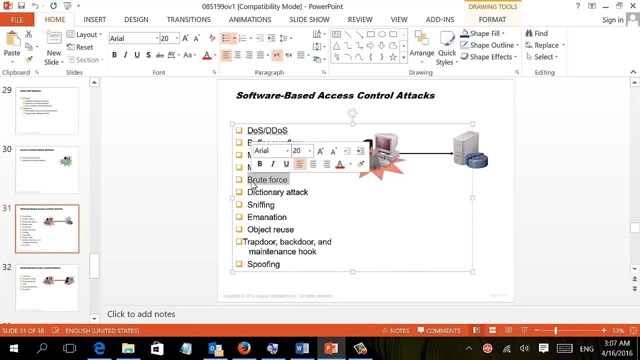 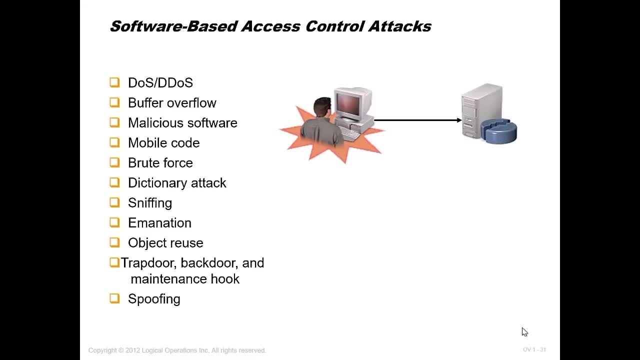 a similar attack, except he's not trying from a dictionary file, he's only trying from randomly. so if the dictionary file didn't work, he's going to try letter by letter and number by number and sign by sign until he gets a password. so you're going to try a's and a, b's and a, b, c's and a b, c. 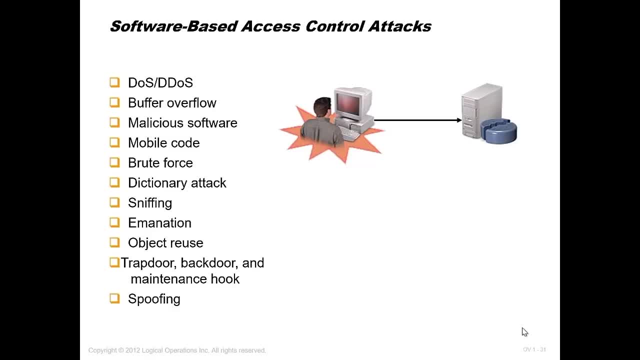 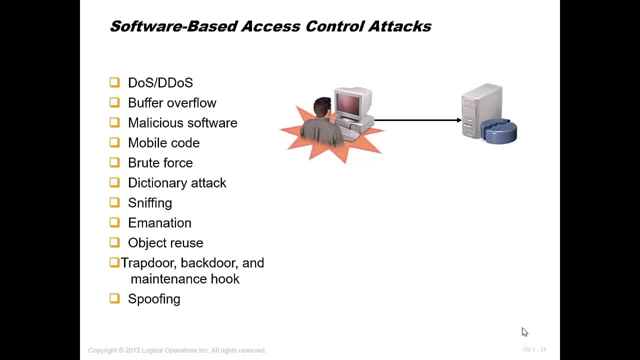 that it should be more than eight character, capital and small and special character, and this is to make the brute forcing very hard. if you have such setting, it take few years to be able to crack or to get all combination of the password. so brute force attack, it's effective. 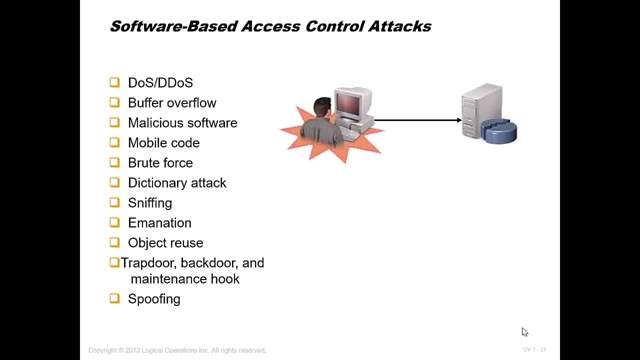 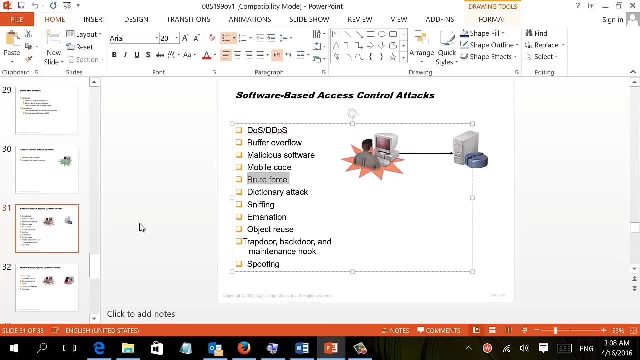 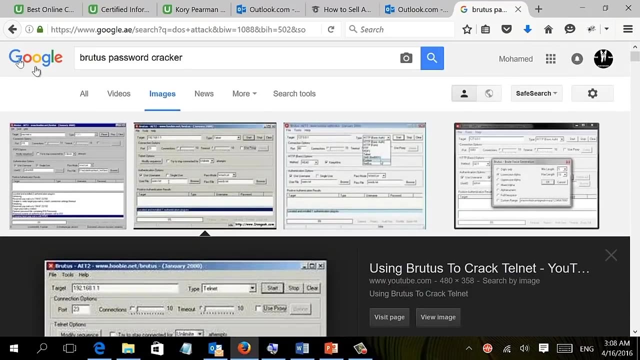 if the password was not a complex password. but if it was a complex password, definitely you cannot use it. I would like to add to those dictionary and and brute force attack another attack from the same family. please write it down because this was one of the exam question called the rainbow. 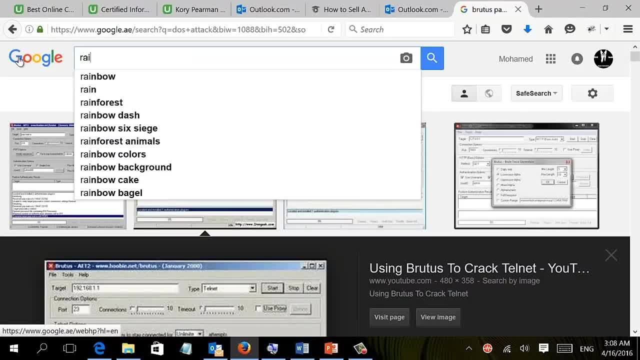 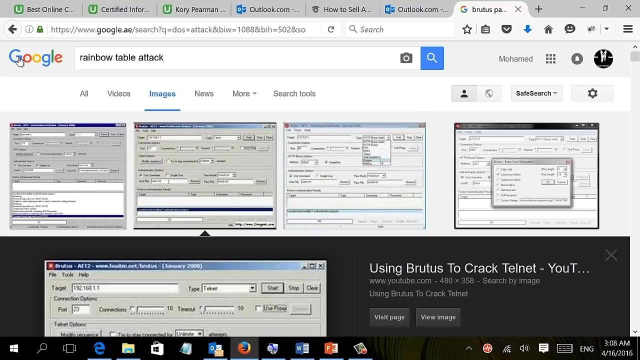 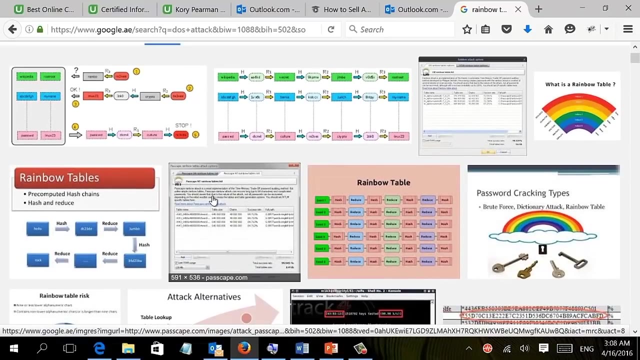 table attack. so rainbow table attack. it's a password cracking attack, except it's a little bit advanced. rainbow table attack. so the rainbow table attack, it's a little bit advanced. what is the concept of rainbow table? let me explain to you now the thing with the dictionary attack or or whatever attack you are. 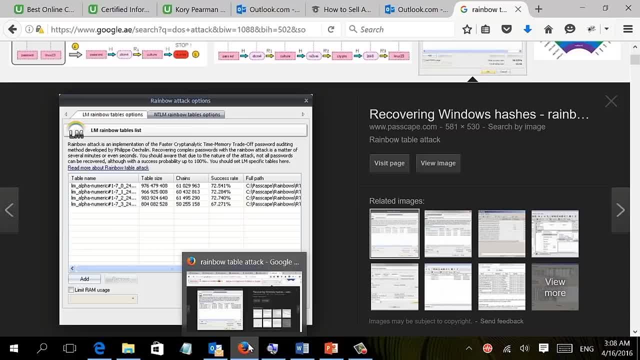 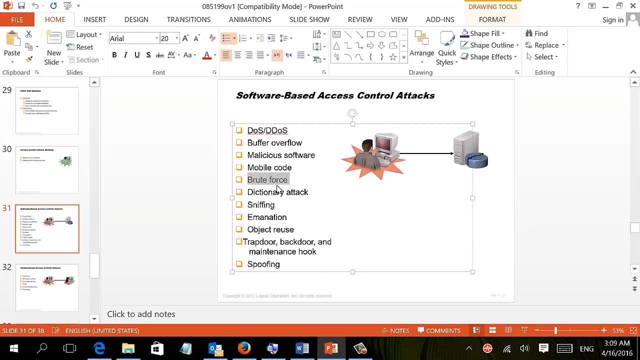 talking about dictionary attack. why is taking too long time? I mean, when we are talking about dictionary attack, why- I'm sorry about brute force attack- why is not that effective? because usually the password are saved on your computer encrypted as hash. so what happened is when you try. 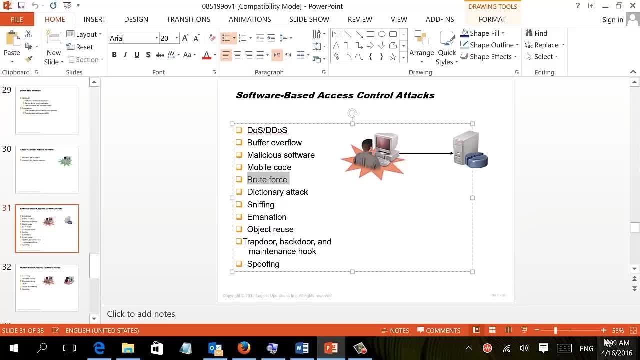 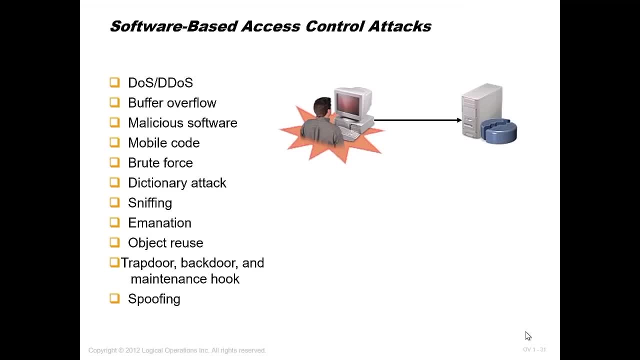 a brute force attack. what happened? he gonna try the a letter and then he will encrypt it. the same type of encryption it's inside on your computer. I mean, if you are using Microsoft Windows and you are cracking the Windows password, Windows are, savings are fine in an encryption called LM hash. 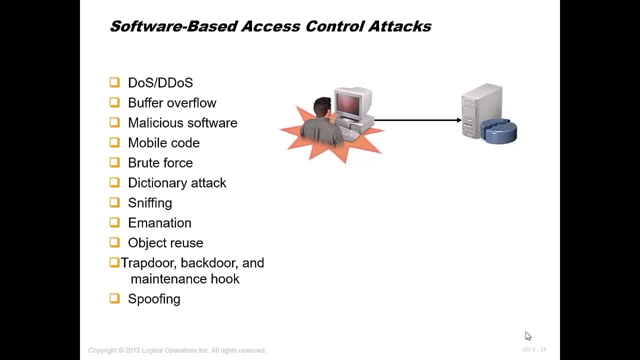 the brute force application will start taking a letter and encrypted to LM hash and then try to authenticate using this password will not work, then he gonna try a b, then a b c, then a b c, and so on and so forth. this will take time because most of the effort will be losted in the encryption. 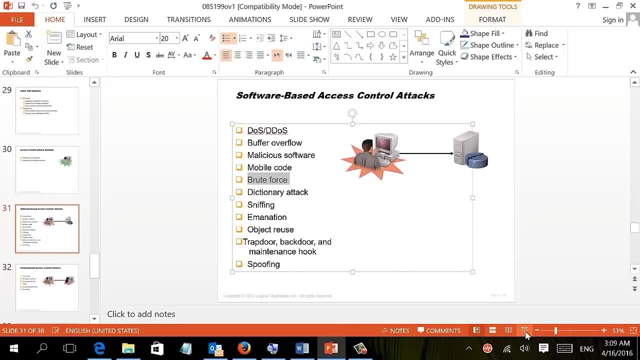 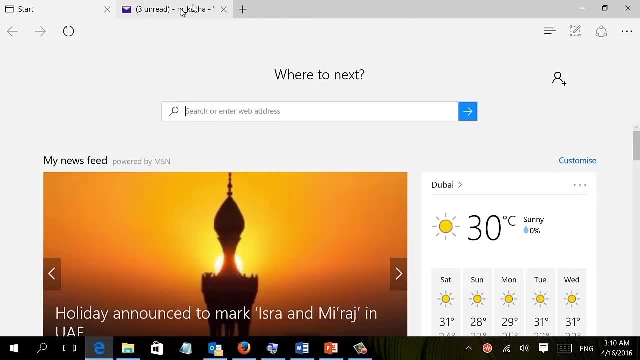 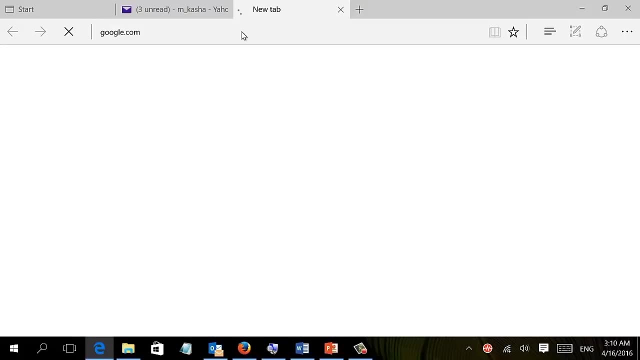 and decryption in rainbow table attack. it's quite different. you go to some website and you download some encrypted file. so, for instance, we can go to- let me see, let's open a Google website. for instance, you can go to rainbow- free rainbow table dot-com and free rainbow table dot-com- and you can go and you can download a table. so you can tell. 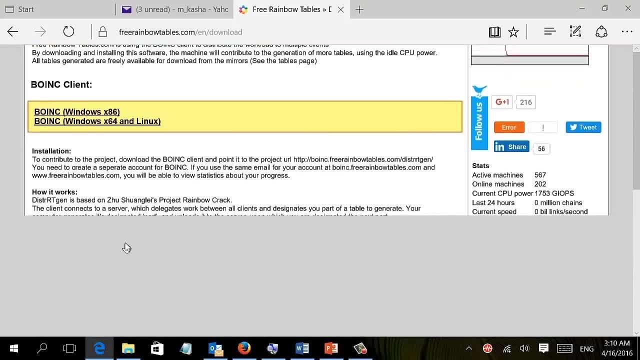 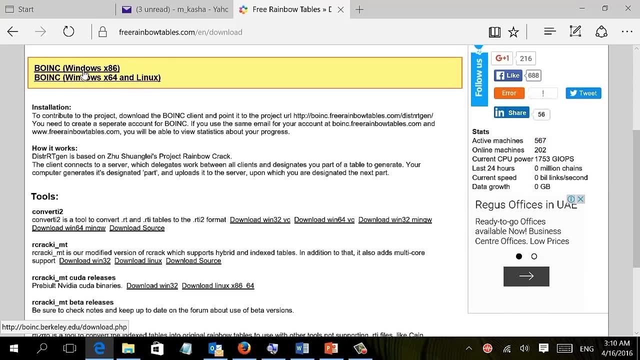 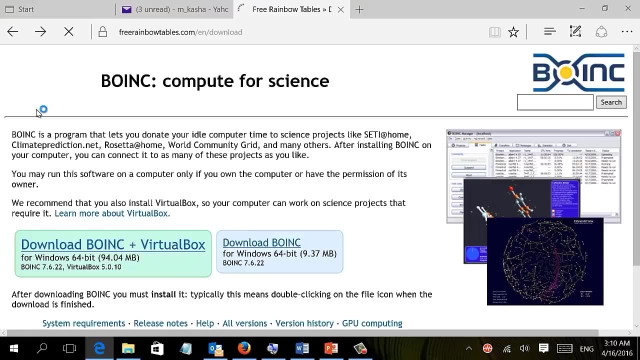 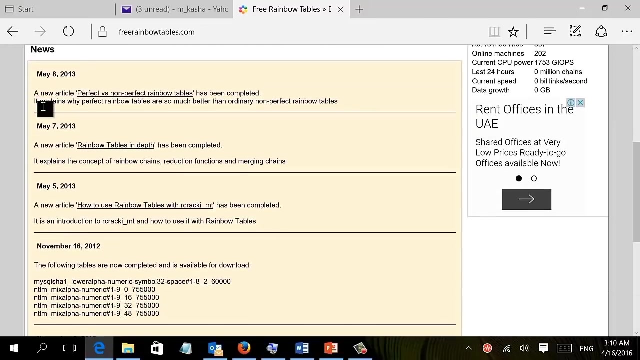 them. I need a table that has LM hash password that has from 6 to 10 letters and has small and capital and special character. so you will be having, you'll be. you have to download the tables. that may be around maybe 20 GB or 30 GB, but when you launch this table, when you launch this table, what happened is: 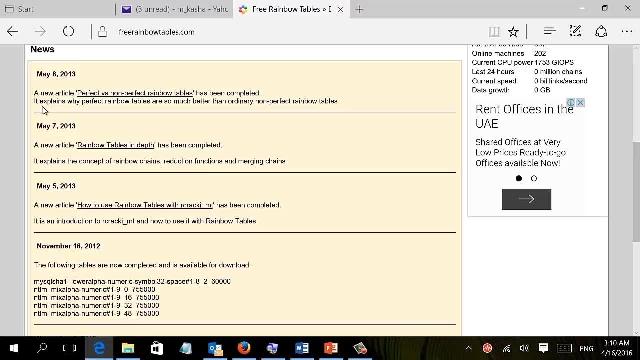 he will just compare encryption with encryption. I mean it's different than brute force. brute force take each letter and encrypted and tested, while rainbow table it's a file that include all password encrypted. so he gonna try to compare encryption with encryption. so it's take less time than brute force and it's very, very. 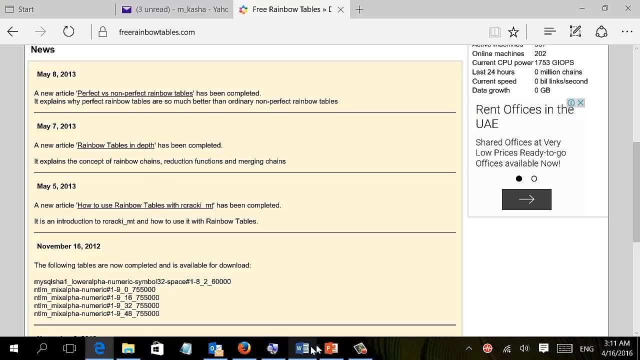 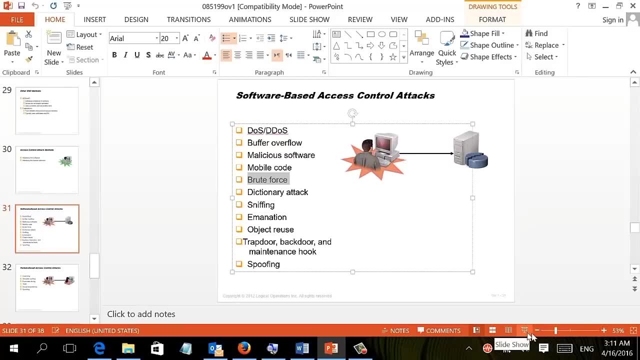 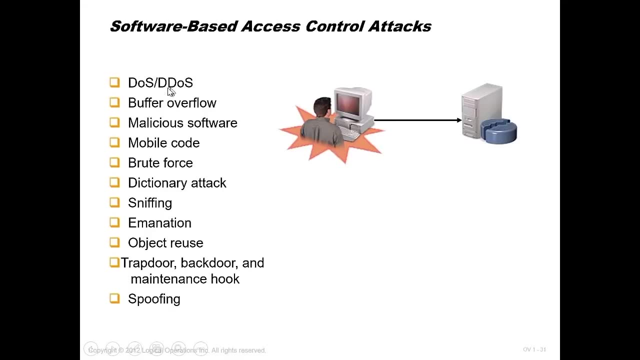 effective. but all of those are considered a cracking: password attack, brute force, dictionary attack and the rainbow table. then we are going to talk about denial of service and distributed denial of service. this is an attack that affects the uh availability of the system, so I can try to launch a lot of traffic on a web server and cause the 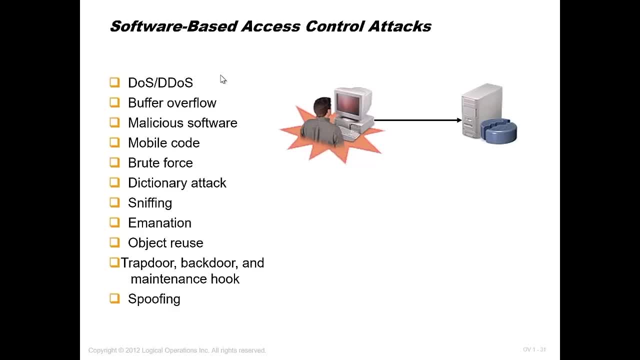 server to be down so the user cannot be able to use that. I mean I can launch some huge amount of traffic on a mail server of any organization. now those people who's working inside the organization cannot use the mail server. now we're going to have a discussion about denial of service in the 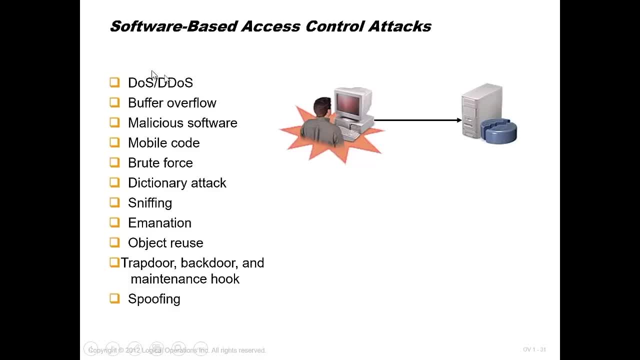 network domain because there is different type. but I want to distinguish between dos denial of service and distributed denial of service or DDoS denial of service. it's an attack that you are doing from one computer to one server, trying to crash the server and prevent user from using this. 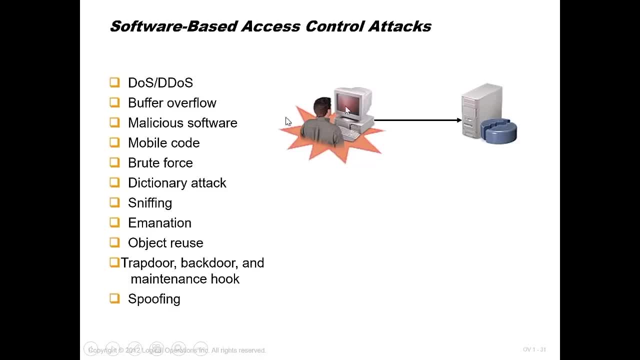 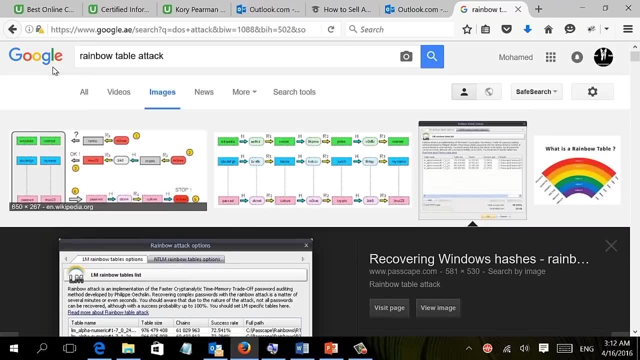 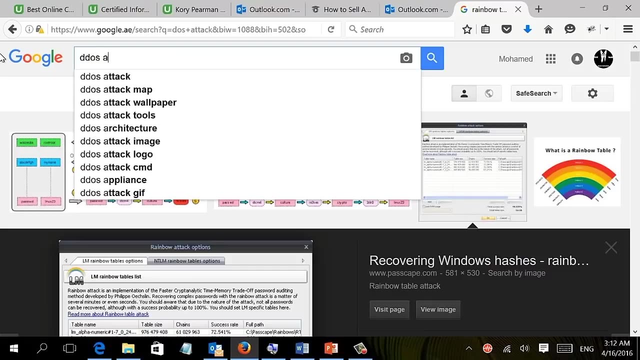 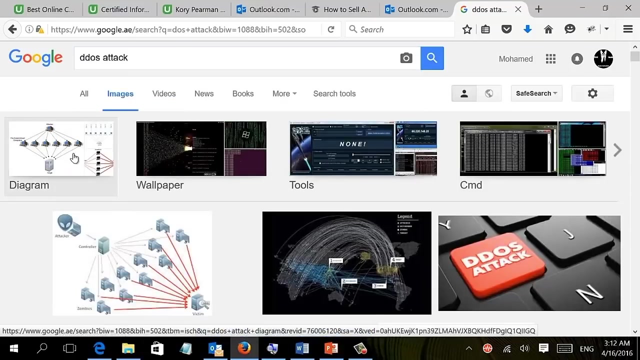 server distributed denial of service that you are attacking one server from many computer and this is much more effective. let's see how it look like. so if we go here and we type DDoS attack, so you can see that one person- it's called the command and control- usually one attacker are. 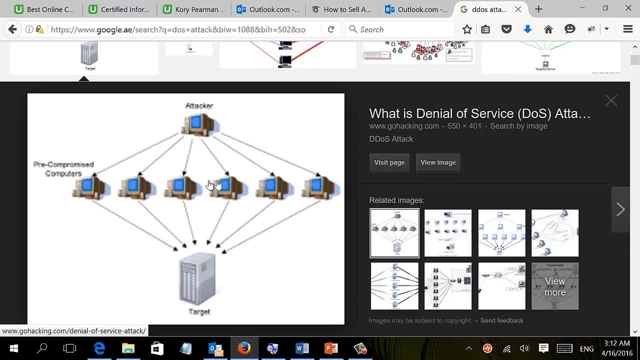 launching some or spreading some malicious code on other machines called the zombie or the dust, and what happened is he have the capability to send a request for all those malicious code- bootnet or zombie or or dust- they have the different name- to attack one server. so it's a very, very effective attack because it's it led to. 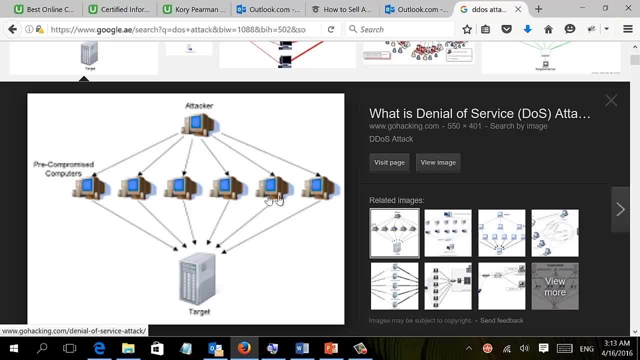 a huge amount of traffic from a huge amount amount of machines. so it's a kind of effective attack. this is called the distributed denial of service and, as I told you, this is called the one thing that is called command and control center, and they are doing that as a business right now. 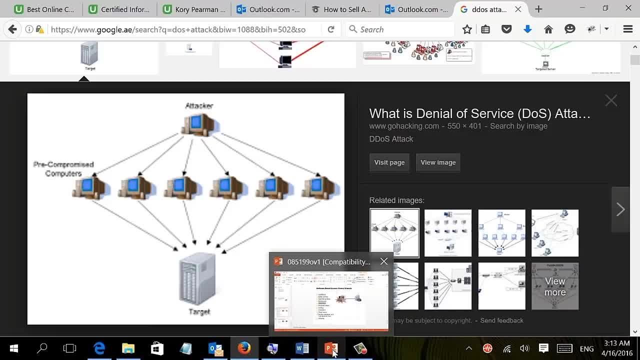 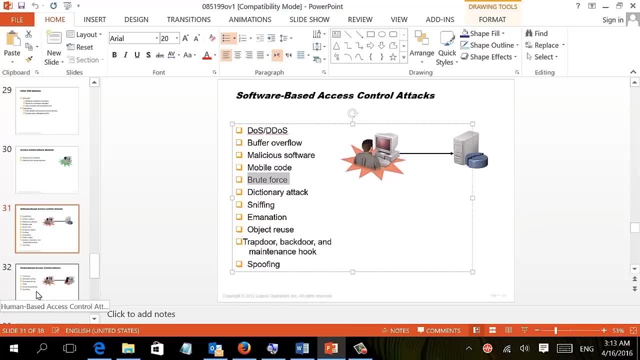 you are going. you can go to the underground Society and ask them to crash any service and it will cost you around 20 or something like that. so it become more as a business right now. now let's talk about different kind of attack. we're going to talk about similar attacks. we're 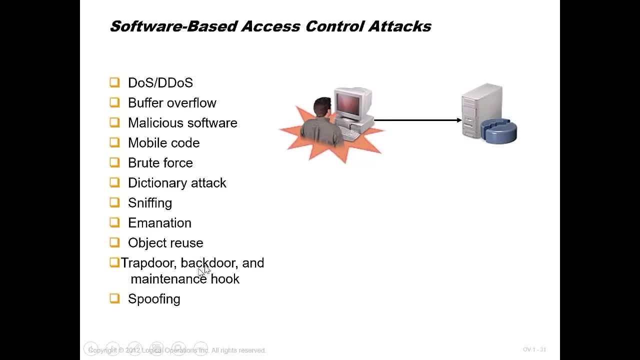 going to talk about the trap door, back door, maintenance hook, Trojan. they are all on the same side. what is that exactly? those are some applications that led to lack of information. so, for instance, the back door, it's some software, malicious software, that you may get infected with. 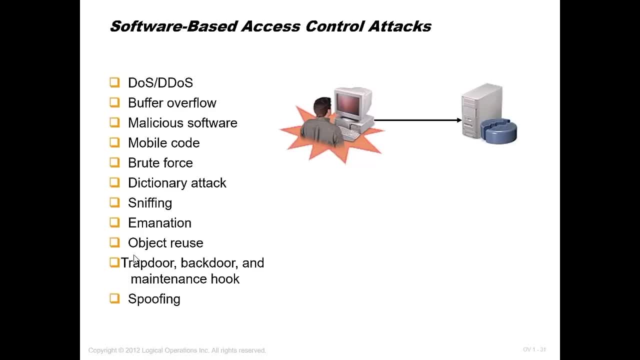 it will open a port on your machine. we're going to explain the port on the network and allow someone to connect to your network. what is the maintenance hook actually? maintenance hook is the same concept, except it has been done for a good use but it has been misused. so usually who's doing the 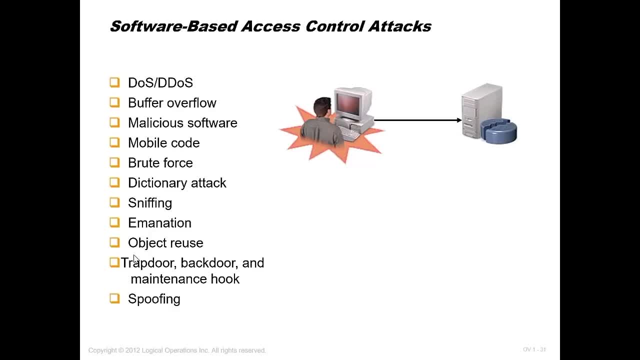 work, programmers or developers. so if I'm doing a program for a company, I can put a back door that allow me to connect to this program. so if they have any problem I can solve the problem remotely. it has been done for a good use, but if someone was able to get the information about this back. 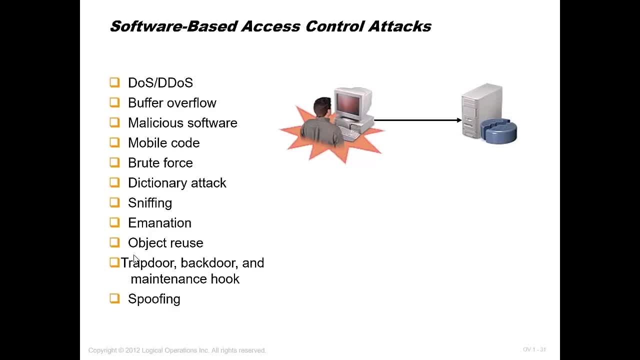 door, he will be able to log into the network and manipulate that. that's why, when you are doing a development for your organization, you have to ask the developer: do not put any maintenance hook. actually you have to make him sign that said: your system doesn't have. 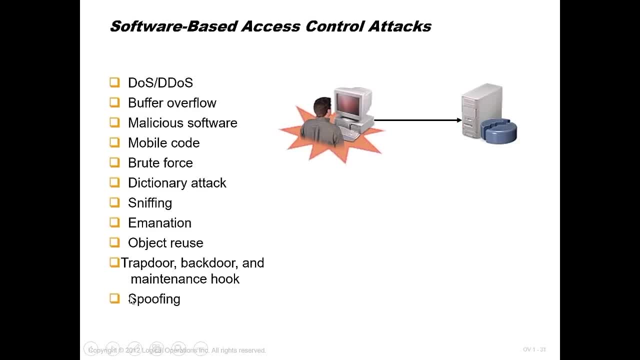 a maintenance hook. so trapdoor, backdoor, maintenance hook are in the same area. we have the buffer overflow and this will be explained also in the network part where I can start manipulating the computer memory. so assume that I'm using a program and this program is taking some information from. 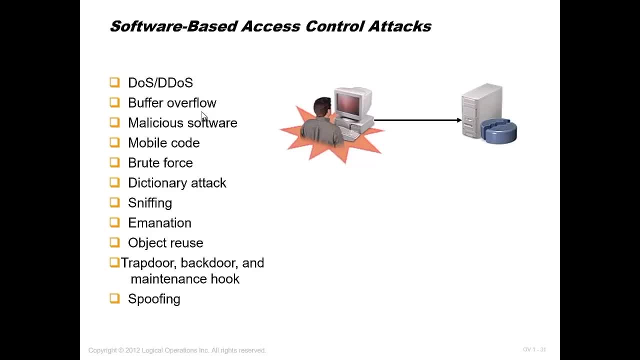 me and put them inside memory and do some processing like calculator. when you are writing the number on calculator, it will be taking and saved into memory and then some processing will be put, or I send to the memory more information that it can uh, manage. what will happen is it will. 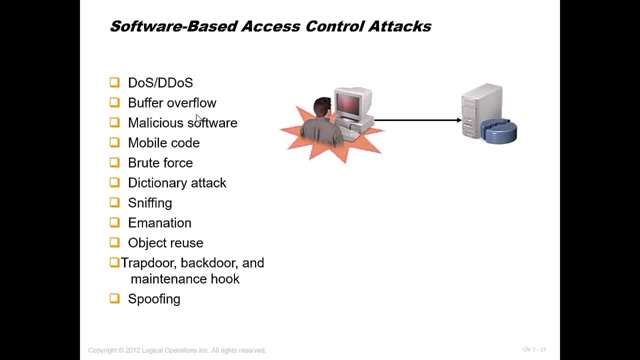 crash, and not just crash, but if I was able to reach the memory. there is some critical area inside memory that whatever I can send that it will be executed. so buffer overflow. it's manipulating memory and will take some proof of concept later on. malicious code like virus and worm and run. 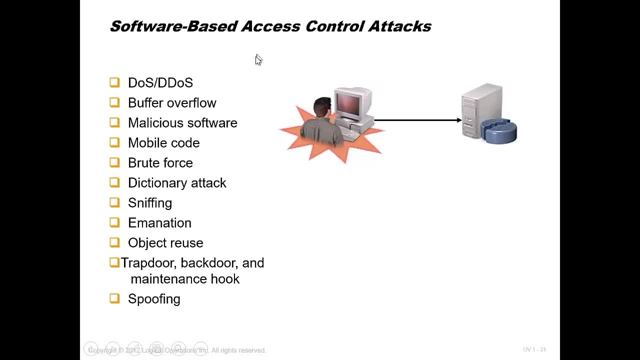 all the hardware or as information. this is also considered a access control, uh access control attacks, uh sniffing. sniffing is a layer 2 attack, usually done inside land where people can have some applications that monitor everyone traffic. so I can have on my computer program that anyone inside 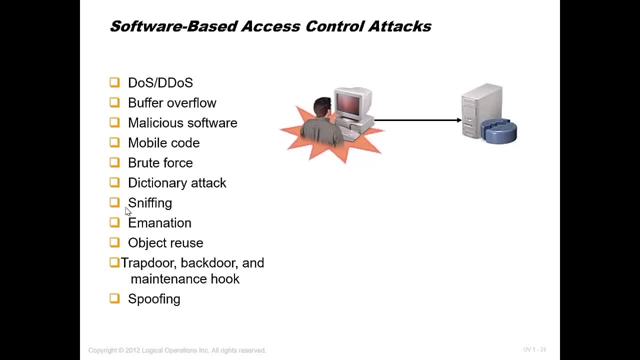 my network, wired or wireless. I can see what exactly he's sending and all the username and password and information. it's an attack related to cabling. uh, I never saw this attack live, but you should know the definition of that. it's just that you can sniffer or you can see the traffic through the 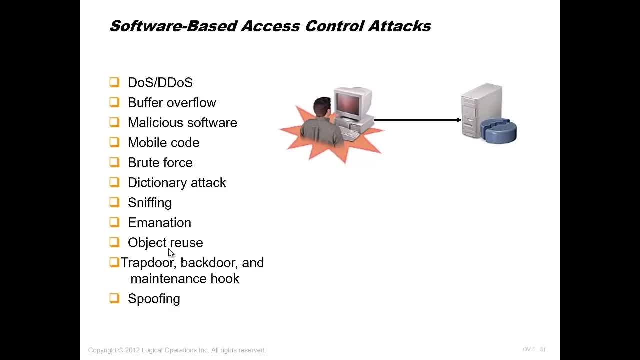 wire. I mean that's why they are asking you for the network wire. it should be hidden because it seems that some devices, when you put them on the network wire, you can see what exactly information is going through this wire. spoofing mean faking. spoofing your IP mean faking your IP or spoofing your Mac address. 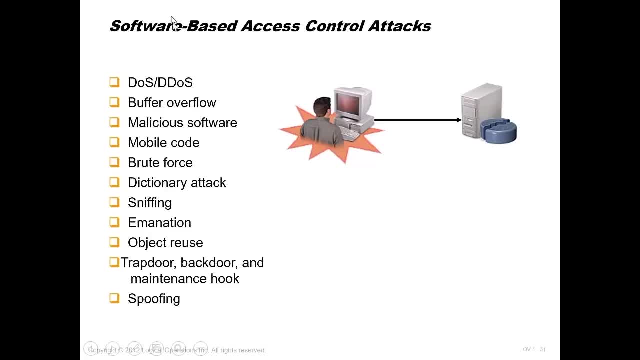 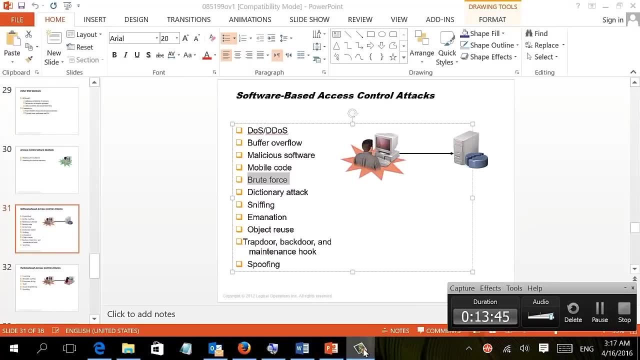 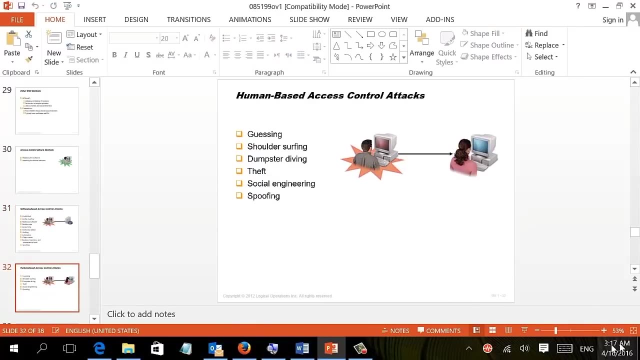 or spoofing email, so this is also considered an access control uh attack. okay, so let's see if we have time for the yeah, so now let's talk about the human-based attack. now, when we are talking about human-based, let me tell you that most of the attacks the last 10 years, the major one like Sony, 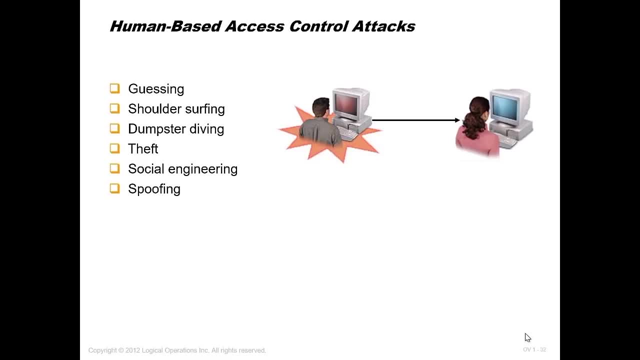 Aramco, Saudi Arabia, you know. so all those attack actually was because of the human based. so a lot of big organizations that, like Sony, they have the latest and greatest technology and they have all kinds of security employers and all experts, and they have been compromised more than one time. 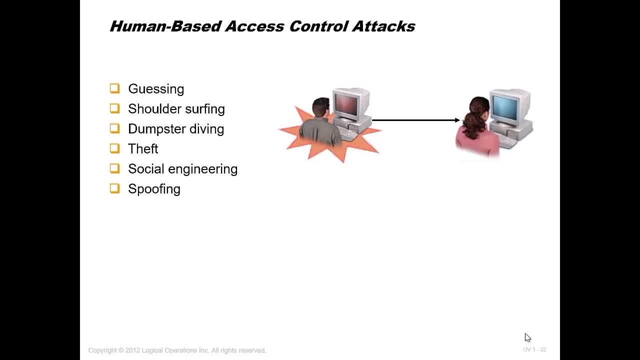 PayPal, master Visa- all of them has been compromised and the major cases, as I told you, is based on the people intentionally or non-intentionally. intentionally or non-intentionally, I can spend one week trying to compromise the network and bypass the firewall and so on, or I can send an email for the employee inside hoping that if 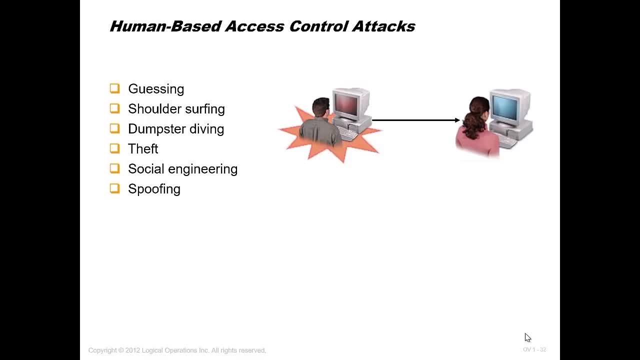 someone opens this email and click on the link, he will let me in. so it's quite effective. so, realistically, the human base is quite equal effective. so we have attacks like guessing password. a lot of people are assigning passwords that is easy to guess, like password pass one to three or 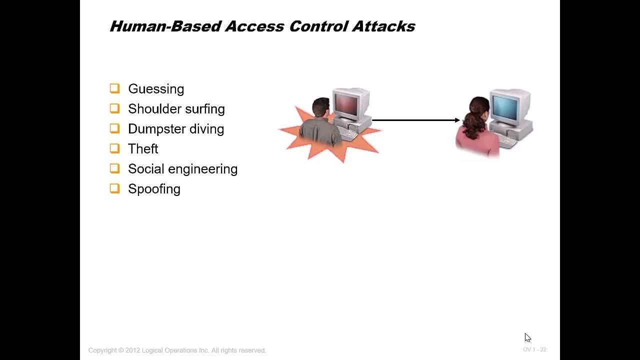 of their family member or you know. so you can try by guessing the password, shoulder surfing, and this is if you are looking beside someone where he's writing the password, dumpster diving, which is looking inside the trash. maybe you can find the sticky notes that has a password on it. 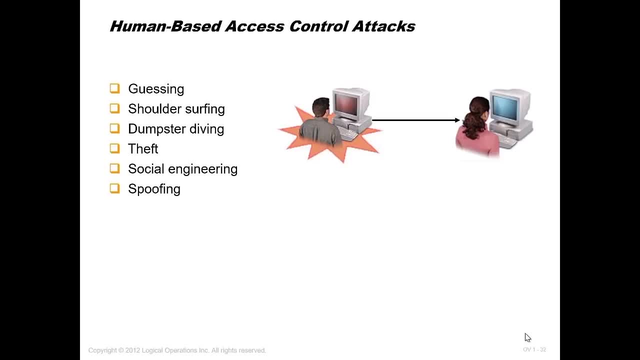 theft and social engineering, and this is the most effective attack where you are trying to convince people depending on their weak awareness. so, for instance, you are calling someone over the phone- you are assuming that you are from technical support- and you search online, you're able to get some information about the technical support people working there as their name. so you mentioned. 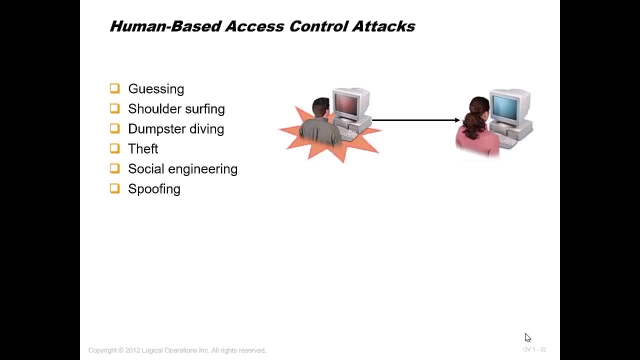 that. i'm this guy from technical support. you have a virus on your machine. please share your password so we can go and delete or remove this password. it maybe seem very basic but actually, realistically, it works and there is a book that, if you get a chance, i want you to read this, called the. 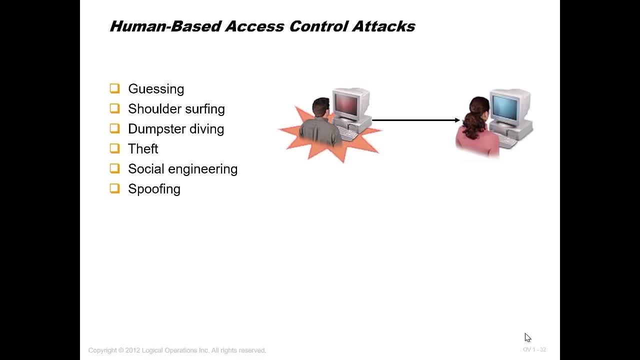 art of deception for a guy called kevin metnick. he was one of the very famous social engineering and he spent most of his life in jail but now he's one of the biggest security experts and consulting. but he was writing his experience- how he was able to compromise banks and fbi and 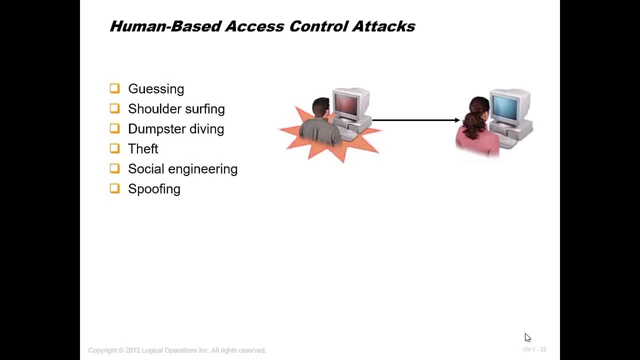 uh, rexon and many, many of the major companies, just by social engineering. quite interesting. so if you get a chance, please read it. actually, you know it will give you a lot of like knowledge about social engineering and how to prevent social engineering and spoofing, which is the same concept, which is faking, so i can spoof my caller id, so i 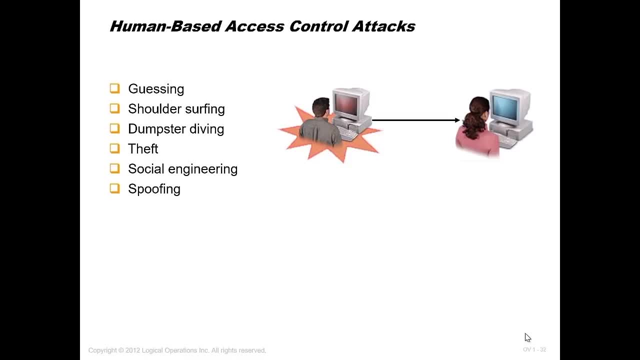 can be calling someone and it will show it's coming from your his bank and i can ask for any information, or i can spoof spoof sms or i can spoof email. so also this is attack related to access control, two parts remaining in this domain, which will be the intrusion detection system. 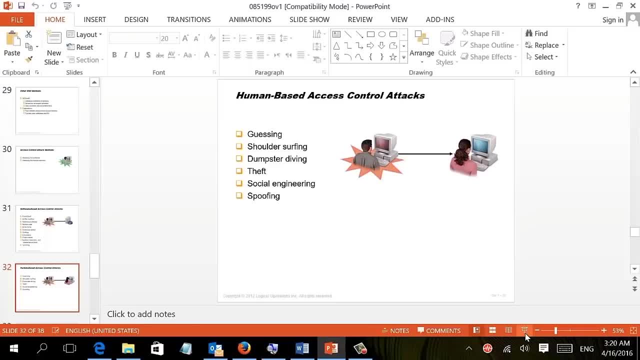 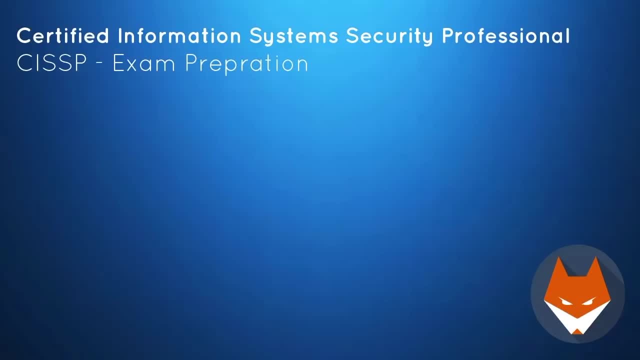 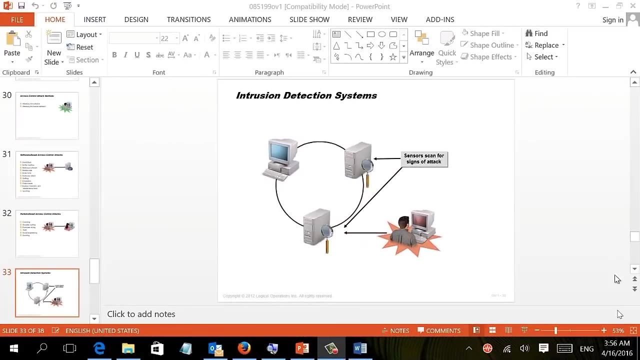 and the penetration testing. we'll be covering that to the upcoming lecture. in this lecture we'll be talking about intrusion detection system or ids, and we're going to talk about different kind of intrusion detection system but during the network and during the physical, will be going more in depth regarding that and 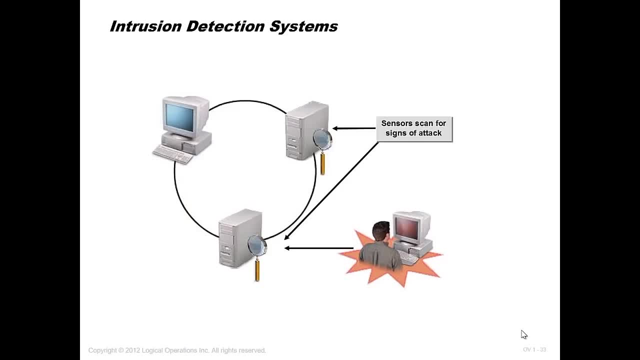 their type. what is intrusion detection system, or the ids intrusion detection system or, mainly, network intrusion detection system? it's a detective technique. so this is how it works. you have an ids- it could be an appliance or a software- and you run that inside your network. it will start sniffing the network. it will start capturing all type of traffic inside your network. 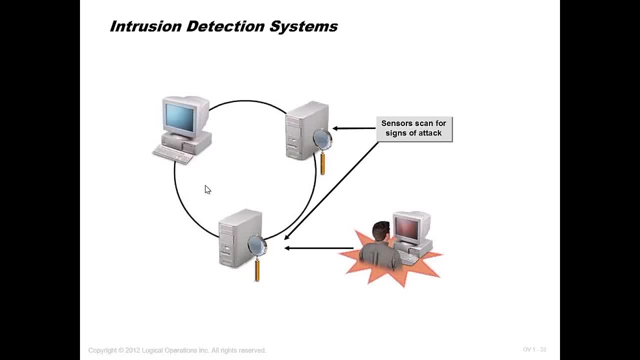 and if he detect any malicious traffic, he will notify you. he will not stop it. that's why it's called intrusion detection, while we have another product called intrusion prevention system. ips works the same way, except when he found some malicious code, he will stop them. so the intrusion detection system: sniffer your network, analyze the traffic. 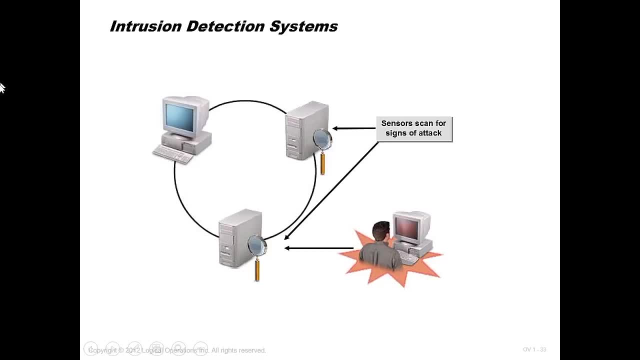 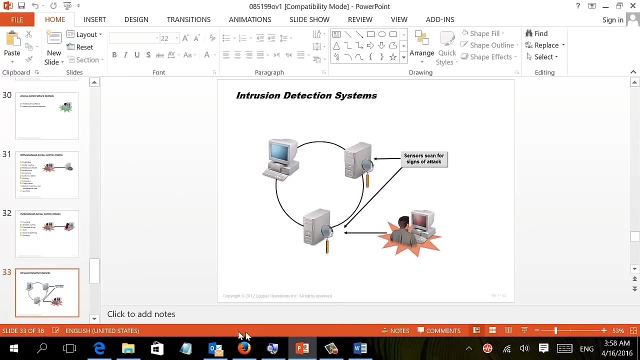 and if he found any suspecting traffic he will detect and notify, but he will not stop it. now, if you need to be more familiar with it, you can install a program called snort. snort. one of the major application for ids to be to go through this applications and see how it works. but for the 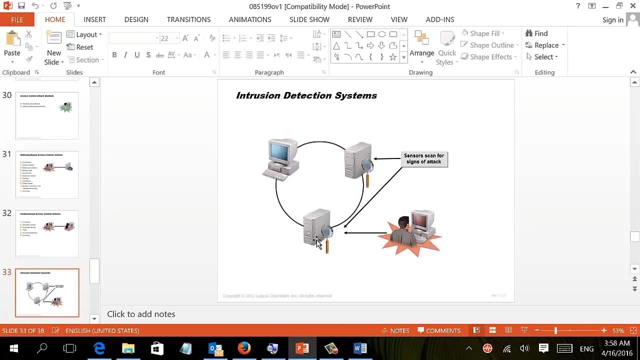 purpose of this course. you don't need to know specific product or you not. you don't need to know how to configure it or anything like that. you just need to know the functionality of ids, under which category it work. it work as a detective layer, it's not a preventive, while. 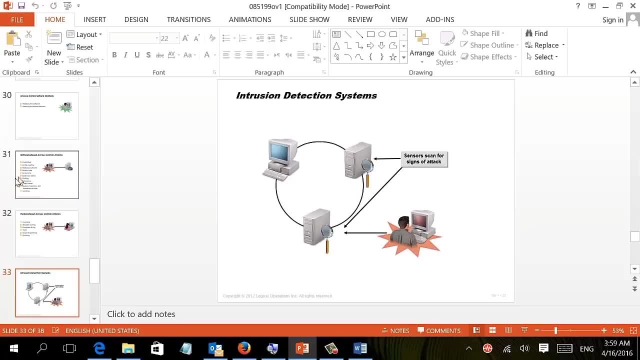 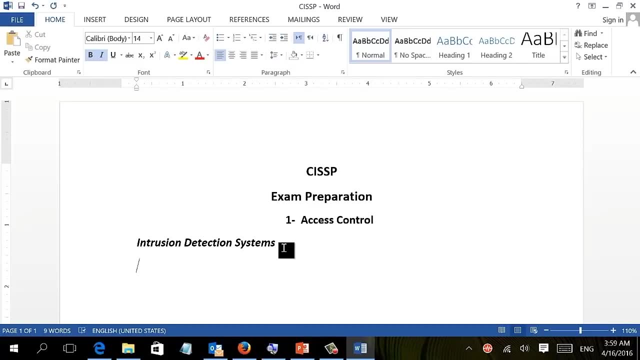 firewall is preventive but ids is detected and we have to see how it works. so we have two different type and some tricky part of here. so in ids we have the signature base, signature based, signature based, and we have the sorry based, signature based and the behavior based. 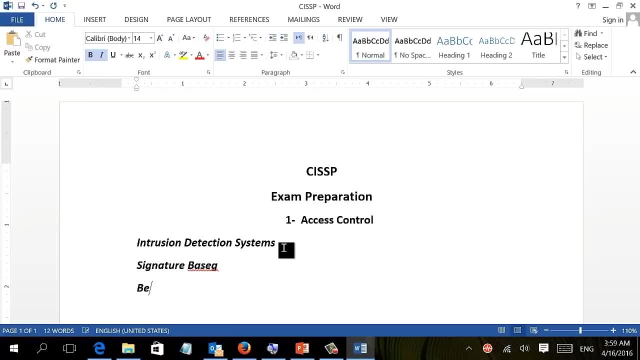 okay, the if you're based. now what is the difference between them? signature based will work as an antivirus, so you put some signatures there and he start monitoring the traffic inside the network and he found. if he found any malicious traffic, he will uh, detect and notify while behavior base. it's smarter than that. 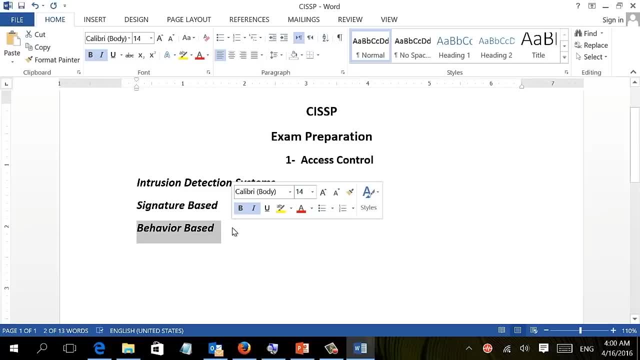 and you will have your base. you let that running for your network for a while, two weeks, three weeks- until he build a baseline and he will know what is normal and according to that, if anything else up, normal, show up, he will identify that as a suspicion behavior. 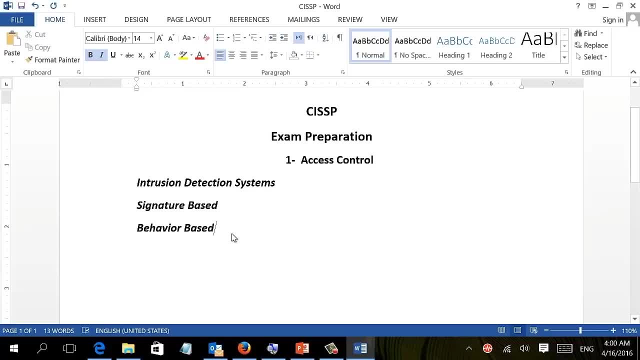 it's like you are getting a security guard in your side or your organization and you don't tell him anything and you let. let him work for a couple of weeks. he will be checking people coming in and out for two, three week. eventually he will know whom are the people. who is working inside. 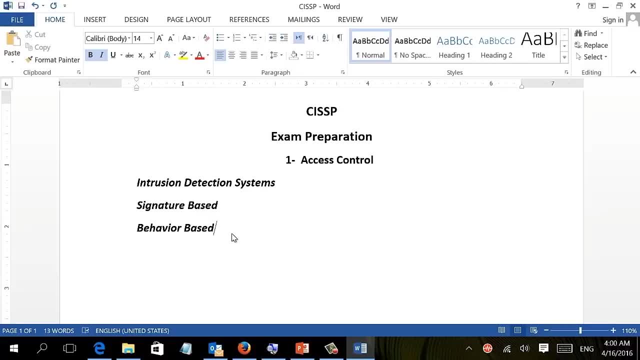 this organization and whenever an intruder show up he will know that he's this guy. do not belong to this organization. it's kind of the same topic, so, behavior-based, it's more smarter, except it take more time to configure because you'll get a lot of false positive and he will suspect everything. 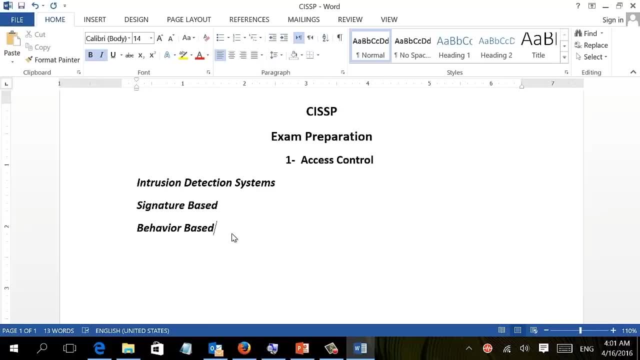 besides, if your network is compromised from the beginning, he will consider compromisation is normal. so this is the two type. also, we have two category of and we have two category of ideas. we have the network with IPS network, these where you have an IPS that mm-hmm sorry, you have an. 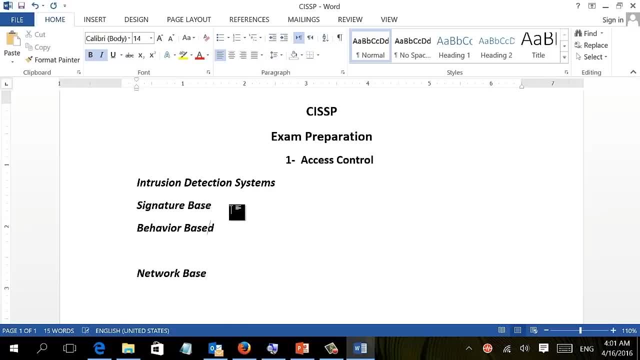 IPS that run inside your network and detect all kind of traffic. And this is working life. I mean he's sniffing the network. Any traffic going from any machine to any machine is going through the IPS software or appliance And we have a host-based IPS. 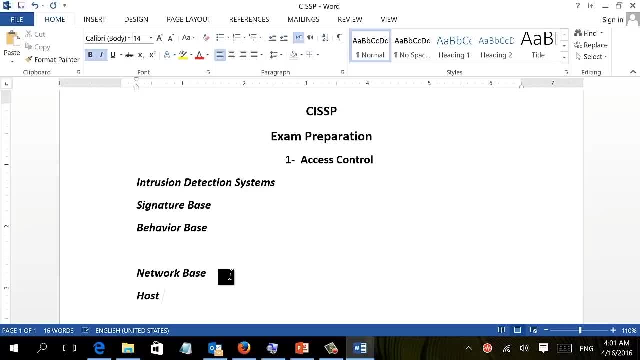 where you can install it on your computer: Host-based IPS. You can install it on your computer and you will detect anything suspicious. Now there is a tricky point here that you may expect a question about that. for an example, Network-based IPS is taking. 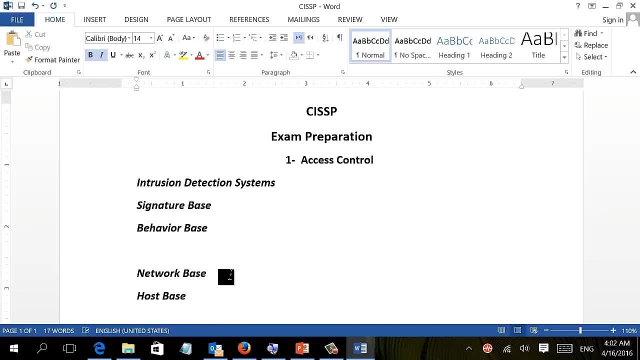 his information from where? From capturing live traffic, While the host-based IPS is taking his information from event viewer and logs. So he's not really working live event viewer. He's analyzing the traffic from the event viewer, for instance, and any log that you have on your system. So this is 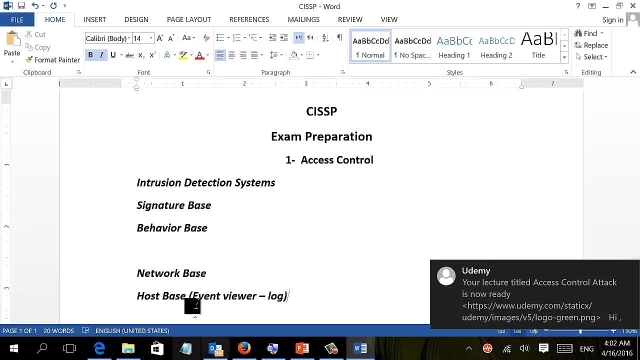 actually very, very important to consider that. host-based IPS- I'm sorry ideas- are using logs and event to analyze the traffic, while network-based are using the real traffic. Now, before closing this lecture, I just want to distinguish between the technical ideas that we are talking about, right? 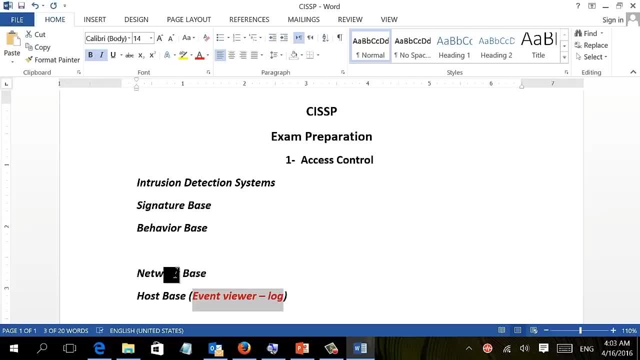 now and the physical ideas that we'll be talking about on the physical security, Because we have an intrusion detection system. when it comes to physical security, You know this device, that they are implemented in stores, that if someone tried to break in, it will launch any kind of alarm. This 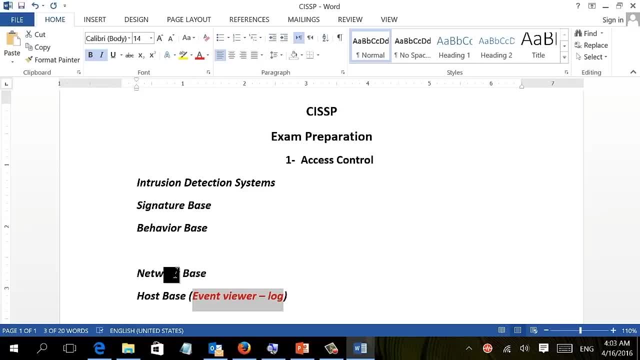 is also considered an ideas and there is type of the magnetic and voice detection and this kind of thing, But this will be explained into the physical security domain, But right now we are talking about the technical security ideas. By the way, another way for 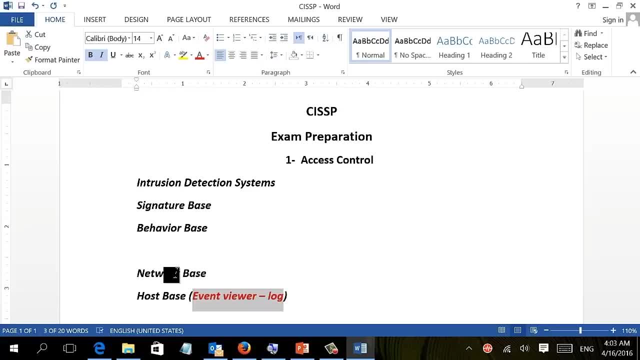 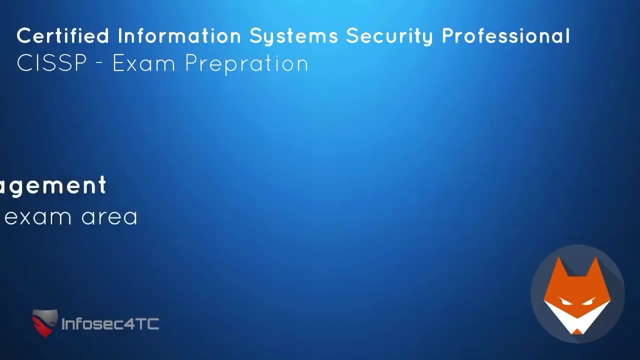 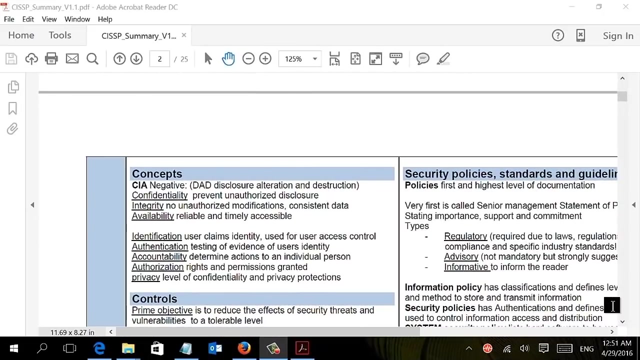 technical inside CSSP. it's logical. So whenever you get asked about logical security layer or logical domains, this is considered the technical domain After the technical security. you will find that the technical security is not the main thing. The technical security is the access. 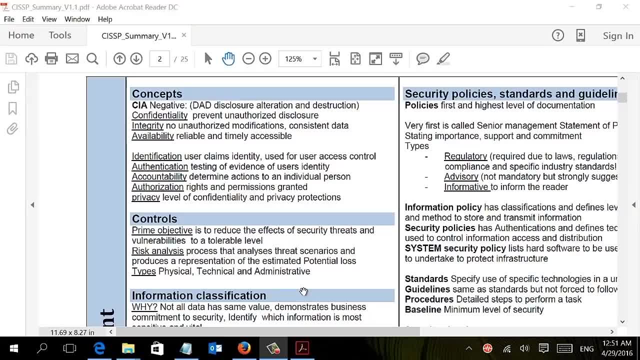 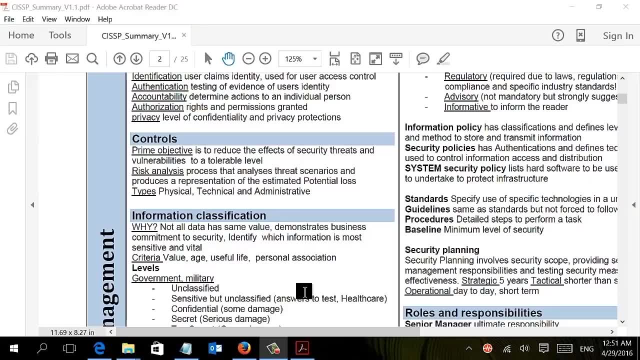 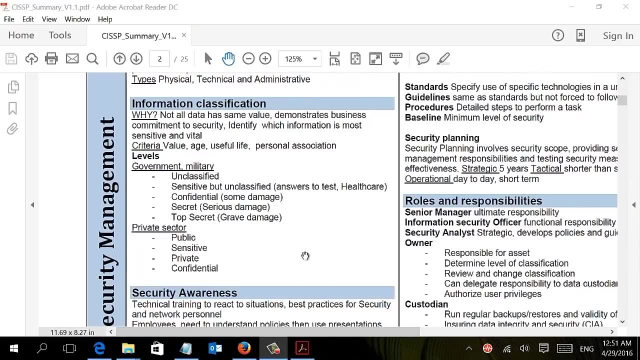 control domain. So we just need to go through the sunflower and focus about some of the important point before going and solving some question and seeing the type of question we may face inside the exam. Now in the sunflower document, some domain: 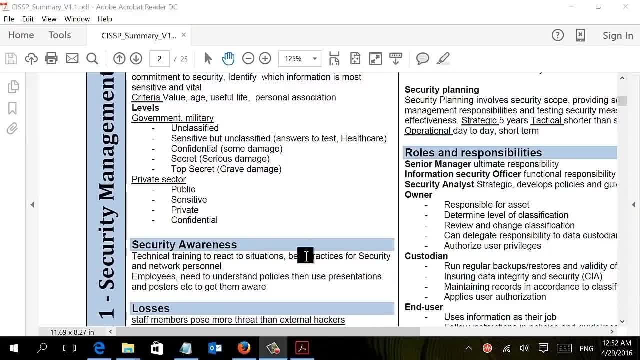 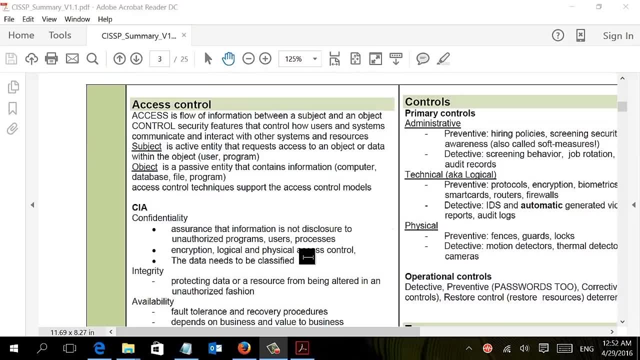 are two page, while some domain are three, or some domain are five- Depends about how long or how big the domain is. Access control is actually two page, So let's see what exactly do we need to check before going there. So the 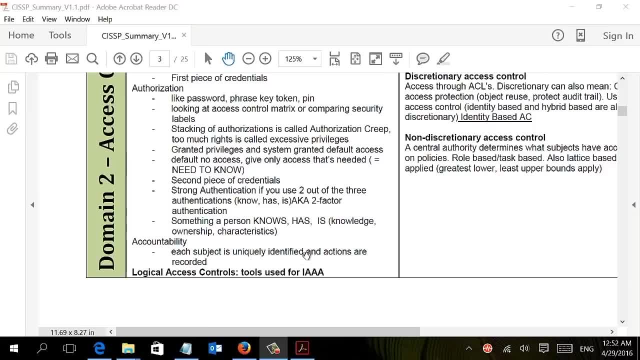 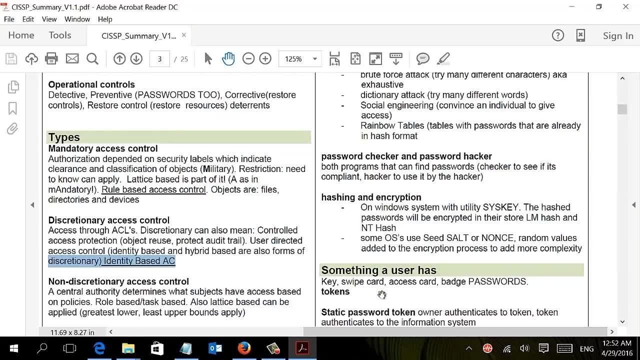 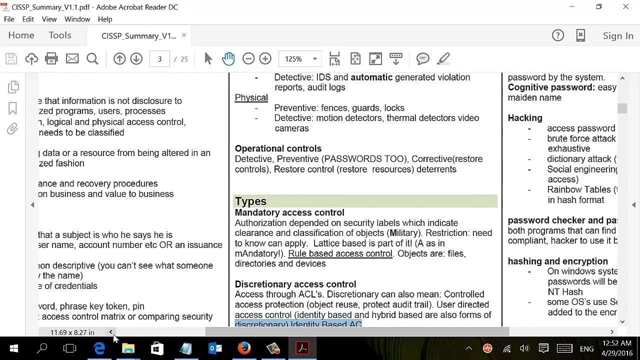 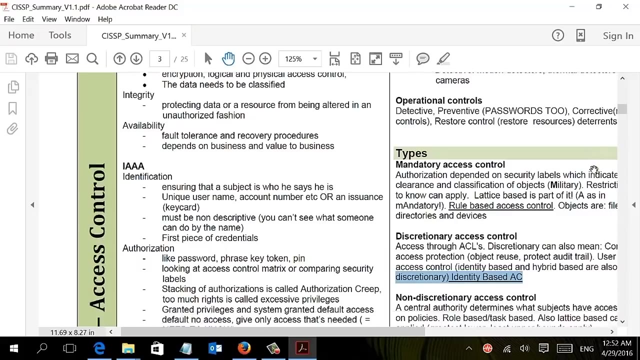 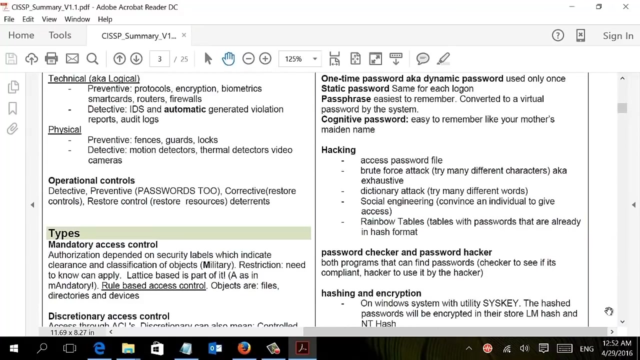 identification and the AAA. this is actually- we went through that- The type of access controls, the DAC and MAC and their specification. This is also important. I'm just, you know, viewing the document as a preventive and corrective, defining or categorizing security Also. this is important. I'm just pointing to. 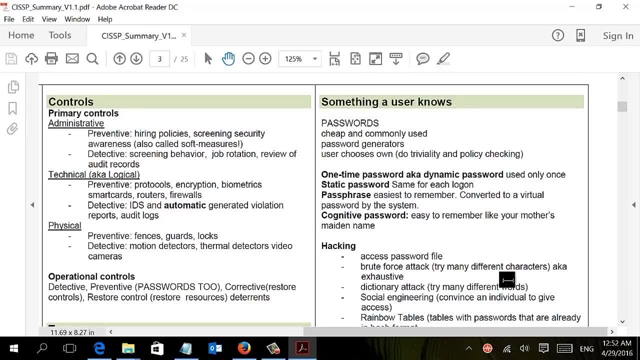 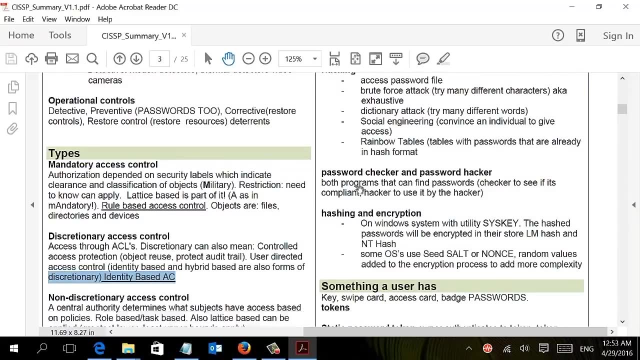 some important topic Now, the type of password. you'll find more than one type. I mean, you'll find this concative password which is things like your mother made the name or something like that Passphrase: one time password hashing. 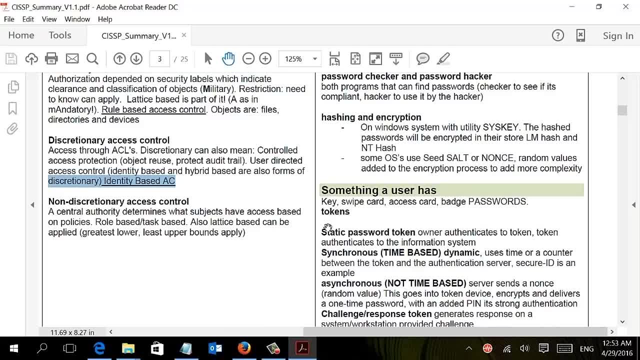 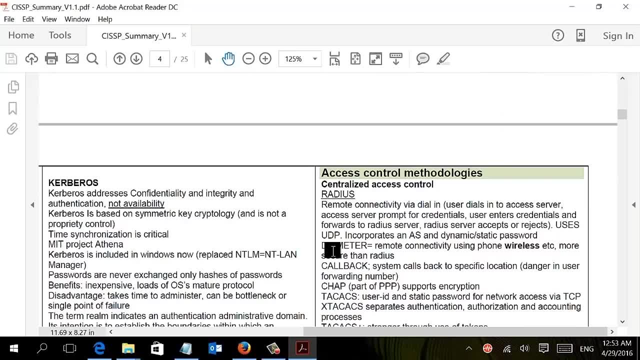 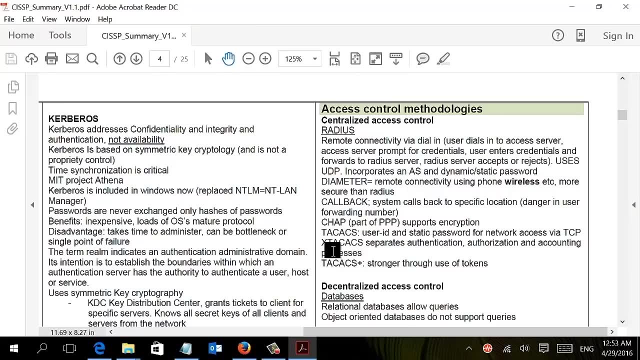 um, yeah, identifying the two different kind of talking device: time based and not time based, synchronous and asynchronous. As you can see, nothing major here. Uh, Kerberos, single sign-on, the step are very, very important And please give specific attention for. 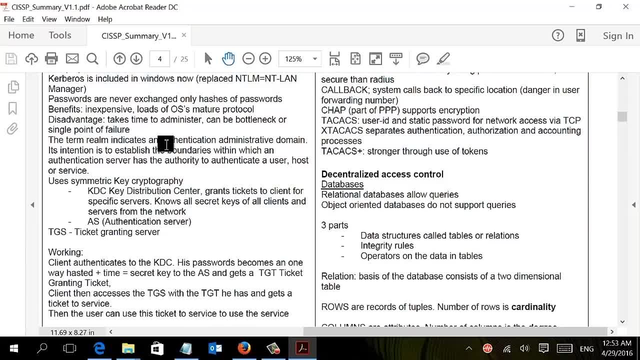 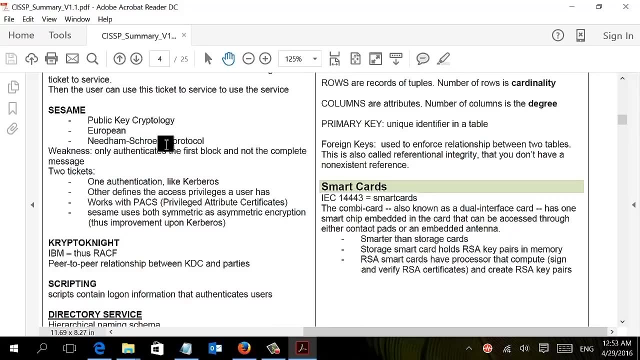 things that is underlined or capital letter. This is very, very important. Uh, this is how the single sign-on work. We explained that in depth. uh, there is other type of single sign-on, like sesame, like uh, uh girl pro night, But, as you can see, just give a. 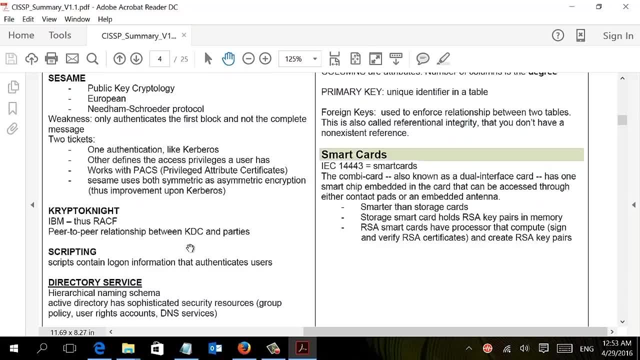 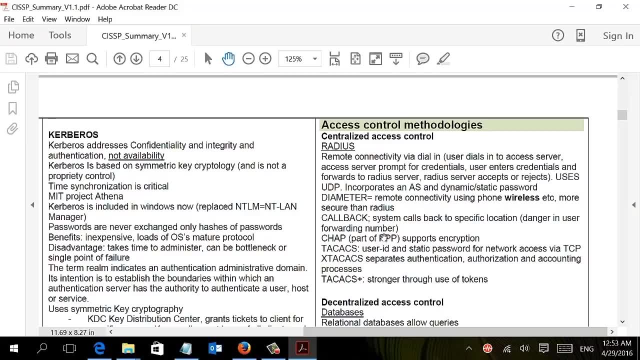 line, but definitely single sign-on is the most important party directory service. uh, some access control mythology like radius. Uh, we already explained radius. the taxi, taxi plus the same concept or same definition are repeated in the network part. Uh, okay. 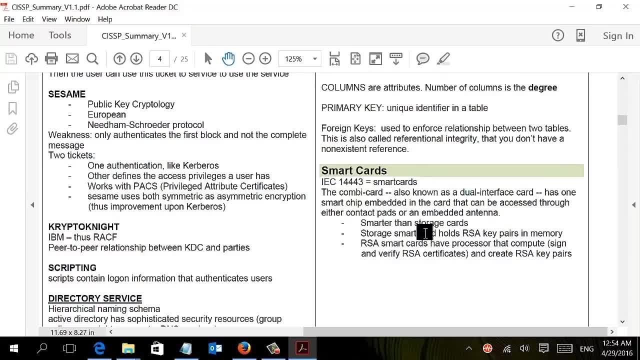 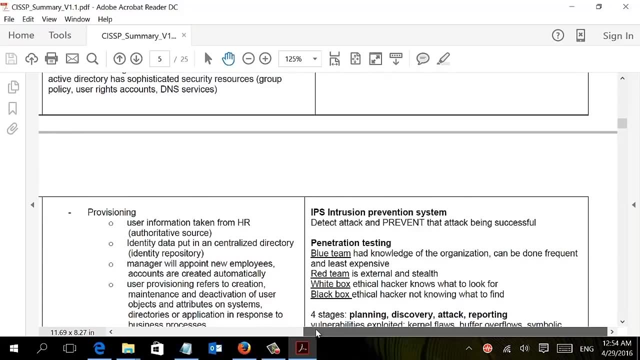 What else? Yeah, standard are sometime important, like active directory or domain services. What is the standard for that? or smart card, What is the standard for that? So the standard number? just write it down inside your CSSP notes: uh, web access management. 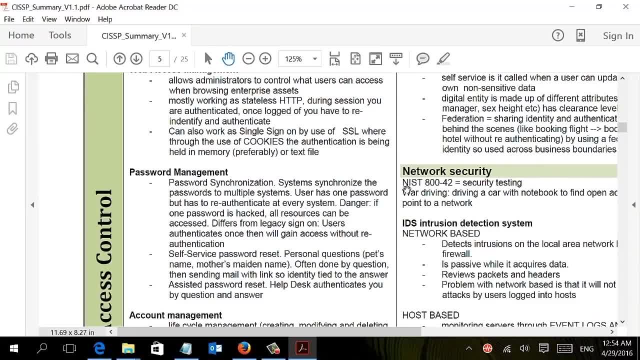 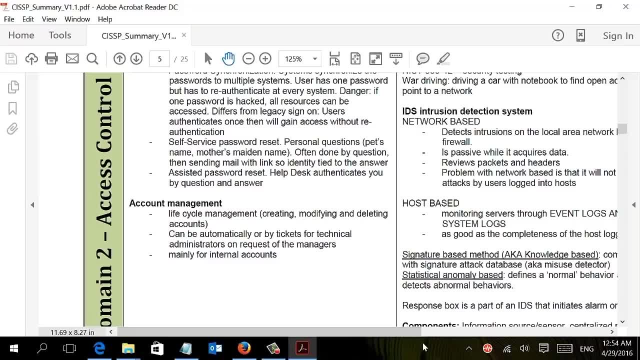 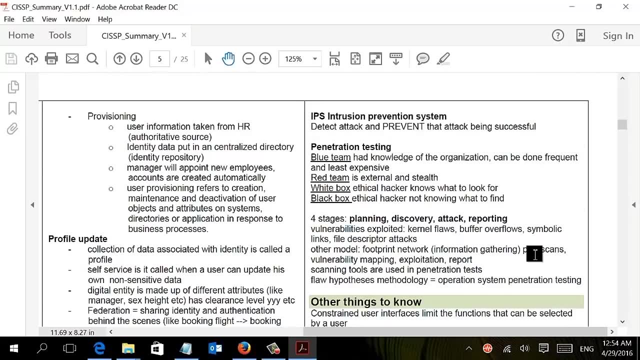 password management profile update, like also the nest publication, are important for penetration testing or any nest publication. you'll find that only you need to be aware of around nine nest publication number. Okay, Uh, in penetration testing you'll notice that there is some different name, like uh, blue team, red team, white box, black team. 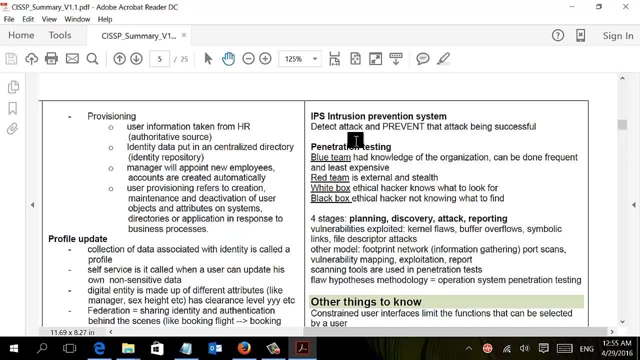 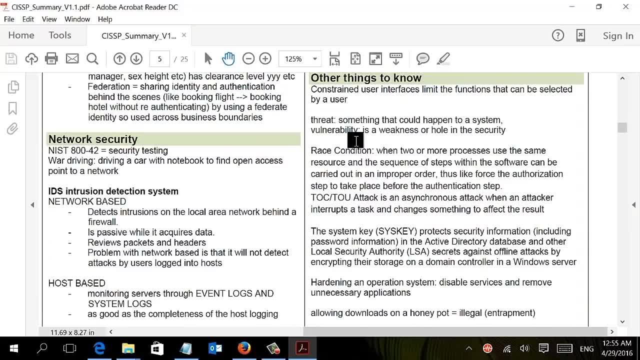 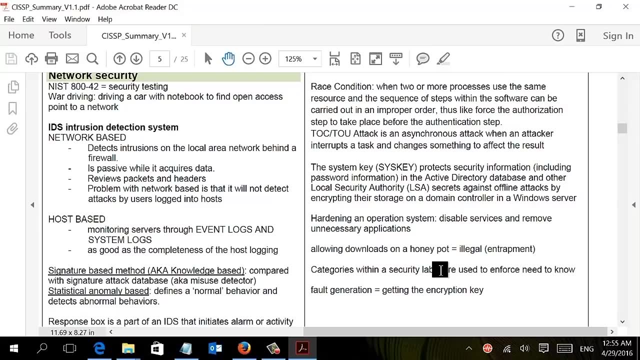 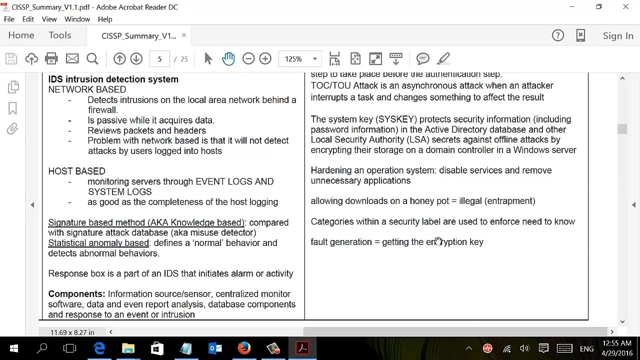 black box. so you know we explain that, that during the domain. but sometimes you'll find them under different name. so you know, just go through it. so, for instance, there is a part here regarding the salt that is used in Linux that we explained put some randomization. no, this was in cryptography. I'm sorry but it's. 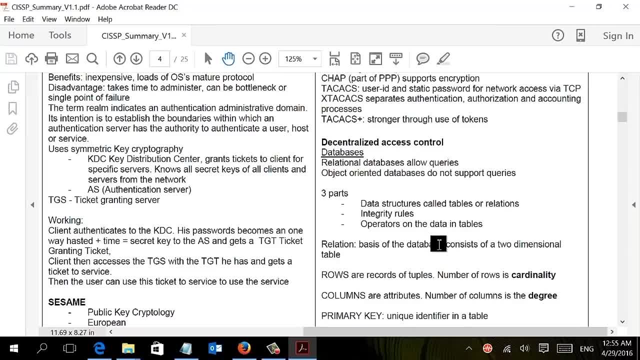 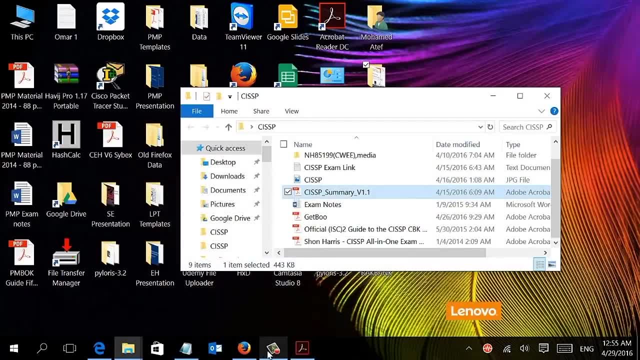 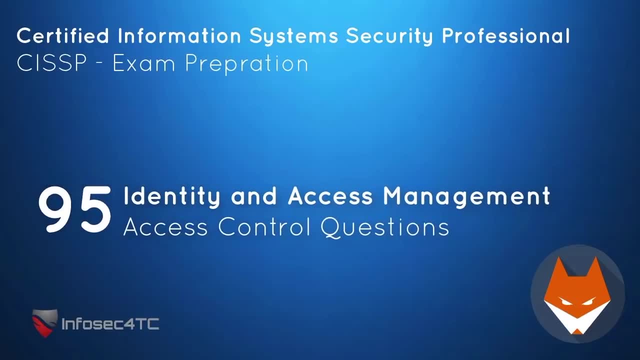 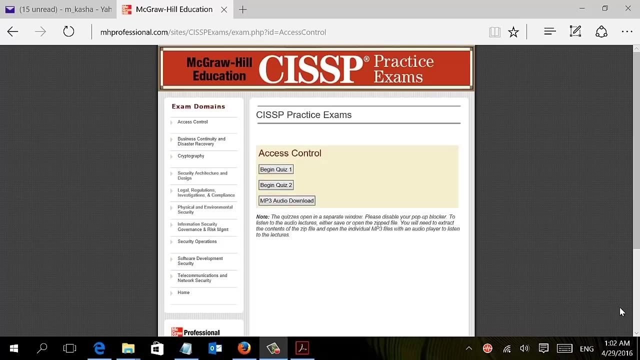 quite easy. okay, now let's go and check some question and see how exactly they look like. according to our discussion at the beginning of this course, we agree that whenever we finish a domain, you need to go to this specific website and answer all the questions that you have in the domain, and then you will be able to. 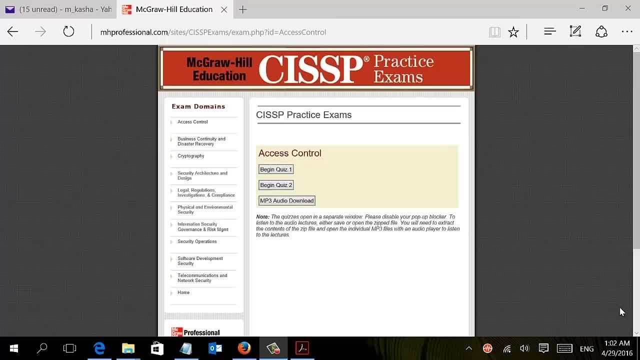 answer your questions during the course with your using help, we can also further learn about the pertinent Dark Web Covering that you can use during the course. so, and after taking the course- and I will show you how many questions that you have- some very important questions related to this domain on each. 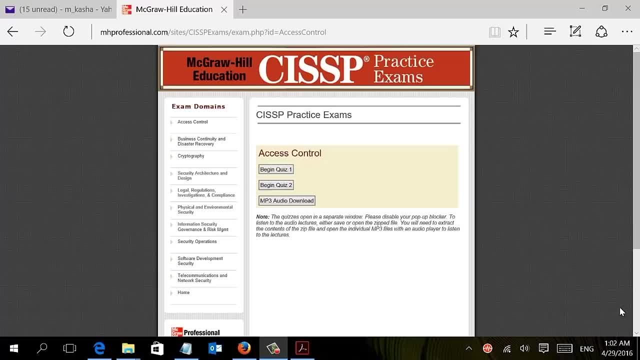 domain they have around 100 question. besides, one of the good benefit about this course, it has a full course mp3 for free so you can download it and listen to it while you are driving or while you have time. The objective before taking few questions- three, four, five questions just to see how tricky the question is‐ or how to practice the question. 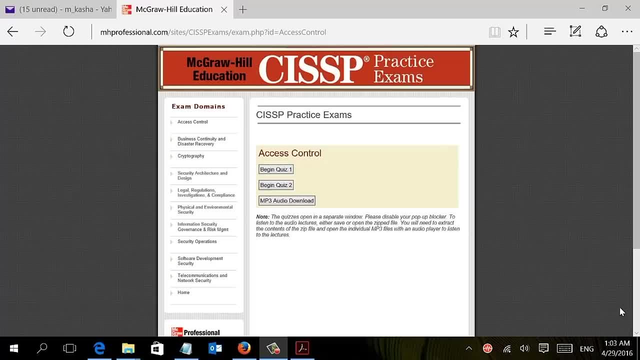 and I want to to answer as much question as you can because, as you notice on the access control, and same concept apply on the remaining of the domain that the exam is. the content is not hard, actually, just a very, very high level, but it's too much. 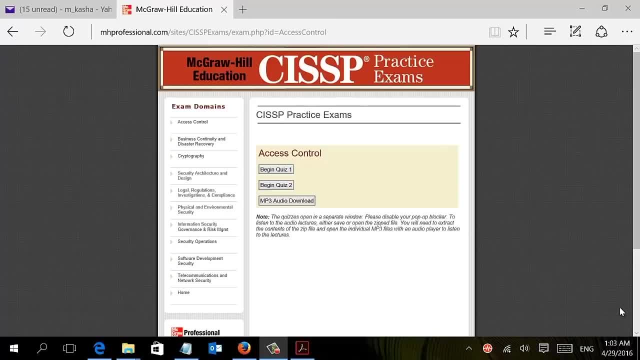 and the problem that people facing- and that's why a lot of people do not clear the exam easily- that the exam is tricky, so you need to learn how to get the tricky word inside the question and how to think the same way. I see square are thinking, so let's see some question. 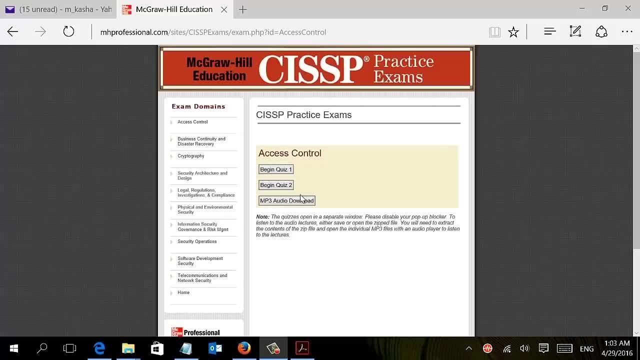 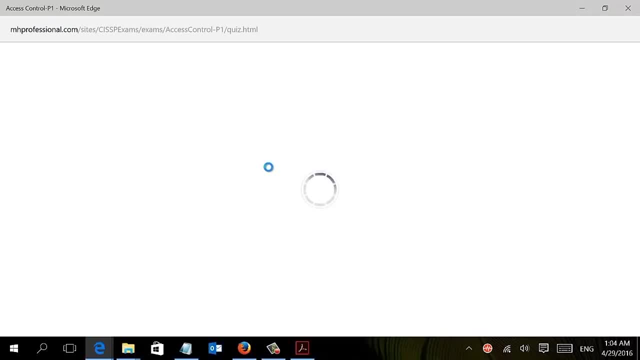 and let discuss that during the question. so I'm gonna- each domain has two questionnaires. each one has around 50 questions. so I'm gonna take like few questions and I'm gonna take like 50 questions and I'm gonna take like few couple of them or something, just to get the idea of the question. now here is 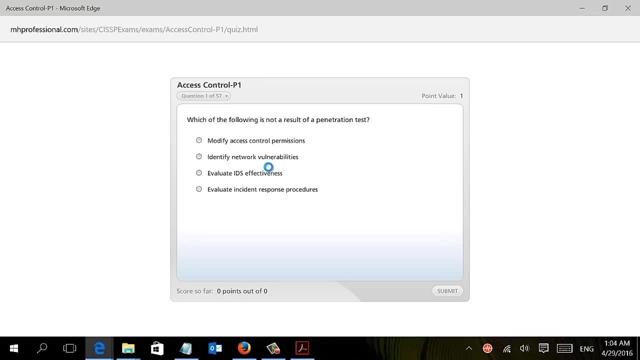 the first question. the question is saying which of the following is not a result of a penetration testing: modify access, control permission, identify network vulnerability, evaluate ideas, effectiveness or enhance incident response procedures. now, response procedures. now, if you think about it, what could be the result of? because one of the things that you should consider for the exam this 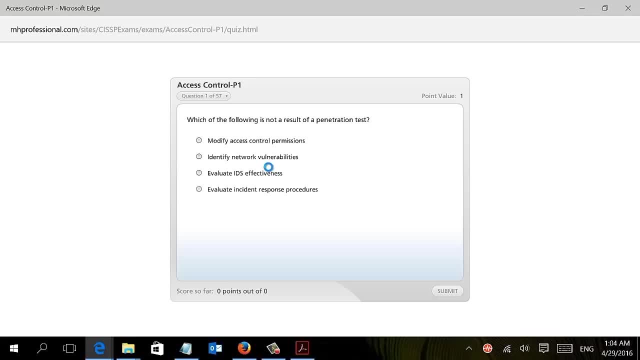 it's not a or the least, or I mean. usually they are not asking straightforward, they will ask it for the opposite. so what? which of which of the link is not a result of penetration testing? so let's take them, for instance, evaluating the incident response. this could. 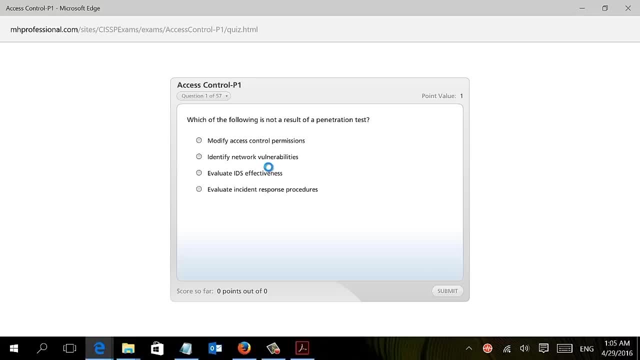 be a a result from a penetration testing. because people are doing penetration testing, they may check your incident response. is user detecting the problem and how they are reporting, evaluating the ids effectiveness? yes, i'm doing a penetration testing. i'm going to see if i'll be detected or 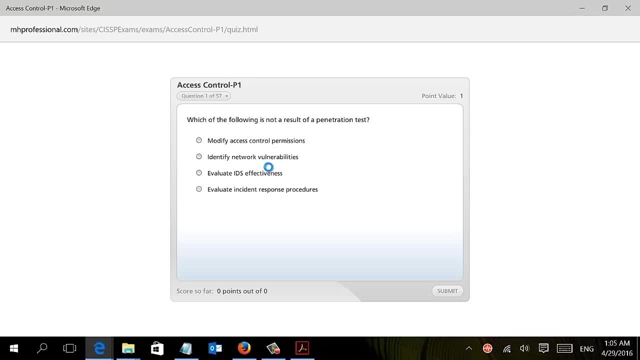 not uh identifying network vulnerability. this could be an uh result for a penetration testing. but what about the first one modifying access control permission? definitely this is not, because actually permission it's assigned based on uh need to know, for instance. so i cannot say as an output of my penetration testing, please give to this gentleman higher permission. it doesn't make any. 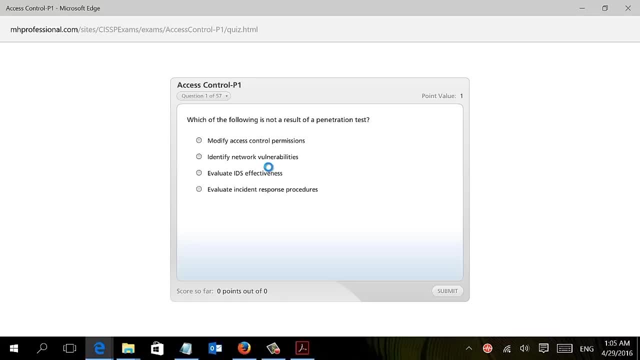 sense who should say that this should get higher or lower permission, their functional manager, or depend on their need to know? so it's not a result from the uh output. it's not an output from penetration testing. so if i select this one, i click on submit. it will give you the explanation now. it's very, very important to read the explanation in both. 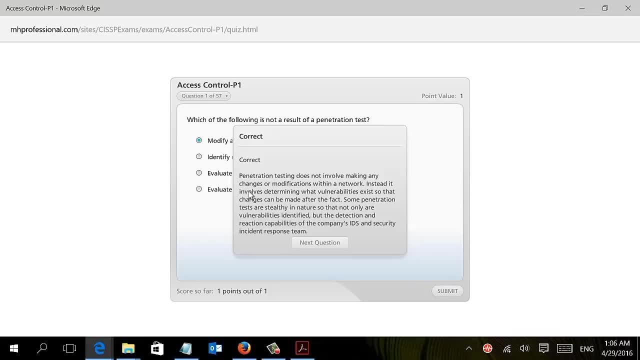 way, if you are right or if you are wrong, because if you are wrong you need to know why you are wrong, but if you are right you need to know: did you think the right way or it was just a coincidence? so explanation is extremely important, so it doesn't matter if you answer all the question wrong. 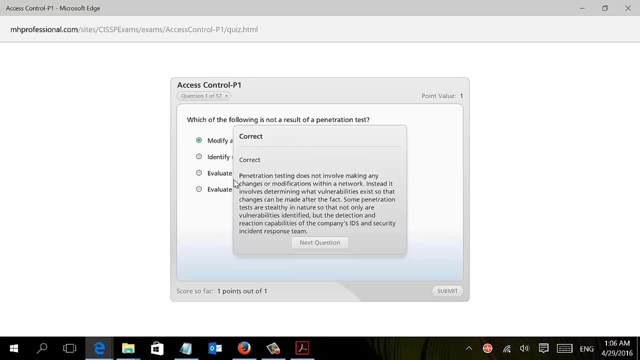 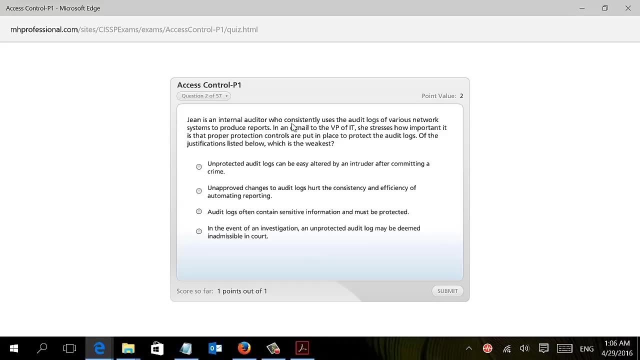 at the beginning, but you have to read the explanation because this is actually very, very important for us. this is a question about uh gene is an internet uh internal auditor who considers audit logs. she is talking to her vice president, explained to her explaining the importance of having logs. so, as you can see here what is the 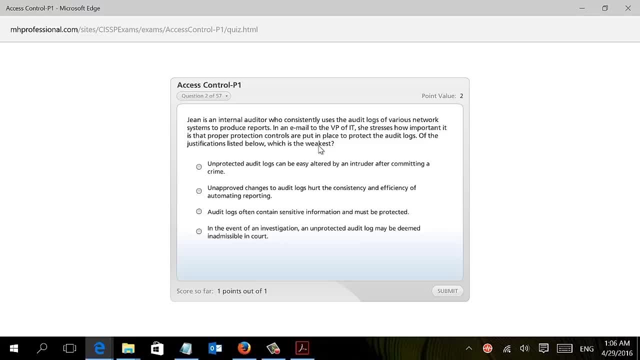 weakest reason. see, he's not asking what is the best reason to have a log, or managing the log, or weakest, but the good thing is that inside the exam they will put that in bold. what is not what? so is it because unprotected log can be easily alternative by intruders after, uh, committing a? 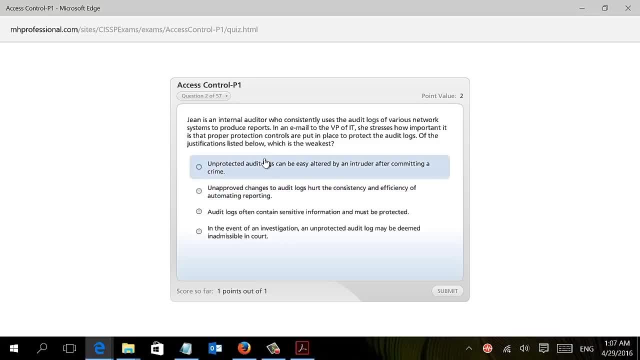 crime. no, this is important or this is true. uh, if you check anyway, because i don't spend the time reading the question- but you find that the weakest one is that the unapproved change to audit log may hurt the consternation of the audit log. because the weakest one is that the unapproved change to audit log may hurt the. 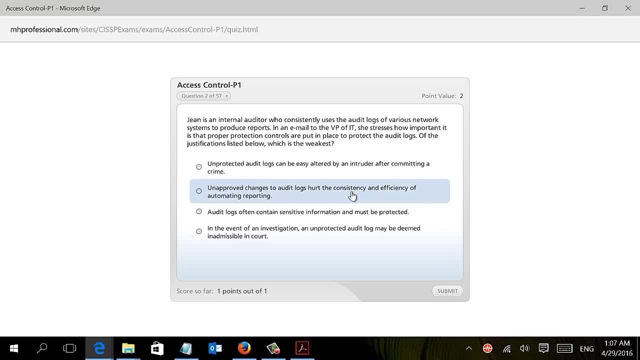 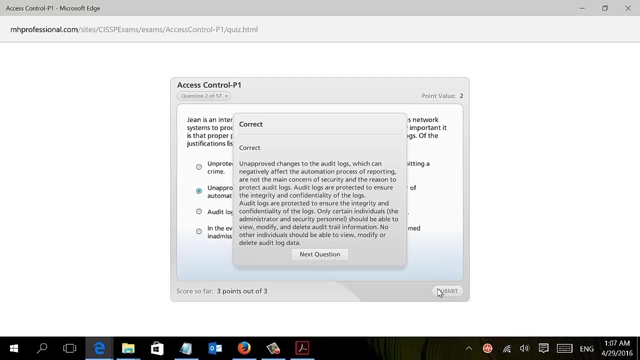 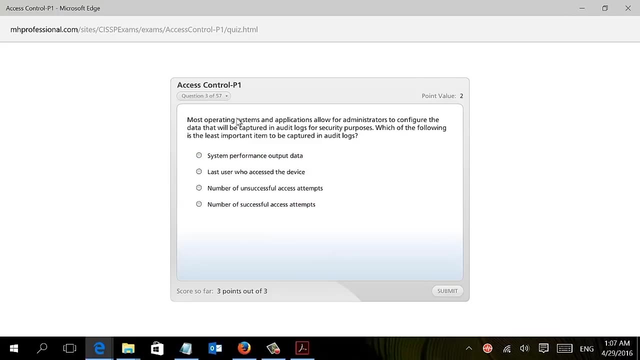 consistency of the reporting, so the report will not be looking nice or something like that. this is not a very good reason to keep log management or something like that. okay, uh, in logs, what is the most? operating system, an application, allow an administrator to configure the default. the data will be captured in an audit log or security purpose. 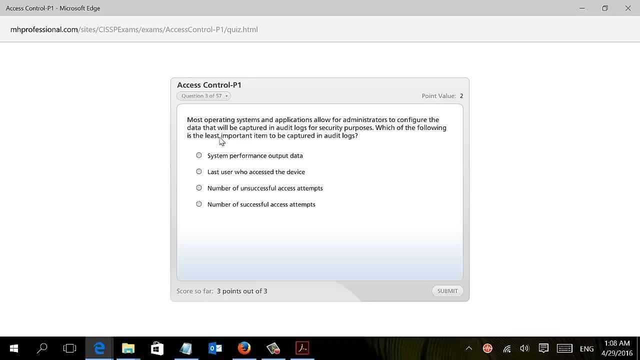 okay, so these are the two things the most important in audit log. which of the following is the least important? see, they always do that least important item to be captured. what, no, it's not very important to be captured. system performance output data laser. i'm sorry, last user. 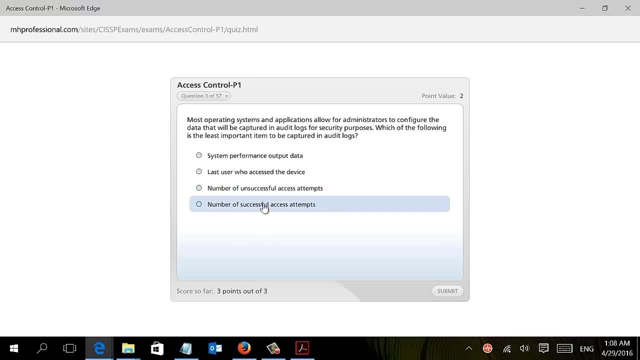 who access a device. number of unsuccessful attempt, number of successful attempts. so this is kind of confusing. i mean it it's better first to remove unsuccessful attempt is very important. last user who attempted all this is very important in case you do troubleshoot. so we are confused between system performance and number of successful. 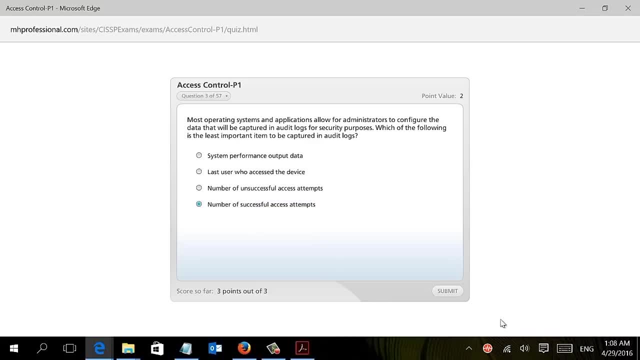 access attempt. so let's see this. one number of successful is incorrect. it's a system performance output. my opinion is that system performance output data should be captured, but i told you that it's all about ic square mentality. so you need to read the explanation. and why this? not because after a while you'll get their mentality and you'll be thinking the 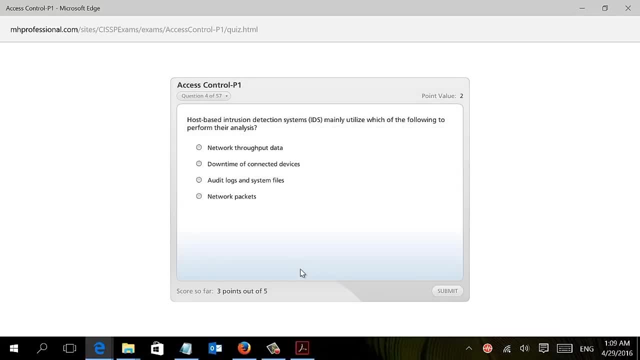 same way they are thinking: okay, host based intrusion detection system ids. we have the host based uh, maintain, utilize which of the following uh performs their analysis? i mean he's getting the information from where the network base is, getting the information from the traffic, but the host base while on your computer. 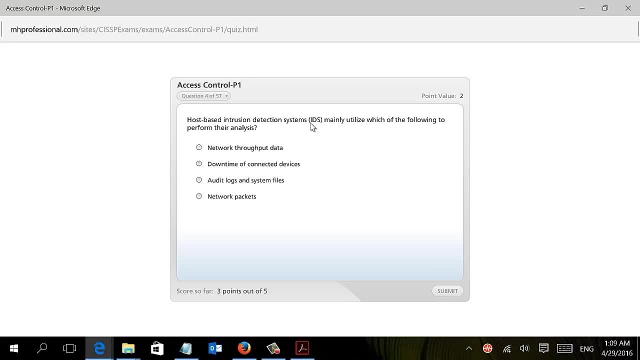 actually the host based ids are getting the information from the audit log and system file. so he's not capturing the live packet, he checking the log event viewer, he's getting the information from there and this is actually was written in the sunflower, it was quite clear, and so on. so i believe that 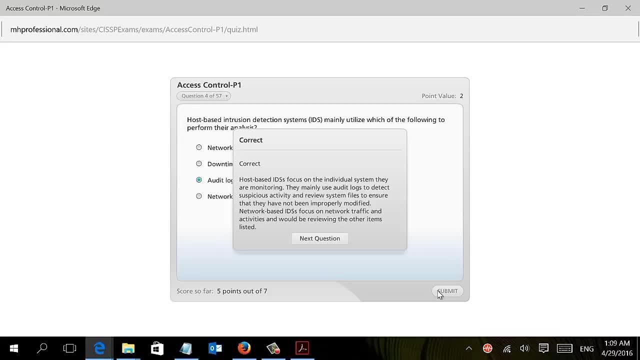 you can see how tricky question is. it's not technical, it's not hard. it just need some attention while you're answering and, most important, it need that you get the mentality of ic square, how they are thinking. you know what i mean. so this is very important and you will not be able to get that unless you. 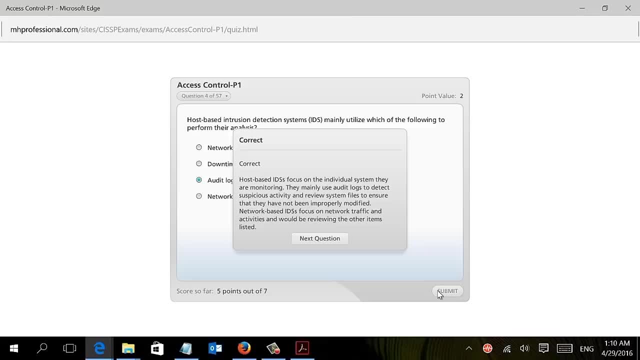 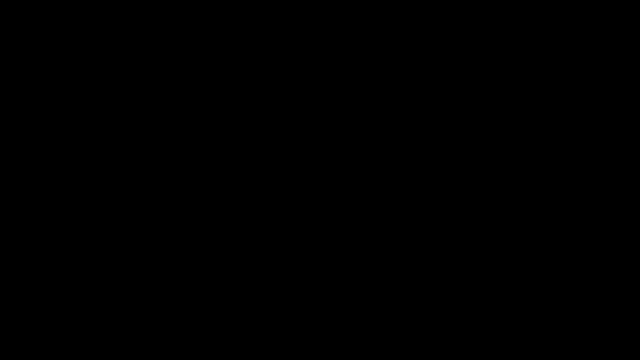 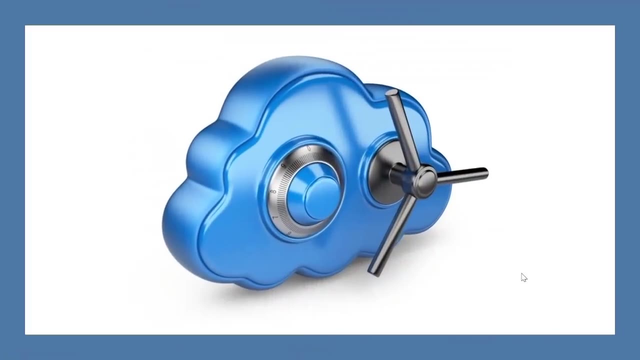 solve as much question as you can. it's not about knowledge, it's about their mentality. it's a very simple question and that's what im talking about, thank you. cloud security is very important topic in the new cissp course and the recent exam include some good amount of questions about cloud security. 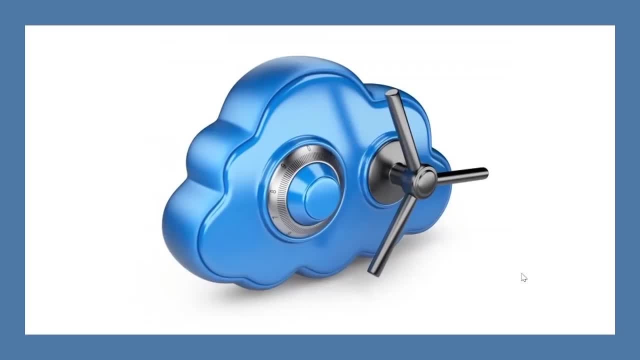 the challenge that i had while i'm preparing this course is that the topic of cloud security was divided into different domains. don't have a separate domain from for cloud security, but the topic itself was divided into the eight domain of the CISSP training and according to that one. 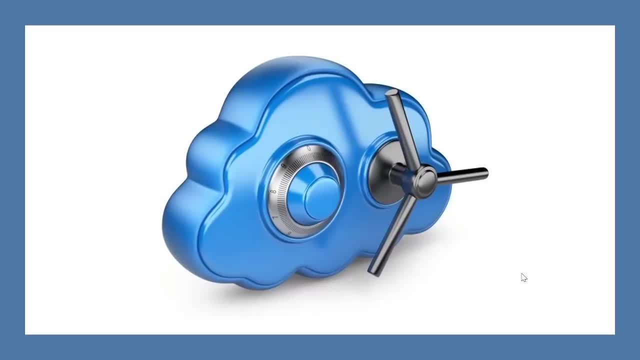 of the domain was explaining the type of cloud services. another domain was explaining the different cloud layer security. a third domain was explaining the cloud security attacks and so on and so forth, and I decided that to combine all those lectures together in one separate chapter. it's not a separate. 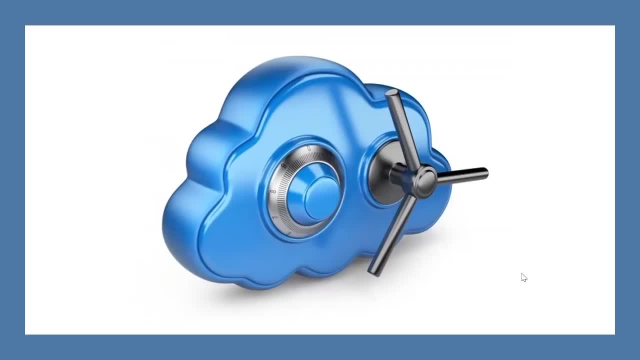 domain, but I think this is very important and by going through those lecture in this chapter about cloud security, you will feel comfortable about any question that you're going to face inside the exam related to nationsetkcom cloud security. the topics that i selected in this chapter was taking from my certified cloud. 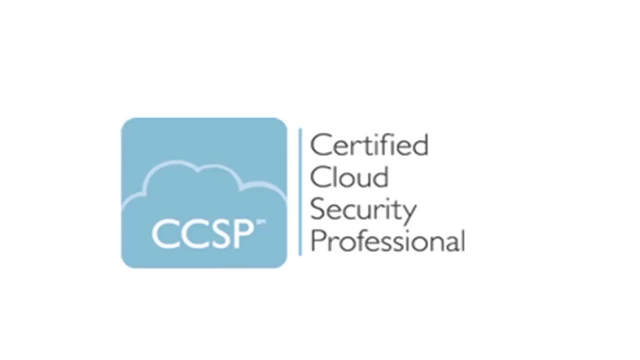 security professional from ic square. there is a lot of common topic between this course and between the cissp, so one of the additional benefit will be by going through the chapter and understand what is a cloud, the different type of cloud services and how to implement cloud security. 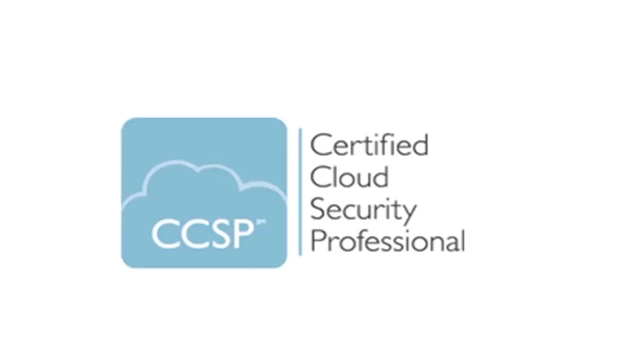 in different layers. it will be helpful for you to pass the cissp exam and in case you decided to take the ccsp after finishing the cissp, it will not take that much effort. so those lecture in this chapter was taken from the ic square ccsp. 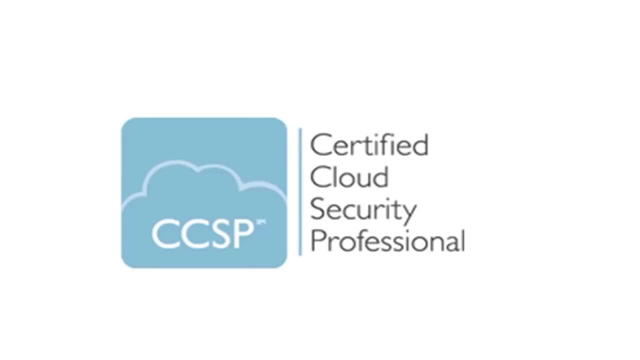 and it's important to the cissp and in the future, if you plan to take this certificate as well, those lecture will will help you to be able to pass the exam from the first item. so let's go through the different cloud security terminology and the best practice when it comes to implementing security in cloud. 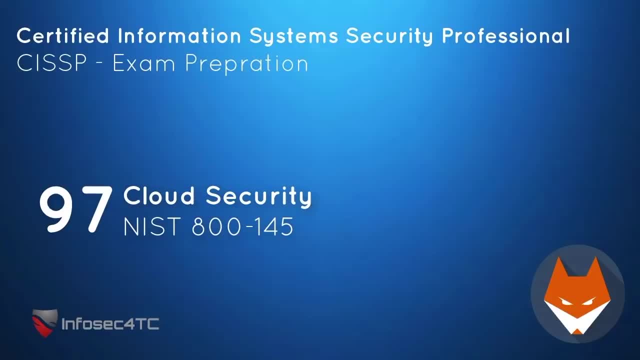 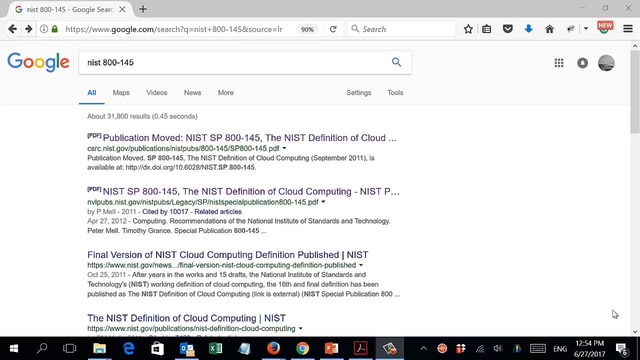 security. before starting to define different terminology related to cloud computing, i would like to refer you to a very important document that will be used during this training, which is nest special publication 800-145. this nest special publication include all the cloud computing definition that will be needed. 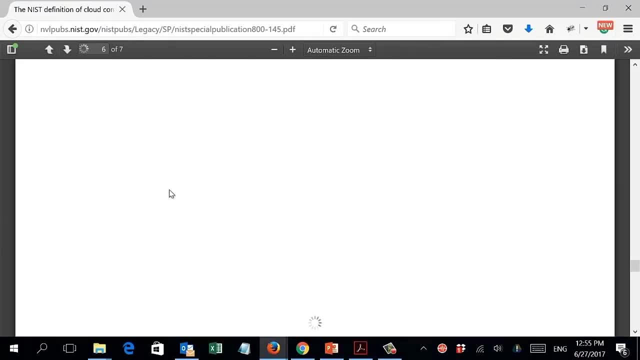 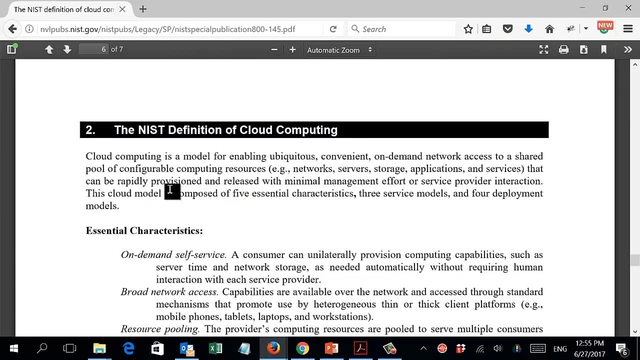 during this training. so you can download it from here, and i also going to attach the document to this lecture. in this document you will find the terminologies that you need to know before starting training. what is the definition of cloud computing? what is the computing resources, the configurable computing? 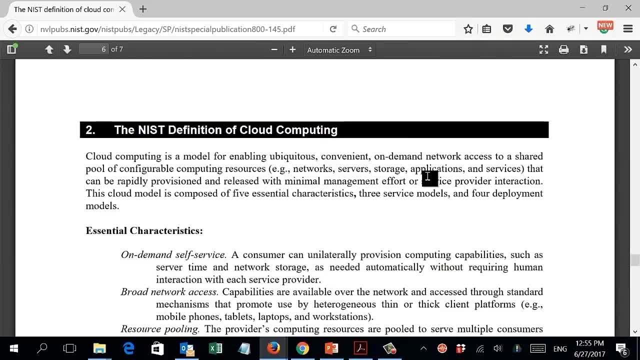 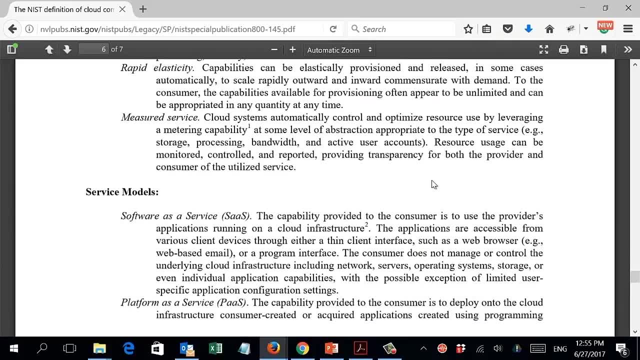 resources like a network or server or storage or application. You're going to see the terminology of service models like software as a service, or platform as a service or infrastructure as a service, and you get to learn the basics from here, but we're going to explain them in depth after a few minutes. 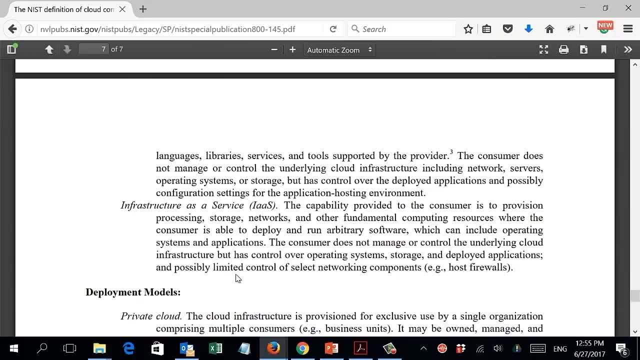 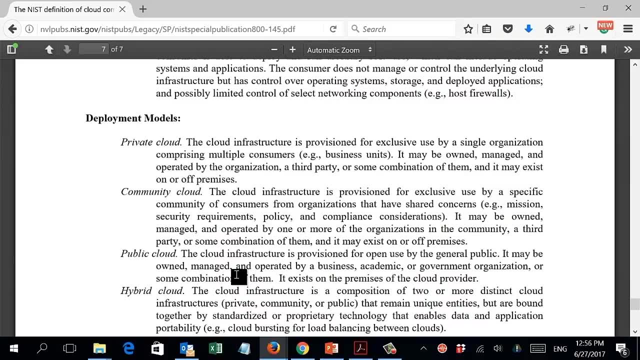 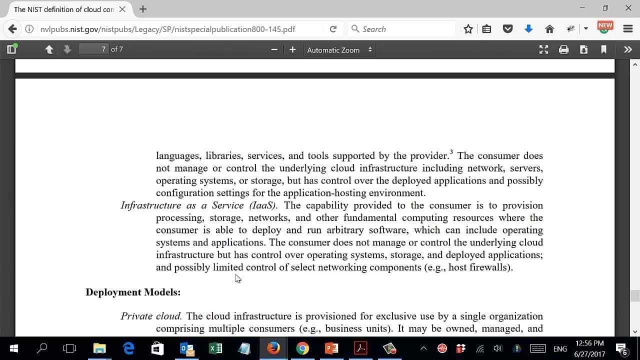 You get to know the definition of deployment models or different type of deployment models: the private cloud, the public cloud, the hybrid cloud. So our main reference in defining the major terminology related to cloud computer will be the NIST publication 800-145.. 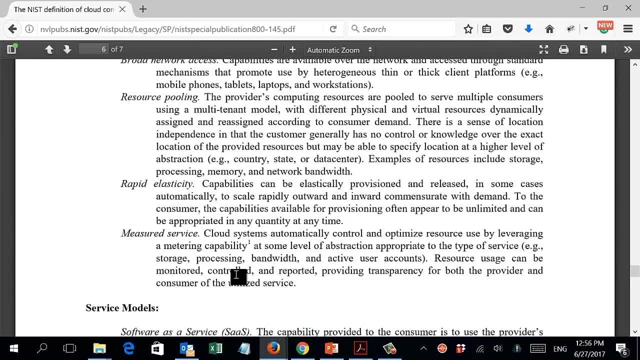 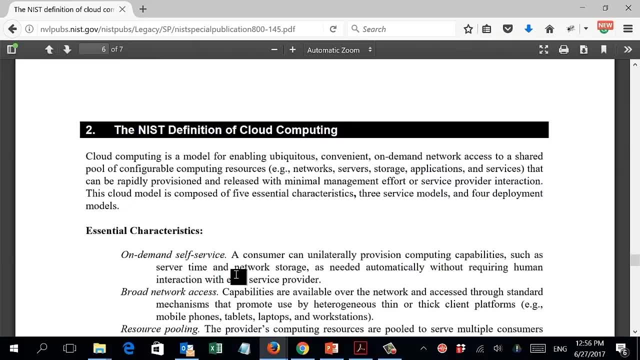 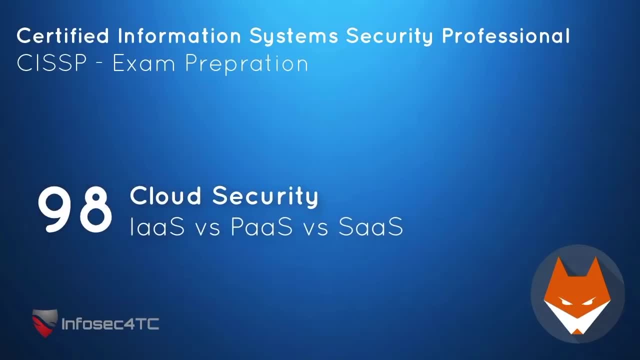 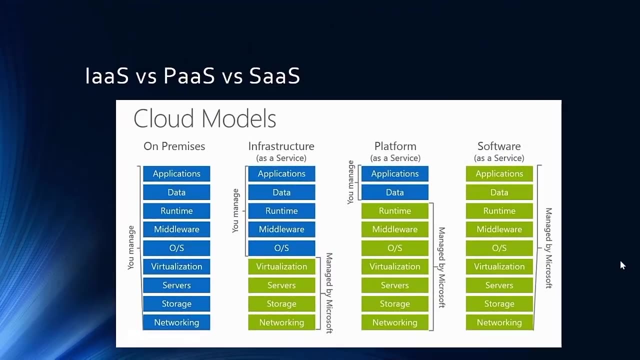 So I will suggest, before starting to download this document: This is a very small document and have a look at it. You would like to learn about those definition before starting explaining them in depth. In this lecture, we're going to talk about the different type of cloud computing services. 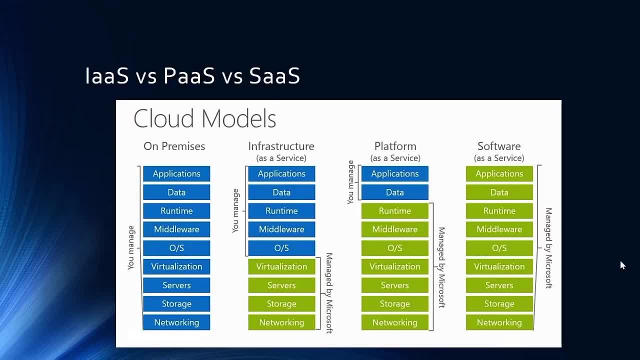 We have the infrastructure as a services, or IS. We have the platform as a service or path, and we have the software as a service, or Mina or sas. now, what is the difference between them? let's check this diagram when you manage your. 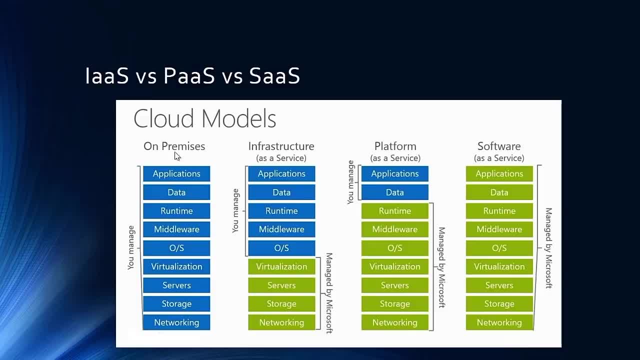 own it services on premises. you are managing the full stacks, up to the cooling and the network and the storage server. everything is managed by you. so the first cloud computing service, which is the infrastructure cloud computing, you are giving a part of those tech to be managed by an msp or a. 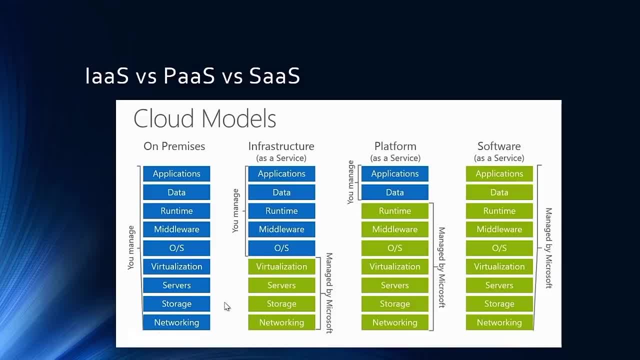 managed service provider. so the cloud computing or the msp, will manage for you the network, the storage, the server and the virtualization, but you can still manage yourself the operating system to be used, the midware, the runtime, the data, the application. so only a part in green will be managed by the msp, the platform as a service you are giving. 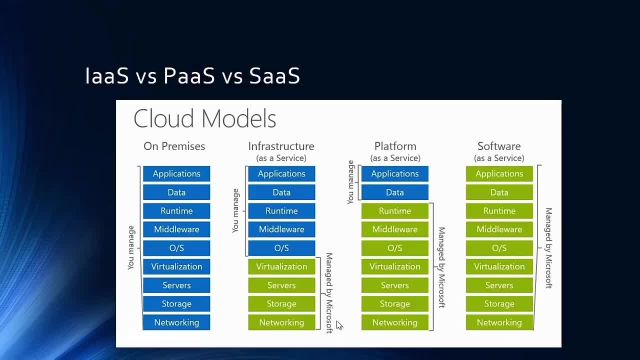 everything to be managed by the service provider except the data and the application. but everything else will be managed by the msp, while the software as a service. you are giving everything to the service provider and you just are subscribing into the service, and a good example for that is office 365. you are just subscribed to use the software. you are not managing anything. you. 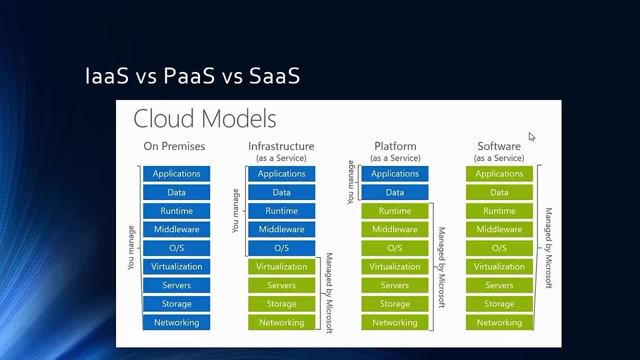 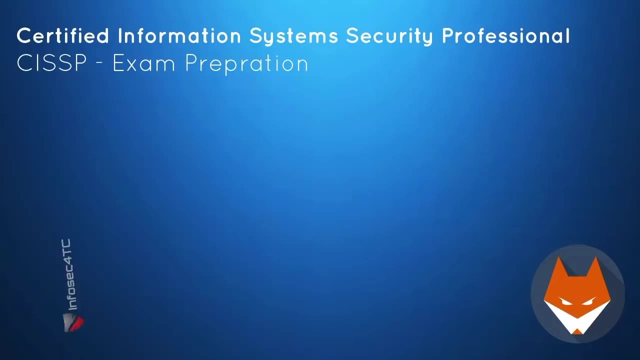 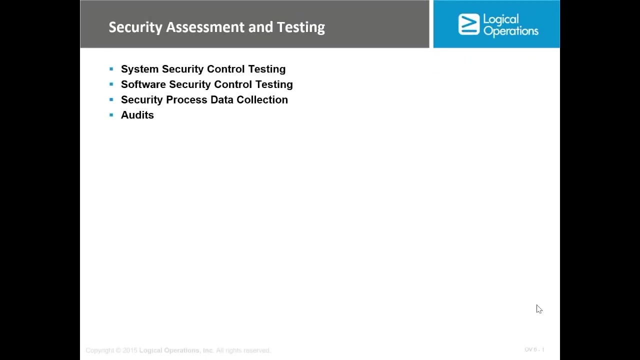 are not managing the network. you are not managing the storage, the virtualization. everything is managed by the msp. so those are the three different model of cloud computing. so let's take some realistic example about the is or pass or sas. in this domain, we will be covering security assessment and testing. this is quite important. 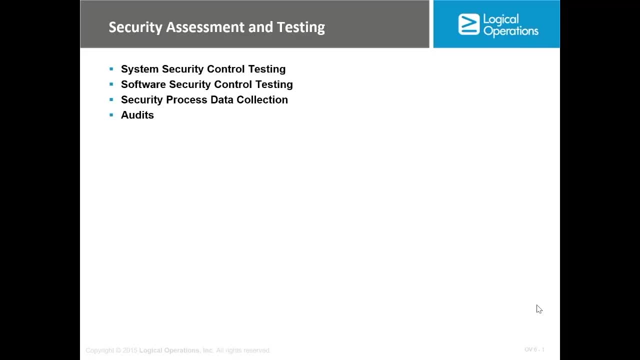 to evaluate if the security that you are implementing in your organization is it effective or not. in a sense that how can you know that the technical security implemented in your organization it's effective? how can you know that the firewall that you implemented recently in your infrastructure it's working effectively and it can prevent any kind of attacks? 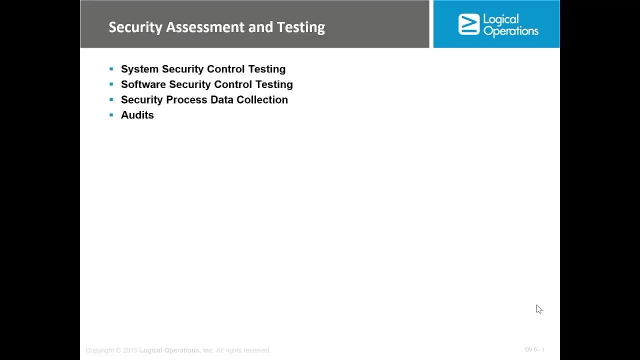 how can you know that the policy and procedures that you are using as a part of the administrative security? it's an effective policy. so security, which is quite important, it's it's not just to implement technical equipment and administrative security, but also you need to evaluate their. 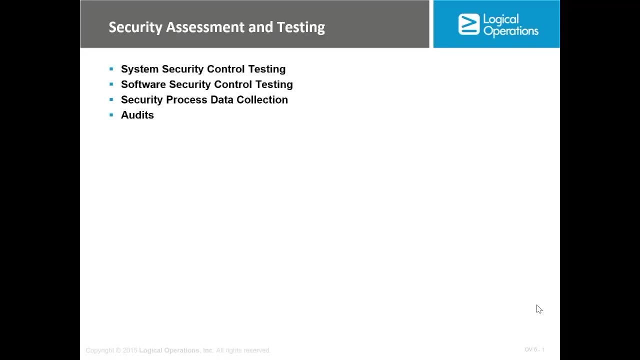 effectiveness. that's why- and this is quite important- most of the security framework like iso 27001 or pcidss or hipaa, most of the information security framework that we are using, is requesting to do a vulnerability assessment and penetration testing once per year. I'm not sure about it's once per year or. 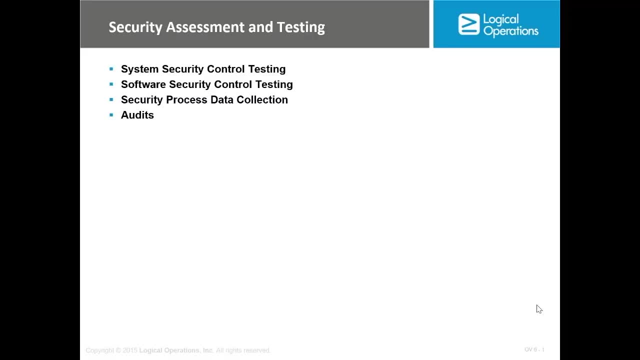 twice per year, but it has to be done frequently. what is the purpose of doing it? why are we doing a vulnerability assessment or a security or penetration testing frequently? just to evaluate that money and effort we spent on security. it's enough and it's effective as well. so in this domain, we will be talking. 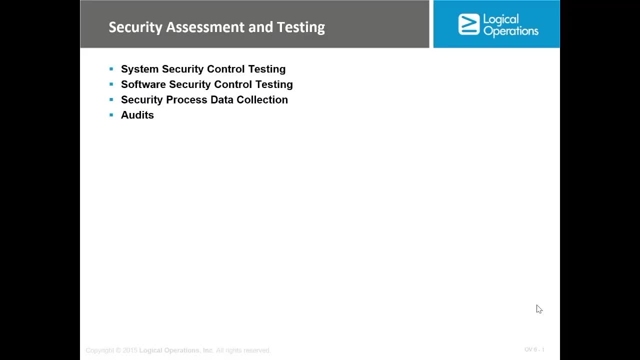 about the different way for evaluating the security, or security assessment and testing. we're going to talk about vulnerability assessment and what is difference between vulnerability assessment and penetration testing. we're going to talk about auditing. we're going to talk about administrative and technical security evaluation, but instead of keeping this domain dry, just 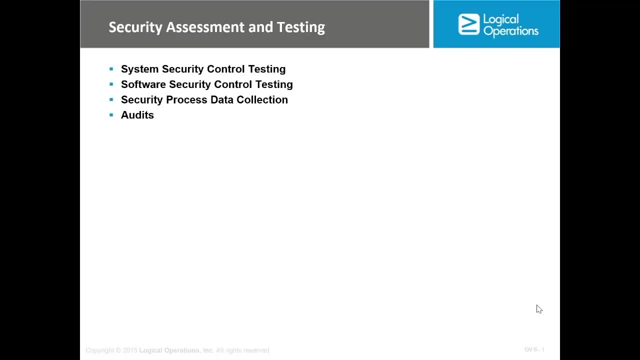 by explaining the concept. I will try to show you some of the tools as well, so you will be knowing, for instance, if you need to do a vulnerability assessment using one of the tools, how can you do that and what will be the output of that. we will discuss topics related to the output for 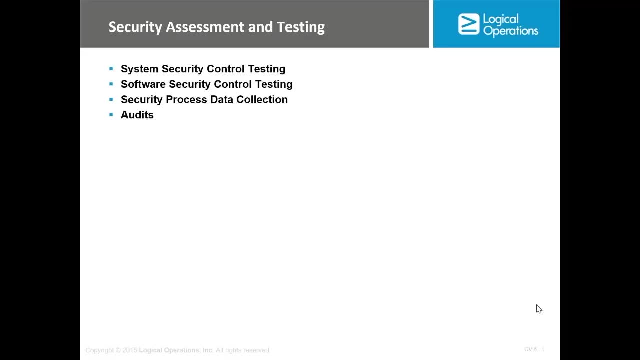 instance, one of the very important topic covered here and in the next domain will be the patch management, which usually it's an output for a vulnerability assessment, and I'm going to explain to you what is a patch management in the first place. so here we're going to talk about the system. 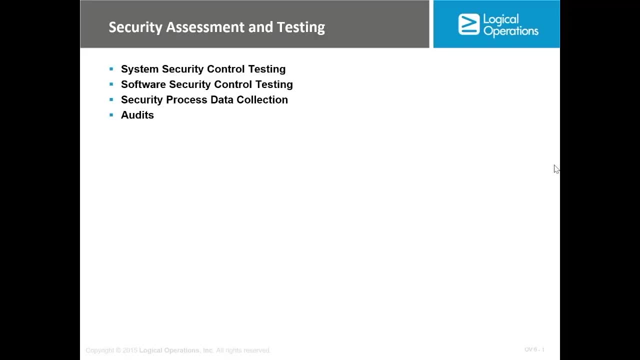 security control testing. software security control testing, where we'll be talking about code reviewing and everything related to software software security, because software also right now is considered one of the weakness in any system. we're going to talk about secure process data collection and we're going to talk about audit. so let's start with the software security control testing. 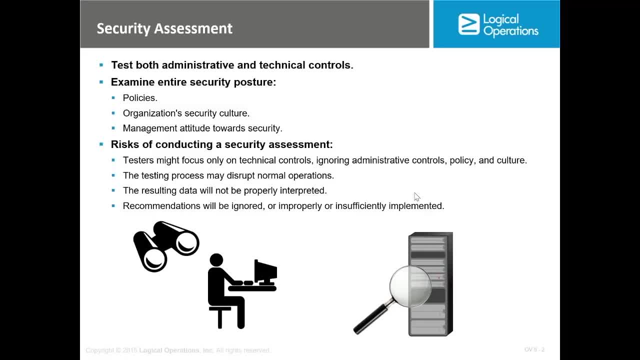 let's start with the security assessment. as we agree, before we start in this domain that we need to own, we need to test both administrative and technical control. so it's not enough to test the technical control if I'm doing a penetration testing or a vulnerability assessment. 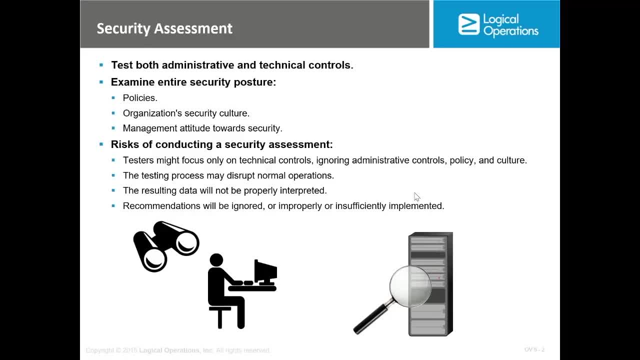 most probably. I'm focusing about the technical control checking. can I bypass the firewall? can I bypass the antivirus? can I bypass the technical security control? and I'm going to test both administrative and technical control. this will not be enough, because what if you have a strong technical control but you don't have an administrative control, which is related? 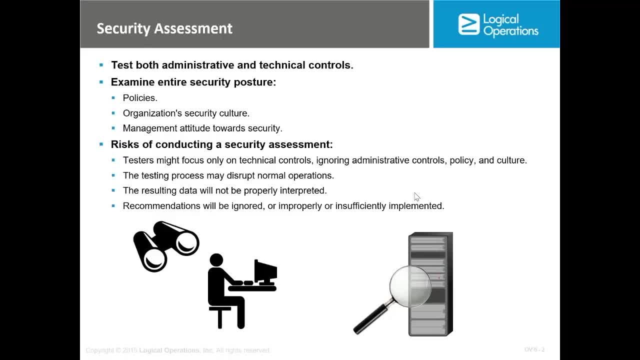 to the policy and procedures. so I'm going to show you how to test both of them, technical and administrative. then you need to examine the entire security posture in ways that we need to examine the policies, organization security, the management altitude to security. are they committed to security or not? so it's a full testing process. 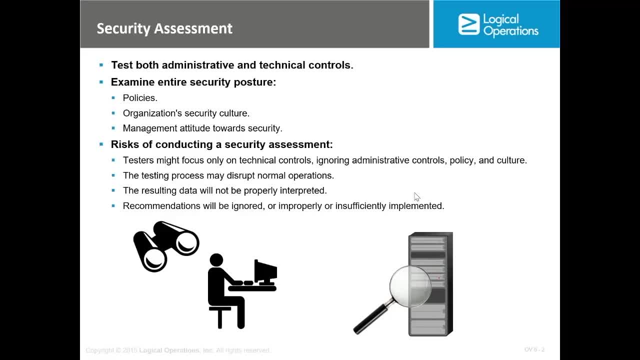 not just a part of it. but before doing that you need to have some consideration, some risk need to be considered before doing a security assessment. first, we need to make sure that if we plan to take or to make a security assessment, it should cover everything: the technical control, administrative control, policy and procedure management commitment. 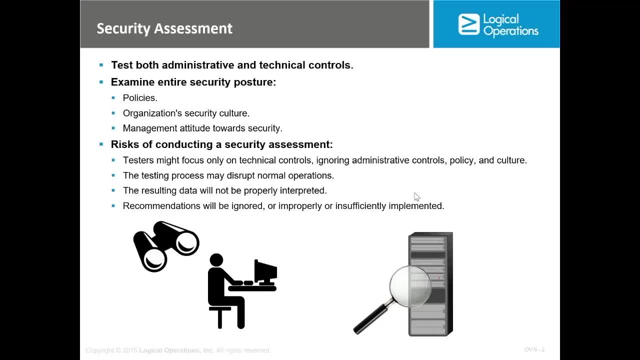 so it need to cover everything related to risk management. then you need to make sure that the testing that you are you are doing will not disturb any production environment. so if you are doing a vulnerability assessment, there is a process for doing it. you should inform the proper team first you. 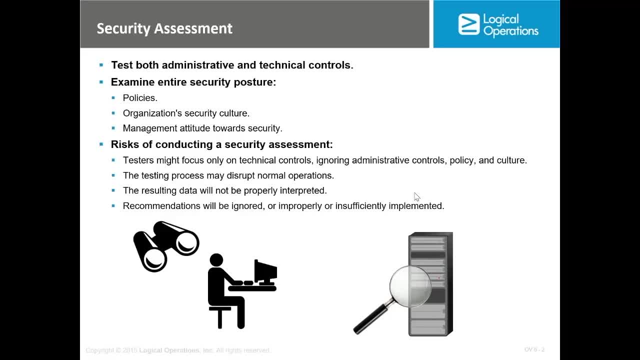 should send them what will be tested, and some of the tests need to be done after working hour. this is quite important. it's not that you do the test anytime, because in some environment- that production environment- if it get affected in any way, it will affect their business and reputation. so it's quite important to consider. 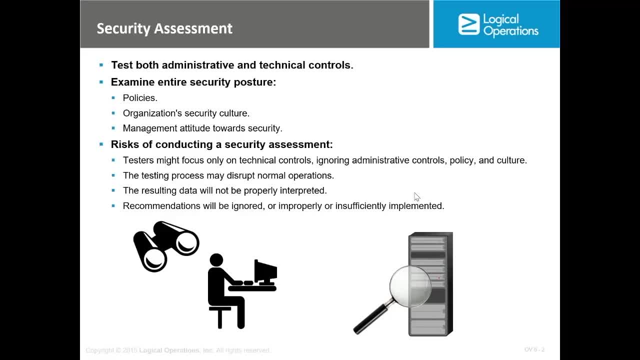 what disturb, what disturb- this disturb may happen due to this testing, then we need to. the result of the testing need to be managed and actually, if you are following any framework, when they audit will come to you, they will check the result of the testing. this will not be enough. so if you are ISO 27001 certified, and because ISO is, 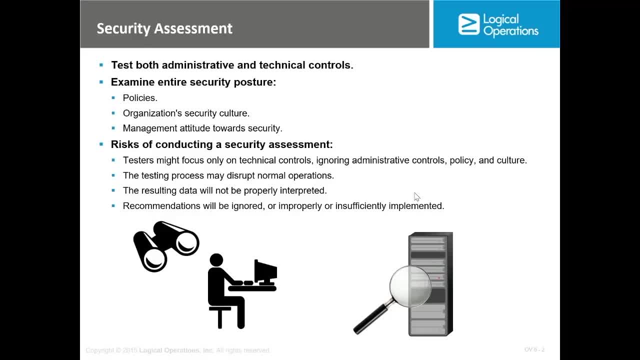 requesting that you should do a vulnerability assessment and penetration testing. frequently, one of the questions that you may get from the auditor is to see the report from the this testing, the vulnerability assessment or penetration testing report. so it's not enough to showing him the report by time or you did the security assessment by time, but also we 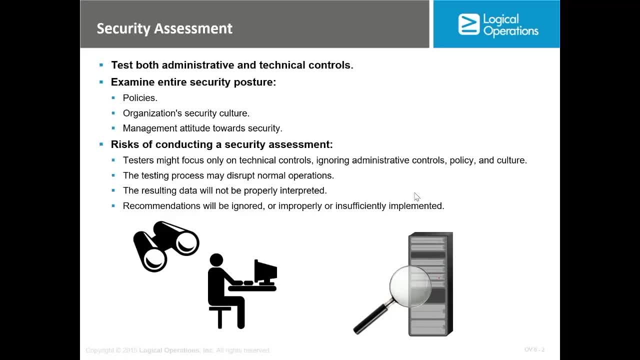 need to show the auditor what task or what action has been taking to close those finding, and this will be explained more in this domain. so testing is a full cycle process. we will be talking about the different way for testing, the full process for test, and I will guide you with some of the tools that we are using. 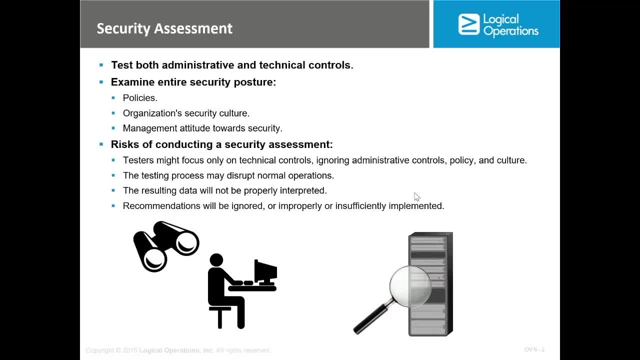 realistically in our environment. and also I'm going to share with you some of the template for the result of the testing because, as I was saying, it's not just, it's not about just conducting the test, but it's quite important to remediate or to close the finding. this is the 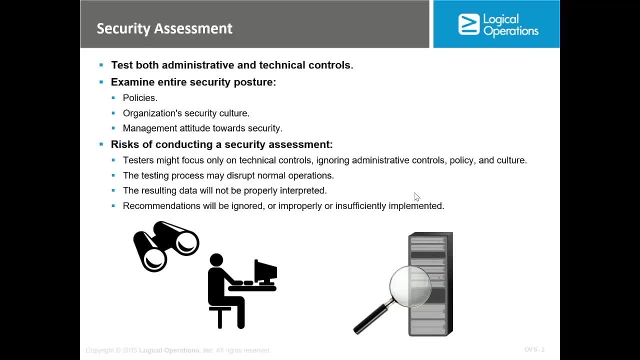 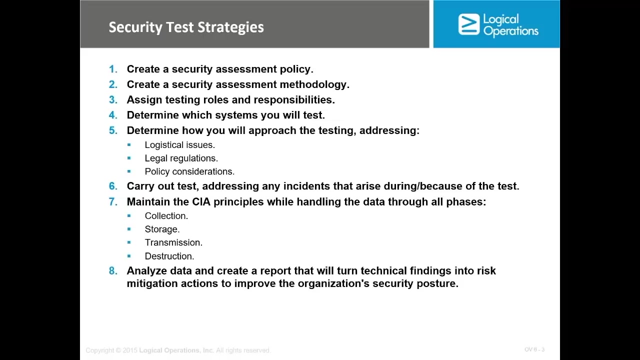 important thing part- and sometimes the finding is technical and sometimes is not, so this is quite important- there is conducting to the security assessment and especially the point related to not affecting the operational work. I'm going to show you how it's usually done in real world in this lecture: the testing. 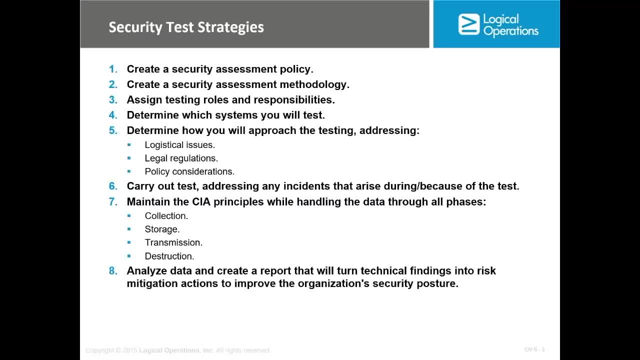 itself should be running according to a strategy. it's not like let you know, you gather with your team and you said, okay, let's do a testing tomorrow. it shouldn't be done this way. the proper way is to have a plan that we are doing a vulnerability assessment testing, for instance, twice per year. 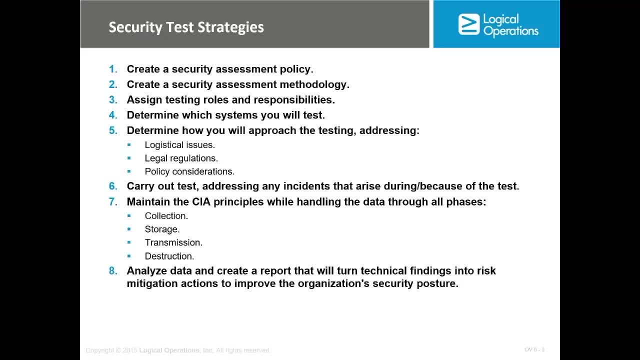 the first quarter and the second, the first six months and then the second, or maybe each quarter of the year. so it should be done according to a policy and then you should write a report and then you should send it to the concerned team to work on those solving. now you will see that this could be in. 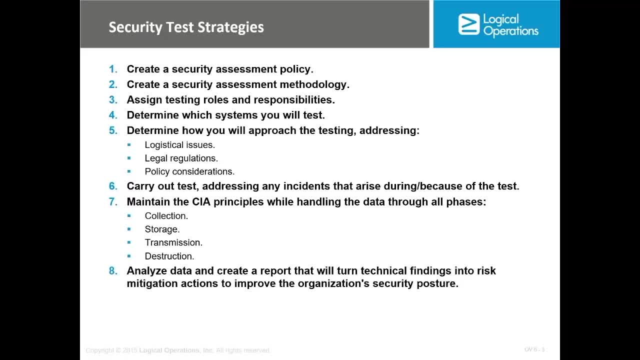 a different way. i mean, if you are doing that, for instance, for your developer team, if you have a developer team in-house, it will be done in a different way. well, if you are doing that for the technical team, also, there is some consideration for doing it. but in general it should be done. 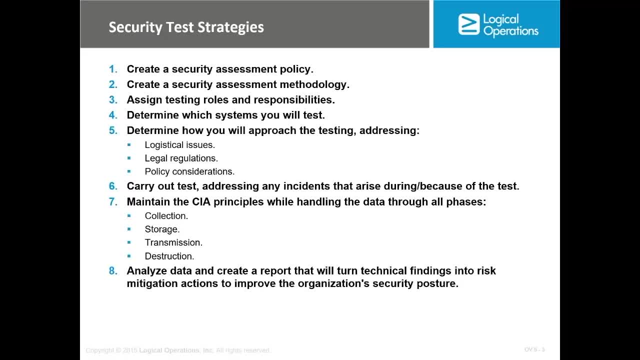 according to a security assessment policy. you should create a security assessment methodology- and this will be showing in this lecture- assigning testing role and responsibility. who is responsible for what? determine which system will be test, and this is important. if you have an infrastructure, what exactly will be testing? i'll be testing the critical one, if you. 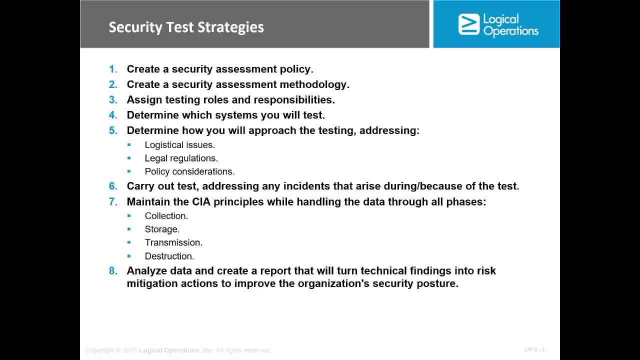 have a server and this server is a critical server to my business. this need to be tested because it, if it get compromised or crashed for any reason, it will affect my business. so, when it comes to the priority, i will not be able to test everything in my organization, but i need to identify the systems that will be testing according to. 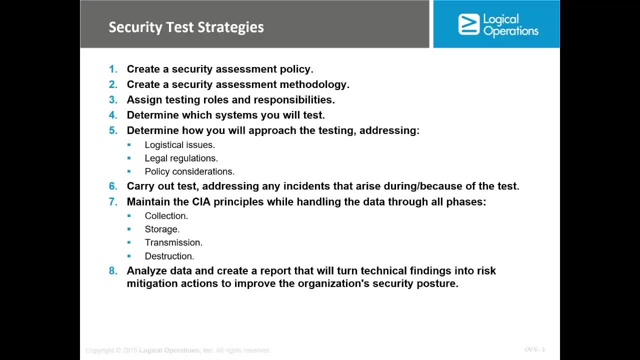 their criticality, then you need to determine how you will approach the testing, addressing the logistic issue, the legal regulation, the policy consideration and also- this will be clarified with some example later on- carry out testing, addressing any incidents that arise during or because of the testing. what if something went wrong? you are trying testing a web application and it crashed. 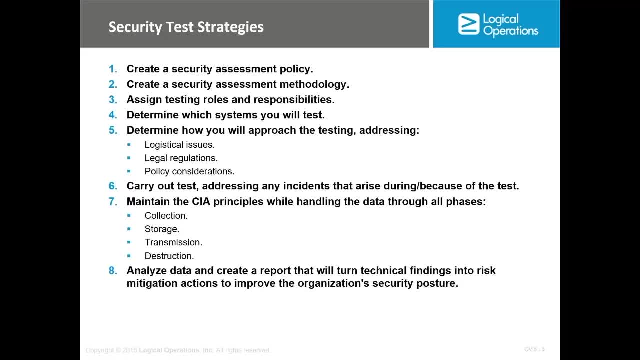 or you are trying to test like a production environment and a problem happened. do you have a rollback plan? how long it will take you to retrieve the system? you should have a plan for that. maintain the cia principle: confidentiality, integrity and availability. analyze data and create report. that will turn technical finding into a risk. 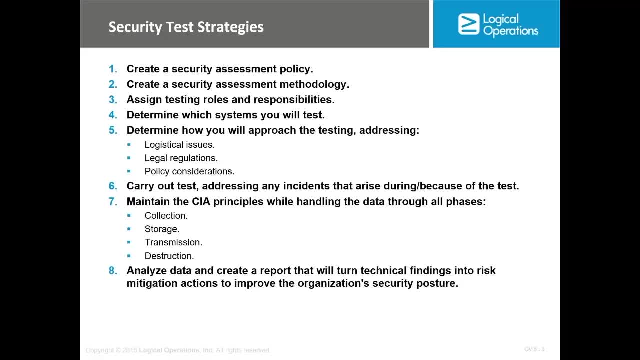 don't forget that the report that you will submit as a result of you from your testing, it will be sent to different entity, including management. you should not keep it very technical report because it will not be easy to understand, but you need to translate the technical part to risk we have this problem that may cause that and we already covered. 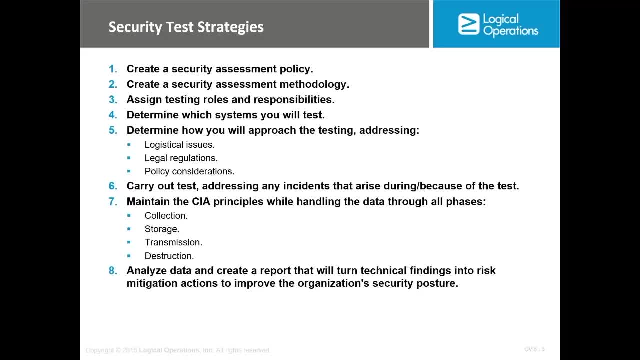 the risk in the first domain. so it's quite important to consider the risk. actually, it's not just important, it's a requirement, it's a government requirement, it's a regulation required. you have to test your security. so let's start and see the different way for testing it. and, as i told, 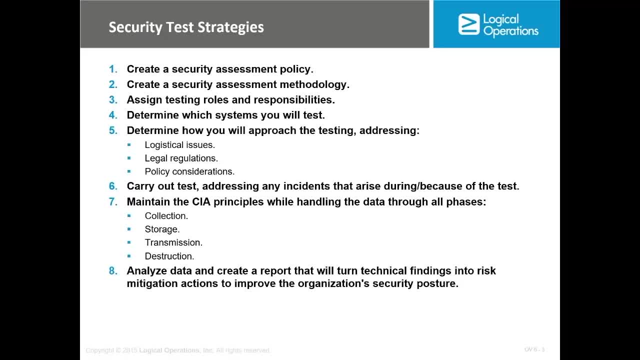 you. i'm going to share a lot of templates and i'm going to share a lot of methodology, and i'm going to share a lot of information and some demonstration, just to prove the concept, of course, that the demonstration will not be a part of the exam, but at least you'll be knowing what we are doing and 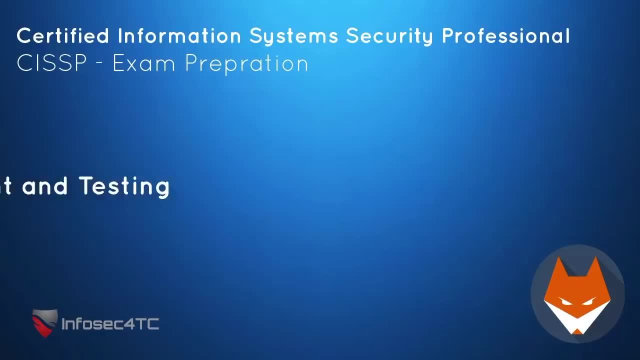 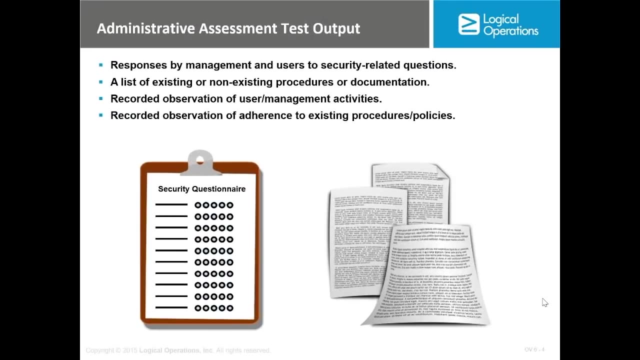 what the result will be getting, and so on. so what should be the output of a security assessment testing? as we mentioned in the previous lecture, we have two different type of security assessment: admission and the second type of security assessment is administrative and technical security system. in the administrative assessment, the output should: 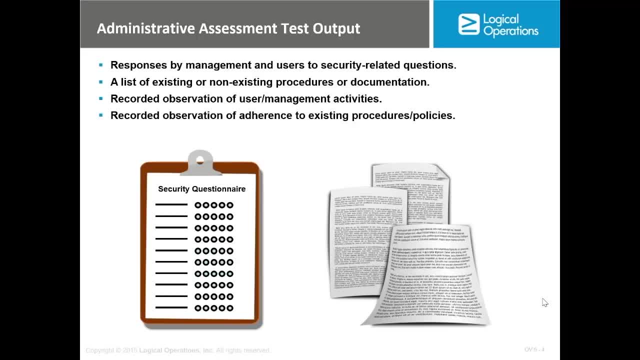 be something like the responses by management and user to security related questions. it could be the list of existing and non-existing procedures or documentation. what documentation is not there? do you have a procedures for access control? do you have a procedures for encryption? do you have a procedure? so you need to check. 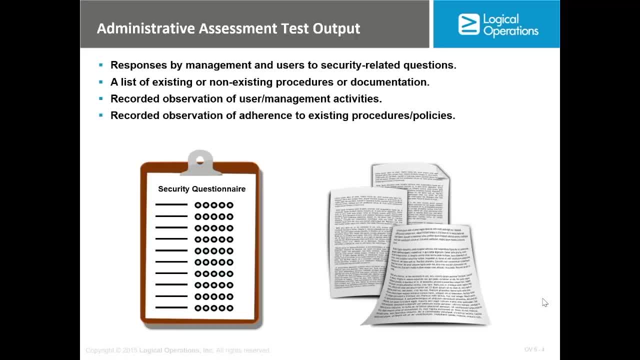 what procedures and other documentation are available and not available. could be the to record the observation of user and management activity. could be to record the observation of existing procedures and policy. so this could be some of the administrative assessment test output and, as i told you, i'm going to show you some of those documents as a templates- of course, not real. 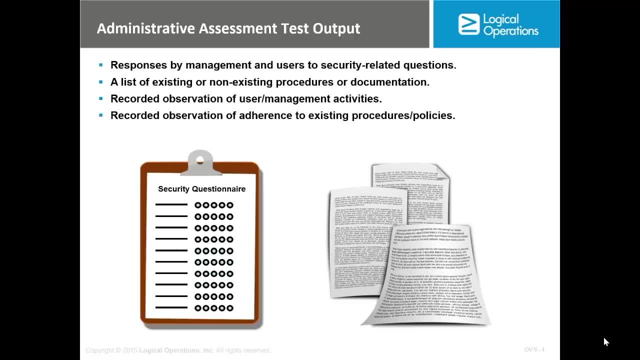 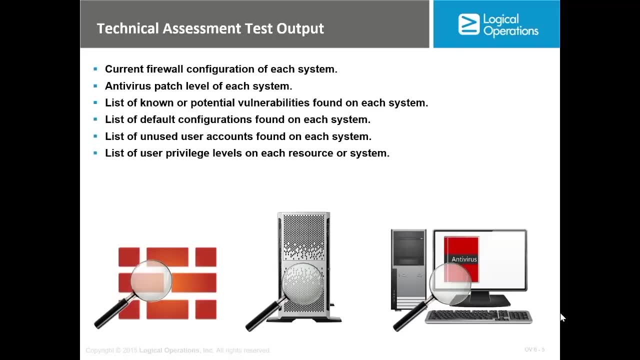 information. but i'm going to show you a sample of the assessment- administrative assessment- while for technical assessment it could be the current firewall configuration of each system. a lot of system will have a firewall, but we do not review the firewall from time to time. and maybe we did assign the rules, but we 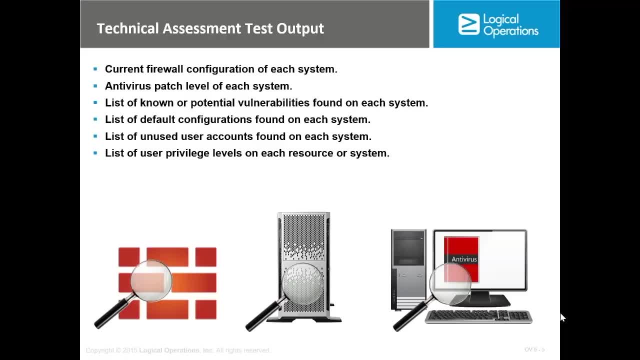 are not using it anymore, so the firewall need to be reviewed frequently. it's quite important antivirus patch management or patch level of each system. are you updating your antivirus? because you know all the antivirus need to be updated and it need to be done through a management system, not randomly on each machine. list of known potential. 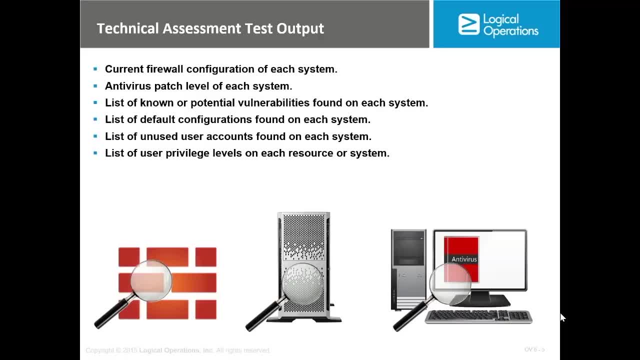 vulnerability found on each system, and this is mainly the vulnerability assessments that we're going to see later on in this course, i'm going to show you a tool that will identify the vulnerability and will rank them according to their criticality. is this vulnerability very critical or less critical or minimum critical? 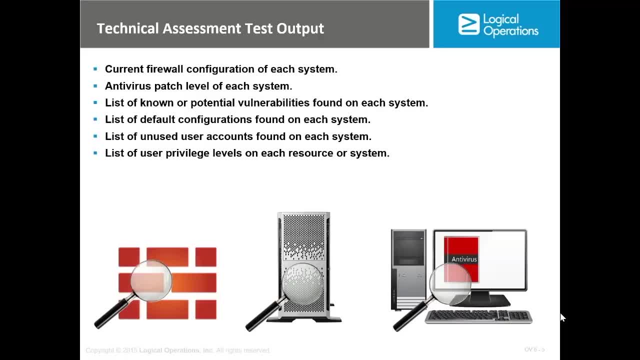 and if you can relate this point to the due diligence and do care that we spoke about in the first domain, that you as an security officer need to be aware of the vulnerability on your system and you can only be aware of that if you are doing frequently vulnerability assessment. 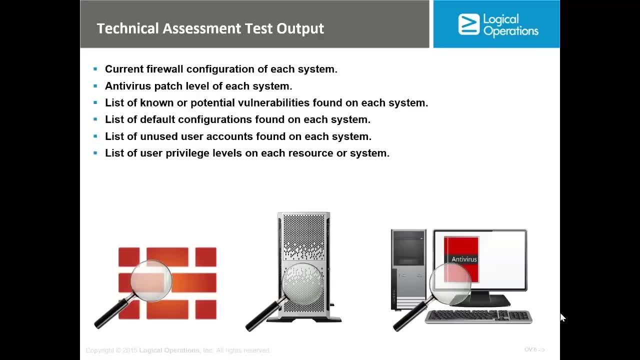 list of default configuration of each system. also, we're going to see that a lot of system will have a default configuration, a default username and password, a default setting- so you're need to make sure that you change the default configuration. a very small example will be the. 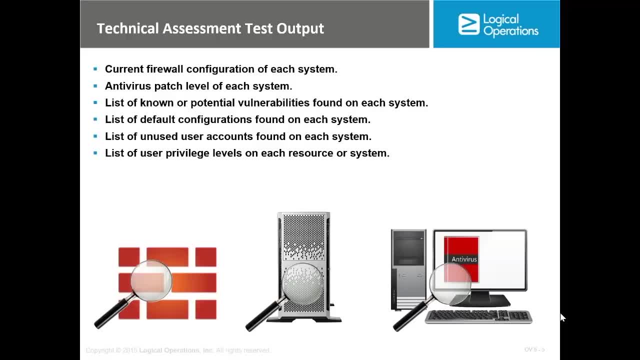 administrative account on each system. do you disable this account by default, the default? if you are using some equipment, router or switches, most of them has default account and you just can go to defaultpasswordcom, wwwdefaultpasswordcom, and it will give you a list of all the default. 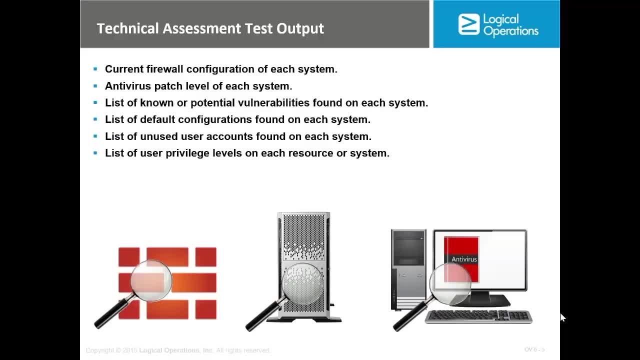 account in different system. so you need to identify the default configuration and default account and you can also check the default configuration in the default configuration and default configuration. now you can see that you have a list of unused user account found found on each system. now you as an organization, you have people coming and then people leaving the company and people joining for 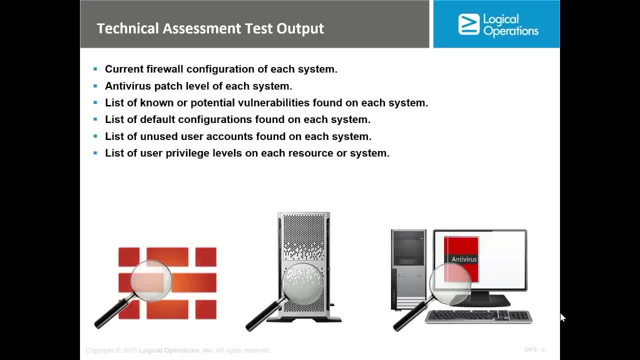 a small period of time for a project and then they leave the company. how do you manage that? do you have user on your system for account or account for users that they are not there anymore? do you verify the account frequently? what is your sequence or what is your process? 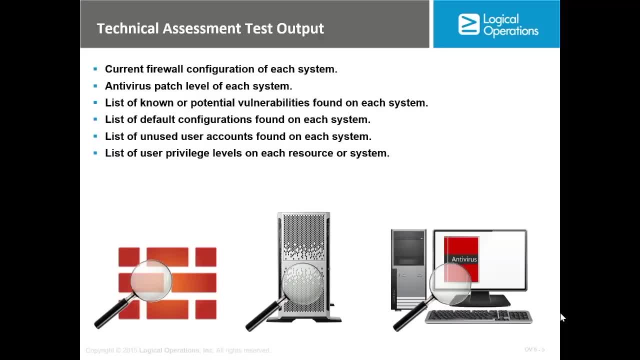 for example, if someone left the company, so you will delete his account right away, or do you keep it for a while? you disable the account and keep it, for instance, for two or three months, according to the policy. don't forget: everything needs to be done according to a policy and then delete it. 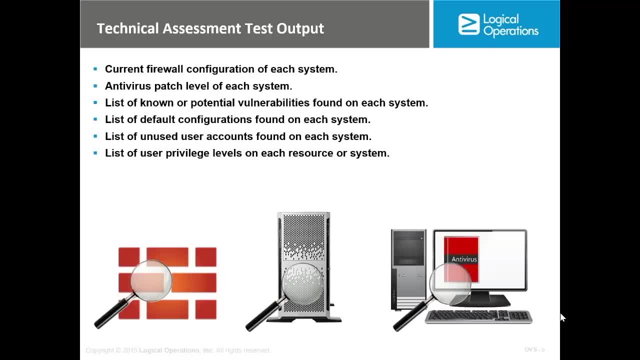 after that. so you should have a policy list of user privilege level on each resources or system. privilege is a big issue, so you need to have a list of all the users who got privilege and you need to be justified. so this is some of the technical assessment output. later on you're going 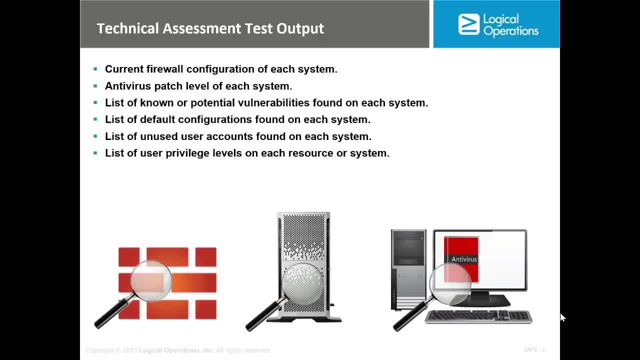 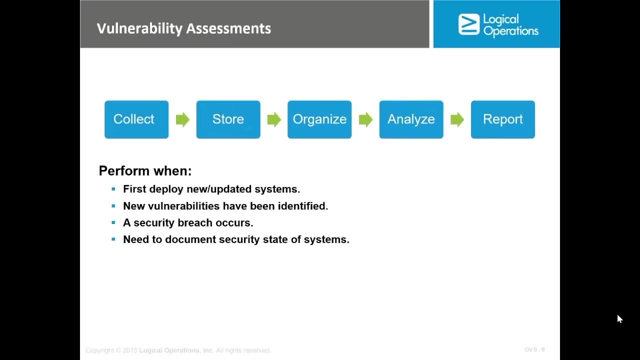 to see some samples of both of those reports, but this is what you need to have in your mind when, as an output for the test assessment, let's start with the vulnerability assessment as a way for testing your security vulnerability and you need to identify your weakness now. you need to consider that not all vulnerability 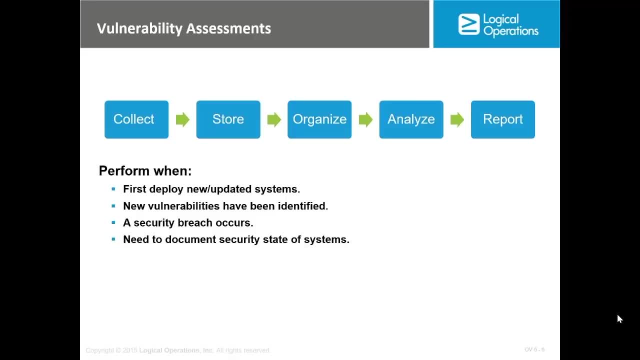 representers, sometimes you may have a vulnerability, but it doesn't have any threats. we already covered that in the first domain. so vulnerability: it's important, but you need also to classify them or to rank them according to their criticality, and we're going to take a couple of demo in this. 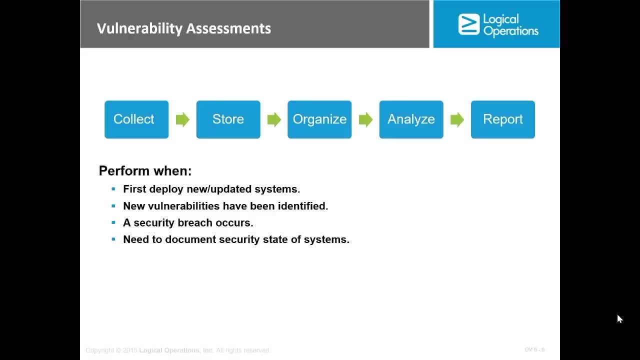 domain. instead of keeping this topic dry, i'm going to show you a couple of examples of tools that you can use to do a real vulnerability assessment process. how it's done, what tools is usually used- free and paid. what kind of report you'll be getting. what is the most important part? 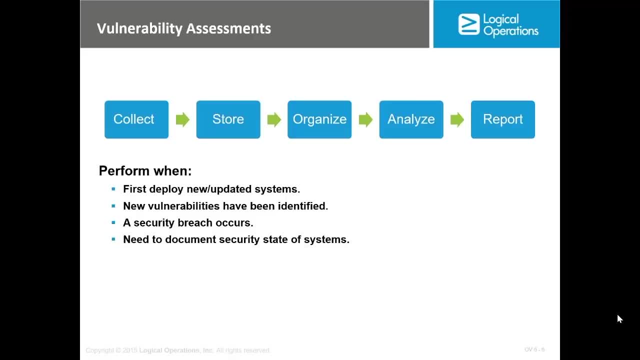 in vulnerability assessment. so before showing you the demonstration using different tools, let's talk about when it should be performed. when should i do a vulnerability assessment? you should do that when you first deploy new, update, new or updated system. so you got new system or you are updating your. 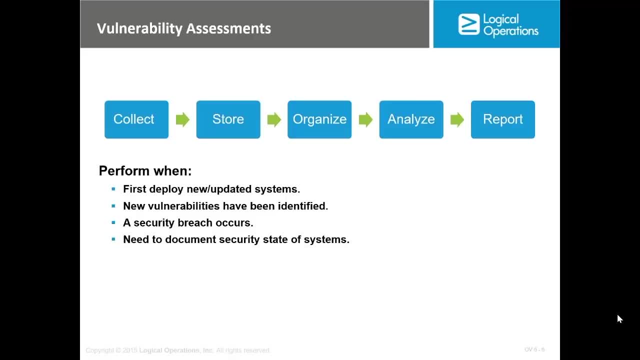 system. let's do a vulnerability assessment just to see if the system is vulnerable or not. the vulnerability has have been identified, a new vulnerability have been identified. so there is some new vulnerability or announced on some of the website. so, for instance, a new weakness in windows system. so i should scan my windows system. is it vulnerable or not if a security breach occur? 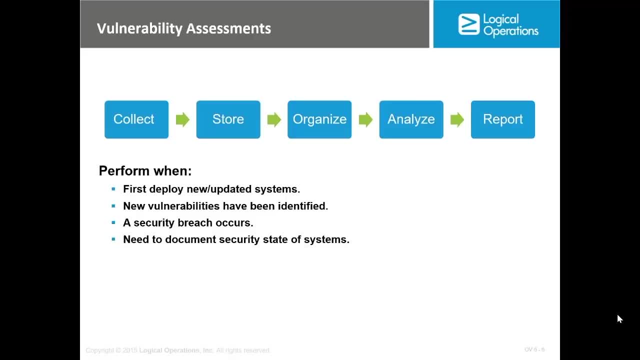 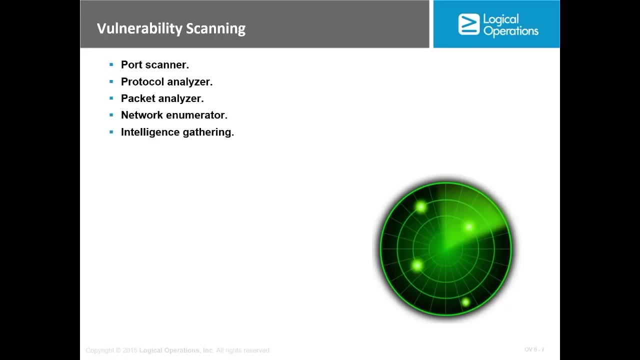 i need to check. do we have any other weakness that may allow any new breaches or not, or need to document a security state of system? so i need to know where i'm standing right now when it comes to security vulnerability. scanning could include port scanner, protocol, analyzer, packet analyzer. 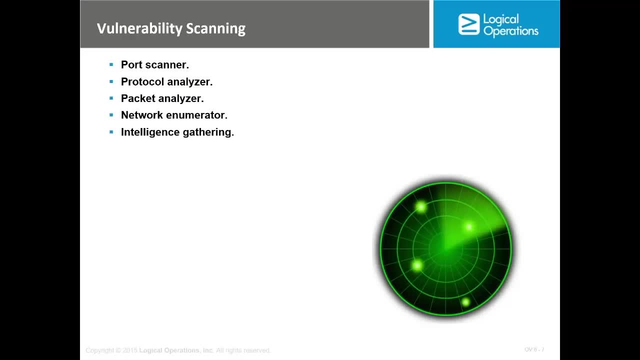 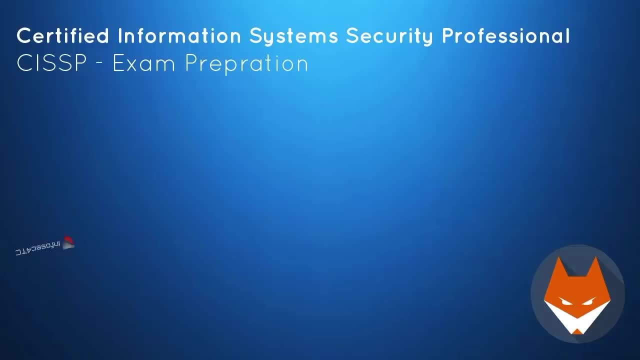 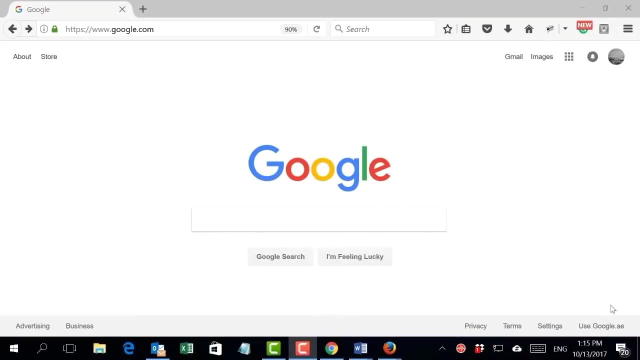 network enumeration and intelligence gathering. so let's see how we are doing that practically. now we're going to start with the vulnerability assessment and a vulnerability assessment as a process. it's quite important for two different reasons. first, this will be a core phase that will be needed for all the upcoming phases, so for the penetration testing, for the reporting, the 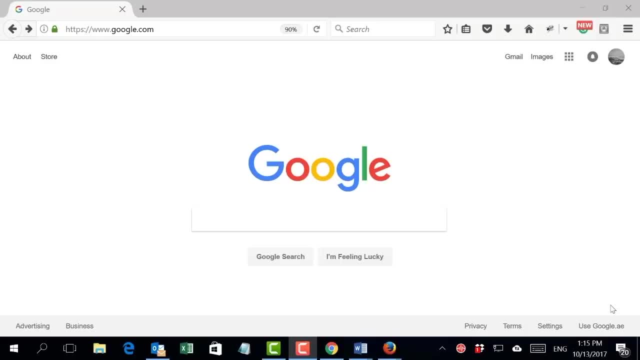 vulnerability assessment is very important to identify the vulnerability and then eliminate the false positive and then try to test the remaining vulnerability- is it exploitable or not? but the second and most important reason, that vulnerability assessment by itself sometimes it's a separate task and it's one of the compliance requirement. so besides the penetration testing you may need to. 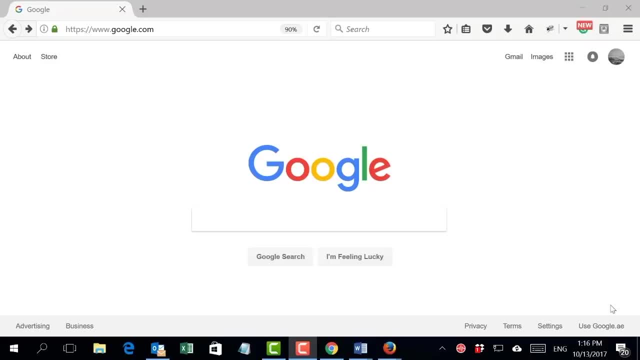 do only vulnerability assessment for any organization. so you can do that. you can run any vulnerability management tools, as you're going to see in this section, and get a report, and you need to fine tune the report so it will be readable for management and non-it people and then show them the 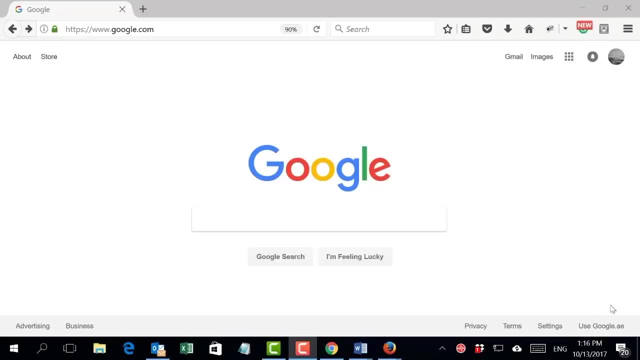 type of vulnerabilities they have and what is the recommended solution for solving them. so what i'm trying to say here is that a vulnerability assessment could be a project by itself, not just a part of the full penetration testing project, and we're going to try to do different type of vulnerability assessment because actually it 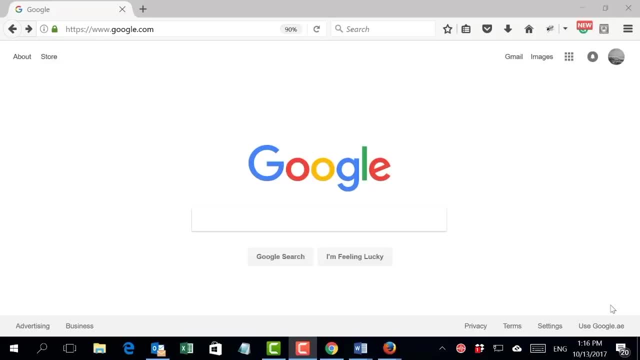 depends on your project scope. if you are doing a network penetration testing, so the type of vulnerability assessment that you're going to do, it's related to the network and you're going to use the tools that help you identify the network vulnerability, while if you are doing the same, 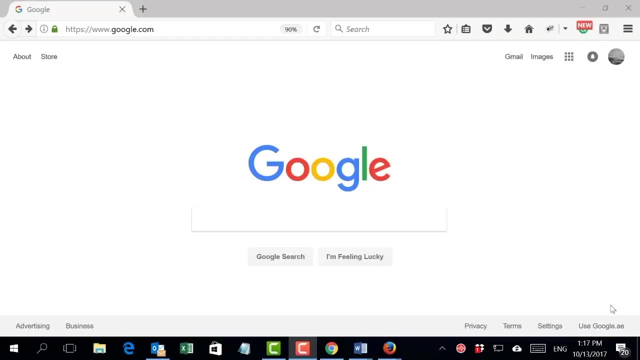 for a web application, you may need the different tools with a different type of vulnerability assessment methodology, so it depends on what exactly your scope. so we're going to use few tools in this section showing you how it works the reporting part, but again, you have to practice that yourself and choose the tools. 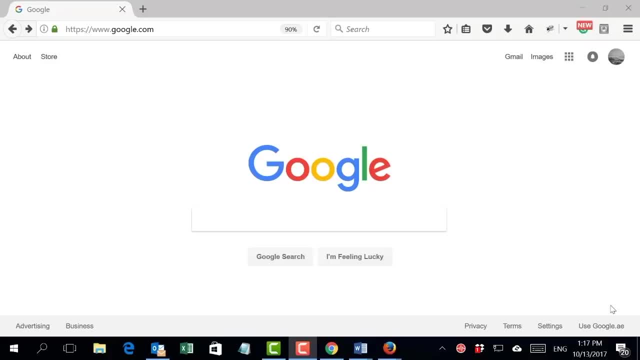 that is suitable for your project and for your scope. so the first tool that we're going to use is nasus, which was one of the oldest, very, very common, very, very useful and effective as well. so we already saw in a previous section how to download nasus and how to 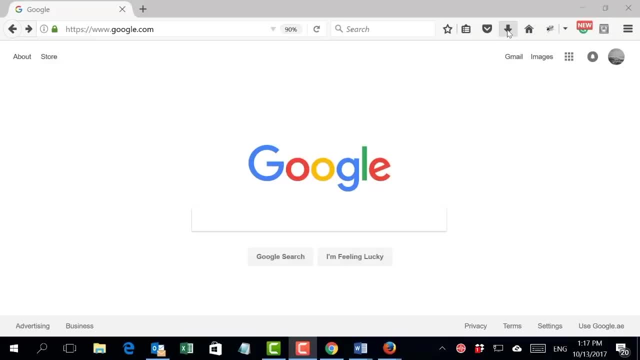 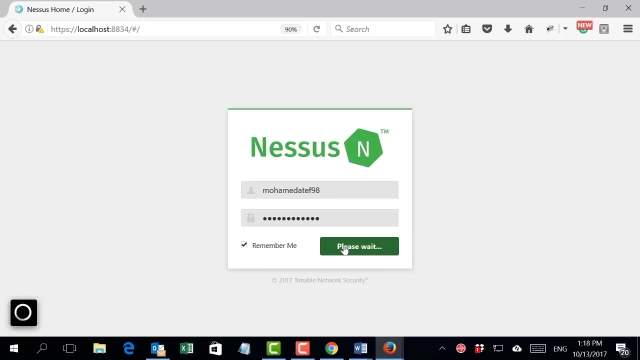 set up nasus. so, if you remember after, it's a web-based application, so it should be inside. i did add the url in my favorites. here you go and this is the login screen we're going to click on sign in. and this is nasus interface. next lecture: we're going to 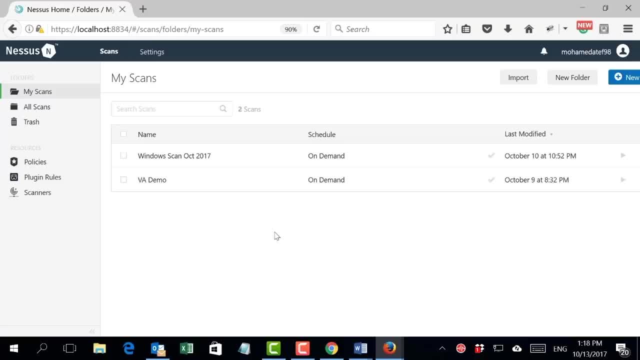 start some virtual machine and then we're going to run the vulnerability assessment against those machine and we're going to discuss the output that came and how it can be used for the next phase or how it can be submitted in report to management as a separate task. 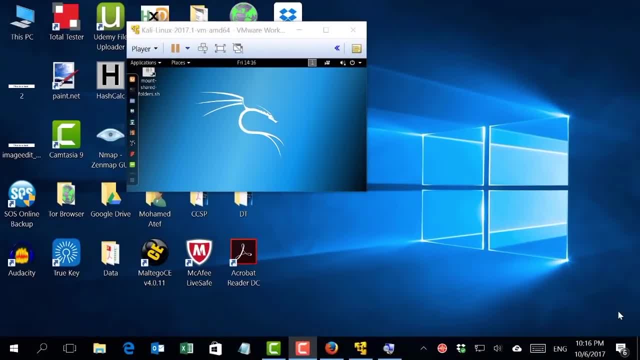 in the previous lecture we saw some of the common vulnerability assessment tools and in the next lecture, in the same section, we're going to see some of the penetration testing tool. now it's not about those specific tools, as i keep saying that you can use whatever is comfortable for you and whatever is suitable for the project. 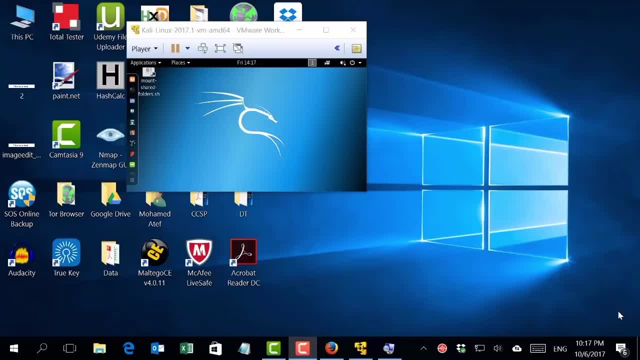 that you are working on, so the project, and according to the scope of the project, you may select the tool. we went through some of the tools, but let me show you some more. three of them in cali linux that include most of the vulnerability and penetration testing tool. 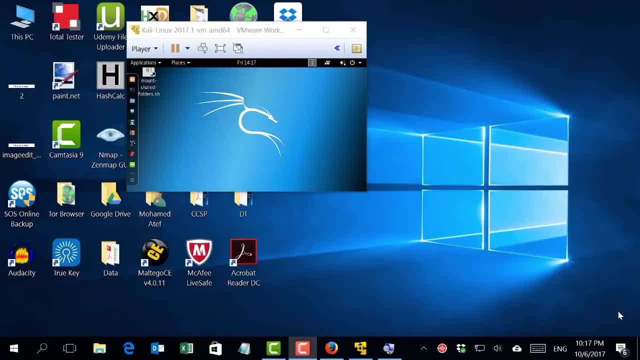 that you may use. so which tool should i use? i cannot tell you that. i'm just showing you different tools and i want you to get used to it and get practice to it, using it, and use whatever is comfortable for you and whatever is suitable for the project that you are running. so, for instance, 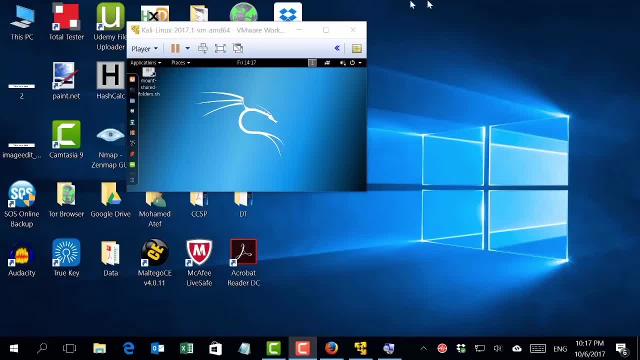 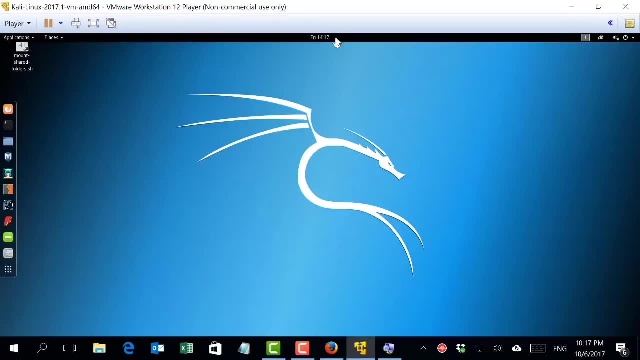 if your project is a project, a web application, website, so you need to scan a web application. there is a lot of tools, there is hundreds of tools who do that, but if you go to cali linux- the ones that we set up in the virtual machine in the previous lecture- 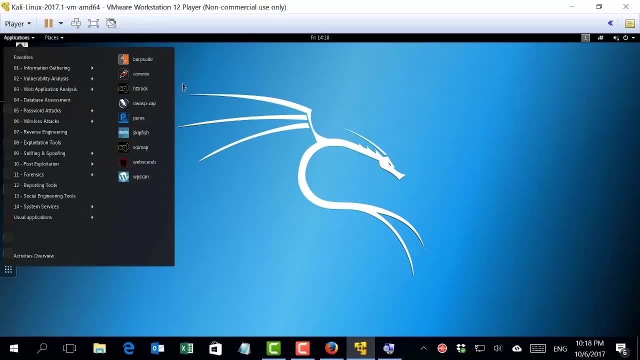 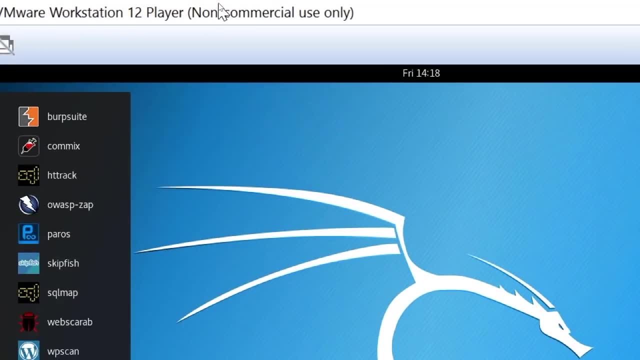 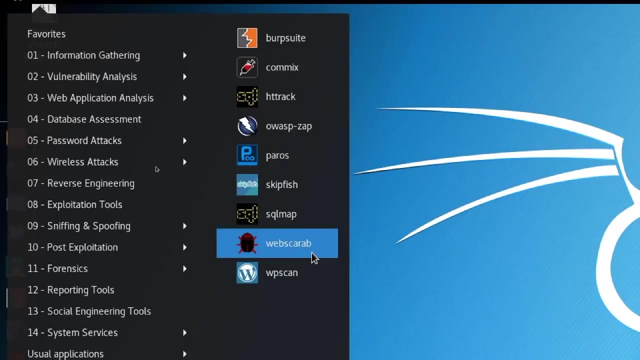 and go, for instance, to web application analysis, you will find a lot of tools that you can use. so, for instance, we have these tools. it's very, very powerful. i used it before. so this is the web application analyst- and you will find different tools for vulnerability, especially for web application. so, for instance, i like this tool very much. 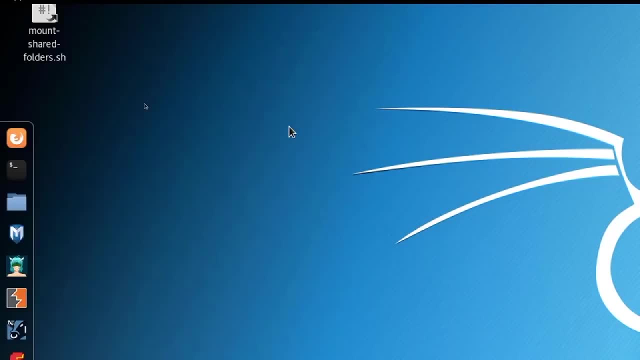 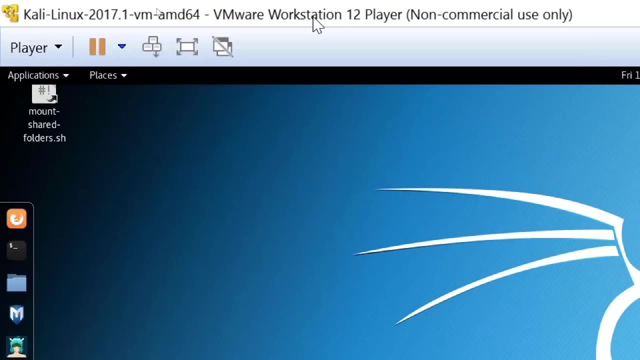 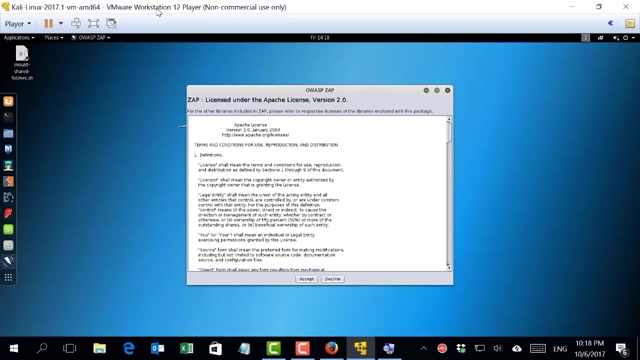 wasp that and we'll talk about that later on. that wasp: it's an open source web application project where you can, or actually they usually publish the most 10 common vulnerability every year. so they will check in the web application how many vulnerabilities are found that match the top. 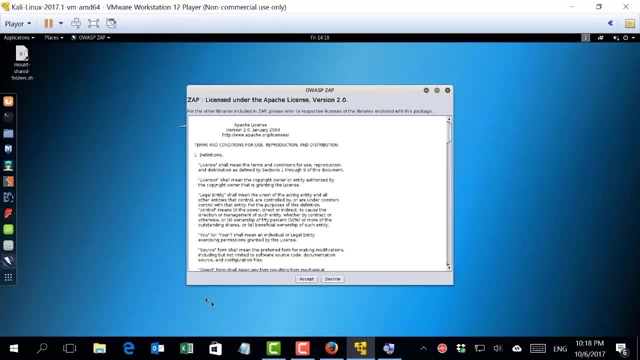 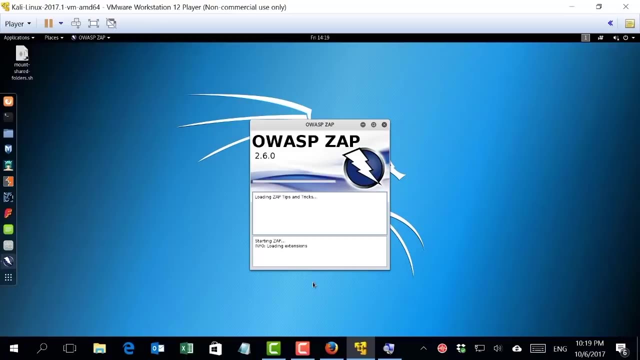 10 vulnerabilities. so this is the interface. it's free tools and very effective, and i'm just showing you the tools. we're going to use different tools, but we will not be able to cover all the vulnerability assessment tools or all the penetration testing tools. we are just getting the concept and i'm i leave to you. 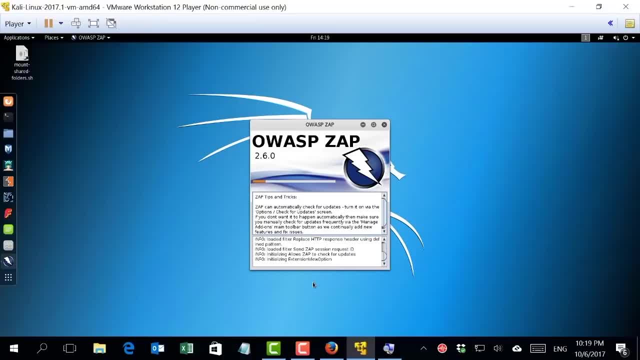 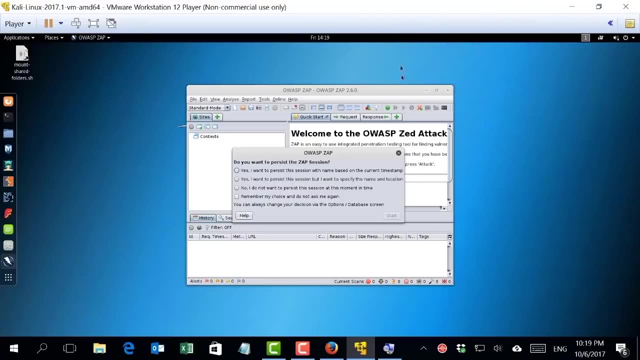 to try to use them and even to search for more and use whatever is comfortable for you. so wasp zap is a web application vulnerability assessment. that is straightforward, graphical interface. it's kali linux, right, but it's graphical interface. so, as you can see, this is wasp zap very effective. 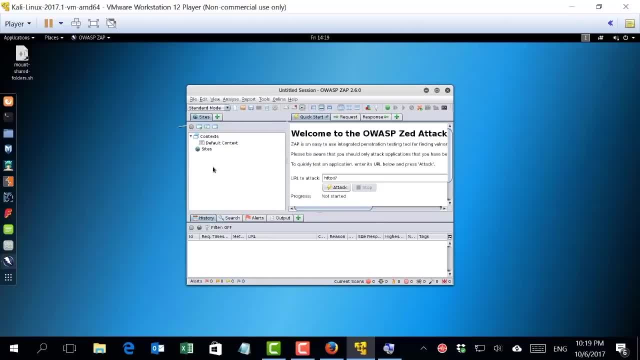 tools and you can add a project- and it has a very good library- depend on the top 10 vulnerability assessment. here you can put the urls that you want to check the vulnerability for and we're going to see some example using this specific tool. so the point here: 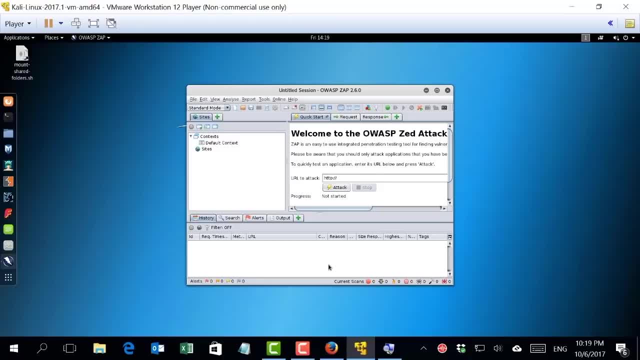 is that you need to have three or four tools that will be used. the point here is that you need to know that there is a lot of tool, a variety of tools and on different platform- on windows and linux- and some of them are free, some of them are paid. so before you start working on penetration, 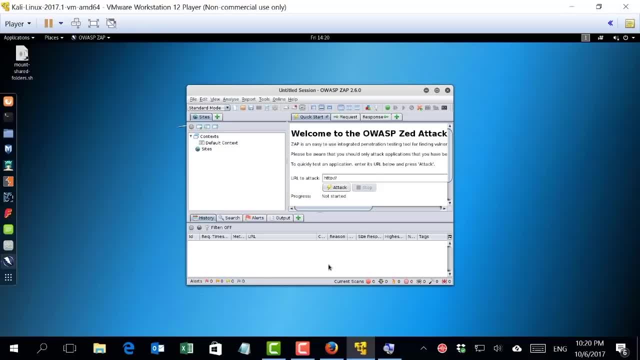 testing project, you need to specify the tools that you're going to use and you never think about the underground tools. so you should not go to those a dark or deep web website and try to get those underground tools. that may cause a lot of problem in your project when you work in a 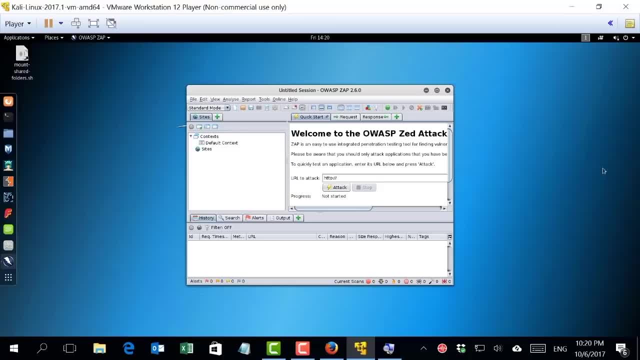 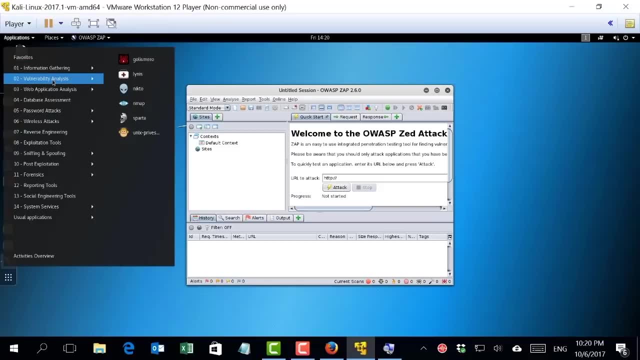 professional level, you have to use the professional tools. so this also is another tool that i wanted to point to, and if you just open your kali linux machine and check, you'll find a lot of vulnerability assessment tool for web application and for system and so on, and you know, you can just. 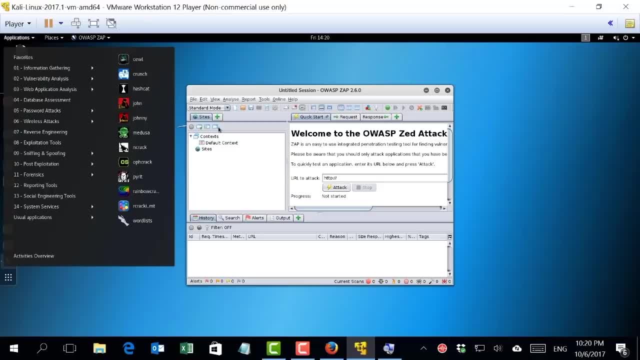 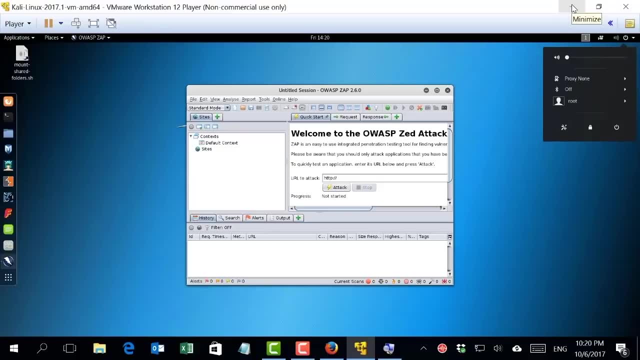 open and go through them in a brief way, because most of them are working in the same way, so you know the same output, but in a different way. another point that i want to mention is that when you do a project, do not depend on only one tools. this is very important, because different tools 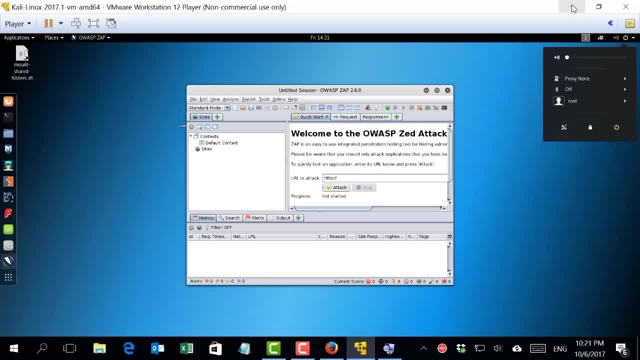 will give you different, different results and, as i mentioned that earlier, using your analytical techniques that we're going to learn during this training, you will have your own report, so do not use those automated report. you will have your own report, so do not use those automated report. 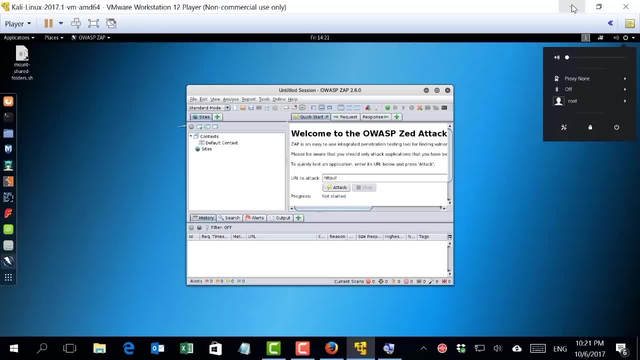 you have to read it and read a report from another tools and read for on the same target and see what could be the false positive and what could be a real vulnerability and real witness. starting from the next lecture, we're still working on get familiar with the tools, but we're 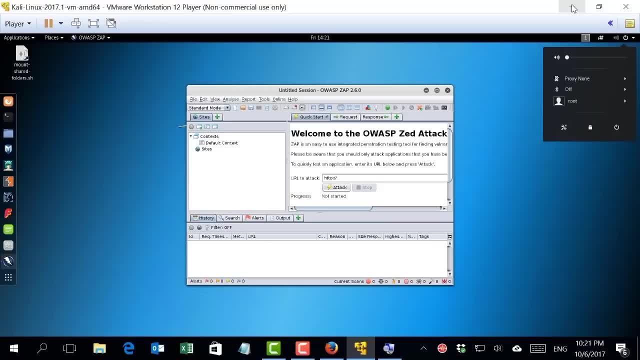 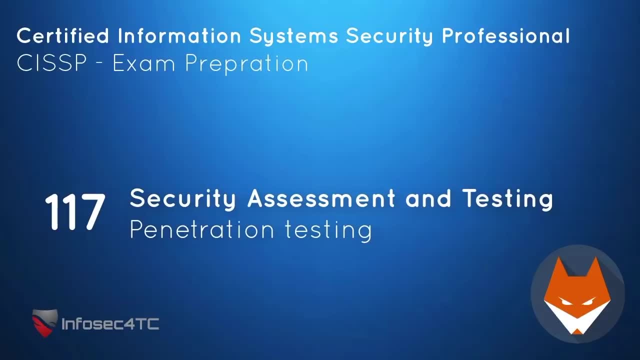 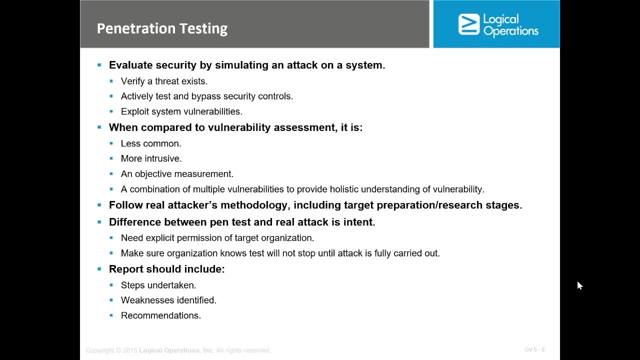 going to point to some penetration testing tools, so let's see some of the common penetration testing tools. let's move to the penetration testing part for evaluating our security now. penetration testing is different than vulnerability assessment in a way that vulnerability assessment will just will, will just identify the weakness, while penetration penetration testing will. 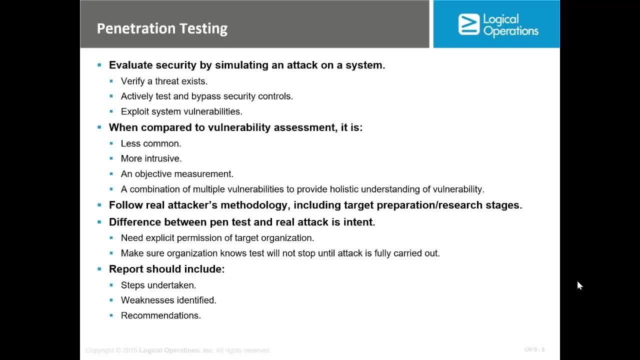 test if this weakness can lead to compromising the system or not. so, for instance, i may have a vulnerability which is an open port. this could- could be considered a vulnerability. now the penetration testing will try to hack the system from this open port. this is an example, very simple example, because actually penetration testing 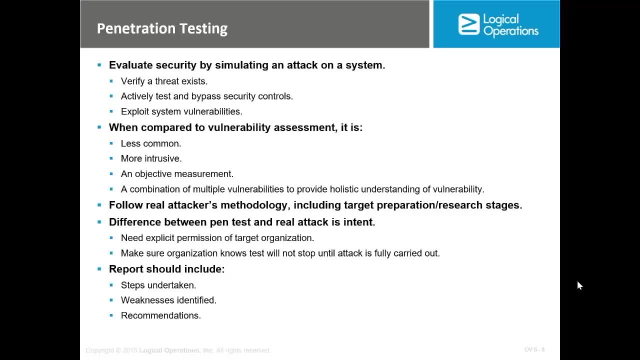 it's much more deeper than that and usually when we do a penetration testing we need to identify our scope. what exactly is our scope for from penetration testing? is it a network penetration testing? is it a white box, a black box? is it a social engineering penetration testing? we 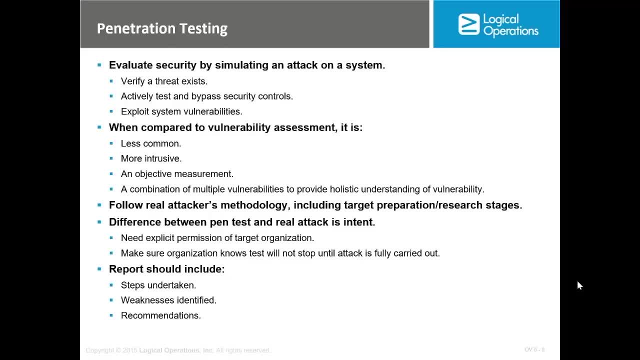 have many type, which you're going to explain in a few minutes. so penetration testing cannot replace the vulnerability assessment and vice versa. both of them are important and both of them are a compliance requirement. so in this section we're going to talk about the penetration testing process. 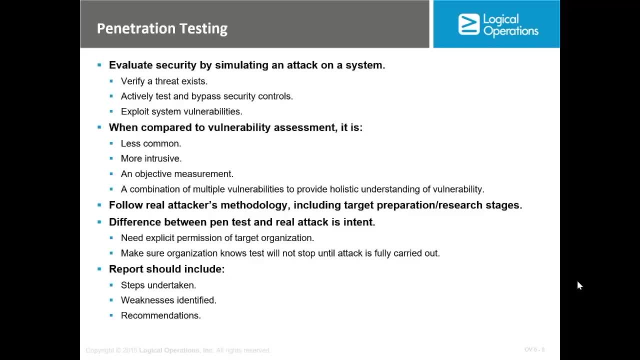 what are the phases in penetration testing, what you should be expecting from each phases, and so on. but you need to understand that when you do a penetration testing to a customer, you need to get some results in a way that you need to show them. i was able to compromise the system. 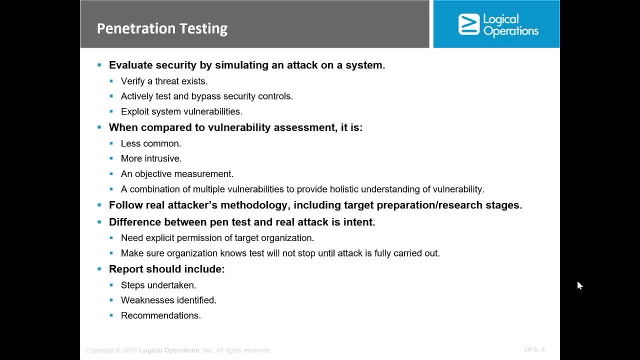 i was able to get access to this database. i was able to create a folder. i was able. so it's not like a vulnerability assessment where you just identify or showing that the management, the weakness. here. you need to show them that you were able to get into their system from those. 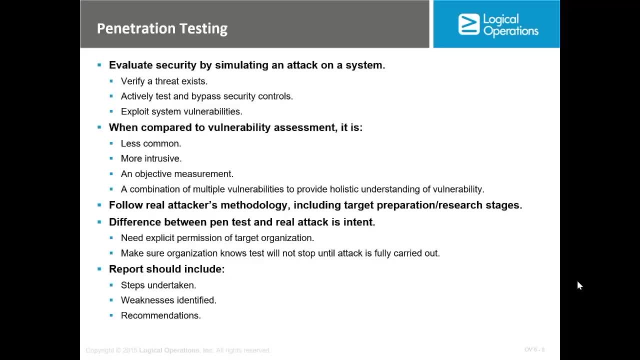 weaknesses. so it's quite important to like use a tool that will allow you to do a proper penetration test. now, penetration testing is very strict. i mean it's not like the way you are seeing it in ethical hacking course. you will not get an underground tool and use it. you have to use. 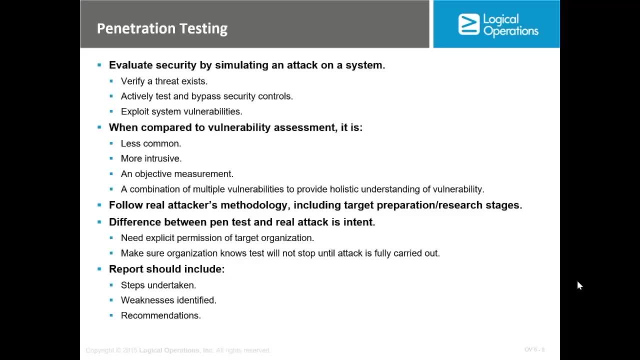 a proper tool. you have to have a proper plan. uh, you need to have a plan for any incident that may happen during during the test and roll back in case of any problem. so we're going to talk about more and i may give you one like example about 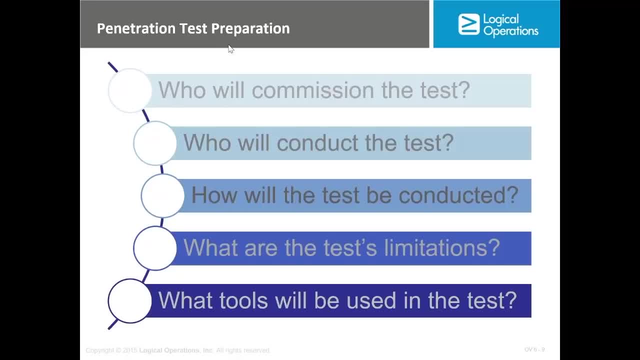 penetration testing tool. now there is some preparation when it comes to penetration testing. who will be commissioning the test? who will conduct this test? who will be the test to be conducted? what are the test limitations? this is very, very important test limitation. it's an, It's not a general test. 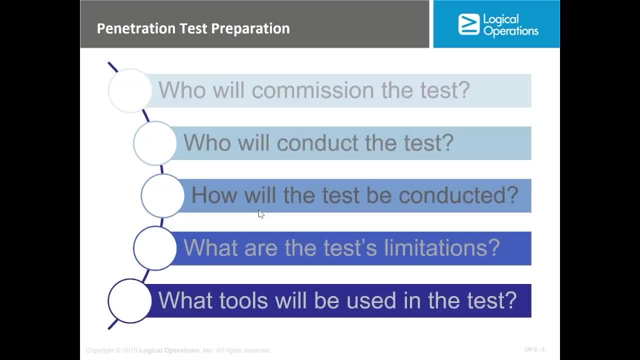 You need to only get or to do the scope of the test. Okay, what tool would be used into the test? This is also very important. Sometimes you may find the tool online. You don't know what is- it's a free tools and that you don't. 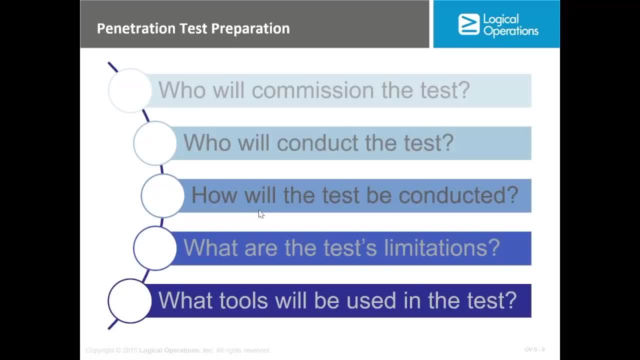 know what damage it will do. and you, when you are working in a professional environment, is different when you are, then when you are testing at home. So all those are quite important to figure out. Now, what are the process or the step for doing a penetration? 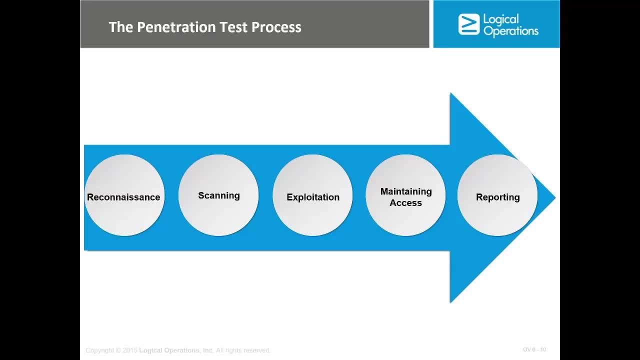 testing. Now there is many phases and each phases got to have its own result and I may give you some demo about some of those phases just to prove the concept. So first, usually we start the penetration testing with the reconnaissance. Reconnaissance is just to gather information about your target. 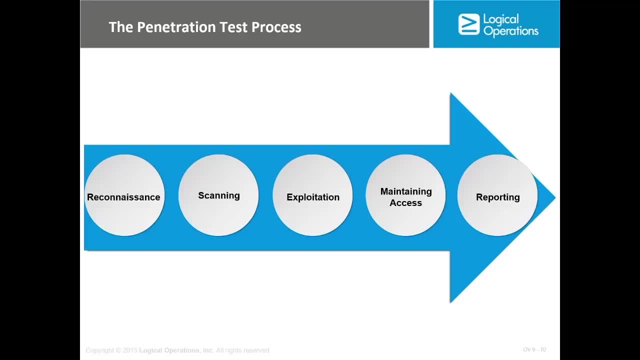 Now don't forget that when someone is hiring you to work as a penetration testing, he's asking you to act as a malicious hacker. He's asking you to do what hacker is doing, So you need to follow their methodology. So usually, start by doing reconnaissance. 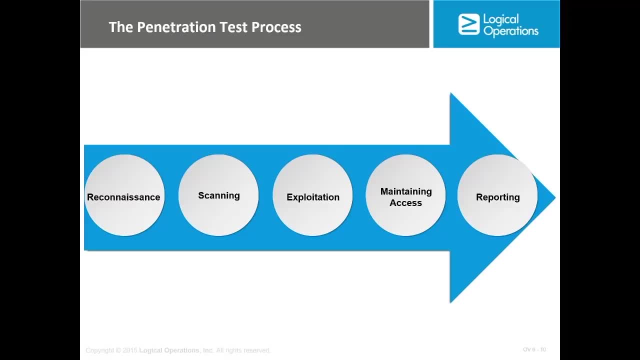 You have a target and then you start collecting information about this target. How much information are available Public online? next lecture: I'm going to show you a reconnaissance lecture to give you an idea what I'm what I'm talking about. but we are using only 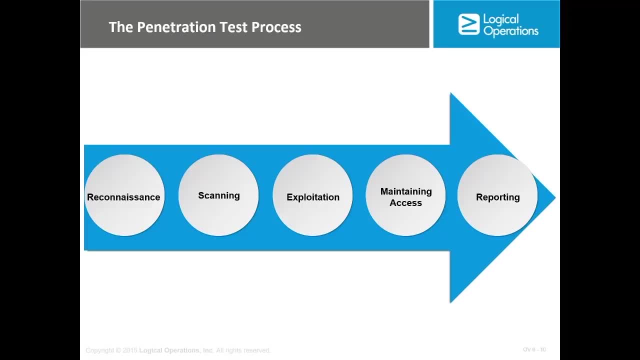 public record for reconnaissance. I can get a lot of information about public record. I can get people email who is working on a specific company. I can get the operating system that those web server is using. All those are free on websites. I'm going to show you a couple of email, a couple of demonstration. 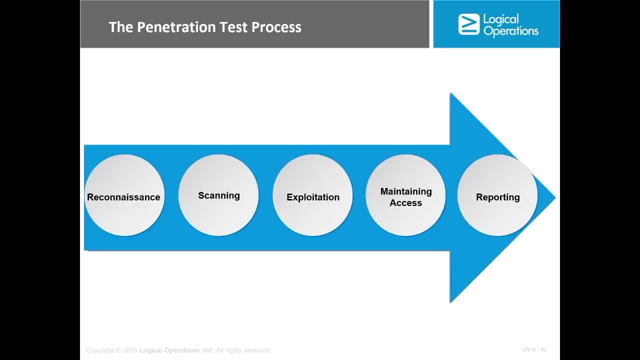 after finishing it and from the reconnaissance you may have into into your report a part related to that, You can say that I found too many information are published public. Maybe you need to do an NDA for your employee telling them you do not need to publish that such information public. 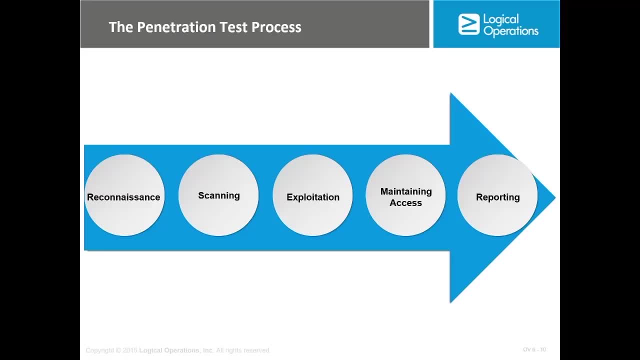 You know, I saw in many websites where people will write down problems that they are facing in their company- technical problem- and looking for assistance. Those are very critical. Some people are uploading like information about the router setting and asking for People to help in different blogs or Facebook group and so on. 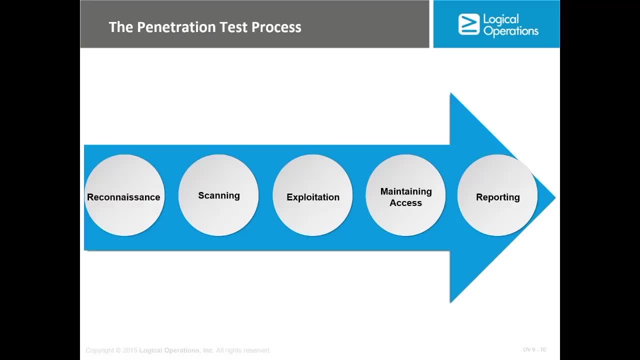 So reconnaissance is just to collect information from public phases. Then we have the scanning. scanning It's to collect technical information or more specific information like open port on the system service running, operating system, network topology. So scanning it's to start getting more information from the. 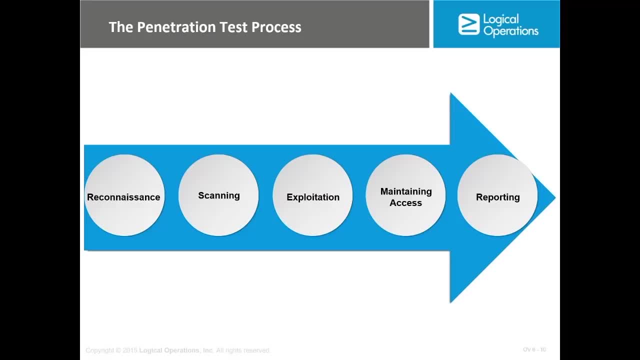 scanning information, I can start looking for weakness. So if this customer- I, from the scanning, I know that he's using Windows XP in one of the machines, then I can look for what are the weakness in Windows XP. and this is quite easy And it's a you know in all web. in many websites you can find like: 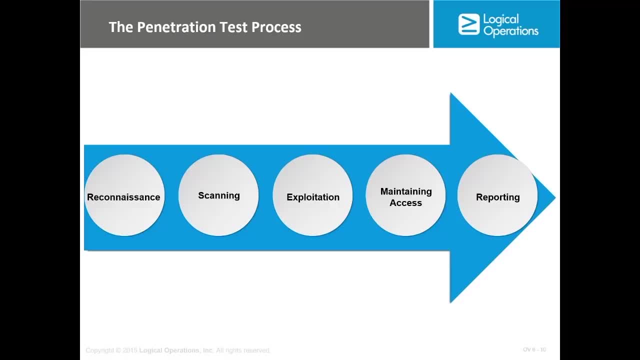 vulnerability website where you can check for any vulnerability related to an operating system or an application and so on, and then exploitation: based on the reconnaissance and scanning and the vulnerabilities that I'm found and how it can be exploited, I can try to exploit the system. 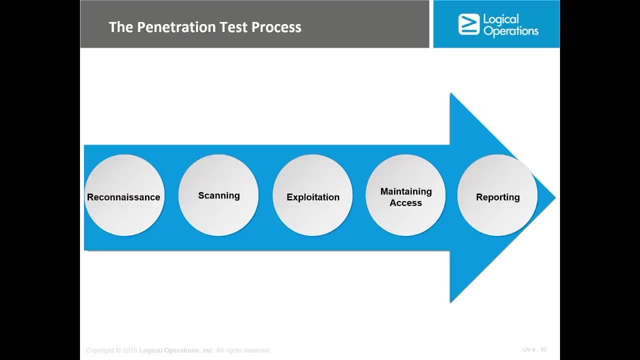 And, after exploiting system or hacking system, maintaining access. So, after compromising the system, I need to put something to allow me to log in every time. I won't, I don't want to go through the same steps one more time. So I need to put like a key, like a back door, or I need to to mitigate. 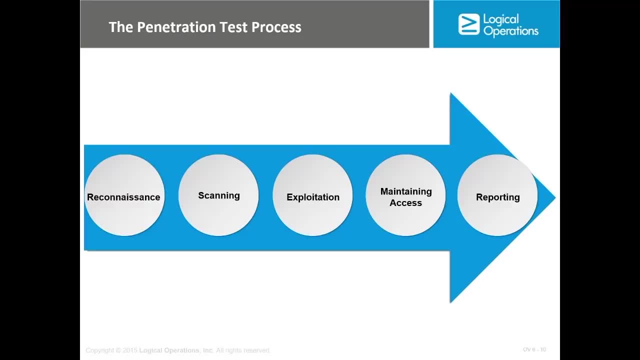 my, migrate my process to a system process, So even the user cannot get rid of me. And finally, I need to write down the report. This is a very high level explanation of the penetration testing. I will put some like videos showing different steps, but actually this: 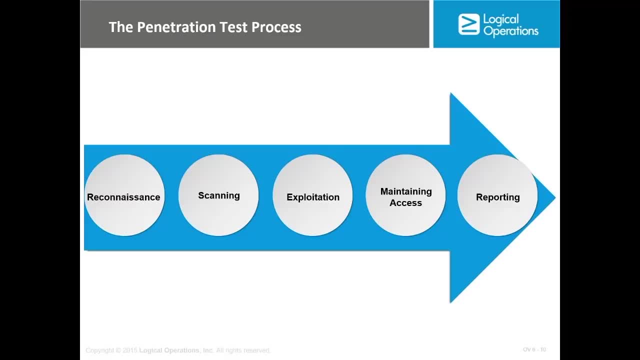 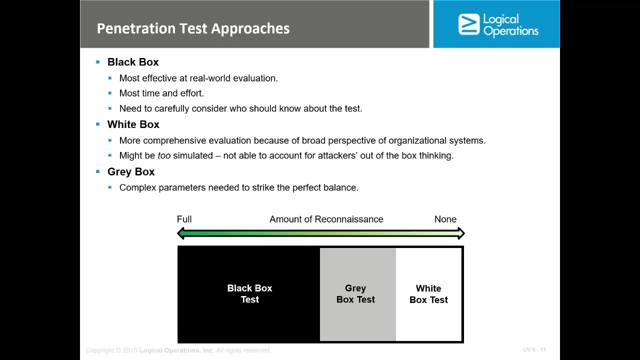 is not the real or the full process, but it will give you an idea about what I'm talking about. But before going or showing some demonstration, I just want to let you know that there is different kind of penetration testing. There is a black box, and black box penetration testing is where the 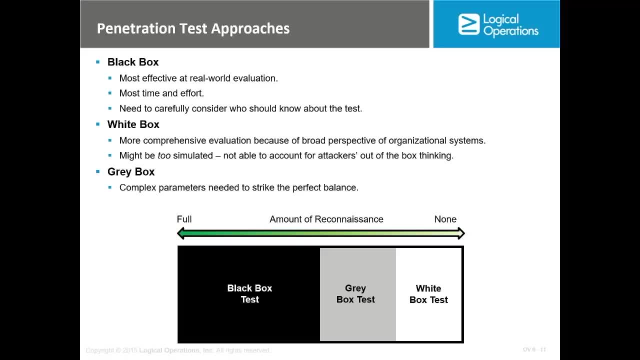 customer will not give you any information. They will hire you and they will tell you. I just want to know: if you don't know anything about our system, Can you get into our system and compromising, and then you have to start everything from the beginning? 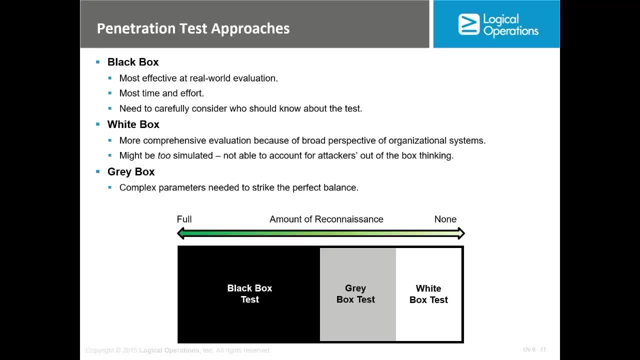 We have the white box, where the you will have some information about your target and you will be requested to do a penetration testing, and we have the gray box, which is a partial kind of information, but also we have The social engineering. penetration testing is very, very common. 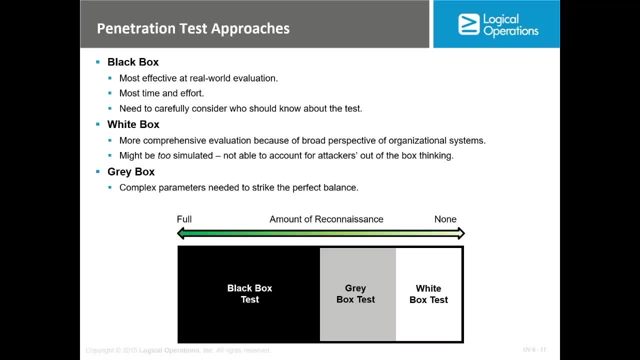 So there is different kind and definitely, definitely they have different fees. I mean, if you are doing a full or a black box penetration testing, you will get paid much more than white box and so on. So let me show you some demonstration about some penetration testing tools. 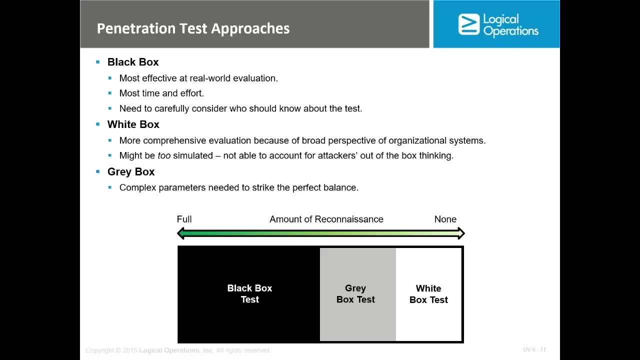 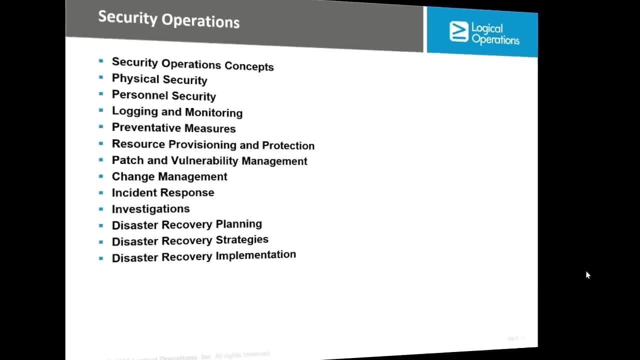 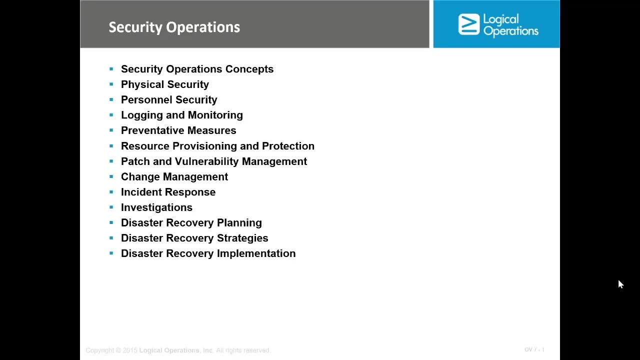 how they are working And then To move to the next part of this course. Now we're going to talk about security operation. Now this will not be a very big domain because actually a lot of those point has been covered in previous domain. 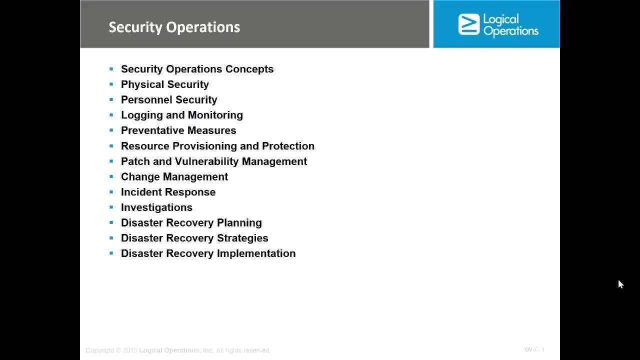 So we're going to talk about security operation concept. I'm going to talk about physical security, which is- which has already been covered in a previous domain- Personal security, logging and monitors and monitoring, which we also covered in a previous domain- preventive measurement, resource provisioning. 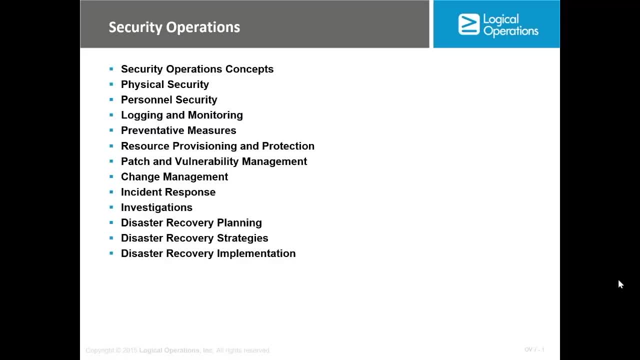 and protection. Now, don't forget that there was a domain where we spoke about some of the main administrative policy things like the least privilege, dual control, mandatory vacation. This is mainly operational And security. We're going to talk about batch and vulnerability management change. 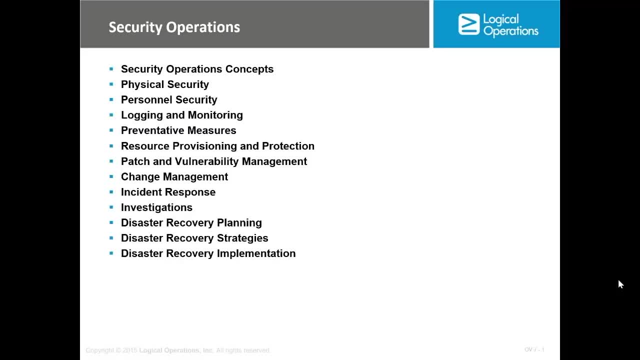 management, incident response. All those point has been covered: investigation, disaster recovery planning, disaster recovery strategy, disaster recovery implementation. So I will not repeat the same lectures but I'm going to just focus about the points that was here and was not in different domains. I don't really feel that this domain 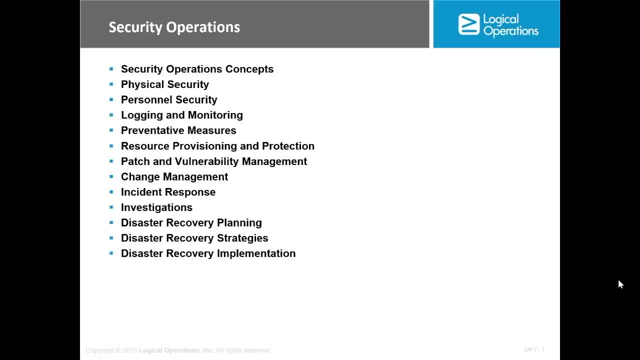 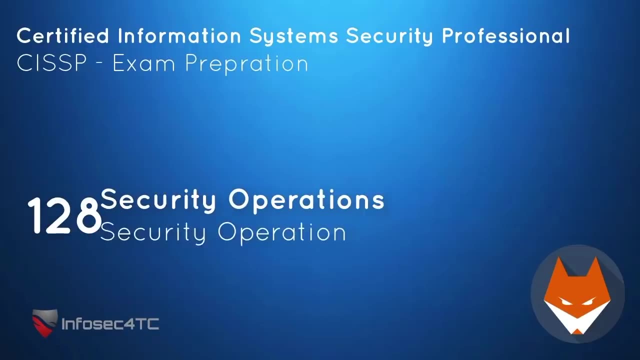 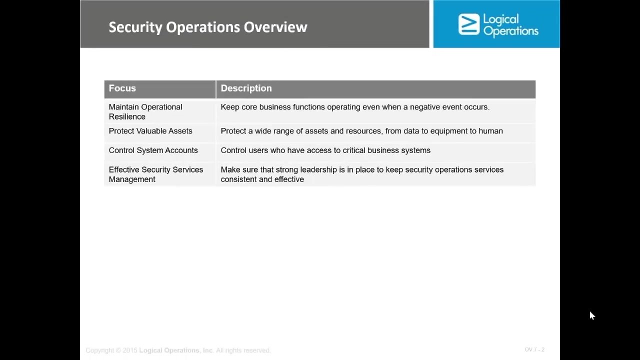 It's different. It's just combining different point together. Even you're going to find things related to access control and so on. So let's go through it and let's just talk about the points that was not covered in previous lectures. Let's talk more about operation security first. 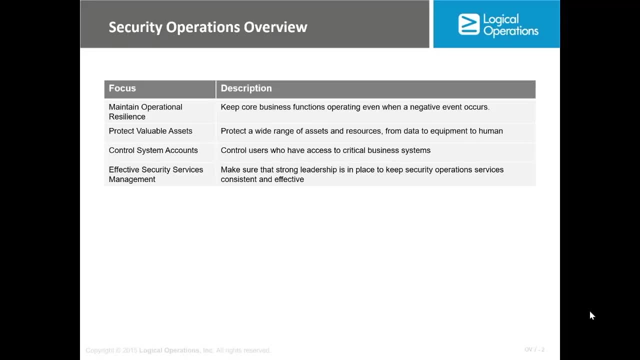 I don't want to get you, I don't want you to get confused when you start reading about operation Security, because you're going to see that most of the topic covered here has been covered in different domains, So you will not spend time or effort while going through operation security. 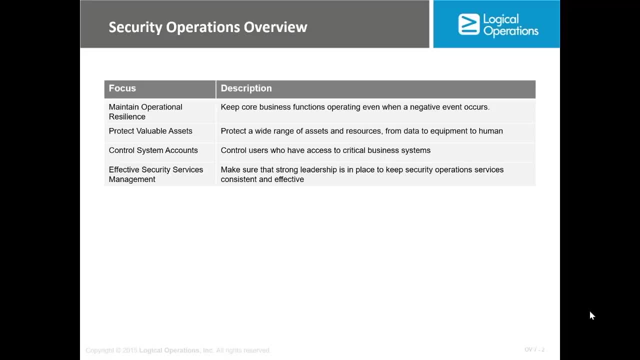 but I want you to understand the concept of operation, security, operation. The point here is that open our discussion. security is usually divided to technical security and administrative security, and physical security as well. The security is generic concept, But here we need to focus on the security related to the business. 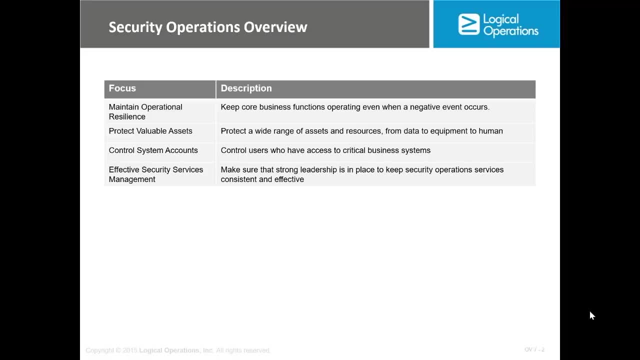 In a sense that security should be implemented to protect the business, not to protect the assets, but to protect the functionality of the business. and I will give you a small example. Assume that you are a government entity and you are issue a license- construction license- So any 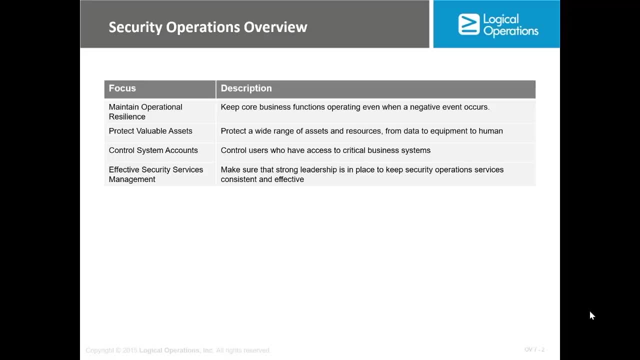 contractor who want to build something, a house or something, He need to have a license from your entity, from your business, And because the issuing a construction license is quite critical, It should be controlled. But what if you left only one employee responsible for that? 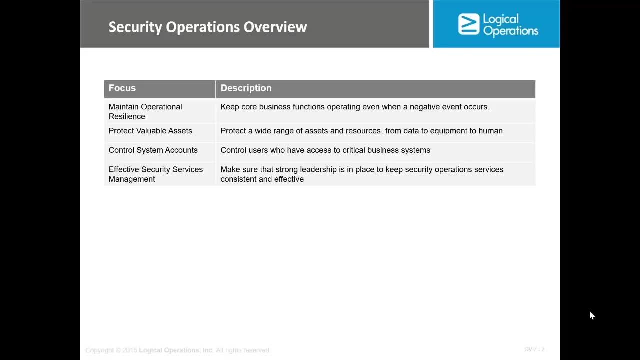 So anyone who need a construction license, he will go to this employee in your government entity and he will request for a license and submit the document and submit the fees and then get the license. What if this employee decided to do something wrong? He decided to like take or do some fraud or take money to ignore some of the requirement. 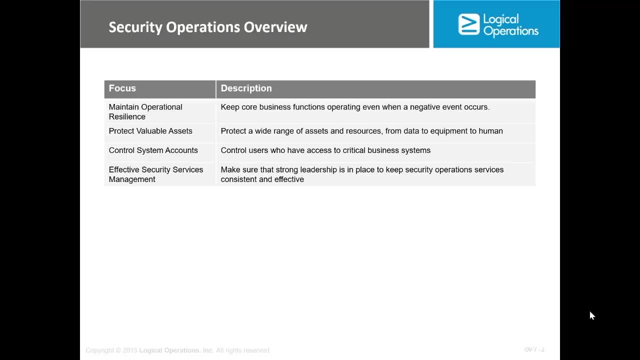 Okay, what will be the results of that? This will definitely affect your reputation and it May get- you may lose life because of that. because people can get licensed easily, They will not follow any regulations. They will build whatever house. then it may end up with crashing or whatever. 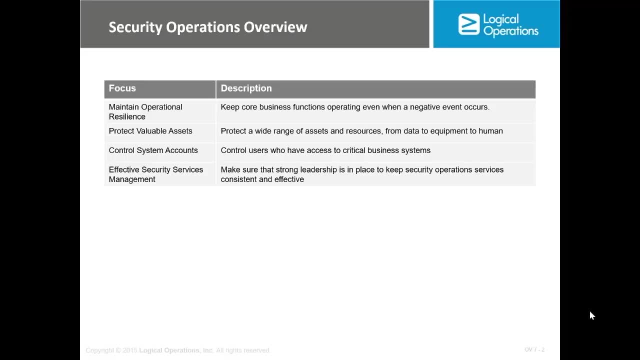 This is a small example. So, according to that, because issue a license is critical, Let me put that, or let me make this process done by three different people, Not only one, not to three of them. each one need to approve other work by doing. 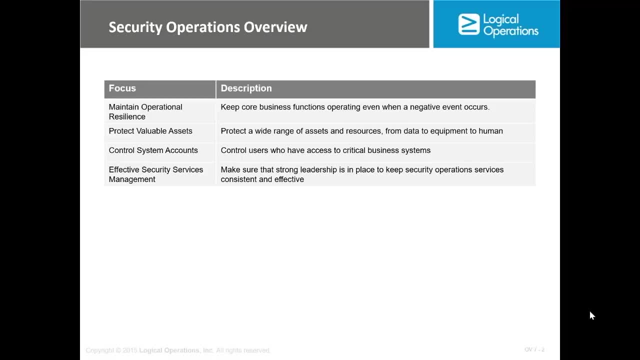 That you are putting administrative or operational security on the operation of your business. So this is like a small example: to identify the critical business function and start putting control on them to prevent fraud and prevent any kind of illegal activity. This is the concept in general and I believe we already spoke about some of the policy earlier in. 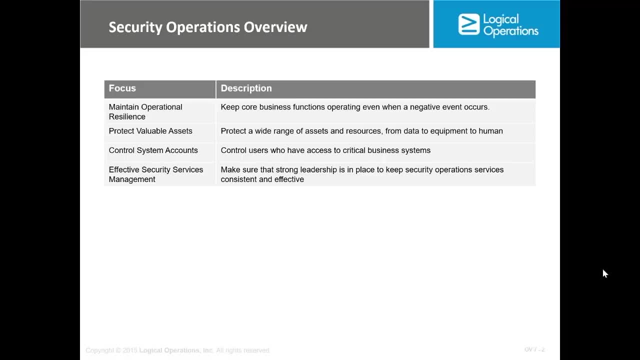 one of the domain, talking about the dual control, talking about least privilege, Need to know and so on. So, in general, the focus of operation security is to maintain the operational resilient. You need to make sure that your core business function is operating well and you are putting all 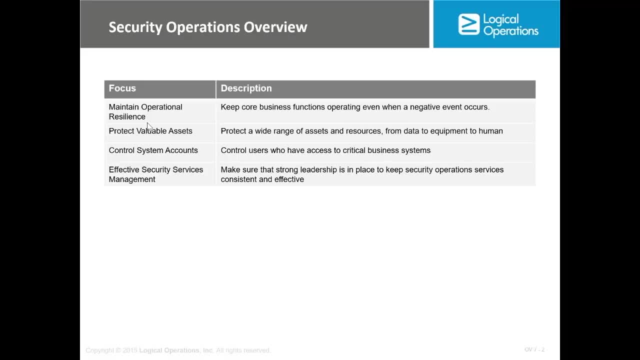 control, not to affect the operation of security, because if you consider the security only to prevent against hackers and virus, this is not enough. But what about people which we, which is most of the Illegal and most of the problems that happen to big organization? 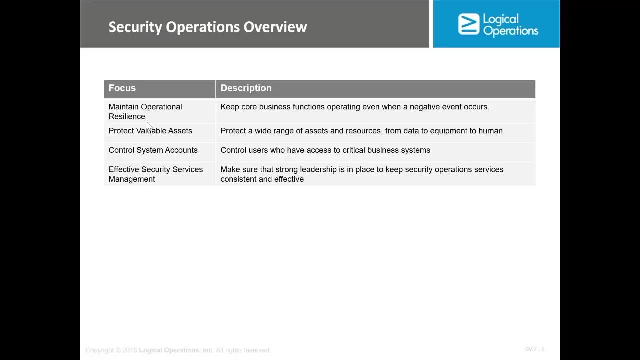 It's because of the corruption inside the company, people start, or employees start, looking for the critical business function and how it's done, and they can get advantage of that. So we are protecting our business, So you are protecting the valuable assets. This can be physical protection or it could be information protection for asset, information, asset protection. 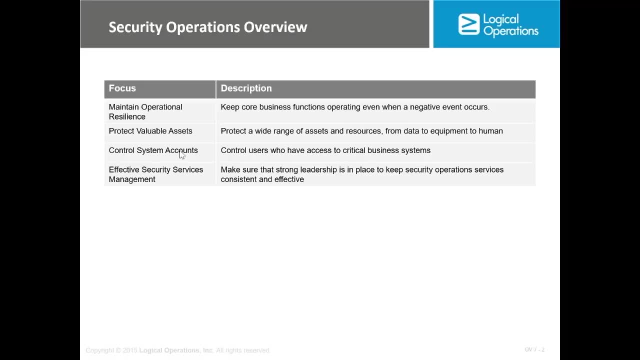 Control system account. Also, this is to control the user account according to their criticality effectiveness of the security service management. So in general, I hope you understand what is the operation. security is security operations all about? now I know that we went through that before. 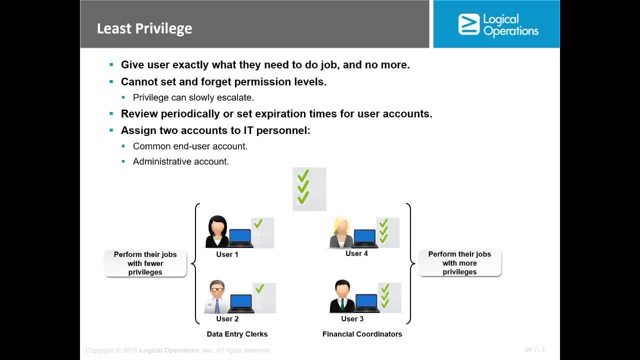 Talking about some of the policy list privilege and so on, but here it's giving you some examples So you can relate the topics that we spoke about related to the policy in information in operation security with the example here. So what do we mean by this privilege? 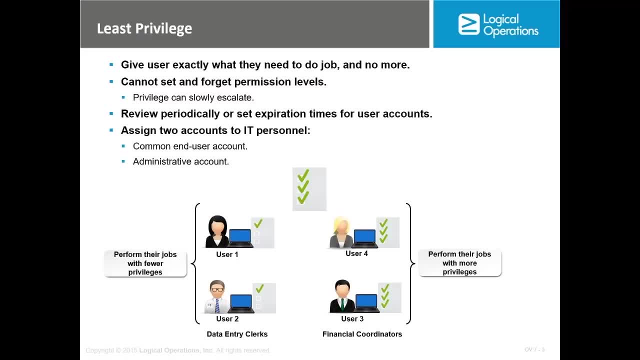 So usually user by default should get a privilege related to his job and access to only the file related to his job. Cannot set or forget permission levels review. Actually, this is quite important to frequently review the access. It's not like you are giving people access and that's it, according to their job description, everything, but you need to use it from time to time. 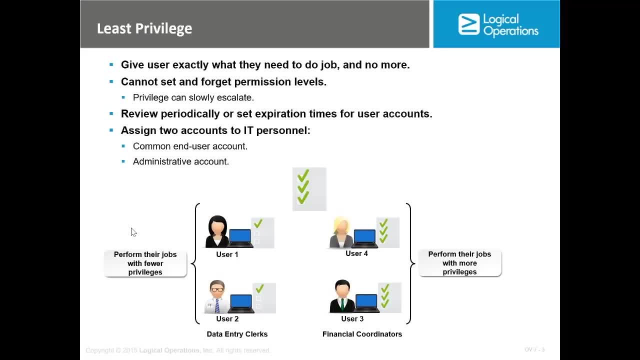 And why we are doing that, because people keep moving. Maybe he didn't leave the company, because if one of the employee leaves the company, according to the policy, his account will be disabled. But what if he moved from one department to another department? You will not, and he still have permission. 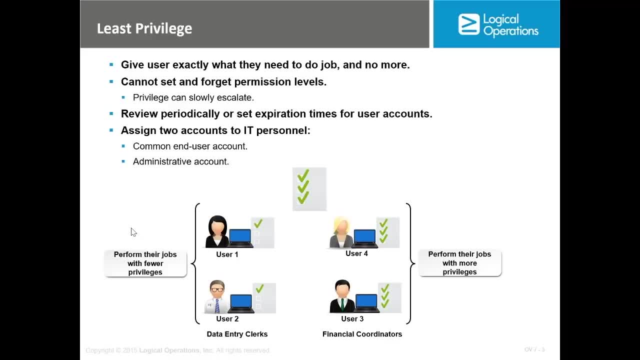 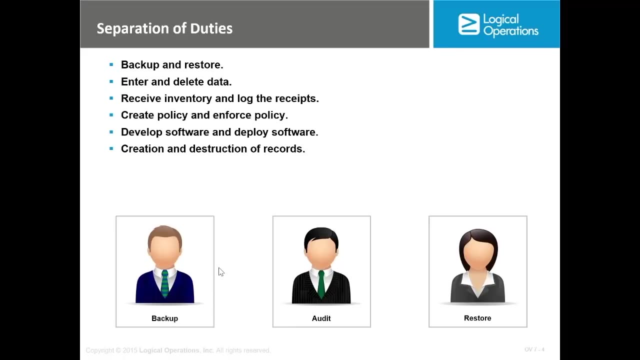 To the work or to the critical file to of the previous department. So you cannot figure that out unless you are reviewing the privilege frequently. common end-user account: You need to disable the administrative account. Another very important policy in security operation is the separation of duties. 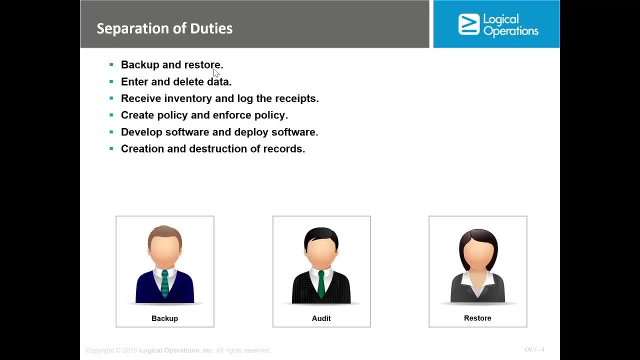 So, for instance, the one who's taking backup should not be the same one who's restoring right, because if you give only one guy the backup permission And restore permission, He have full access to your data and, whatever your business is, you could be a bank and this guy could be hired there. 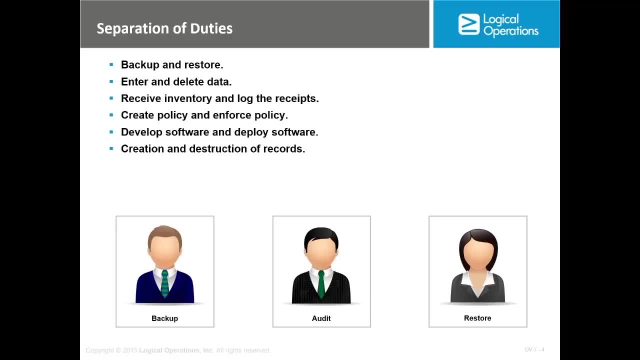 He's taking low salary and he decided to get all the information. But when you give backup to someone and restore to someone else, you know to be able to do something illegal. those two people need to be combined and this is not easier. get the one who are like deleting should be different than the one who are entering the data. 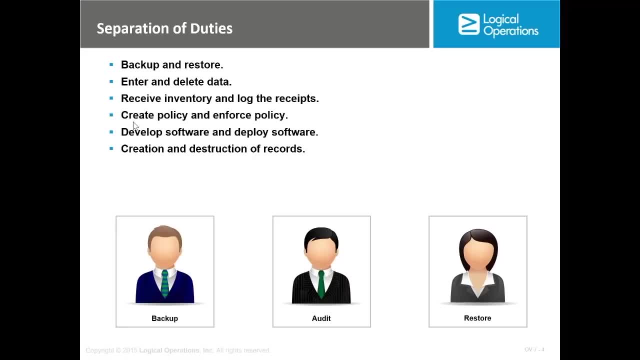 And so on and so forth. Now this may be quite obvious, but actually the way they ask about that inside the exam, It's the in a different way. Sometimes it could be not a technical scenario, Like, for instance, someone is working in a coffee shop and two people is working on coffee shop. 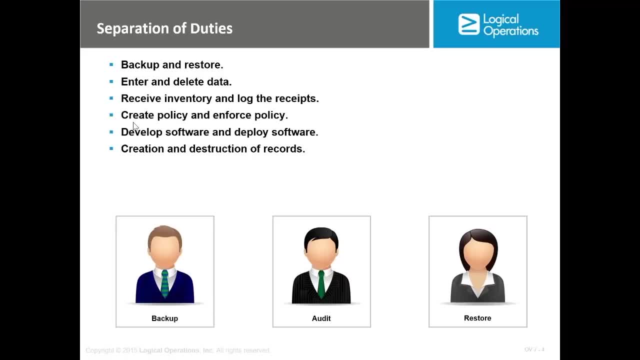 I remember the rules of question like that, but I don't remember the exact same syntax. But the point was two people are working in a coffee shop And one of them is working the full day, So he got a key to open and close the coffee shop, while the second guy is working only a part-time. 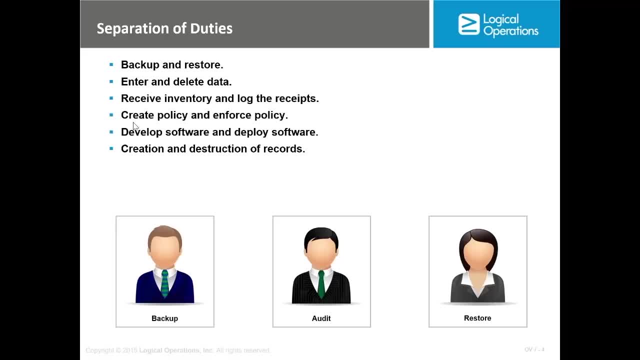 So he requested a key. He's not the one who opens a coffee shop morning time or evening time. He requested a key And the management or the owner of the coffee shop refused to give him this key, Because he's not why he needs a key. 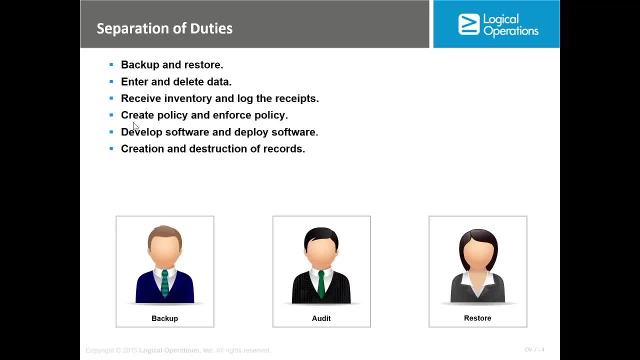 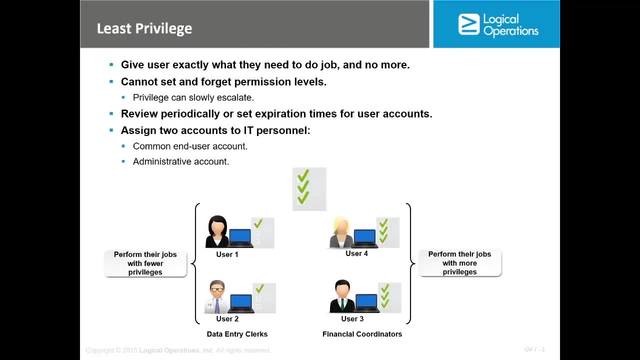 He's not opening the coffee shop or closing. under which policy do you consider that Okay? and I remember the answer was least privilege. I mean why he need access to the key He will not using. so what I'm trying to say is that sometimes 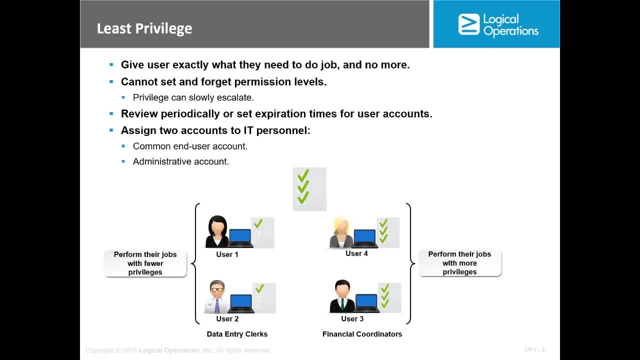 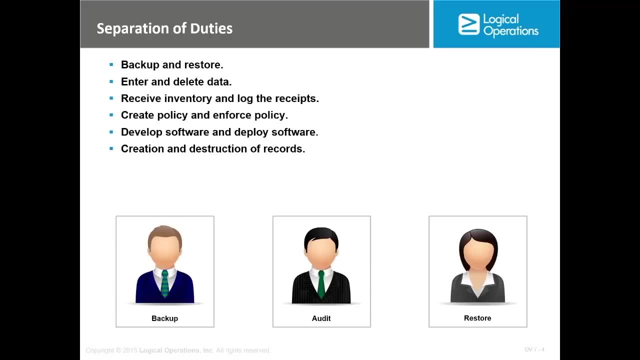 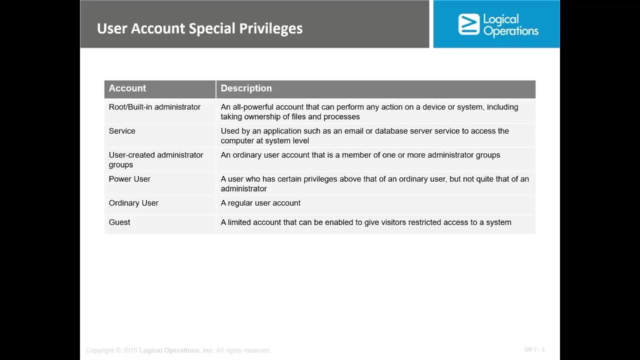 The question will be not straightforward, not that obvious. He will give you a scenario and then you need to consider which of those rules least: privilege or separation of duties, or Dual control, or need to know which policy apply on the situation. So you need to understand the concept behind it. 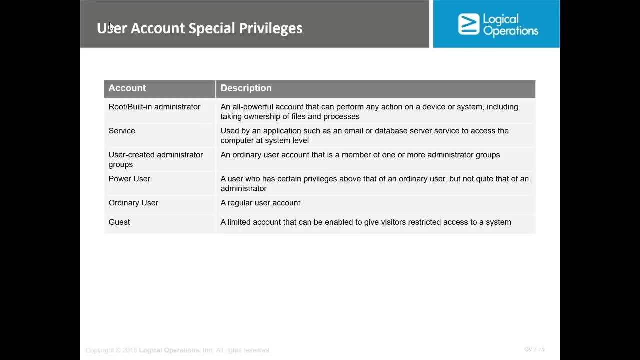 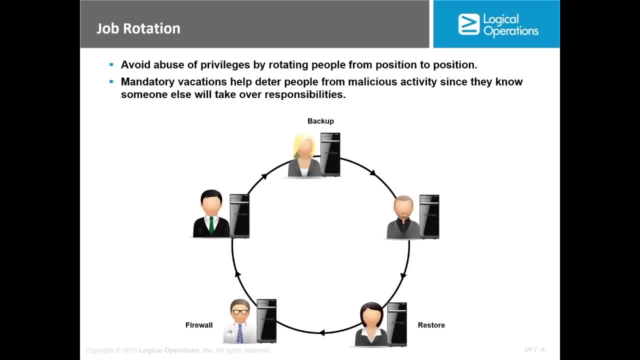 Why we are doing it. The user account special privilege: who need to have a special privilege on his account Job rotation? This is actually very Critical in ways that you need to do it in the right ways that will not be affecting the business. 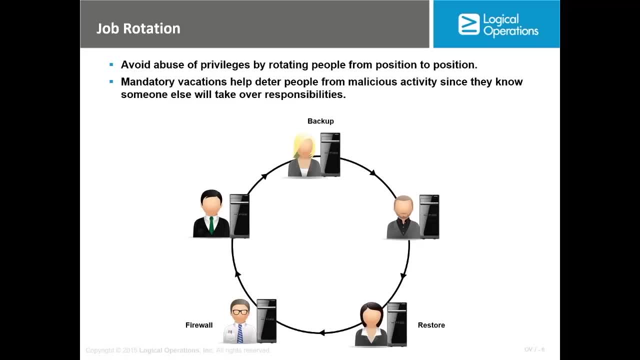 I should not keep specially the critical and sensitive position. I should not be keeping one guy to the same position for a long time Because if we do that, you know he may use it, misuse it. So from time to time people who are working in backup need to be moving to the restoration and people 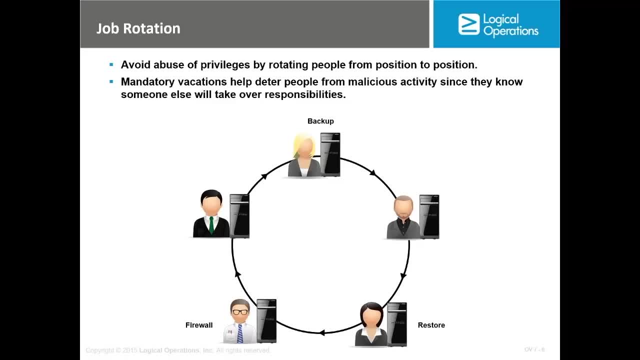 From restoration in firewall but actually realistically in real life. I saw that implemented in financial positions, especially in big organization, like as a finance manager. will be moving to like payroll- still He'll be doing something related to finance, but we do not keep one guy for a very long time in his position. 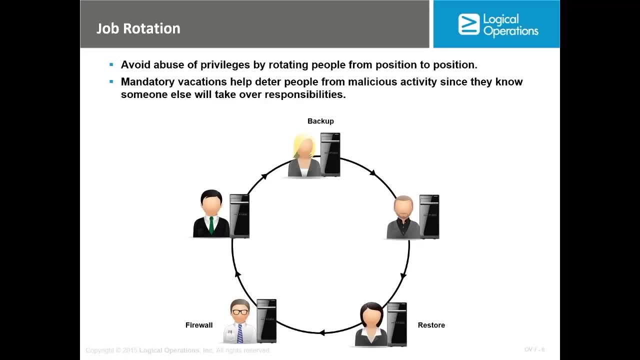 I know that we already spoke about that in the first domain, but still you need to review them and relate them to realistic scenario And also be aware of Other policy like mandatory vacation or need to know or dual mental control, And don't forget all those has been explained in depth into the sunflower document. 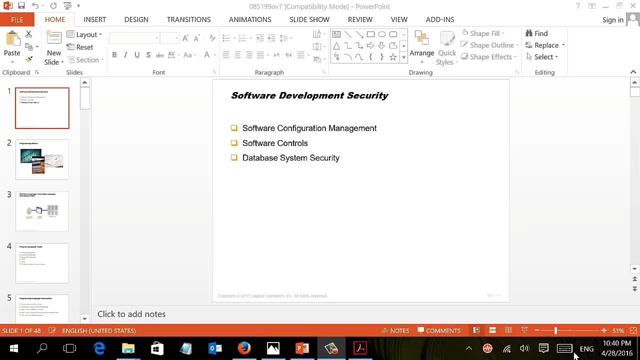 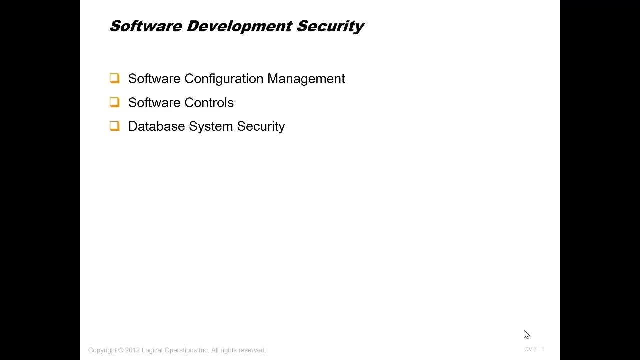 The last domain in this course will be the software development security, And this is actually one of the challenging domain because of the amount of terminology in this domain And, unless you are from a development background, you're going to need to do a little bit of effort there. 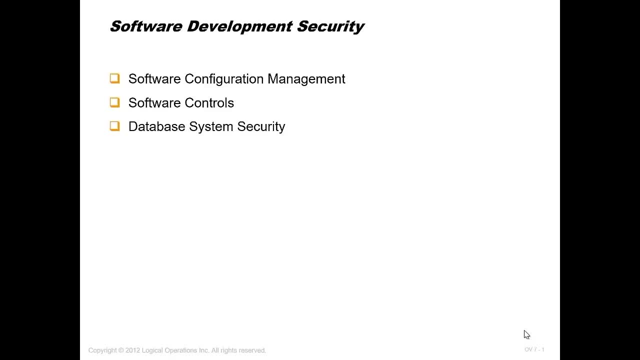 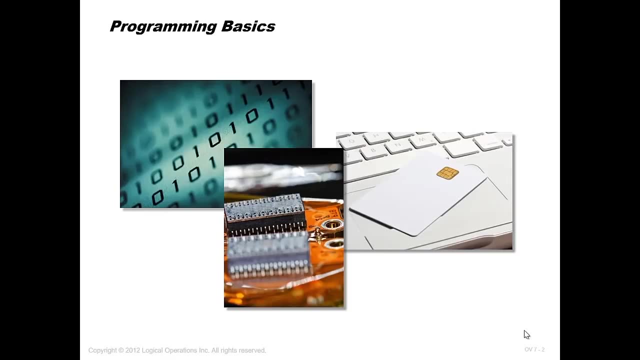 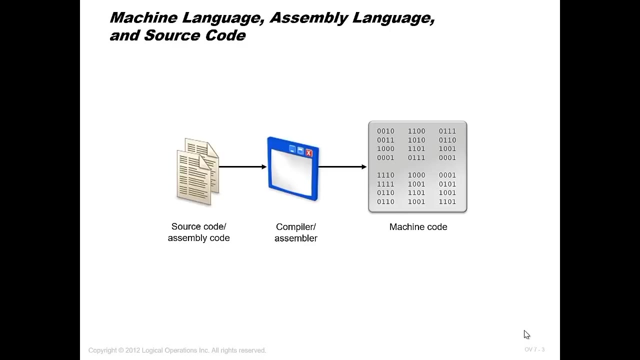 But I'll be pointing to the important part in such domain. Now, on the first part, there is an introduction part regarding the different programming language and the programming language, What exactly it consists, and we have the source code that will be compiled to machine code. 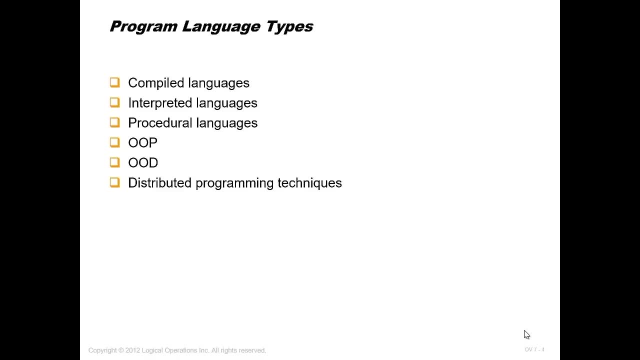 So just explaining how the process of programming is going. Language also has been categorized. to compile language like C language that you are writing them in English, Then it need to be compiled to the machine code So it become an executable. We have interrupted language. 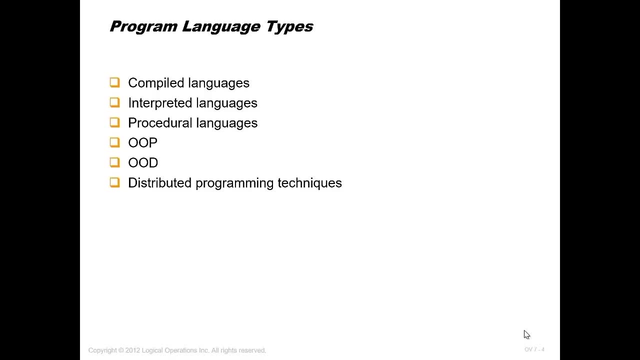 We have the procedure language object-oriented distributed programming technique. It will be good to read at least one line about each one of them- It's not the subject of the question, but just to be aware of- And we have different generation of language. 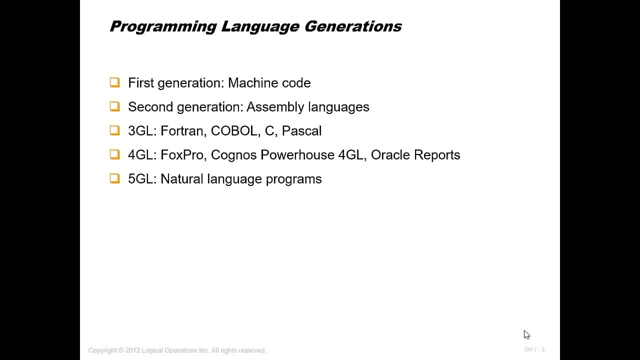 So we have the first generation, the machine code. Second generation will be with a little bit higher assembly. Then we have the third generation, Fortin and COBOL and Pascal. fourth generation, FoxPro and Oracle and so on, And now we have the artificial intelligence. 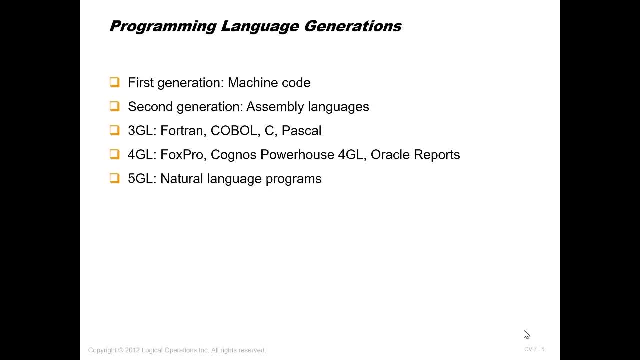 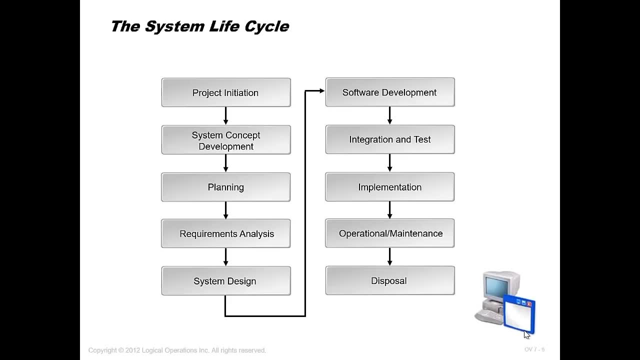 And the fifth generation. They are saying that we are on the 4.5 generation right now. Anyway, this is an introduction for different language and for different programming language. Things start from this part, which is the system lifecycle. Now, if you are doing a software development for an organization, what should be the process for that? by the way, 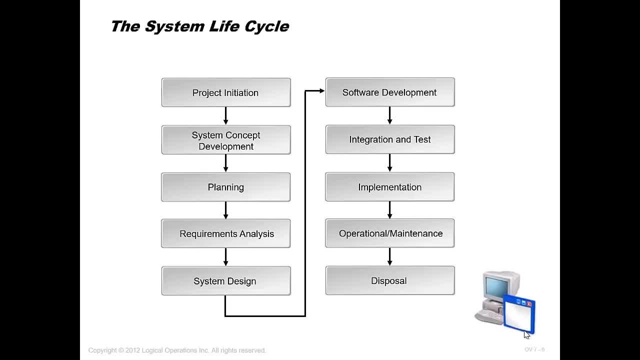 Right now, according to security Statistic, the major compromisation for any system can be done- Or usually it's done- through application layer or people layer. I mean no one is compromising through network right now. So a lot of compromisation. 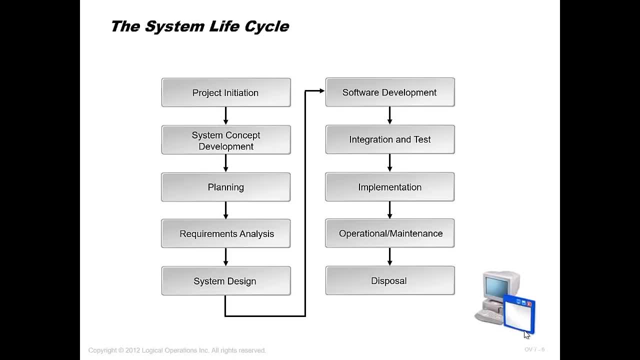 It's more effective if it's done through the application layer because of the weakness inside the application. So my point is: you may have a hundred percent secure network, but because you are running an application that is not secure, It will lead to compromise. 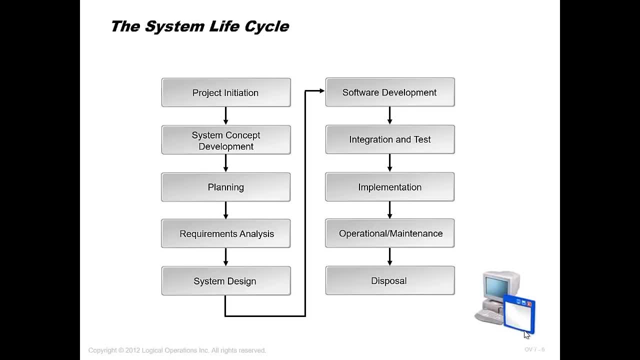 The system and the major compromisation that happened a few years back, done through the software. I mean, I don't know if you heard about PayPal- has been compromised. No information has been stolen, but it was denial of service: MasterCard, Visa card and everything like that. 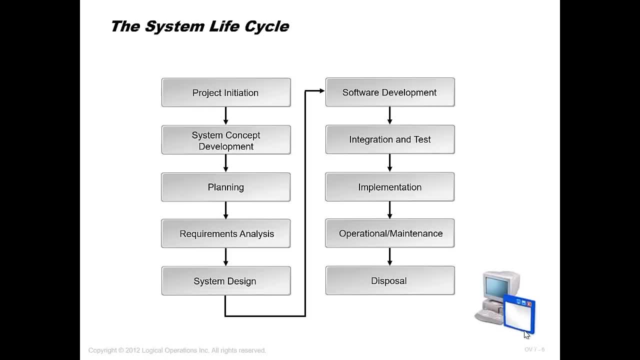 And some of those actually had some problem with SQL injection or which you're going to explain this part. So my point is: usually there is Weakness inside the application because it's has been made by people and people do mistakes. So what is the system life cycle? 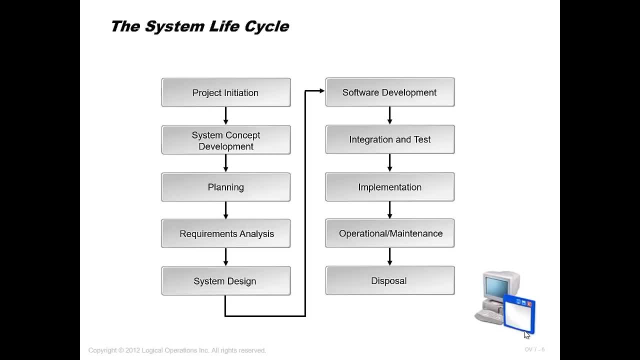 What is the proper system life cycle? It should start with progress, project initiation, Then system concept development, then So after all, it should be starting with a project, because it has a start date and end date, and then planning the project. Then you start collecting requirement, requirement analysis. 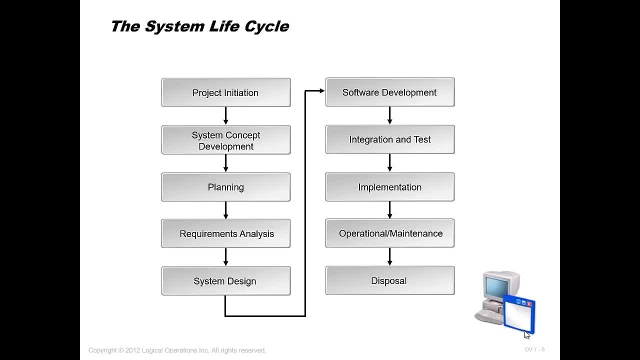 Then you do the system design, and then software development, integration and testing, and then implementation, operation and maintenance and finally disposal. So this is the life cycle of any system And this is how it go, I mean, even realistically. it's usually a project and it start by collecting requirement. 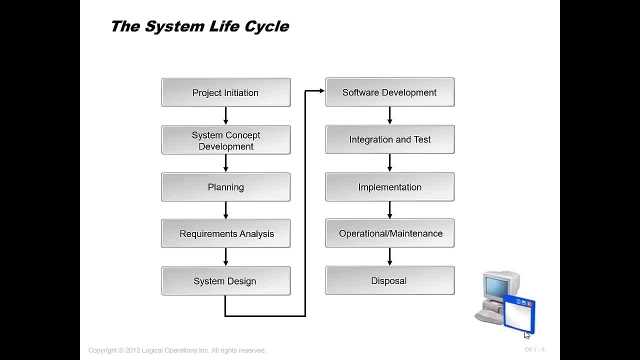 It need to be planning because resources need to be assigned, Budget need to be assigned. Then you start collecting requirement from the customer, What exactly he require request in such application, and then you do the design and software development and then testing and then implementation and operational and finally disposal. 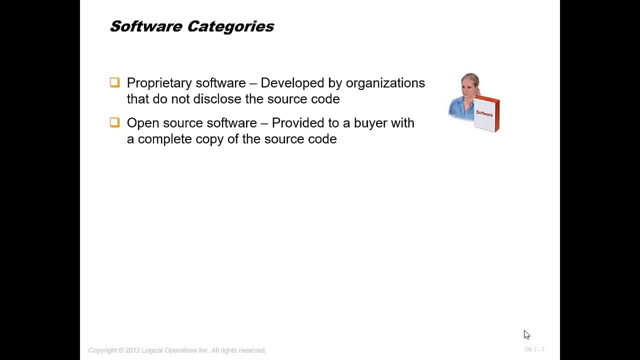 In software category. We have two different kind of software. We have the proprietary software. I mean the software that you are not allowed to see the source code, like Microsoft Windows, for instance, When we bought Microsoft Windows or Microsoft Office or any Microsoft product, they will not give us the source code. 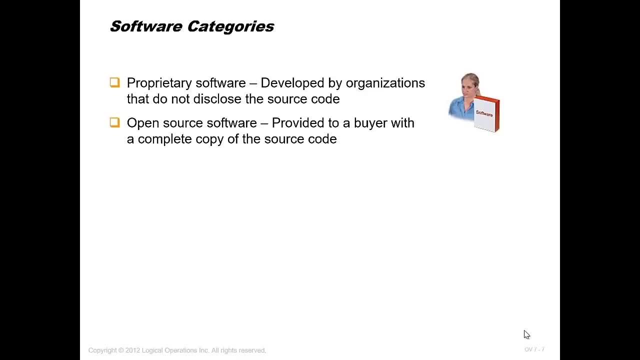 They will give us only the executable and a license to use it, While Linux is considered an open source, So you can see the source code. A lot of people think about open source that is like free- No, it could be paid, But after all you can have the open source, and right now there is actually a lot of. 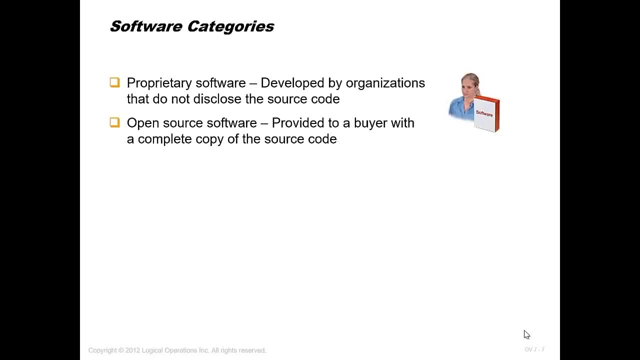 Discussion about that, but I believe that people eventually will go with open source, because open source has been Reviewed by many people, because when you like Linux, for instance, it has an open source, So many people can review it. A lot of flow will be discovered and it will be more secure. 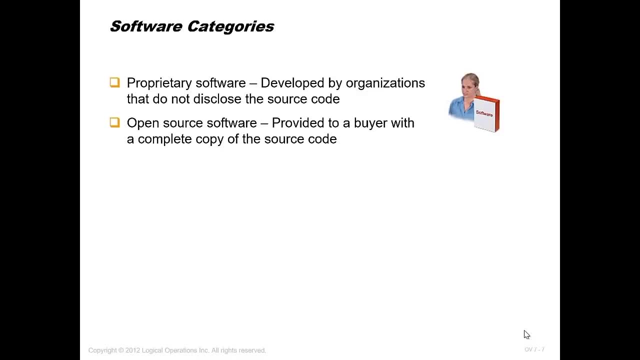 Well, if you are getting Microsoft Windows, you don't know how it has been written. So from time to time Microsoft release a patch or a service back to The problem, but you never know what was the problem or you know if still they have a problem or not. 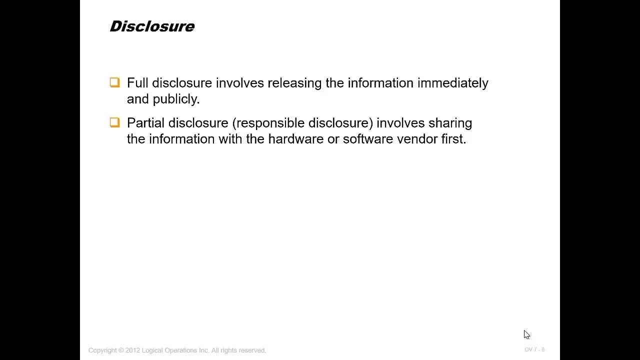 Also, when you are buying the software, we have a full disclosure and we have a partial discussion. Are we going to release the whole information or a partial information? Now, this is all just introduction. I mean it's not really an important subject. 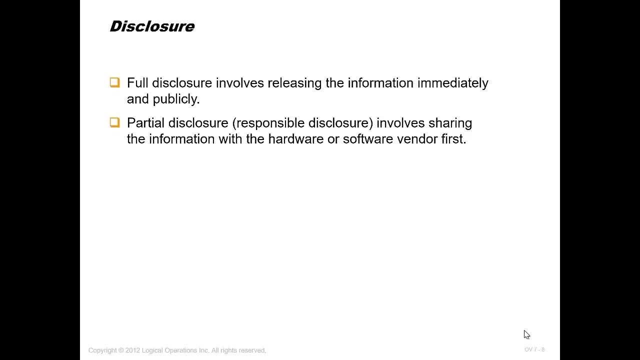 Common sense and just an introduction. Starting from next lecture We're going to start Talking about the important part inside the software development, Like. what is an escrow agreement? It's very important from a security perspective. What is the security models, system development models that is used? 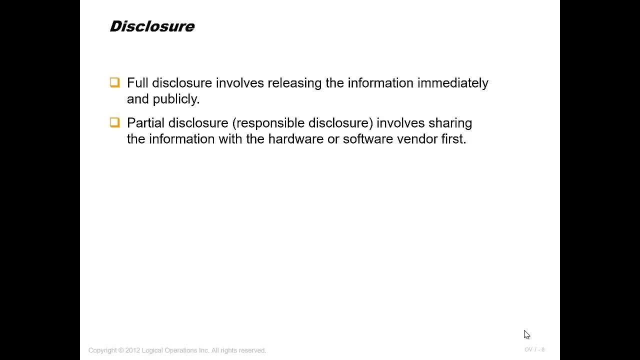 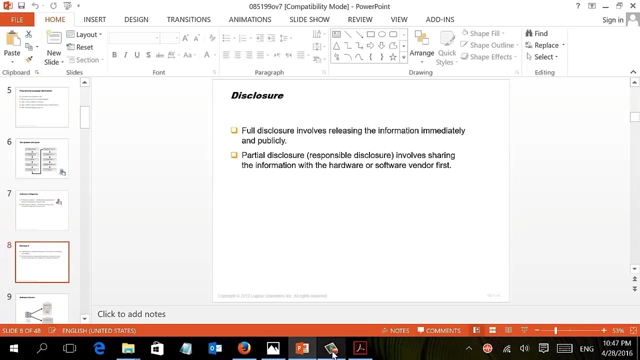 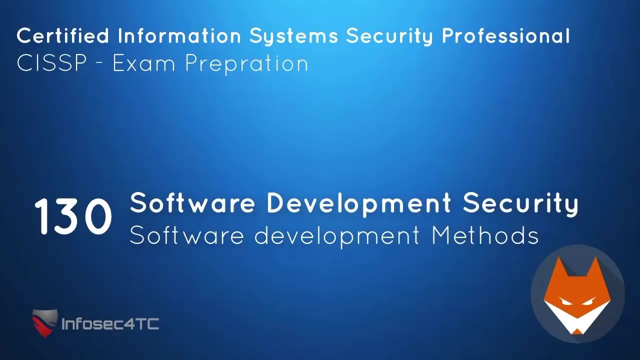 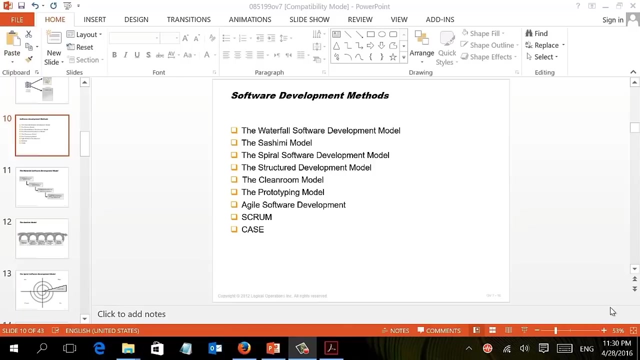 What is the most common attacks for security? I mean, starting from the next module, things will be a little bit in-depth. So this was just an introduction and let's see the important part in the software development Domain. In this lecture we're going to explain the different software development methods. 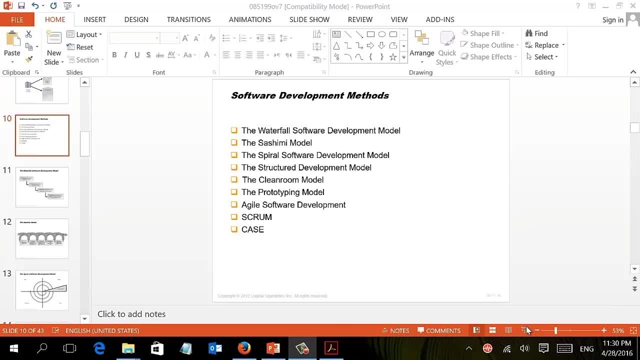 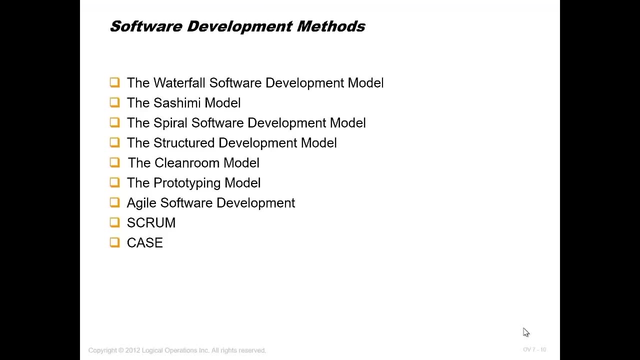 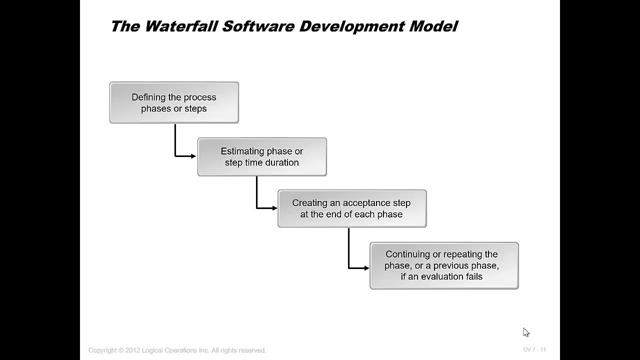 When you do a software development, there is different methods, and each of those methods has its advantage and disadvantage. So the force first Is the waterfall software development model. This is the process, how the software will be developed. So, as you can see, it's a sequential process. 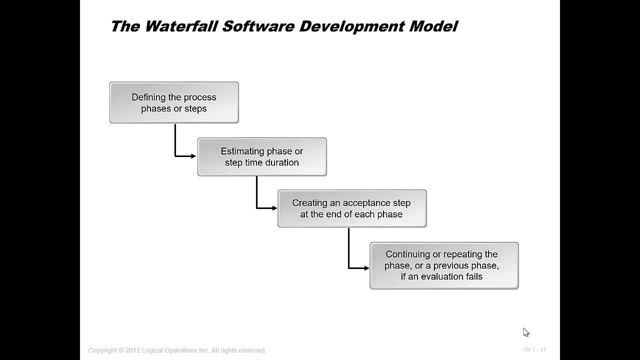 So it starts with defining the process phase, then estimating phase or steps and durations, and creating an accepting setup. Then it's not about knowing the name of the step, It's the model itself. So model itself, that whenever you finish one phase, It will be closed and then you can start the second phase. 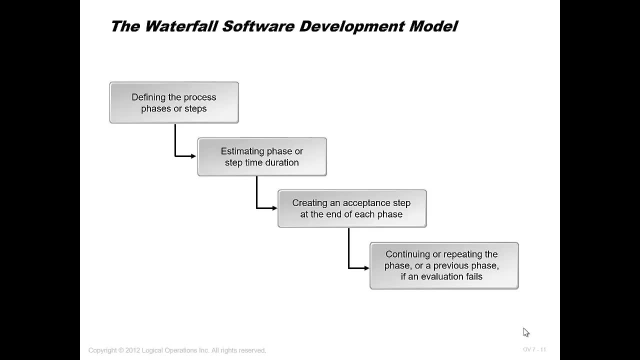 That's why they call it the waterfall models, because it cannot be going from down to up. It should be going from up to down. So whenever you finish one phase- for instance, you finish collecting requirements, That's it, You start the design. 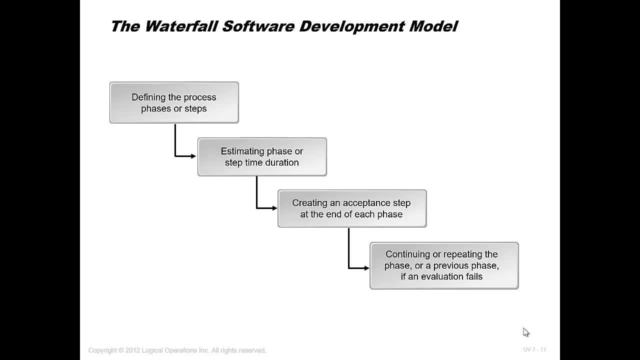 You cannot get back to the collecting requirement one more time and from a security perspective, And this is actually a good model because you, whenever you finish A phase, you close all the risk associated to this phase, So you start a new phase. So this one depends that when you finish a phase, you don't get back to the previous one. 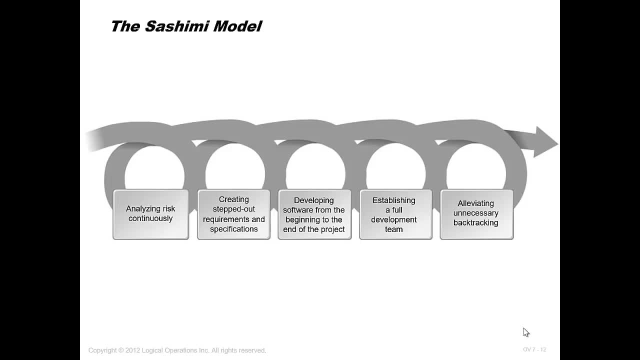 This is called the waterfall model or software development model. An opposite model is called sashami model, which is you are doing everything parallel. You are collecting requirements, You are doing the design, You are doing the implementations and you may get back to the collecting requirement or the design. 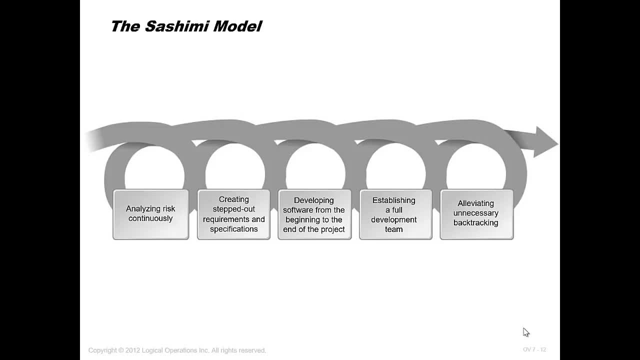 So the all phases of development is done parallel together. This is called the sashami model and maybe security. here It's a little bit a concern. but effectiveness is very, very important because sometimes when you work on a project, especially in develop software development project- customer had some new requirement. 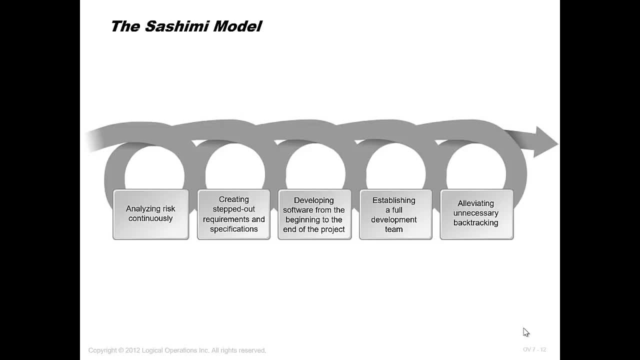 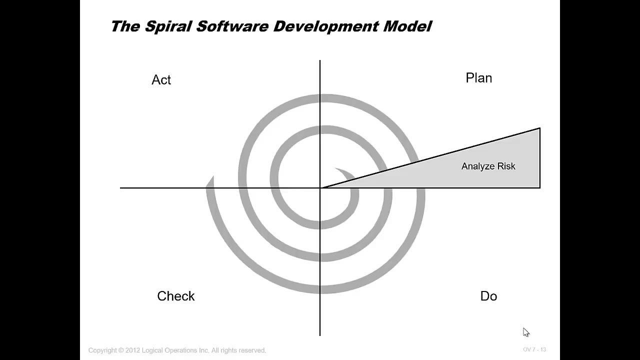 If you are following the waterfall model, you will not be able to get his new requirement again Or get back to the design phase while you are. when you are doing sashami model, you can do that. Third model is called the spray software development model or has another name: plan to act, plan to check, act or PDCA. 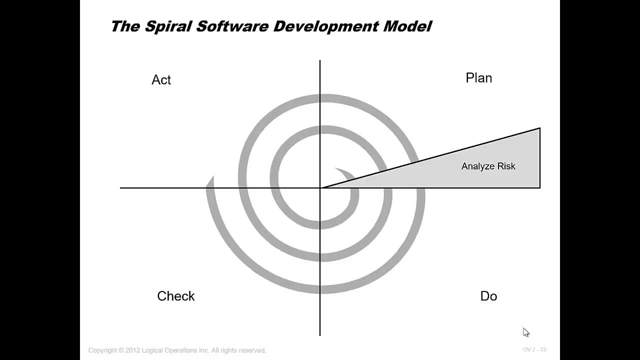 This is actually more as a quality model that it's a continuous process. It's not closing, So you plan, you develop, you check for any weakness. if there is any problem, you act and then you plan Again. so it's a continuous process. 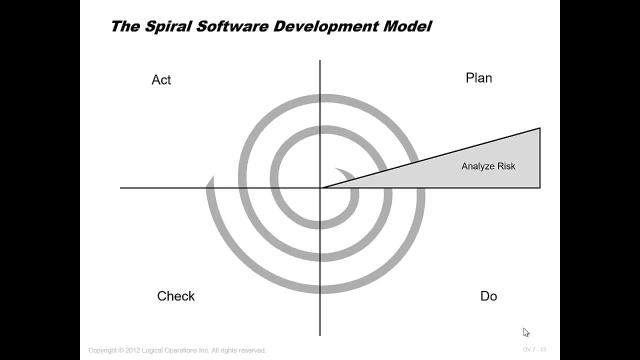 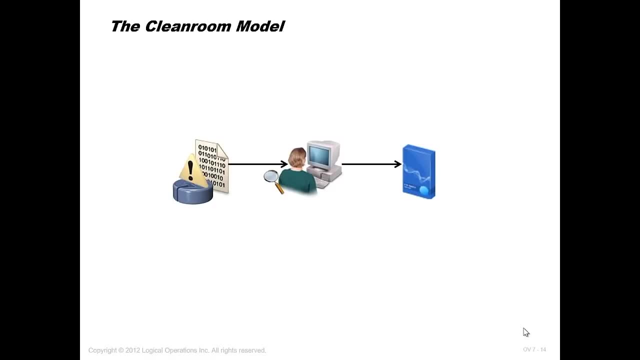 And the finder of this model is called the meaning, but it's more as a quality model. Another model is a clear room models, and the concept of the clean room model is that if you do a process or you spend time at the beginning in your software development, 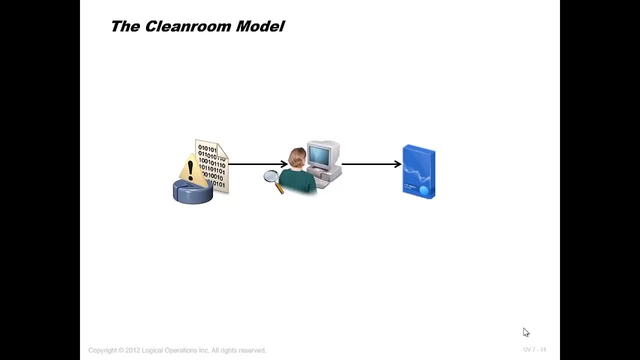 it will prevent From keep doing change after that. So if you did the software in a very rush way, then the customer will keep asking for changing requirement and for modification and so on. But if you spend more time at the beginning maybe the project will take longer time. 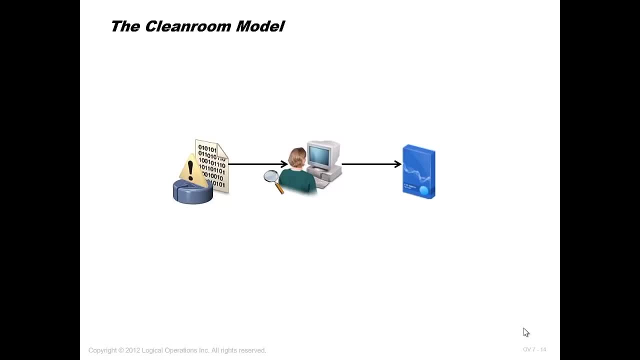 but eventually you will reduce the amount of change needed or amount of modification inside the application. prototyping model is just to give a sample because especially in software development, Sometimes the developers team spend long, long time preparing for software and then when they show the customer after going through the process of planning and 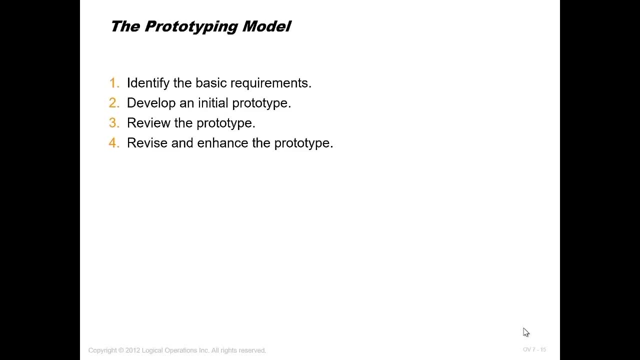 requirement, collecting requirement and designing and implementing. then when you start showing the customer, he said this was not what I was expecting, So it's very, actually Risky process. So prototyping Is to, once you Agree with the customer about software and collect the requirement. 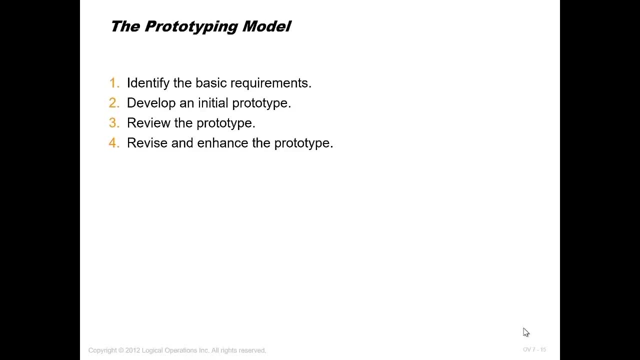 You do him a prototype, a sample of the application showing this is how it look like. So you are limit, you are doing some limitation for his expectation, So he will know eventually what he'll be getting. This is called the prototype model, Agile software development. 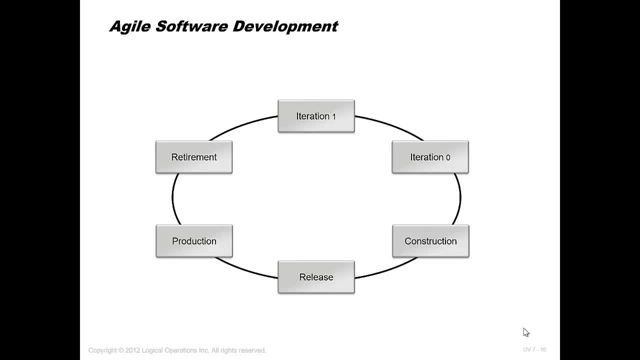 It's more into the another project management Model, so it's not really software development model, It's a project management model. The idea of Agile is that when you do a software development, it usually take long time until you get deliverable for the customer, because there is a lot of process that you are doing before getting something life. 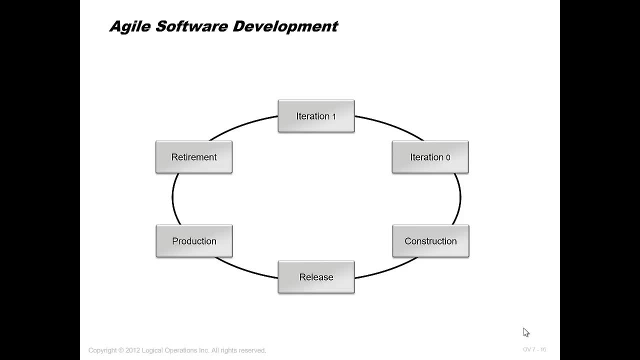 You are collecting requirement, You are doing system analysis, You are doing designing. so it will take time Until the customer can see something. Well, if you follow Agile software development, the good thing about Agile is that customer will be involved During the whole project. 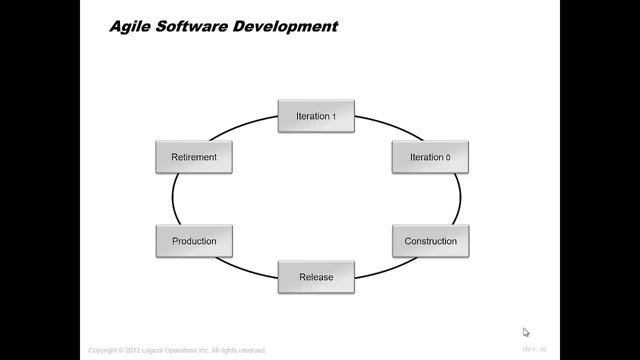 He'll be getting deliverable during the whole project. So it's designed in a way that you can divide the work on different phases and customer will always get the better deliverable, So you don't have to wait for a long time until he gets a project deliverable. 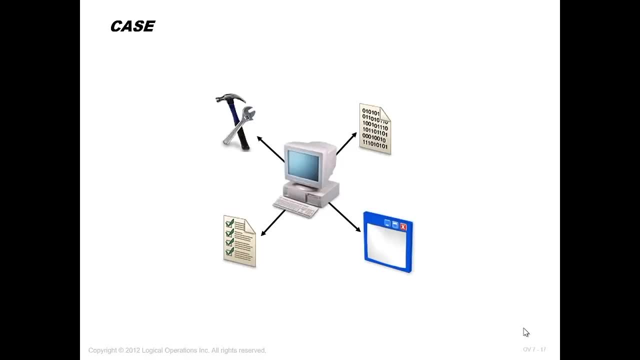 Case or Case It's something. assistant for software engineering. Yeah, computer aid, software engineering- This is actually software. It's software that allow you to design a program and allow to design the flow of the program. Where is the input, Where is the output? 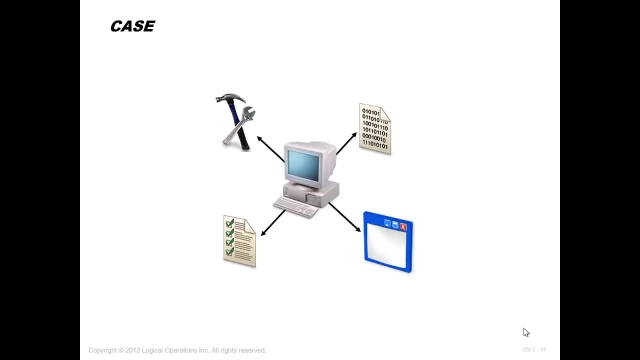 And it's very, very complicated software. I mean you need like four or five months to be able to analyze the software and definitely need to become from a development background. So case is a software, Computer aid, software engineering, that allow you to design your software and designs the input and the flow of the information and so on. 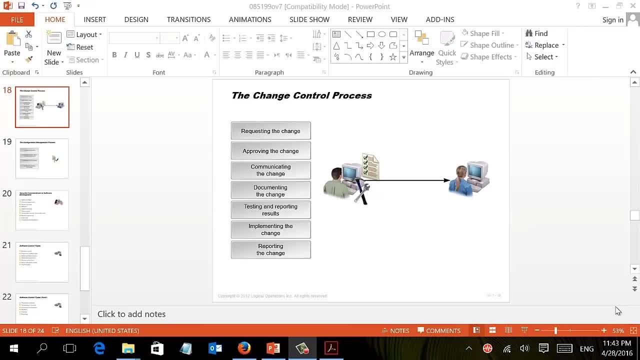 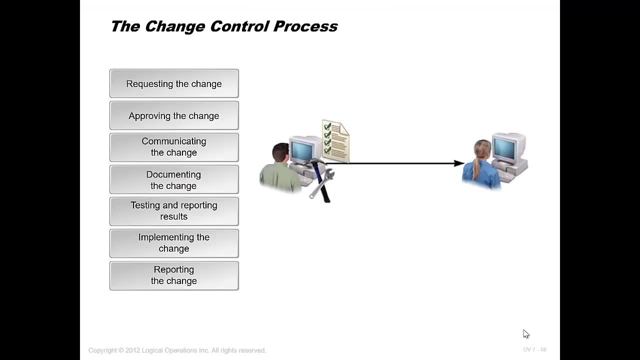 Now, once we get a software developed In our company And it's up and running and it's saving our data and information, Now change will be requested from time to time, So, for instance, one of the user or one of the manager may request a report. 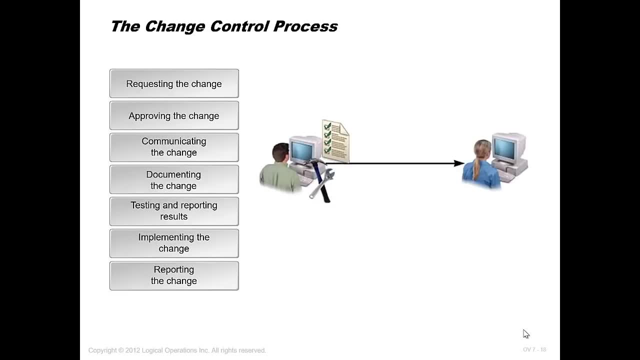 One of the user may request some modification, adding some screen, So a change will be requested. Now it's very important to consider the process of change request in your organization, How change will be processed. a process, I mean if someone need a change, they need to change something inside the program, at the field or at the report. 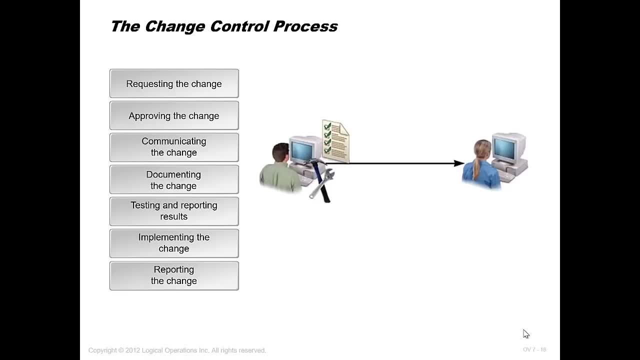 He just need to call the developer and ask him to do a change. It should not be done this way, because maybe this change will affect any other things from security or from efficiency. So you need to have a proper change request process. Most of the organization has the change request. 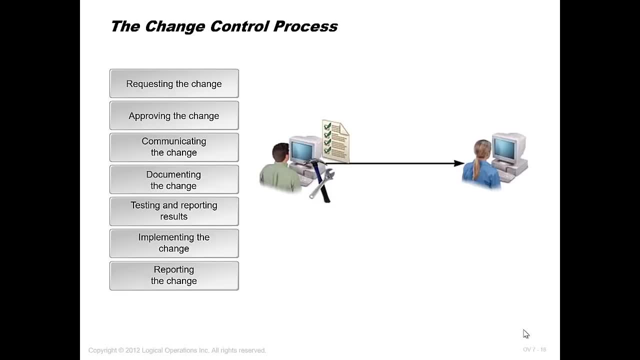 Let's start with requesting the change. So the employee who needs a change will write a request, maybe on a paper on or soft copy, and send this request. This request will be checking and it will be assist. I mean they will be the effect of change, of doing such change. 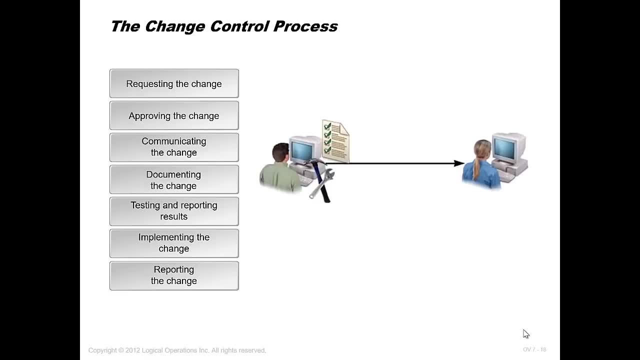 So according to that, it may be approved or it may be rejected. And then so it will be approved the change, then communicate the change document. the change, So it will be, can be traced: who did this change and why. because when you are doing a change request you have to specify why and then test and reporting and implementing the change and report the change. 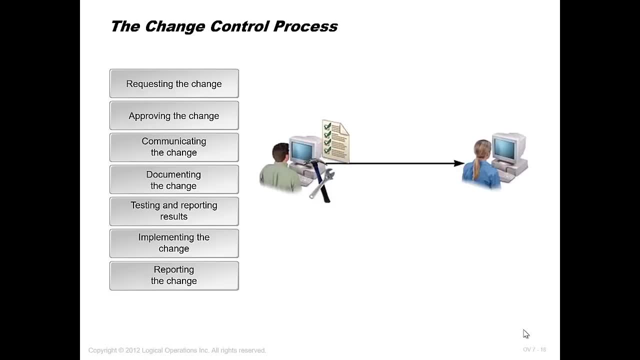 So the point is, it's not about the steps in such a slide, It's that you should have a change request process And this change should be documented. and it should be for a reason, because unless you are not doing, unless you do that, people would keep change for any reason. 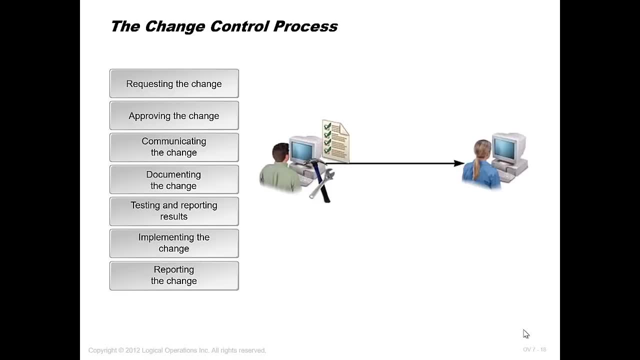 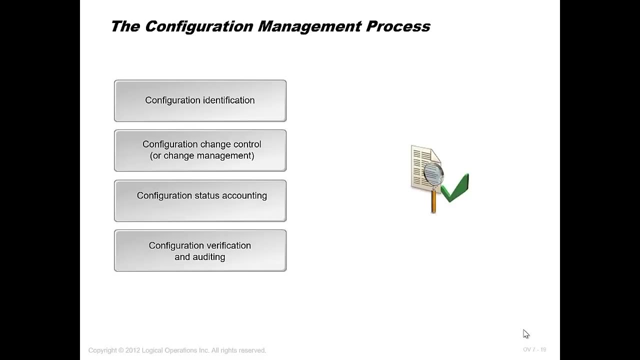 They said: okay, I don't like the screen color. You cannot change inside your systems that will affect your security. because of the same concept apply for configuration, So also should have a configuration management process. if I need to open a firewall port, if I need to change something inside the configuration, give a permission or something like that. 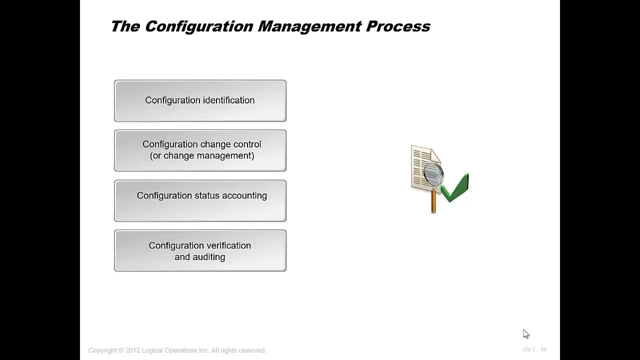 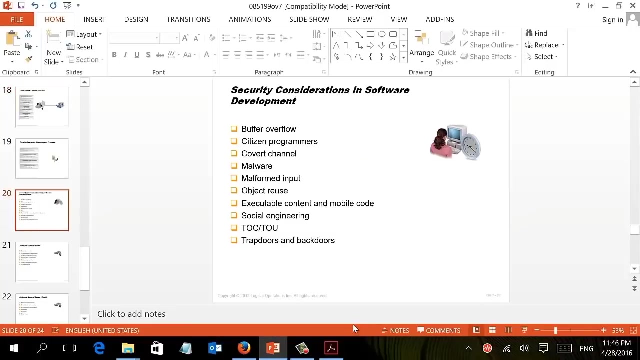 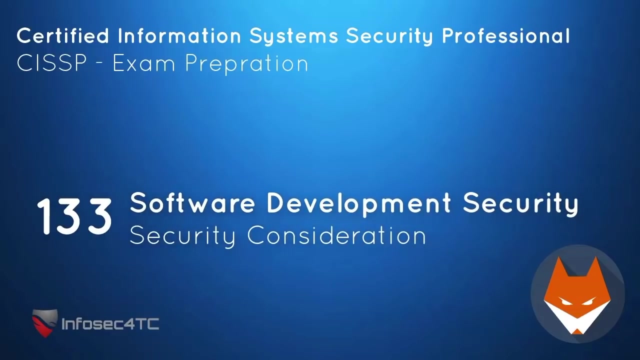 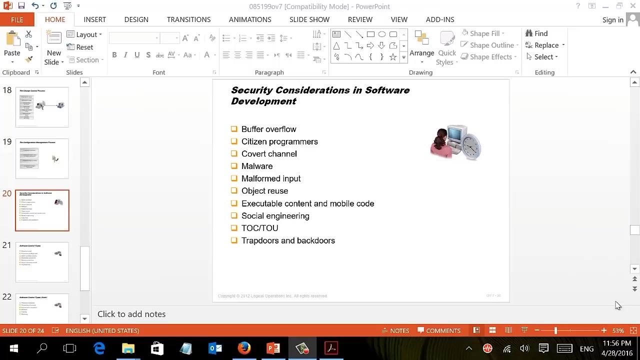 So also it should be assigned And it should be tested, and it should be approved or rejected and then it should be, it should be applied. so change management and configuration management: This is a very important process inside the software development lifecycle. This lecture will explain some of the security consideration or let's say, some of the software attacks. 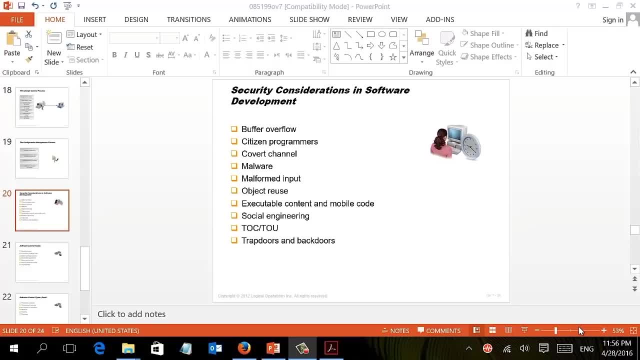 We agree during this course, that attack is very important for the exam and the good thing that you're going to find that most of those attack we covered in different modules, So we spoke about buffer overflow, about cover Channel, malware, mail form input. This is a very, very important attack when it comes to software. 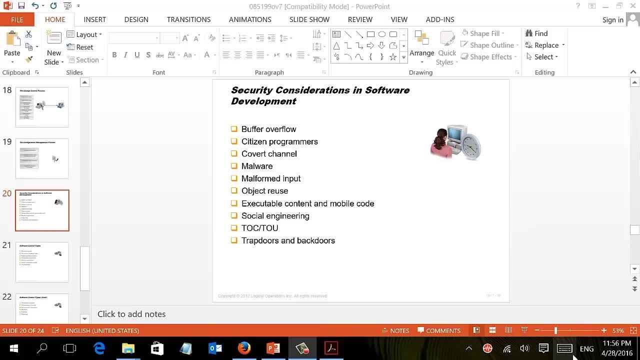 And we are talking about manipulating the input, like SQL injection and cross-site scripting. specially SQL injection was one of the attacks that is very, very till now, with it's, considered one of the highest attacks. That's why, after this lecture, I added two small demonstration about SQL injection from my ethical hacking course, just not to keep talking theoretically, but also to show you how the poor validation of the input cat lead can lead to a full 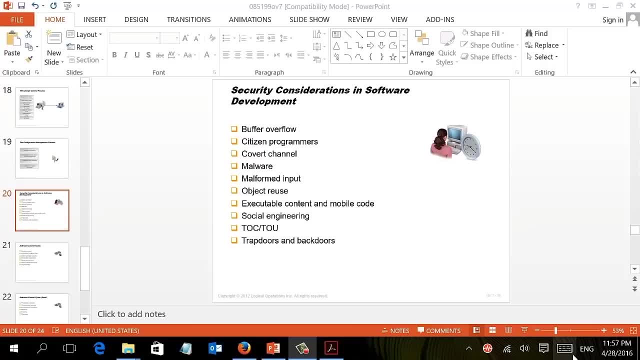 Compromisation of the system. So just to get out of those theoretical and definition So on, I added two different lecture, very interesting lecture about SQL injection. I want you to watch those lecture and to watch those attacks and to let me know what is your opinion, how that can be prevented. 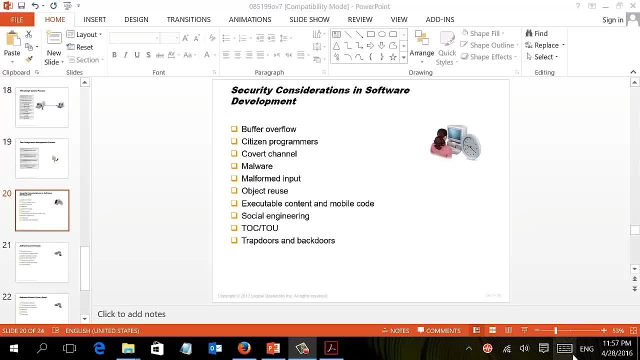 In your software development lifecycle. we spoke about object reuse, We spoke about social Engineering, TOC, TOU- We spoke about that when we saw the tempering the data and trapdoor and backdoor. So most of the attack has been covered on a previous section, but I wanted to add couple of videos just to show you one of the attack in a realistic way. 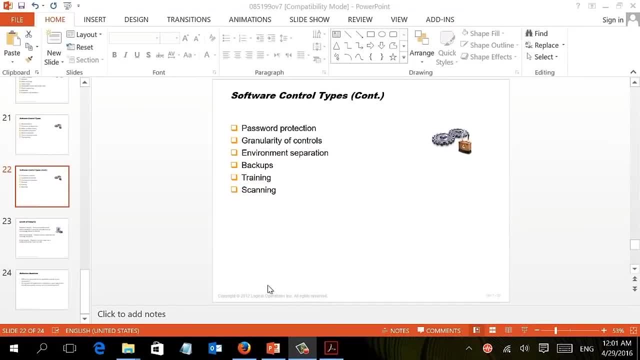 Finally, in this module Or in this domain, we're going to talk about the software control type. what control I can add to my software So it become more secure, so we can harden the security kernel, We can work with the privilege state. 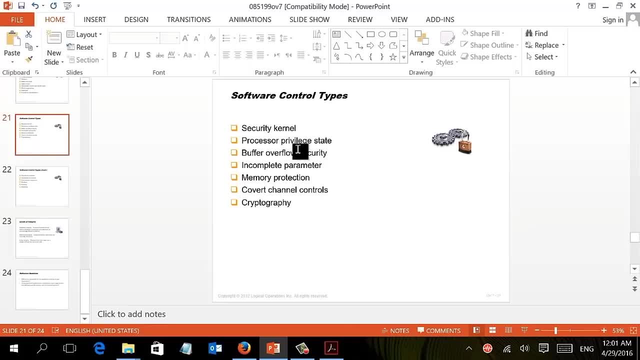 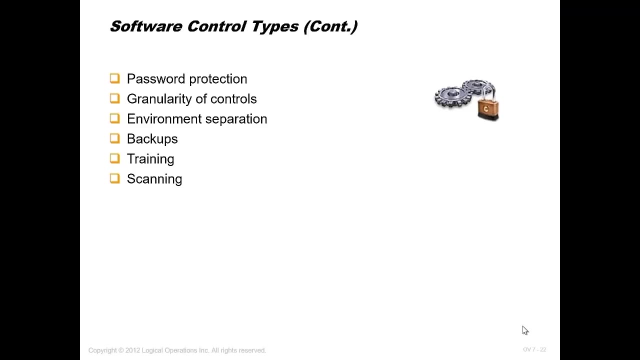 We can try to prevent buffer overflow by validating the input. We can try to manage or protect the memory cover channel cryptography. This is all will allow to secure our Software. we can also try to protect password by having a policy for a strong password environment separation by considering the place where the 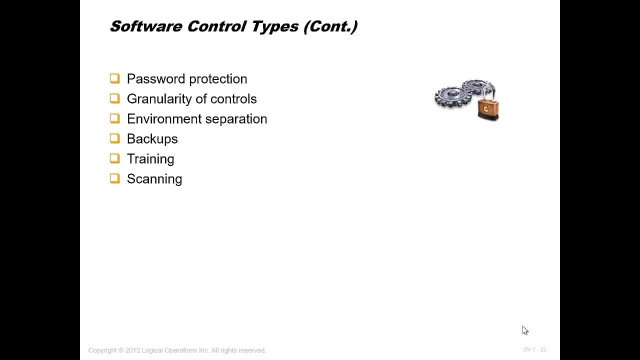 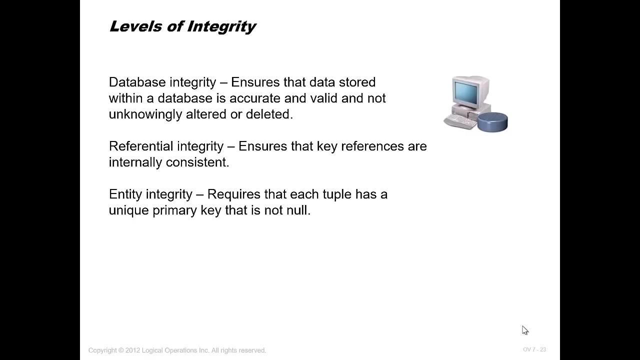 Information are saved, They are secure, They are far from theft or any environmental damage, taking back up, doing training and scanning the system eventually. So those are some of the controls that we can implement To harden our software. Also, one of the things that you need to consider is the level of integrity is a very important concept inside the software, because the thing is, if you have a software, 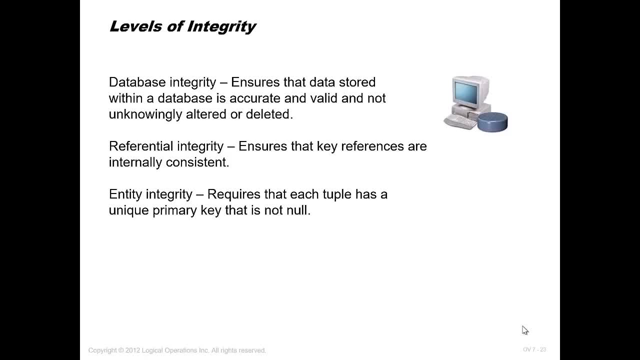 That we will save your data. Now, besides the protection part that you are protecting against hackers or against any malicious activity, What if someone- one of your employee, with not actually, I mean he's putting the input in an Integrity way? So he, for instance, he had some financial information but unintentionally he wrote some wrong number. 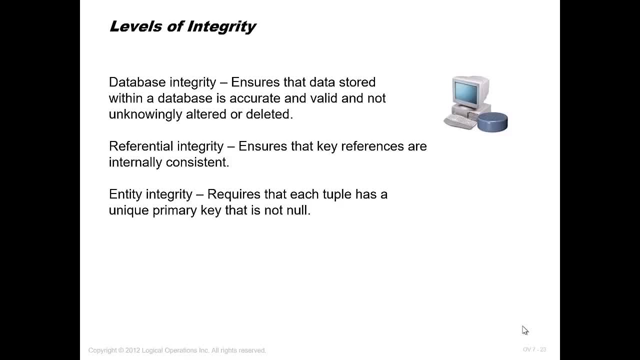 So after all, the information will lost the integrity. It's not an attack, It just a bad behavior, or someone is not giving attention while he's putting the information. So you should provide some kind of integrity, like two people validate the information or, for instance, you know those. sometimes when you are putting your information and you are 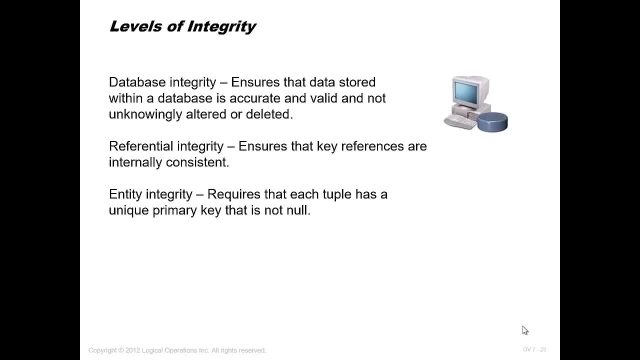 Putting your ID or social security, They will only accept number. or we are putting your cell number or mobile number, They will only accept number. You cannot add Letters. This is to provide the level of integrity. So, as a security professional, you should beside harden your software. 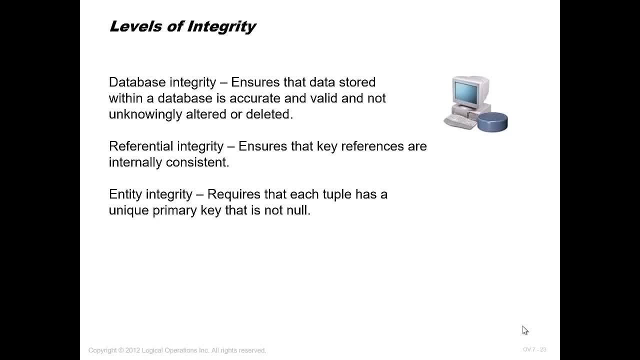 You should also provide some level of integrity for your information, to make sure that whatever information has been input are valid and they are not actually Losing any kind of integrity. So it's a very important concept as well.